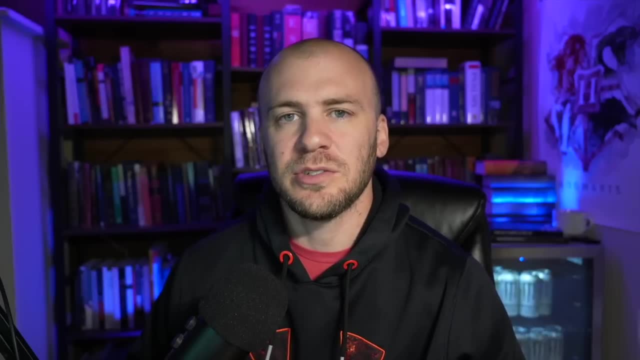 Hey, thanks for stopping by my channel. The purpose of this course is to take you from a complete beginner who doesn't even have a Kali Linux machine set up on your computer, to someone who's able to successfully go out and find bugs on bug mining programs. 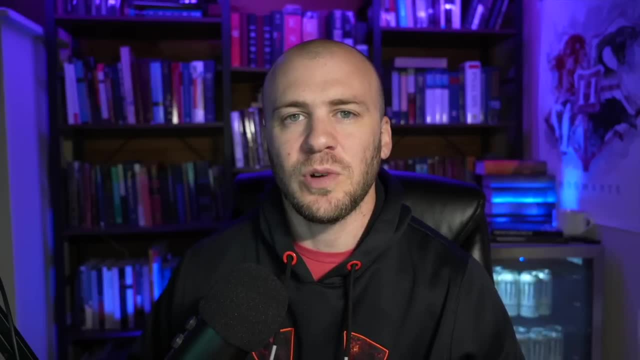 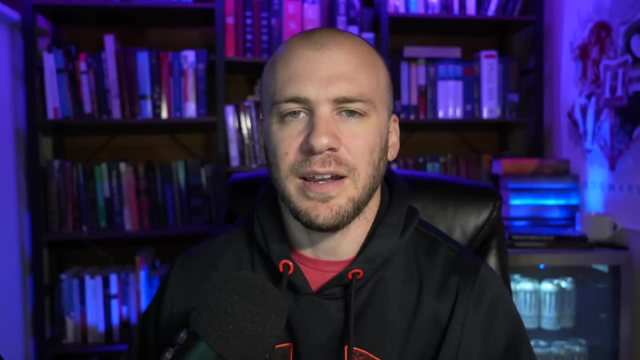 be able to read the activity and other people's exploits and understand what is going on. So I see a lot of videos on YouTube and Twitter threads saying this is everything you need to study in order to become an ethical hacker, And I decided, instead of just making a roadmap or some kind of 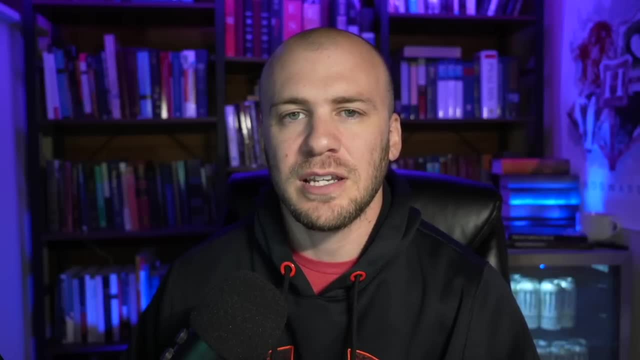 Twitter thread. I'll just give you a video that is going to take you through the process of what I think everything you need to know in order to become a bug bounty hunter. you'll have a great foundation for recon. you'll be able to find the most common vulnerabilities. you'll be able to 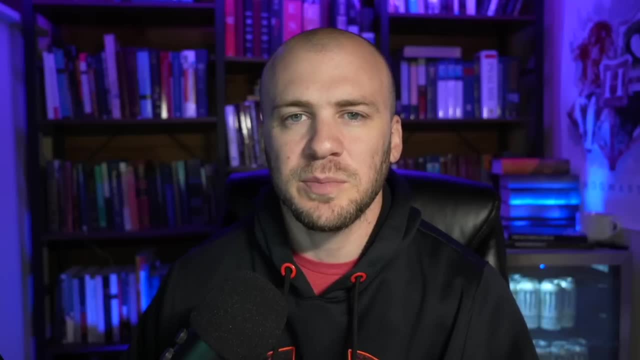 understand some of the more complex vulnerabilities and how to exploit them. And what I do in this course is not just tell you what you need to study. I actually walk you through the process of studying, learning and understanding these exploits. So if there's anything specific you 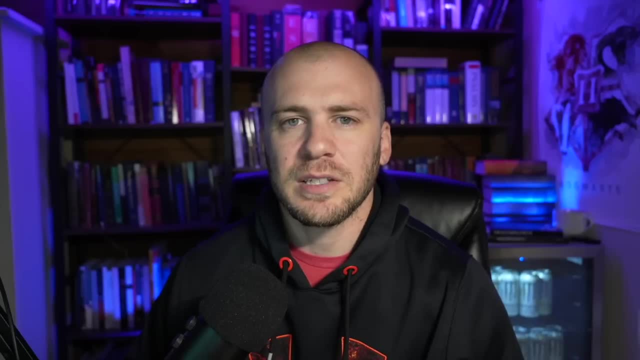 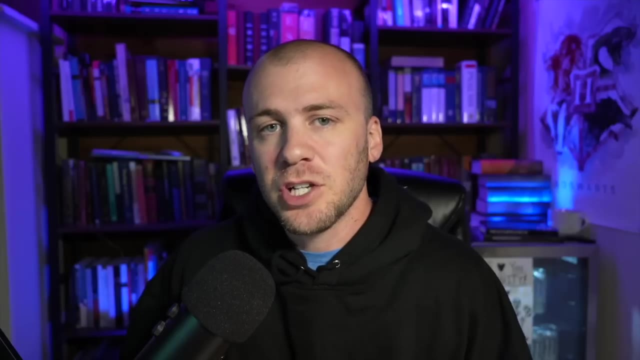 want to learn in the world of bug bounty hunting. you can look for the timestamp for that specific vulnerability And you can go ahead and skip to that section of the course, because you can always come back later. All right before we get started and jump into this course. 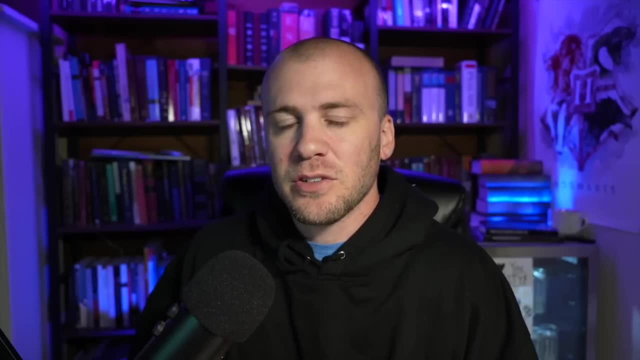 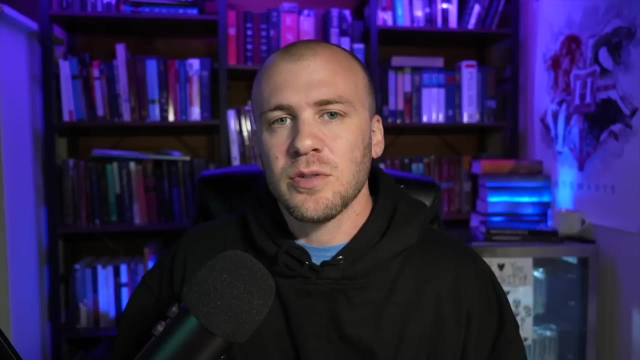 there is one thing that I want to mention. These courses and videos do take a long time for me to put out, And my YouTube channel is small enough that no one wants to sponsor me. So if you'd like to buy some hacker merch that looks kind of like this or this or maybe a little bit of this, 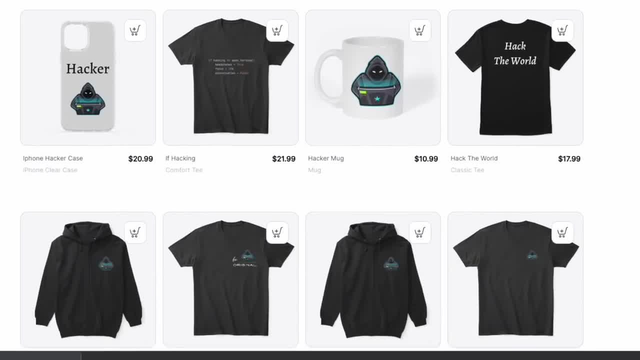 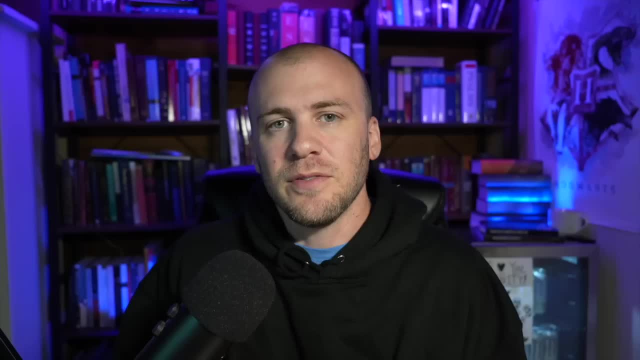 then you can go ahead and click the link in the description, Or if you would like to buy one of these courses, or if you would like to buy this course or another course or just a section of this course and be able to save your location and come back to it. you can check out. 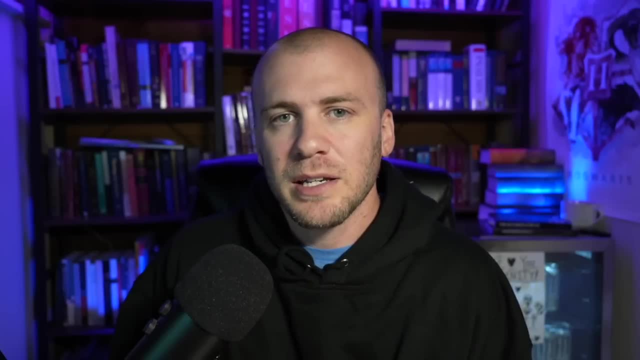 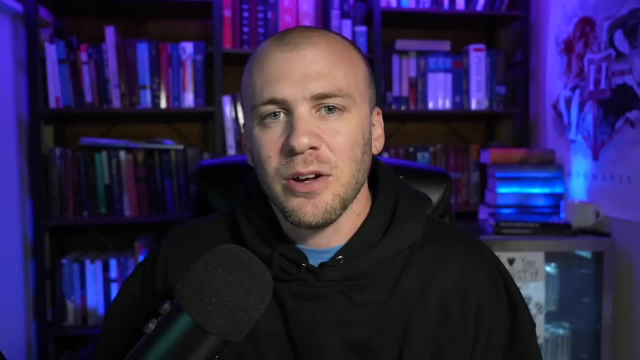 the link in the description that is going to lead you to my website, And if none of that works out, that is totally fine. You can go ahead and enjoy this free course here on YouTube, And I hope that it's helpful and beneficial for you in your journey to become a cybersecurity professional. 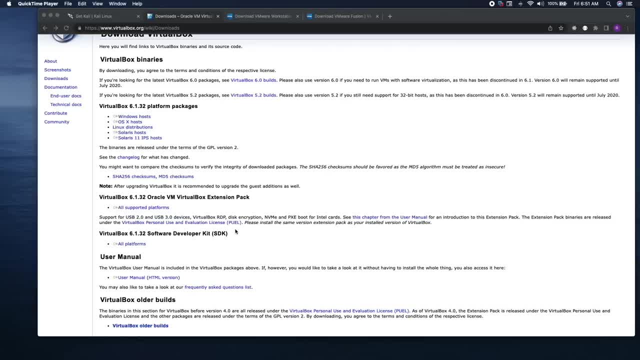 Now let's go ahead and jump into it. All right, it did not take long for us to come back to this course. So if you'd like to buy one of these courses, or if you would like to buy one of these courses, or if you would like to buy one of these courses, or if you would like to, 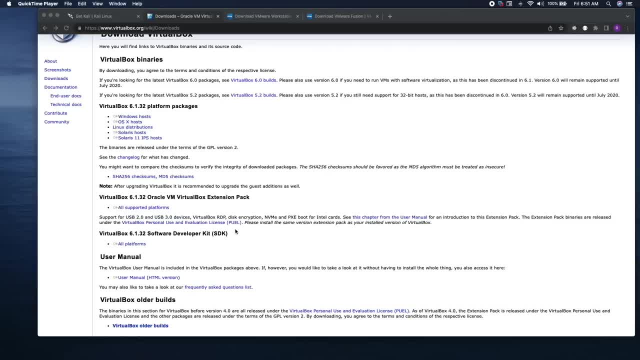 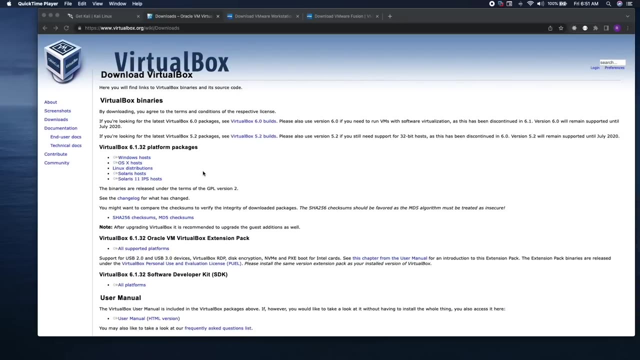 come to a crossroads where you get to decide what kind of virtual hosting software you would like to use. there is a free software called VirtualBox. You can download it here. you can download it for a Mac, you can download it for Windows And I strongly recommend you avoid VirtualBox. I tried. 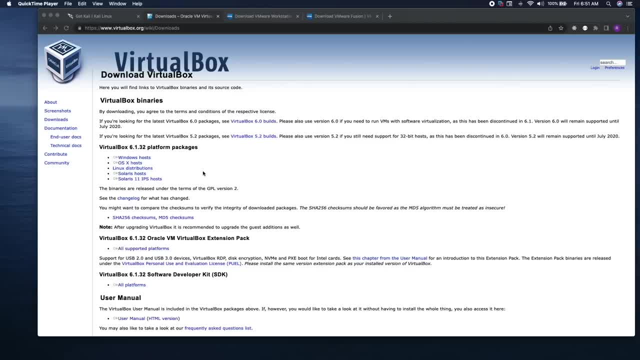 using VirtualBox when I first started, and this was quite a while ago, So maybe it is better now. But when I ran VirtualBox I struggled for months because I did not want to pay any money to have a good virtual machine hosting software But after it kept on lagging and freezing. 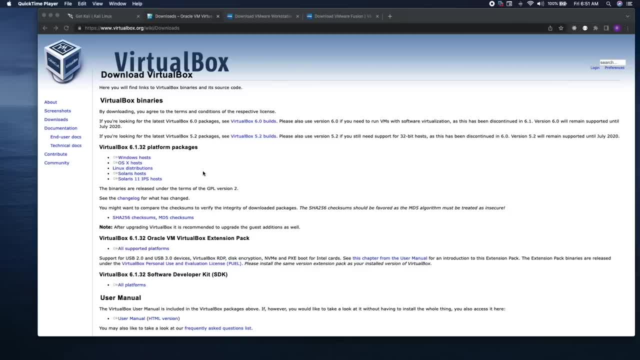 and I couldn't get Hack the Box to work, I decided I was done with VirtualBox and I was ready to pay money. If you want to avoid paying money and you want to try VirtualBox- and maybe you'll have better luck than I did, you can go ahead and download it here. 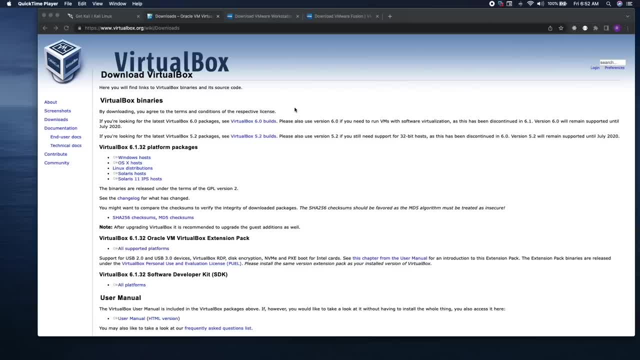 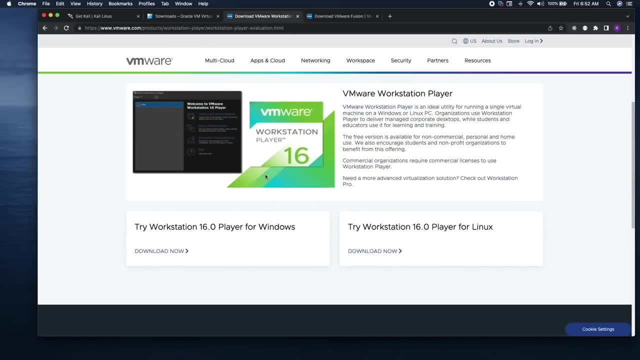 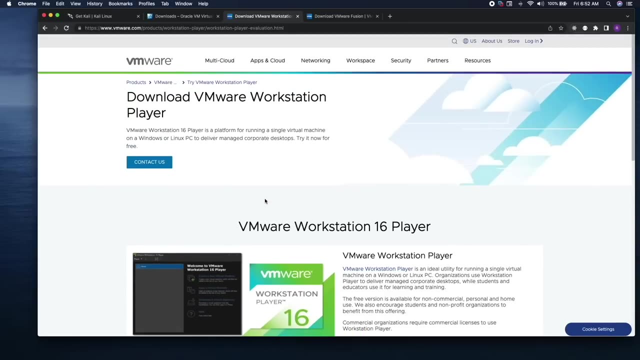 and we'll walk through the steps to do that. Or you can run VMware. If you are running on Windows, you will download it here and I'll have this linked in the course resources. You will download the VMware workstation and you will run this as your virtual machine hosting software. VMware is. 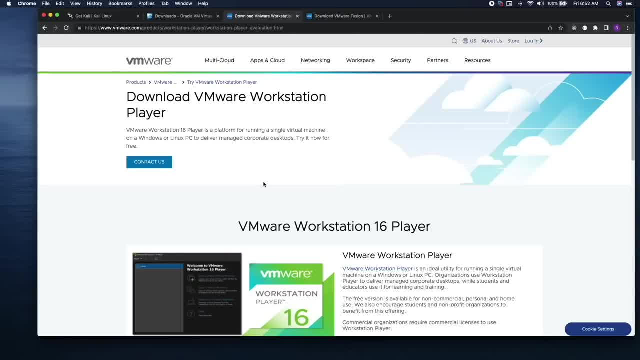 my go-to. I still use VMware. You get 30 days free, So if you're struggling with VirtualBox, you can try VMware for free. You can run your Kali Linux machine on VMware and give it a test. I have never had any problems. 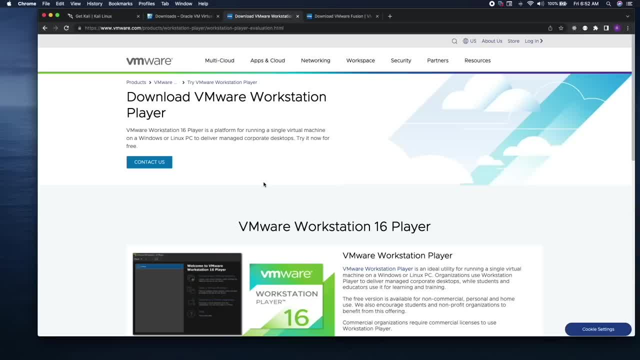 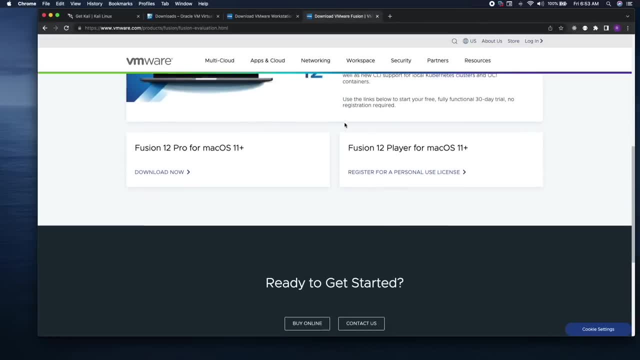 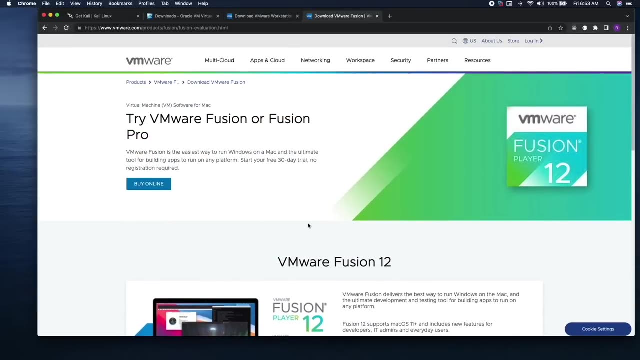 with VMware and it has worked really well for me, So it is the one I recommend. So you can download it for Windows or you can download it for Mac. I am running a Mac and I run VMware Fusion, because that's VMware's software for Macs. 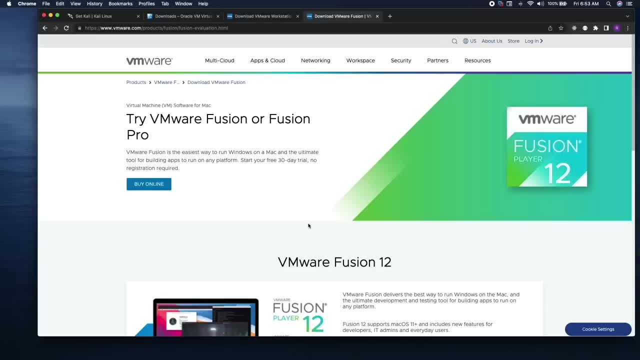 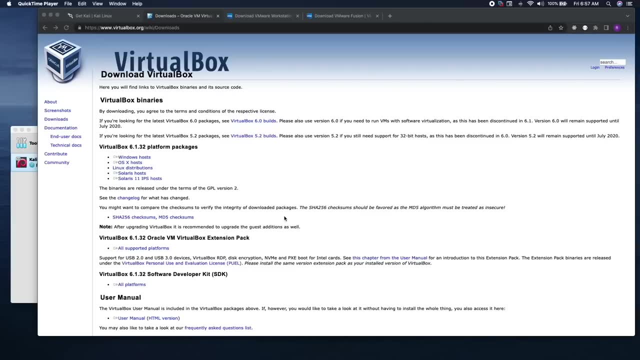 your decision. you can choose which one you would like and begin installing it in the next video. all right, if you have chosen virtual box as your virtual machine hosting software, may the force be with you and you have much better luck than i did. if you are on windows, you will go ahead and 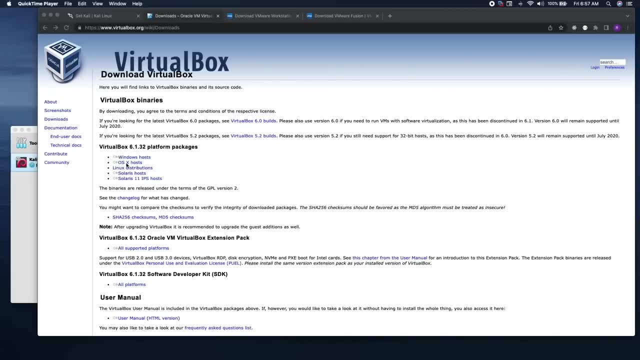 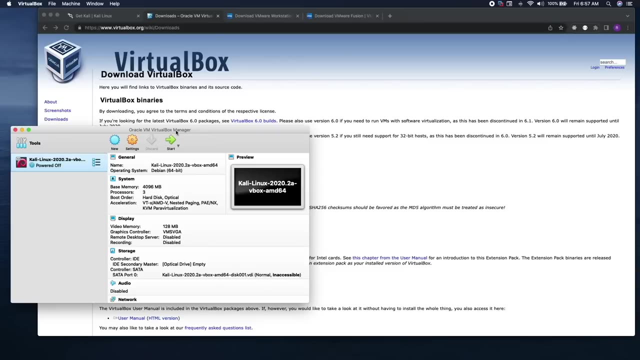 download for the windows. if you are on mac, you will download for a mac. i have already downloaded virtual box. it is really simple. you click download, you will extract the download and then this is what you will be brought to: a virtual box manager. i have a really old machine, that's actually. 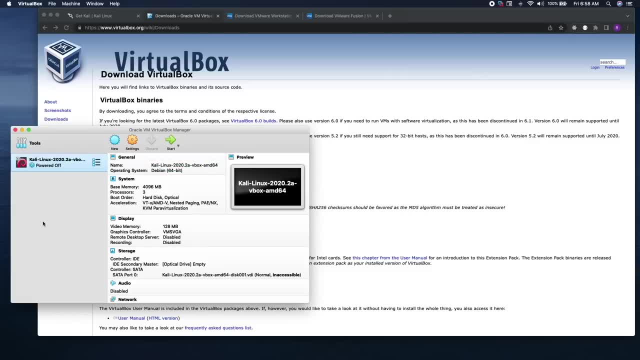 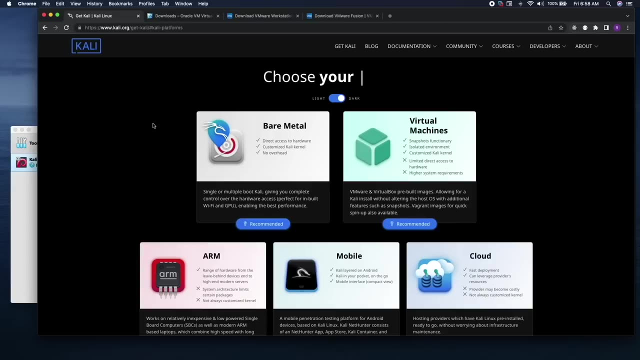 deleted off my mac. now you can see, the last time i ran virtual box was in 2020 and i downloaded the, this virtual machine from Kali Linux, and so what you'll do is this will be listed in the course resources. however you will come over here, you will go virtual. 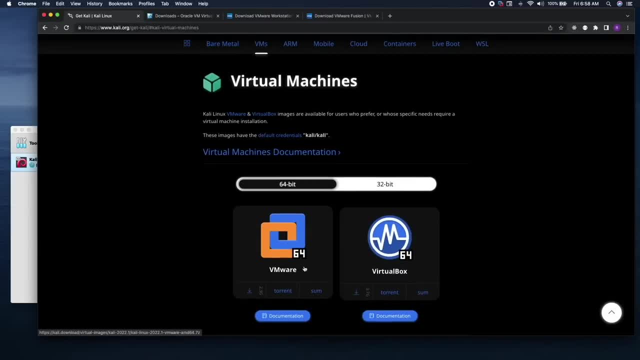 machines. it will ask you: do you want to use VirtualBox or VMware? and you will choose VirtualBox for the sake of this video. it is quite a large download. I am not going to download it because I am running out of space on my Mac, but you 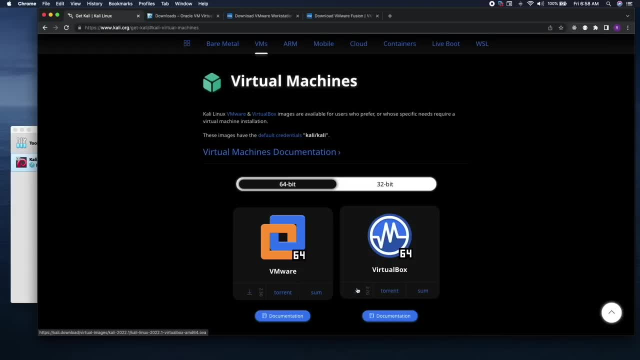 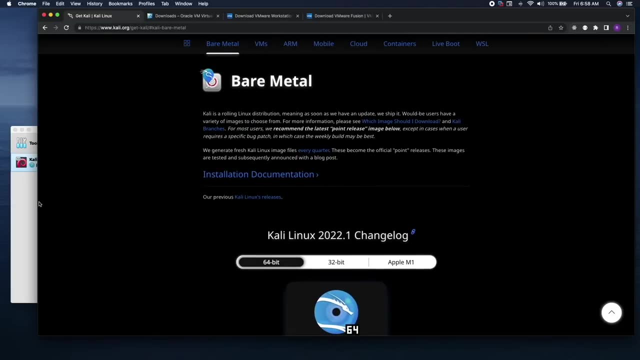 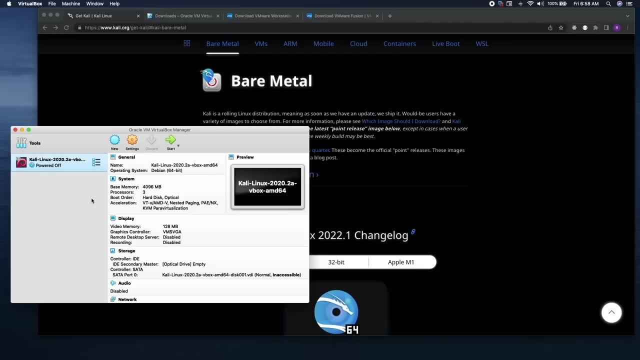 will hit download, it will save to your downloads- if you're on a Mac, I'm assuming it'll save to your downloads if you're on Windows as well- and then, once it is finished downloading, you will open up your file that it is in. you will extract it because I think it downloads as a zip, and once you have done that and 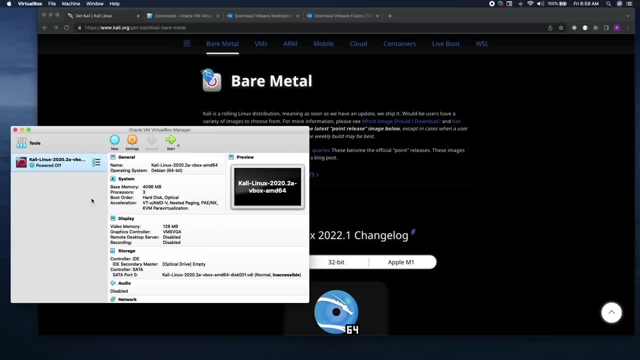 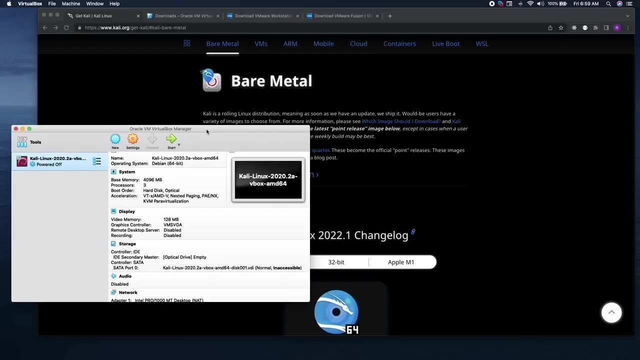 you are ready to open it. you will right click on the VirtualBox image that has finished downloading. you will right click on it and it will say open with and you will click on it and it will say open with. and it will say open with. click open with virtual box and it will bring you to this page. It might actually even try. 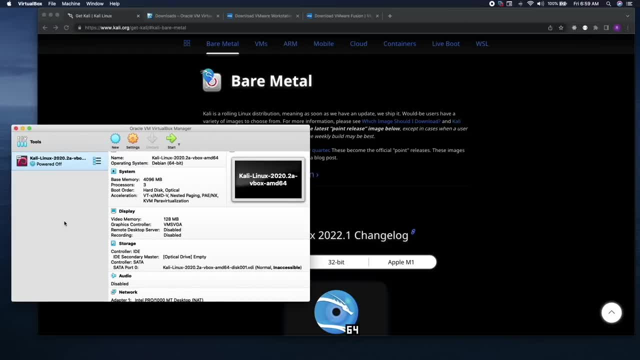 to open the machine and start it and you can let it run and then shut it down. You'll want to shut it down because there's a few things you need to set up on it before you do within this settings tab. Okay, one thing I forgot to mention. when you launch your box, or it. 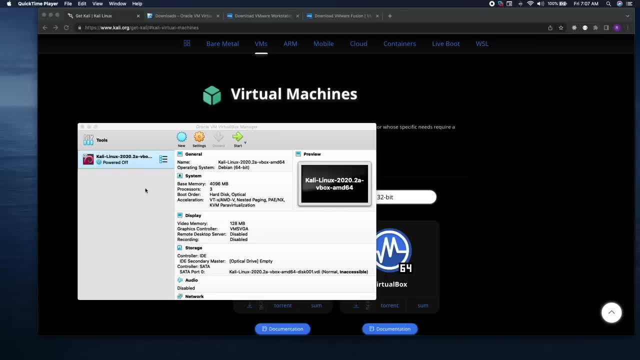 automatically starts. you will need to click I copied it. when you are prompted It's going to ask you where the machine came from. I forget the other option. All I remember is you need to click I copied it And if you save this machine on like an external hard, 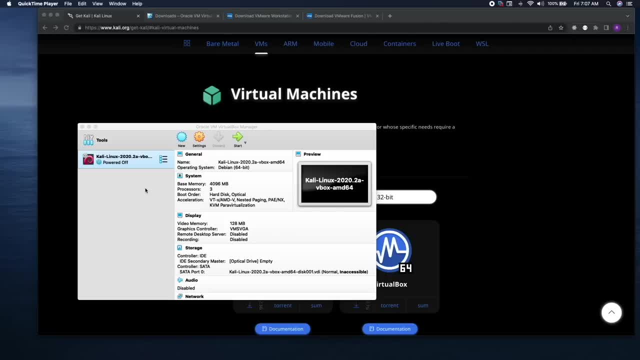 drive or something and your computer- either your Windows software or your Mac, whatever you're running- crashes. you can always grab your old virtual machine off that external hard drive And when you put it back onto virtual box it's going to ask you the same. 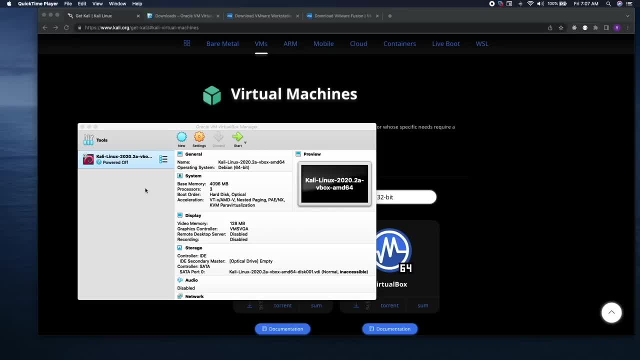 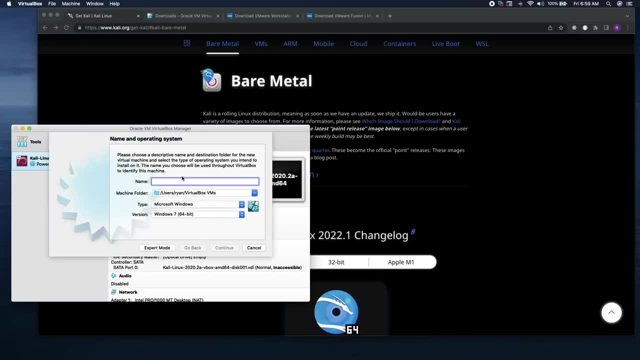 thing and it'll ask you where the image came from and you will select. I copied it, So remember to select that. Also, you can, instead of right clicking and opening it, you can, come in here and name your Linux box that you've just downloaded from Kali Linux. You can go to the place where 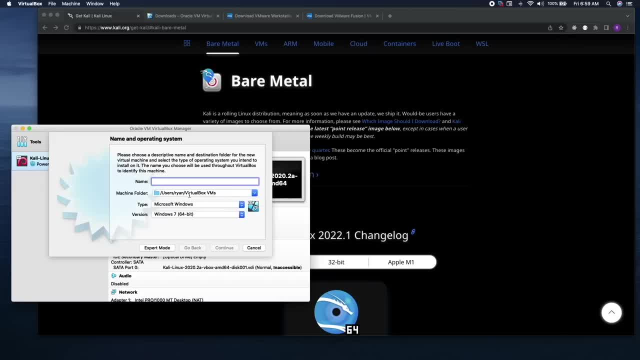 your virtual box is stored and you can click on it and then you can open it. I don't recommend that way because it is more challenging and I remember struggling to get that to even work. It's easier just to open with let the box start to open, either let it open all. 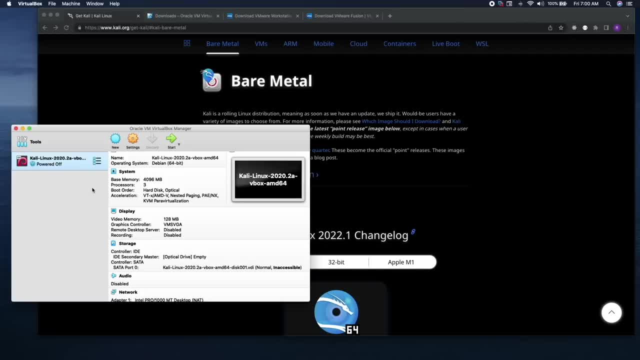 the way up. So you can see here that the default credentials to log in, as Kali is your username and Kali will be your password. However, shut it down once that's happened, because it will begin to lag. If you don't, you'll need to come into your settings and this will matter based. 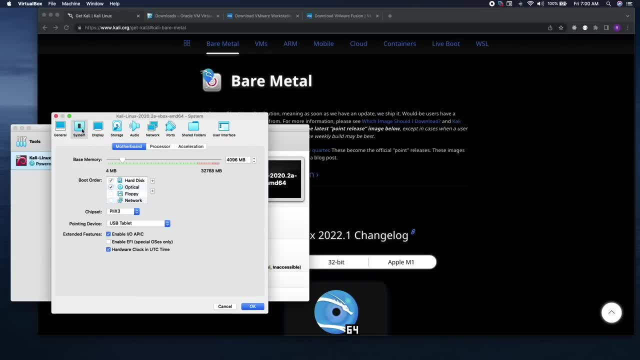 on how much Ram space you have and how many CPUs. We will go over to our settings. We will want to adjust our RAM to as much as you can dedicate. I think I do somewhere around eight to 10.. Okay, So I'm really not sure how much I give it. I know that it's a lot, especially on virtual. 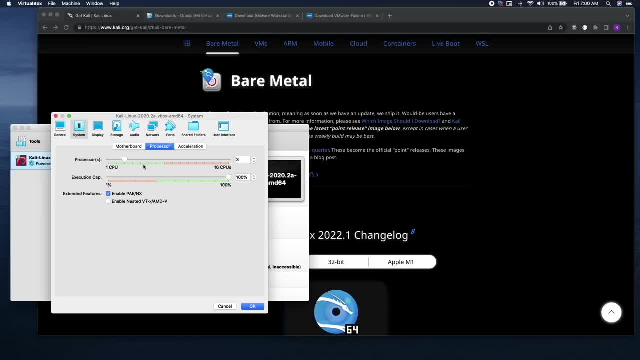 box. It's going to eat all the RAM you give it. It will also eat all your CPUs. I typically dedicate four to the machine- I think the one that I'm I work on the most. I might even dedicate eight. I might even have more than that. I'm not really sure, but the more 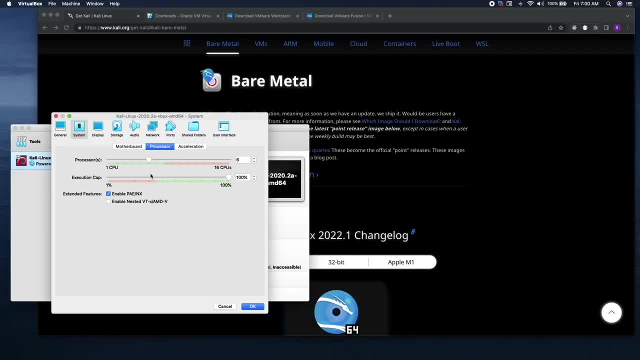 CPUs you can dedicate especially to virtual box, the better, because it will use all of what you give it. And if you don't have a lot, that's okay. You just might have a lot of RAM, So you can use as much RAM as you can. 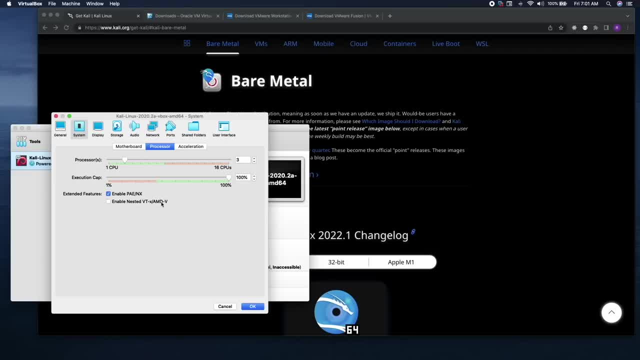 Okay. So you might not be able to run hash cat, which we will get to way later in this course. I think it'll be somewhere around eight hours into this course. You might struggle running hash cat, but that's okay. You will be able to copy everything as I have ran it for us. 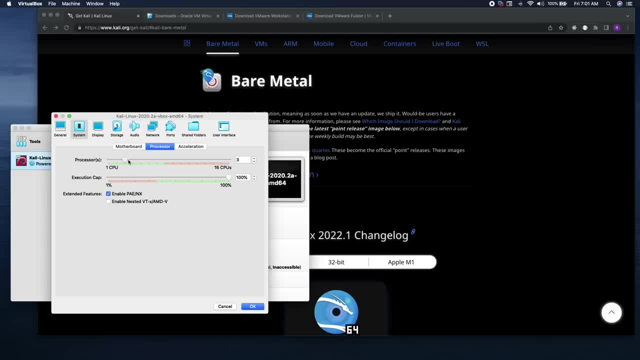 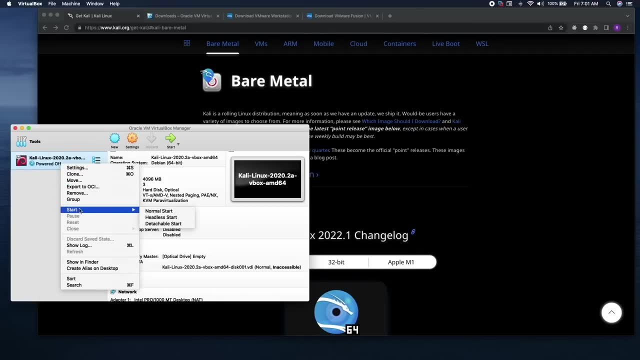 in the videos. And that is it for setting it up. You'll hit Okay, I'm going to close out of it, and then you will launch the box. You can right click on it and then you can go to start and you will start the machine. 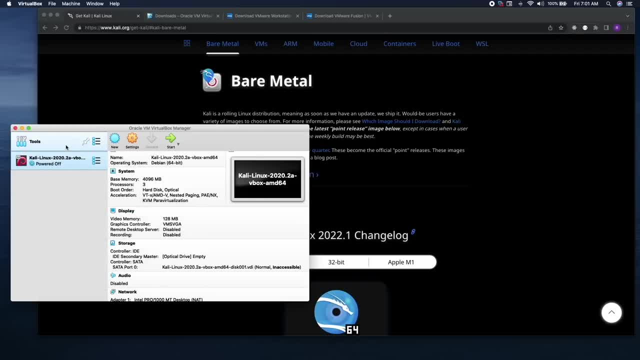 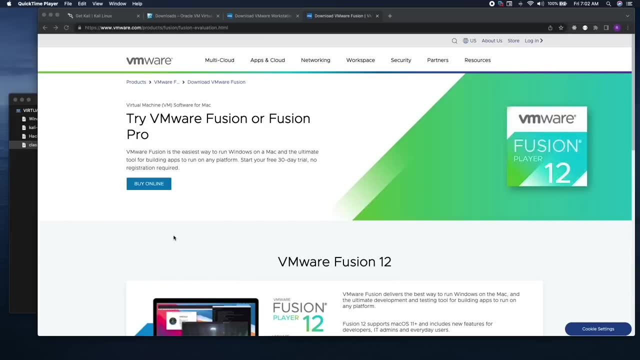 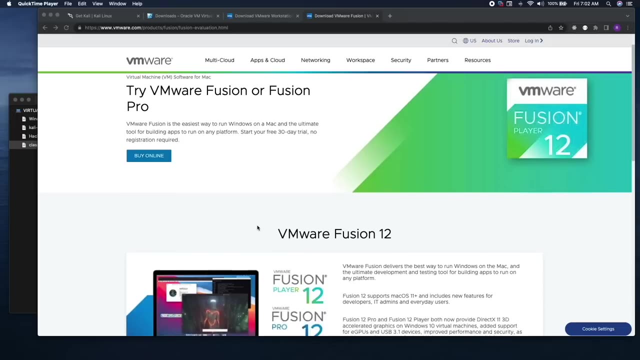 You will log in. Okay, So I'm going to click on the inside. All right, If you have chosen VMware, this video and setup is for you. If you have chosen VMware, I think you have chosen wisely, So what you will do, I am running VMware fusion, so I would come down here and I would download. 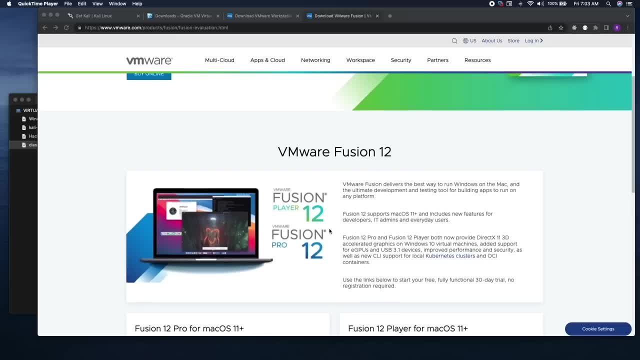 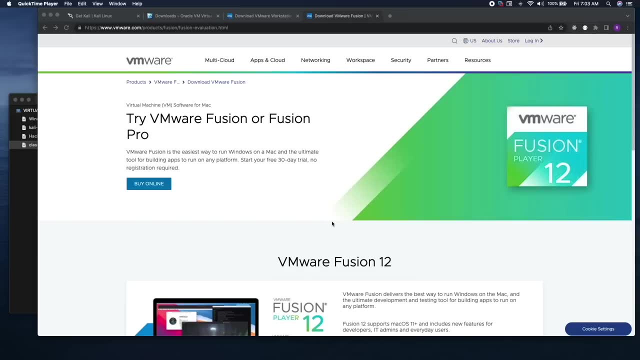 the VMware fusion player. I have already downloaded it, so I am not going to do that again. Once it downloads, it will save into your downloads and you will extract the zip. Okay, grandi the zip if it is in a zip folder, and then you will open, you will drag it on. 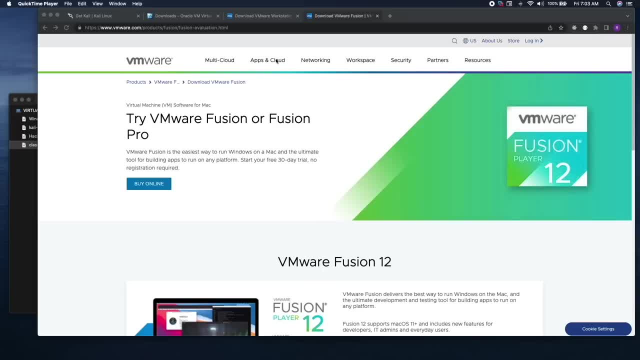 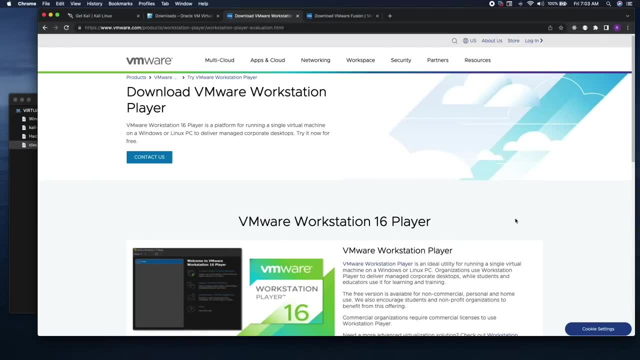 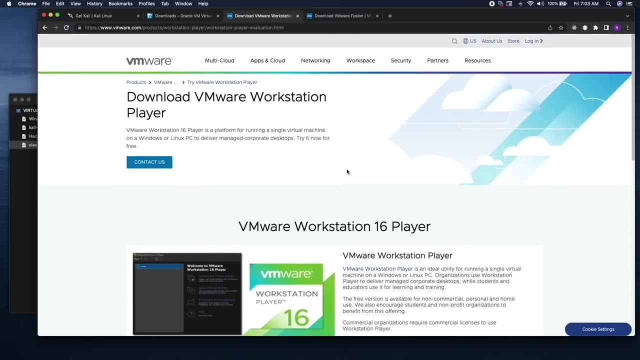 a Mac, You'll drag it into your applications And then you can launch your VM 살 fusion software. If you're on windows, I actually have a windows box over here which I have not downloaded VMware fusion On or VMware on, but I'm assuming it is going to be done just the same. 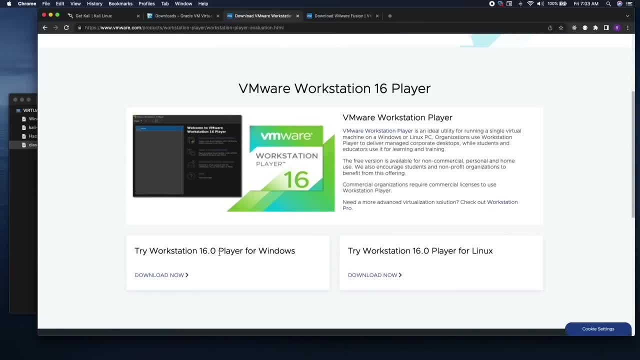 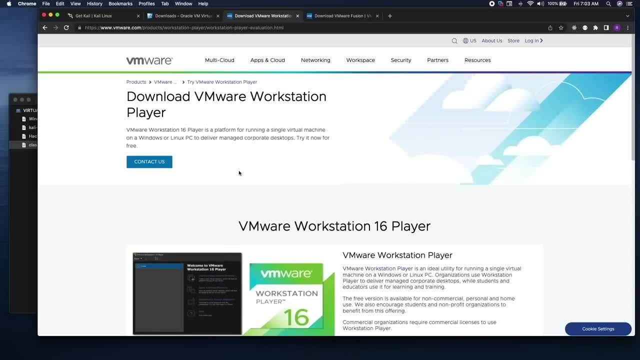 You would come into a VMware, you would come down to windows, You will download it, You'll extract it- if it downloads into a zip, and you will then launch that and you will have something that looks similar to this and it'll look: here you go, it'll. 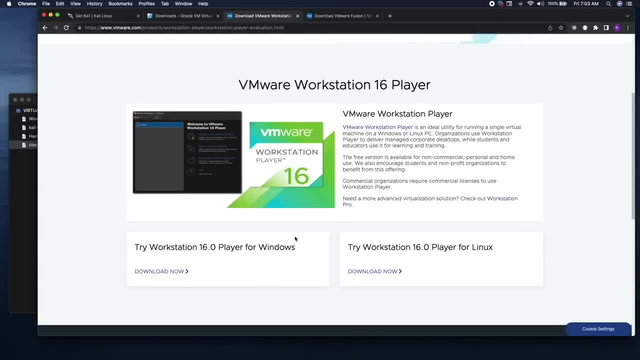 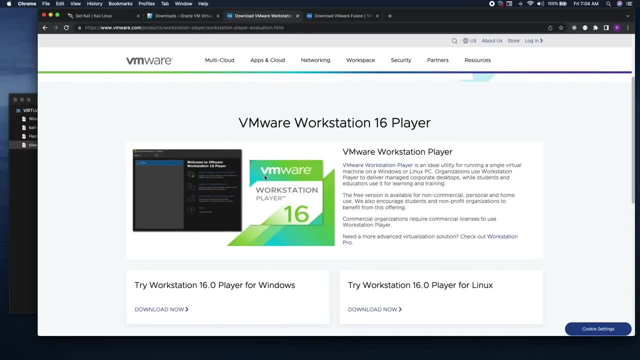 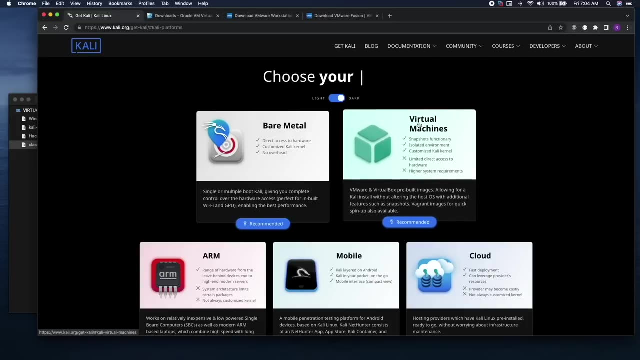 look like this: basically exactly what I have here, and then from here we are going to put our virtual machine into our virtual hosting software, so we will go to Kali Linux. this is also linked in the course resources. we need a virtual machine, so we shall select that if you chose VMware. 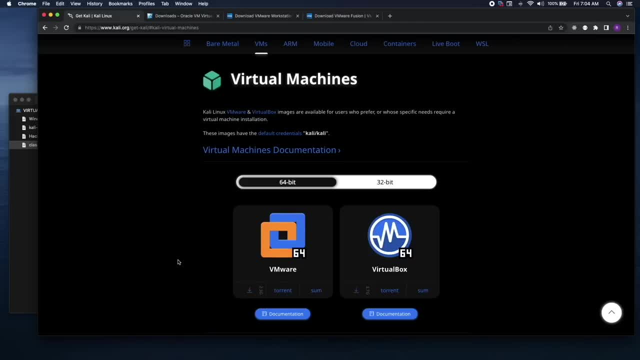 you will download right here. it's 2.3 gig. I am fairly certain this is zipped and you will need to unzip it. there's a several different ways to unzip it and you will have to go about unzipping it however you choose once it is unzipped. 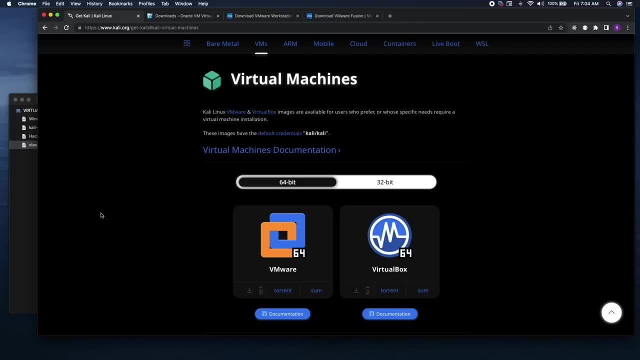 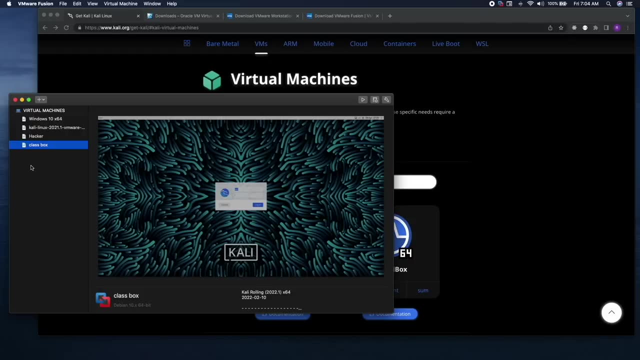 you can actually go into the downloads, where it is saved, and you can just click on that unzipped image and you can just drag it over here and you can drop it it or you can right click and then select open with VMware fusion. one thing to remember: when you open it it's gonna say where did this image come from? and 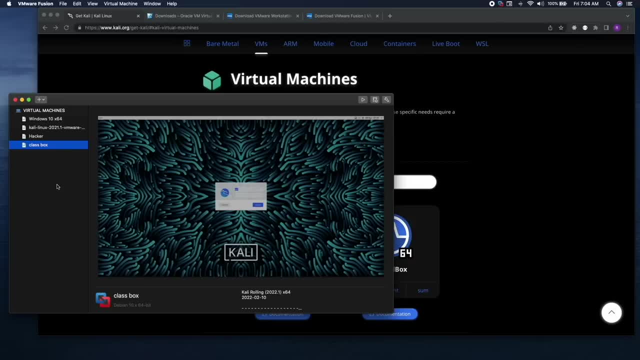 you're gonna say I copied it. it's important to click I copied it or you will not be able to get the image to open. now that we have the image on our box, we will want to adjust our settings. you can right click and go to settings. 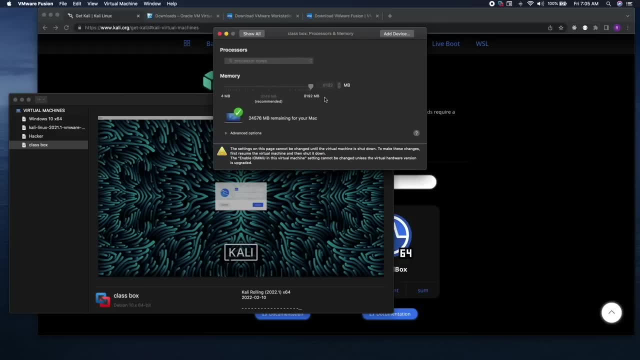 we will want to have our memory really high. I went ahead and just put as much RAM as I could dedicate towards it, and I have five processors, five cores, dedicated to the machine as well. you will want to dedicate as much as you can spare. if you don't have a lot, that's okay. you won't be able to run hashcat as. 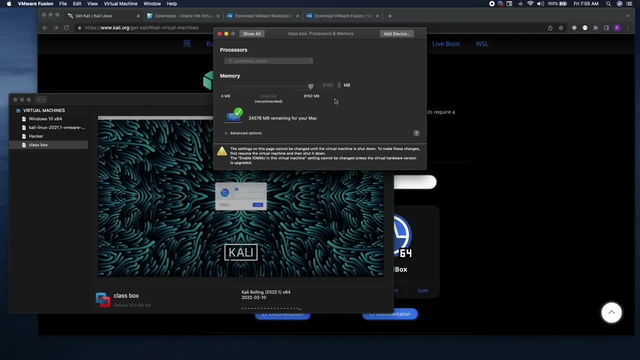 we will see later on. I have tried to run hashcat with less cores and less RAM and it would just air out and say that there is not enough space to run the hashcat. and it will just air out and say that there is not enough space. 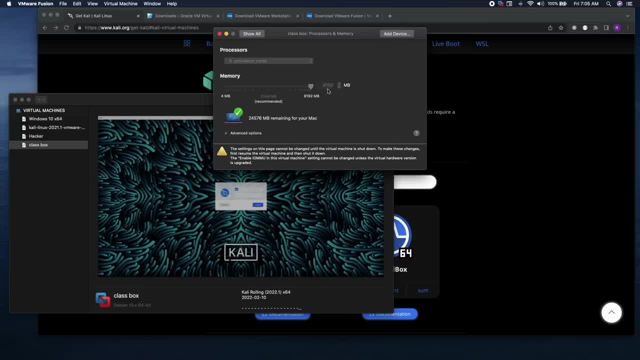 or memory dedicated to the machine, and that's fine. if you don't have that, I will be able to show you all of the cracked passwords and hashes as we go through this course. but the more you have to dedicate to your machine, you will be able to faster crack password passwords and hashes, but this will not. 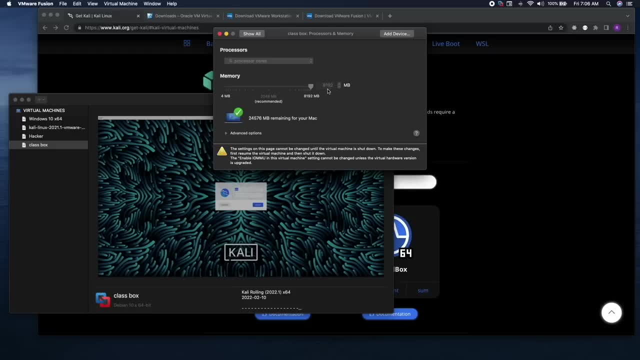 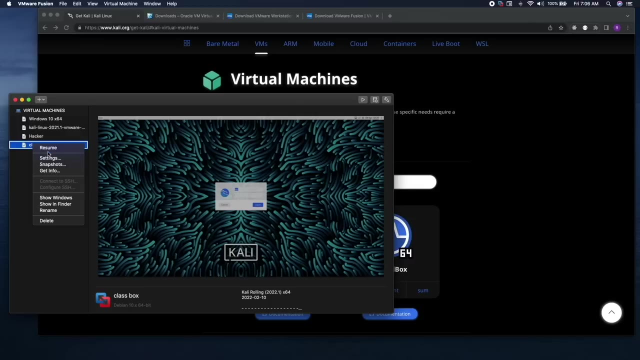 be something that we encounter until at least eight hours into the course, so you will likely forget about this and you can just run it with however much space you have to dedicate and, with that, your default credentials. when you launch your box, you will right-click and you can resume, or you. 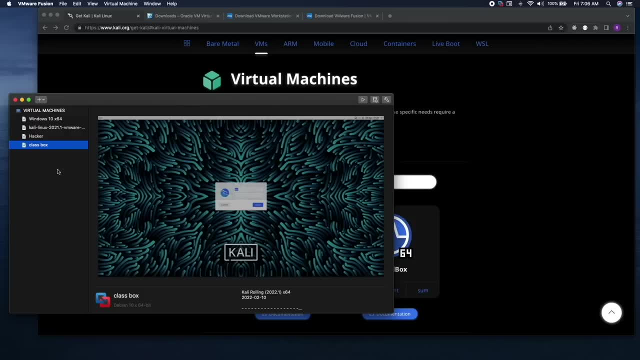 it'll say start if it's in a powered off state, and your default credentials will be the username Cali and the password Cali, and with that I will see you on the inside. in this video, we're going to talk about how to scan specific targets in. 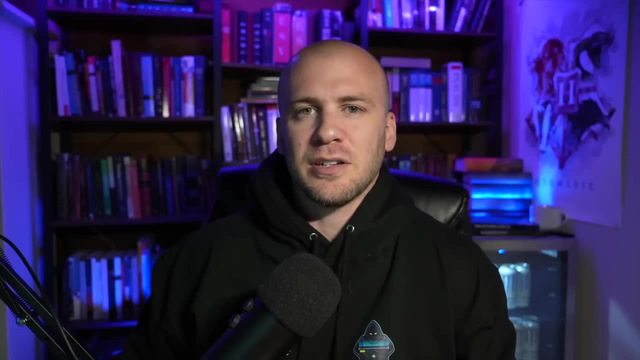 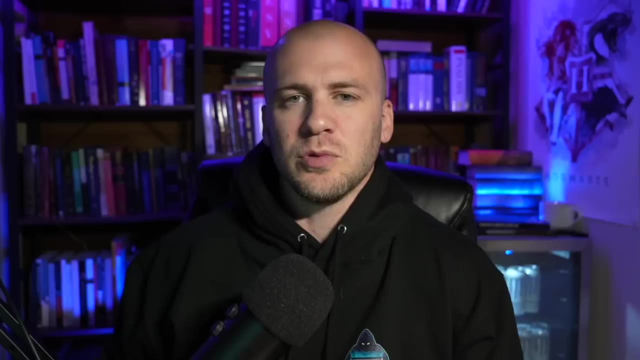 bug bounty programs as well as fuzzing our targets without getting ourselves into any trouble. I know there's a lot of interest in learning how to scan and fuzz bug bounty targets, because sometimes you'll be reading through a program's rules and it will specifically say that there is no scanning allowed. now there's a couple. 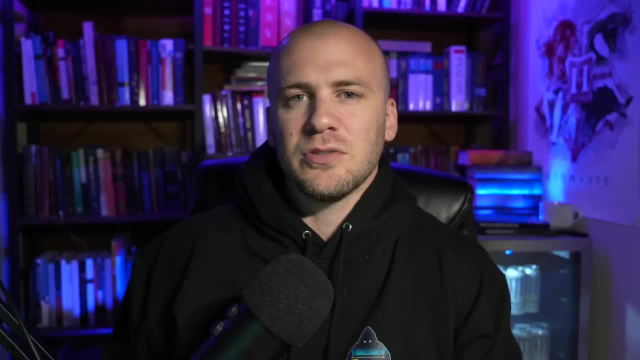 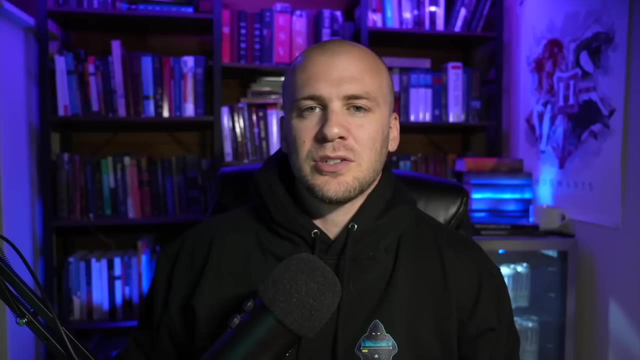 ways to get around this and if you watch my Shodan video, you can actually use Shodan to scan your bug bounty targets and then you don't have to worry about anything because you're using Shodan, and that is one way to get around scanning a. 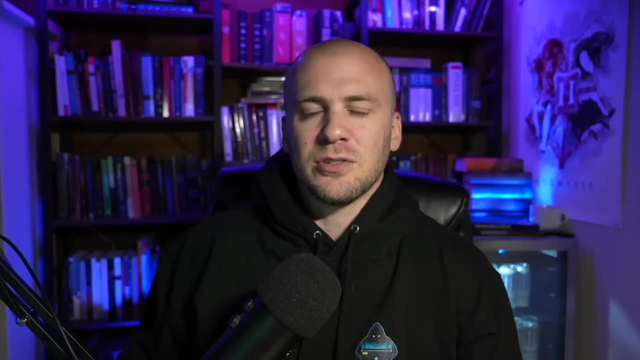 target and staying in the clear. now you can use in map and fuzzing tools to do this as well, and that's the purpose of this video. so we're gonna go ahead and look at this and I'm going to show you how to do this without getting yourself. 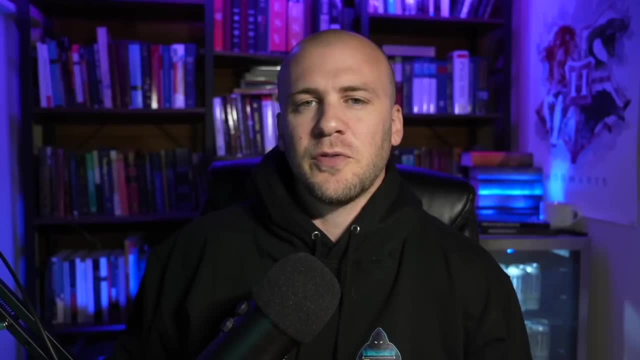 into any hot water and to be able to scan these targets without any issue. before we get going too far, I want to explain to you why you're not allowed to scan these specific targets, and there's really two main reasons. one, the company doesn't want a bunch of bug bounty hunters using fup, which is going to send. 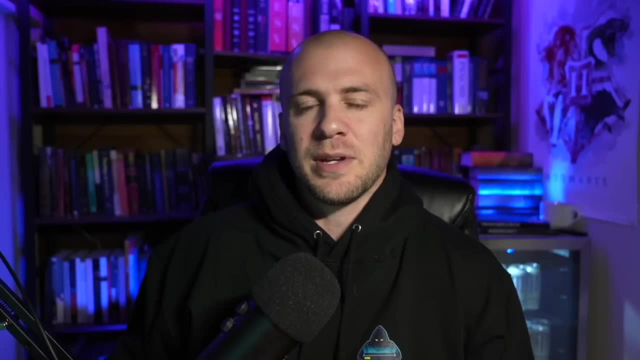 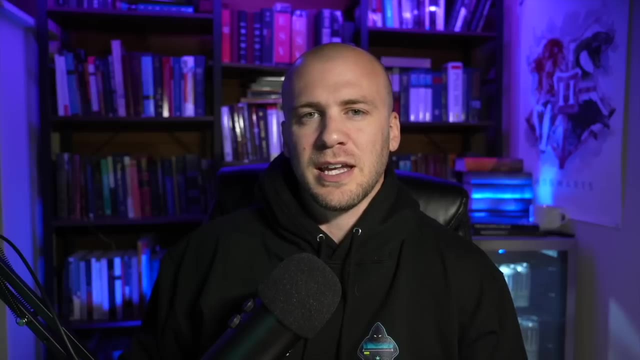 several hundred requests per second to their server and have them get dosed, and sometimes, if you do this, you will actually get rate limited or even have your IP banned, which is why I always recommend using a VPN. but there is a way to get around this and I'm going to show you that at the end of this video and 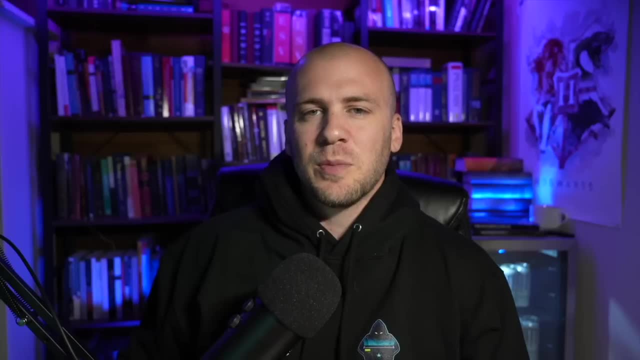 the second reason a lot of programs are going to tell you they don't want you scanning the network is people will use a vulnerability scanners and this is just really a big no-no: don't use vulnerability scanners. recently a program went live and then they were getting scanned so much with. 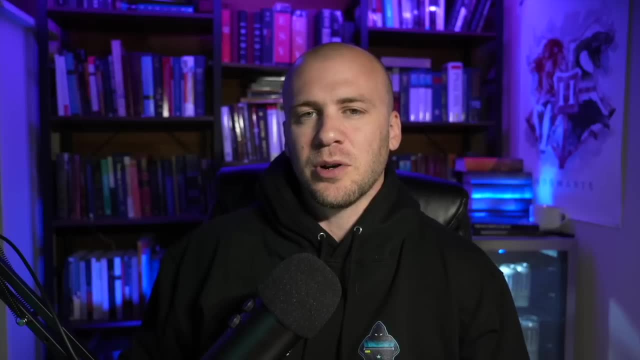 vulnerability scanners that they actually removed themselves from the bug bounty program. so don't use vulnerability scanners. these are the two big reasons why a lot of programs will say no scanning, and so just be aware of that. if you're going to fuzz for directories, make sure to slow down the 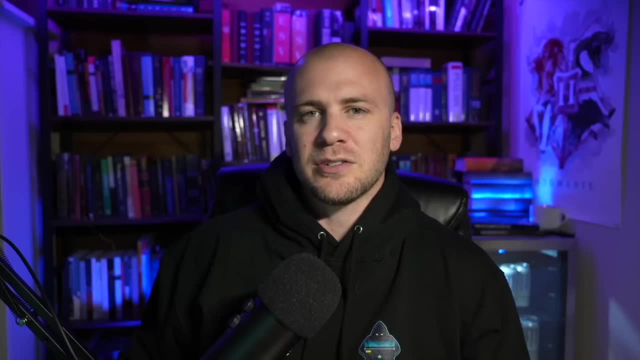 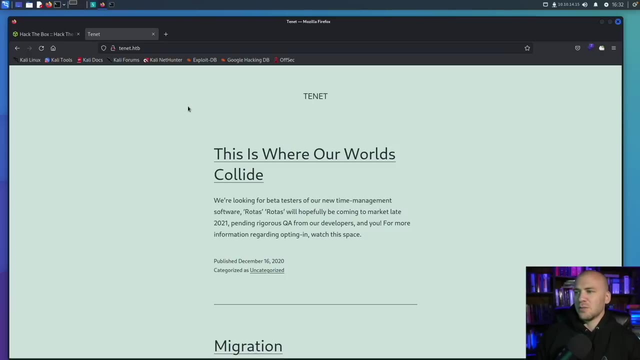 amount of requests which I'm going to show you how to do. and don't use vulnerability scanners now. first I want to show you how to use in map without getting yourself into any trouble, so I've gone ahead and opened up tenant from hack the box here. if you follow my channel at all, you will know this is my. 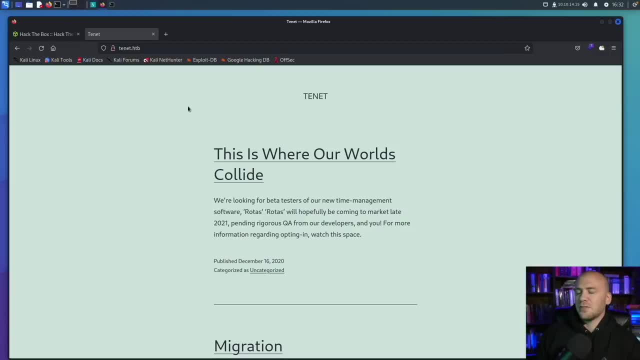 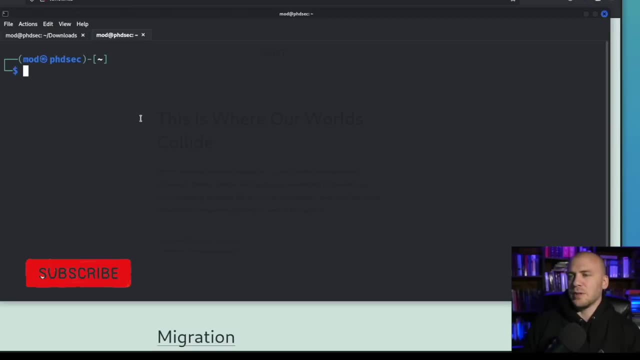 go-to box for web app education, and the first thing we are going to do is run an in-map scan. so we have opened up our terminal here and you're probably familiar by now with an in-map scan. now this is the typical in-map scan that I 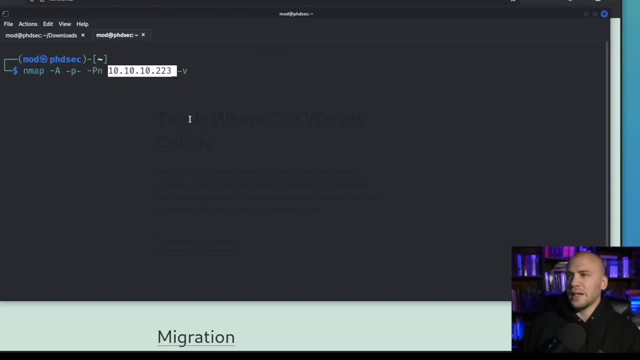 like to run change the IP right here. so, if you would like to jot this down, this is how I run an in-map scan if I'm doing a capture the flag. but we are not doing a capture the flag, we're going to be scanning a bug bounty program and and it's going to 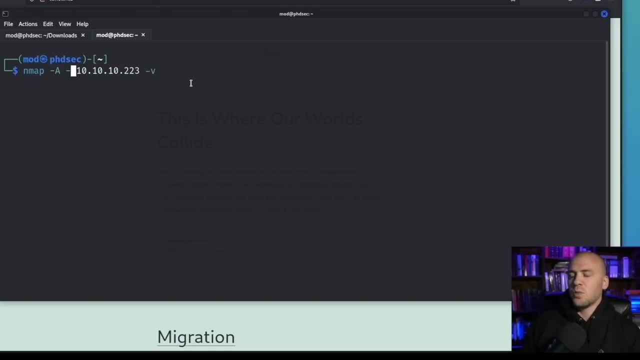 look a little bit different. so we still want this dash a. we will want a dash capital F, and this is only going to scan the top 100 ports. the reason I'm telling you to use the dash F is because if you're new, you're probably not going to. 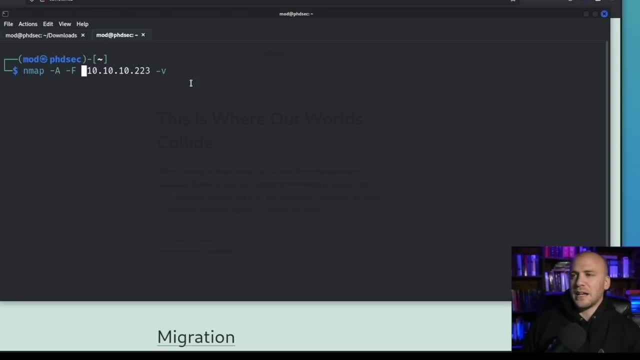 know which ports you want to look at. so I have a list of ports that I use when I run an in-map scan. because you don't want to scan all 65 535 ports- I think that's how many there are. you want to scan just a specific number of ports, a? 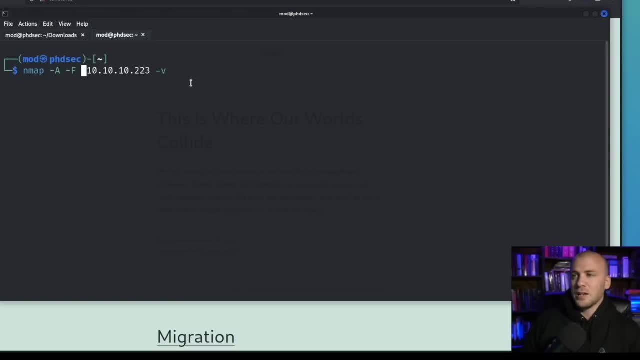 lot of networks are not going to want you going out and scanning their entire network, but it's okay to go out and scan the top 100 ports. they're probably not even going to notice, and I'll show you how to make it so that they're not going. 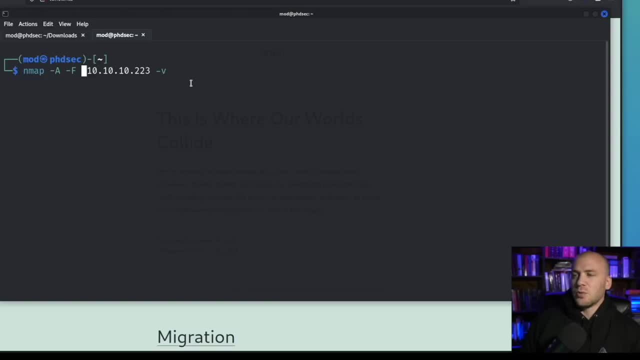 to notice and you're not going to cause any kind of intrusion and they're not going to care. so we want to run the dash F for our ports and then you're going to want to run a dash and then a 1 or a 2, this is going to really slow down your network scan. I think that Nmap runs on. 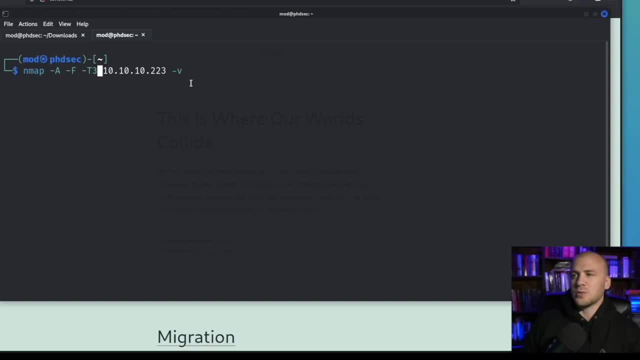 a T3 automatically, and if I'm in a hurry and I just want some ports to shoot at, if I'm in a CTF, I'll run a T5. That's as fast as you can go, but if you run a T5 in a CTF you can actually miss. 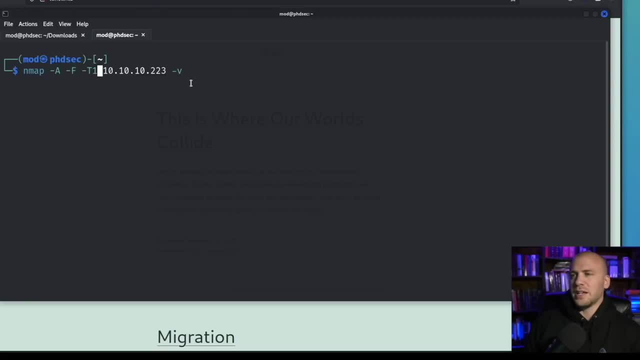 some ports. So if you're really nervous about running any kind of scan, you can go ahead and run a T1, and they're not going to notice that you're scanning their ports. This is going to really slow down your Nmap scan and then this dash V right here will tell you the open ports. 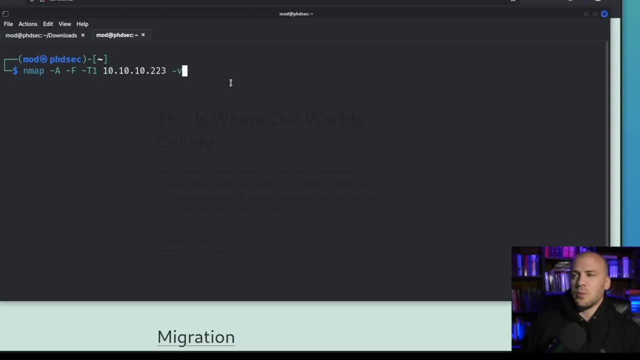 as it hits them. So this is going to run a really slow scan on the top 100 ports and nobody's going to notice, So you can go ahead and run this and it says that there are two ports and it's going. 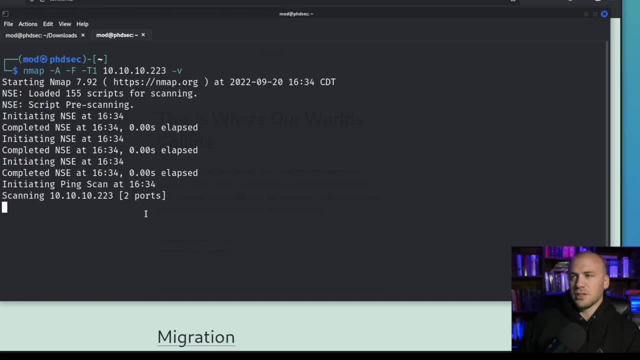 to pop down with the ports as it hits them, And so eventually you're going to see port 80 pop up, and I'm not really sure what other ports are open on this program. but this is how I would run an Nmap scan, And so you can see right here it tells us that it's scanning the top 100 ports. All right, 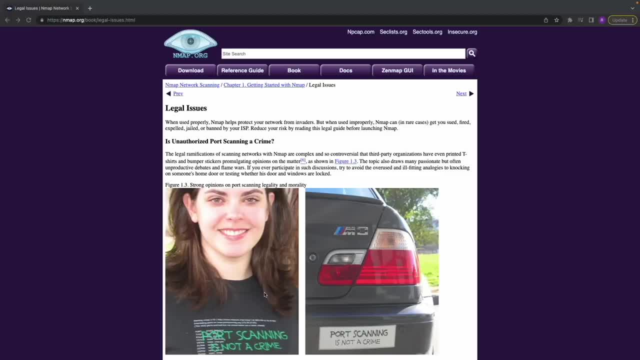 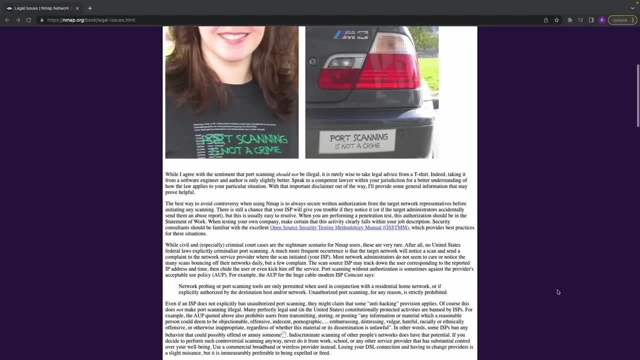 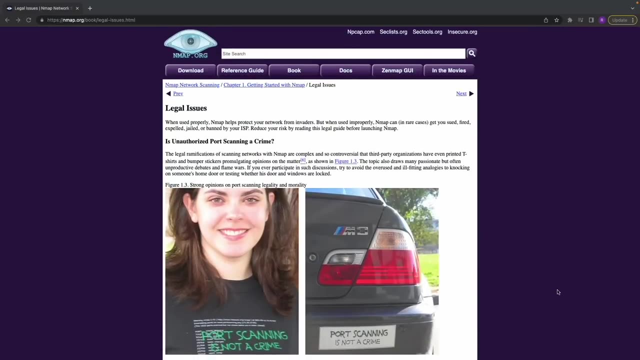 so I decided to go ahead and add in this Nmap network scanning legal issues page. So if you have any questions about using Nmap legally on your specific targets and you're still worried about it, you can come and read this right here and it's going to give you a kind of the legalities of using on different. 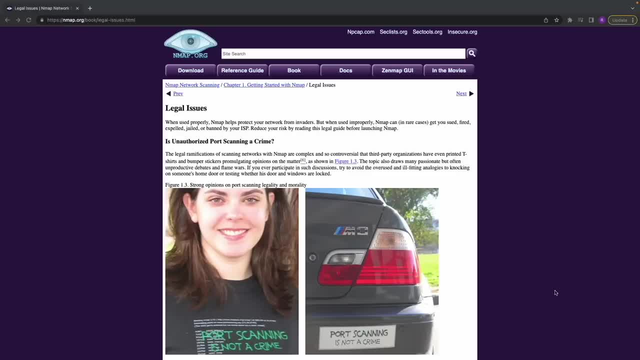 networks. I am not a lawyer, so I decided to go ahead and add this disclaimer in there that you are using this at your own risk and you should check with the laws in your specific state on port scanning. So this is how I would run an Nmap scan, if I'm running one on a bug burning program. 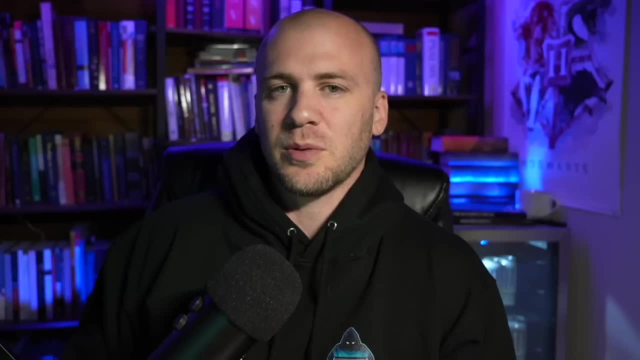 This is going to be a really safe scan to run, and it's going to tell you the information that you want from these specific ports- which ports are open, what versions are running on your target, So you can go ahead and play around with Nmap. This is how I do it, though, and I want to show. 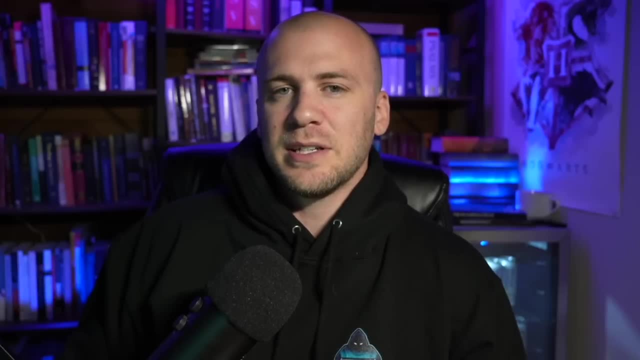 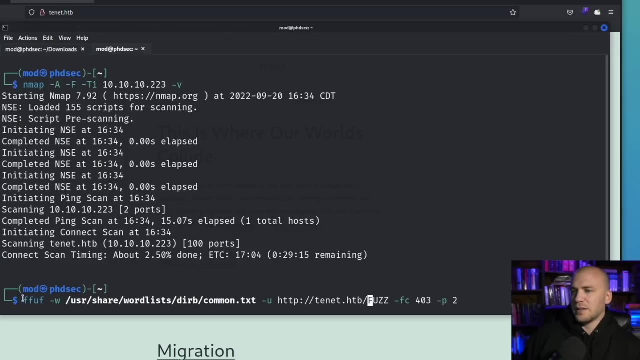 you how to fuzz for directories in a safe manner, And you may still end up getting rate limited, which is fine, especially if you have VPN. you can just switch your VPN, So we're going to go ahead and run FUF now, and this is the syntax for FUF. I'm going to show you this with this. 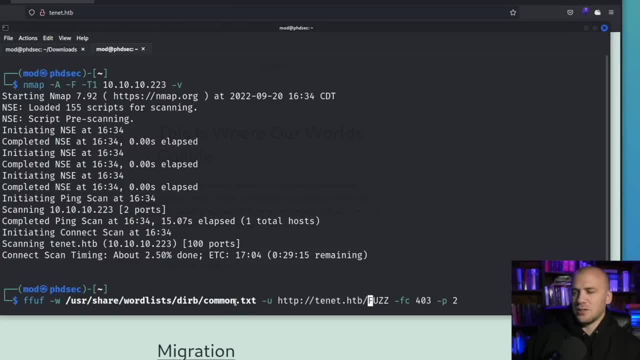 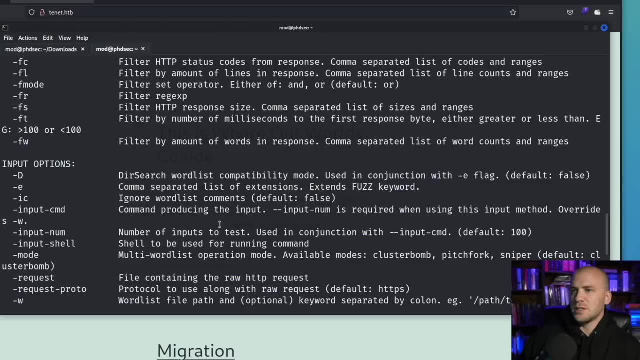 common word list right here and then we'll go ahead and run FUF. So we're going to go ahead and download Seclist and you can see a better word list than what is default on the Kali machine. We can actually see what we have as options here and you will see that I'm using the FC to filter. 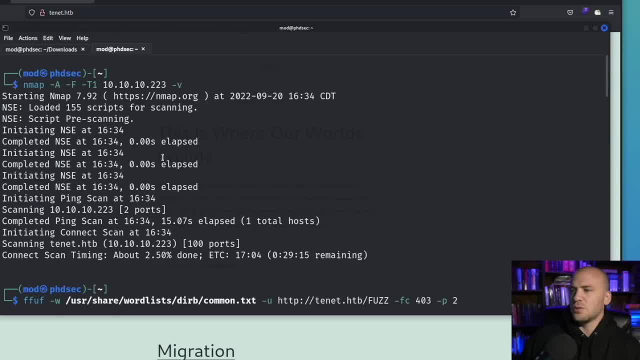 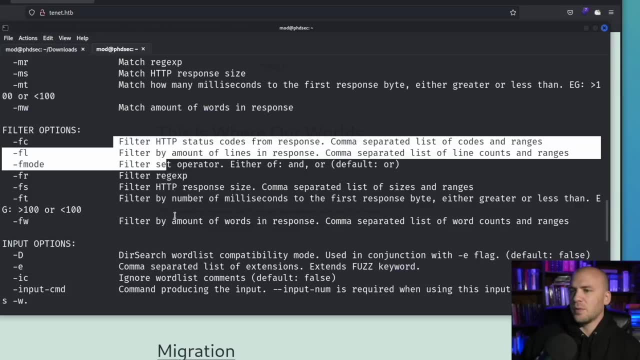 out specific codes that I don't want to see, And I think I had a 402 on here, a 403.. I don't want to see the 403s, but you can leave those in if you want, And then you can filter with other ways. 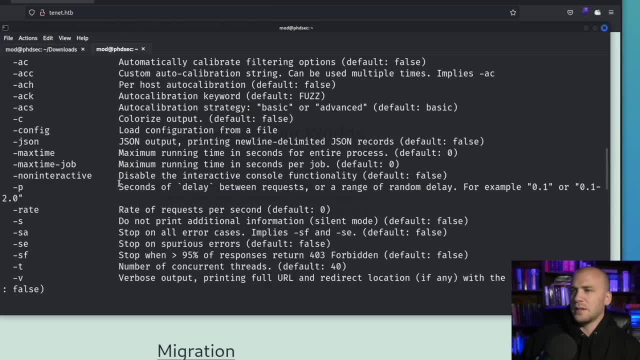 but we're looking for that dash P, and it is right here, And it's going to tell you how to delay your requests and you can slow them down by however much you want, from anywhere from 0.1 seconds to two seconds in between requests. Okay, so we have this request here. 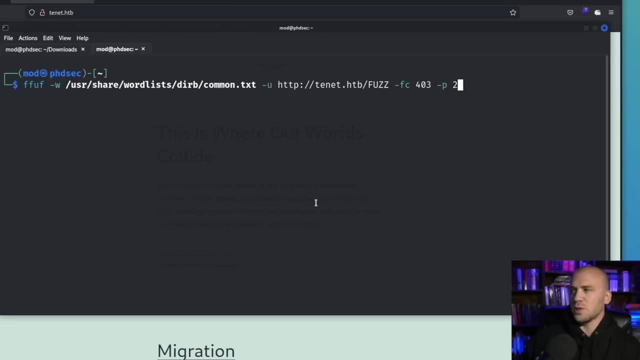 and let's say we really want to take our fuzzing really slow. You can run this with a two second delay or a one second delay in between requests. We don't really need to filter out by the not founds- And then we're going to run our word list and we're going to run the common word list. 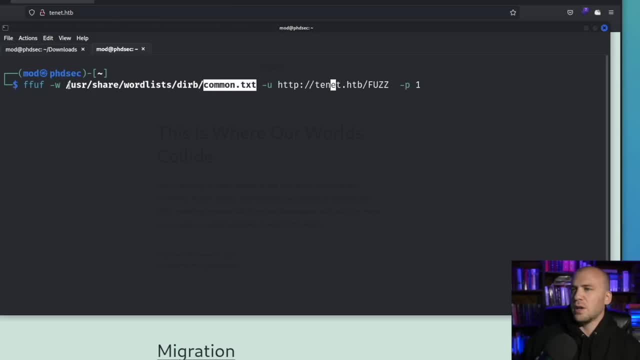 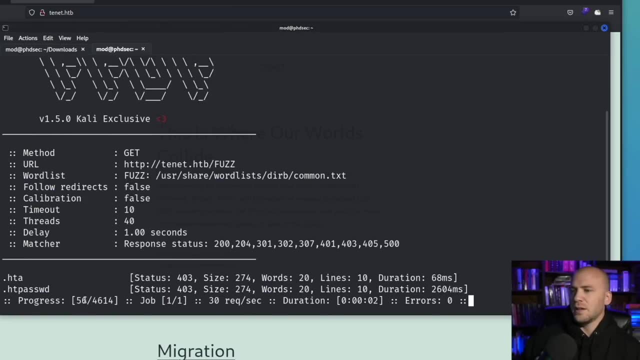 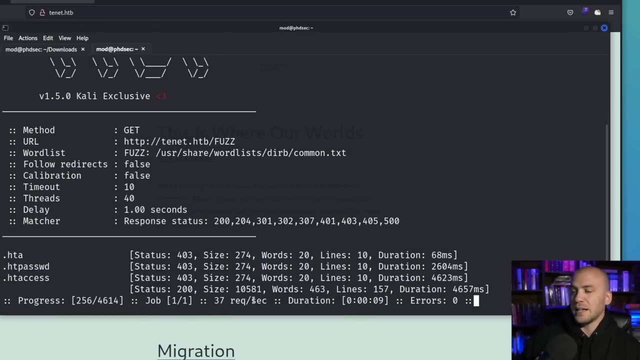 thecommonwordlisttxt. So if you want to, you can go ahead and run it just like this and you will have this word list. So if we run this, you can actually see right here the progress. you can see the number of requests that are being sent, And so it's sending 37 requests every second, which is 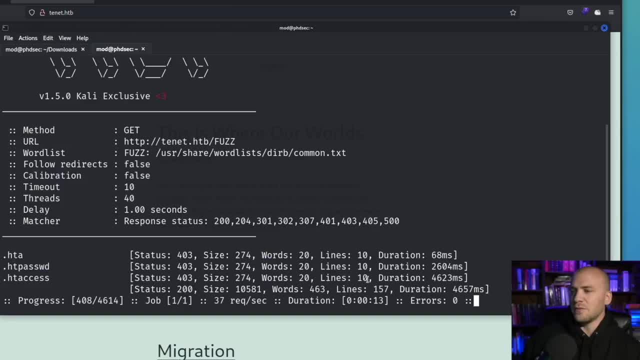 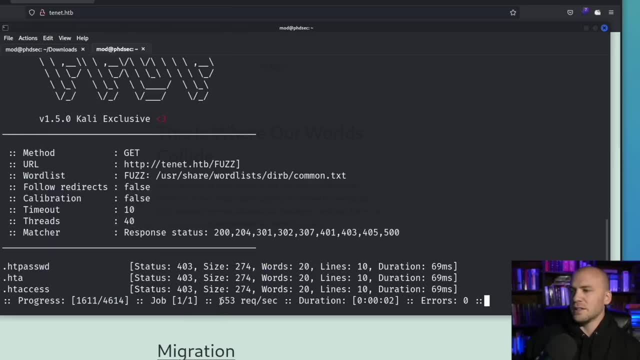 actually kind of a lot. One of the things about FUF is it is really fast. you can actually will actually show you how fast this will run without slowing it down And you can see right here: it's sending 680 requests- Around 600 requests per second, And that is really fast. you're definitely going to get yourself. 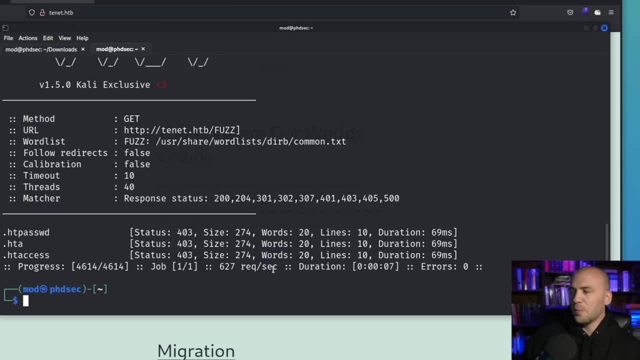 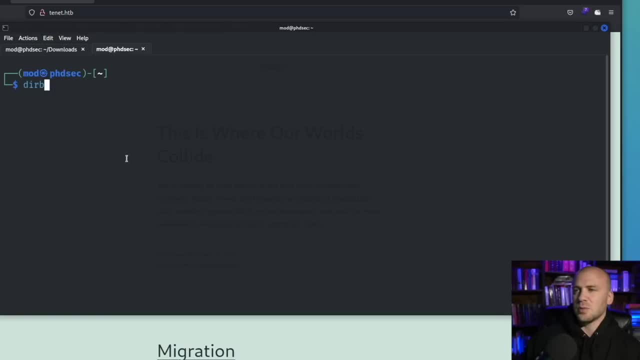 rate limited or or picked up running requests that quickly. But FUF is my go to tool. I often tell people that you can run a derp just like this And you shouldn't find yourself in any trouble because derp is pretty slow. But I like to use FUF because of the options that are available with it. 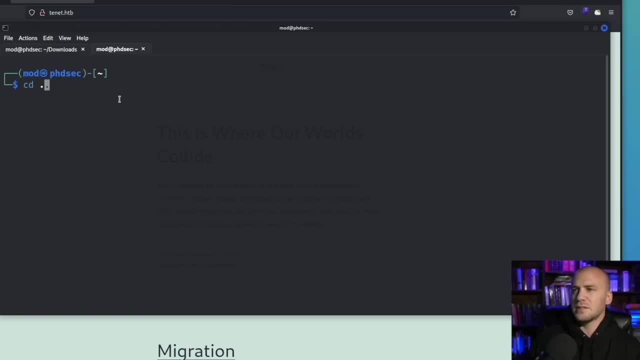 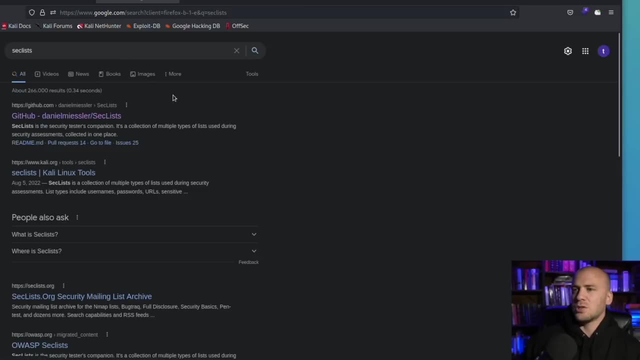 Now I want to go ahead and show you how to install SecList. I'm actually going to come back here. I do have SecList already installed, which will save a second Some time. but you can come out to Google, go to their GitHub page right here And you can run a git clone. 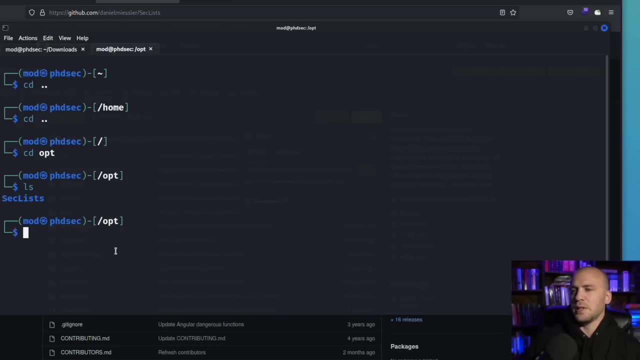 So we'll copy that right here And you'll want to CD into your opt and then you can type in a git clone right here, just like this, And you can see it's the last thing I actually installed on here. This will take a little while to run and then you can CD into the SecList And you can start looking through all. 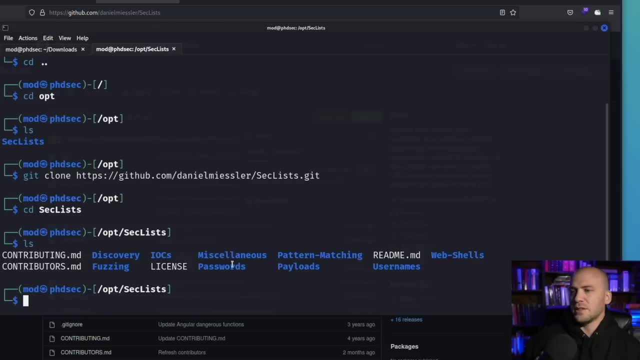 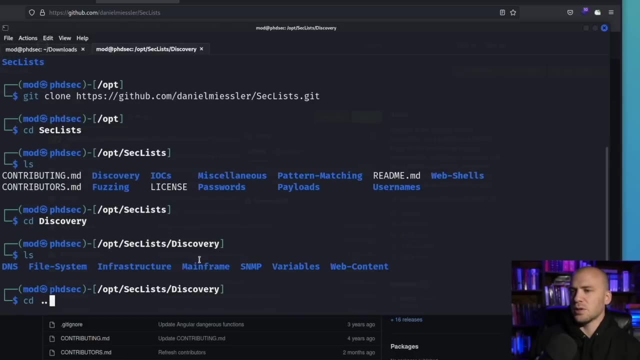 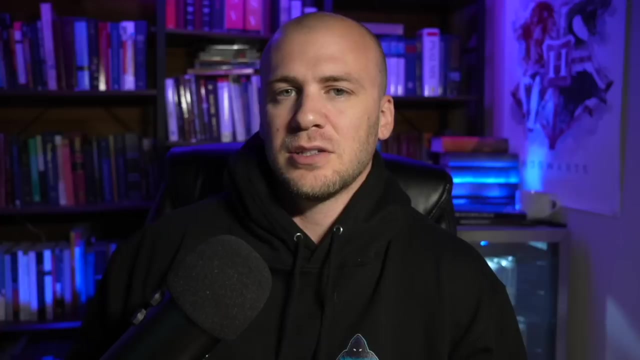 of the different word lists that they have in here. So you have a fuzzing directory, you have a discovery directory. I actually think the discovery has some pretty good word lists- And then we can CD into the fuzzing- because that's what we're doing- And there is all of these different word lists for you to pick from. 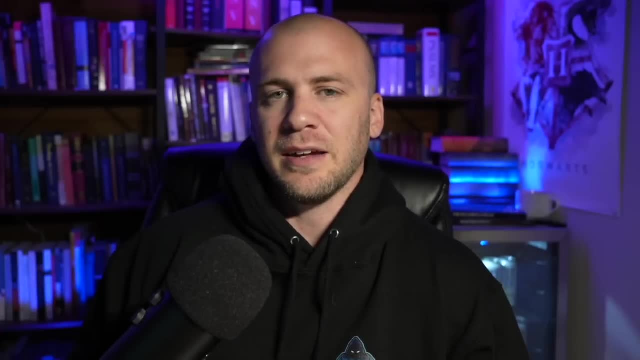 when you're doing your fuzzing. So this is how I would recommend scanning a bug bounty program if you are looking for specific ports to be open or you are checking for directories. So good luck with your bug hunting. we're going to be covering the tool Shodan For the purpose of bug bounty. 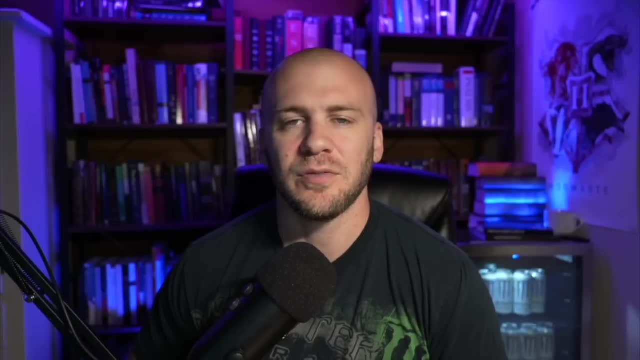 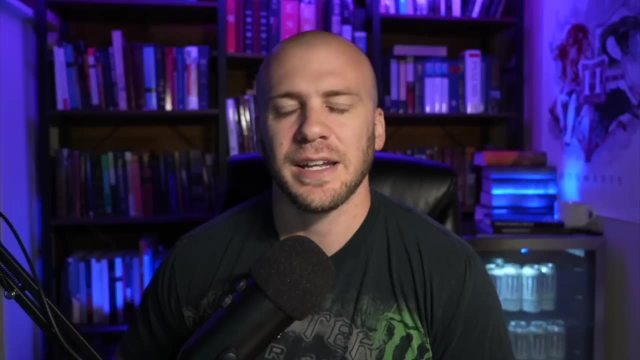 hunting and searching for vulnerabilities, as well as information disclosure and how to use the tool within the command line, as well as the actual browser. Shodan is an excellent tool for those who are new to the world of bug bounty hunting or those who are timid when they read a program and it 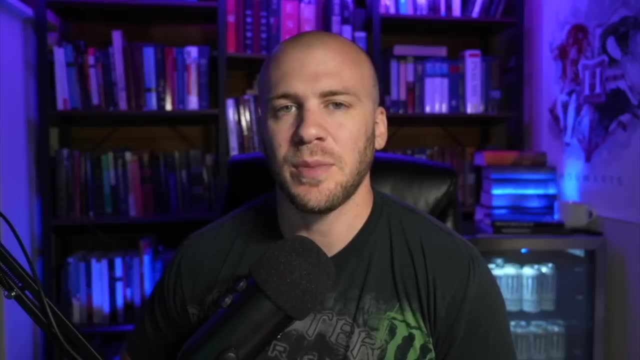 says that you should not scan a network and you don't really want to run in map and you're too afraid to actually scan the network. You can go check out Shodan, because Shodan scans the network automatically and then stores all the information in its database. 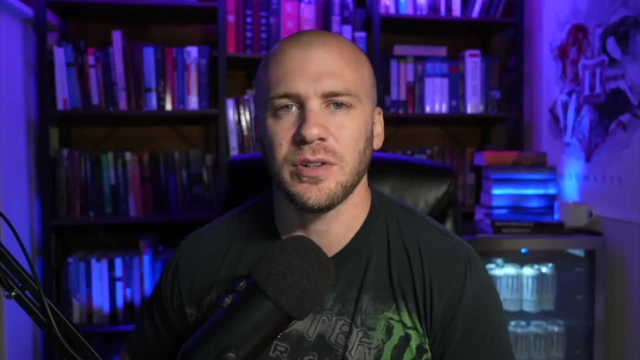 So all we have to do is next. All we have to do is next: and then stores all the information in its database. So all we have to do is next. so all we have to do is next. what queries to run? to pull the information from shodan and read their information from when they 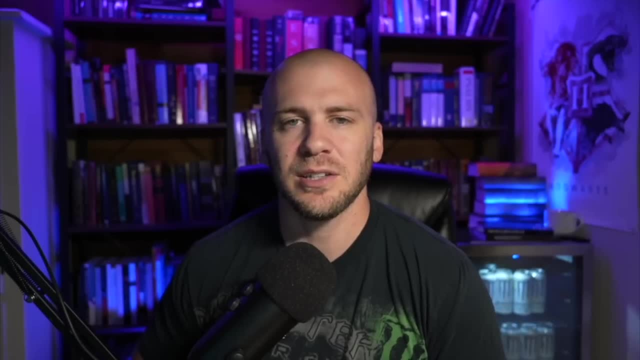 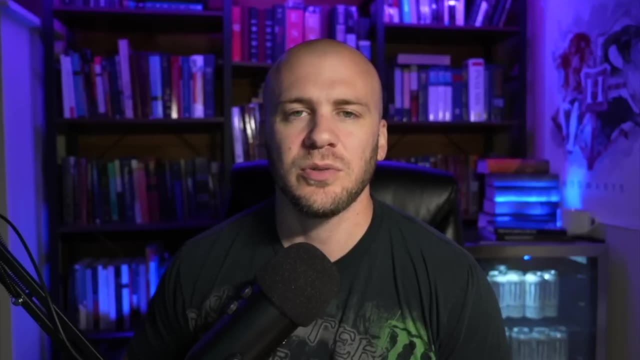 have crawled the network or the web browser previously, and then we have access to all of that information without having to scan the actual target, and you don't have to worry about breaking any program rules. so the way shodan works is actually: goes out and crawls every single device. 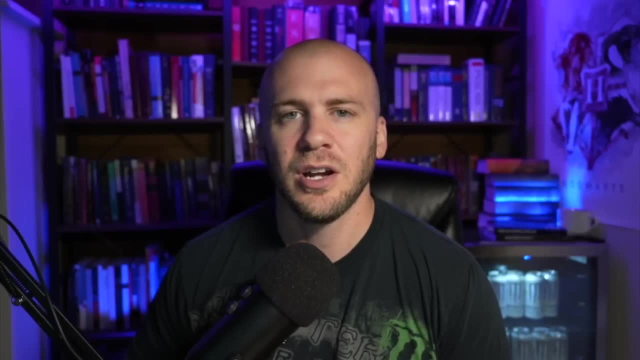 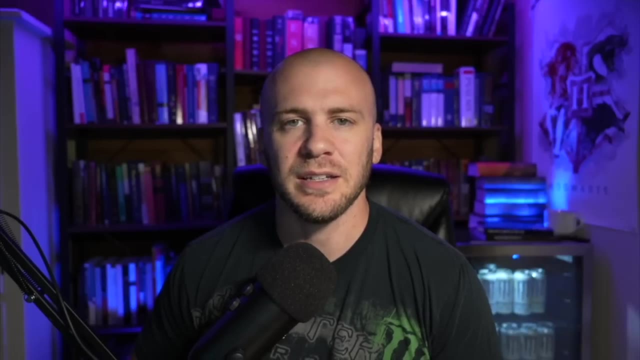 that is connected to the internet, whether it be your thermostat, your refrigerator or your web security cameras, and it'll see if there's any vulnerabilities. it'll store the information, such as the software that is currently running on it, and if it has any vulnerabilities, it is now. 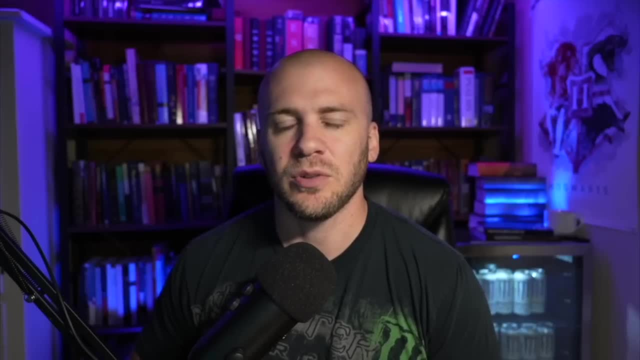 open to the web and anyone can access your information, your thermostat refrigerator, your webcam or even your printers. if they have any vulnerabilities, then the whole world will know it, because all they have to do is query that specific version, such as wordpress 1.4.7 and. 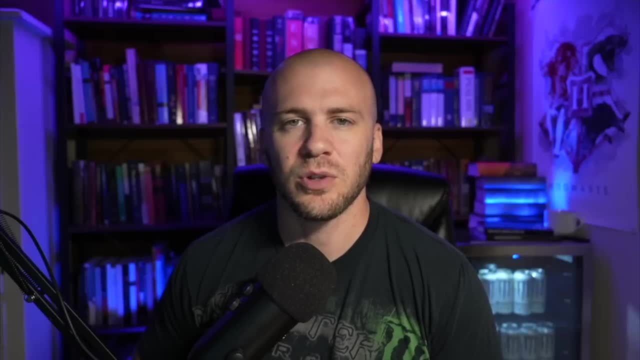 if you have a web application that is running that specific wordpress version, the whole world is going to know it because there will be a cve on it and you will be open to a potential attack. so the way shodan works is it just crawls all of the internet and stores all of the 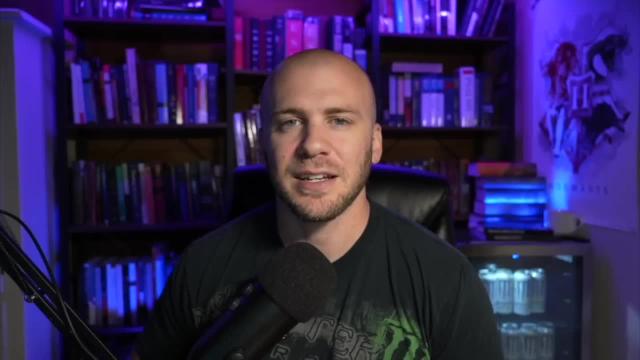 information that it can possibly grab for anything that is connected to the internet. so what we're going to do in this video is run queries on shodan, but because we're going to be doing this with a free account, you're only going to be able to run a very limited amount of commands or scans if 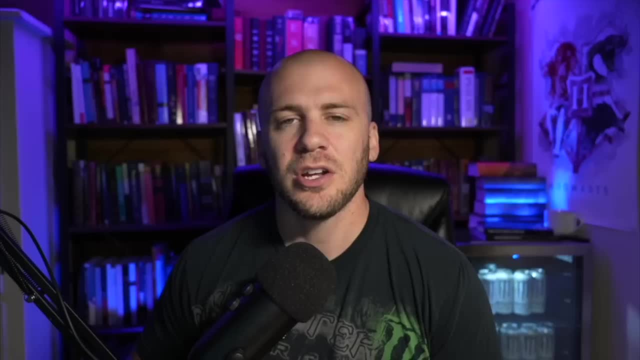 you're actually wanting to use the shodan scan feature, you're going to actually have to pay for it. i think it's 70 a month, which is kind of steep. i personally would rather just scan it myself with in-map and look at the ports i specifically want and read the information that comes back. 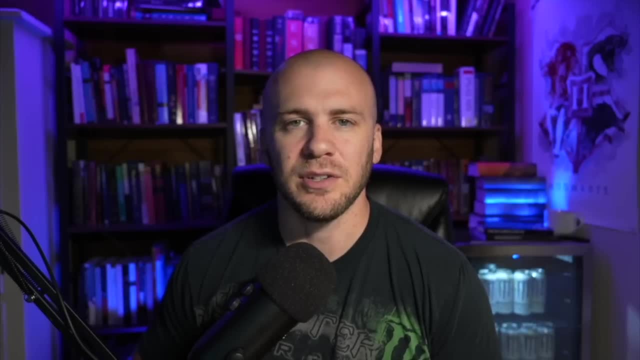 that way, but i know that some of you would probably rather just pay the 70 a month and have access to the monitoring feature that we're going to cover a little bit later on. so typically, when i think of the people who are going to enjoy shodan the most, i often think that black hat. 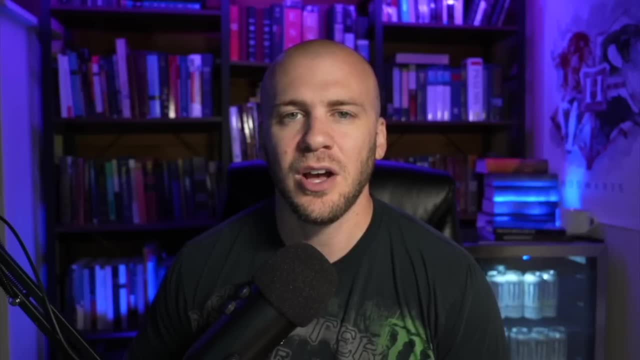 hackers are going to be the ones who love shodan the most. because it stores all the different version numbers and if a new cve comes out and somebody says, okay, we have this vulnerability to this specific software, they can just scan all of the internet and find out what devices are. 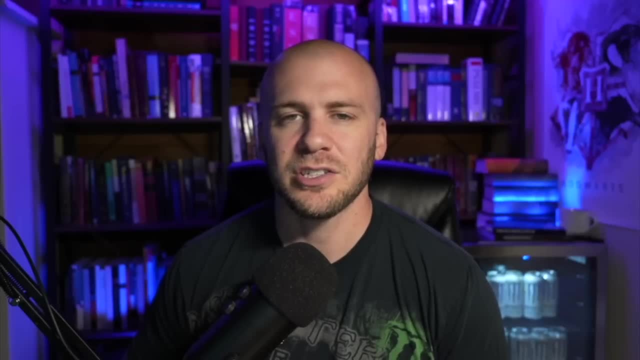 running that specific software, because black hats don't really care, they can just attack anything. but this can also be helpful for bug bounty hunters as well, because if a new cv comes out, you can go out the same way as a black hat would and say: show dan, show me all of the devices running the. 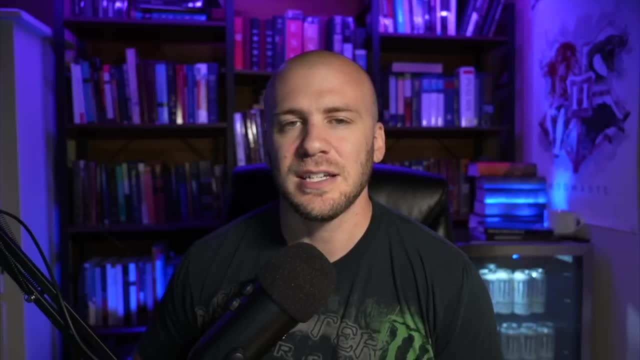 specific software that are vulnerable to this cve, and then you can download all of those devices and look through them to see if there are any web applications that are running that specific software and then see if they have a bug bounty program and report it. this is going to be kind of 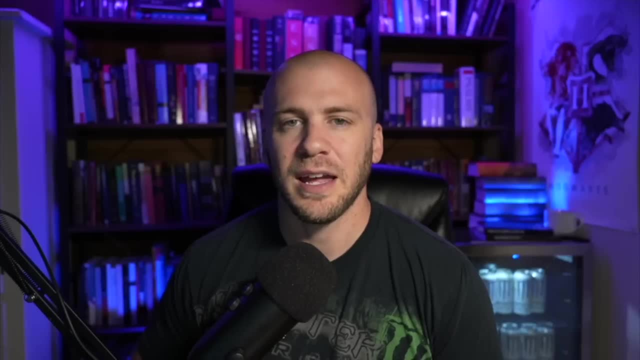 tedious, but it'll be really easy to do, bugs to find and vulnerabilities to report, because all you have to do is read the downloaded file and look for open bug bounty programs on those specific web applications. so an example of shodan being used in a really massively way, kind of for an unethical purpose, can be seen on. 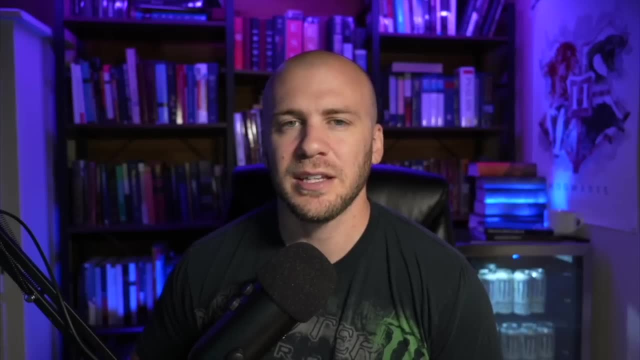 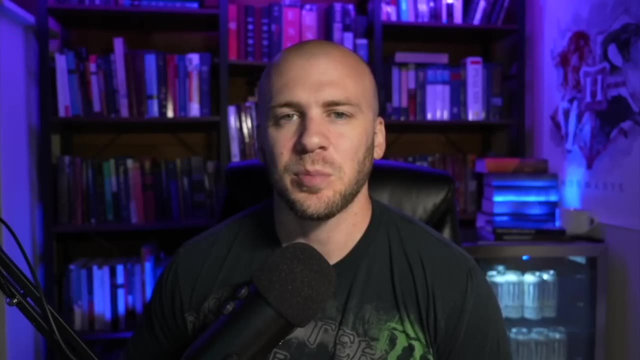 darknet diaries. i forget the name of the specific episode. i think it came out a couple months ago and the guy goes by the hacker giraffe, where he actually used shodan to look for vulnerable printers and he printed subscribe to pewdiepie to over 50 000 different printers. he was able to do. 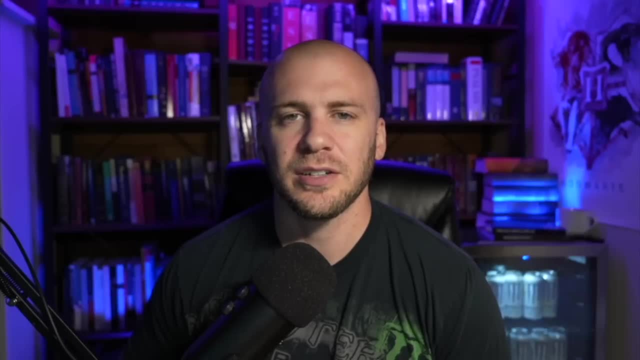 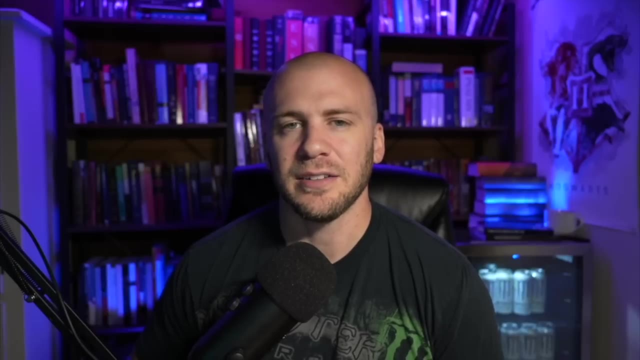 easily and really quickly, because he was able to just use shodan to look for vulnerable printers. and so in that episode of darknet diaries- i think you can just look up darknet diaries, hacker giraffe and listen to it if you want- all that guy did specifically was go to shodan and look for 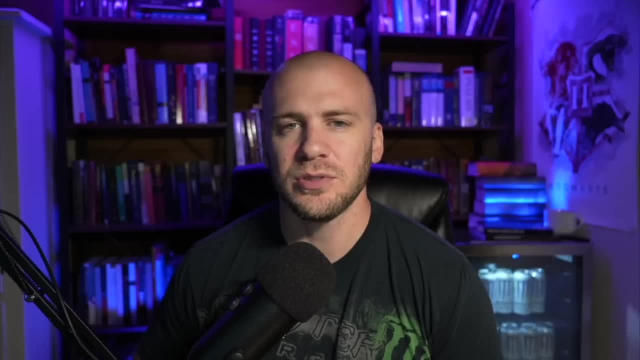 vulnerable printers and it seems like that's kind of one of his go-to tools is to go to shodan, look for some vulnerable software and then look at all of the devices that happen to be vulnerable to that specific software or cve. so let's go ahead and jump into it. here we are. i have 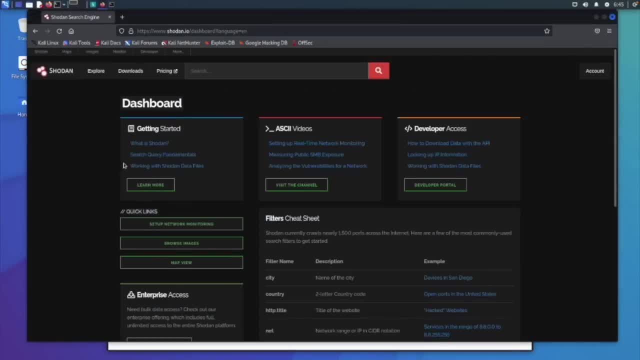 gone ahead and opened up a terminal, which you will want to do, and then you will also want to go to shodanio. i'm already logged in. you'll click login over here. i personally just log in with google, and this is a non-paid account, so we are going to be looking at basically the exact same setup that. 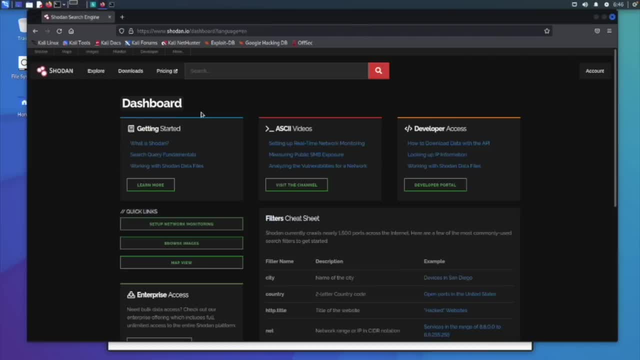 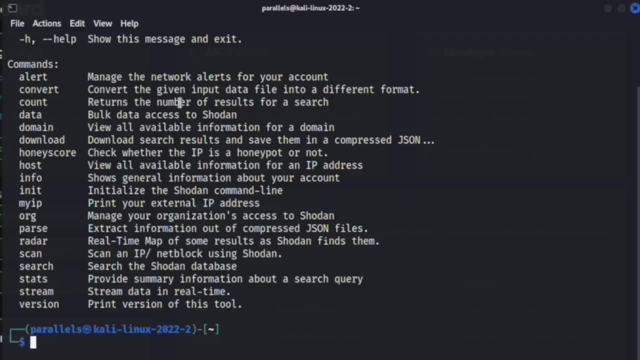 you're going to have when you first open up shodan. the first thing we're going to do is be using shodan from the terminal. so if you just come in here and type in shodan and hit enter, you're going to be able to see the list of options. now these options are going to be default and shodan should. 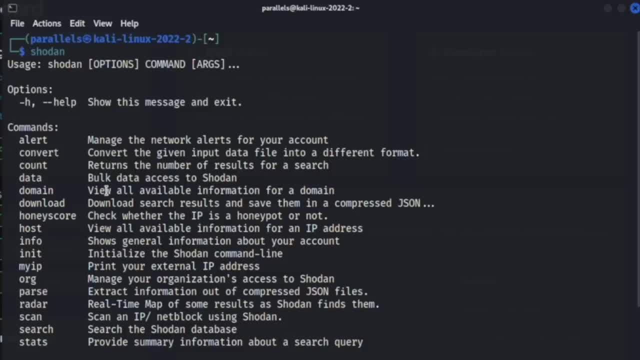 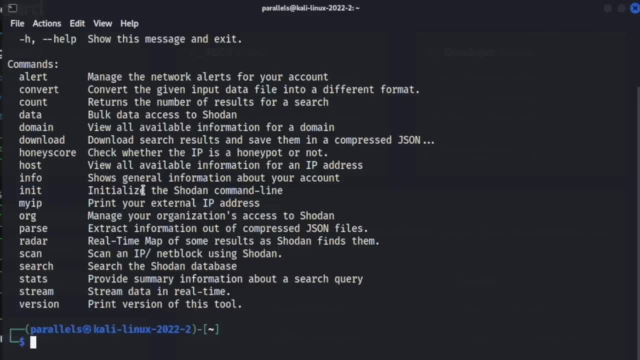 already be installed on your kali linux machine. so i'm not going to actually walk you through how to install shodan, because we're going to run it straight from here, first in the terminal, and then we'll go through and actually check out the browser version later on. i've decided to 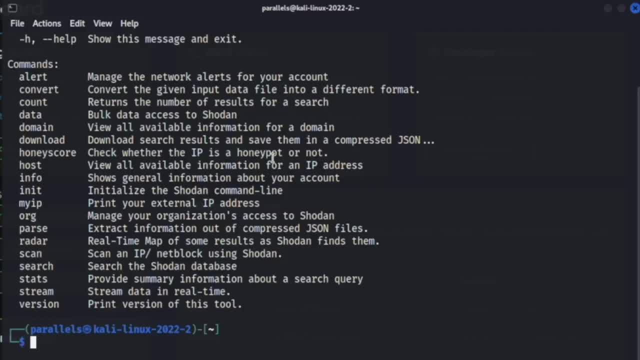 show both the terminal and the browser, because there are some people who really like running things straight from the terminal and you'll be able to play around with it and figure out exactly what you like. and then there are other people who like the graphical user interface and they'll like the browsing version better, and so what we're? 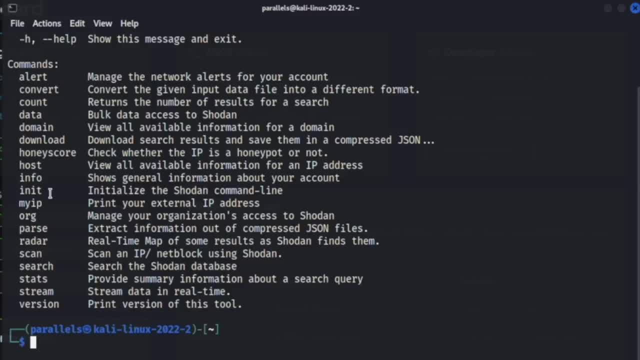 going to do is go ahead and initialize our shodan for the terminal, and you can see this right here, this init. so we're going to end up running a shodan in it, but we also need to have our api key, so you'll want to go ahead and log in. so you'll want to go ahead and create an account and log in. 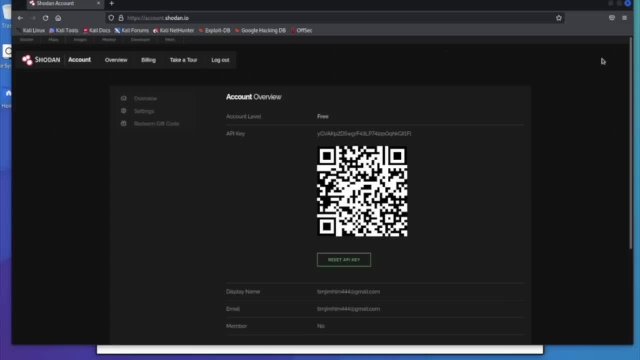 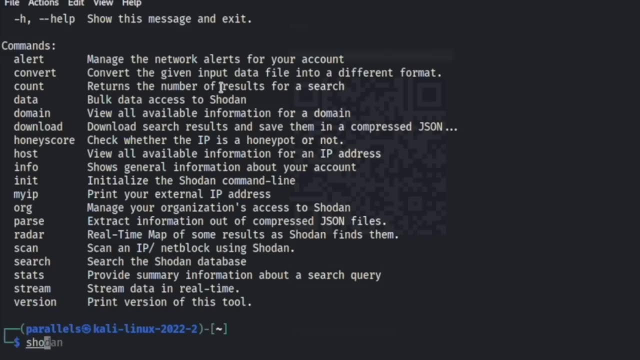 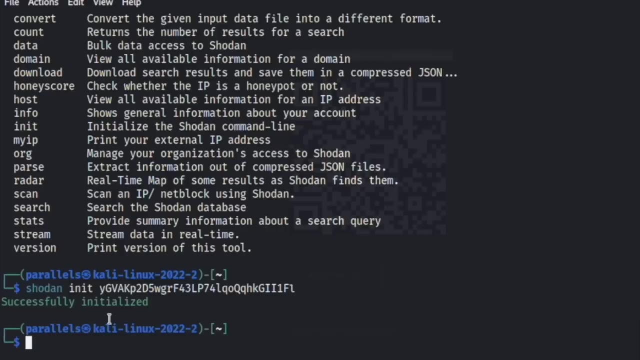 to shodan, just like this, and then you will click account and you'll be able to grab your api key right here. so we'll copy this and come back to our terminal and we're going to type in shodan init, and then you will paste in your api key and hit enter and it tells us that it has. 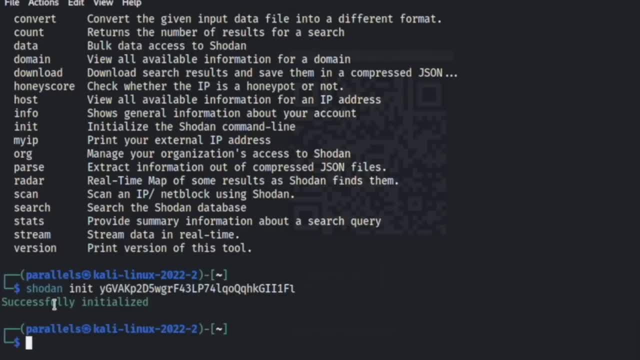 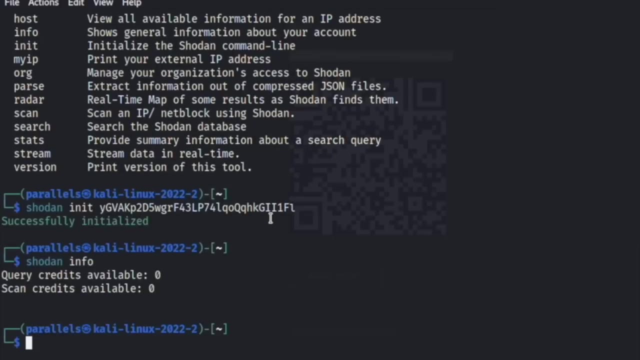 successfully initialized and now we are ready to start making some shodan queries. so the first thing we can do is just run a shodan info right here and see what it tells us about our account. so we can type in shodan info and then hit enter and it's going to tell us we have zero. 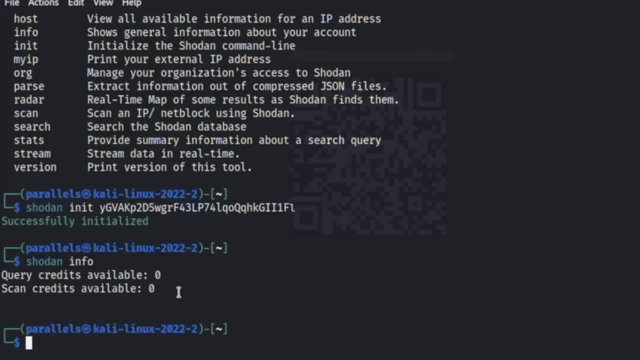 credits available and scan credits available, and that is probably because i have already ran some queries with this over here on the website, but it's not really going to make a difference. i'm going to show you how to run these queries. i just might not get the results back that you will. 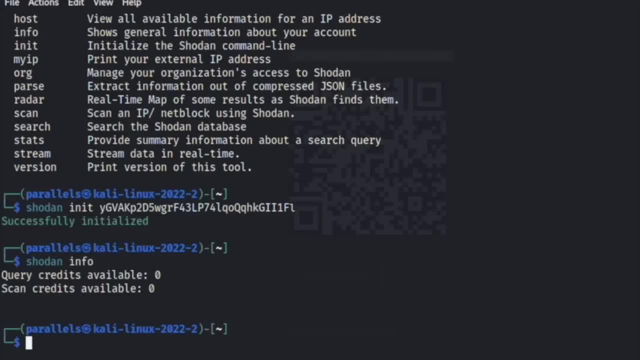 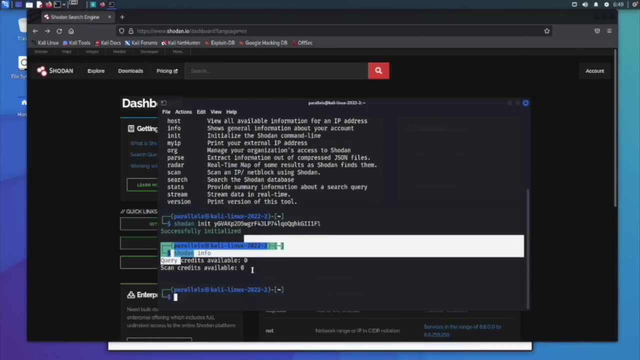 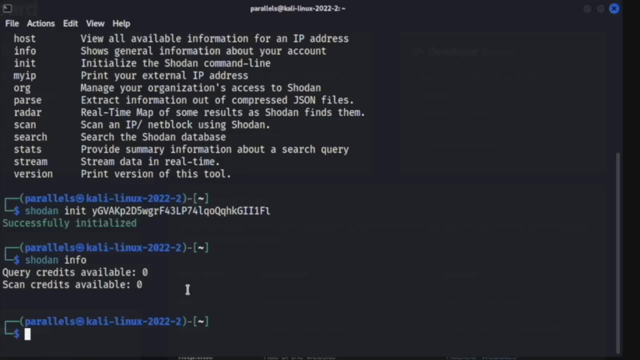 every time you make a request, whether it is over here on the actual browser or it is inside of the terminal, it is going to use one of the credits that you have, but you can always pay and subscribe to shodan and have more credits. most of the bug hunters who are successful will have a. 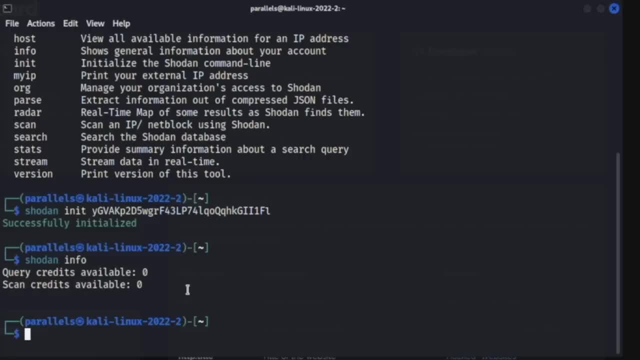 paid subscription to shodan and they really like using shodan and we're going to cover why it's helpful. but personally, a lot of the stuff you're going to be able to get on shodan, you can find your own self by running some different tools which i've covered on my channel previously. but 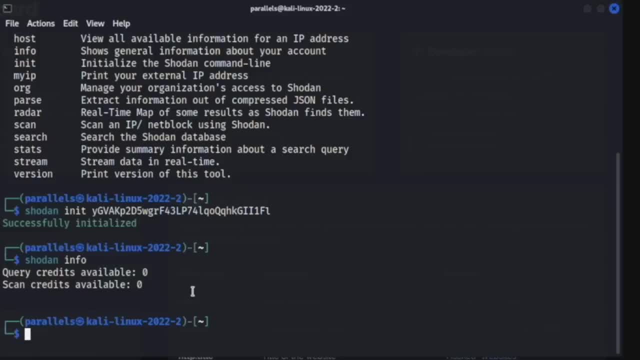 that is not the purpose of this video. so the second thing i want to show you is: often, when you want to run something like, let's say, we want to run this shodan scan right here, what we can do is we can run a shodan scan and then a dash h and it's going to tell us: 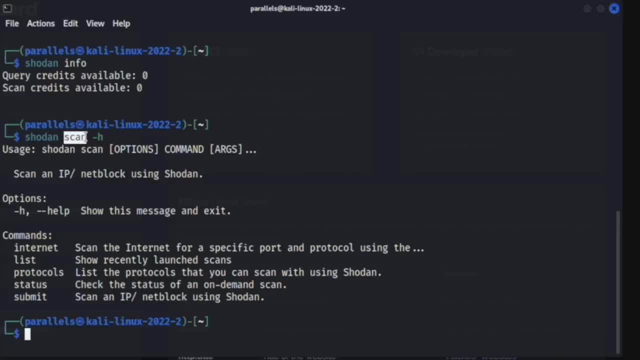 the options for the actual scan right here, so you can run a shodan dash h and then you can run the showed in scan dash h and it's going to tell you the list of commands that you can run with each one of these. with each one of these commands that comes first. so when you're using shodan, 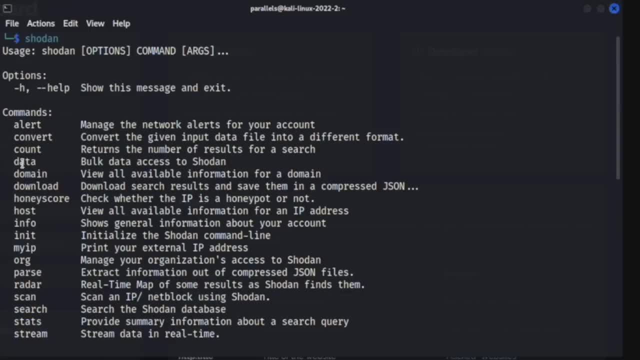 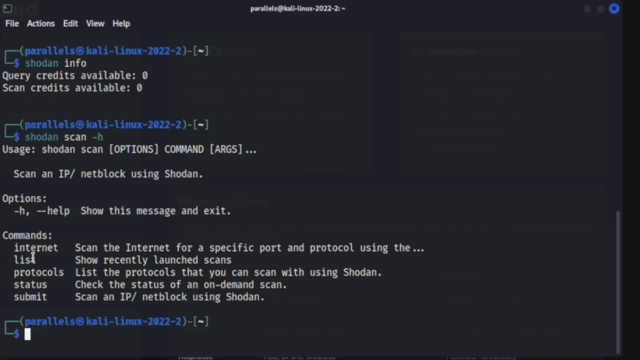 it'll be really helpful for you to know that you can run the dash h with each one of these, so that you know exactly what you're going to be getting back and how to get the information that you want in the future, and a lot of your understanding, from these. 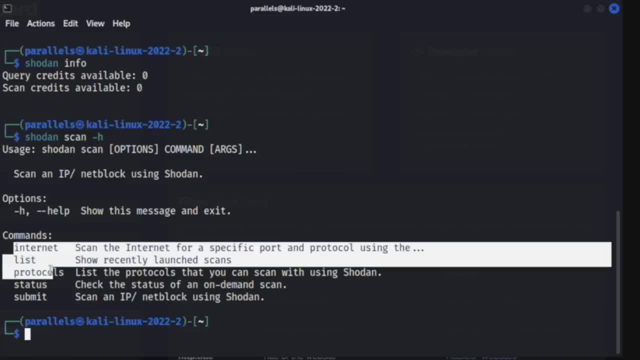 right here is going to come from playing around with them and reading the documentation and just pressing the dash h on each one of them and figuring out what exactly they do. so one of the first ways to check out shodan is we can just say shodan and then count, and then we'll say wordpress. 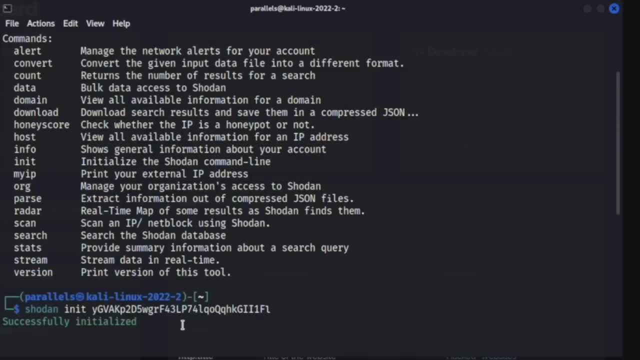 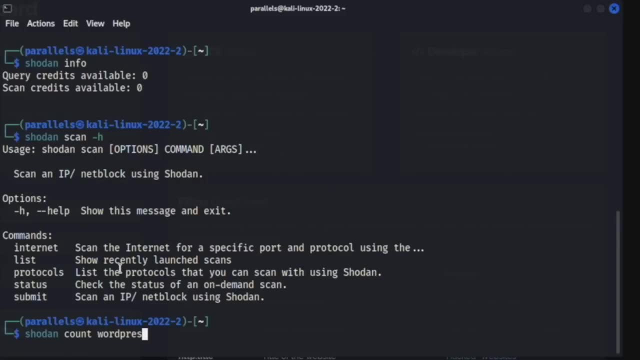 and when you run this- this might not work for me because i don't have any credits, but when you run something like this, you can see that we just want to count the number of results for this search. so what will happen is shodan will go out and count all of the servers that it has, and it's a. 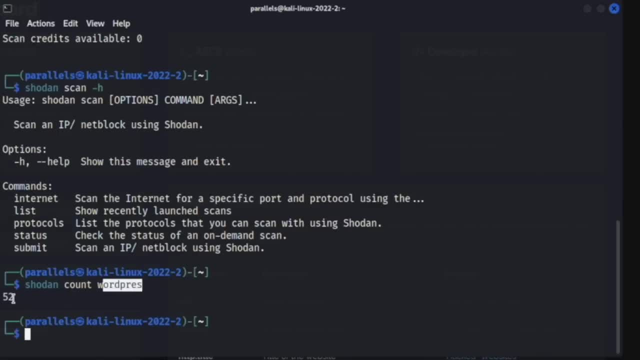 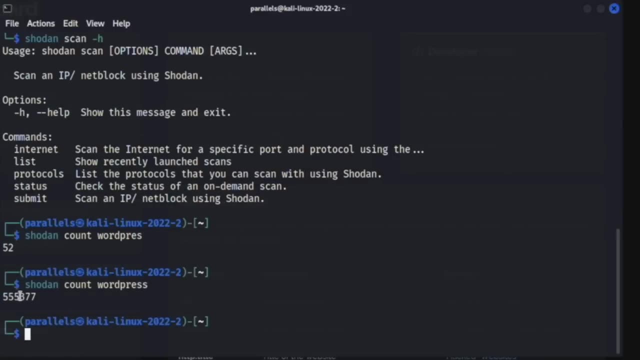 database that are running this wordpress right here and it actually did tell us. it tells us it has 52, but if you wanted to run something a little more specific, i spelled that wrong. that makes more sense. so 500 000. so if you were to run something like this, you might want to say you were looking. 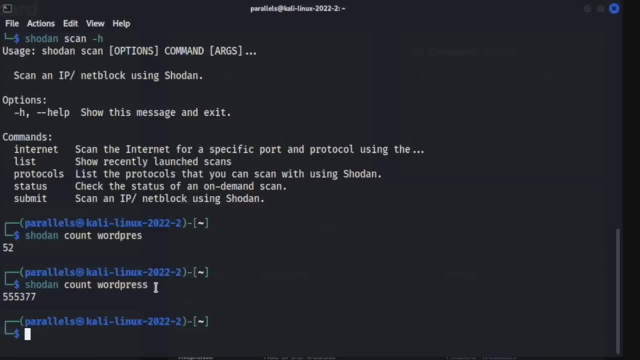 for a wordpress version 1.4.7, because that's what your target is running, or there's maybe a new cve update. so if you were to run something like this, you might want to say you're looking for a out there and you just want to see, okay, what web apps are running wordpress 1.4.7, and then you'll. 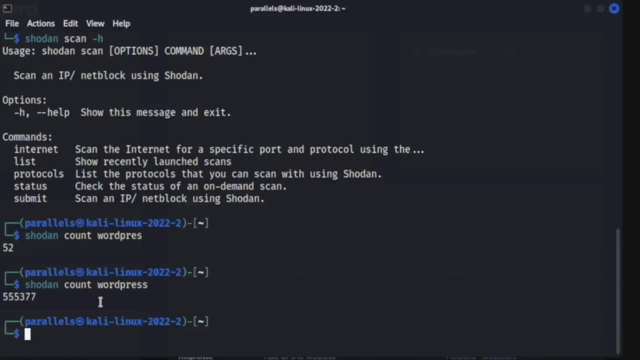 get. shodan will give you a list of those actual web apps that are running that and then you can see if any of them have a bug bounty program and then report to them. hey, this new cve for this wordpress has come out, so it saves you from having to go out and actually find a specific target and 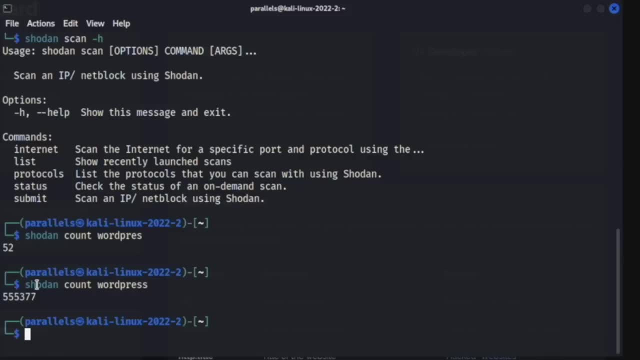 then looking to see what it is running, because shodan will actually do the heavy lifting for you, and so all you have to do, if you are a bug bounty hunter, is say: this is the version. a brand new cve has come out for it, so you'd say shodan 1.4.7, which i actually don't even know if this is a real version. 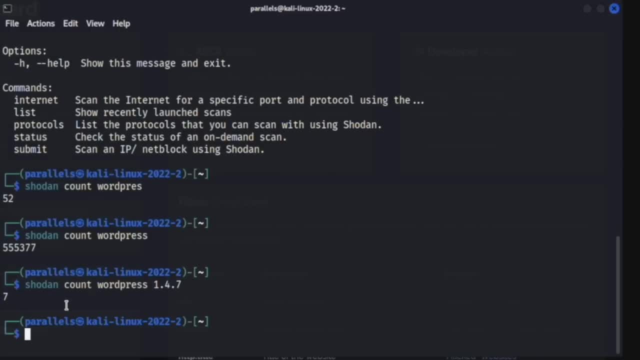 you would run this and it is, and you would say, okay, there's seven web apps that are running this version currently in the shodan database. and then you would just go out and look to see if any of these seven have a bug bounty program and if they do, you can report. hey, the cve came out and you're. 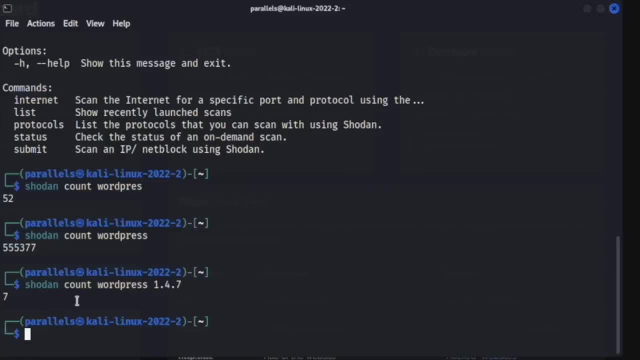 vulnerable to it, and so that's a really good way to run it. so if you're a bug bounty hunter and you're really crazy about this, you're gonna be rollin it hard. we're gonna use a really, really simple way to find bugs and it's all based on recon and you really don't have to do any heavy lifting very. 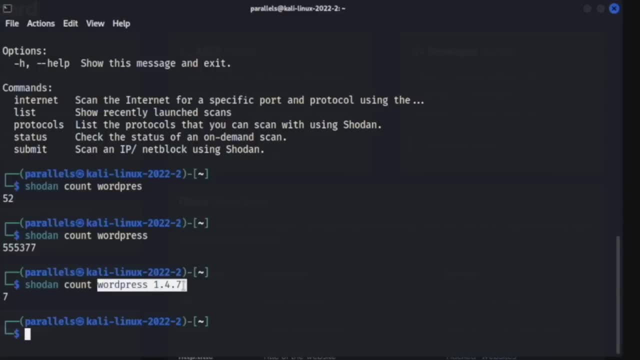 simple. you've seen how fast this has gone and you could potentially have found a bug if this version were vulnerable to a cve that had just come out. so if you're familiar with in-map, what shodan does is pretty similar. it goes out, scans the network and it brawls all of the internet and pulls the. 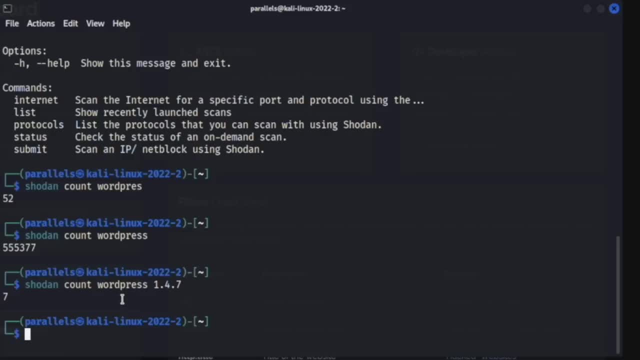 banners, the versions, what's running if it's apache, if it's windows, if it's got wordpress running, and with Shodan we can just query all of this and it stores this in the database and that's how it already knows that there is seven web apps running this WordPress 1.4.7, because it is already all it. 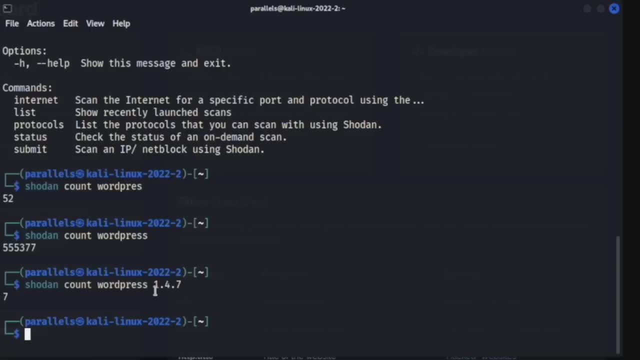 has to do is check its database, and it doesn't actually have to go out and scan, but showed. but we can scan with Shodan and we're going to look at this in a little bit. but I just want you to know how Shodan works, and it already has stored all of this information on there, so now you can see how. 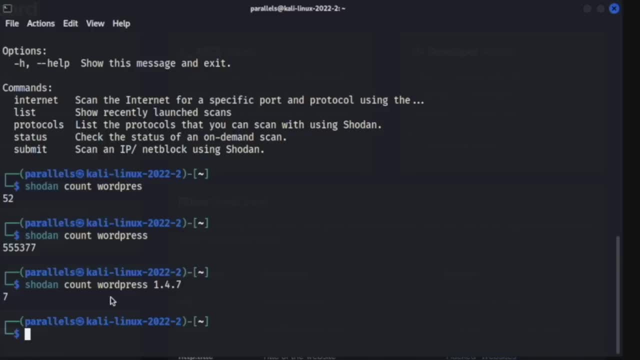 this is kind of a go-to tool for the black hat hackers, because they don't really care if these seven web applications have a bug bounty program or not. they just are going to attack it and see what information they can get out, because they don't really care about following the legal rules. 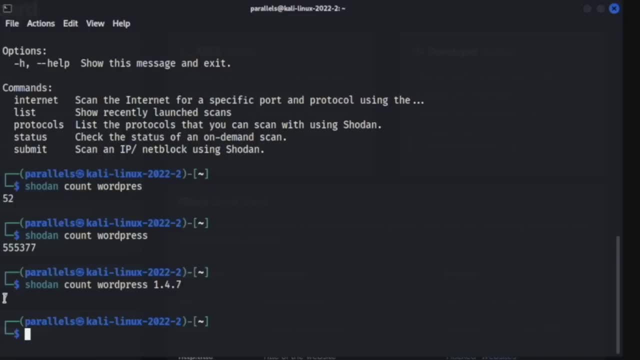 and the law, but as a bug bounty hunter, you need to make sure that these seven web apps, if they were vulnerable to a CVE that could attack WordPress 1.4.7, you would want to make sure you do everything legally. You actually don't exploit the CVE. there's no need to actually go and try and exploit it, you can just. 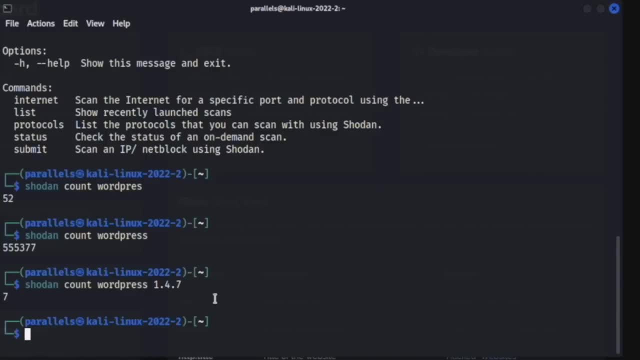 report it. hey, there's a CVE that came out and you are vulnerable and you should be rewarded for it, and so, as a bug hunter and a penetration tester, we're looking for very specific targets and then we can just run through the seven real quick and see who actually is vulnerable. so now, if we actually 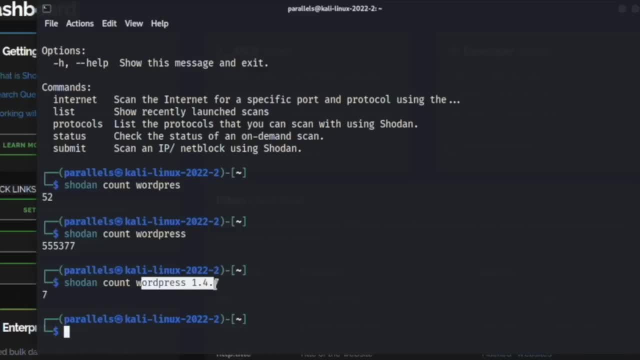 want to see what these seven web applications are that are running this WordPress right here. we can use the download feature Within Shodan. now I personally, if I was attacking a specific target, would just run in map instead of using Shodan for this. but I want you to be aware that you can actually pull down version numbers of 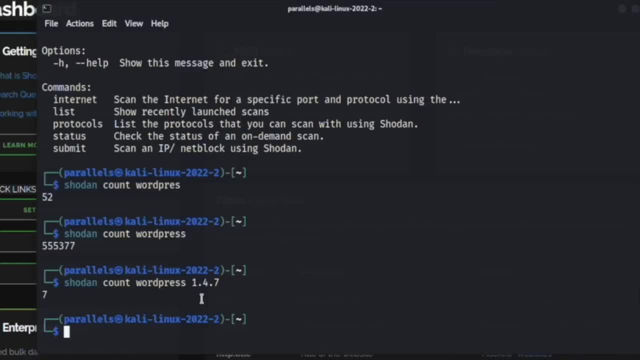 web apps with Shodan itself, but personally, I would run in map just to grab the banners in the version of a specific target. this is something that you would be using if you were just looking for a CVE that just came out, like we were previously talking about, and we would use the download function for 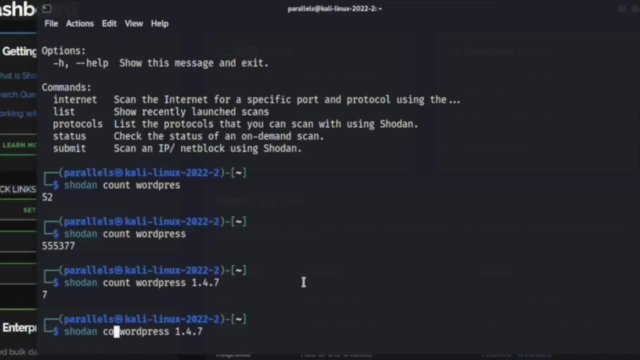 this. so we would just grab Shodan and then we would say download, and then we're going to download the file as, let's say, WordPress file, and I'm not actually sure if it will work with this version number. I've only ever ran it without the version number, so maybe we can throw this inside of quotes and see if this works. 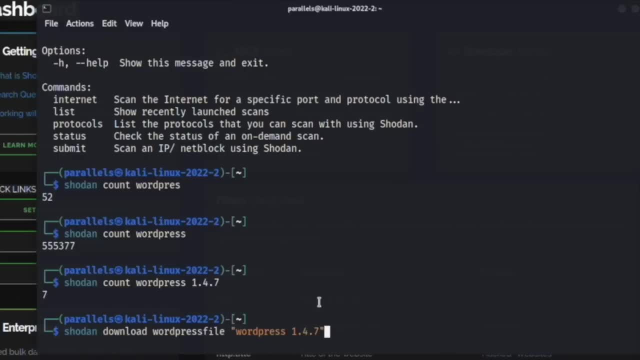 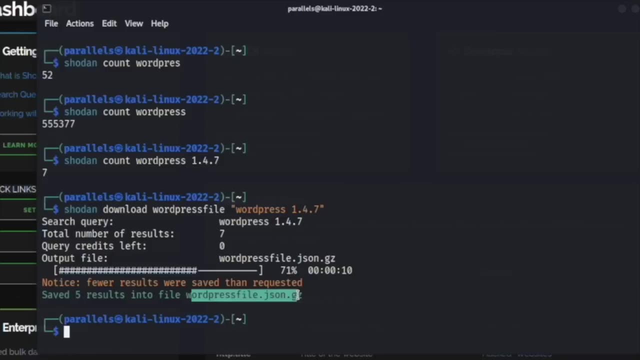 if not, we will just run it without quotes and see how that runs. so we'll run this and it has saved five results into Our WordPress JSON file, dot GZ, and we can unzip this and grab the file by typing in G- unzip. and then we want to run our. 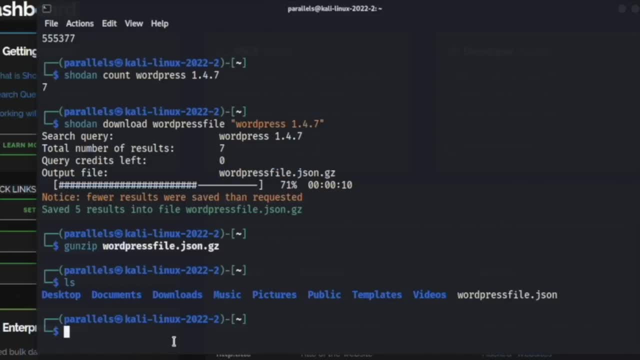 WordPress file and then, if we LS, we should have our WordPress file dot JSON. and I do not have G edit installed, because this is a new machine. and if you don't have G edit installed either, you can sudo apt update and I've already done a sudo apt update recently, so I'm going to sudo apt. 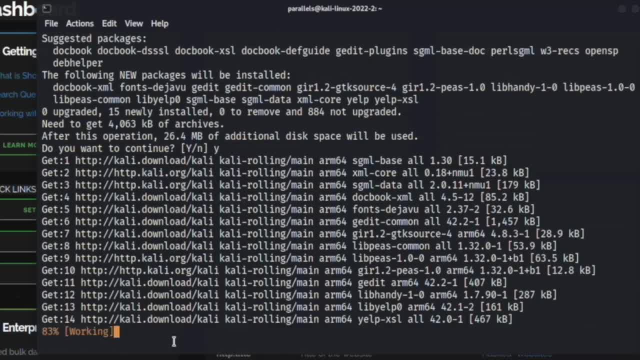 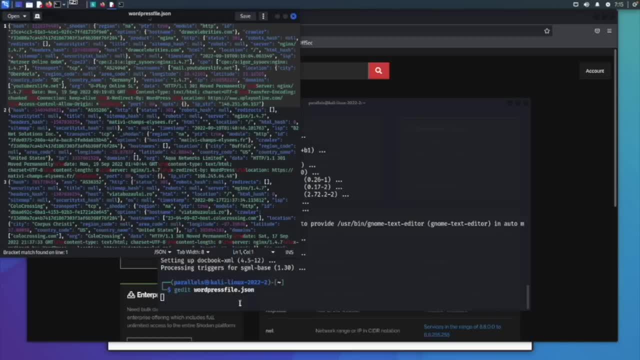 Install G edit and this will only take a second to download. and now we can G edit our WordPress file right here and we can look at the contents. and this looks really messy. so what you can do is actually just copy this: hit a command a and a command C, and then we can come over here and we can just type in: be a. 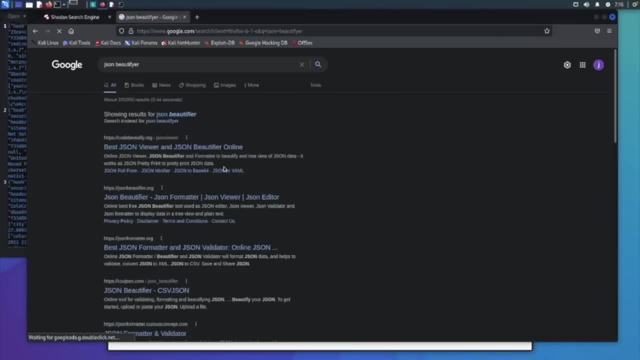 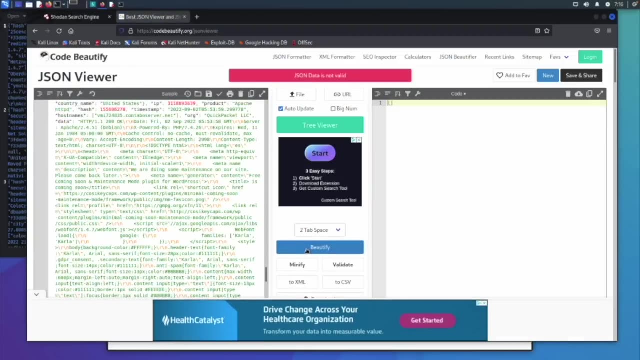 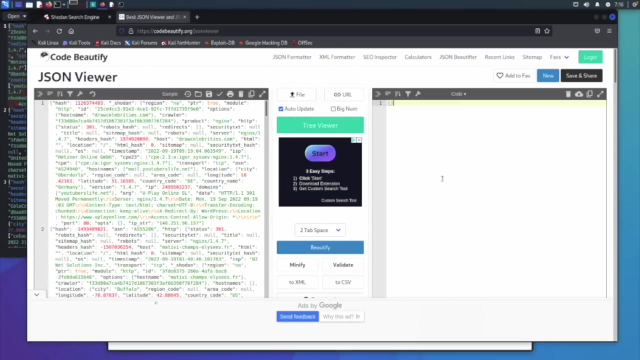 you to fire like this And we can just click on the top one and see if it will work for us. paste in the JSON For us type: you can click beautify and now we have our results right here. so it actually looks the same over here. it actually didn't make any difference, so maybe this one doesn't work for us. 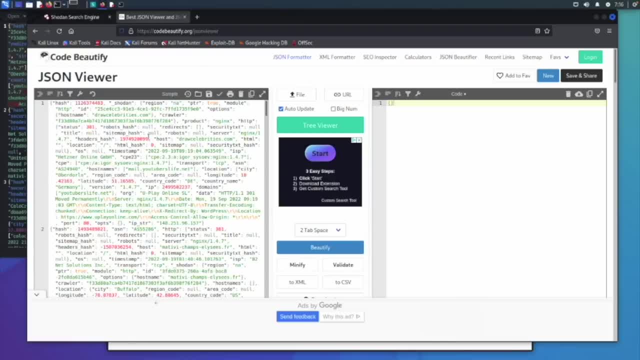 It tells us we have an error. okay, we're going to just look at it right here so you can actually see right here you get a hash you are told it's from Showed in. it'll tell you the region from where the web app was coming, where the web app is coming from. 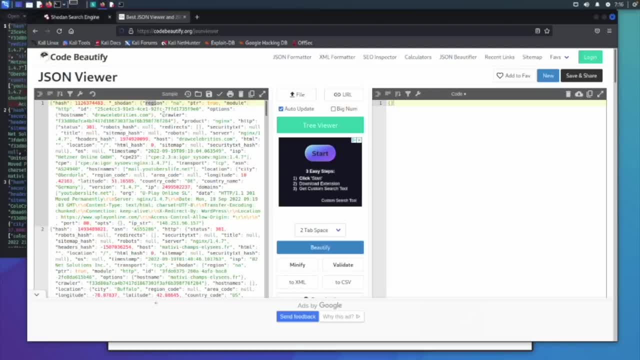 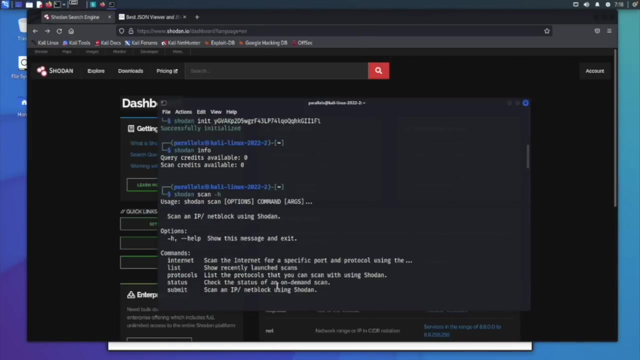 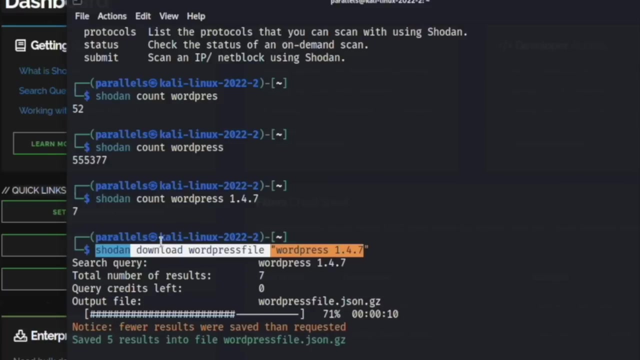 It's going to give us the Time Time Time that it was crawled. we get the server that it is running on and we have all of this different information here that it that showed in has crawled. from this specific target. we actually grab an ASN number if you were looking for a specific target and you needed to, and you needed to pull down a version, and you were looking for a specific CVE and you wanted to download so you could actually see what the show. Dan databases. 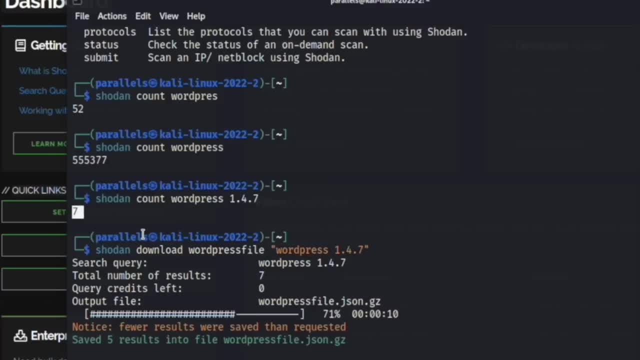 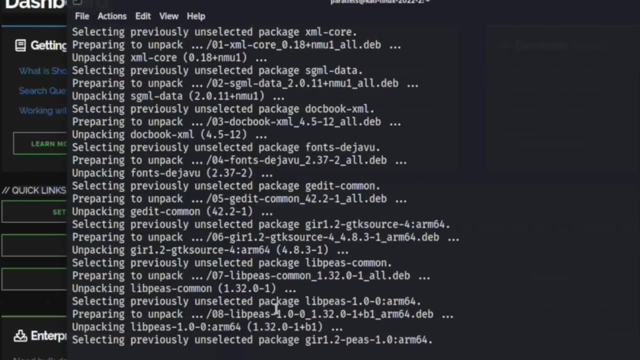 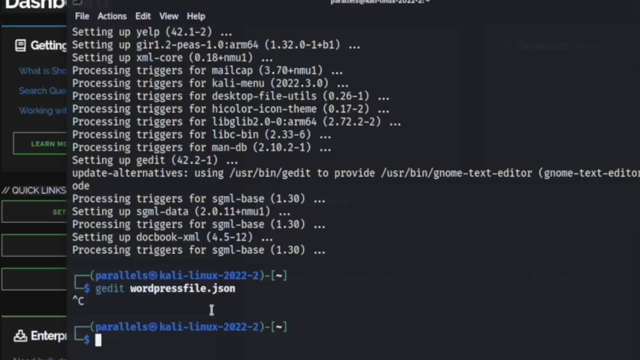 Have stored for the word. press one, point four, point seven, instead of just seeing all the seven of them, you would download it into a file just like this right here, And then you would unzip it and then you can get it and actually look at the contents of the file and find the servers and the subdomains, the URLs, the AS numbers, and there's a lot of information in there that's going to be really helpful for you in your 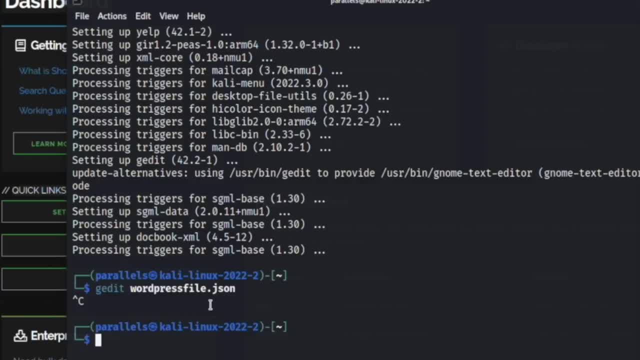 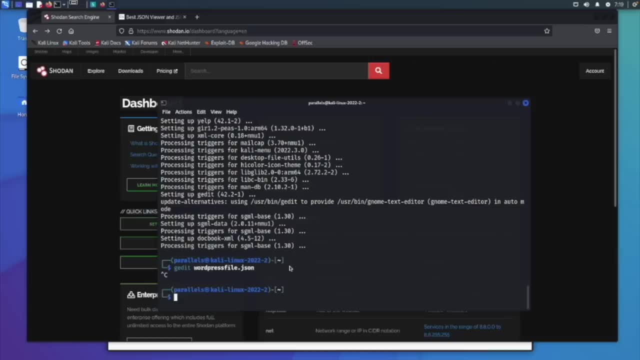 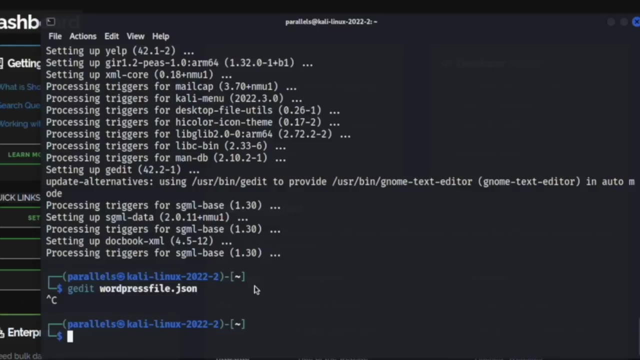 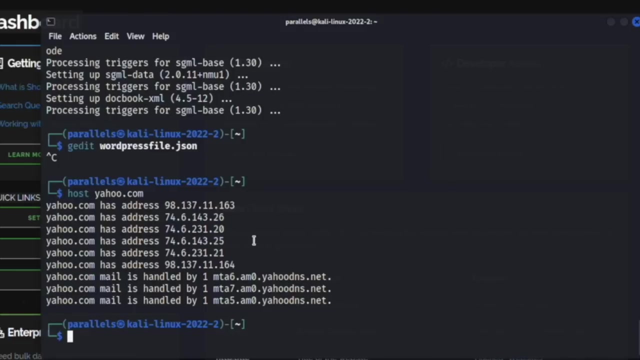 Recon phase if these targets are actually vulnerable and they do have a bug bounty program. so one of the other things You're able to do with- showed in is run a- is to run an IP address on the show Dan crawlers, and so you're in one of the ways to grab an IP address. so one of the ways you're gonna be able to find the IP address. there's several different ways that are gonna be really easy. so if we wanted to run to say, a host, yahoo dot com, it's going to give us back right here this range of IP addresses that are running on yahoo dot com. and if you wanted to just ping yahoo dot com, 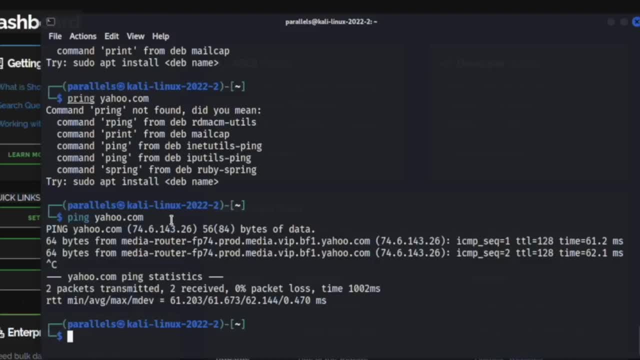 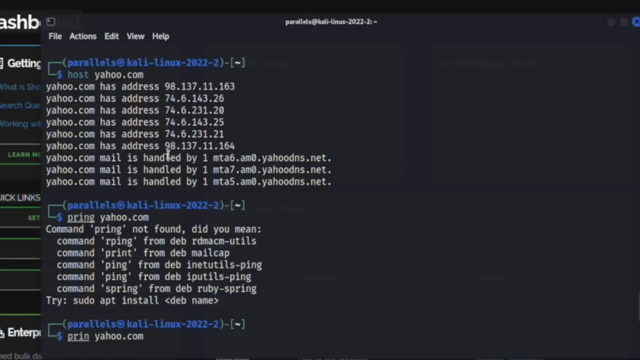 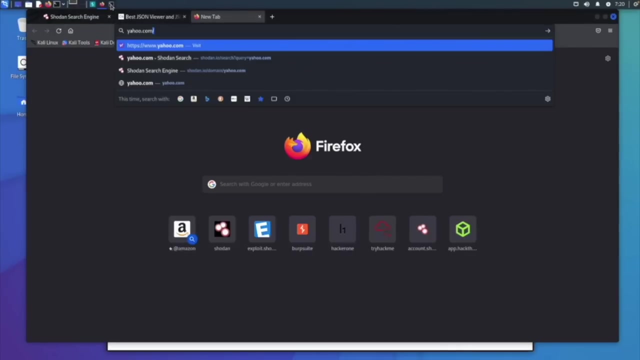 And if you wanted to just ping yahoo dot com. And if you wanted to just ping yahoo dot com, we will be told: right here is one of the IP addresses that we were able to ping. so if you look for this seven, four point one, four, three, two, six- we can scroll up and see that this is one of the IP addresses right here. you're actually able to find IP addresses through a burp as well. so what we can do is come over here and open up a new tab, type in yahoo dot com, and we can open up burp and 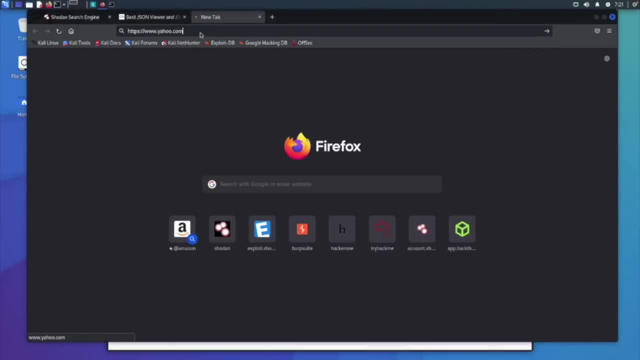 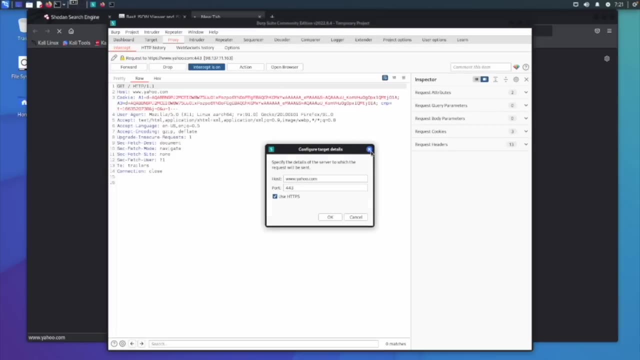 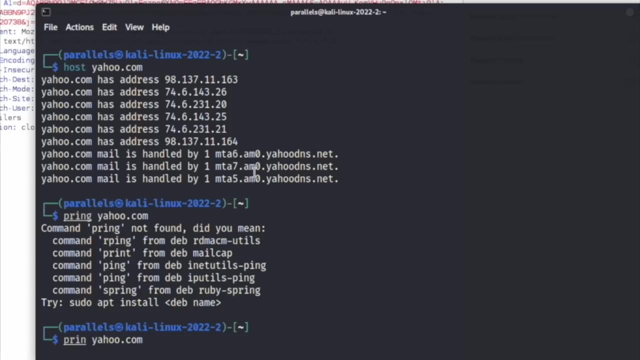 And if we run this, you'll actually be able to see right here on four, four, three. you have this nine, eight, three, seven, one, one, one, six, three, and if you come back here you should be able to find right here. and so there's a several different ways to find IP addresses for a specific domain. I'm actually going to close out this, but this is one way to do that, and then you can just type in a show, Dan, and then we would type in host, and then we can grab one of the IP addresses that are running on yahoo dot com. 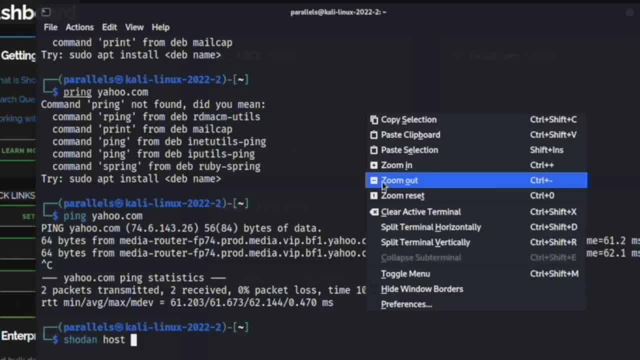 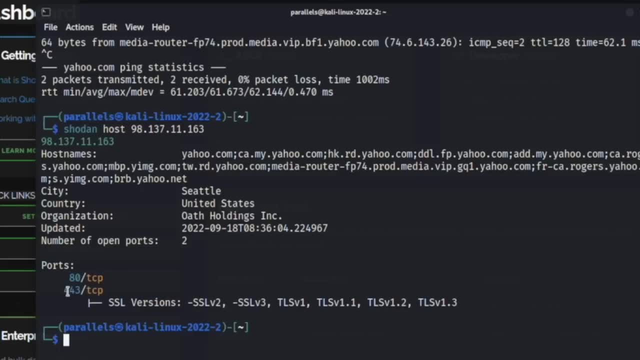 These IP addresses that we just saw and run it within showed in and it's going to give us some information right here. it's going to tell us that this port 80 is open and port four, four, three is open, and it'll give us other information. if you specifically want to look for an SSL certification, you can find those and it's going to tell us it's running these different versions and you can go check to see if these SSL versions are out of date or what you can do with these within your recon phase. you also get 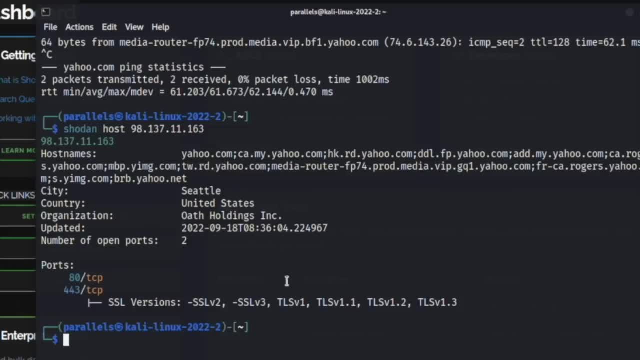 These other host names right here that can be associated with IP ranges, and you can run a show Dan host with an IP range and it's going to pull down a bunch more information for you within the entire range. it'll give you all of the ports that are open within with the IPs. and so the difference here between what we're able to find between Google and showed in is Google goes out and crawls the pages to see what is reachable, but showed in crawls all of the internet connected devices, and this is why you would find 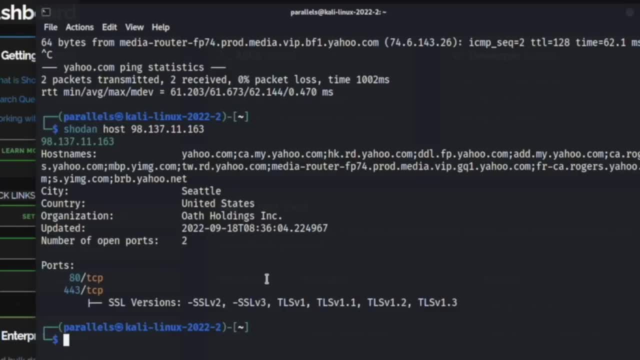 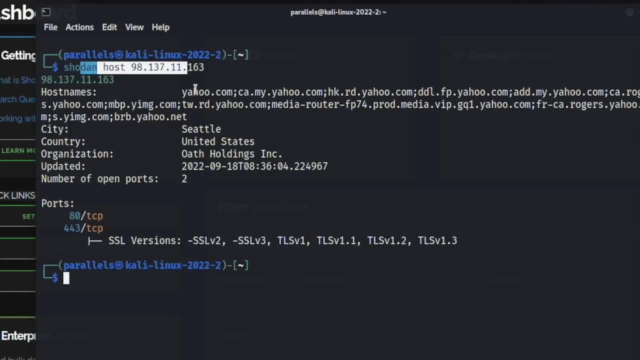 A refrigerator that might be connected, or a webcam, or somebody's property cameras or literally anything that is connected to the internet like a thermostat and showed in actually crawls everything that is connected to the internet and stores the data. so one of the good things about running a show, Dan, like this is sometimes you are going to come across a bug bounty programs. they're going to tell you that you are not allowed to scan a specific network and, as new bug bounty hunters, I know there is a lot of questions about what 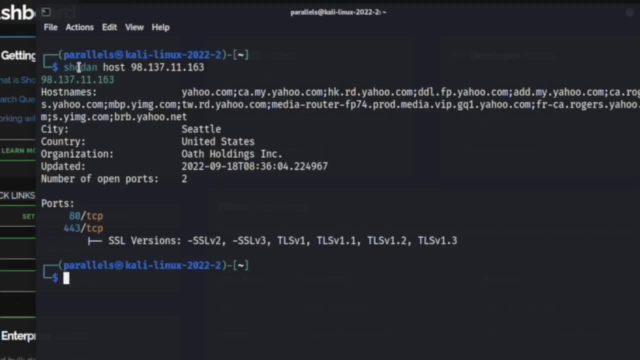 What You're allowed to do and what you're not allowed to do, and so showed in is a great way to scan a network without actually scanning a network, because showed in already has stored all the information that you're going to be looking for and you just have to go out and find it. you have to know what commands to give, such as this one right here. if you're looking for open ports, I personally would rather just run in map with the ports that I want to find, such as port 22, port 80, 443, 1443, 3389 or whatever other ports you might. 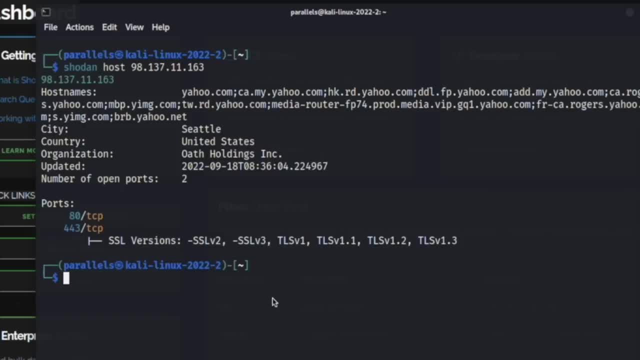 come across, but I would rather run in map with specific ports. but I know there are some people who really worry about this and showed in is a great option, such as this showed in host right here to grab other domains. you can grab subdomains and you can scan for ports and IP ranges, and so this is an option if you're worried about scanning a target in order to grab subdomains and open ports. and what I like to use for running subdomains is a mass and I'll go ahead and link my a mass video in the description if you would like to look. 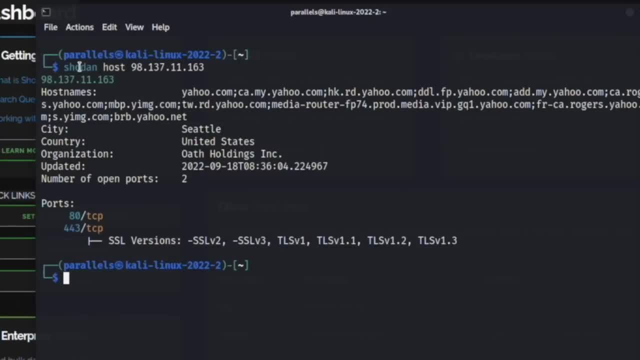 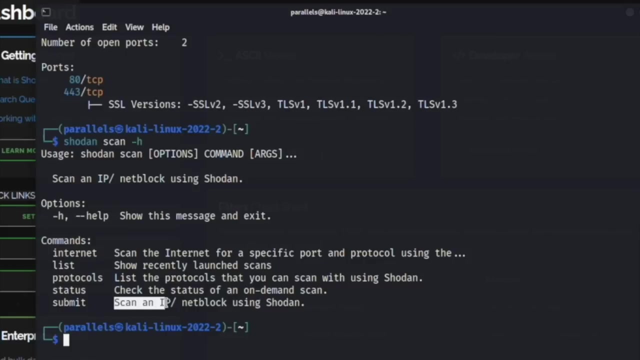 more about that. so let's go ahead and look at scanning a host instead of just looking at this right here. the showed in host. so with showed in you can actually just type in showed in will go scan dash H and we can look to see what our options are for scanning a IP. and so it tells us right here we can scan an IP and we can say showed in scan and then we can give it the IP that we want and we'll just run this same IP address right here and see what information. 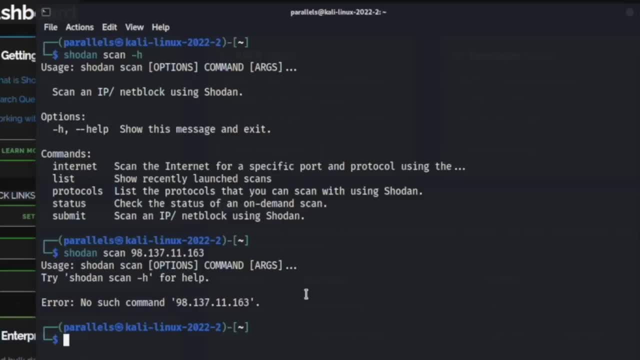 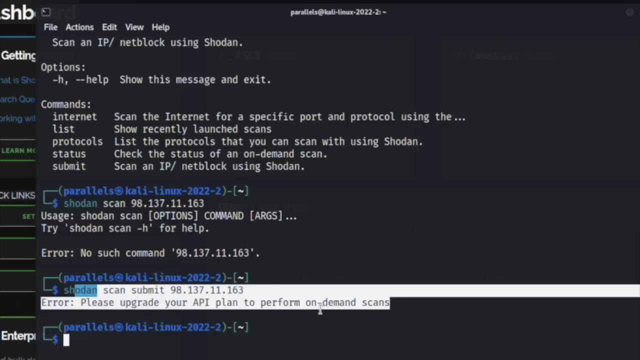 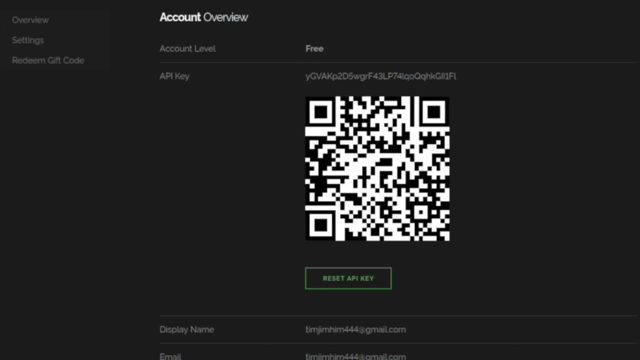 it gives back to us. it tells us we need to give it a command so we can say: submit right here, because we're going to submit an IP address. it tells us that I don't have any credits to actually run this scan submit. so I would need to actually go and pay in order to get my my API key right here- some credits, but I am not going to do that. so this is another way to go ahead and scan a network or 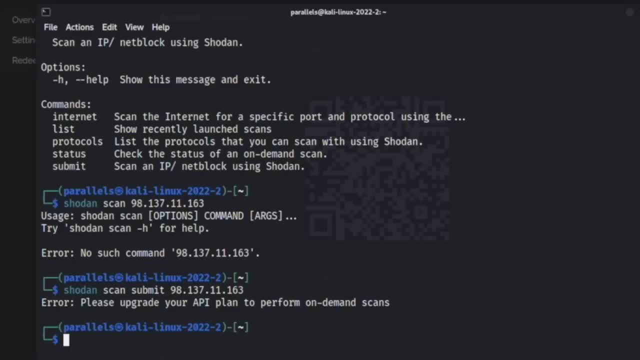 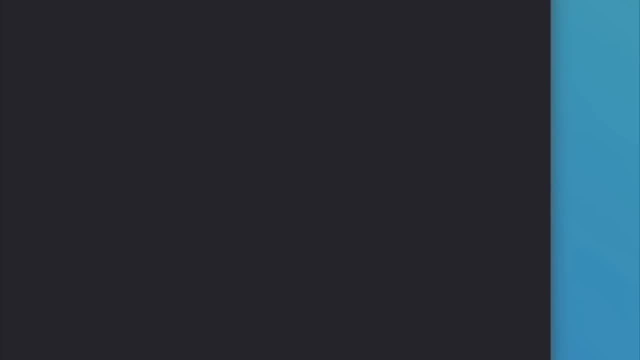 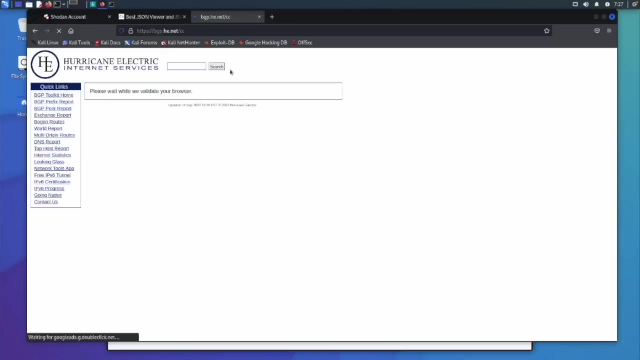 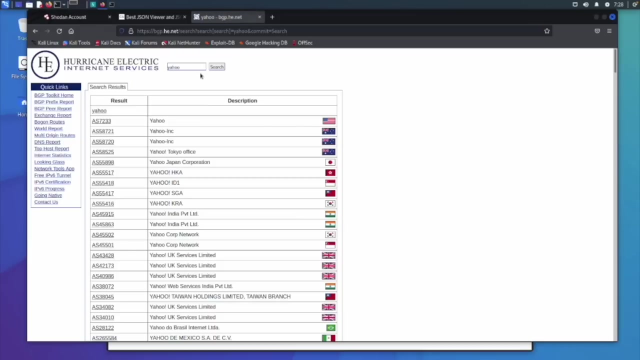 an IP address to find what is open and do a little more recon with this. you can also go out to- I can never remember what it's called hurricane electric, I think it's vgph enet. all right, so here we are. we can just type in yahoocom, and I've shown this before in another video, so we'll just go yahoo, and this website seems to be running really slow. but you would just run the search up and it has come back so you can grab these AS numbers right here, or these ASNs. 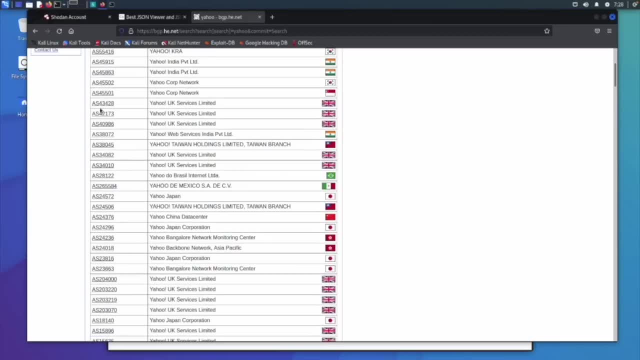 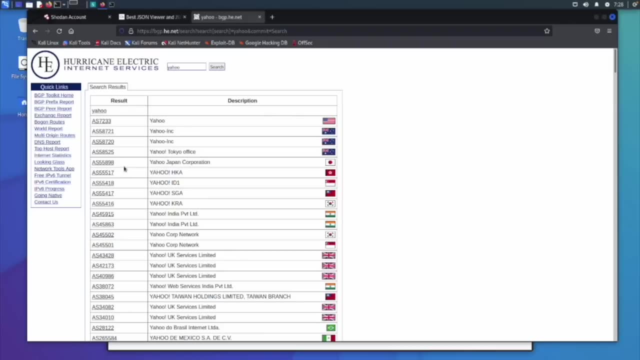 is the easier way to say it, and I would run these through amass personally because it would be easier, but you can run these through showdan as well. showdan is going to be a lot faster because all it has to do is query back to the database, whereas amass seems to take quite a bit longer in getting you the. 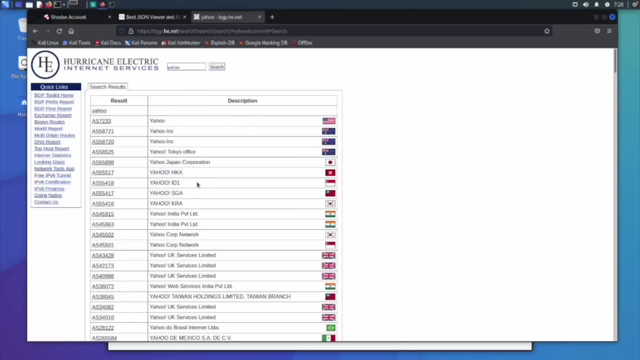 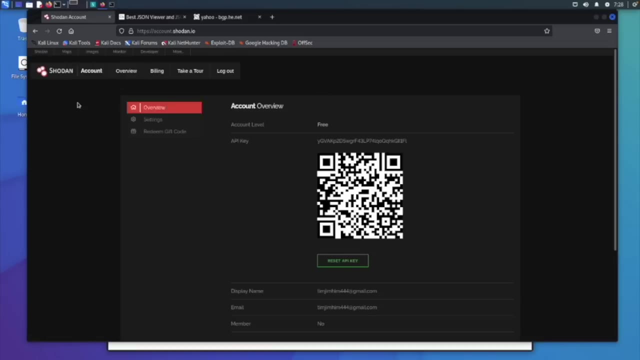 information back. but you can come out here and grab a network range, scan a network range. you can look through these ASNs and see what you can find right here. I've already made a video about that so I'm not going to go into to my much detail about that. but, like I said, I personally would go with nmap if I was going to scan any kind. 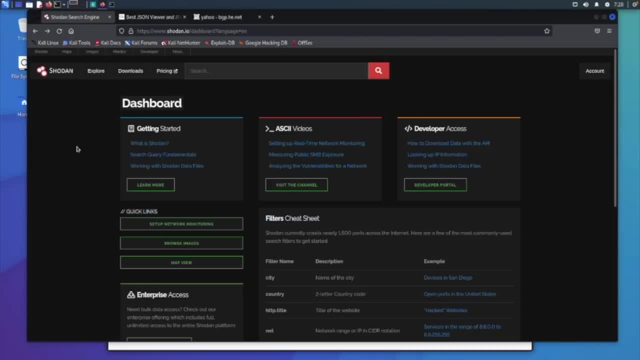 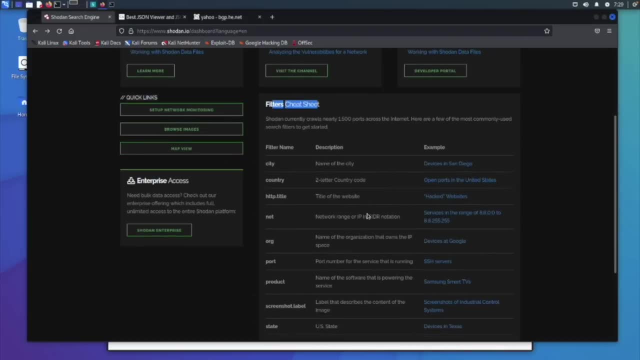 of network or anything like that. Now we're going to move on to the web browser, so what's really cool about running Shodan in the browser is they give you this filters cheat sheet, so if you wanted to look for a specific network or a range or a site arrange, you can do that right here through. 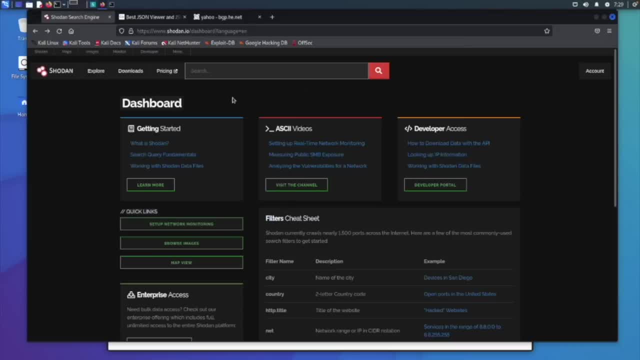 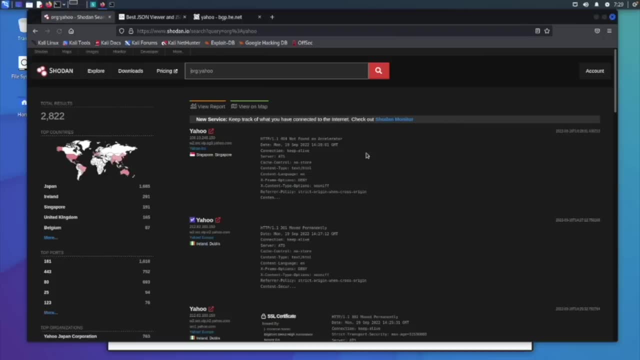 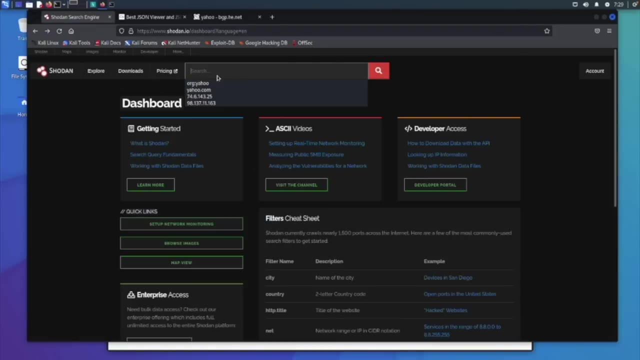 the search filter, and the way you would do these commands is by typing in, say, we wanted to find the organization yahoo, like this: we can search it and it's going to pull it down for us. Let's see what else I've ran up here. If we delete this, we can run an IP address- and we already ran this one- and it'll. 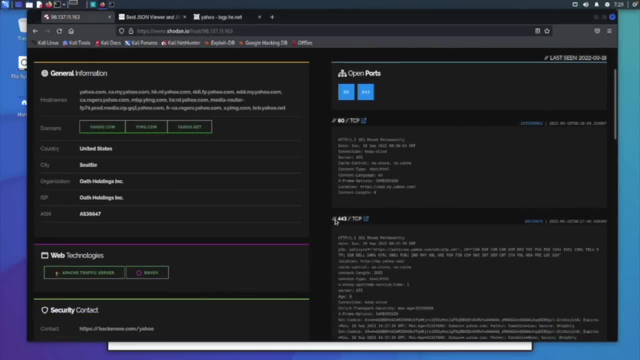 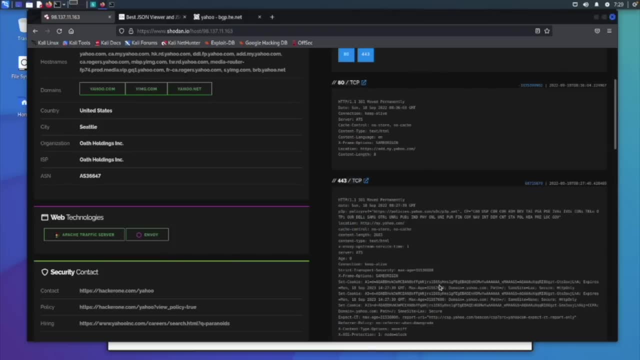 pull down the information. here's that port 80 that it said was open. here's port 443, and it has grabbed us. So we're going to take a look at all of the banners right here and we can read through them and see what is running. You can also download the reports from here as well, One of the cool things about. 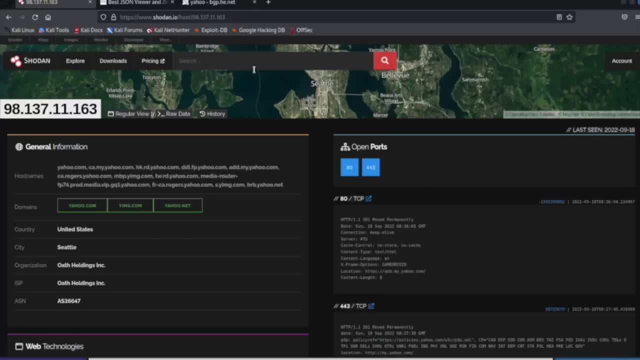 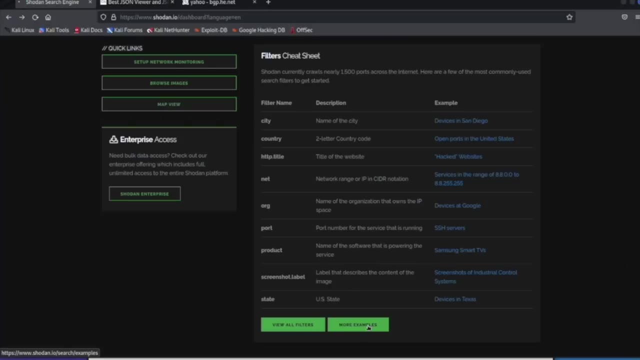 one of the cool things about running through the browser is you can actually look for sensitive information disclosures if you just continue to look through here, and you'll need to read through the cheat sheet- and I would also recommend reading through- like their documentation, because there's way more examples that you're going to be able to use. so if we want to, look for something that's running Apache. with a specific Apache version you could look to see if you're able to run. maybe there is a Apache 1.7.4 that actually has a vulnerability. you can come up here and you can just type in the product Apache with the version number and see if you're able to find any vulnerabilities for that Apache version, just like this. and you would run through here and say, okay, these people might be vulnerable to this. do they have a bug bounty program? 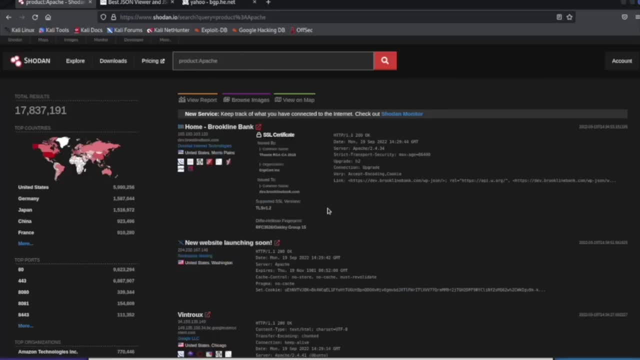 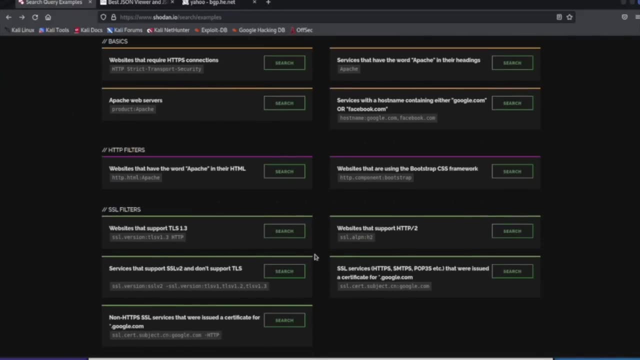 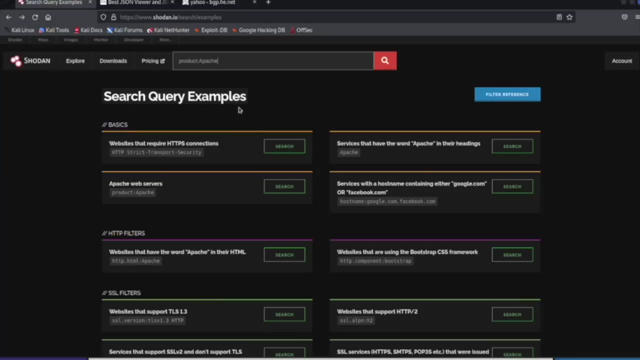 Okay, these people are running this version, do they have a bug bounty program? and so there's a lot of different ways. you can be creative with looking for known vulnerabilities, new CVEs, looking for bug bounty programs that are vulnerable, and then you can look for sensitive information with Shodan, because it doesn't know what is going to be sensitive or not. it's just going to grab all of the information and store it in the database and it's up to you, as the bug bounty hunter, to look at that specific target and see if there's any sensitive information that's going to be sensitive or not. 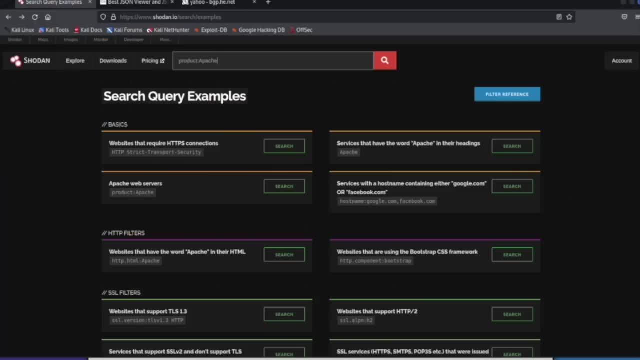 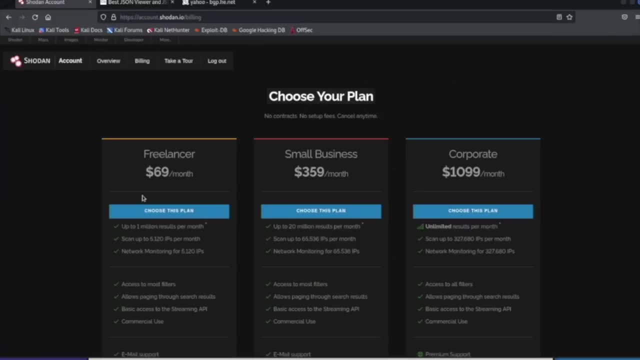 So you can look for sensitive information being disclosed on Shodan and then you can report it. okay, and one of the last things I want to cover is the monitor function, and you have to have an account in order to use this, but this is something that you might be interested in. the monitoring is you can enter in a specific target, such as yahoocom, and it will update you whenever a new software comes out or whenever there's an update made to the program that you are trying to monitor. it'll let you know and you can be one of the first ones to go and check out. 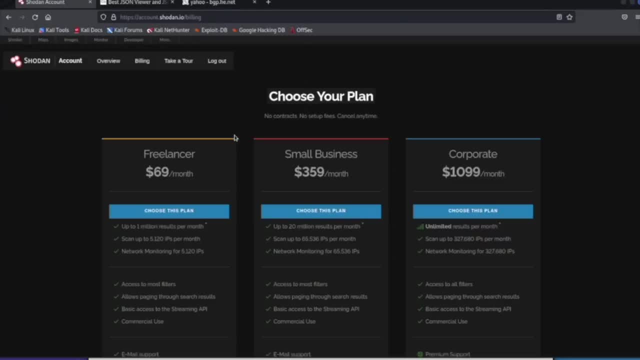 that new subdomain or domain, if it is in scope or if they update a software, you can be one of the first ones to go see if there are any CVEs out for that specific software that they have updated. so the monitor is one that bug bounty hunters really like to use, because you are able to get notifications of when things change on a specific target and you'll be one of the first ones to know, one of the first ones to be able to go out and test it. but you will need to be willing to pay $70 a month. I personally 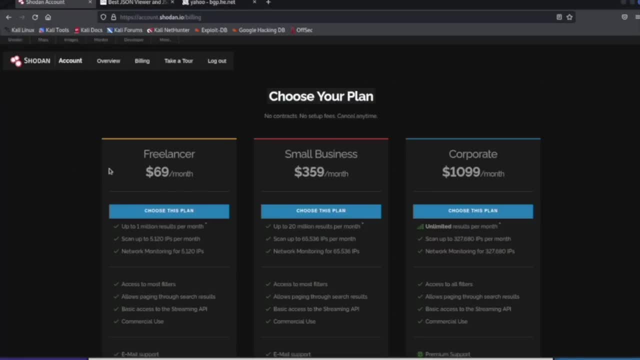 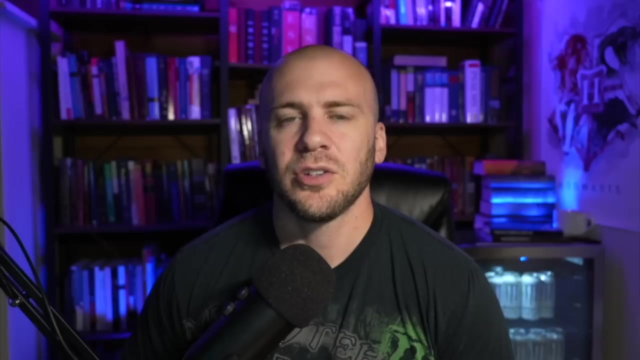 don't think it's worth it, but I know there are a lot of bug bounty hunters who do think it's worth it. so it might be worth it to you to monitor and just pay the $70 a month so that you can follow specific targets and be one of the first ones to go out and check those targets for vulnerabilities. so that concludes our video on Shodan. one of the things I want to make sure you understand is that when you run a Shodan scan and you're thinking about trying to exploit something, you need to make sure that it's in scope and has a bug bounty program. 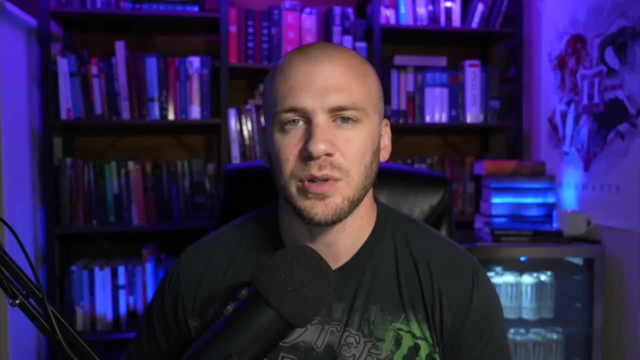 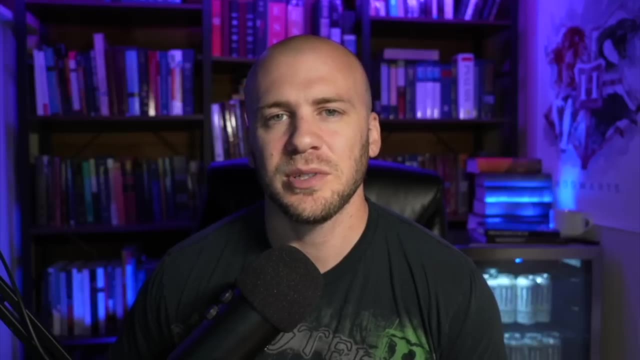 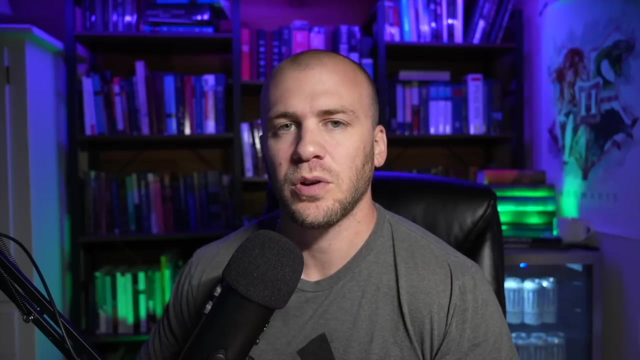 other than that you're going to want to make sure that it's in scope and has a bug bounty program, otherwise you could be getting yourself into some illegal trouble- and make sure before you go ahead and start looking at a specific target to see if it has a bug bounty program. so if you have any comments or questions, please let me know down below and I'll try to get to those as soon as I can. thanks for watching. we are going to be covering how to take notes for the world of bug bounty hunting- or maybe you are wanting to become a penetration tester. note taking is going to be really important to you and your method of note taking and actually being able to go back and overview what you have already done and gone through. 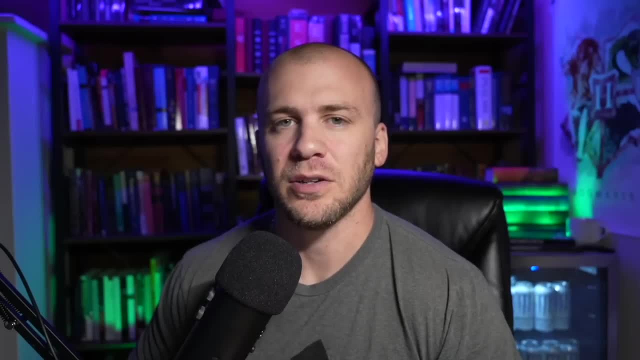 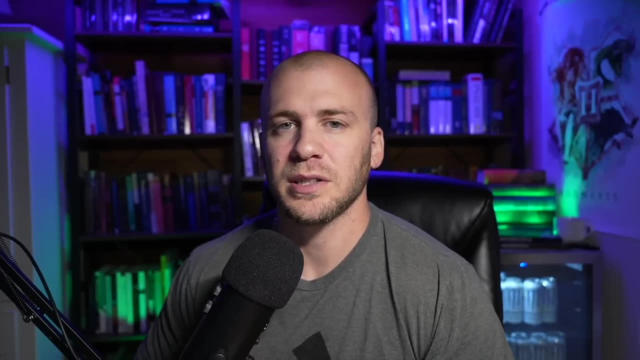 through your checklist is going to be really important. so in this video, I'm going to show you how I take notes and we're going to use cherry tree within Linux because everybody's going to have access to this. I personally use OneNote, but it's going to be really similar to what I'm going to show you in this video. 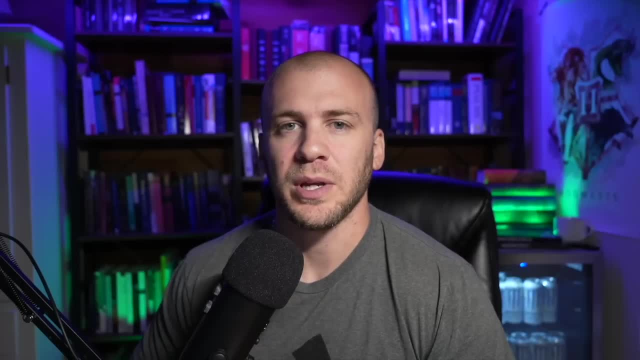 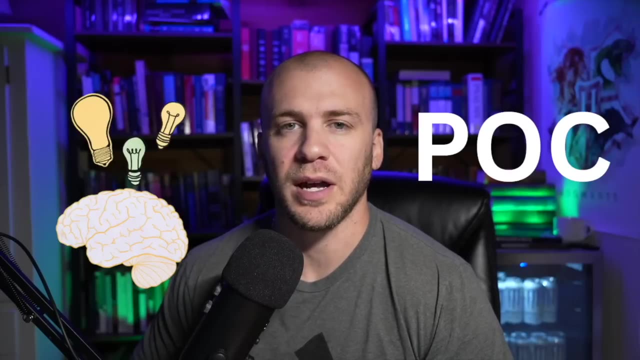 some of the benefits of taking really good notes is going to be having organized thoughts, being able to write a really simple proof-of-concept. you'll be able to have screenshots and be able to see what you have previously done, and you're not going to waste a lot of time going back to subdomains that you've. 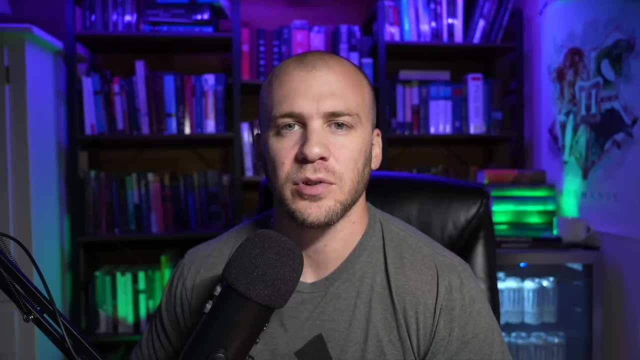 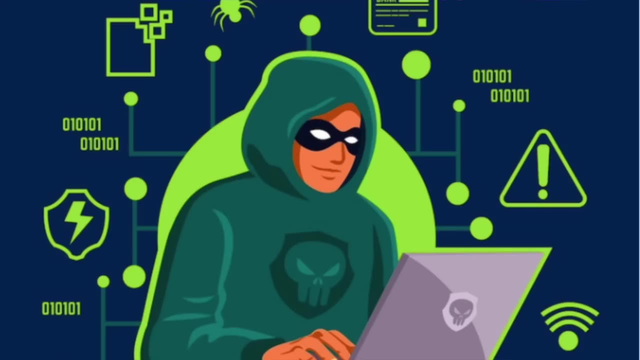 already enumerated and looked at, because you already know this, already have all of your notes there for you and know that you've already looked at it And if a new vulnerability comes out, you can go and see when the last time you enumerated looked at this. 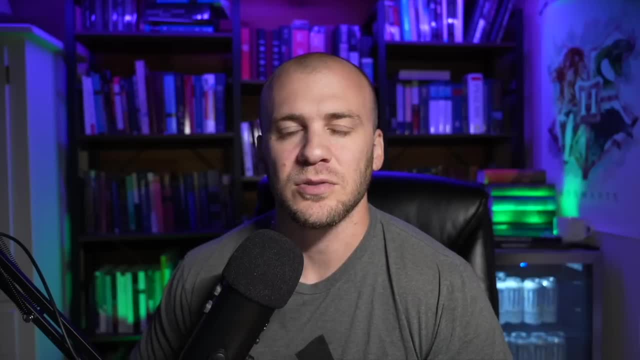 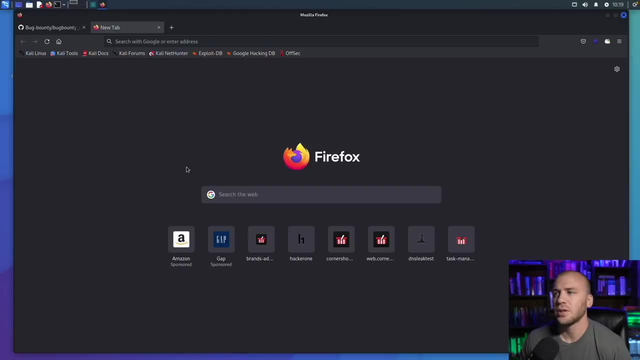 specific subdomain and know if the new CVE is going to be applicable to this specific domain and the software that's running on it. So with that, let's go ahead and jump into it. So here we are on our Kali Linux machine. we can come up to the little drop down menu and we can type in: 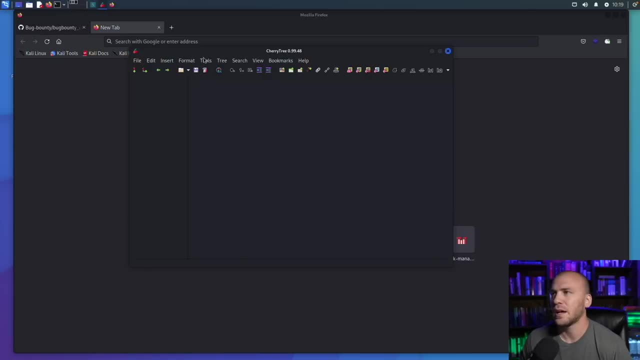 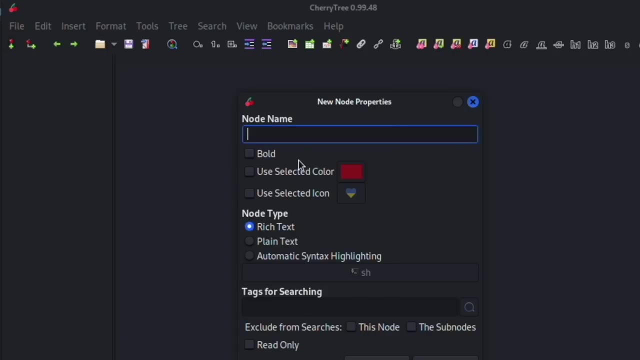 Cherrytree, and it will be automatically installed if you're running at Kali Linux. So using Cherrytree is going to be really pretty simple. The first thing you're going to want to do in your notes is you're going to have the main domain and all of the information that you found on it. So 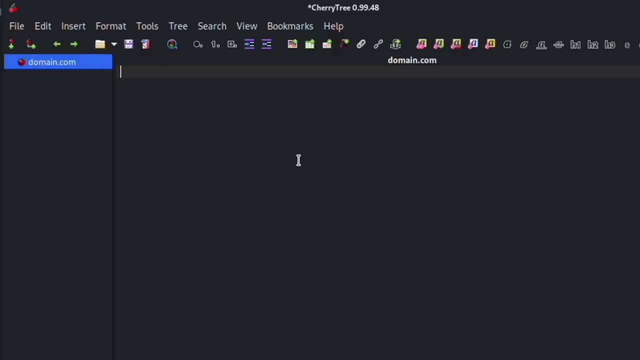 you can type in the domaincom and this is going to give you this parent node right here, And you can also change up your note taking method. And maybe you want to have the main domain and you have each subdomain right here. Like this, you could have subdomain one. 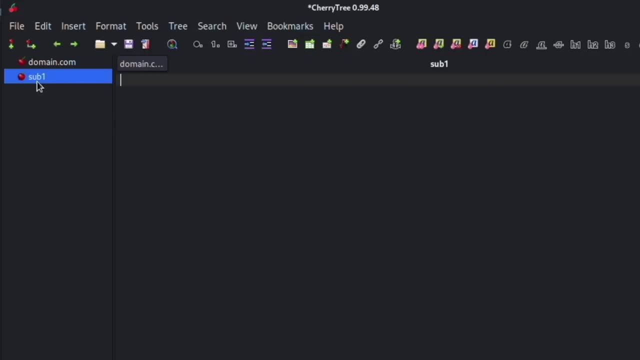 only it would actually be the subdomain name right here And then you'll have all of your notes from that subdomain. But if you do this, there are some programs that have like 800 subdomains and this would take forever to do, but you can come in here and do every single subdomain, like 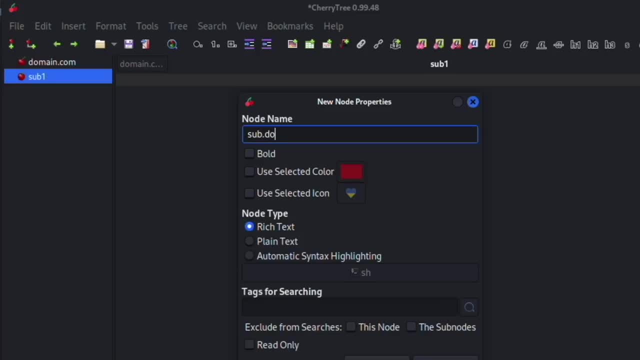 this, And so it'd be if we could just say subdomaincom. spell that wrong like this, and then you would have all of your notes within this specific subdomain. So if you decided to go this way, one of the things I would suggest doing right out of the beginning- 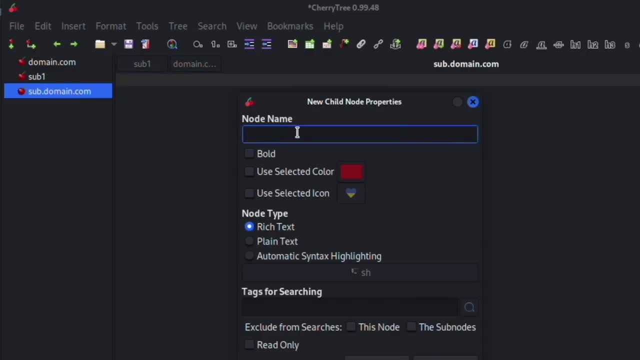 is when you put in your first sub node is maybe just call this the software right here And you can run. you can say that it's running some kind of CMS, maybe it's running WordPress, and then you'd have the version of 4.2.4.. And then you can know that this is what's running. 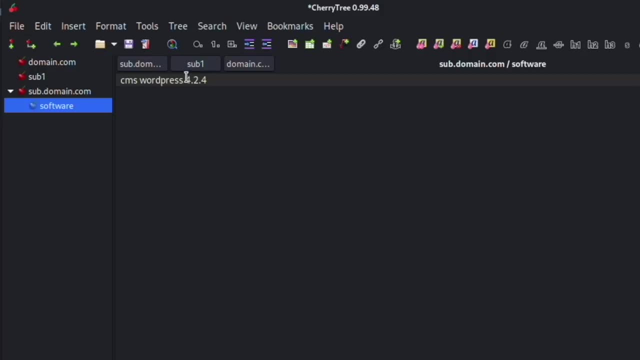 SUDWAY. in the future, if there's any kind of CVE that comes out for the WordPress version that's running, you can come back to this subdomain and see if it's vulnerable to that new CVE. Another reason: you're going to want to have some kind of list of the subdomains, So let's. 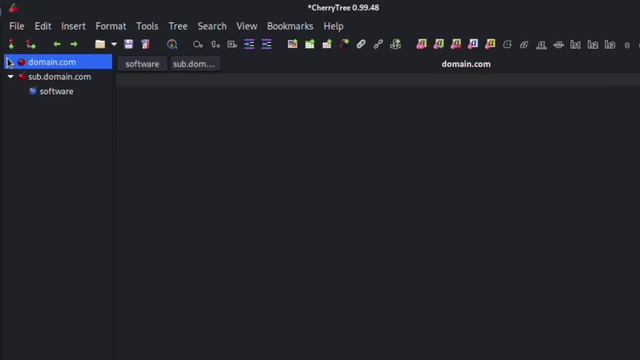 go ahead and delete this one right here. So it looks a little better If you decided to run a bunch of subdomains in here, so we can type in sub1.domaincom And in here you have a list of all of your subdomains. you can have actually subdomains in here within this specific thing. 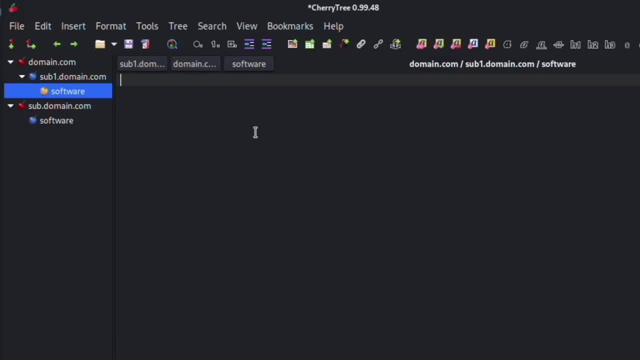 that you're looking at. So in here we could say software, And you can see how this is going to organize our research for us. And inside of the software in here you would put your WordPress and then the version that it is running. So these are a couple different ways to kind of organize. 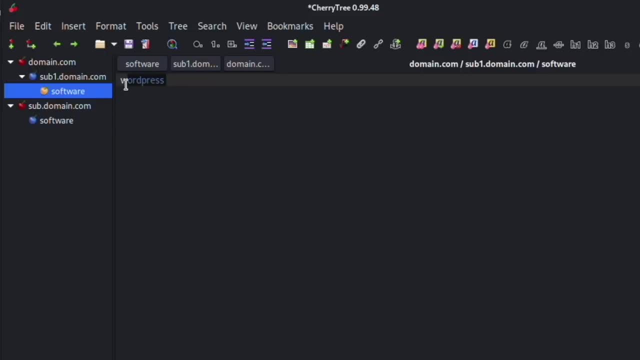 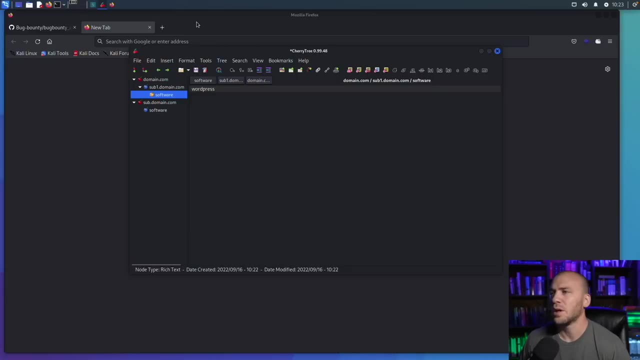 your notes, And another way to save time instead of actually going through and typing all this out, is on this box. I already have Wappalyzer installed, So I could just come. we can come to the browser and type in like googlecom and open up Wappalyzer to see what information is there. 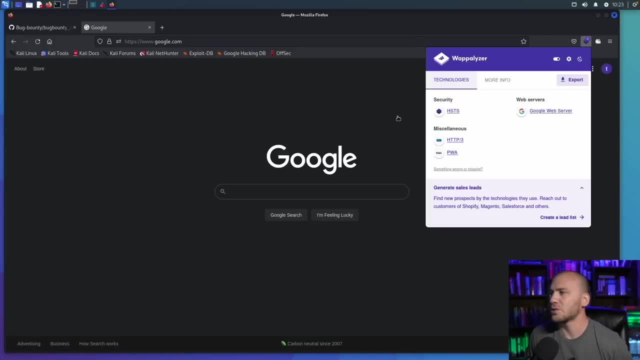 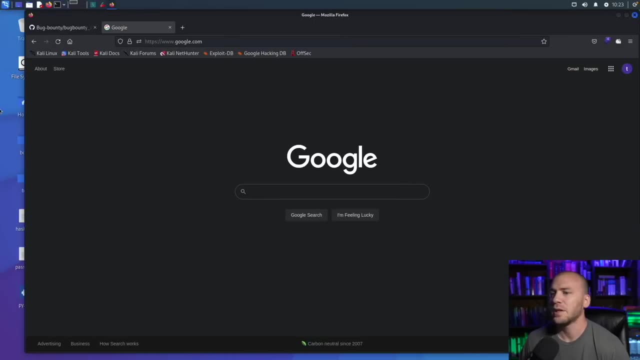 And now we could open this up Right here And I could just screenshot this and pull that screenshot over to my Kali machine And then I can put it into Cherrytree. So I could grab this and pull it over and put it into. 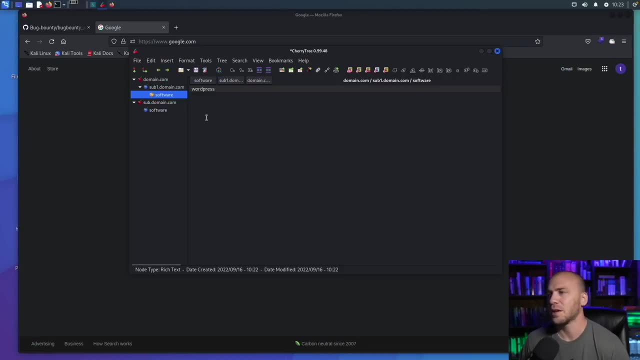 Cherrytree. I actually don't have this specific Kali box set up to do that, So it's not going to work for this one. But on my actual personal Kali Linux machine that I use, I can just pull screenshots back and forth over to my Kali machine and save them inside of Cherrytree. 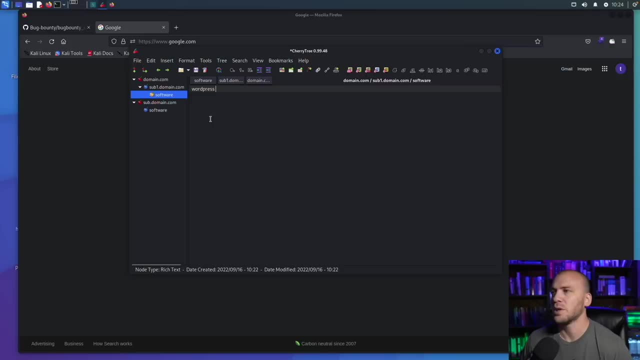 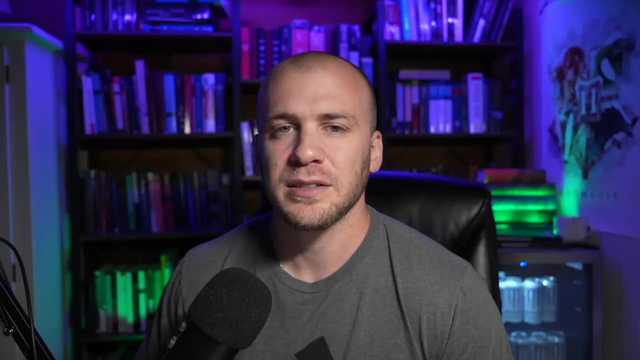 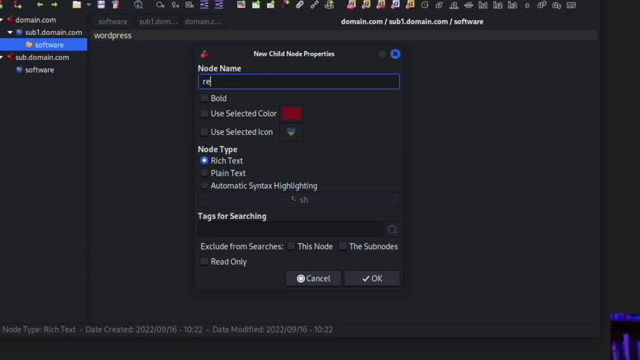 But I use OneNote So I don't really have to worry about that too much. So screenshotting and adding information in here is going to be helpful as well if you have that capability, And one of the things I like to do is at the end of a recon session is make a node like this and we'll just call it a recon. 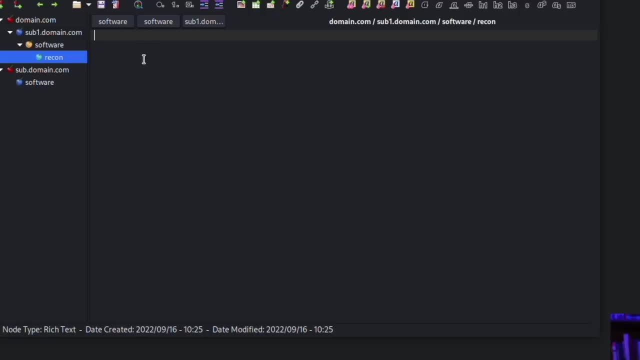 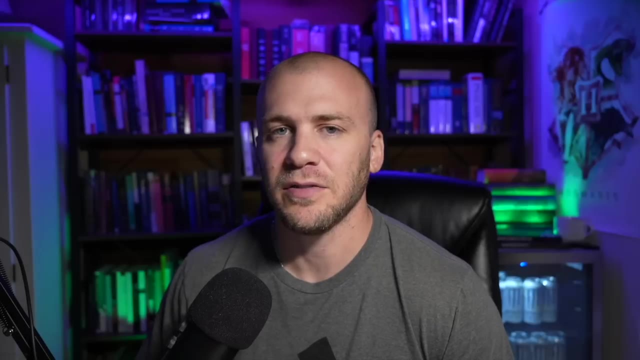 node And then in here I write down all the tools I ran and the way that I collected all of the information. So that way I have a clear set of notes And that way if I ever come back to this specific target I can see if maybe I've missed something or maybe I've learned some kind of 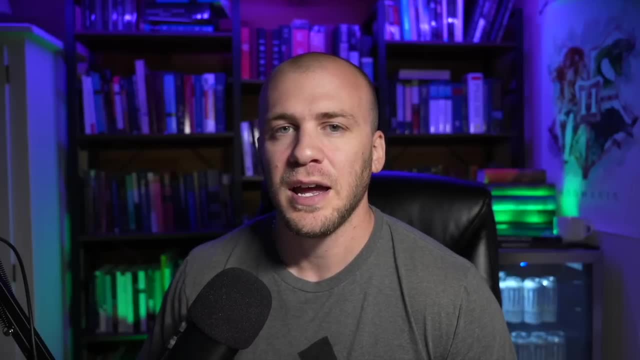 new recon technique that I can try out on this specific target And I'll know what exactly I have done on this target and what I can do in the future to further analyze the information on my specific target. So make sure to write down your methodology of your recon and attack because it may change in. 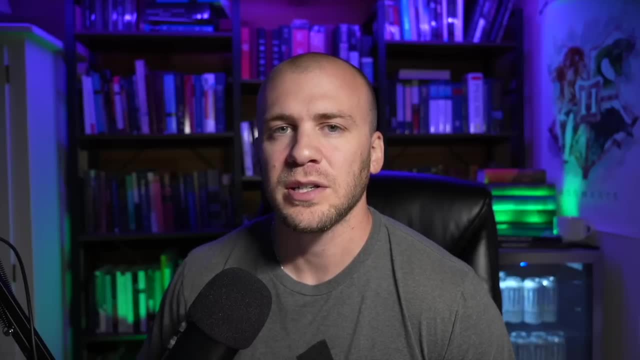 the future And you might be able to go back to old notes and old targets and further do enumeration and testing. And, lastly, one of the things that is going to be really helpful for you in your note taking process is to have some kind of 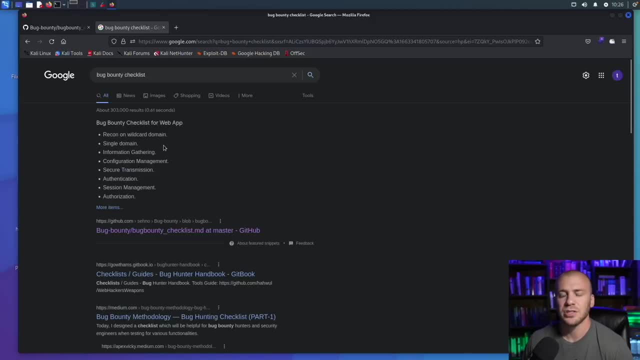 checklist, And so one of the last things you're going to want to have is a good checklist of vulnerabilities and recon, And you can just go out to Google and look for a bunch of different checklists and find whichever one works best for you, Maybe copy paste it and put it into a Word. 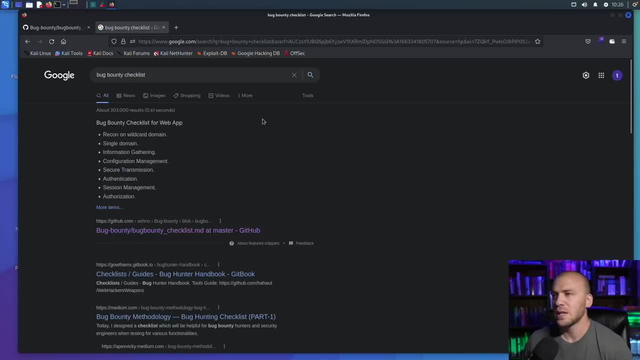 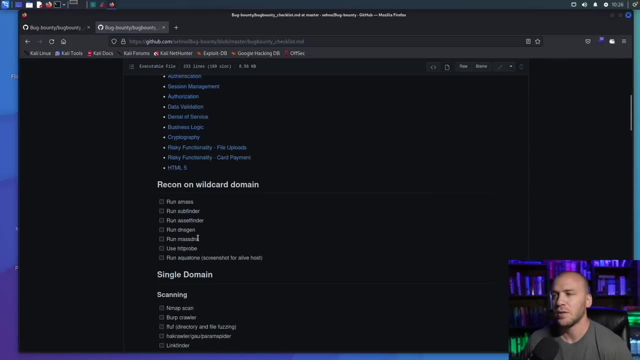 document and modify it and make your own. But in the meantime you can just Google bug bounty checklist and click on one of the checklists and then look to see what is in here and you can follow their recon. Maybe there's something in here you don't like. I used to use HTTP probe but I decided. 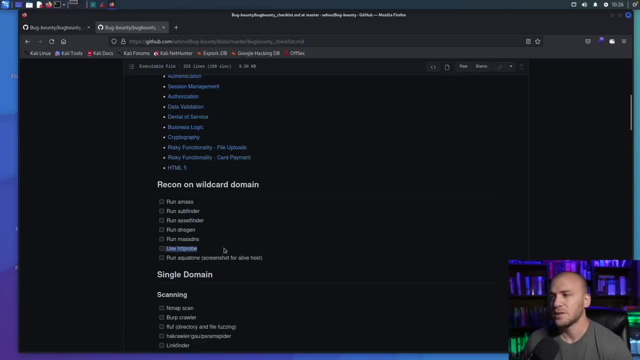 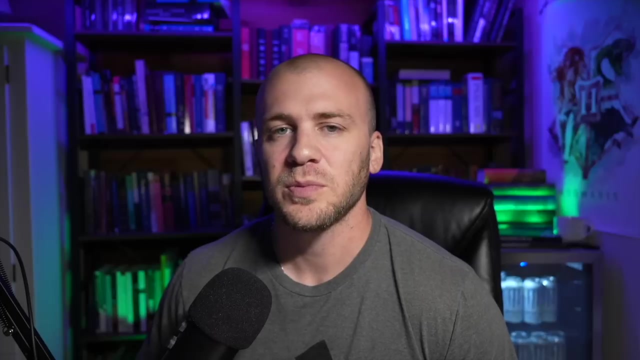 I actually like going out and checking things. I don't use this anymore, but it would be helpful for you to have something like this, Some kind of checklist, so that way you don't miss any bugs or vulnerabilities or maybe hidden subdomains that you would have otherwise missed without a checklist. So this will be really 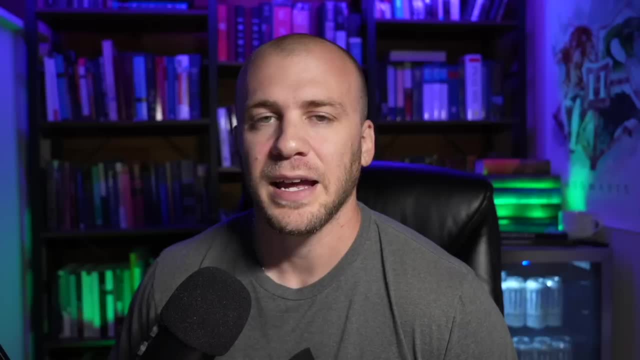 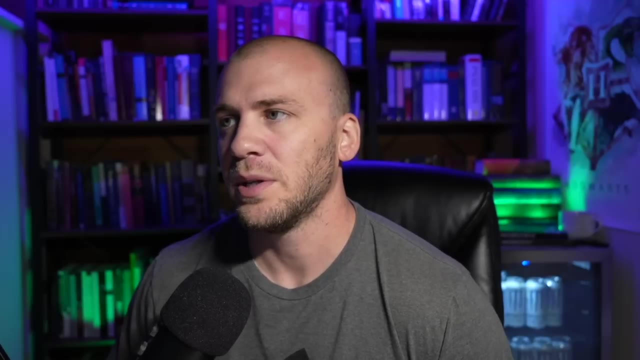 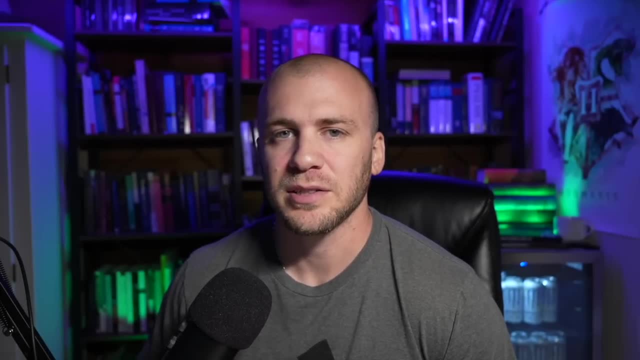 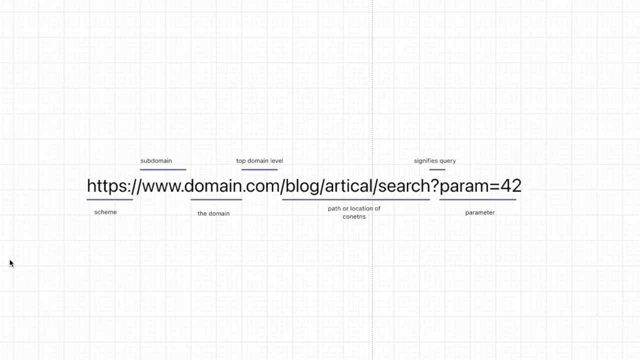 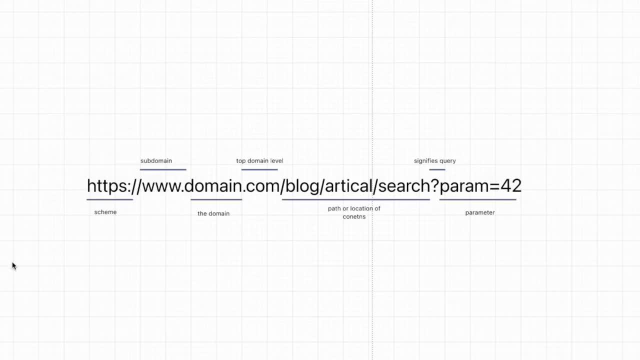 you can get an understanding of what is going on when you look at these. It's really important in your recon phase to be able to know what URLs look interesting that you can copy and paste into your notes so that you can come back once you have finished your recon phase and actually start. 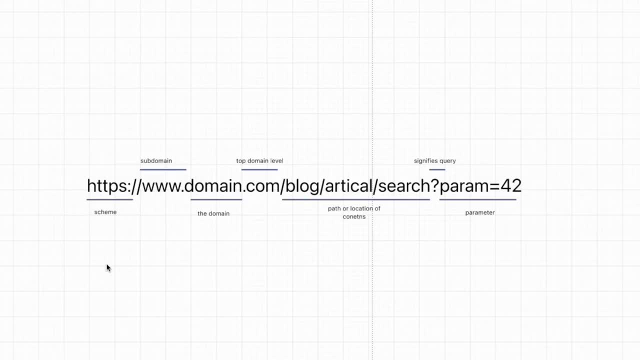 testing. So I've gone ahead here and just typed out a basic example. I'm going to go ahead and and you're probably all familiar with HTTPS and HTTP protocol and it is labeled as the schema. The www is not always there. This is labeled as the subdomain because sometimes this could be a 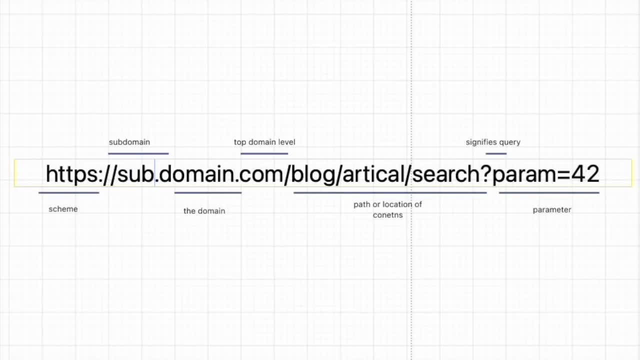 this could be a subdomain, listed as subdomain, And so this is actually a subdomain, but that is the same thing as the www, And so right here we have the domain name, which would be like googlecom, And I'm not really sure why the com is actually listed as the domain name. 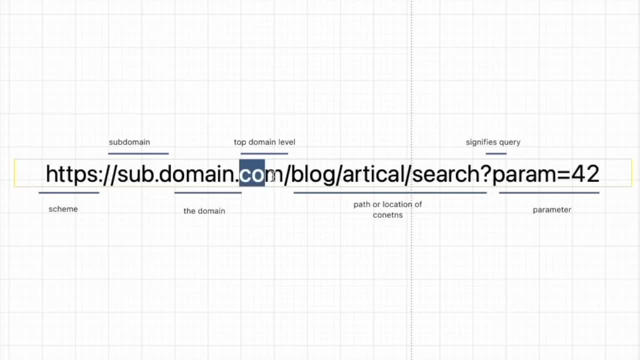 But it is listed as the top domain level because you can use in here like uk fr for different countries, a net, a org for an organization, And it's still called the top domain level. But that is this portion of the URL. So all of this is a pretty basic. 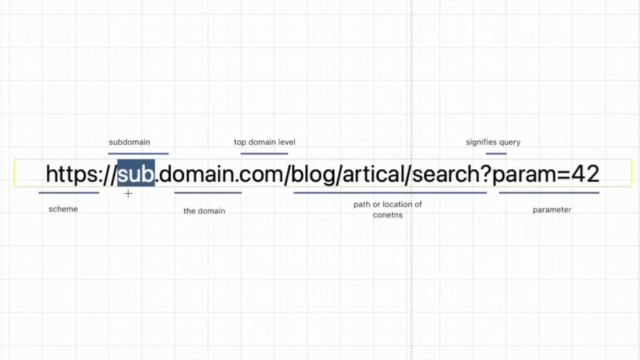 You can fuzz this right here. the subdomain And the most popular subdomain fuzzer that I can think of is WFuzz. I'm sure you can use other fuzzers, but WFuzz is one that seems to work really well for me. 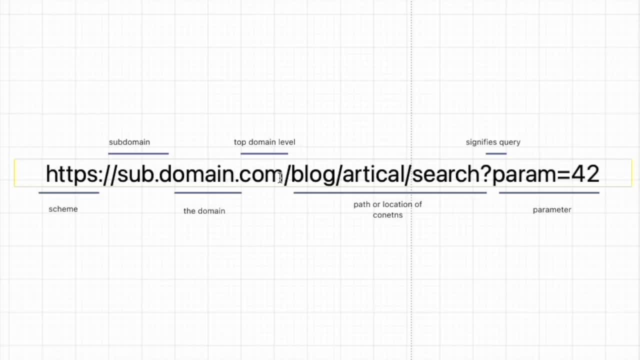 when I'm doing a subdomain And then right here is when we start to run into the path or the location to the contents- is how I have it labeled here, But I usually think of this as a directory. This is a directory, And then eventually you're going to hit a actual page. 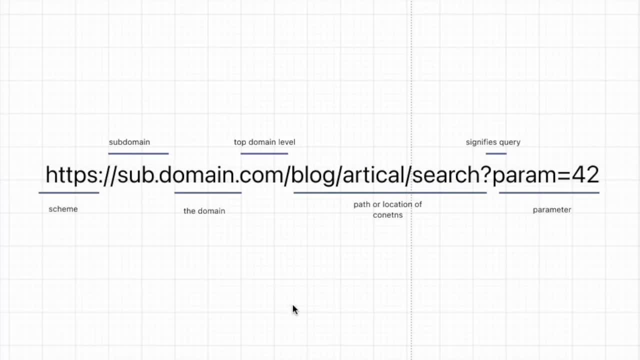 And you can actually delete some of these and you could just go to blog and see what's there, But this is the path or the location of the page. Now here comes kind of the good part for us to look at And before we move on, you can actually fuzz for different directories. 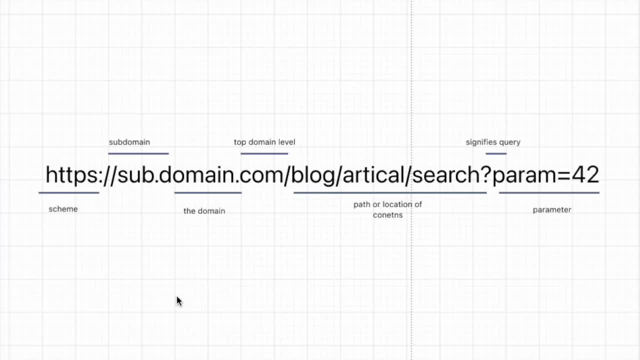 right here. the same way, you would fuzz for subdomains and look for different directories within the subdomain or domain. and now when we move on to right here, the question mark. what you need to remember about the question mark within the url is that it signifies a query and a parameter. 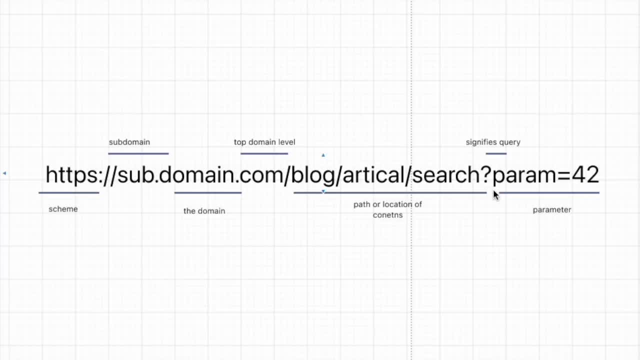 is about to be dropped in and this is where we can start messing with the url to see what information we can pull back from the server. so you can try. you can try and look for an lfi and rfi and ssrf and actually right back here you can look for directory traversals. but you have a. 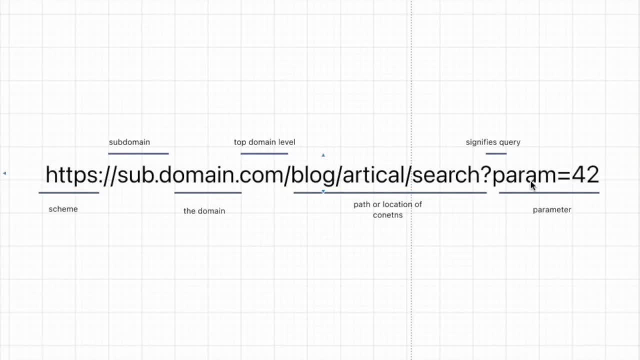 parameter. usually it'll be labeled. usually it'll be labeled as something other than parameter. one of the ones that automatically throw up a red flag for me is when i see a parameter that says url and then this query: you're going to look to see if this is querying the actual server itself. 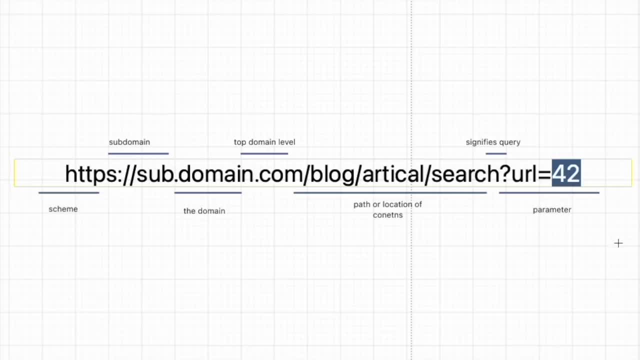 and if it is, you can start to look for a server-side request forgery or something along those lines. but let's say, this just has a like an id right here of 42 and you can go ahead and start changing this 42 to other numbers and 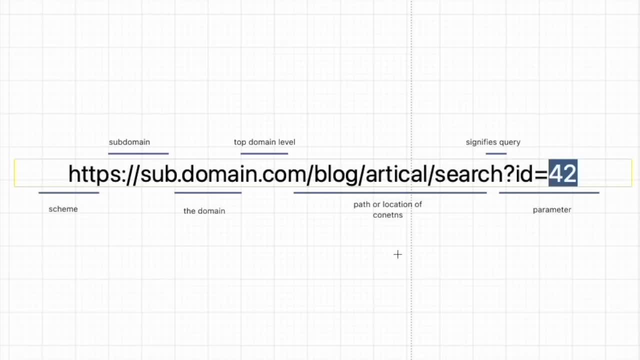 see what information you can come back and maybe see if you can access some information that you're not supposed to. so this is a url, and one of the reasons i wanted to show you this is because when you're in your recon phase and you're not yet testing to remember to save urls that look really. 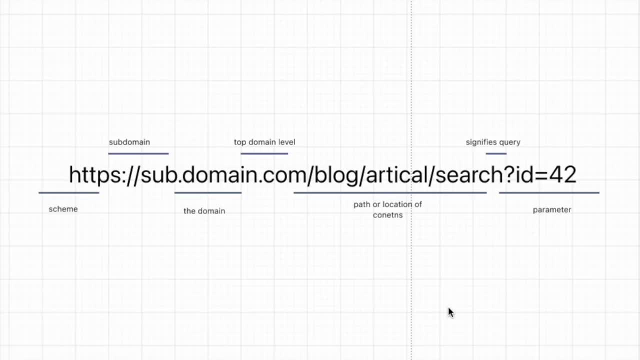 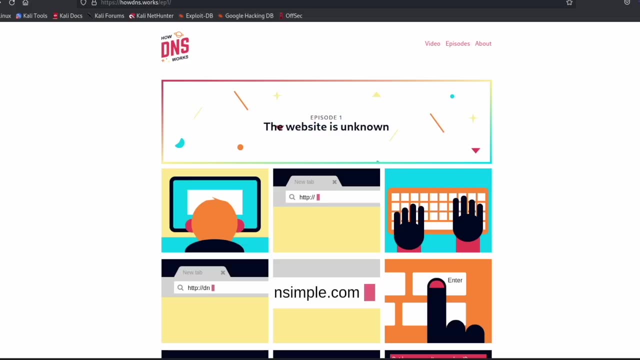 interesting to you with different parts that you're able to change or fuzz that you think might be useful, that you should not have access to. in this video we're going to talk about how the dns works or the domain name server, so if you decide you want to type in something like googlecom. 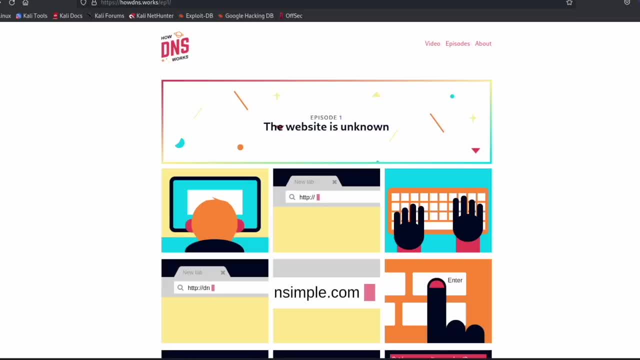 how does your browser know where to go and find the google ip address to resolve the web page to you? so i googled how dns works and had to go through a few pages before i found something that was actually good for an example, and i thought this was a really good example. so we're going to 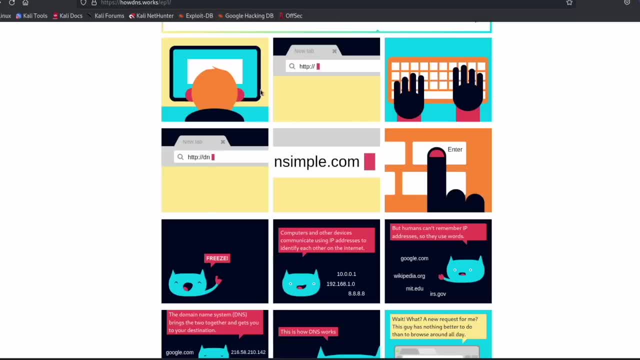 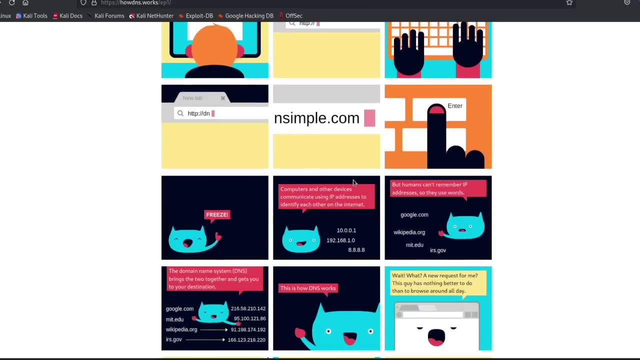 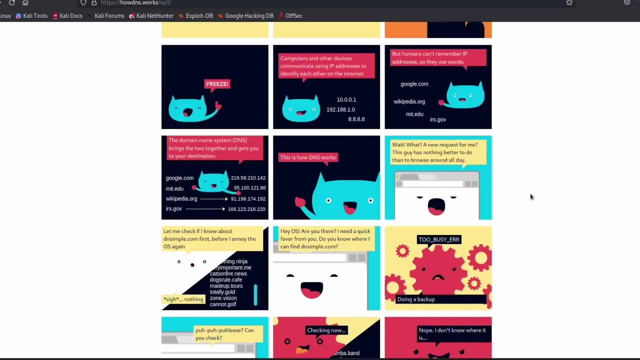 go ahead and walk through it. so you have a person right here who types in a domain right here and they type in dns, simplecom, and it will check the web browser's cache, which you will see right here on your local machine, to see if you have visited this page before. so if you ever go to facebookcom. 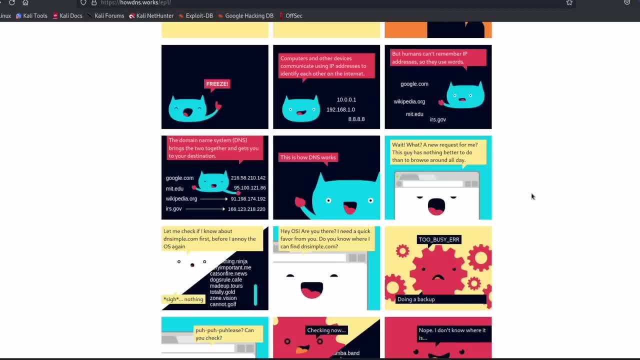 and you're logged in. in the future. next time you go to facebookcom it automatically logs you in because you have stored your session and cookies in your github browser. so you can go ahead and log into facebookcom using firefox and then you go to chrome and you try to log into facebookcom. 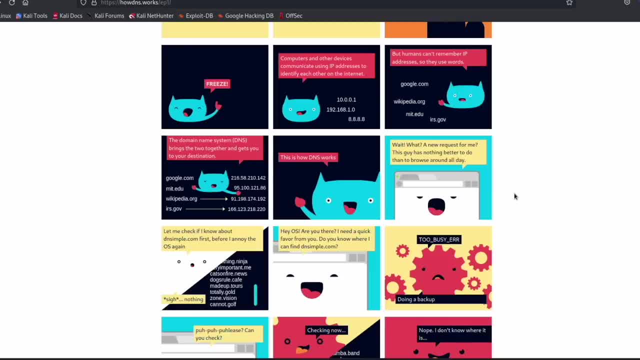 you're going to have to re-authenticate because it doesn't have that stored in your browser cache. so the first place when you type in a web address it is going to go to the web browser to see if it's stored in the cache. and before we move on here, you can see right here googlecom: they have. 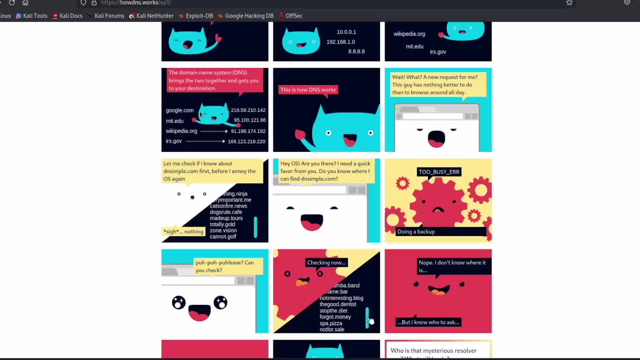 an ip address for that and if you go to the web browser you can see that they have an ip address. the reason you have actual domain names attached to ip addresses is because it's easier for us to remember a domain name, such as facebook, rather than a string of numbers for facebookcom or a. 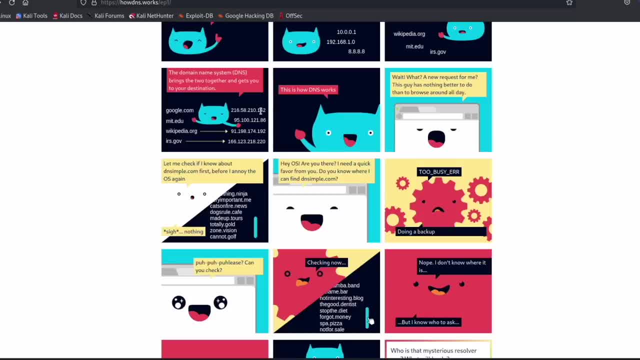 bunch of other web apps. we just remember we need google. we don't need to remember this string of numbers right here. so the purpose of a domain name is to give you an easy way to remember the contents of a specific ip address which is going to resolve to either google or facebook or 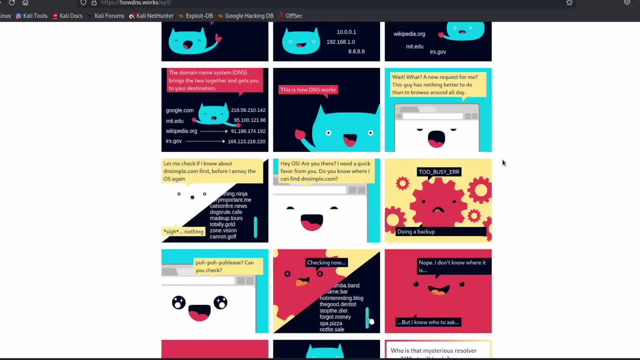 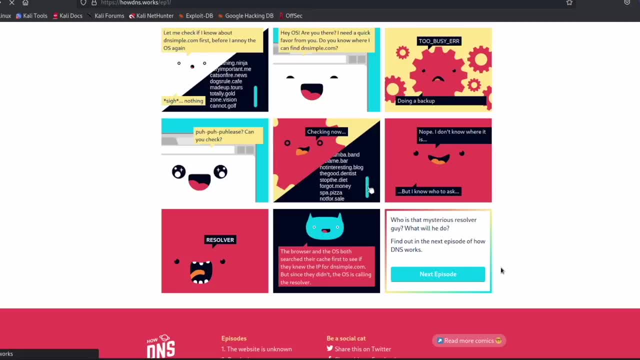 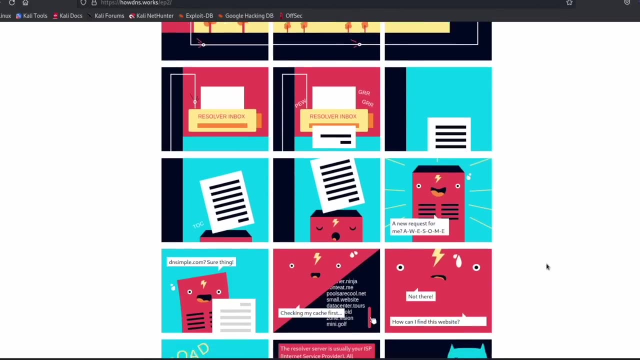 facebook or any other ebay site. so that is the purpose of the domain name. so after you're using the domain name, you're just going to have to re-authenticate, and you need to remember that after your browser tries to gather the information and it's not able to, we can go to the next page. 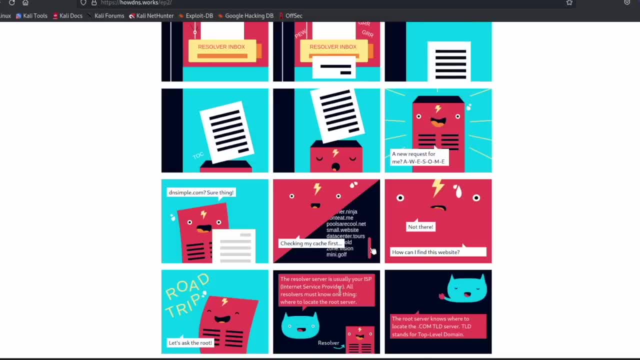 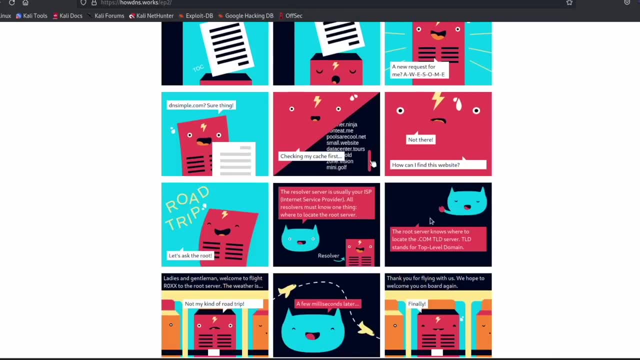 and it shows the packets moving out to the isp server, which is going to be your internet service provider, which we're told right here, and it's going to ask: how do we find this website and where to find the location for the com tdl? and we've talked about the tdl before. it is the top. 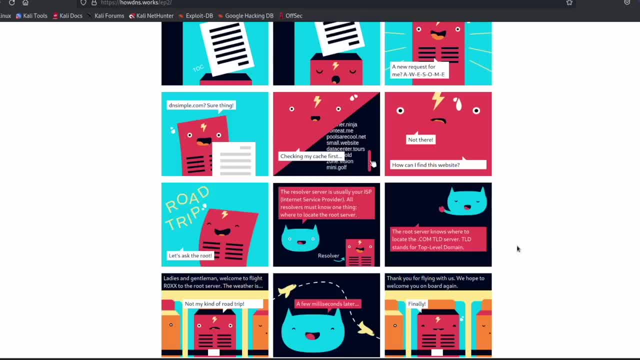 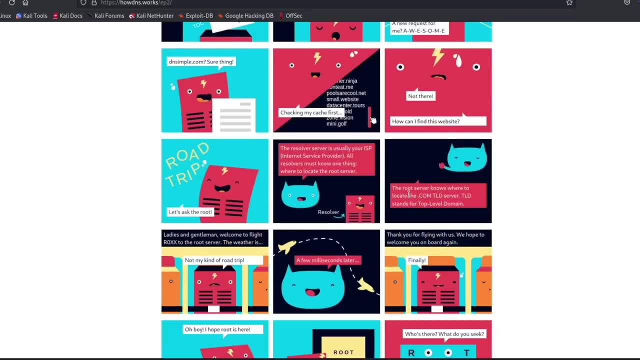 level domain, which can be comorgeduukfr and many others. so those will be the top level domain servers and it's going to tell you to go out to the root server and the root server is going to give the information back for which tdl server you are looking for. that's going to contain the 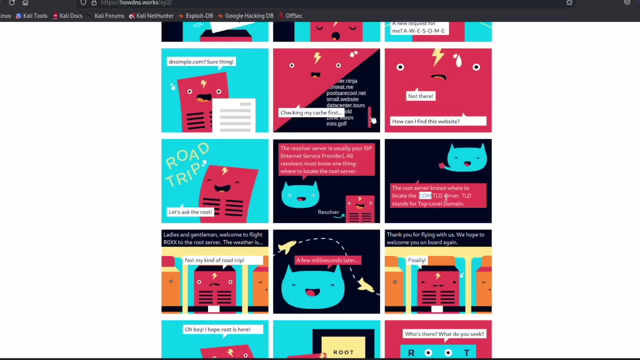 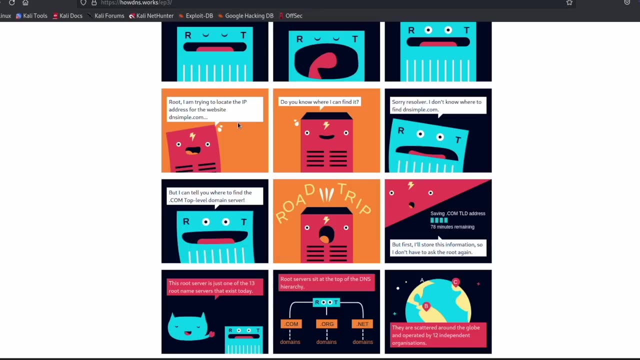 information you want. so if you want the com tdl or if you want the org tdl, and the root server is going to pass the information on to the next server in line to give you the information. So here we are, at the root server and our packets are going to make the request and we're going to 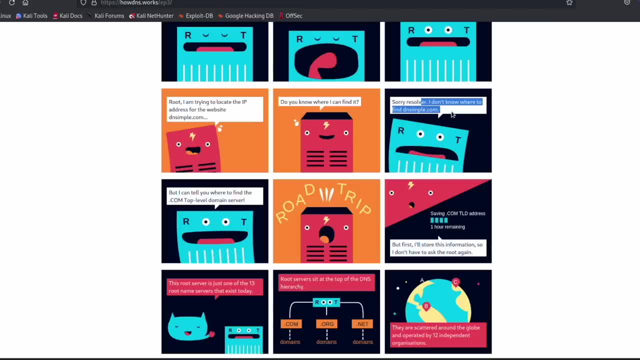 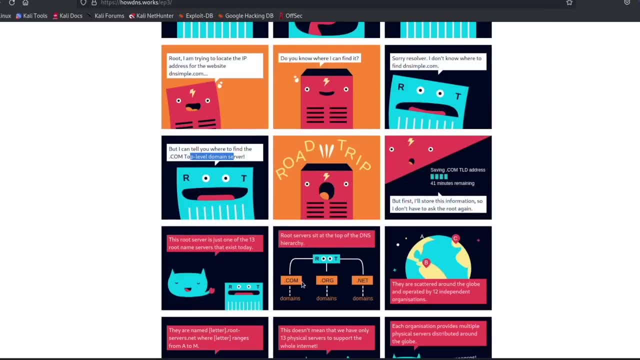 be told that it doesn't know where to find dnssimplecom, but it's going to be able to tell us where the the tld is located and it's going to send us on our root server way. so you can see, here is root and here are the tlds and it's going to send us to the right one. 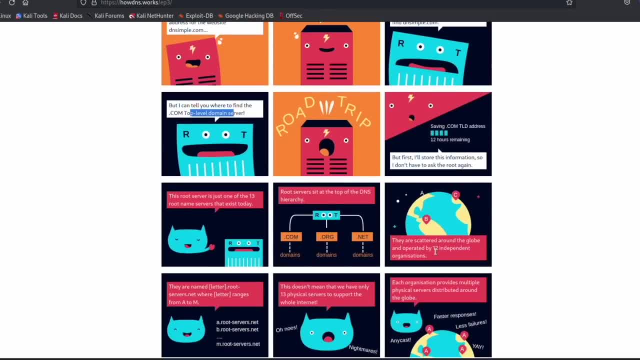 so, before we move on too far, if you're wondering how this would work with, say, something like the tor browser, my understanding of how the tor browser works is that it's going to encrypt all of your data so that the isp isn't actually able to track the web application that you are trying. 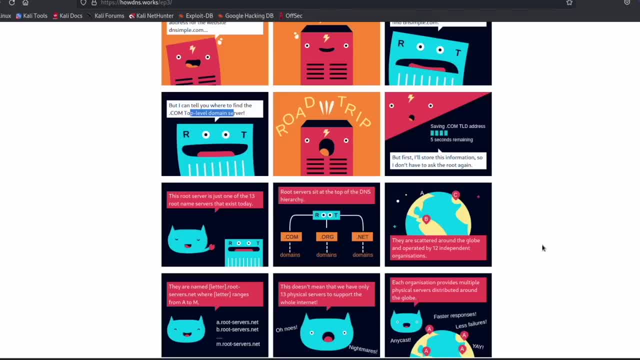 to reach and the tor network opens up a bunch of nodes for your encrypted data, and it doesn't actually go through this process until- actually until after it has reached the exit node. and that is how your isp, your internet service provider, is not actually able to track where you are sending. 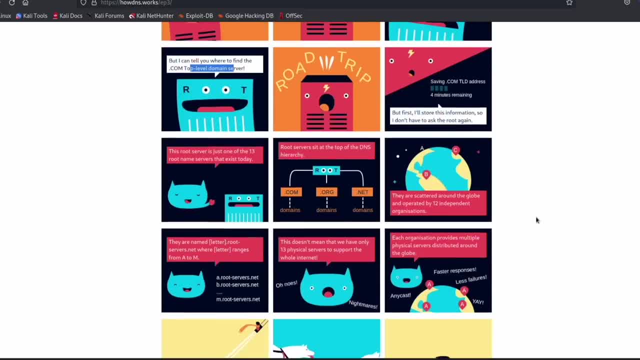 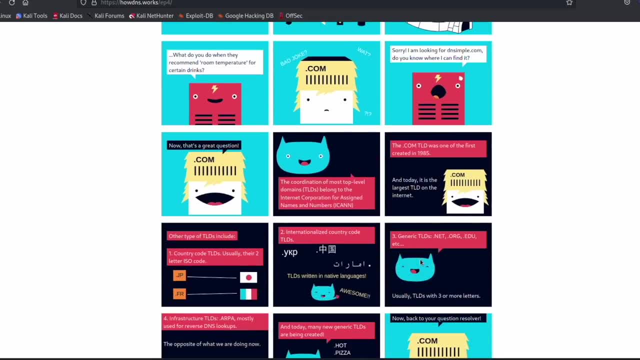 your requests to, and the same thing would work with a vpn as well. so on to the next page and it gives a little bit of a history that we don't really care about on the tlds, and finally we make it to the dot com tld and then we're going to go back to the vpn and we're going to go to the. 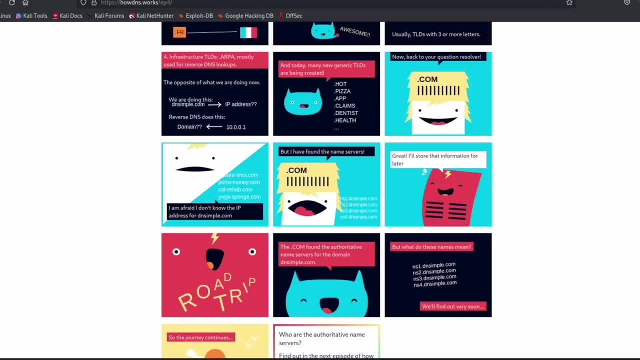 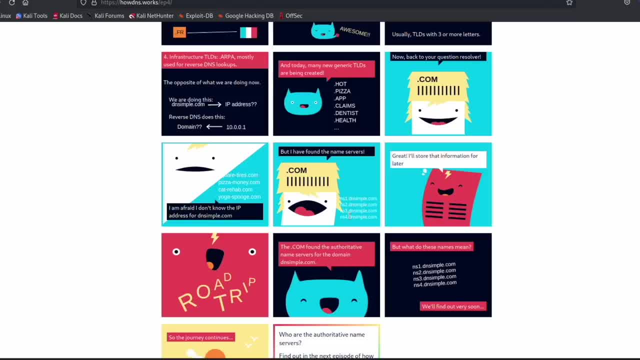 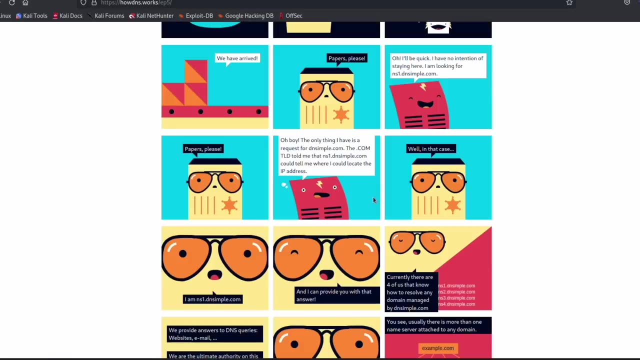 to data and we're going to go to html and it's going to see if it's some rabbit1 full html. so, server at this point, and you get sent on your way to the next page and here you make it to the ns1 and then s1. it says I can give you the IP address and then you 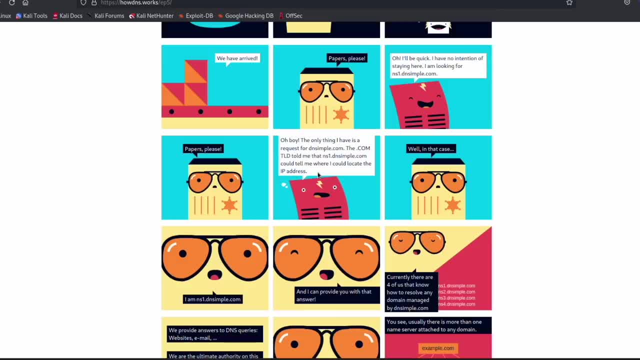 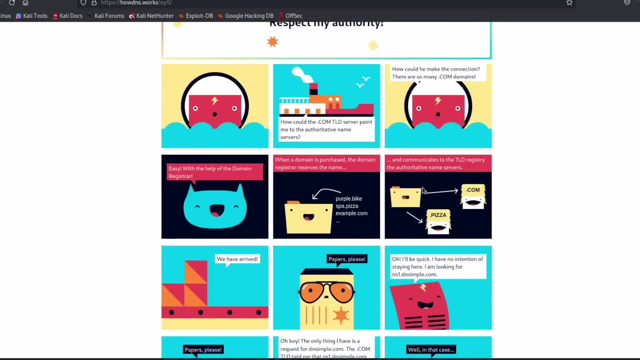 get the IP address and you're able to resolve to that specific IP address that you queried in the beginning, such as a googlecom. so I hope this made sense. if not, you can watch it again or you can read through this. you can see the URL is: 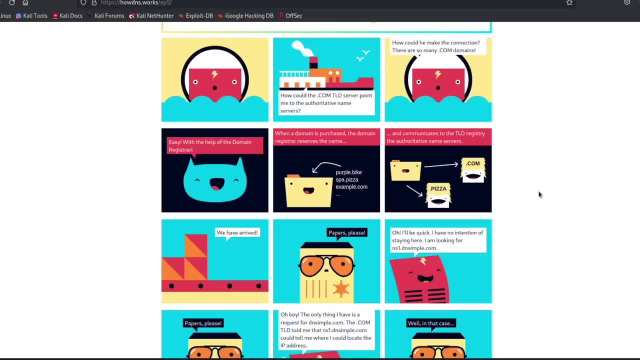 right here for you to go to, or you can google around and read. maybe something else explains to you how DNS works. if this was too confusing, and if not, you don't necessarily need to know all of this information to move on into the world of ethical hacking, but I thought it'd be helpful for you to understand. 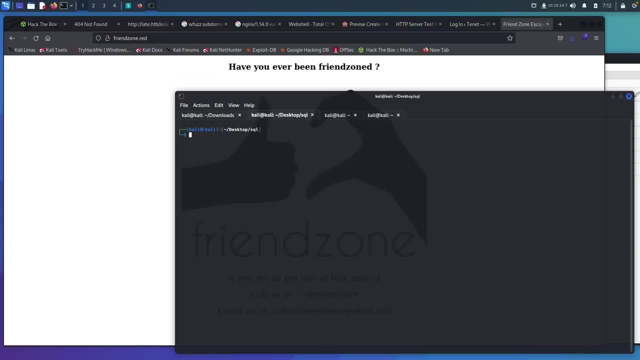 how the web works. all right, in this video we're going to cover a tool that is called dig and it will check for zone transfers. you're gonna hear about a zone transfers. it is a great way to find additional subdomains. You can use FUF and GoBuster and WFuzz and try and 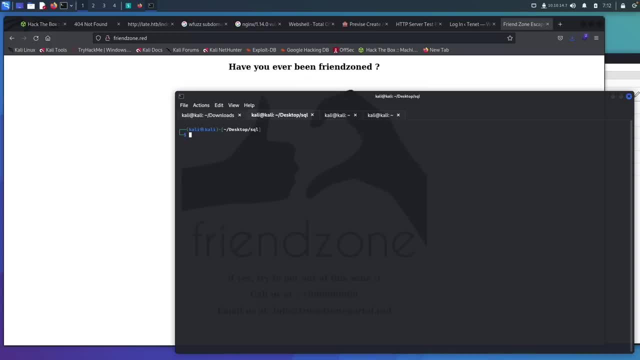 brute force for subdomains and use Sublister, but you can also use Digg. It's really quick and if there are any subdomains, it's a really helpful tool because you'll find them right away. So a DNS zone transfer is supposed to replicate a DNS database between DNS servers, which means 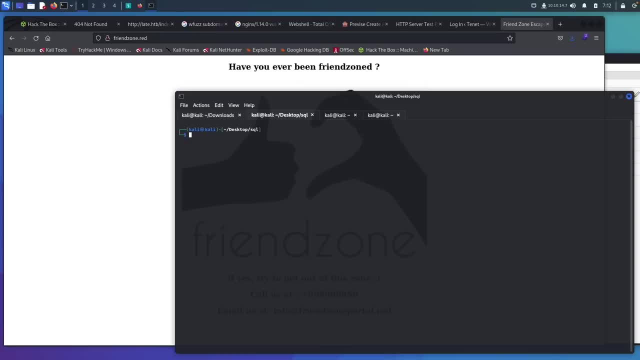 if it is vulnerable to a zone transfer. it will give us information like subdomains and some other information which we'll see in just a second. So we'll go ahead and run this. I have opened up the box friend zone from hack the box because it is vulnerable to a zone transfer. 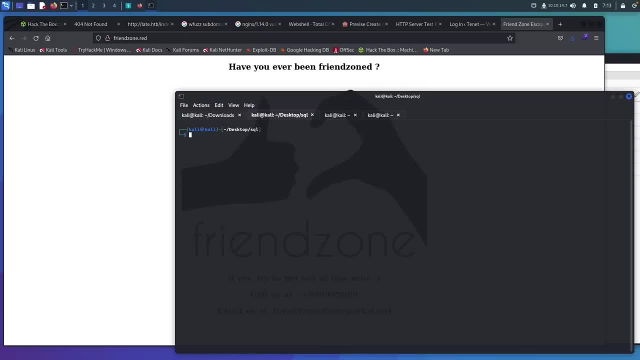 And if you find a bug mining program that's vulnerable to a zone transfer, you're not actually able to exploit it and hack per se the web application, But when you find a zone transfer and something is vulnerable to a zone transfer, you can report it as information. 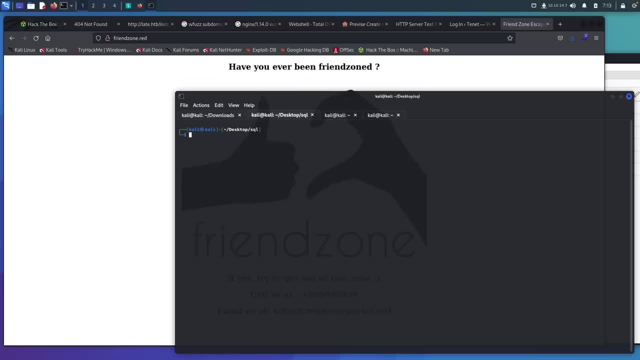 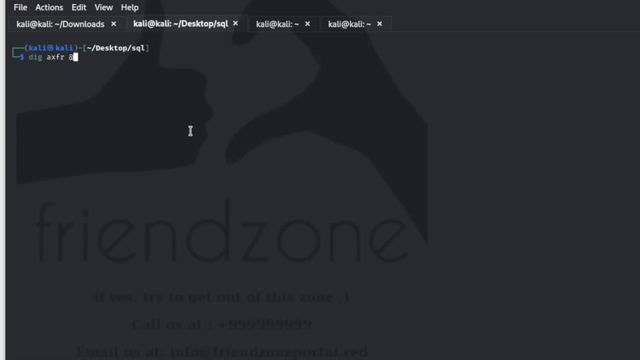 disclosure, because it's something that should not be open to the world. So the easy way to test this is with a tool called Digg, and we'll just type in Digg, So we'll go Digg, AXFR, and then we will say at, and then we're going to use the IP address And then we'll use friend zone, because that is. 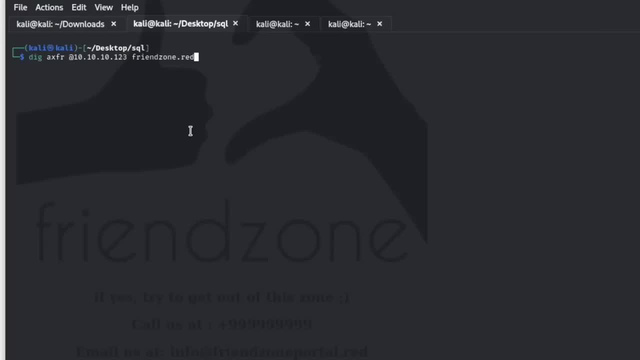 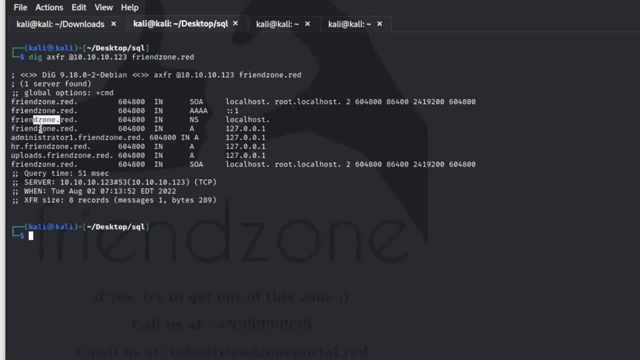 the domain that we are after dot red, And then we can run this and see what it spits out. for us. We have friend zone, friend zone, friend zone and administrator one, So this would be something that would be worth checking out. We have this HR. We have an uploads, which would also be something. 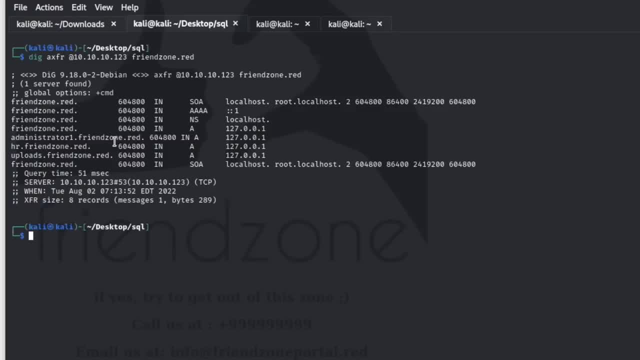 worth checking out if you're doing a CTF or if you find this information out in the wild And so you can actually save all of this into an out file and we'll just call it zone, Just like this, And then from other recon, that is done on this box. you also find a another domain. 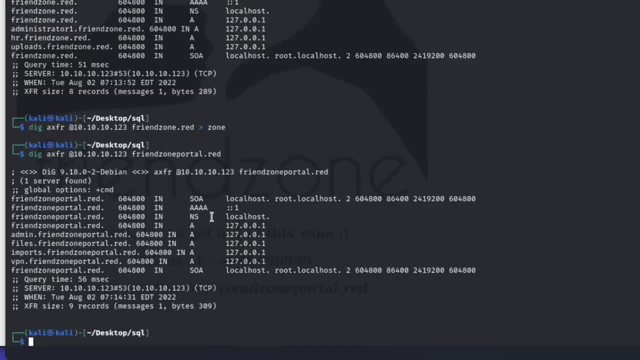 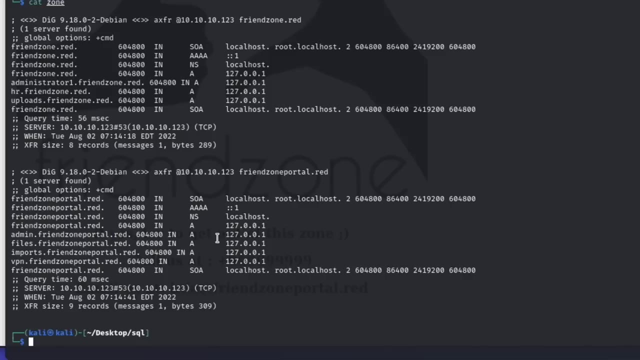 called friend zone portal, just like this, And we can run it and we find admin files, imports, VPN, and you have all of these files as well, And so, if you double care, it will just append to our file. So if we cut out zone, we have all of this information. And now, if you have taken my 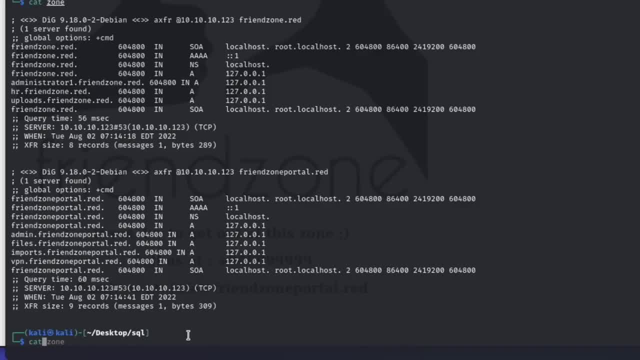 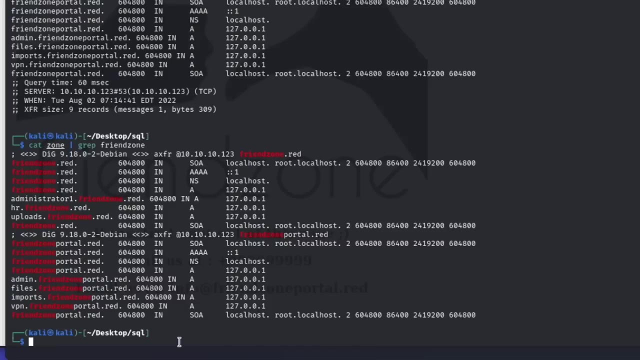 little bash course. you know that we can cat out the zone and we can go like this and we can say grep friend zone and make sure that works, And so it'll point out, it'll give us all everywhere that friend zone is located, And then we can say grep in and then we want to hawk for our cut and 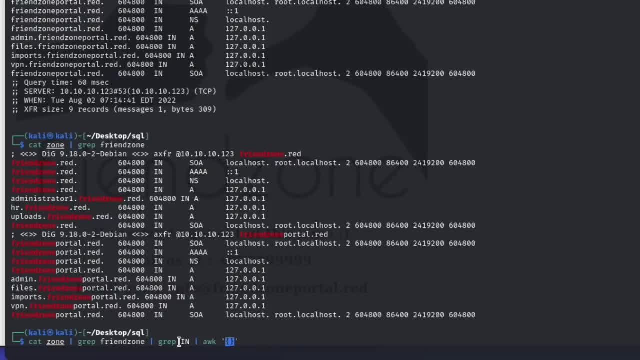 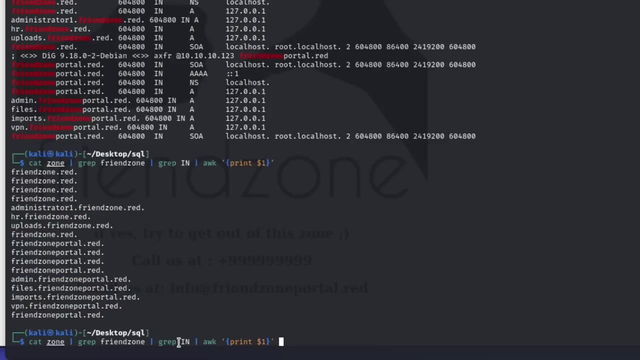 go ahead and put in our curly braces and quotes And we can say: print dollar, sign one, because we only want what is at the front of this file, And then we will see what happens. Yep, That's what I thought was going to happen It. 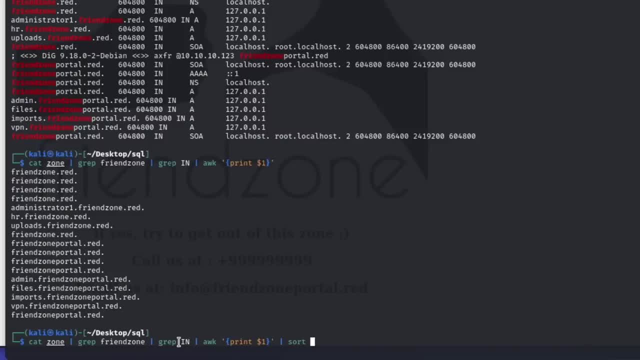 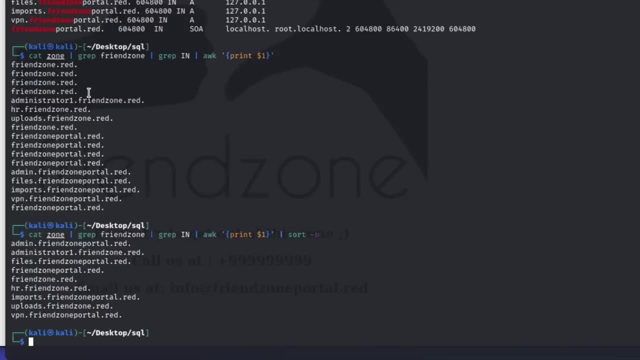 gives us what we want, And then we can say: sort dash U, and this should get rid of our replications right here. And it does, it sorts it out for us and we get rid of a lot of the repeats, And now you have this nice little happy five. 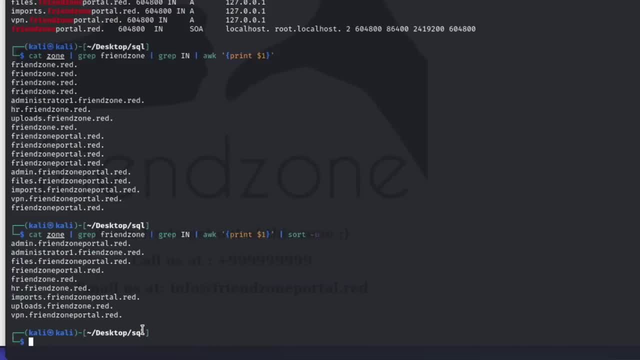 So let's go ahead and take a look at the file with just the subdomains that we have pulled down from the zone transfer. So zone transfer is something you should always look at And if you're in a hack the box, you might have to add more of these to your Etsy host file, But out in the wild these would be really good targets to go ahead and try to attack and find exploits on. So this is the zone transfer with the dig tool. You'll want to remember it whenever you see a port 53 that is open. That is the. 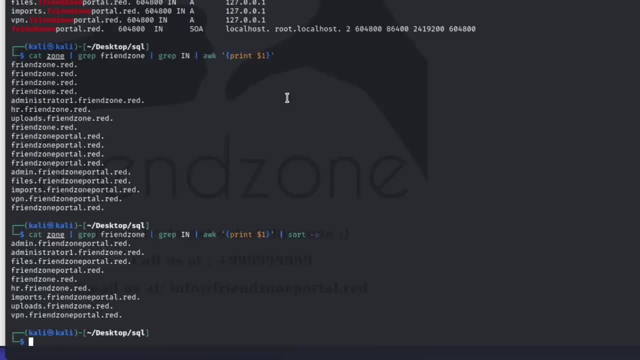 port that is used for a zone transfer. So a few things to remember about this specific tool. If you run an in-map scan- port 53, if it's open- you can always try for a zone transfer and see if you can pull down additional subdomains. It's a great place to grab subdomains. You can also report it as information disclosure if you are actually able to pull off a zone transfer. So with that, we will move on to the next tool. All right, I want to cover two more. 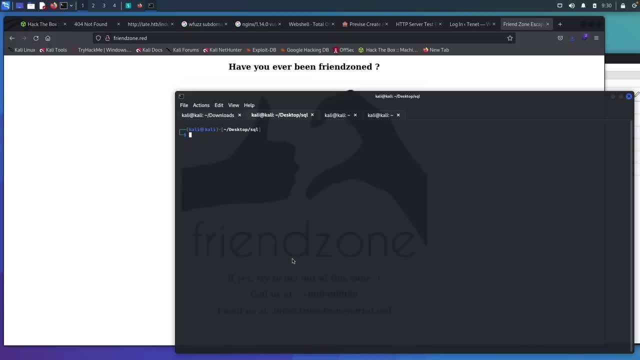 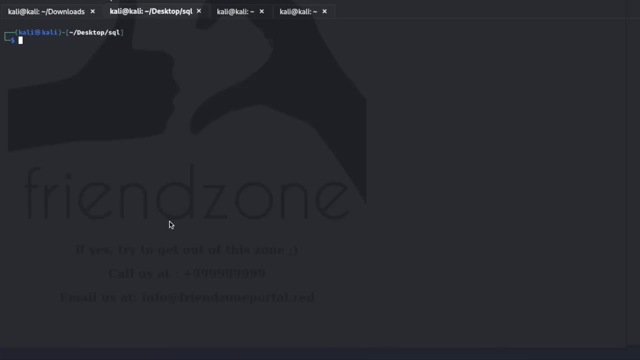 tools that are recon tools that you're going to hear about, but I don't really use a whole lot because I don't think I get a whole lot of helpful information from. but you're going to see these and pretty much every penetration testing textbook, every certification course you ever come in contact with, And they are who is? and NS lookup. We do NS lookup real quick because it doesn't give us back a whole lot of information, So we can just type in NS lookup, just like this, And then you can do something like wwwgooglecom. 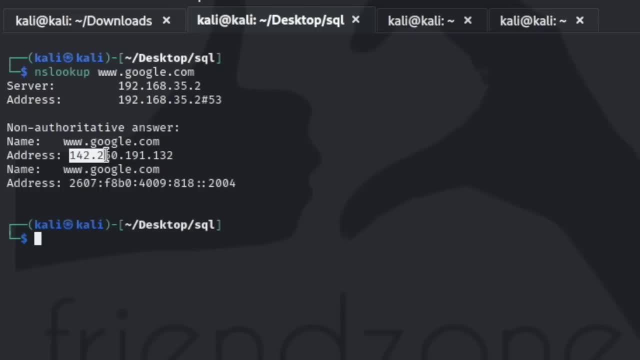 And it's going to tell you their IP address, the domain name. You're going to get the IPV6 name back and it's going through port 53. And so this is a tool you would run if you see port 53 open, same as dig, And you can get just a little bit of information back with NS lookup. So you'll hear about this and you will definitely see it in the future. This is what it does, But then there's another one that you're going to hear about and see regularly, And it's who is and NS lookup. 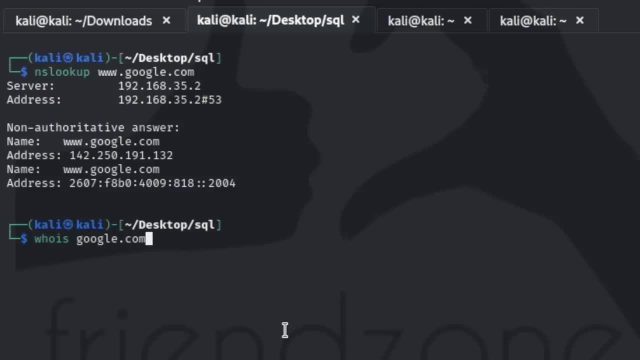 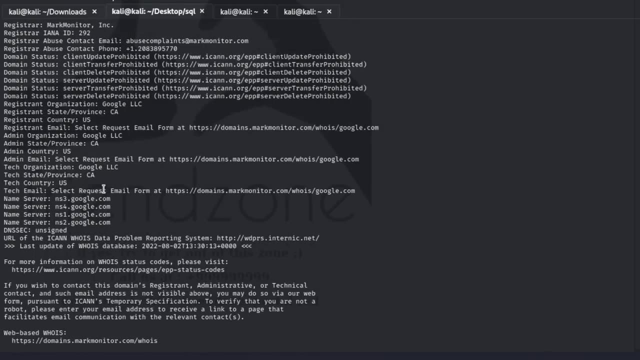 And so if you type in whoisgooglecom, you're going to get back a whole bunch of information, And if you're ever doing like a penetration test, this is actually a good one to run, because sometimes you can get back email addresses and a phone number and things like that about the company, But you can find out a little bit more about the company. So right here you see they're using the Google domain servers right here, which isn't that surprising, being from Google. But if you look at this right here, whoisgooglecom- 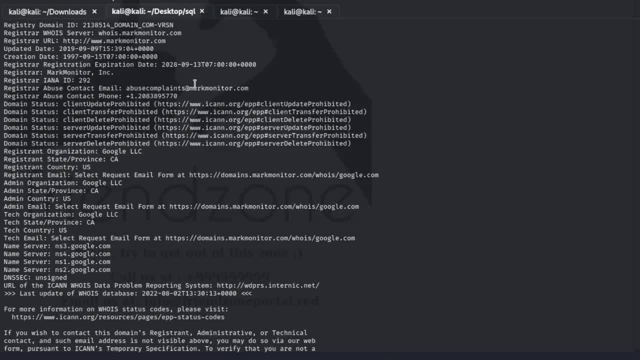 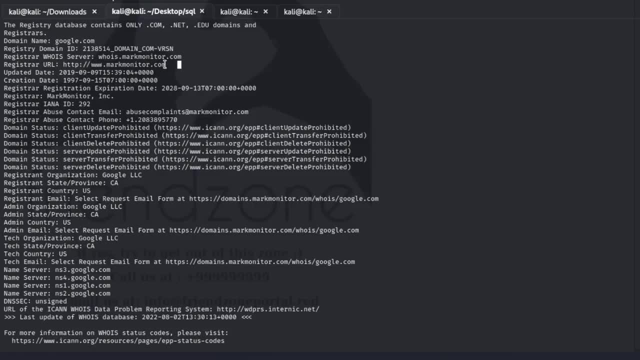 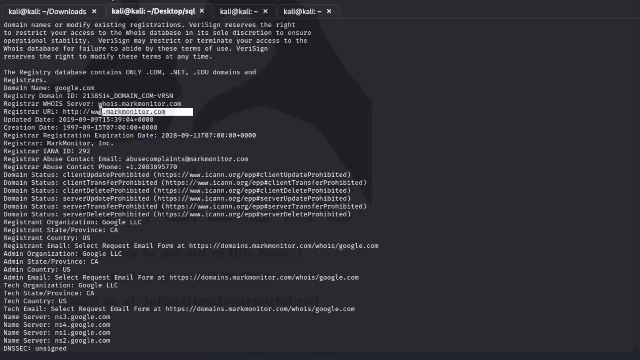 is Google registered with. It's not even registered with Google domains, which is kind of ironic that Google does not have their own domain name registered with themselves. I'm guessing they must trust this mark monitor more with security than they trust themselves, which I mean is saying something. I think Google should probably switch that. But anyway, if you know why they're using mark monitor instead of Google domain names, then you can feel free to let me know. 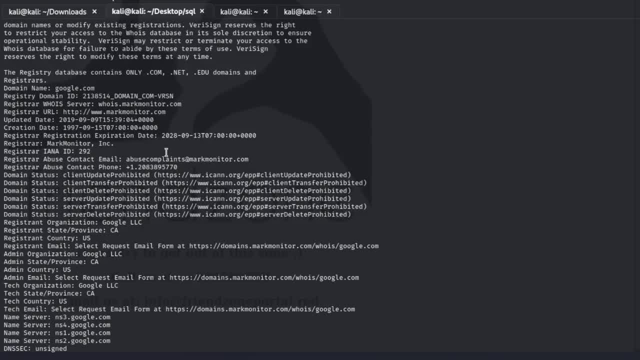 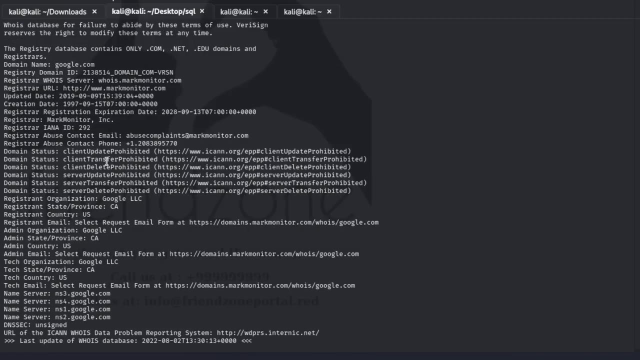 In the comments. maybe they're just using it just because they've never changed it once Google domains came out. Anyway, this is who is and it just tells you more information about the domain name and where it's registered and the kind of the security behind it and who's running it And you can look up to see if there's any vulnerabilities or anything like that. You're probably not going to find a whole lot from who is other than just about the domain name, where it's registered, who's registered with an IP address and basic information. 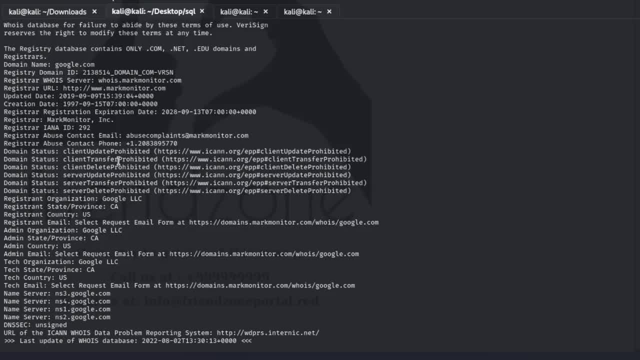 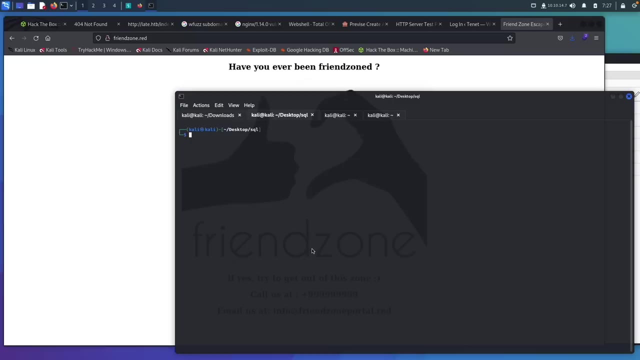 Like that. So these are two tools that you're going to hear about for sure in the future and would be worth remembering, But I don't use them all that much because I don't find them to be that helpful. I wanted to let you know about them because you will see them and hear about them in the future, And now you know what they are and what they do. Another tool that would be worth your time investigating is the harvester. It looks like this, And this tool will go out and look for other 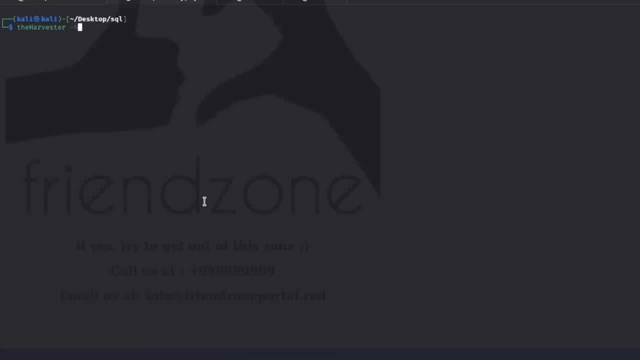 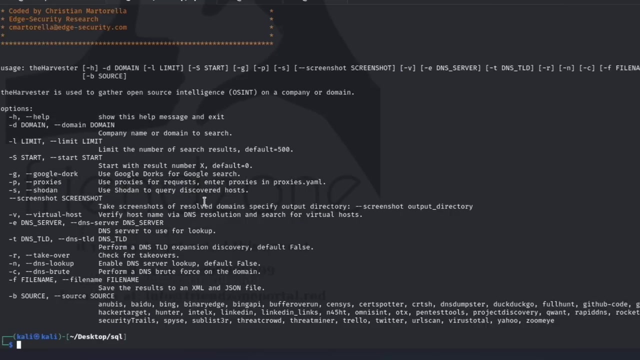 domains and subdomains And it will also find email addresses- if you're a penetration tester, for you to try and target. And the usage is really pretty simple: You just type in the harvester and then you would pass in a domain with the dash D and then you can pass in the source that you want to look for something. So you would just use domaincom And then, let's say, we wanted to use Google. You can. 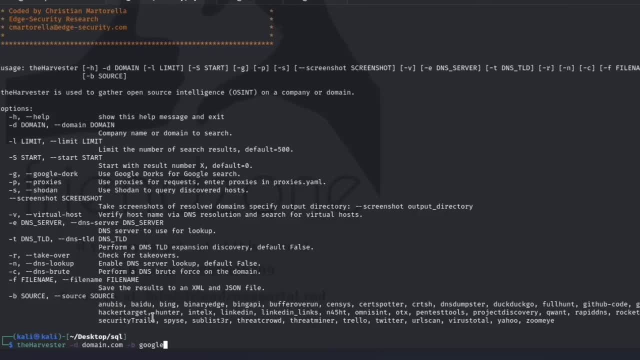 put in a dash B and then Googlecom or any of these other options down here for the source, And it will go out and it will try to look for domains and it will scrape all of these search engines for subdomains, email addresses and things of that nature. So the harvester is a penetration testing tool that you're going to hear about from time to time, And it's one to be aware of and know that it exists. You're probably not going to use it in any way. 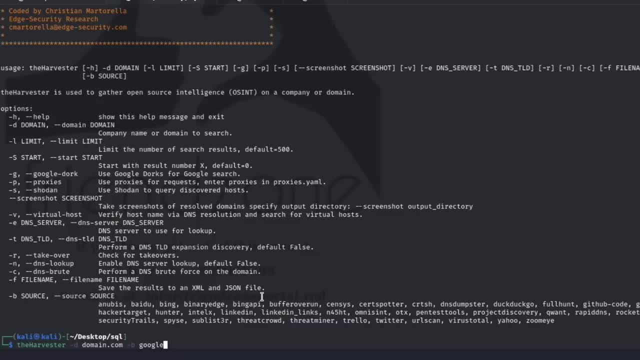 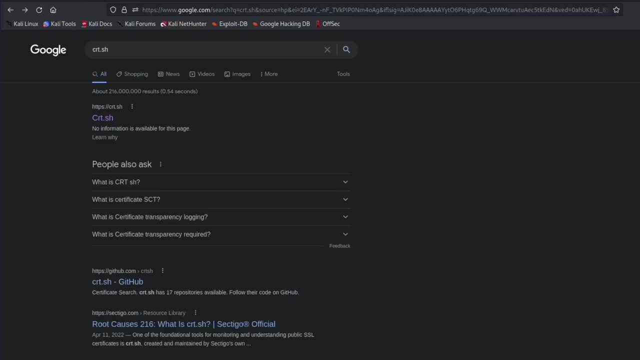 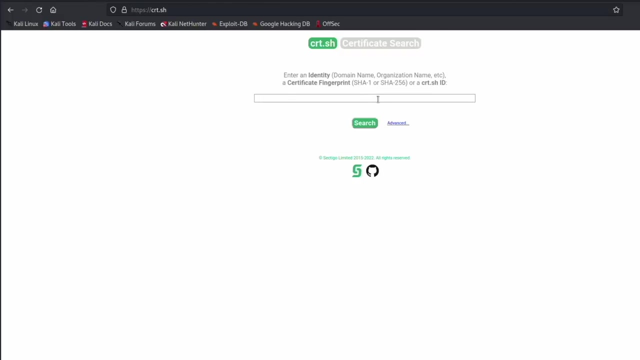 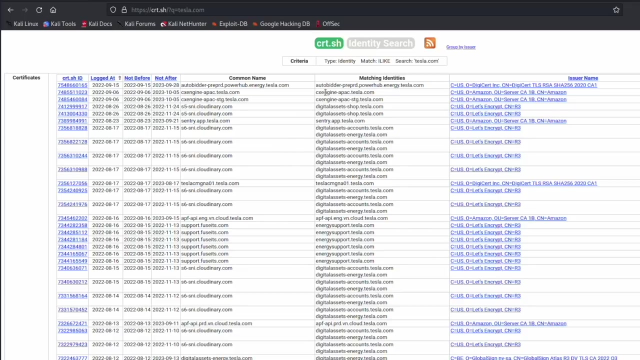 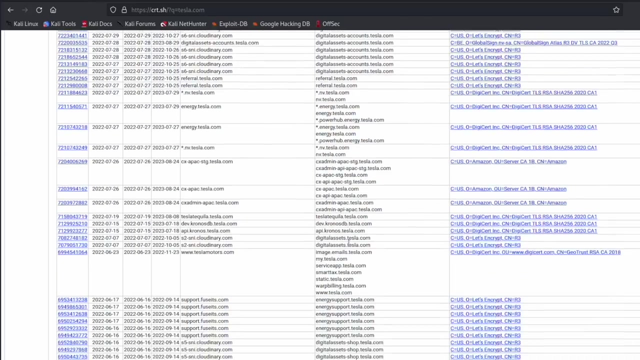 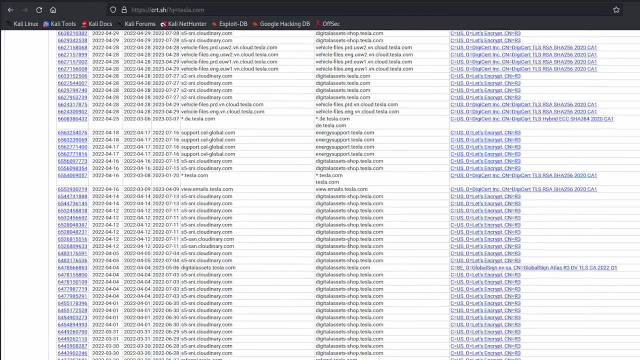 You're probably not going to use it in any pursuit of certifications or CTFs, but it is a really great recon tool and one you should know about and be aware of. So we'll go ahead and open this up and I'm going to type in teslacom and we can hit search and look at the subdomains that it pulls down. And you're interested in this middle row right here because if you look at this closely, you can see these subdomains right here for teslacom, And so this will give you a bunch of subdomains for you to go out and look and test for bugs and see if there's any information out there or anything you want to test against. 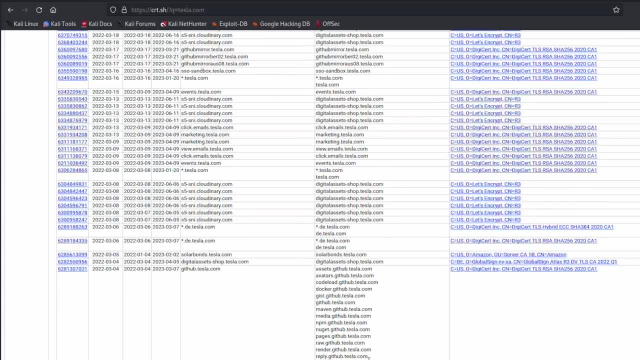 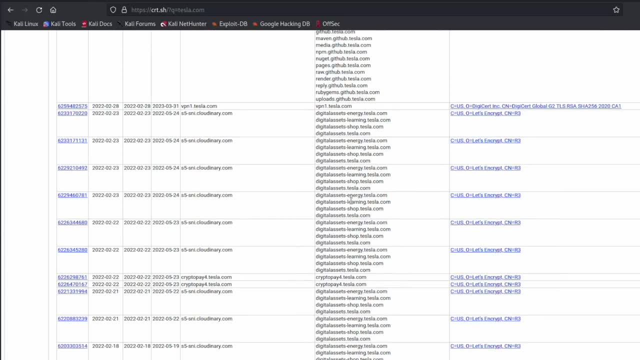 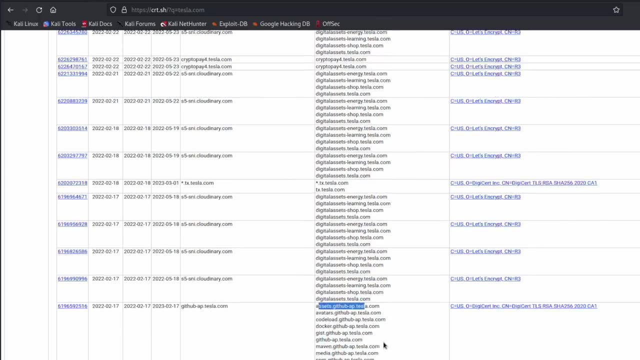 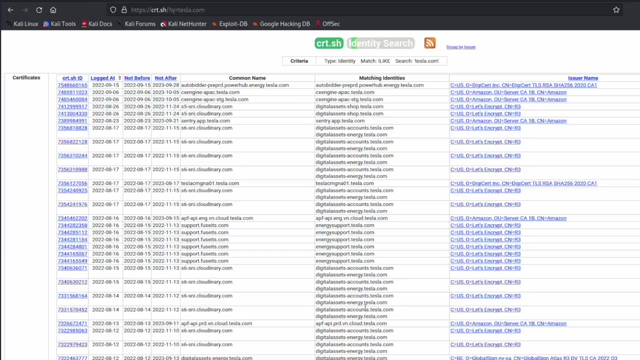 When I look at something like this, one of the first things when you have so many subdomains is to see which ones look specifically interesting to you, And then you can go and check those, but always make sure that they are in scope. So you'd want to make sure that this assets, first of all, is owned by teslacom, and then you'd want to make sure that it's in scope. And second, a tip is to look for the dev, Typically these dev sites and these dev subdomains right here. 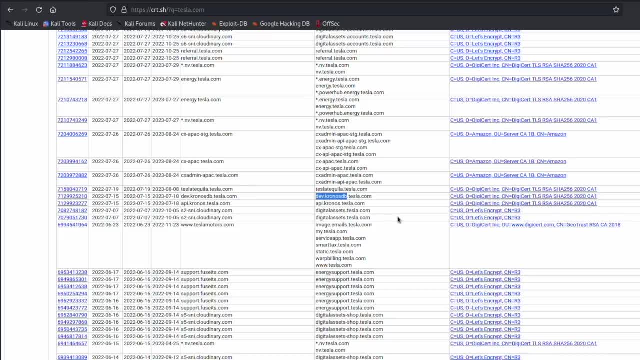 Are going to be hosting information or new software or new code before it goes live on the actual main domain, And so these devs are always something good to look at. Another one that's good to look at is look at like admin portals and see if you can get into any of those, or fuzz for directories. 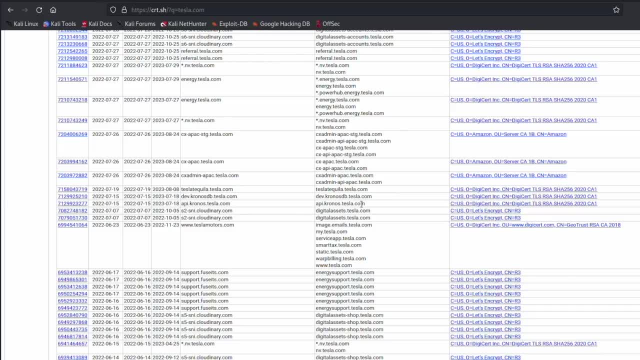 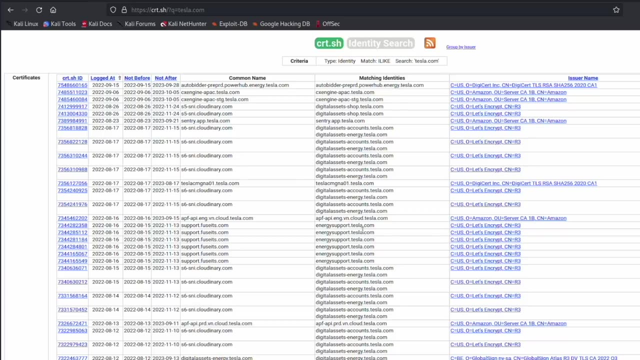 Because there might be something there that you might need authentication for in order to see, but you can access it without being authenticated. So the devs, the admins Pages, like those, this API would be interesting to look at, And so you can come in and look at all these subdomains. If a mass and sub lists are not pulling back enough subdomains for you, you can always come to srtsh and check this out. 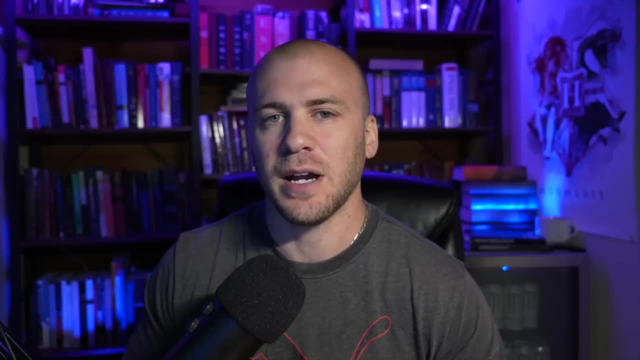 So in this video, what I think we're going to do is I'm going to show you how to grab all of the different possible URL targets for you within a bug bounty program, And then we're going to start to narrow it down to the URLs that are actually responsive, And then the ones that I think will be helpful for you. 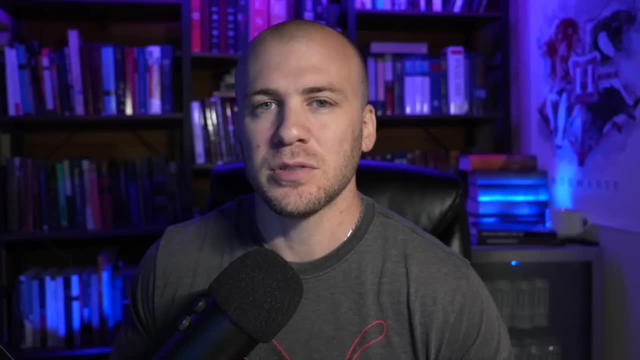 So I'm going to show you how to find the most obscure URLs within a bug bounty programs for you to target, but always make sure to remember that these URLs are in scope. that's gonna be really important. So always check that, because sometimes you'll see URLs that maybe are several years old and a specific bug bounty program has forgotten to remove them. 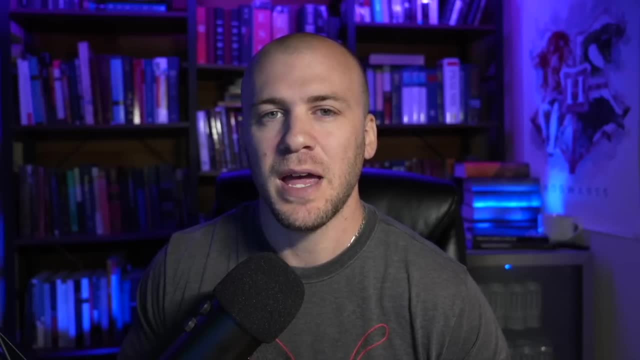 And you're going to think this is a really great target, but it will end up falling into the category of out of scope. So make sure, as you go through your recon phase, to only target URLs that are in the bug bounty programs- any scope. this is something that I really struggled with In the beginning. I would end up out of scope. 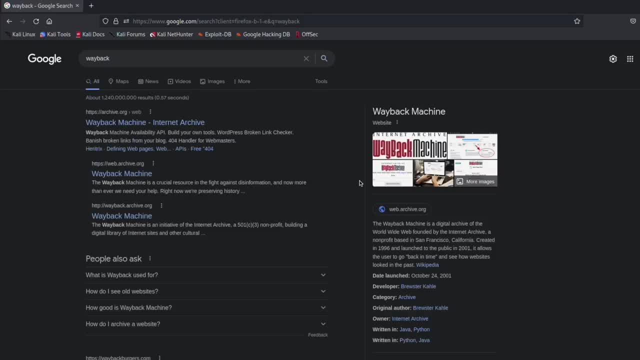 so you don't want to do that? All right. there is something called the Wayback Machine, which is really cool, and we're going to be utilizing this, and thanks to Tom Nom Nom for making a Wayback tool that is really going to save us some time, as well as a couple of other tools. So if you want to, 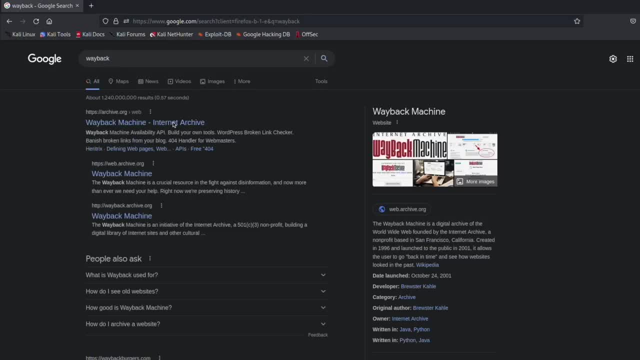 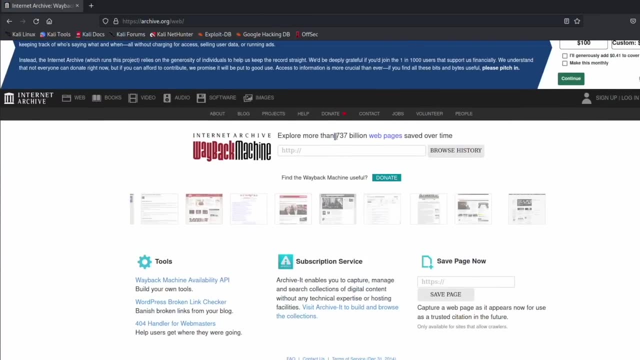 check this out online. you can type Wayback into Google and you'll be brought to the Wayback Machine and we can come right in here and it tells us at the top that it has saved more than 737 billion web pages. and let's go ahead and check out what this does. So we can type in yahoocom. 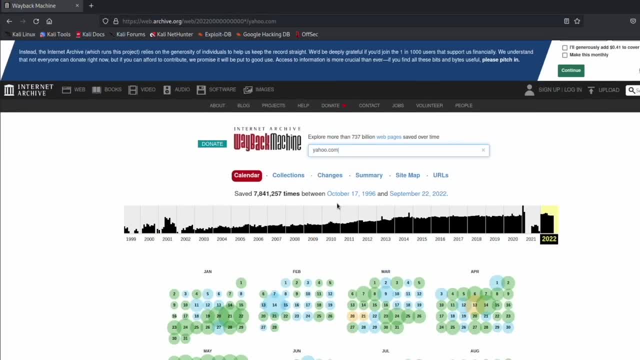 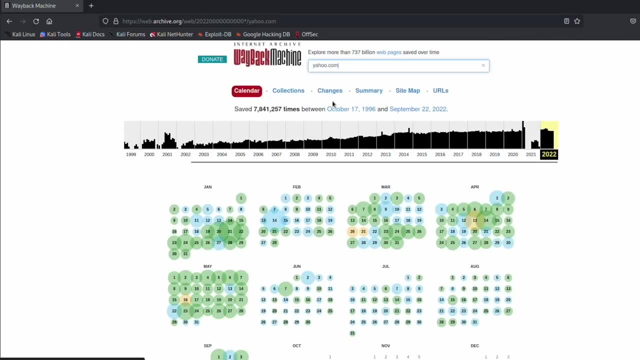 and it's going to give us all of the screenshots that it has taken of yahoocom from October 17th 1996.. So this is why it's called the Wayback Machine, and it doesn't just take screenshots, it'll actually store the URLs and you can go back and check out the timestamps. 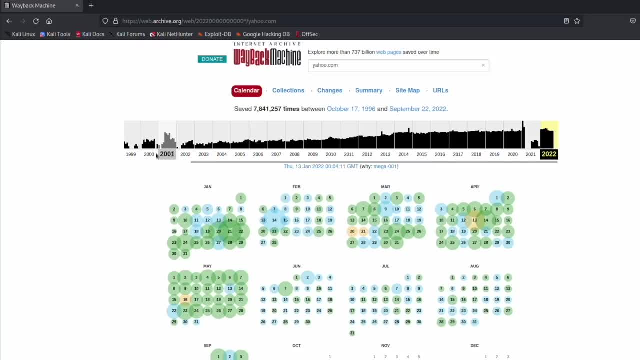 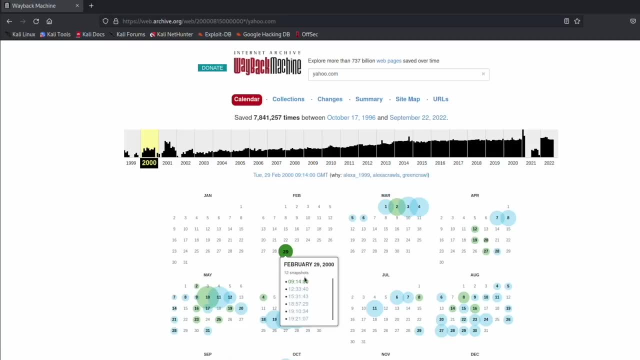 And it'll show you what the web page actually looked like at that time. So if we click back here to the year 2000 and let's say we want to open up February 29th 2000, we can do this, So we'll. 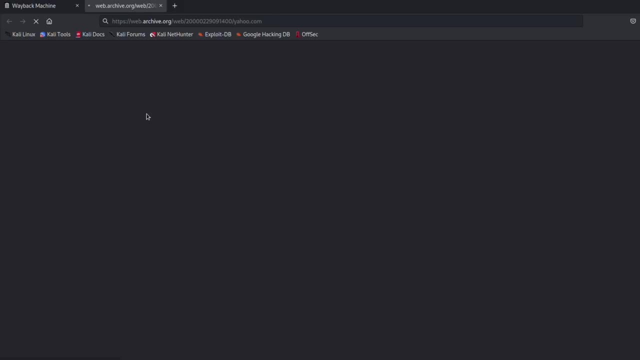 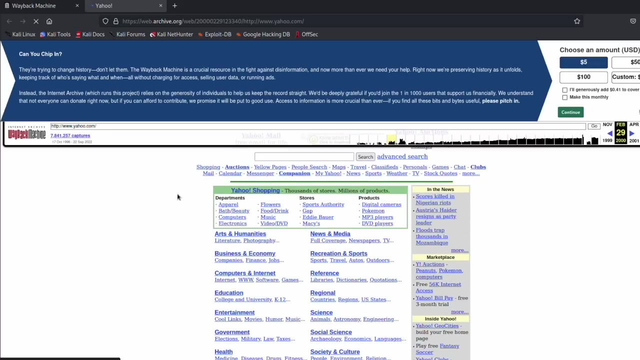 right click, say, open in new tab, and it's going to render what that page looked like for us from its archive, which is pretty cool, And so this is what the main page looks like, and some of the HTML might not render quite right, but that's okay. So we just really want to grab the URL and a lot of 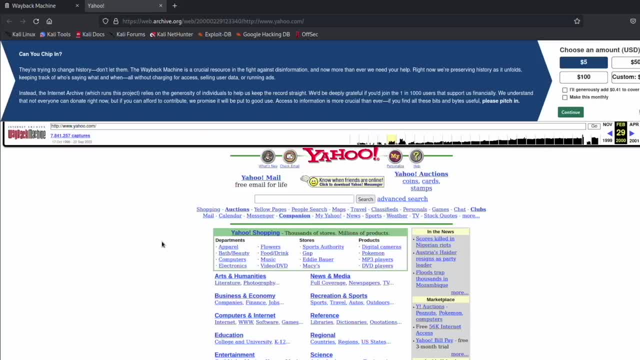 the links. Well recap, the first thing we want to do is we want to be sure that all the web pages that were available at that time are still being hosted on our specific target and they have not removed them, which does happen. programs and companies will be hosting up specific subdomains And then, after a 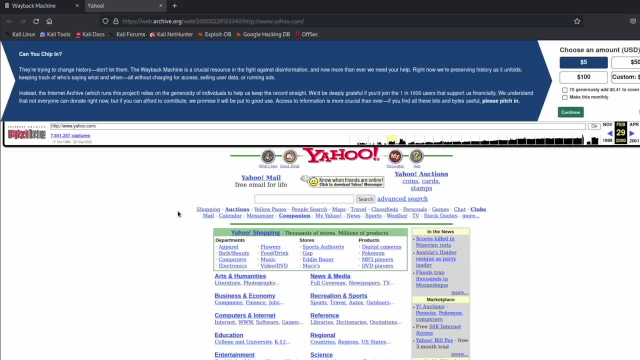 while that subdomain is no longer in use- And this is really common with with blogs on large companies. Say, PlayStation comes out with a new video game, they'll create a sub domain all about that video game, and then they will forget about that video game, and years pass by. 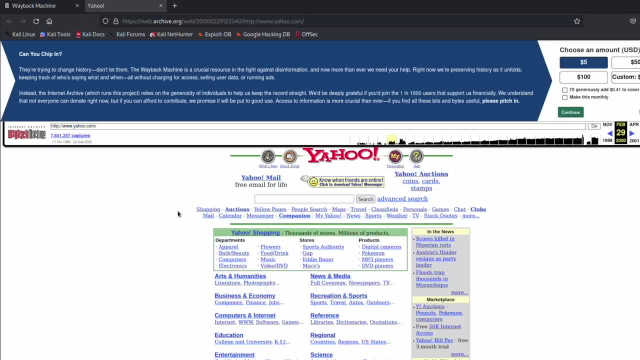 subdomain will still be up and it won't be updated and it might be vulnerable to new exploits and CVEs, And so that's why we want to look back into the past and see if we can grab any subdomains or URLs or links that may lead us to bugs that other people have not checked for within those. 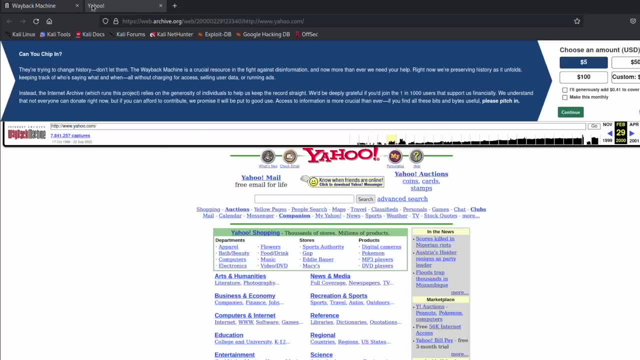 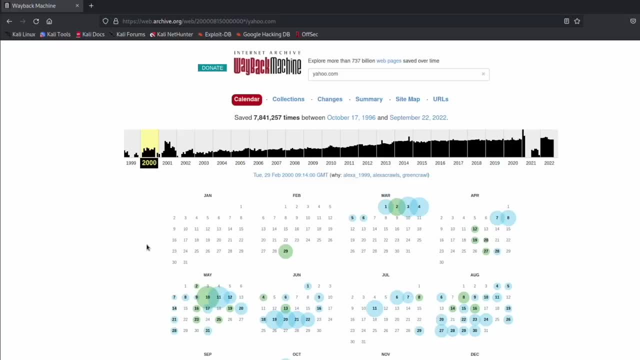 forgotten subdomains and links. So this is the Wayback Machine. You can come in here and get a feel for how it works, And now we're going to go ahead and install the Wayback tool by TomNomNom. So what you will do is come to Google and you're just going to type in Wayback TomNomNom and it's. 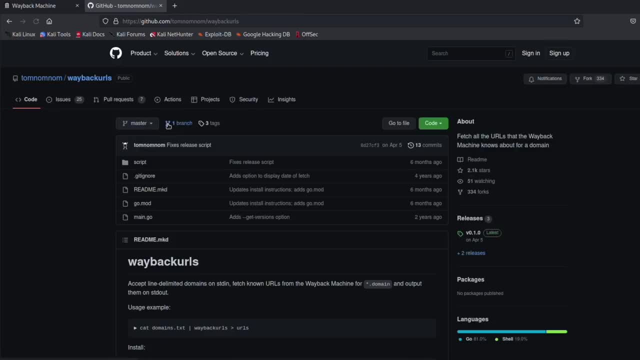 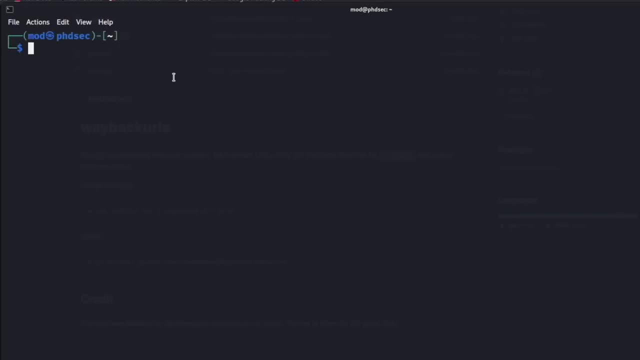 going to be the first tool here for us, And we're actually going to have to install the Go language before we're able to install this. So what you can do is open up a terminal and come in here and just type in Go And if it doesn't turn green, then you do not have the Go language installed. 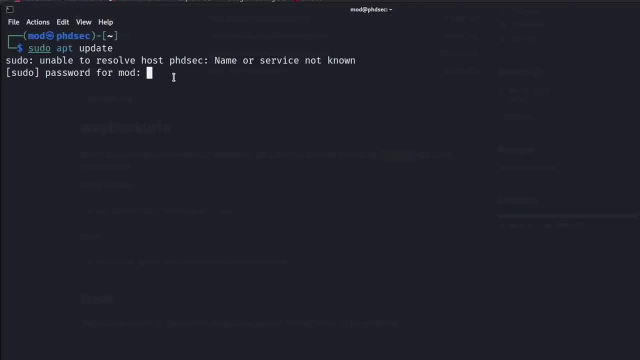 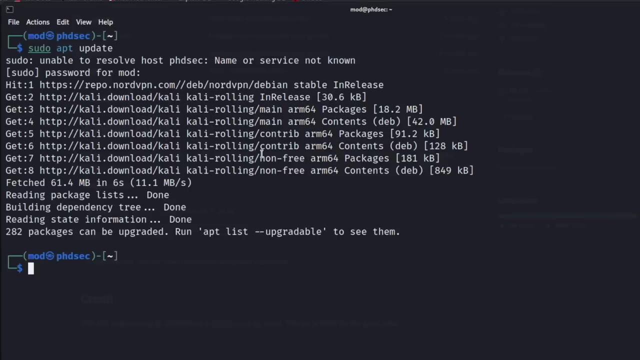 So what we're going to need to do is run a sudo apt update, just like this, And let this update, And if yours doesn't update or gives you some kind of warning, you might have to run a sudo apt upgrade and then run the sudo apt update. So now that we're all. 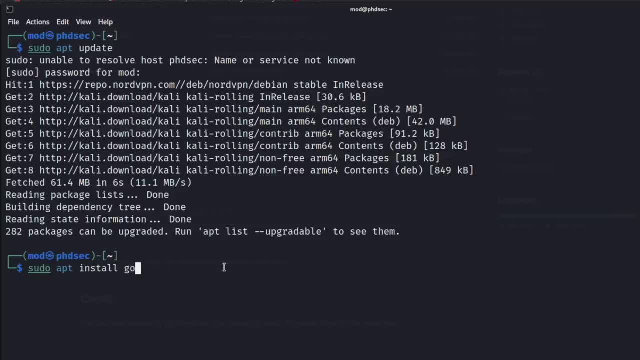 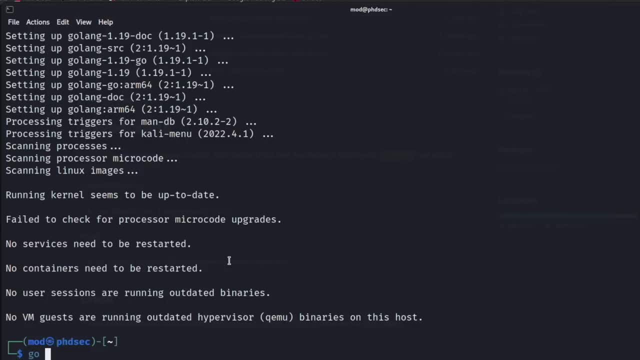 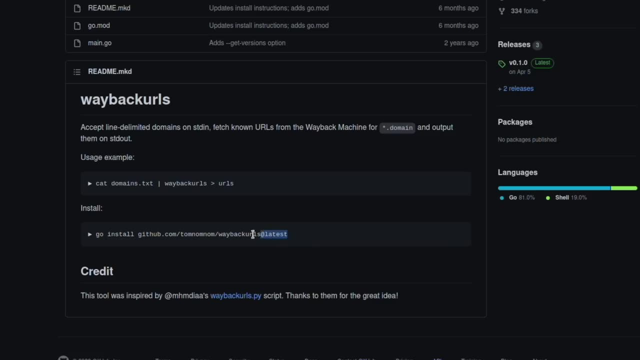 update. we can run sudo apt install Go lang, like this And we'll say yes. And now, if we type in Go, it should turn blue for us or some other color, meaning that we have the Go language installed. So we can come back to the TomNomNom site and we can just highlight this and we can just copy this: 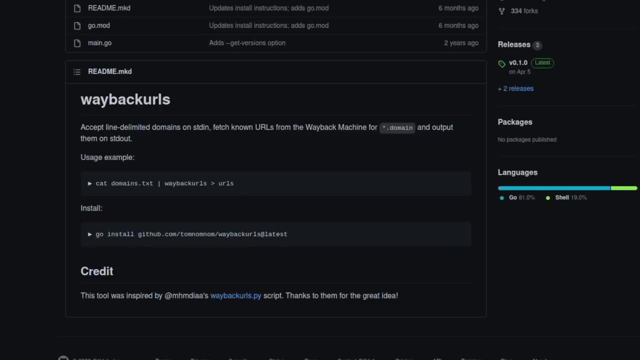 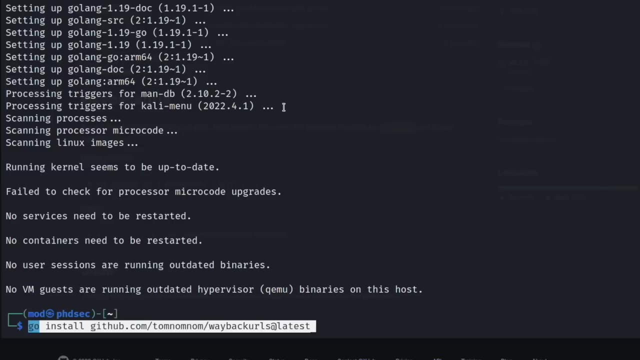 right here And we can just copy this right here, And we can just copy this right here And we can paste this in, And I think we're going to have to run this as a sudo. Okay, So when I ran it with 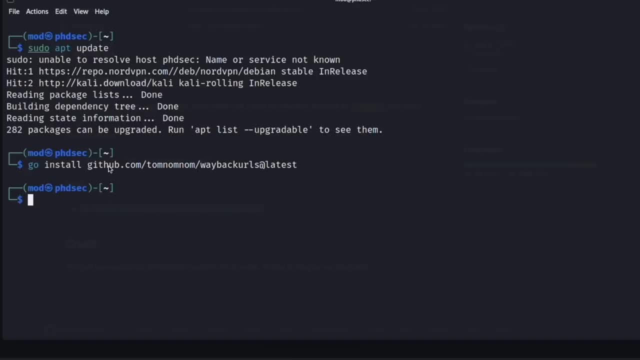 sudo. it didn't work for me. So when it actually installs the proper way, it's going to run just like this and you're going to see nothing in the output. And then what you're going to want to do is cd over to the Go bin And it's going to look like this. Then you'll hit enter and you're going. 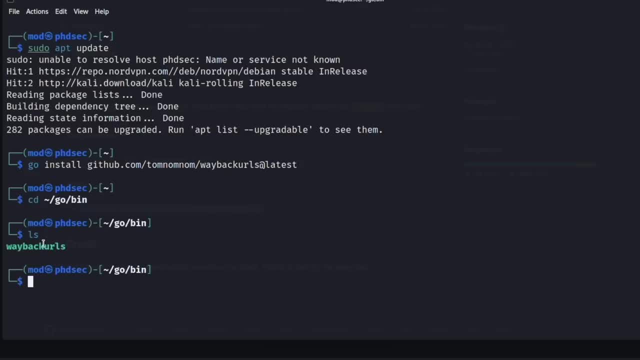 to automatically come into the directory like this: And then, if you ls, you're going to see the directory that you installed And then you're going to see the directory that you installed And then you're going to see the way back URLs within the file here And the way we're going to. 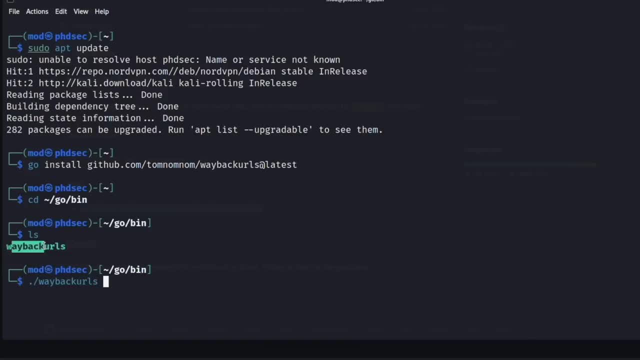 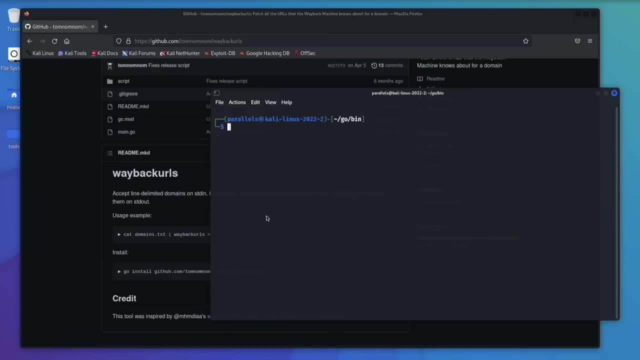 run. this is with this dot slash and then the name of the tool that we want to run. And just so you can see what it looks like, you can run a dash H and see the output here. Okay, So my other VM was freezing, So I went ahead and opened up a new one, which is just fine, It will all work the same. So. 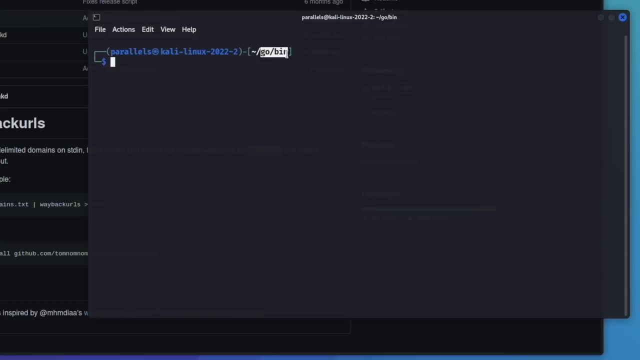 I went ahead and installed it on this new machine and you're going to find it in the Go bin, And so if I run an ls, you're going to see I actually have a couple other tools in here, but I'm going to show you how to install those in just a second. But this is the tool you just installed, right? 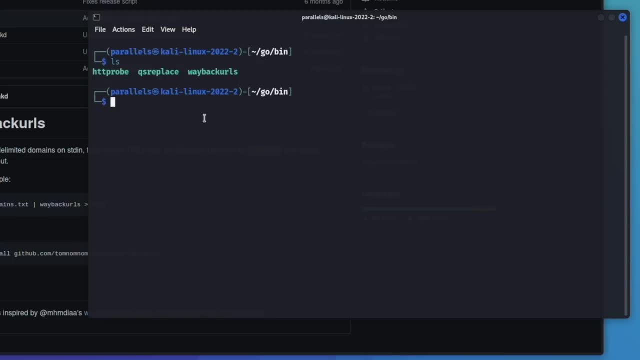 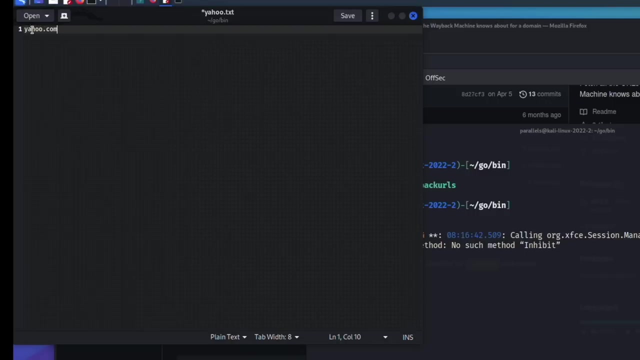 here. So the way we're going to run it is really simple. but first we need to create a target domain for us. We're going to gedit and I'm going to gedit, yahootxt, And we can just type in yahoocom And this is going to be our domain, that we target And if there's any subdomains in here, 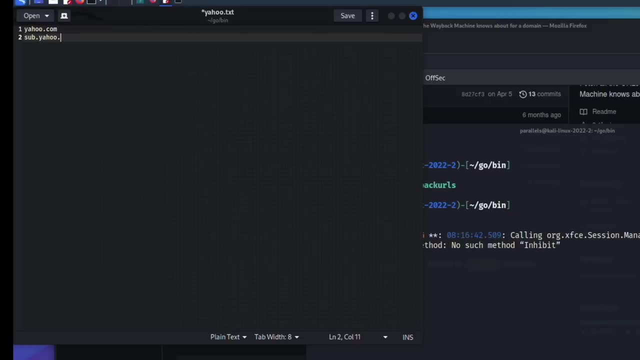 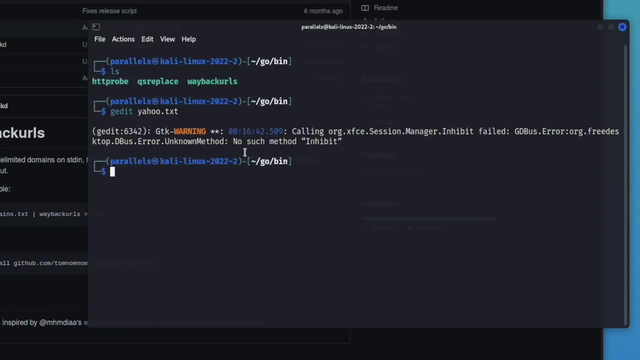 you'd want to paste in like a subyahoocom And I'm going to show you how to grab these subdomains here in just a second. So we're going to leave it just like this. We will save And now we can run the wayback URLs tool And while it runs, I'll show you how to grab the subdomains. 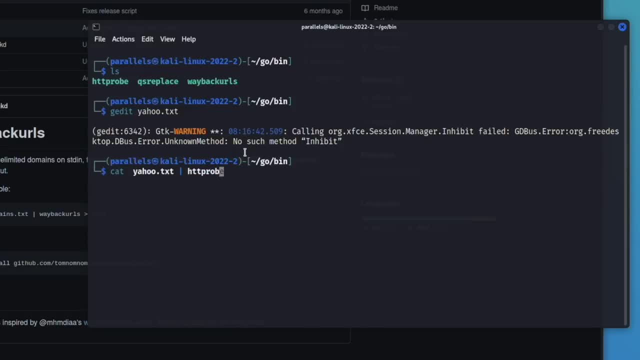 So what we'll do is cat that file that we just made and we're going to run it into the wayback URLs, just like this, And then you can actually save all of those into an out file by pointing, and we'll let this run. And now, while that runs, we're going to go ahead and grab some subdomains. 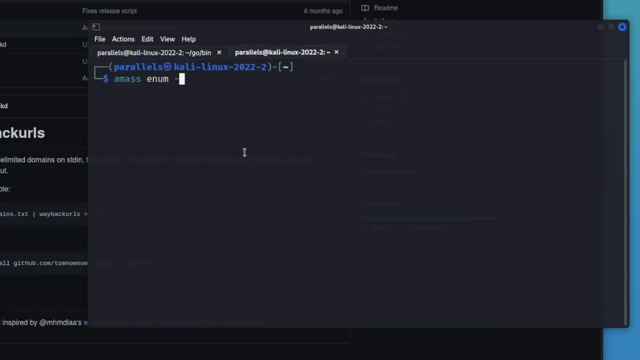 So we're going to run an amass enum dash passive dash D yahoocom, And this might take a second, and it's going to give us a ton of subdomains that we would want to run the wayback tool on, And so our goal is to find really old pages on these subdomains from the wayback tool. 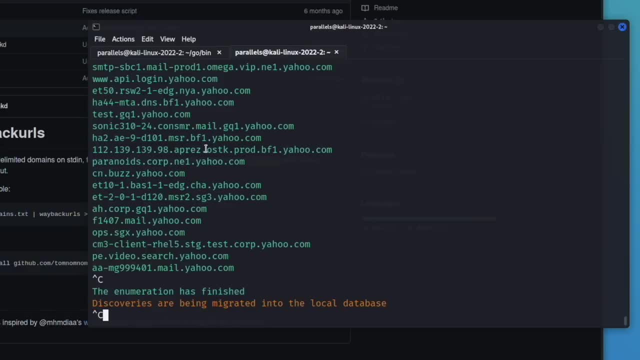 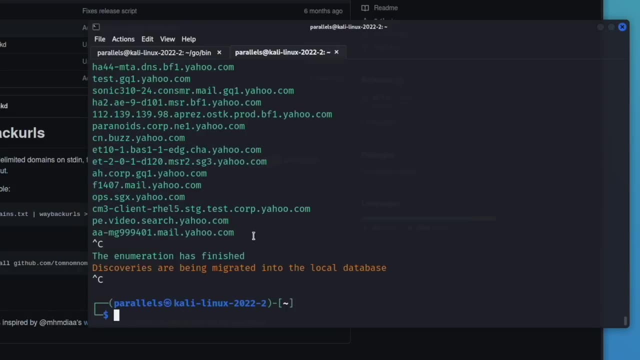 that are going to have some vulnerability. So we'll go ahead and close out of this, this, and what we're going to end up doing is just grabbing like 10 of these because I don't really want to run the way back to on all of these. you would run it on these if you were actually looking. 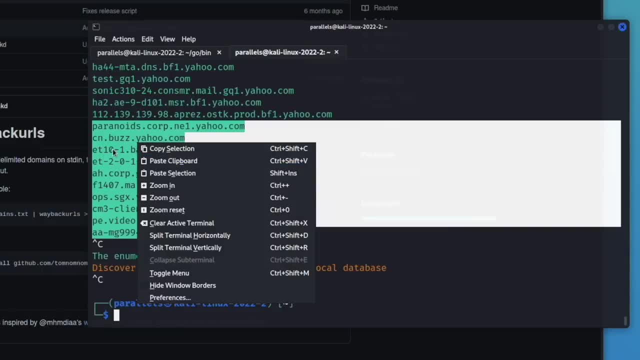 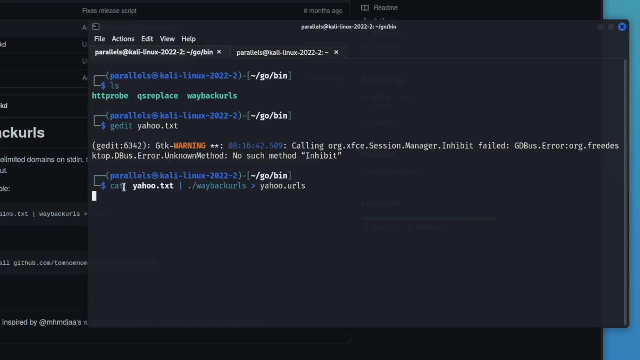 for any vulnerabilities within these pages, but my goal is just to showcase the tool for you, so we will copy some of these urls and come back over here, and this is still running, so, oh, it just finished. so what we'll do is: now we can gedit our yahootxt like this, and what you would do is you: 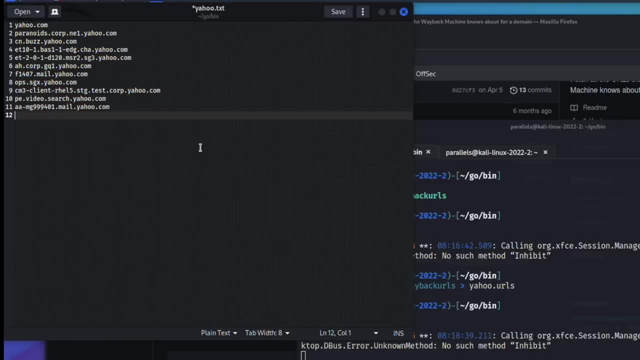 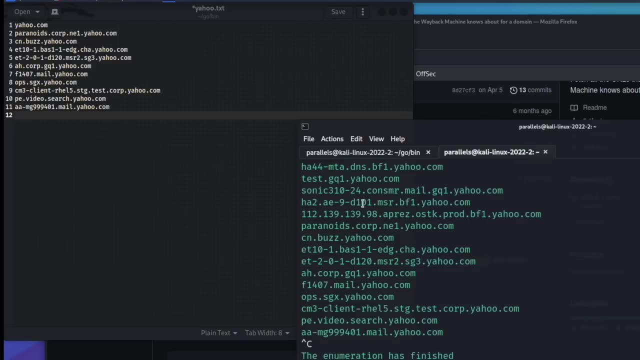 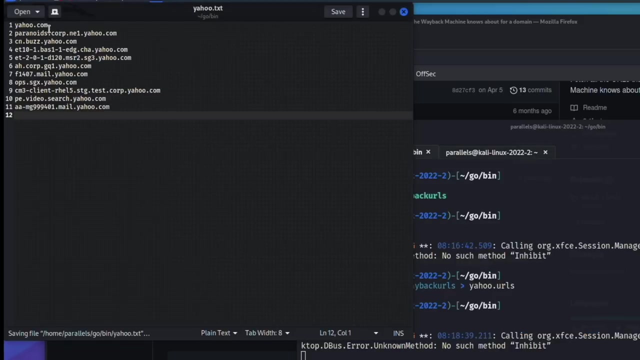 would run all of these subdomains in a file, just like this, so you might want to save this amass right here into an out file so that you don't have to copy and paste. but that's okay that we're not going to do that and we're going to save this. and now if we ran it, it would run and grab the valid 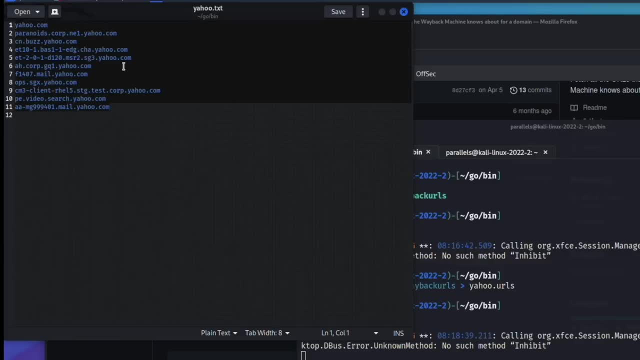 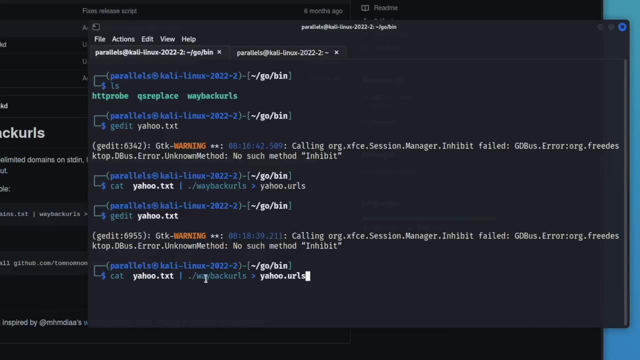 urls for all of these documents, all of these subdomains for yahoocom. so now that we have that saved, what you would do is you would run this, the exact same way you did right here, and it would run this wayback tool on all of those subdomains that we just put in that file and it would save them over here in the urls for us. so 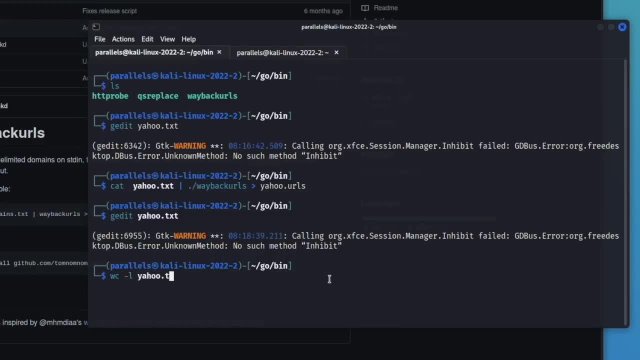 what i want to show you is, if we run a word count right here on this yahootxt, it's going to show us that's the file that we made, so we'd want to run it on the urls and it'll show us that we have more. 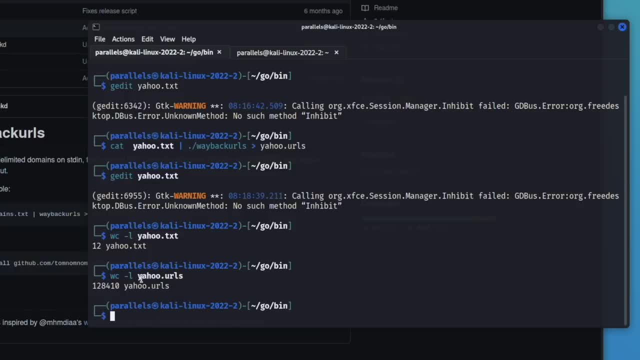 than 128 000 valid responses from the wayback tool, and we don't necessarily want to visit all of these 128 000 urls. and if we ran the wayback tool with all of these subdomains, i bet we would have well over a million different urls, and we don't really want to check all of those. so now we want. 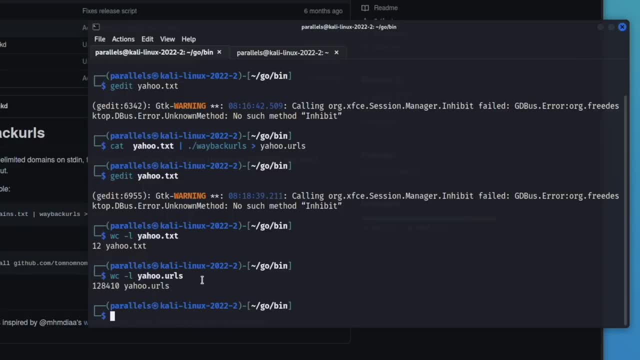 to see which ones resolve in order for us to know which ones to target. so what we would do at this point is: you're going to run a sudo apt- install http probe. you're going to run a sudo apt- install http probe. and you're going to run a sudo apt install http probe. 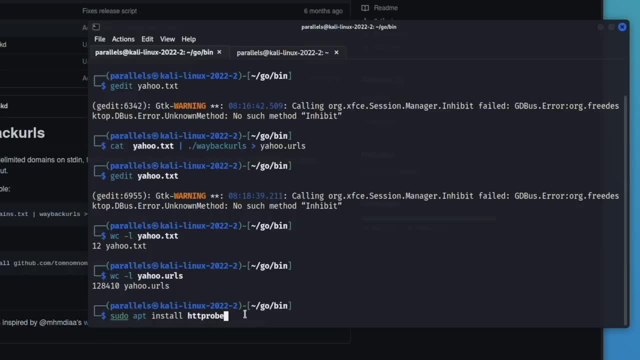 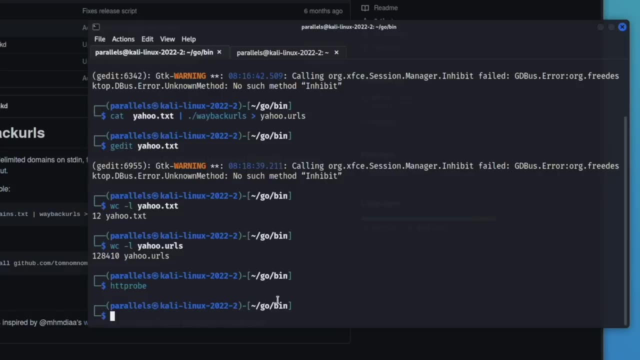 and it's going to look like this. i already have it installed so you can go ahead and run it and then, after you run it, you can type in http probe to make sure that it's installed, and it should turn blue for you, just like this. and the way we run it is the same way we would run the. 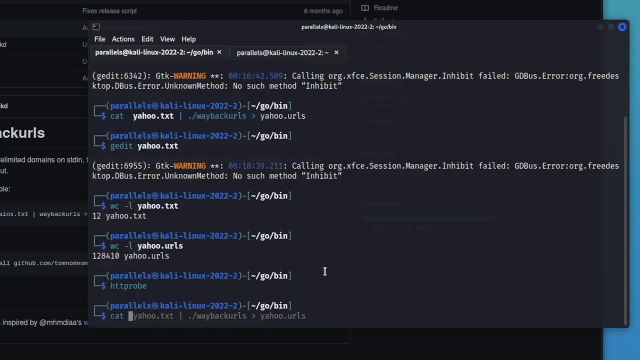 wayback, just like this. so we're going to go ahead and cat out our yahoo urls, just like this, and i'm going to actually delete the valid urls. you can save it into an out file if you want. i'm not going to, i'm just going to let it spit out to the console and then cancel it. 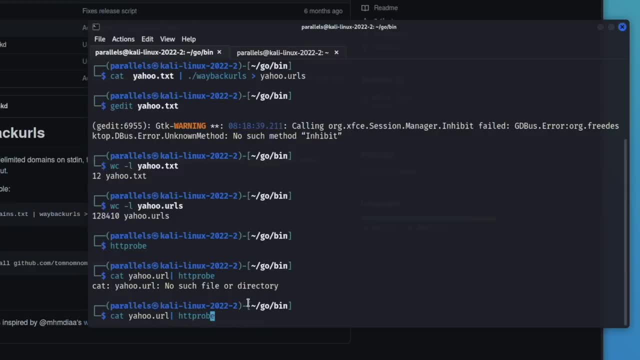 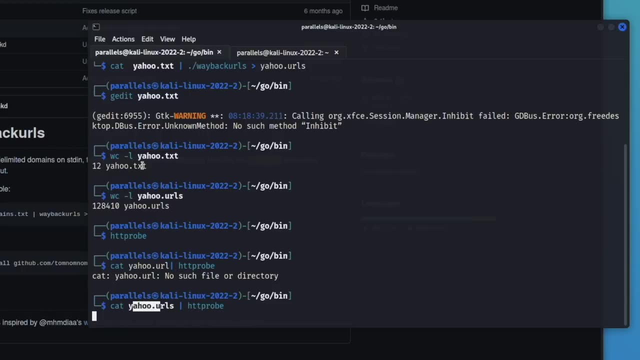 and so we would go ahead and run this- and i think this is urls with an s like that- and it's going to go ahead and start running this- all of those 128 000 urls that we pulled down from up here- and it's going to start printing the valid ones out down here in the terminal for us. i'm going to go ahead. 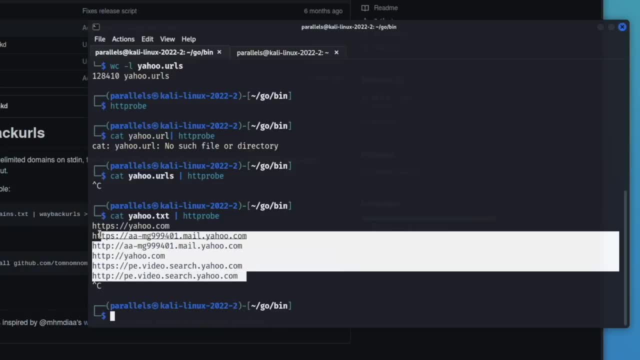 and cancel that. the valid urls are going to get printed out just like this into the terminal, or you could save them into an out file and then, once you have the valid urls, you can start to look through which ones you think are juicy and you want to target. one other thing i want to show: 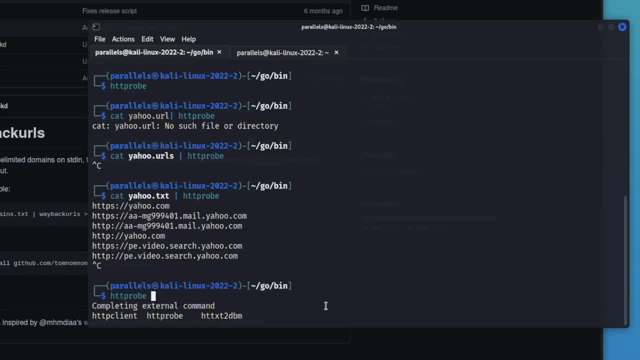 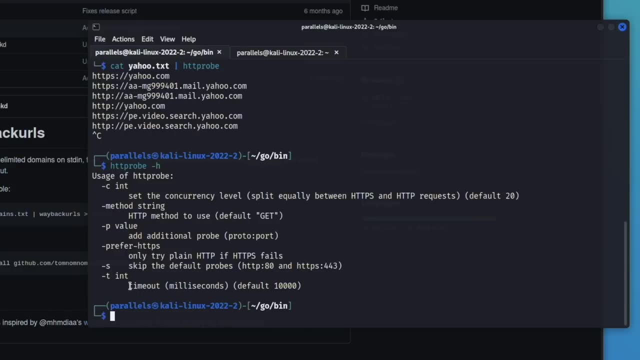 you is, if we type in our http robe, just like this, and we run a dash h, just like this, you can start to see if you want to give them a timeout in milliseconds. so i think there's a thousand milliseconds in a second. so if you wanted to run an http probe and you didn't actually want to, 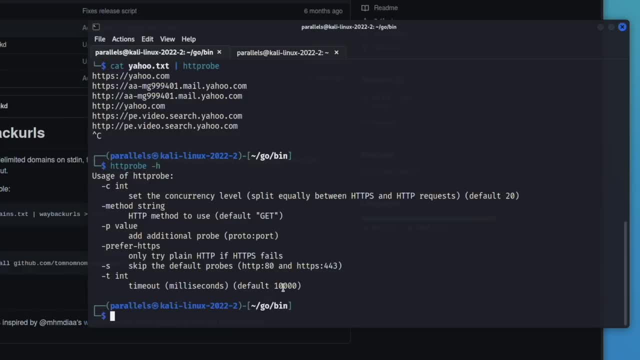 wait for it to try and resolve each one for the default event. then you could just go ahead and wait 10 seconds, which is kind of a long time. you could change this and see if the web url resolves in like a second. that's probably what i would do. so i would run a dash t and i would say 1000. 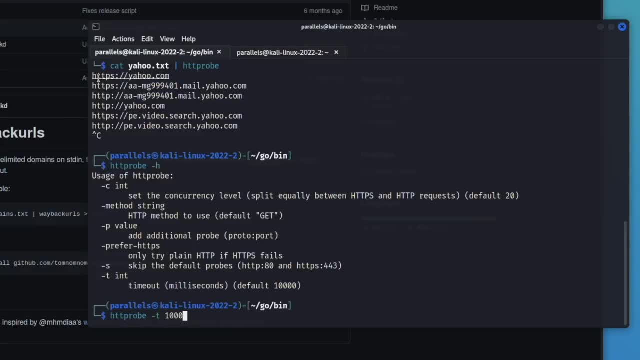 instead of 10 000, so that way it only takes a second before it moves on to the next url. so if it went to this url and it didn't resolve by default, it's going to wait 10 seconds to go to the next url and if you're running over a million subdomains that's going to take forever, especially. if it didn't resolve, so i would run it with a thousand. so that way it's one second. so if this did not resolve within a second, it's going to go ahead and go to the next one. so this is one of the most comprehensive ways to pull down the max number of urls for you to target within a bug bounty. 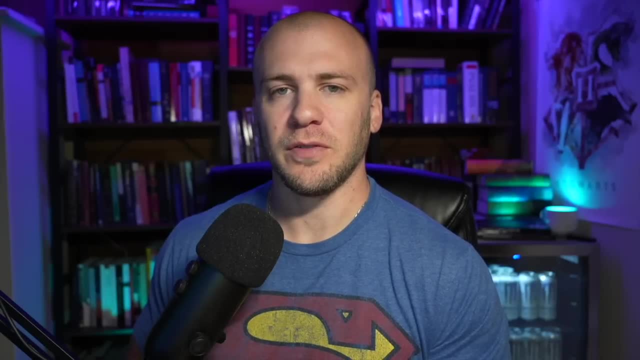 program. in this video i'm going to show you how to find subdomains which are going to be really important for you. if you do any kind of bug bounty hunting or penetration testing- because subdomains are usually targeted the least and usually what happens is beginners- just log into the main page. 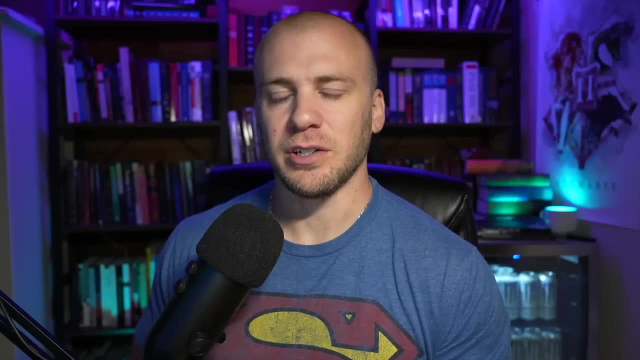 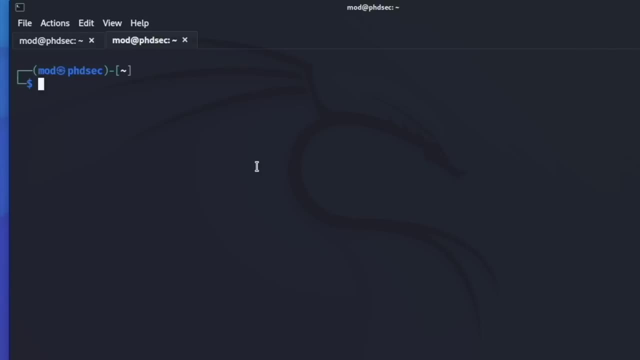 the main page and it doesn't really work out for them and they become really frustrated. so let's go ahead and jump into it, okay? so here we are. we have opened up a terminal and you're going to go ahead and sudo apt update and then you're going to type in sudo- apt install sublister. i just want to. 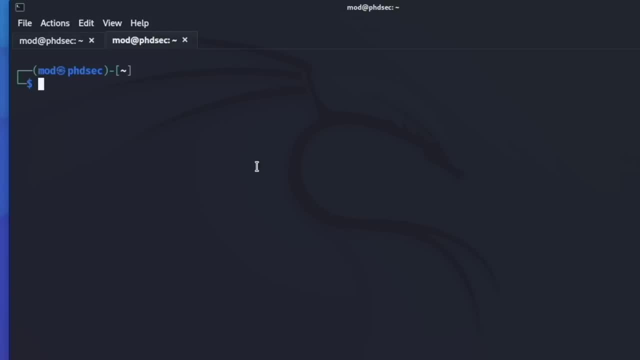 show you sublister because it's really popular and i used to use it a lot, but i've really stopped recently because it's not pulling down as many domains as i would like. so if we just type in something like sublister and then yahoocom, we'll see what it pulls down. so you'll type in sublister. 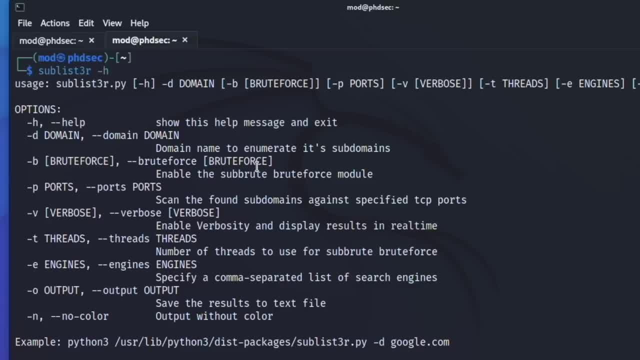 dash d for the domain. actually we can type in a dash h for help and you can see what all it's able to do. so we're going to type in a sublister dash d and then we'll just type in yahoocom and it's going to go out and search all these different search engines and then bring back. 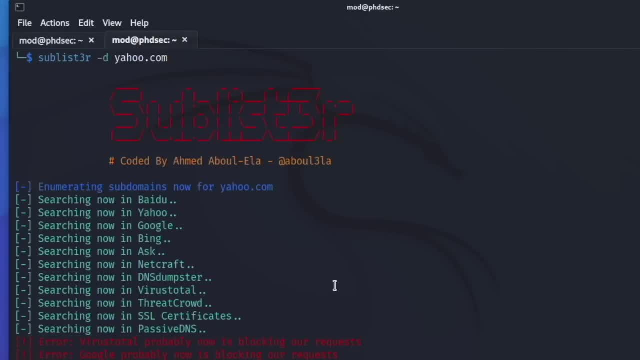 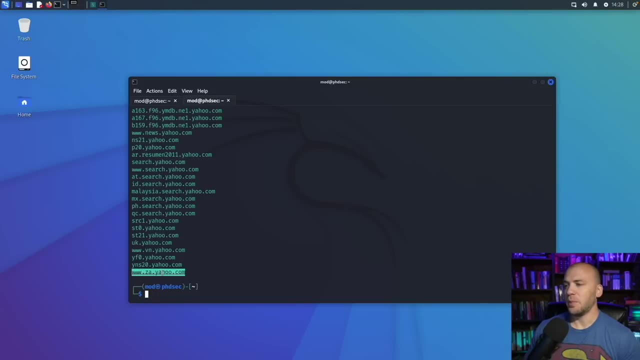 the results and remember, when you see all of these subdomains that it brings back, that you need to check to make sure they're in scope sometimes. i'll show you what i do is. i just open this up and i'll be like, okay, here's a subdomain, here's a subdomain and let's. 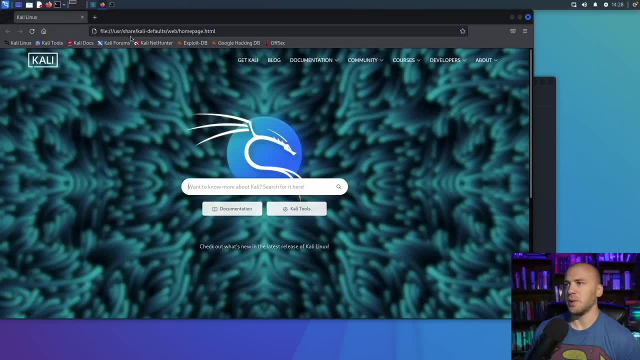 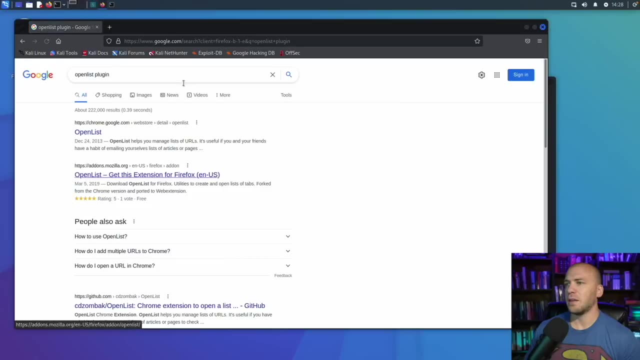 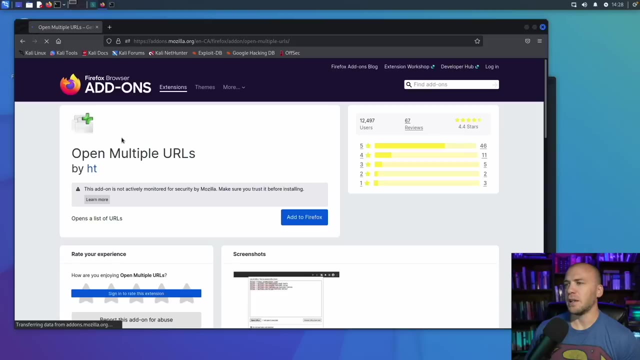 subdomains, and i'll show you what i think is the best way to do this. so if you're in firefox, you're going to want to download something called open list plugin and we want it on firefox, so we'll just go ahead and add this and it's telling you right here what this is going to do. 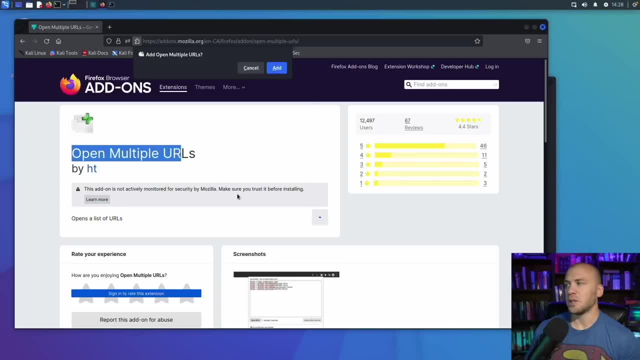 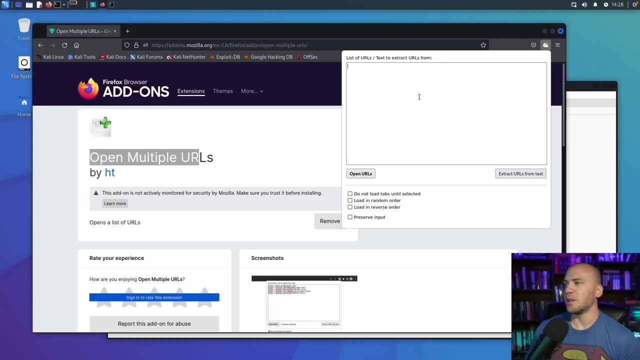 it's going to open multiple urls at a time, which becomes really helpful for us. it says: we want to add, we're okay with adding, and here it is. so we now have this right here, and what open list does is, when you have all these subdomains and you want to see what happens, you can just copy these. 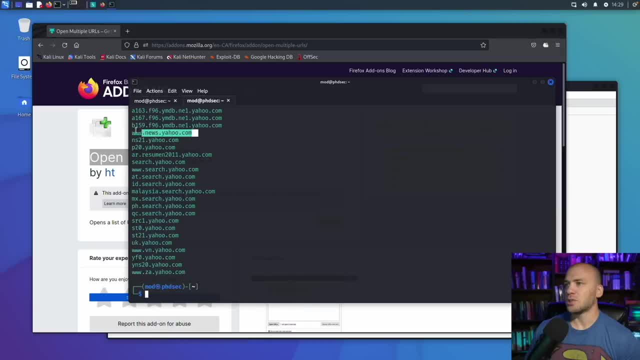 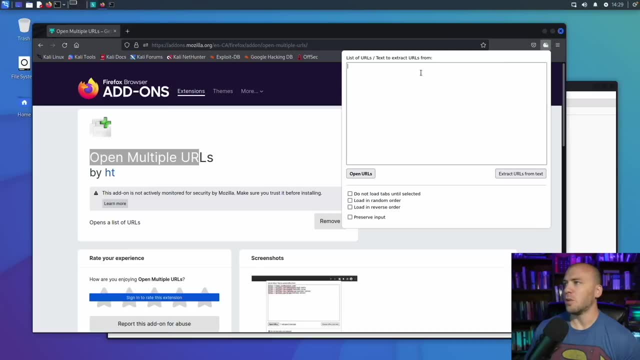 and then you can paste them in. so we'll just grab this one because i don't think it's going to have anything on it, so we'll copy this one. we can come over to open list and we can just paste in a bunch of urls. so what we would do is you'd really just copy a bunch of these instead. 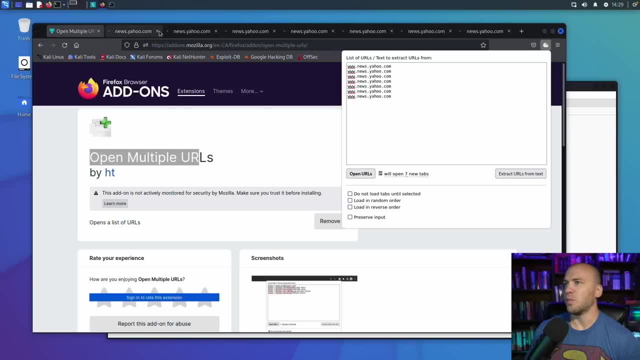 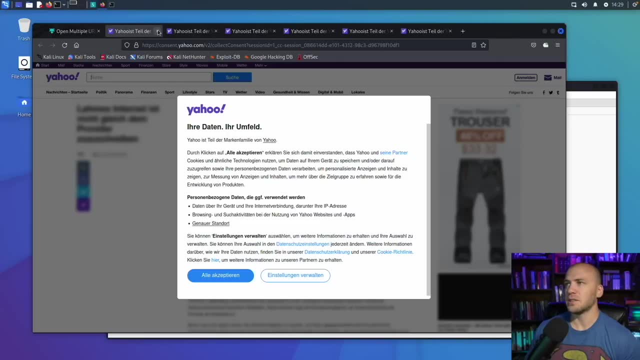 of the same one over and over, and then, when you hit open urls, it's going to open all of these tabs for you. it's going to be a lot faster than having to open one at a time. so here they are. it opened all those for us, so that's one way to check out the subdomains you do find, but that's. 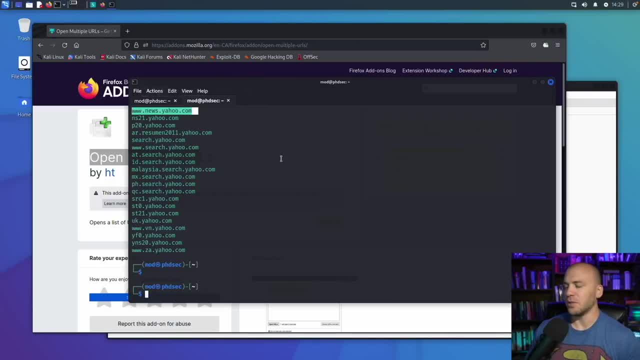 not the purpose of this video. that was kind of just an afterthought that popped in my head as we were shooting this video. so you have sublister and here's a list of subdomains that it's brought down and you might be able to say, well, that's a, that's a decent sized list, so we'll scroll through. 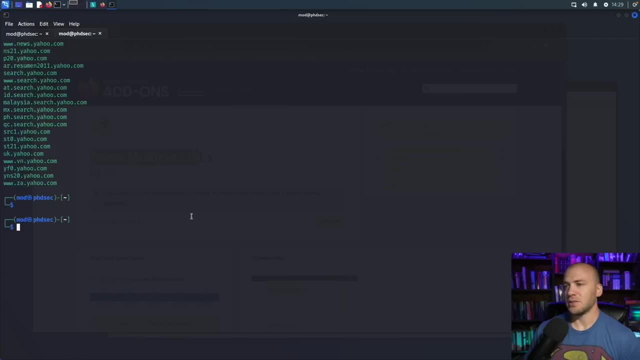 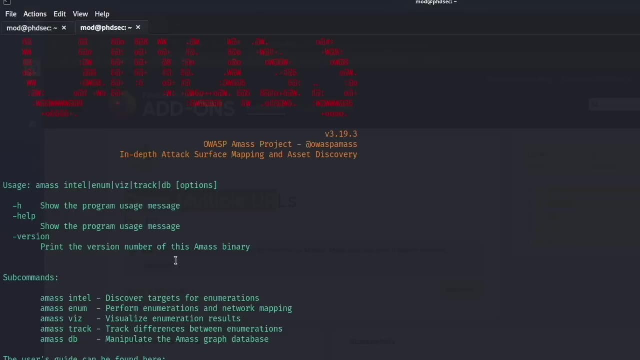 it here. it's fine, but it's. it's not as big as we would like. so one of the tools i've been using here recently is amax, and you can just type in amax, dash h and you can see exactly what it does and it's going to tell. 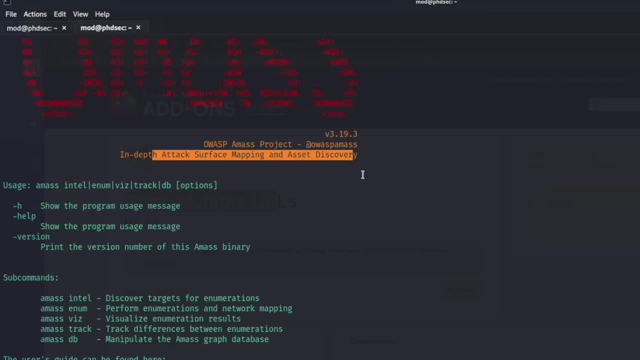 you. it's an in-depth attack attack, surface mapping and asset directory. amass is really cool if you can get it to work. so sometimes amass can be a little bit finicky, but it'll work for us for what we're about to do. you just type in amass and then we want to use enum because we're going to do 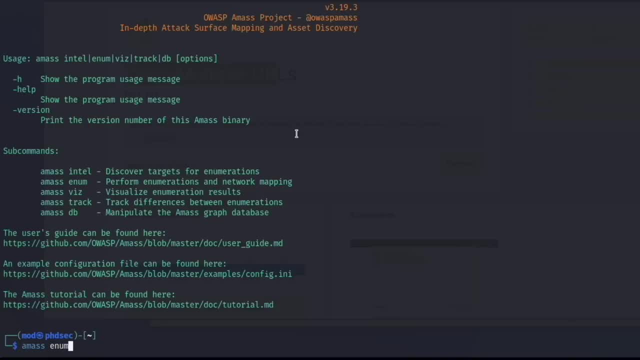 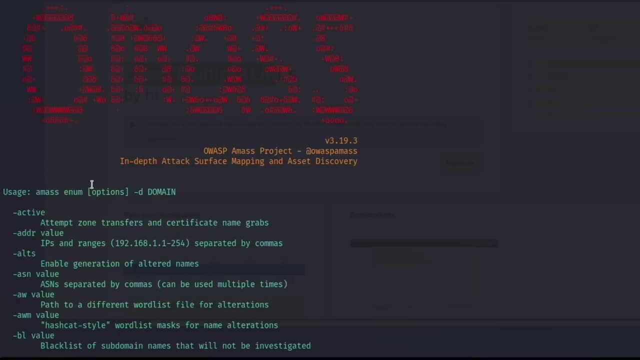 enumeration right here and then if you hit a dash, if you just hit enter with amass enum, it'll tell you everything you can do with the enumeration. and we're actually going to scroll up and we're going to run a dash d and we're just going to give it a domain. and sometimes i like 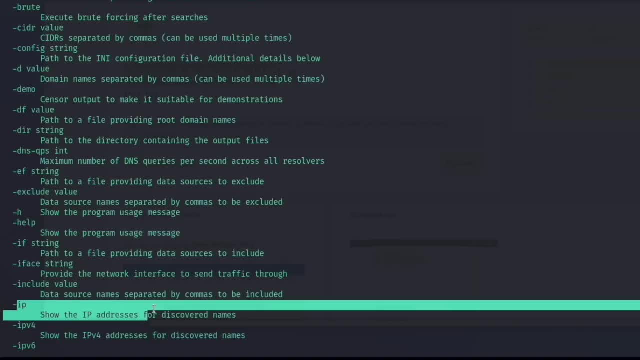 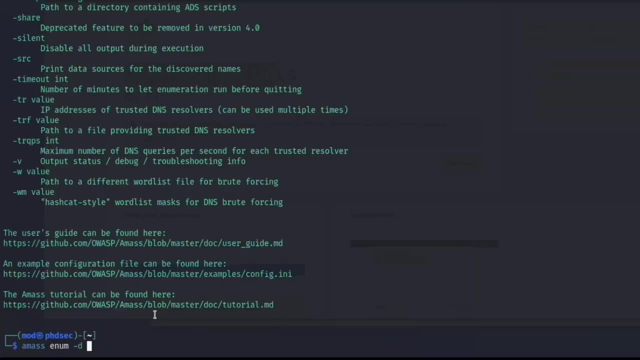 to run a dash ip to grab the ip addresses for the discovered names, which can be really helpful. so we're just going to run amass enum dash d and then we'll just run yahoocom. actually, now that i see this is running and it's actually taking a little while, let's go. 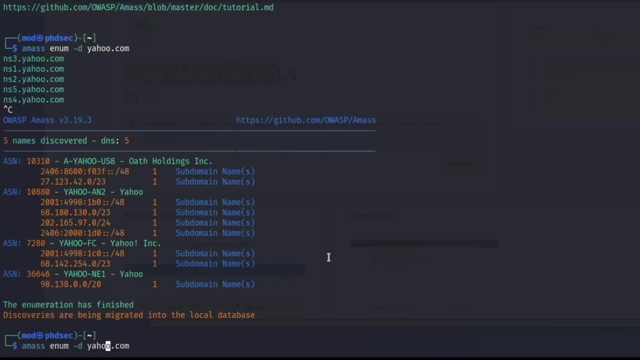 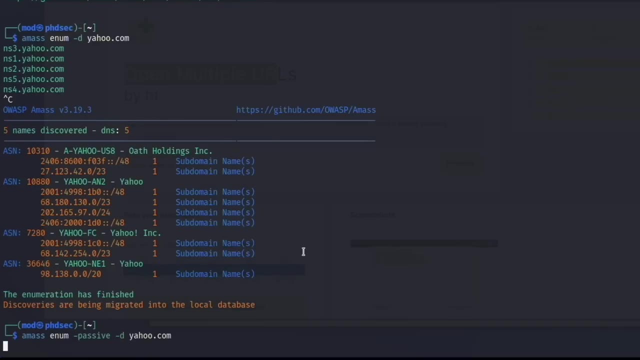 ahead and close out of this. i want to run an amass enumeration and i want to run a dash passive and then the domain right here and then run this, and this should run a little bit faster than what we did have going okay. so amass is still running, but i want to show you. look at all of these. 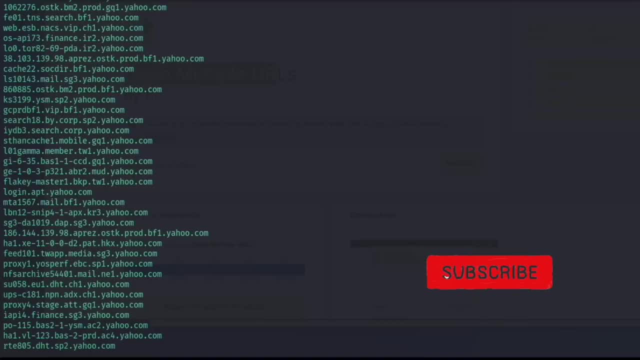 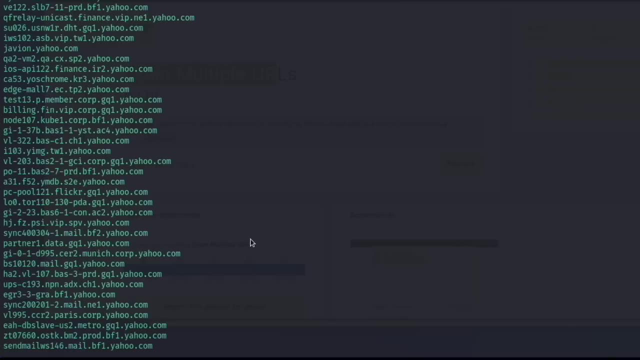 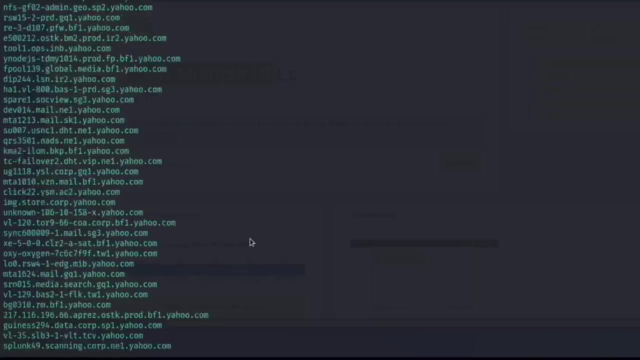 subdomains that it has pulled down. for us this is going to be way more. it's so many that my terminal is actually lagging, so we'll go ahead and close out of this, so that way it stops. and if we just scroll through here, look at all of these subdomains. this has way more subdomains than we had with. 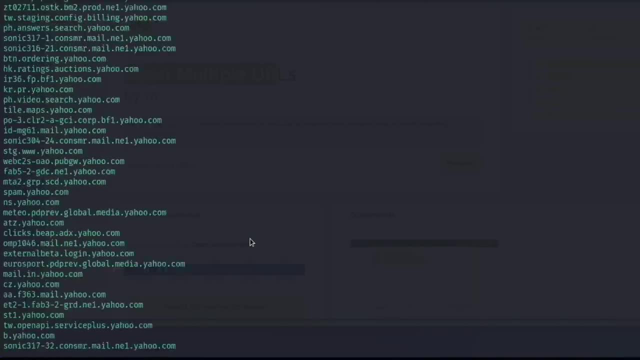 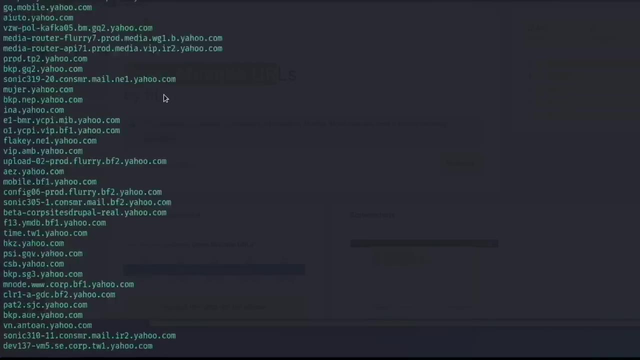 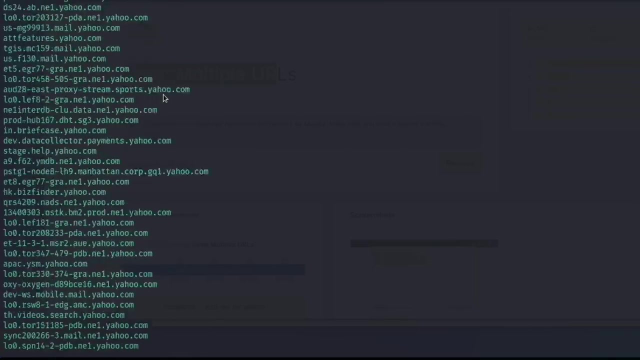 blister. it is an insane amount. so all of these subdomains you'll want to check to make sure that they're in scope. but look at all these yahoos like. this is a crazy attack surface. if you can find a program that has a really wide scope, then you will then most of the subdomains. 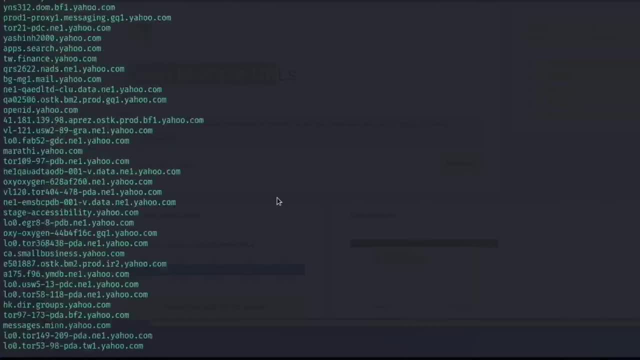 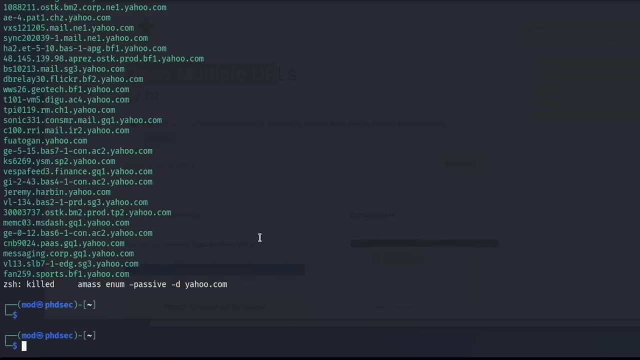 you find will be in scope, but make sure to always check. if i can't believe, i'm still scrolling. there has got to be like nearly a thousand subdomains right there. so amass is something you'll want to. i love amas enum, and then i run the passive because i think it runs a little faster and 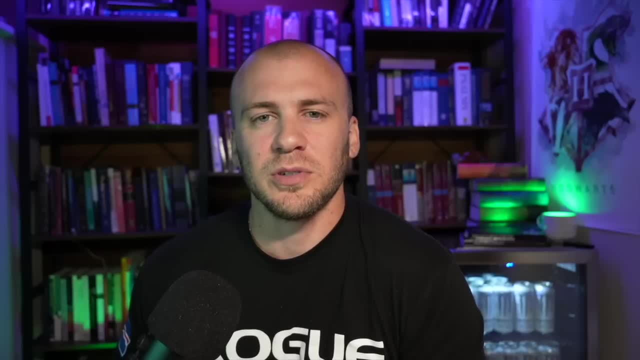 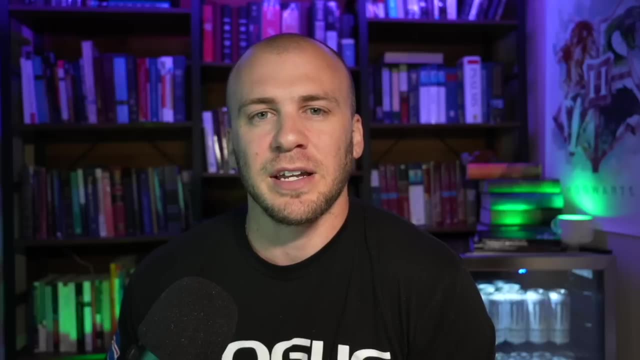 then yahoo. in this video, i'm going to show you some cool recon tools that are going to be able to help you figure out what kind of technology is running on a specific website that you may be trying to target, and an easy way to find out some version numbers and search for vulnerabilities. 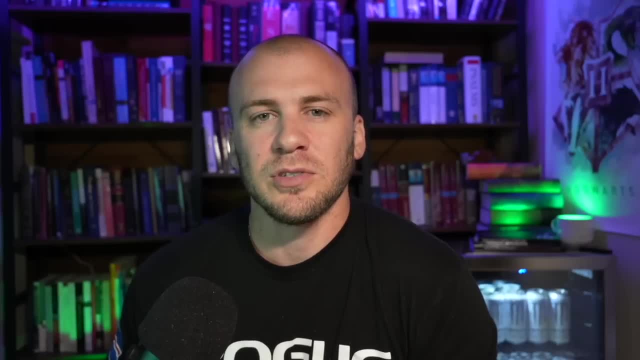 this can be really helpful for you to know what is being used and what technologies are running on a specific website, so that way you know what kind of attacks you should be looking for. so with that, let's go ahead and jump into it. all right? so here we have our subdomain and we're going to 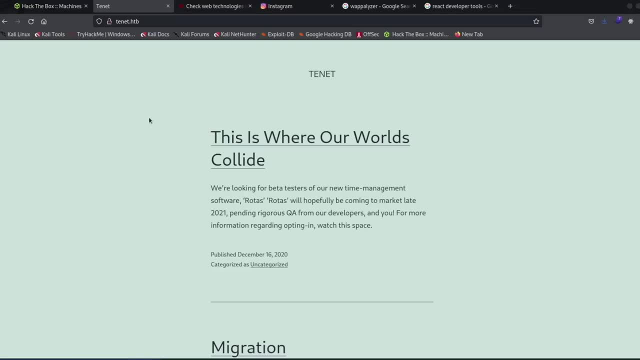 look at the web application and here we are at tenanthtm. this is a box from hack the box. i decided to use this because if there was something vulnerable on a live web application, i didn't want to accidentally show any information. so a few ways to find out what tech stack is being used. 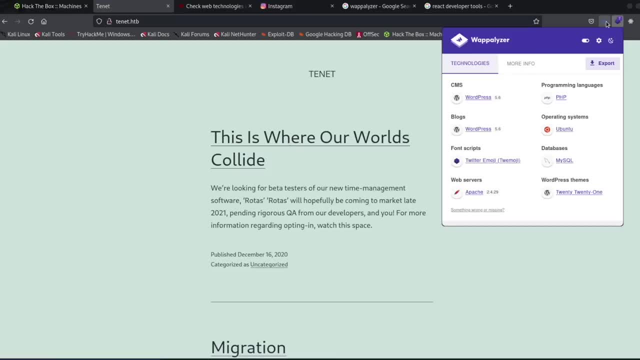 is with a tool called wapalyzer and it is right here. i already have the extension installed and you just come up here and you can click this extension and it will show you what it is running. so you're running wordpress 5.6. go to google and type in wordpress 5.6. 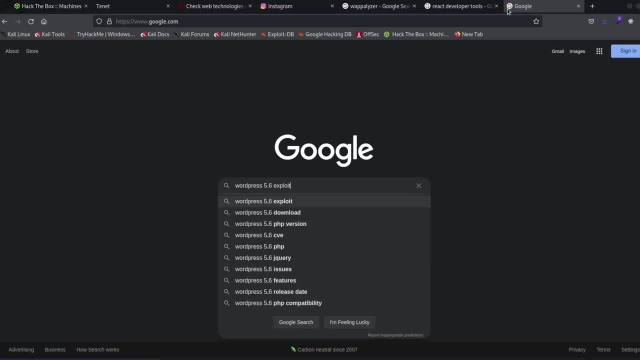 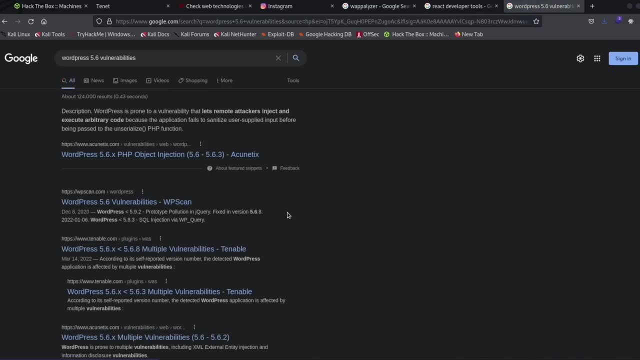 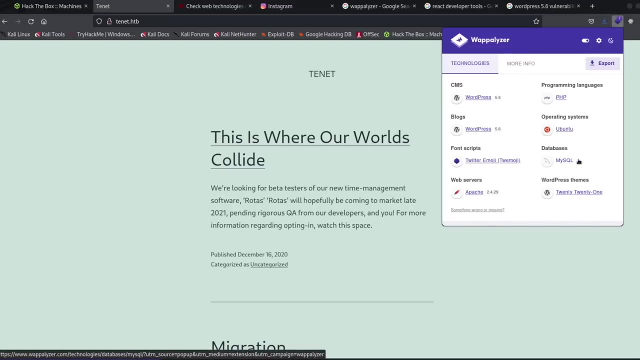 wordpress 5.6 and then you can type in exploit or vulnerability and just read to see if there are any vulnerabilities or anything that needs to be patched with this specific vulnerability. sometimes inside of here you'll see something like this database. this is really helpful for targeting sql injection. so you have a mysql database. so if you find any places, 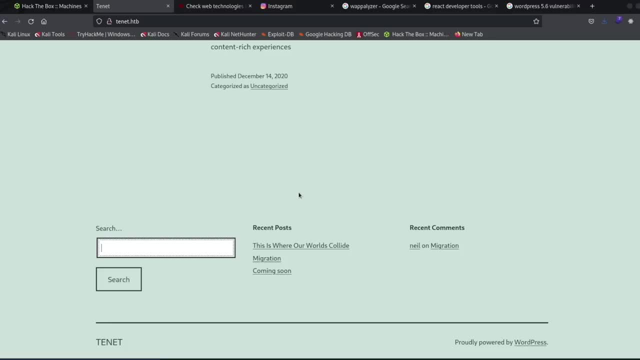 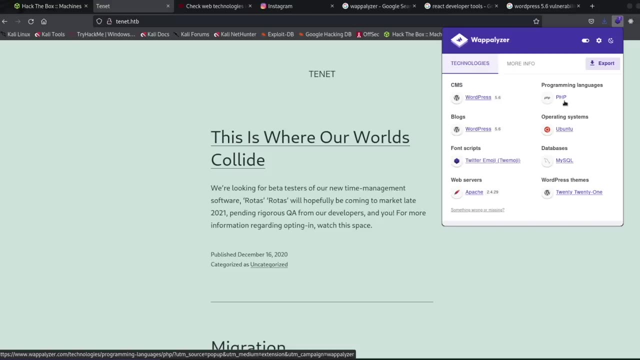 for any inputs- which i'm not sure if there are or not- you can try to pull out some kind of sql. the wapalyzer tool is really helpful in giving you the programming language. so if we're on a web application and we are testing it, if there is something like the programming language of php. 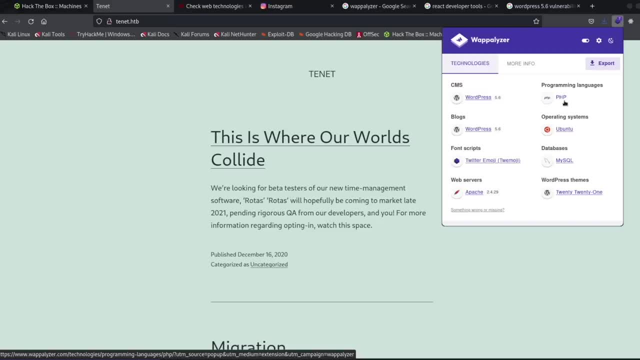 there are some very specific ways to go about manipulating php or checking for php, type juggling. there's different things you can do knowing just the programming language, and then something like this: right here we have, the web server is apache, and you can do the same thing we did with the 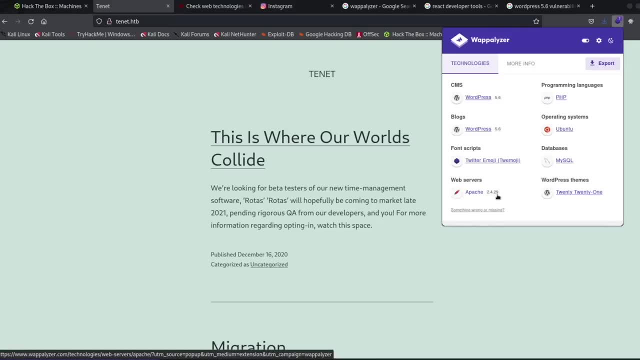 wordpress 5.6 and we can go out and see if there's anything that needs to be patched with the web server is apache, and you can do the same thing we did with the wordpress 5.6 and we can go out and see if there's any vulnerabilities here that maybe have not been patched for this specific website. 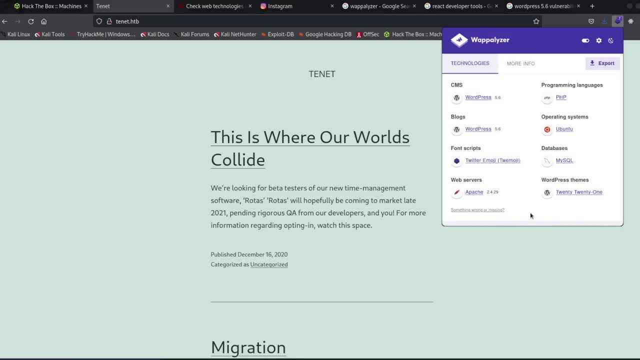 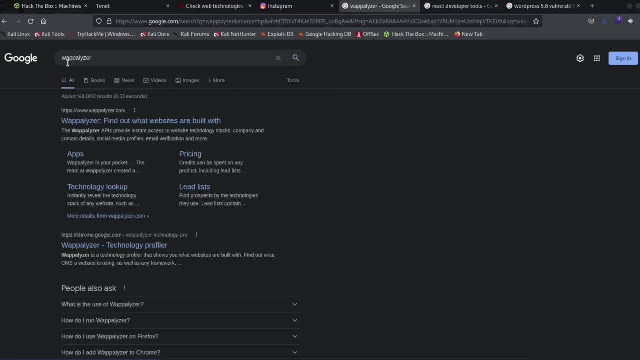 so wapalyzer is a really great way to find out what kind of technology a web application is running, and so if you wanted to install this, you can just go to google, type in wapalyzer and you can type in wapalyzer and we want. i'm on firefox, you might be on chrome and we can do firefox and 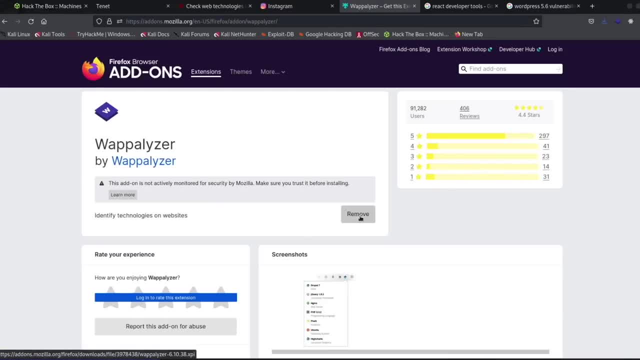 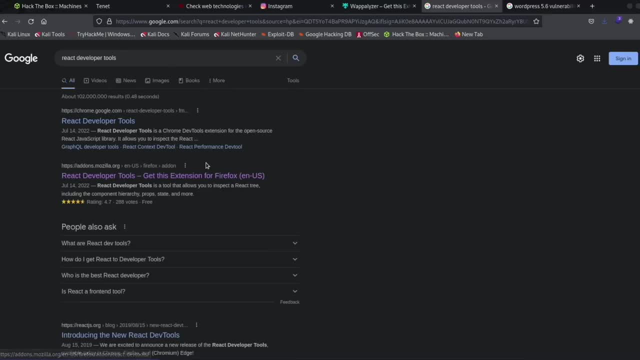 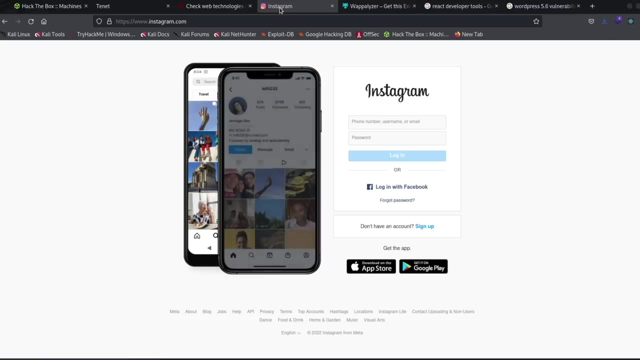 then here's the extension and you can just come over here. instead of remove, you will click install. and the second one i want to show you is the react developer tools. this is a really cool extension. it will be right here, and whenever you're using something that's using the react framework, it will light up for you. so i went ahead and opened up instagram. 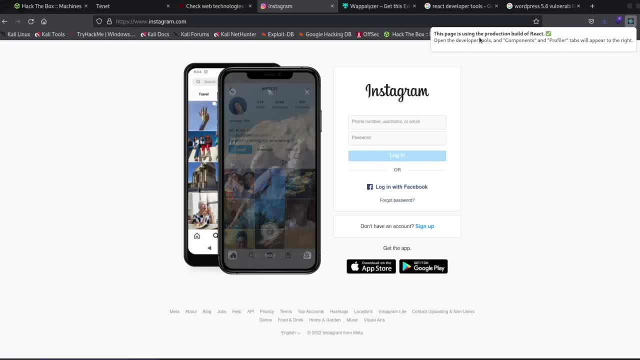 and you can see it light up blue right here and it'll tell you this page is using the production build of react, and so we know instagram is using react and there's actually a lot of popular websites that use react, such as ubereats, discord, instagram, skype, pinterest and many others. so 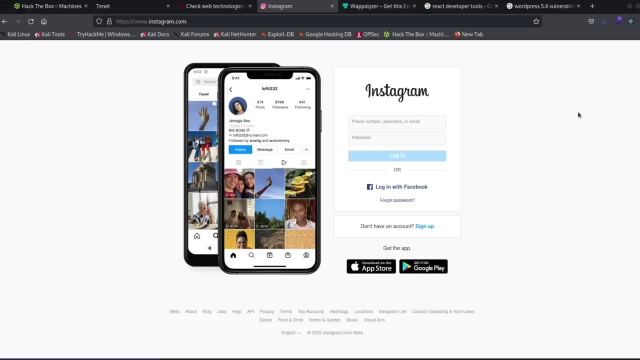 knowing what is running, such as react. you're going to know that there's javascript. and then there are a lot of common frameworks that are used within react and you can google those. we're not going to go into those in too much detail. and then one of my favorite: 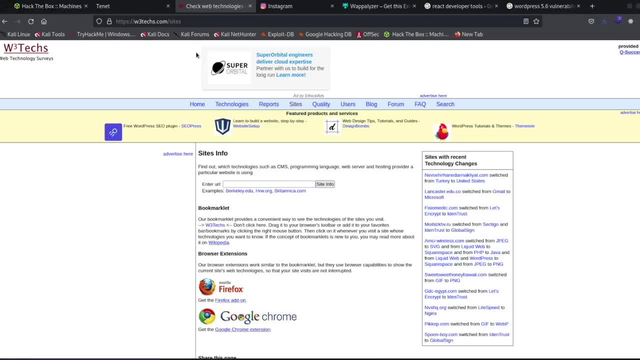 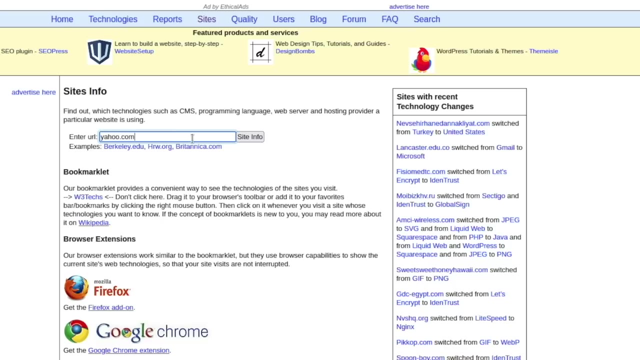 websites is right here, the w3 text. this is going to do something very similar to wapalyzer. so right here you can just enter a specific url and it's going to tell you what is being used. very similar to wapalyzer. so if we just type in yahoocom, it will pull back for us. all of the 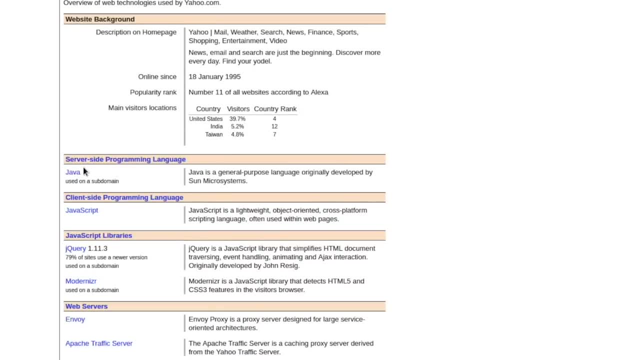 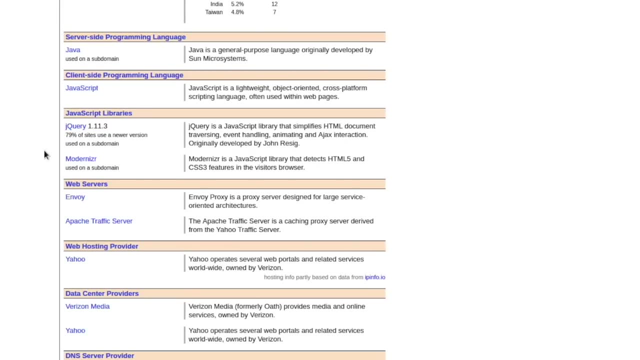 technology that is being used. so it says it has some server-side programming with java javascript jquery. so you have this really old library right here and it tells you there is a newer version, and so there's a lot of information in here and if you have any questions about something like javascript, 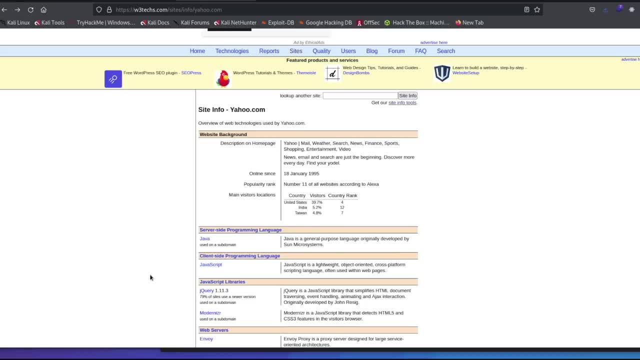 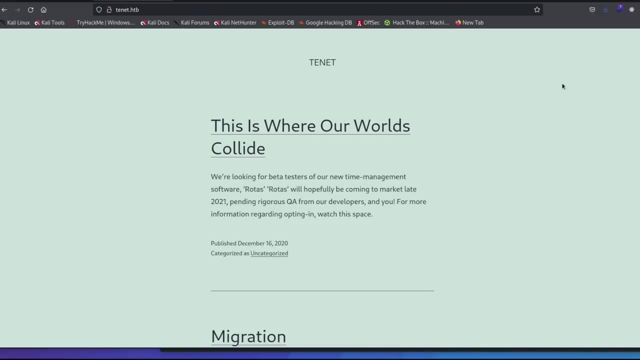 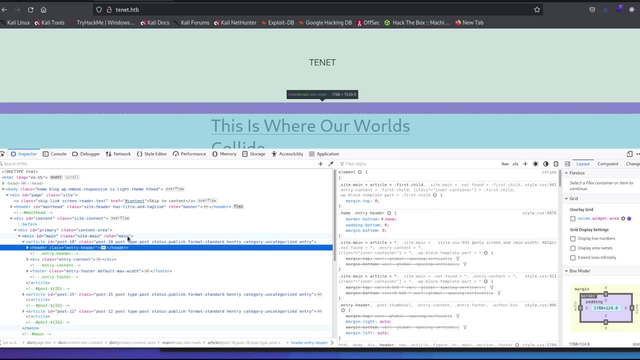 you can click on it and it'll tell you what javascript is or jquery, and how it is used. so there is one other way to kind of find out what kind of tech stack is being used. so if you come into wapalyzer and we look at this, we can also come in and try to figure out what is being used. 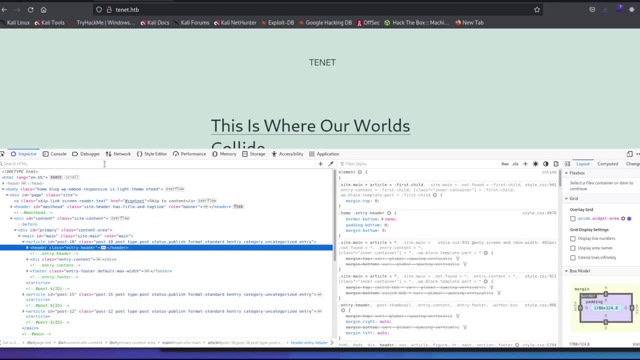 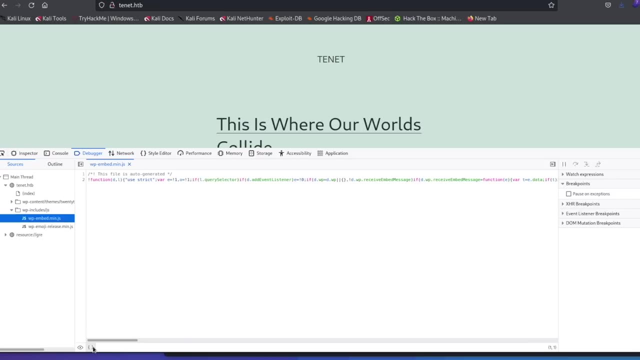 within the javascript. sometimes you'll be able to see comments or be able to work out what is being used on the website by coming in here and clicking on the debugger right here and it'll tell you here is the js and we have the javascript, and then you can click the pretty print down at the bottom and 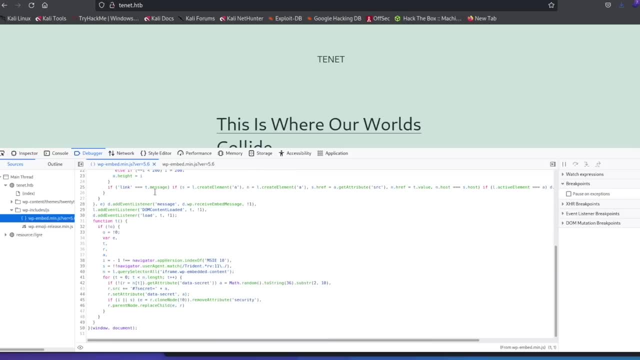 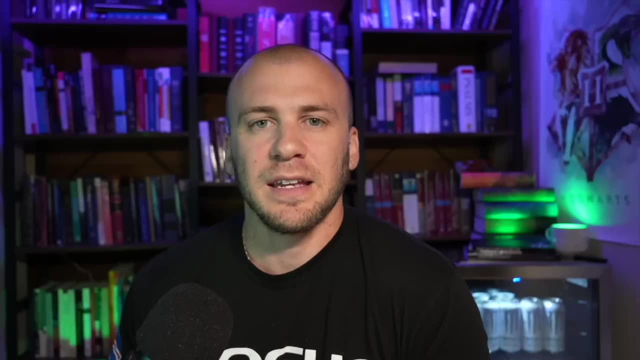 you can look through this javascript and see what you are able to find inside of here. so we're going here. so these are some of the common ways to find out what technologies are being used on websites. they can be really helpful for you to know what's going on and exactly how to attack a website, and 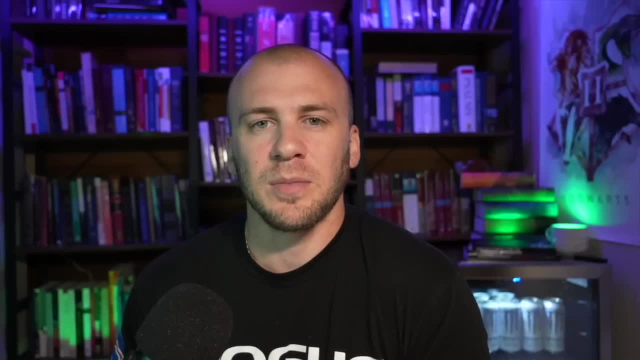 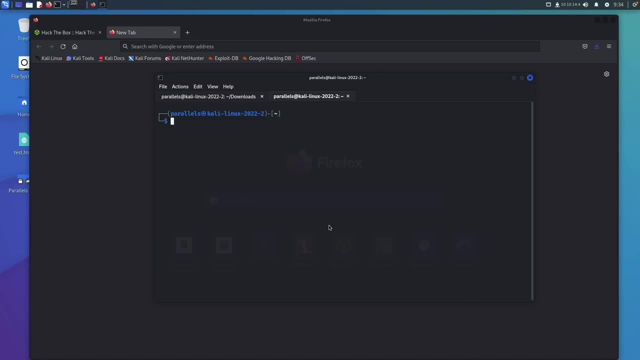 these can be really helpful for you in your recon phase and maybe even lead you to some kind of vulnerabilities just because you have a version number given to you. okay, so now i want to show you the tool in map and if you followed my channel for any length of time, you're familiar with the 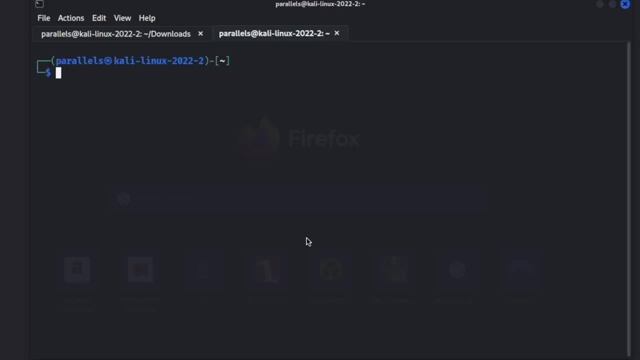 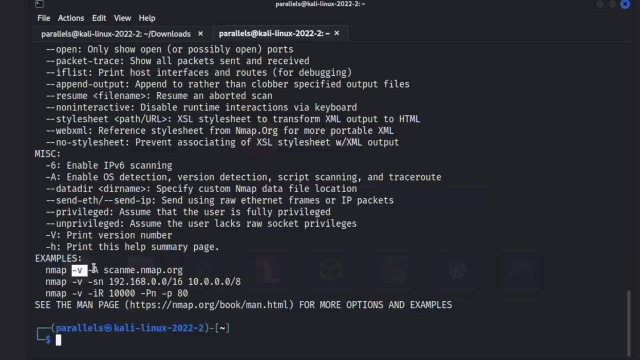 tool in map, but i want to show you how i like to run this tool and the information i like to look at is in map. so in map is a port scanner and if we run in map dash h, it's going to spit out for us all of the things that we can do with in map. one of my favorite things to do is run the dash v with. 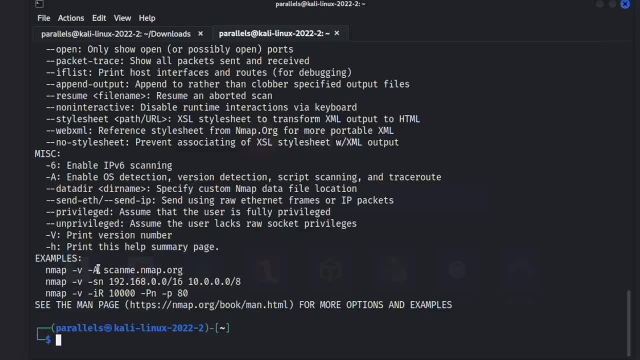 a dash a. this is going to tell us about the open ports as they come back, and this is going to give us all the information. so it's going to tell us right here: enable os detection. it's going to do script scanning and it's going to look for different versions as well, so we can go ahead and 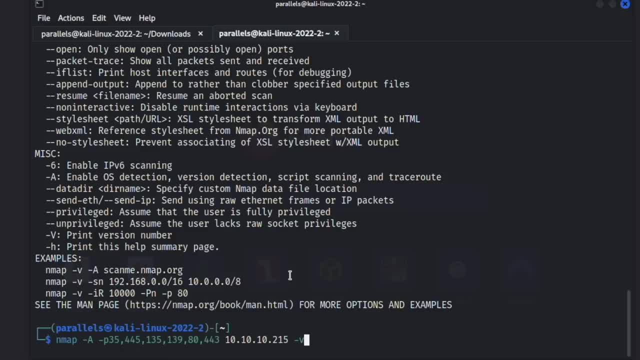 type in an in map dash a and we're going to go ahead and type in in map dash a and we're going to type in in map dash a and usually you would run a dash p dash if you're doing like some kind of ctf. 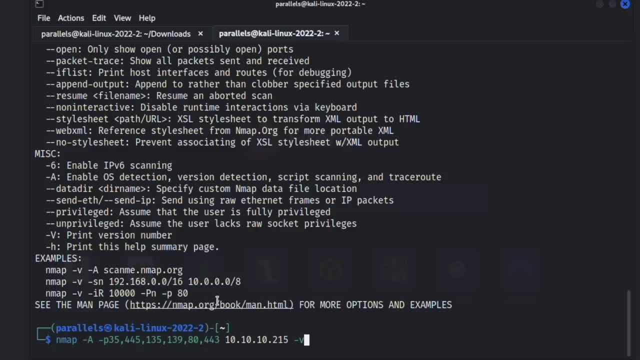 but if you were doing a bug bounty program and you're not wanting to knock on the doors of all the ports, you would just run the specific ports that you would like to see if they are open. and so i've gone ahead and opened up a hack the box and so if we run this, this is what it's going to. 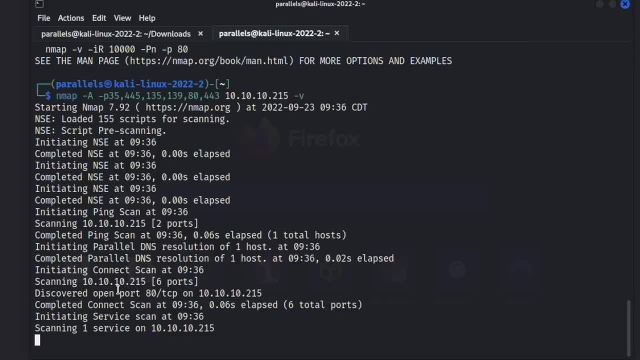 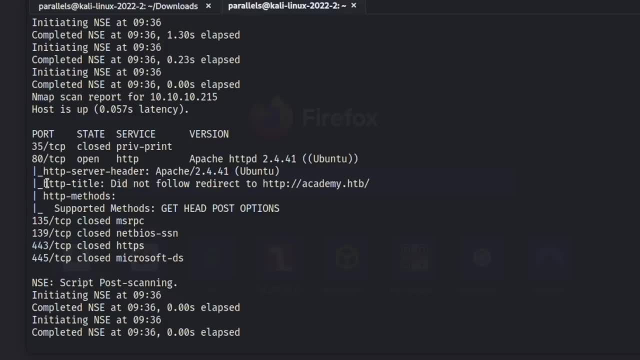 look like and the dash v is going to give us back the ports as it finds them. so it says a port 80 is open and it has finished and it tells us about the open ports. and one thing to note is that the hack the box is. it says it did not follow the redirect so it went out to see if port 80 was. 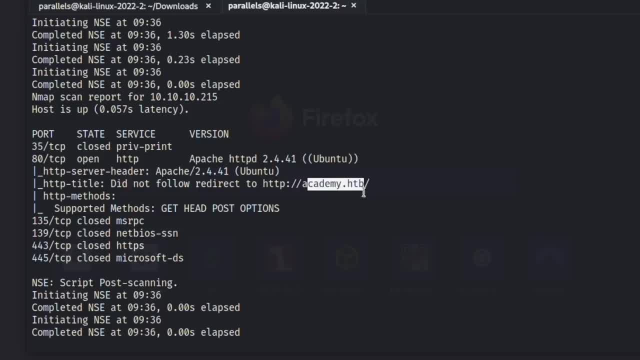 open. we were redirected to academyhtb and if i actually wanted to open that and i keep getting this not found right here- that is because i need to add this to my etsy host file. but we're not going to do that right now. that's not the point of the video and we are told we have the apache. 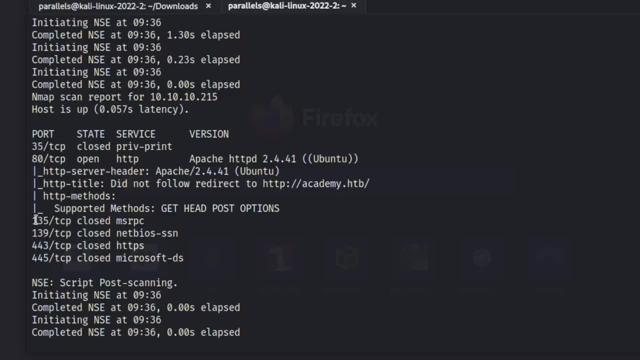 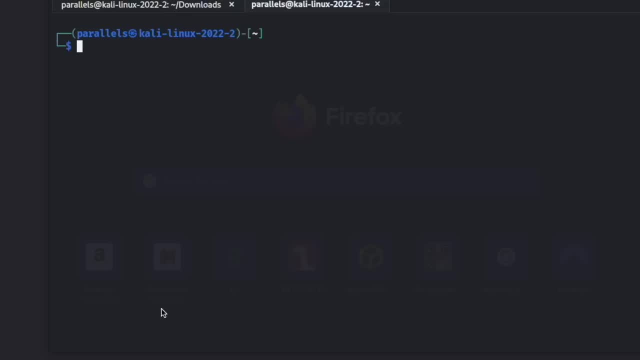 version and it tells us our methods and it gives us these ports are open as well. so this is how i like to run in map, and so we will continue on. there is one last way to search for subdomains and directories that i think will be helpful for you to know, specifically subdomains. we've seen this before. 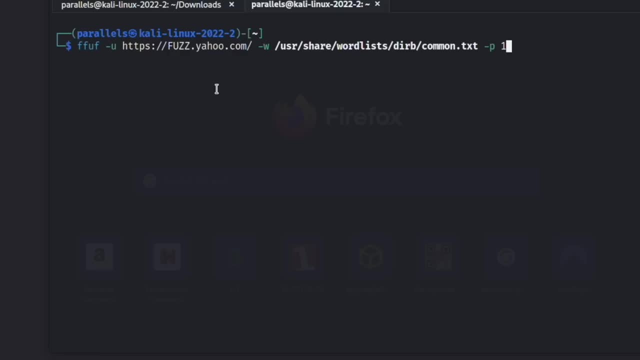 dealing with directories, but we're going to use the tool fuff, and this is the syntax that we're going to use. we're going to go ahead and fuzz for subdomains on yahoocom. so the tool is pretty simple to use. we just type in fuff the url which is going to be right here and the location that. 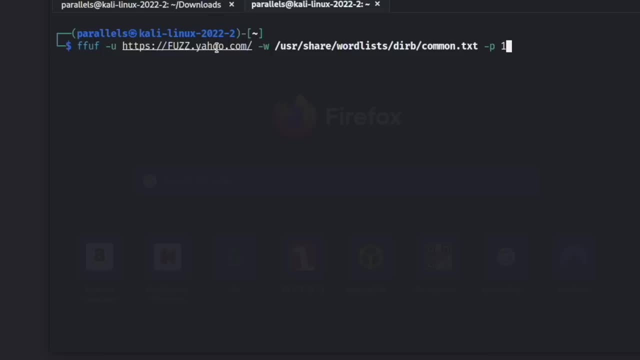 we want to fuzz, which is for subdomains before yahoocom, and this is going to brute force for us- any subdomains that come back with the status code 200, and then we're going to use our word list, which is right here, and then we're going to use 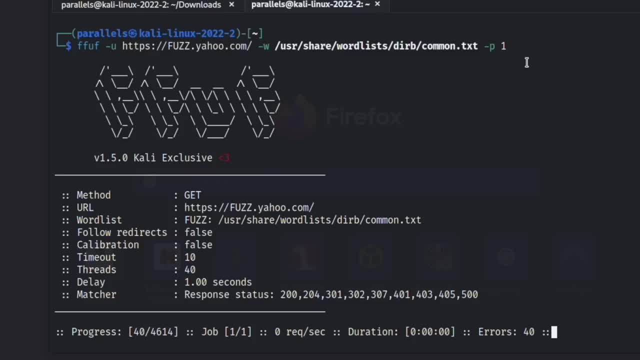 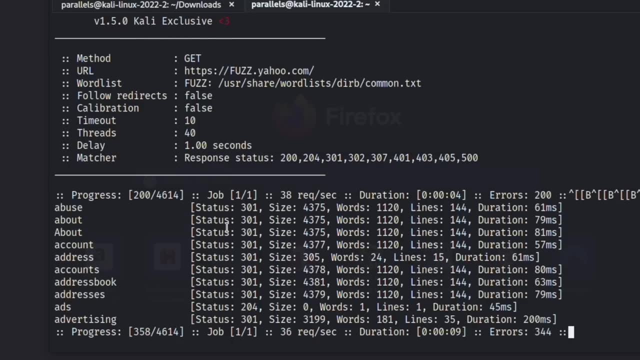 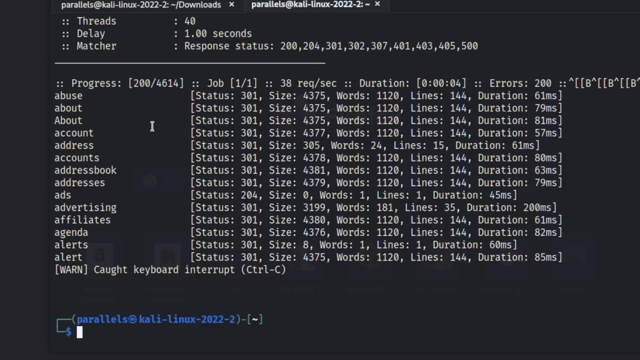 a slowdown of one second. so we can go ahead and run this and you should be able to see subdomains start spitting out as it finds them, and here are a few different subdomains and i want to just- we'll stop this right here. i want to show you so we got this 301, which i believe is going to be a redirect. 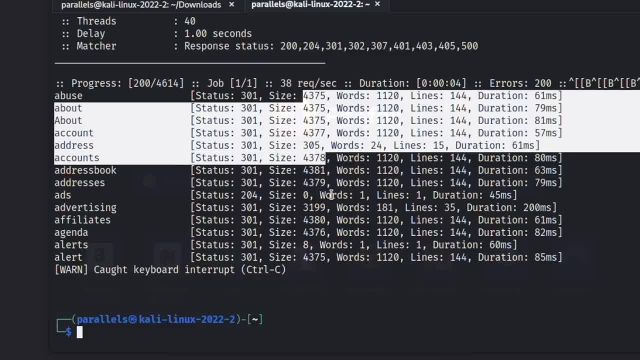 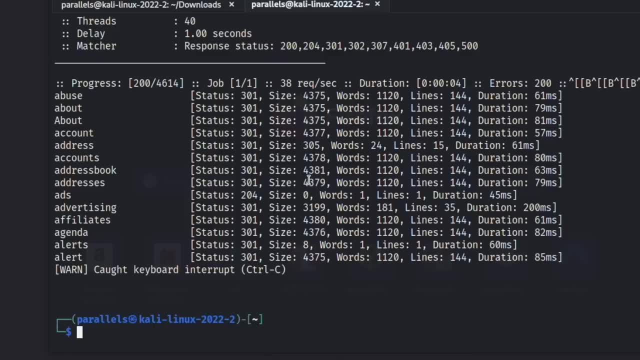 but we have different sizes, different ways to do this, so we're going to go ahead and fuzz this subdomain, and we're going to go ahead and fuzz this subdomain and we're going to go ahead and check these out anyway, but just in case, we didn't want to see these 301s, what we can do is, i think, 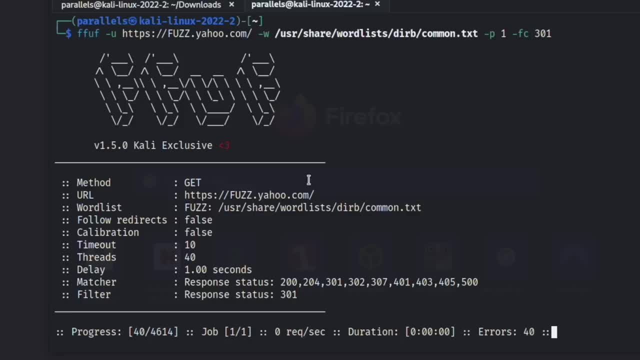 it is a dash fc and we can say 301 and now it won't show us any of those 301s. sometimes that comes in handy when you are fuzzing and you keep getting 401 or 403 and we really don't want to see. 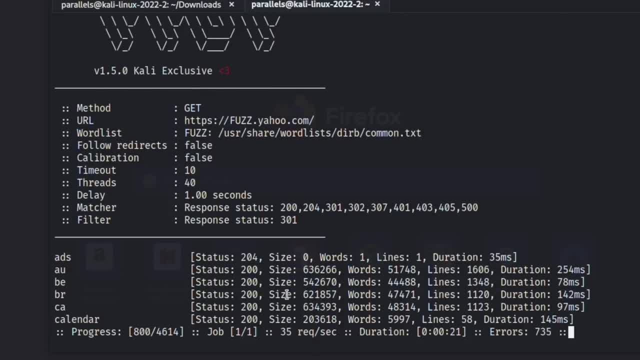 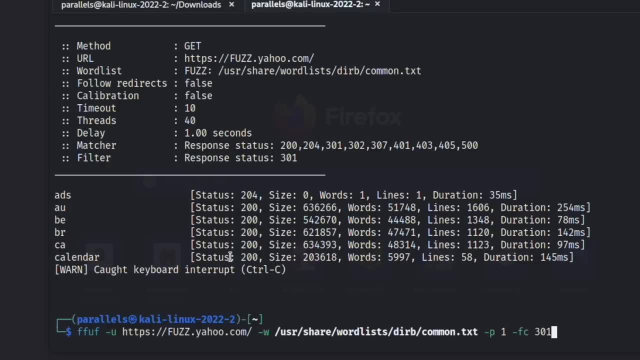 those, and so you can see here are some 200s. so if we wanted to, we could go out and look for these subdomains and see if any of those subdomains would be present here, and we could go ahead and of them look interesting to us now. i have mentioned this before. you can also fuzz for. 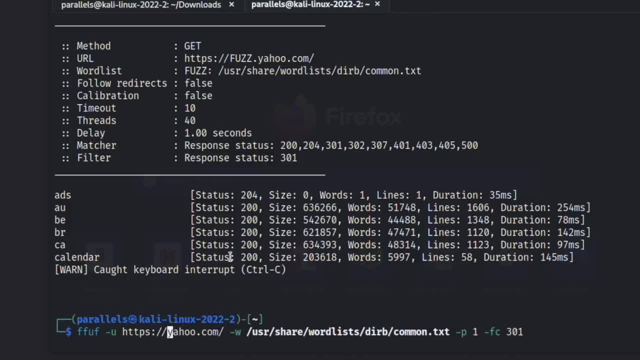 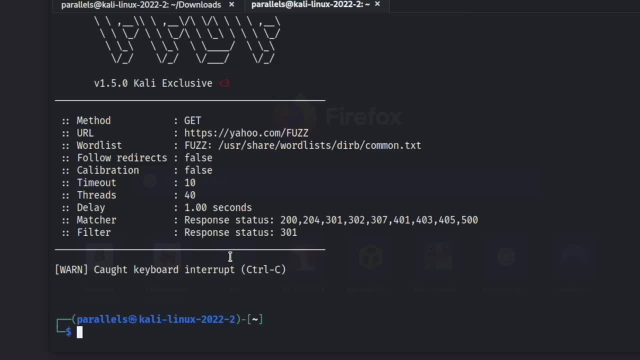 directories, and you can use the fuzz like this in this location, and now, if we run it, it's going to look for directories. and lastly, one thing i also want to mention is when you are fuzzing for apis, fuff is also a really great tool for this. so we'll go ahead and delete this, and if we were, 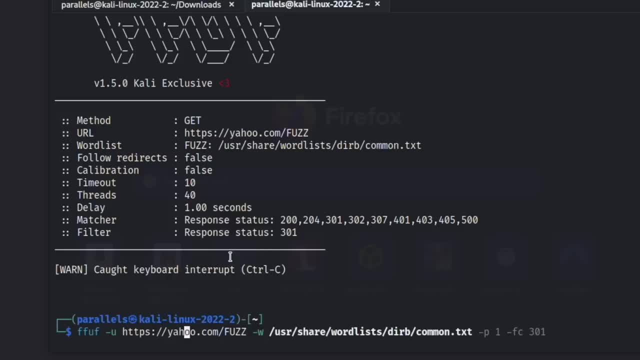 going to be looking for. let's say, there's an api that looks like this- apiyahoocom- and we wanted to fuzz for valid endpoints and see what we could find. we would just go ahead and run fuff like this and look for endpoints and then go. 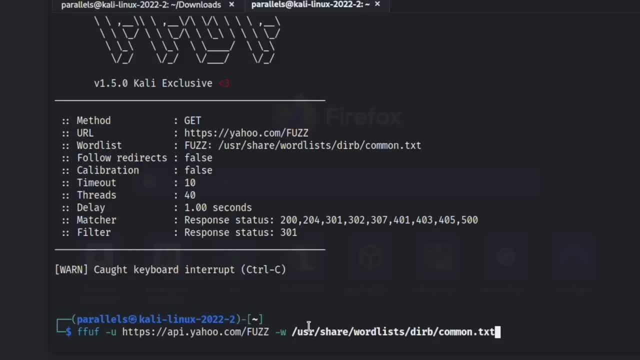 out to the web page, if we are able to, and look at the json. if not, i have a tool that will fuzz apis for us and actually give us the json right here in our terminal, and you can go check that video out. i'll link it in the description. if you would like to build that tool, it'll save you some. 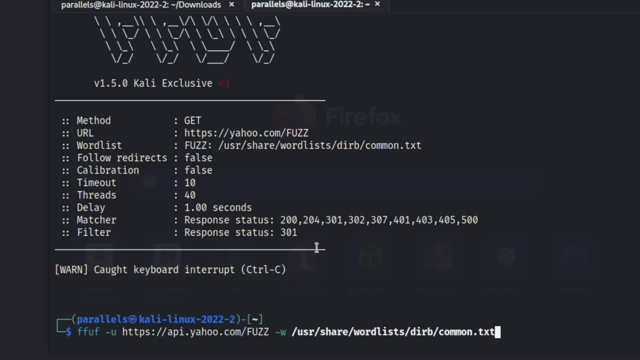 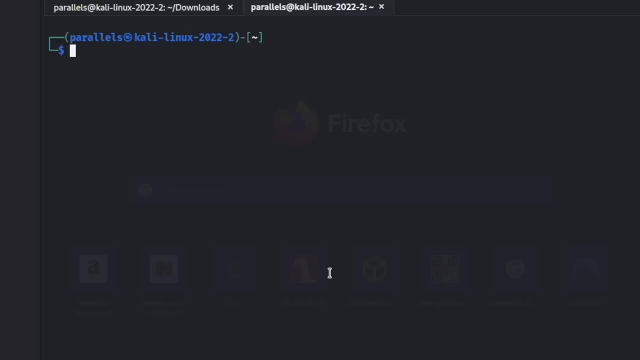 time having to go out and look at the json itself and it'll just print it right here in the terminal for you. so with that, that is fuff and how we fuzz for subdomains and directories, all right. so it is always good to have a couple of tools in your tool belt so you can go ahead and run derb like this and 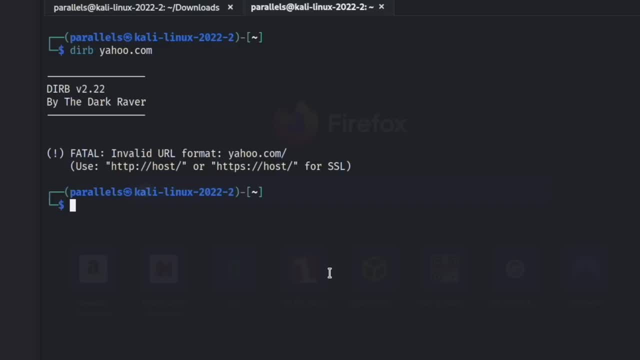 we can run a yahoocom and we don't really need any more than just this right here. so it's just an https, we'll run yahoocom and it'll automatically start fuzzing for us, just like that. it's really simple to use. so sometimes fuff might give you some errors or it's not working quite right, and it's always. 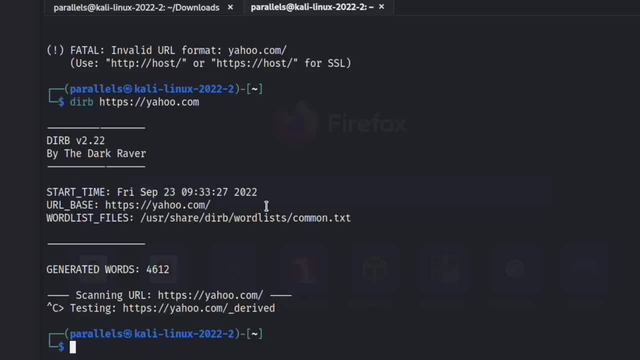 good to know of other tools. one of the cool things about derb is you can run it recursively and so once it runs all the way through your word list and it, let's say it found yahoocom football, the next time it runs it'll run yahoocom football and then it will look for. 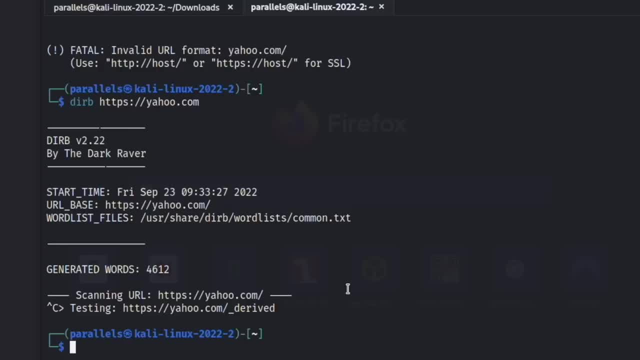 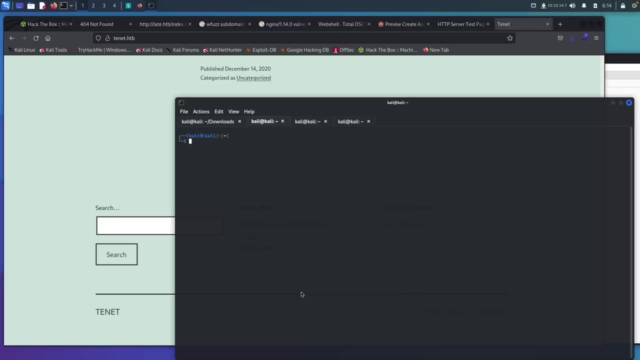 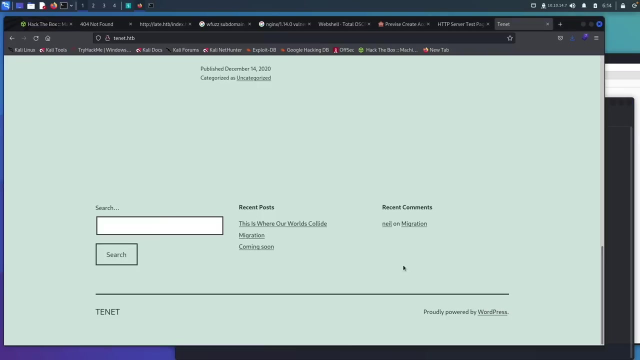 more directories within that football directory, which is really so. derb is also a backup fuzzer, just in case fluff isn't working for you. another helpful tool that you're going to use, especially inside of ctfs, is wp scan, and you're going to use this with. 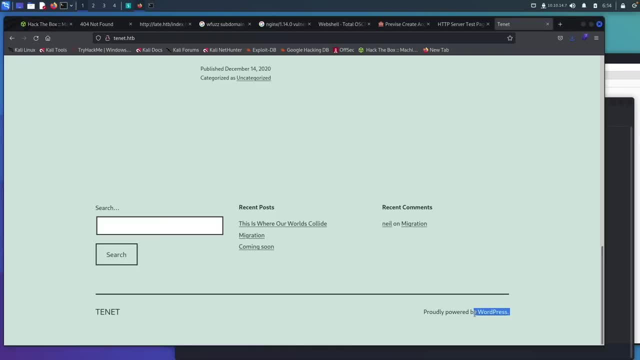 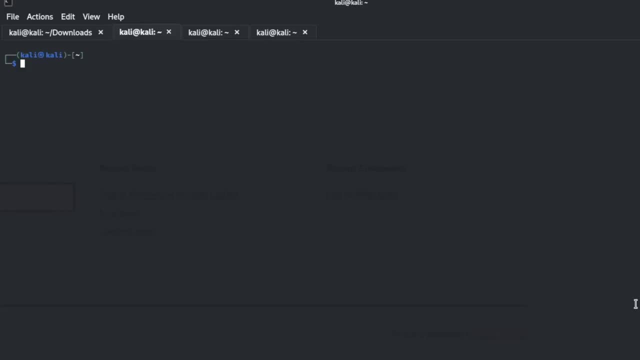 wordpress sites. so i've gone ahead and opened up hack the box and i have a tenant running here, and if you have a hack the box subscription and you're wanting to follow along, you will need to add tenanthttp to your etsy host file, which i have already done. 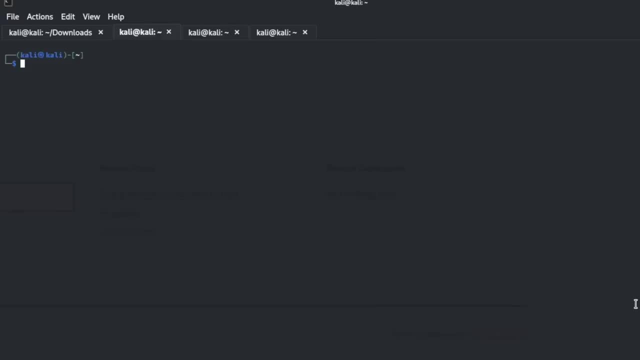 so the wp scan tool is going to go out and look at all of the plugins on the wordpress site and see if any of them are vulnerable, if any of them are out of date. it's going to check the actual theme and see how old it is and how long it's been since it's had updates and we can go ahead. 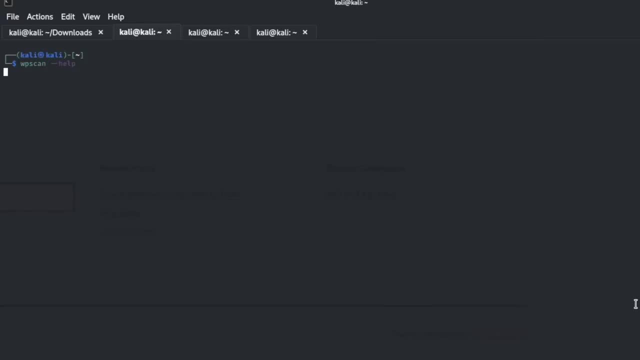 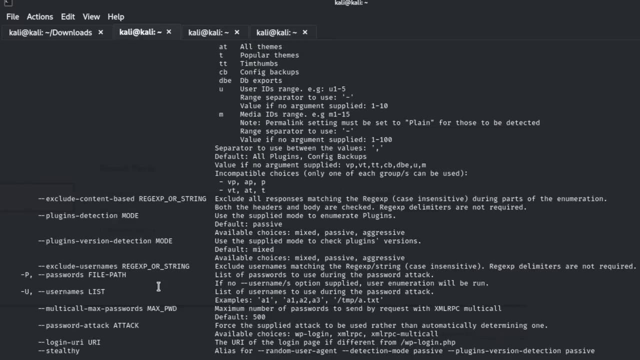 and check out wordpress scan right here, the wp scan dash help, and it will tell us all of the different flags and everything that we are able to use. and one thing that i can never remember what it actually looks like is this right here is the dash dash plugin detection. so what we will 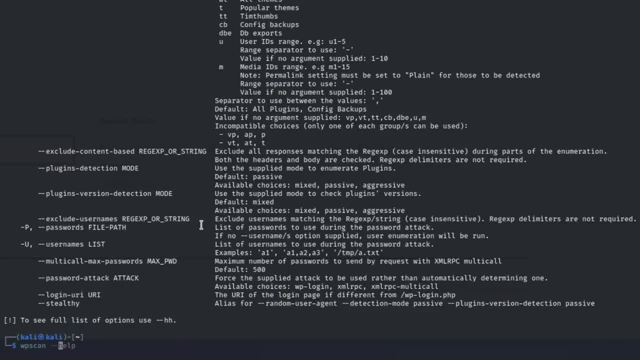 do is we'll type in wp scan, dash, dash, url, http, slash, slash, and then we're going to go tenanthttp and then this dash e right here is going to tell it that we want to check all of the plugins. i sometimes call it all ports out of habit, but i think it's all plugins. we can actually just look. 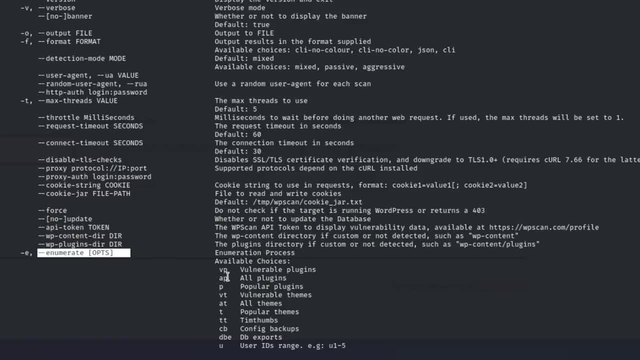 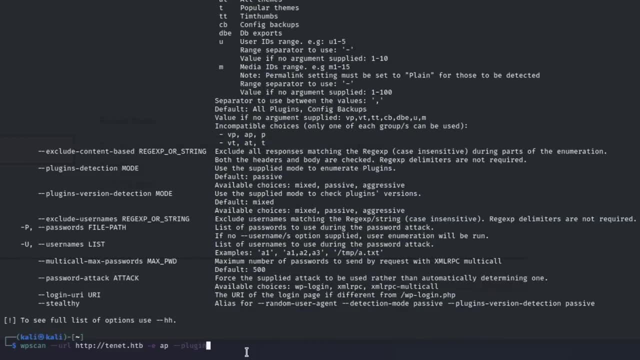 if we scroll up, we're going to enumerate all plugins right here and we want to use the dash dash, and then we want plugins dash detection, and then we want to use aggressive, and then you can do a dash o if you want to save this in an in a file. i pretty much never do that, i'll just open a new. 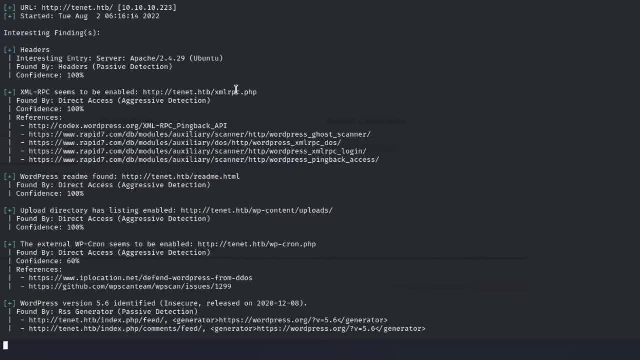 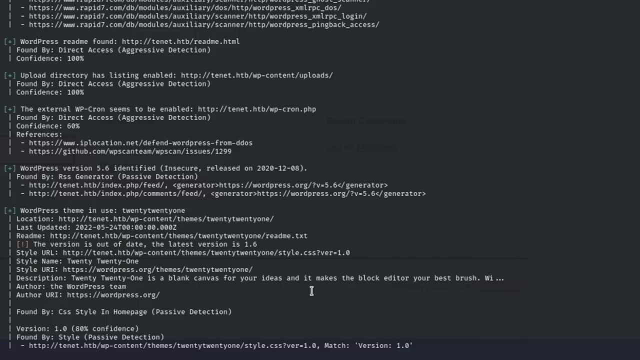 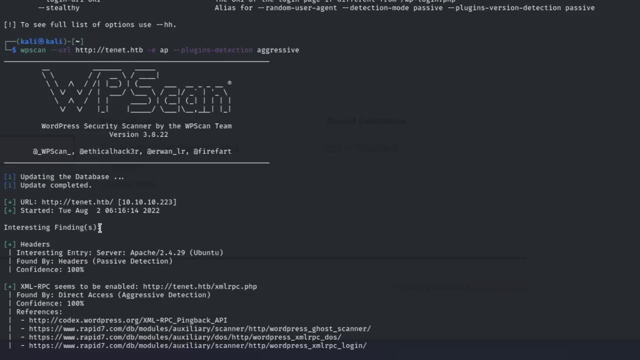 tab and come back. sometimes i'll have a whole bunch of tabs open up here and it's not always that helpful. so it will flag things like this and tell you that a version is out of date, and i told you this in the last video. but i especially am really bad with wp scan, because you get a lot of information but you 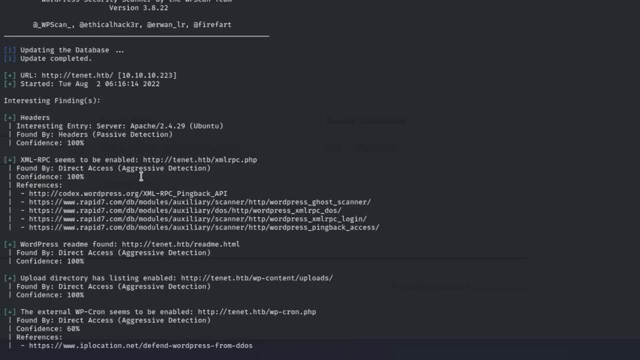 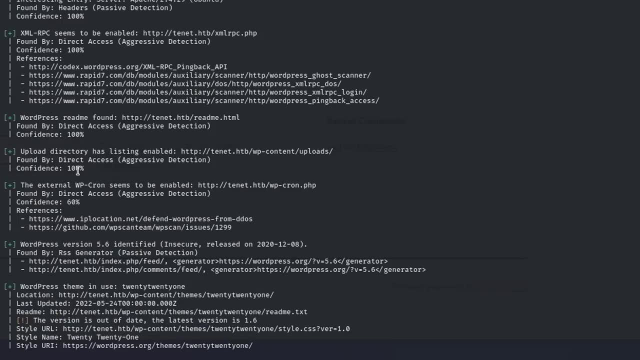 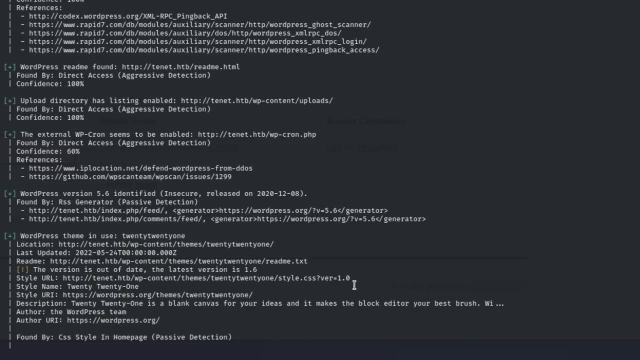 should read all the way through all of this. i remember doing a ctf about six months ago and i ran a wp scan and i just like, skimmed through it and i ended up missing a vulnerability that gave me remote code execution, and i wasted several hours of my time enumerating when i should have just read the entire scan. so make. 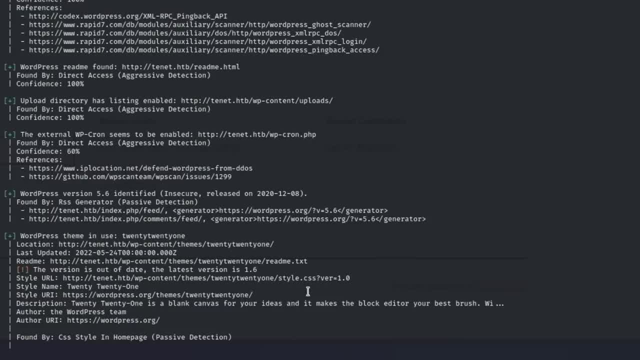 sure you read the entire scan when you run one. it might take you a little bit of extra time, but it will always be worth it because it will give you information, even if you think it might not be helpful, like right here. it doesn't flag this, but it might be worth going out and checking. 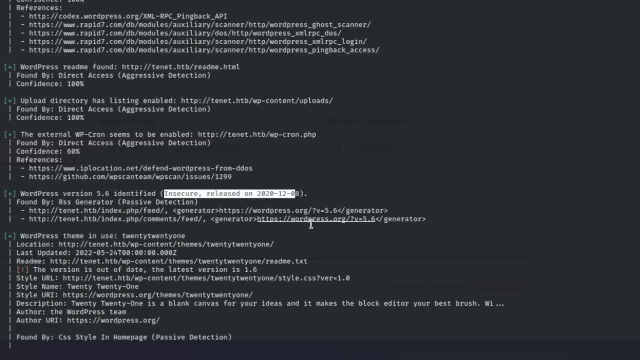 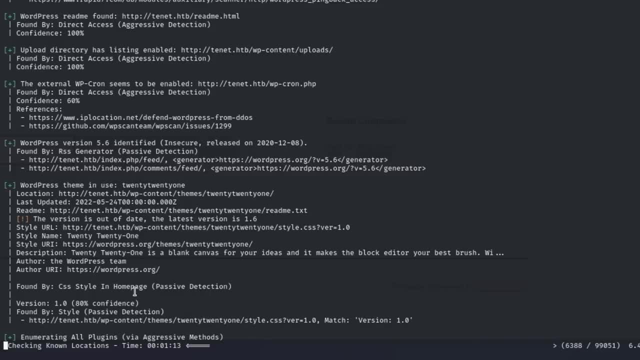 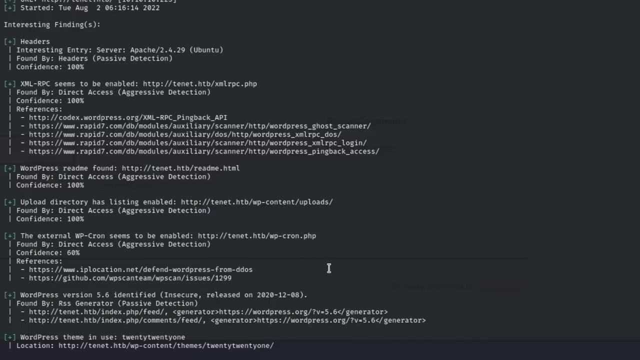 this version 5.6. it's insecure on this specific release and you can go and check this. the different version numbers and this might take a little while because we're running the aggressive, but that is okay. so this is wp scan. you're going to want to run this whenever you come across. 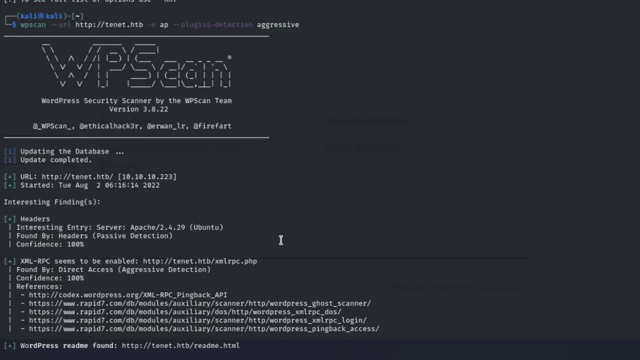 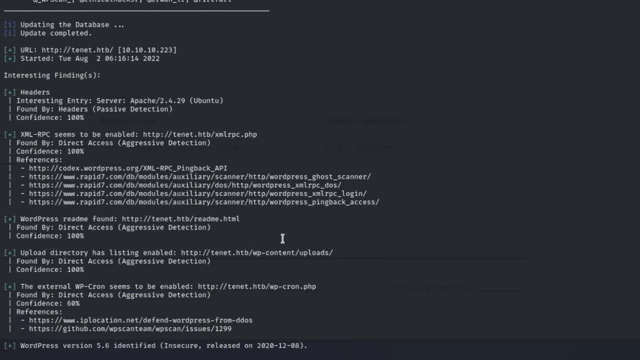 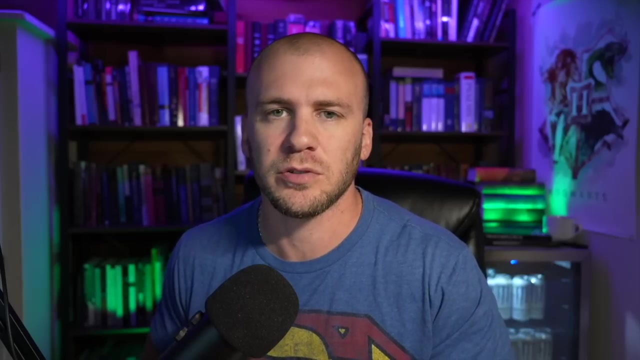 wordpress web applications. it is going to be your friend. you're going to use it regularly throughout your penetration testing career, especially in the world of cts, and always remember: read the output. in this video, we are going to cover how to choose a bug bounty program to attack. One of the first things you have to do is figure out a target that you want to start. 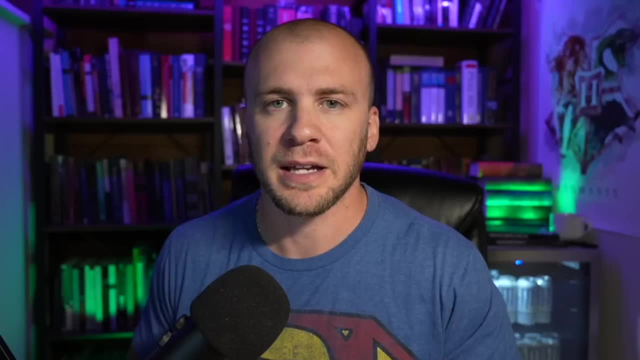 doing your recon on, And sometimes people can become paralyzed by analyzing all the different targets and trying to figure out which one they want to attack first, And so I want to try and help you figure out how to narrow down your options and then specifically choose one, and 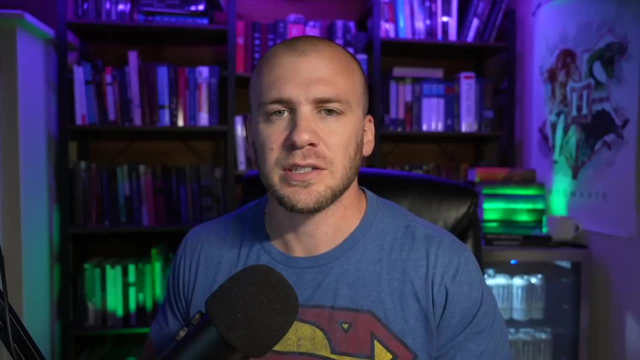 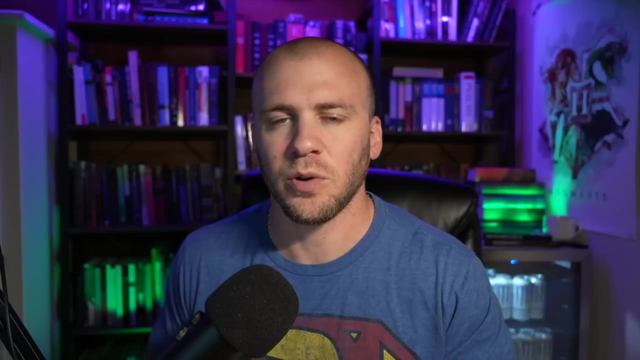 then start your recon process with. So, before we jump into this too far, I kind of wanted to give you a little bit of encouragement, And I'm not really a Star Wars fan, but I came across this a really long time ago and I found it to be really helpful. And it says: you want to know. 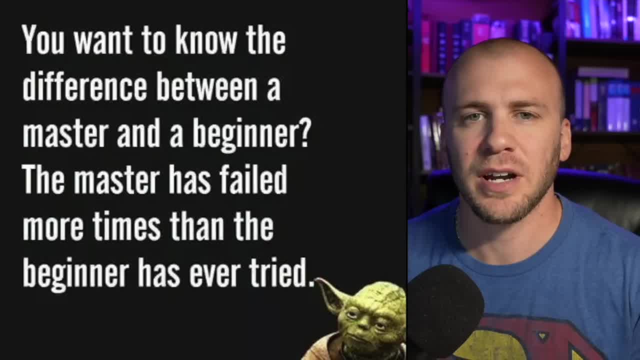 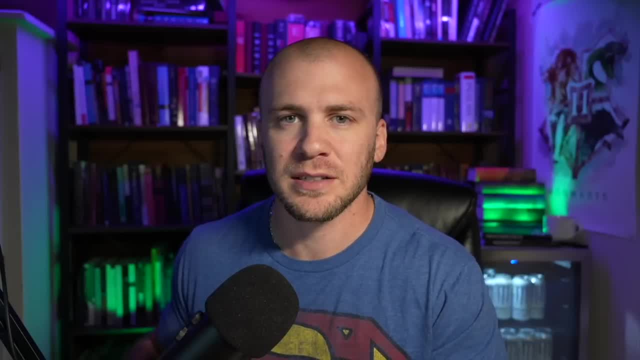 the difference between the master and the beginner. The master has failed more times than the beginner has even tried, And I think this is really helpful when trying to figure out how these top hackers are finding so many bugs and so many other people are struggling. It is 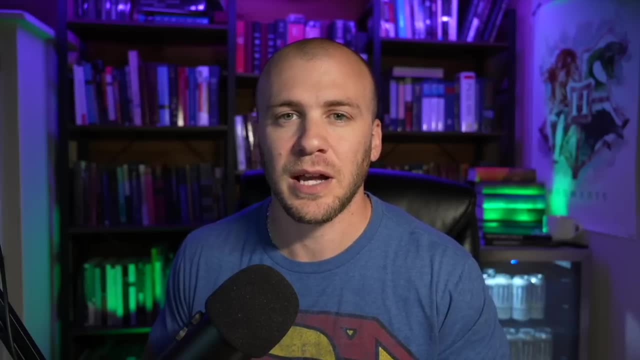 because they have dedicated a lot of time to specific platforms and to learning this craft, And so we just have to keep moving forward every day and you'll be getting better at it, And I think that's really helpful. And I think that's really helpful. 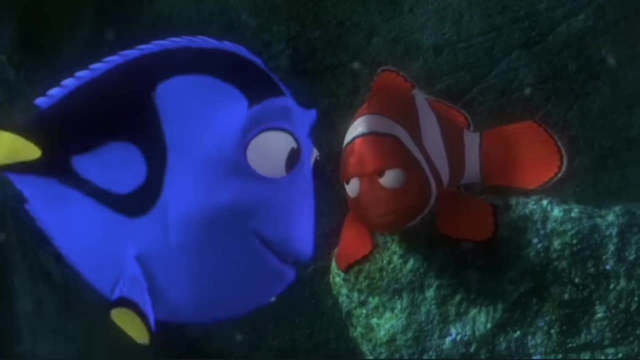 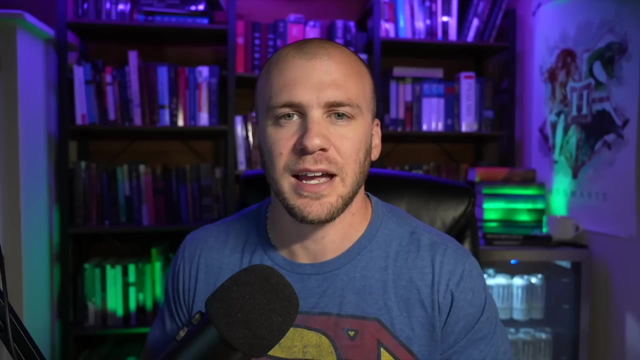 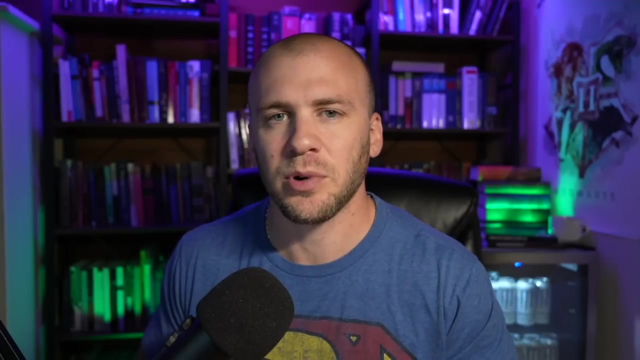 So I decided to add just keep moving forward to a t-shirt recently, because it really does show the perseverance that you have to have in the field of cybersecurity. So let's go ahead and take a look at hacker one and narrow down some potential targets, And I'm going to show you my 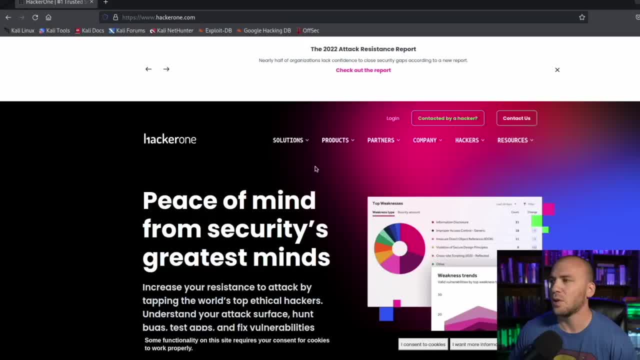 process for doing this, So let's go ahead and jump into it. So here we are on hacker one, And one of the first things I like to do is I'm going to go ahead and show you my process for doing this, And one of the first things I like to do is come in to the hackers and then we need to go to the 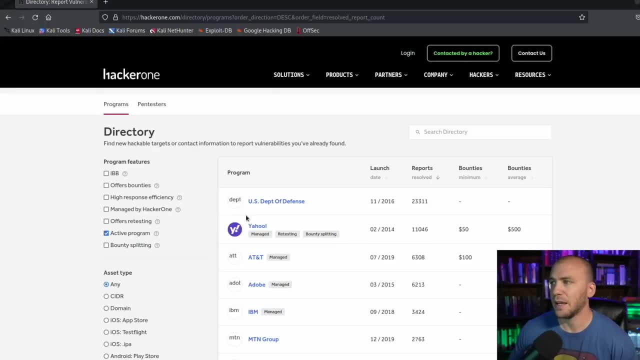 directory so that we can start looking for different programs. And now I like to click launch date and I like to sort by the date. I want to go from the newest first. I accidentally clicked it one too many times And I actually believe you have to be logged out of hacker one. 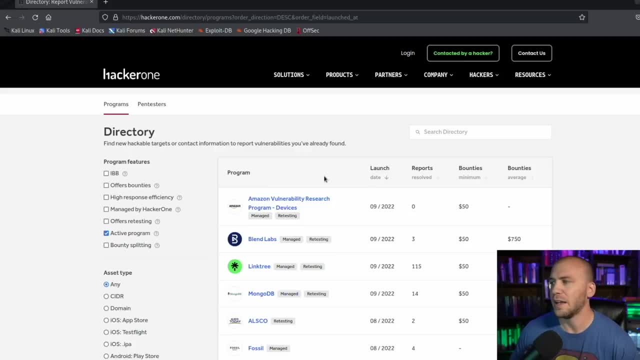 to have this feature work. So, if you're logged in, go ahead and log out and then you can look through here, And then, once you have them all sorted out, one of my favorite things to do is open them up and look at the scope And then, once you have them all sorted out, one of my favorite 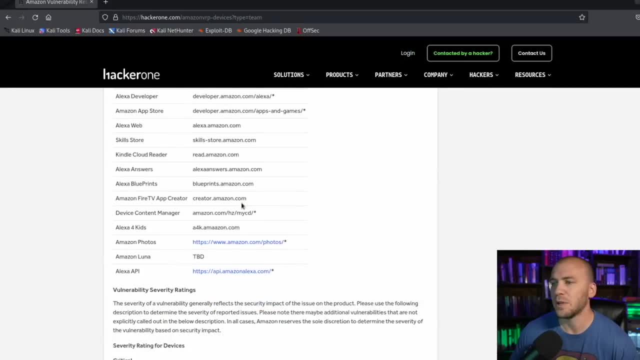 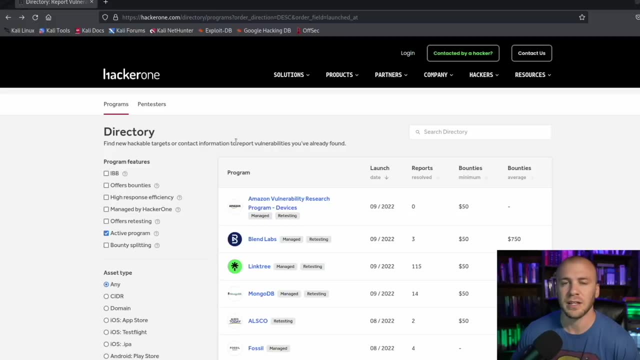 things to do is open them up and look at the scope. I like to see how big the scope is and make sure that there is a really large scope, because one of my personal biggest struggles is: I will open up a program and I'll get started And then in 20 minutes I find myself out of scope and this 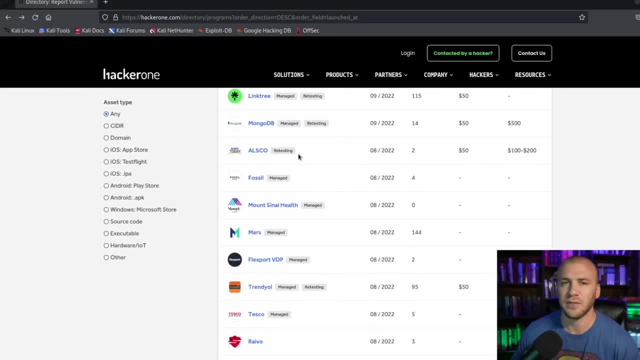 can be a problem, So I really like to have large scopes. It also means that you have a lot larger attack surface and there's going to be a lot more diversity in where different bug bounty hunters have been looking and testing, And so you're more likely to find a bug. 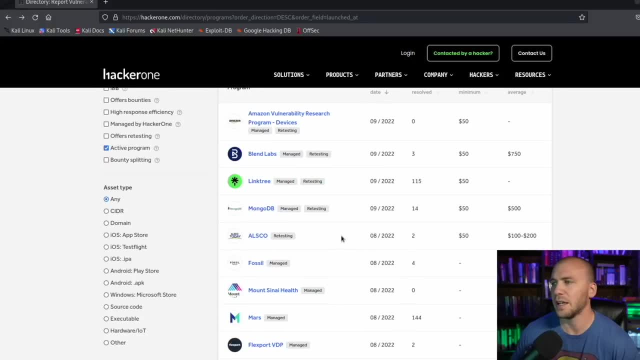 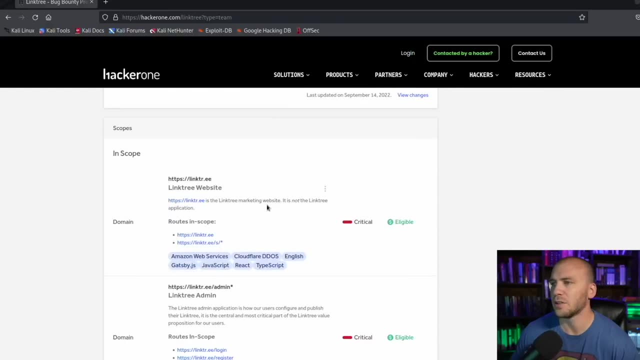 So let's go ahead and look at the scope. I like to see how big the scope is and make sure that there. Let's go ahead and scroll through some of these and let's look at some of the scopes. Maybe we can look at this link tree. I have actually never looked at this, but you can scroll down and look. 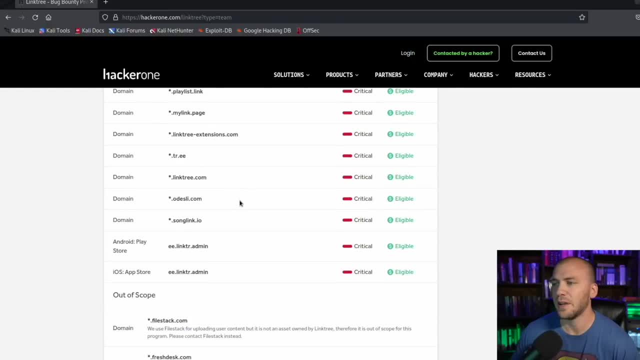 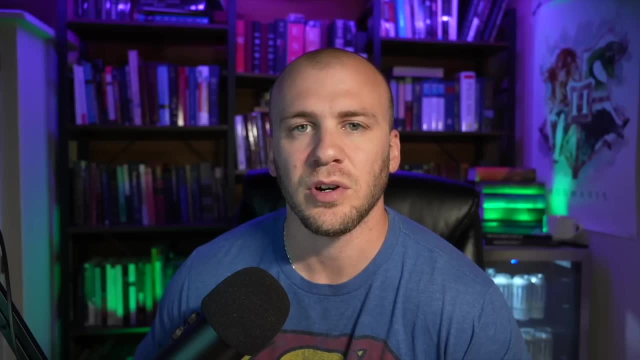 to see how large their scope is, And it seems like they have a pretty large scope, And then you need to make sure you stay away from these specific ones, And so make sure, when you are searching for a target, that it has a large scope. And one of the second things you should search for is 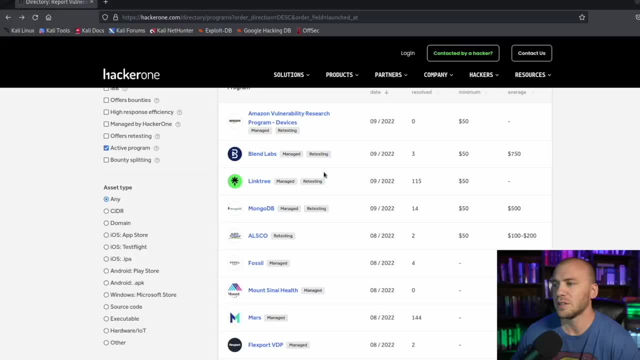 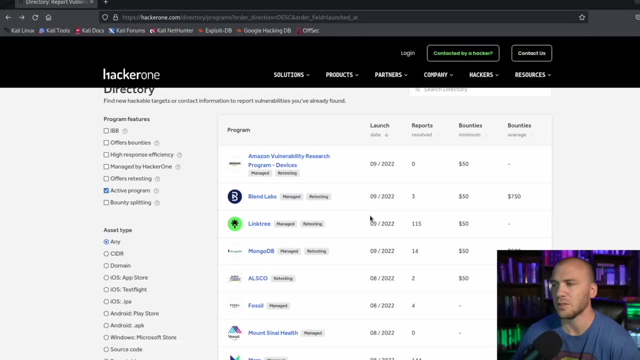 something that you're really familiar with. So I've noticed that there are a lot of scopes, that there can be a lot of currency trading programs on here, And I'm not familiar with a lot of the online currency trading programs, So that's something that I'm going to just avoid. But 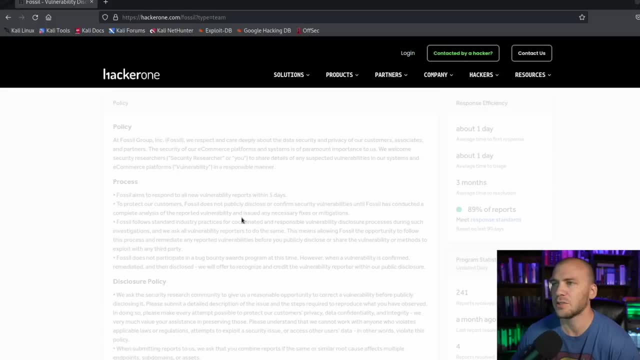 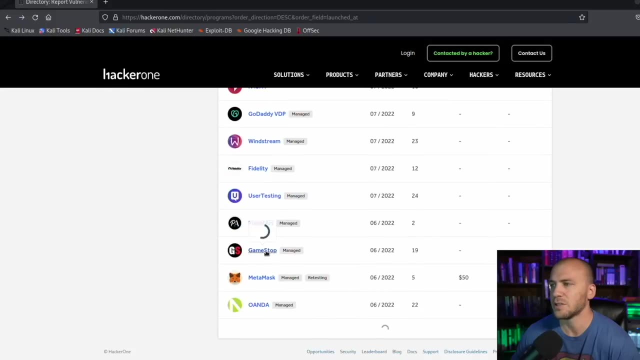 maybe you're into shopping and you're like I want to check out Fossil, I want to see what kind of scope they have, And you can come in here and read about it. Maybe you're really into gaming And I'm pretty sure here's GameStop. There are quite a few game style programs on here And you 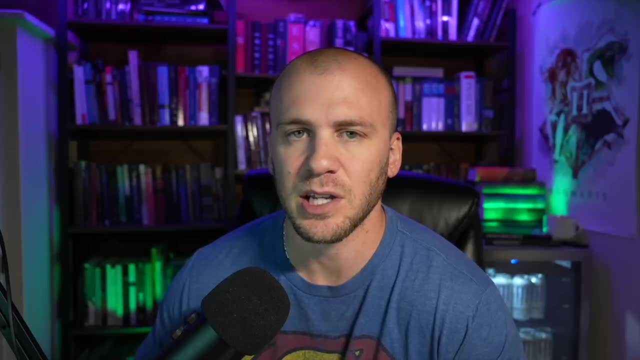 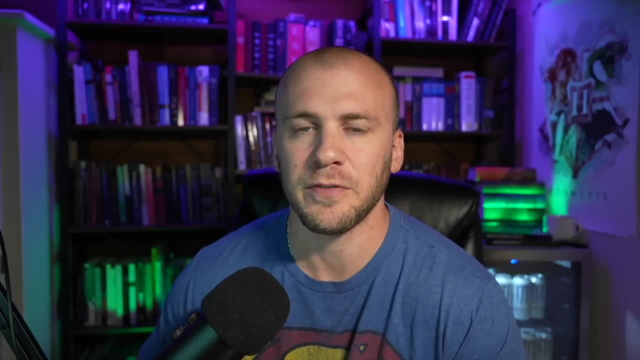 can go ahead and attack those. I'm pretty sure PlayStation is on here, GameStop is on here And if you're familiar with those websites already, those are going to be something you're going to want to attack because you're going to already know how the web app functions and what. 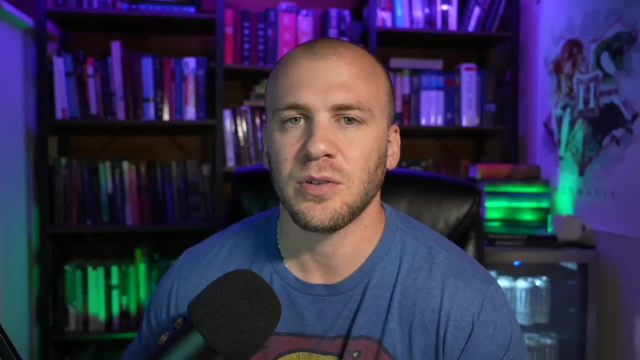 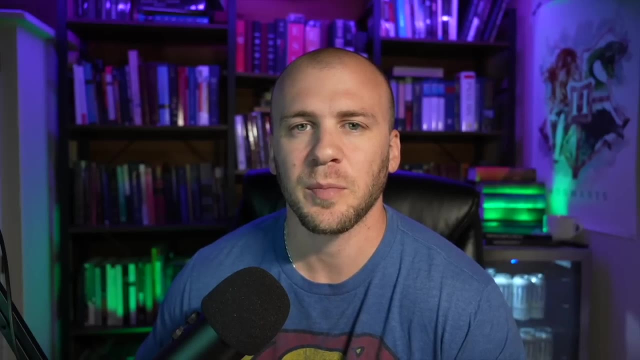 should be happening when you click on different links or log in. And so pick a program that you personally are familiar with and are already interested in. And a sub point to this is: pick a program that you're really interested in, because you are going to be interested in clicking through. 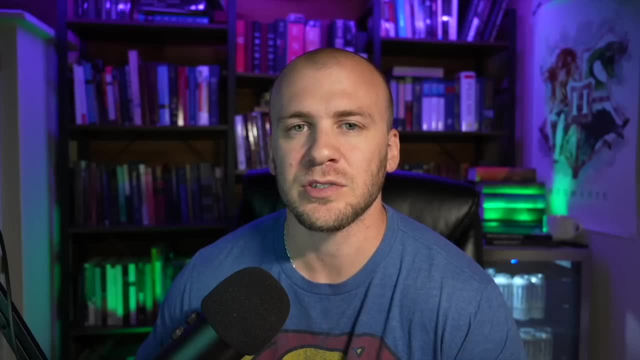 the website, seeing what's happening, what products there are, and maybe you'll be interested in looking at the products And it's going to help you figure out how the website functions, just because you're going to be a normal user And there's going to be things on the website that you want to look at and click through and 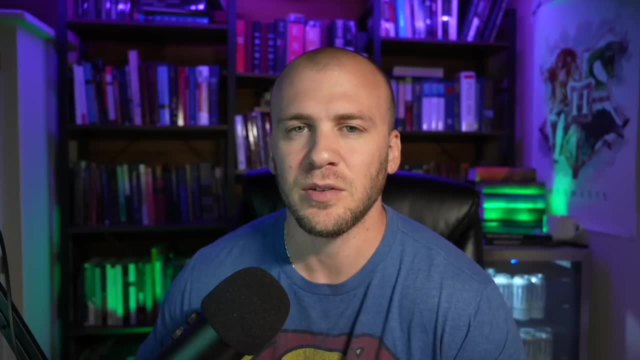 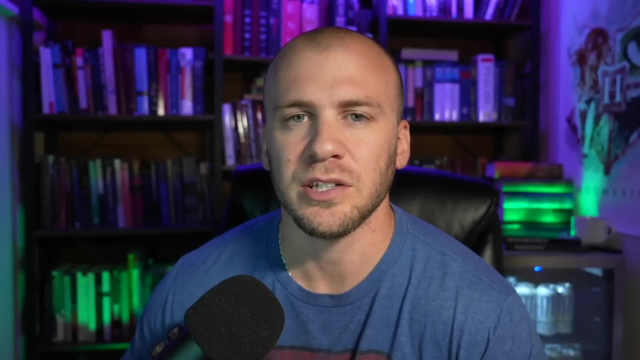 check out the functionality, but you're also really interested in what they have to sell. This is going to really help in keeping your interest, And so pick a program that you're familiar with, or one that offers some kind of service that you're really interested in, or 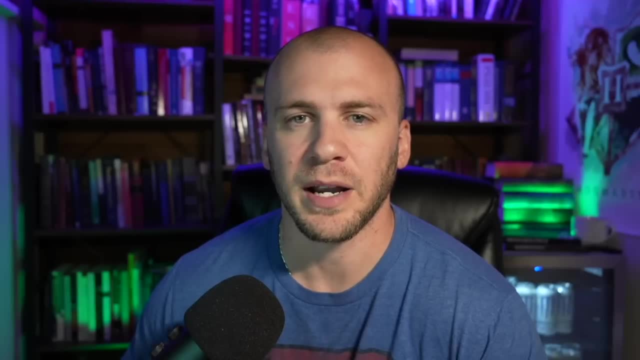 products that they're selling that you would be a potential buyer of. Now, the reason I told you to sort the programs by date is because the newer the program, the less likely they are going to have already been tested by a bunch of different penetration testers or bug bounty hunters, And 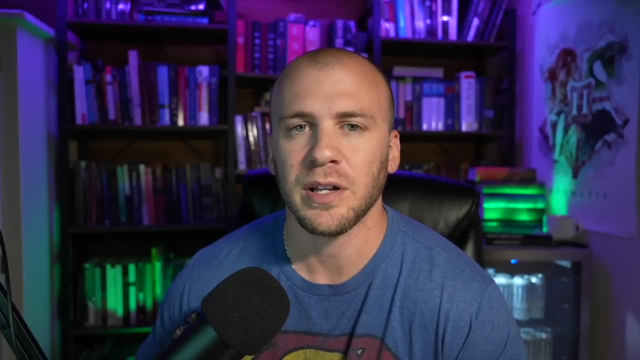 this is really going to help you land a vulnerability before anyone else, because the web application just hasn't been picked over as much as the older programs. And another tip to this- and is really popular and probably really common knowledge- is to choose a program that is unpaid. 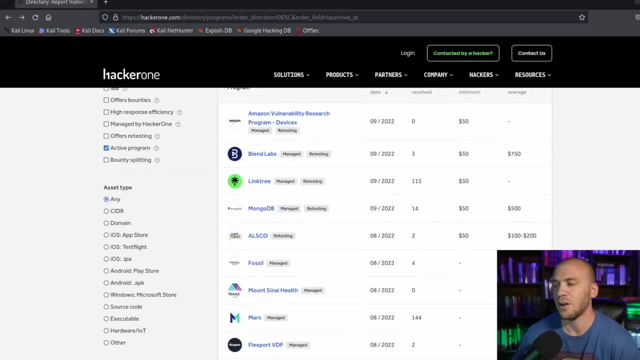 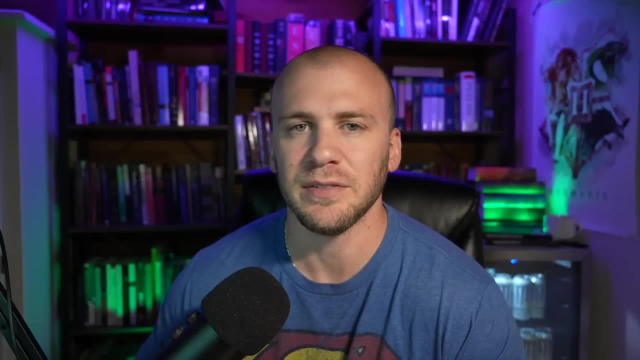 So you can come down to one of these unpaid programs and hack on one of those, because the top hackers are going to be going after the programs that offer rewards and financial gain, because they're doing this for a living And if you're just trying to get that first bug. 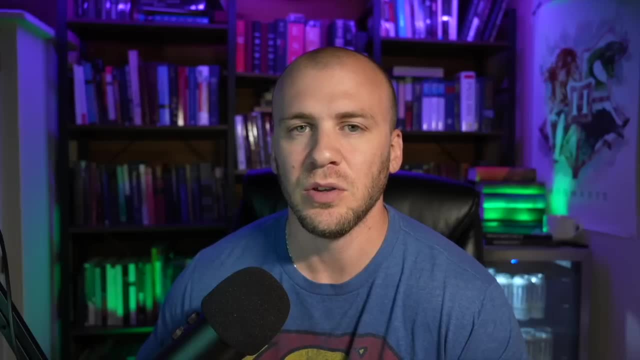 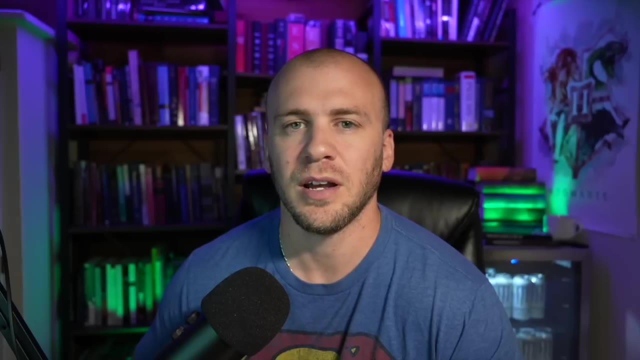 then you can go for the unpaid programs and then also the newest unpaid program. And the last tip is kind of an OSINT tip And I think this is really going to help you in your ability to find bugs based on what the developers are posting. So go on to all the social medias and 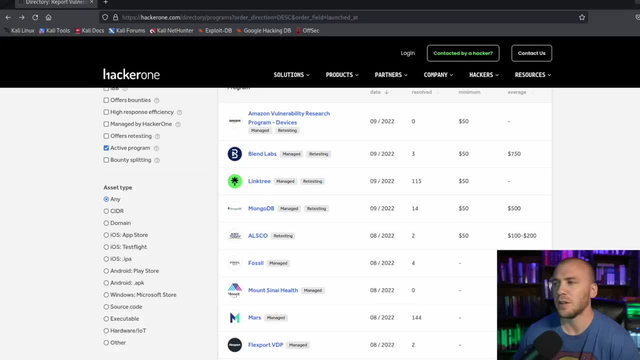 follow the developers that work for a specific company. So if I was going to come over here to MongoDB, I'd want to find the developers that work for MongoDB on Twitter, find their GitHub pages, follow them on Twitter and then go to the developers that work for MongoDB on Twitter. 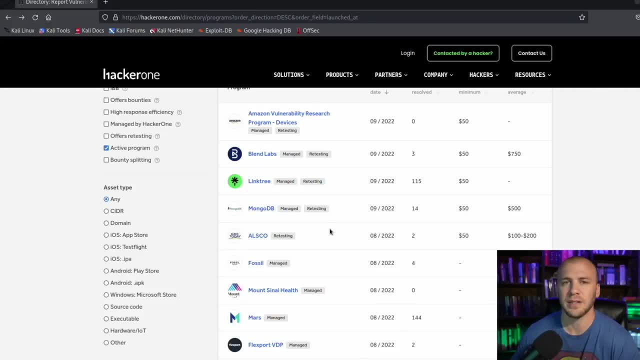 Any social media that I can, because developers will often brag about the different software that they're using and they're implementing into different projects. And then, lastly, they're going to be pushing their new code to GitHub, And if you are following them on GitHub, you can go. 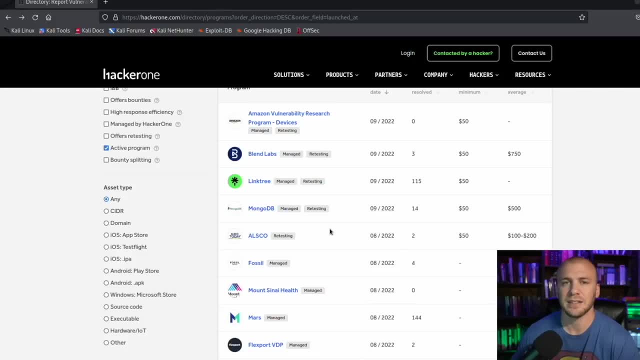 and check out the code that they have published before anyone else and see if you can find any vulnerabilities within there, or maybe they have pushed some sensitive information to GitHub that they otherwise shouldn't have, And so following the developers is going to be really helpful. And and one last thing the developers will often do is when they 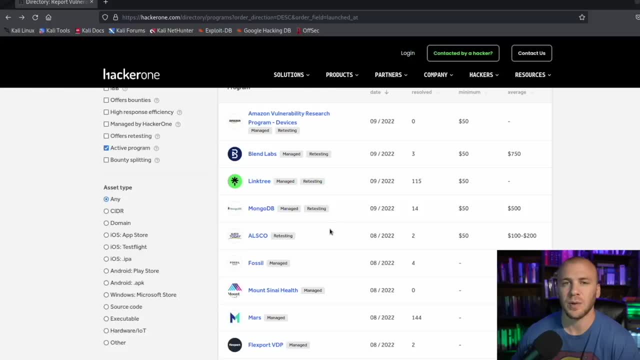 launch a new subdomain or a new area of the web application that wasn't previously launched. they'll often post about it and they'll tell you what is going on on that specific page. And following the developers is one of my last tips. and trying to choose a program, If there. 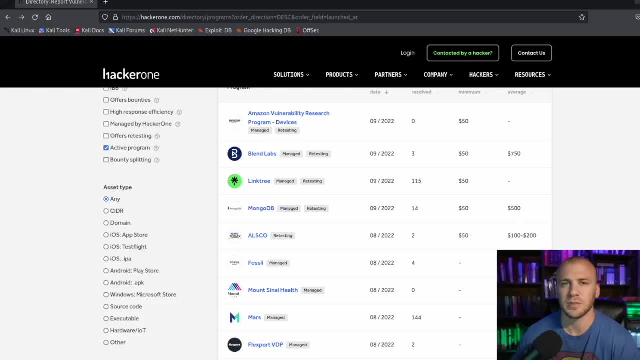 are a lot of developers that you have the opportunity to follow on a specific program. this is going to help you be one of the first ones to find new pages, as well as code that is being pushed to GitHub. Thanks for watching. I'm going to be installing a few tools here and it 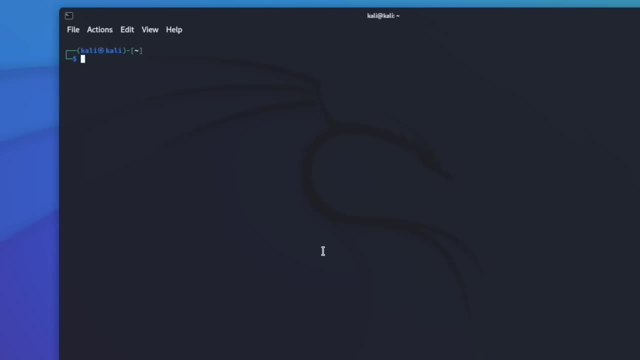 won't take very long. but the first thing I want you to install is gedit, And I already have installed it just like this. So if I hit enter, it will pop open this little text pad for me here and I can write information and create files. I like to use it instead of nano or V or vim. 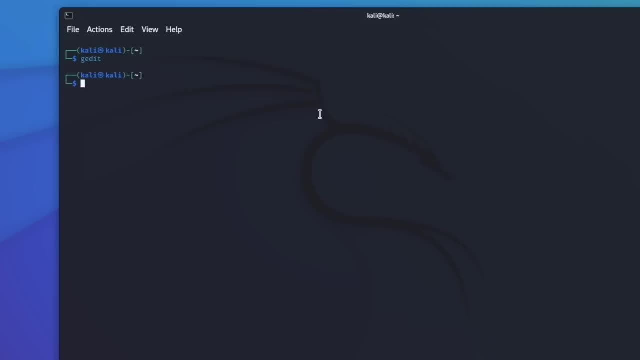 because it's just a lot easier to move around. I can actually use my mouse to click around in that side of the text file. So the way to install this is type in a pseudo apt install, just like g, edit. you'll hit, enter into your password and it will install for you. And then the second thing: 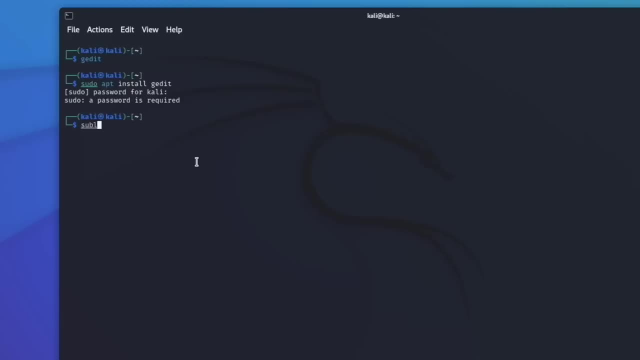 I want you to install is sub lister. So if we type in a sub lister like this, not like that, like this, you can see that it doesn't do anything for me. but if I type in pseudo apt install and I 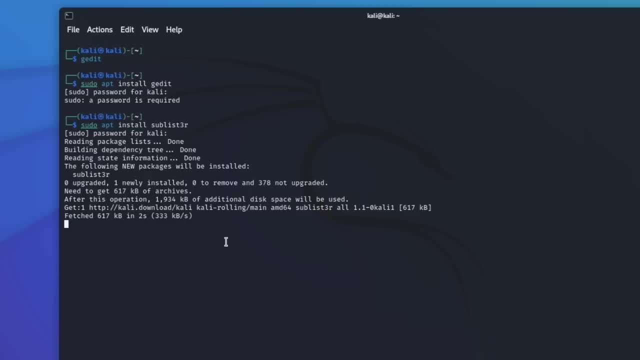 hit enter, type in your password. it will go ahead and install sub lister for me. And now, if I type in a sub lister like this, it will turn blue and now be ready for me to use And we will install Thuf. I don't think Thuf Oh. 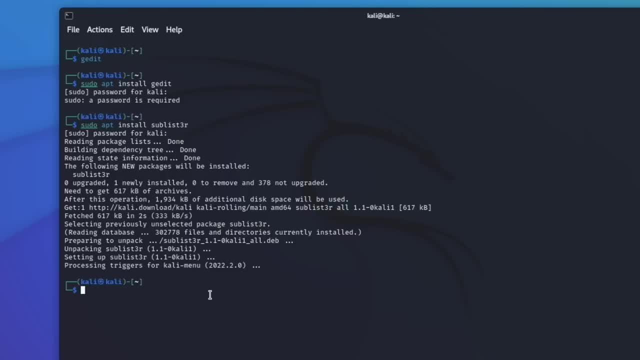 it is already on the Akali box, So we don't need to install any other tools. Those are the only two we need to install And we will go ahead and start looking at how to use the most common tools for the world of bug bounty hunting- One of the most popular tools for finding sub domains- And 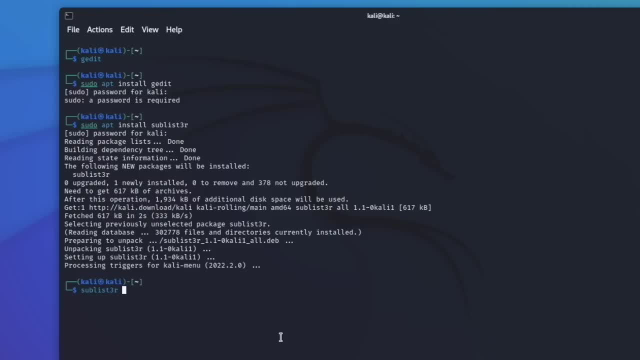 the way you use it is just type in sub lister, just like this, And then we'll type in the domain you want to pull down sub domains for. So we'll type in w, w, w. we need actually a dash D in here. So we type in dash D and I think we can actually just type. 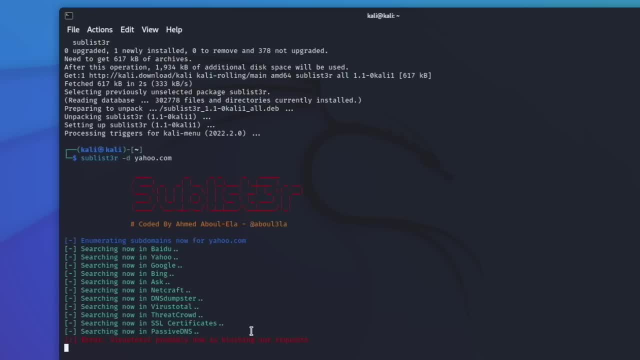 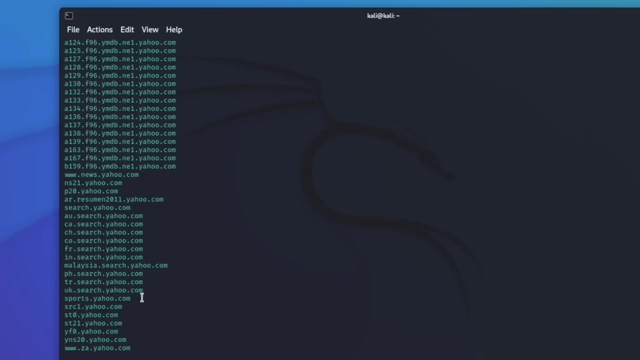 in yahoocom and hit enter and it will automatically go out and start searching, raining for subdomains for us. One of the important things to know is that when it pulls down subdomains for us, not all of them are going to be in scope and you should definitely check to make sure they're in. 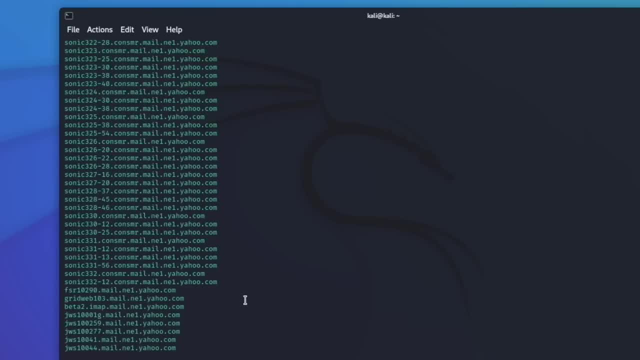 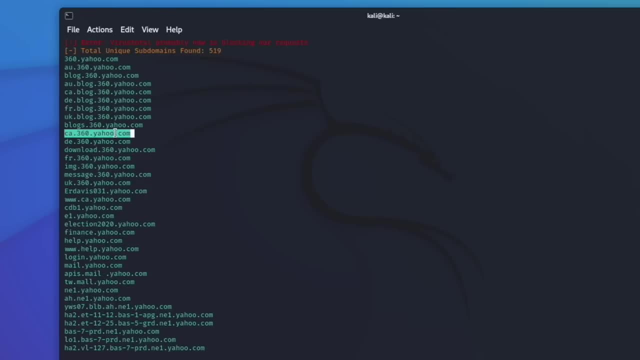 scope And some of them may not even be For the, even be owned by your target. so in this case we're looking at yahoo and some of these might not even be owned by yahoo. so one of the things i like to do is, if i just open up this url right here, 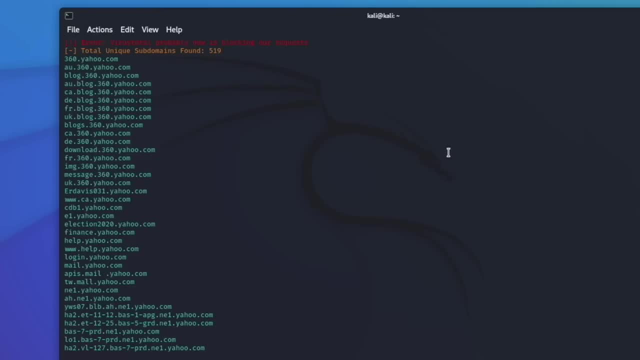 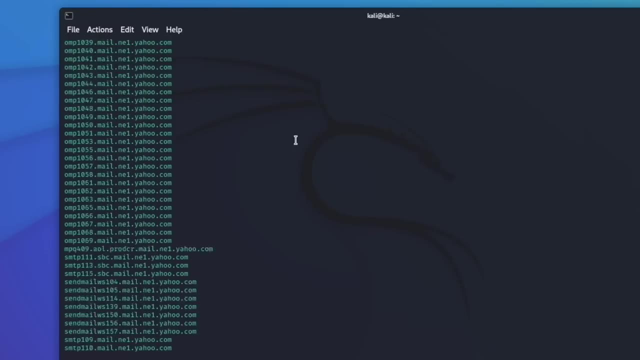 and at the bottom i like to look to make sure that it says it is owned by yahoo and so this is sublister. this is a great way to pull down subdomains. there are other tools and other ways to use this, but this is one of the most common and from here we can actually brute force other 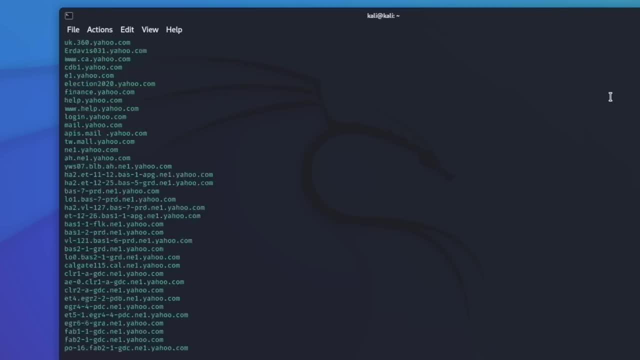 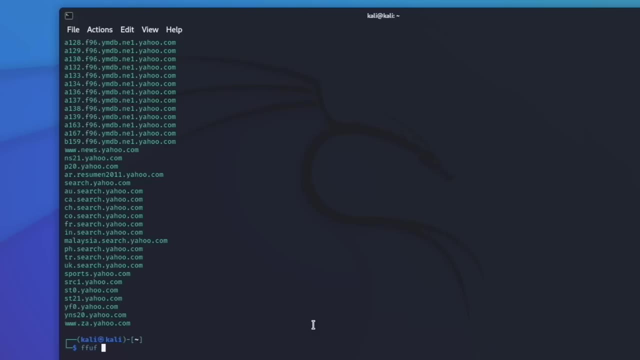 endpoints with fuf and we'll go ahead and check that out. so, with thought, this is one of my favorites because because when it brute forces it goes so quickly i actually like to slow it down. or if i do run fuf, i always use a vpn, just just in case my ip gets banned. i can just change. 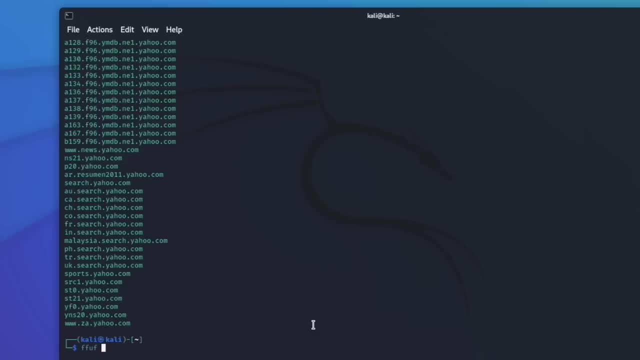 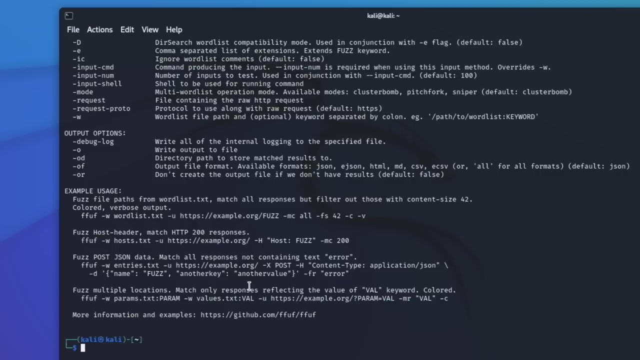 my vpn to another ip address and continue on. but i usually do slow down fuf so that way the server doesn't think i'm trying to dos it. so when you use fuf it would look something like this: we can type in a fuf dash help and look at the usage we're shown. 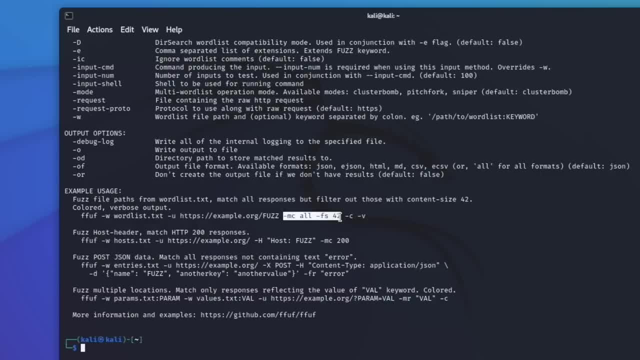 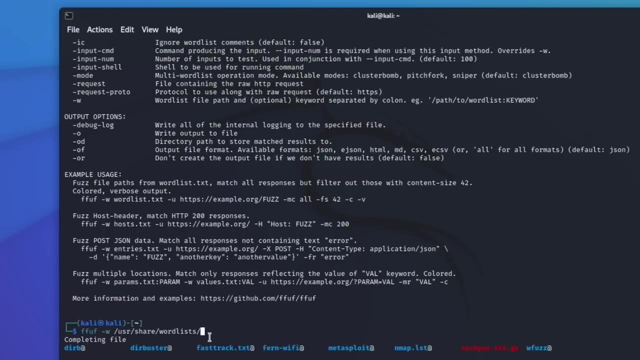 right here. you have to have a word list and then there's some other flags in here and the url. so what we would do is use fuf dash w and then we can go. i think we can type in user share word list. what are my options? derb, slash, smalltxt. 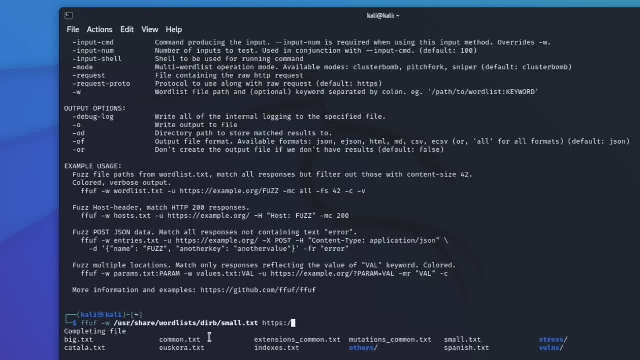 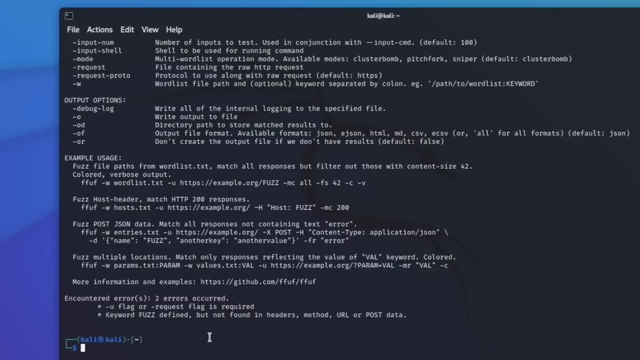 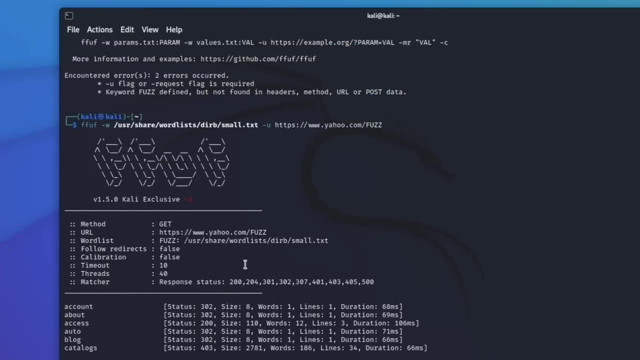 word list and then we would type in https, wwwyahoocom. and then we type in fuzz like this: if we hit enter, we need to have our dash u right here and if we hit enter, it'll automatically start brute forcing for us right here where we put fuzz to see if there are any extensions. 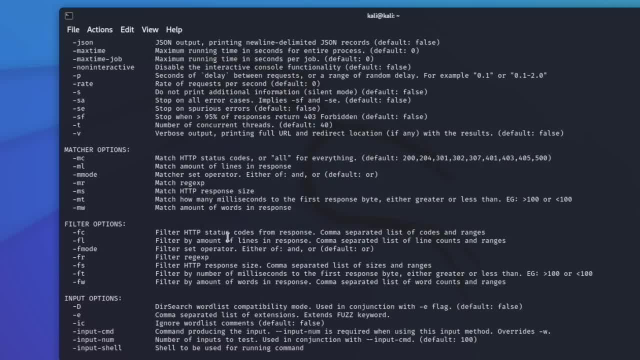 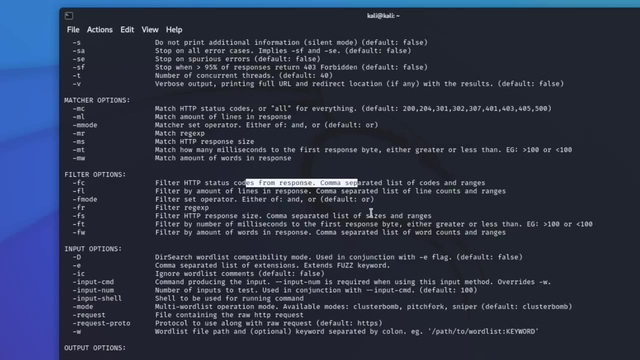 that we can find a few things to note. we use the dash p right here for the delays and you can also use the filter options right here in order to filter out. let's say we wanted to filter out by a response code or we wanted to match a response code we could get rid of. 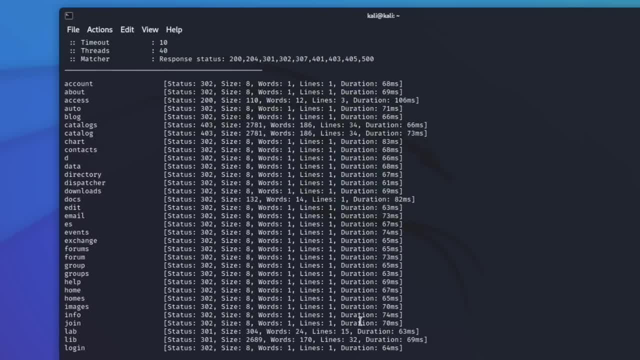 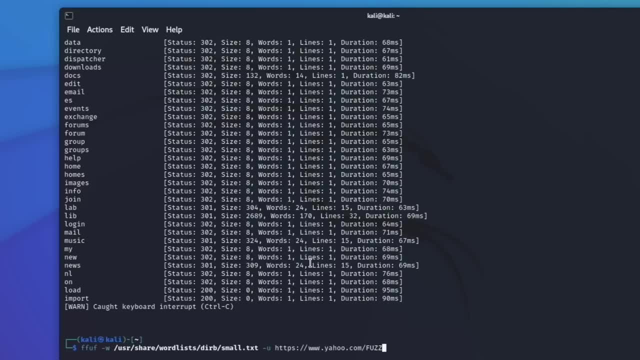 these 302s right here or anything that has one line or let's say one word, and we can just filter out with fuf that way. so that way the output doesn't go quite so quickly. so we can just come up here and we could say: 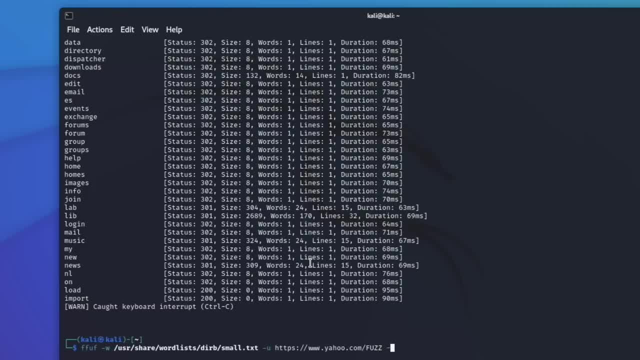 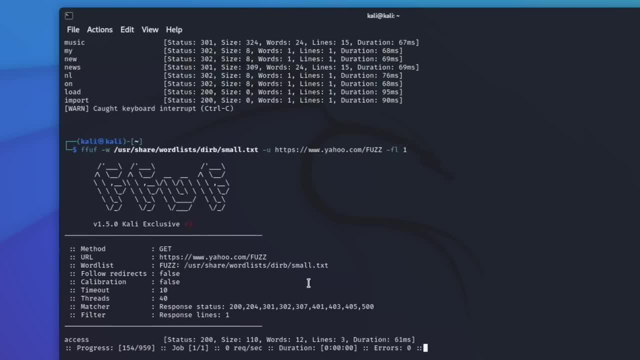 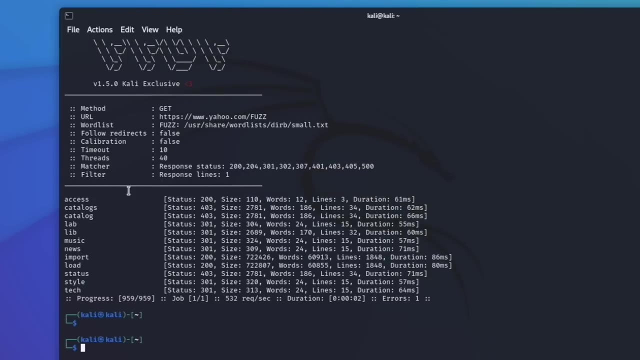 fl. so we're going to filter out. we need a flag dash fl and where we could filter out by the line right here and we can say anything with one line: don't return it to us. and now you can see it running and what is brought back has more than one line on it and there's other ways to filter these. 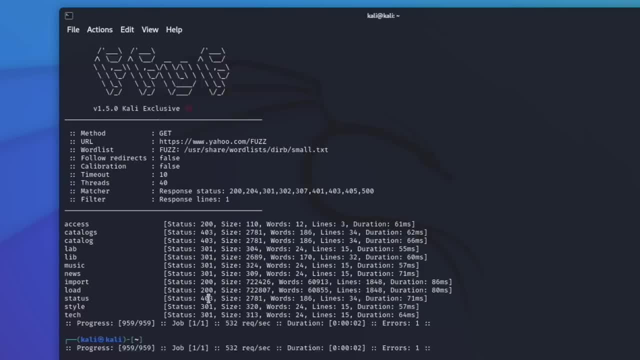 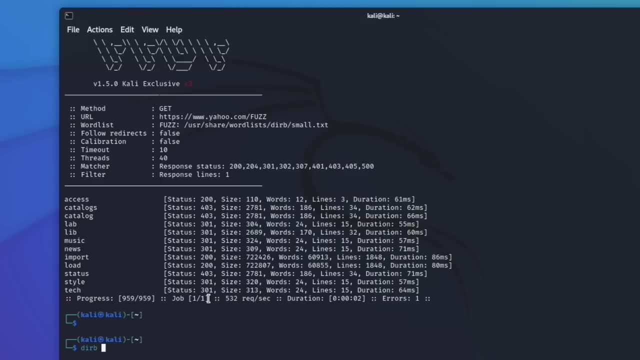 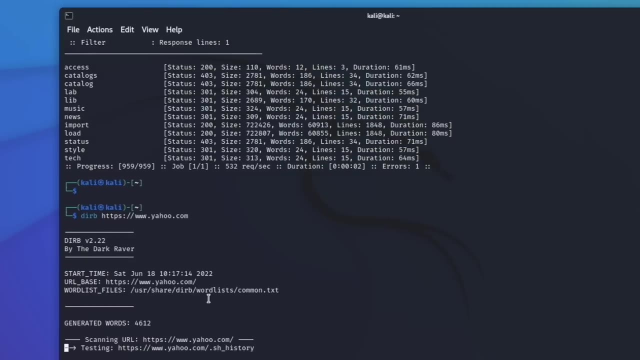 out and you can go ahead and play around with fuff. it is one of my favorites. the other one i like to use is derb, because it's really simple. you just would type in derb and then you type in the url that you want to attack, and then you just hit enter and it'll automatically start testing. 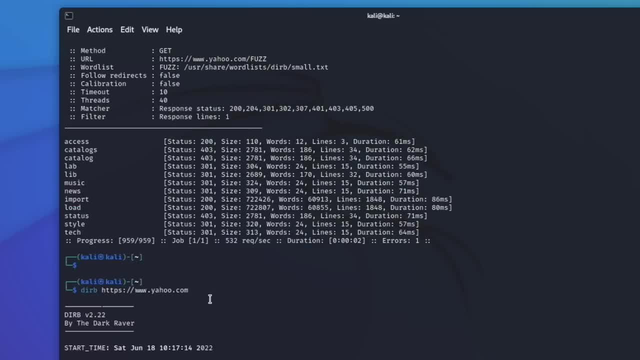 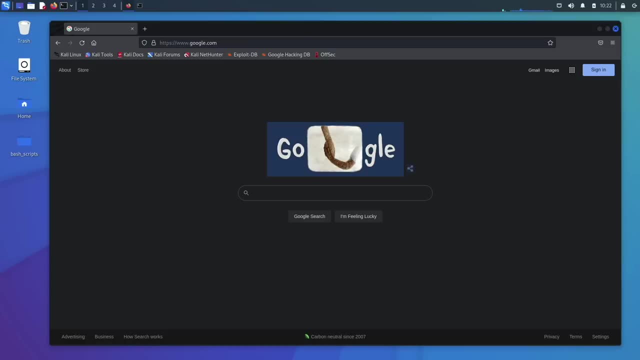 for you. so those are my two favorites. i like to use derb if i just need to do something quick and simple. if i'm looking for speed, i will use fuff. all right, there is something called google dorks or google dorking, and i'm not really sure why it's called this. so if you know, you can. 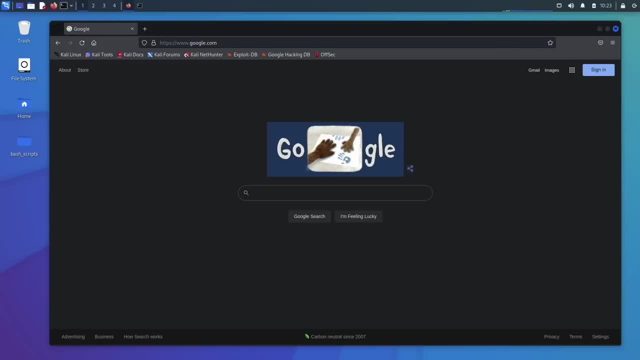 leave a comment and let me know why it's called google dorking. because that's what it's called, because that just seems like a really weird name to me. maybe i could google it and find out. but the thing about google is pretty much everything on the internet is stored inside of google, the 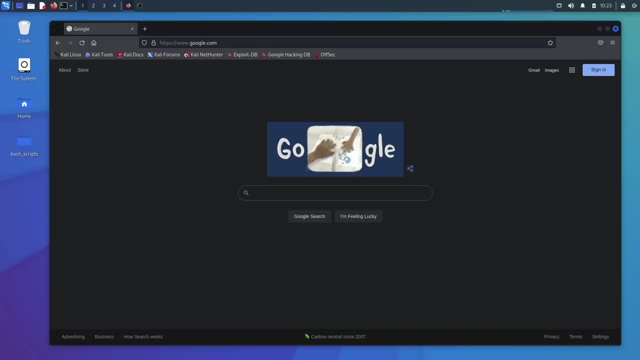 search engine. you just have to know how to look for it. google is constantly crawling the internet and storing new files, new urls and more information into their database. you just have to know how to find it. so let's say i was looking for for a doctor named charles hodge. what i could type in is just charles. 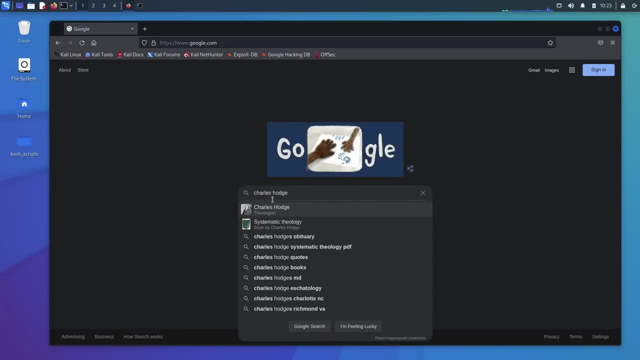 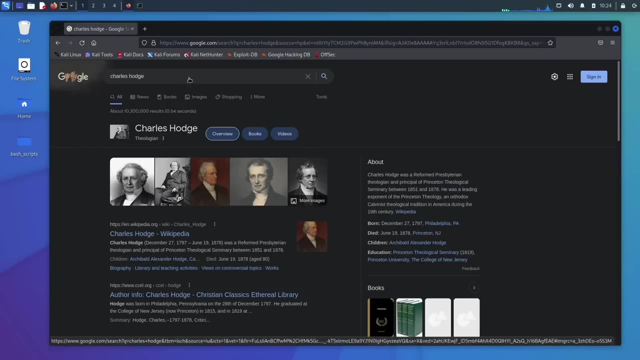 and then type in: hodge, we'll go with charles, charles hodge right here. this is what i was going to use and we hit enter. this was princeton theological seminary's president, but this is not the, let's say, md that we're looking for. what you can do is just add quotations and put in md and 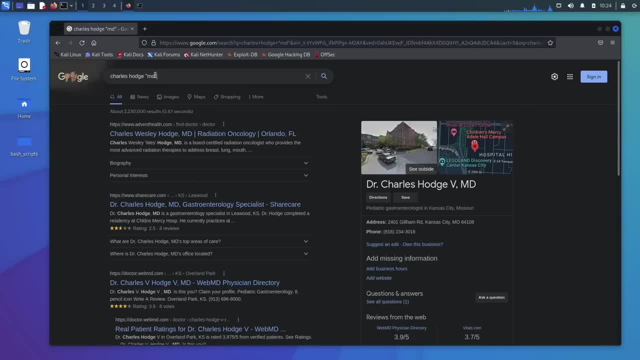 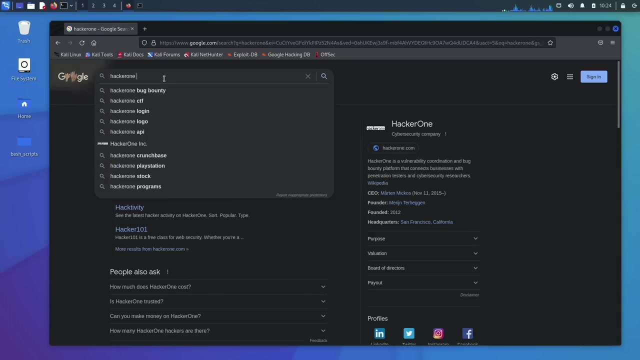 now everything that comes back will be medical doctors or you can put in literally anything you want into these quotations and it will find it so. an example of this is: if we say we want hacker one, it'll pull up hacker one. and let's say we want the hacker one programs. if we type this in, it'll pull. 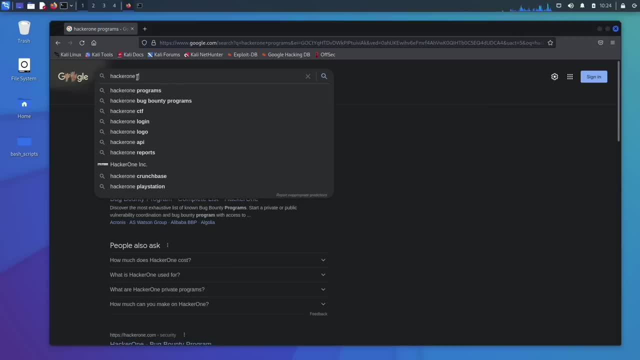 it up for us anyway. but what we could do is add in the quotes just like this, and say the programs and hit enter, and now everything that comes back will have to have programs inside of the search. so this is one of the ways to use the google dorks. you can also do this with github as well. 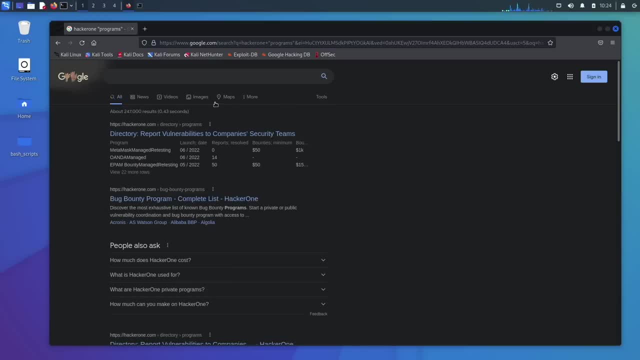 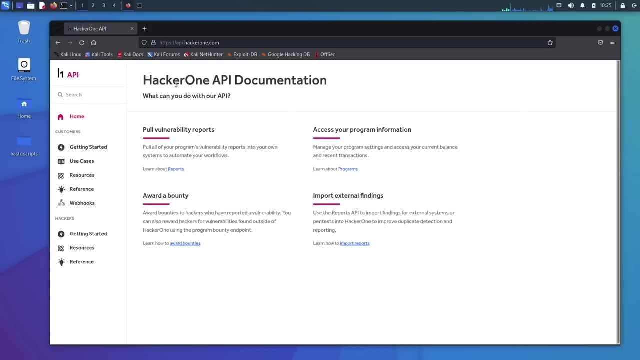 when you are searching through the github code, you can type in the a specific word, like, let's say, we're looking for hacker one, and then we type in quotes and we want to look for an api. it'll pull down what has an api and then you can come in here and you can look to see if they have an api that. 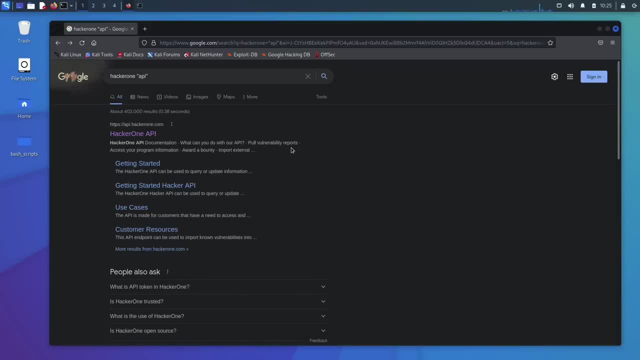 you can use. so using quotes within google will help you narrow down your search and you can see your search and what is brought back. and, as i mentioned, this is something that you should do within github as well, when you're searching for, let's say, api keys or passwords or something of. 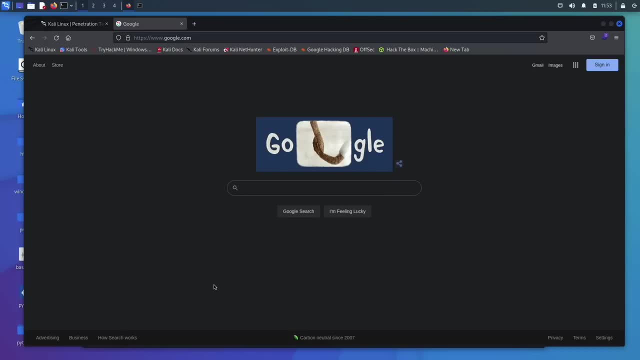 that nature. and now we're going to move on to burp. okay, in this video we are going to be setting up our proxy burp and right now, if we just hit enter on google, it loads. just fine for us. but when we set up our proxy, we will. this is going to not work and i'm going to show you how to. 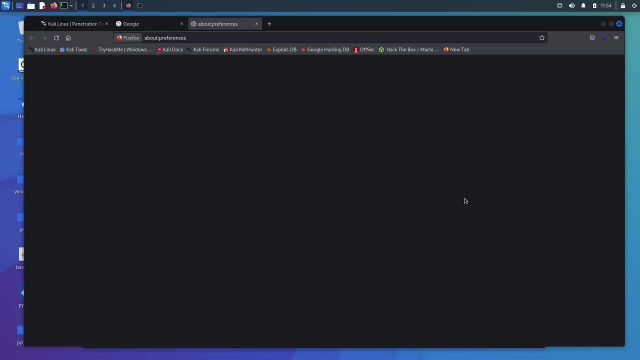 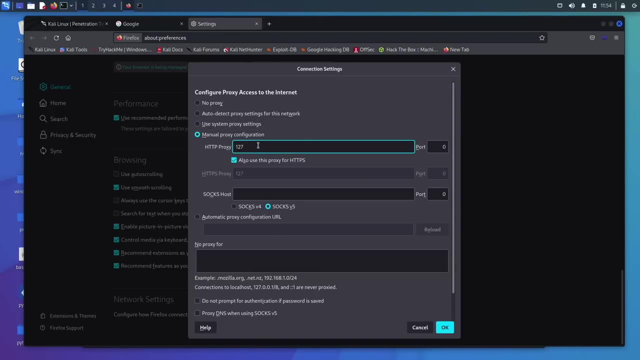 set it up. so we will come over to these three lines. we'll go down to settings. scroll all the way to the bottom, click settings, go manual proxy configuration. we're going to go 127.0.0.1 because this is the default with port 8080 on burp. so if we say okay to this and we come over to google now, 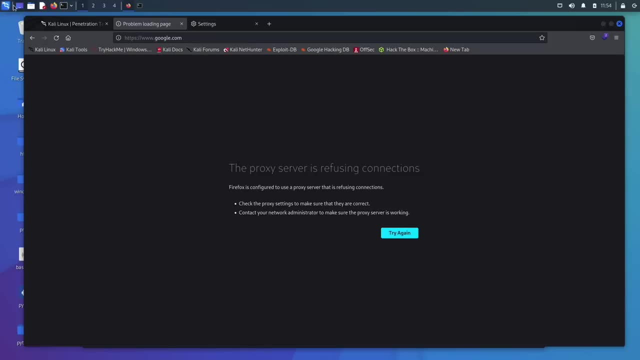 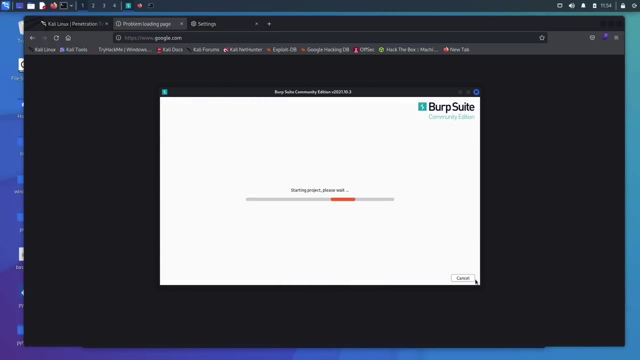 and we try and run it, it's going to tell us the proxy server is refusing connection and we will need to open up burp. and if this is the first time you've opened burp, there might be quite a few things you have to click through in order to. 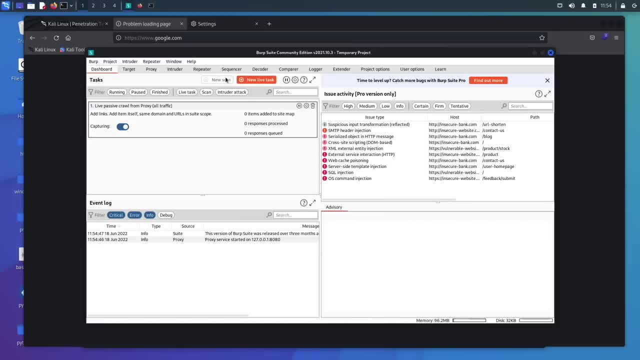 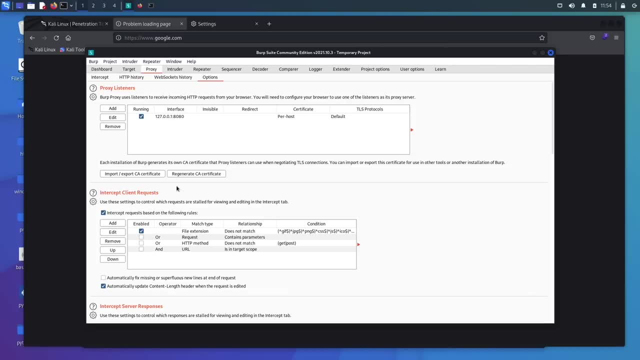 actually get it to open. but once you get it to open, it will look something like this. so if we come to proxy and options, you will see right here this is what we have set up and we're going to need to import these certificates. so you'll click this top one next and we are going to go next. we're. 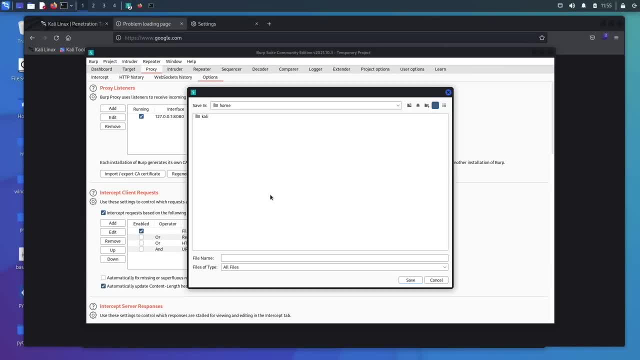 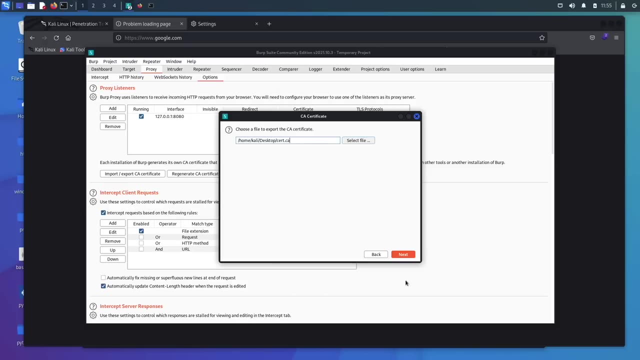 going to open up file i guess we're going to select, we're going to have to, and in the file that we select we'll go to our desktop. this is a great place to store it. so we'll name the file certca and we can save this. it will save to our desktop. we'll say great, and now that this? 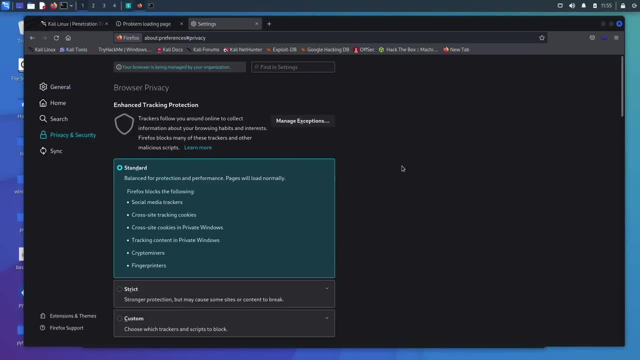 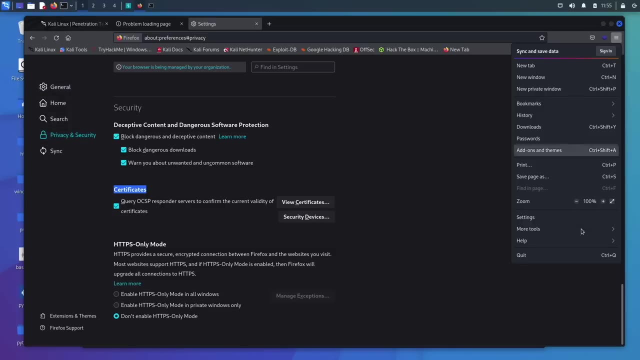 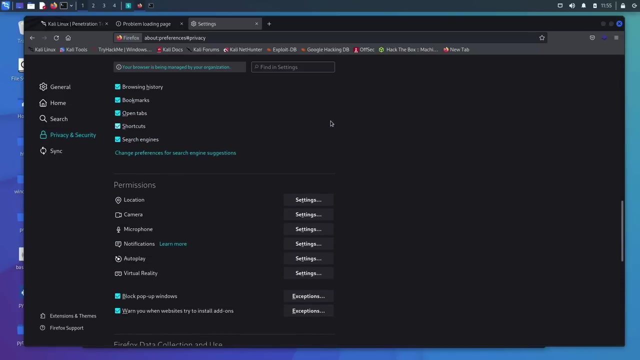 has saved. we're going to need to add this into our security. i've already added it in, so i'm not going to add it in again, but it'll look just the same. you'll scroll down. once you've gone three lines to settings, we'll just show this again: settings, privacy and security. scroll down. that was too far. 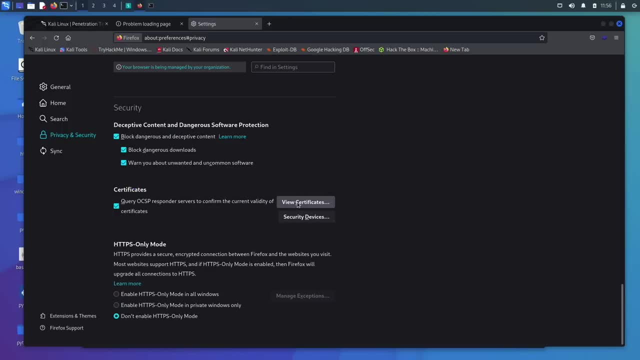 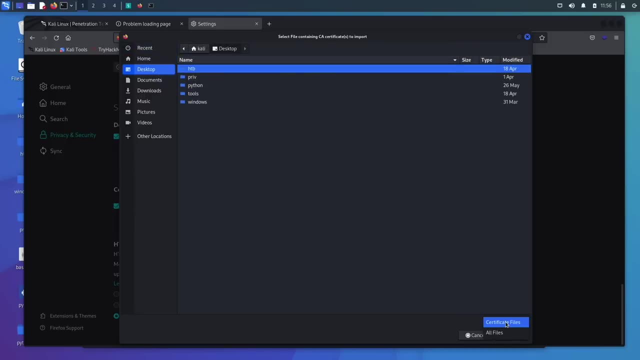 scroll down to certificates- i guess it's all the way at the bottom, you'll click view certificates and then you're going to import and we're going to go to our desktop and we're going to say we want all files and then we're going to save the cert that we just opened. you will click open and 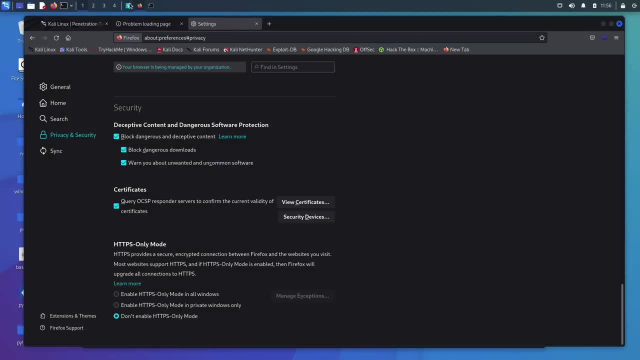 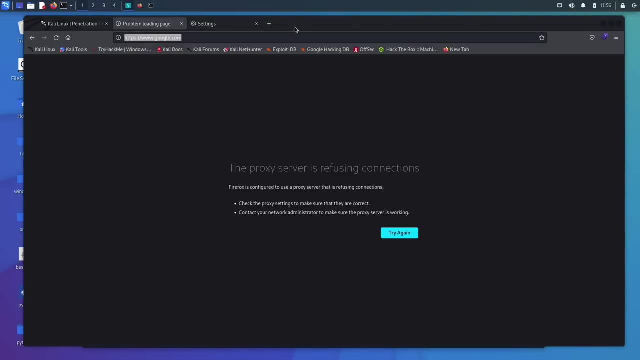 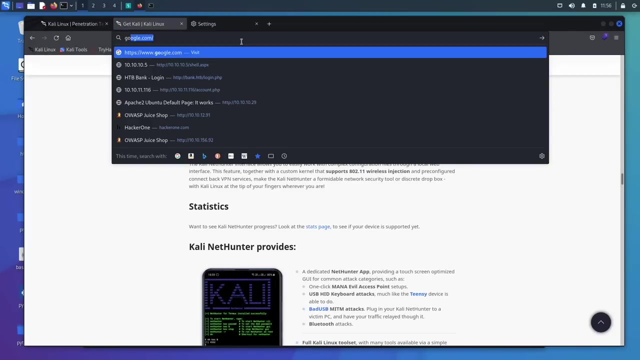 i have already installed it. so we'll say okay, okay, and now when we come back over here to google, we'll need to turn our proxy interceptor off. we can test it to make sure it works and it does. i accidentally clicked one of the little tabs down here. so if we say google, 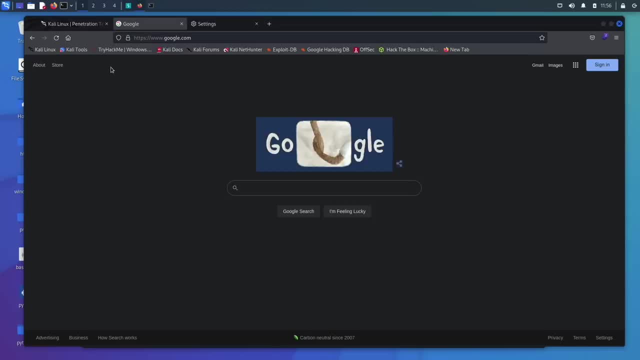 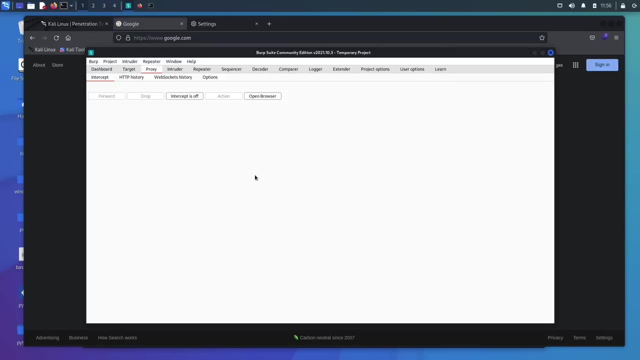 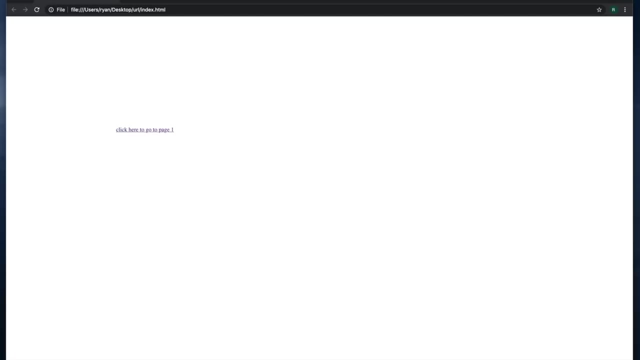 we are now running as we need to, and, if we need, we can intercept a request, just like that, but we're not going to get into that just yet. so that is how you set up burp and we will continue on. okay, we are going to be starting our url portion of this course. just what exactly we can. 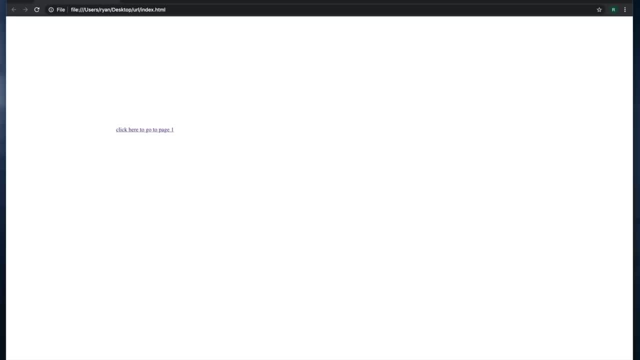 learn from the url what we can do in the url, which is actually quite a bit. the url is actually something that you can learn about how the website functions. you can look sometimes you can see information. personal information, sensitive data can be stored there. so, for example, if in this url, 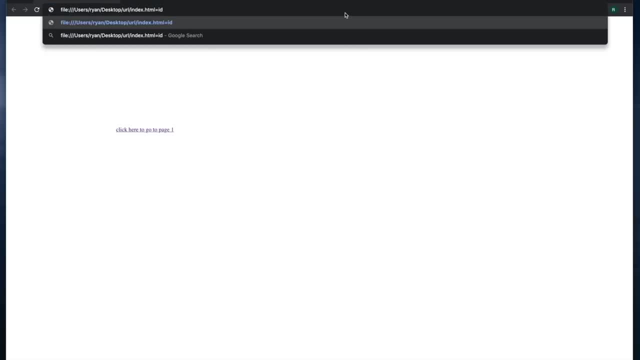 it had an id of my name or my email address. those are things that you wouldn't necessarily want in a url or, specifically, if a password was in there. those are things that you could actually report if you had sensitive data in there. but we're basically going to be looking at how we can. 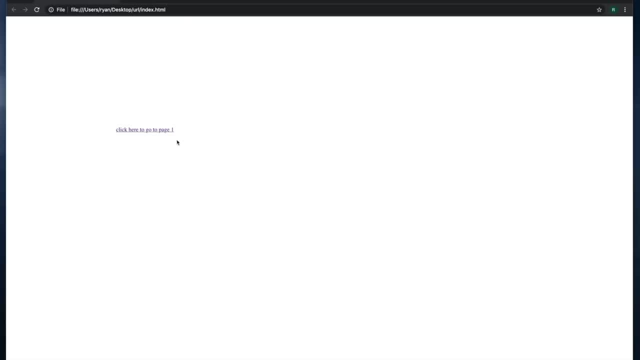 manipulate the url to our advantage and what we can do specifically with pages. so i remember when i first started down this path of wanting to learn web app pen testing. sometimes you'll go to a capture the flag website and it will be just a blank page and i remember coming to the blank. 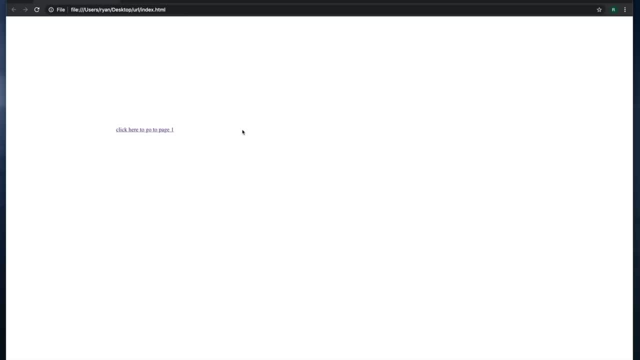 pages and thinking: oh, my goodness, i have no idea what i'm supposed to do. but for you, we've already gone through the recon portion of this course and you know to go to derb and just start looking for directories. and then also we're going to be looking at how we can manipulate the url to our advantage. 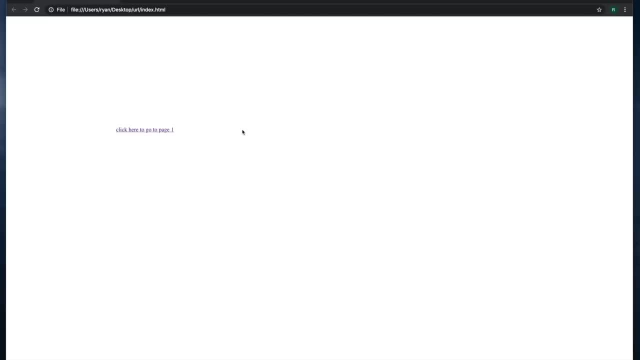 so we're going to be looking at the source code. i mentioned it briefly earlier, but it's something that can be really helpful, and i'll show you why. so i made this very, very basic html website. what i'm about to show you something that derb would probably find, but if it doesn't, you can kind of 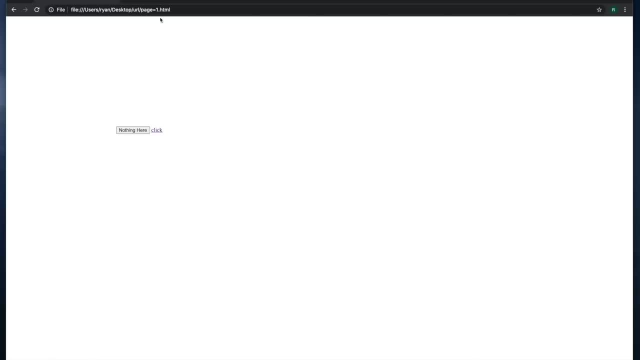 see how this is going to work. you can come in here and you can just go page one, and then you can go: okay, well, if there's a page one, is there a page two? and then you hit enter. oh, page two is blank. and then you go page three and then you hit enter. 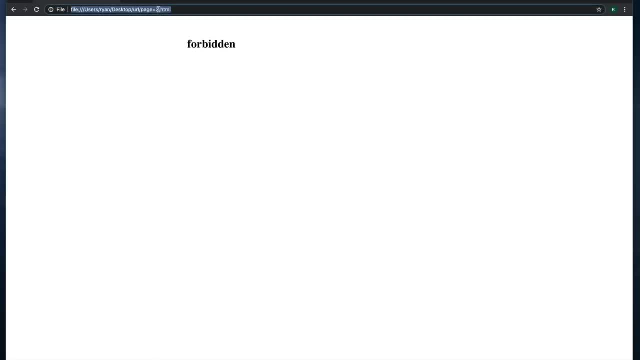 and we hit a forbidden page, and so if we have this forbidden page, there's something on it that we're not supposed to be able to access. well, how can we get there? this is when remembering looking at source code can be really helpful, and so we can come over here and we can go. 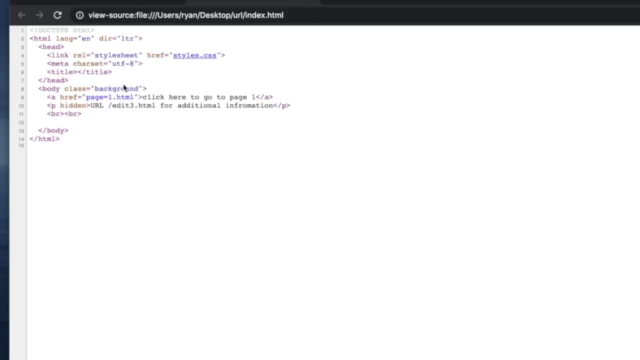 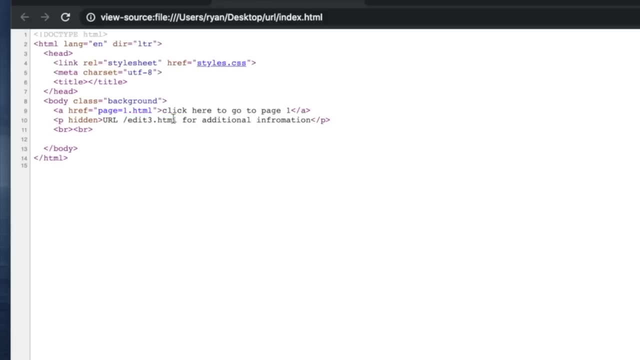 view page source and you can look through and see just how basic this really is, and you can see that we have something hidden and you can go there is this directory or this file for more information, and so you can come here and you can copy this and you could paste it in. 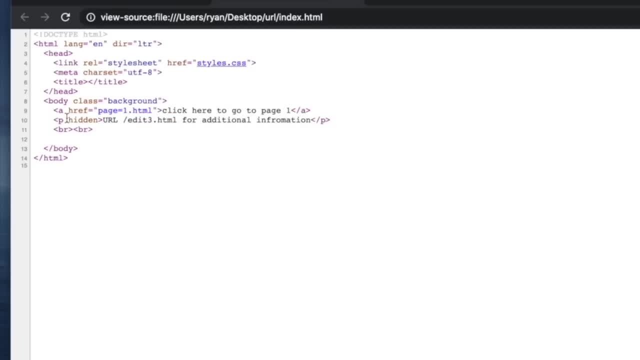 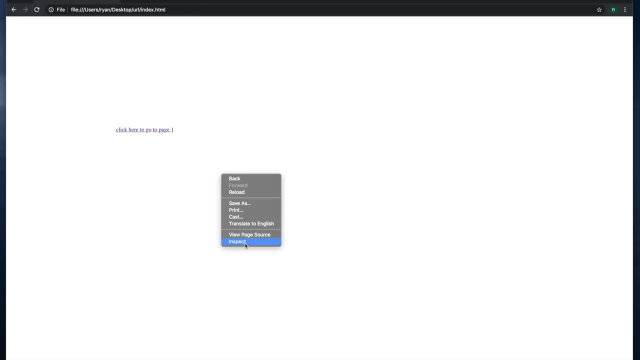 up here. another way to come across this is you can see that this is hidden. we're going to cover this in more detail as we go through the course, but as you go to this, the source page- one other thing that's really helpful to look through is to right click and just go inspect. you can inspect. 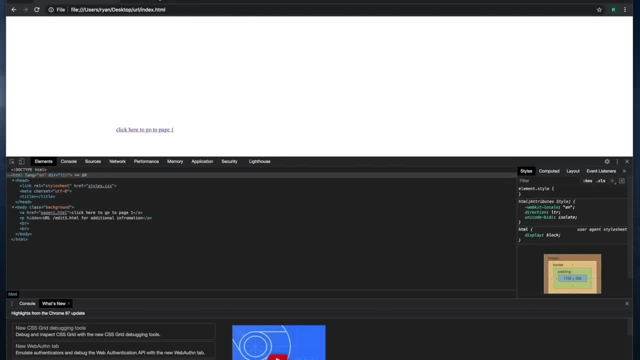 what is on the page. so basically, the same thing that we saw was the source, but you can see where this is hidden. sometimes you will have login pages and there will be hidden fields that you can open up and try and manipulate, and you can just actually type this into text and it'll. 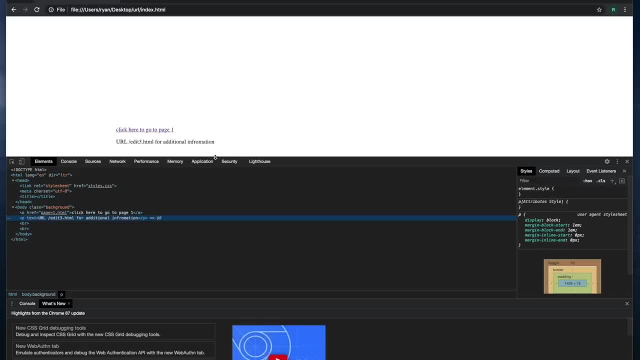 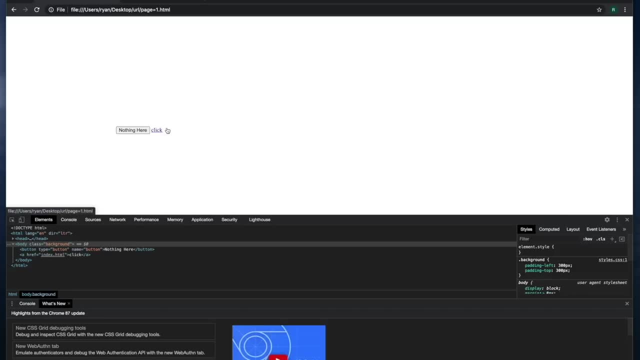 actually show up on the page as plain text, and so we have this file here. if you remember, we had page three was forbidden and we're not able to enter into it, but we can try. this html actually won't be on any website, so i just didn't take the time to remove it, and so we'll ignore it and act like it isn't there. 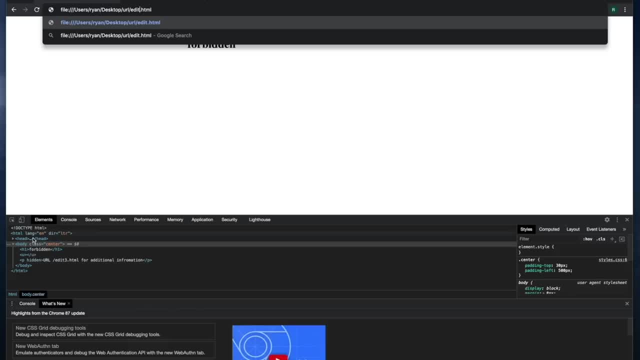 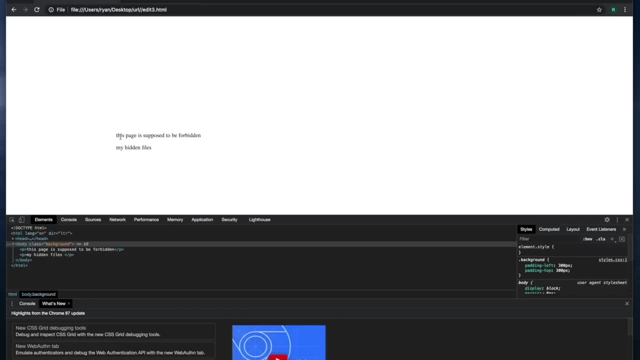 but if we remember from this, right here we have this edit 3, which i'm guessing is our page three, and then this would be: this is the forbidden page, where you can access files. now we're actually going to go and practice something very similar to this, and when you do, 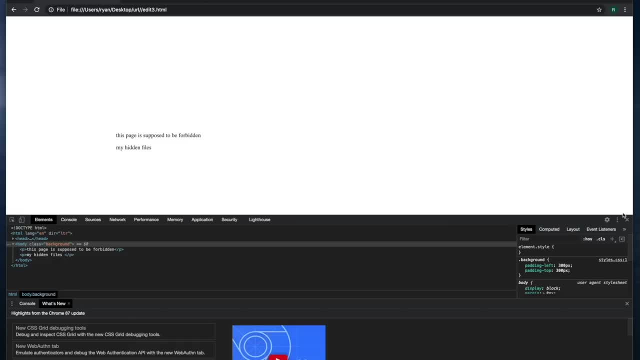 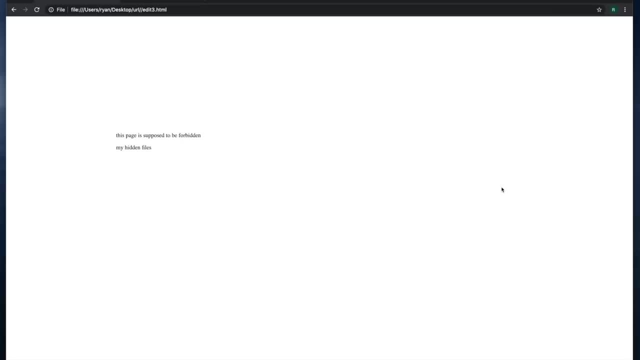 this. what you're going to need to do is go to google- i would encourage making a new gmail account and then going and signing up on hacker one- and then we're going to be using hacker 101 101 to practice what we just saw. for us to be able to gain some practice. It is a CTF. 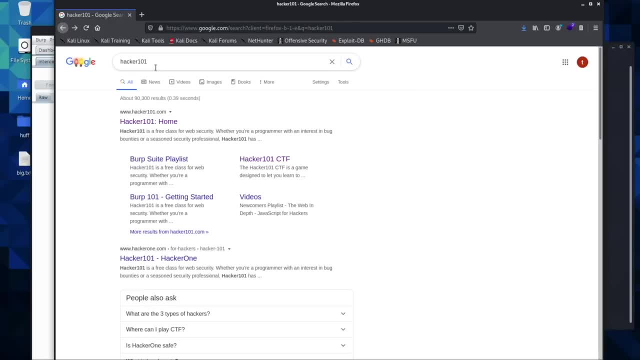 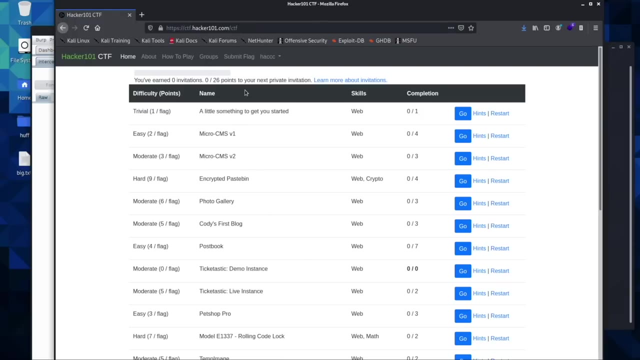 Okay, we are going to set up our HackerOne account. you can actually come into Google and type in Hacker101.. This is going to be their capture, the flag practice area, And you can actually click this. and what will happen for you to actually? I've already logged in, But what will happen for you? 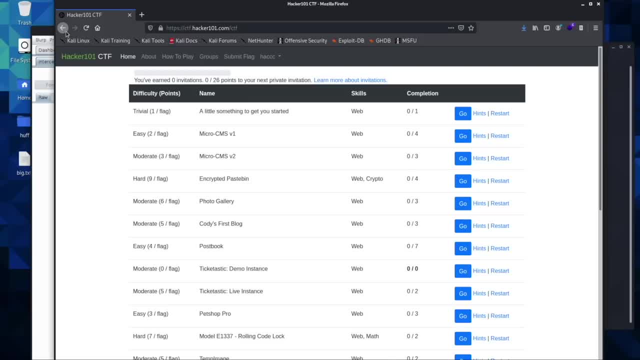 is it's going to say it'll bring you to a login page And once you reach the login page you will have to go and create your own account with HackerOne. And once you create your account with HackerOne, you can navigate back to Google, type in Hacker101.. And then click on the Hacker. 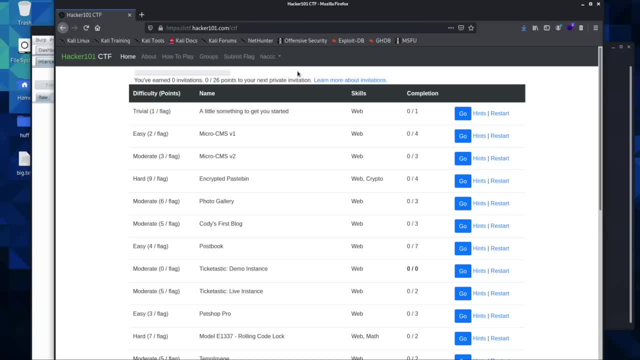 CTF, And then it will bring you back to login. you'll click the blue button and then you will log in and it will bring you to this page. And if it doesn't bring you to this page page, you have a navigation bar very similar to this one. 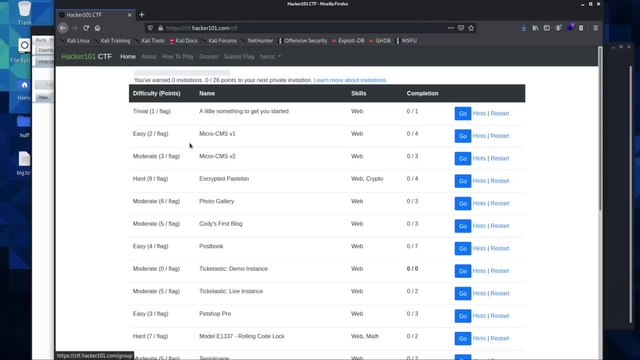 And you will just click on CTF And then you will be at this page. but you're going to have to register in order to reach this page, And then what I want you to do, as we begin working with actual vulnerable websites, is go ahead and click go. this is the going to be the very first. 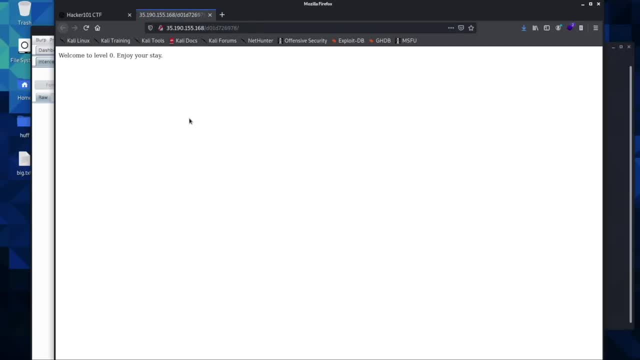 challenge I have for you. Once it loads, you're going to be brought to this page, And the way HackerOne is going to work is you're going to have to go to this page and you're going to have to go to this page. and you're going to have to go to this page And the way HackerOne has set up their 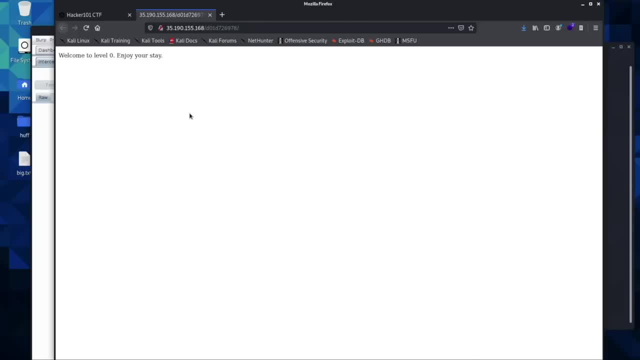 training program is that you will have flags and then it'll have a bunch of random numbers, And once you reach that flag, you will know you have found the area of the website that you were not supposed to find or is supposed to be vulnerable, And so with that, I want to have you pause this. 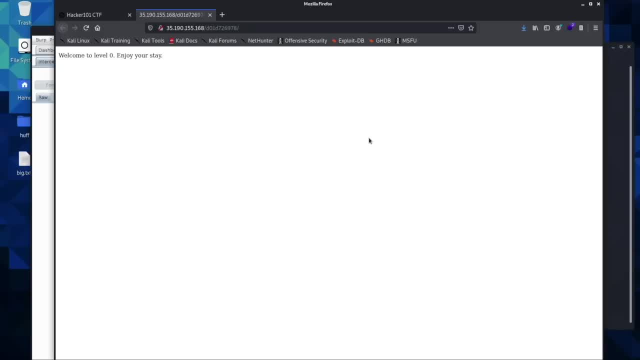 video and see if- what you've learned in the last lesson- you can figure out how to find the flag all on your own. So with that, pause the video And I'll see you in the next one video and give that challenge a go. Okay, if you got it, that is great. If not, I'm going to go ahead. 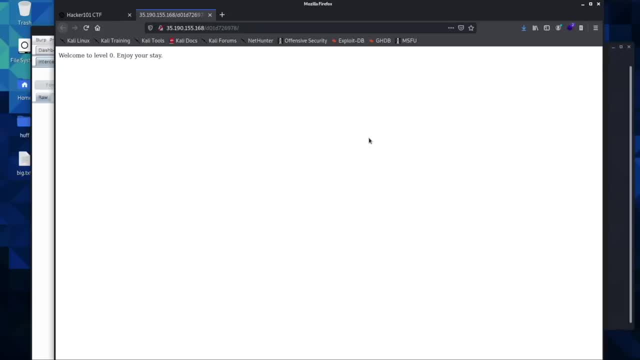 and reveal to you how to find this specific flag. Before you do, I would challenge you to go back and watch the previous video And just see the steps that I walked through, And then go ahead and come back here and give it a try, Because I am certain with what we have covered, you can find. 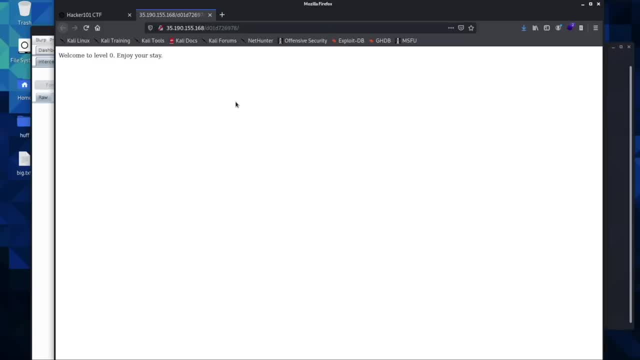 this flag on your own. So if you want to find the flag, go ahead and do that And I'll see you in the next one. So the way we find this very first flag is by coming in here and just right clicking And then going to. 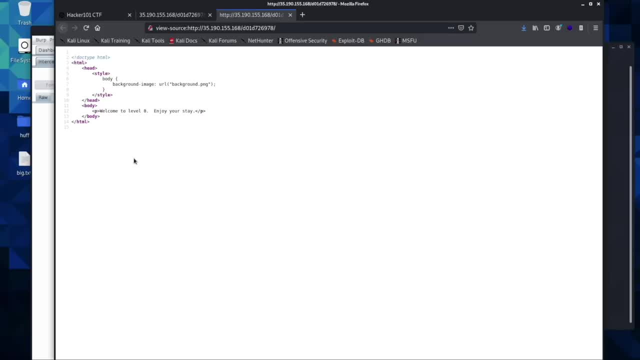 view page source. And then we can look at the page source And we can see what is in here And it has a background image And then here it is Backgroundpng. Just a little bit ago I actually came in here to 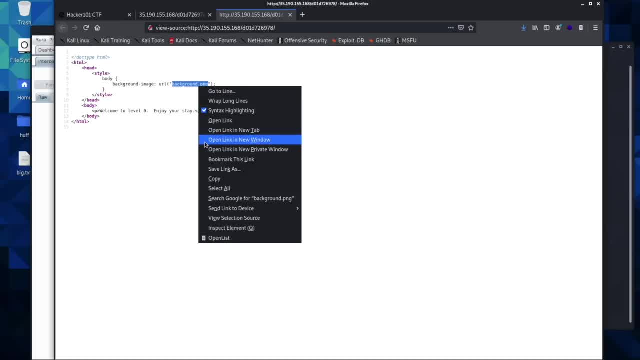 try this, And my guess was this is going to be the background image, So I'm going to go ahead and look at the page source, And then I'm going to go ahead and copy this, And then I'm going to go ahead and. 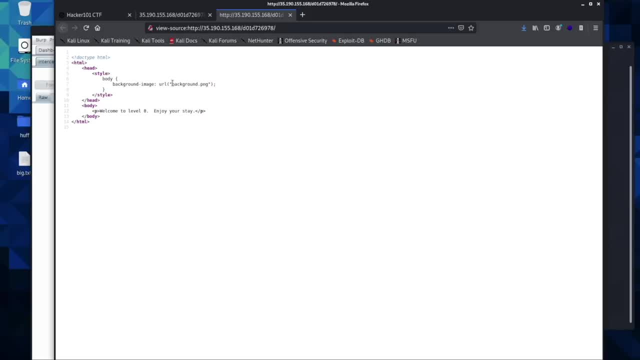 paste it at the end of our URL. I'm going to paste it And then hit enter, And then here is our flag. We're going to move on into the next video And I'm going to help you get set up on what you're looking. 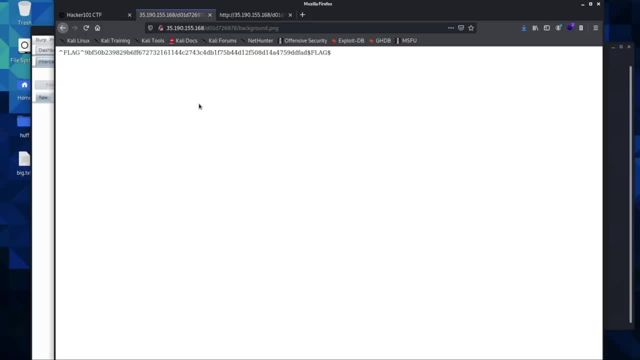 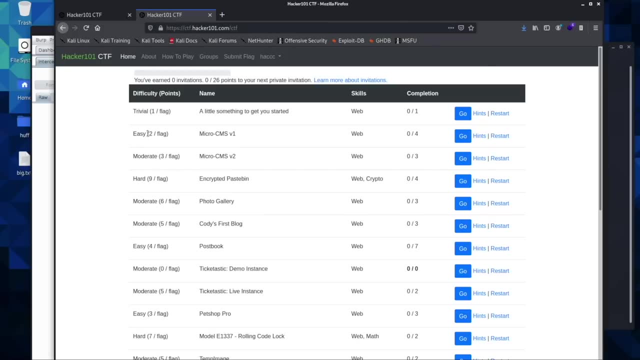 for, And then I'm going to turn you loose and see if you can find the next flag on your own. Okay, we are ready for challenge number two. We are going to come into the first easy program we can enter. We are going to only find one of these four flags. We'll actually come back later. We're going to go ahead and 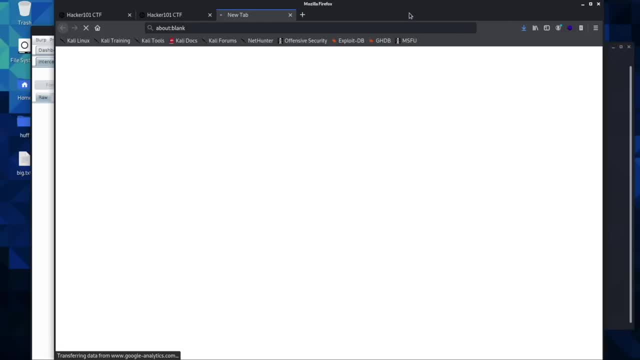 click, go And pull open this vulnerable website, And I'm going to turn you loose once this loads, Because everything that we have done so far, that we have covered, should give you everything you need to know to find the flag that we're looking for in this specific capture the flag, And so with that, I want you to go. 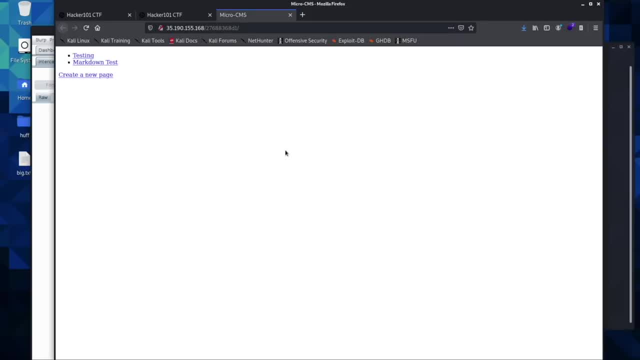 ahead and click around in the website and see if you can find the flag, And so we can go ahead and pause the video now and see if you can solve the first challenge. I believe we've covered most everything you need to know to find this flag, And so the first thing that we would do is just go ahead and click on the flag, And then we're going to 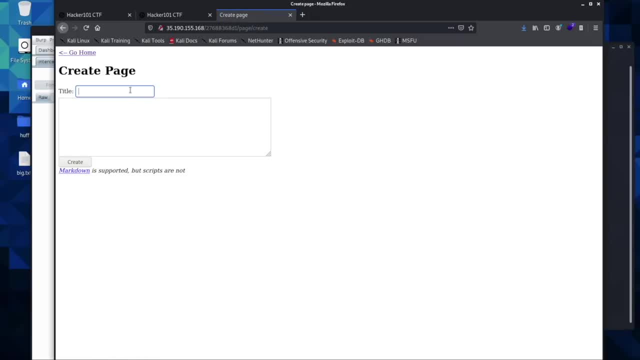 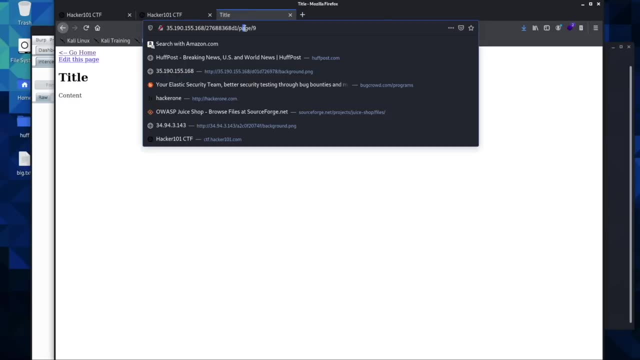 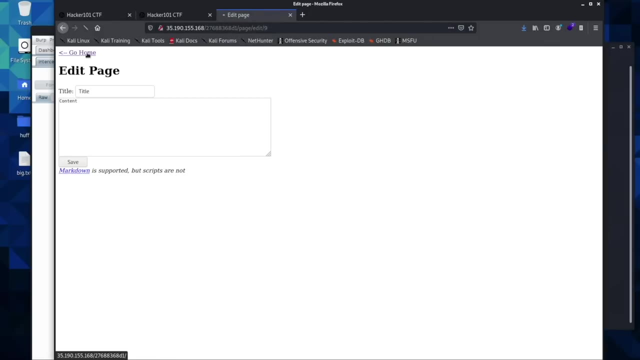 just start clicking around And you can maybe make a page and see what happens. We've got a page here, We're on page nine And so we can go back. We can edit this page And we can see. we can edit our page nine. We can go back. 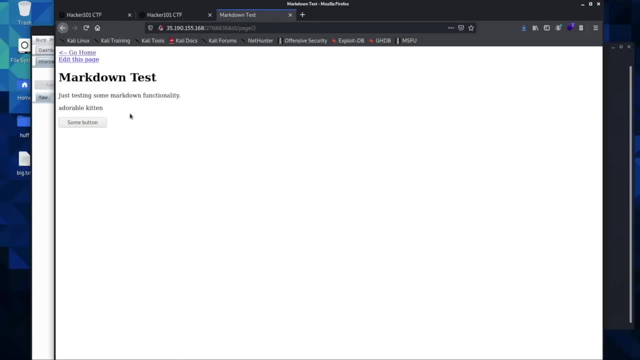 We can click on the markdown test and click the button. that doesn't really do anything. We can come in and view the page source And we can look around. There's not really a whole lot here for us, And so we can go back And we can go to home. We can go to. 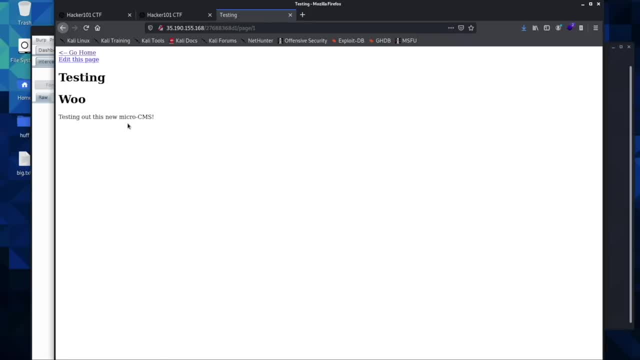 testing And just as we continue to click around. a couple of things that stand out to me in our URL is that we have this page So we can come into. let's just go into the page that we created. We can come in here and just go page one. 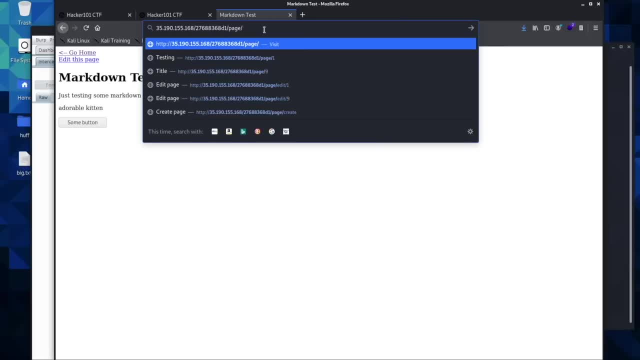 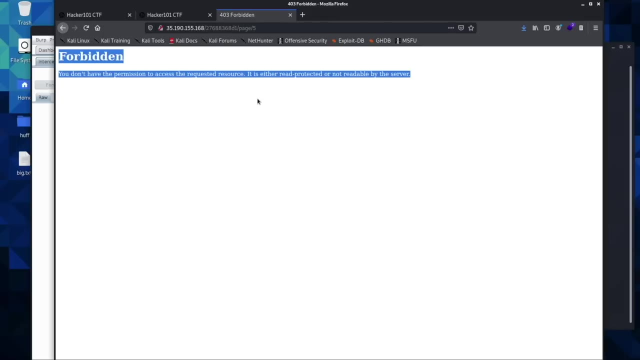 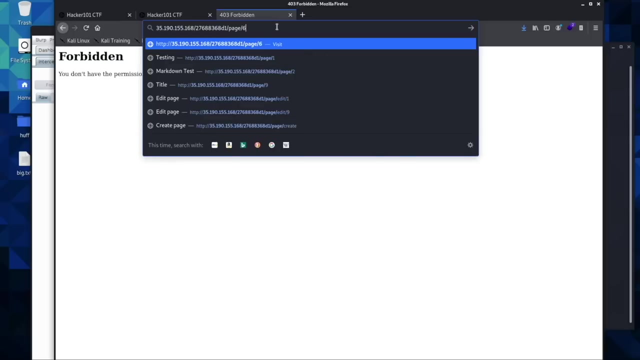 Page two, page three: not found. Well, we know there has to be at least nine, because we have created page nine. So go to four, five And then we hit the forbidden page. If you remember, in the example that I showed earlier we have seen a forbidden page before, And then we'll keep going. We'll go all the way up to page nine and look at every single one. 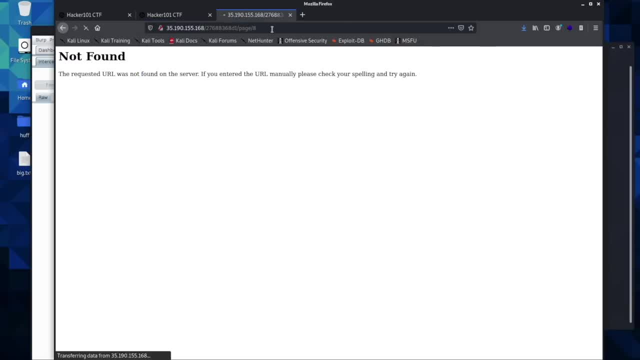 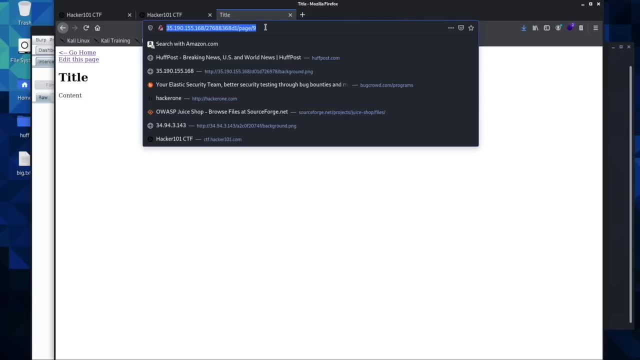 Every single option we have, because we know that's how far we are, as we've created. So we have all these, And then page nine should be the one we created. So what page was that? That was forbidden. It was page five. So how do we? 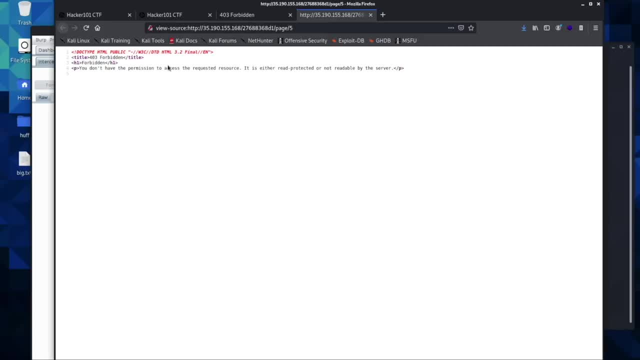 access this. We can go view page. source says we don't have permission and it is forbidden. Well, there is another way to view this page And if you remember from the example website that you created, if you had done this yourself, it would fit if you didn't have permission to see the page. So that doesn't have that permission. 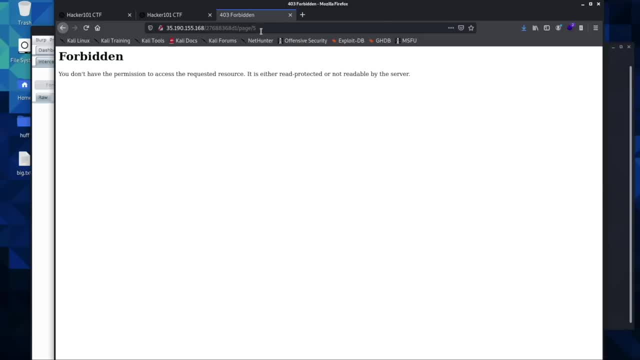 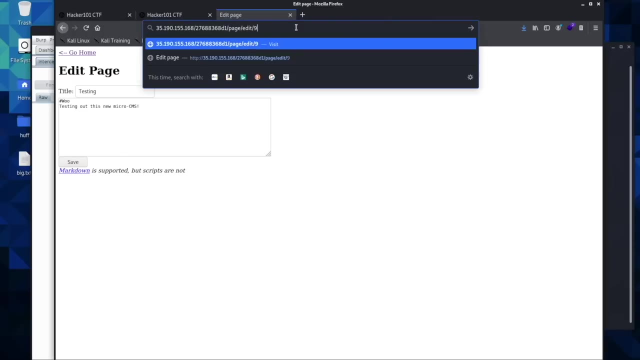 If you have not recognizing what you're saying, then that's not house I made and showed earlier. you would know that we can try and get around this because we have the option to edit this page and so if we edit this page and we know we can edit the page that we made, maybe we can edit the page that was. 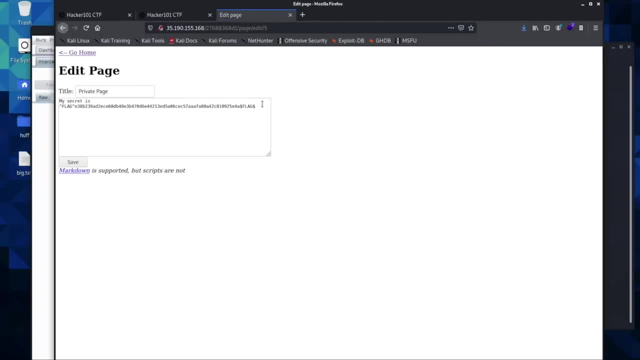 forbidden, so we can come in here and put in five and there it is- there's the flag. so I hope you found this. I think by now we've covered everything needed to find a flag like this in the URL. I have a few more challenges for us to go ahead and. 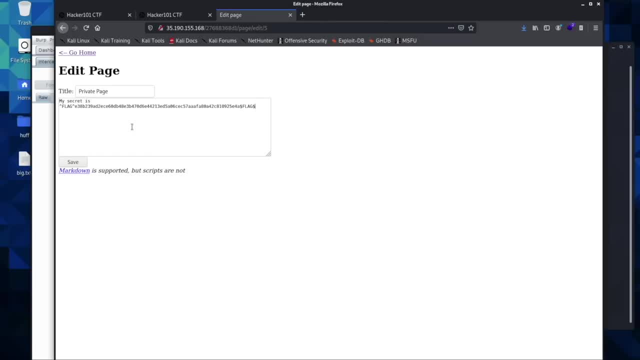 try. they're going to be on a website called over the wire and I will actually help you navigate to that page and get logged in. we don't actually have to make a user or create a user, which is very nice and so it's very easy to access and 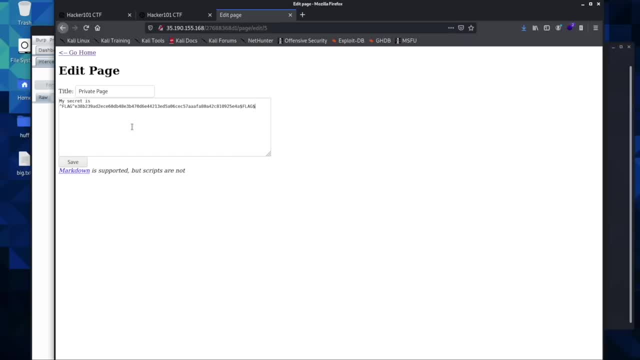 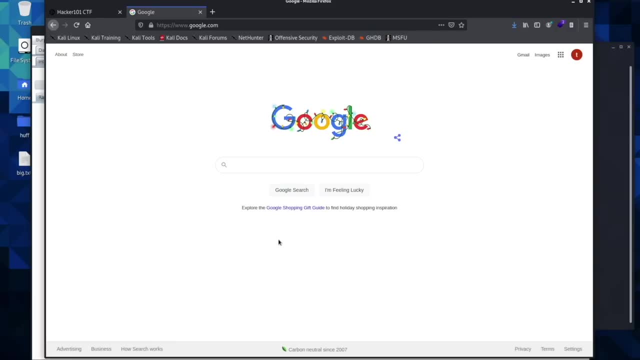 you can do that by clicking on the link in the description below, and then you can access it and to practice on, and so, with that, I'll see you in the next video and we'll get that all set up. okay, we are ready for a few more challenges, and 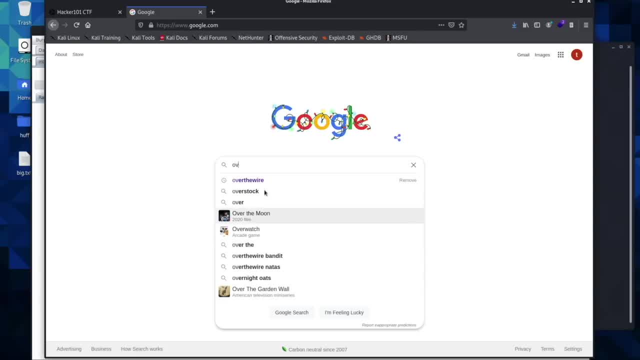 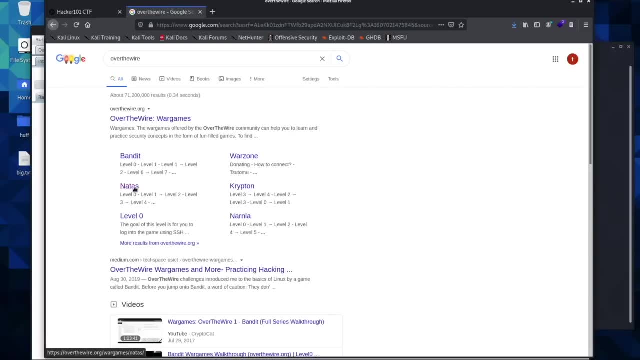 so we're going to go ahead and head over to a website called over the wire and you can click on it or type it in, and we're going to go ahead and click on notice this is where we're going to be working out of. we can click on that and 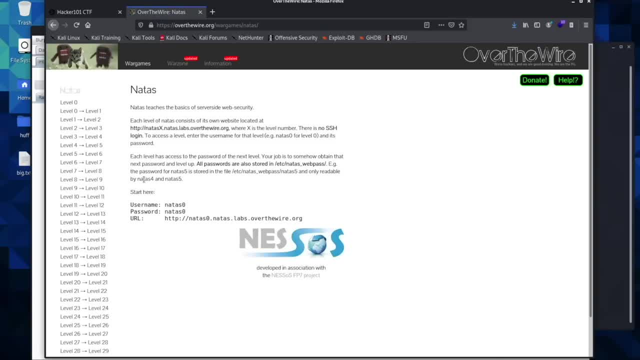 it will pull it open, and this is where we're going to get started. I'm going to to go ahead and open a new tab to keep this one open. so we're going to start on level zero. password is going to be level zero, and so all we have to do is copy this url and paste it in and then hit. 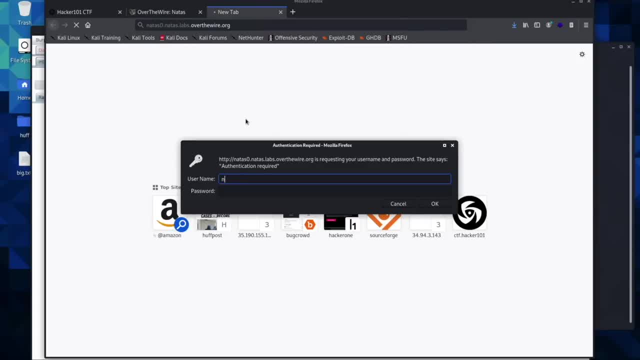 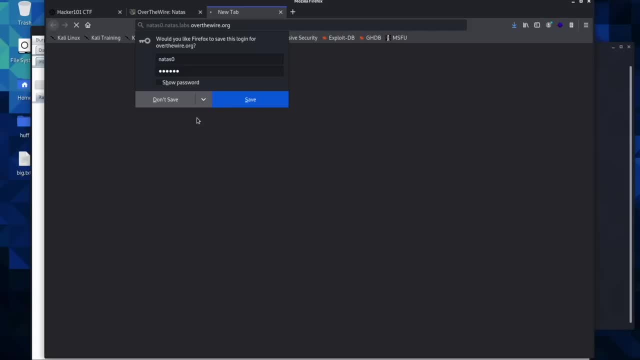 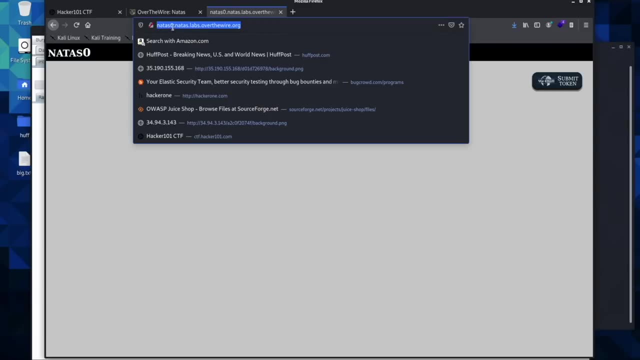 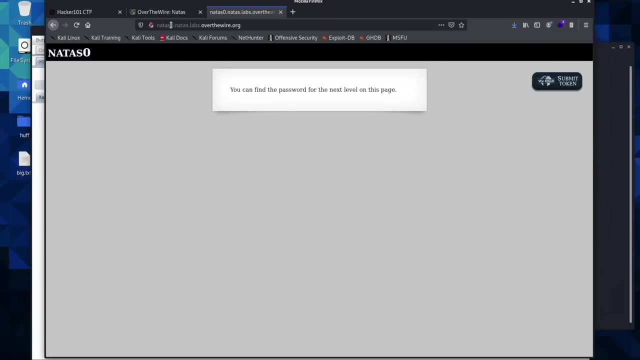 enter and our password is going to be notice zero and notice zero, and then we'll hit enter and every time you find a new flag you will come up here and you will change the zero to a one, the one to a two, the two to a three, and it will prompt you and say username. and so we have not a zero. 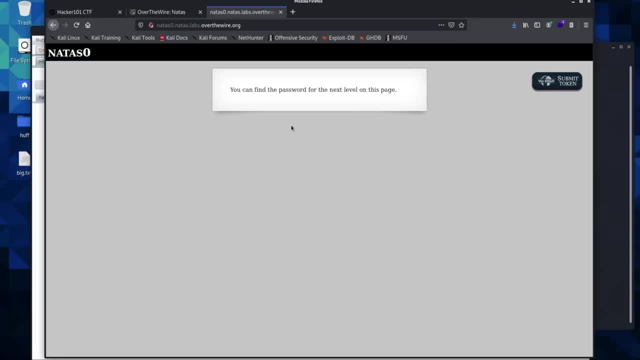 right now. the next username will be notice one, and then the flag that you find will actually be your password for the next level. we have gone over everything needed to find this first flag, and i want you to you go ahead and try and do that now. okay, hopefully that went well for you and you were able to. 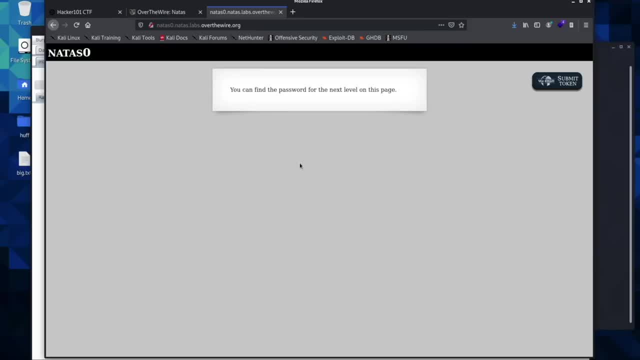 find the first flag. but before we get into that and get going too far, there's one thing i forgot to mention in the recon portion of the course, something that we will use in notice and you will use later on in your bug: bounty hunting: career is the robotst. 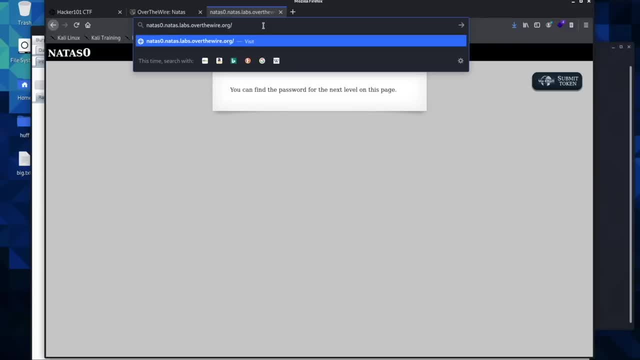 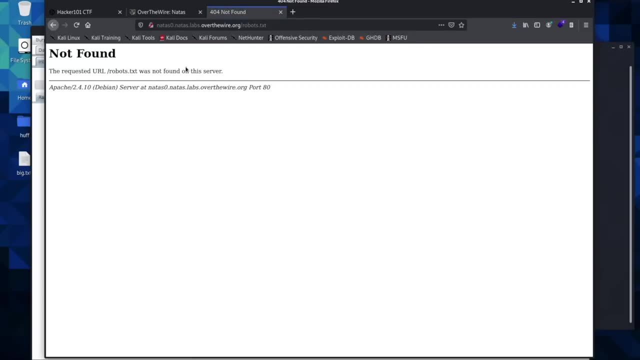 xt file so you can have the way we get to that is, you just hit a forward slash and then you hit robot dot txt, and then you hit enter and it will take you to a page. this one doesn't have one set up, but it'll take you to a page that doesn't allow search engines to find it. so sometimes 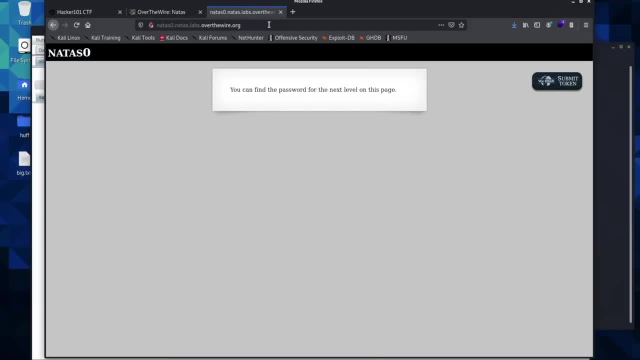 websites will have files that they are hosting online that they don't want google displaying, and so they'll have a disallow or allow for google and bing and yum器, and you will find that sort of foreigner's asterisk in search engines. but i don't think this is enough already for me, so we're going. 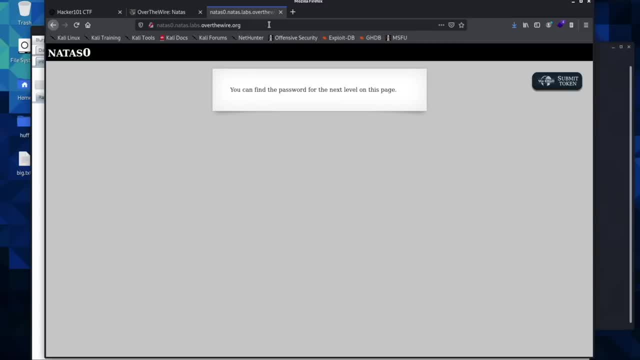 to try and make it extremely simple and we'll just hold the interrogation button and we'll follow where we meet and we'll craft this one and close ouriz, Sami, or do that to be it, and have to have a proper gaat to include it- yahoo and other search engines to go through and crawl their website and it will go through. 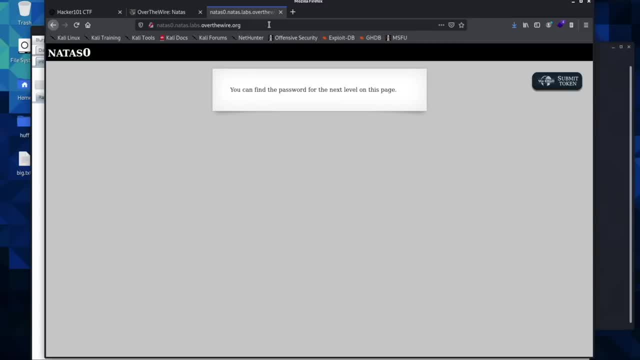 that robotstxt file and will say: do not allow google or bing or yahoo to crawl through these files, and so it's always a good thing to check the robotstxt and roll through and see what's allowed and what's disallowed, and then visit those disallowed files and see what's in there. 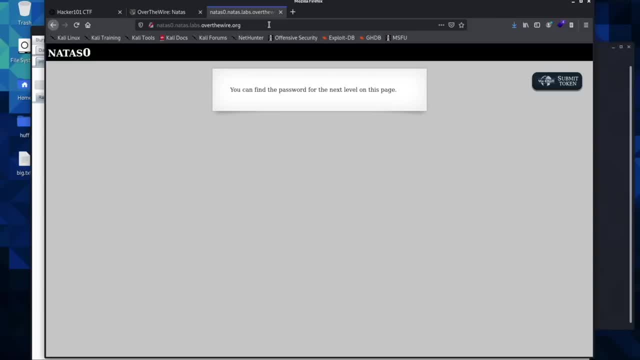 or those domains or directories that we find, and so with that we'll go ahead and solve this challenge, and so i hope by now you know one of the first things we do is to go ahead and view the page source or, you can expect, inspect the element. either one works. i like to view the page. 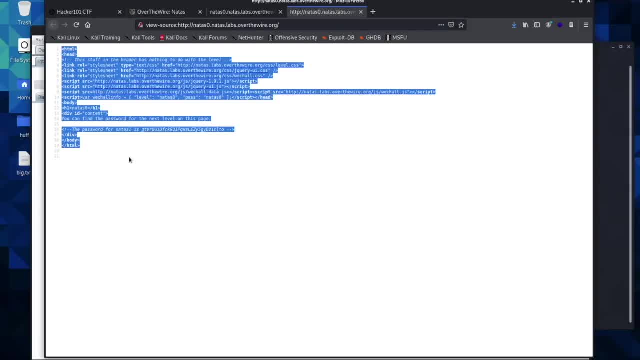 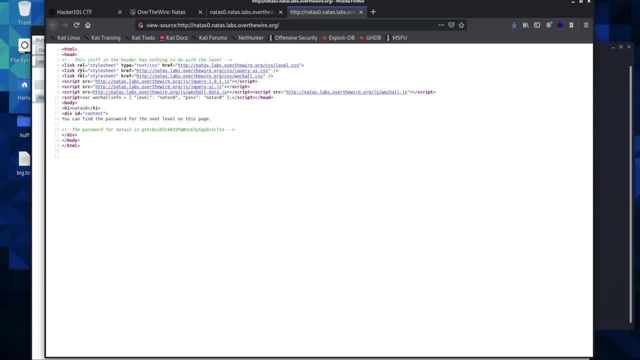 source, because it gives us a more complete view, and so one thing i want to mention about the notice levels is everything inside this head tag, which will be from here to here, doesn't have anything to do with the page source, so we're going to go ahead and do that, and then we're going to 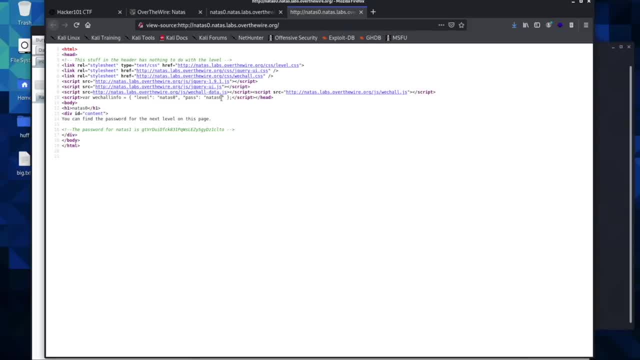 do with the level, and so sometimes you'll see the password for the previous level up here, which the next one would be right here. this is our password for this challenge, and so i hope you found this, and next time, if you view the page source, this password will be right here and 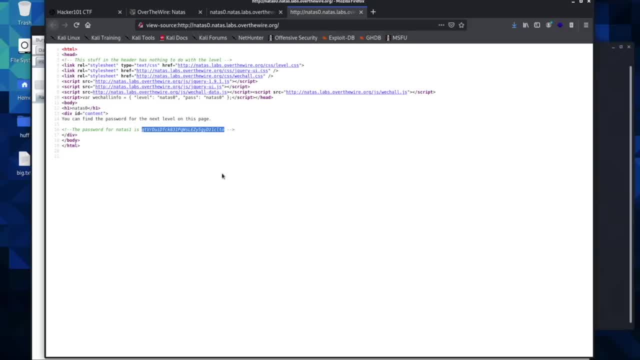 just so you know, it's inside the head tag and so it's not actually anything that's going to be relevant to us, and so here's the password for the next level, so you can go ahead and copy this, and the way we get to the next level, if you remember, is come up here: 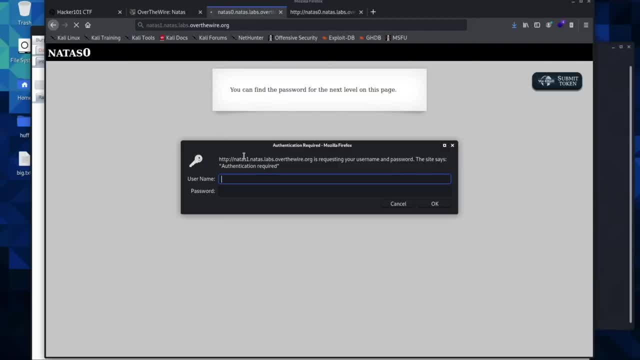 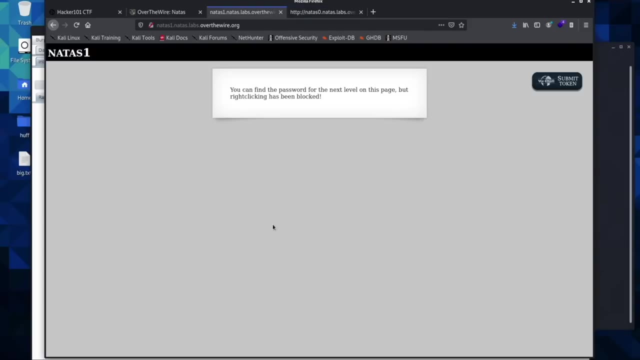 go to notice, it changes to one, it will prompt us for the username which is going to be notice one, and then our password, which we just found in that flag, and we hit enter and that takes us to the next level and if you want to go ahead and try and solve this challenge, you can do that now. 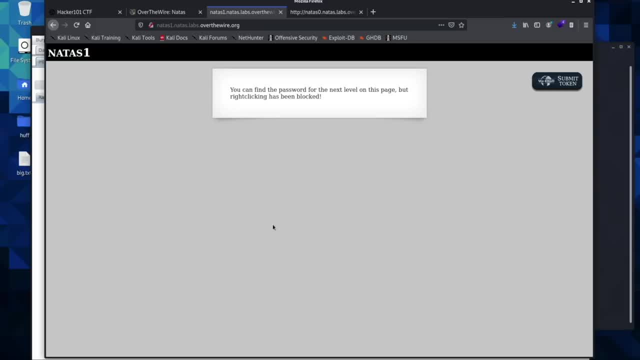 i'm going to stop this video and we will solve this challenge in the next lesson. and so this one says that we are not allowed to right click. it's been blocked. however, for me, if i go ahead and i use my keyboard to right click, if i hold down control and hit the right click or click. 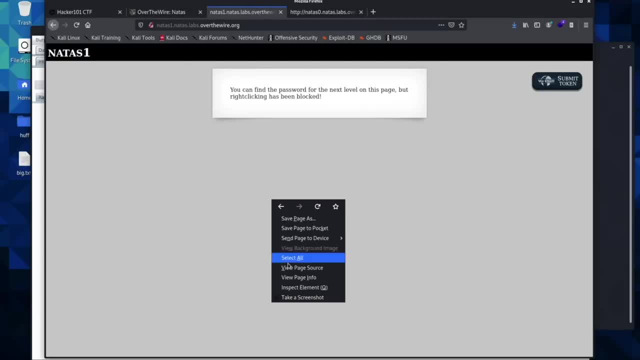 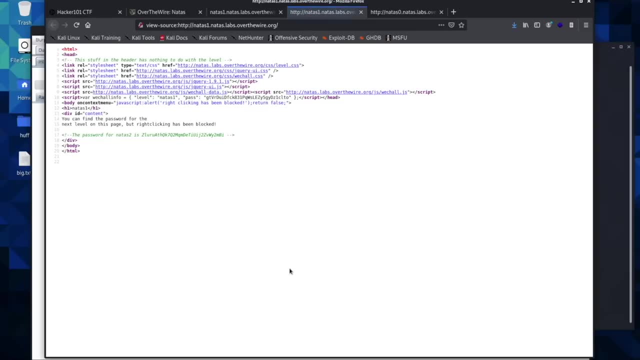 then it works for me, and so my right click is available through using control. and then i do the exact same thing. i go to view page source and then, once in here, you can look through our code, and then they've got it commented out. the password for notice 2 is: and then here's our. 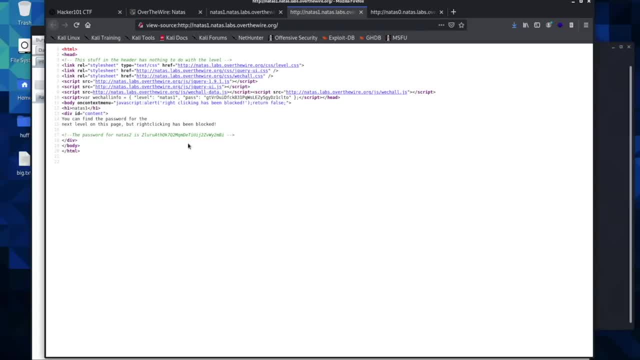 password. now, this may seem really easy, but you will actually find people who have put in these comments, in the code of a username or a password or an api key and has they just have forgotten to delete it, so they'll put them in here while they're developing the site or while they're. 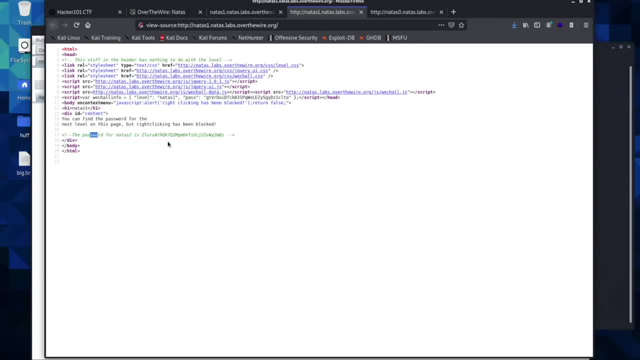 writing their code and they need to remember their username, their password or their username and password, and they need to remember their username and password, other sensitive information and you will actually come across it just being hard coded right onto the site, and so that's why we check the code and sometimes you will find, like a you will really 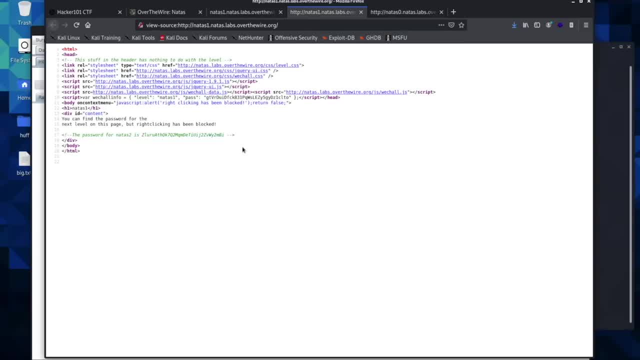 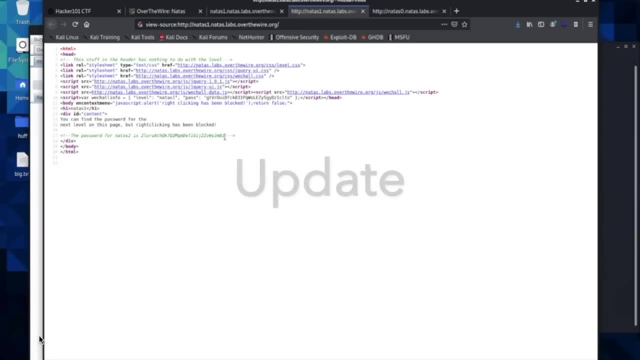 find something just like this: a username and a password. these seem very easy, but they're also very practical and they're something you will come across pretty regularly. all right, this is an update, since i originally made this video and was saying that developers will come across these passwords. i was working on the back end of a web app and i accidentally 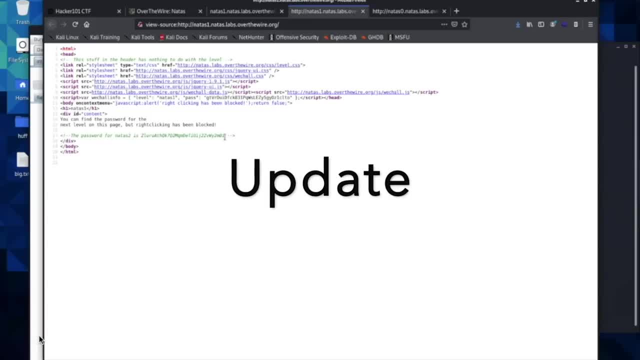 pushed my database username and password to the public github page. so when i say this happens, i mean it. i have done it. i'm sure almost every single developer at some point has pushed something sensitive to github and it is something to watch out for. so there is my update, and so i 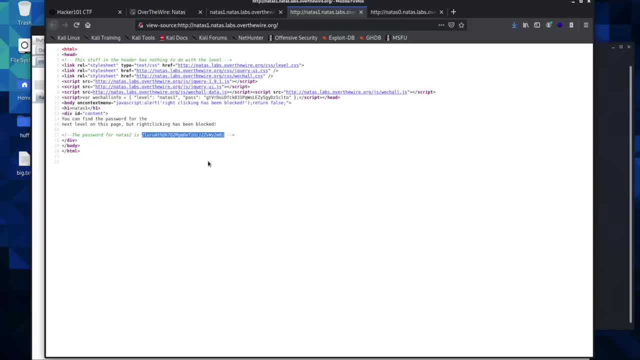 want to. i guess i shouldn't say pretty regularly. you will come across them. most people will come across them. most people will have already reported these. this is why it's important to be one of the first ones on a site to pick a specific target and make sure you keep up to up to date. 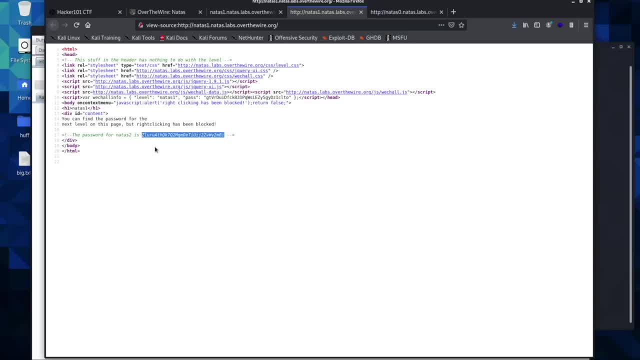 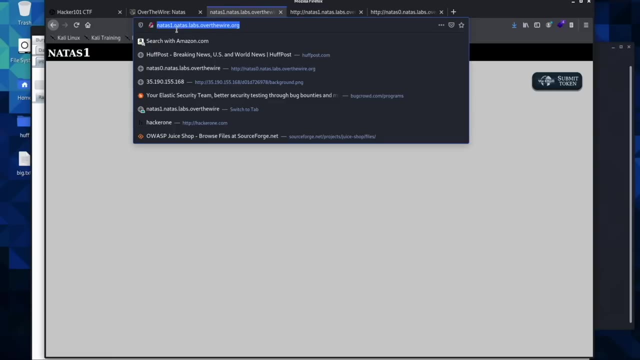 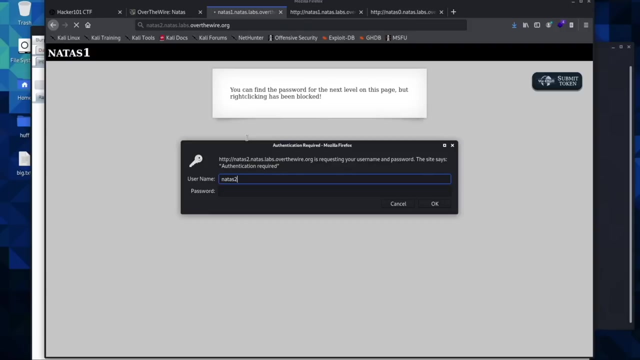 what's coming out new on different domains and different subdomains as you continue to work through different programs and your bug bounty hunting. so we'll go ahead and copy this password, we'll come back to our main site, we'll type in notice2 and we will type in notice2 and paste our password. i'm going to not save this. and then here we are. 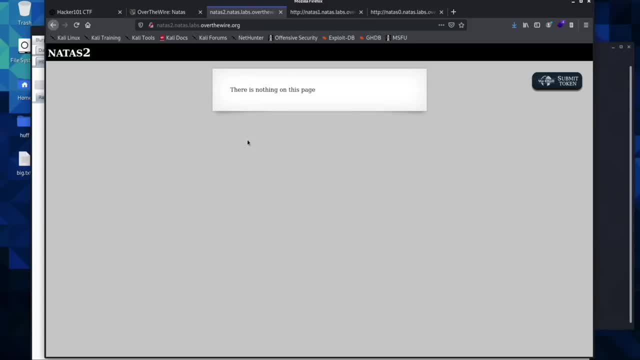 again, it says there's nothing on this page that should give us a clue. everything we need to know to solve this challenge we have already covered previously. i think there's a little more to it that will cause us to need our critical thinking skills, but we have covered everything needed to. 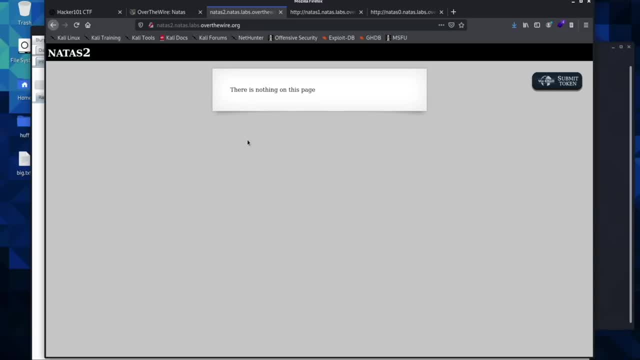 solve this challenge, and so i'm going to go ahead and give this a go and we'll go over the solution. okay, how did that go? hopefully you were able to solve this challenge. i'm actually going to show us a couple different ways that we could solve this challenge, just so that we have a 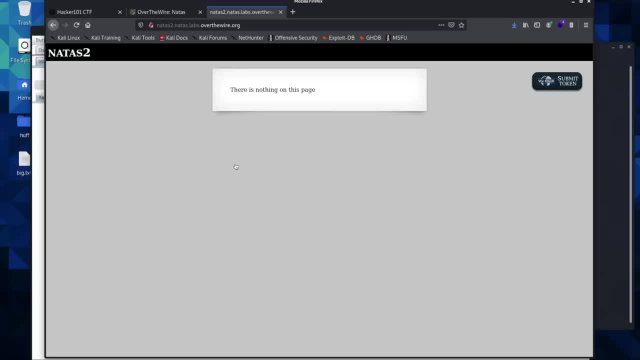 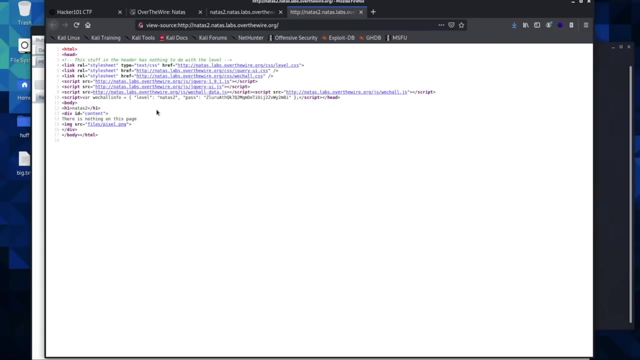 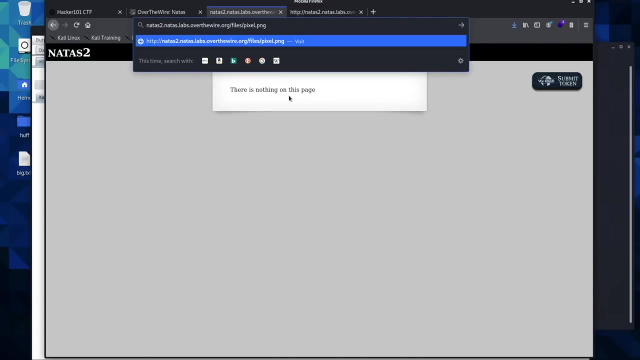 more rounded understanding of how the url works and how different files and different directories are included into domains. and so with that, i thank you for watching this video and i hope you enjoyed it and i'll see you in the next video. bye, and so as we paste this, we can go ahead and hit enter and see where it takes us and when. i first 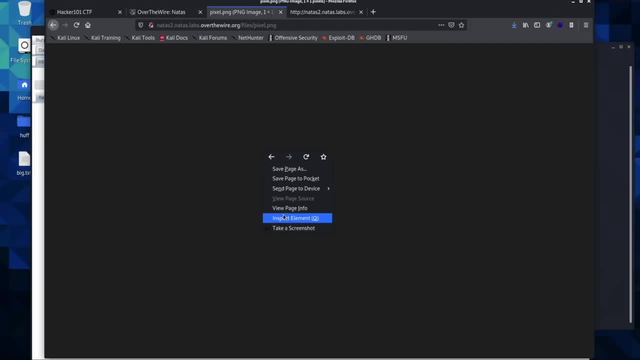 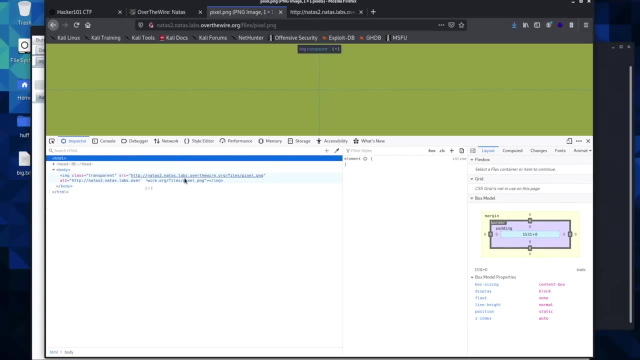 solved this. i went and i checked to see if i could inspect the element, to see if there was anything else on this page other than this picture, or maybe there was something inside of it that would help us. and when i was looking here at the url, i noticed that this is a file or an image. 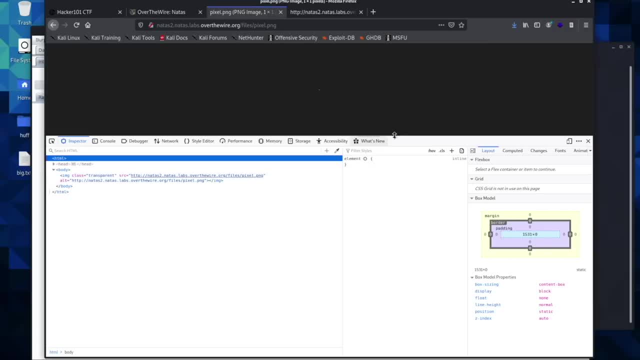 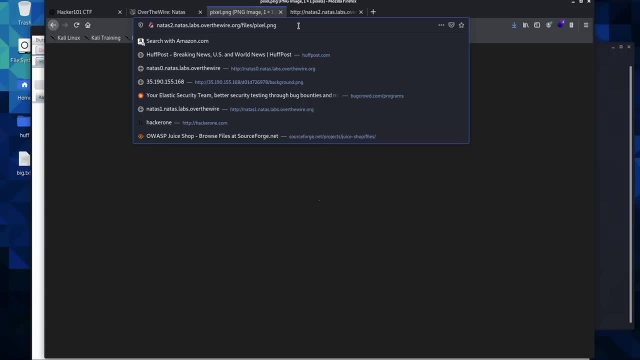 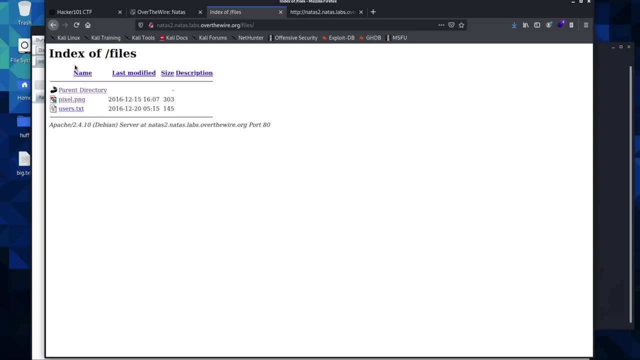 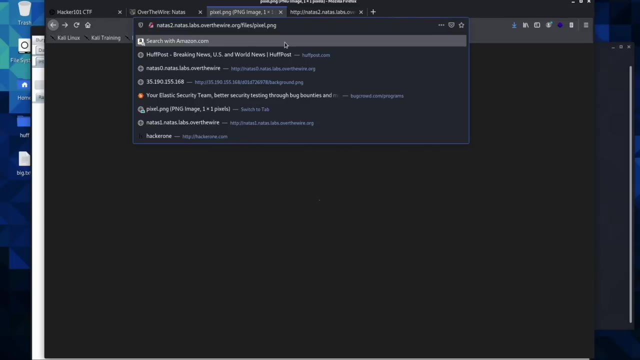 and it's inside of a directory called files. now, if you remember, we can actually go back directories and you can actually just delete the pixelpng and it will take you to the previous directory and here it is, or we can go back and just another way to see this is you can do just like like we learned in our home folder or in our kali linux. 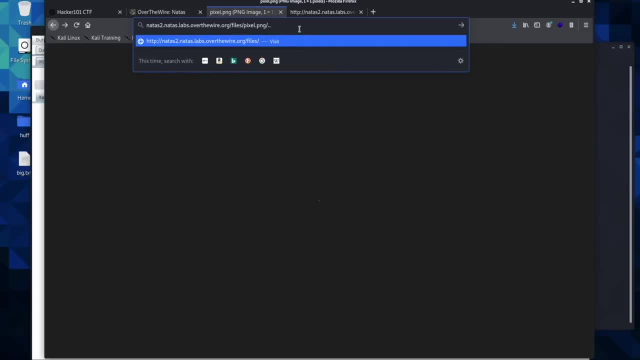 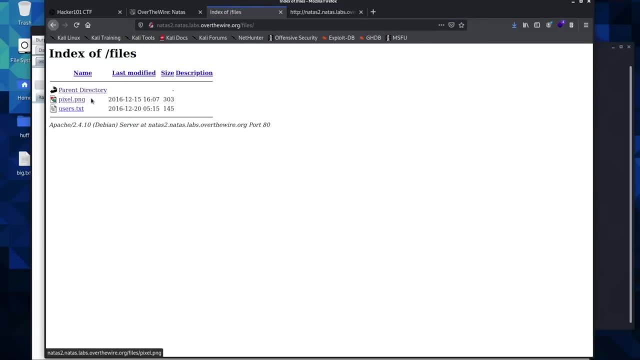 terminal you can put, have your slash and you can go dot, dot, slash and you can hit enter and that will take us back to our directory and we can go back to our directory and we can go back to our one file or one directory. and so we've already viewed the pixel and now we've been in the parent. 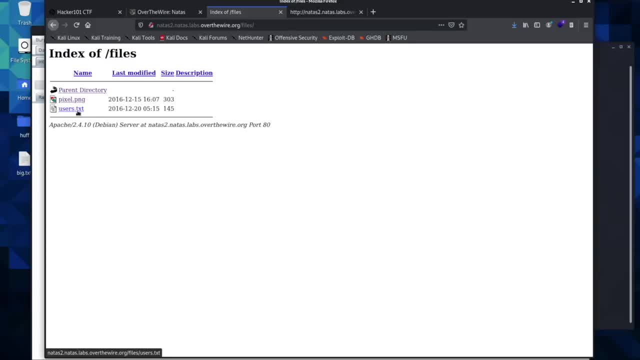 directory, but now we can see this users dot txt, and so we can click this and it'll take us into a new file and here's usernames and passwords, and so you have alice, bob, charlie, and then here's notice three. so this would be our username, and here is our password. 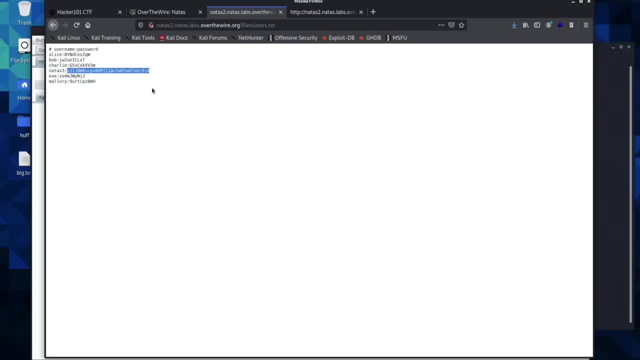 for the next challenge, and so we've seen all of this before. we have seen that we can find in our source code things that don't show up, or hidden files, or hidden images, and so we've seen this before. so i hope that you would have copied this and have pasted it. 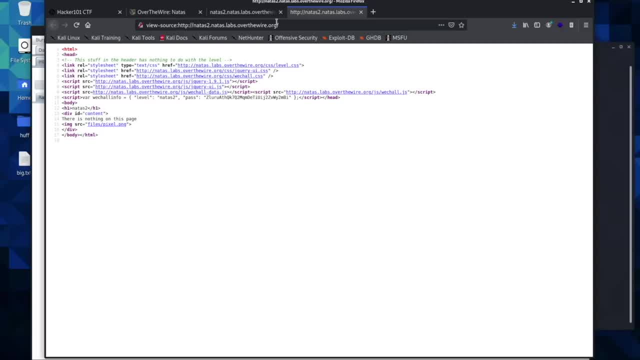 and we've also seen what's called the directory traversal- going back or deleting and moving into different files and different directories- and so i hope that you were able to solve this challenge, and so we'll go ahead and get set up for the next challenge: different ways to install. 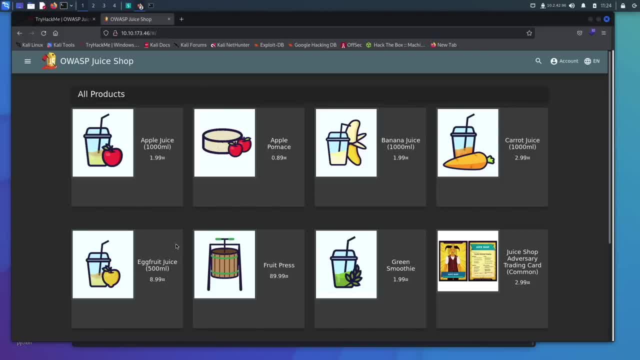 a wasp juice shop and you can watch the next five minutes of the video and see which one you think looks easier. i personally think the try hack me a wasp juice shop right here is the easiest way, but i'll show you how to download and install a wasp juice shop onto your local machine and you. can decide which way looks easier. if you want to go ahead and get set up for the next challenge, so we'll go ahead and get set up for the next challenge. so we'll go ahead and get set up for the next challenge. so we'll go ahead and get set up for the next challenge. 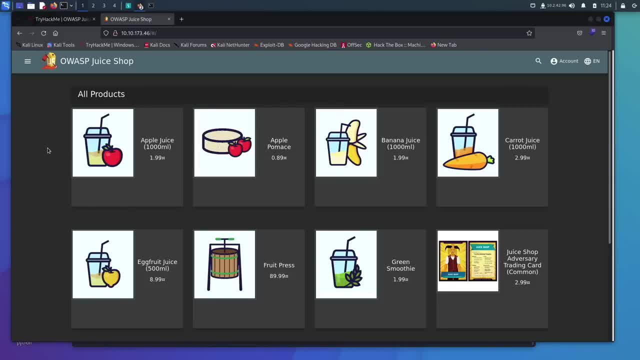 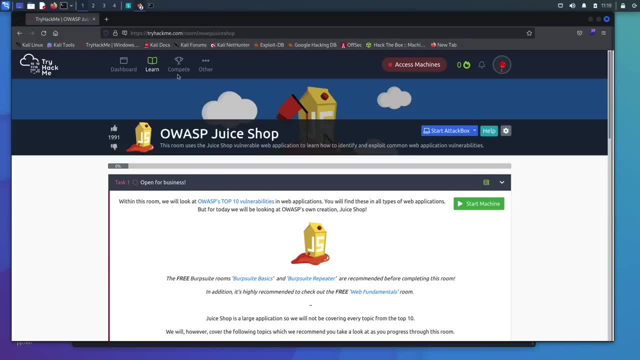 and you would like to run, so i'm going to show both of those to you now. since i originally have made these videos, a wasp juice shop has now been put on try hack me, and it's really simple to just go to try hack me, make an account with them and connect with. 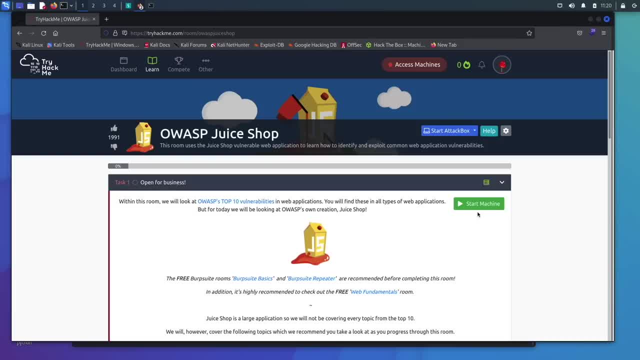 their servers and then open up a juice shop box. so you can either install it the way that i have already shown in the previous video, or you can come to try hack me. it is free to make an account and open up a wasp juice shop, and from there everything will be the same. 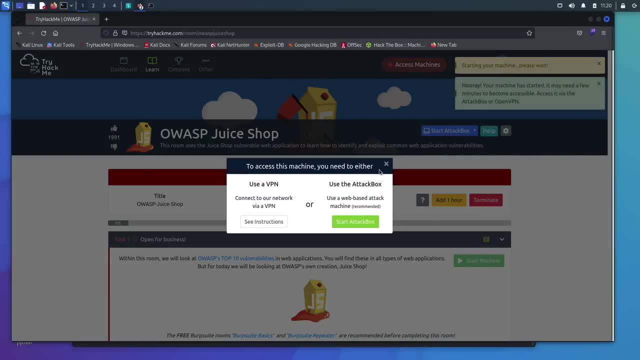 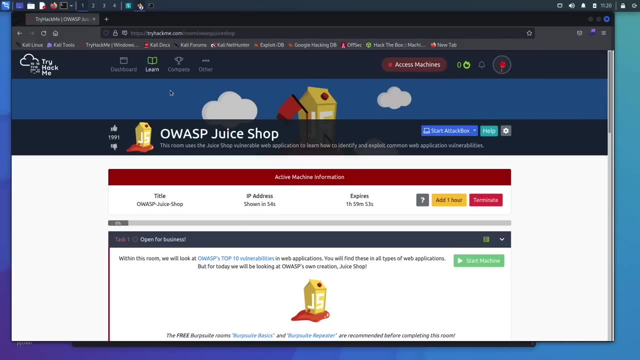 you will just click start machine and it will open up a machine like this and then, once this gives you an ip address, you can copy it to your clipboard and open up a new tab and paste in the ip address and it will open up juice shop for you. now i'll let this load and i'm going to cut this. 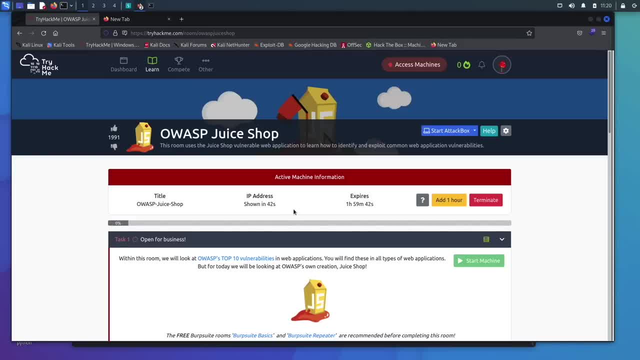 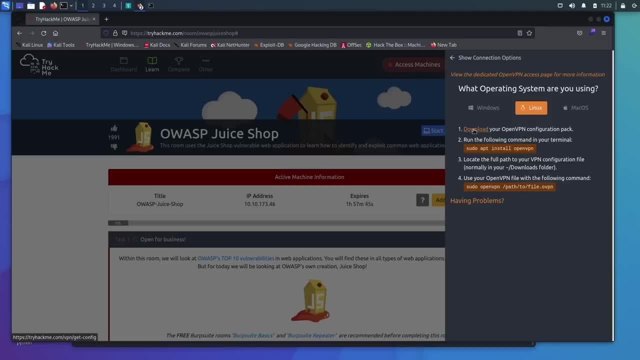 and then i'll show you how to open it up and everything will look just the same. the way you're going to do it is: you're going to connect to the box. it's come up to access machine. you're going to click open vpn download right here and it will download your vpn for you. you'll come over here. 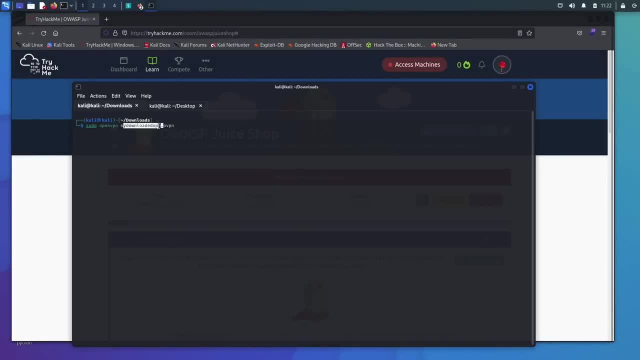 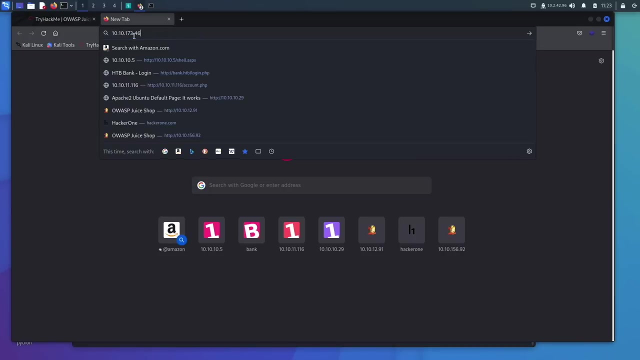 you will cd into your downloads and then you will type in sudo, openvpn, and then whatever your vpn download name is, and you'll hit enter, enter in your password and it will connect you. i'll go ahead and do this now. okay, i have connected to the vpn and now we can copy this and with our new tab, 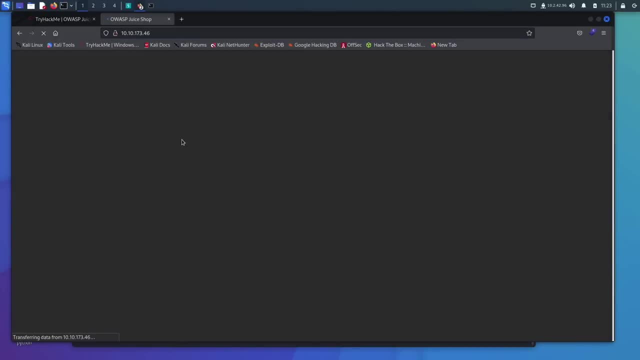 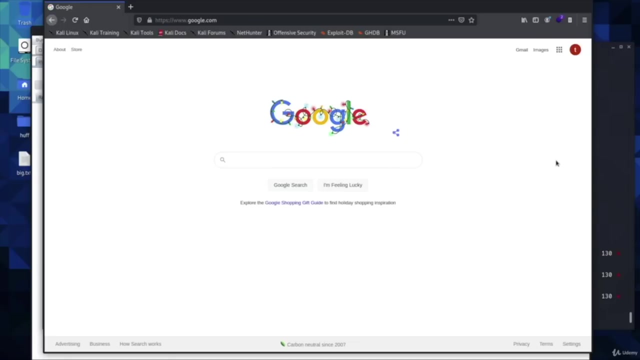 paste this in and we will be brought to the juice shop web app and we will accept the cookies, num, num, and then we are ready to start. so it's up to you which way you would like to install juice shop. okay, we are going to go ahead and install a vulnerable web app on our local machine. 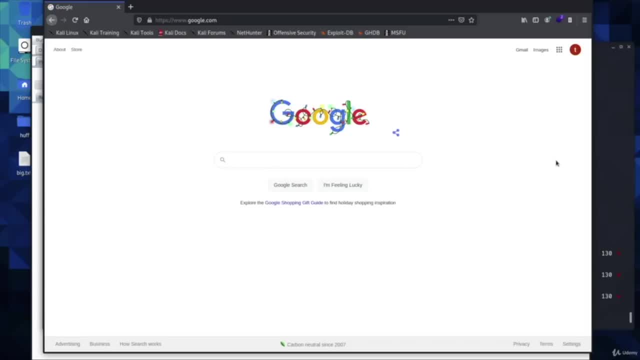 it's a great place to practice. it's put out by owas, which is going to be a great resource for you. rather than just seeing me show you how to do something or listen to me tell you about it, this is going to be a place that we actually go out and practice, and so we're going to download. 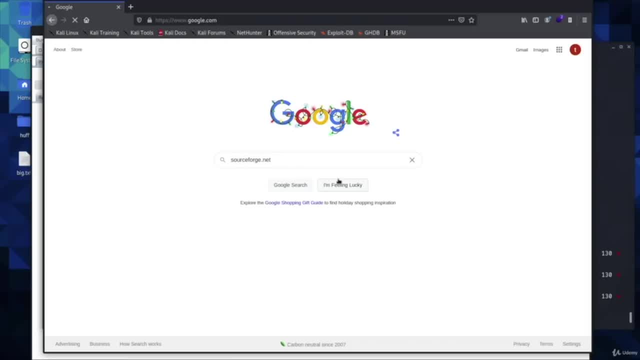 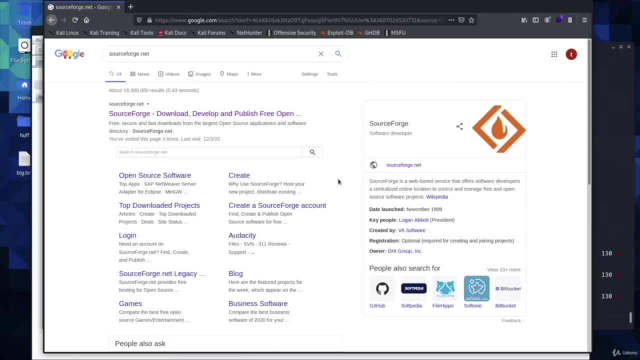 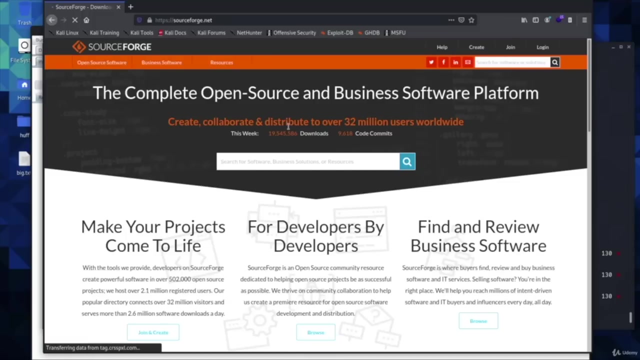 it by going to sourceforgenet and i'm going to have this linked for you in the resources and you can go ahead and click on that link and hopefully i can get it to a link directly to the download so you don't have to navigate through any of this, and this is actually my second time trying to. 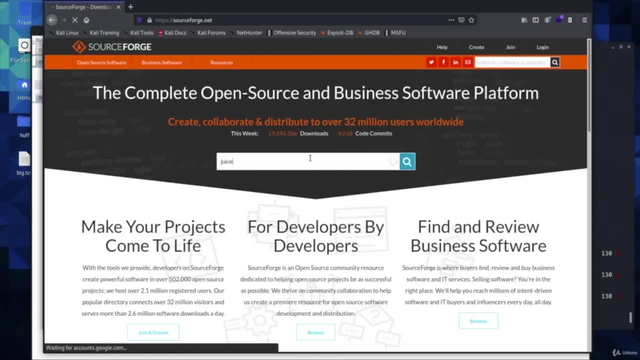 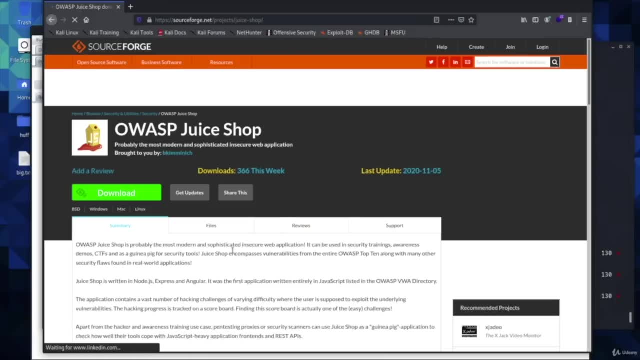 download it, because the first time i downloaded the wrong version and i don't want that to happen and so hopefully that link will work for you. but if not, you can follow along and i'll show you how to get to the proper download. so we type in juice and we click on juice shop. it was the second one. 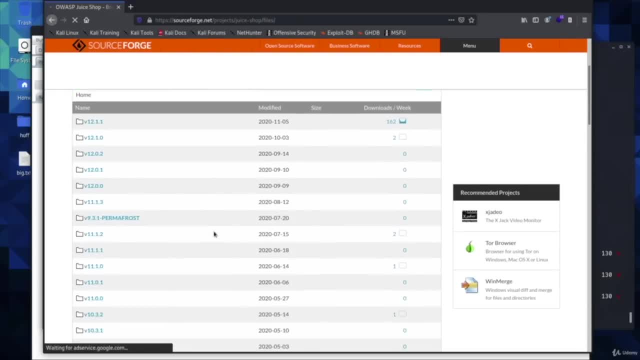 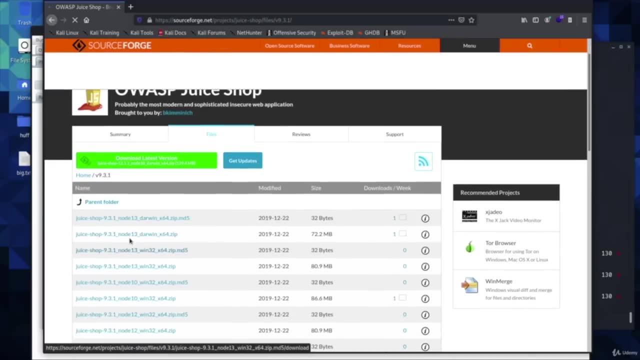 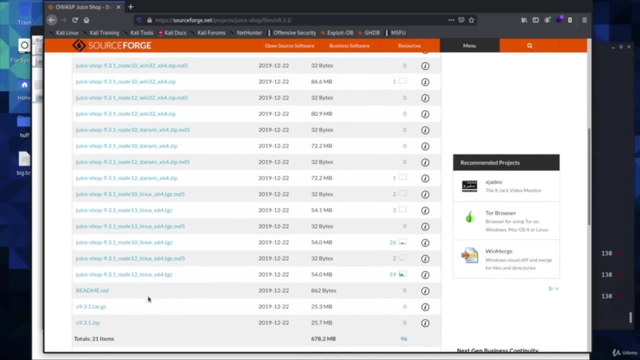 in the search engine. we'll go ahead and click files. we want 9.1.3, which is right here. we're going to be installing node 12, and so we need to make sure that we get node 12, and it's on linux, which is way down here at the bottom. this is where i 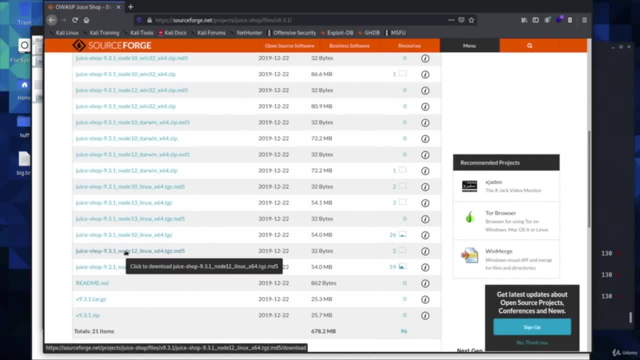 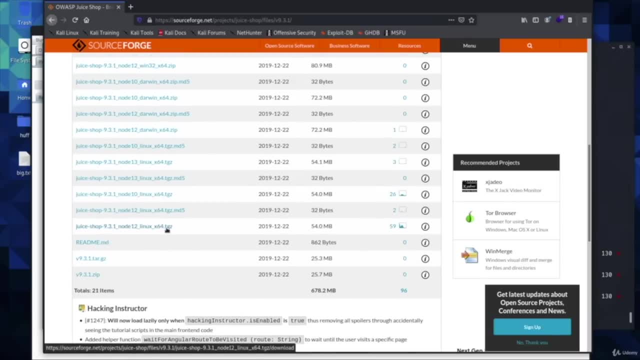 went wrong the last time. so we have juice shop, node 12 with linux. this isn't the right file. that's not the file we want. this one right here is one we want. we want the tgz, and so we'll go ahead and click that, and after you click this it might take a little bit for the download to. 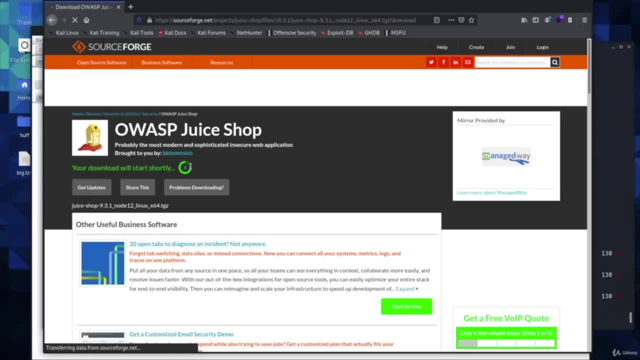 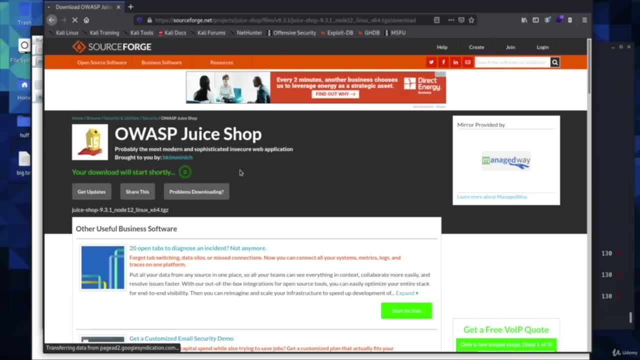 go ahead and take place, but you can go ahead and click it. your download will short, begin shortly and then, once it downloads, we'll go ahead and save it and it will automatically save to our downloads. and so i'm going to go ahead and pause the video and i'll resume it once the 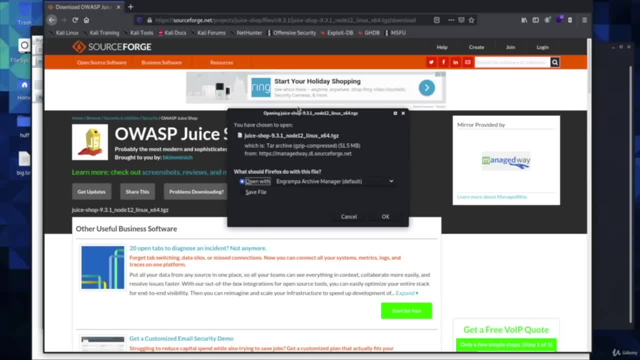 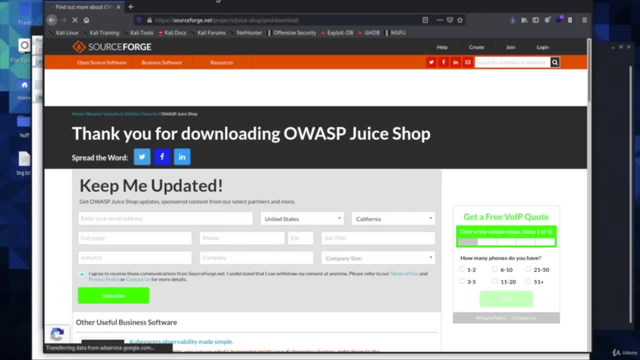 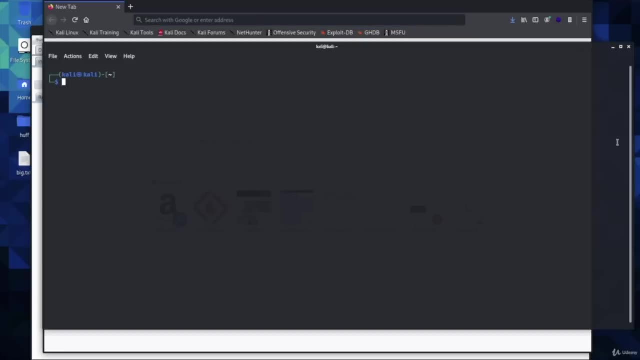 download has popped up. okay, there's our download. we're going to go ahead and click save file and this is going to save it to our downloads. we can go ahead and click: ok, i'm going to go ahead and close out of sourceforge because we no longer need that, and then we're going to navigate. 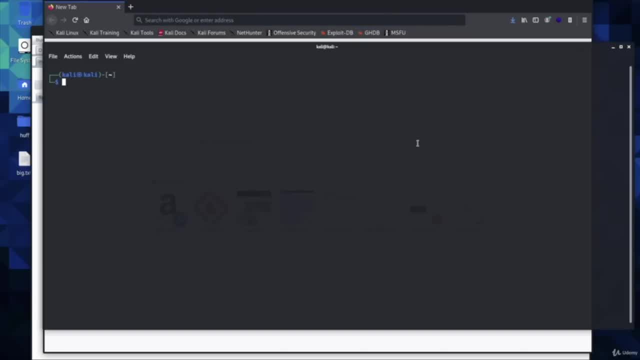 over to our terminal. i am in the home directory, so i'm going to go ahead and cd to our downloads. i will ls, and then here's the file we just downloaded. we need to unzip it, so we're going to go ahead and type in a tar and then we will go dash xvzf and then juice shop. 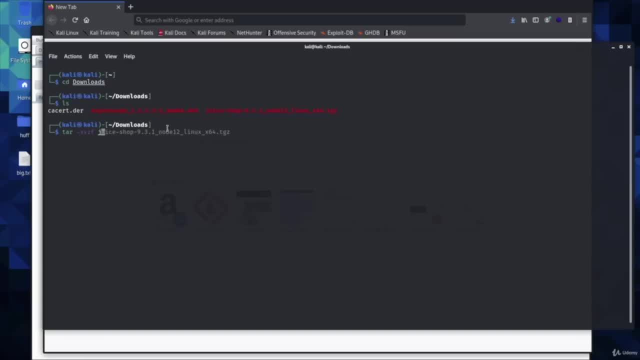 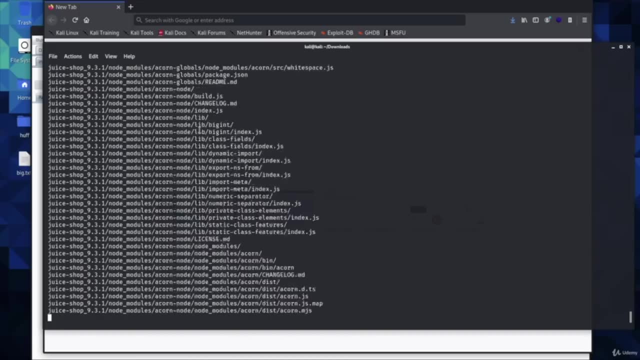 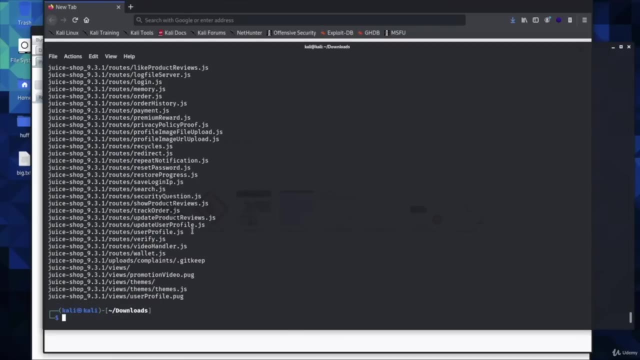 yours isn't going to pop up like mine is because i already typed this in once, and then i'll tab to autocomplete and this will go ahead and extract all of the content for us, and then, once this is finished, you will need to install nodejs and then npm, so we'll go ahead and type in sudo apt. 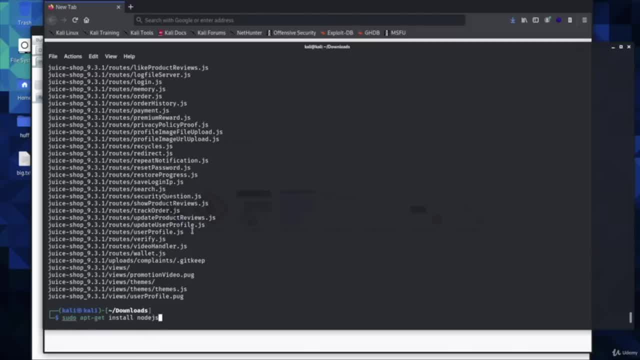 get install and first you'll go nodejs. i already installed it, so i'm not going to install it again, but you'd hit enter and it'll say: are you sure you want to? you will put in y and then you will hit enter and it will go ahead and finish the download for you. it might take up to a minute. 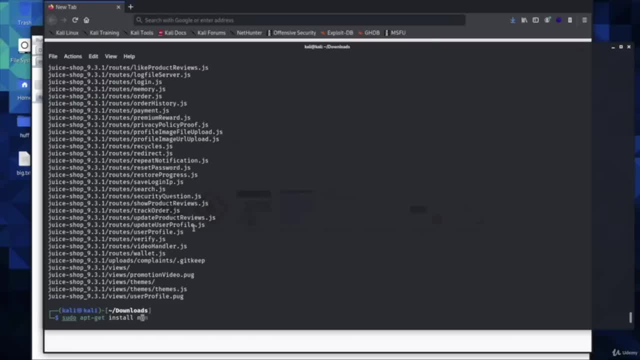 because there's a lot of files, especially in npm, and so we'll go ahead. and second, you'll do sudo apt, get install npm. you'll hit enter. you will enter your password for the first one. you won't have to enter it for the second one, and that will go ahead. and 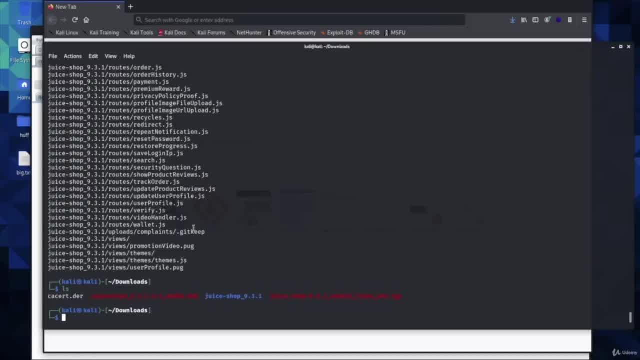 run and install npm and then we're going to ls in our downloads and we're going to change directories into juice shop and so we'll cd into our juice shop folder and every time you run owasp juice shop and you want to open it up and you want to practice in this 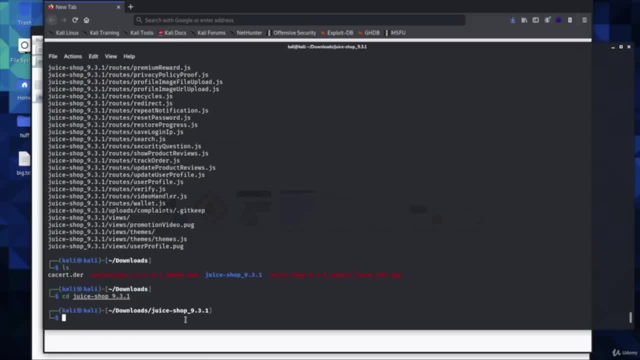 you want to open it up. and you want to open it up and you want to practice in this vulnerable web app. you will have to cd into your downloads and cd into juice shop, because when you spin up your server, it is going to spin up whatever content is inside the directory that. 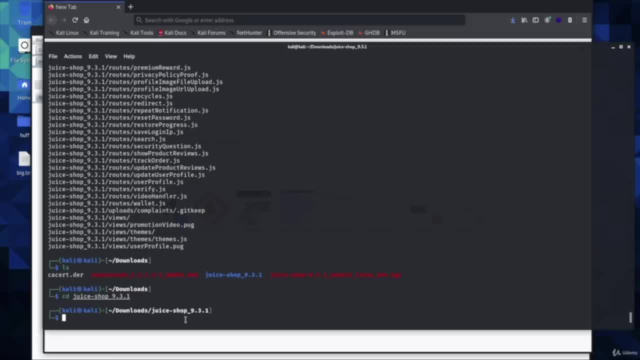 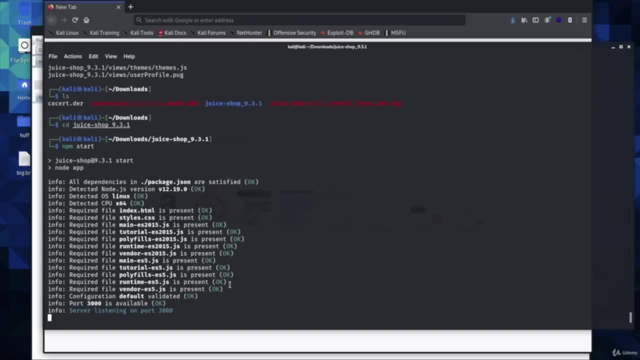 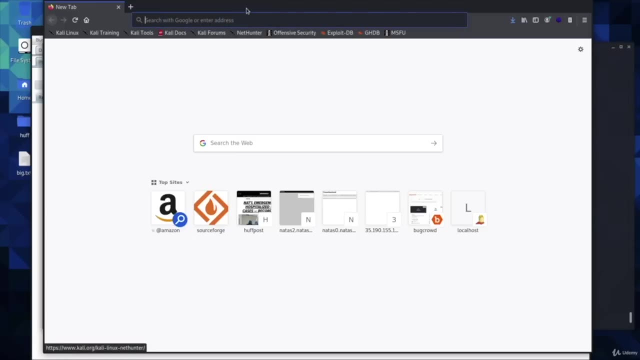 you're inside of, and so now to start npm, we just type npm, start and that will go ahead and spin up our server for us and it now says our server is listening on port 3000 and then we can come back to our search engine and 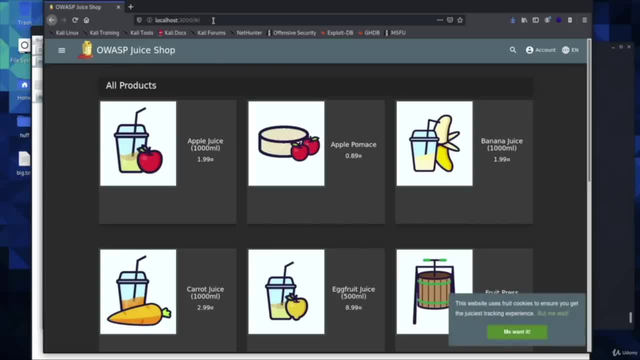 you can type: this is what we'll be typing in, just localhost 3000, and you'll type that into your browser. and this is now our vulnerable web app that we're going to be practicing on in the future lessons. but before we get to practicing and seeing what we can manipulate and what 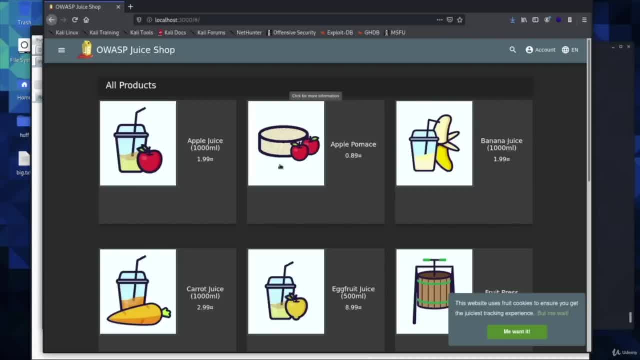 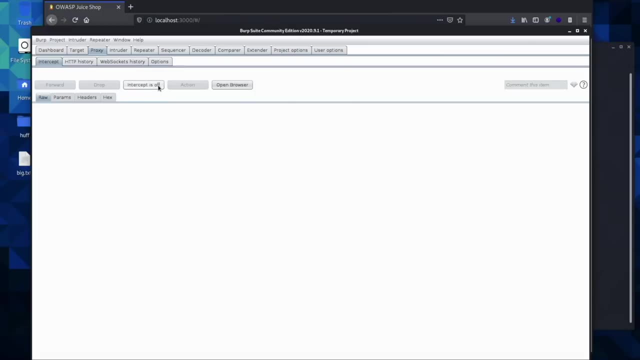 vulnerabilities we can find. i want to walk us through a little bit of what we're going to be looking for and how to identify different vulnerabilities and how we're going to use burp to help us find them. but you will notice that if you have burp running and you turn your 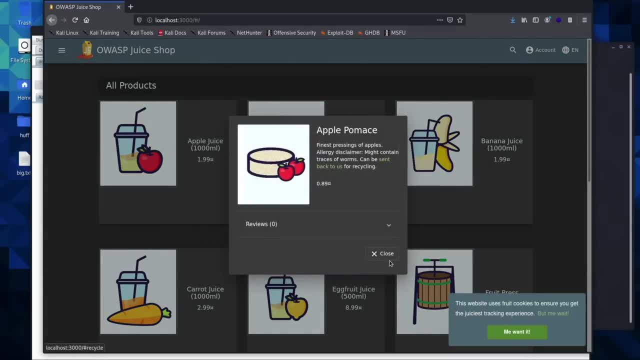 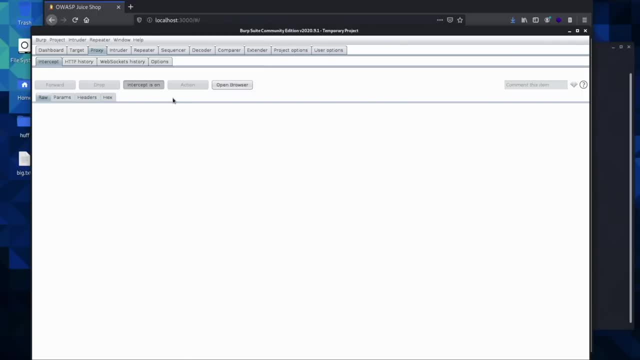 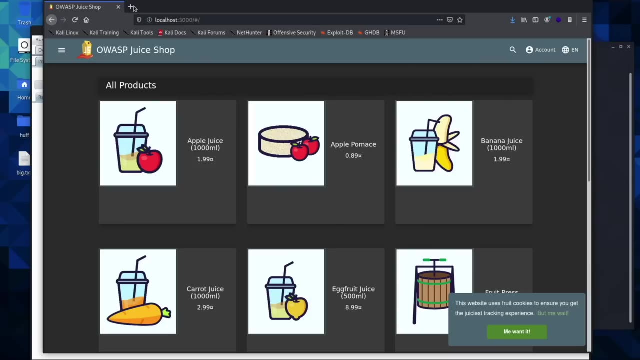 proxy on and you start clicking on things and you refresh the page. burp is not intercepting anything. it is not working for us. so we need to configure our traffic so that it goes through our proxy and we're going to do that by going over here opening a new tab we will type in about. 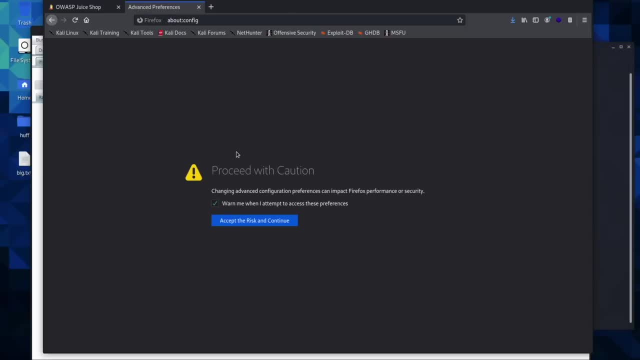 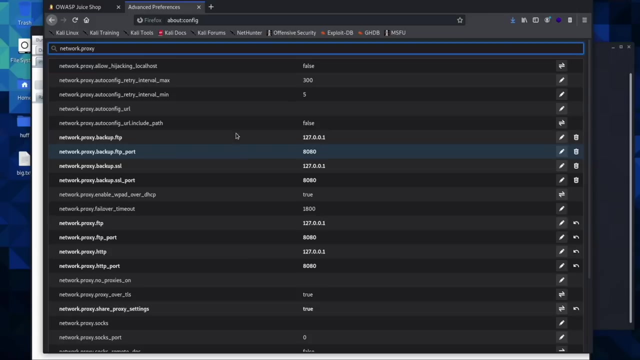 fig and hit enter, and i will warn you to proceed with caution because this will change how your browser functions. so you want to accept the risk and continue, and we are going to type in network dot proxy, and this one right here: allow hijacking localhost. we'll click this. 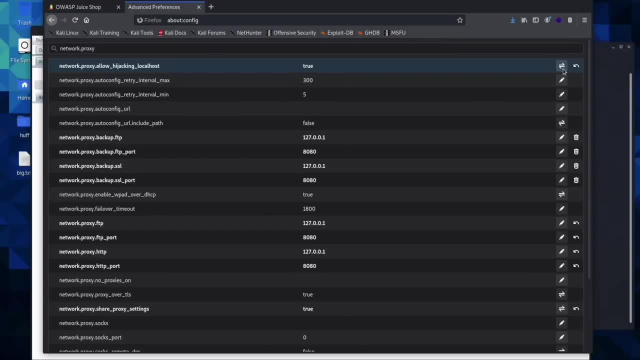 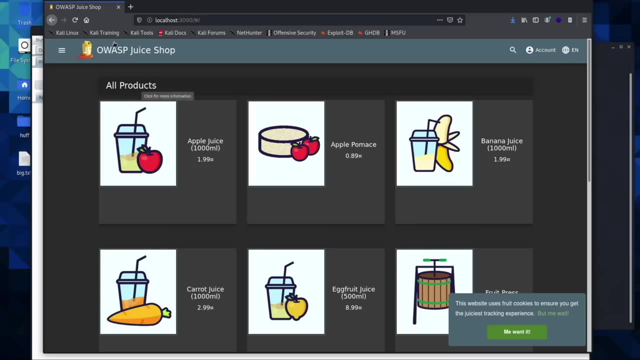 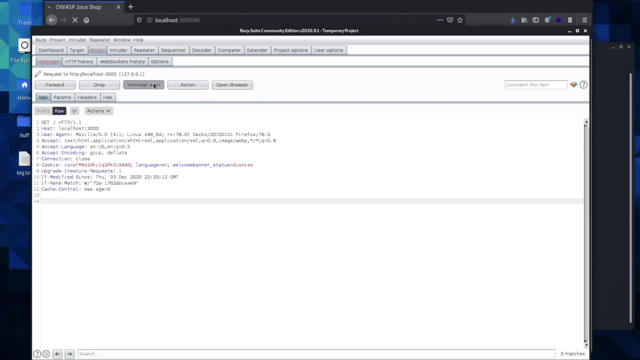 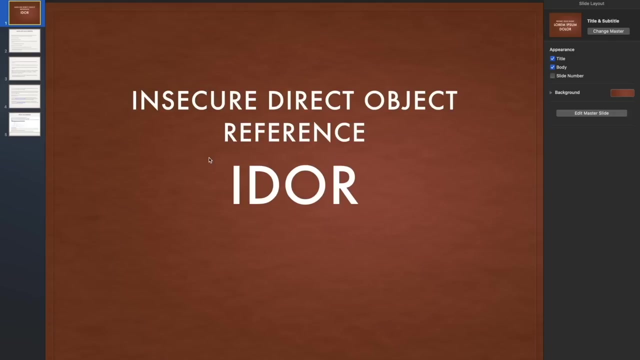 and we need it to change to true and then we can go ahead and close out of this tab. and now, if we refresh our page, you can see that our traffic is running through burp and we are able to intercept the requests. okay, in the next few videos we're going to be 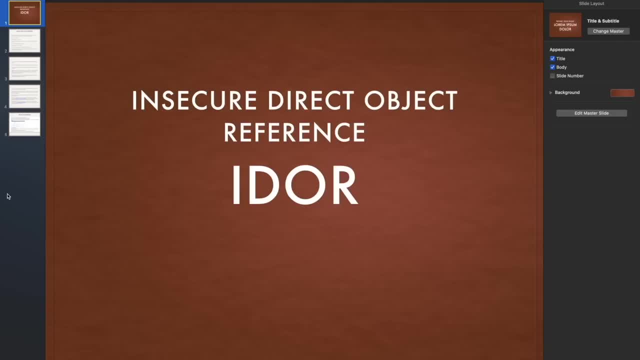 going through a couple different powerpoint. the reason for this is i think it's really important to have a little bit of experience and a little bit of experience on how to use the in-house data tracking software, but i think it's really helpful for us to have some kind of foundation. 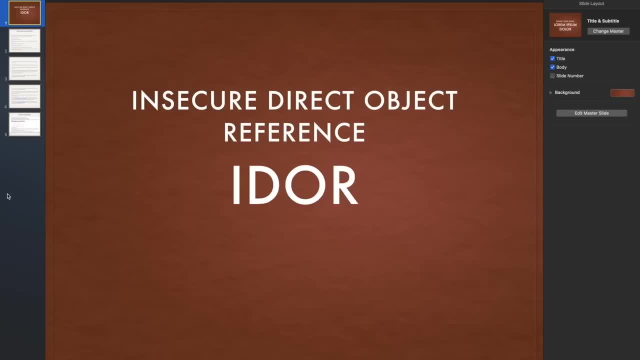 before we begin looking at examples. i think by the time we get through the powerpoint you're going to be a little confused and probably still not know what exactly we're looking for, what's going on. but my hope is that, with the powerpoints and then just a couple of examples, 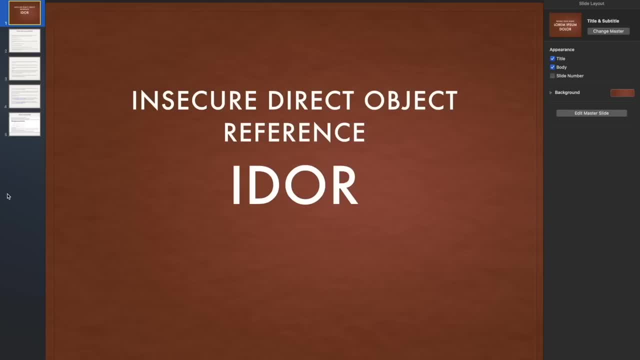 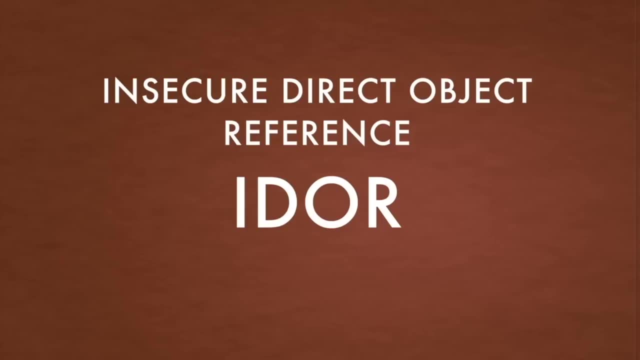 you'll be able to start finding some of these bugs on your own, and we're going to be practicing on hacker 101, as well as juice shop, which we just downloaded, and we're going to be looking how to use Burp before we begin looking at trying to exploit some of these vulnerabilities. I think 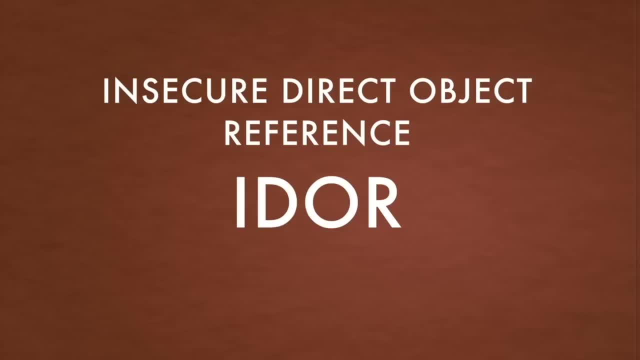 that you will be using Burp a lot, And so it'll be helpful to go through and kind of look at how it works and explore just a couple of its functionalities before we begin our exploitation of some of these vulnerabilities. And so we're going to be looking at IDORs business logic. 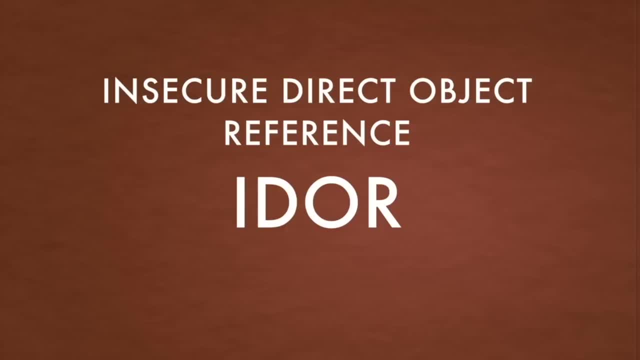 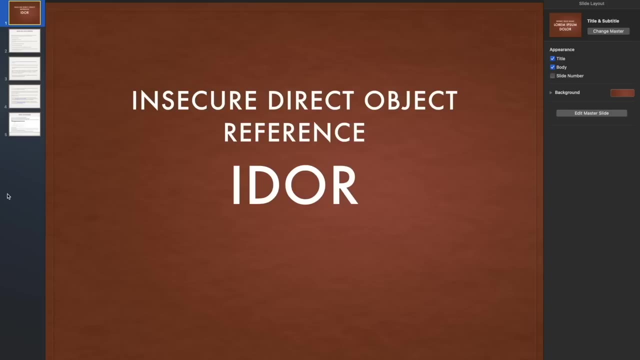 errors, and we are also going to be looking at manipulating user input and cookies and tokens as well, as we continue in this course, And so we're going to begin by looking at insecure direct object reference. These are called IDORs. That really doesn't tell us a whole lot, but 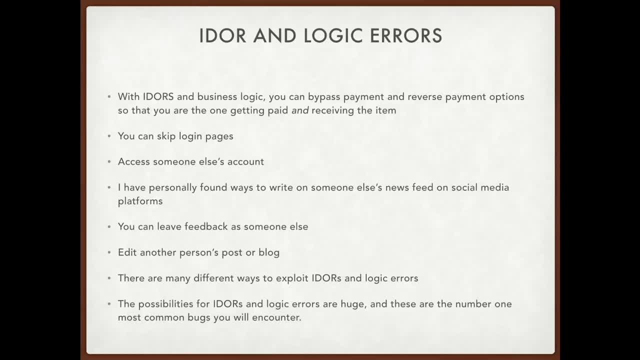 they're really simple to understand once we get going. These IDORs are going to be just parameters that we can change. that we can so that we can bypass specific functions. on a web app with IDORs or business logic errors, You can bypass payment options, You can reverse payment options so that you're the one 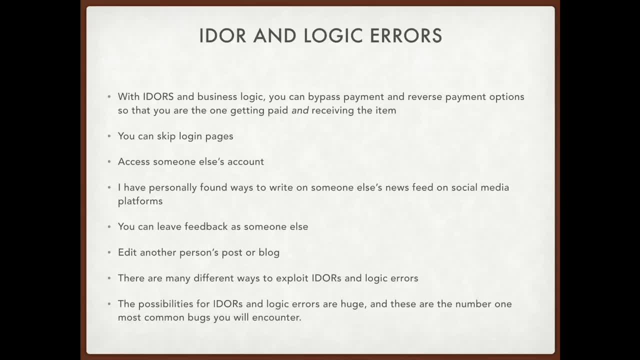 getting paid. You can put things into other people's carts. There's a lot of different ways you can use IDORs And when you're out hunting on your own, you're going to have to be creative, because there are many different ways that you can exploit IDORs. You can skip login pages. 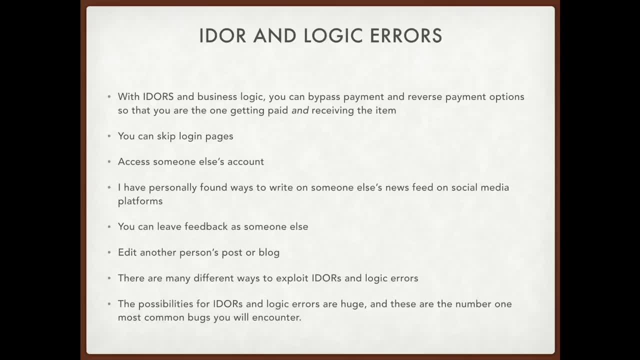 You can access someone else's account. I, personally, one of the first bugs I ever found was being able to write on someone else's social media platforms. It was actually just one platform And there was just one specific area of the web app where I was able to change an ID and write on someone else's wall. 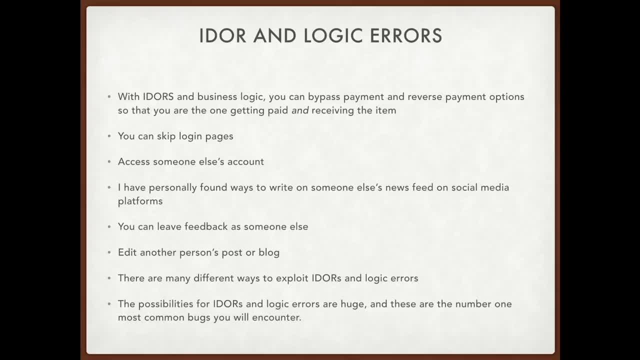 of their news feed, And so that is an example of an IDOR. You can also leave feedback on someone else's name, You can edit another person's blog or their post, And so these are just examples of IDORs and different ways that you are going to be able to find them, And IDORs are probably. 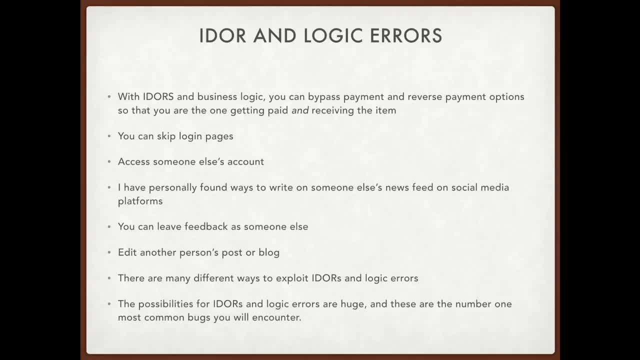 IDORs and business logic errors are going to be the most common bugs out there, which is a great thing, because it makes it easier for us to find them And they are easy to find as well, And so IDORs are something I think we should learn very well, And we are going to have a significant 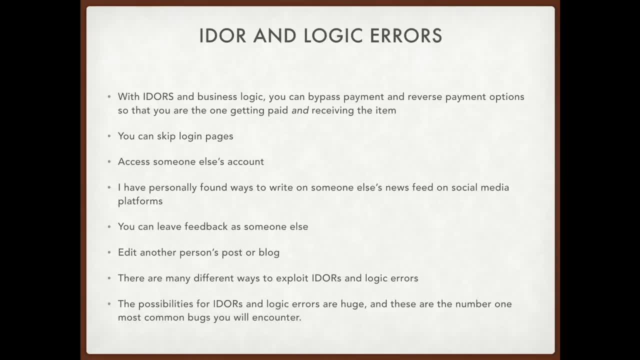 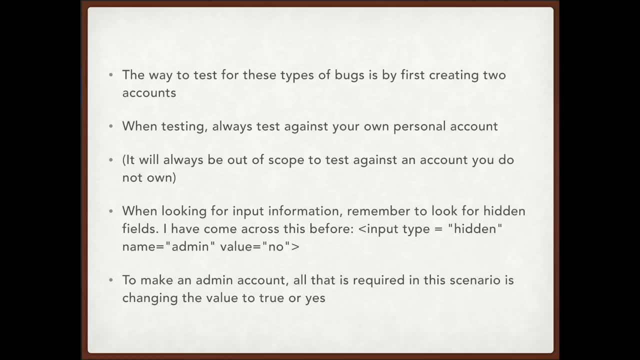 amount of time to practice these, because there's actually a lot of different areas and ways to practice these, especially in juice shop, which we just downloaded. The best way to test for these, and I think the only way, is by creating two different accounts. It is always good to create. 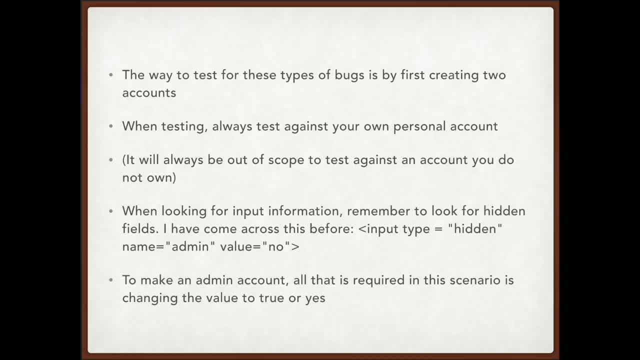 two different accounts because you will have to test in real life against your own accounts. You cannot test on someone else's account, So you can't write actually on someone else's wall- this would be out of scope- or you can't leave feedback as a different user. these will always be out of. 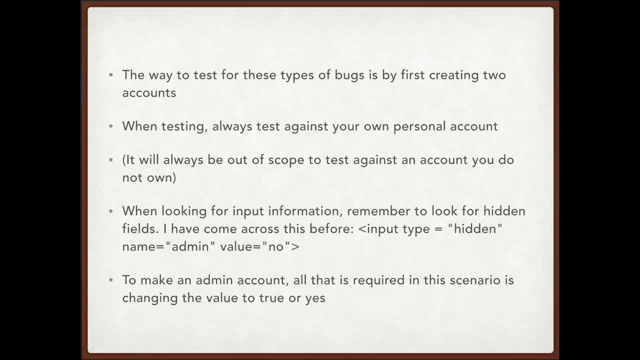 scope. you don't want to ever mess with the functionality of the application or the people who use it. you will only use your own accounts to test against, And it also makes it easier to use your own account because you already have a second ID number that you can use. 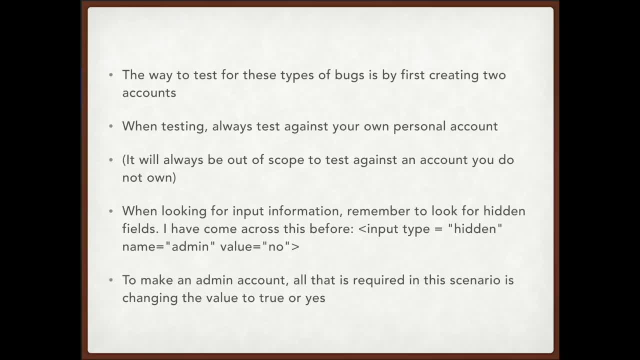 So you will have an attacker account and a victim account that you will use, and so you don't want to test on someone else's account. An example, or a simple example to remember, is to look for hidden inputs. You will actually see this as well in Burp. When you create an account, it won't say: 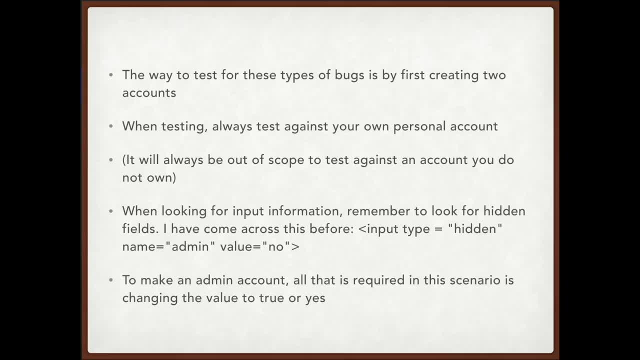 input type hidden, but you will see such as a name and your username, and it will say: are you an admin? And then it will say: value: no. An easy way to show one of these errors is just to change this value to yes or true and you will automatically have admin privileges. And we're actually going to 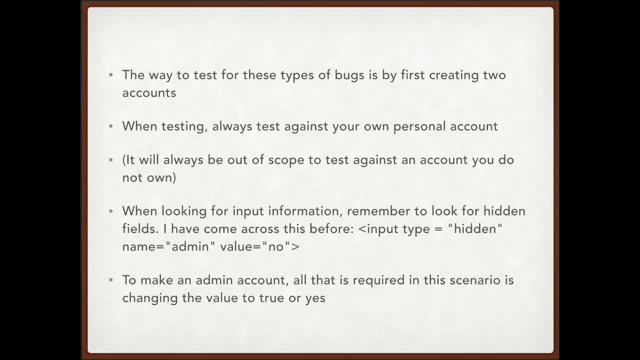 be able to test this out in juice shop, something just like this. So you'll get to see this in action, And so we're always looking for parameters and things that we can change to get us somewhere that we should not be. One of the other places that you will find IDORs is on the bottom right corner of the 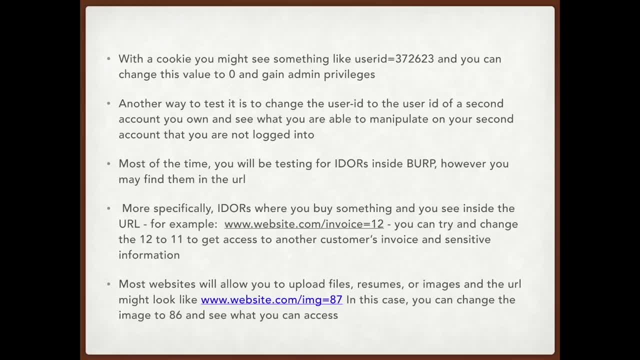 screen, And that is in cookies. A lot of times, cookies and tokens will host user information, So that's how websites will keep you authenticated- Not all of them, but some of them will be through cookies, And so you will have inside cookies. maybe you will see something in your cookie like user ID, and then a. 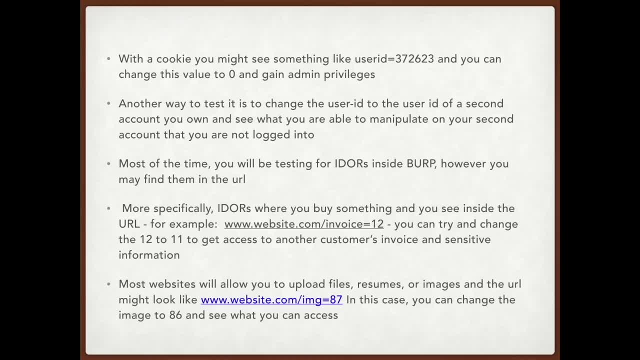 number and you can change the number to something else to see if you can access that account. For example, if you had two accounts, you would take the user ID of your victim account and you would replace it on your attacker account and see if you can access parts of that application that you shouldn't under. 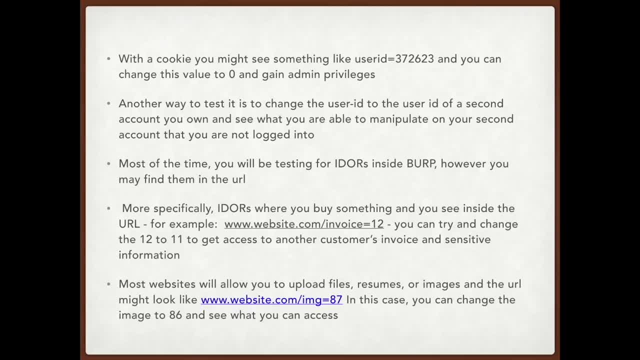 another user. If you were getting malicious with this, you would change the value to zero or one and see if you could gain admin privileges to the web app. And another way to test for this is to see if you can log in, save your cookies first, or your tokens, and then log out and then see if you. 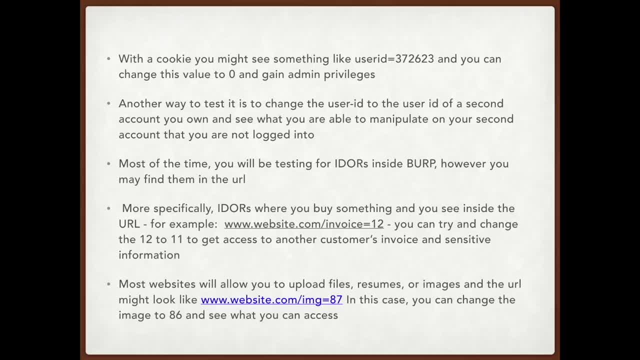 can log in and delete your previous cookies And then you can click OK And then you can see if you or tokens and then repaste in your new ones and see if they have been terminated or ended. if they haven't, this would be a logic error, because when the session has ended, so should the cookies or 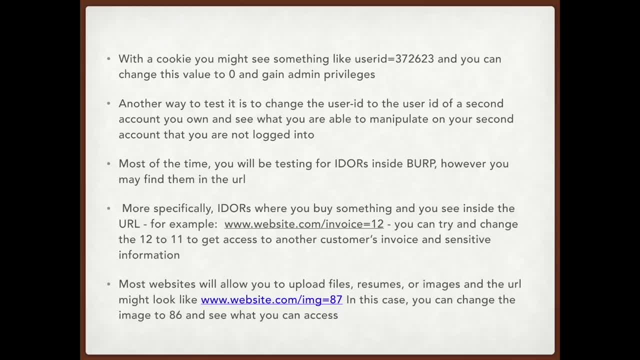 tokens, and so you can see what to manipulate and where you can manipulate different things within cookies and tokens as well. these aren't specifically idors, but they're similar. they're similar enough that i think they can be included together and so when we're testing, we're going to 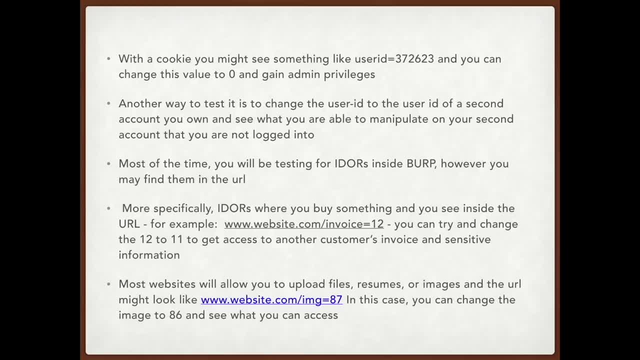 be using burp. this is going to be where we're at the most. sometimes you will be able to see these in a url. for example, if we have this example here: wwwwebsitecom, and let's say you have an invoice, you just purchased something, and it says your invoice number is 12, in a url you can just: 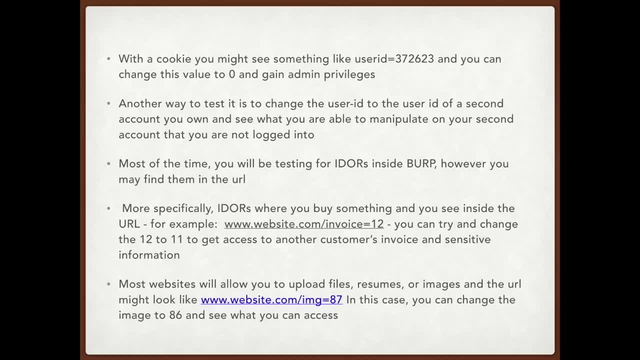 change this 12 to an 11 and see if you can access another cup of burp customers invoice and if you could, this would be a sensitive information disclosure. it's something you shouldn't be able to access and that would be a simple idor. i think they're easier to test for. 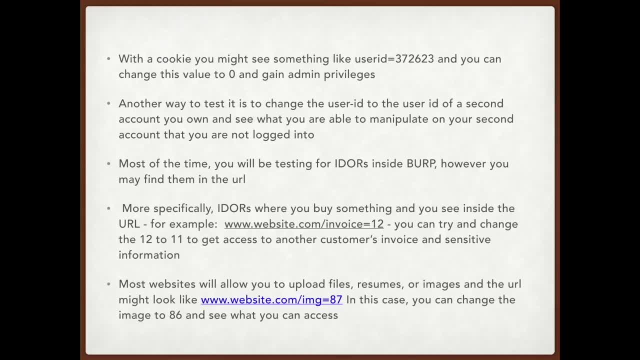 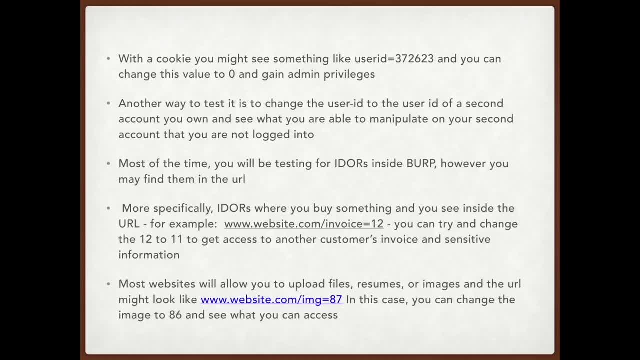 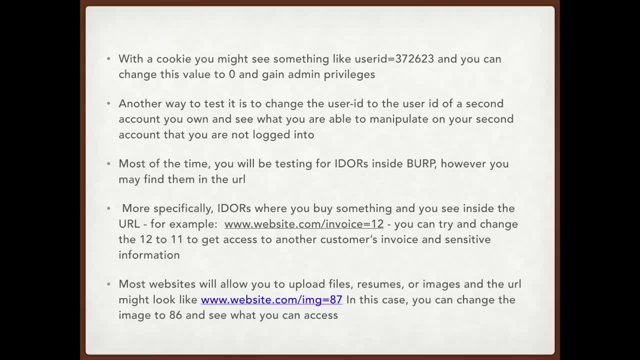 and it says: resume equals 87 and that's your resume. you could change this and see if you could access someone else's image or resume, just like you would have with the invoice, and see what you can access. but remember, out in the wild we are testing our own accounts and so i actually have 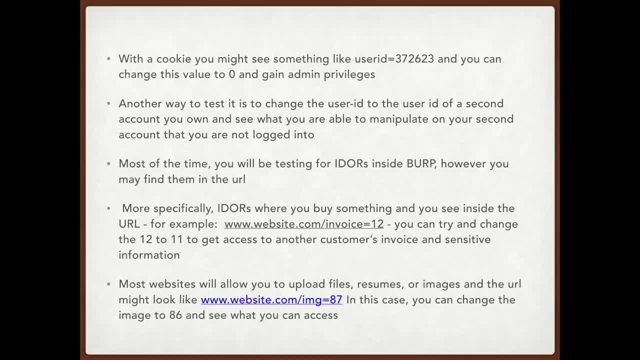 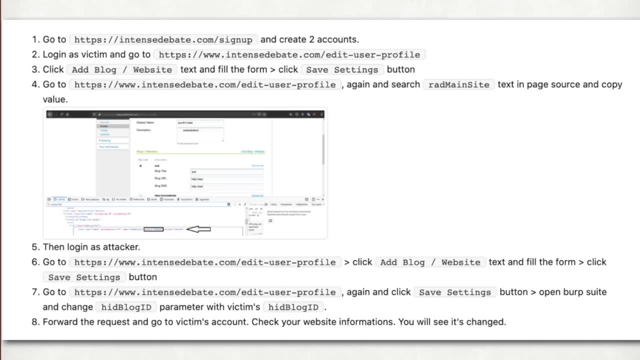 an example here for us. i pulled off of hacker one of an idor that somebody actually has found, and so we'll walk through exactly how he pulled this off and so you went to. he goes to the website, remember creating two accounts. he has a victim, logs in as the victim, he creates a blog on the site, he saves it, and then what he ends up doing. 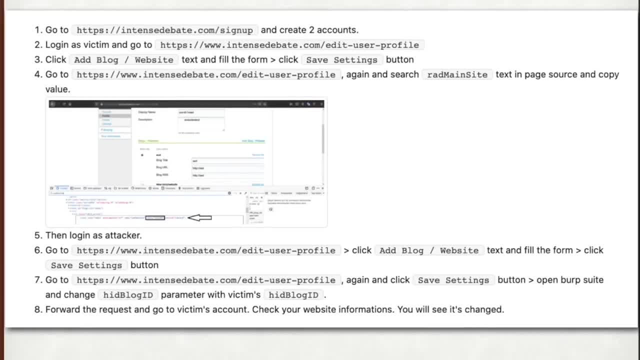 is going into the victim account or the attacker account and he does the same thing: makes the blog and then from there he clicks the save button and then goes to the edit user profile and saves it, opens up burp, and then what happens is he can change. 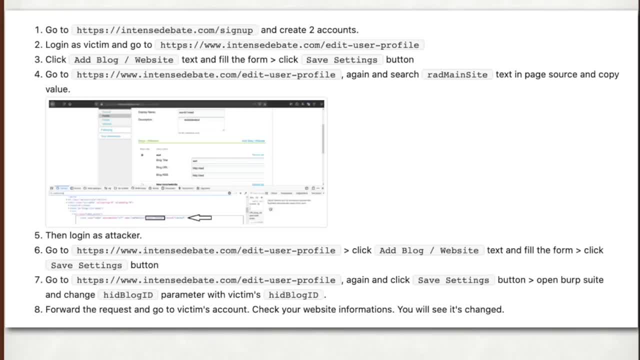 the id with the victim's id and this is: this would be a clear idor accessing something that you shouldn't be able to, and we've seen things similar to this with the urls earlier in changing urls, and then he forwards the request to go to the victim's account. 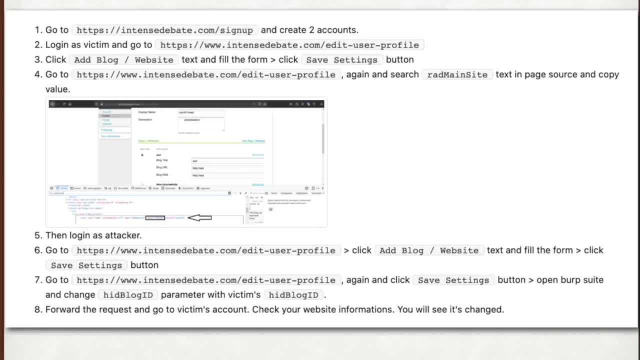 and the website information, and you can see that it has changed, and so this is an example of an idor. i think we'll be able to make this sound a whole lot easier once we're actually walking through them, and so i want to go and talk a little bit more about 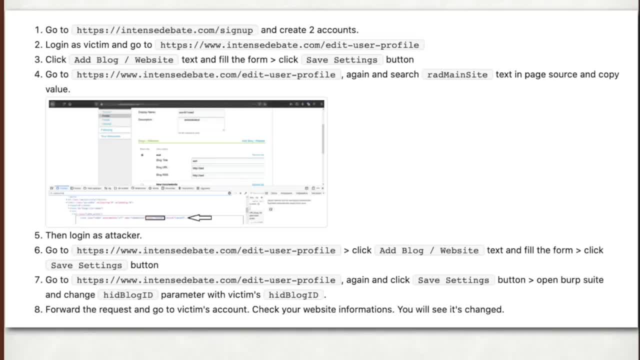 cookies and the url and what exactly we can do with them. then we're going to look at how to use burp to find idors, and then i want to turn you loose and let you try and find an idor on your own. in this video we're going to talk a little more about. 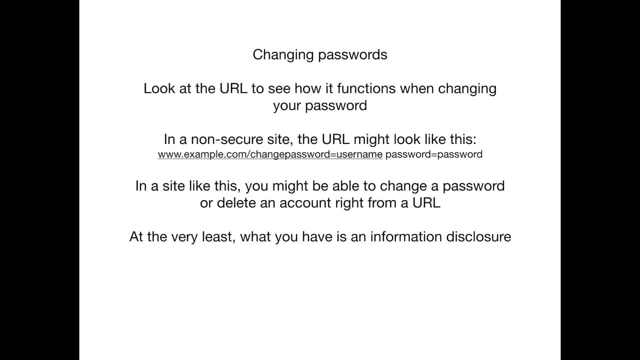 urls and what we can do with them- cookies and tokens- and then we're going to look at something called cybershef and then we'll move into burp and exactly how it is going to help us in its functionality. but before we get there, i was talking to my wife. 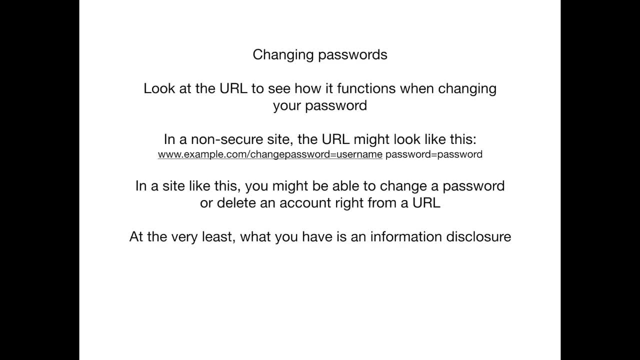 and i just said, hey, i think i'm going to have to warn that, uh, my powerpoints are going to be full of errors, because i actually made them just for bullet points for myself and i was going to keep them on my second monitor for about an hour and i believe i've gotten that right from there, so i'm going to keep them up here for awhile. 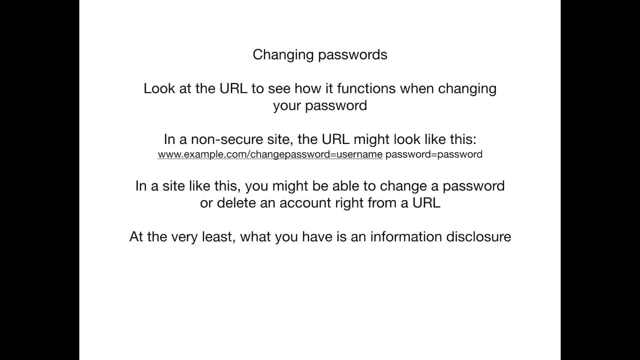 second monitor and then i realized i didn't have anything to show you and i wasn't just going to have a blank screen. so if you're wondering, how can somebody with a phd have such poor quality powerpoints- they were originally just my notes, and so i decided, rather than sit here and comb, 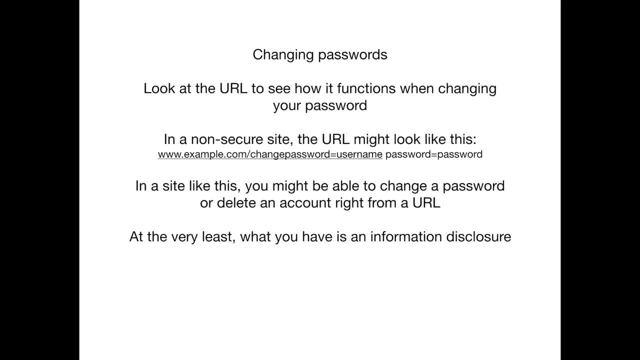 through them and go back over it. i will just show you. this is basically what my notes look like when i take notes and walk you through. walk you through them, just so we can have a better understanding of a few more exploits before we move into burp. so first changing passwords. 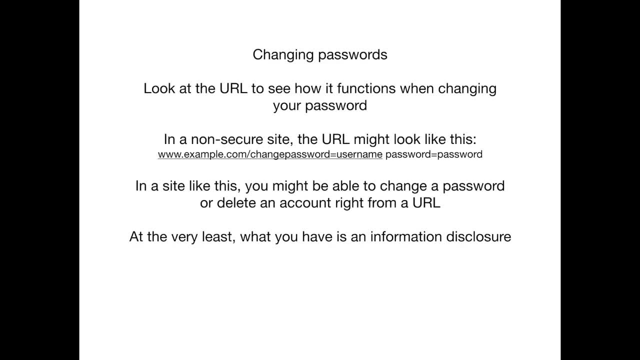 you will actually come across this in juice shop when we are practicing and more as we get further into the course. sometimes you will see a url that looks similar to this, or, in burp, it will pop up at the bottom of a post request and we will have something similar to this like: 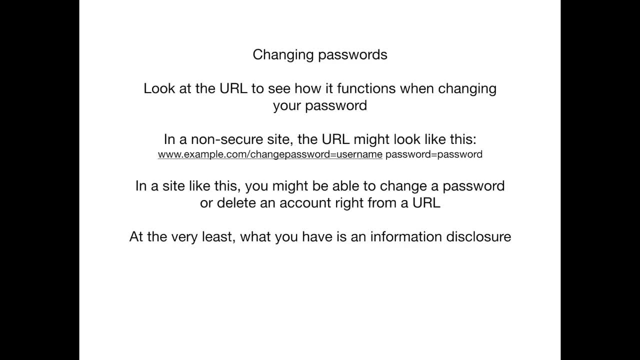 a change password, you will have the username and then the new password will be stored right here and in something like this you could actually grab someone else's username and, on your victim account, try and change the password to it and see if you're able to pull. 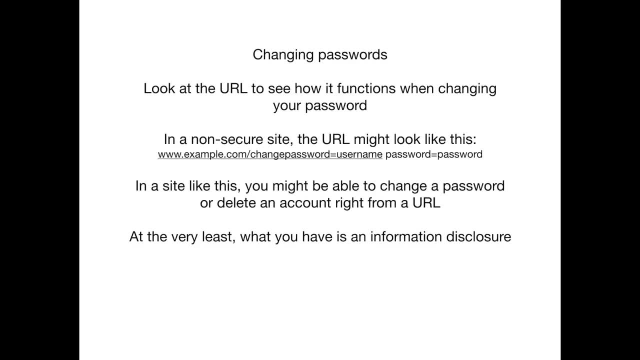 that off, or you can go ahead and see if you can maybe delete your victim account by, instead of having change password, you'd have delete account or delete user or just delete, and then you can put the username here and you would obviously not have the password. you will also, in burp, be able to. 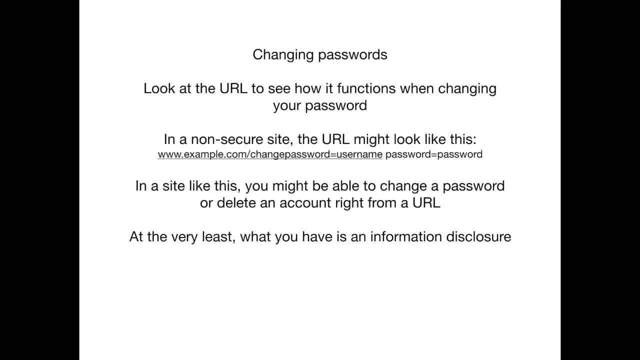 have delete, instead of you'll have put post delete options and you can try and delete the account through burp. and if you are unable to, even if you aren't able to pull any of that off, if you have a url that has a username and a password in it, even if it is encoded with something as simple as base, 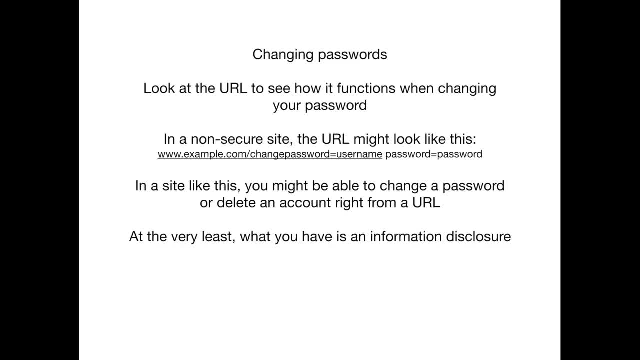 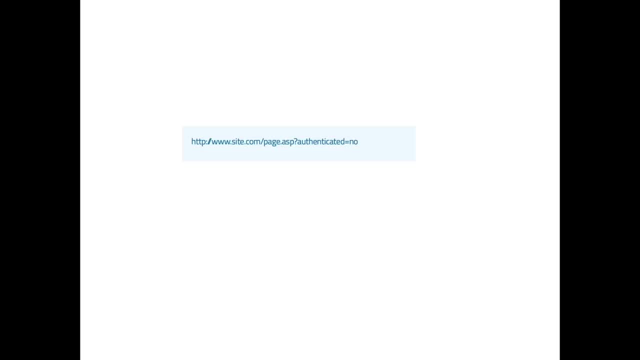 64. this would be an information disclosure and we'll get to why this would be an information disclosure in just a few slides. we talked about this a little bit in the last, the last powerpoint in the last video. if you have a website, something similar to this, which actually just copied this out of the oosp guide and the oas, 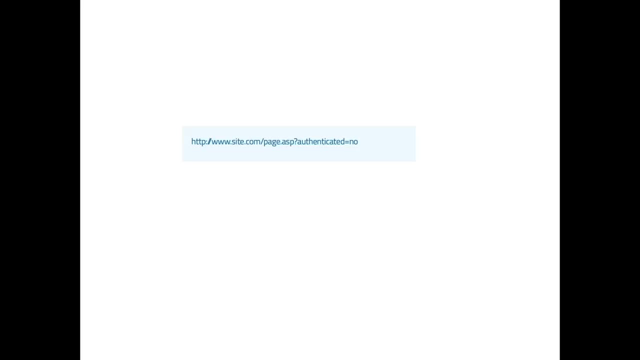 pen testing guide, as well as another image that we're going to come to here in a second. sometimes you'll come to something like this if you are logged out and you copy and paste in a url that requires you to be authenticated and it says authenticated no, and it does not allow you. 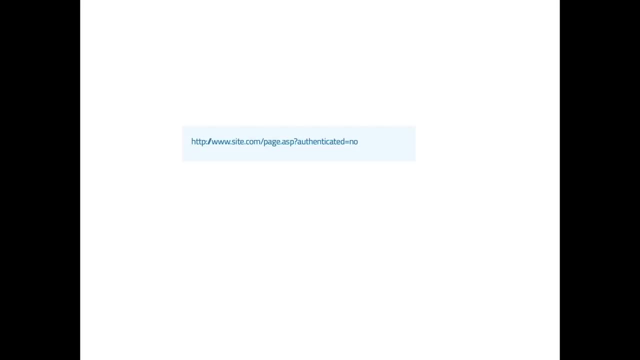 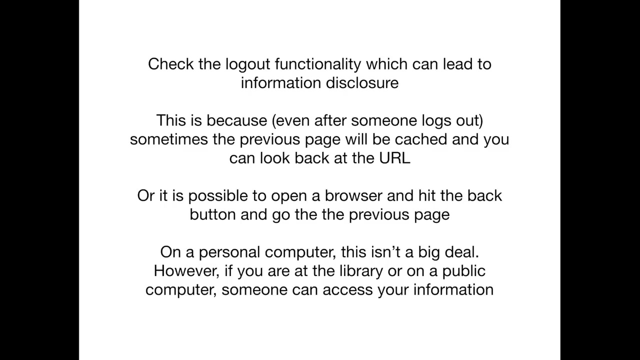 to view the site. you can just change this authentication here to yes or true and see if you are able to access the site and see what you can gain access to, and then we can check the logout functionality. and this is why it is an information, information disclosure, if you have. 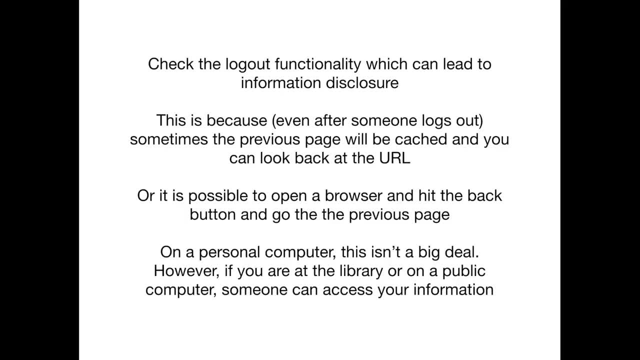 a username and a password in the url, because it is possible for you to log out on your computer and then close the browser and you'll be able to open up the browser and back up your experience. okay, so anything Karl is gonna do, that's available in the safe widely here. so i'm gonna go ahead and right click here and we'll get on my business plan update after this or the webinar is open. so i dip it right click still to clear this and refresh it. that's available here and that's why the email is on that mobile screen. so that's where the incoming details are up. so comment and i'll be able to take that. 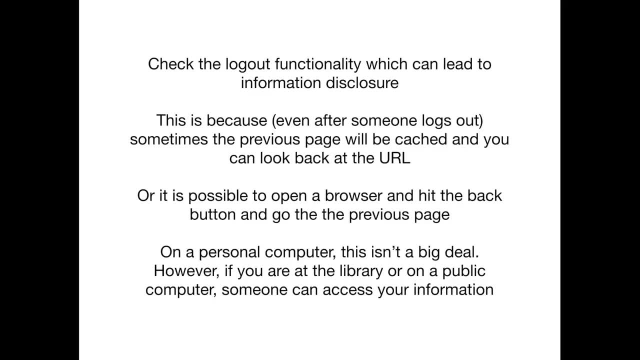 browser and it has a cache- the previous page that you were in- and you can go back into the history and open that page and if it opens- even if you're not able to go to any other links because you're not authenticated anymore- but if it opens that URL and your username and password is in there, it would be an. 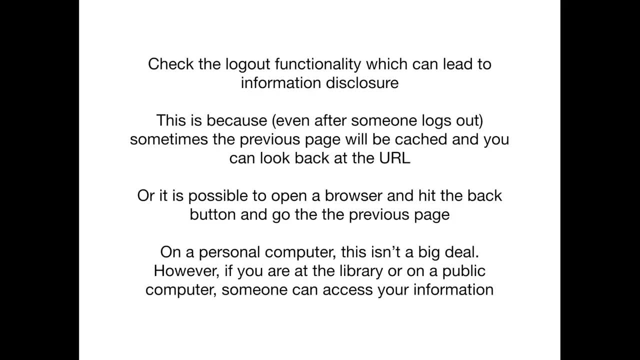 information disclosure, or if you log out and you don't close the browser, it's possible to hit the back arrow or the back button and go to the previous page and have the information there, and this can also be more than just information disclosure. if you're able to hit the back button after you've logged out and 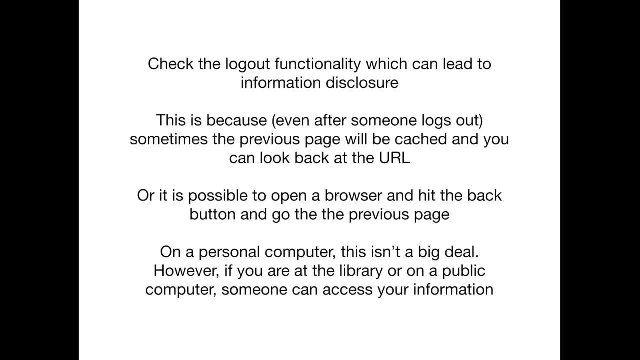 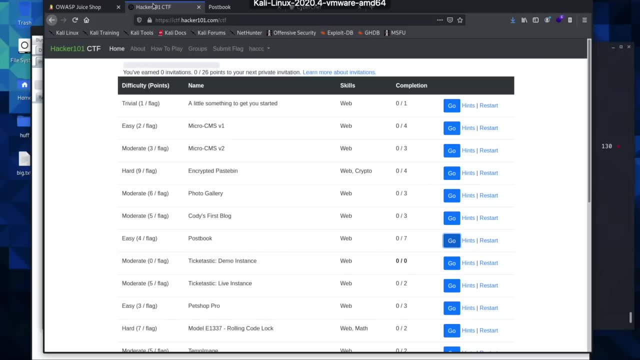 then browse the site again and it reauthenticate you. this is something that's listed in the OWASP guide. it's something that happens. it's not very common, but it's something to check for and you might be thinking this isn't a very big deal, because that's what I originally thought I was. okay, we are going to in. 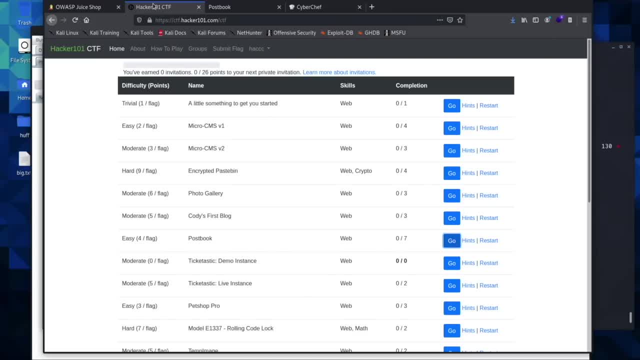 this video, go through some of the functionality of burp, and so I'm going to go ahead and have you navigate over to Hacker 101 and get into their CTF and we're going to open up post book and you can go ahead and click, go and pull it. 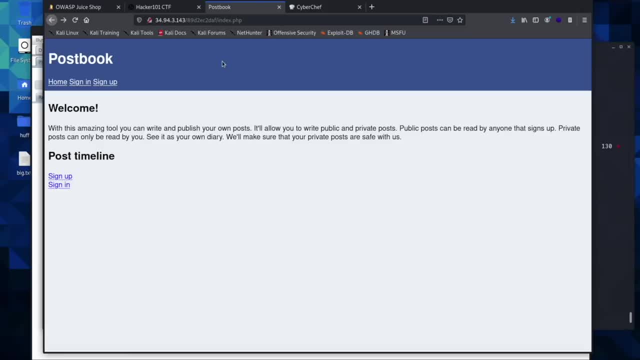 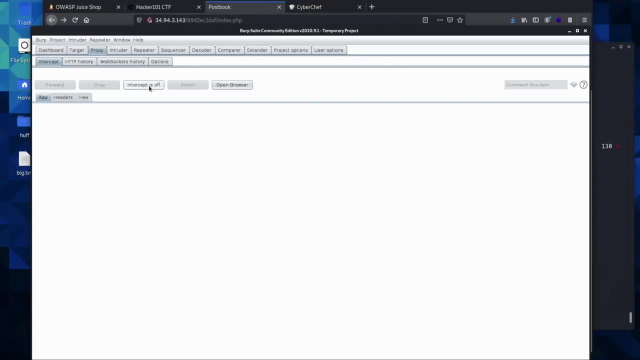 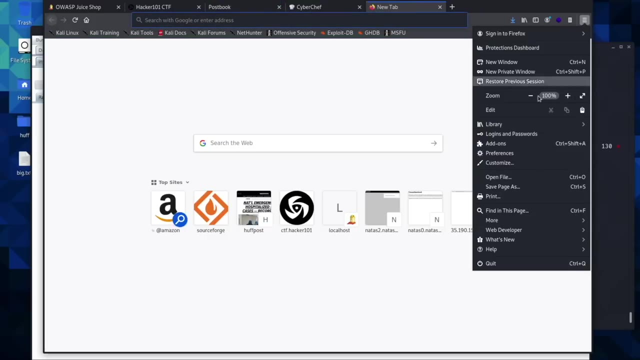 open, and when you're there, the first page you'll come to will look like this, and so we'll go ahead and come over on burp. you can turn your intercept on and make sure that you are sending all of your traffic through your proxy by coming over here. we'll go to preferences scroll. 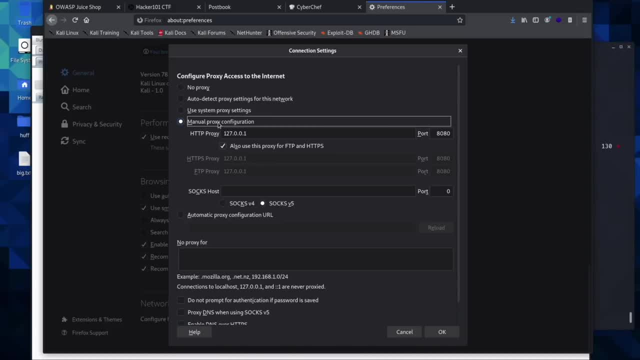 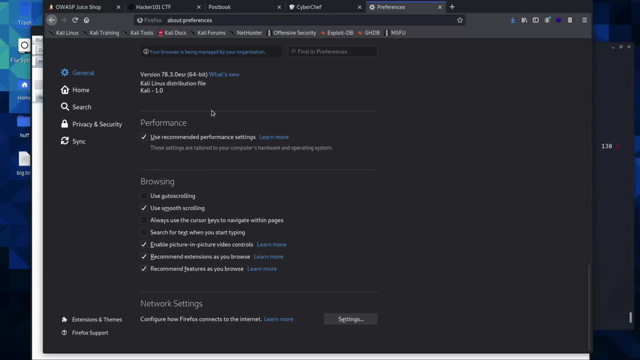 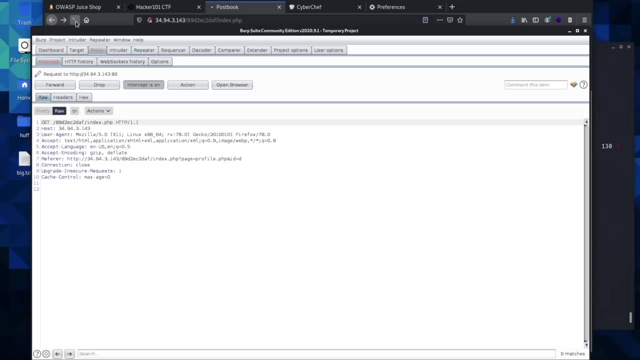 down to setting and make sure that you have manual proxy configuration, and then it looks like this: and once you have that done, you can click OK and your proxy should now be set up to intercept your traffic. and just to give it a test, you can refresh the page and make sure that it pulls through here and you can. 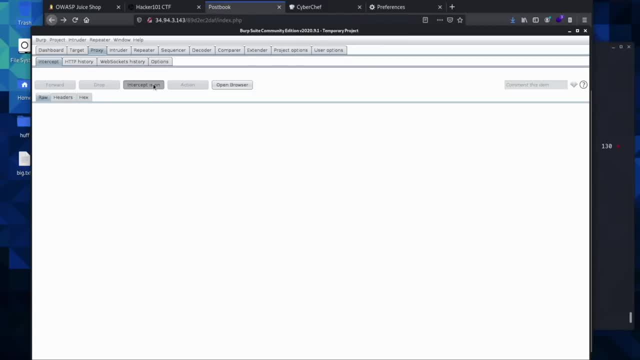 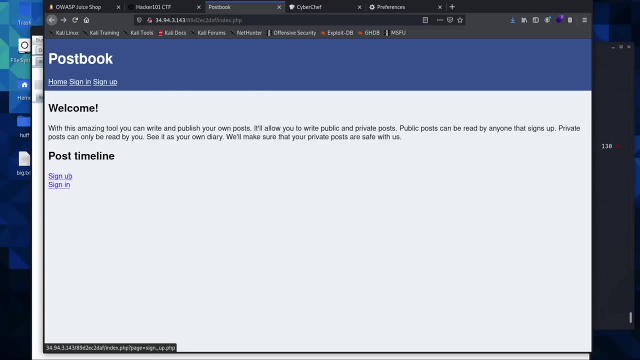 forward all of the requests we intercept, or you can just turn it back off and then turn it back on, but we are going to come in here and we are going to sign up, and so we'll go ahead and click sign up and you can just see what's going on in. 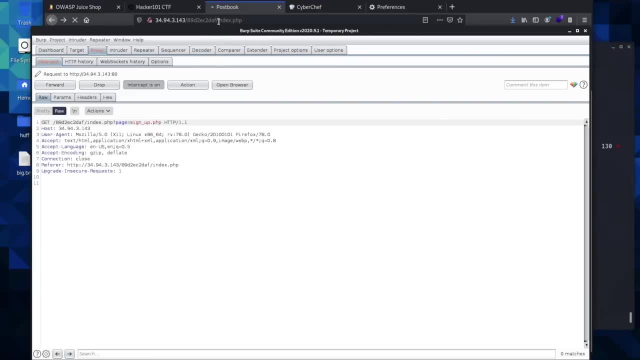 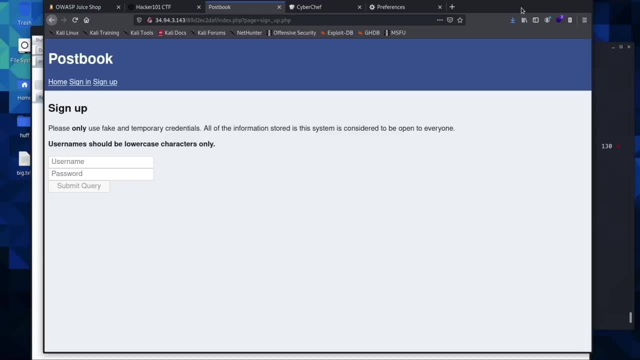 here we're have our sign up PHP. you can see it's pulling that from our URL. we have a get request. we'll forward that and we'll come back over here and we're going to go ahead and click sign up and we're going to go ahead and. 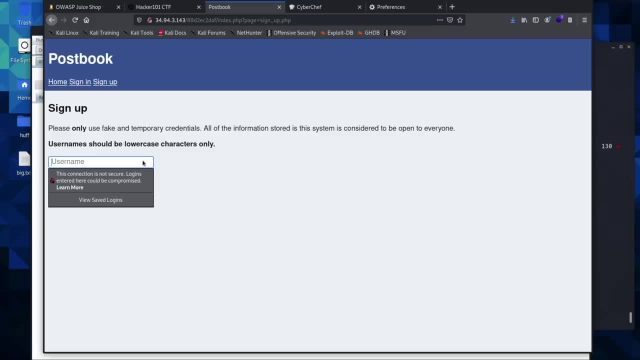 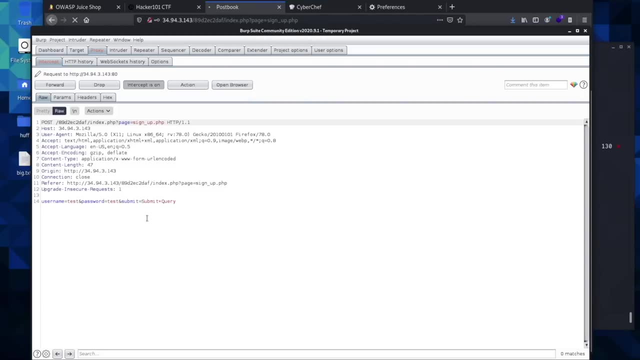 this is where you're going to make your username and we can just type in test and password can be test and you can submit your query and then in here you can see your username and your password. and if you wanted to actually try and mess with this and see what we can do with it, we would send it to repeater. so 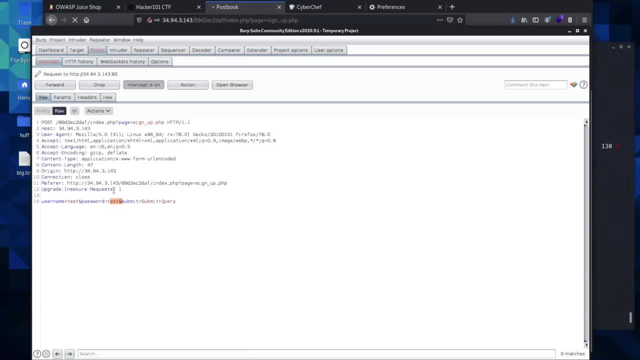 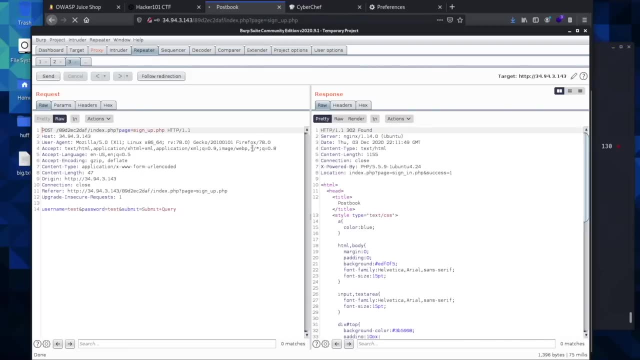 you just right click and click send to repeater, and over here we can send this request as many times as we would like to, and so in here we can go. we can change the username and click test one and then send it, and we are getting a. 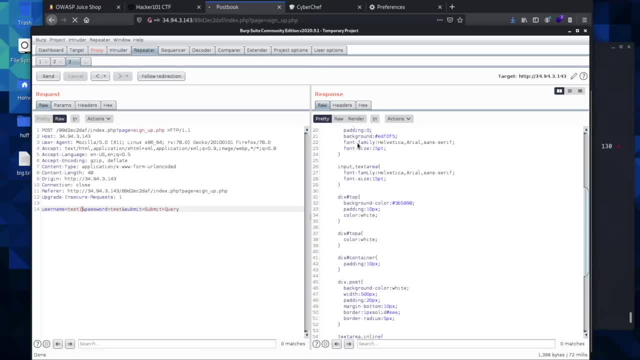 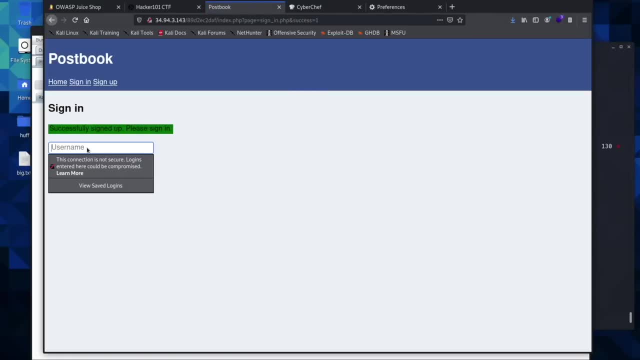 302 in response. so let's go ahead and shut this off and see we have successfully signed up and I think we actually created the test one account as well. yep, so we have made the test account and the test one account. and while you're in, 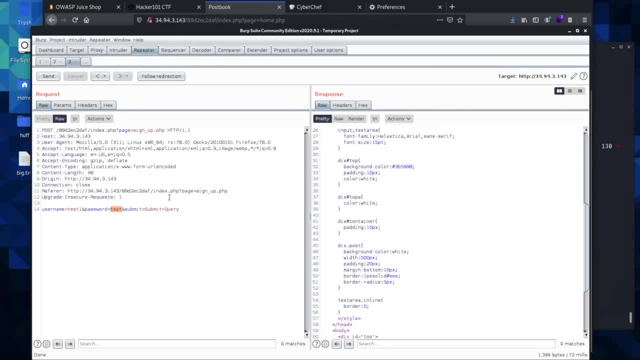 repeater over here. you can see that this would be not a very secure way of submitting these things. you will actually come across this pretty regularly, even on large, very common websites, and you can see what what you can do here. you can try and manipulate things and see just what you can do, and 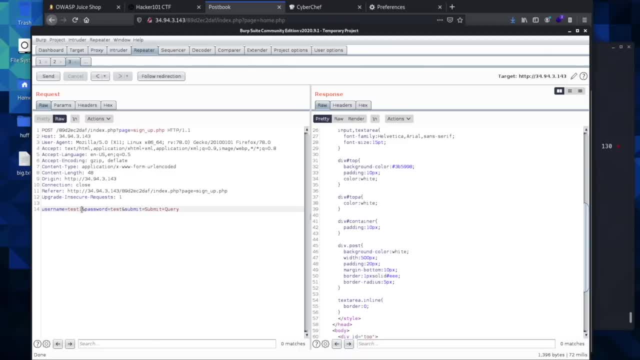 maybe type a get request and change to a different URL and see what response you get over here. there's lots of things you can do and in repeater you can send this as many times as you want to the server and really just try and figure out if you. 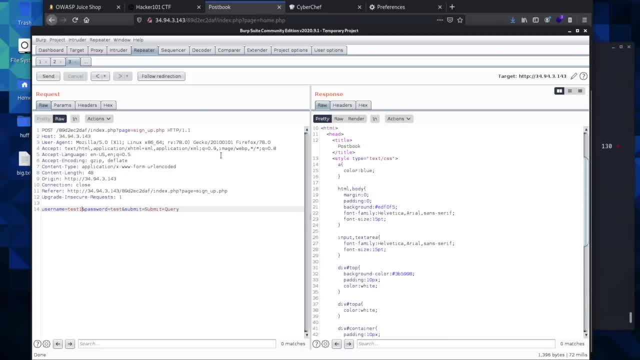 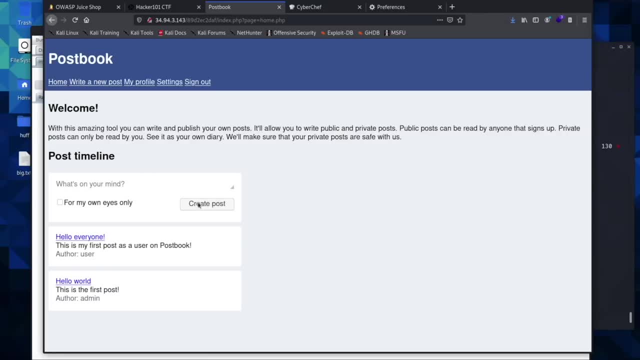 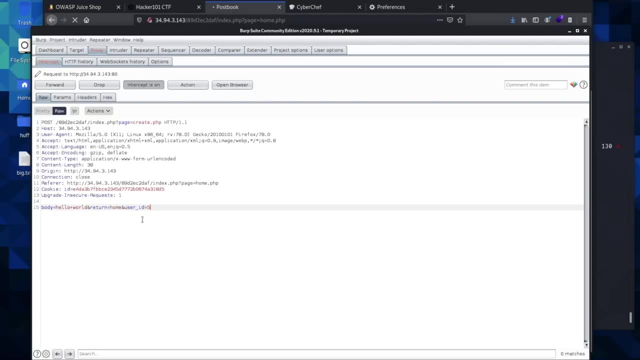 can get anywhere, that you shouldn't be with this, and so we're going to go ahead and come back to our proxy turn it on. now we are going to just create a post. go hello world, create post. we have a user ID of five and remember every time. 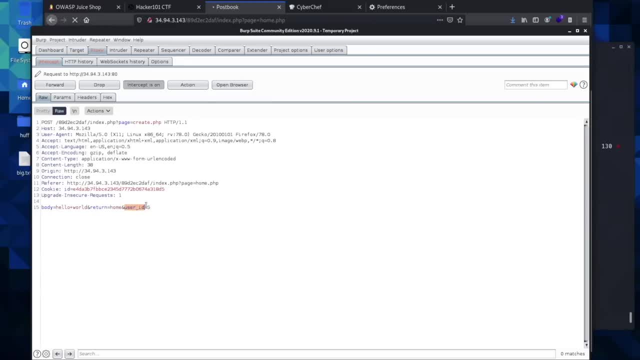 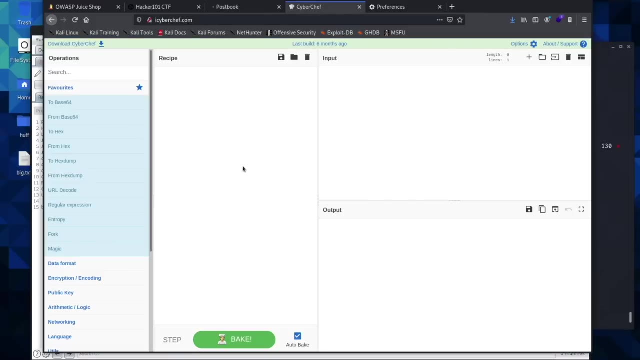 we see ID, we should be thinking: I door, what can we change? where can we go? what can we get which? and we have the body of the message over here. we have a cookie over here. you could bring this over to cyber chef and see if maybe there's anything in there. 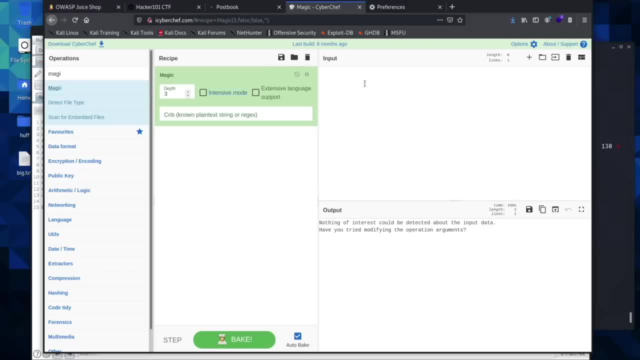 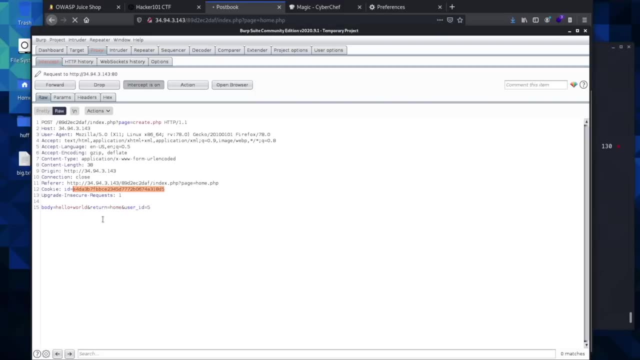 of you, remember. we just go magic and then we would pace it in and you can see we didn't get anything of our cookies and so that's ok, we can come back here. we can send this too, says we get a redirect. you can follow the redirect and then come down here and 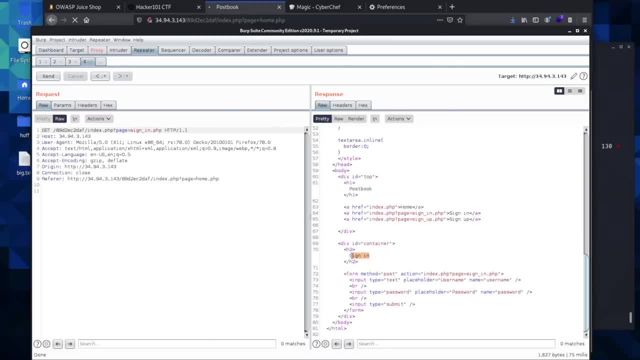 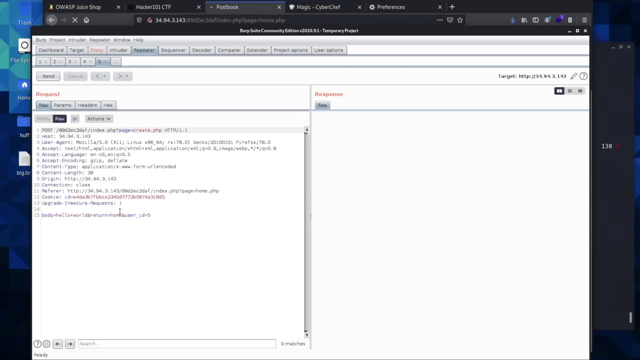 see what your response is, and it says we need to sign in, so you have to be authenticated, so the cookie is necessary, something that we have to have in order to continue on, for authentication purposes. but, as you can see, this is kind of how I would just go about testing at the beginning. just see what I can do. 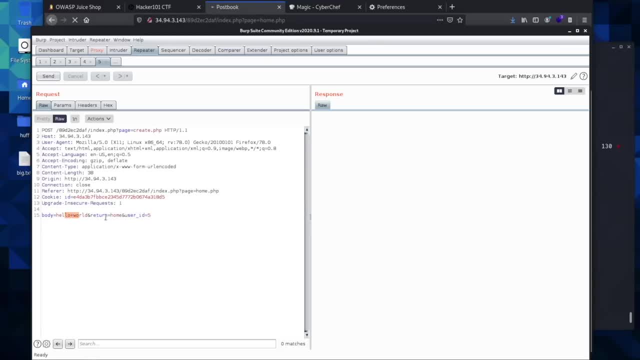 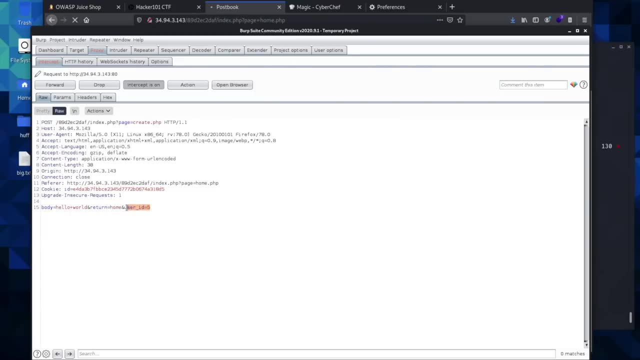 with this ID what I can do with burp, with body, see where I can get, where I can go, see what responses come back, and with that I think I've given you a pretty good clue here with this user ID there is an IDOR in post book. I'm going. 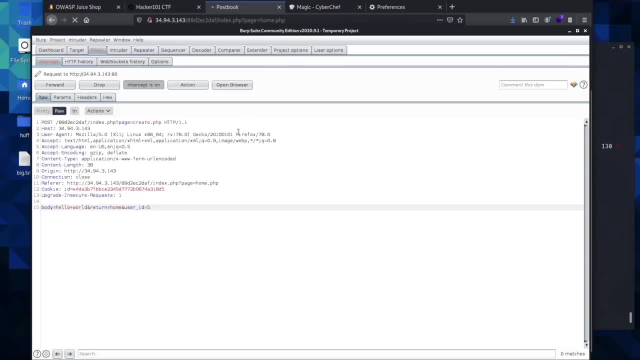 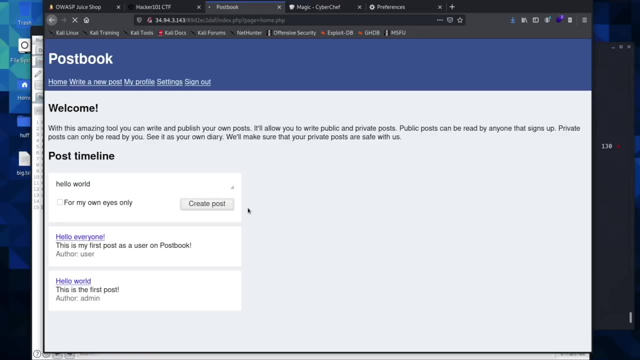 to give you the challenge now to open up burp. come in, make an account or two accounts and see if you can find the IDOR. before we go ahead and solve this challenge, I want to introduce you into one more functionality in inside burp that is going to be helpful in the future as you're doing bug bounty hunting and 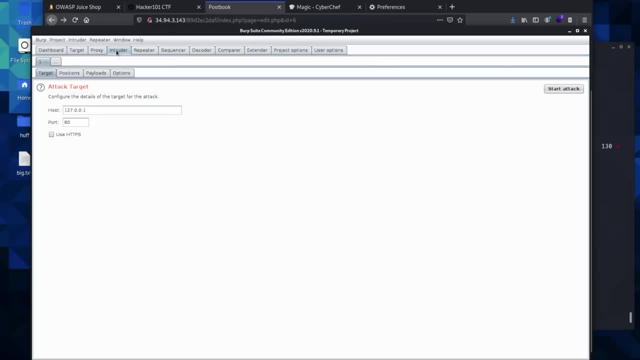 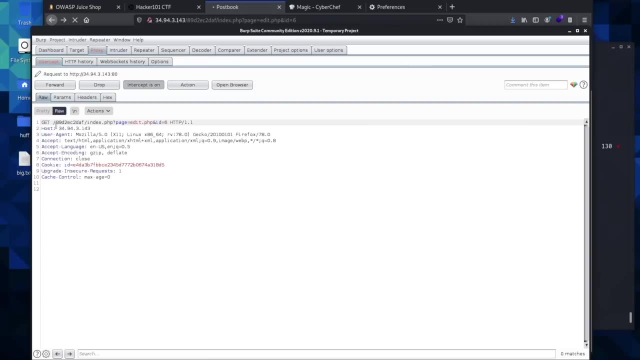 that is the intruder. we're still right here in intruder. one of the things we could do with intruder is, as we come in here and we just refresh this page, we have this id of six. let's say there are thousands different numbers in here. what you can do is send this to intruder and it will. 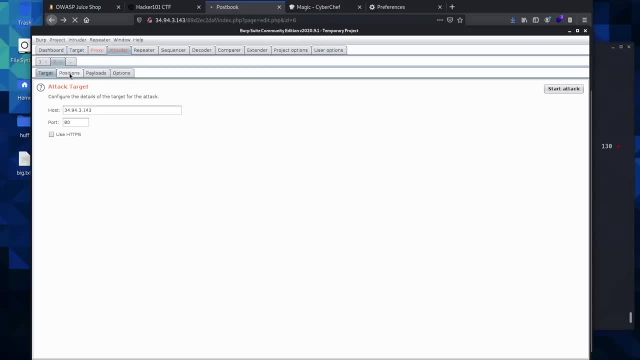 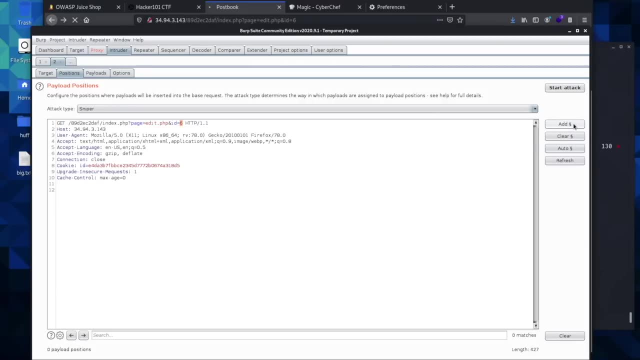 actually go through these numbers for us. you can come over here and you can go to position and we will clear this and you'll highlight this number six and what it does is it will go through every number we specify in here and replace that number six and then give us back the response so we can. 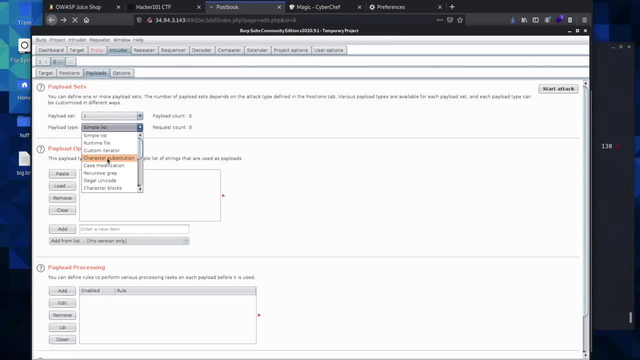 come over to our payload and we can go simple. we can do a simple list and then we will put in just numbers. we'll do one through ten. so you just go one, two, three, four, five, six, seven, eight, nine, ten, and now we have just a simple list and we have just the one position and we're going to go ahead and run. 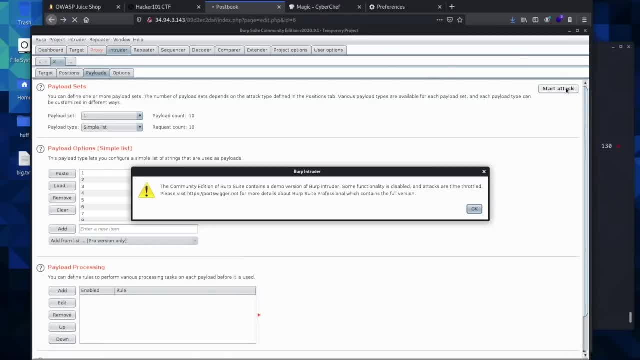 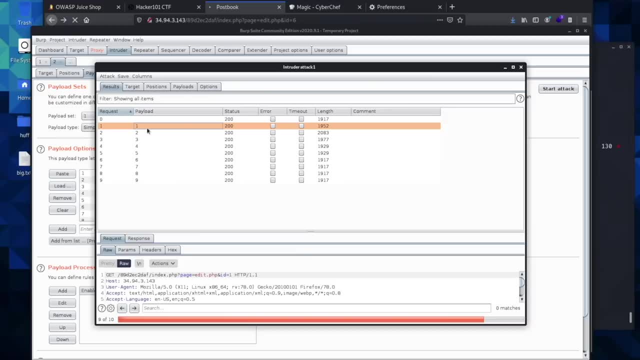 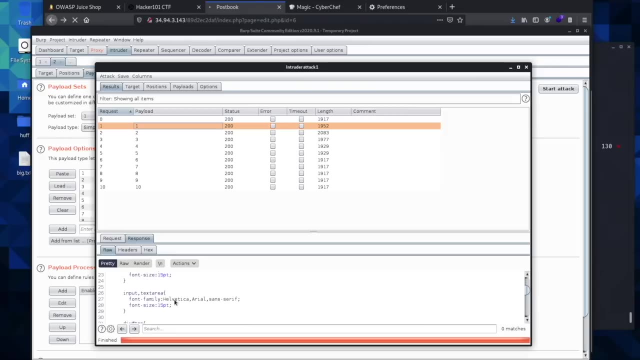 through these numbers and so what you do is you click start attack and go okay and it will automatically replace that for us, and then we can click on these and see what we have in the response and you can come through and see if we have found anything in here. says: write a new post. my profile it doesn't. 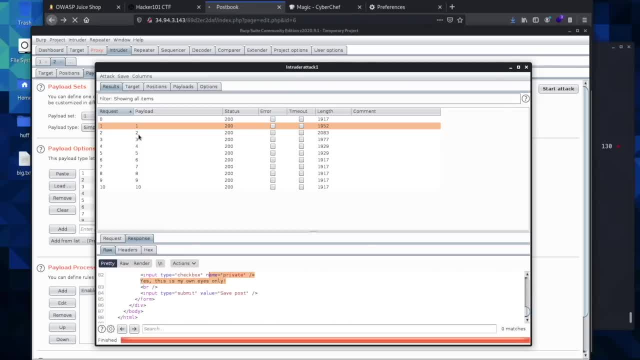 look like anything private. this is, for my own eyes, only number two and we have. we see the same thing and this one actually has someone put in actual content, and then you can go down to number three and you can see how this would make it easier, so you don't actually have to go through and do one, two, three, four manually. you can, but you 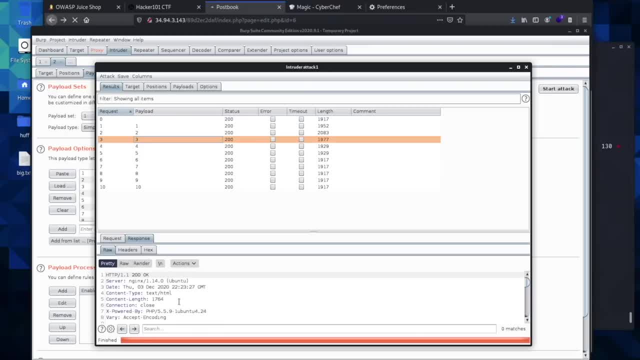 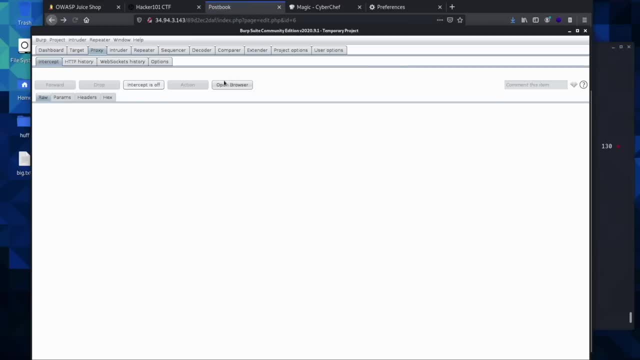 don't have to, and so what we would do if we wanted to get more malicious with this. as we're looking for an eye door, we can come back into our proxy here and you can turn it off, or you can use burp. I'm going to use the URL just because it's what we're used to, but I would encourage you to actually. 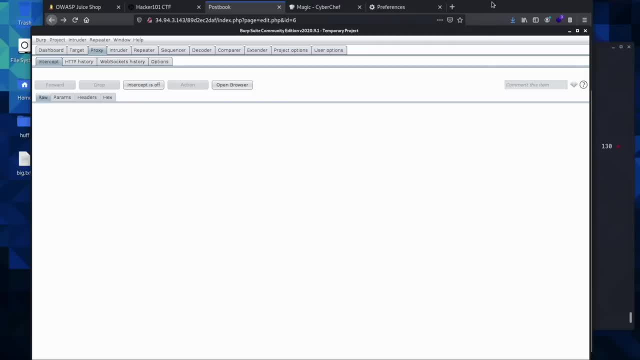 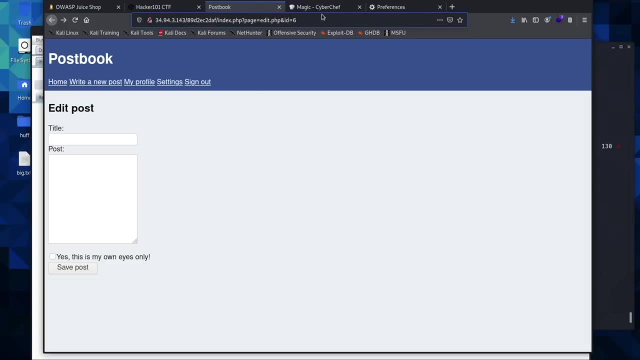 try this with burp- going to show you how i would do it with the url, and then you can actually come in here and see if you can run this exploit and find the flag with burp and without using the url. and so what we do is the exact same thing: you can come in here and you can just go one. and then somebody posted this. 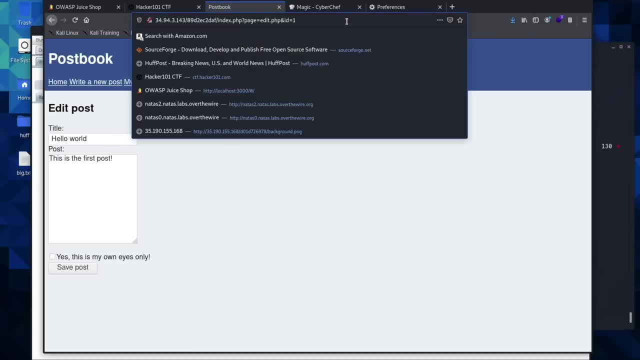 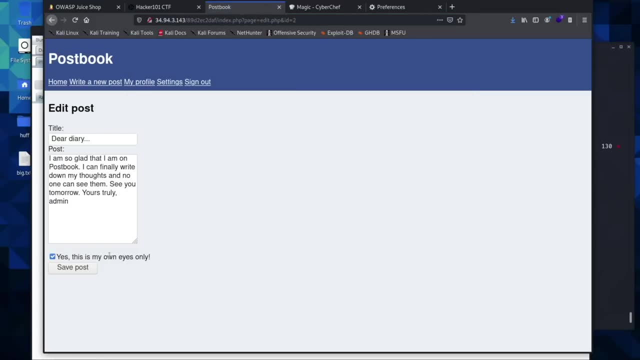 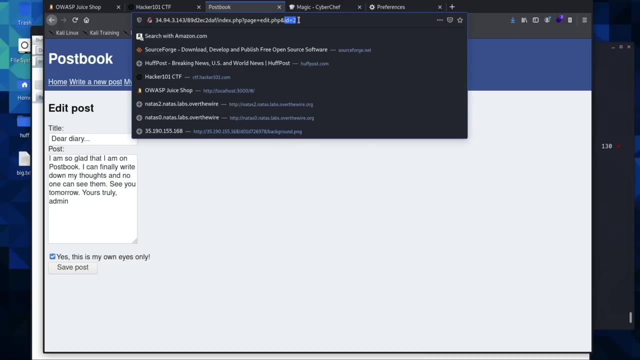 it's not private, it's too public, and you can come here and you can type in two, and this actually has the check box. yes, this is my own eyes only, and so this would be something that is not supposed to be seen by everyone, and so this would be considered an eye door if this was. 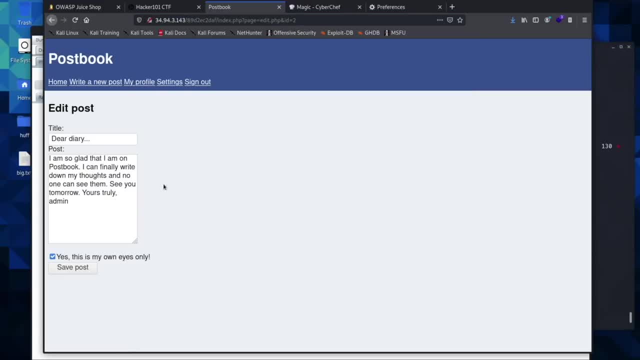 an actual program, you could report this as an eye door. and not only that, you can write inside someone else's entry here and then you can save the post. and in saving the post, i am not actually sure why there are two flags, maybe one for writing on someone else's. 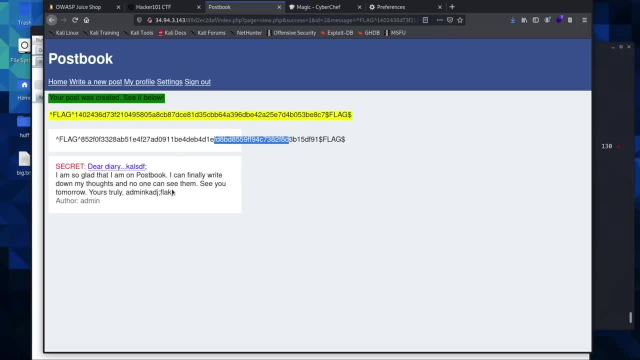 wall and one for the i door. i'm actually not entirely sure, but you can see the author was also an admin, so we made it beyond just a regular user and into an admin, and so this is how i doors work. we're going to be moving from postbook into juice shop and the way i want to. 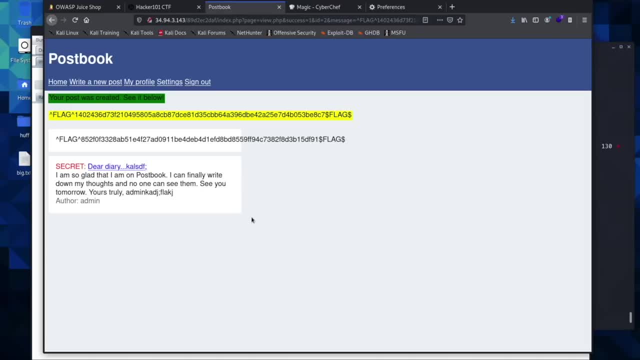 work through the juice shop vulnerabilities is by giving you just little hints and maybe telling you where, what part of the application there is a vulnerability, and then setting you free. and after you have spent a significant amount of time and you're starting to get frustrated or you want a clue, just continue watching the video and i'm going to work through. 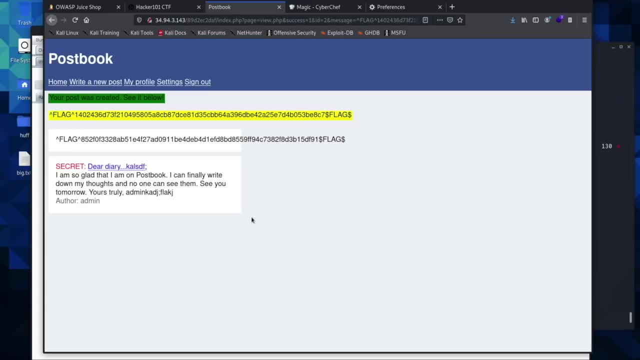 some of these vulnerabilities step by step, but i want you to give it a shot and try and figure out where the vulnerability is and see if you can solve the challenges on your own, and only if you're really struggling come back and get another clue and then pause the video again and 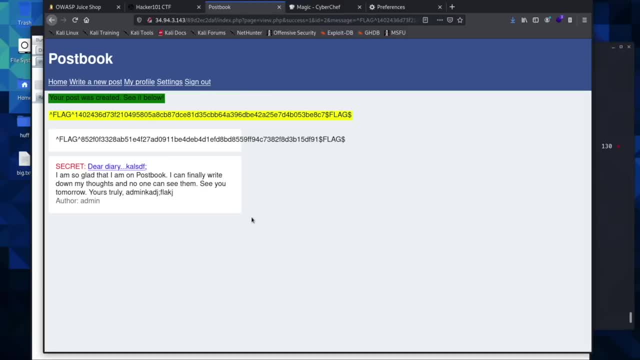 see if you can figure out the rest of the challenge on your own, kind of like we have been doing. but from this point on it's going to be a lot more difficult for me to show you very specific vulnerabilities on multiple websites, because at this point juice shop is going to be our main place. 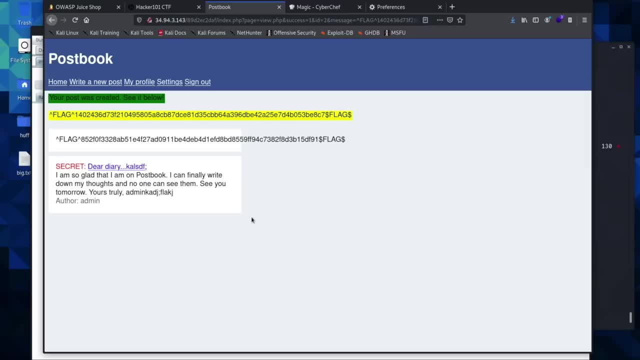 of working, because there's not a whole lot of options when it comes to practicing specific to you. so i want to give you clues of where they might be located in the application and then set you free to try and exploit them and then, only when necessary, help you. another clue: 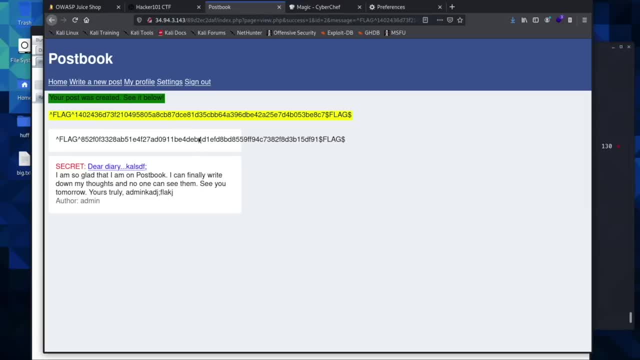 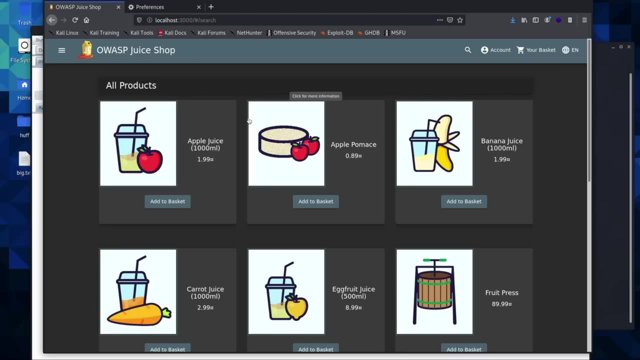 and so with that, you can actually continue playing around in post book and see just what else you can do in finding eye doors. okay, we are ready to find our first eye door on our vulnerable web application. so you can come in here and try and find it on your own, or i can give you a. 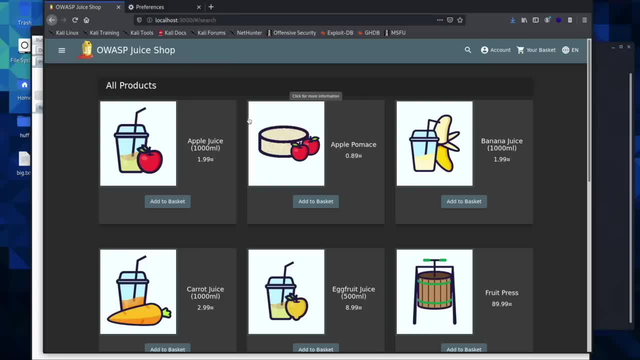 tip on how to get started. if you want to try it completely on your own, you can go ahead and pause the video now. browse the application. intercept your traffic with burp and see if you can find the eye door. your first tip is going to be: we'll find the eye door in leaving. 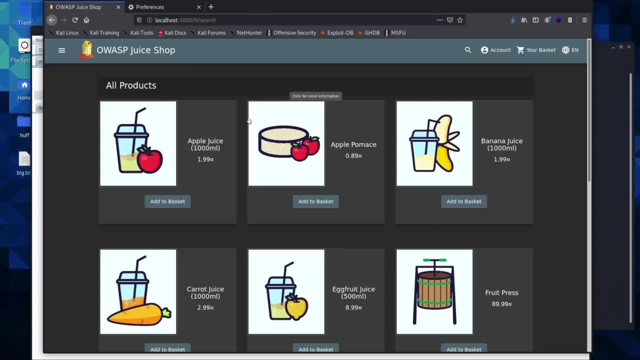 customer feedback under someone else's user, so you can go ahead and try and find that now if you want, or keep playing the video for the next tip. okay, the next tip is going to be creating an account. you will. i already created one. i figured you didn't want to. 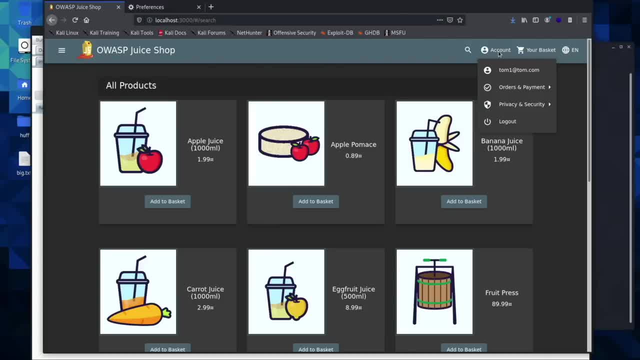 sit through me. create an account so you can actually just come up here. click on the account setting the account tab, go to login, create a login and, once you're logged in, try and find how you can leave feedback as someone else. we are going to go ahead and solve this challenge if, at any time, you 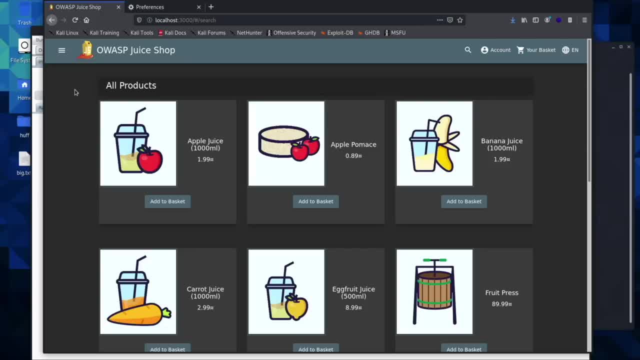 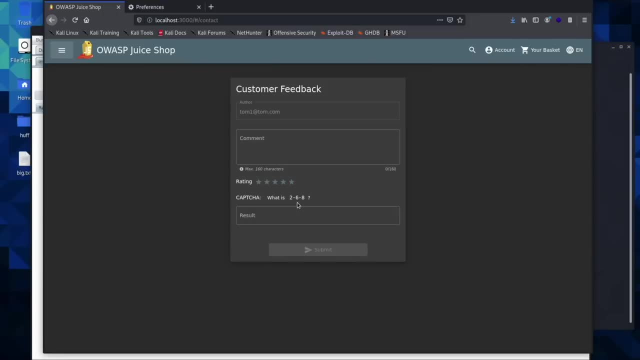 feel like we have gone far enough and you have enough clues, you can pause the video and try and solve it on your own from that point forward. but we're going to come over here to this menu. we are going to click customer feedback. now i want to give you another helpful tip. if math is, 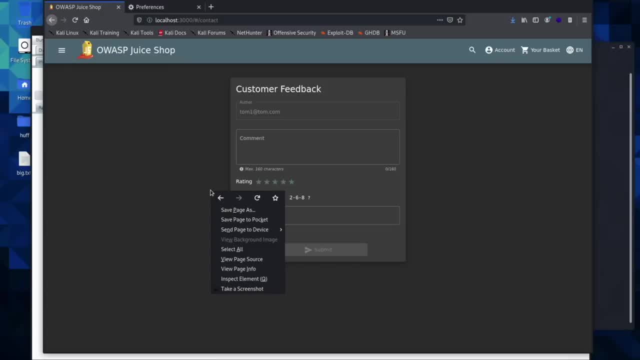 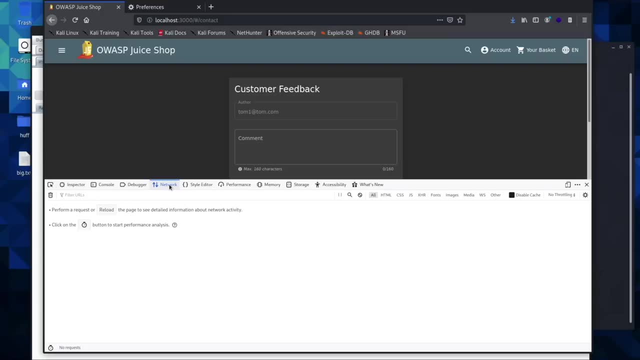 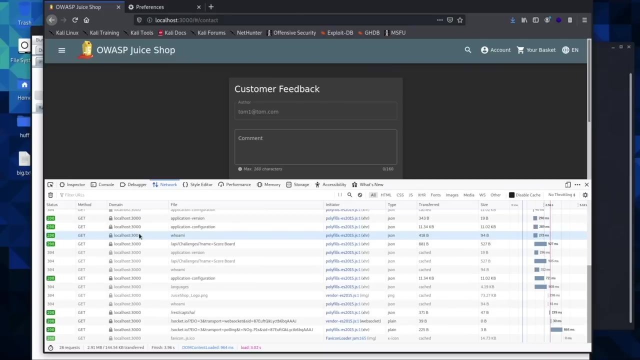 not your strong suit. you can add your own feedback in your опять regular, yelled out well to the videos. for this video there are actually open up and inspect the element. you can come to network and then you can refresh this and in our network we will get a whole bunch of get requests and we will look. 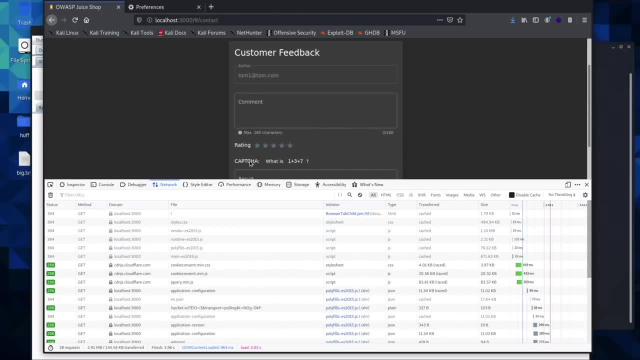 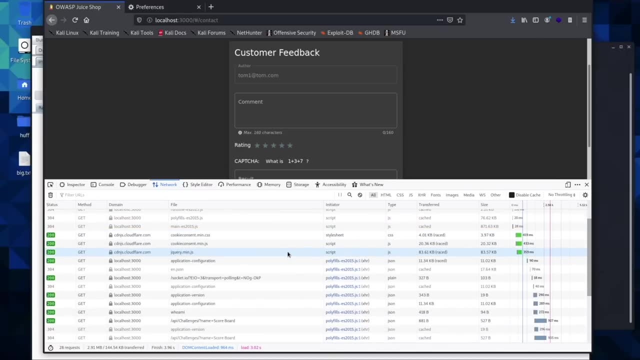 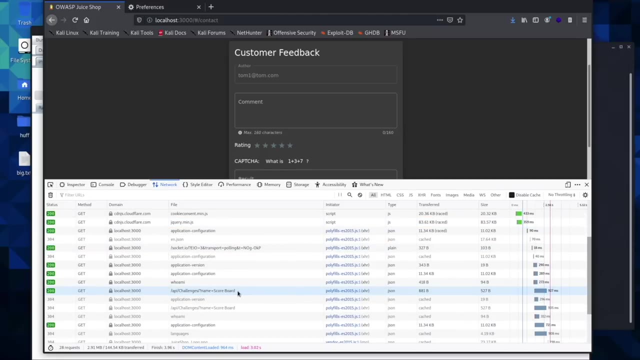 through and find the one. since this is called captcha, we're going to find the one that is labeled with captcha and in there it will have for us the answer. and you see this request. we are going to look at the scoreboard at the end of this video and i'll kind of talk through what this is. 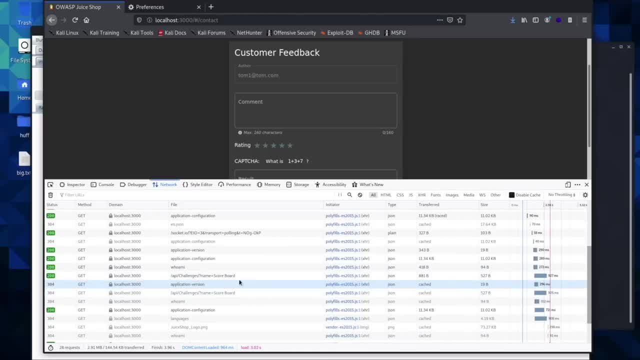 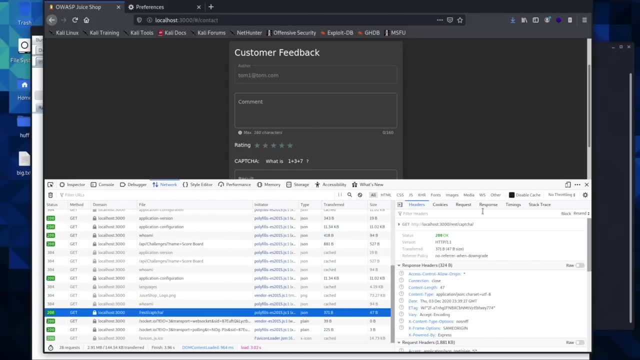 but we're going to go to this as soon as we solve this idor. but as we continue scrolling through and we're looking for the capture, right here you can go to the response. our answer is going to be 11.. so it will solve for you whatever math problem you have, and that's the easiest way to get through. 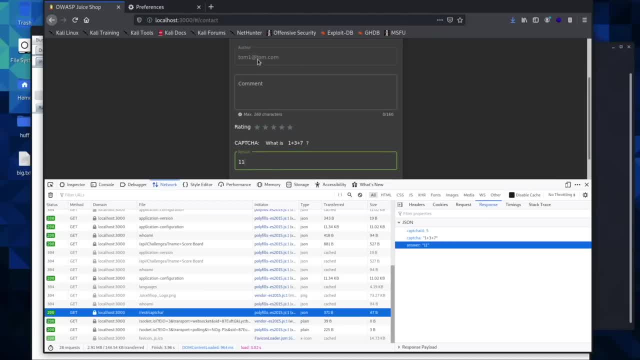 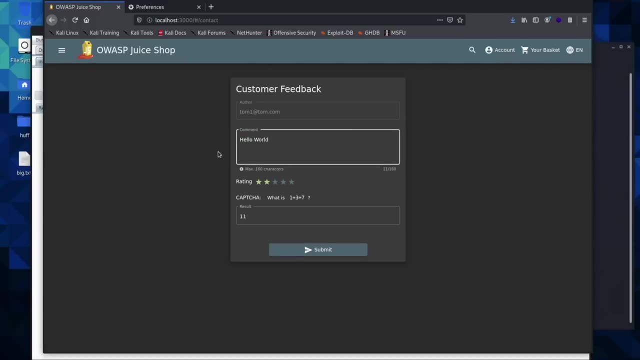 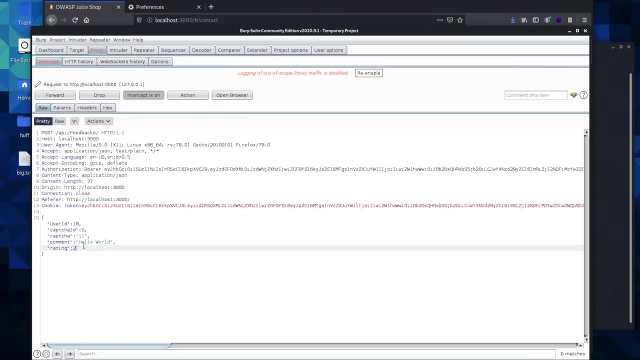 these, and so our answer is going to be 11.. it has our user name. we can leave a comment. i like to just leave hello world. we will give it a rating and then make sure to intercept when you submit this. so we'll hit submit and now we have our user id. if you want, you can go ahead and pause the video. 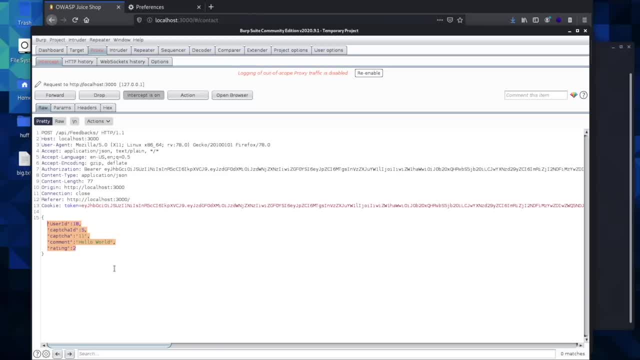 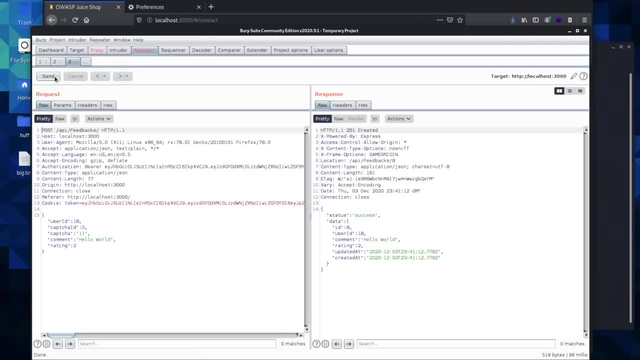 and see if you can figure out what to do from here. what we will do is we're going to send this to the repeater. we can come up here, open it up. we can send this request to make sure it goes through. it says it was created so we have successfully left feedback. but we want to leave feedback as someone. 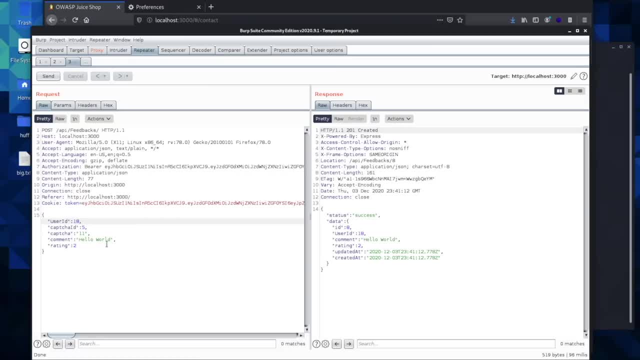 else, and so what we do is we want to leave feedback as someone else, and so what we do is we can change our id to: let's just go 14.. just pick an arbitrary number that's less than the one we were using or the one we were assigned, and then we can send it and it says it was. 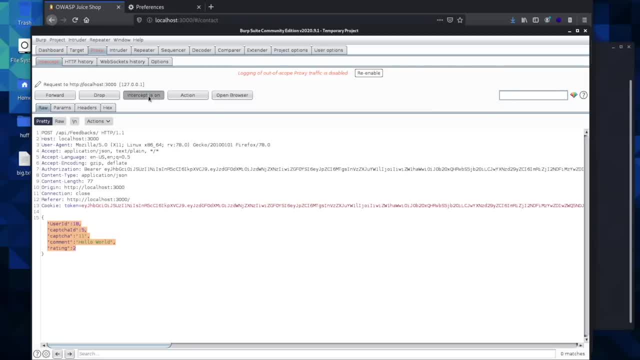 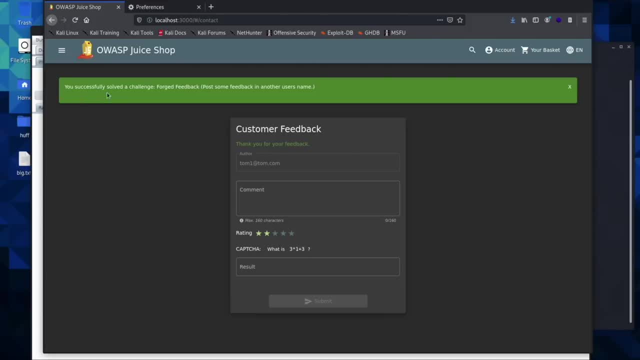 created. so now we should be able to turn off our proxy intercept. come back to our web application and it tells us we successfully solved the challenge of forging feedback. so this is an example of an eye door where we are leaving feedback under some other user's name. and now i want to go to the scoreboard real quick. this is where you can see the challenges. 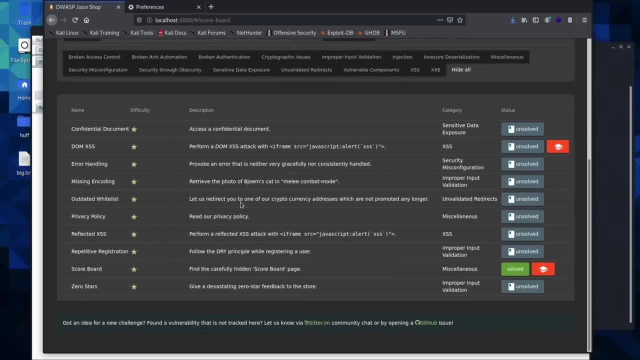 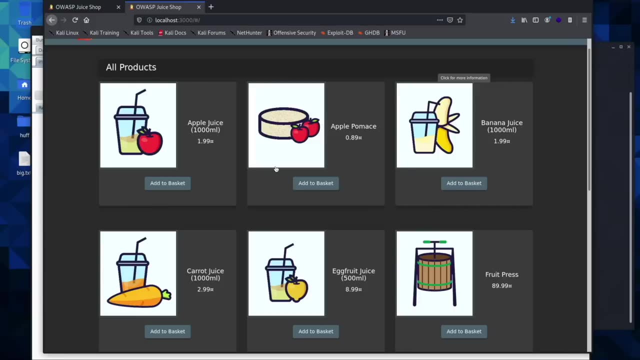 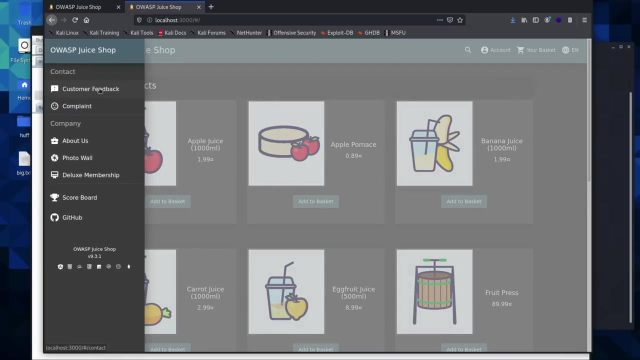 and you can see all of the challenges that are available on this web application. all right, i was playing around with the comment section in the products and i realized you can actually leave feedback as someone else other than coming over here to our customer feedback. you can actually lead feedback. 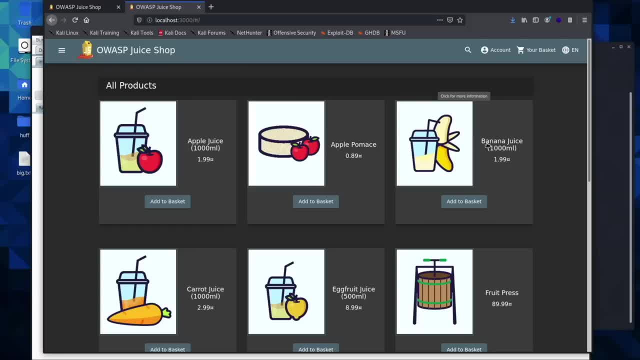 from a different user right here on these products, and maybe you actually figured that out in the last one, and if you did, that's awesome, and if not, you can go ahead and try and solve this challenge on your own and then we will go through it together. so if you want to give that, 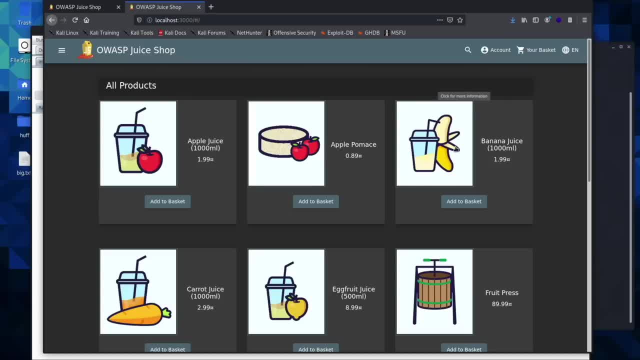 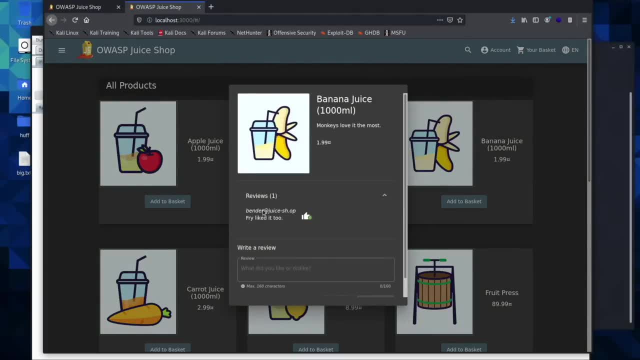 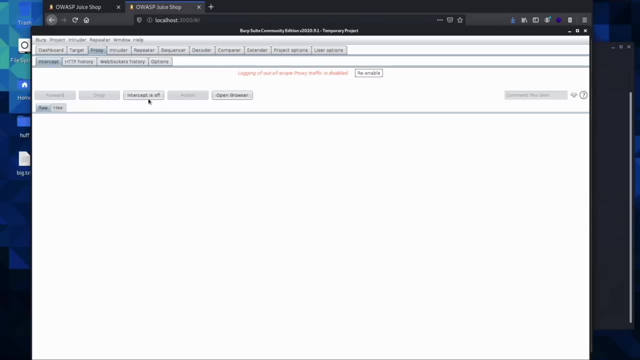 a shot. you can go ahead and do that now. okay, we are going to just open up one of the items that already has a review, so that we have a name that we can leave feedback under, and what we'll do is come over and turn on our intercept and type in 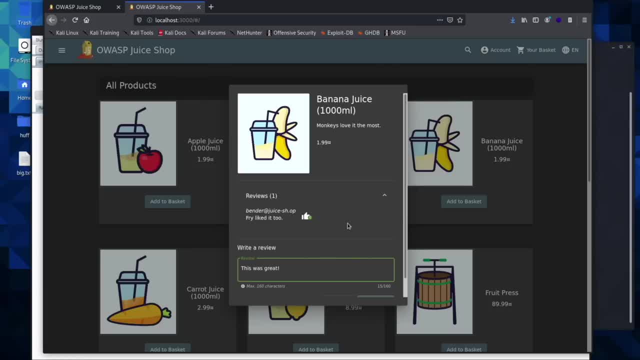 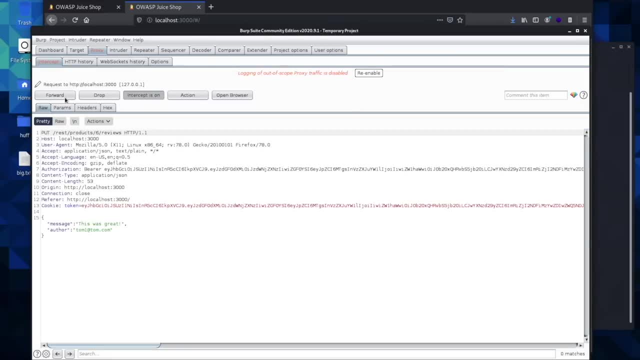 something in search bar for you, and then We'll be making a new�를 as Kat thief. okay, so in search bar it comes up with news and in search bar we'll the creation status, which is making it pieces made. but we want to make an issue of union in leaderboard. 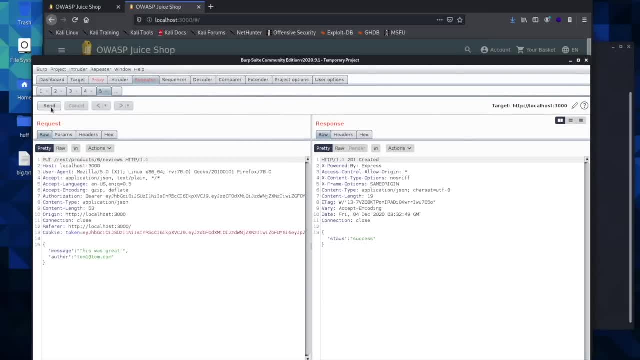 in theuls that we use in search. when we make that decision here, we'll go over to our inventory section and we'll go to give in feedback in our nosso żyko. there we go. that was awesome. Thank you so much for your time to this. through this. we'll go ahead and start with notes. 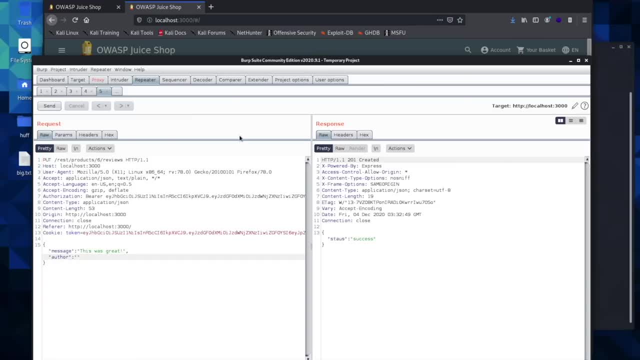 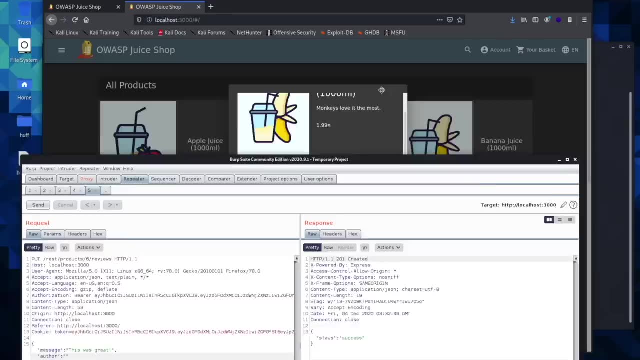 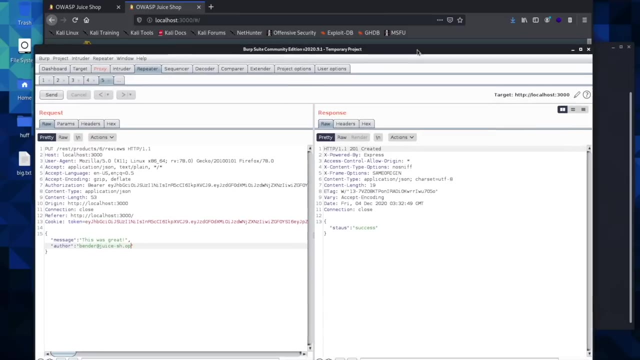 In search By. Хотя. we'll do it. every single link content, link content. then we'll send. of having our name in here, we can put in a bender at juice shop, was it dash? i think that is how it was written, and then we should be able to send this and we'll actually just put in something. 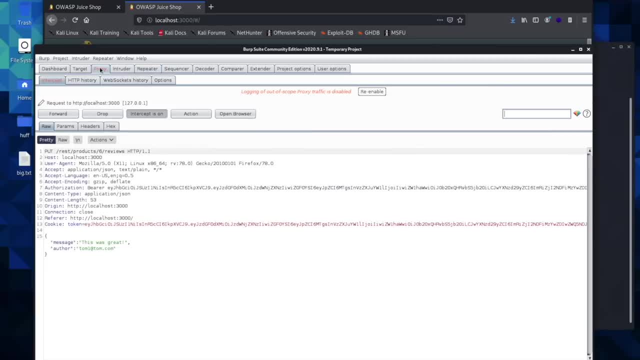 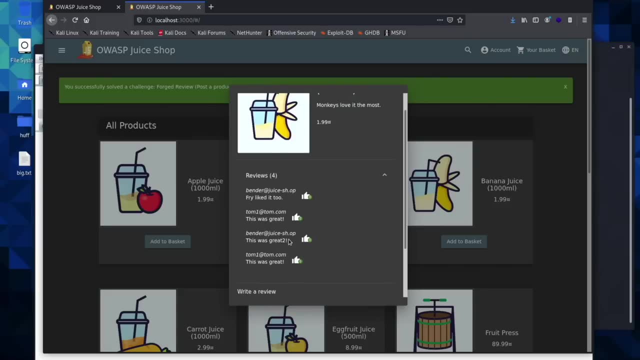 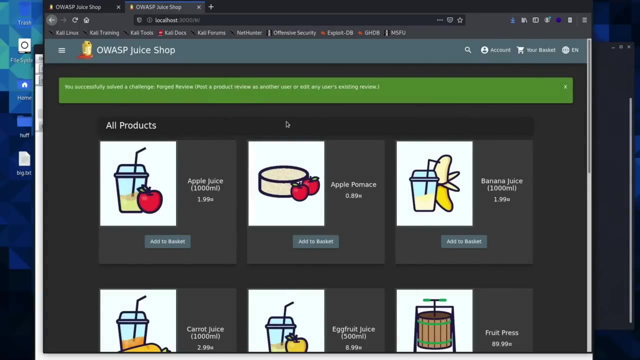 else here and send it and it says: it was created. we'll turn the intercept off and you can see here it was. it was created under someone else's name and it actually says we have successfully completed the challenge again. okay, our next challenge is going to be one that we 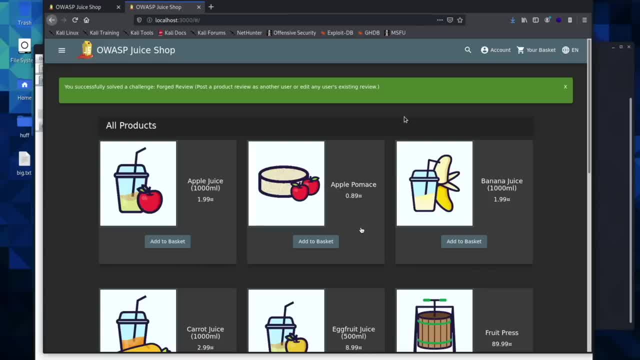 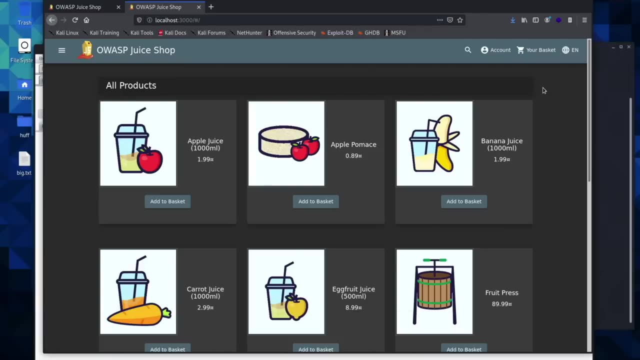 have talked about, but we have not actually seen and i have not come across any vulnerable web apps to actually test this on and show it to you. but we have talked about it and you might have to use some of your googling skills or just, if you get stuck, follow along with the video and get a hint before you move on. but 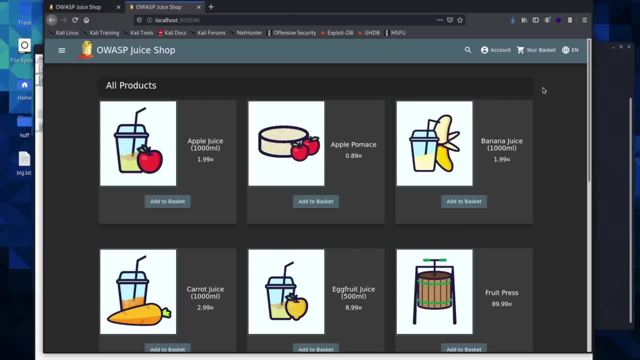 we are going to create an admin account and this is something that is very possible that you will come across. it's not very common, but it does happen that you can find ways to create and admin account or escalate your privileges, so we're going to go ahead and make sure our intercept is. 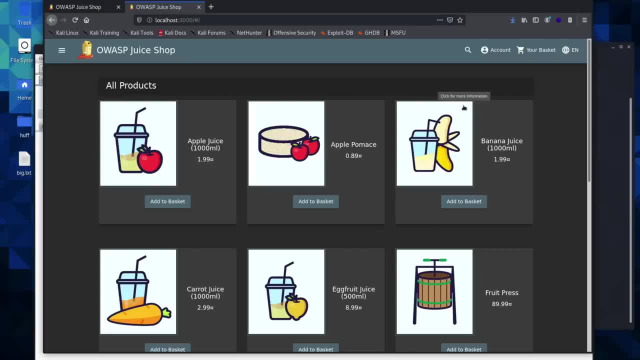 off, and what i need you to do is go ahead and create an account and see if you can figure out how to get the account enrolled as an admin, and so you can go ahead and try that. now, i think what i will have to do is log out, and i'm going to make a new account just the same. 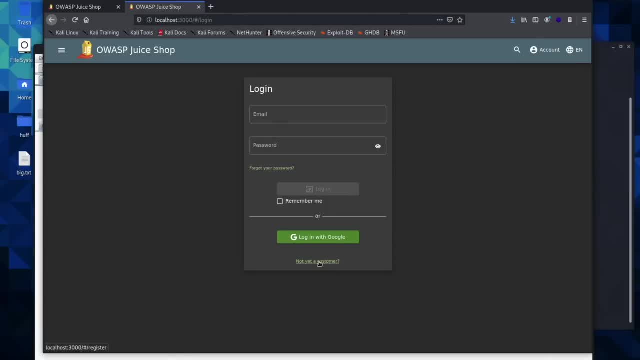 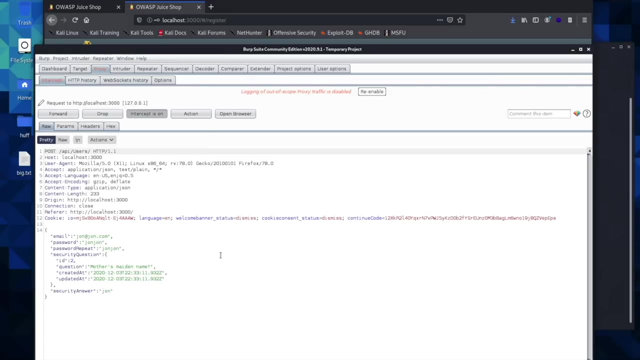 and i will come in here and go not yet a customer. this time we'll go john at johncom and as soon as you get this done, we will turn on our intercept and we will register the account. now what we're going to do here is we're going to send this to. 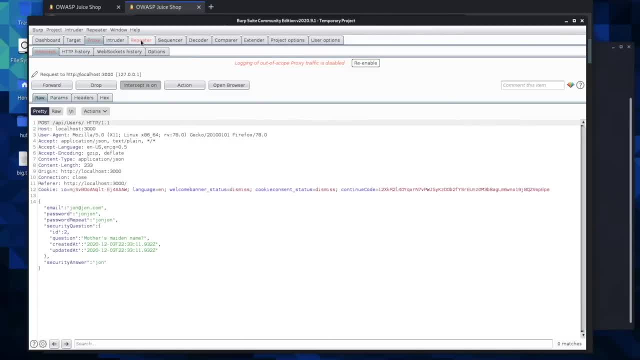 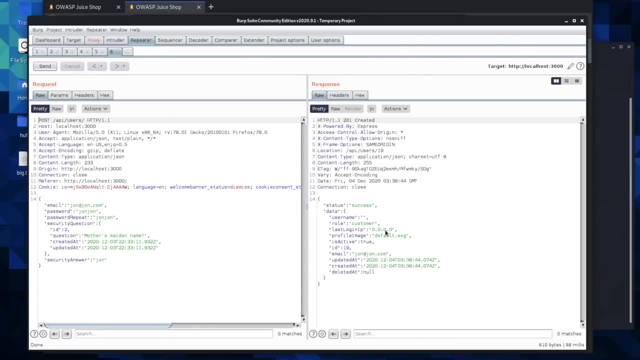 repeater, and over here is where we'll work on escalating the privileges to an admin, so we'll send this and just to get a response to see what we have here. so our role is a customer, and this tells us that we're going to need to change the role, and so i actually just did this. 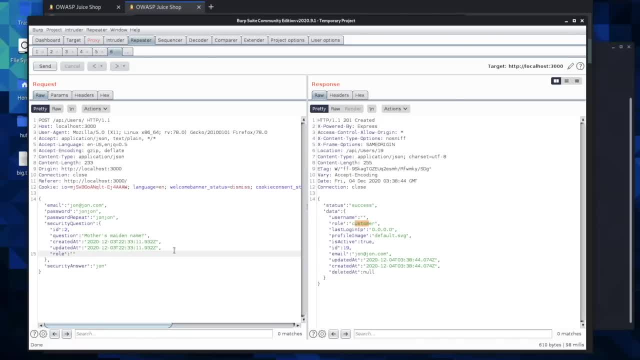 a few hours ago, i was just working through the application and i'm going to show you exactly what happened to me, because this will give you a really good idea of just the trial and error that we go through when we're testing applications. so i came in here. 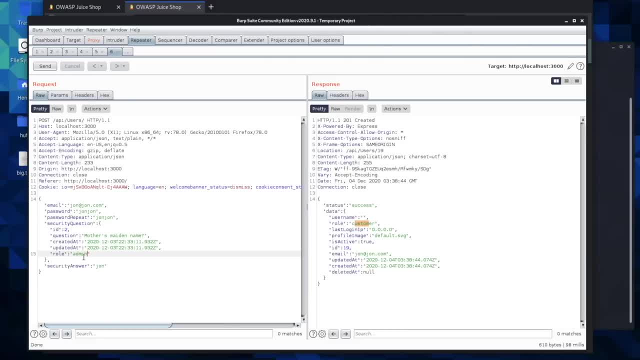 i typed in role, just like this, and i typed in admin, and if you send it, since this user has already been created over here, we're actually going to have to change this to one. and if we send it, we can see we've now created another user, but the role is still customer and so i changed this to. 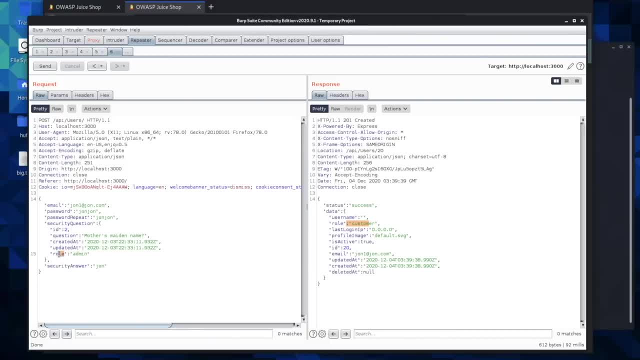 administrator and it still didn't work. so i tried to change this to user admin and then change this over here again. and we are still a customer and i've tried user, i tried admin, i tried administrator and finally what happened was i deleted this and i came up here. 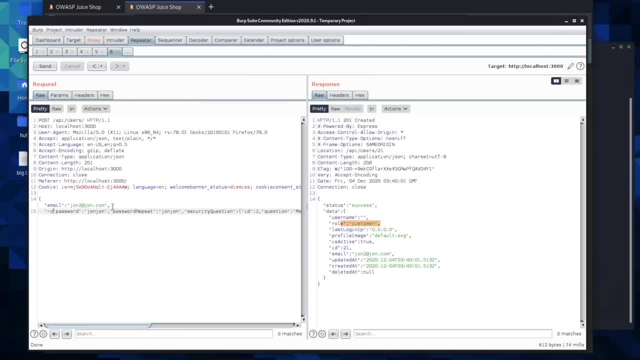 and i tried to just move our input to see if that would make a difference, and i typed in admin just the same as before, and that looks good, and we'll change this to a three and then we will send it. and now you can see, our role is now admin. so we have created a, an admin user. so if you take this user, 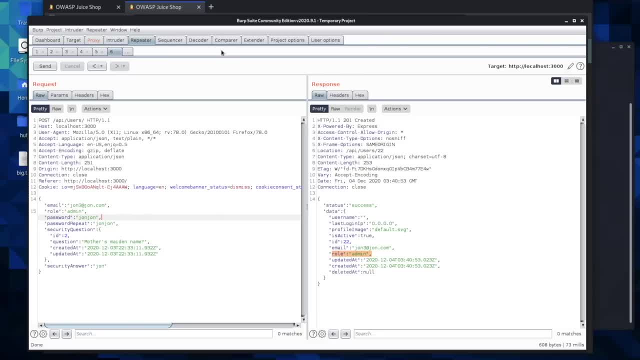 with this password that you just made, you can log in and browse the juice shop application as an admin, and so you'll actually see things like this in the wild. they're uncommon. you can actually go on hacker one and read the hacktivity and see where people 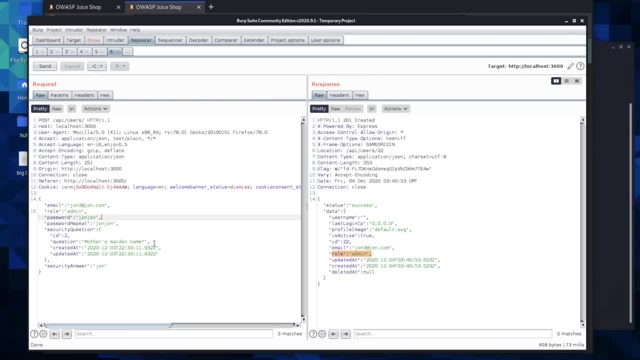 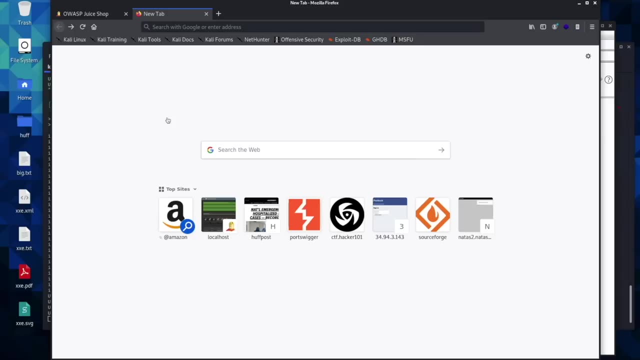 have actually got this to work and you can see. just read the articles and read the submissions to observe how people have pulled this off. some of them are going to be more complicated this than this, but some of them really will be this simple. okay, what i need you guys to do for this? next, 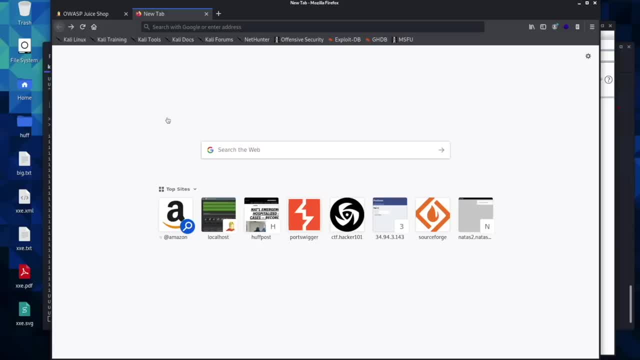 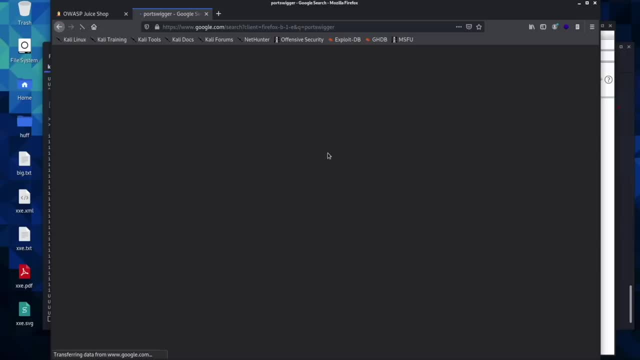 lesson is: go ahead and open this up here in your browser and go ahead and open this up in your open up a new tab And up here we're going to go to port port swigger and you can go ahead and search, for it should be the first one And we're going to open it up And we're going to. 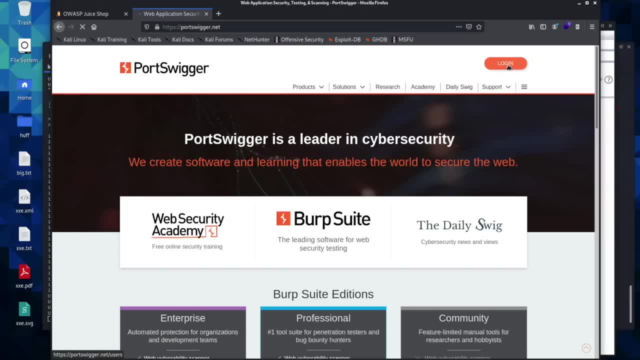 move over to the login button. I've already created an account, And so go ahead. click on login, create an account. we're going to need it, especially in the coming lesson, So go ahead, click the login button, make an account, And I'll see you once you're logged in. Okay, 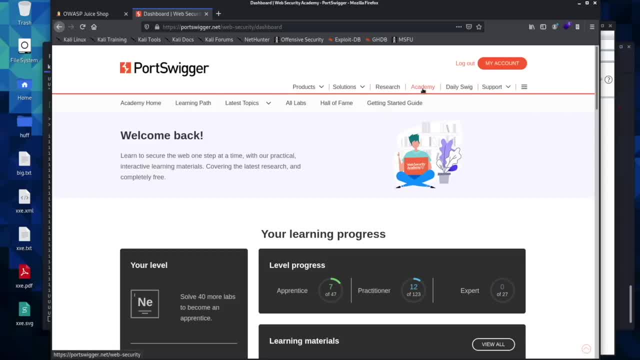 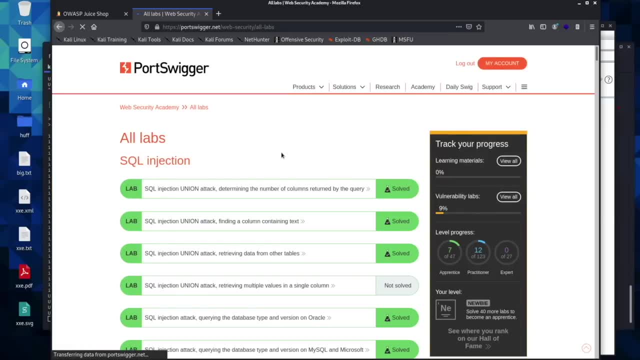 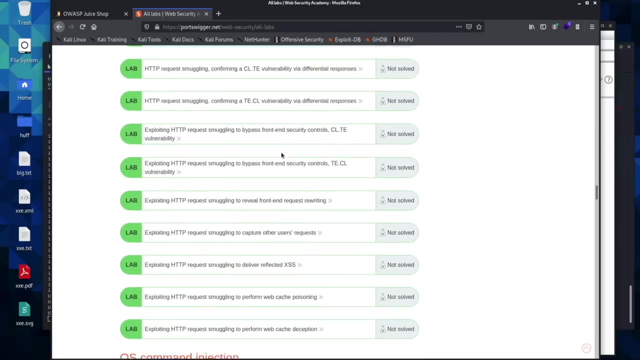 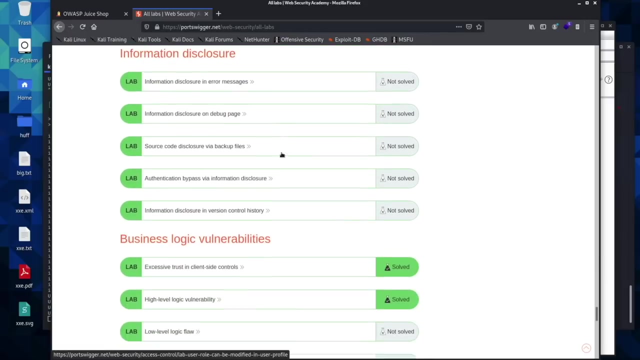 once you have reached your login page, go ahead and click on Academy And then go to all labs And once this loads, we're going to go ahead and scroll down until you find business logic- And I business logic, errors, vulnerabilities right here, And we're going to be working through these. 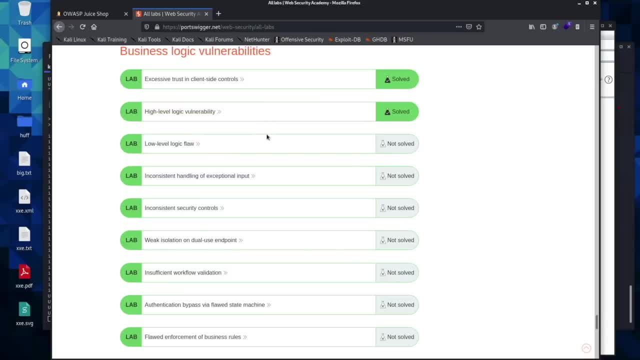 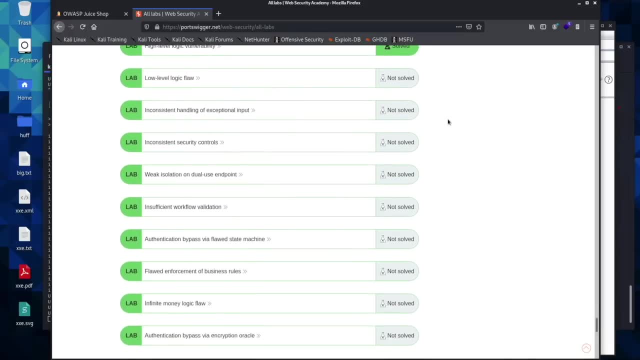 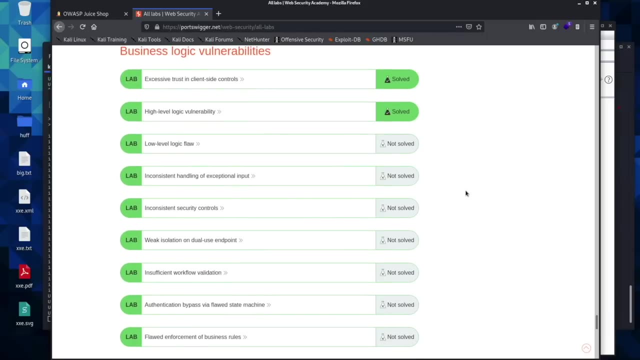 right here And so let's continue going forward. So these actually say solve, because I already made the videos for these and I realized that I never actually explained how you guys should get here and get to these labs before I started filming these videos. So I'm going to edit the. 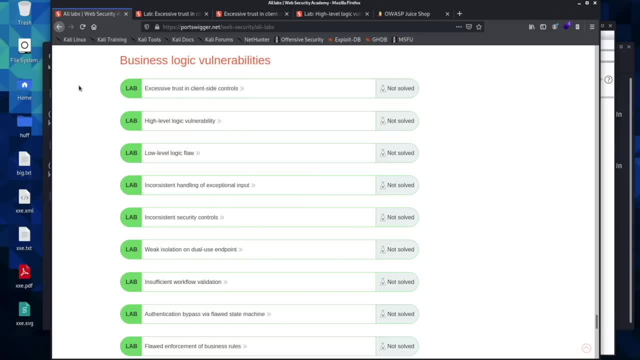 video, and these are going to turn into unsolved. Okay, we are going to look at a few business logic vulnerabilities, And so these are very similar to the IDORs that we have been looking at, And so we're going to go ahead and start here with this one. 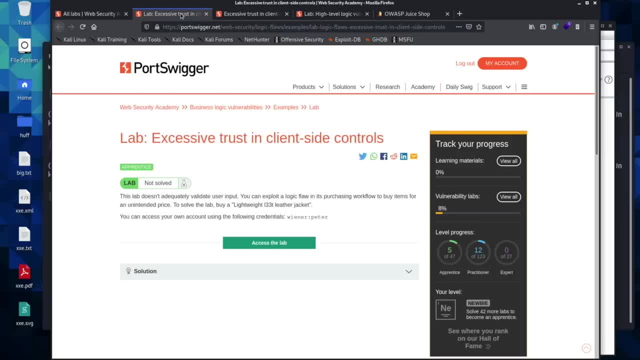 right at the top, So you can go ahead and click on it And we can look and see what exactly they have for us. And it says that it doesn't validate user input And we're to buy this lightweight jacket. you can go ahead and 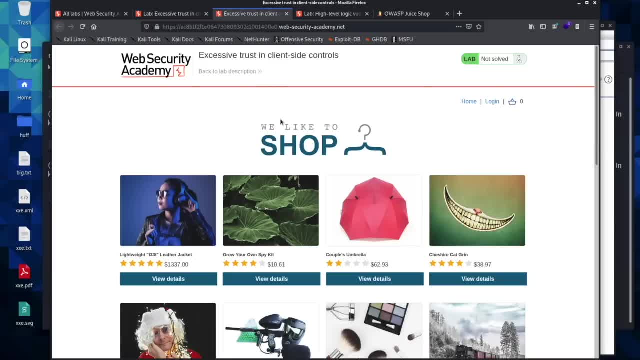 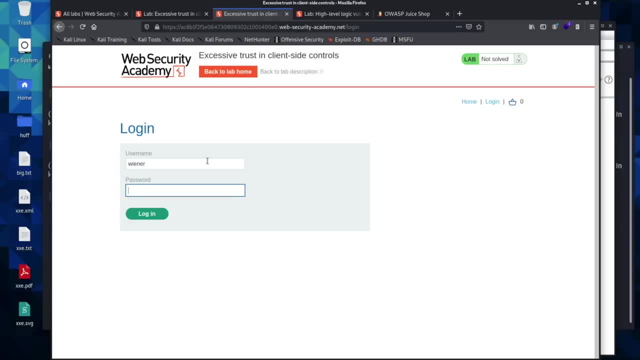 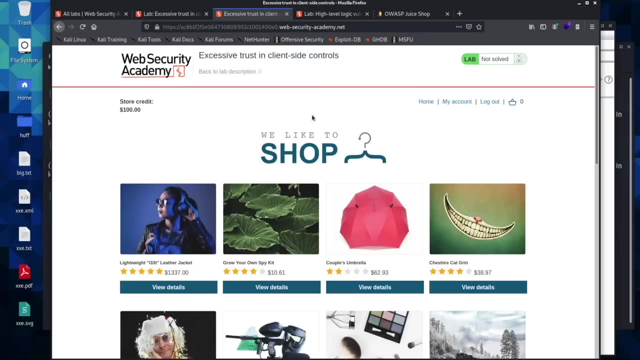 open up the lab, And this is where it brings us. It said we needed to log in, So we will go ahead and do that, And it gave us the login credentials. So log in. And now we're supposed to buy this jacket, So I guess we can go. 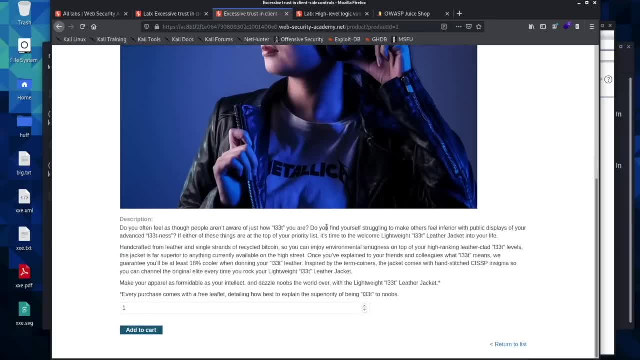 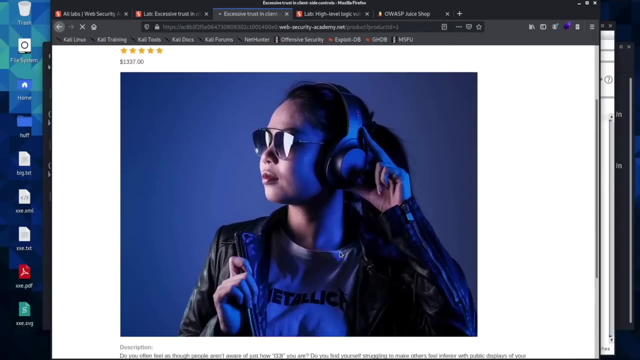 ahead and view the details and add it to the cart. Let's actually come in here, turn the intercept on. We'll add it to the cart And it tells us our price right here. I don't know exactly how much we're allowed to spend, But I think we. 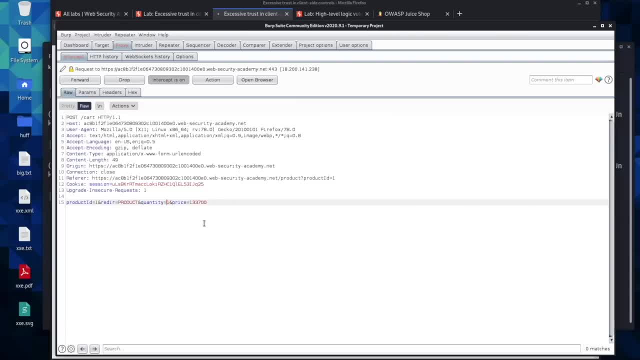 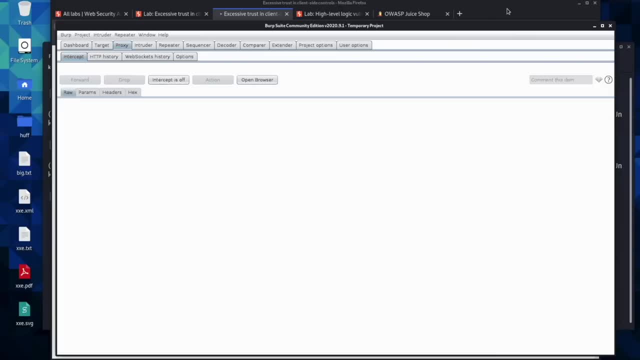 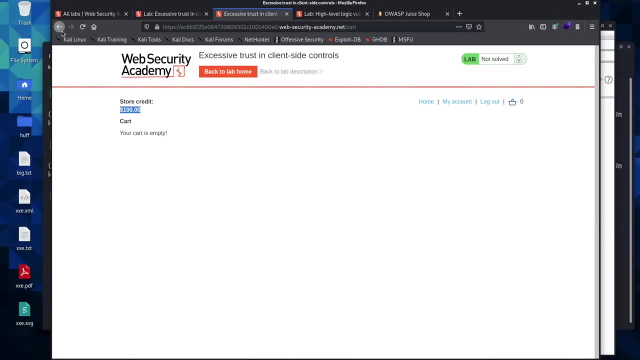 should be able to. Let's see if we can make this a negative number And we'll go ahead and forward that And then we'll just turn that off And it did not add it to our cart. We have $100. to spend on this jacket and this jacket is way over $100- $1,300. so we'll go. 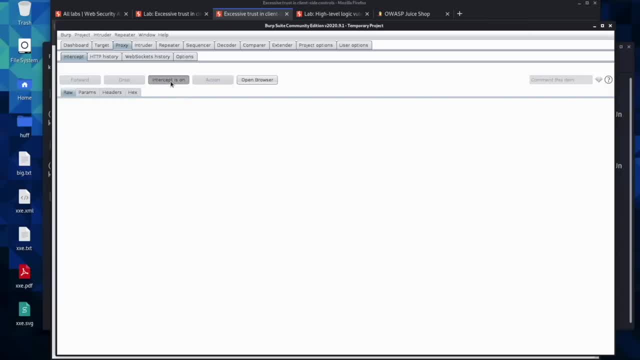 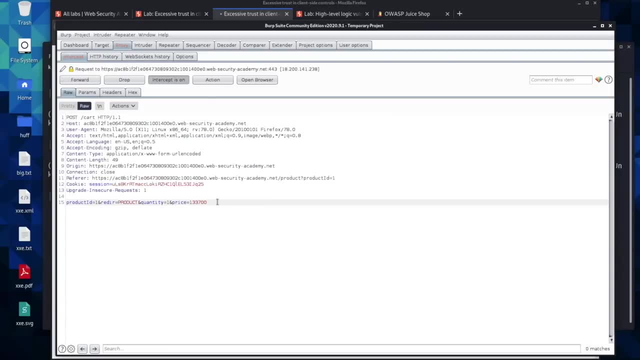 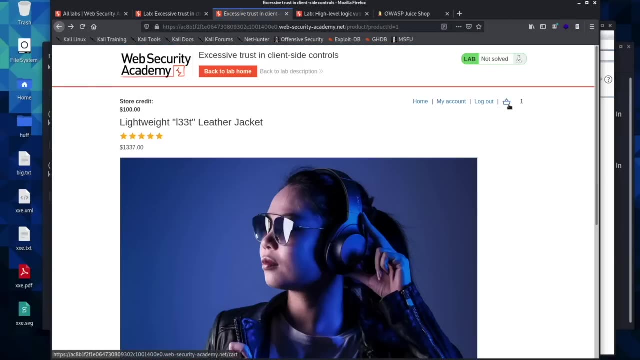 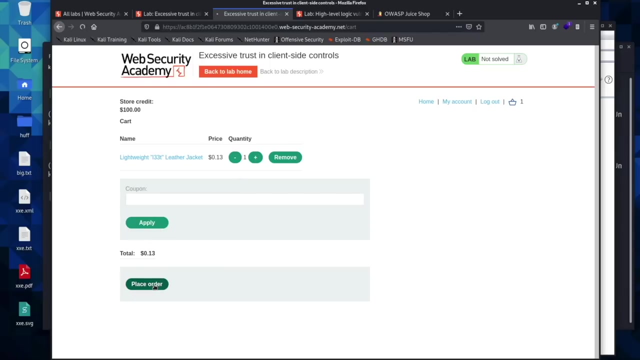 ahead and see if we can turn the intercept on. add this to cart and let's just change our price here and see if that works. okay, we were allowed to add it to our cart, so we have no need to apply a coupon, and we should be able to. 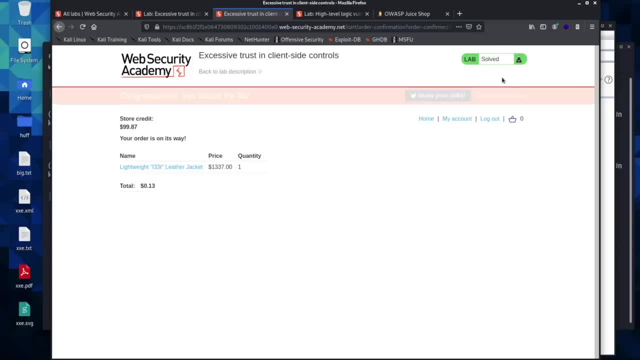 place our order and it says we have solved the challenge. so things like this and business logic errors- I doors and business logic errors- they're going. they're going to be things that you have the opportunity to find. these are pretty common that you'll find these business logic vulnerabilities. they happen when 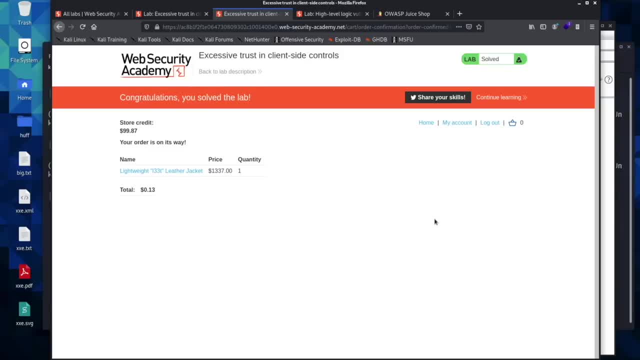 developers get lazy or they're just not really paying attention to what they're doing. I've actually seen really advanced developers make very simple mistakes that made their web applications vulnerable just because they weren't paying attention, and so you can find these. they're pretty common. I know there is at least one bug: bounty. 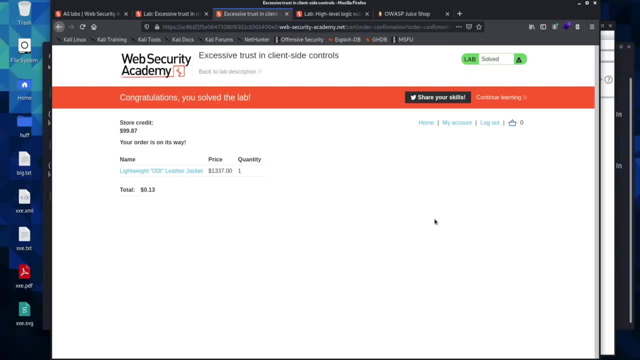 hunter that this is all they do. they look through burp or they look for business logic, errors and what they can change, just to find stuff that they shouldn't have, and that's what we're going to talk about in this video. so we're going to talk about some of the things that you shouldn't be able to, and 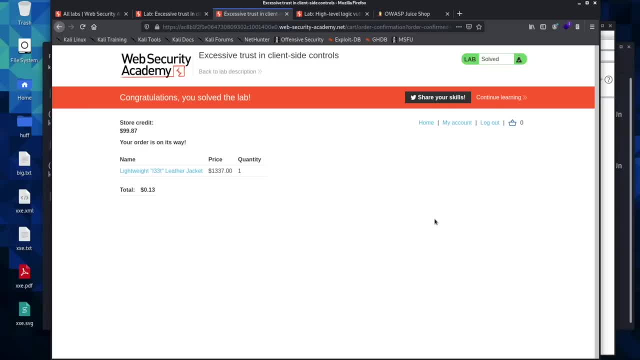 vulnerabilities. these are pretty simple and they do take a long time to find, but you can find them just by doing really simple things, by just changing numbers and inputs. sometimes you will find stuff that has been encoded. it'll say like you'd have the lightweight jacket, let's actually go back. I'll just show you. 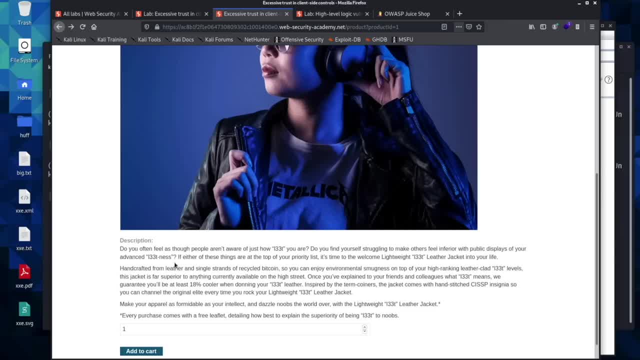 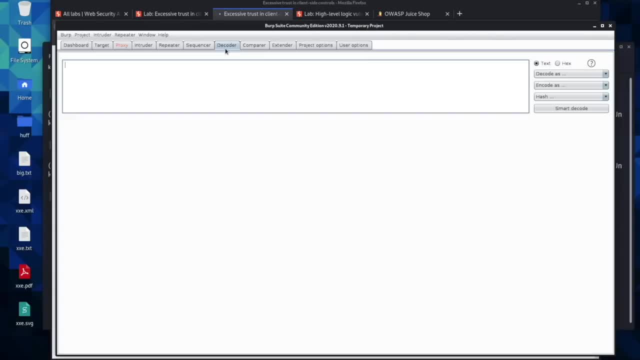 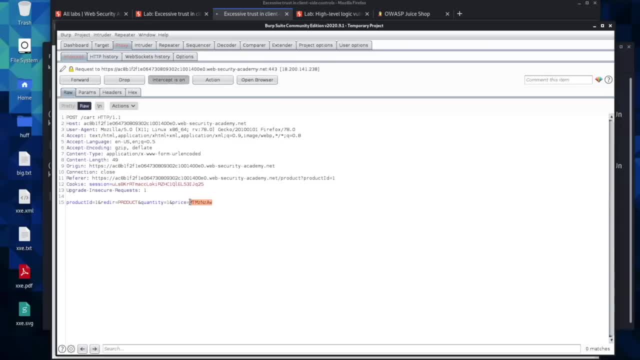 you see something like this. you'd have to take this and you would come to your decoder. or you can go to cyber chef and you can put it in and try and decode. the price rarely gonna see it where. it's just a plain number, but this is way more. 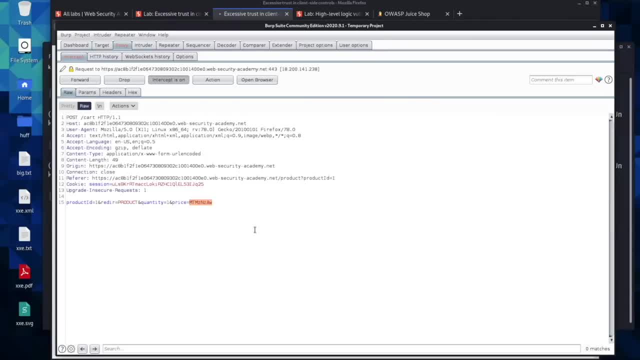 common that you can put in and try and decode the price. rarely gonna see it where it's just a plain number. but this is way more common that you would just see a number here and that you would have to decode it. sometimes these prices will be stored in places other than just something plain. 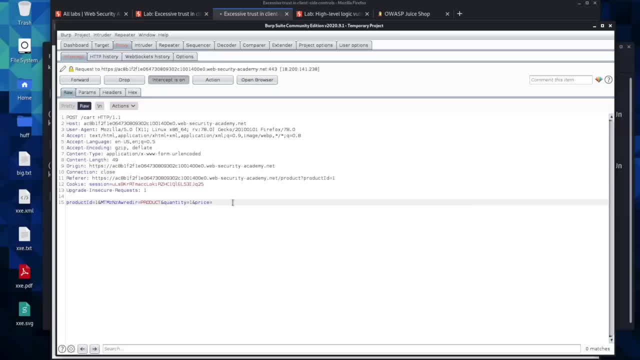 and simple like this, and so it's something that you're gonna have to look for and poke around. they do take a while to find, but you can find them right off as a beginner who knows very little. and we're gonna look at one more and then I 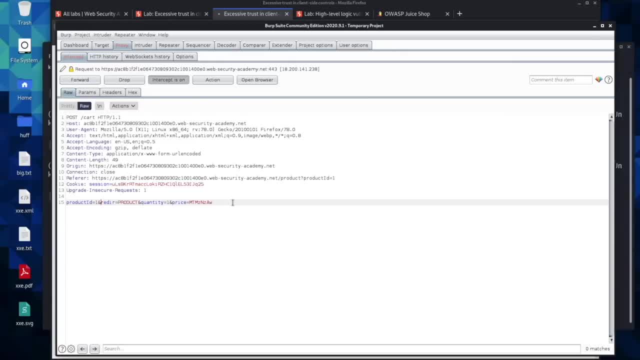 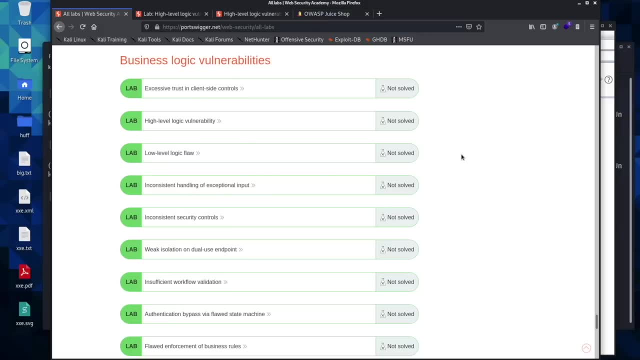 want to send you off on a challenge and see if you can find a business logic error on your own. okay, we are going to continue with the business logic vulnerabilities. we're gonna go ahead and open up this second one and after this one, I'm going to set you loose on a challenge. so what we'll do is we'll go. 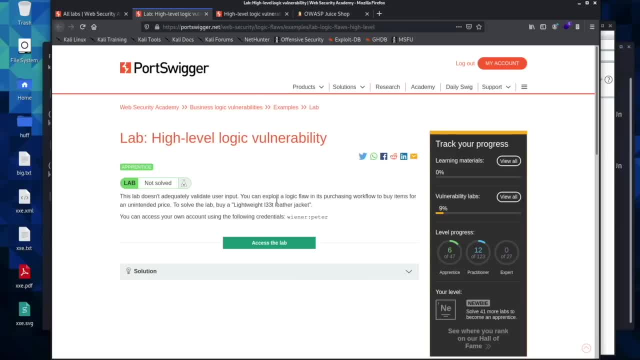 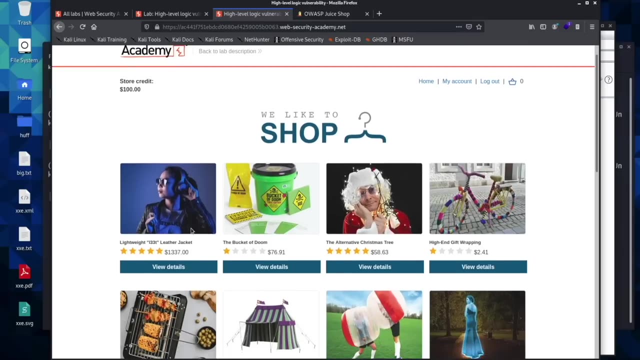 ahead and open this up. it looks like the same as the one before. we need to buy this jacket and we have our login user right here, so we'll go ahead and log in and we'll try and proceed with buying the jacket. Okay, here's our jacket, So we'll go ahead and view details. We'll 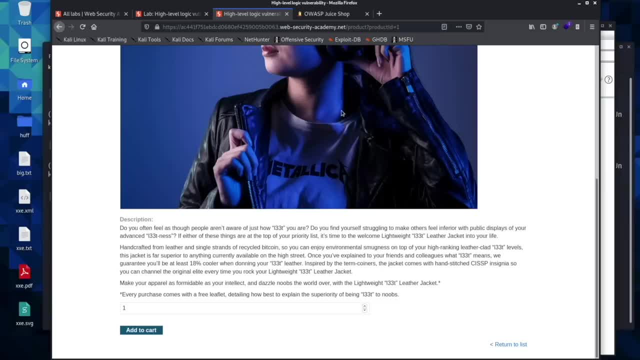 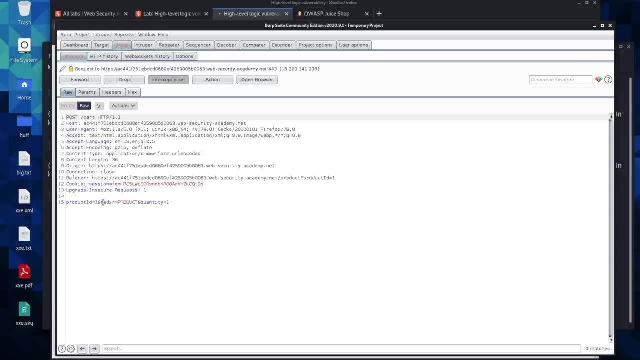 add it to the cart. We're going to do the exact same thing we did in the last one, And I'm going to do it the exact same way by starting out: Oh, we don't have a price, So we got our product ID. 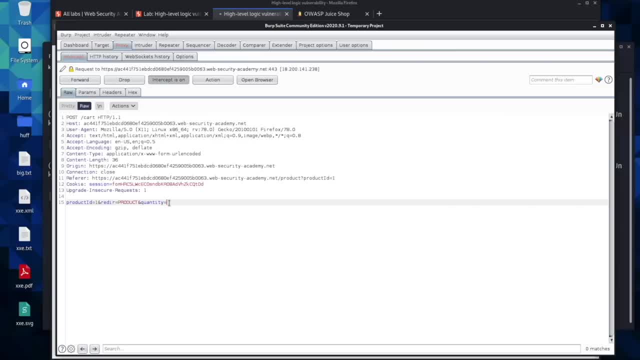 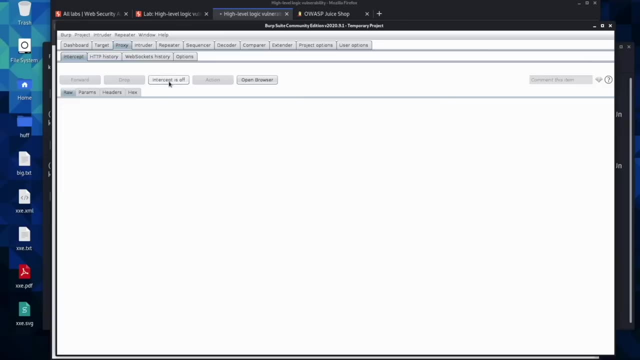 our product and here's our value. Let's get two of them And I'm assuming we have the same amount of money in our cart as we had the last time to spend. So we'll go ahead and just put the negative sign in front of the two And we'll see if it allows us to put in a negative number And we 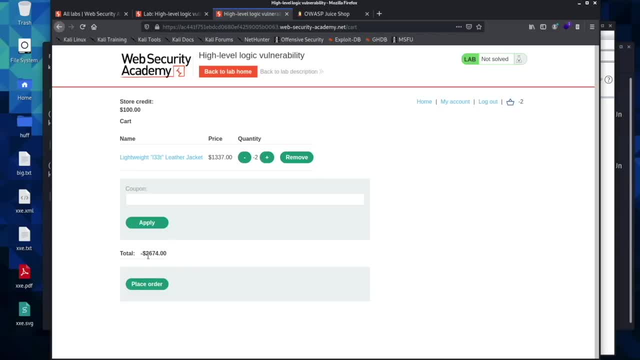 were So in our cart. if we go look at it, it says we have negative $2,600.. That means they are going to pay us. See if it'll go down by using these buttons. It does So you wouldn't even have had. 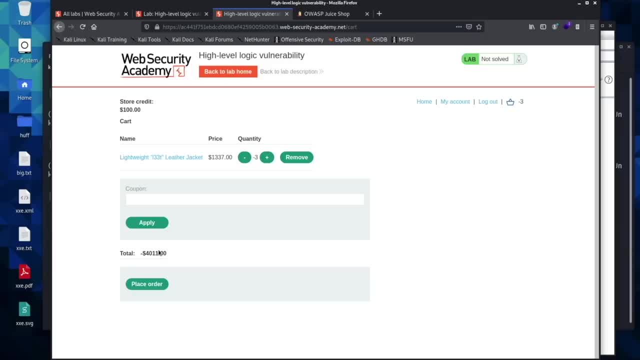 to have done this in Burp. You could have just come over here and click this button, And it means they're going to pay us this amount of money. So when we place our order, we're definitely going to be able to buy our jacket And our store credit is going to increase. Our price is not allowed to. 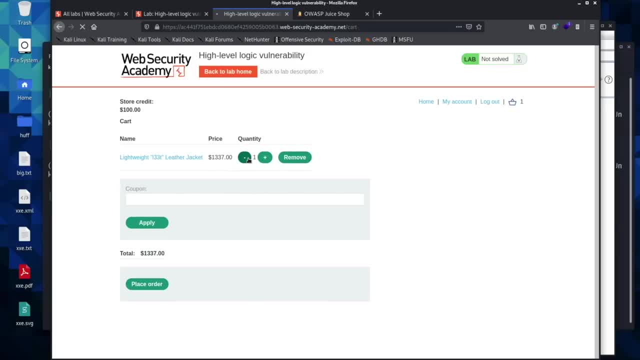 be less than zero. At least they have that in place. So we'll go ahead and okay, made our cart empty. We're going to have to go back and put that back in our cart. So what I think we'll do is: 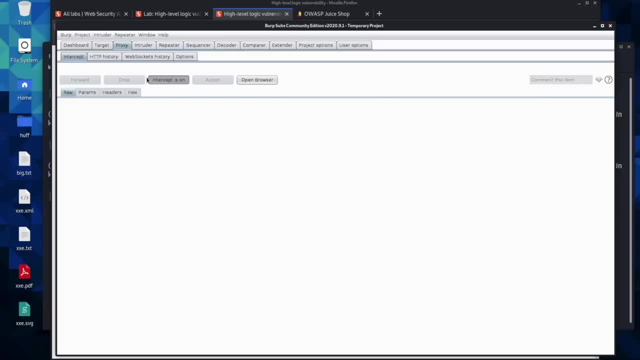 we'll add this to our cart as well, And we're going to go ahead and put that back in our cart. I'm not sure how many of these we're going to have to add. We'll go ahead and add one in So that way. 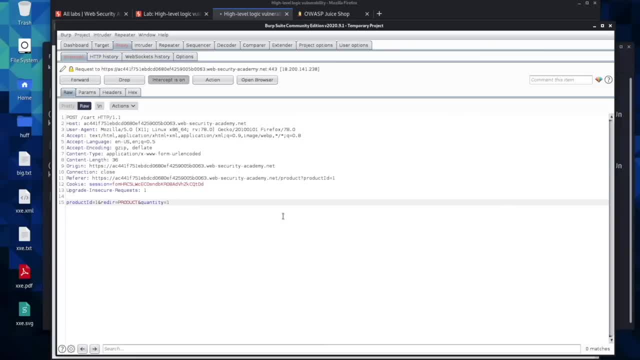 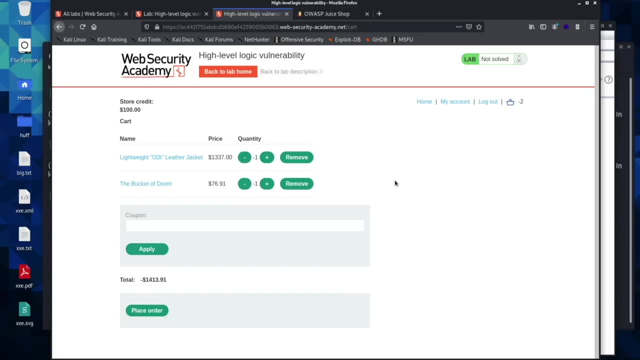 we can buy our jacket, because that is our challenge. We'll go ahead and make sure that's negative Forward, Turn that off And now we should have two negative items in our cart. It has to be above zero, but less than 100. So what we can do is we can just continue to subtract these. Oh, we'll add these. 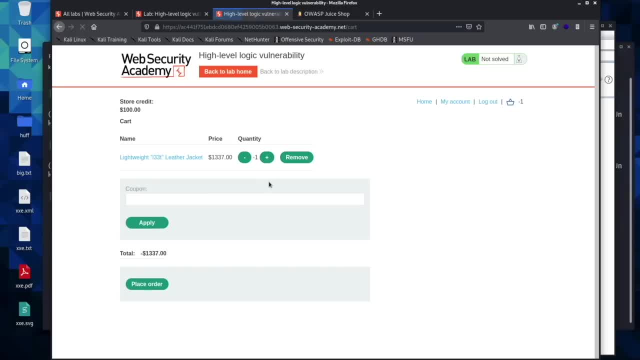 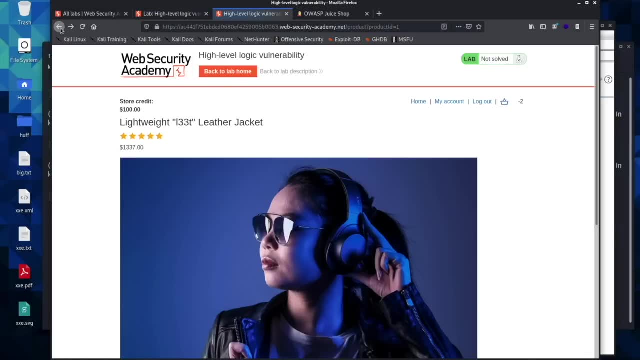 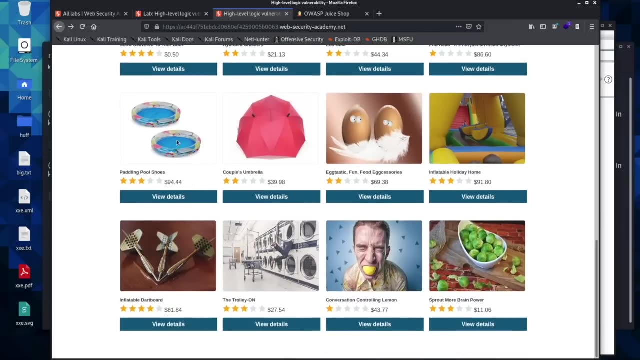 We'll go ahead and add these until we hit our price. Okay, It went back to zero and removed it from our cart, So we'll go back over here. Back over here, Let's find something a little more expensive, so we don't have to add that so many times. We'll go with the pool. Come to burp. 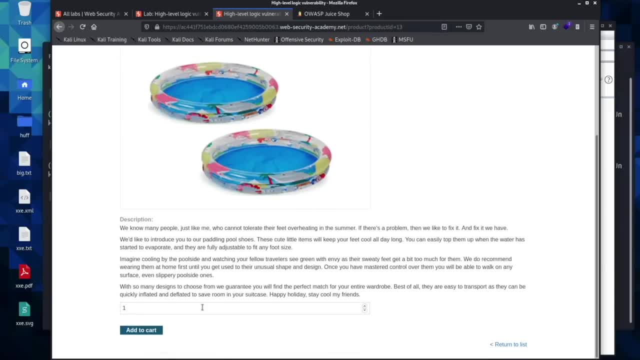 Turn our intercept on, And this is exactly how this would happen if you were testing it. It's going to be a lot of trial and error. We're going to need- I'm going to guess- at least 15 of these. We'll just go ahead and add them to the. 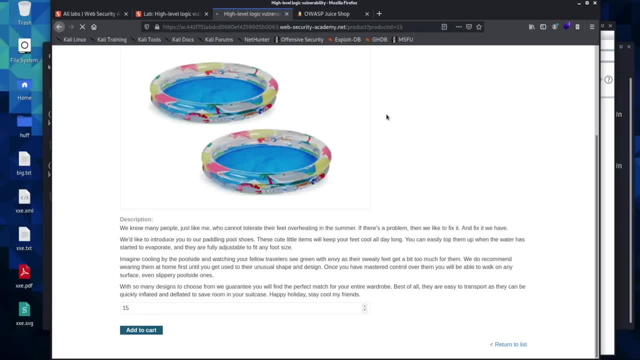 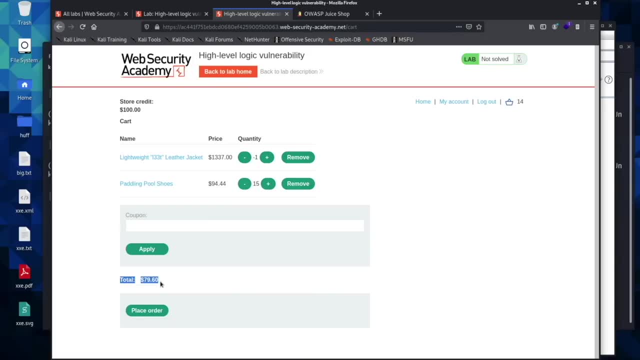 cart. We don't need to intercept that And go back to our cart And there our total is now $76.. So what we did is we just added 15 of these pools, which got us close to $1,500.. And then we or, yeah, $1,500. 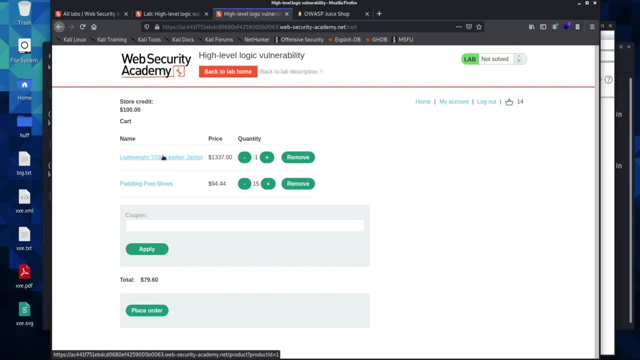 And then what we did is we went ahead and added our jacket in at a negative price, because it wouldn't let us purchase anything at a negative number, And we only have $100 to spend, And so this should solve the challenge this time. So we'll go. 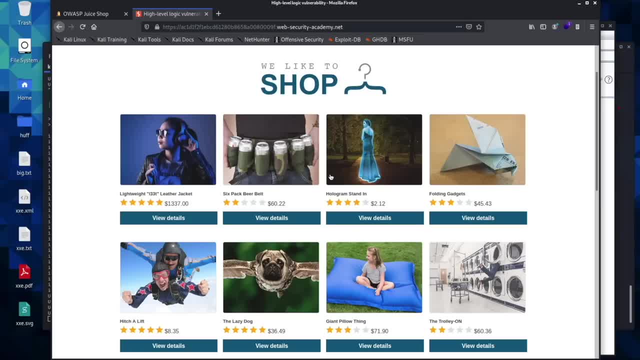 ahead and place our order. So I just wanted to add that you saw me make a lot of mistakes and a lot of trial and error in this video And I want to thank you for being patient, But I also decided not to edit out. 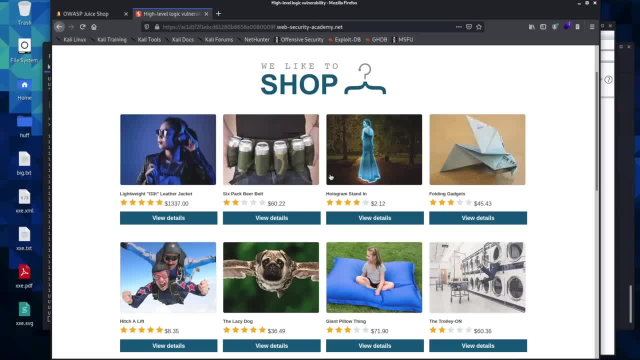 I wanted to help you with both the clicking that I had to do and the failures from this video, because I wanted you to see what it's realistically like as you test web applications. and as you're on the hunt, You will be doing what I just did the majority of your time: Just trying to see if things work And, as they fail, you just 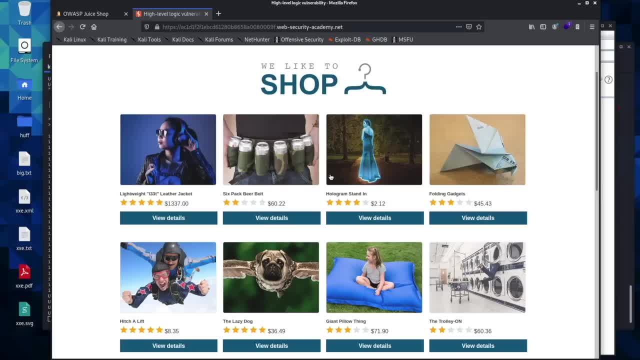 go on and you try something new And you try a different way to try and exploit the application or the vulnerability. And so I want to just encourage you that as you become frustrated or frustrated, you should try to exploit the application or the vulnerability. And so I want to just encourage you that as you become frustrated or 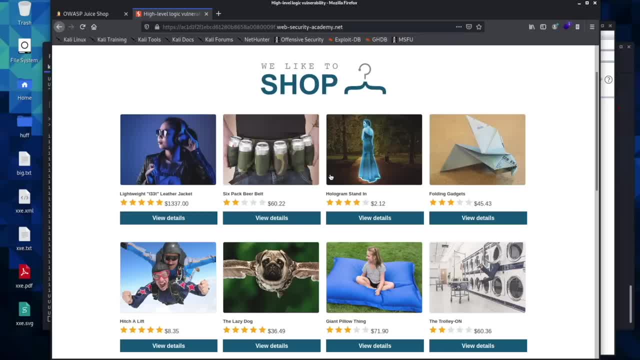 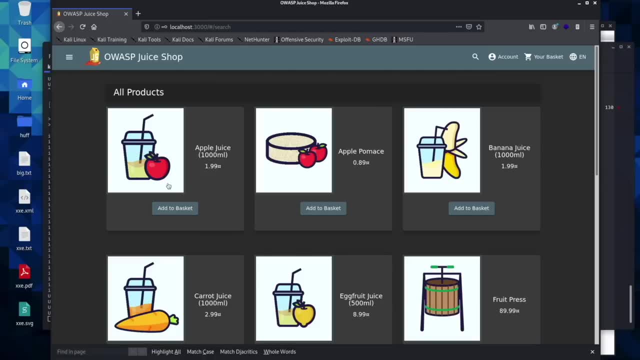 frustrated. you should try some weeks that there some things aren't working, to just keep pushing on and see if you can find the vulnerability. OK, it is time for your challenge. So if you navigate over to your shop and get running, what I want you to do is try and solve. 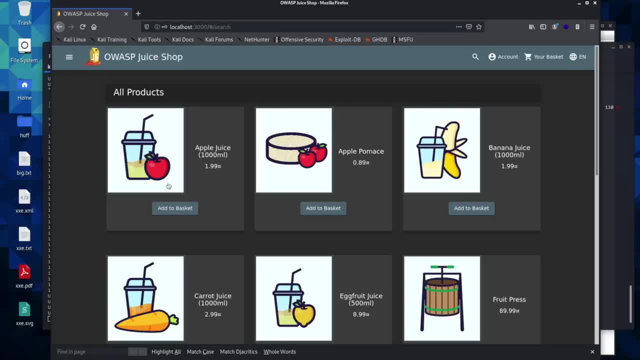 the challenge to where you actually are being paid two or three or four hundred dollars or more from this application. We just work through a few labs that are similar to this, So you can go ahead and try and this challenge and when it's done, you should get the green bar at the top of. 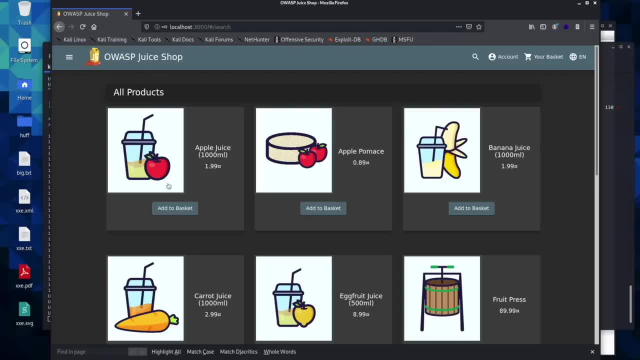 your screen. that will tell you that you have completed the challenge. so I want you to go ahead and pause this video and give that a try. okay, how did that go? we're going to go ahead and walk through this in the same manner in which I would. 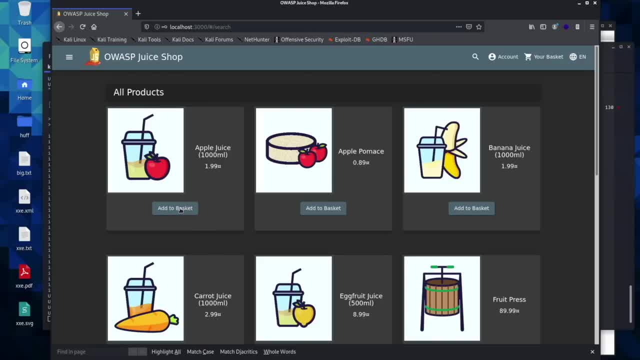 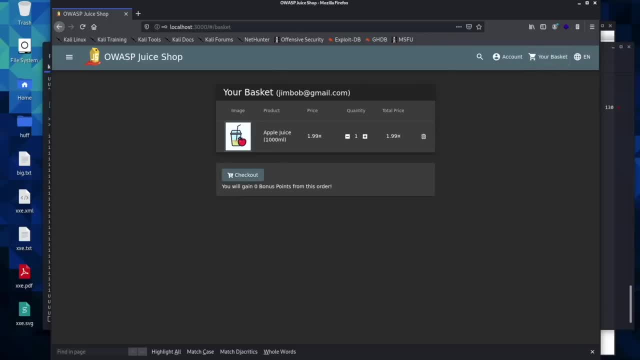 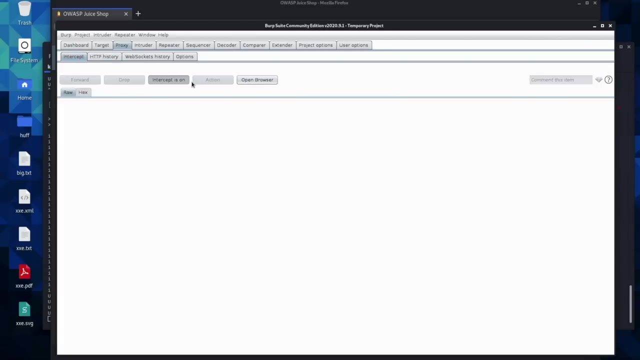 solve this. so go ahead and add something to your basket and then we'll check our basket and then at this point what I would do is I'd go ahead and turn the intercept on and walk through the whole checkout process and see if there's anywhere that I am able to modify and see if I can modify this in any way. 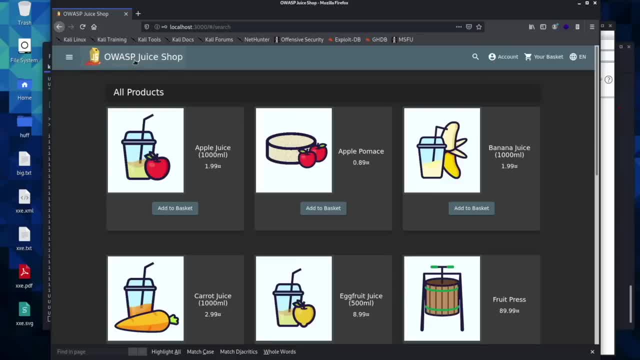 shape or form, and what I think I'm going to do is I don't actually want to walk through and have you watch me put all my that information in just to solve this challenge. so we'll go ahead and see if we can actually modify this before we get there. so it says we have basket. 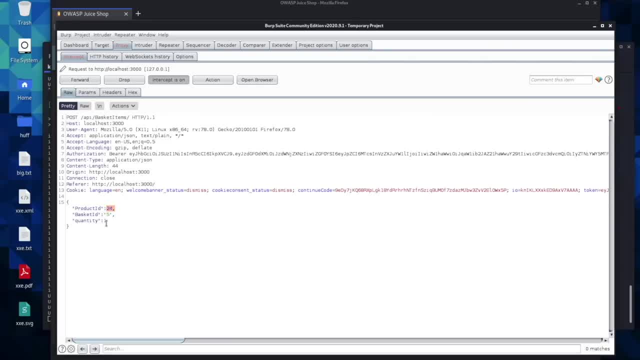 basket ID of five. we're buying product number four. let's see if it will. let us do what we did in the previous challenge and put in a negative amount. so try 99. turn the intercept off. it says we were able to add those to our, to our basket. 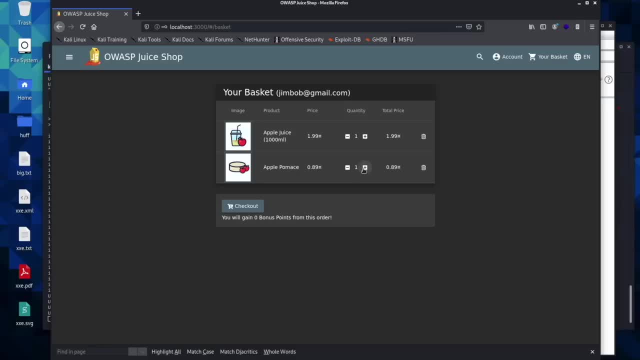 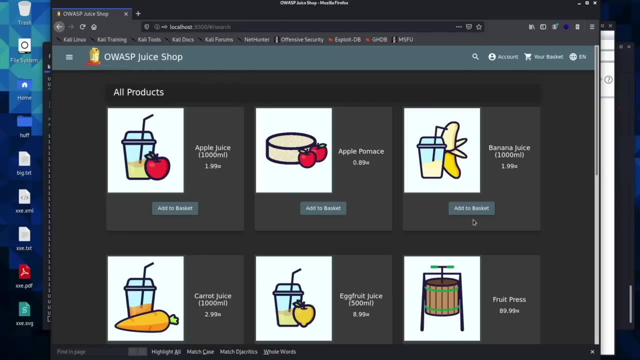 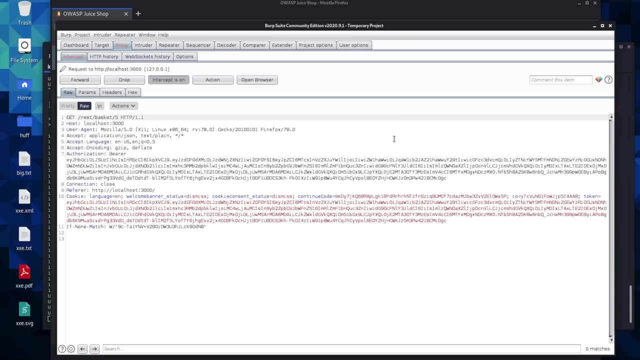 and they're gonna pay us. ah, that didn't work. okay, they're gonna pay us if we do that. so we'll go ahead and we'll try that again. a hundred dollars wasn't enough, so we'll come back to our products. we'll add to our basket. I forgot to turn burp on. add this to our basket. well, forward. 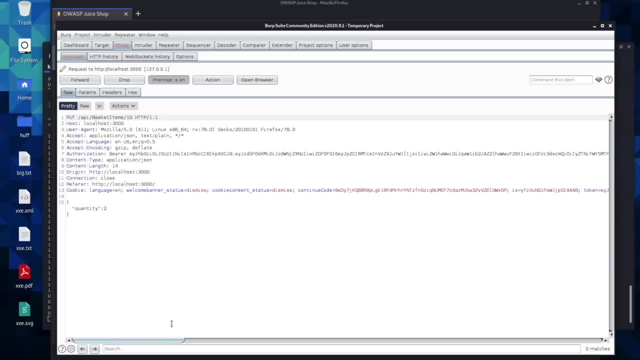 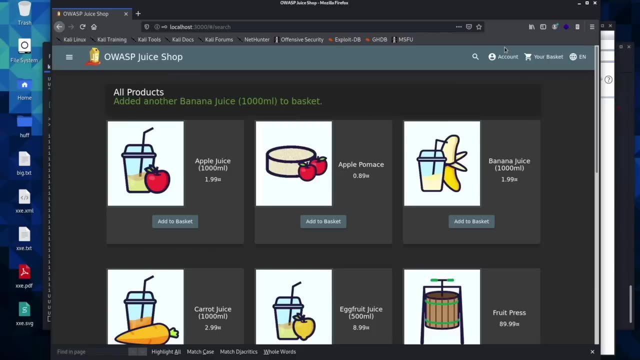 forward. here's our quantity. I wonder if the rest of our contents at the end of this string. well, we have our quantity. so what we'll do is we'll type in negative and we'll do 200 this time and we'll forward that and go to our basket and that's more like it we're. 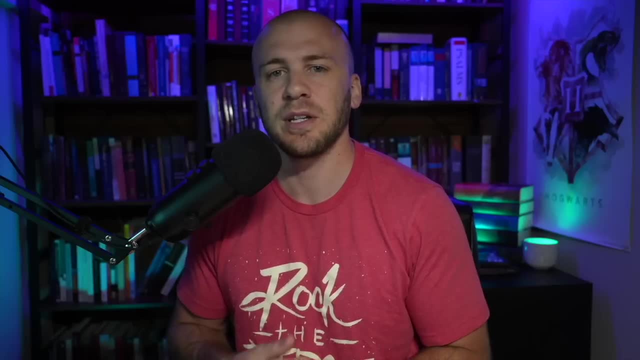 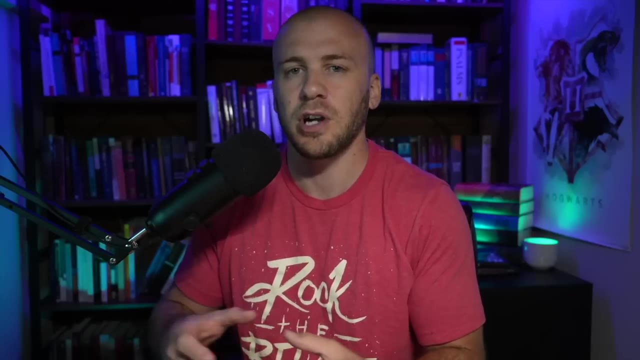 gonna get paid $400, so you do at this point. so for the next few minutes I'm gonna show you a little bit of a walkthrough and explain sequel injection from the Notis website and I don't want you to actually go there or try and do. 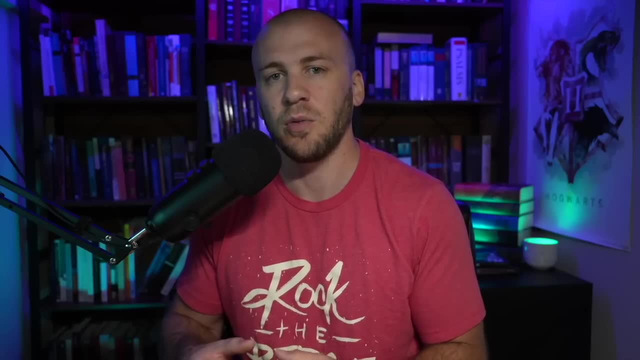 this walkthrough. we're gonna have plenty of practice when I have you create a count with port swigger and we walk through the ports- lifer, sequel, injection labs, and so, for just the next few minutes, as we go through the Notis example, I'm and then I'm going to go through this job and I'll show you how this П Seit Пast is available in DCS, and then I'm. 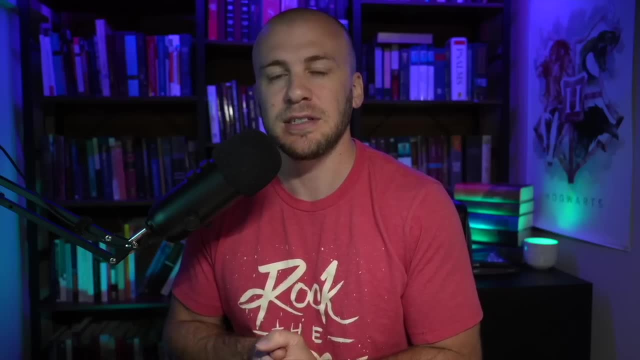 going to show you what the code actually looks like in a MySQL database, and I actually wrote a react app that's hooked up to a nodejs back-end with MySQL as the database. so you can kind of see what the code looks like, not that you need to. 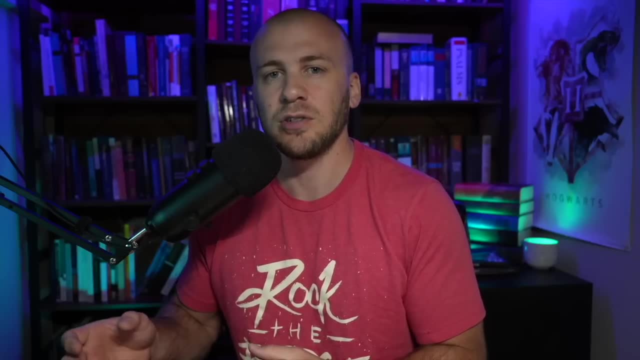 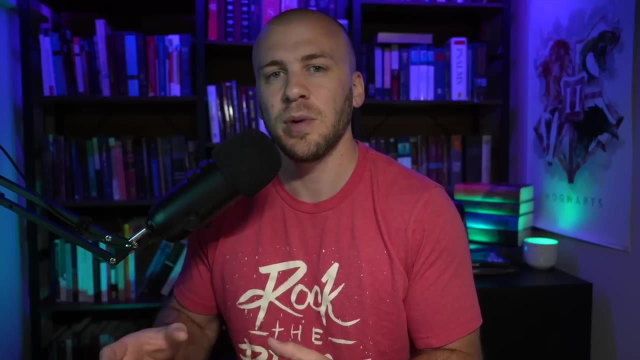 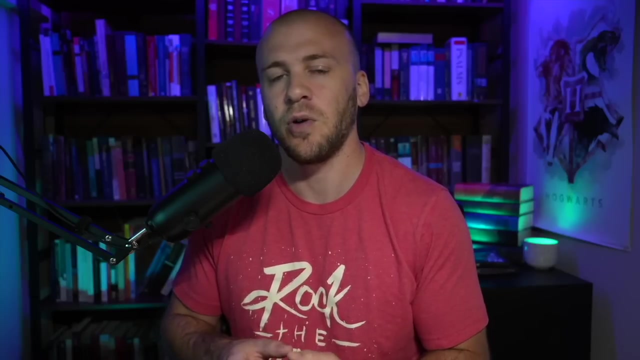 memorize it, but it might help a little bit. then we are going to move from there into a port swigger and try to walk through the SQL injections together. so for the next few minutes, as I am on the notice website, just try and follow along and maybe catch a few nuggets of detail to understand. and then, as I walk you, 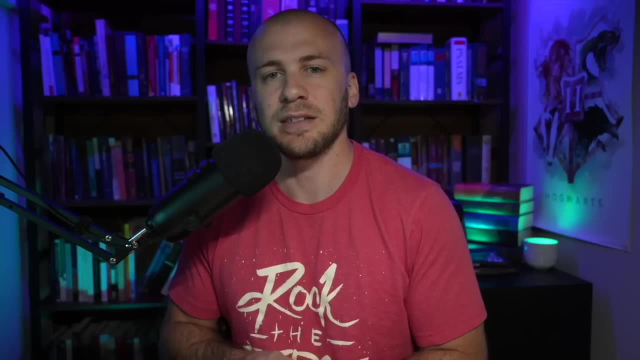 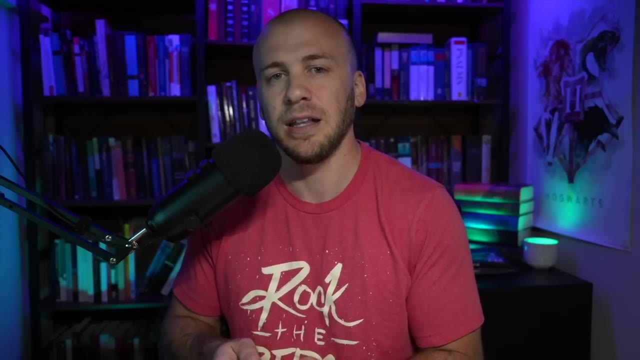 through the actual back end of a sequel database. I hope that you can understand it and maybe even do a few of the port swigger walkthroughs with me and then come back and then watch the MySQL database explanation again and hopefully it will begin to click. this is one of those attacks that is really really. 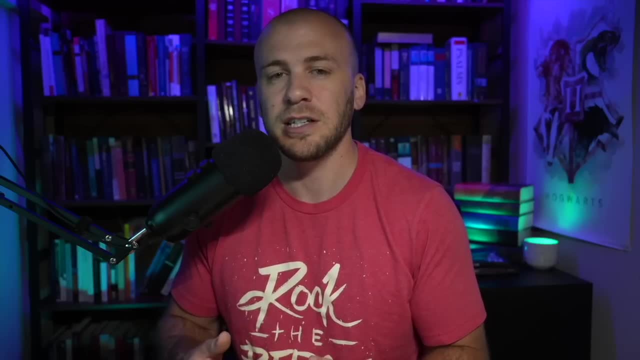 common, and so it's something that you should know and, upfront, I'm just gonna tell you. it might take you watching this and going through these labs several times to fully grasp the SQL injection, but that's okay. it takes time to become an ethical hacker. so with that, let's jump into it. 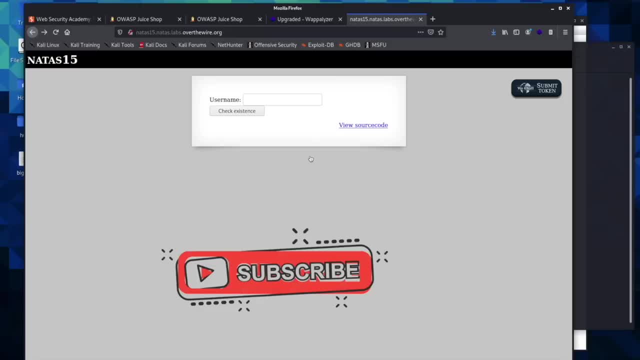 okay, we are going to begin working through some SQL injection. this is something that you can find. there are bug bounty hunters that dedicate their time only to looking for SQL injection, so this is something that you find when you are learning. you can become really proficient at it and this can be. 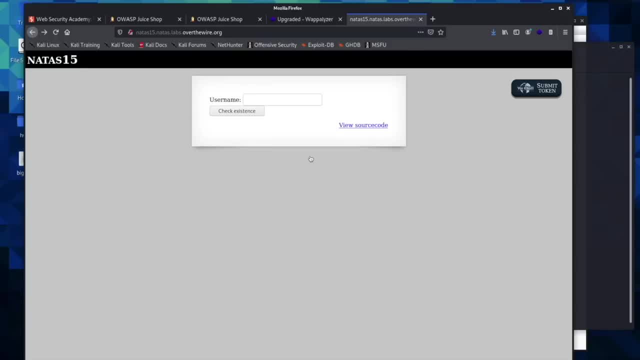 something that you primarily search for. so this is something I suggest learning and learning. well, it's easy to look for. you don't really need to know a whole lot about SQL databases in order to find these, but it does help in the bug bounty world. it's actually a lot easier than if you find these on a capture the flag. 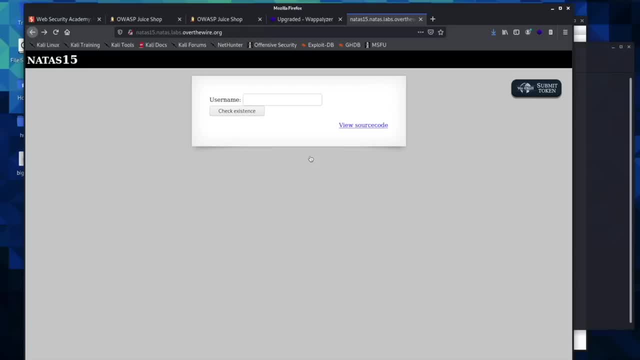 because all you have to do is put in a time delay to prove, to have a proof of concept. but in a capture the flag you'll have to know a little more than what we're going to go over here. but for the sake of not going through and learning how to program in SQL databases, 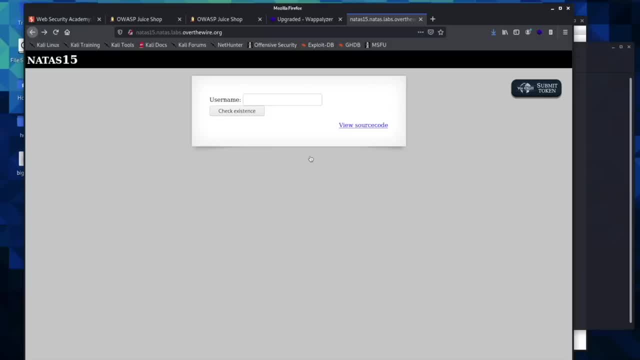 that I think it would take just too much time, and so we're going to go through how to find these. if you were to start looking on bug bounty programs- and I went ahead and opened up Nautus 15- you don't have to go through this or work through this. 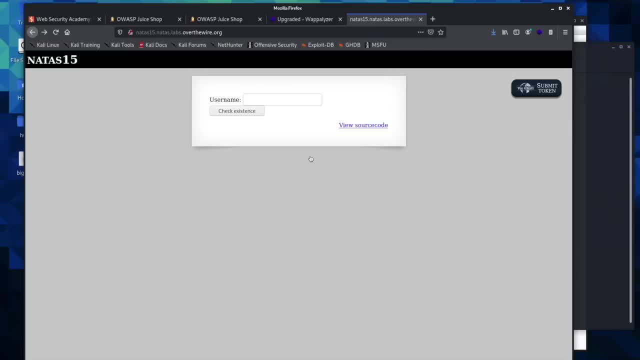 we're only going through this to show you what it's going to look like, and then we're going to actually go over to Port Swigger and we're going to work through their practice SQL injections. and so just to give you an idea of what we're doing, when you come to a login form such as this one, 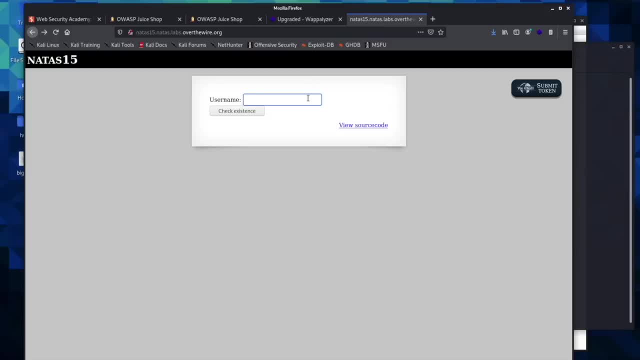 one of the best things you should do- and you should regularly check for- is just to put in a single quote, and then you would hit enter and see what happens and it says this user does not exist. what we're looking for is an error in the query, so I would. 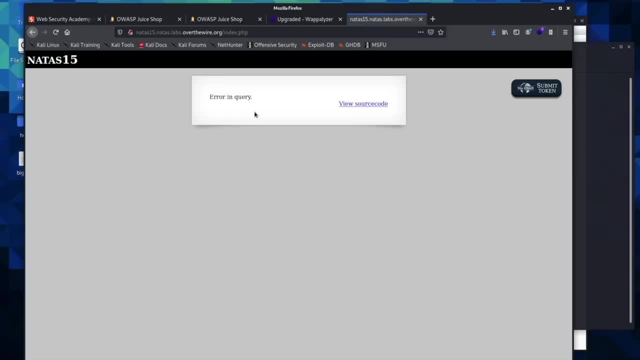 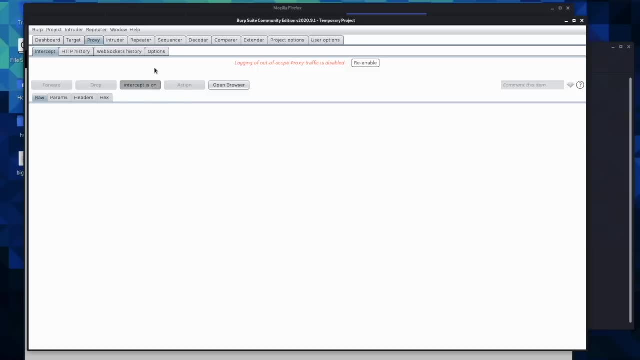 go and I would do a double quote next and I would hit check existence. and if you can hit an error, this is what we're looking for and I'll actually show you in BERT, because this is where you're probably going to be sending your request through. so you'll hit check existence. you. 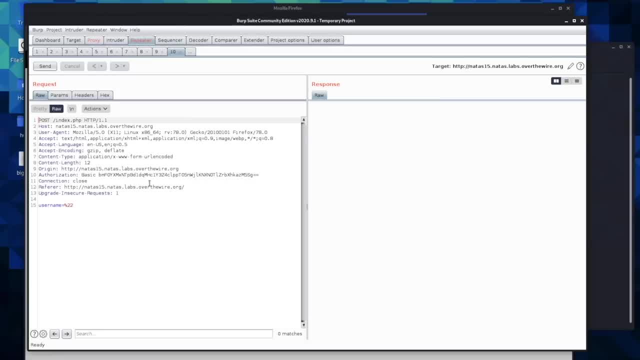 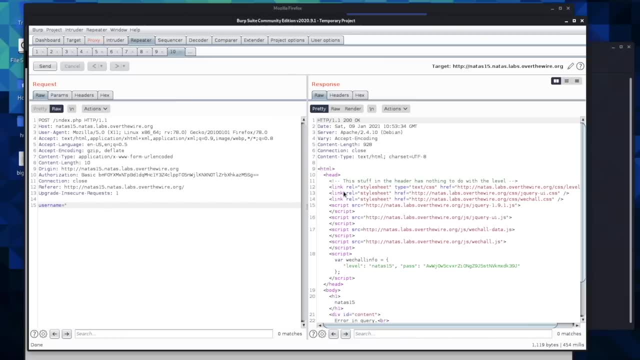 would send this to your repeater- and I'm actually just going to go ahead and change, see it- and then you would hit send and it says we get an error in query. what we're going to see here in a little bit is we're going to see this be a 501 and internal service Network error, and 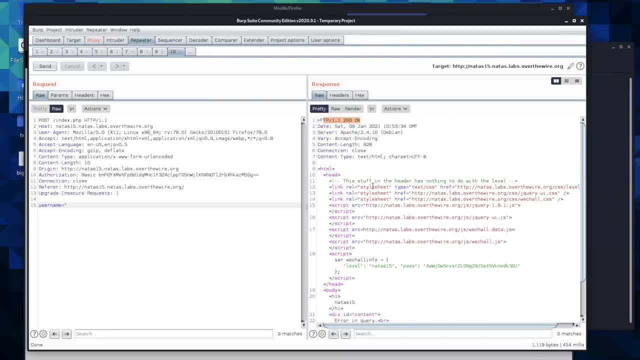 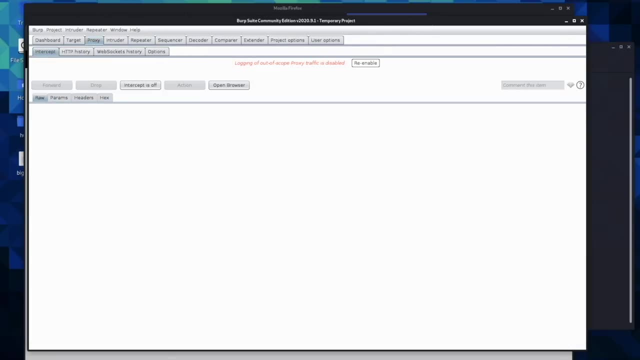 that's usually what you'll see. start finding these, but you will find what is called a blind SQL injection. we're going to look at those a little bit later. so we still have the error. so what do we do? error is we're going to start the enumeration process, but we're actually not going to do that. 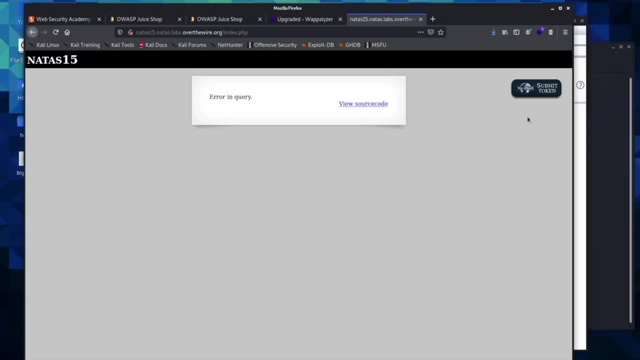 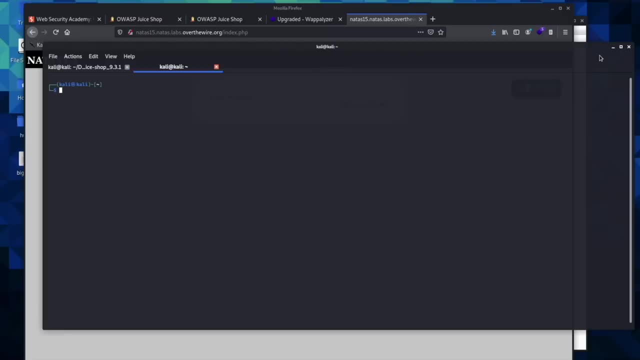 here. i just wanted to show you kind of what we're looking for here so that you can look for it on your own in the first port swigger lab and see what you can find, if you can find it on your own, but just to give you a little more of an idea of what's going on in the background. 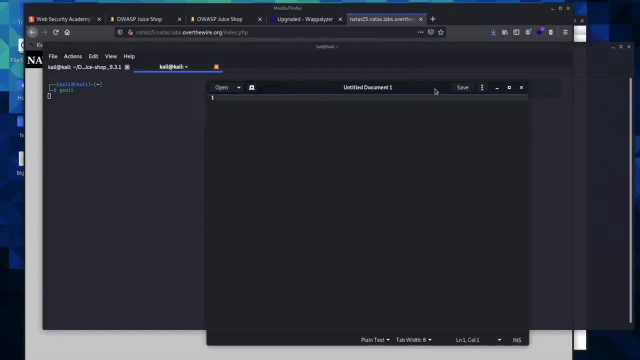 the sql database and sql language is going to look something like this: select all from users. this will be where username equals and this is what we input right here. so this would be our input. so what we did is we took this. this is what it will look like and this is what we can. 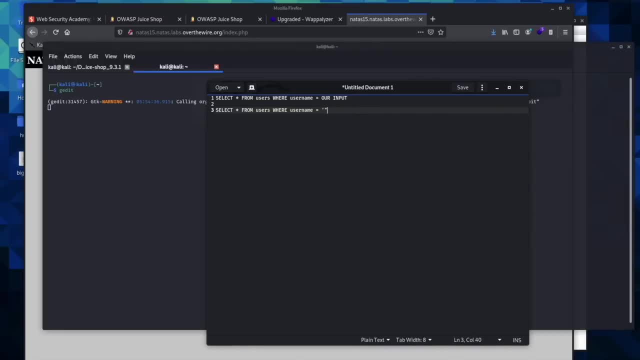 put in here, so you'd put your single quote or your double quote and, in the case of the notice web application, what it has is a something like this: and then here's where you're putting your query, where you're putting in to see if the username exists. 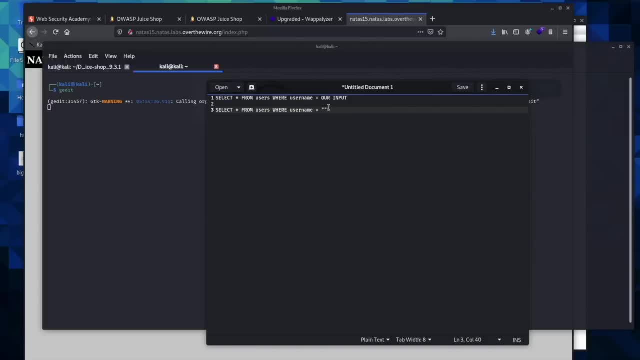 and so when we put in another double quote, what happens is you break the query and this produces the error right here, because it doesn't need to be there. it shouldn't be there in order for this to work in programming, and so that's how you break it. okay, what we're about to go over is going to be: 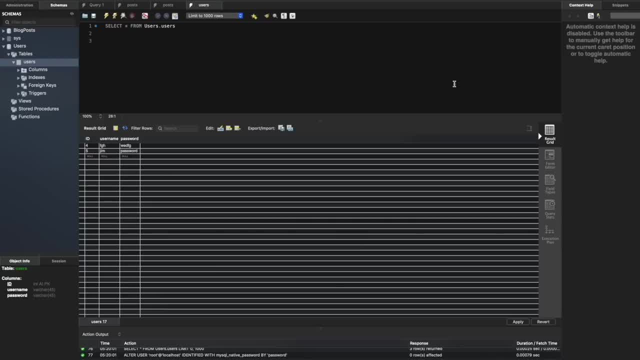 a little advanced, but i think it will help you visualize what's going on beyond more than what i just showed you in the last video. so what i have up is actually my sql workbench. we have here just a simple database username i was testing. here's an actual username and password. 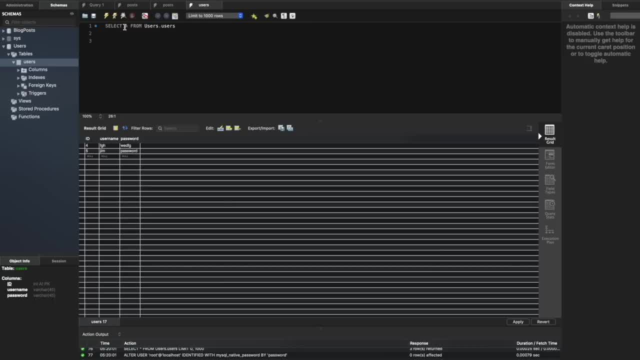 this is what a table will look like, and so in our query we have select all from users, which is our schema, and then the table, which is users. that's not capitalized letter here, and so this is what a table looks like, and what's going to happen is this is running on a server and when we send, 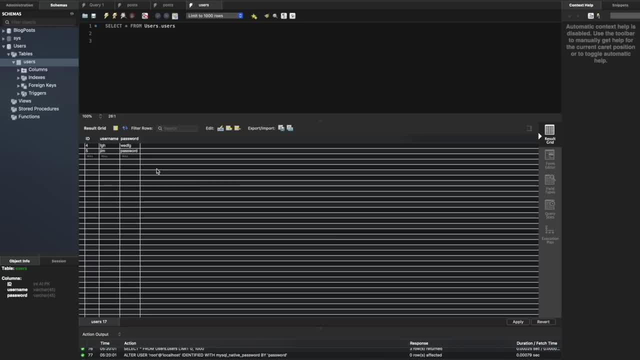 a query to the back end of a web application, it will reach out to the server and see if our query is true. so i want to pause here because- so this is an update. i want to pause here and explain something a little better that i noticed i didn't do a very good job of. when you make a query, you're. 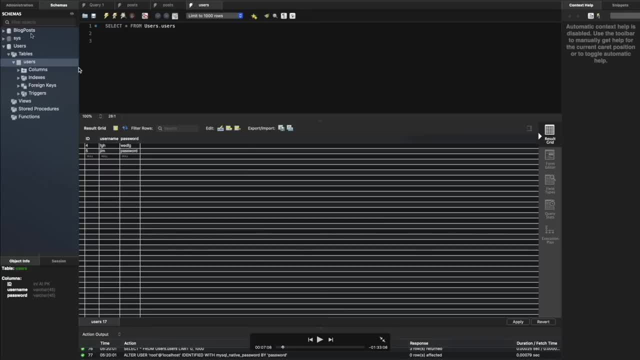 going to have to do a lot of work in order to get a query to a database. the whole reason i wanted to show you the workbench is so that you could see. these are the tables. so if i came over here and i said from select all from blog post, then we're going to be grabbing the tables from inside. 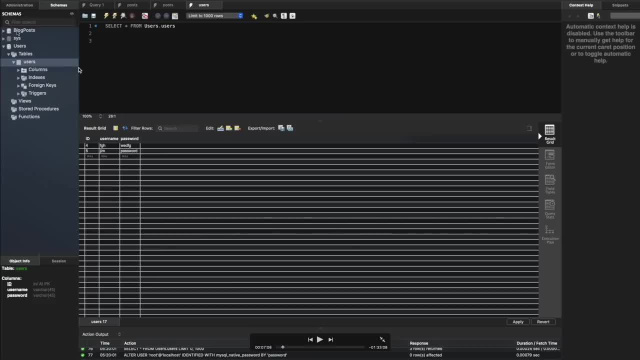 the blog post and so when we look at this, select all from users. this is showing all the databases. so this is a database, this is a database and we're selecting from this database right here, the users, one that we see right here. this is the database and this is the table within the database. so 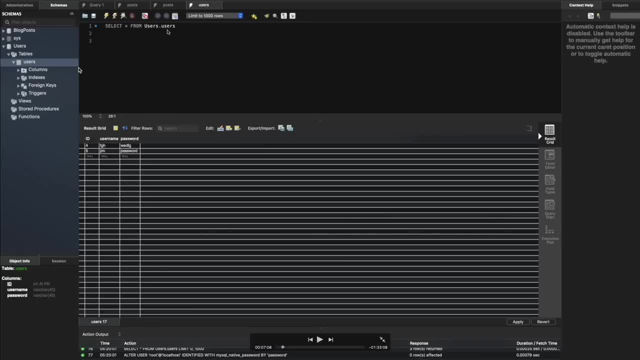 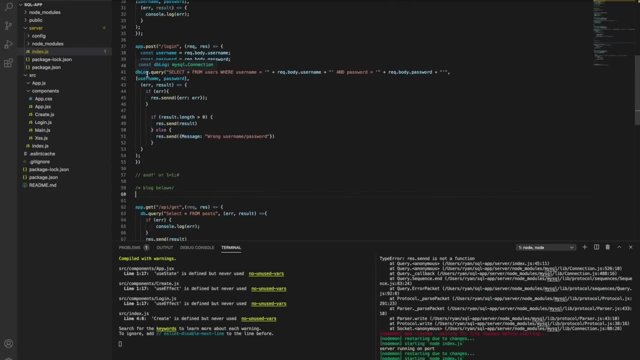 select all from database and then table. this will be really helpful in the future when we learn to run sql map and we need to know the context of sql map, and so this is what it will look like. the code will look like: we have our database and we're querying our database and we are selecting all. 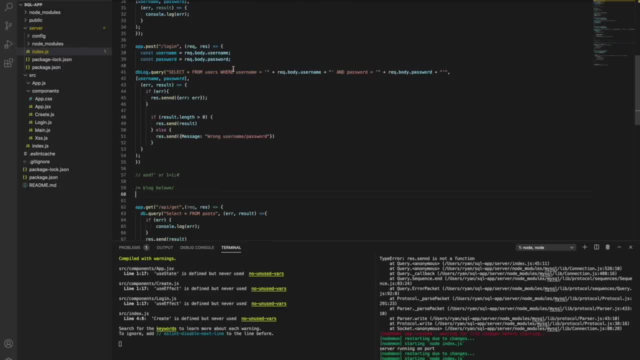 from the users table where the username equals, and then you can just pretend this is blank, because this is where our input is going to go in here. so we're selecting all users from the table where our input is at and the password is equal to the other input, and so this makes sure that we have an actual username. 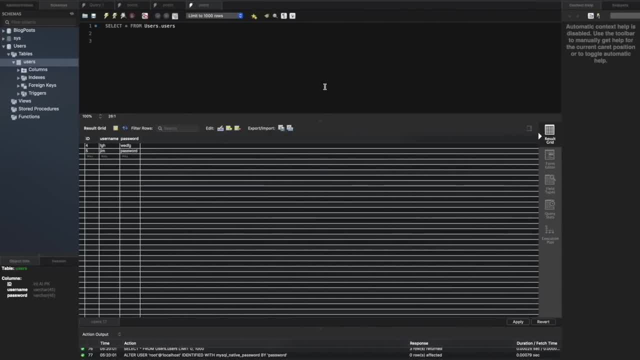 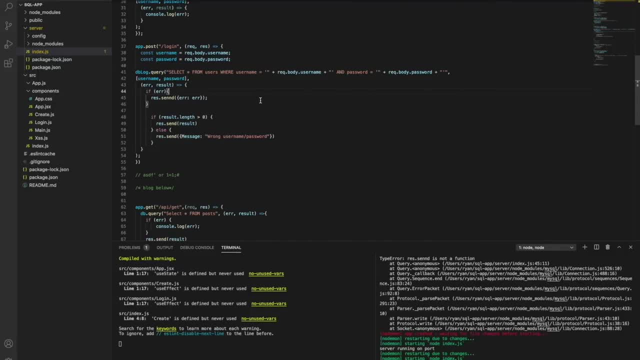 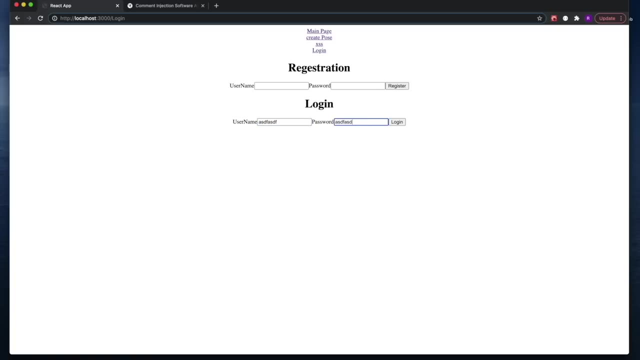 and then it makes sure we have a password that matches our username and our password from our table. and so what this looks like is over here we have have our login here, and if we type something in and we type in a password and we hit login, it's going to say wrong username. 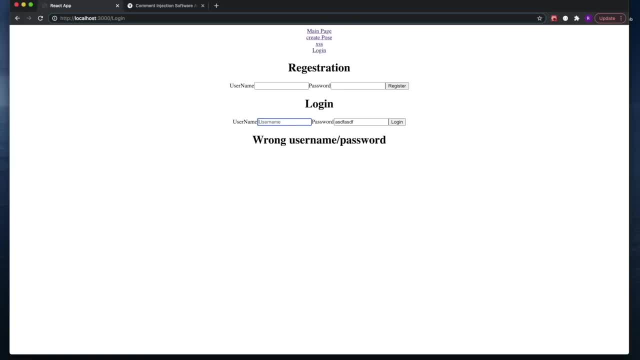 slash password. and so if we come in here and we actually have our actual login made, it'll say we are logged in. and so when we do a sql injection, basically what we're doing is sending in a request that we decide what it's going to be to the database, to the back. 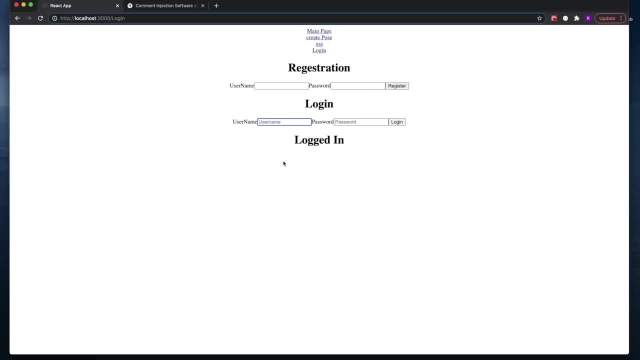 end of the website that reaches out to our database server. so this is a pretty simple sql injection that we're going to be covering here, and we're going to be going into union select statements after this video, which i think are more common than what we're about to go over. 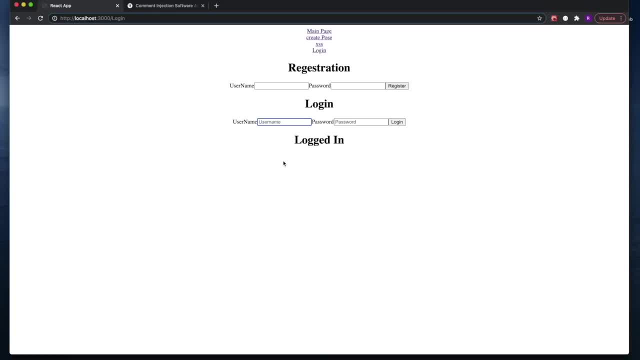 and so it's very important to learn the union select sql injection statements. there are some of. There are some bug bounty hunters that dedicate all of their time only to Sequel injection, So I just made this. I'm shooting this video because I really want you to understand what's going on. 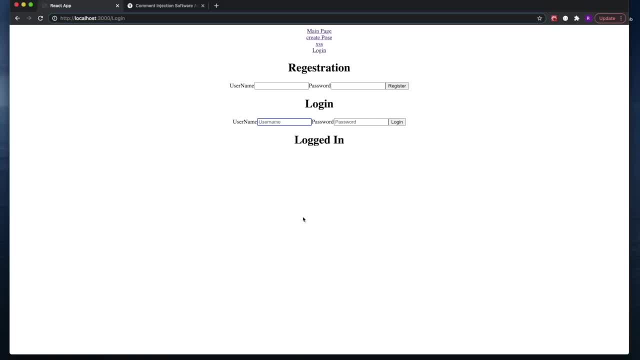 And it'll make more sense. Don't worry, If it doesn't make sense right now, You may have to come back to this video more than once and go over the union select statements labs on your own and then Come back to them after a day or two and just continue practicing them until you really have them down. 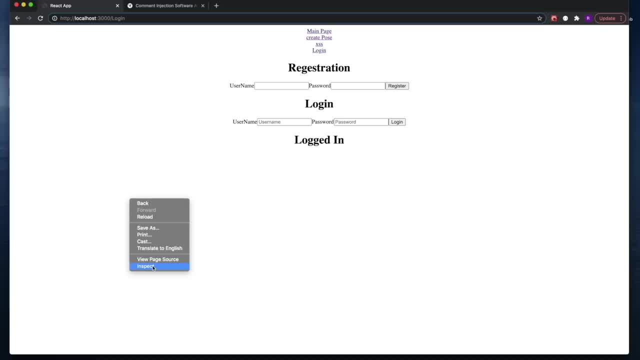 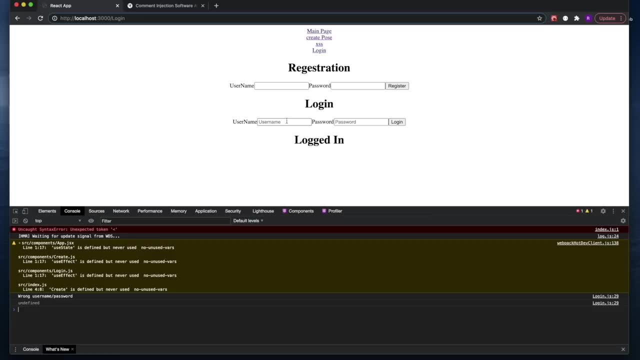 And so one of the things that we're looking for when we do a sequel injection is- I'm going to inspect this so you can actually See this happen. We're gonna have our console up. ignore my errors, because my code is not perfect when you put in a single quote. 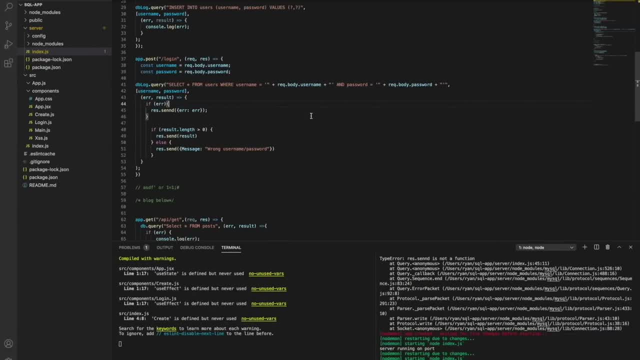 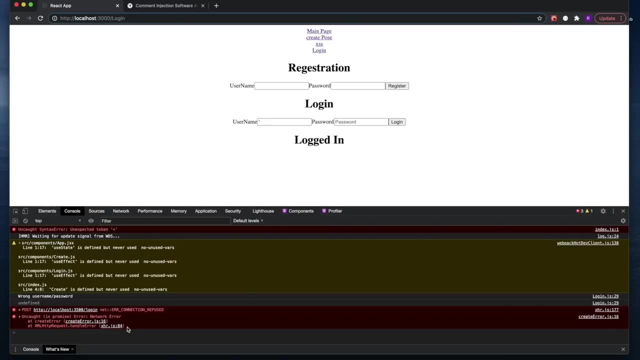 it will break this right here and It will give it will crash our server. So if we go ahead and throw that in, you see our Connection is refused And if you come over here, you can see our application has crashed, which means I need to. 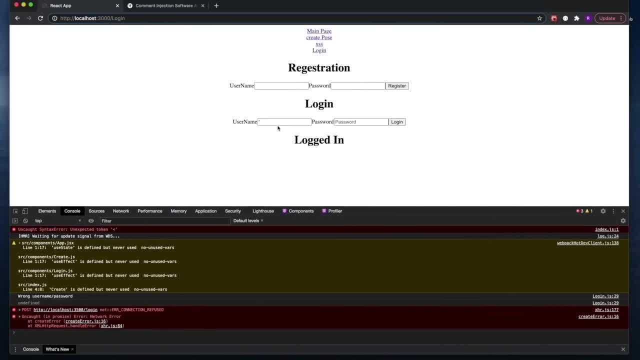 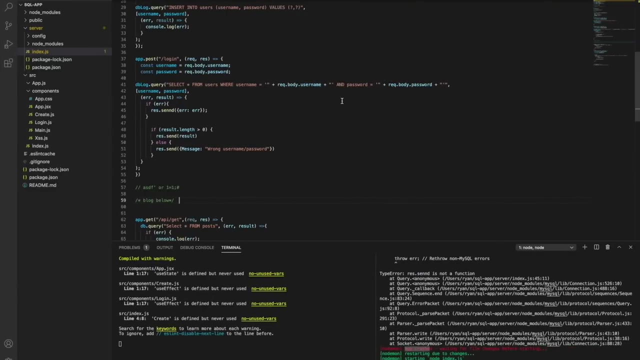 Restart it and now our applications running, and so when you send that, you'll have an internal server error, Which is what we essentially just got right here. And so how we get past this is By actually giving it a statement that is true, so that it will give us back the first. 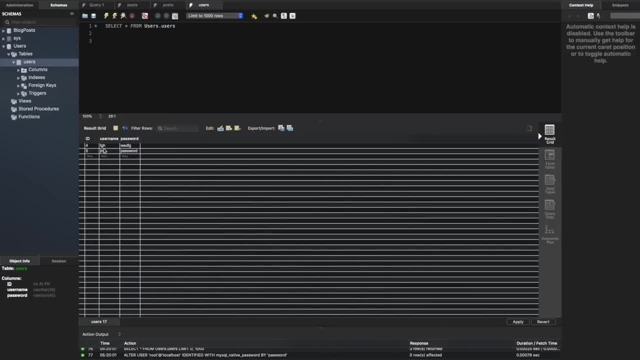 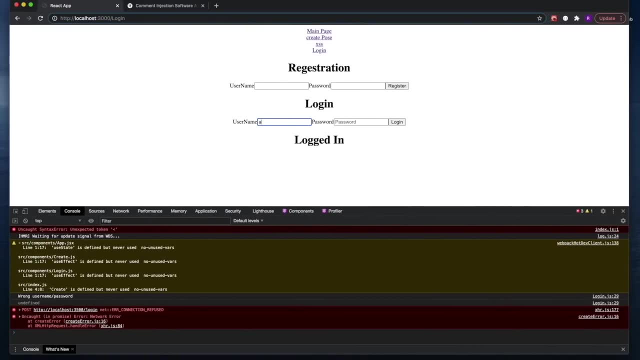 character, the first login in the database. It'll give us back the first username and password, and so we're gonna make a true statement right now. And so what we'll do is we'll just throw in- it doesn't really matter, and then our single quote, and then we'll have or. 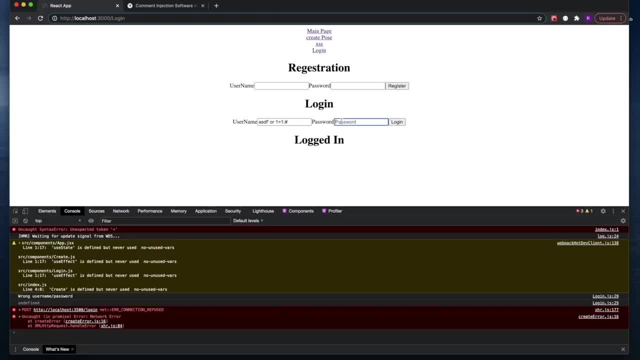 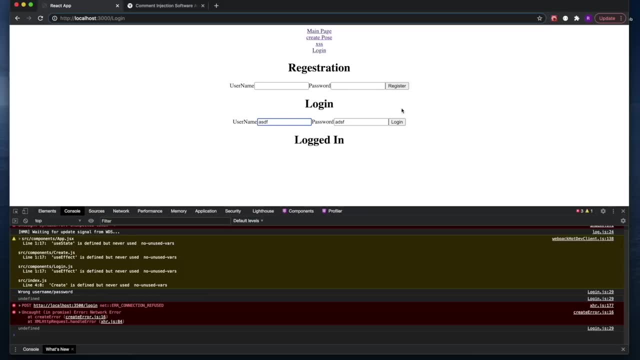 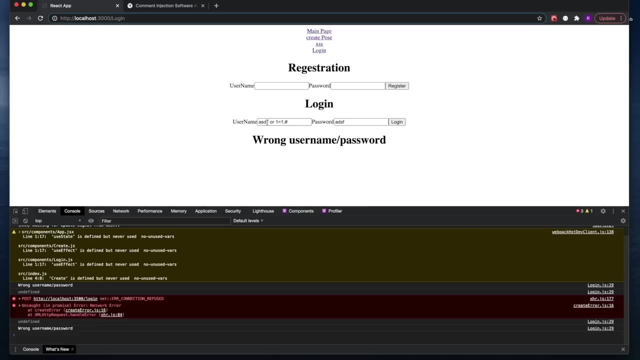 one equals one, and then we comment out everything after that, and then our password doesn't matter either and it says we're logged in. but if we just have this right here, it doesn't really. it'll tell us that we're not logged in, because this isn't correct. so if we have this in here, what we're? 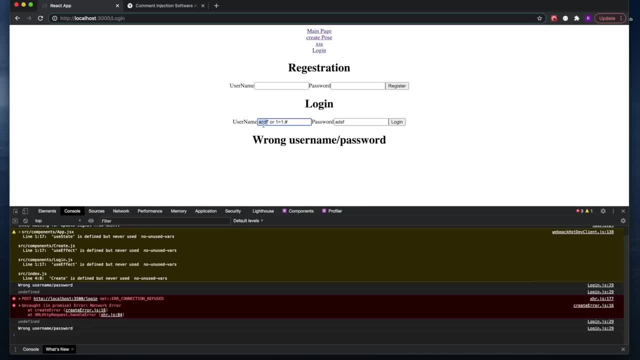 saying is: is this username right? is this a true username? and the answer is no. you see, we have wrong user, a username and password, but one equals one is always true. and then we comment everything out after this statement with this hash: so our password doesn't work. so you see how this is all. 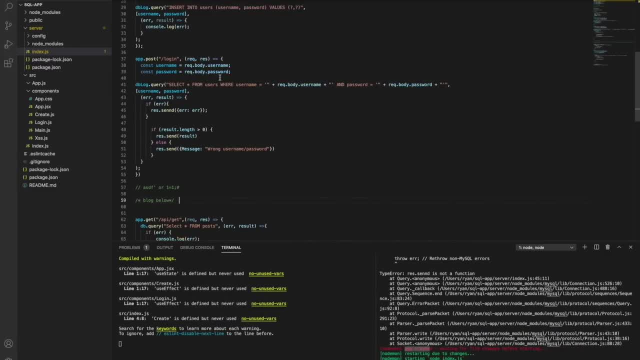 in one line of code. this is all getting ran together. it's making this query all together and what we're doing is essentially commenting out everything after our username and then we're so. the password doesn't even matter. so when i say we comment something out, we're commenting out. 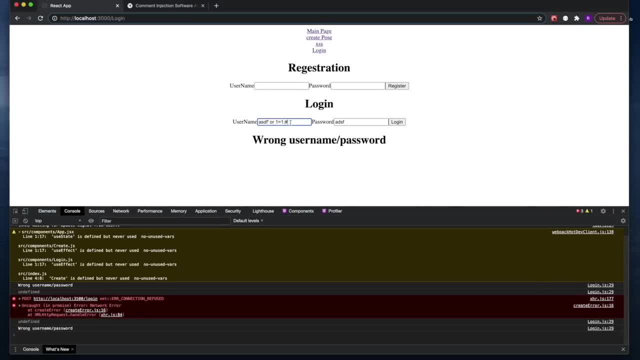 everything after our statement and so we throw this hash in here and everything after it's commented out. the password doesn't matter. i think we can get by with no password, because i don't have it set up right now that you have to have any characters in here and it will come back as true. 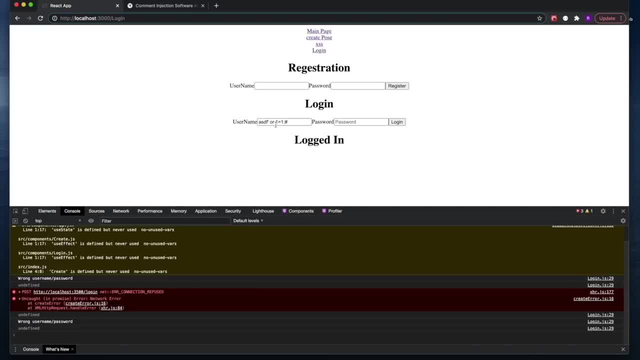 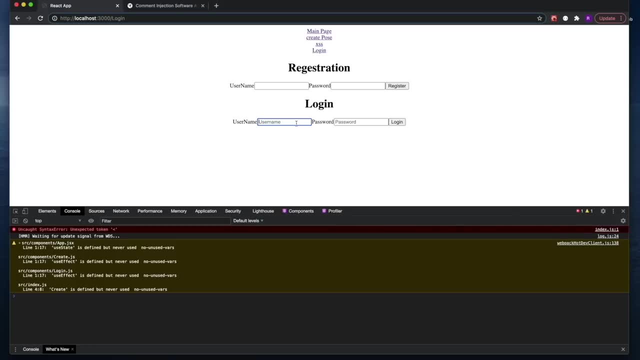 and this is what i'm talking about when we say sequence statement and we're querying a database or a server, okay. there is one other thing i really want to show us. we're going to go over this again, exactly what i'm showing you right now in another couple of videos, but i think it'll. 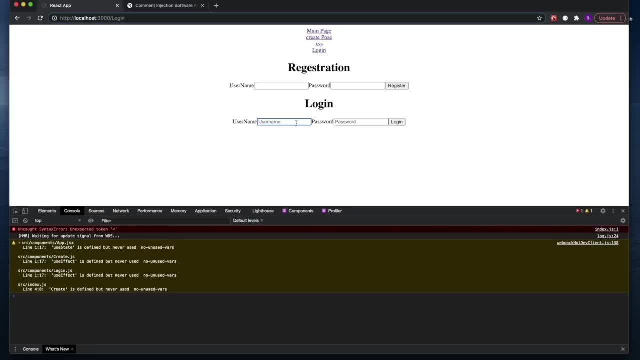 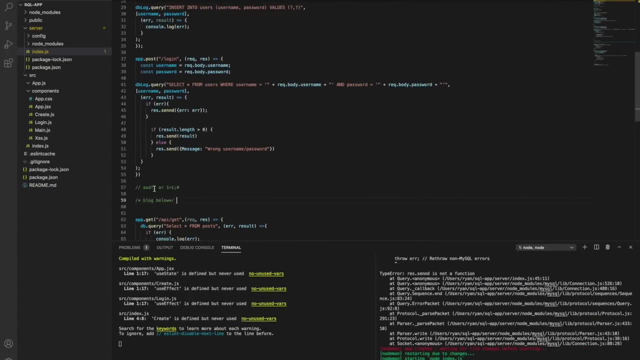 be helpful to see it. so one other thing is: whenever you give it a database, a true statement it's going to come back with without an error, or saying it's a logged in, it's going to come back as true. so we just saw the statement that looked like this: we had our username. 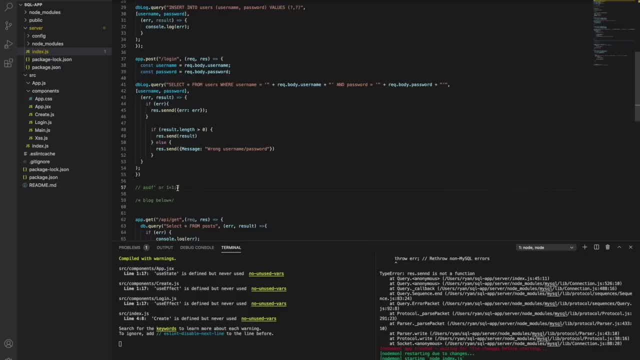 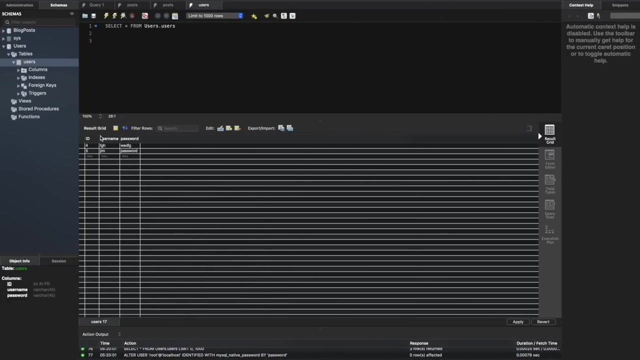 and then we had: or 1 equals 1 and 1 equals 1 is always true, and so it comes back as a logged in or it comes back as true. there are other things we can do to get get information from a database. see, we want these username and passwords and we have an id, so we have three columns here. 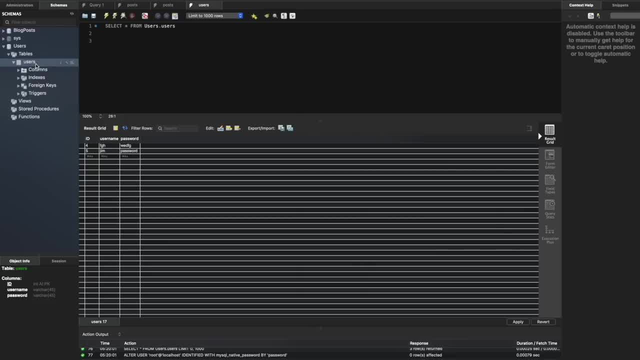 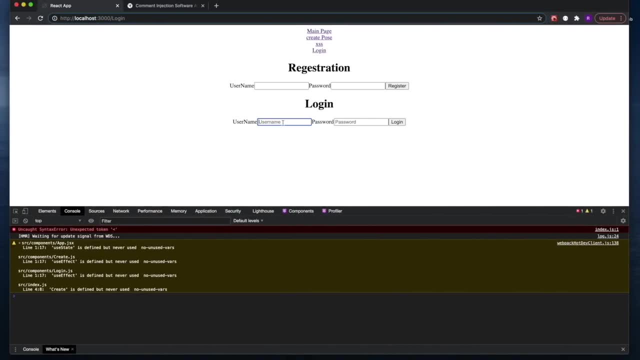 that have information in them. let's say, we know the table is users and we want to know how many columns we have. what we'll do is to pull down something. true, want to pull down the number of columns because we don't actually know how many there are and we 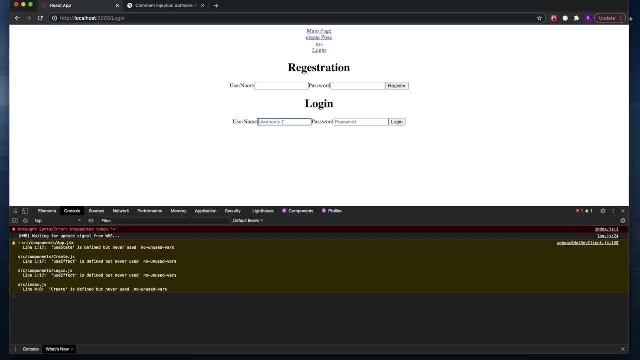 want to just find out some information from this database. you can actually come in here just like we did before, put in our random username, that doesn't really matter. and then this is what I mean when I say a union select statement: so we're going to connect union to our statement here, so we 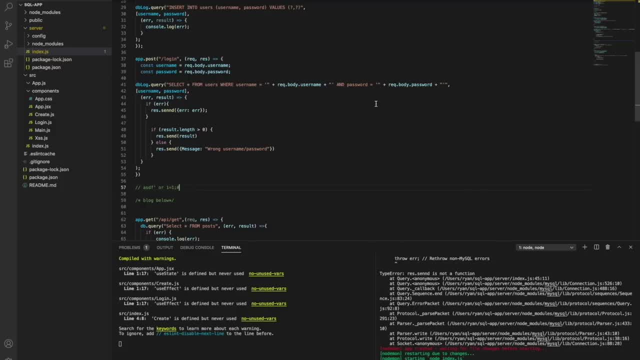 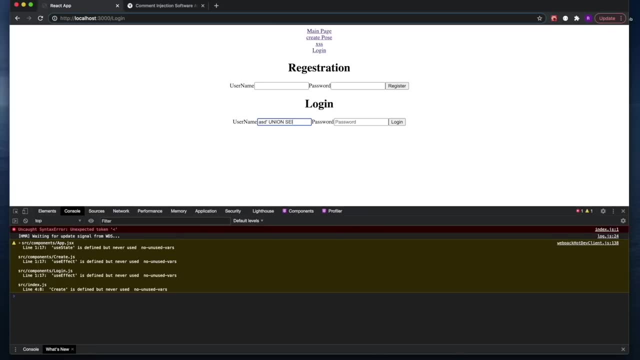 have select all from users where username equals these things, and then we're going to add to it. we want to add a union select, if I can spell. we're going to select null and this will tell us: is there one column in our table? and we send this, we're going to crash the server. I'll go ahead. 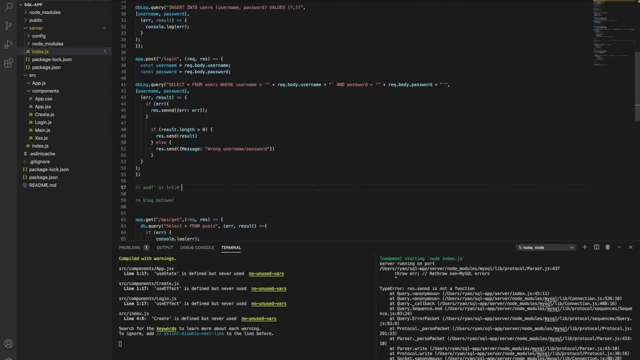 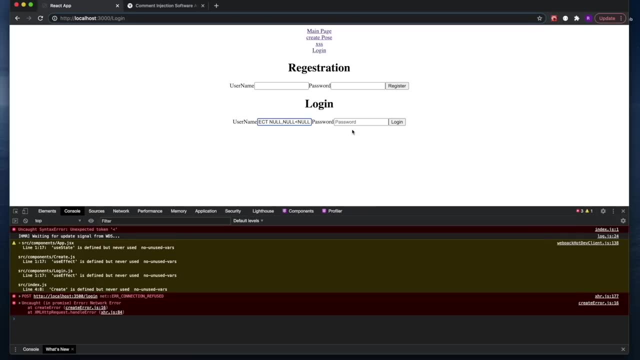 and send it so you can see we crash the server. I have to come over here, restart the server and then I'm just going to give you: there's three columns. we know there are three columns, so we'll throw in null two more times and this will say union. 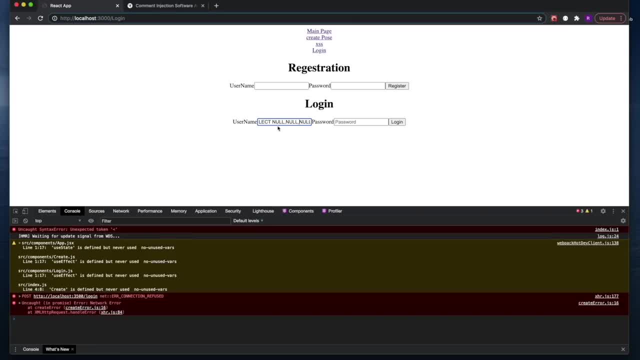 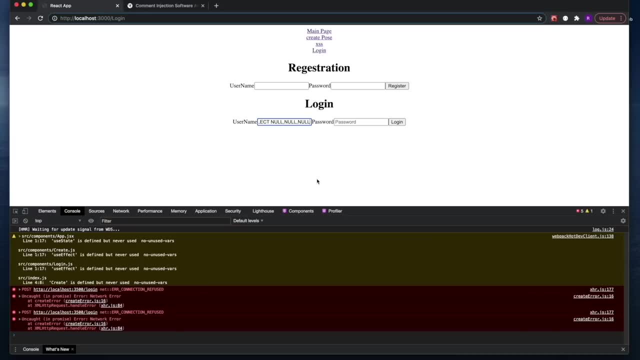 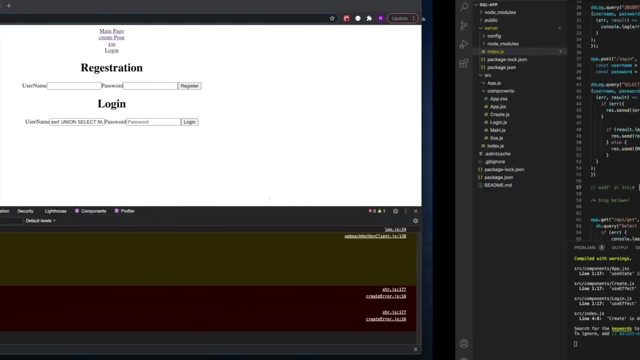 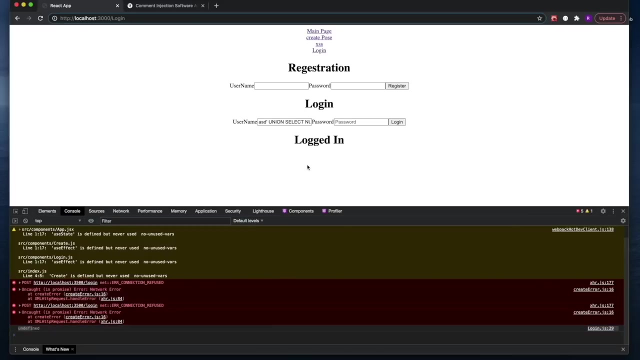 select, which is going to pull down how many columns there are, and if we send this, we have. we didn't. we got in crash the server because we didn't comment out the rest of the string that we were creating. so here we go. we'll log in now. we have no undefined. came back, which means we have no errors, so we'd. 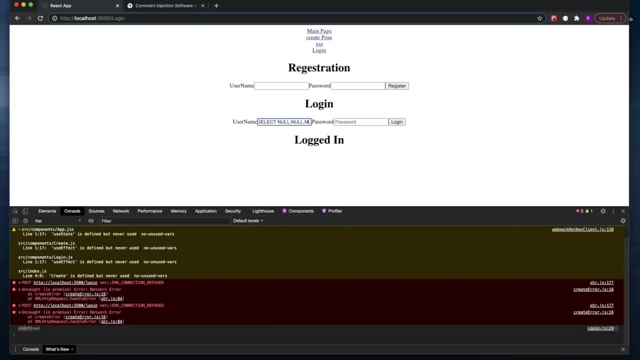 know there are three columns and so this is going to come up and one of our very first SQL injections that we're going to be doing on the port swigger web application and their labs that they have set up for us to a practice on, and you feel free to continue practicing in there. but 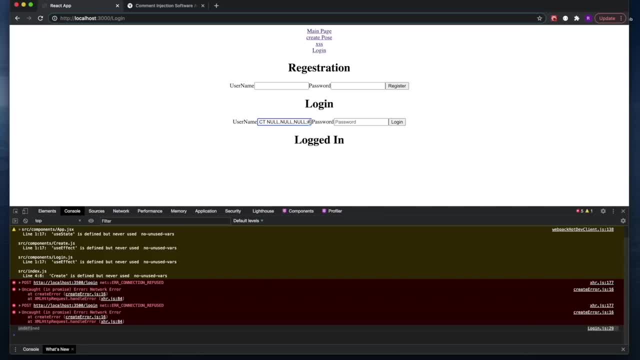 this is something we're going to be doing and we're going to be going in a lot more detail, and you'll have to pay attention to this comment because it will change between two dashes without the semicolon, based on the type of database that we're using. so I do apologize. 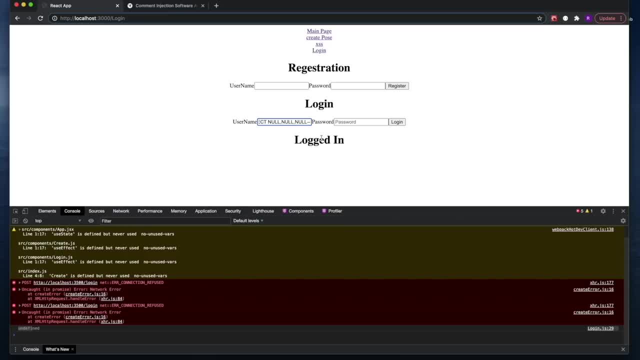 if this seems confusing, hopefully it becomes more clear. it's in the top ten most common vulnerabilities. I think it's in the top five most common vulnerabilities. looking little difficult right now because you've never seen it before, but by the end of this module in the course if it's. 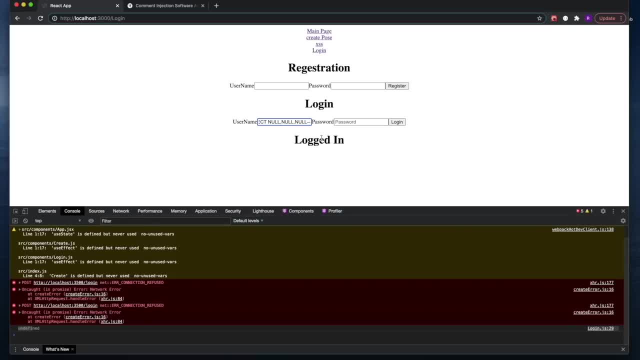 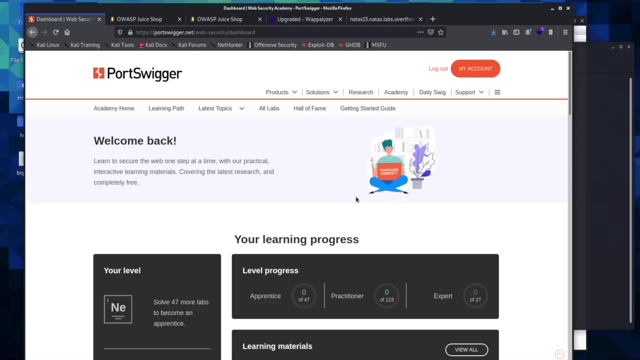 still unclear, you can go back and try it again and go back through this module and it will become more clear and you will memorize how to find the these vulnerabilities. so with that, I will see you in the next video. okay, we are here on portswiggernet. 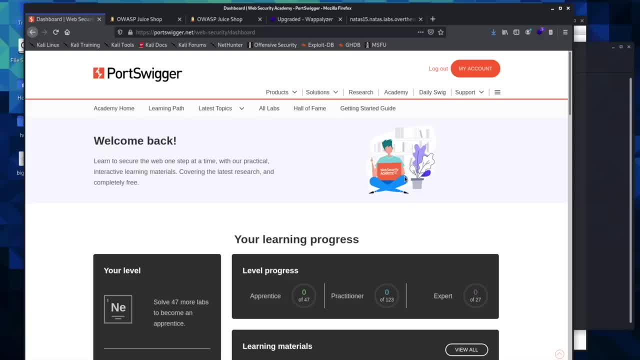 you can go ahead. I actually went ahead and logged in and created a new account. you can come in here and you can come up here, click sign in and then create a new account and then, once you've done that, come back to the website and you will go to Academy. you can go ahead and click that and it'll. 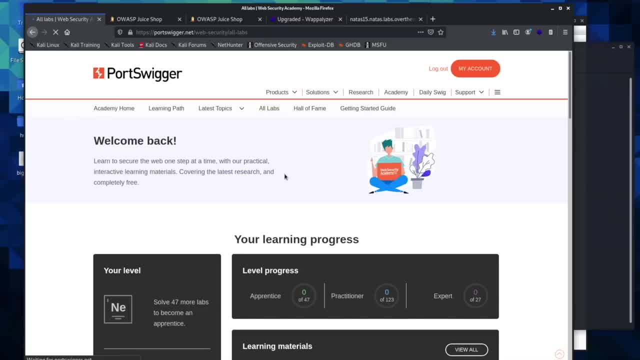 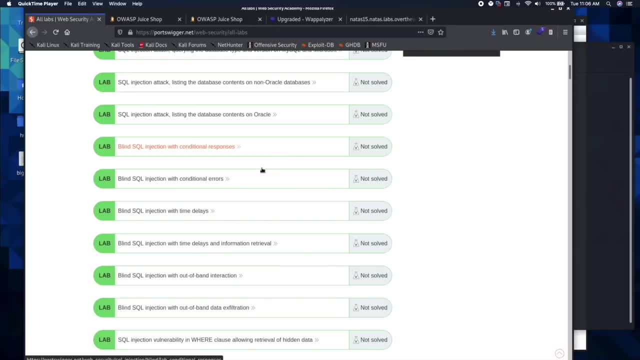 load up and then you'll go to all labs. we'll take us to some of the labs we're going to be working through and the sequel injection. if you are having a hard time finding this exact URL right here, I will put a link to it in the description or you can just type this out in order to get to all the labs there's. 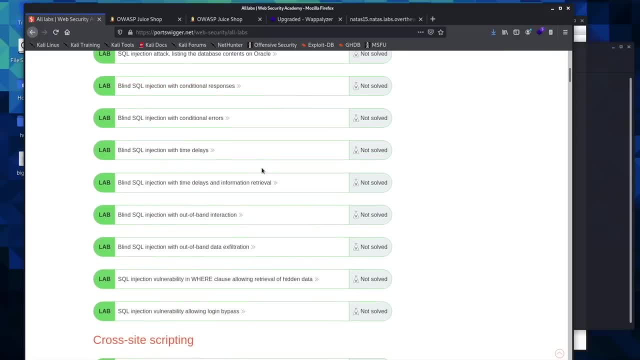 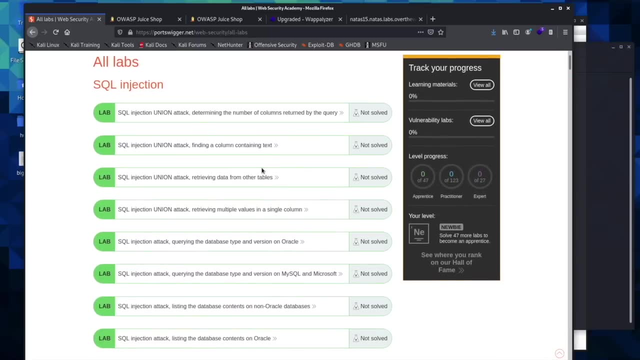 a whole bunch of them. we're not going to be going through all of them because some of them get kind of repetitive and it has been a while since I have done these- at least a year- and so I actually thought what would be good? I'm not going. 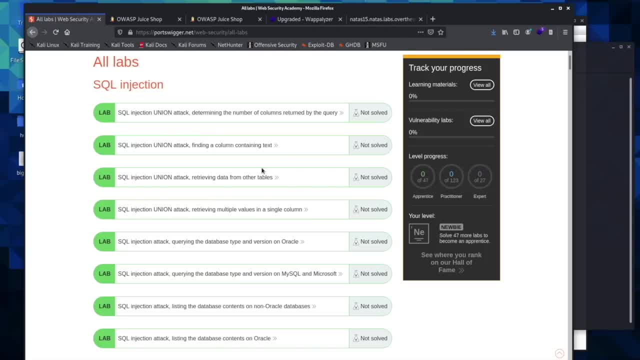 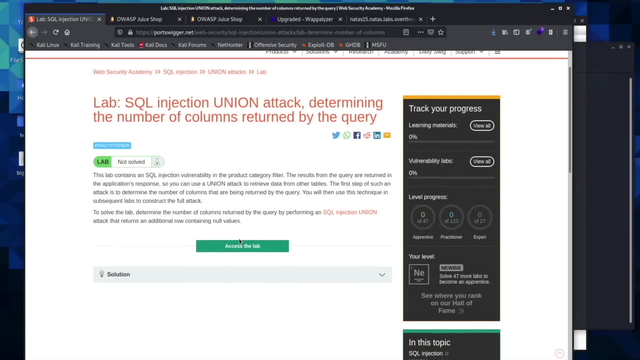 to rehash any of these before we go through them. so you are going to see me make mistakes and you'll get to see my thought process and you'll kind of just get to see how I work through these, and so, if you want, you can go ahead and open up the first one and then I like to open it up in a second tab. 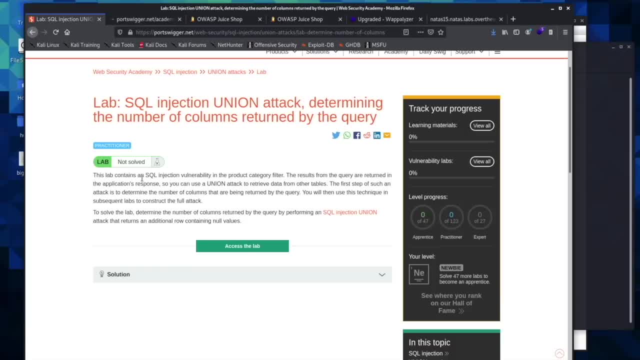 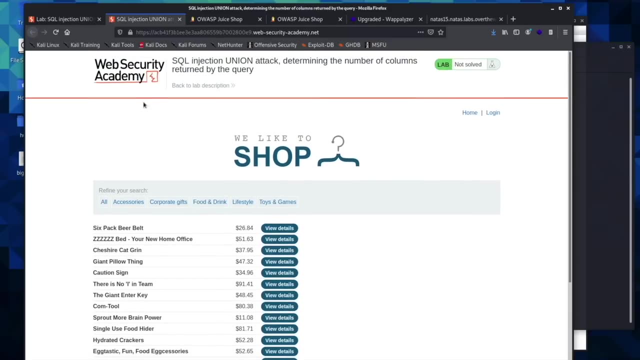 over here and they'll give you some instructions and kind of tell you what you're looking for here. they'll actually tell you where to find some of the sequel injections, so you don't have to spend your time clicking through the whole web application and trying to figure out where things are, and so they kind of point you in the 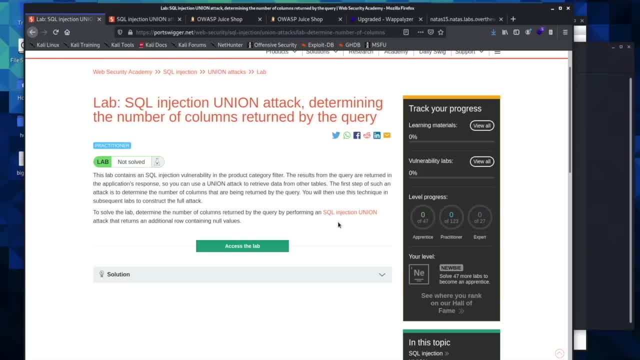 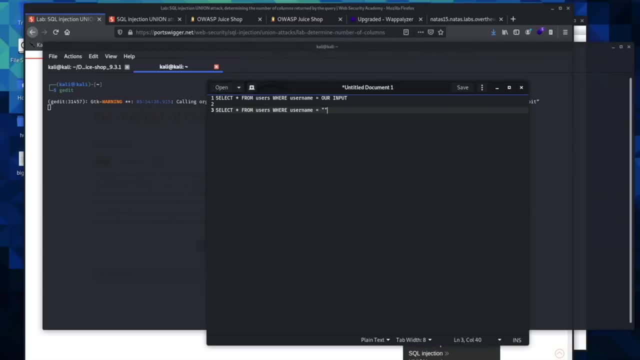 right direction, and so we're looking for a sequel injection with the Union attack, and so what this looks like- let's, uh, open this back up. this is what their side of the query looks like, and then we will be typing in: you would close, close it off. in our case, it's going to be a single quote, Union select, and then we're going to be. 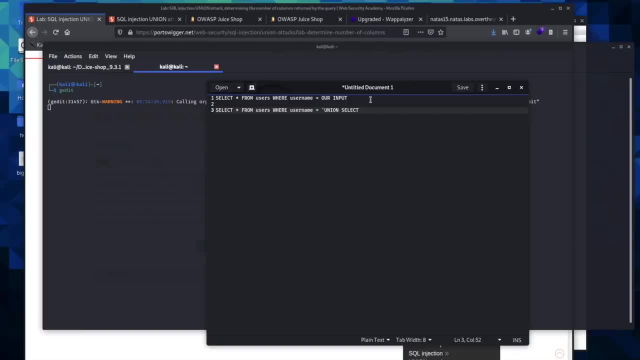 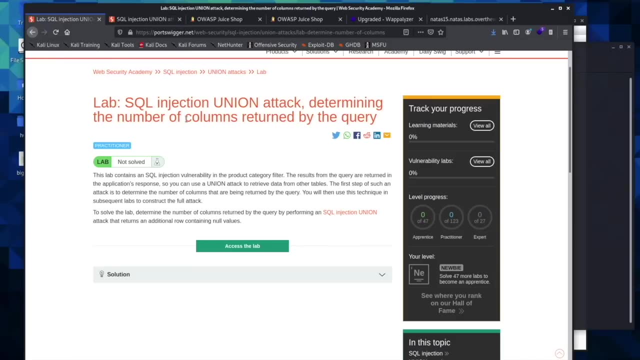 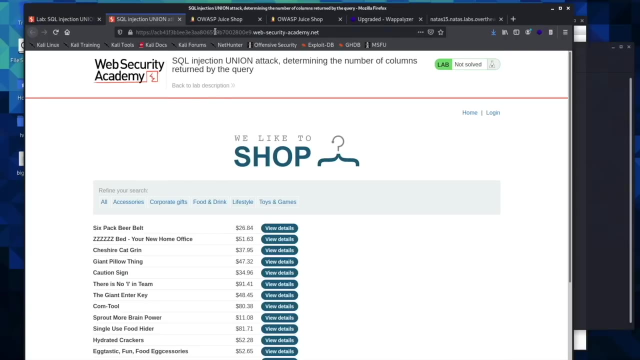 looking for the number of columns and what we can find within this vulnerability. so we come over here and it says: find the number of columns returned by the query, and there's a couple of ways to do this. I think I'll show you both. I think they both work in this program and you. 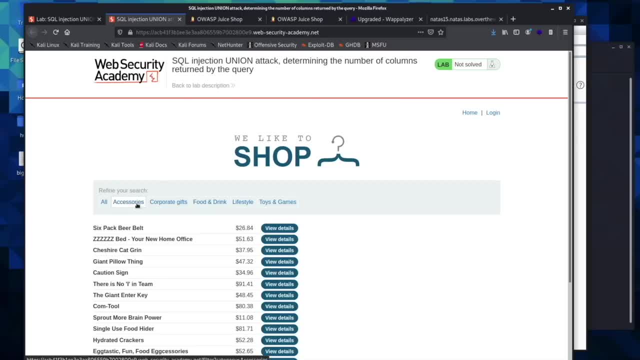 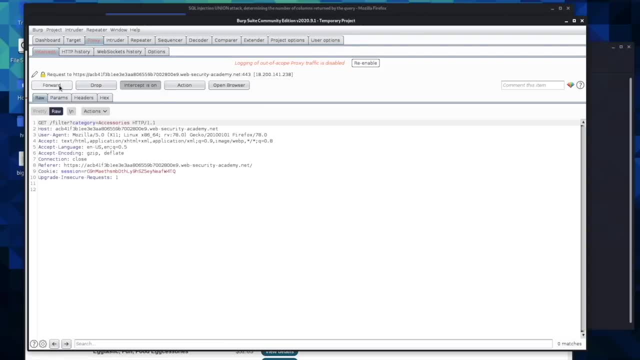 can decide what works best for you. so you can come in here- and I actually want to first give you a chance- I'll show you kind of what we're looking for and see if you can find it on your own. so you can come in here, send one of these to your repeater and see if you can find the. 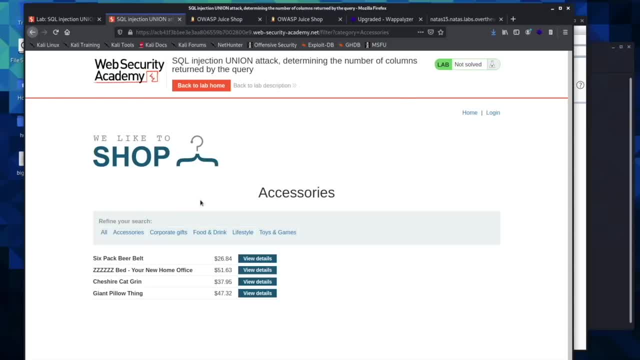 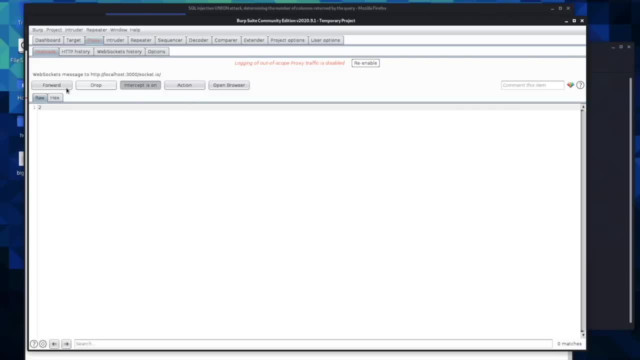 sequel injection without any help, and it's okay if you haven't- we really haven't covered this a whole lot, but in the coming videos we'll be able to do this multiple times over and over, and so you'll get the hang of what we're going through and what we're looking for. okay, I'm going to send. 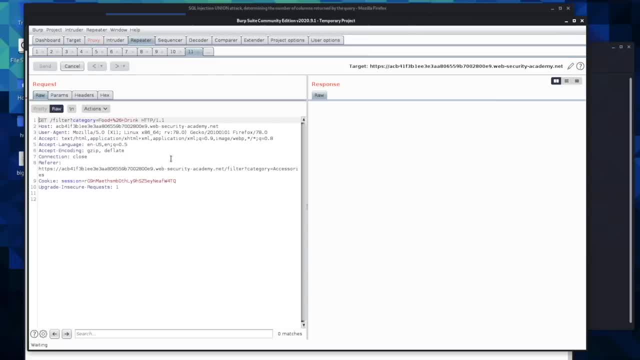 this to the repeater. I'm not actually sure where the sequel injection is even at. I think it will try right here. okay, that's what we're looking for. it is going to be right here, and so we're looking for this right here. this is what I was talking about in the last video. 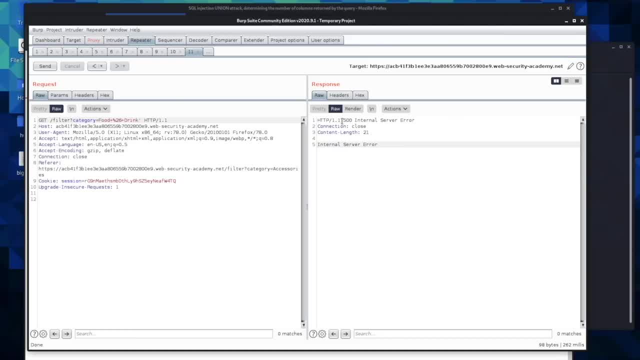 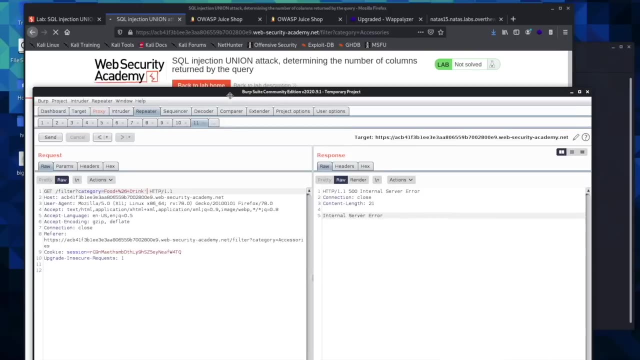 the internal server air. if you can produce this air, what you should immediately be thinking is there's going to be a sequel injection here somewhere. it is here somewhere. you just have to figure out how to exploit it. challenge actually tells us to do is we're looking. 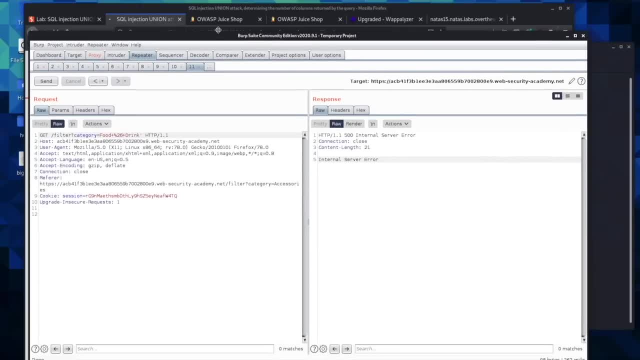 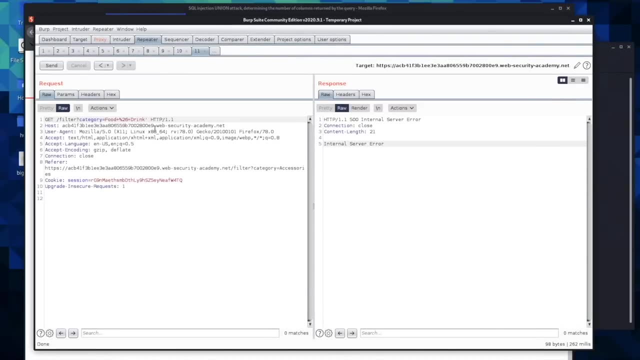 for the number of columns returned, and so we're trying to figure out how many columns are on the specific table. and so, if you think of an Excel spreadsheet, you have rows and then you have columns, and what we're trying to do is figure out how many columns exist on the table and when. 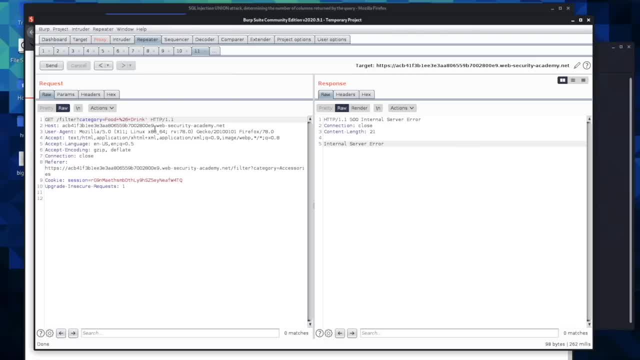 you're doing a sequel injection. we're going to be looking for passwords as we go through the port swigger program, but there are a lot of other things you can look for and we're going to get to those and exactly how to find them, even though you're never really going to. 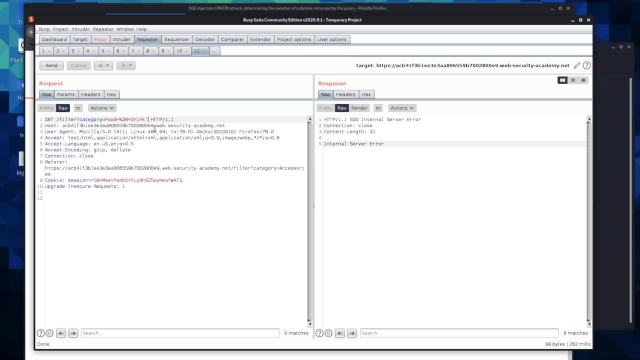 pull down actual information on a bug bounty program. I wanted to walk through as someone who doesn't know how to program and sequel what to do if you come across a capture the flag and you're trying to find specific things such as usernames or flags or passwords, and so we'll get. 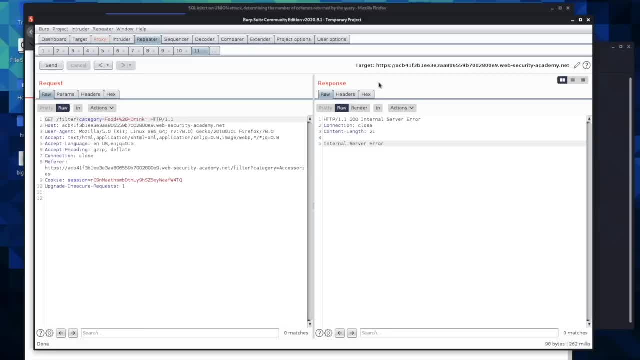 to that in the coming videos. but now we have produced this internal server air and so we know we are looking for the number of columns using the union attack. so we have our single quote which breaks the query, and then we type in Union and because we are sending this request, we have to send a plus for the space if you don't have the. 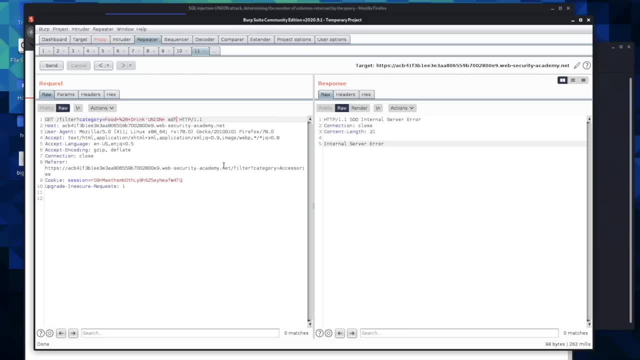 plus in there, or, and you actually put a space in, it will break what we're trying to send. so Union select, and then you put in here null, which is just nothing, and then you send it and it comes back with nothing, and then you just hit comma. 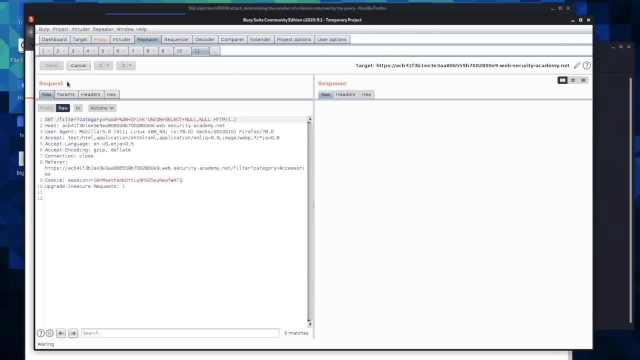 and then you put in no and you'd send it, and it still sends us an error. so we put in no again and we send it. and oh, you know we forgot to do was you have to close out the rest of the query. so in here we have to put a dash dash, so that comments out everything after our statement here. so and then 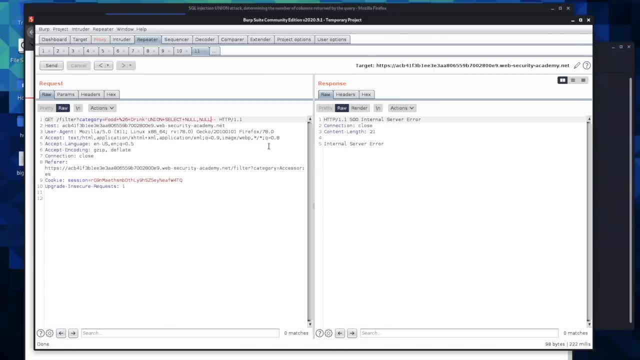 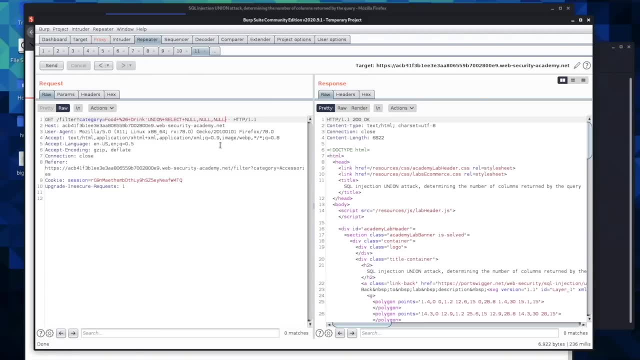 we'd come over here and we'd put in no again and it still says we haven't found the number of columns. and so it hit on the number three. it came back. okay, so this statement would be true. so when the statement is true, it'll send us back a response. 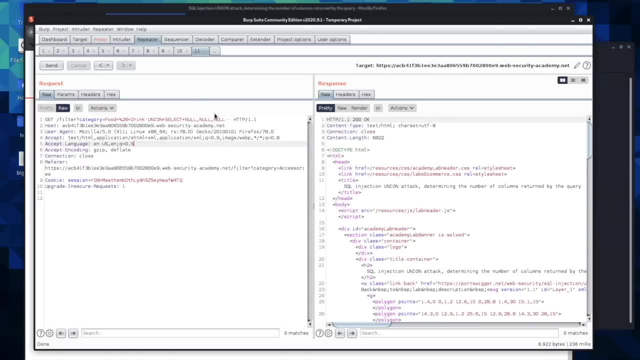 and so we have our response, which means there are one, two, three columns inside this lab. we're working on and, as I said before, notification stops. today's program will be back next week and we're going to sorry. we will continue to update another video. until then, have a great night and have a great sorwoo. 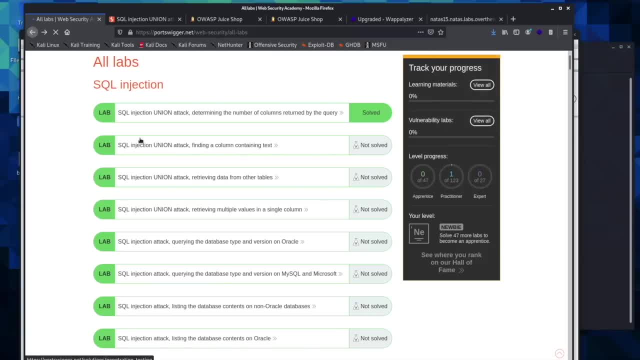 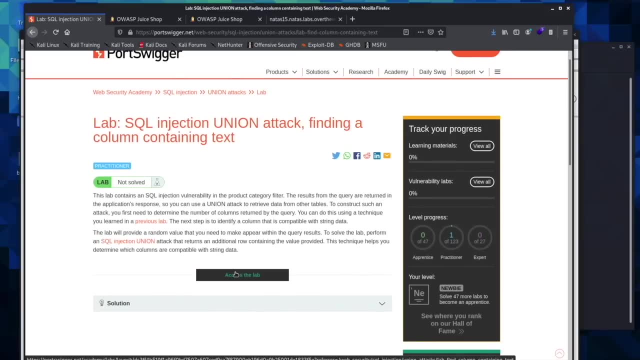 bye and, by the way, as you can see, this video was made possible by a Paola, and I'll see you tomorrow. come into the next one. we'll read the instructions and we'll work through it. what i would like for you to do is go ahead and open up the second lab and click access to the lab, and i want you to go. 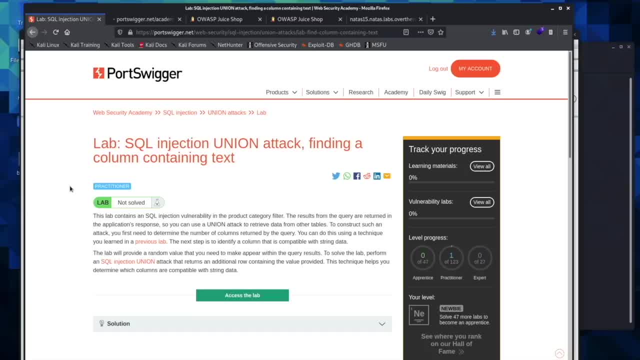 in here and do exactly what we did last time and see if you can remember how to find the number of columns in a sql table. so you can go ahead. you can open that up, see if you can find it and then, if you want to try and figure out how to find the columns containing text, you can google around and 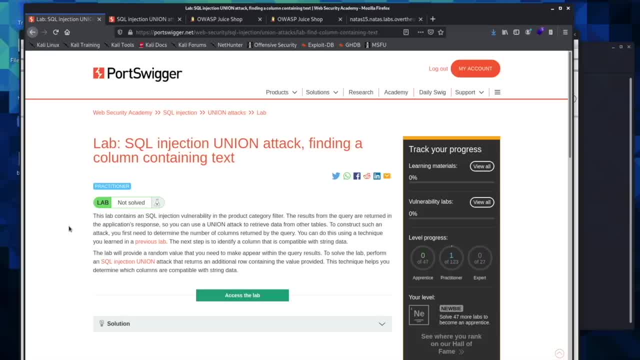 see if you can figure it out. if not, we're going to work through it now and you will have the opportunity to practice finding columns containing text, as well as continuing to find the number of columns in a table in the future. so this isn't your only chance to try and practice this on your 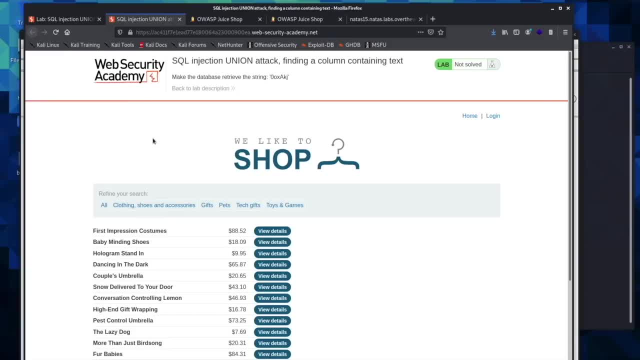 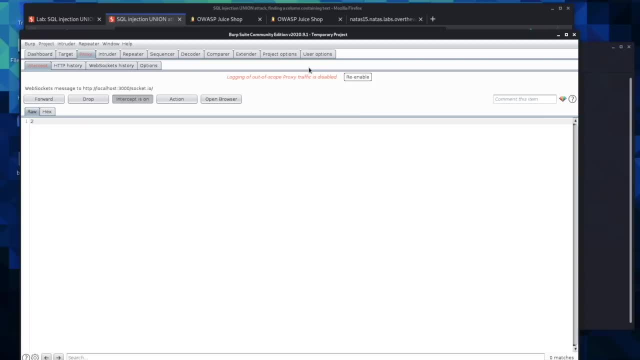 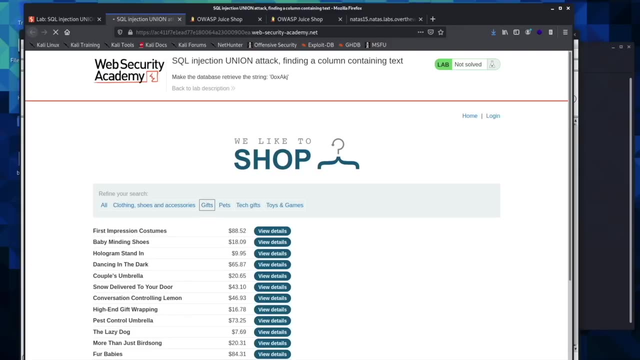 own. okay, if you are able to pull down the number of columns, then you have figured out or learned what we went through in the last lesson, but if not, we're going to go ahead and work through this one again. so we'll come in here, click on one of these tabs and we'll have a request sent, a get request. 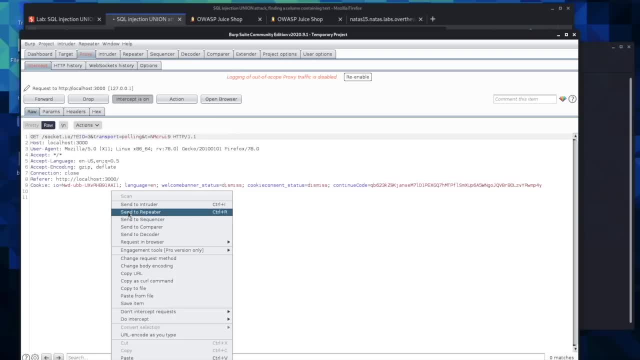 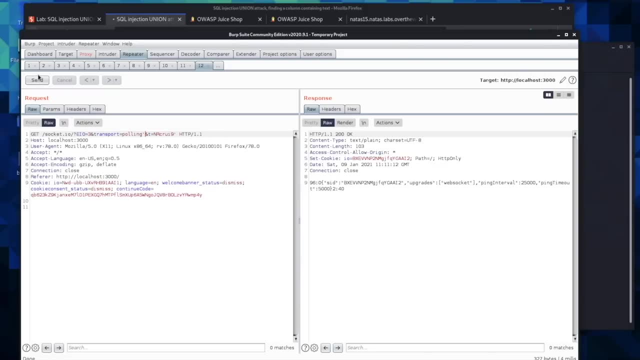 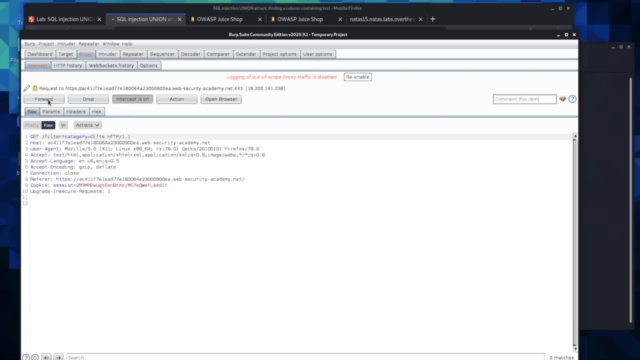 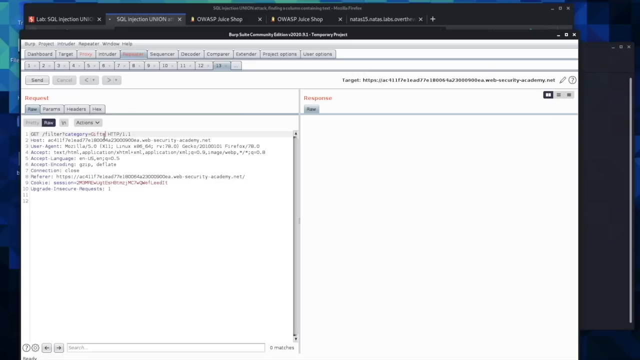 and then we will take it and send it to repeater. see if we can find a. an internal server error might not actually be in this one. let's see, there it is, send this one. so we'll send this to repeater and put in our single quote. 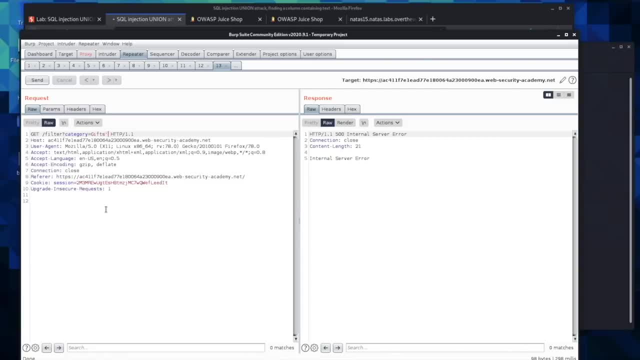 there is the error. so this is where our injection is going to be and so, if you weren't able to find it, you can go ahead and from here and see if you can solve the challenge and pull down the number of columns in this lab. so you can go ahead and give that a try. now, what we do here, if you remember, is we: 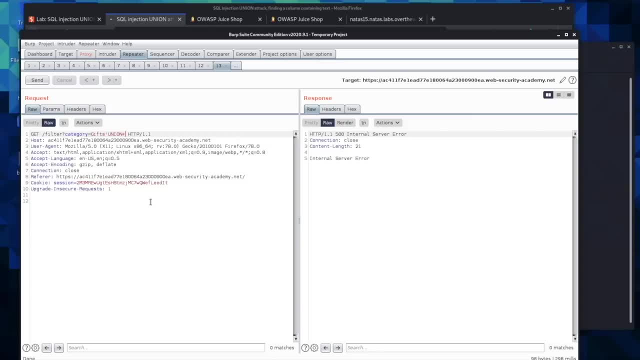 type in union and our plus, then we select and then we have our plus and then we type in our first null value for the column and then we comment everything else out after the request is sent and it says we still have an error and so we try this in. you actually don't have to. 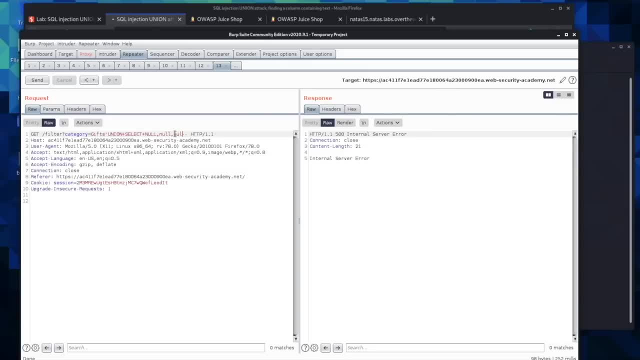 have these in all caps. it's just kind of common practice, for what people usually do is have things in all caps. i'm not really even sure why. so if you know why, you can go ahead and let me know. so we found, we pulled this down. we found one, two, three columns, and so if you made it this far, 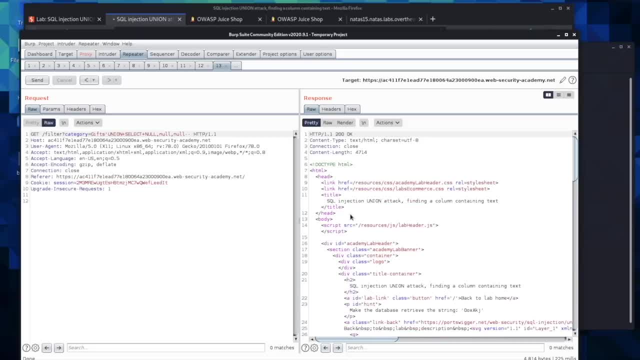 good job, congratulations. you have learned how to pull down the number of columns. but now we're supposed to pull down on which column has text or which ones um take text, and so if you've So you would put in your single quotes and then you put in a string and then send it. 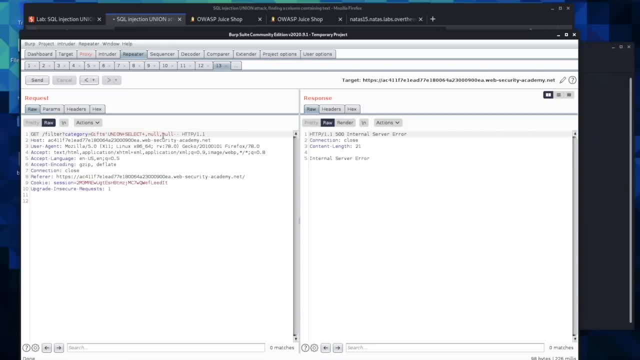 And that one came back as an error. so we'll try the next column- And it is the second column contains text- and we'll go ahead and try the final column as well. Okay, so it would be. the center column is the one we would go after to try and pull down. 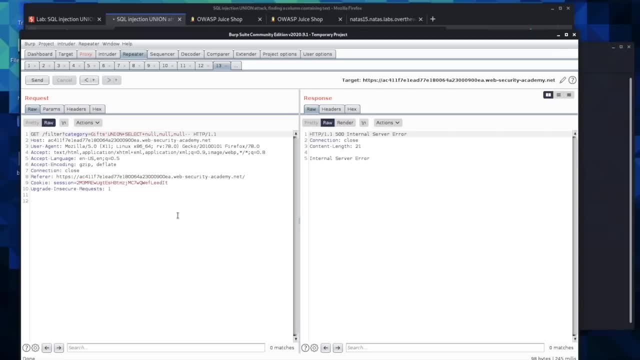 information which is not actually available in this lab, but it is going to be available in the coming labs. So in the next lab I want you to try and go through this, find the category of where you're going to find your error and then try and pull down. union- select the number of columns. 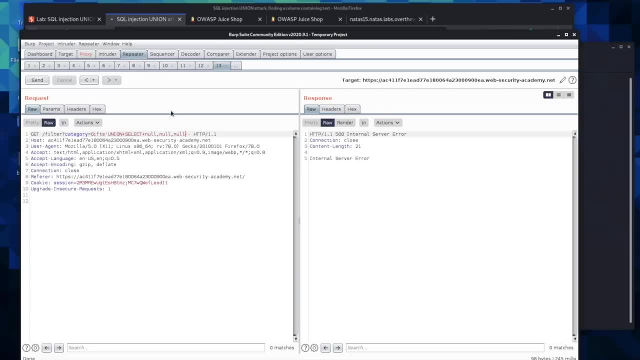 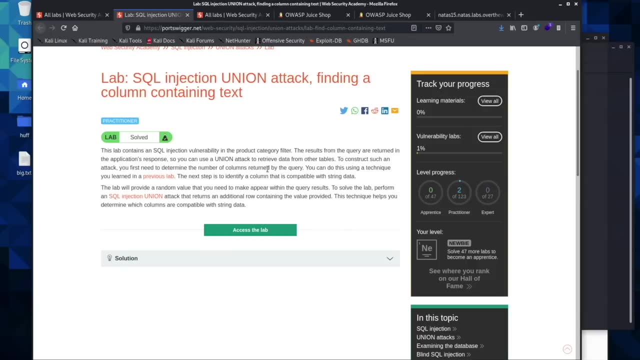 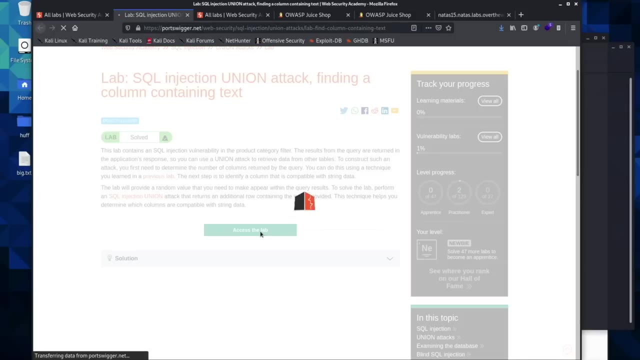 which column contains text And then we'll work through how to actually pull down the information from that column. Alright, I did not notice after I had closed the video that the lab still said it was unsolved. And for those of you that is bothered when a lab goes unsolved, or you want to see them. 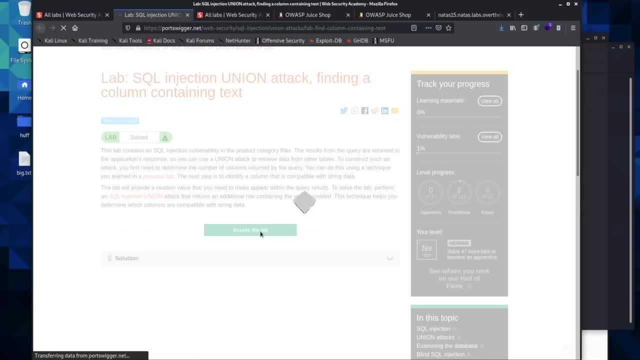 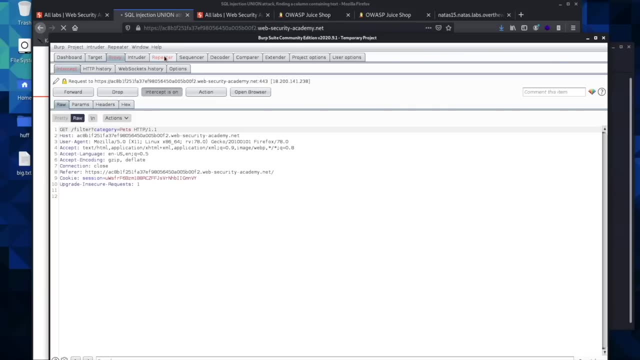 all solved. I'm going to go ahead and do that now. So we'll go ahead and I'll show you. Okay, I'm going to show you where to find that. If you want, you can go ahead and try and find it. 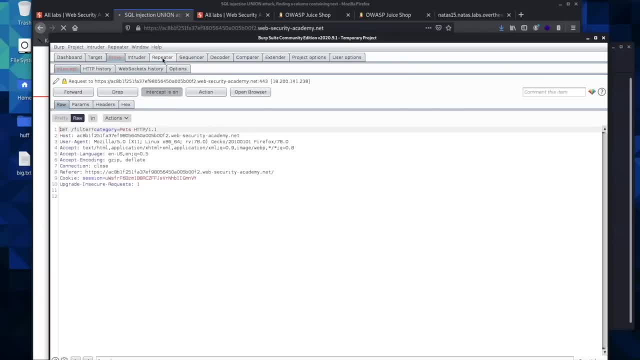 I actually think this is a good challenge. I think you'll be able to find it. Just go ahead and go into perform the SQL injection, Find the one that contains the string and then look through the response and read through it and see if you can find the answer to solve the challenge. 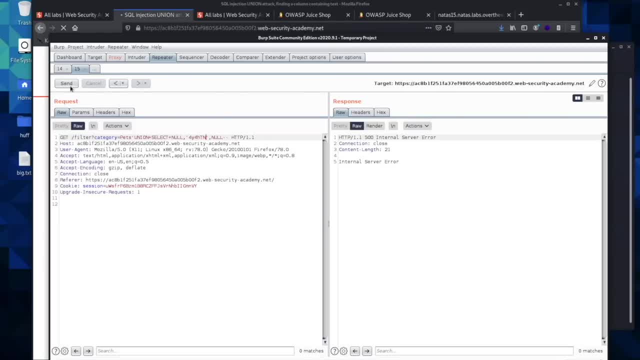 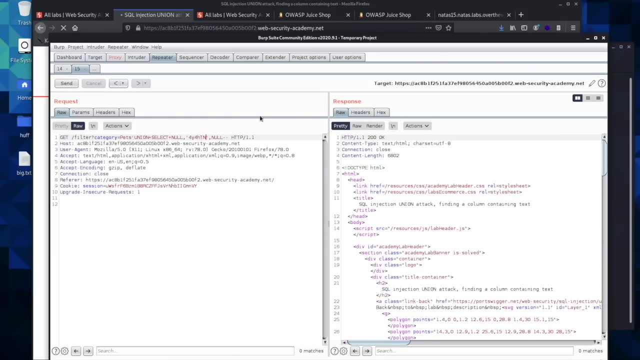 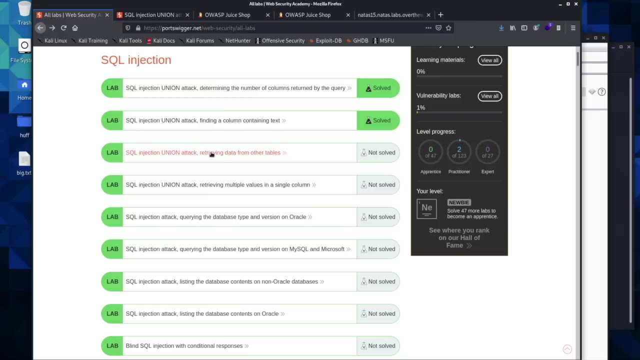 This here solves the challenge for you. Okay, So now the challenge is solved and I will see you in the next lesson. Okay, we are back with the third SQL injection challenge. You can go ahead and click on it and read through the prompt. 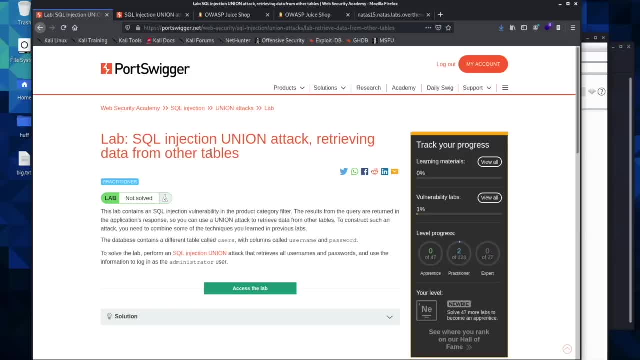 I'm actually going to give you the challenge to see if you can pull down which column or columns contain characters and will accept a string, and then I'm going to walk you through it. I'm pulling down data from the table and then I would suggest practicing so after we go. 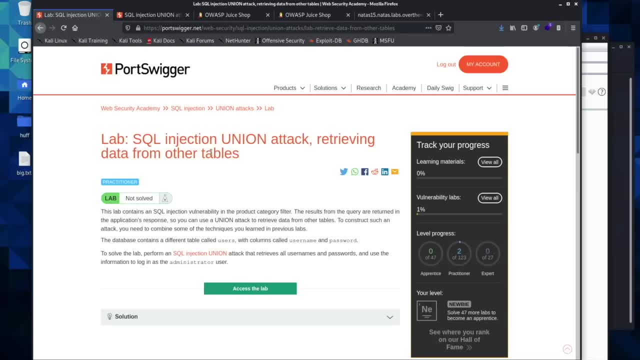 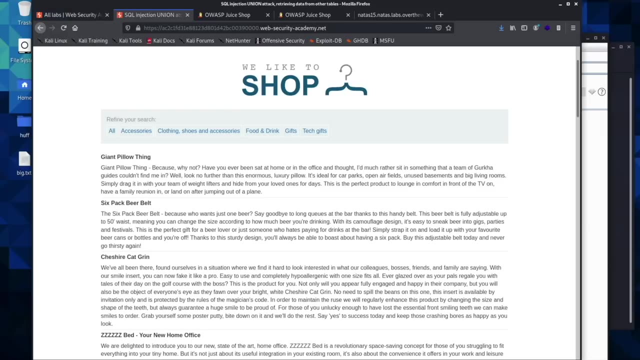 through it on this lab, to try and go through it again without the video before you move on to the next lesson, so that you can continue practicing things as you see it happening. So we'll go ahead and enter into the lab and it's going to be pretty much the same. 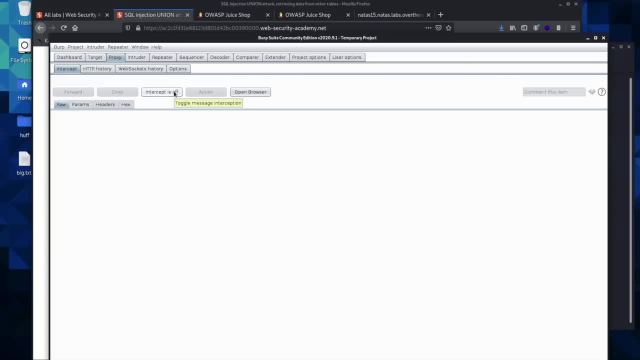 So if you want to go ahead now, I'm going to wait a few seconds- You can pause the video and see if you can complete the challenge and pull down which column or columns that contain a string, before we go ahead and continue learning how to enumerate. 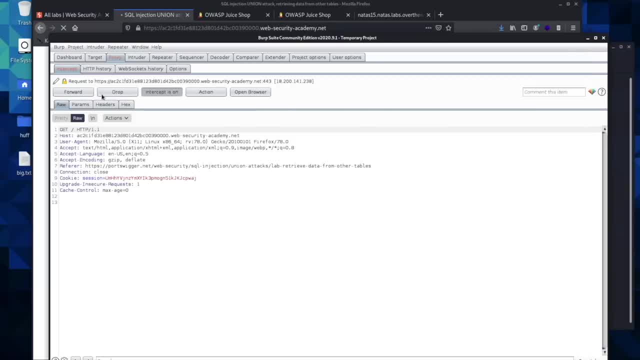 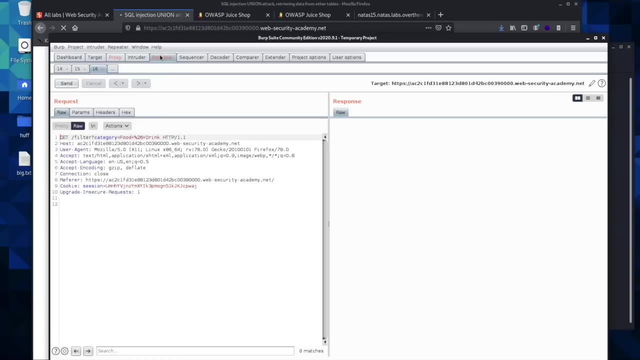 the table columns. So by now this should be pretty familiar to you. We're going to come in here. we're going to look for our request that I apparently asked. Okay, We'll send this to repeater. We'll make sure that we get our internal server error and then we'll try our union select. 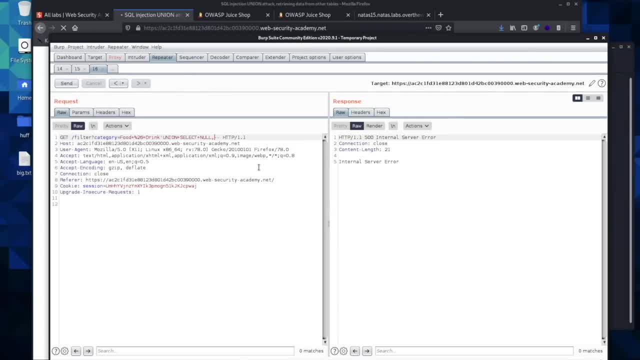 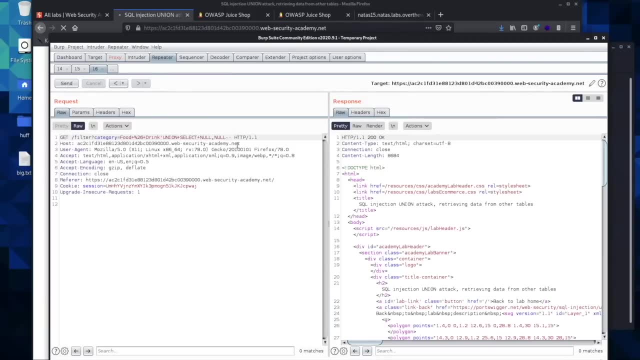 attack and send it and see how many columns we pull down. So there's only two in this lab. So what we'll do now is we're going to pull down. We'll show you the table, So I'm going to show you how to do that. 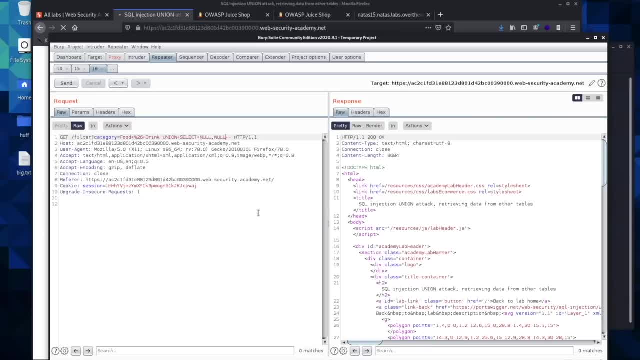 Then I'm going to give an explanation of the best way. if you don't know any SQL, or you don't know how to write any SQL statements, how to find table names, If you find this and it capture the flag and you don't want to go through the long process, 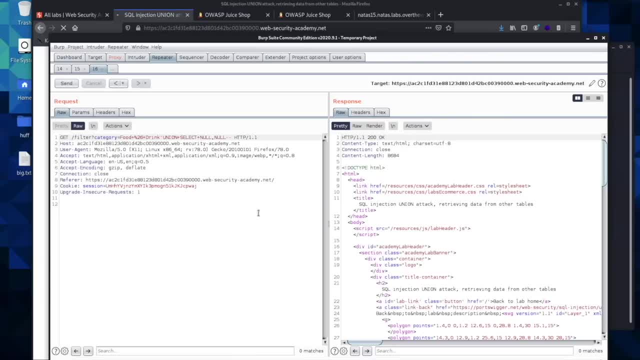 of trying to figure out the table names through writing SQL statements. But before we get there, I'm going to show you. This is what we'll what we'll do. We have two columns. you'll see. check to see if they'll accept a string, and that one does. 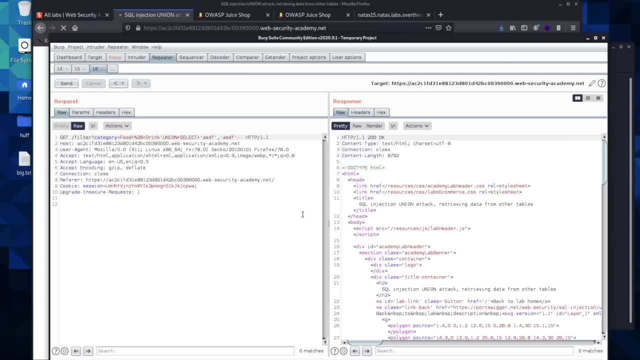 I'm going to go ahead and leave it, and that one does as well. That means there's both these columns have information within them and let's say there was a third column. If we were to write our SQL statement, we would have to include all three columns because the 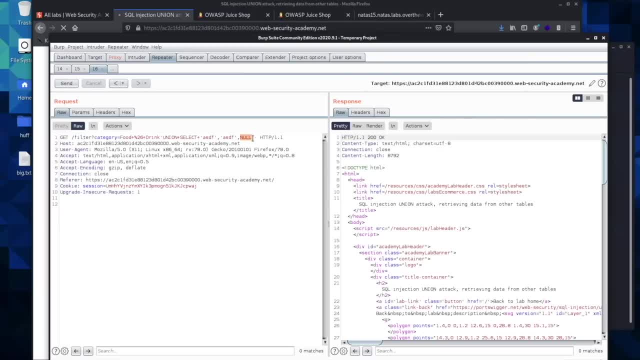 query has to be considered true. You would just leave the the null statement in here- and we're going to see some of these in the coming videos and just to give you an idea that you can go ahead and try and do these, you do null plus username. 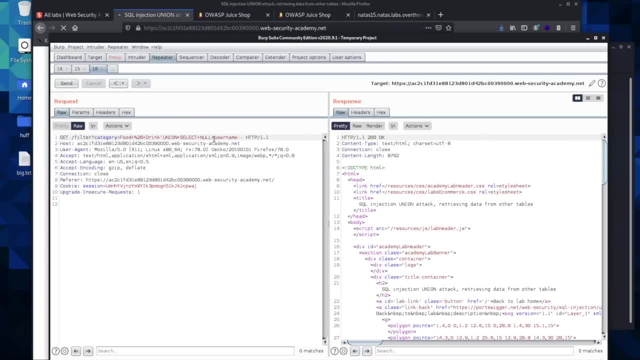 See, this is what you have to do: Leave this as an empty column. but in our case, we don't have three columns, so we're going to Just go with the ones that we do have and the ones that will accept a string, and so we're going to pull down usernames and then we're also going to look for the passwords. 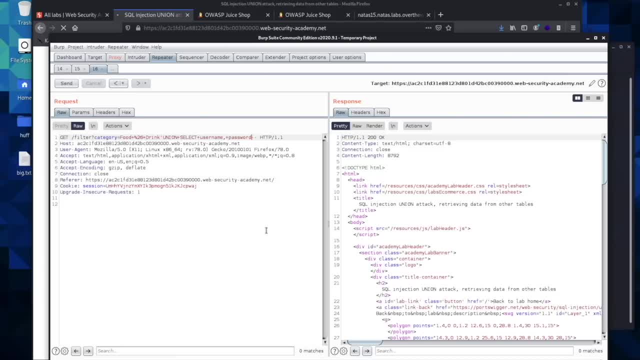 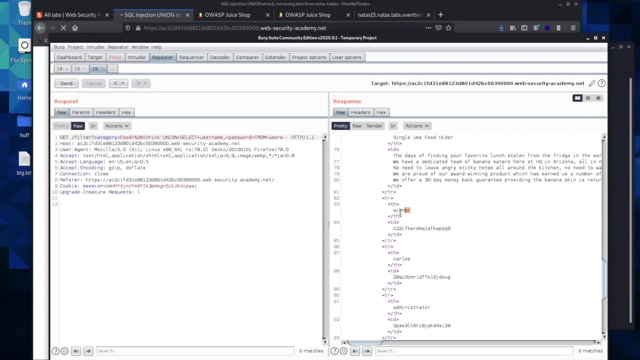 in the table. So we look for the password and this should pull down for us the username and the password from the users table And see: this looks like a user, This, This looks like a password, This looks like a user, This looks like a password and this would be the administrator. 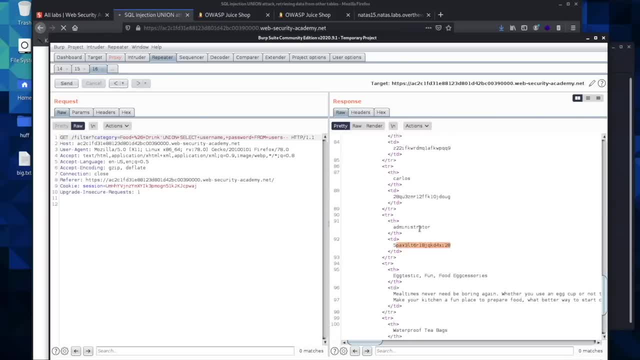 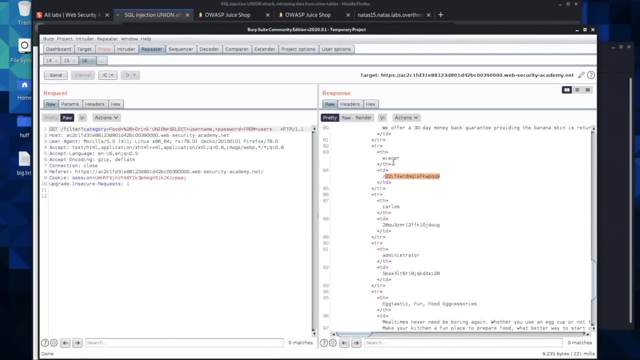 This would be his password. So, in our response, we have pulled down the usernames and the passwords that are within the table and this would give us access. if we wanted to, you could log in as these people. if this was a real website, you would have access to their accounts. 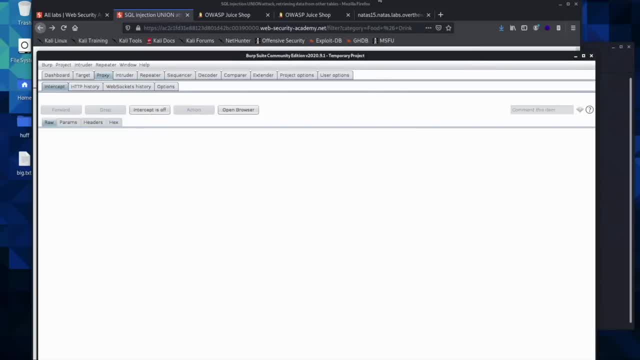 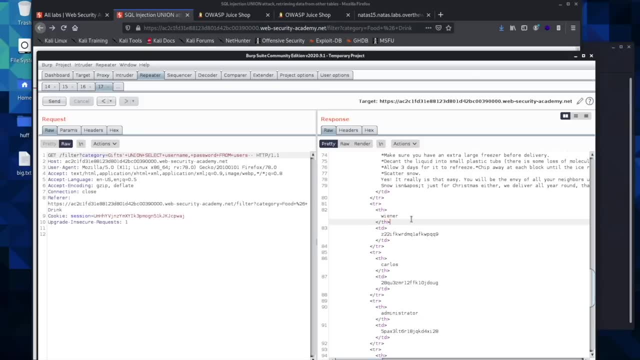 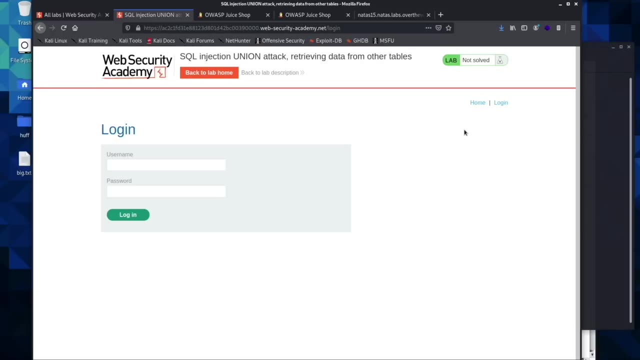 You can go ahead and turn your proxy off so that the web page loads and then you will have the usernames here and the passwords and you can come over to log in and you can give them a try and see if you're able to log in and see if this solves the challenge. 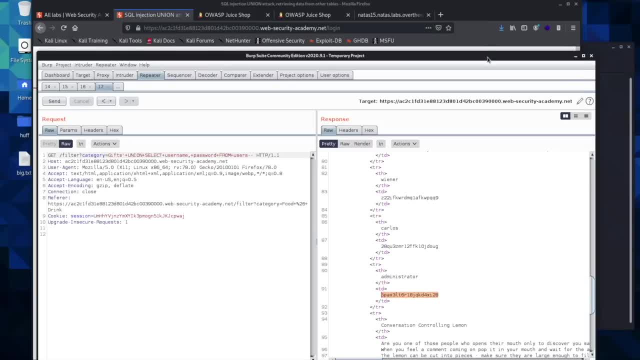 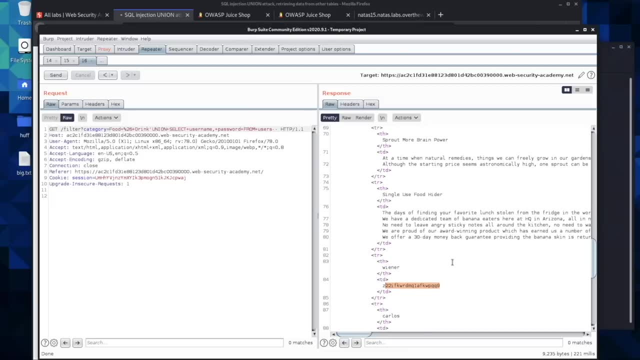 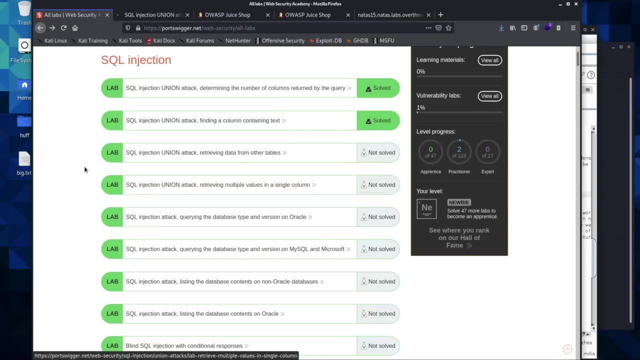 There, that one solved the challenge for us. so with that, I want you to go ahead and see if you can figure out the next challenge without any help, See how far you can get and if you can make it through. and we're going to skip over this. 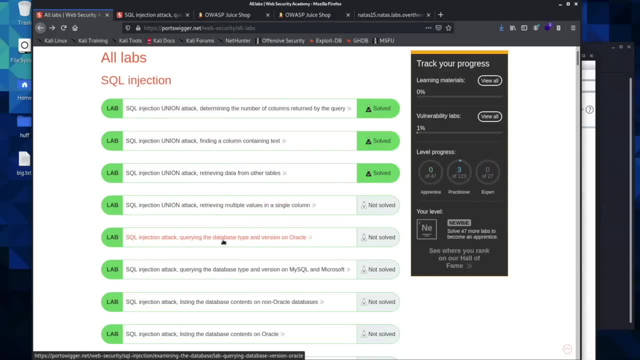 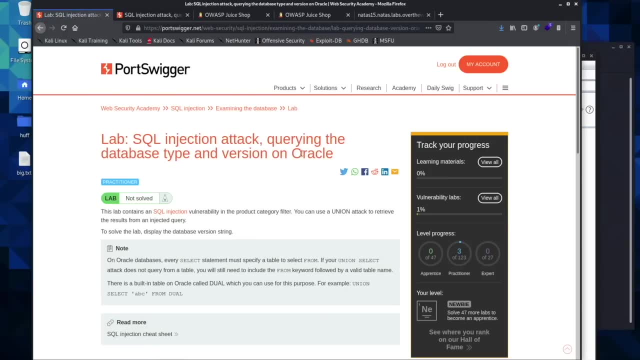 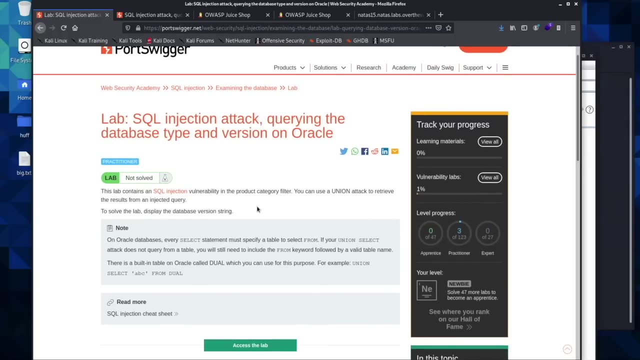 fourth lesson and we're going to jump into the fifth lesson and you can go ahead and open this up And read through it. this time we're going to be in an Oracle database and so we're going to be trying to pull down the version that it is running, and so with this tip we can. 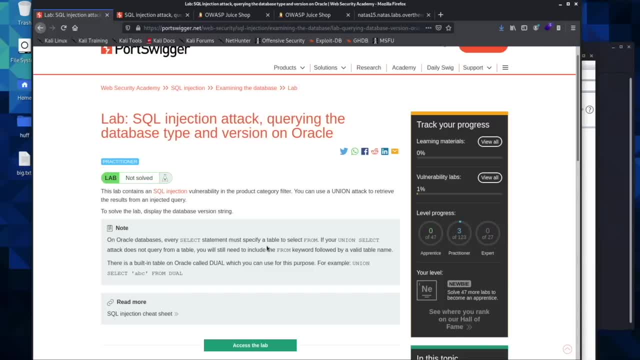 see there's a built in table called dual, so they actually give us the table name this time for us to run through, And I think, with what you've learned so far in the SQL injection cheat sheet, you should be able to Figure out how to solve this challenge. so if you want to go ahead and pause the video, 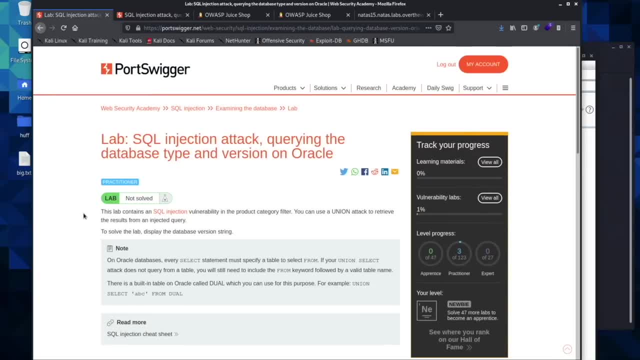 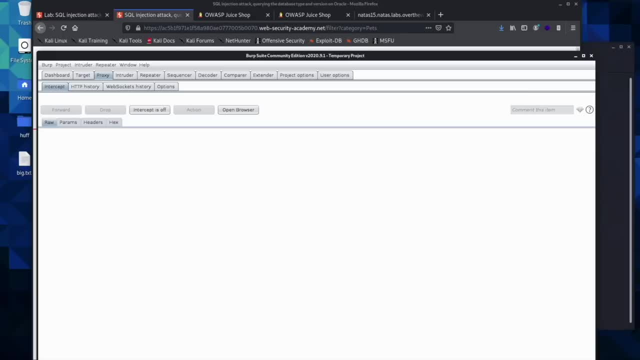 now and try. you can go ahead and do that. if not, we're going to walk through the solution together. so we'll open up the page, we'll go ahead and turn our proxy on- And this should all be familiar to you by now. so we're. 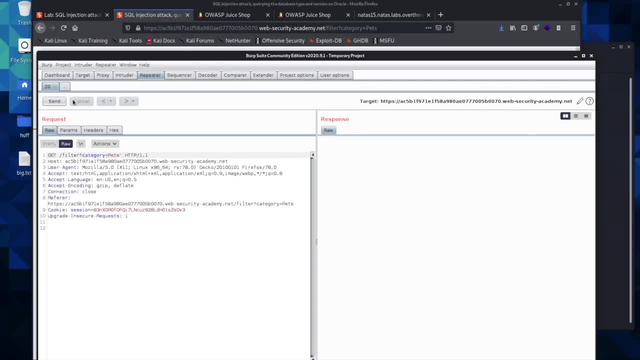 Sending that to repeater. we make sure that we get our Internal internal server error and then we move on just like we have before. so we type in union select And then we'll check for a Single column. but if you remember the table name we were told 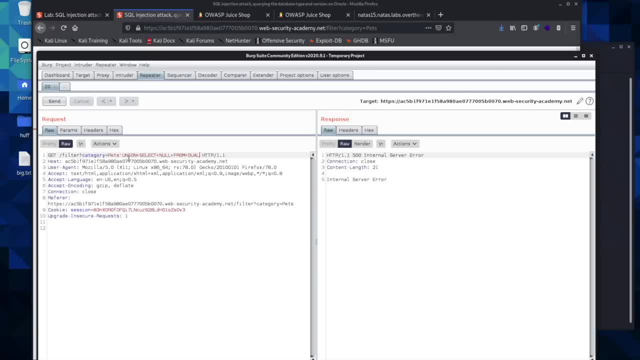 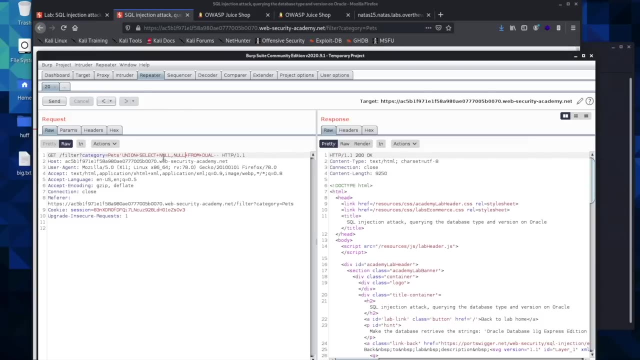 Is Called dual, So we can send that. And we still have an error. so let's try for a Second column. And we see that there are two tables or two columns and the table name of dual, so we'll come in here. 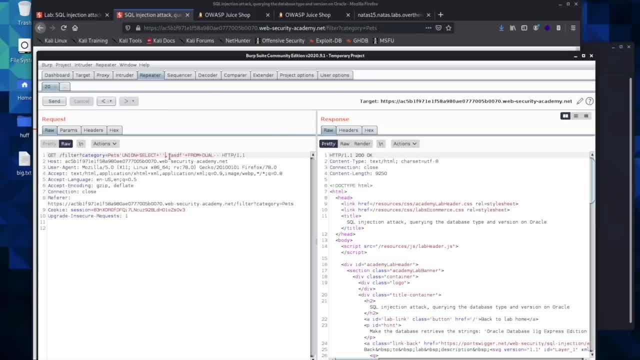 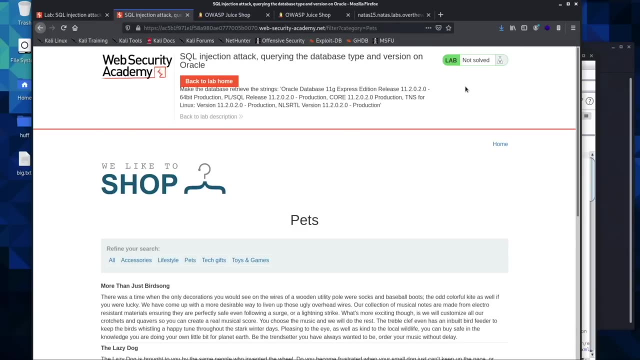 And make sure They receive. they can receive A string And they can. so what we'll do now is we're looking for. if you remember The version name, we're trying to pull down the version name inside the response. So come back to burp. 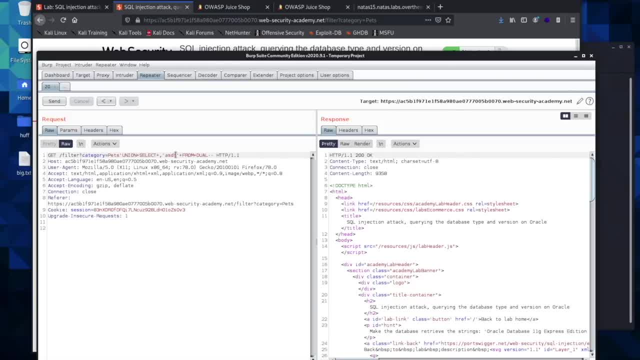 And since these can receive string, we type in here banner And then, if you remember from the previous lesson, if we have multiple columns, they can receive a string And we're not actually going to use one, we have to leave it With Null, so that a way that column receives an input. we just don't want anything from it yet at this point. 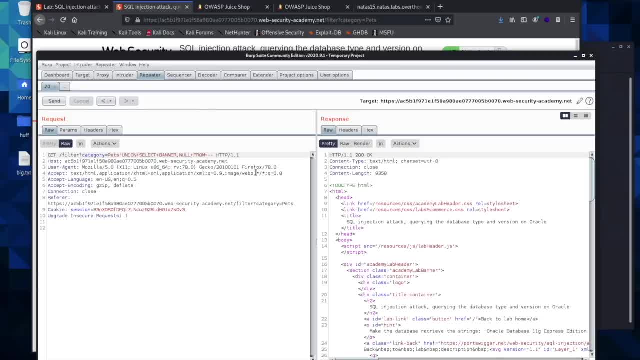 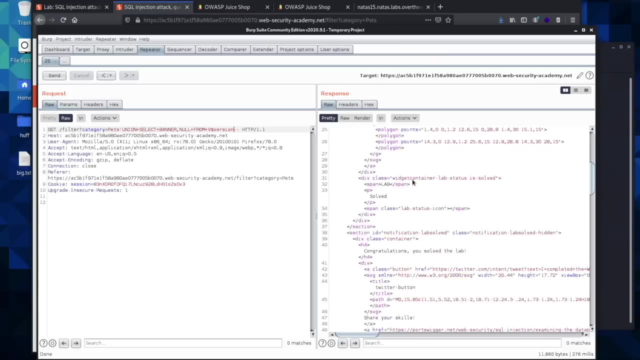 And then for Oracle, the way you pull down a version Is The Dollar sign and then just the word Version. we'll see if that sends it for us. I saw this change In the background to solve. so that gets us our information that we need and so we should be able to. 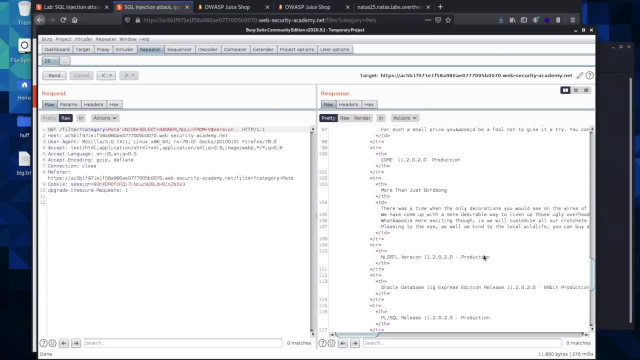 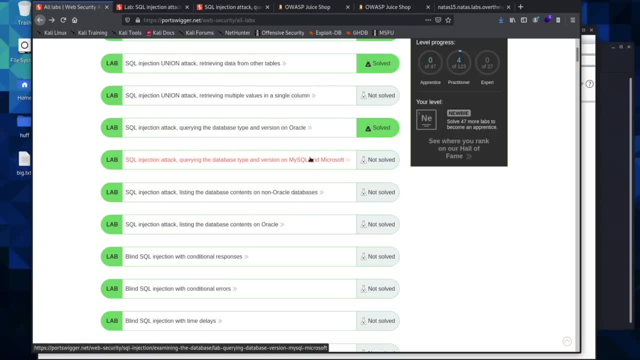 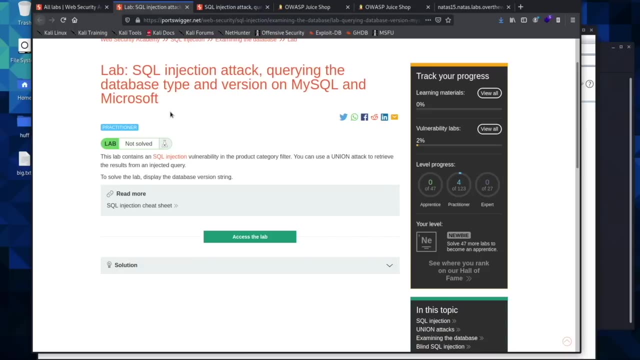 Scroll through here And we find it right, right in here. okay, in this lesson we're going to go ahead and open up this one: the my Sql and Microsoft. I would just go ahead and tell you they are trying to pull a quick one on us because, instead of using the typical 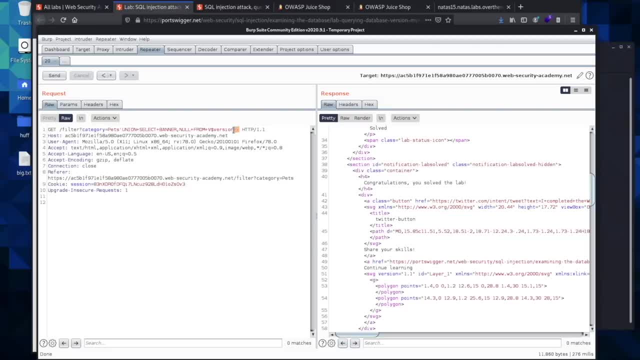 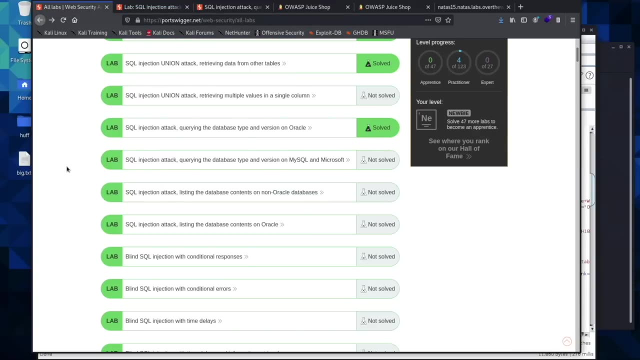 Dash, dash right here that we use and Microsoft to close out or to cancel or to comment out everything After your query you use. you will use a hashtag And that will Stop me. I will come across that and I can sometimes not figure out what's going on and I can spend a significant amount of time trying to figure it out and in the end, 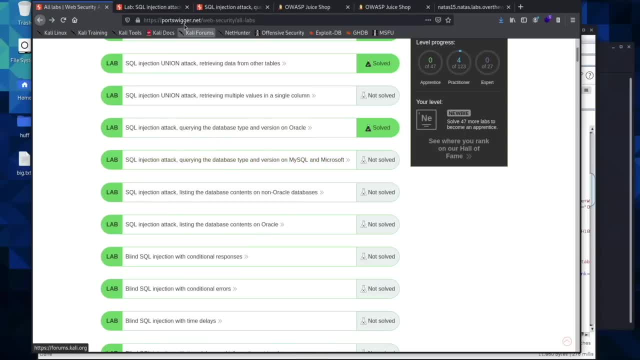 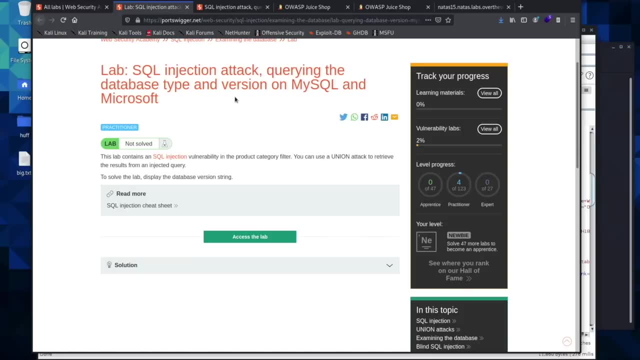 I was using the wrong comment, and so it's one thing to be aware of. and in this lab, We're going to inject an attack, we're going to pull down the type of type and version of my sequel that's being used, and so this is. 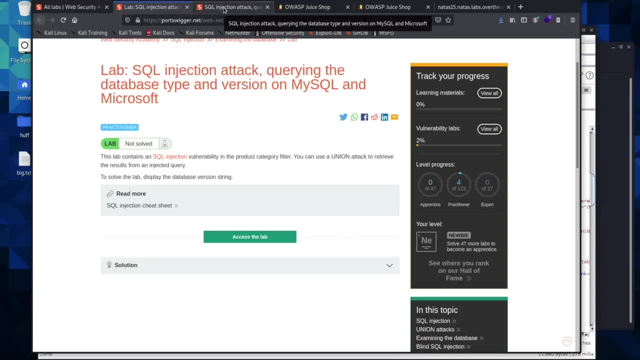 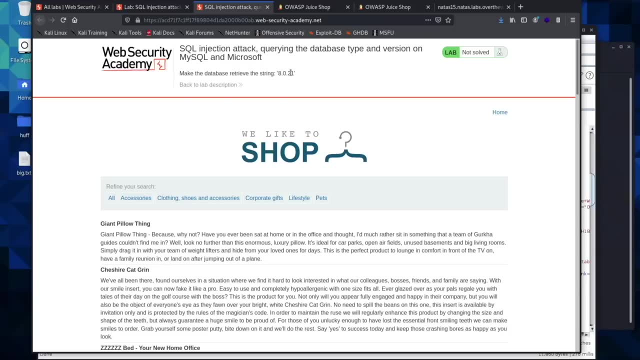 Very, very similar to the last one. and when you go ahead and open up the lab, We're looking to make the database retrieve the string. so I'm actually not entirely sure how to get this to say salt. so we're going to be figuring this out together for, I guess, first time. so 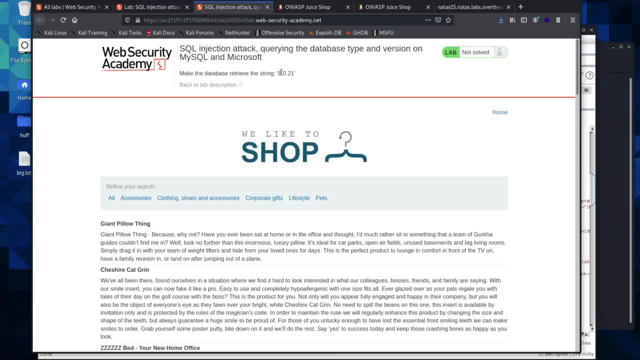 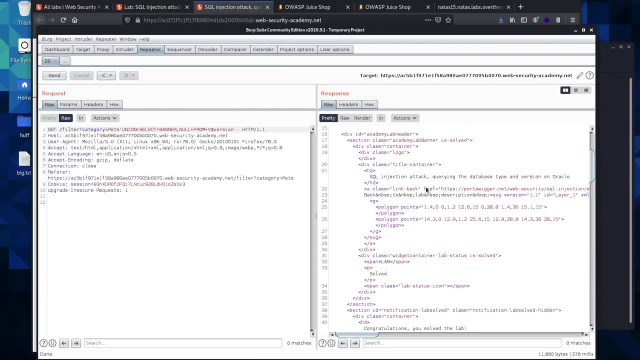 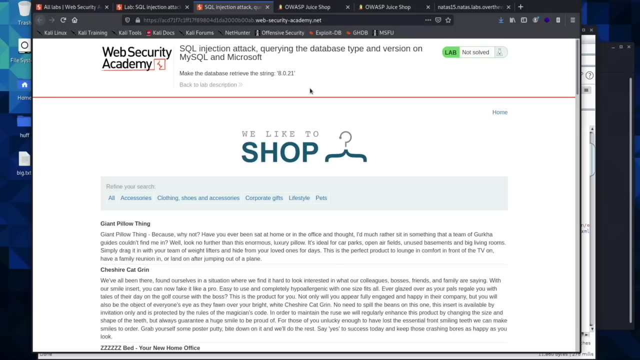 I'm guessing what we're supposed to do is use our union select attack, Pull down the response that we get right here and try and find The version which will look something like this that it's using, and then go back and put it into a string. 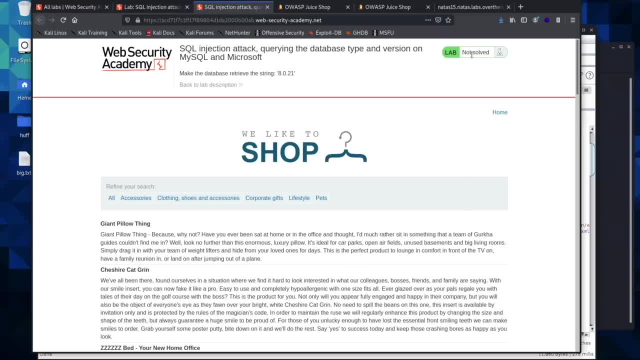 And it should give us the solved problem solved up here. so if you would like to go ahead and give this a try on your own, you can go ahead and do that and I'll give you a few seconds and you can pause the video and then we'll walk through it together. 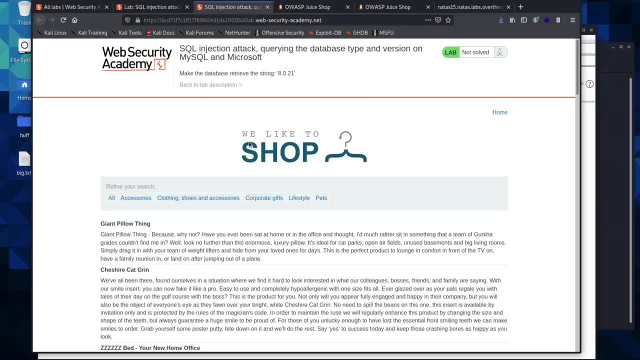 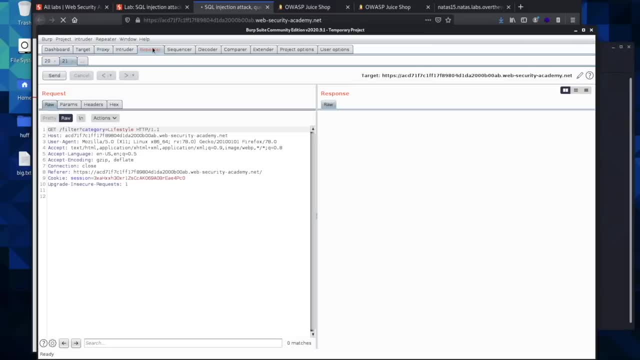 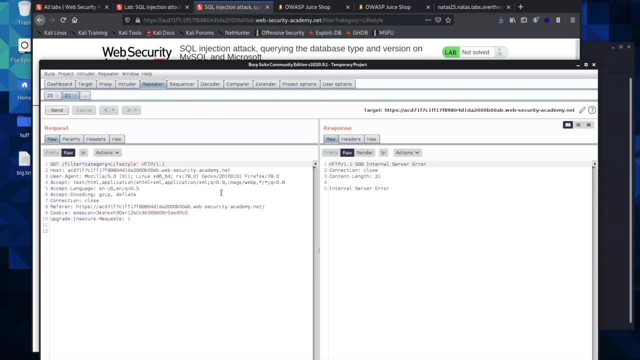 We're going to continue the same way. we have been turned on the proxy. pick a Category, Send it to repeater, turn the proxy off, Lower this so when it comes through a solid we can see. it will see if we get our error and we do. 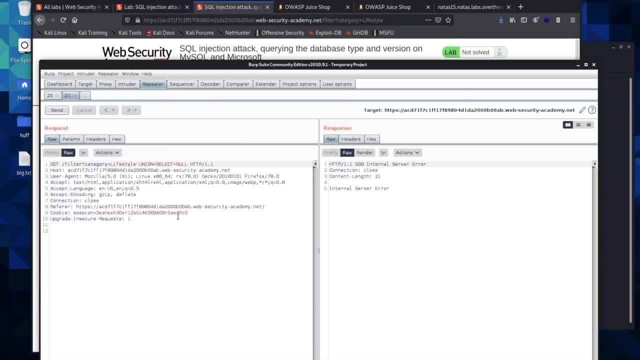 Try it for No. and then, don't forget, the way we comment out is with the hash or the pound symbol- has more than one column. it has two columns. so what we will do is we will make sure They can both Receive a string, and they do. and so the way we pull down the version in Microsoft MySQL is a little different than the way we did it with the Oracle one. 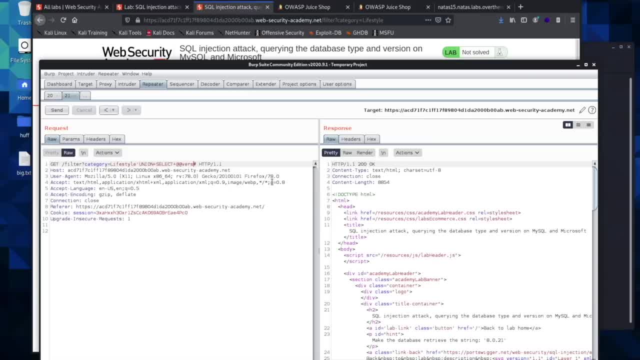 Will go with the two. at symbols, you type in version, and if you looked through the cheat sheet, you would know this is how you pull down the version For Microsoft, and so we do. is we type in no, because you have to have both columns Filled and then we'll send it. we came back with a positive response and so we'll look. 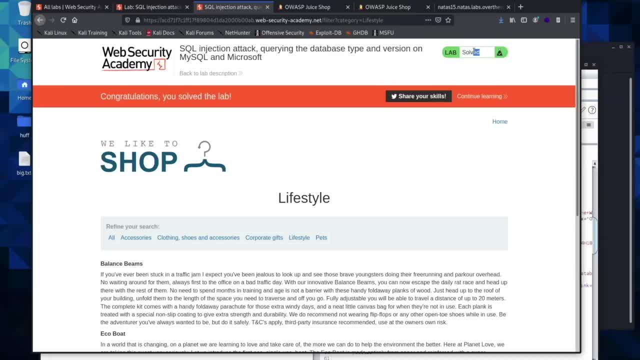 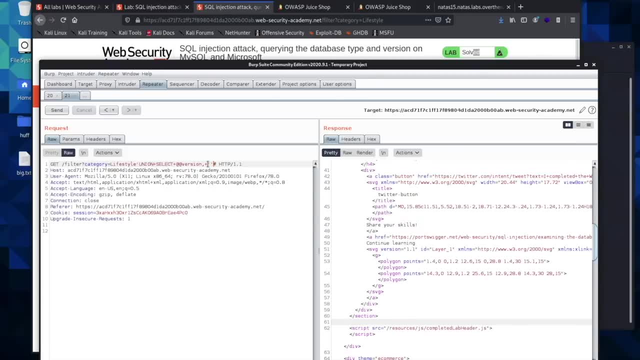 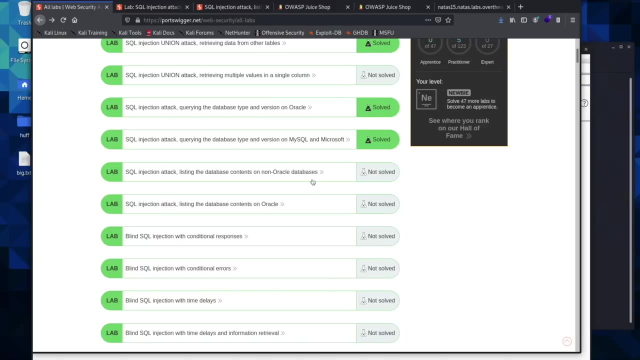 And see if we can always solve it for us. it already said salt. I thought we were going to have to find a version number and send it through as a string Right here. okay, at this point, things are going to become progressively More difficult in pulling down user names and passwords, especially once we get to the blinds. 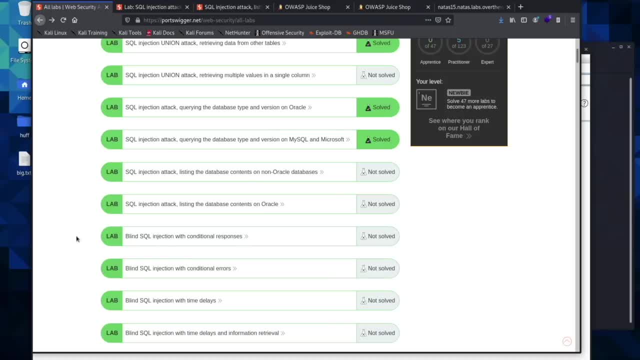 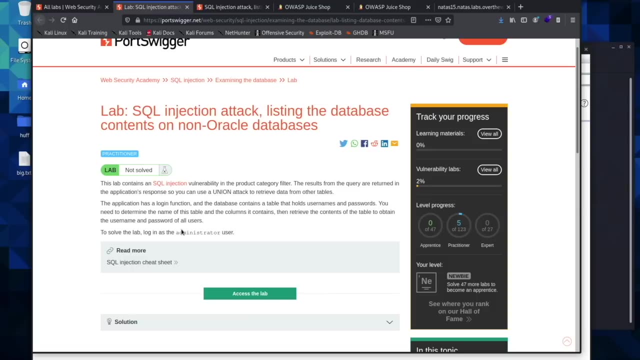 SQL injection, because this is something that we have not seen before, so we're going to be preparing for that by going into this lab right here. You can go ahead and open it up, and we are going to be pulling down the user name and passwords. are going to log in as the administrator. 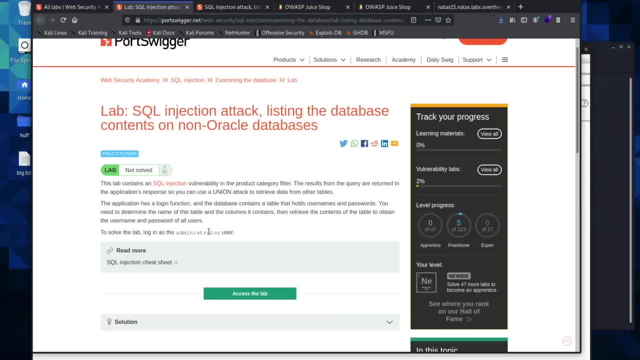 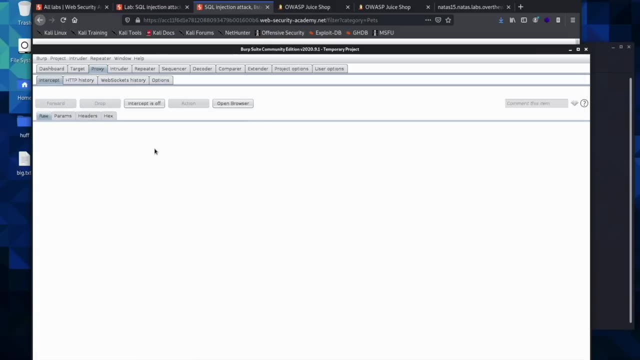 To solve this challenge. I think you can go ahead if you want and practice pulling down how many columns there are And which ones actually receive a string, And you can go ahead and pause and do that if you would like. if not, we're going to go ahead and solve it together, so we'll turn on. 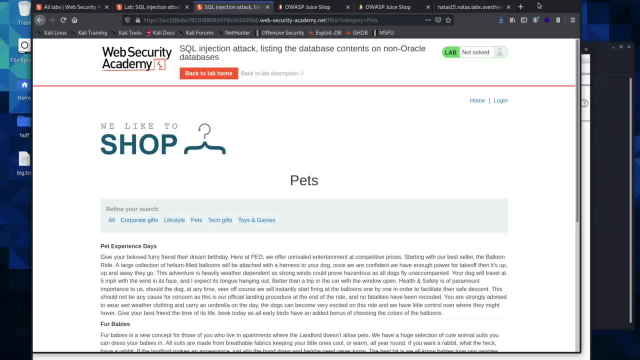 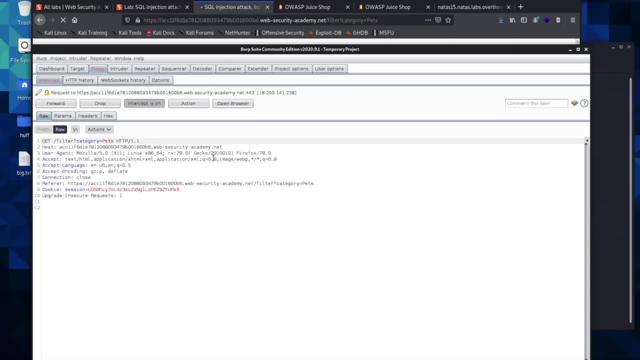 The interceptor, and we're going to be seeing them- new information that we haven't seen before. it's going to seem strange, but I'm gonna do my best to explain Exactly how the SQL statements work- default tables and what we're looking for. so we'll go ahead. 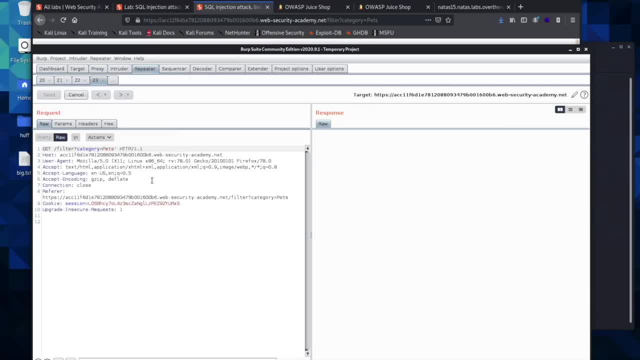 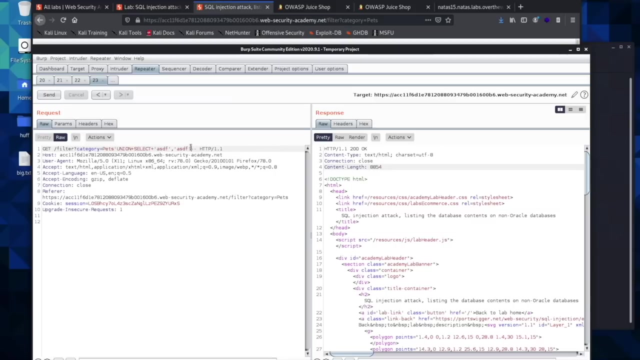 Send that to repeater Off. Send that to make sure we get our error and how many columns there are String and they do so. at this point things are going to be a little bit different than what we've been doing. we're actually going to be trying to pull down some information. 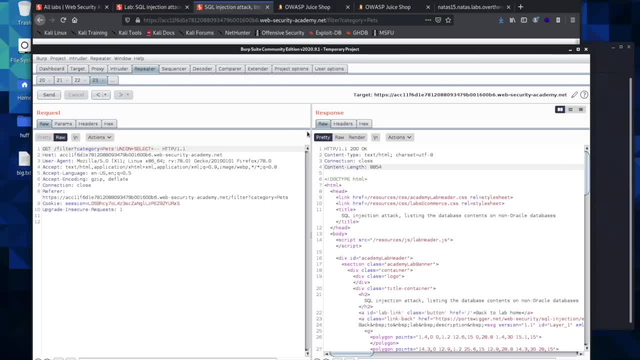 From these tables, and so what we do, The first thing we have to do is figure out the table name. so if we have a grid like an excel sheet, you have your columns that are going up and down, your rows that are going across and the name of the table. the first thing, 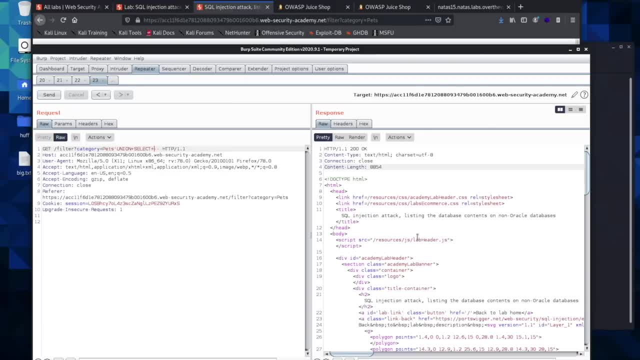 We have to know is the table name in order to request the columns and then individual Cells within the table for us to pull down. they contain the user names and the passwords. So we have our union select and then we come in and we type in: 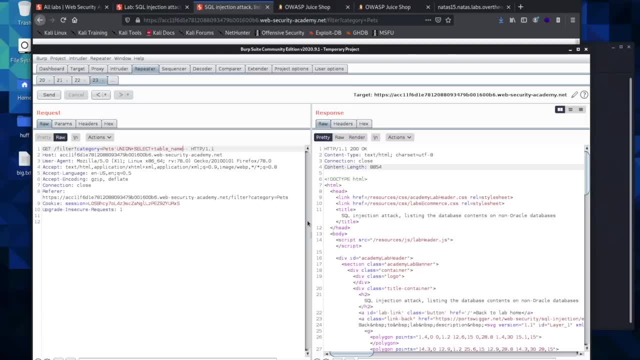 Table name, and so this is what we're looking for. if you remember, we're replacing one of the null values with the table name. Then we leave the second one with the null value, because we're not going to be pulling anything from it just yet. 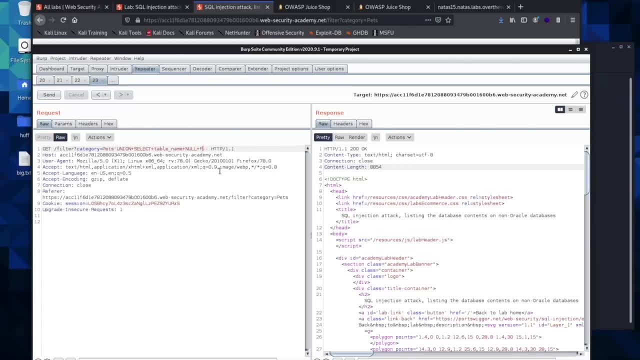 And then we go from The information Schema and this right here, the information schema, dot tables, and this is A default table that you're going to have on every sequel database. so that's how I know this is there if you were to go into sequel. 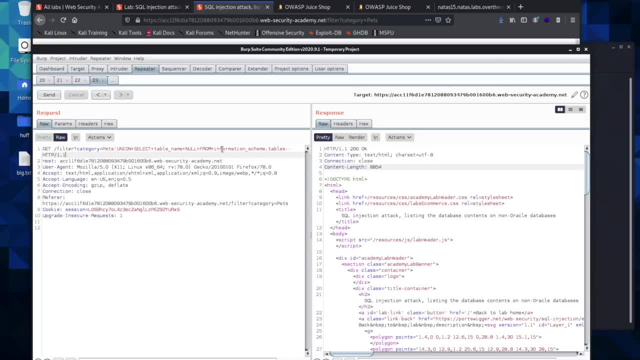 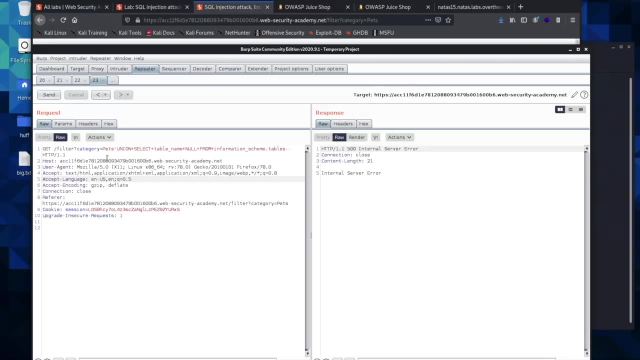 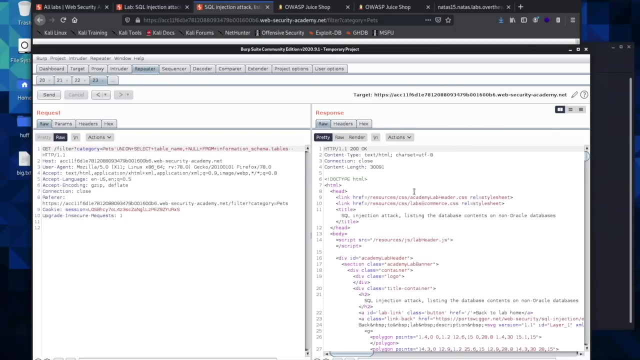 And you would open it up. you're going to have several default tables, the information schema tables. this is default, it's always going to be there, And so this is how we know what to put in for our injection. Then we can Send it and we have an error, which means I'm guessing I have a typo schema. there was my typo and we pull down and we'll look through our response. 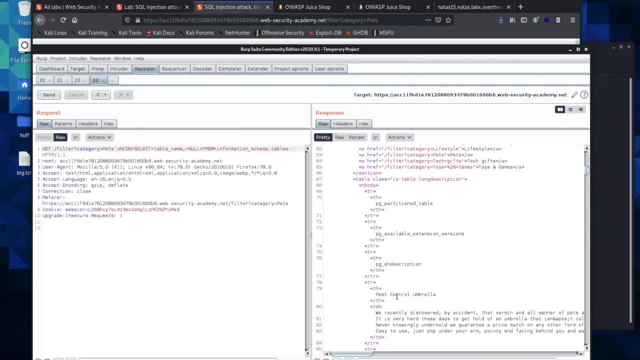 And see the pull down the table names That we have here- and there are a bunch of table names, but if you remember the one we're looking for, we're trying to log in as the administrator, so we're going to need The Users table right here. users, this is the name of users table. I would suggest copying it. 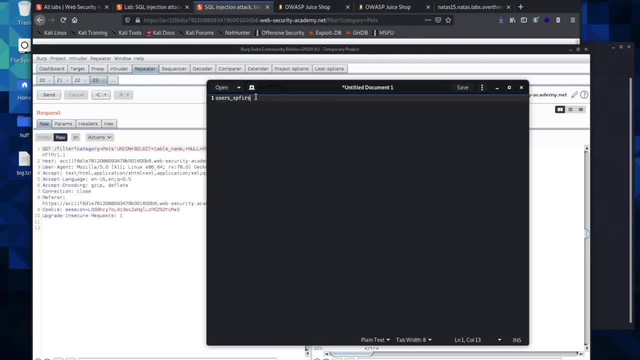 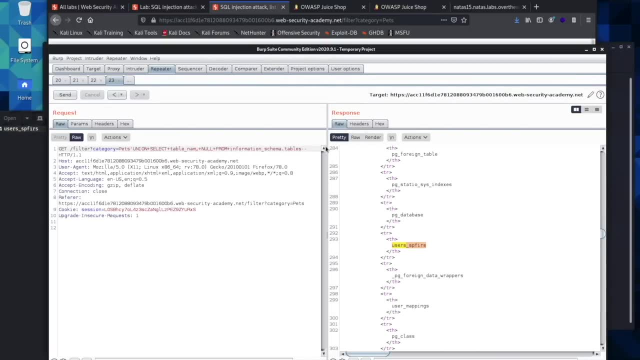 And having a text file open Because we're going to need this information. so now we're going to look for the column name so we can delete this. so the table column is what we're looking for now. So we're going to actually deleted the wrong part of the. 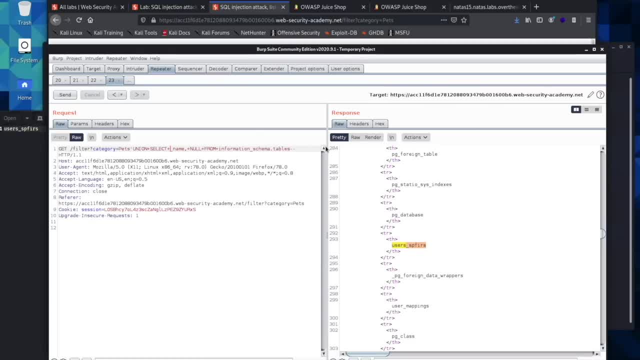 Request. So the table: we're looking for the Column name And we're going to leave this information, schema, Dot, Columns And this Looks right. and now we're going to add to this because now we're looking for the columns from a very specific table. 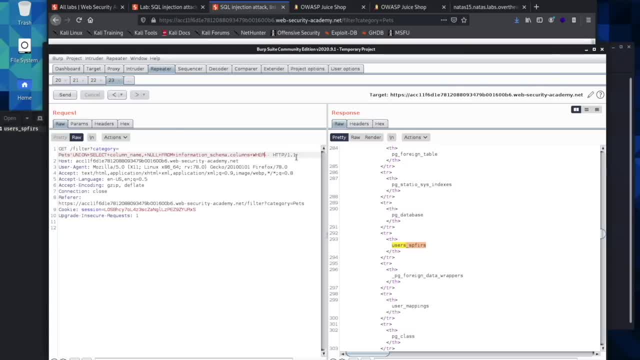 So now we add a plus And we'll say where The table name Equals, And then our users table That we just pulled down. so we'll type in Table name And then we Equals And then our double quotes. 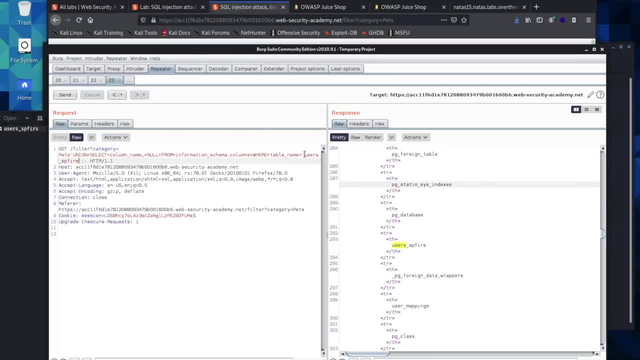 Think I've actually got that copied still- And then we paste in our Users table. So what we have going on Is our union select, so Everything that's coming before this Doesn't really matter. we're adding a query onto it. 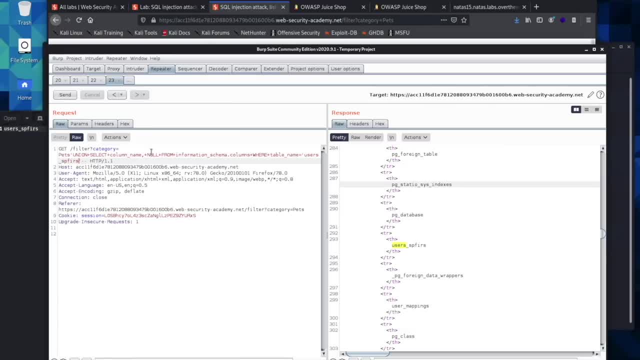 We're looking for the column name. We Have our Second value, Retrieving null, because we're not looking for anything from it just yet, From the information schema, which is One of the defaults Within the sequel database And where we found the table. so now we're looking for columns. 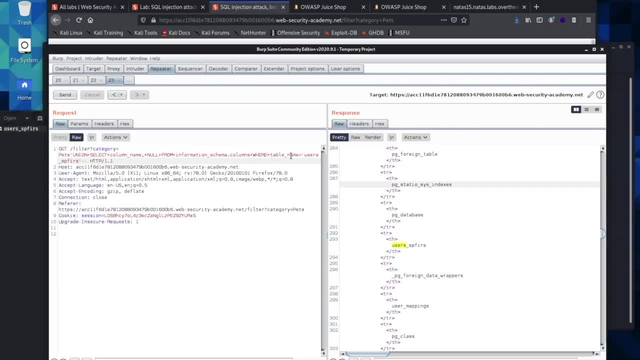 Where The table name. so we're pulling down the table name Equals users. this is going to give us The columns Within the table That is named Users, With some random characters, And so we should be able to send this. 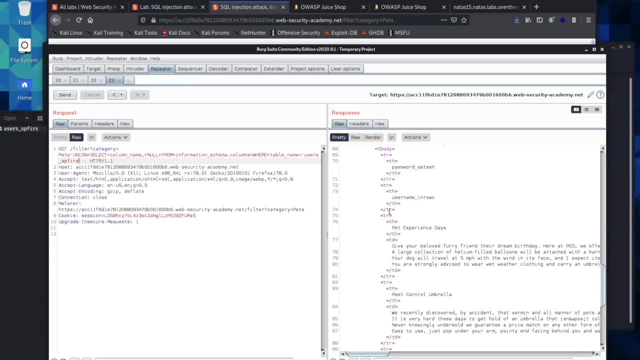 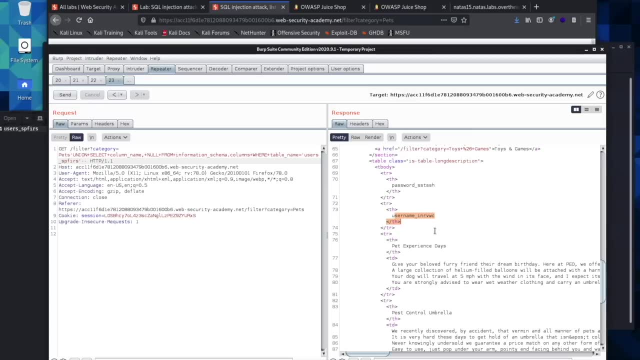 Now we should be able to scroll down And we have Column names, So the passwords column And the Users column, And so now We should be able to change our query and pull down The passwords And the Username. so I'm going to go ahead and copy. 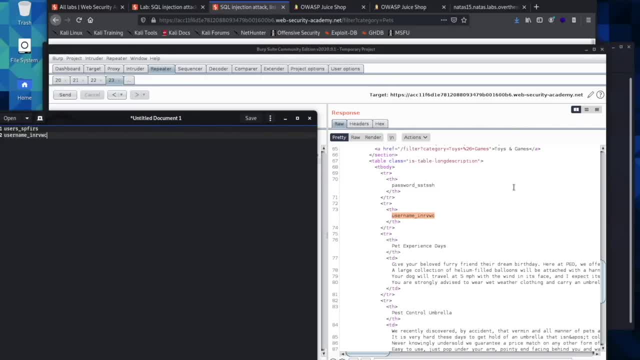 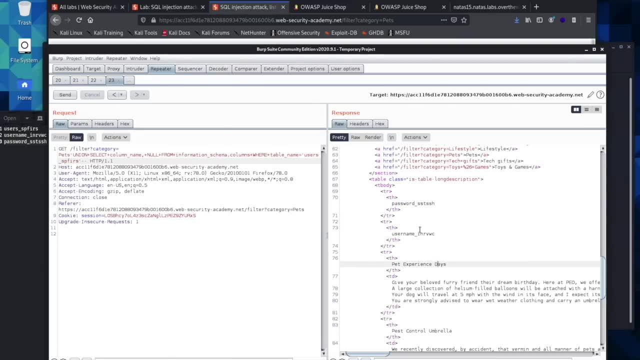 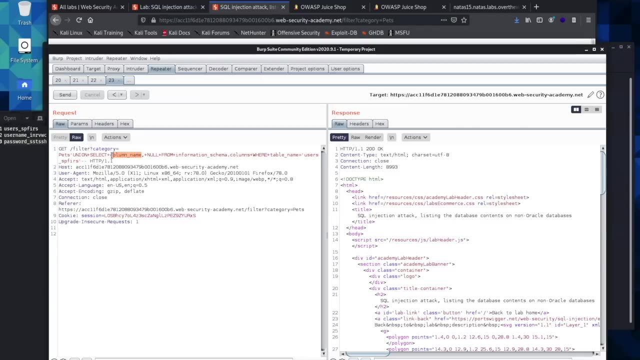 These We have the username And the Password columns. these are the ones That we are Interested in, and now we're going to change Our Union statement. so now, instead of point on a column name, We're going to be looking for the username. 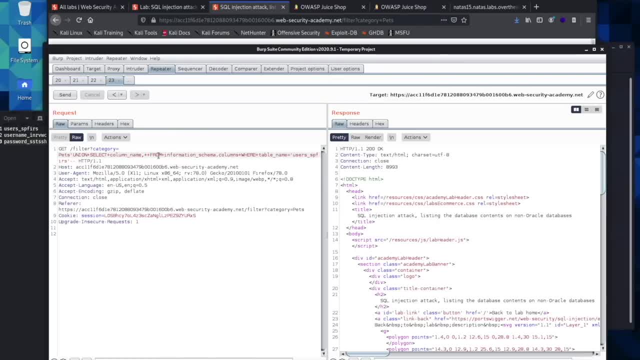 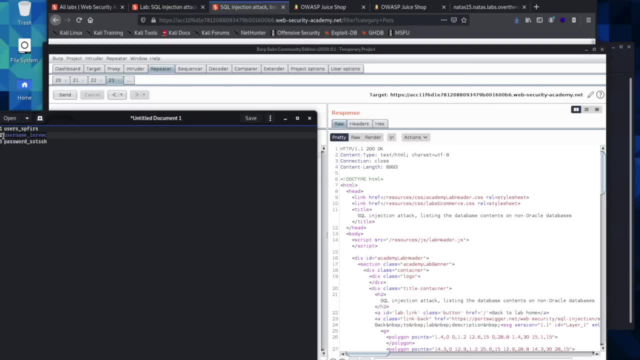 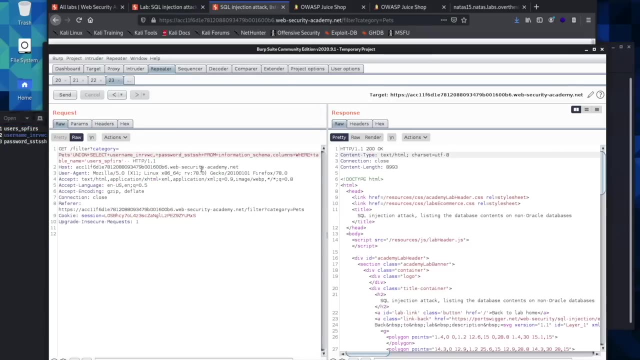 And the password so we can delete our No And we can insert the password Column And here we'll put in the username column In the First slot instead of the column name And we're looking for The username And the password. 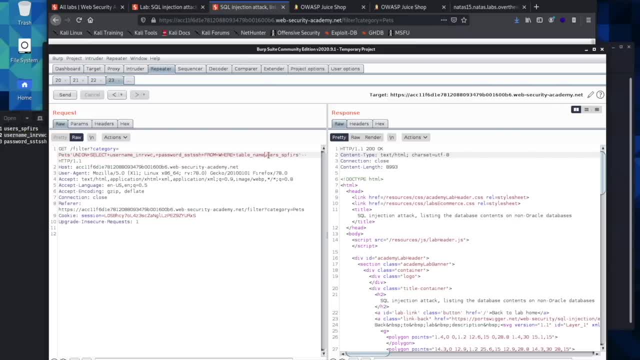 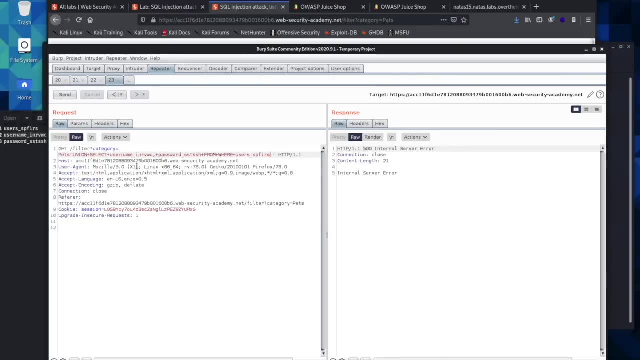 From users. let's see if that Works for us. and it does So, we Should be able to come through now To solve the challenge. we have The administrator and A another user so we can copy you. 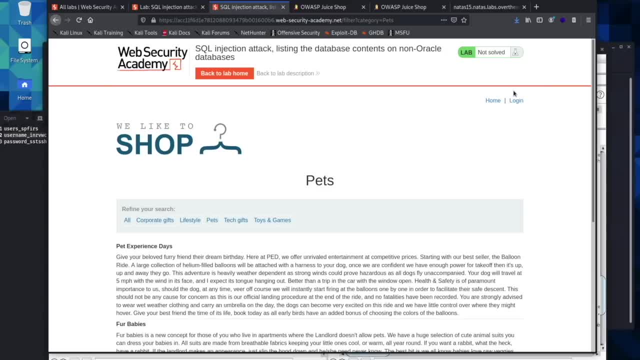 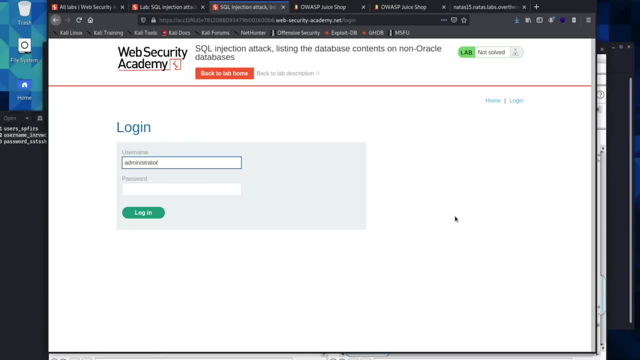 The administrator. We can come back To our lab. remember, to solve it. we have to log in as administrator. We can path in administrator And then we can come back to burp burp and copy our password, and this should solve the challenge for us, okay. 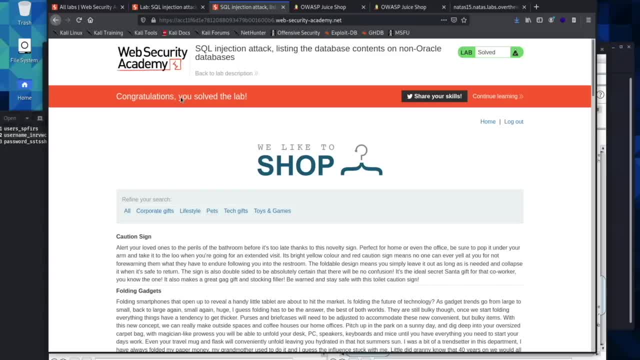 now that was very- I don't want to say- complicated, but it was a big jump from where we have been coming and where we've been coming from, and so, as we get ready to go into blind sequel injections, it's going to become even more complicated. so you might have to go through this lab several times and make 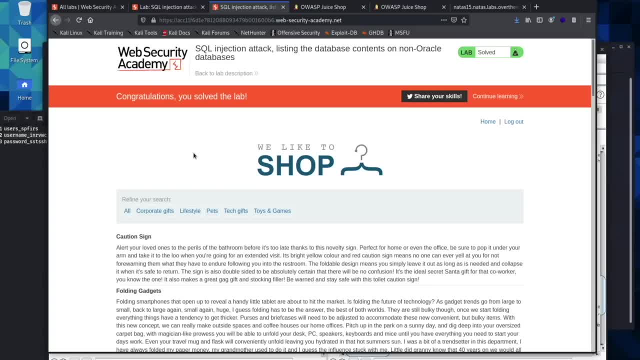 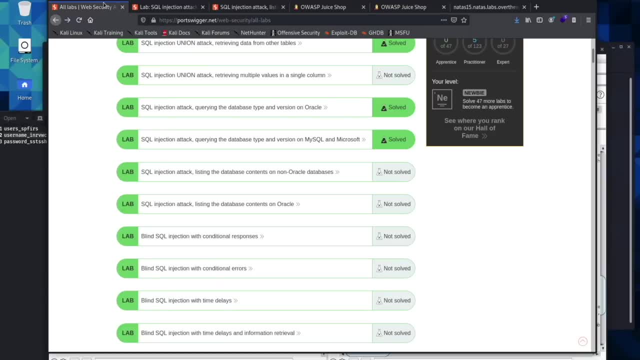 sure that you really understand what's happening. make sure that everything that's built up to this point is working together. the next lab, I believe, is an Oracle lab. okay, so you can try and solve this one. it's going to be similar to the one that we just did, only can use the sequel cheat sheet. we'll go ahead and. 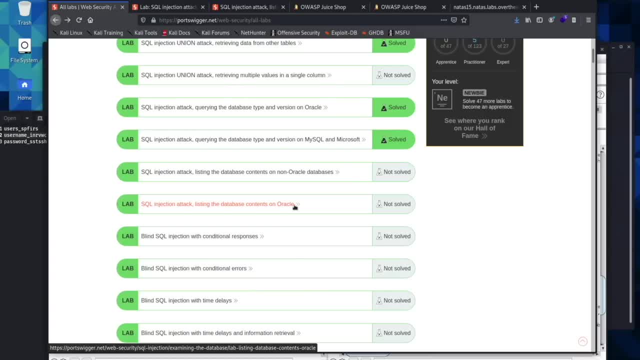 walk through it again, just so we were able to explain why it's so complicated. so I'm just going to go in. we can have one more practice before we get into the blind sequel injections, because these are going to use everything we just learned in this lesson, plus quite a bit more. we're going to be 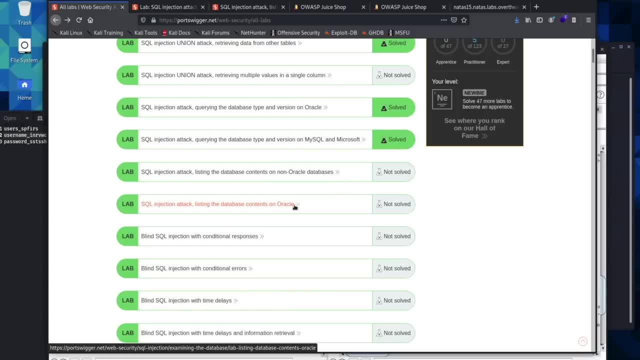 looking at new aspects within burp and exactly how to use the intruder tool within the burp program. so i think it's very important at this point. if i can stress it enough, we're going to have quite a bit of practice going into the blind sequel injection, but it's a lot more difficult than 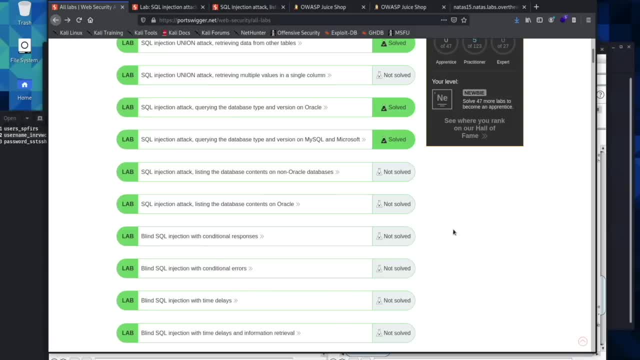 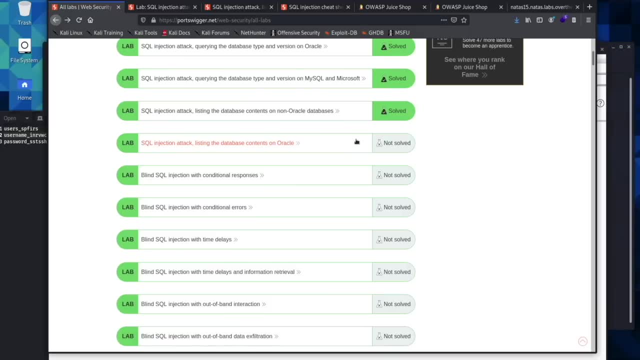 what we just went through. if you've never done this before, so go through this again. if you have to make sure you understand what's happening and what's going on. i want you to try and solve this lab completely on your own. i'm going to give you two clues before you start. but other than that, 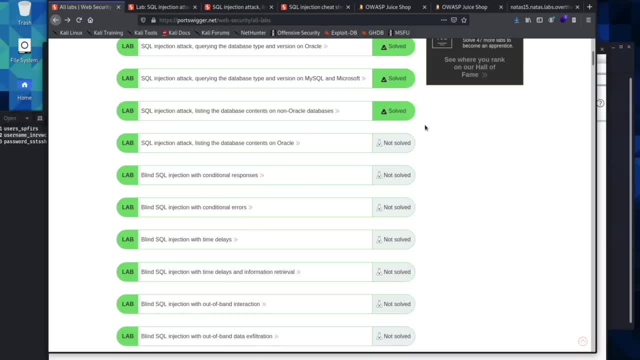 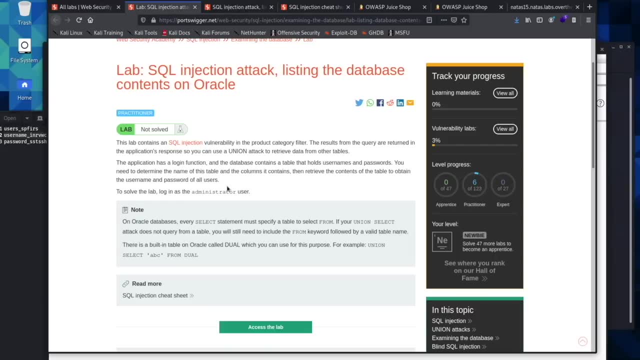 you have already learned everything necessary for solving this challenge. we'll go ahead and open up the lab and, if you remember, when we do go through an oracle database, you have to use from dual when you're trying to pull down the number of columns within the table. and so, since we're looking for 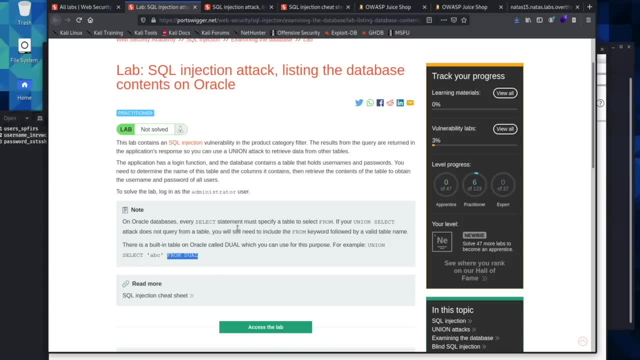 the, we're going to have to log in as the administrator. that should give you a clue to at least how many columns are going to be within the table, and so the other clue i wanted to give you is, if you go ahead and open up the lab and you're going to have to log in as the 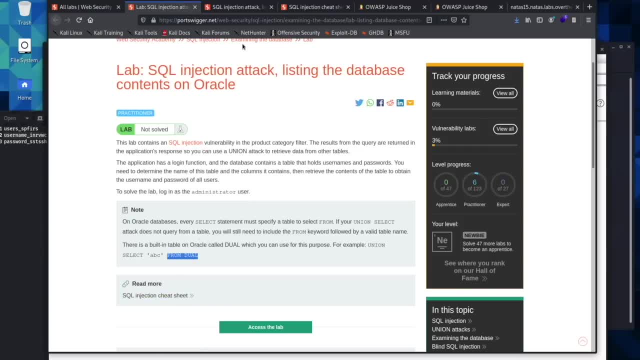 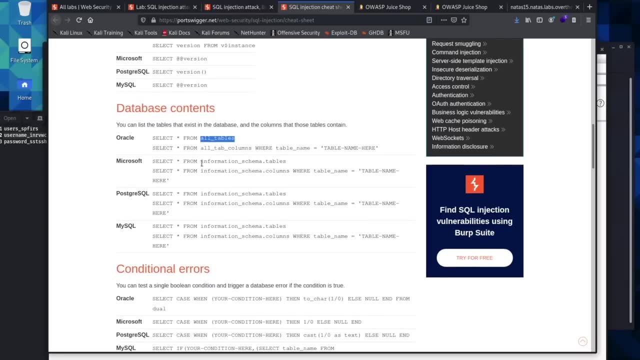 administrator, you're going to have to open up the sql injection cheat sheet. when you pull this open, you're going to be using from all tables instead of information schema. so in the last lesson, we used information schema as our default. well, that's not what we're going to be using this. 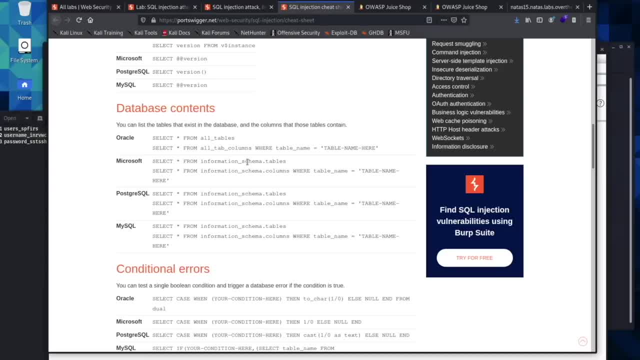 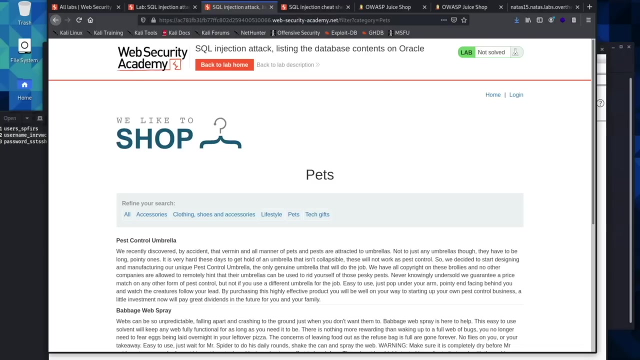 time. this time we're going to use all tables. everything should be the same as it was last time. the only difference is we're going to be using all tables instead of information schema, and so you can go ahead with that information and try and solve this lab, and if you have gotten stuck, we're going to go ahead and walk through this together now. so 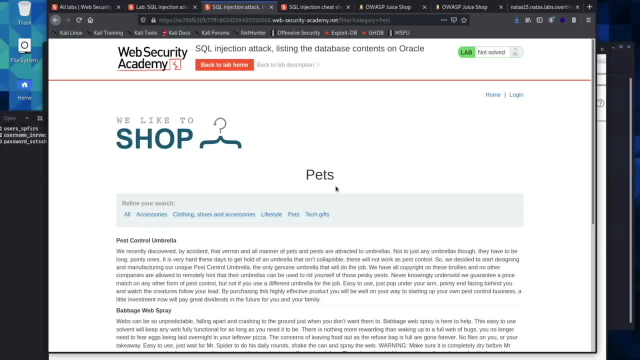 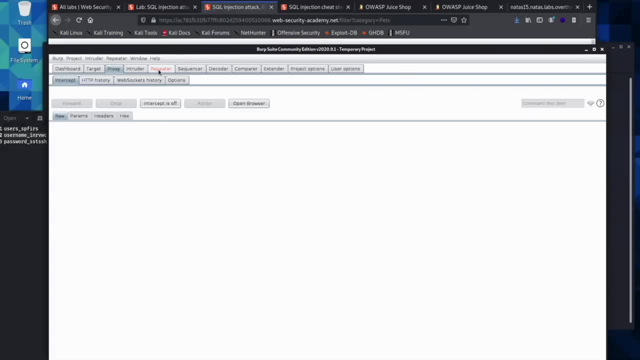 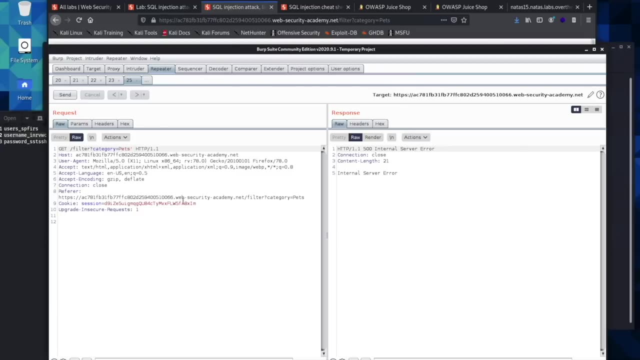 the first thing is turn your interceptor on. we're going to go through the normal procedures here. we're going to send it to repeater, turn the intercept off and make sure that we have our error appear, which we do. so this is telling us we have a sql injection. we are going to 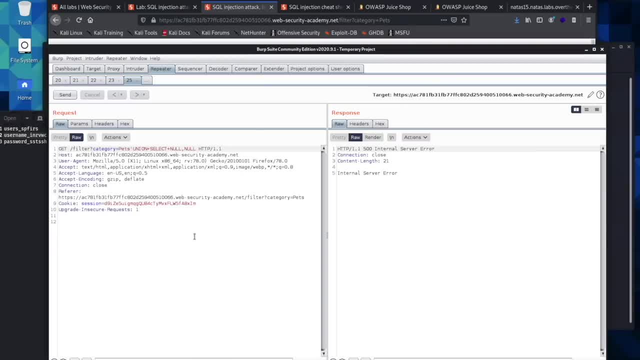 pull down the number of columns. i know there's at least two, because we were told that we have to log in as the administrator, which means there's at least a user's name, a username and passwords column. so we have at least two of those and then we'll go ahead and send this and it comes back. so there are. 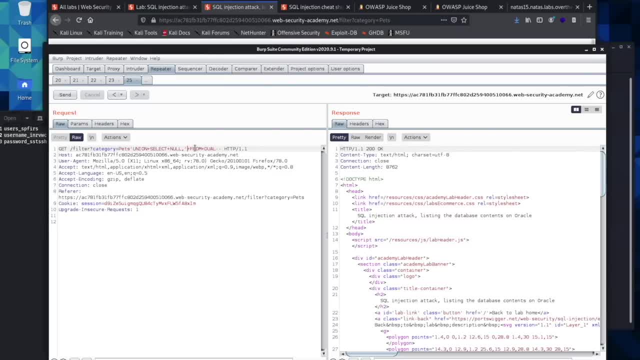 two columns. both of these are going to have to retrieve a string in order for us to pull down a username and password, so i'll go ahead and check it anyway, but i know it's going to come through and it does now. this is where we are going to start practicing what we learned in the previous. 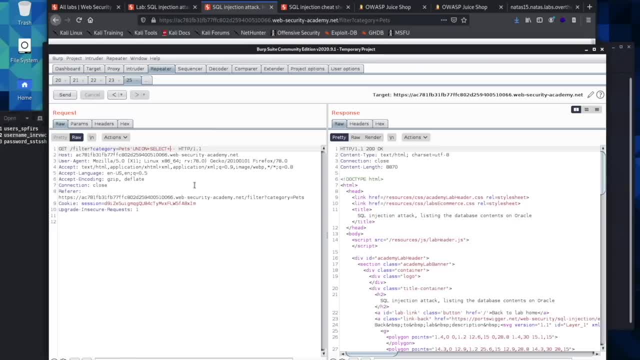 video. so, if you remember, the first thing we have to do is find the table name so we can go ahead and type in our table name, and this is from we used information schema. but, if you remember, this time we're going to use all tables and there we go, so this should give us all tables, if you. 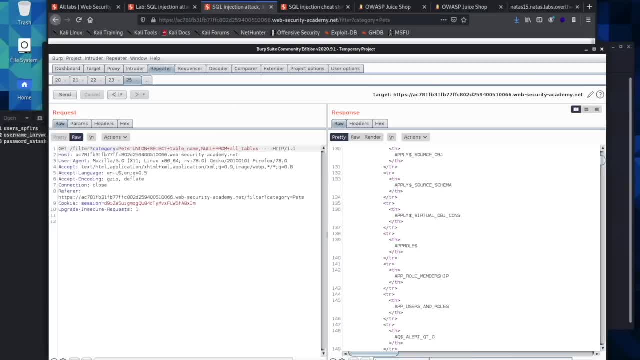 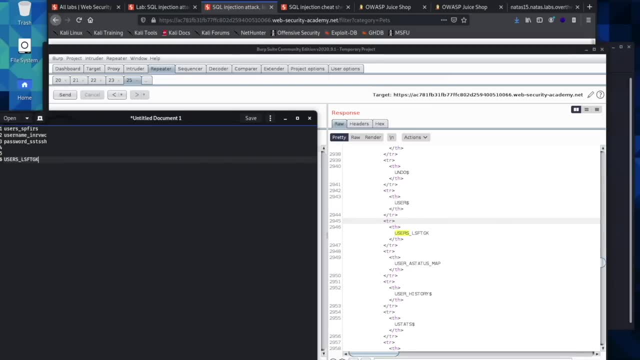 remember last time there was a bunch of them, but we are looking for the users. I'm guessing this is the one that we need history. we're gonna go ahead and pull down the information. well, this is, grab a couple of them just in case, but I think that's gonna be the right one, so we'll keep this one. this is the one. 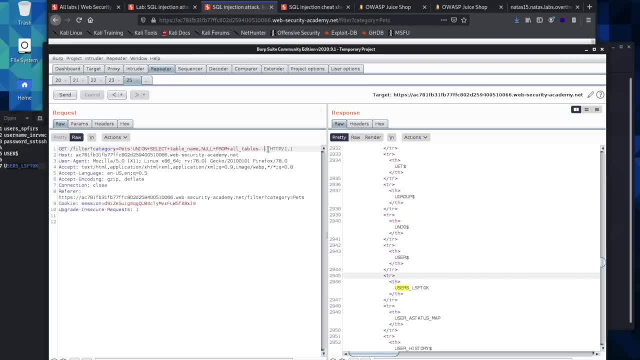 we're gonna roll with. now. what we'll do is we'll have to come back up here, if you remember, and change. now that we have the table name, we're gonna go ahead and insert this and see if we can find the column name. so we'll change this to. 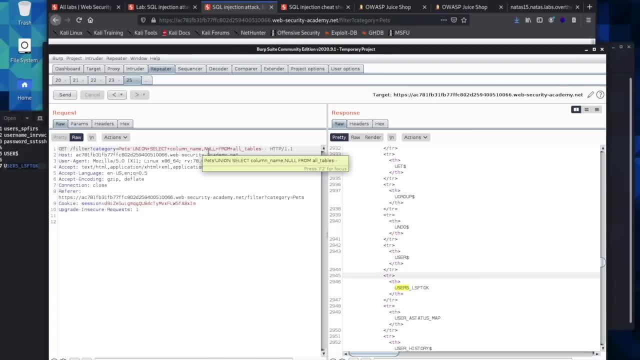 column and we'll leave our null and it is from, and this time we're going to input in our table into our injection. so we're gonna go ahead and put that in there and then we're gonna go ahead and we're gonna go ahead and put that in there and then we're gonna go ahead and 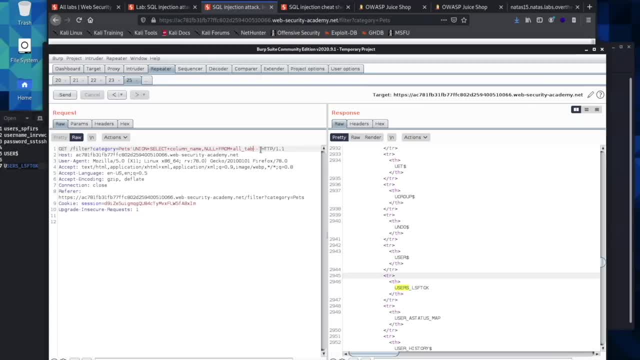 So we have from all of our tables- and we're looking for at this point the columns where it is equal the table is equal to the table name that we just pulled down. So we have where and then we'll type in our table name and then equals our table name. 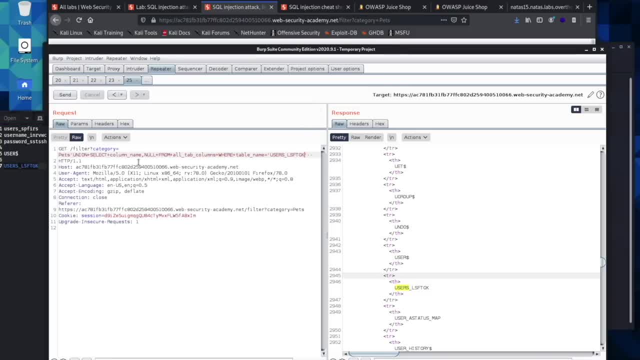 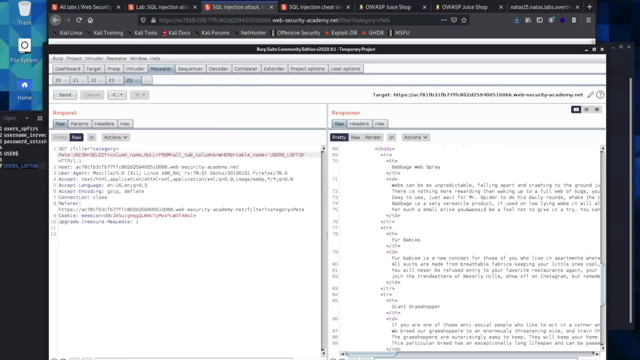 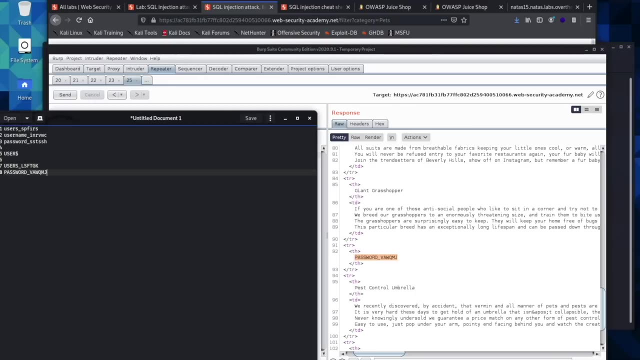 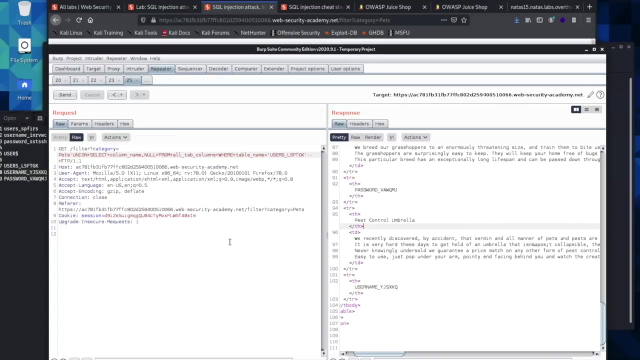 And we'll go ahead and look this over and then we'll send it. and it came through. Now we have to hope that we have our columns. So we have a password column pulled down and we have the user name. Okay, now we have to change our injection one more time. 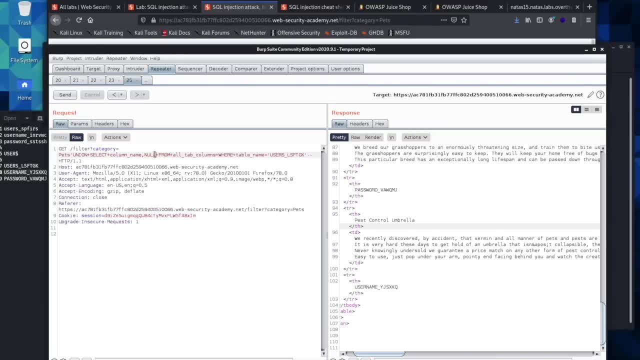 So this time we'll be getting rid of our null value and we're going to be putting in first our user name, And then we're also looking for the passwords which will come from our second column, And this is going to come from our table name, which I actually think we delete this. 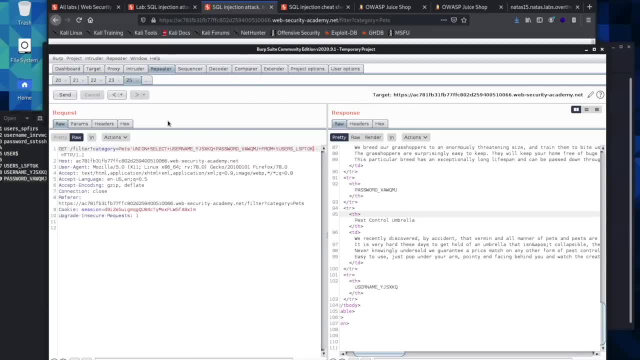 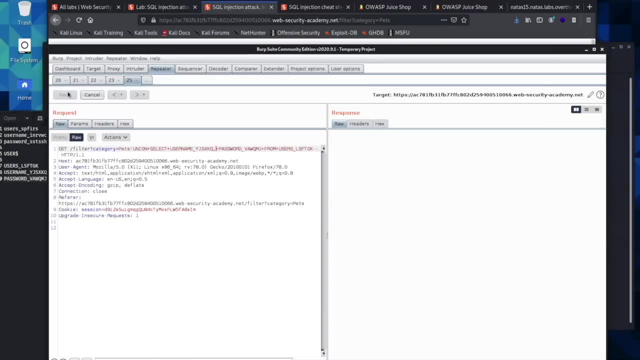 We'll delete that, And we'll delete that And this, And we have an error comma And we have pulled it down, So this should have our user names and our passwords in it, just like the last one that we walked through. 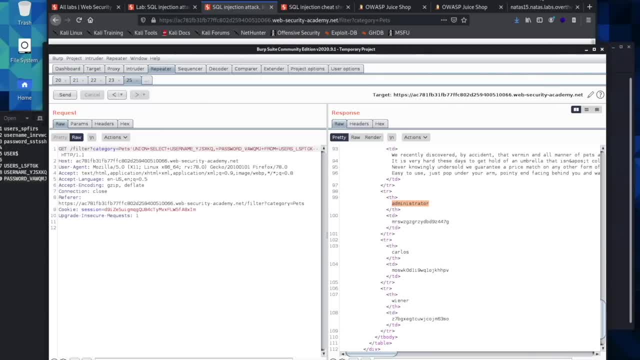 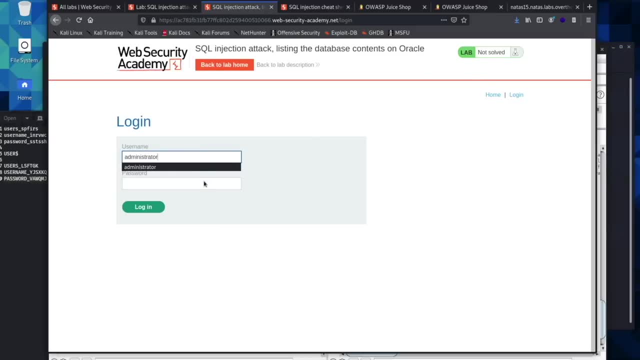 Here's the administrator and the password And so, if you remember, we have to log in to actually receive the solved lab up here. So we'll go ahead, paste that And we'll copy and paste this And send it And we have solved the challenge. 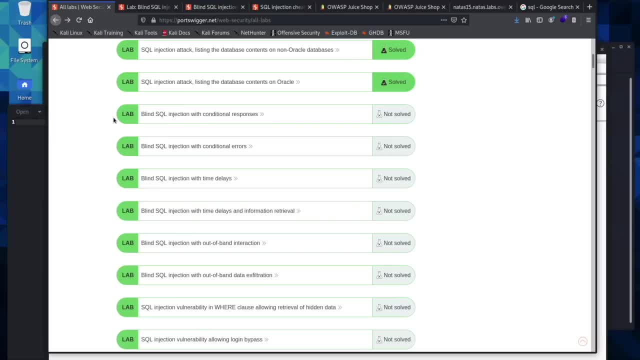 And we are ready to start the blind SQL injection. We are going to go ahead and open up this lab While it's loading. I thought I would just tell you this is going to be. the next couple of labs are going to be a little more difficult. 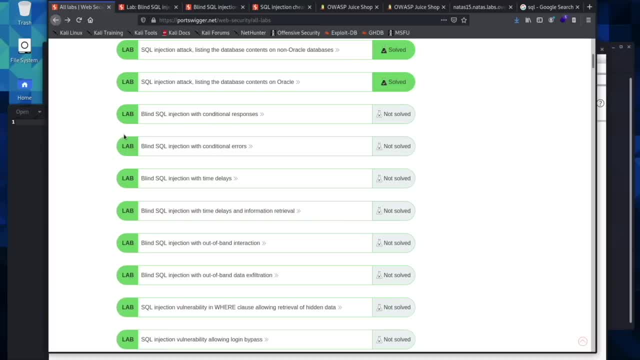 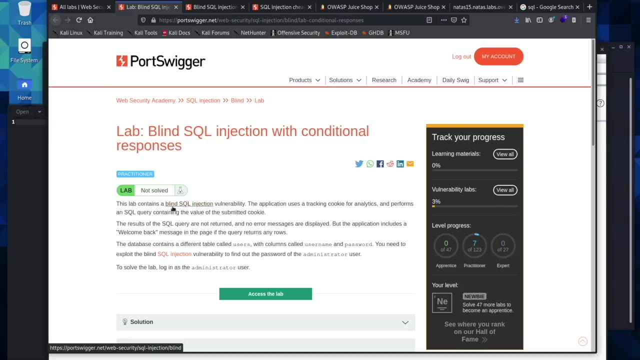 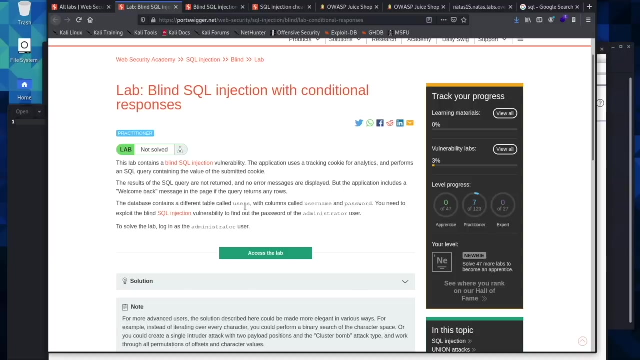 And I think that you should practice them Just to get this ingrained into your mind: What exactly is happening? Because we're going to be adding quite a few new steps, But they actually let us skip what we have been practicing, Because in the instructions they give us that we are going to be working with a table called users. 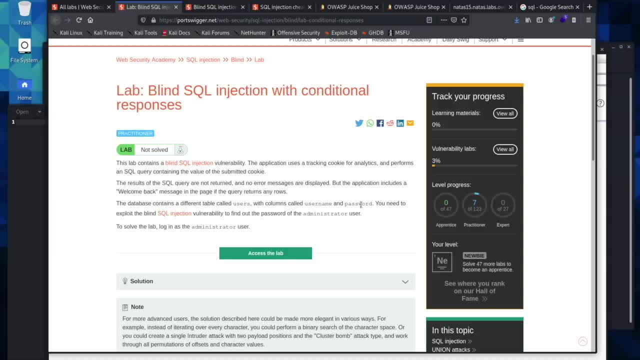 And two columns user names, or the user name and password. So we don't have to go find the table And we don't have to find the columns, But we do have to still log in as the administrator to complete this lab. 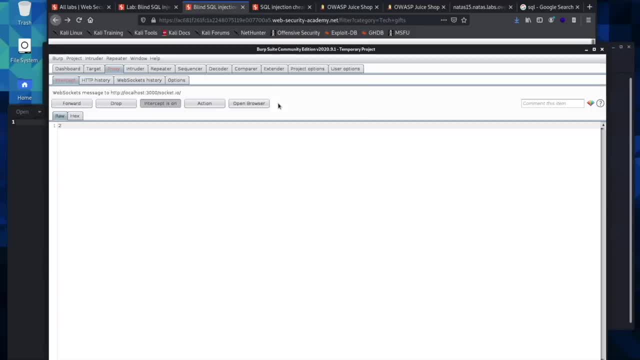 So you can go ahead and open up this lab. Start this lab exactly how we normally would: By opening up one of these tabs, Forwarding it And then sending our request to the repeater, Because what you're looking for is a request with this tracking ID. 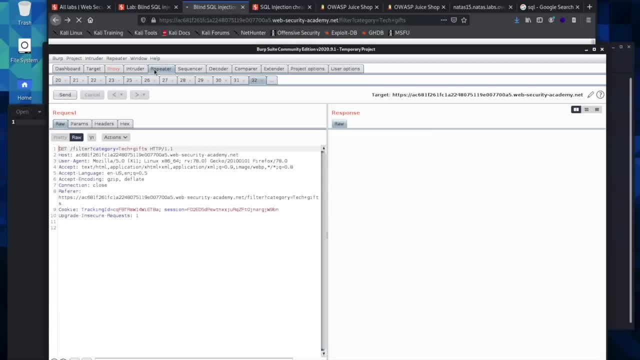 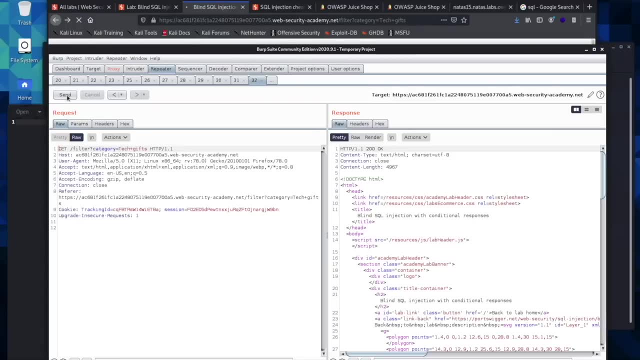 You need that tracking ID because that's where the SQL injection starts And that's where the SQL injection is going to be. So we'll send this And you can send it a few times, And what I'm looking for is this content: length. 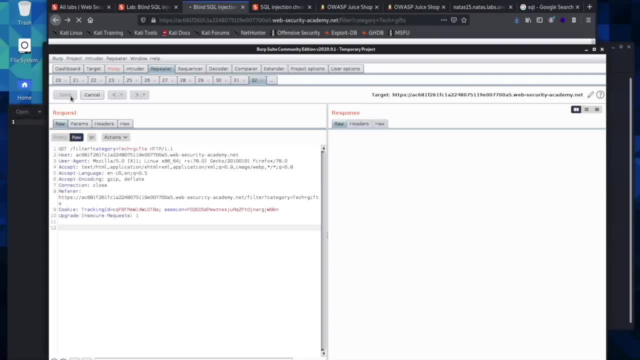 I want to make sure that it does not change, And sometimes you will send this on some web applications And it will change every time, no matter what you do, The exact same GET request, But for us, in our case, it stays the same. 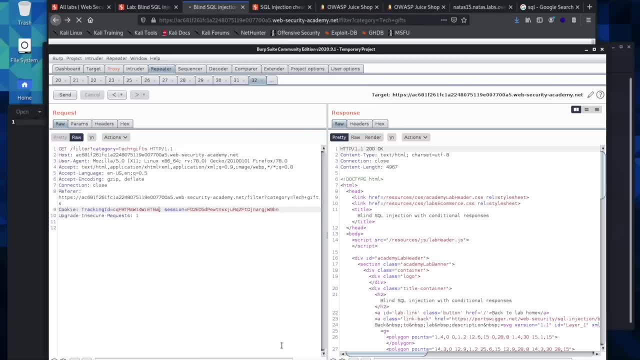 Which makes this lab much easier to solve. And when you have this tracking ID, You can also check it as well for the SQL injection, And so you send it And you can see the content length has changed, So it's 4906.. 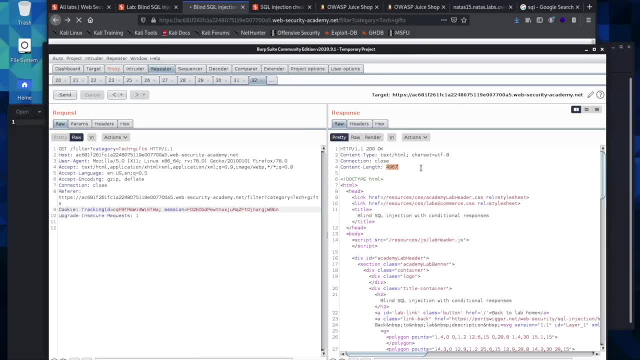 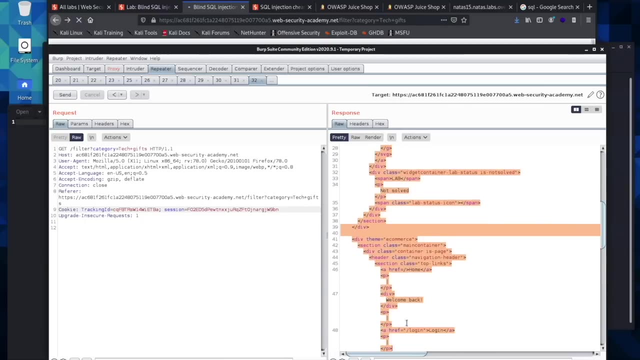 And you send it, And now it has changed. This tells us there is a possibility of a SQL injection. So what we're looking for is what has actually changed in our response Here. what I like to do when I come across a different response. 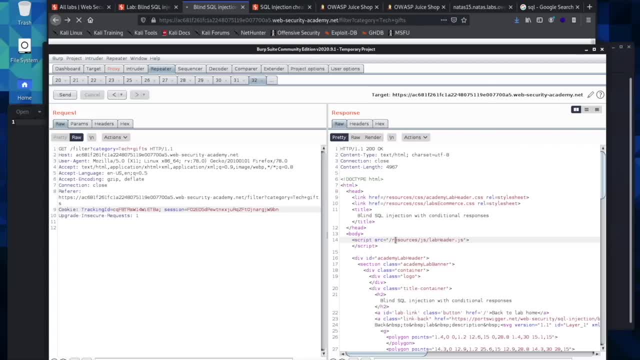 Is to copy this and take it to a text editor. I think it's easier to read through and to look at And I also can search Which we are going to do right here. So when it comes back without any modifications, We have the. 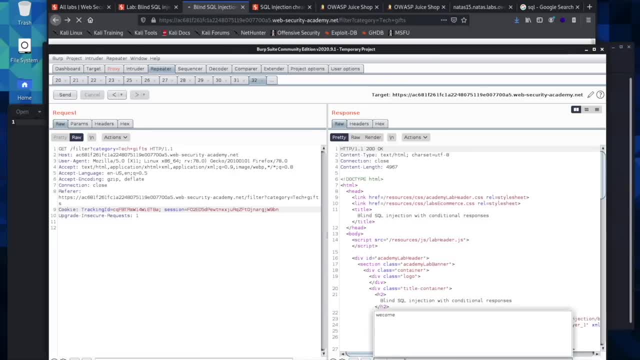 Let's send this again. We have the welcome back is on the page And we put in our single quote To try and provoke an error. The welcome back is gone. So you can see we have zero matches Right here, And so with our zero matches, 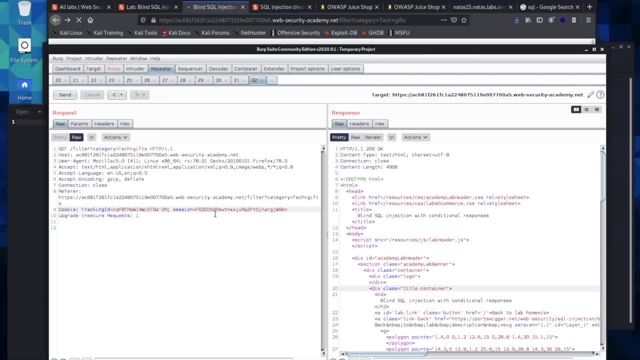 We want to send a true statement To make sure that we can really add on to this query. So we go or One equals one And then comment this out. That comes back as true, So we know that we can give Some kind of request. 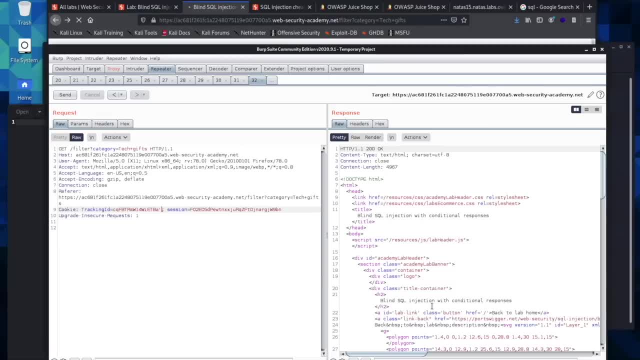 And see what comes back true. What is actually true And is on the database Will come back with this welcome back, Which is what we are going to have to pay attention to. And so, because we have already been told what the table name is, 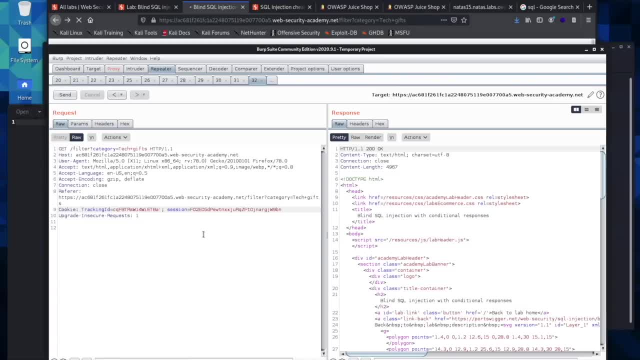 And the column names, We can go ahead and start to look for information From this table. So we will type in our usual Union Select, And this is where it changes, Because we are going to now add a character Into our query. 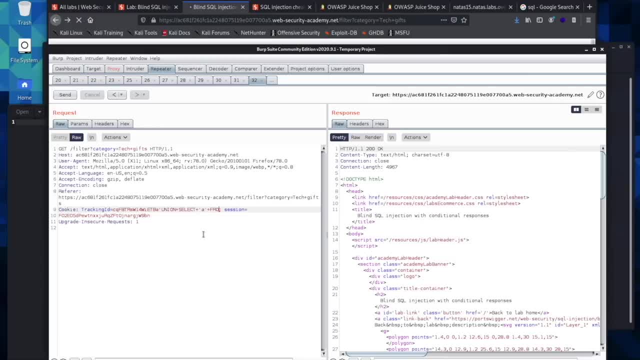 So we are going union Select From And then we are going to go to our users table Where the user name- Oops, User name Is equal to. And then, remember, We were told we need to log in as administrator. 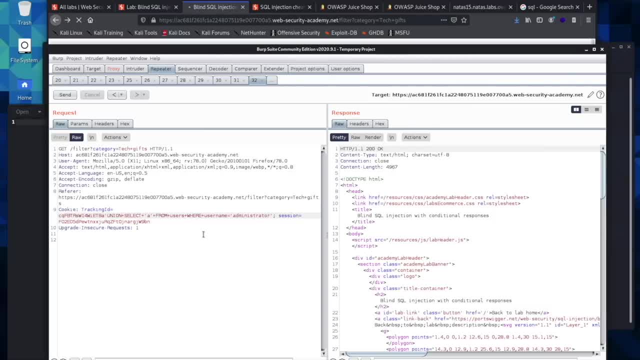 So the user name we are looking for And we are going to send this And see if it comes back as true. And it does. So we have this And now what we can do Is we can actually add on to it. 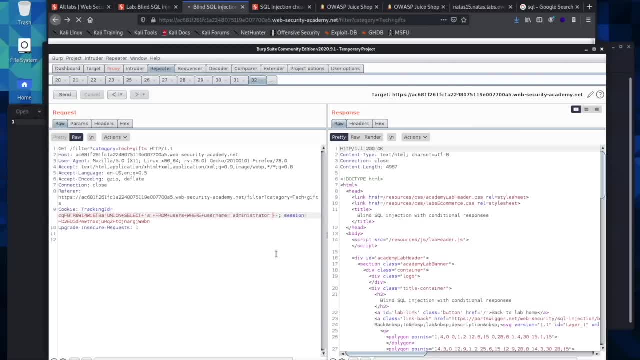 And we can look for The length of the password, And so you can come in here And you can look to see how long The password Is And you can pull down The length of the password And you can come in here. 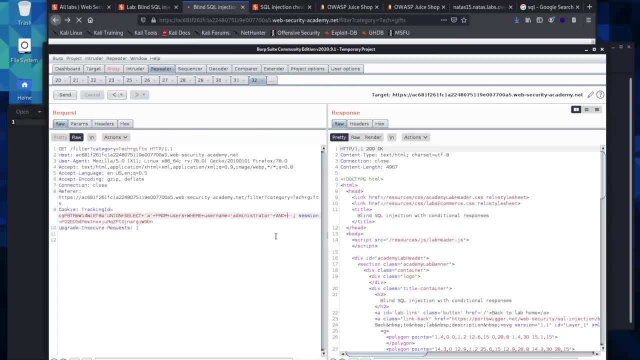 And you can go Plus and plus Length, And then we add in The password And then you would add: Is it greater than, And then you can start Right here and you can start sending To see Is it greater than one. 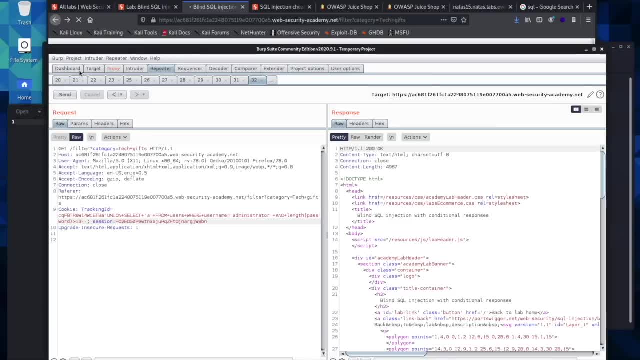 Is it greater than two, Is it greater than three? And you can send this to The burp repeater And just continue seeing Is it greater than? And looking through this, What I am going to do Is I am actually going to. 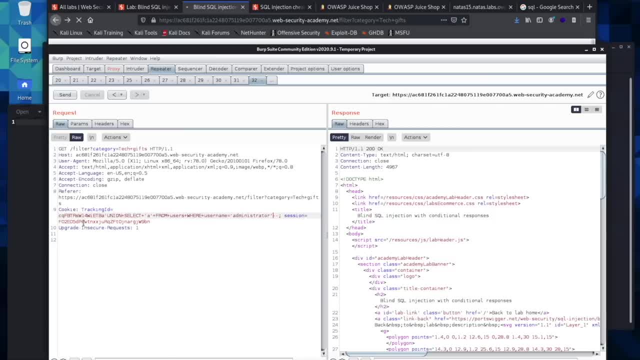 Skip this process For the sake of time, Because we are going to have to go into burp intruder And start looking For the actual password, And so what we are going to do Is we are going to Send this query. 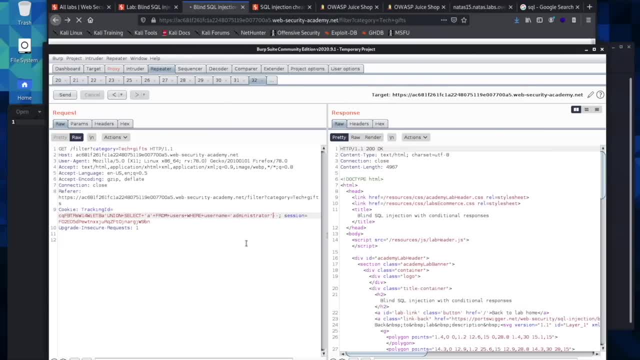 Over to the Intruder And see what we can pull back. So I am going to go ahead And take this Query here, And what we are going to do Is we are going to take this And we are going to add into it. 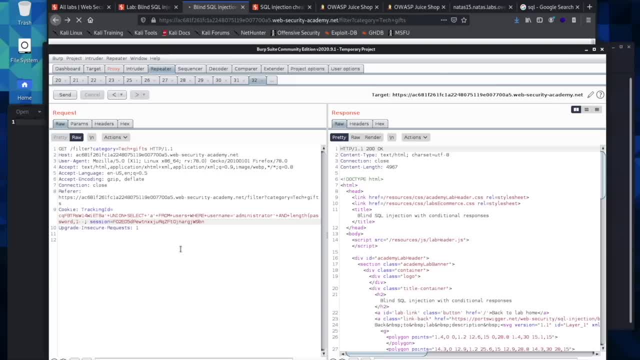 The characters that we are looking for, And so you would add in that you are looking for The first character And only one character, And then you are going to Slide the query And then you are going to start with The character A. 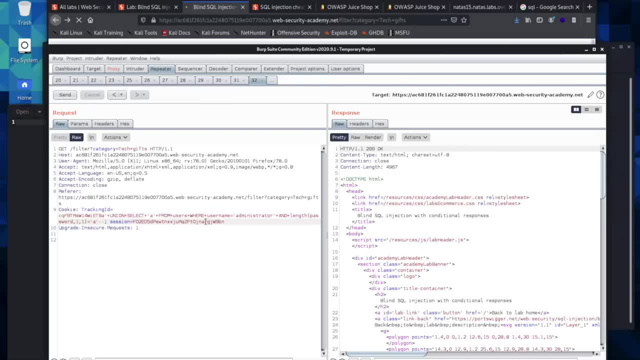 Now this, at this point, I am sure this is the first time you have ever seen Anything like this. It is, it looks very strange And it is going to feel really strange Doing things like this. It is new and it is kind of confusing. 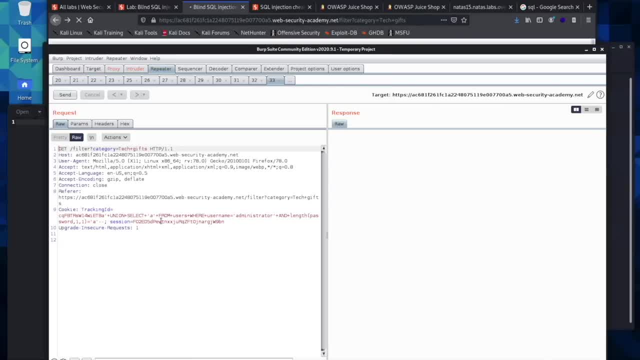 So we will send this not to repeater, To intruder, And so we have this new string That we are sending And we have a string from Users where the user name Equals administrator. So we are looking On the table name. 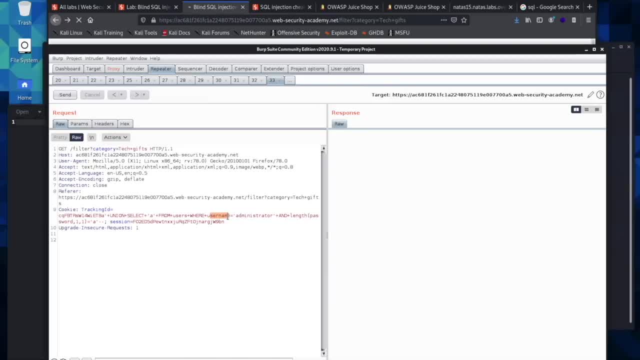 Users under the column User name For the Administrators password And we are Looking for The actual password At this point- And this actually I just noticed- We are not looking for The password We are going to be looking for. 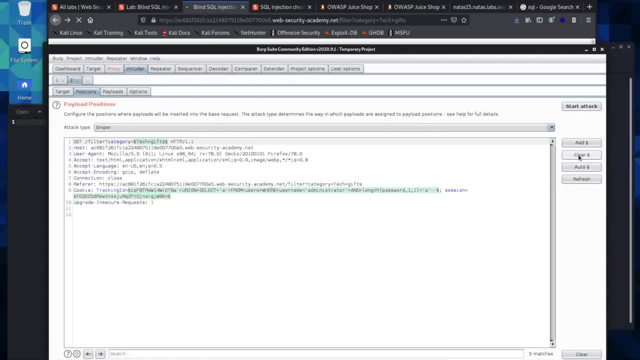 The substring. So we will come over to intruder. We will look at our positions Because we have already sent this over here. We will clear Where it wants us to start querying And we are looking for The substring In the password. 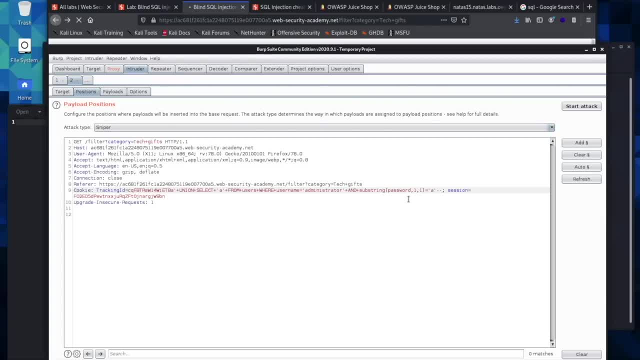 And so we will go ahead And set this up. What we do at this point Is we will add The- whatever those symbols are, To tell it: this is Where we want to shoot through, Or we are going to use The cluster bomb. 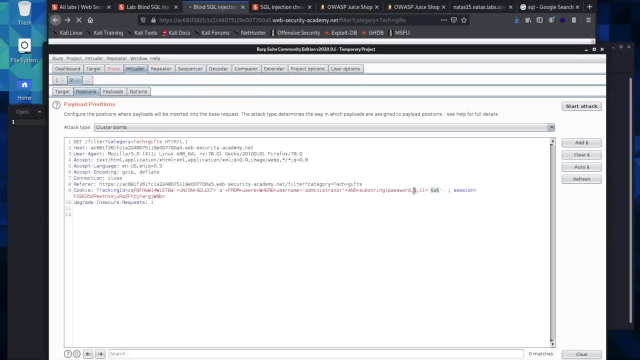 So this is where we are going to be going through And sorting to make sure we have The right characters, And then we will add right here, Because, if you remember, This selects the first character And then it is going to go through the first character. 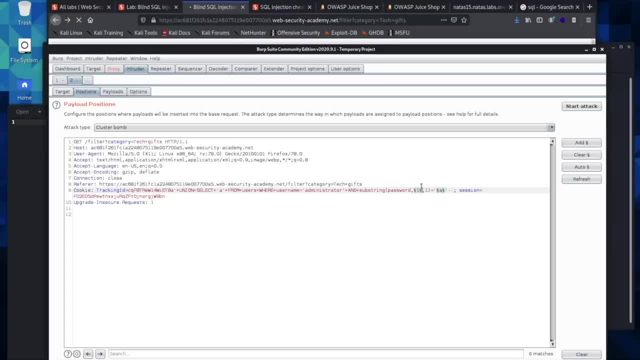 For all the characters that we give it, But then we want it to go through The second Character as well, And the third and the fourth and the fifth, Until we reach the end And we have the password. I don't have the professional version of burp. 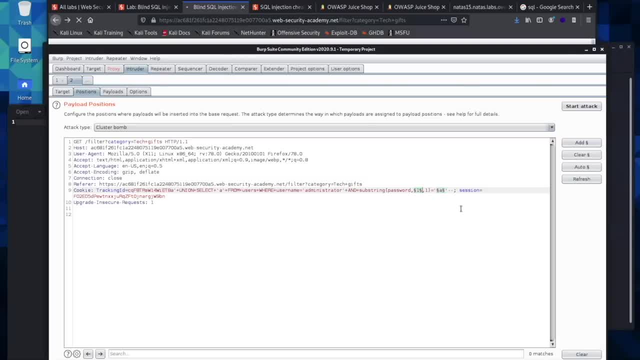 On this system, And so this is actually going to go really slow, And once it starts, I am going to go ahead and pause the video So you don't have to wait for it to pull down The password, Because it will actually take a while. 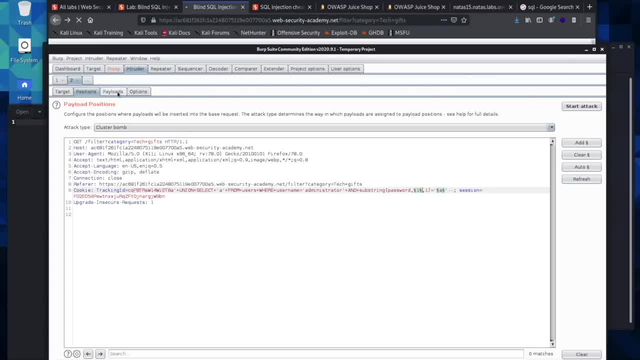 Without the professional version of burp. And so what we are going to do now Is we are going to set up our payloads, And so, if you remember, Payload one is going to go to This position And payload two is going to go to this position. 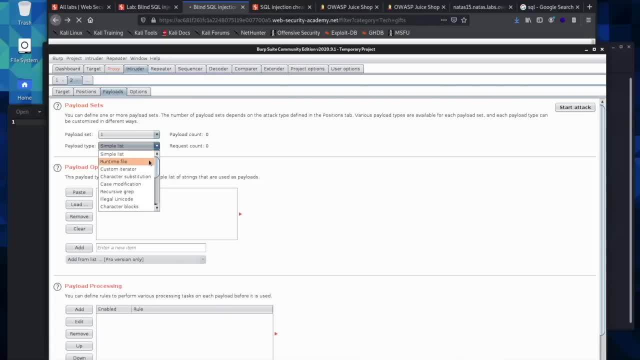 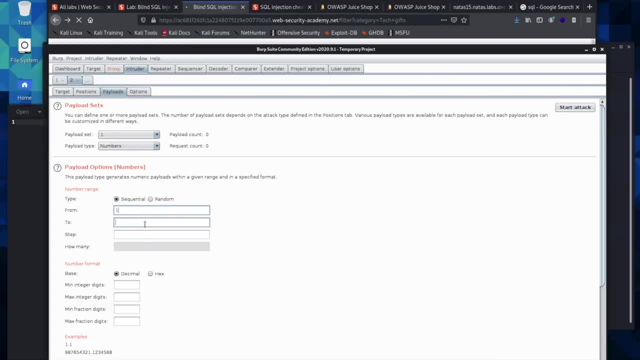 So the first payload, We are going through numbers, So we will find numbers And we are going to go From one And this is when I guess it would have been helpful. I am just going to go really far. This is when it would have been helpful. 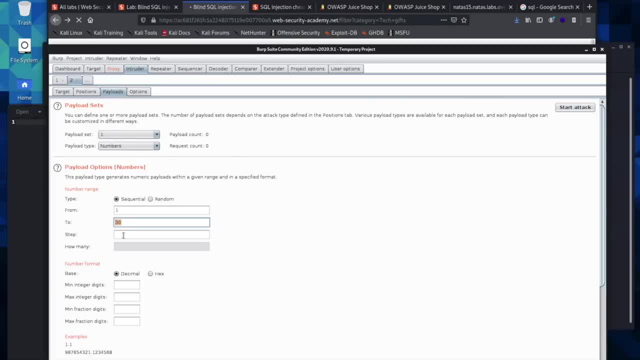 To see how many characters were in the password, So you would have known how far you needed to go. And then we are going to go By a step of one, So it is going to go up one character Once it goes through all 30 characters. 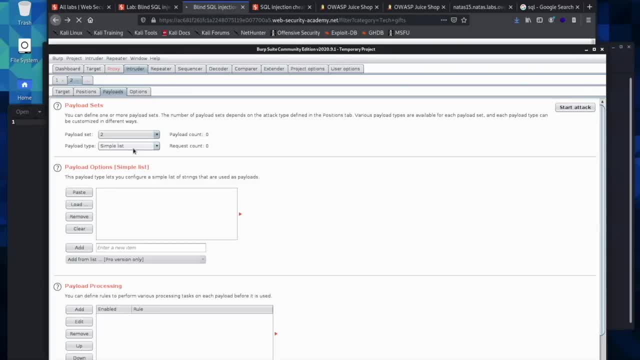 And then Position two. We are going to be going through The alphabet. See if it has The alphabets in here for us. I believe it does. When you add these in, It would be A lot easier To go through. 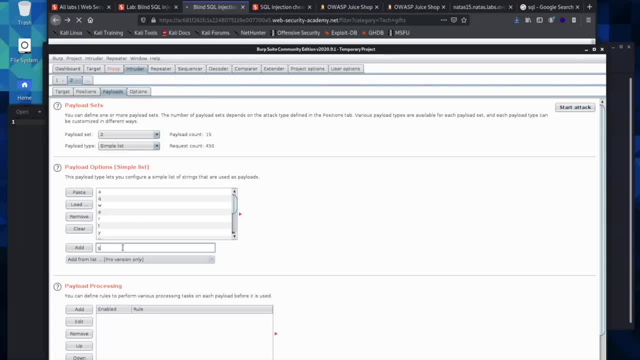 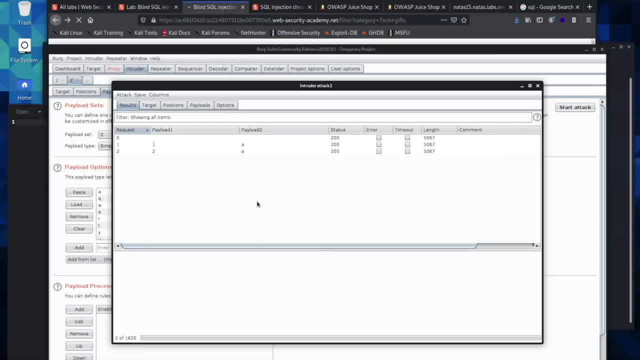 These Without having to do this, But I will edit this out. Alright, I believe we have all of the characters Added in. What we can do is we can go ahead and Start the attack And we can say, okay, And now it is going to go through. 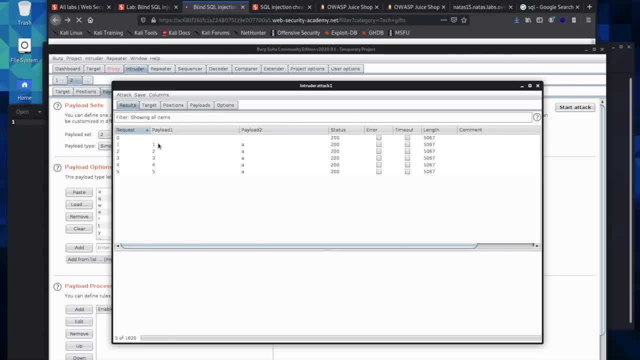 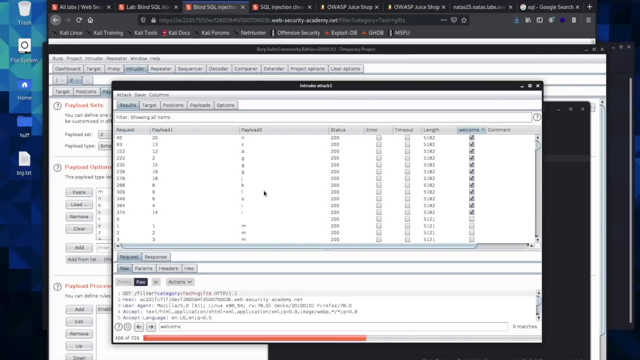 And start working through all of those Characters. So is position one an A, Is position two an A, Is position three an A, And it is going to go through Each position Until one returns true. Okay, I have gone ahead and cut the video. 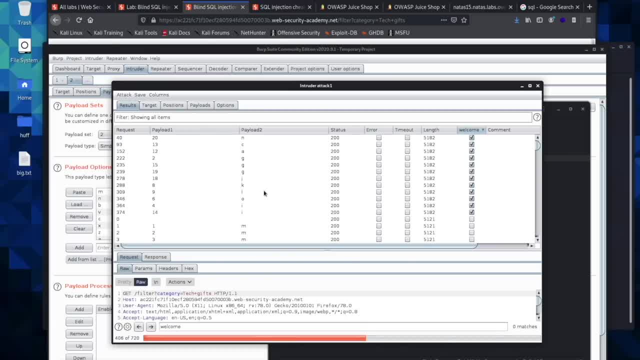 In the middle of where we were After starting the attack And you can see that it has been running And we have pulled down Some of the characters that we have needed, One of the things That might be helpful If you copied. 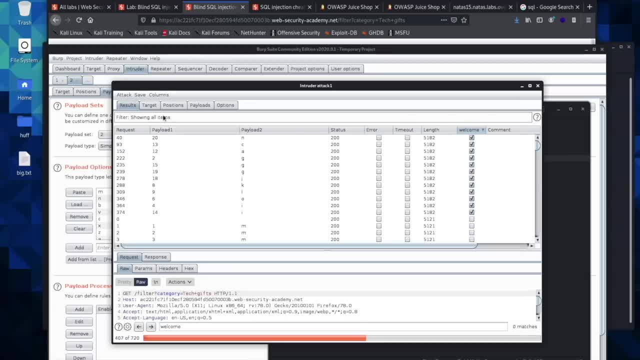 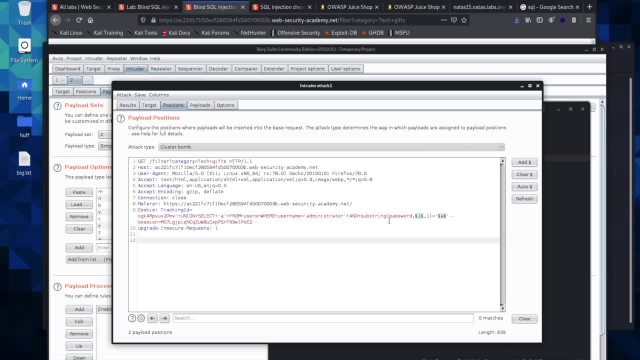 Exactly what I had typed in Into the payload Or into the query. Here I actually had an error And I had to go through And change that And fix it. And then that ran for a little while And then also my computer fell asleep. 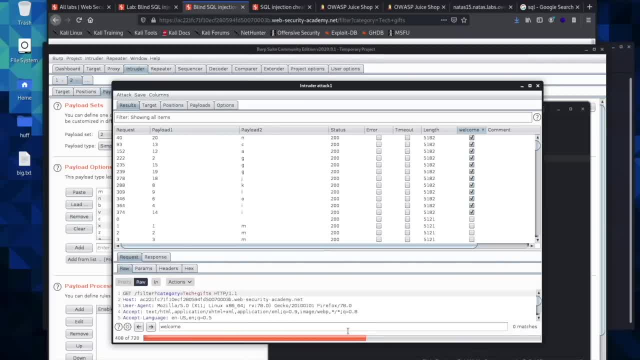 While running this And it closed out my query And so I had to restart it, And so this has been running For what feels like forever, And so I am going to go ahead And we are going to stop it here. And it is also a lot faster. 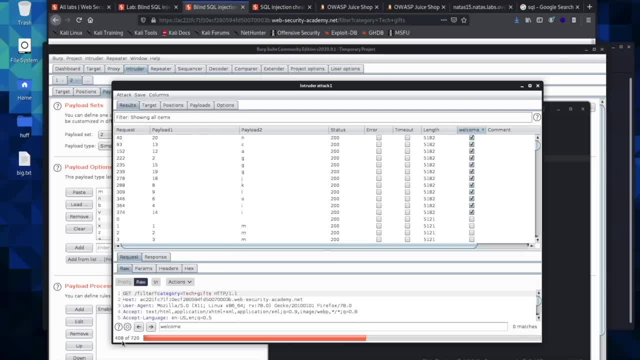 Because, if you can see, It is sending one query Each time to the server And it is very slow- Anywhere from 10 to 15 seconds- And it is because we have sent so many, And this is one of the things burp does. 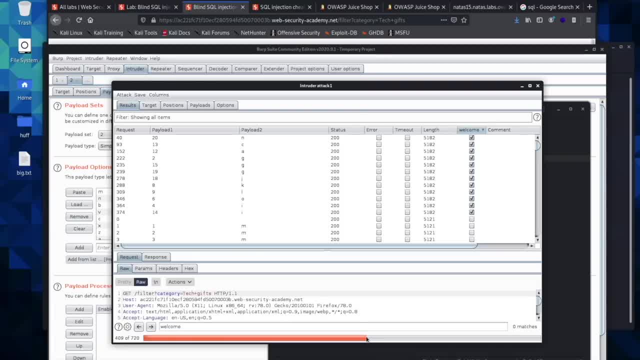 In order to get you to buy burp professional So that it will send them really fast. So they have throttled this down, But I am going to show you a way That you can kind of get around this And send your queries a lot faster. 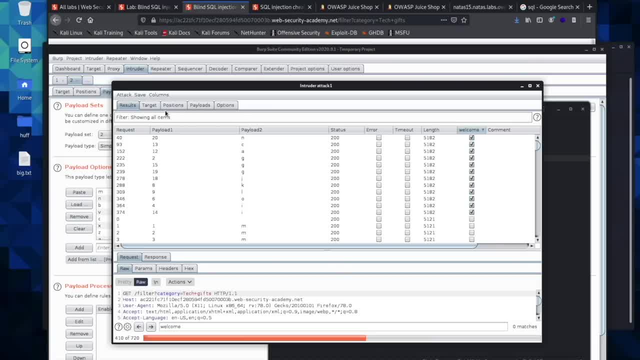 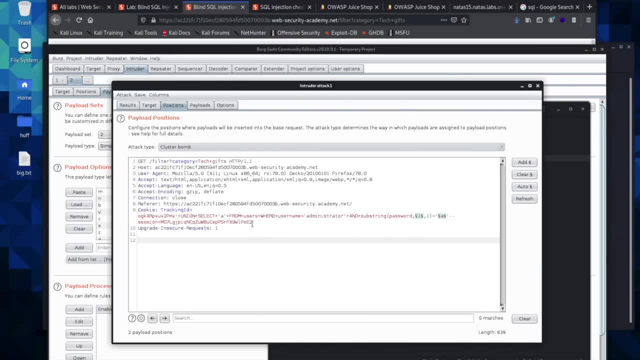 So before we start that, I kind of wanted to show you our positions, Just in case it wasn't clear. Remember, in our query We are selecting from the users, The table users, Where the user name, Which is the column, And we are looking for the name of administrator. 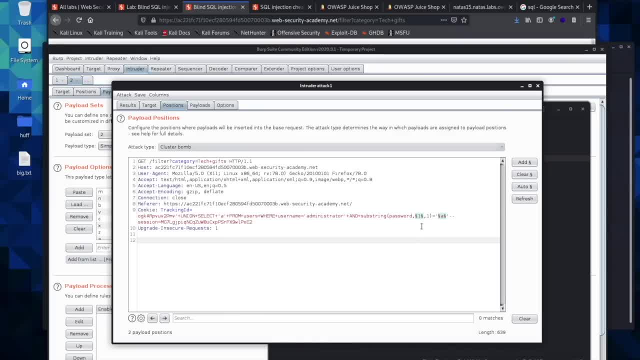 Inside the password column, And so we are sending. This is the first character In the query, So this would be position number one, And then it will change To position number three And it will send A All the way through. 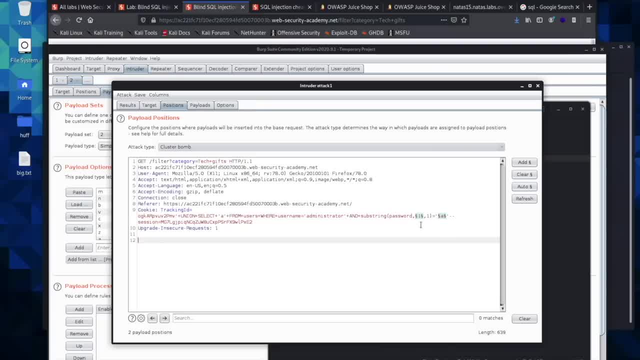 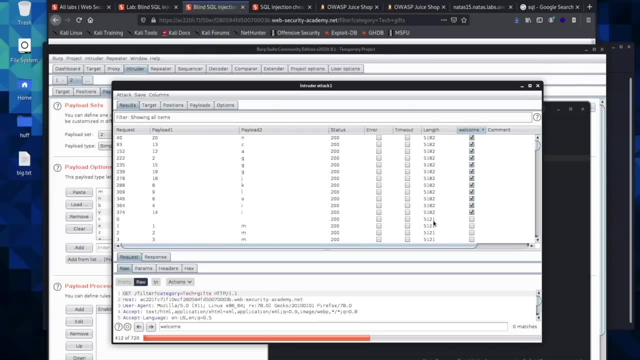 However many. we set those positions- One, two, three, four, five, six- To see if an A comes back as true In any of those cases. And if it comes back true, We will see something like this: You can see the length has changed. 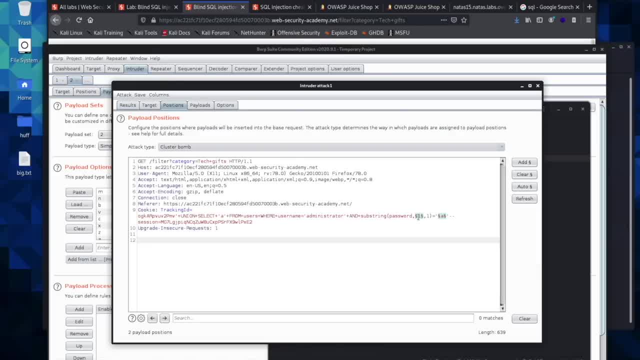 And the welcome back is present in the response, And then, once it goes through all of position, one For all of the alphabet, It will go to B And then it will start over And then it will go through like that. This is a very automated way. 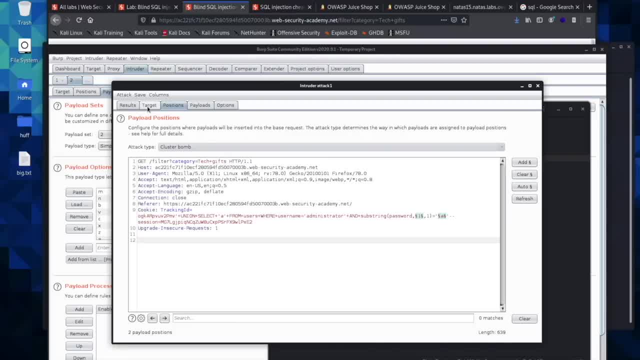 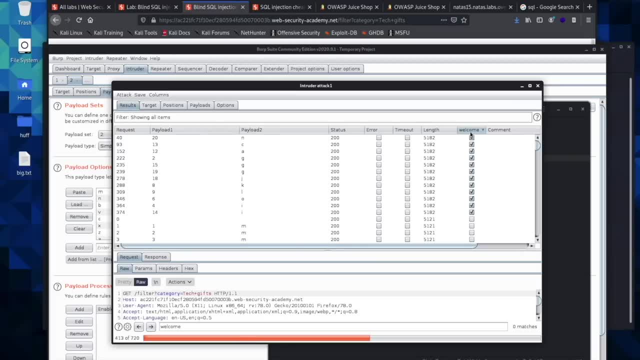 We don't have to really do anything. We just set it up and let it run. But if you don't have burp professional, This can take a very long time. And one thing Before we go ahead, And I show you how to organize this. 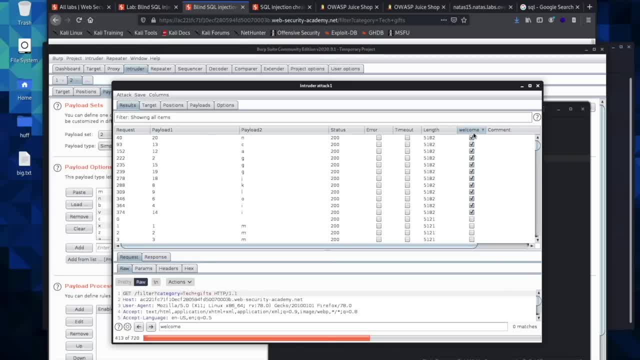 To find the password Is that, in order to get this welcome back To show up, What you do is, you can check in your response And you can have your welcome down here, And if you can see these, it matches, So we will come back. 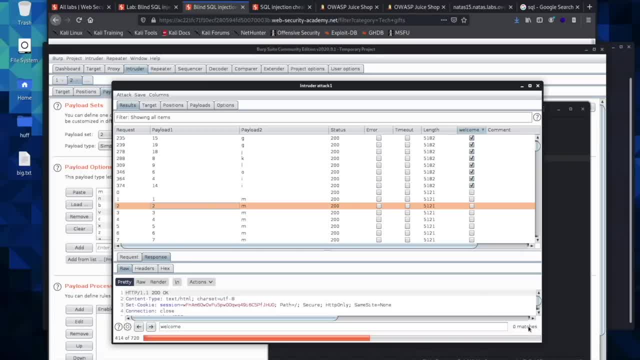 Which means it is true And we have a match For these down here. it is not true And there is no match, And so we can sort out the true characters that exist And in which position they exist. So there is a G in position two. 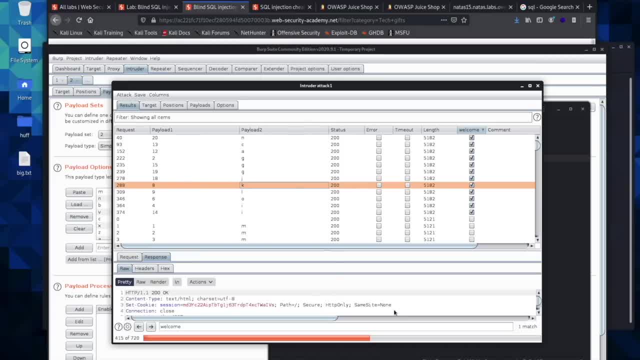 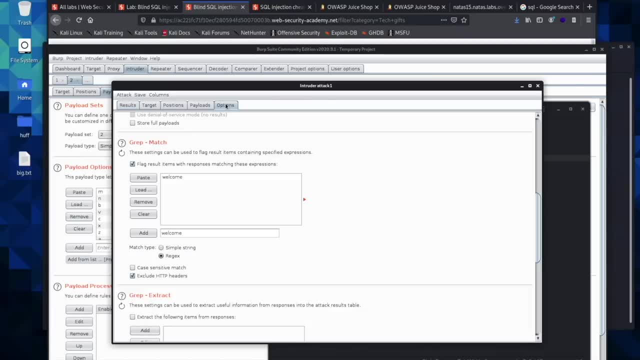 There is a G in position fifteen, We have a K in position eight, And so on, And so we can know. this is where there is characters And this is how it is true. But in order to get this welcome up here, You will scroll down. 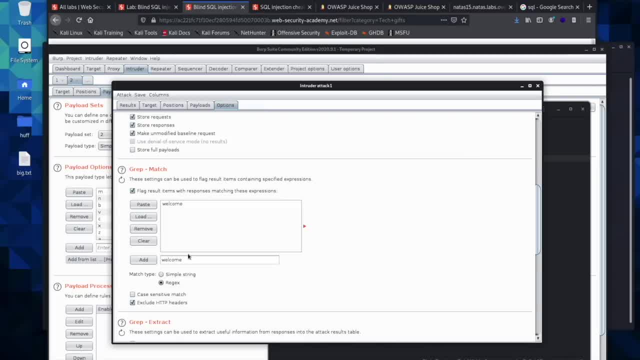 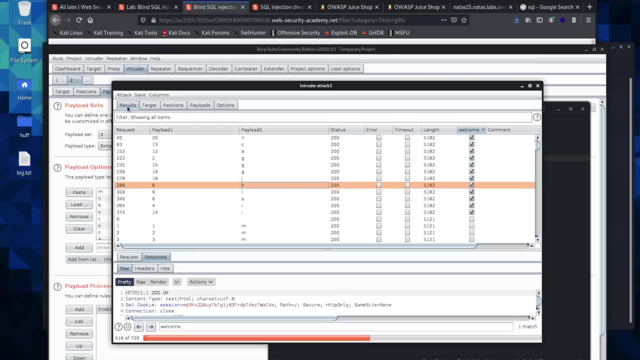 So it will start you up here. You will scroll down to grep match, You will clear what is in here And you will add welcome. You will get a little pop up, You will just click okay, And then it will bring you back to your results. 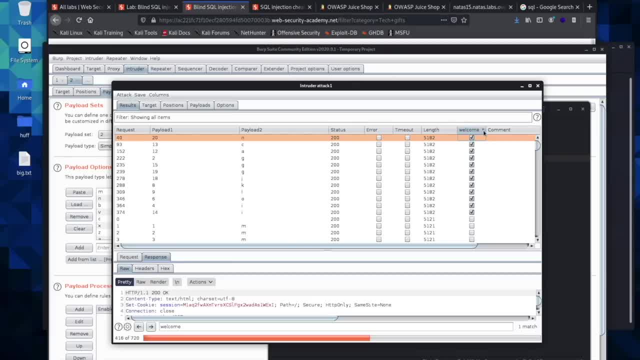 And it will look like this, And what you do is you just click this And you click it again Until we have the arrow facing down And it will have all of the characters there For you as it runs. So what we want to do with our password. 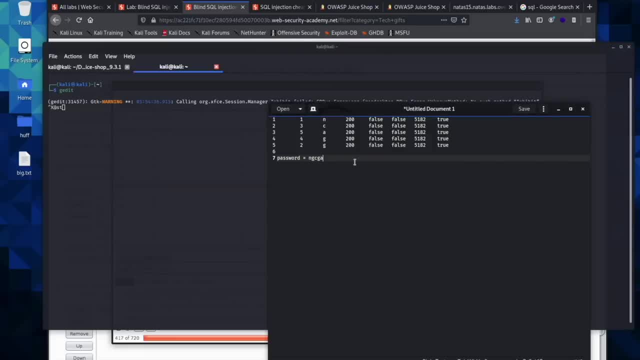 Is to have a text file open, Which is right. here We have our text file. We will delete this And we will delete this And we will paste this in. So what we have here, We will also delete these, Because these are just our query numbers. 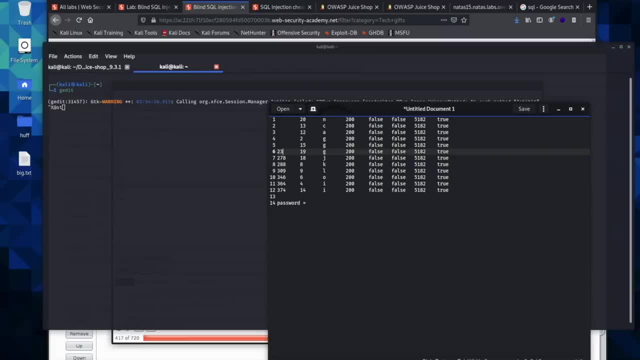 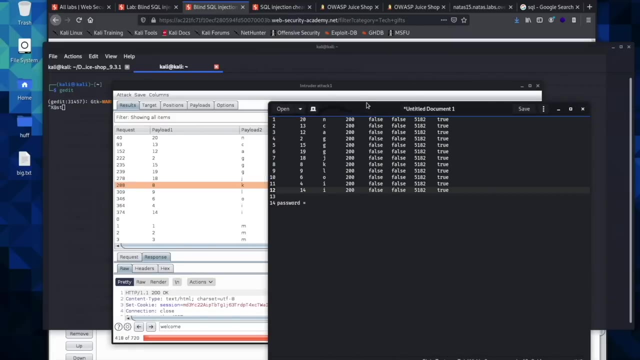 On how many get requests were sent To the server, And I think the less numbers We have, The Easier this will be to understand. So this, if you remember, Let's open this back up And have our text file. 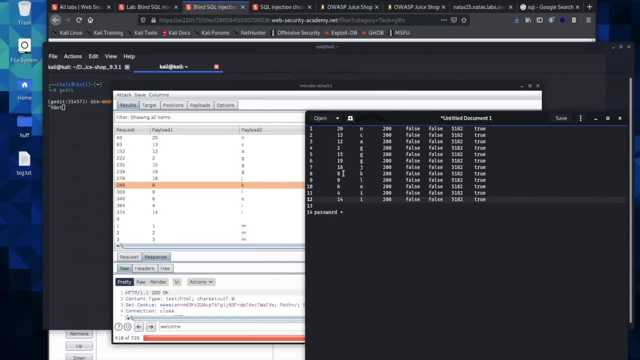 This is the position From payload number one And this is the character that has come back In payload number two. So what you would do? So let's say: this is what we have brought back And the query is finished, Even though we know it is still running. 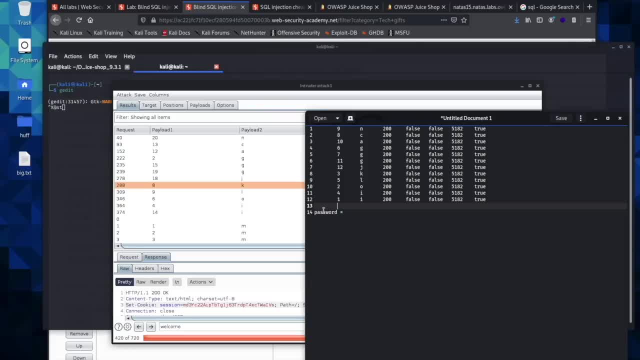 And it is going to take five more hours For it to finish running. So what we would do Is take position number one Is I, And then we would look for two. Two is O, Position number three is a K And then position number four. 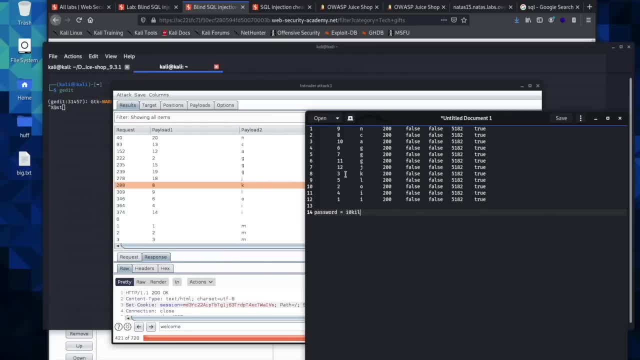 Is an I, And position number five L, And position six is a G, And then you would go along And you would just continue Doing this all the way through. So we get six, And then we get seven, And then eight is a C. 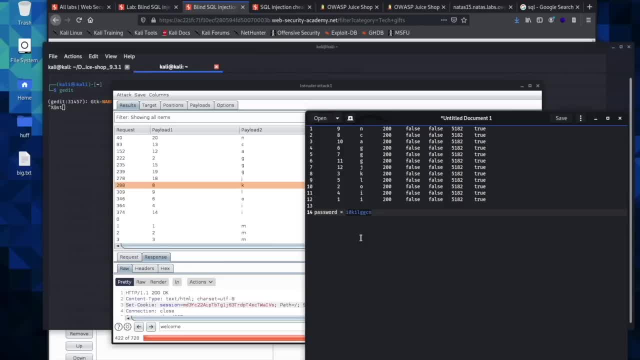 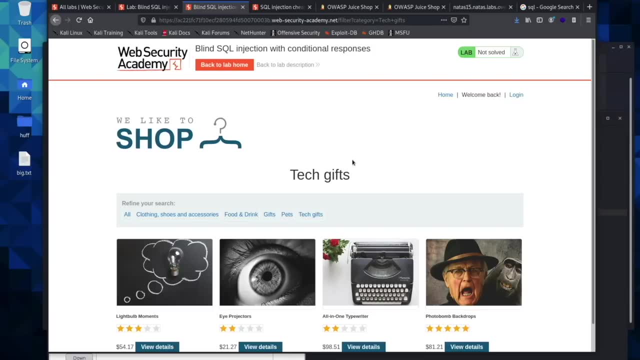 And this is your password, And so we were told That the username is administrator And the password is What we are pulling down right here And we would come over here, We would go to our lab And this is where we would come in. 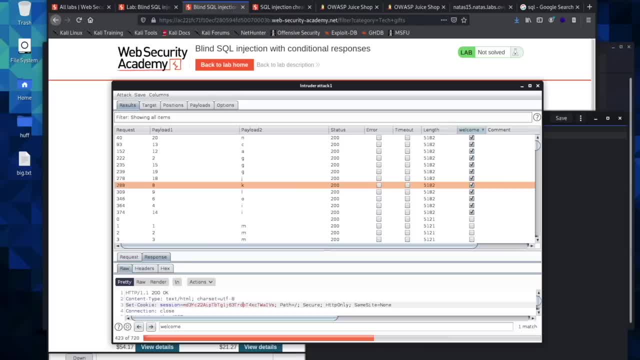 We would click log in, You would use administrator And then this password that we have just pulled down. So if you want to let your intruder run For ever, Because it is really slow, Especially once you get past about position, After you get past request, 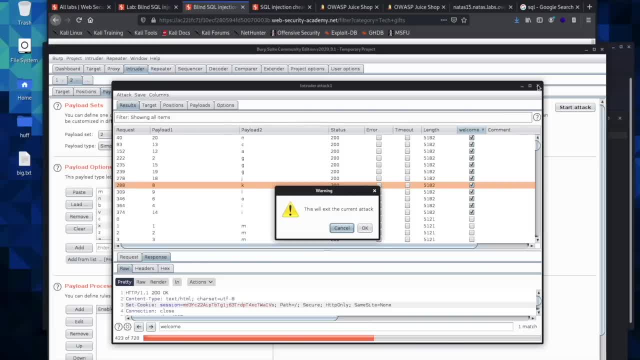 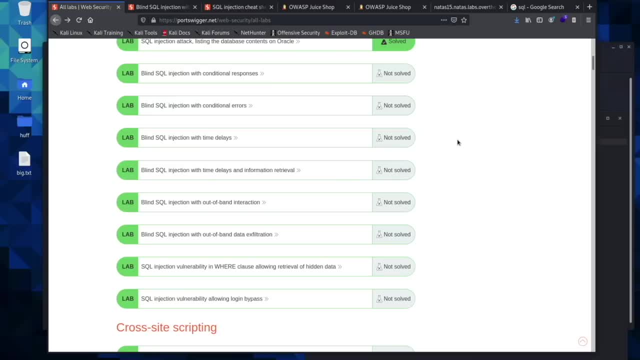 Number 30 to 35. It really slows down, So I am going to go ahead and close this out. Okay, we are going to look at the Blind SQL injection With time delays. So what you will do is, If you find what you believe to be a SQL injection, 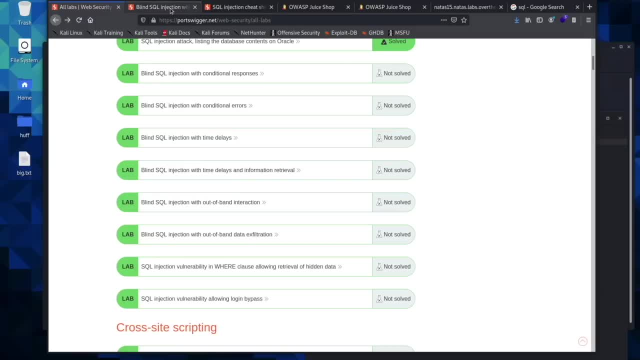 You will inject a time delay And they are pretty simple. But I also want to look at the cheat sheet, Because they are going to be different And we are only going to be looking at This one right here: The blind SQL injection with time delays. 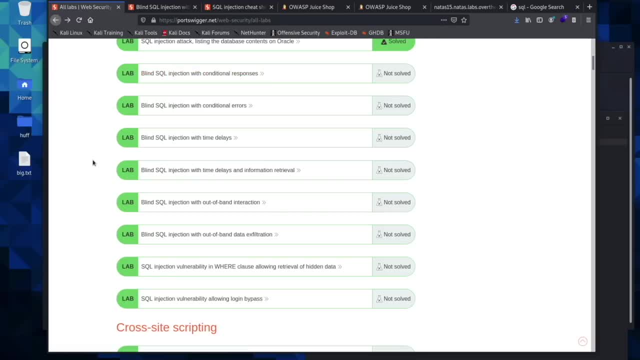 Is really simple. To the one with conditional responses Which we just looked at. The only difference Is you would be running A case then statement Which, if you are a programmer, It is like if then? And you are going to be saying: 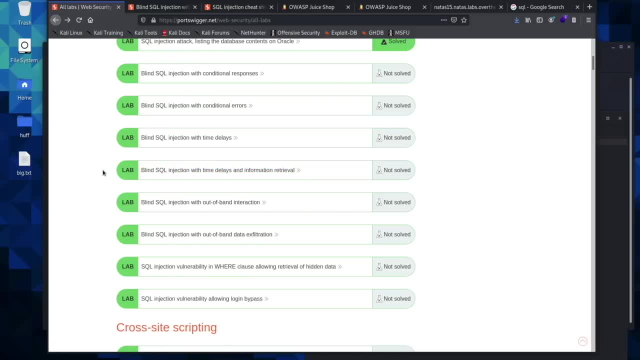 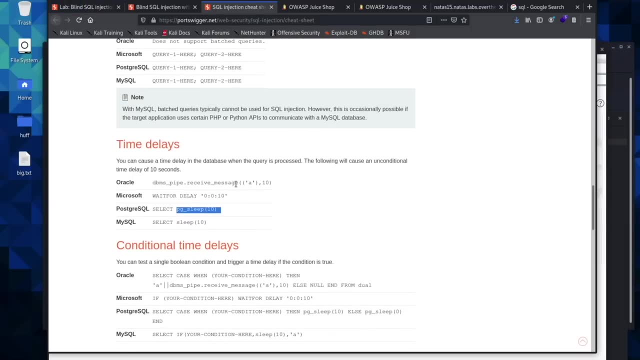 If this is true, then sleep Rather than if this is true. So with the cheat sheet, These are all going to be different, So you will have to run this To get your program to sleep For your delay with Microsoft. It is going to be like 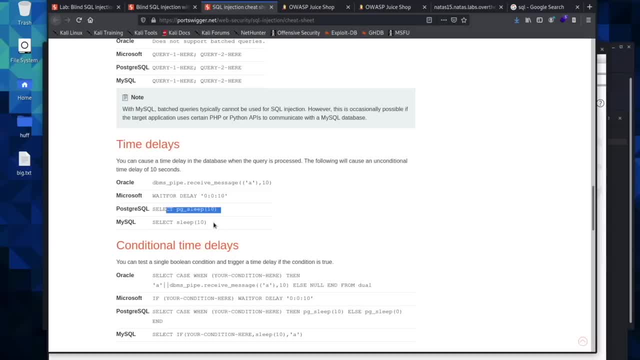 Your syntax is going to look like this. For PostgreSQL It is going to look like this, And MySQL is going to look like this, And so each one is going to be a little different And you might have to just try each one. 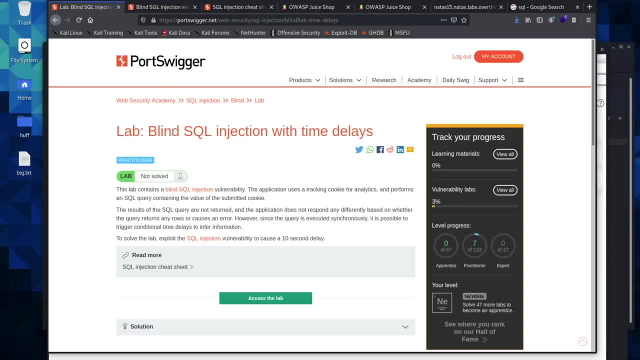 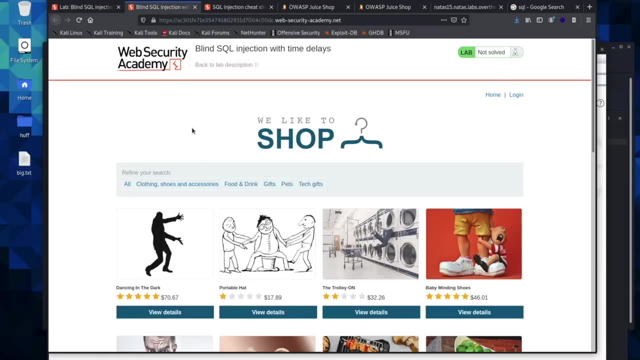 And see what comes back for you. Okay, so this is We are going to have to To solve the lab. We need it to sleep for 10 seconds, Which is kind of a long wait, Which feels like forever When you are waiting for a response. 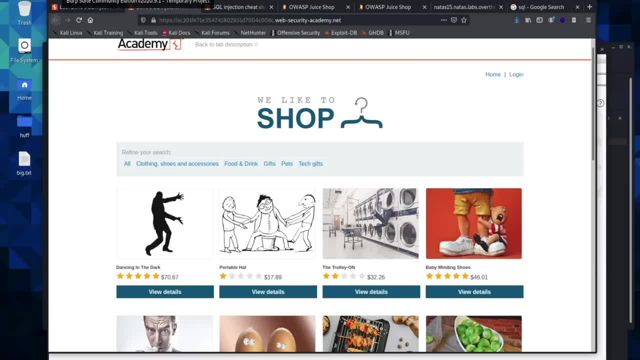 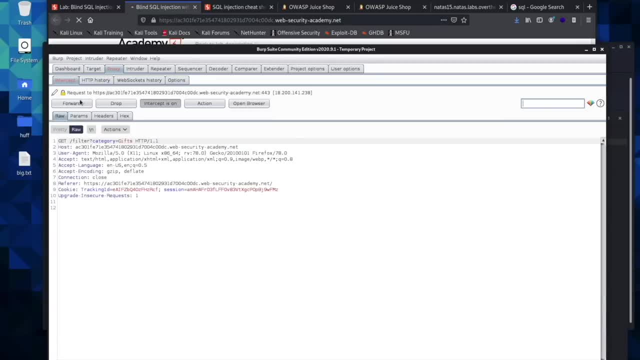 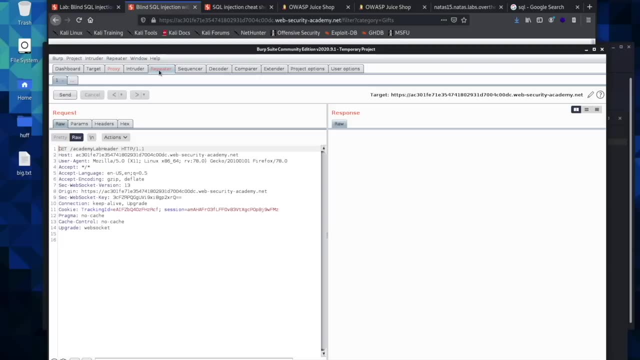 To a get request. So we will go ahead And turn The interceptor on Open this up. I think I clicked in the wrong spot. There is a tracking ID. We have one right there And This will look. Let's see if it is. 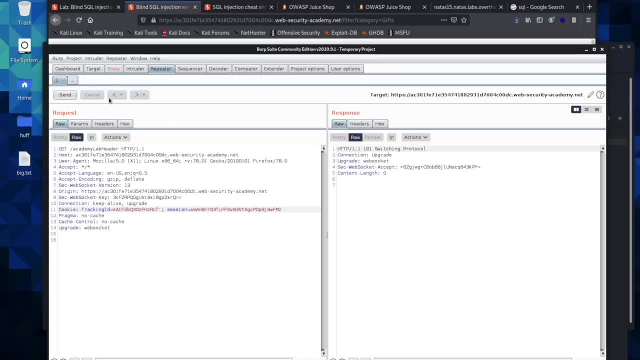 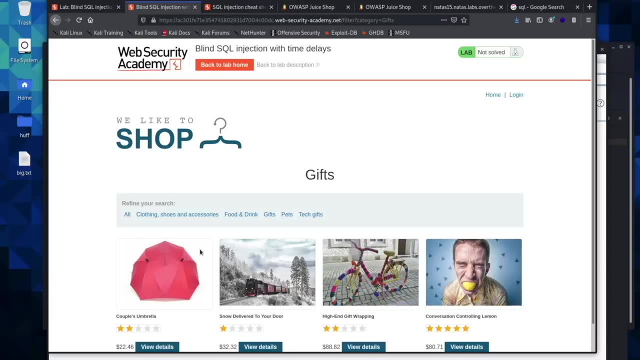 It says it is blind, So it is not going to Have anything for us. I am actually going to Go ahead and go to an item So that I know I am in the right spot And you guys don't have to watch me fumble around. 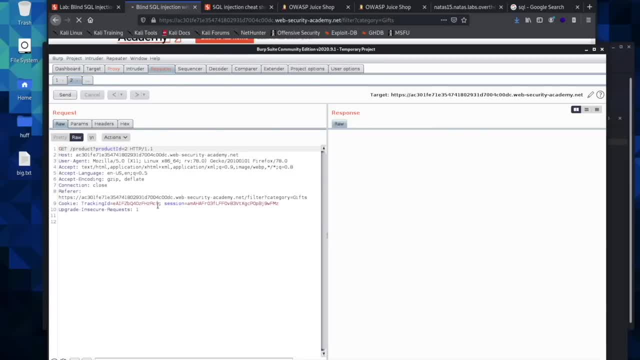 Like you are right now. So we will go ahead and send that to repeater, And the SQL Objection that we are looking for with the time delay Is the PostgreSQL. PostgreSQL right here. So what we will do is We will use this syntax right here. 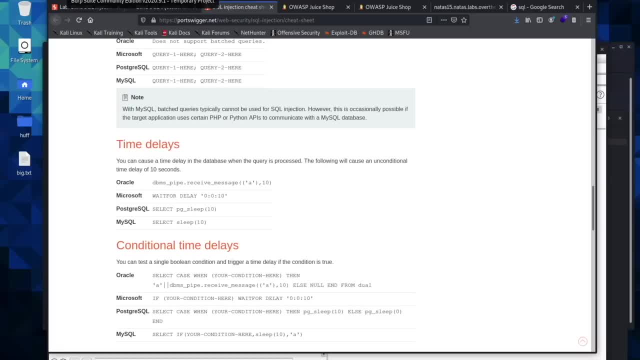 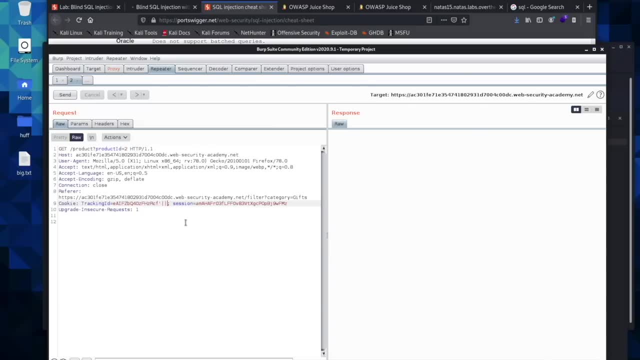 The pgSleep10.. We are going to have to Concatenate it To our query. So it is just two types. Which is just above your enter key Or your return key, if you are on a Mac And then you just type in. 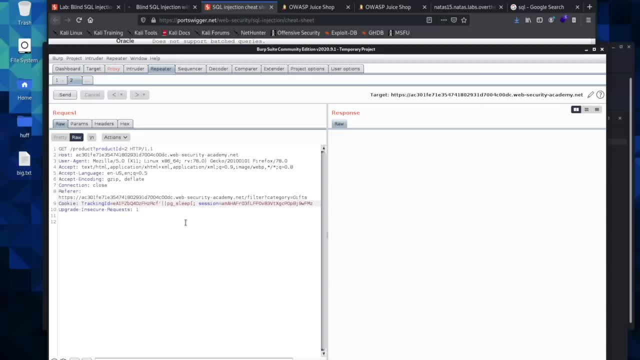 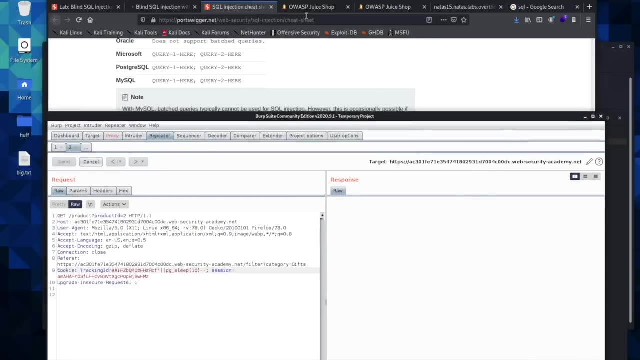 The syntax exactly Like you just saw, And then we don't forget to Comment out the rest, And that should take 10 seconds for our response To come back, And once that response comes back, We should have A solved. 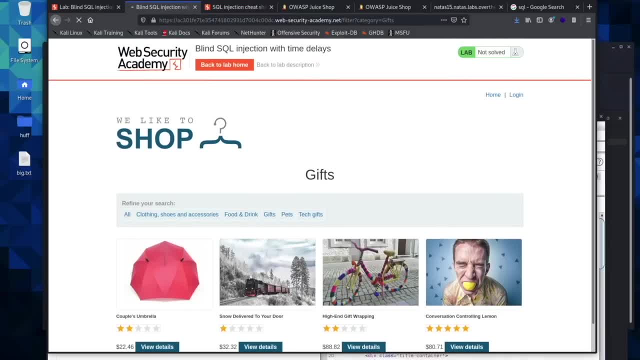 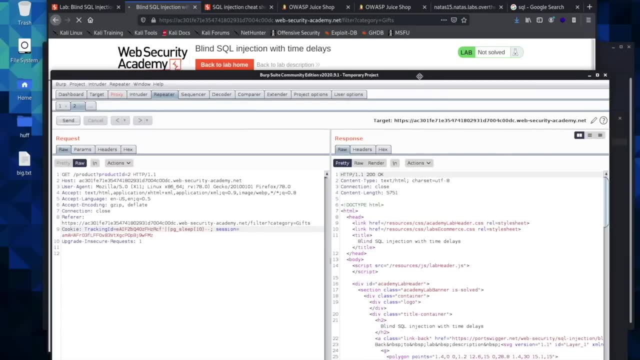 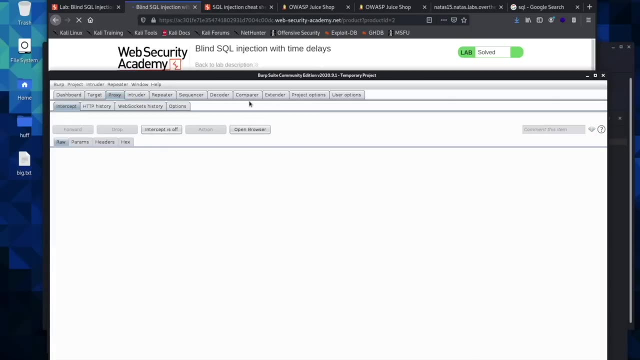 Up here, And so the time delays are really simple, They are really easy to run And This is how you do it. I am not sure why they didn't come back As solved. Maybe we have to go ahead and Forward this. 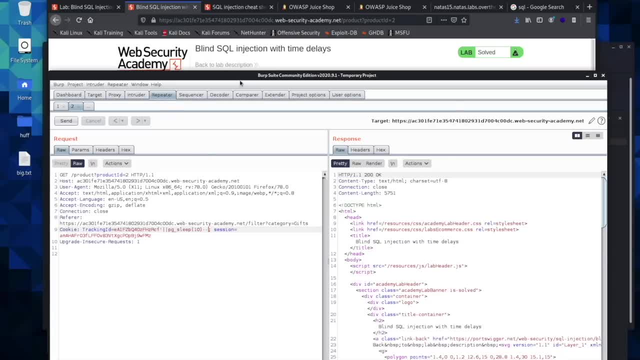 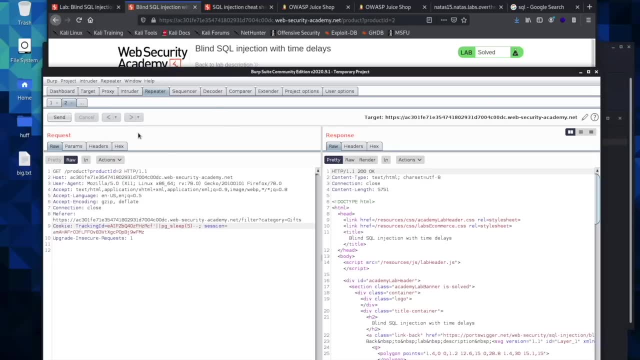 There it is. There is the solved. So they are really simple to run. They are really easy. Proof of concept: You can change this to 5 seconds If you are impatient, like I am, And wait just 5 seconds Instead of 10.. 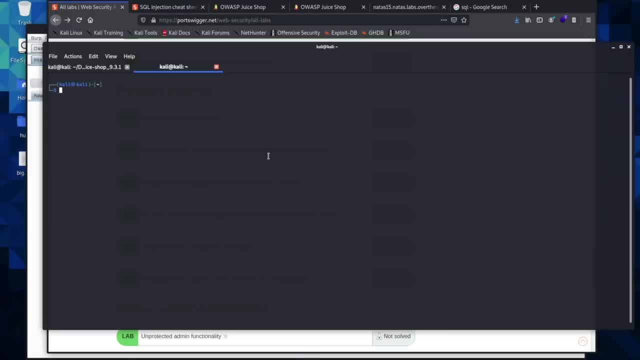 But you have to do 10 here To solve the lab. Okay, we are ready to start Directory traversal. We have talked about this Just a little bit earlier, When we talked about navigating through files And we talked about going through files. 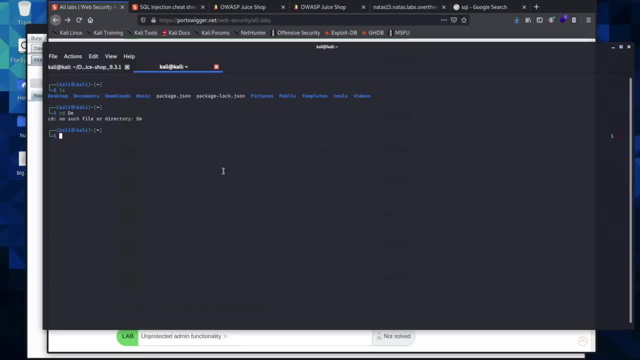 Such as this: So we would cd into the desktop And it changes us Into that directory And so we are able to go between directories And go into different files And the way we go backward. If you remember If I wanted to go back to my home. 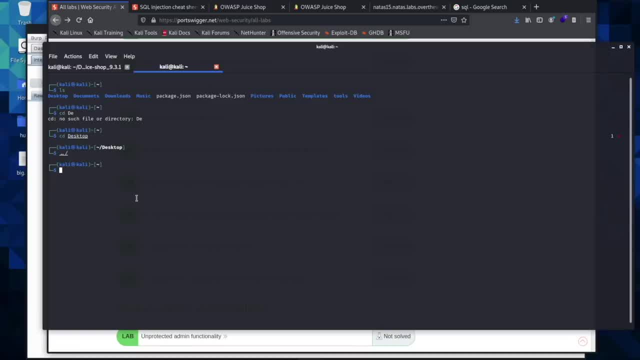 I would just go back one directory, And that takes me back. A good way to practice this- And maybe you have done this earlier- Is to open up your home folder And just up here In your little search bar You can practice going backwards. 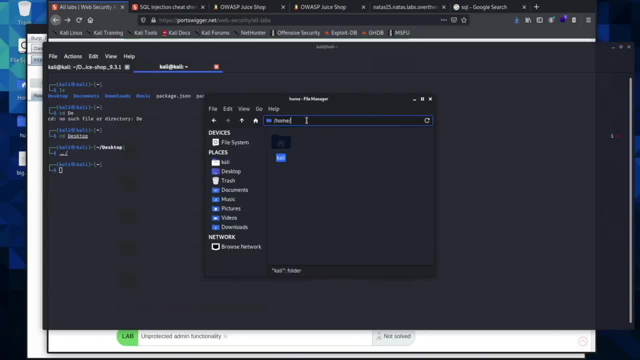 Or you can Practice going forwards, And so we would just be Going forwards like this, And then we can go forward again And we can go into our desktop, And then, if we wanted to go back, We would just do two dots. 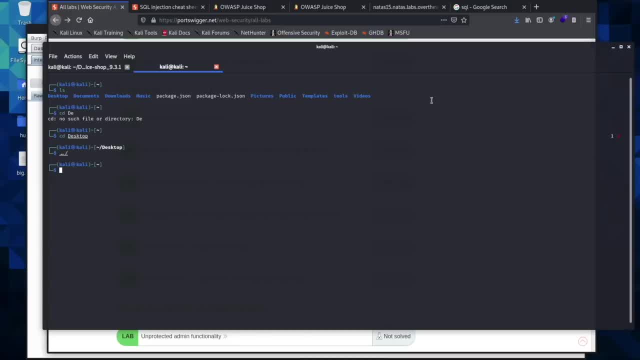 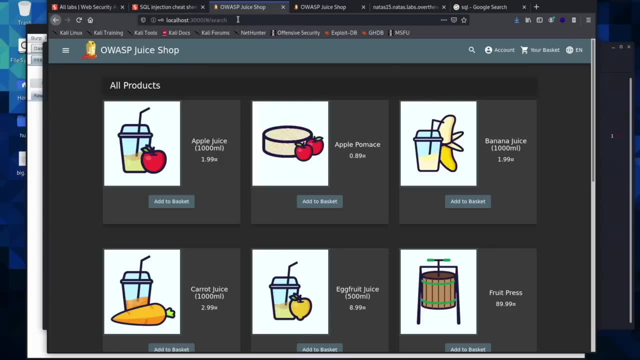 And a slash, And so in directory traversal We will be going through files Only on In our browser. So we would be going backward Through here In the previous lessons, And so we are going to go ahead And open up. 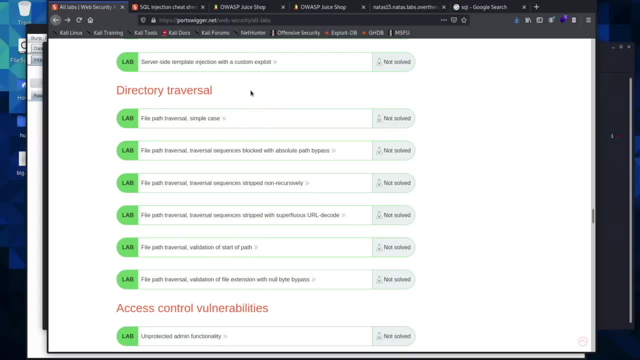 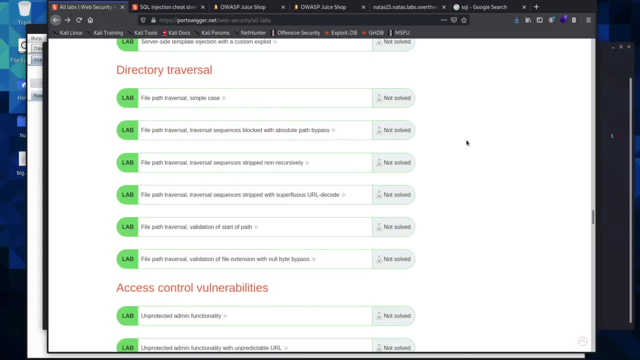 Our port swigger in our labs, And you can scroll down Until you find the directory traversal, And then we are going to walk through A few of these manually And then I am going to show you a tool That does this for you. 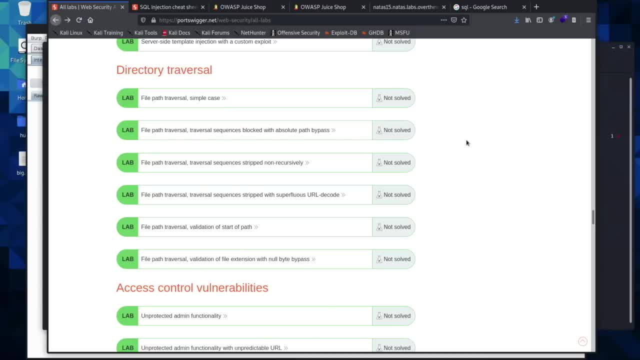 And I will Pull up a directory traversal That is found on hacker one, Just so you can look at it And you can see That these are not Something that is lost out there, And somebody has found them all, Actually, recently. 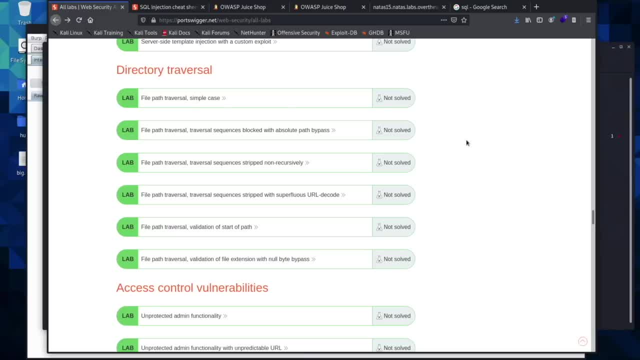 I would say within the last two years, Someone found a bunch of directory traversals. They were able to pull down files That they should have never had access to On the department of defense, And so if you would think of any organization, 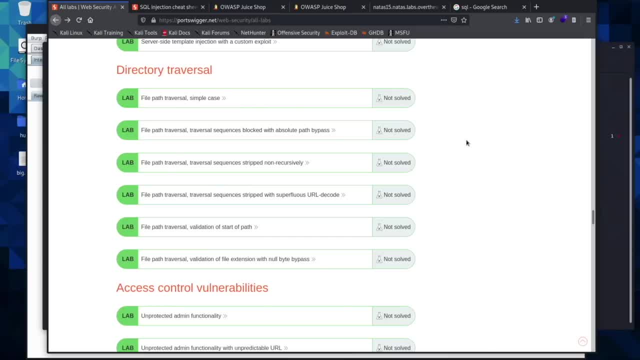 That is going to have good security. You would think it would be the DOD, And these were found Recently within the last two years Directory traversals On the DOD, And so it is out there And they happen. I have actually found a few of them. 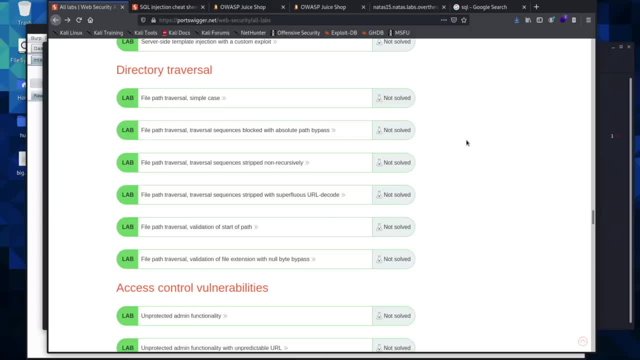 And we will go through them manually, And then I will show you an easy way To fuzz through with a tool That will actually pull down And tell you where A website is Or a web application is vulnerable And exactly which exploit they used. 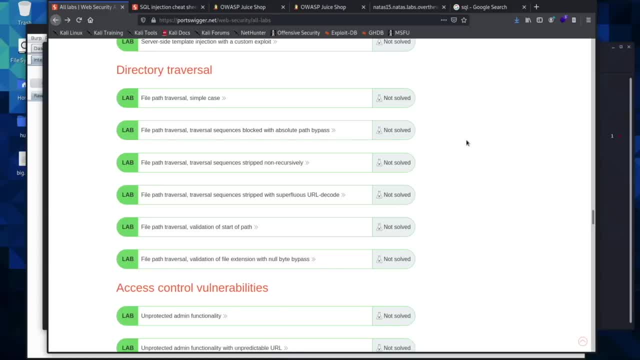 To prove it is vulnerable. So we will do that. After we go through some of these manually, We are ready to go ahead And open up our first lab, And you are going to be able to see Just how easy these are to find. 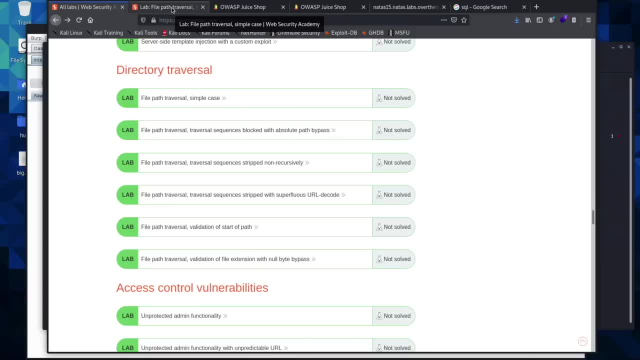 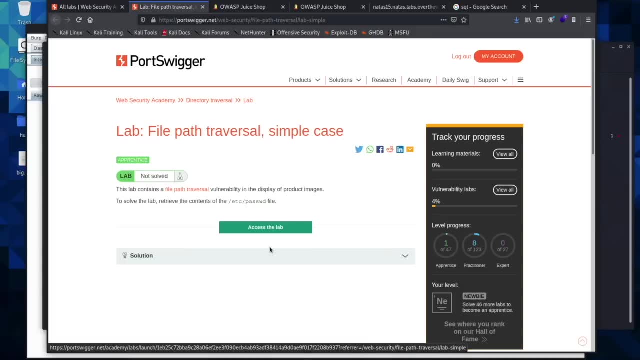 Manually. I think they are really simple And anyone can go and try these With really knowing very little About how the web application Or locating files Works in general. You can pretty much find these Straight off your very first day. 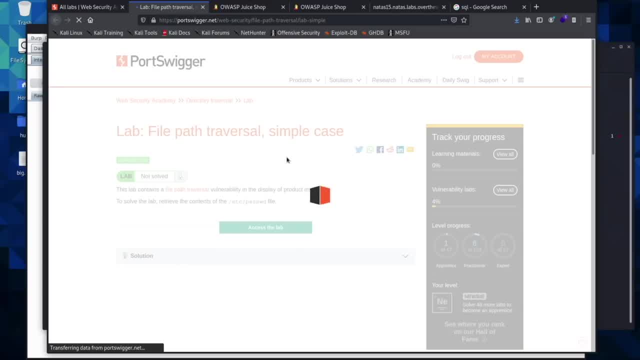 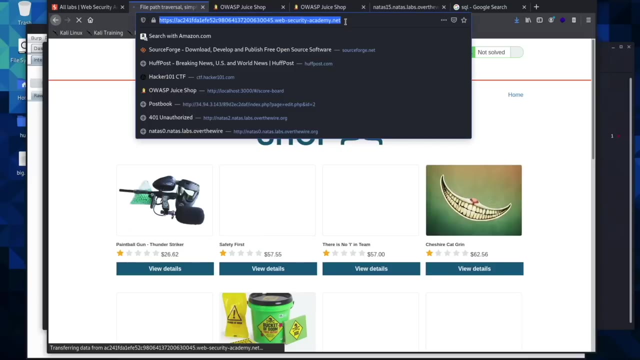 So we will go ahead and access the lab And turn this on, Turn on our lab, And while that is opening, There is a few ways, A few different ways To look for these. Probably the most common Is going to be up here. 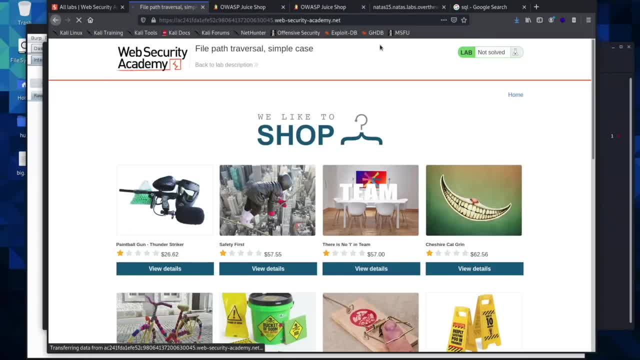 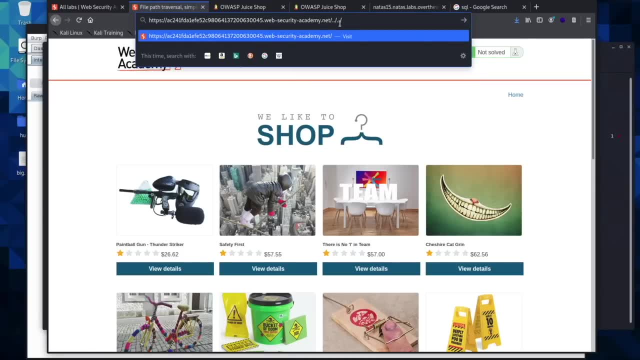 In your address bar. You will come up here And this is where you will search for them. And I will just go ahead and show you What you would do Is: you would pull this open And you would hit your slash And you would go dot, dot, slash. 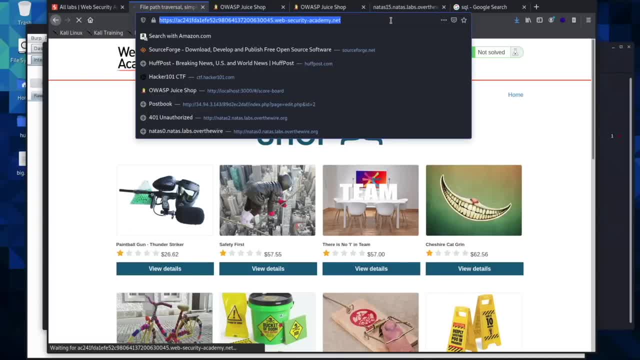 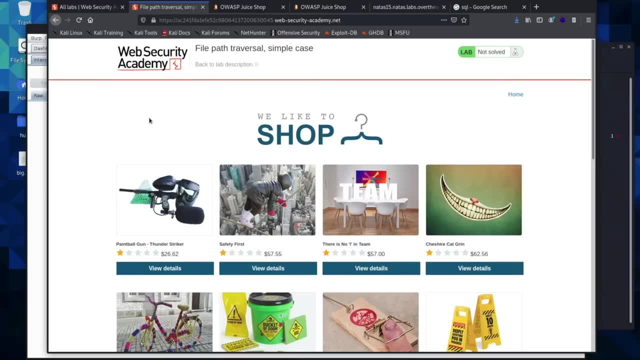 But it is not going to work for us In this bar, We are actually going to have to use burp for this, And so we will go ahead and Turn it on, Turn our intercept on And we will view details. And so what? I am going to go ahead and do. 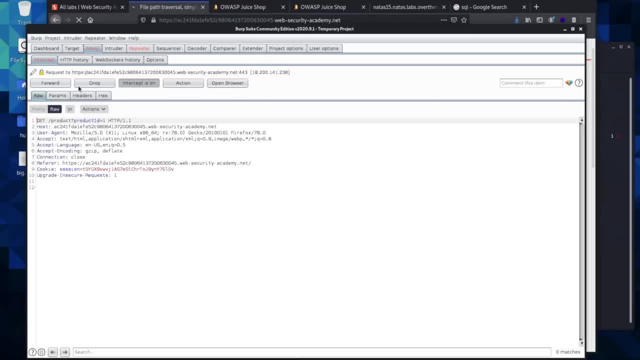 Is send a few of these Requests to repeater, Because I am not actually sure where exactly We are going to find The traversal. So we will go ahead and send that to repeater as well, And I think that is it. 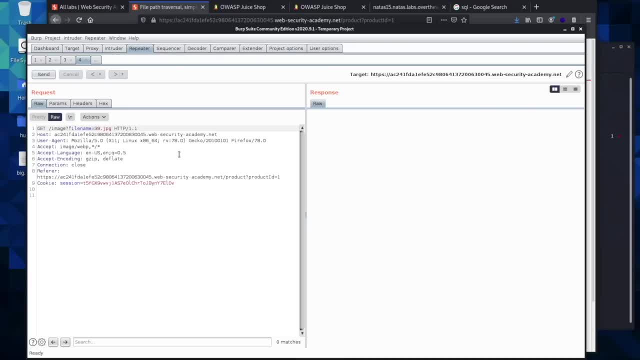 So we will go ahead and open this, And so, if you remember How to go backward in our files, We will actually start with the first one we sent. We will go ahead and delete this, And so we are looking for the product ID. 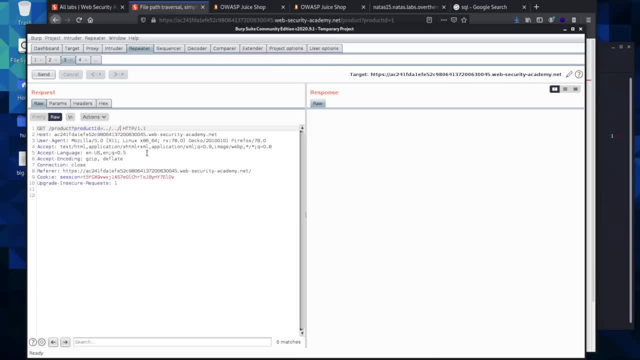 And you would go dot, dot slash, Dot dot slash. And then what we are looking for, If you remember, in the lab description Is the Etsy password, And so we just type in ETC slash password And then you can send it. 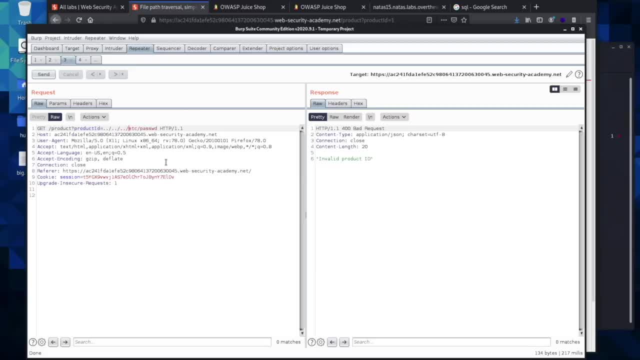 And it says Bad request, And so we will go a couple more And see what happens. Okay, So we are getting a bad request. What we will do is go over to our other Get request, And we will go ahead and do the same thing. 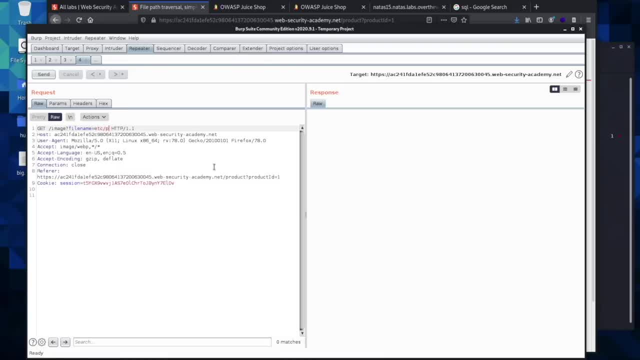 I like to go ahead and start out Just like this And then add to The path traversal As we go, And so I just go Just like this And see How far We have to go Before we can actually find. 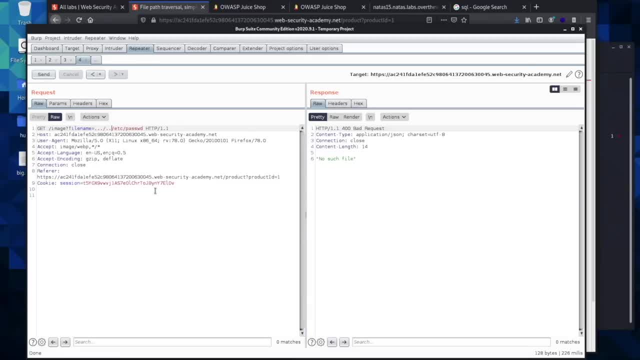 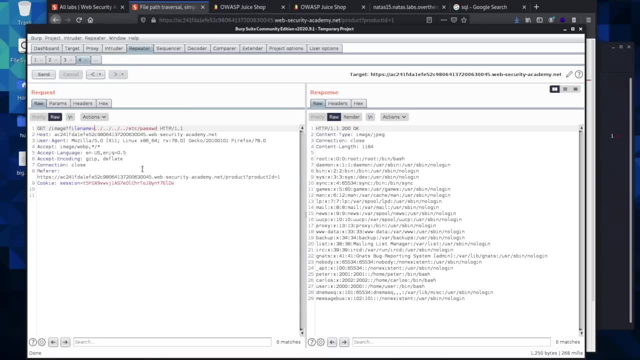 The files, In this case before we solve the lab. Okay, so there, it solved it. So it goes back To the root folder And then it goes forward Into this file, And then it will go forward into the password file And then it pulls down for us. 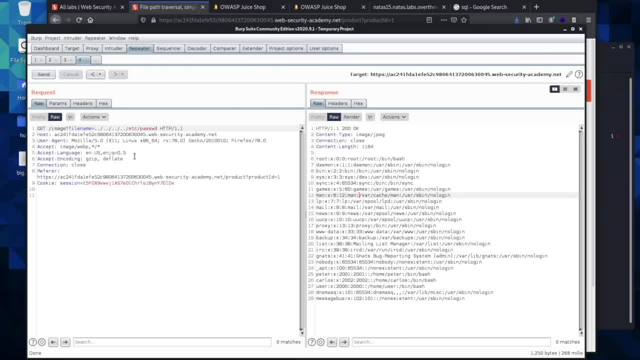 Information that we should not Be able to have access to, And so for us, This should solve the lab For us. So each one of these just goes back one file, And it goes back until it hits the root folder, And then it will go forward. 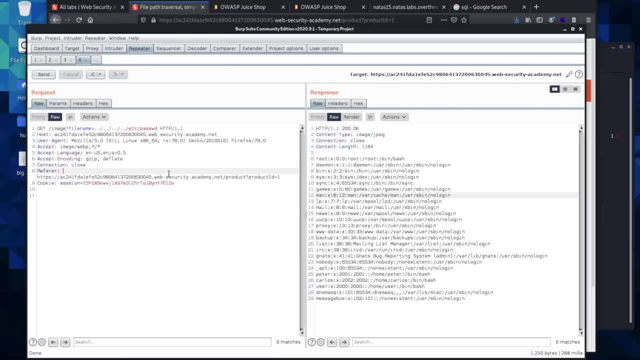 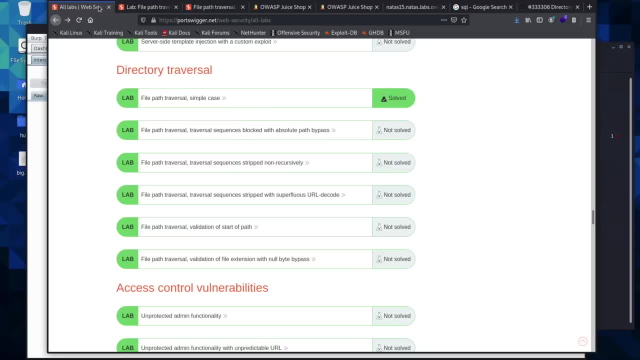 Into this directory, Into this file, And that will give us information That we should not otherwise have access to. Okay, We are ready to Go ahead and solve our second lab On path traversal. So you can go ahead, I think, with what you have learned. 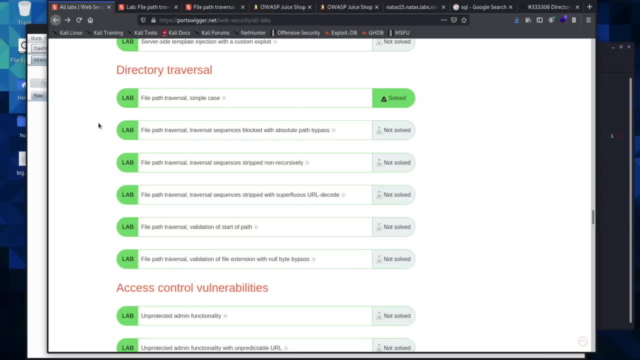 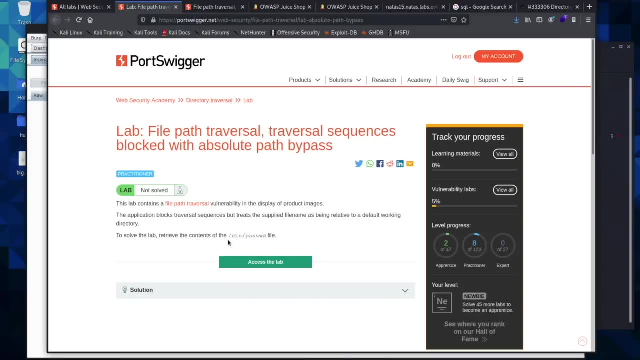 So far, in the very first lab, You should be able to solve the second lab On the directory traversal. So if you want to go ahead And give it a try, You can open up the lab, Which I have already done, And you will be looking for the same file. 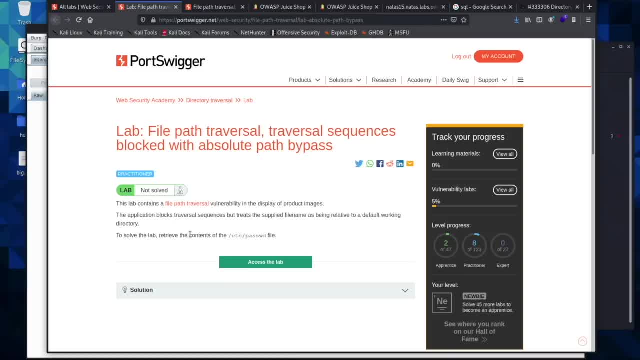 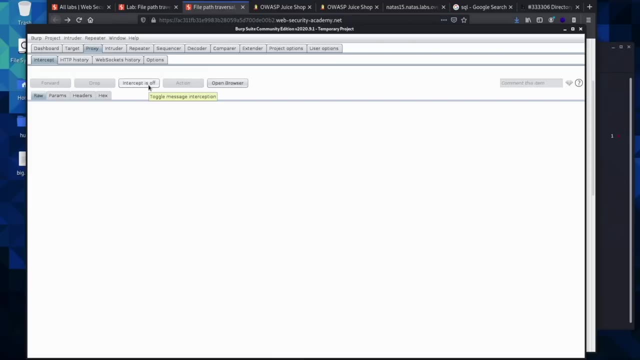 We were looking for last time, The etsy password file, And that will solve the lab for you, So you can solve this challenge. Okay, How did that go? Hopefully you were able to solve it Without any trouble. If not, we are going to go ahead and walk through it now. 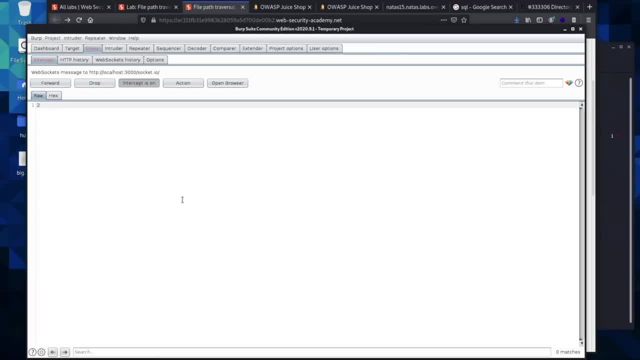 We are going to go ahead and turn on our interceptor And we will click one of the View details Just to make sure we can pull down The same Get request we had last time, Which was not the product ID, It was the image file. 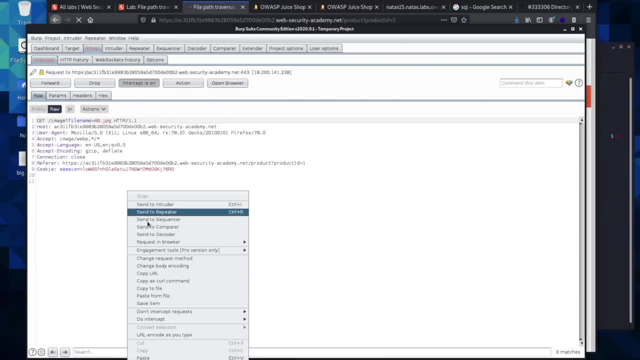 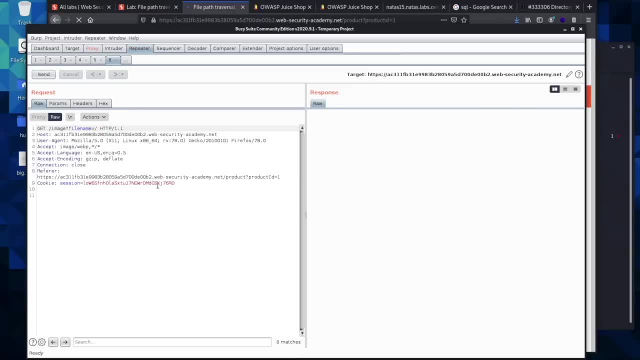 The image file name. So we will go ahead And send that to repeater. And while we are over here, We are going to start out just the same way we did last time. We are going to come in here And start with our etsy password. 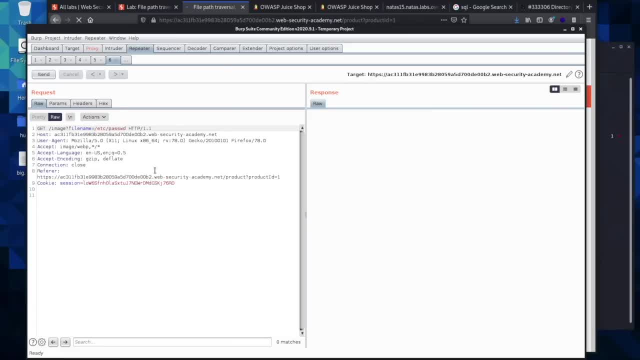 And then, as necessary, If we need to, We will go ahead And add in the dot dot slashes, But we always start at the beginning And go forward if, Or go backward if necessary. So we will go ahead and send this. 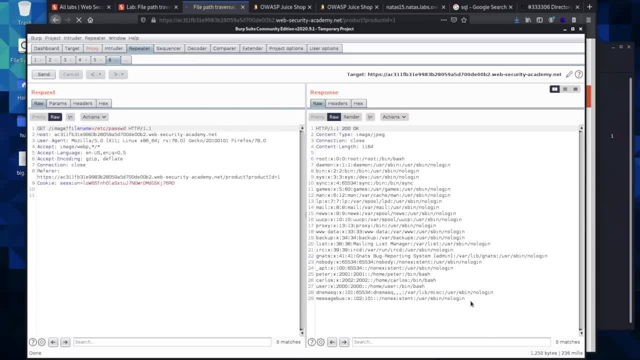 And it can, And come back on the first try. So hopefully You were able to solve that challenge, Because they are going to get a little more challenging To do manually, But not all that difficult for us. Okay, we are ready for the third challenge. 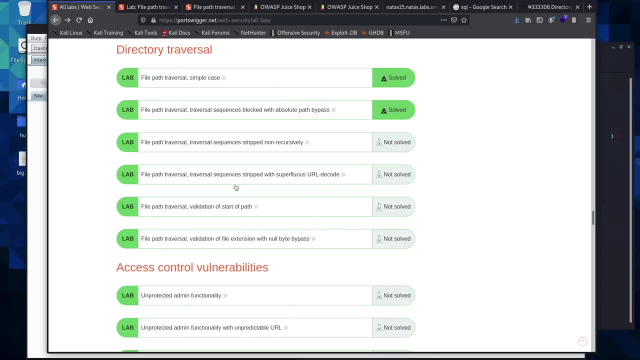 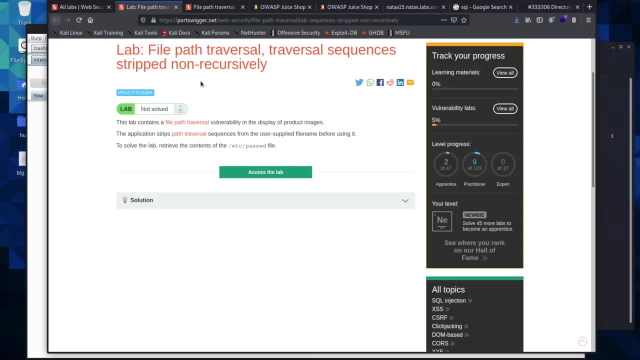 That we are going to be looking at For the path traversal And this one, we are actually told What has happened. So go ahead and open up this lab And we will see Our instructions here, And we are told that The sequence is stripped away. 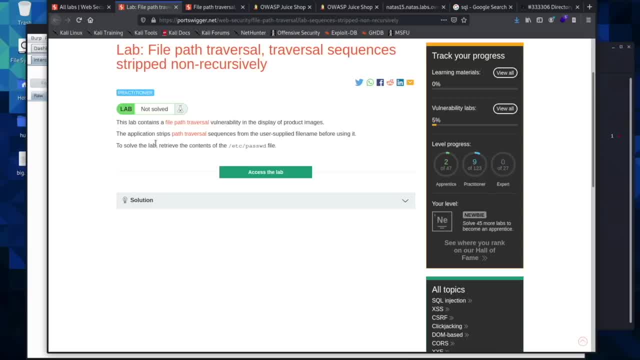 Non recursively, And so what we will have to do Is modify the attack Just a little bit And pretty regularly. Especially with cross site scripting, You will see developers That know of a way, Or maybe a few ways, That an attack can be performed. 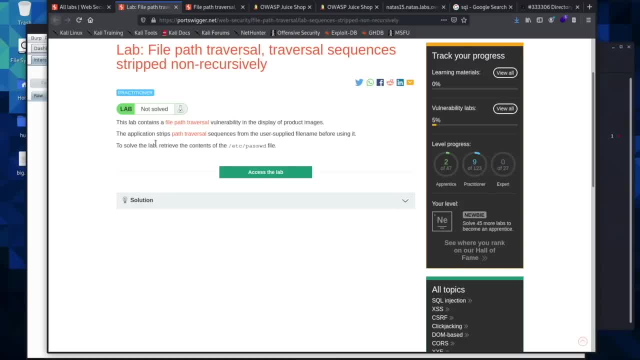 And so they will just go ahead And strip out just specific elements Or sequences Within a Attack or a payload, So that they won't go through. But there is almost always Another way to pull this off, And so actually in this lesson, 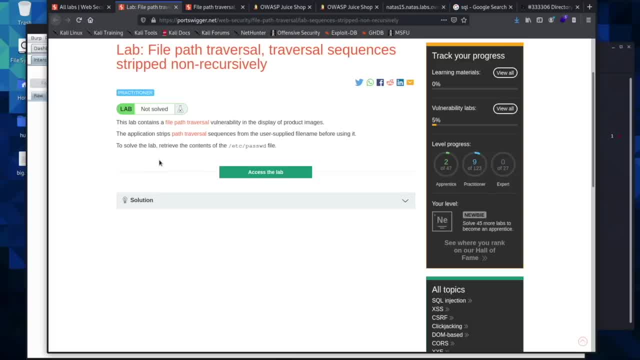 And the next one, We are going to be able to observe Just how you change payloads And really, in bug bounty hunting, What you are going to be doing Is a lot of trial and error Until something works, And so we will go ahead and open up this lab. 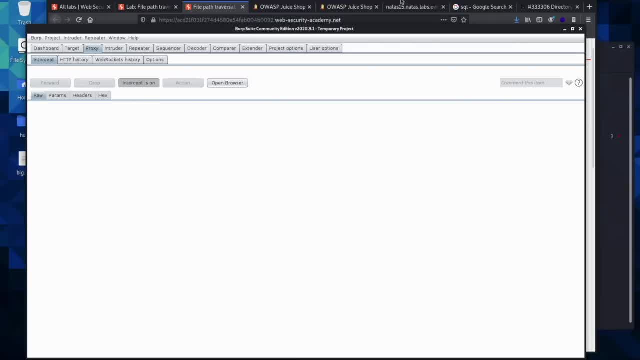 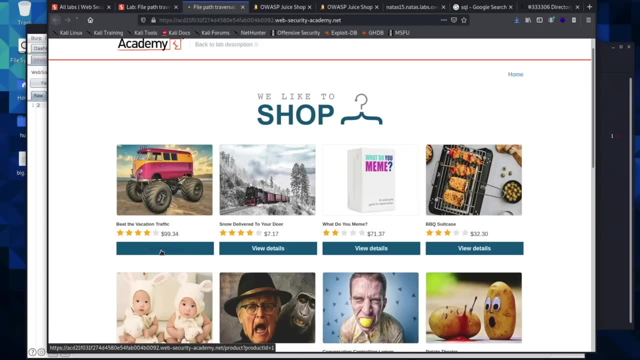 And once you are in here And you are using your intercept, We will go ahead and turn that on And my son would think this is the coolest toy ever, And so we will go ahead And view the details. We will get our get request. 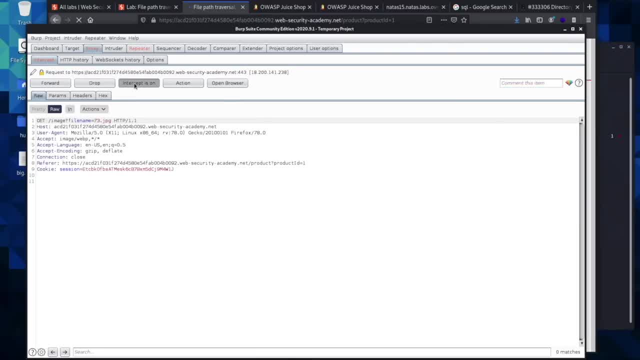 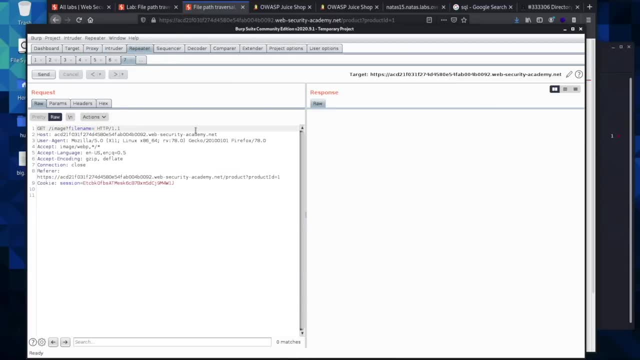 That we need right here. We will send it to repeater, We will turn the intercept off And once we are in here We will go ahead And we can start out With the etsy password, And then we will send this. 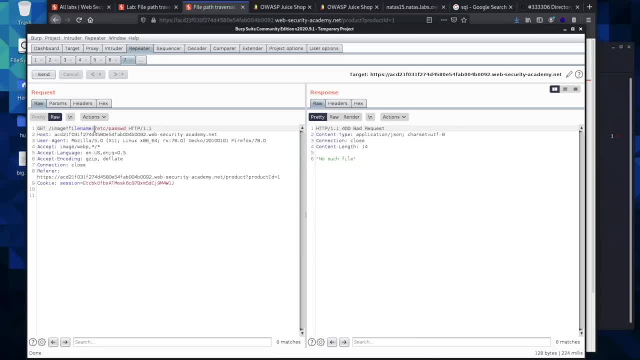 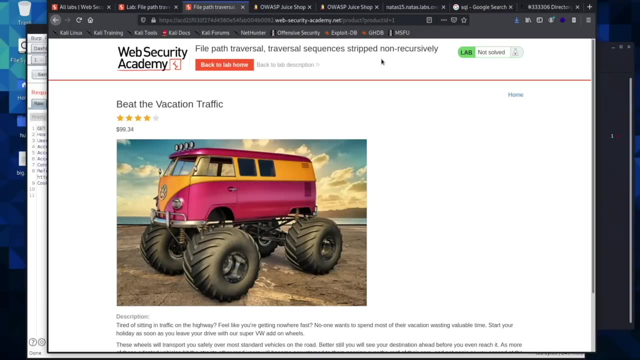 And it comes back With a bad request, And so you can go ahead And try going back, And it comes back With a bad request. And I actually know what is going on, Because we are told That the traversal sequence- 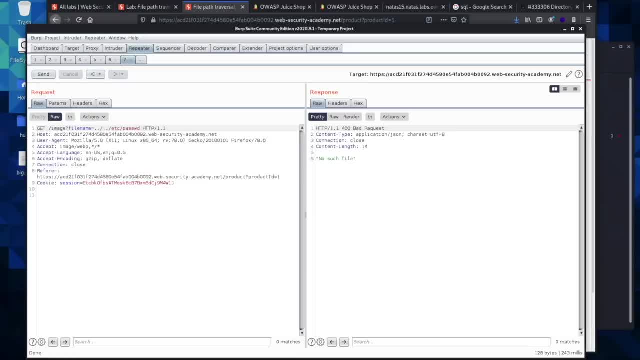 Is stripped away. So what we will have to do Is try something different, And so what you can actually do Is go four dots With two slashes, And then this is A different process In pulling down The etsy password file. 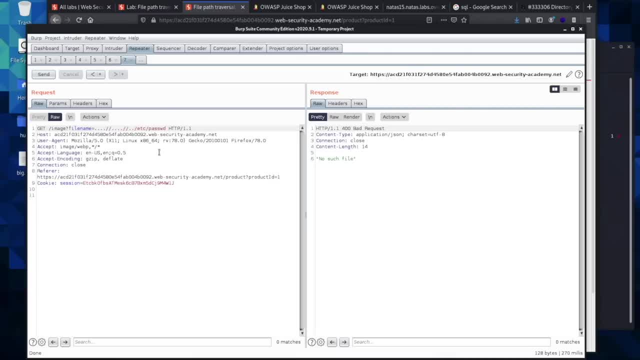 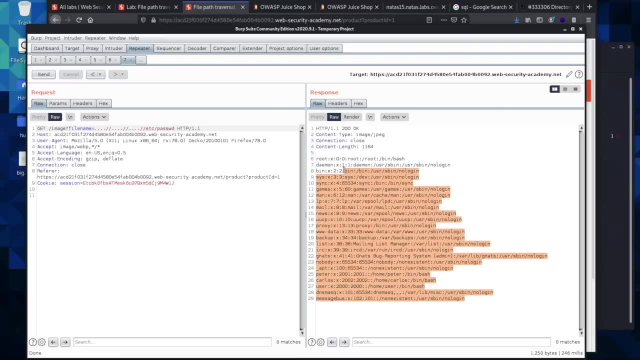 So we will send this, And then we will One, two, three, four, Continue going And we are able to find The file we need. Now, when it comes to remembering All of these Different ways that you can try and find, 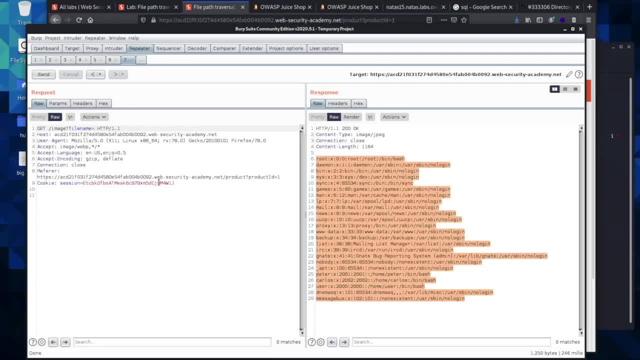 A directory traversal. It is not necessary To try and remember these. That actually does all of this for you, With Hundreds and hundreds Of different ways To pull down an etsy password file, And so I am just showing you. 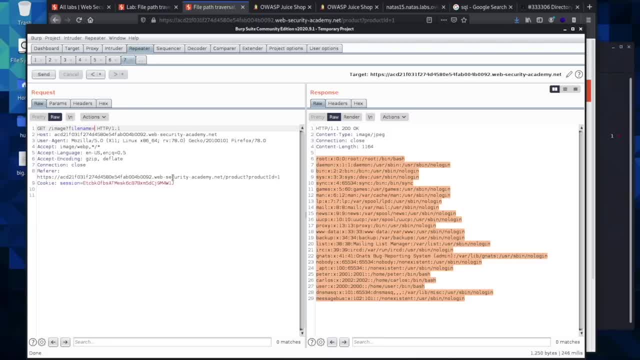 Manually how this works, So that you know what is going on And you know how to find these, Just in case you are not allowed To run a scanning tool Or anything like that On a specific web application. But you do not need to try and remember. 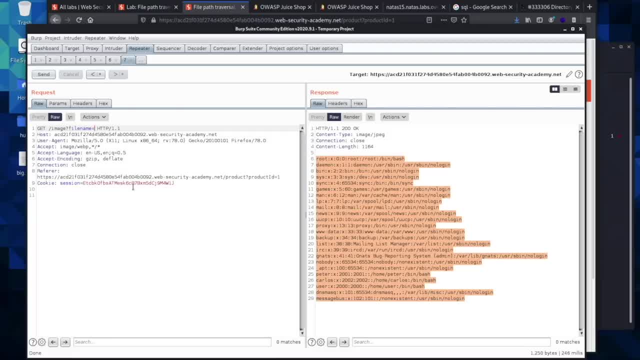 All of these different ways To pull down the etsy password file, Because you will have Sources available That can do it for you Or remind you exactly how to pull off these attacks. Okay, we are going to be Working through our final path: traversal. 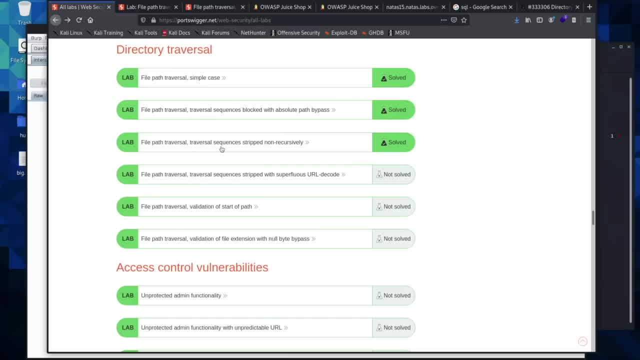 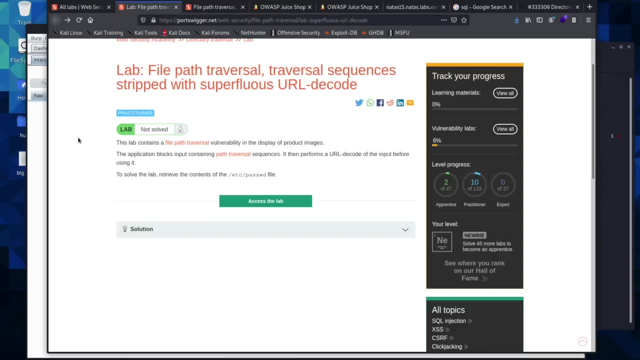 Before we Look at how to do this with the automated tool, And so you can go ahead And open up this lab And in here we can Read our instructions And exactly how to pull this off. And so we are told that. 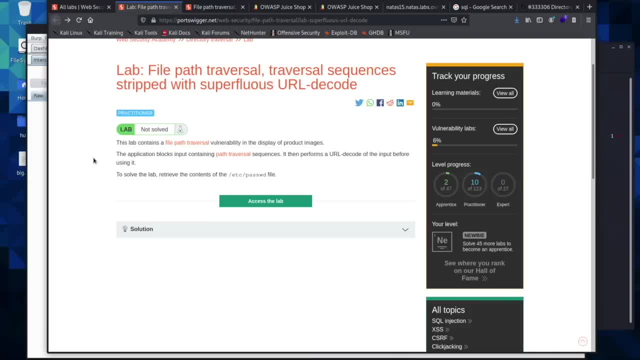 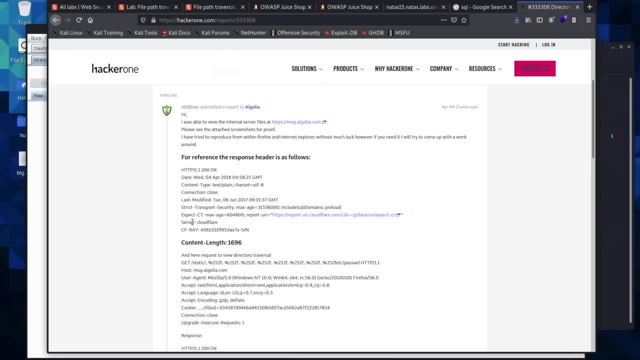 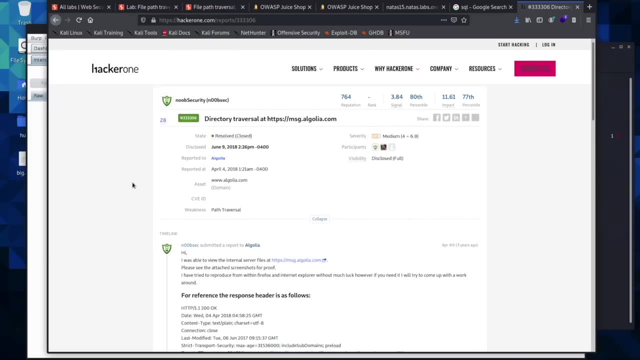 It has URL decode in it, And so This is actually Very similar to A exploit that was pulled off, And I came across this Not too long ago When I was looking through Path traversals and how they were pulled off. 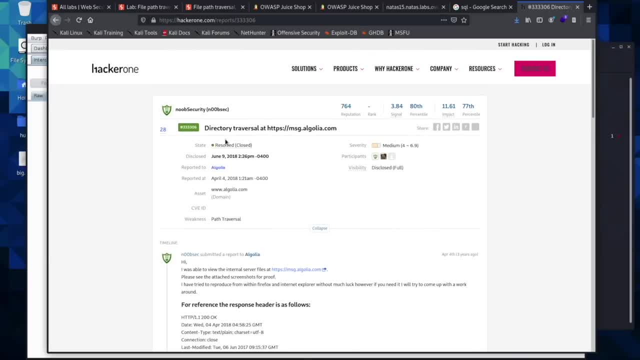 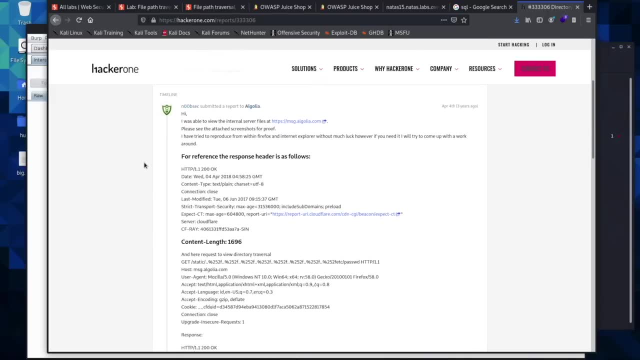 On the hacktivity, And so we have. This was done June 9th 2018.. So quite a while ago, A couple years, But this is going to be pretty much The exact same exploit We are going to be doing in this lab. 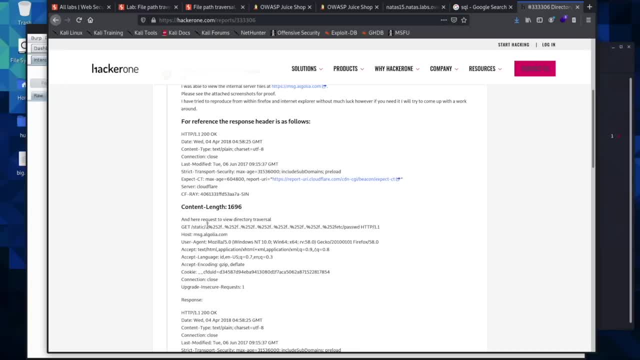 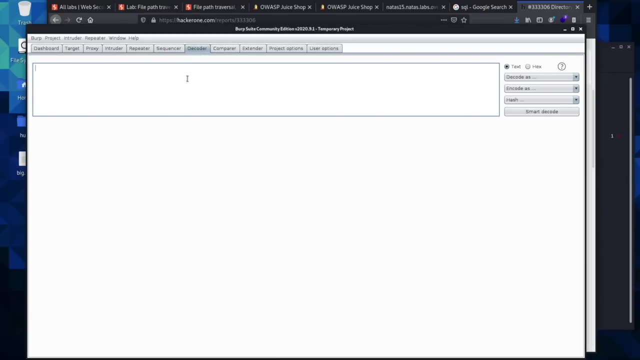 So just to show you That these labs aren't Just theoretical, But they actually do Help you perform these exploits, And so you can see here, This is the URL encoding, And so a simple way to look at URL encoding. 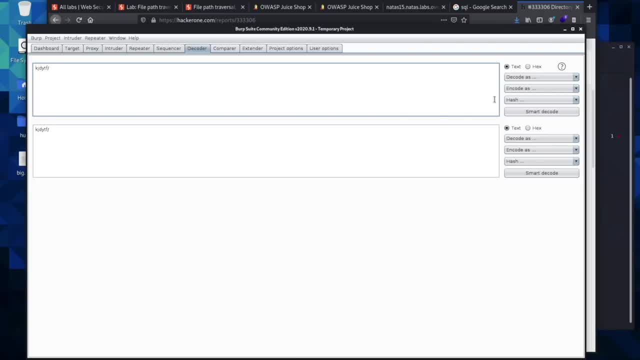 Is. you can come over here to the decoder, You can type in some gibberish And then you can encode it As URL And you can see the URL encoding Pulled down here. And so what we are going to be doing, 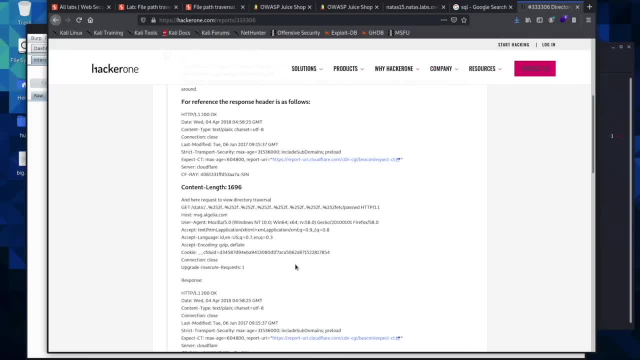 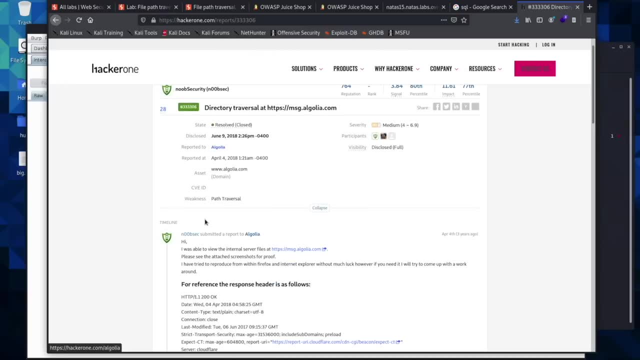 Is doing something very similar To what this guy has done here, And you can actually see He actually paced It- pulls down the file That he should not have access to. So what we are going to do Is come in here. 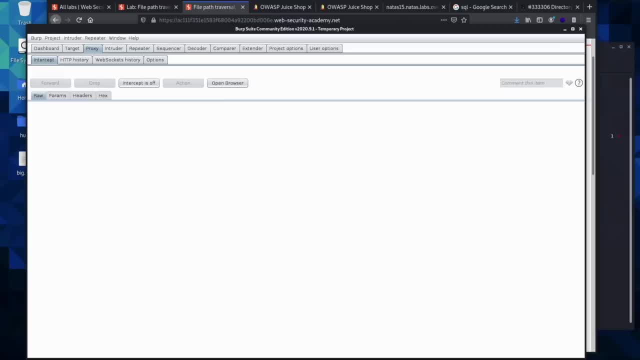 You open up the lab, Click access to lab. Same as we've been doing in the last few lessons. We'll open up burp And we'll look at the files. Of one of the files We will look for the get request. 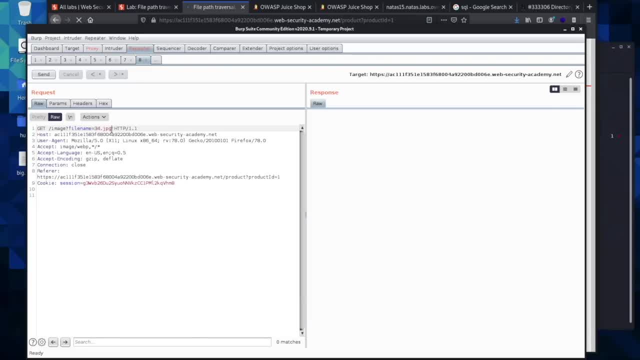 With the image file name, Send it to repeater. And now what we are going to do Is very similar To what we just saw, So we'll start out Just like normal. You can go ahead and send this, And then we are going to type in: 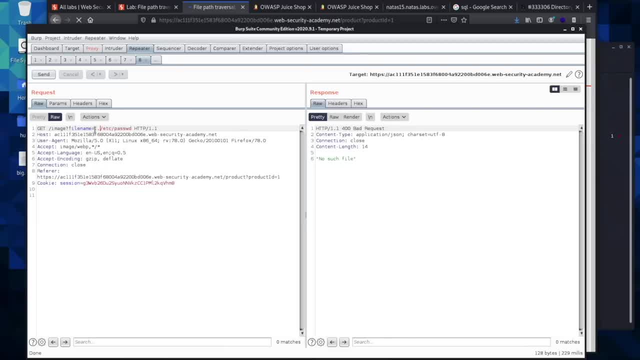 The URL Encoded version Because it's going to decode it for us. Send 252f And that should Pull it down For us And we'll go ahead and delete that Because it's encoded in there So we can send that. 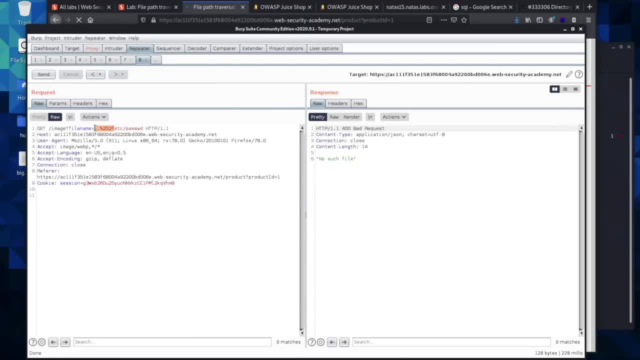 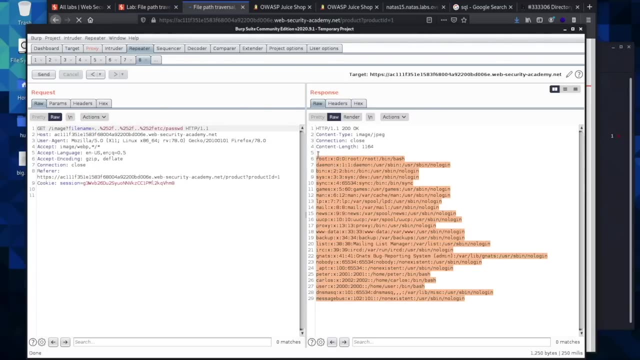 I'm going to do, Rather than type this Is I'm going to go ahead and copy it And then paste it, And then send it, And then paste it And then send, And there we found the file, And so you can actually. 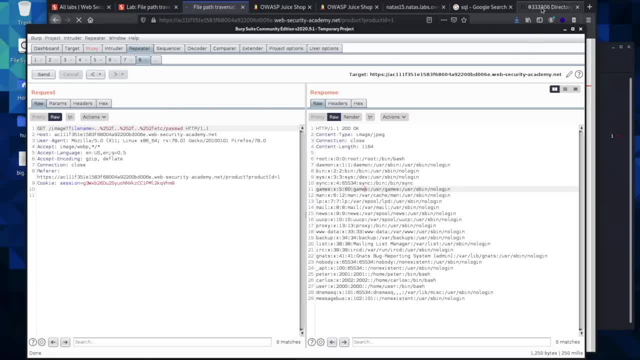 Really easily see how this is very practical Here. we are practicing it Here. someone actually pulled it off On a live website And so if we come in here And we turn our proxy off, We should solve the lab. And so in the next lesson. 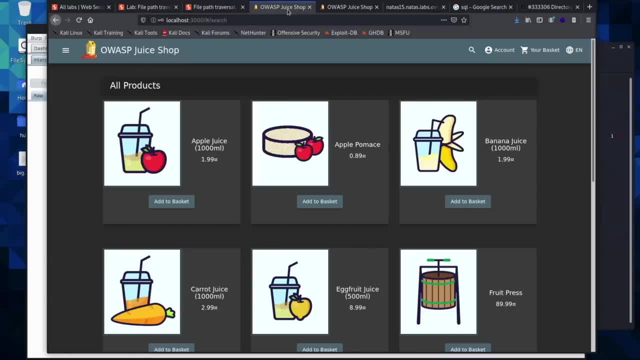 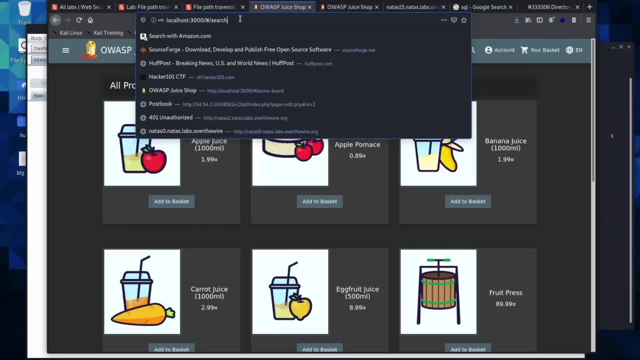 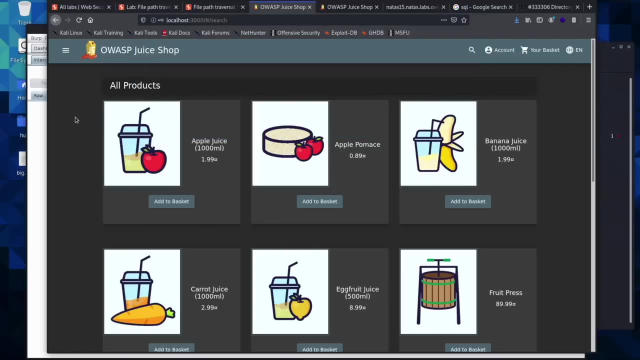 You are going to be required To open up juice shop, Because this is the URL we are going to be using To pull off the attack On our Automated tool, So you can go ahead And open up juice shop And get it running. 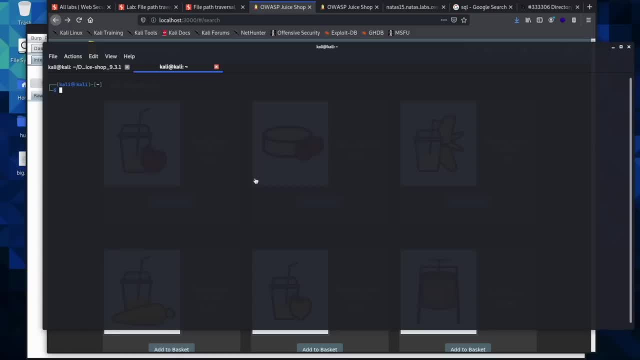 Okay, we are going to be looking at the automated way To find directory traversal Exploits And so you can go ahead and open up A terminal And have juice shop open And running. And just to make sure you have the tool installed. 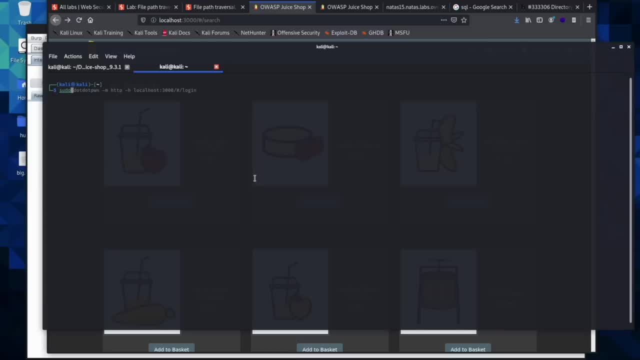 You can come down to your terminal And you can type in: Pseudo apt get installed. It should look exactly like this, And then you will hit enter. It will require your password And you can go ahead and type that in And it will run. 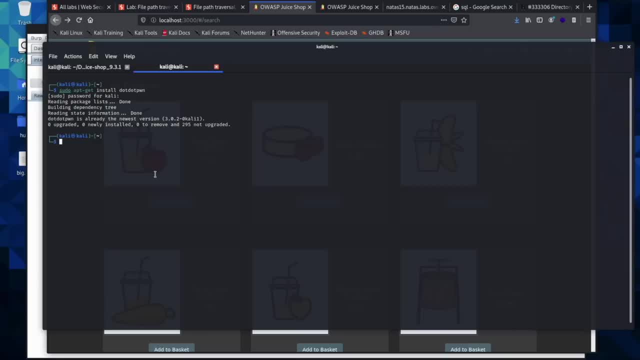 And it might ask you: Are you sure you want to install? And you can press y And then hit enter or return, if you are on a mac, And it will install, And so the way to run this tool Is very, very simple. 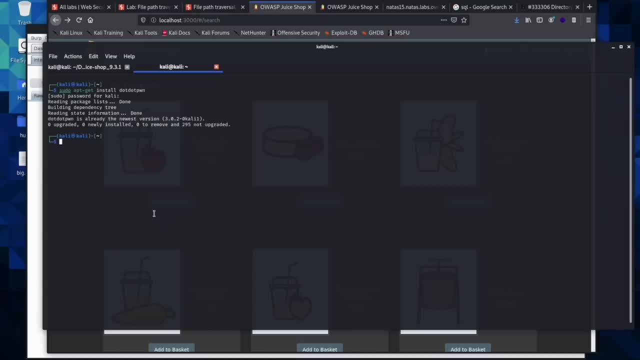 You would just type in Dot dot pwn And then we will give it The corners that we want it to follow. So we will just type in Dot dot pwn And then we will go dash m And this is. 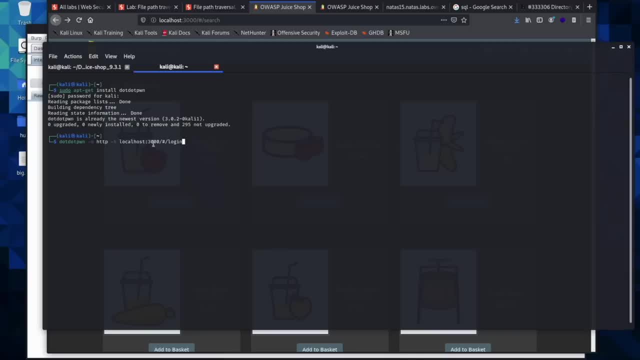 I actually already ran it Just to make sure it would run on our local server, And so this is what you will type in. You will type in dot dot pwn, And then you will flag m http And then you will flag h. 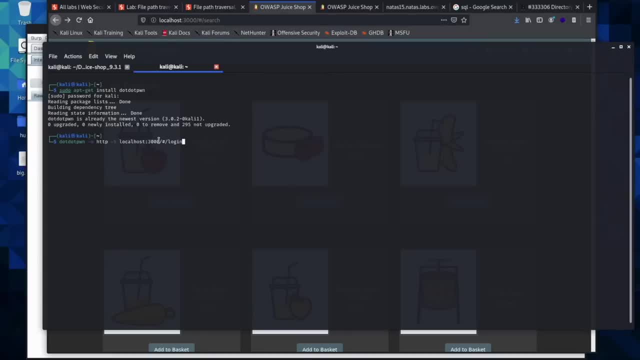 And it is our local host, And so I actually just came up here And copied and pasted The page I was on And it is running. It will run for us. Oh, it did not run for us, Because we have to run it as sudo. 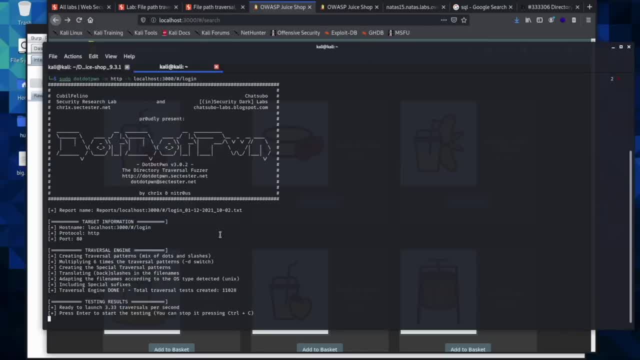 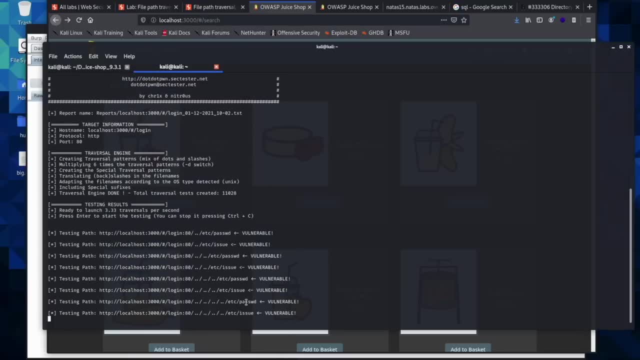 As our super user. And now it is running And it will ask us Press enter to start the testing And then we will go ahead and hit enter. And now you can see, look It is running. all of those for us With the dot dot slash, dot dot slash. 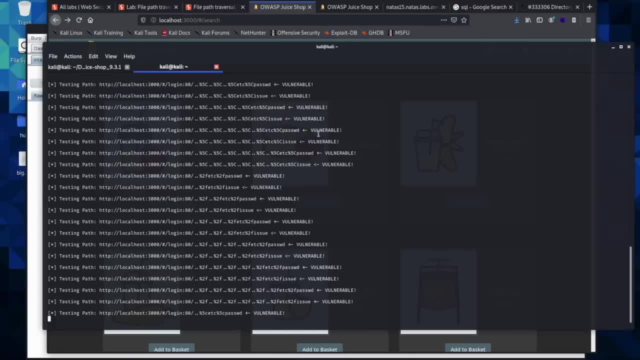 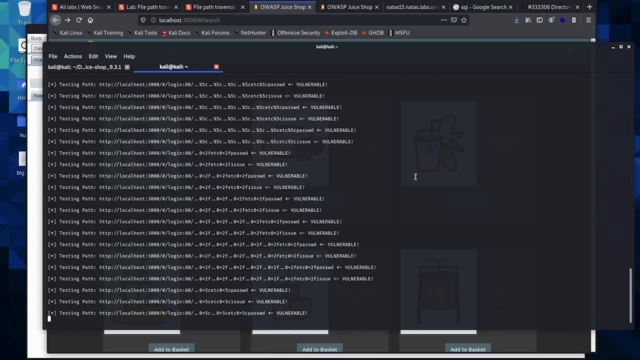 And then it encodes it And it just runs through. Now this web application is vulnerable. I think it is vulnerable to all of them. They did not do a good job When building the web application For making it secure to this attack. 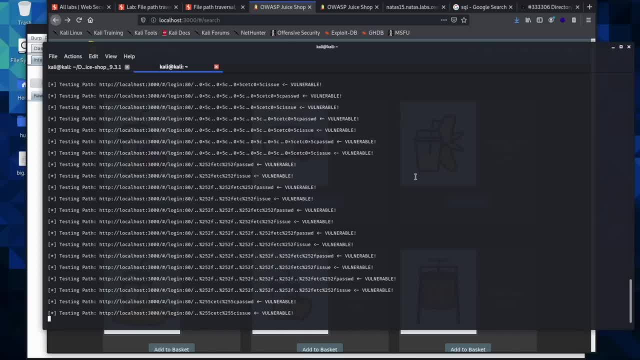 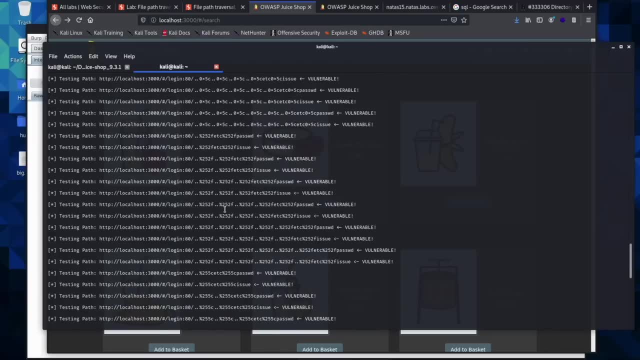 And it will run. And there are hundreds Of different ways to send. There is the one we just saw With the percent two five, two f And it runs it for you And it will tell you. For us it would have been right here. 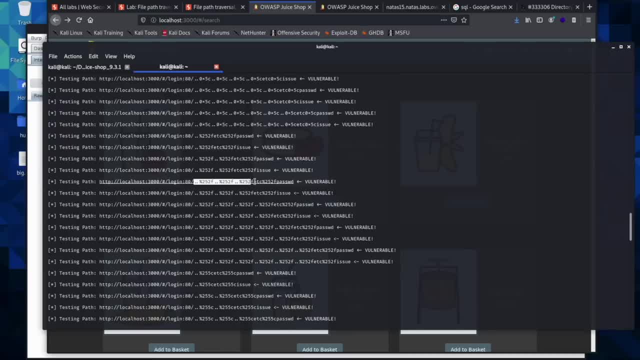 We would have had three paths to go back Before it goes forward Into the etsy password, And so it would have found it right here. It would have flagged it as vulnerable. So now you can see just how easy it is To run this. 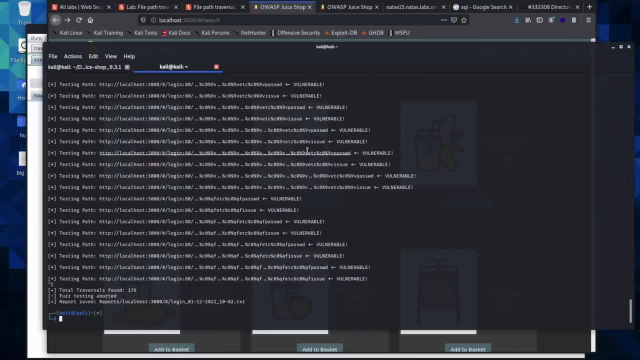 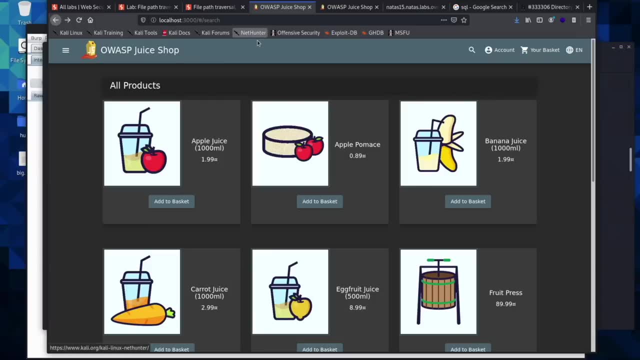 With this tool And you can go ahead and hit command c To close out of it so that it will stop running And it might have actually Went ahead and solved A challenge for you. If it didn't, You can go ahead and type in. 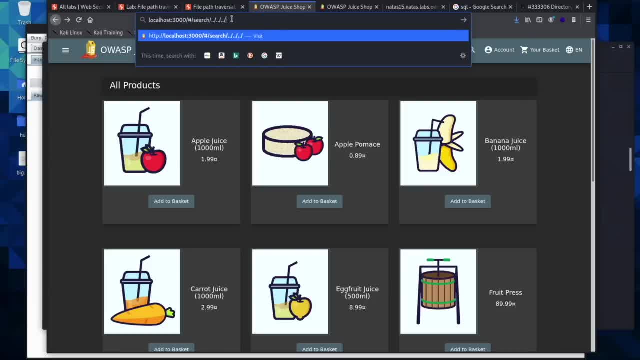 Dot dot slash, dot dot slash, Dot dot slash Any of these Because it says it's vulnerable to them, And then type in etsy Slash password And it should pull down. I think I already solved the challenge- It should pull down that we have accessed. 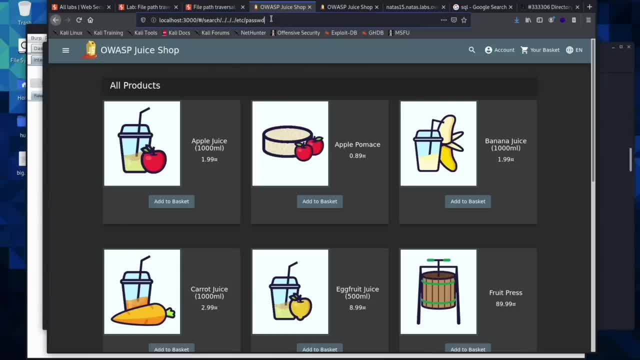 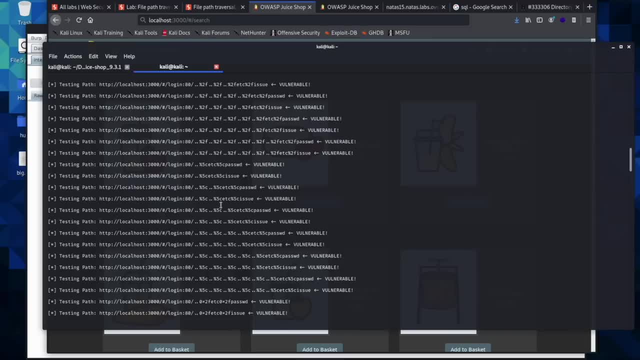 A file that you should not have had Access to, And so that will solve that challenge for you. It's pretty simple. Running this tool is really easy, And it takes a lot of The manual testing that we just did Out of account for us. 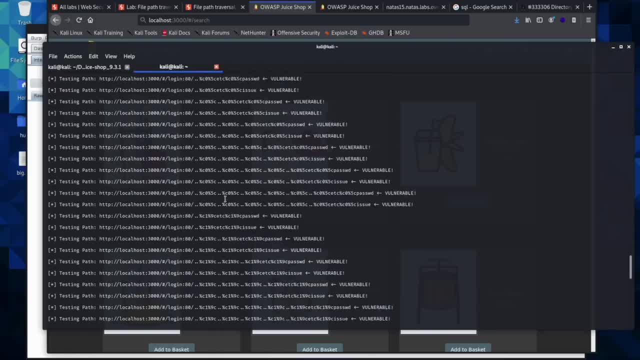 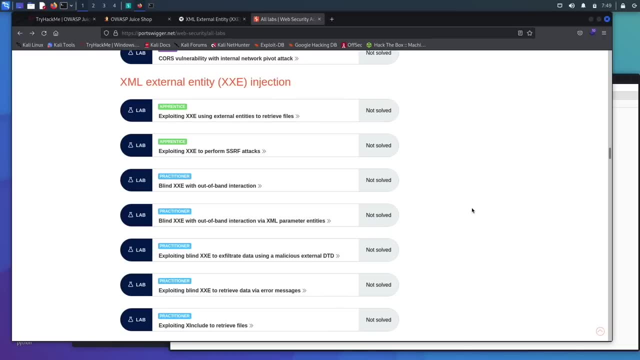 And you can find hundreds Of different ways to find a path At traversal. Okay, we're going to start by looking at the XML injection at this point And we're going to start a really easy XML injection. This is one that you're going to see that's probably the most common. 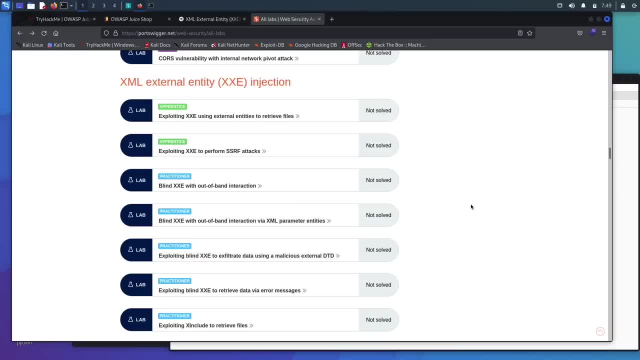 And then from here, we're going to look at Some more uncommon XML injection methods, But they're going to be a lot more severe, And so this first one is really simple. You can go ahead and open up this Lab on port swigger. 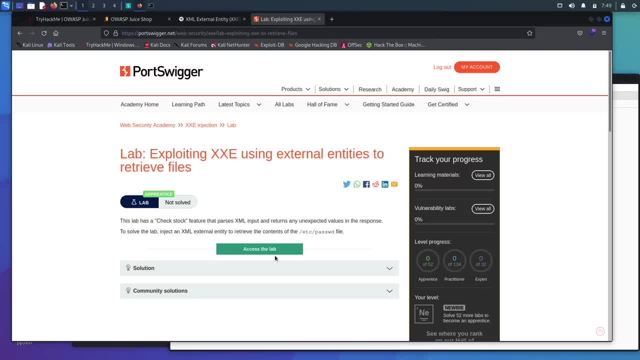 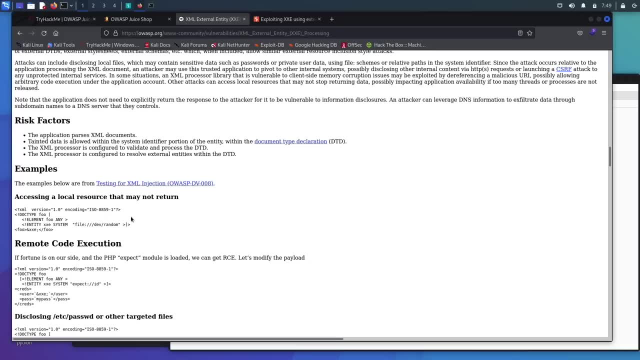 Right here And I want to walk you through. We'll go ahead and click access lab. I want to walk you through What is happening. So, when we look at this XML injection, I want to focus just on these two lines. 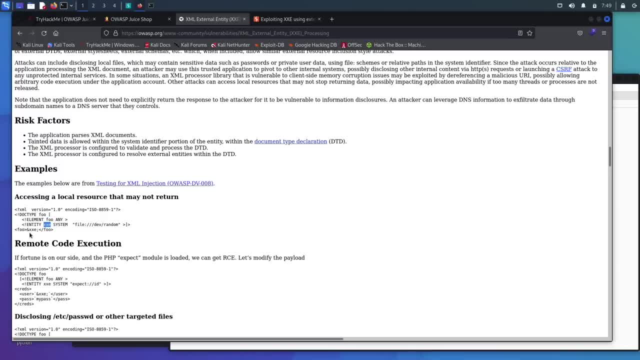 When you see this xxe right here, We can change this to be anything we want, And we see it down here. It is the same thing. This is the xxe being called And telling the xml file That we want it to do something. right here. 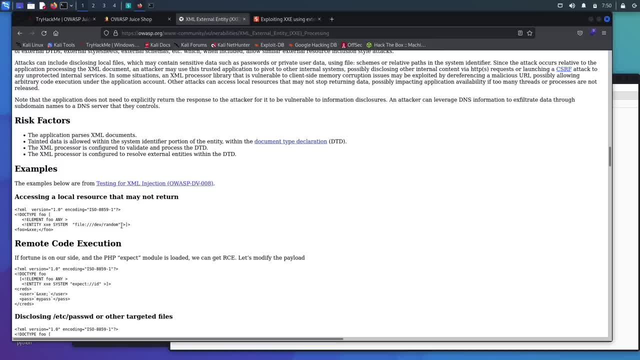 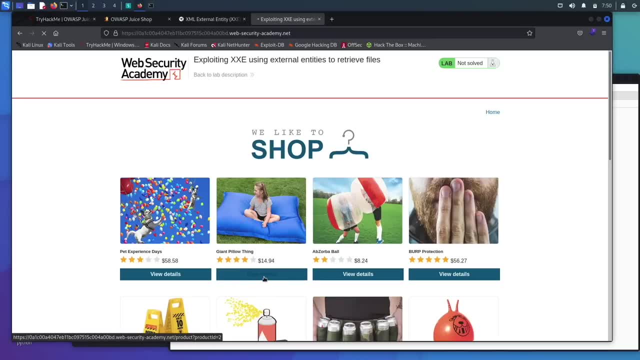 So we're going to tell the system To open up the xxe passwd file, And so I will show you What this looks like. When you come up here And you click view detail, We will need to turn on burp. 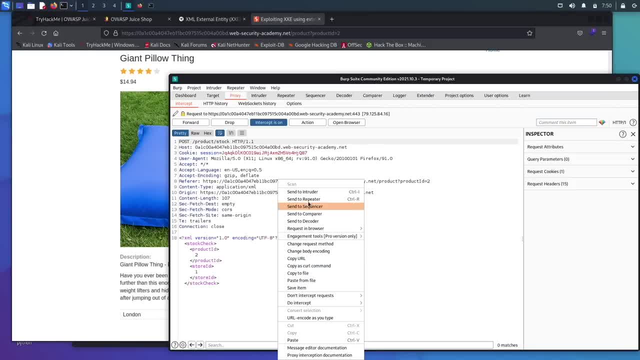 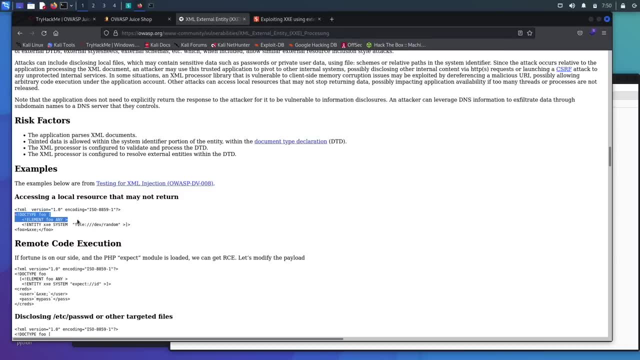 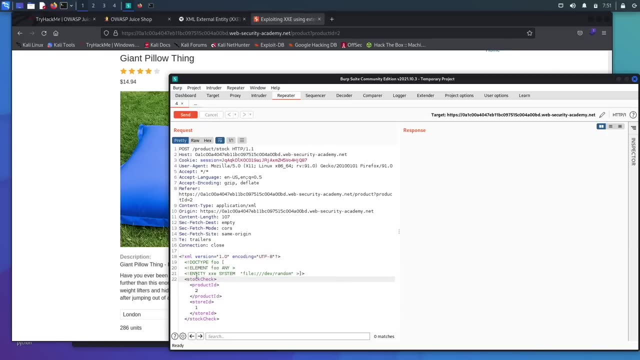 And Forward this to repeater And we can now turn this off And we're going to need This right here, So we can copy And we'll paste it in right here At the top, And now we're going to delete this first part. 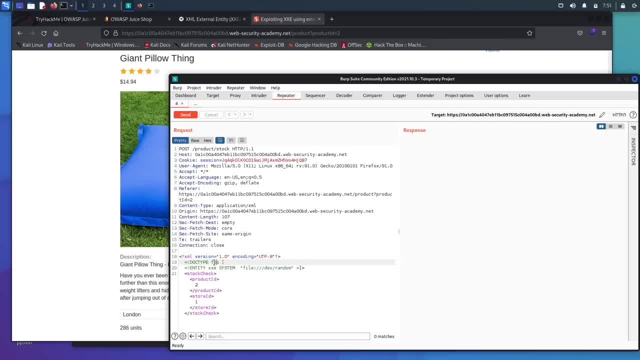 Right here And we're going to change. I guess we'll leave our doc type as foo And we're going to change this Right here to xxe And this right here To passwd, And then down here where it says: 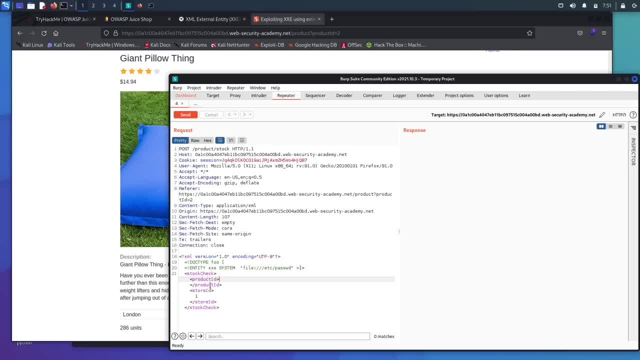 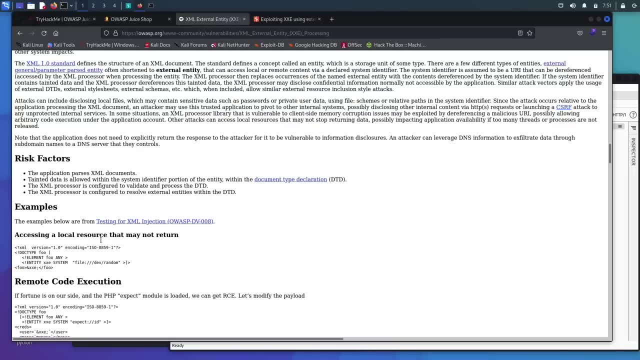 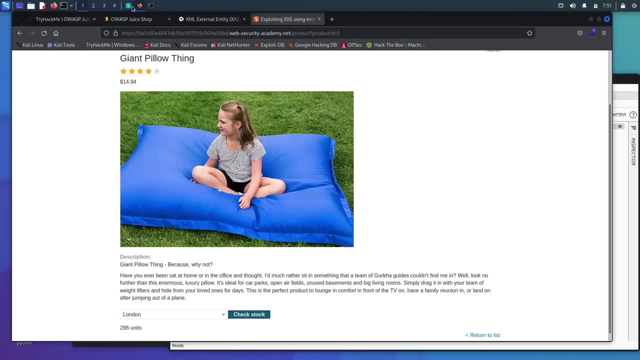 The product id. What we're going to do Is we're going to use This right here to tell the system We want it to do something. So if you remember What this looked like, over here We have the And. 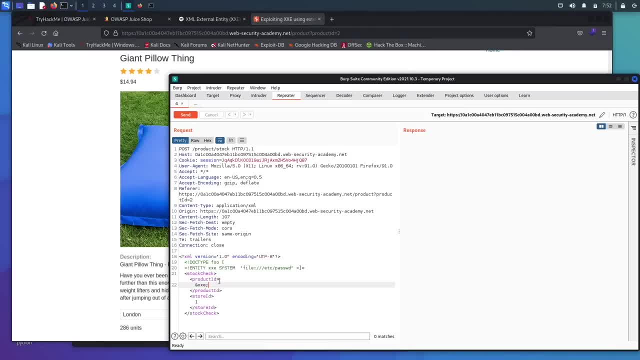 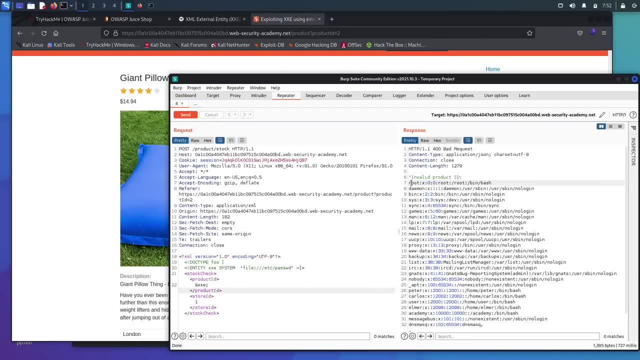 xxe. with the colon We need burp, And where that product id was We can paste this in, And now we'll send it And see if we have any errors, And we do not. This is a pretty big Vulnerability. 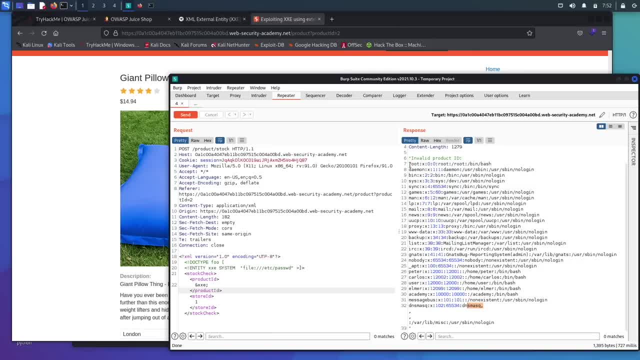 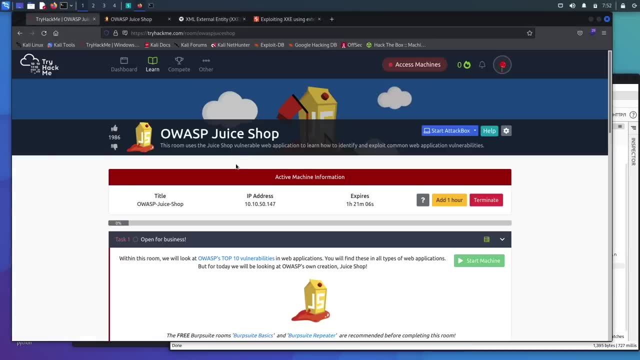 This is something you shouldn't be able to look at. This is actually. This is something you shouldn't be able to look at, And it will give us users That are on the system. So from here, we're going to move on to. 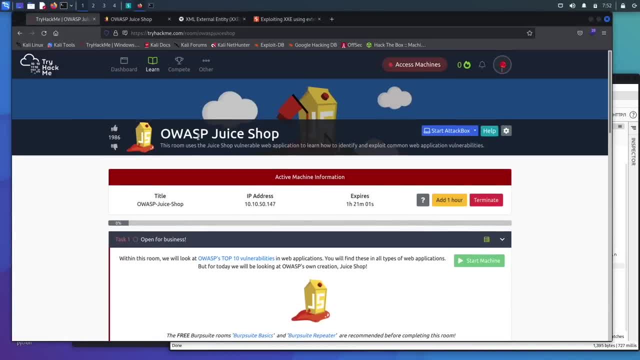 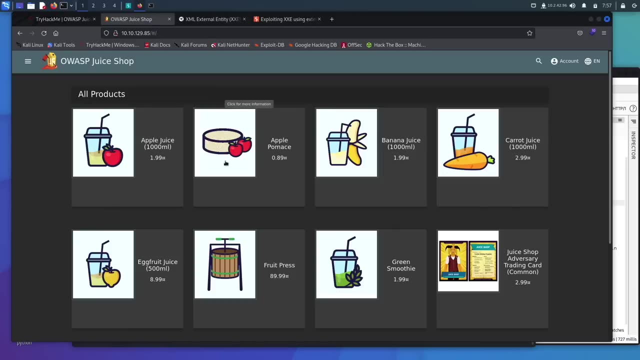 Tryhackme And we have juice shop, Which is a really great place to practice A lot of web application vulnerabilities, And we will hop over here And pop open a machine And I'll show you How to upload XML injection. 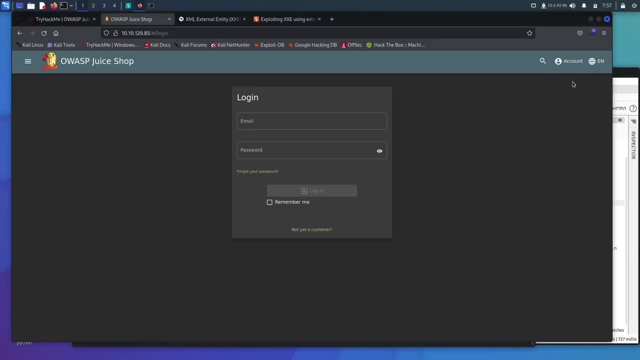 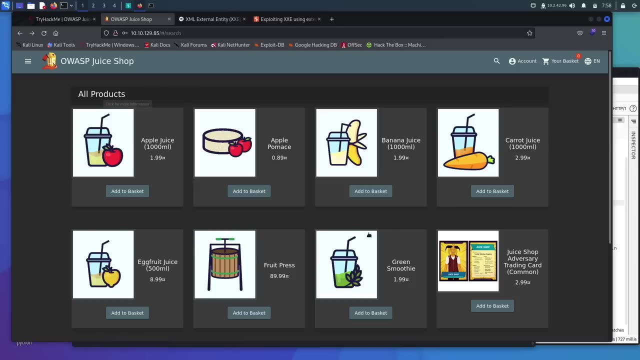 We'll come over to oosp juice shop. You will need to click on login And create an account. So I'm going to create an account And then we'll be back at the home page And I'll show you where to start from there. 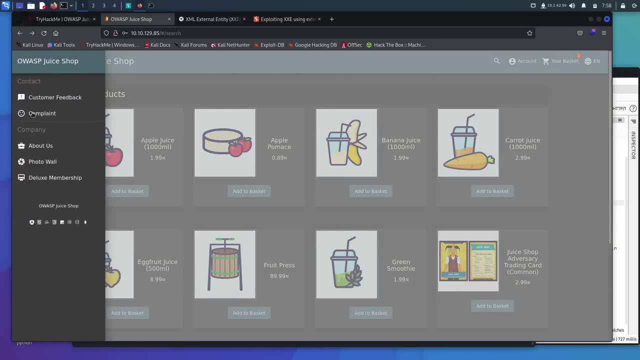 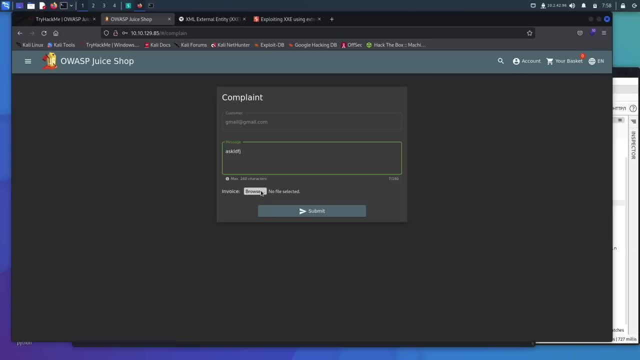 Okay, so we are all logged in And we are now at the front page. We'll come up here to the three lines We're going to say we want to file a complaint And we'll just say A bunch of gibberish. 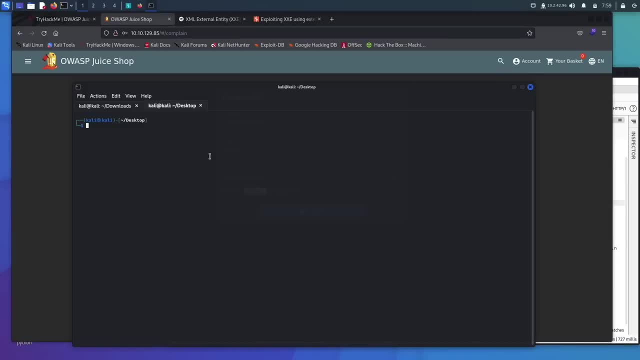 And now we're going to need to upload a file, Our XML file, By coming over here And gedit, And this is what we'll just name: our file, So that way we know what it is. I'm going to make this on my desktop. 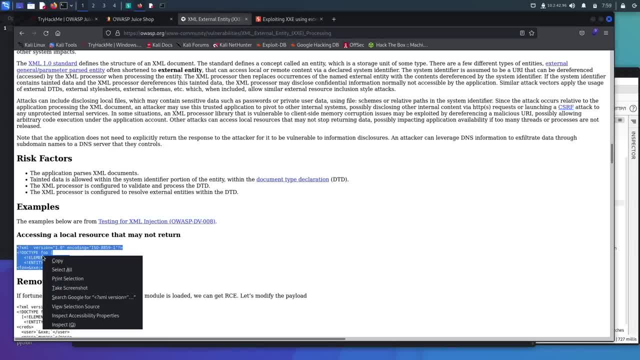 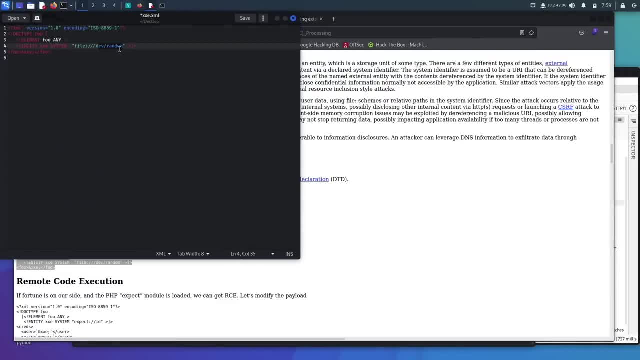 So that it's easy to find. And now we need our code to inject with. So we'll copy this, We can move it over here to our file And then we'll just change this To etsy Pass Wd. 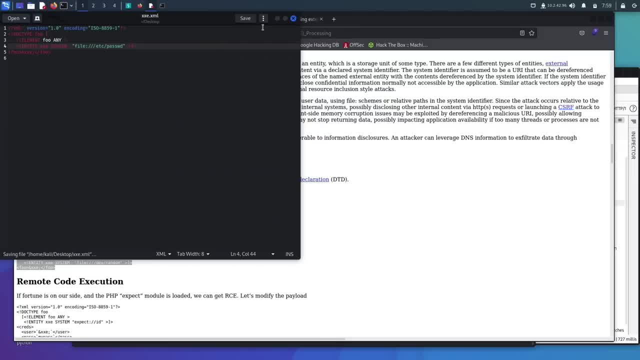 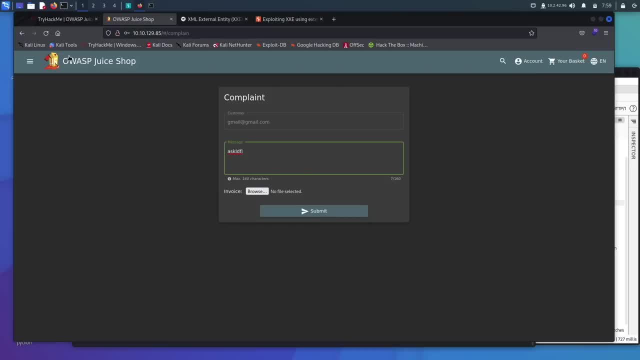 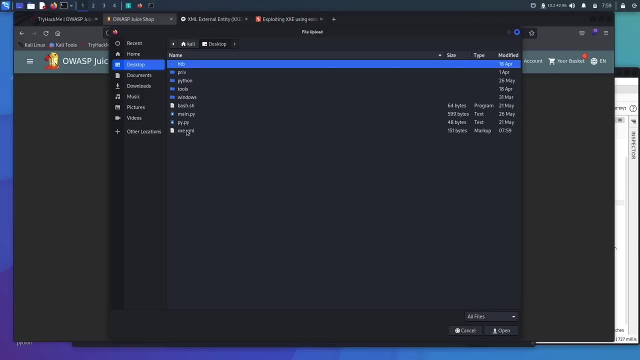 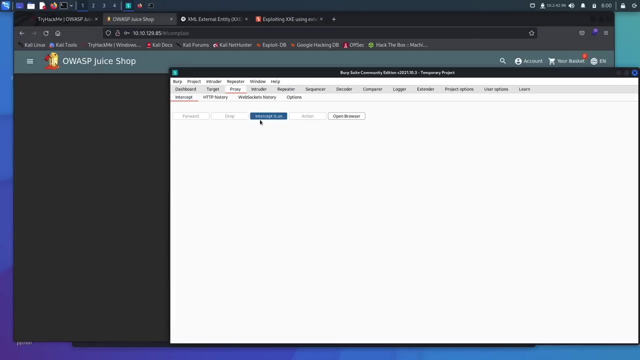 And Save it, Close it And come back over here to juice shop And click browse. We go to our desktop. We want all files XXE Open. We need burp to intercept this. So we'll come back to our proxy. 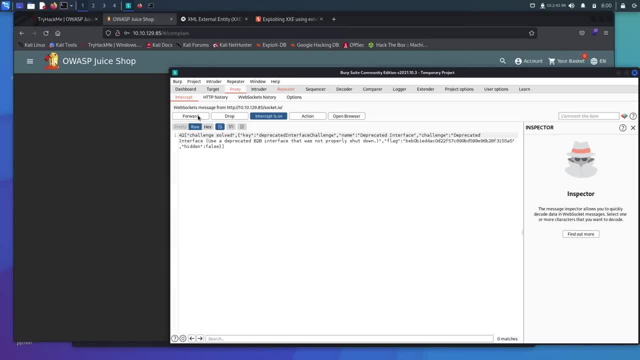 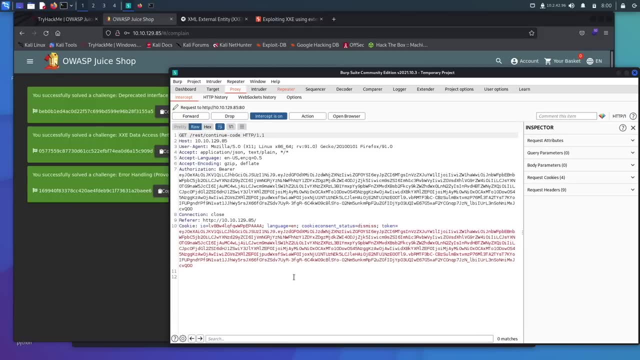 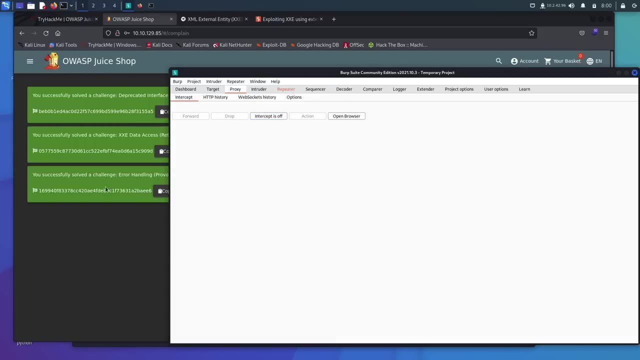 Intercept And submit. Send this to repeater. So we're going to send a couple of them. We'll send this And we'll just turn repeater off And hope we got it. So it says we've solved several of the challenges. 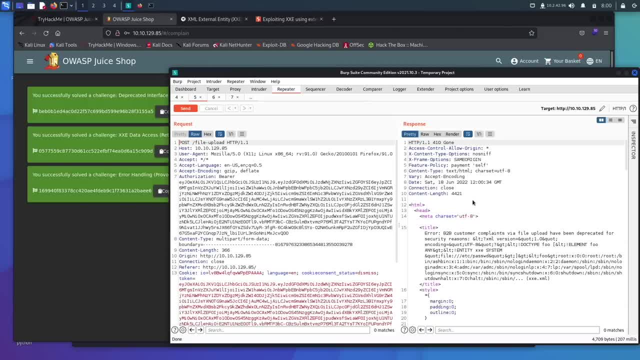 We'll come to repeater, We'll go back here to the first one, We'll send it And right here is the passwd file. It doesn't come back in quite as nice a format As our original one That we had done on port swigger here. 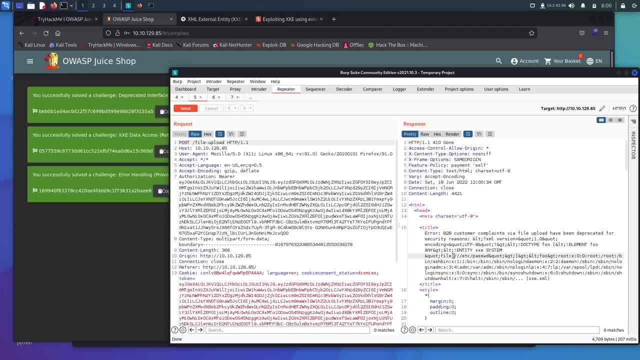 But we have the xml, The xml injection worked And we have the passwd file And here's the root user. So this is a file upload Xml injection And now we're going to cover a xml injection. That's going to lead us to. 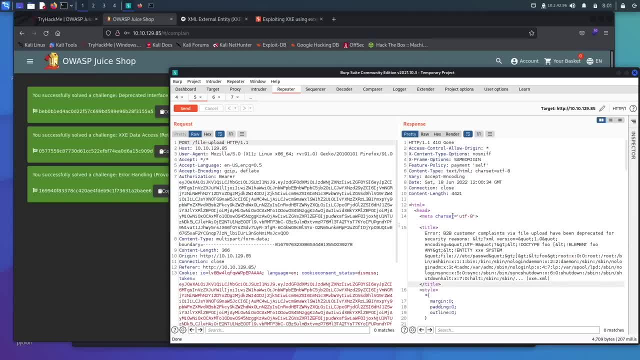 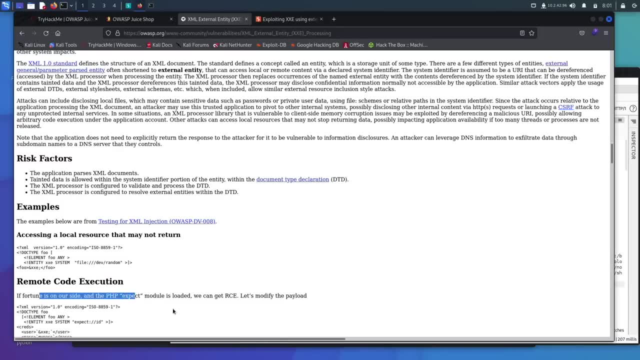 Remote code execution And you can actually see right here They tell us Remote code execution. If we are lucky And the php accept module is loaded, We can get remote code execution And we're going to go ahead and try this. 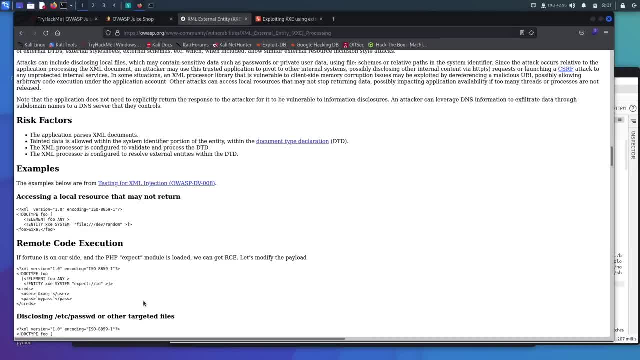 But this is on hack the box, And if you don't have a subscription to hack the box, That's okay. This would be something I have never seen Outside of hack the box, But it's something to be aware of, So we'll go ahead and I'll open up hack the box. 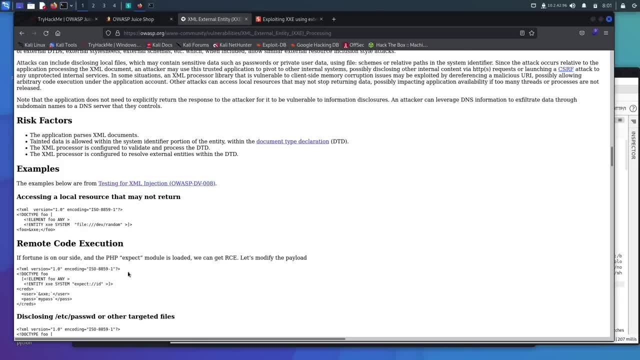 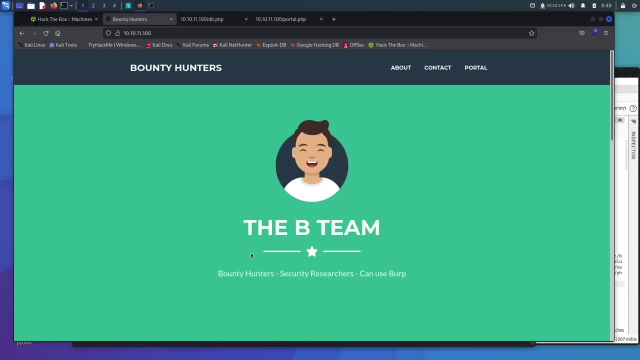 Launch the box And get all set up, And then I'll walk you through an xml injection With hack the box. Alright, I have popped open here for us The hack the box machine. This is the landing page, And if you run a dirt buster, 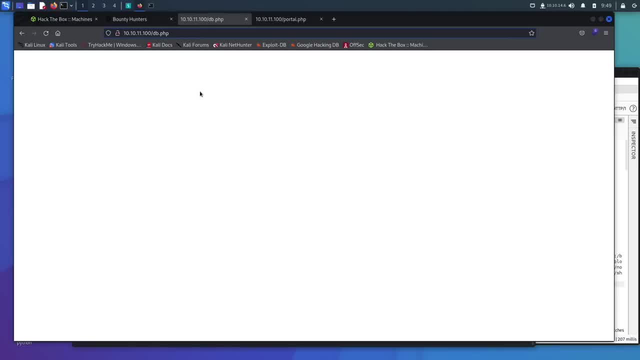 Or fuff, You will find this dbphp And then we have the portalphp And we click this And we are brought to this page. Now, if we go to test it, Grab our interceptor And we just put something in here. 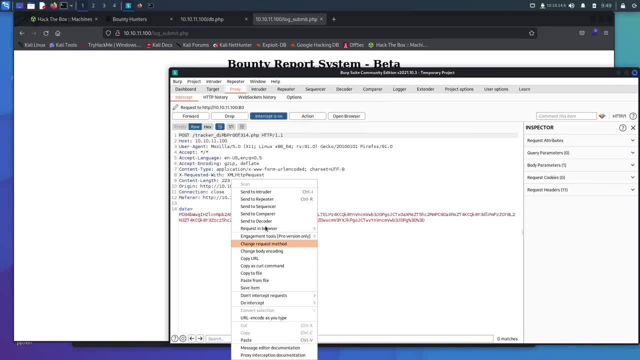 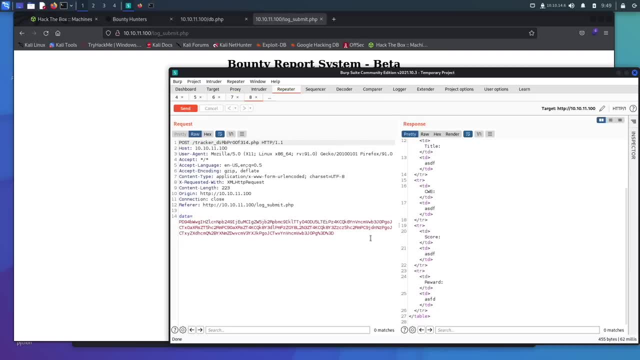 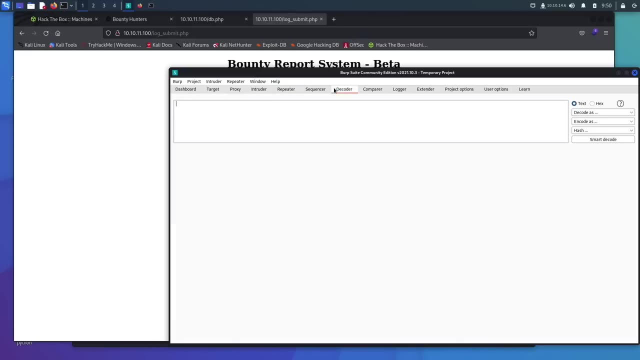 And we send it. We'll send this to repeater. Turn this off, Send And we have this, This value, right here: Data, And this is what we get back. We have this data parameter right here. We can copy it. 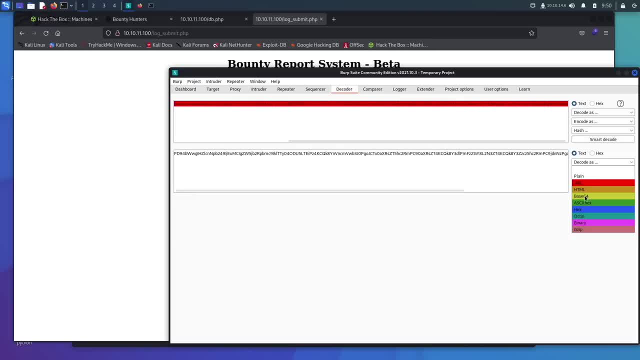 Come to our decoder And we can decode as url, Decode as base64.. And we see we have this xml. We get an xml return That has been base64 encoded And then url encoded. And so what we can do with this? 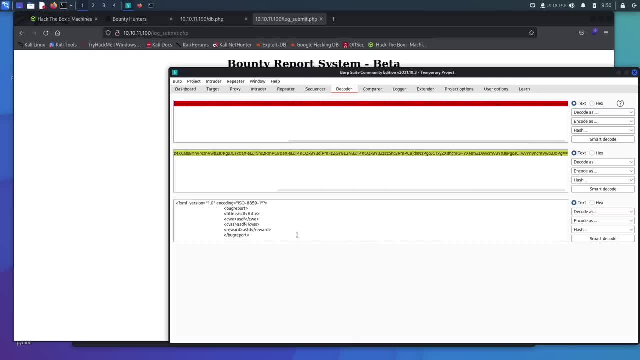 Is: try and add to it Or adjust it. Let's see if we can pull off An xxe attack By just reversing this. We can add in our own payload And then we can encode it as base64. And then url encode it. 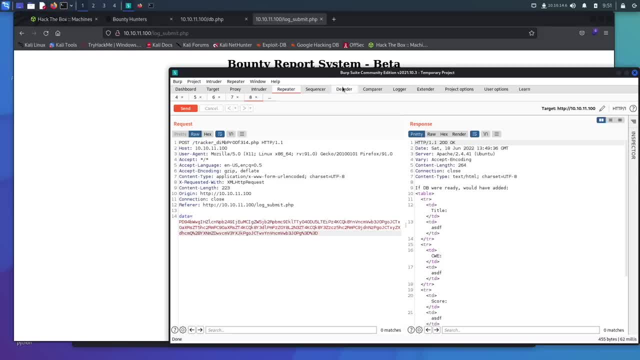 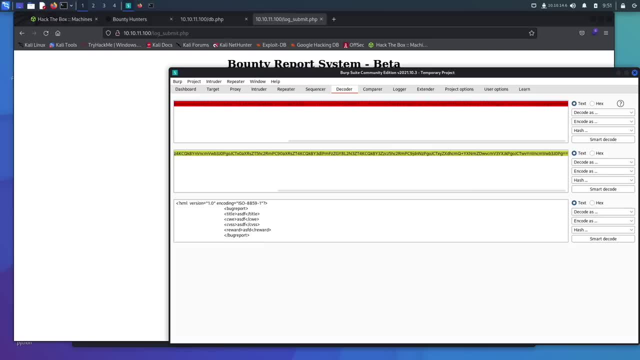 And put it back into the repeater tab Right here. So what we'll do is Come over And we'll just try to pull down the. We'll try to pull down the etsy passwd file first. Okay, One other way to look at this. 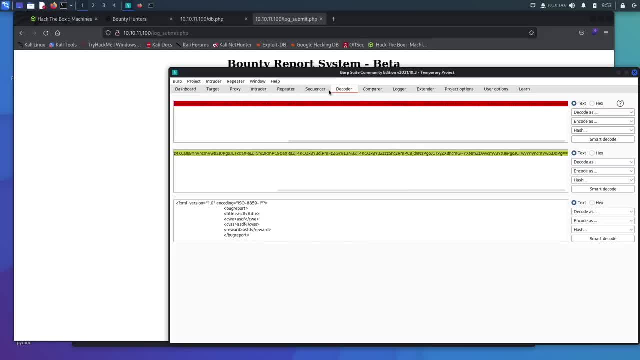 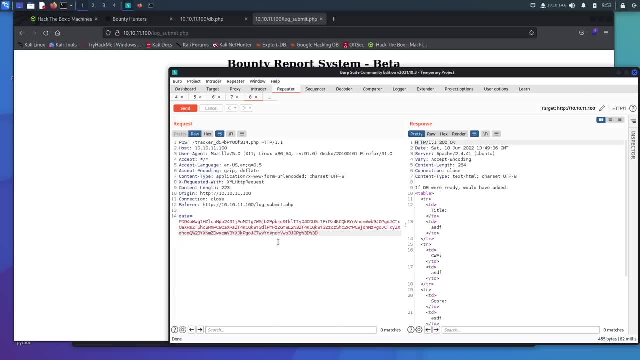 That is a lot easier Is to go into the repeater, Coming into the decoder And decoding this as url And then base64 to get to the xml file Is we can go to our repeater And remember we have this data here. 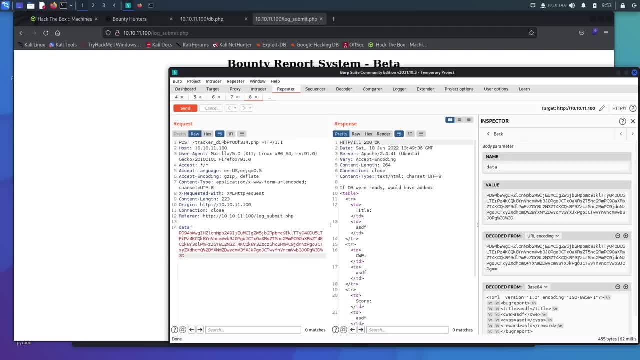 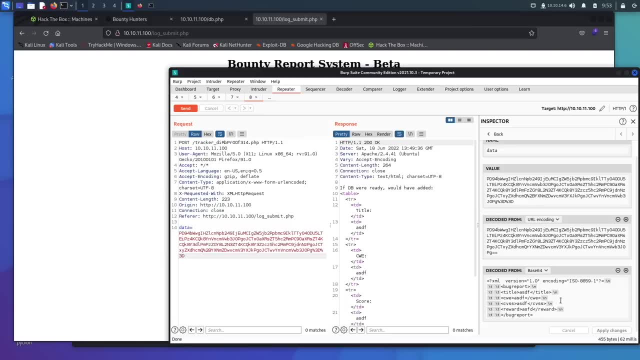 We can come over to our inspector And then we can click this little arrow right here And it will automatically decode this for us And we will land right here And we can actually do our changes Right here, Apply changes and resend this. 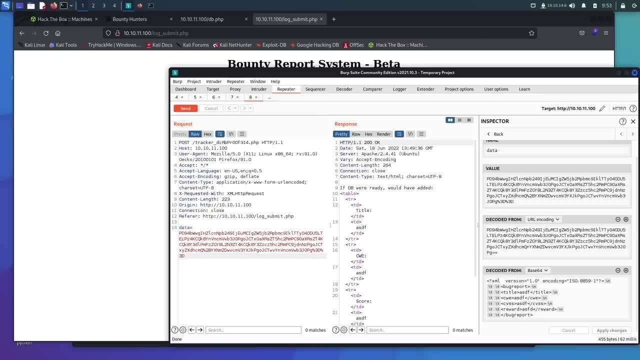 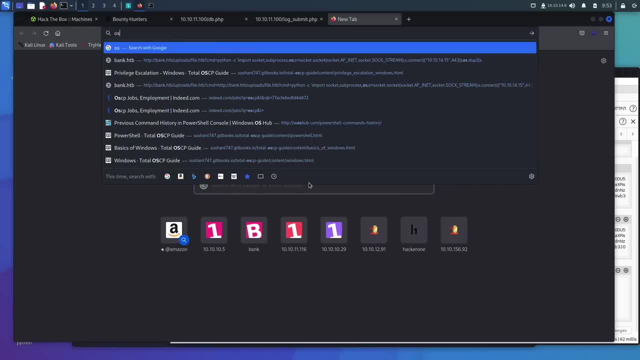 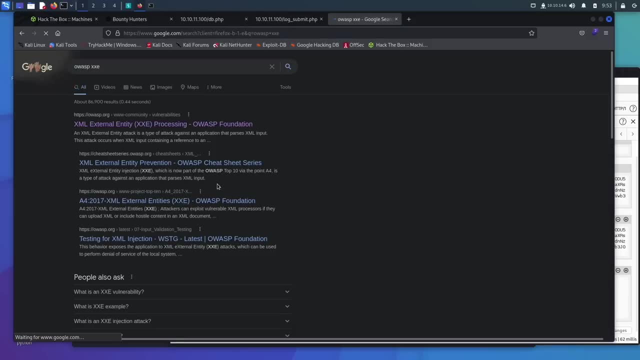 And get our input, Our response brought back to us. So what we will do Is come over, We'll go to OWASP And we will grab the xml Right here, the xxe. We'll open this up To grab our payload. 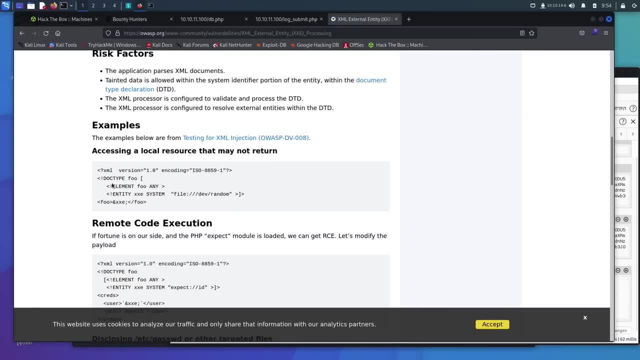 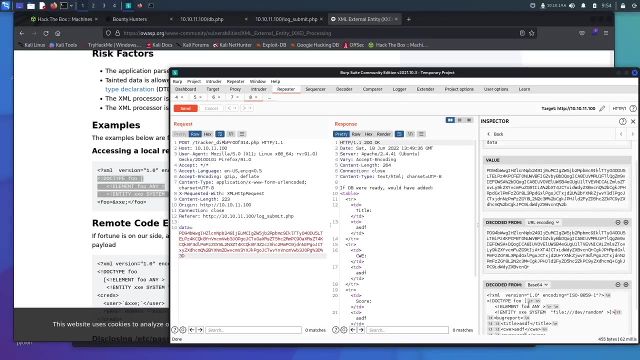 This is not the one we were in earlier, But that is okay. So what we will grab Is the doc type And the file system. We can copy this. We'll put this on A new line Right here. We'll actually try to. 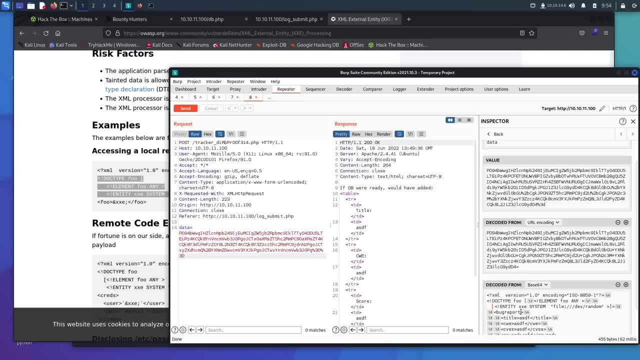 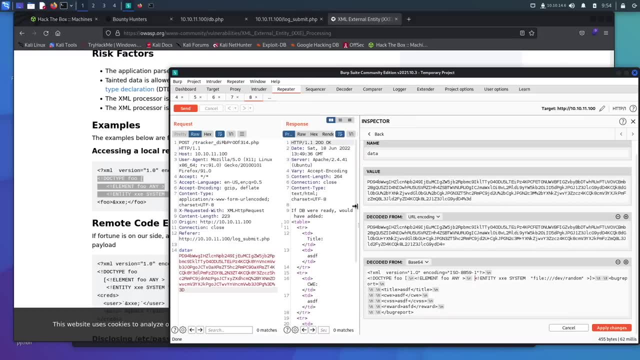 See if this will, let us put this all on one line, So that it looks better For us Now that we have this on. Well, not one line, But it's a little better. Here we go, Now it's on one line. 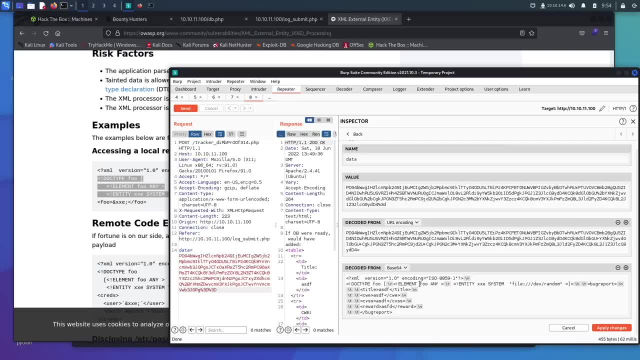 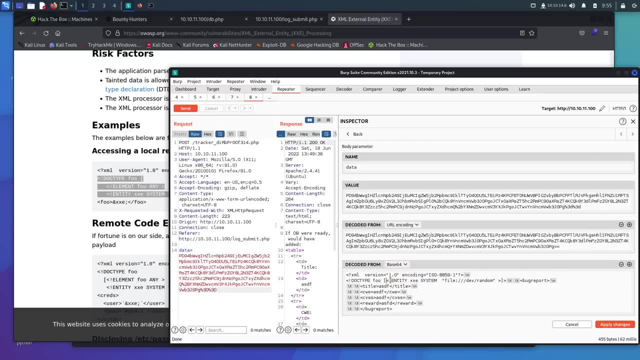 Similar to what we've been doing before Is: we can just leave this However we want. We're actually going to delete This. We don't really need that And it looks a little better for us. This goes on a different line. 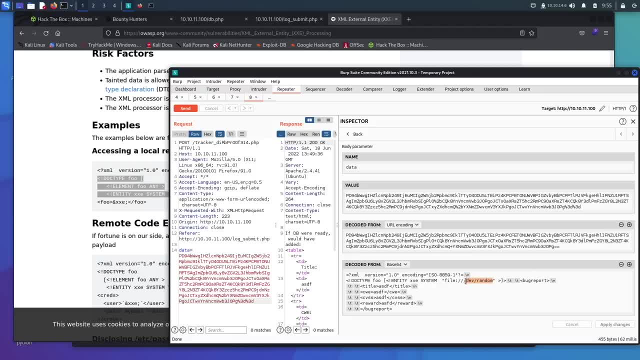 Guess we'll leave it. Okay. So here we go. What we can do at this point Is type in etsy, Slash, passwd And then down here We can go Our and symbol And our semicolon And apply changes. 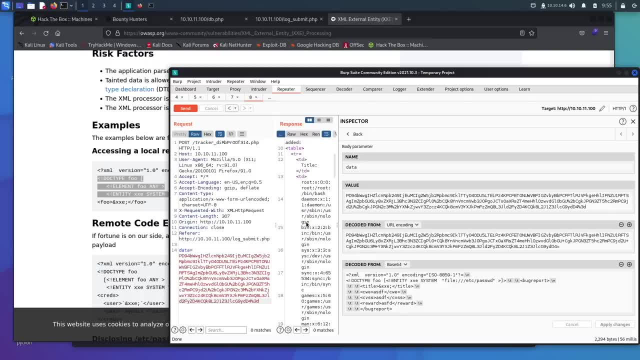 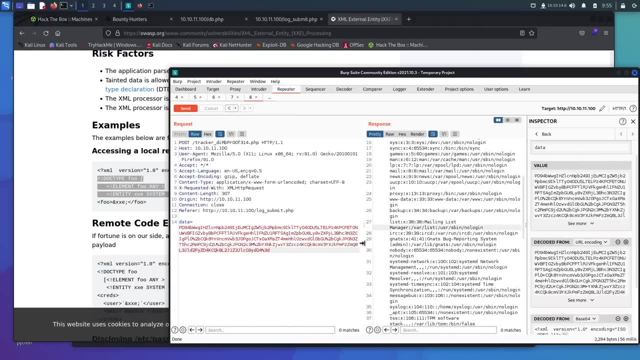 And if we send this response, You can see right here We have the passwd file Brought down for us, And so one of the things We always should look at, Especially when we are on a hack the box, Some kind of CTF. 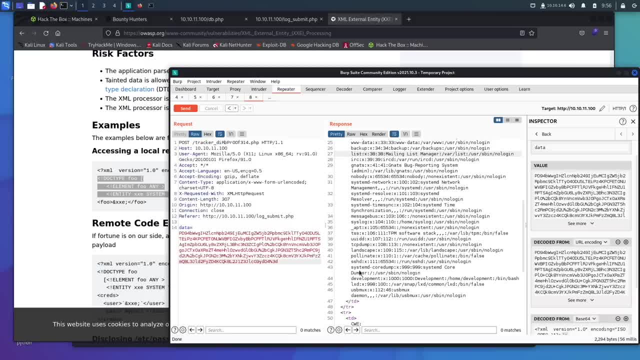 Or even a pen test Or a bug bounty program. You really wouldn't do this To attack some of them. So we have the development user. Here's the user ID. We have root, obviously up here And what you can do. 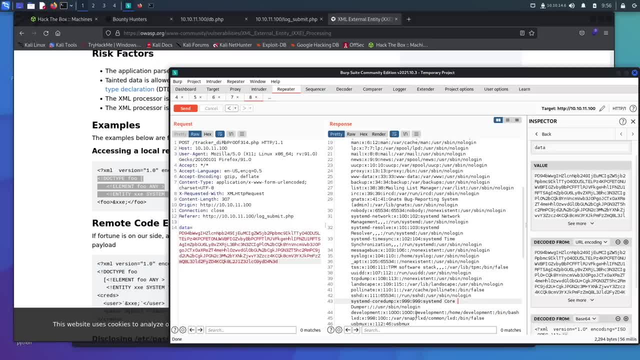 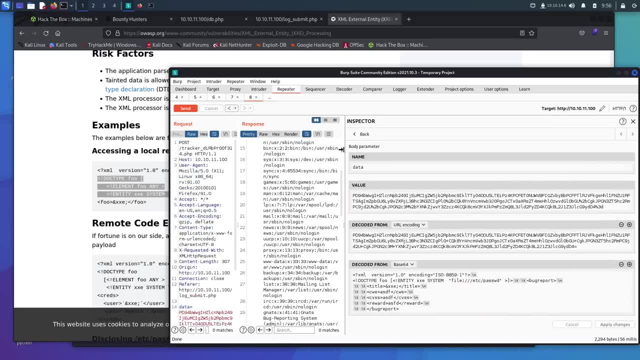 Is just look for the ones that have been bashed, And those are the ones that will have a shell available on them. So we have development and root And a quick look I'm not really seeing any others. And now what we can do. 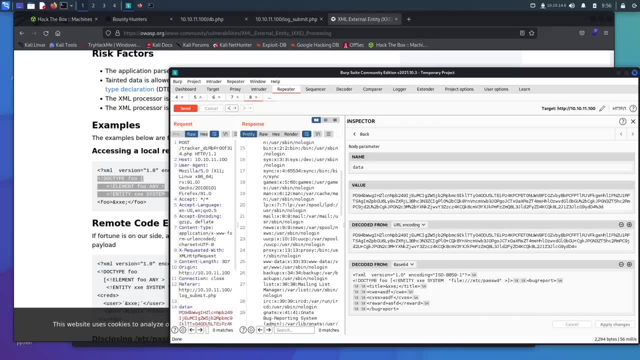 Is: try to pull down That dbphp file, But in order to do that, You will have to use a php wrapper, And those are something I would suggest learning, Because you will see them Every now and then, Whenever you see a php system running. 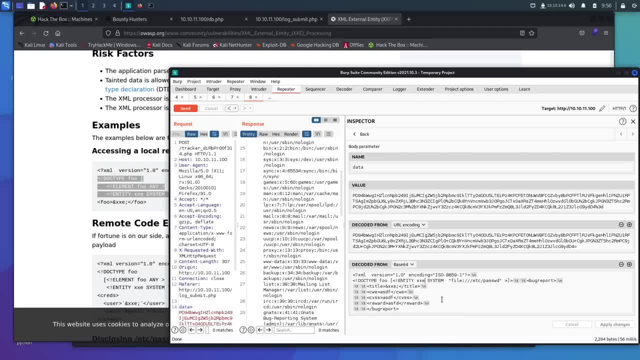 A lot of times You can think php wrapper And see if you can pull down information That you should not be able to, And there's a lot of different places You can use those php wrappers, But one of those places Is going to be right here. 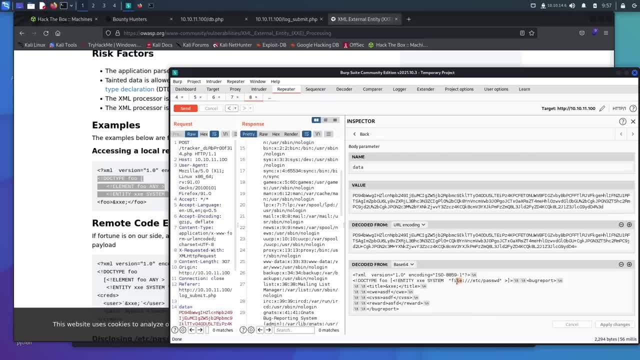 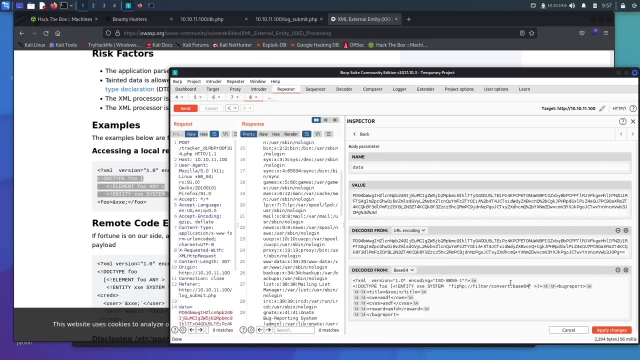 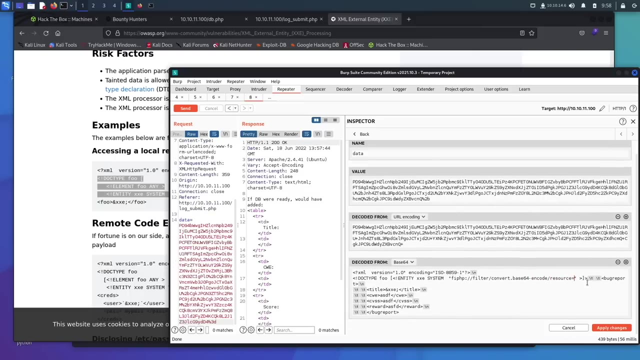 So, instead of pulling down a file, What we're going to do Is type in here php, And we can delete All of this And type in Filter, Convert Base 64- Encode Resource Equals And instead of the etsy. 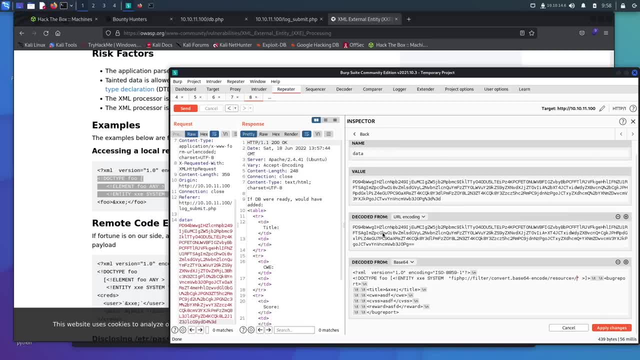 Passwd file. What we're going to be looking for Is the dbphp. Typically, if you're familiar with Doing ctfs or any kind of pen testing, You will know that You can find the files inside. You can find the files for a web application. 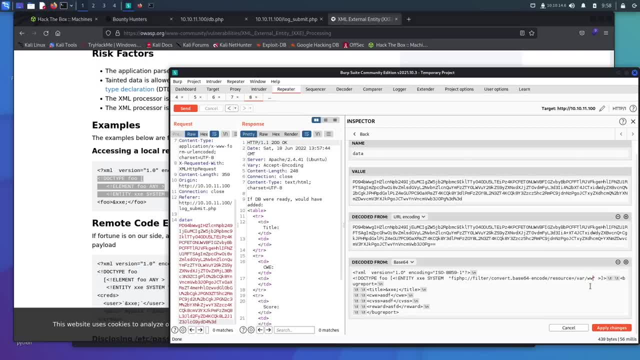 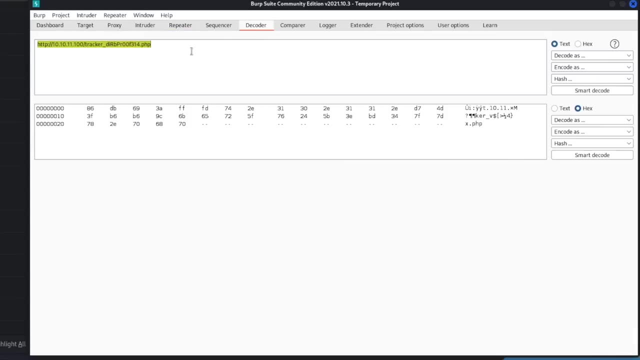 Inside of vars, Slash, dub, dub, dub, Slash, html, Slash, dbphp- And this is pretty standard for where You're going to find files On a linux system And we can apply changes, We can copy this, We can go to the decoder. 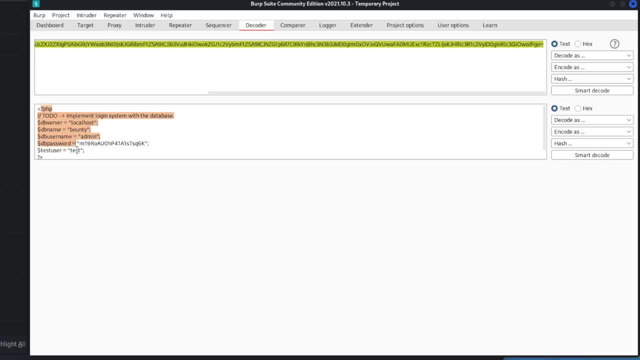 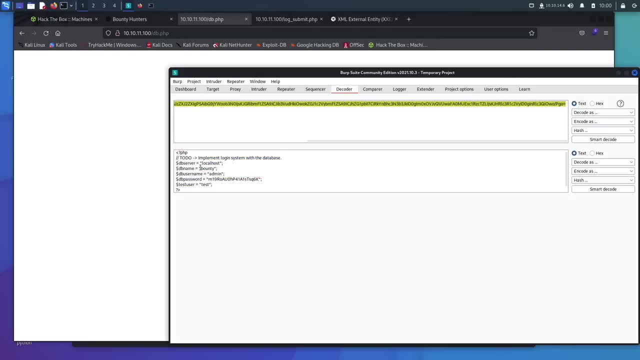 And load it With base 64.. It tells us that we have this in our response, So this would be what was brought back With our php filter And we have a User name. Right here We have the database name. 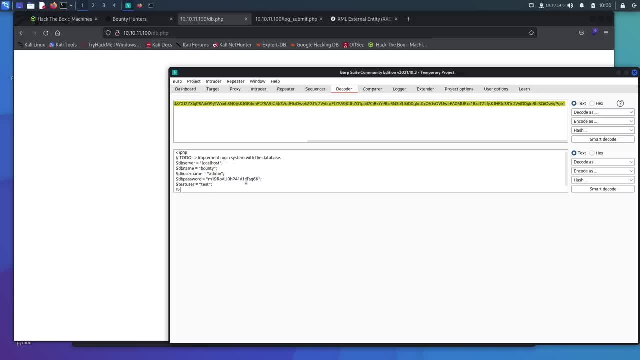 We have a password right here And we should be able to ssh in As the development user Using this password right here, Because we know it's really common For people to reuse their password To remote code execution. So if we come over here and we say ssh, 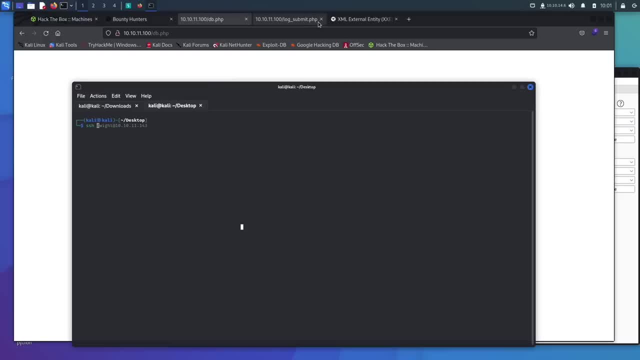 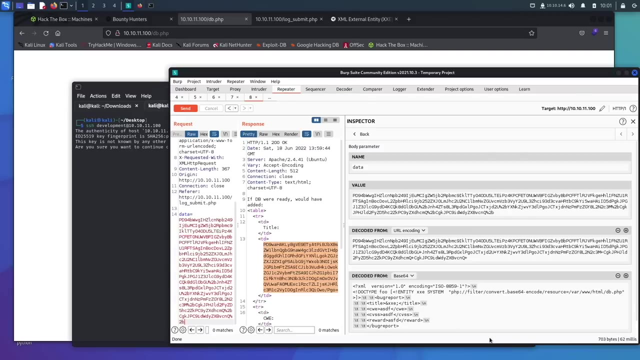 And then we say What was Make sure we had that user right? I think it was Development at 10, 10, 11, 100.. We might have to Grab that User Again. We'll say yes And come over to the decoder. 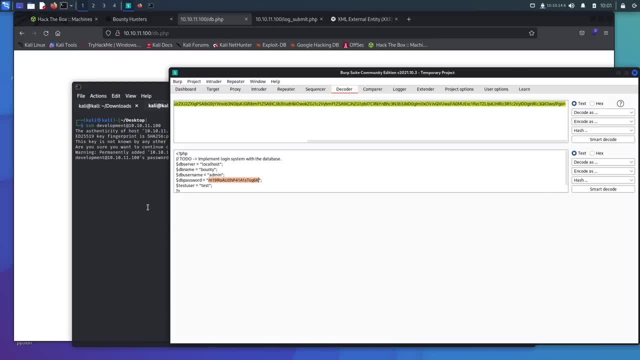 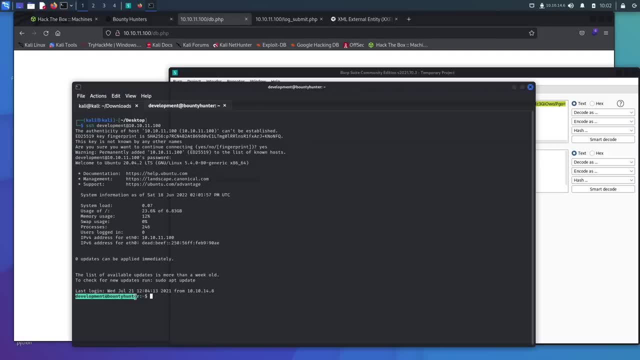 Grab the password And Paste that in, And it worked. So this is how you can get Remote code execution On the box using On a server using Xxe, And so with that, This one was really complex, But xml injection is something you should look into. 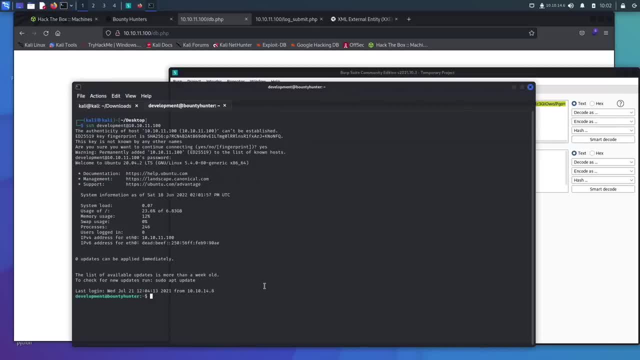 And try to learn. I would suggest going back to port swigger And maybe practicing a few of their Xxe challenges, as well As juice shop And just play around with it Until you feel like you are comfortable And you understand what is going on. 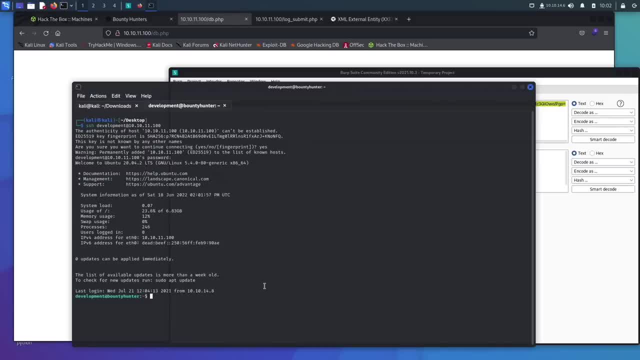 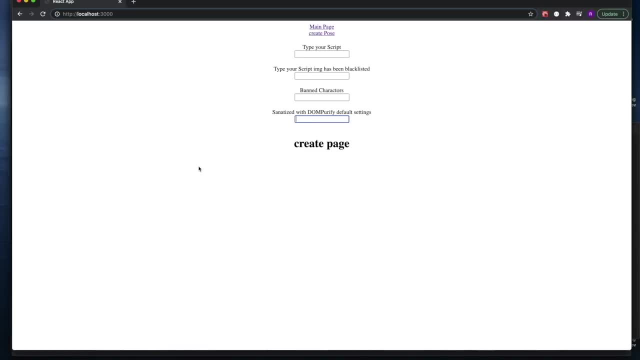 So there are three different ways That you can use xxe In the cyber security Testing world. Okay, one of the Most common vulnerabilities Is going to be cross site scripting, Or it's also known as Xss, And this vulnerability 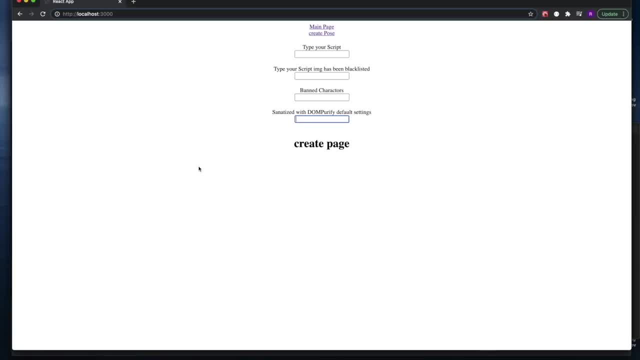 Is common, So going to be pretty hard To exploit Without knowing Some form Of html and javascript. So there are basic Payloads that you can go in And you can just test A bunch of them And I'm going to show you a list. 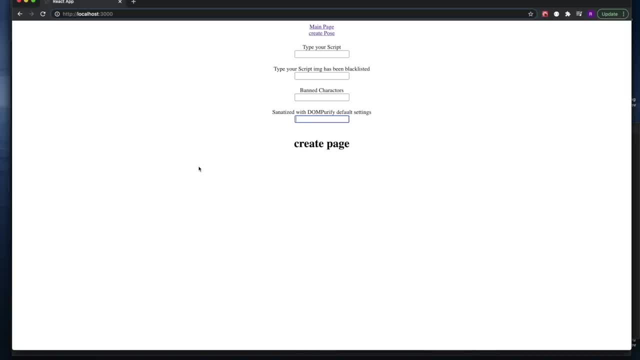 That I found It's got over 6500.. Different ways to Try and exploit this, But most of the time you are going to have to Change and modify the content. But we'll get to that In just a little bit. 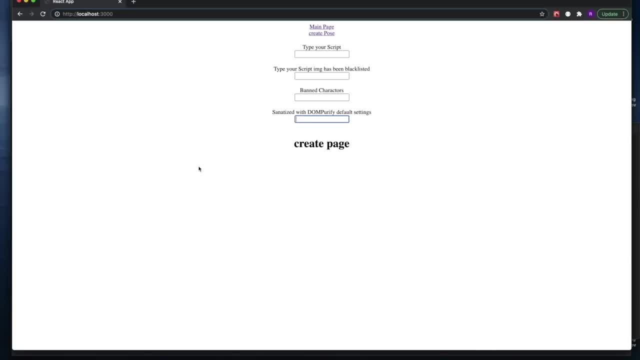 I'm going to show you just a couple of Cross site scripting Examples here, And then I kind of want to show you The code of what's going on. I think you'll be able to understand it, Even if you know. 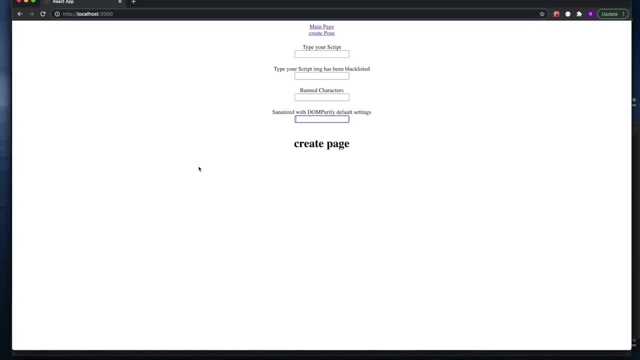 Xero programming. So with that we'll go ahead And I'll show you an example Of what cross site scripting is, And then I'll explain why it's So dangerous. This is going to be the most basic, Simple form. 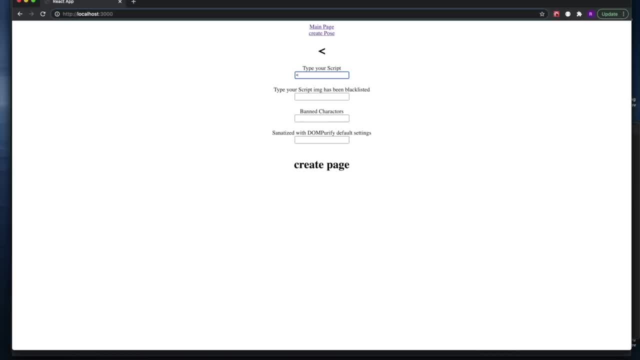 Of cross site scripting, And so all we want to do is Have an alert pop up, And if you can pop up an alert On a bug bounty Program, You will be able to submit that For a vulnerability, And there 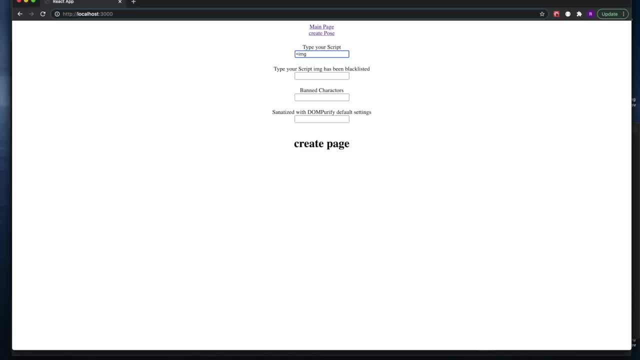 You'll see them A lot of places. A lot of people like to look for them All that often, Because I think most people look for these And if it's not stored Cross site scripting, Then you're not really going to get paid. 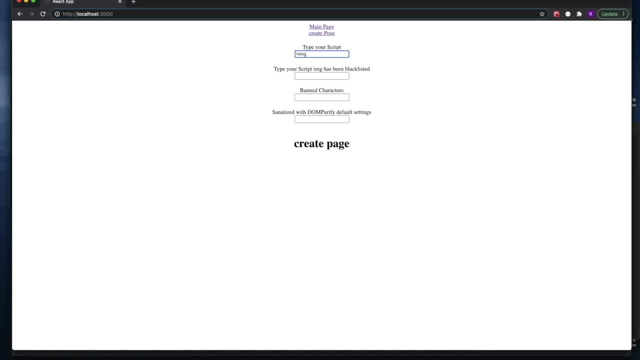 For the amount of time That you put in You'll get paid, but just not enough For the amount of time it's going to take to find them. So we're going to do this with an image, An image tag, So we'll go. image source equals. 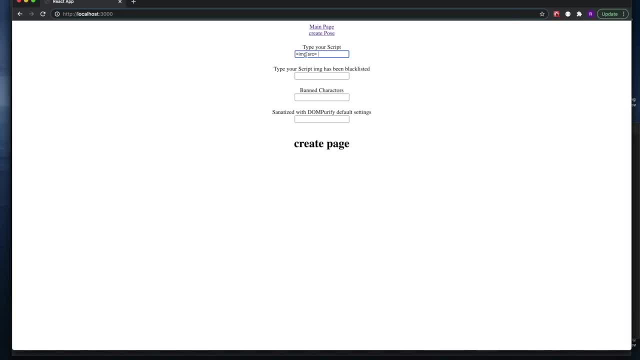 And then we leave it blank, And when this is blank, It's going to make an error. So, on error, We want to Alert, Which is going to Give us the Ability to pull off The cross site scripting, And we're just going to alert. 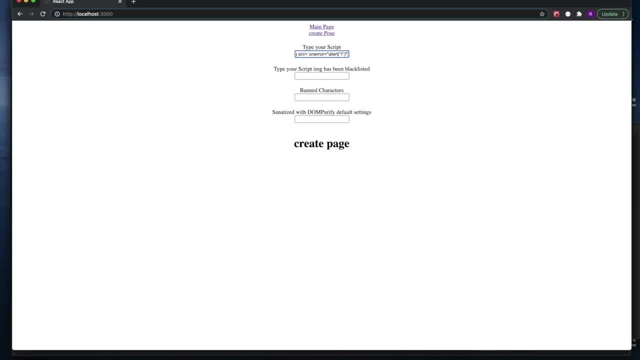 One, And then we will Close the tag, And I have Made a Mistake somewhere. Let's go ahead and delete this. And there it is. So we have the alert pop up And it says local host one. Now what you can do: 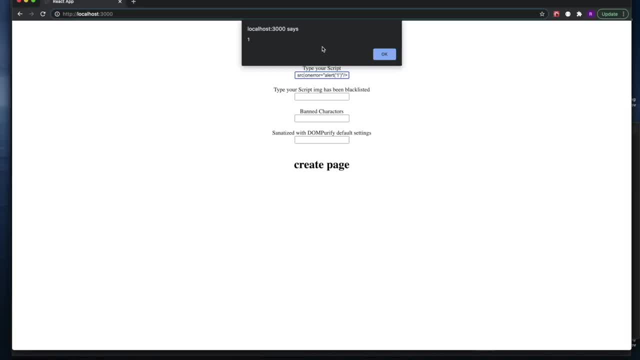 With the cross site scripting, And why it's so dangerous Is not because you can just pop things up on Somebody's screen. But what you're able to do Is you could make this look really fancy And you could say: log into wifi. 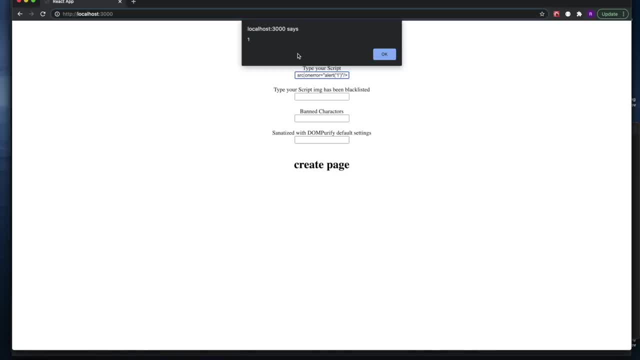 Or log into this page, Or you were accidentally logged out And people can Type in their user name Or password And then, all of a sudden, you have their credentials. You can put alert document dot cookie right here And then all of a sudden, 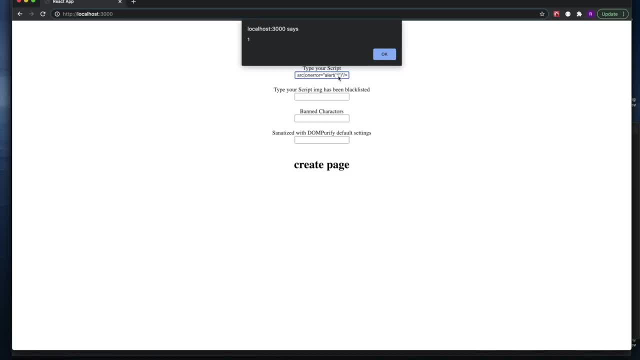 You can steal their session, And so there's quite a few different ways That you can Use this to get malicious with it, And so that's why It's so Dangerous, But it's also really common. It's going to be in the top ten vulnerabilities. 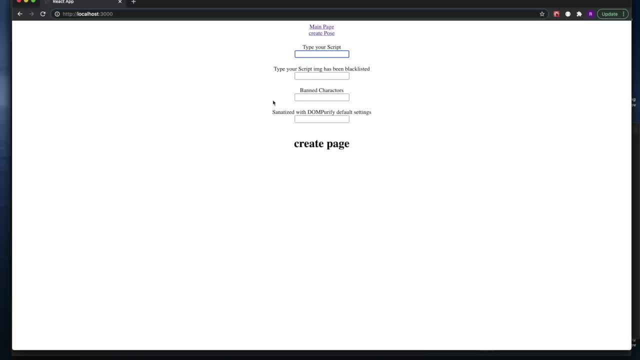 That you're going to find On pretty much any list, And so right here Is a different version. So right here Is just plain as can be. You can type whatever you want And nothing's going to get blacklisted. So right here. 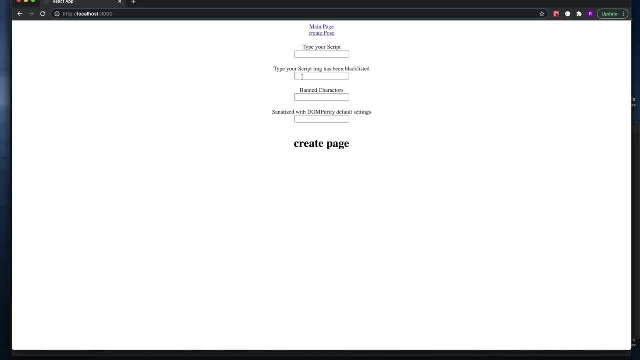 I have made a little. It's really short. It only has the image tag, But you can type your script. The image has been blacklisted, So what I mean by that Is, if you watch And it automatically deletes it, This will happen. 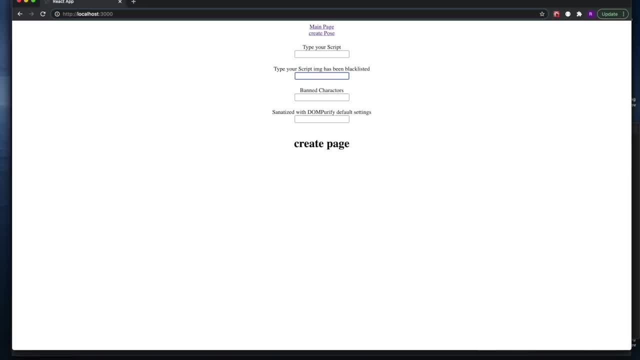 On Programs that you're going to test, They'll have characters that are blacklisted. I have come across it Regularly. I have come across blacklisted Characters when I was trying To do a sequel injection, So you'll come across blacklisted characters. 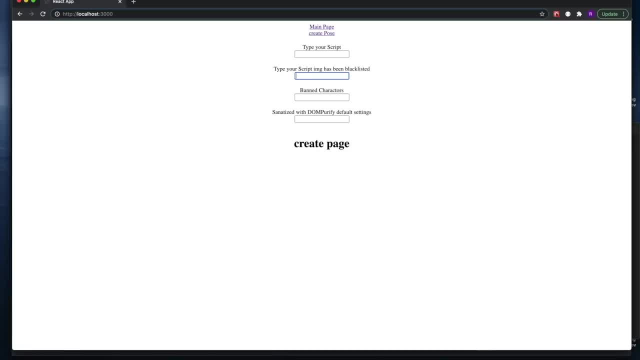 What you'll do Is: you can go out And you can find encoders And you can encode Reloads In order to fit your specific needs. And in this case, It's pretty simple. All you have to do Is go I. 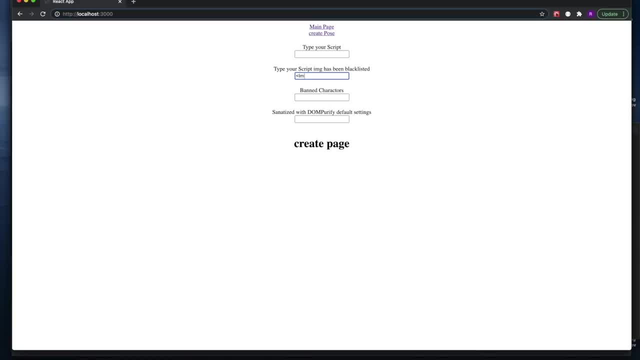 And make a capital M And a G And it doesn't get deleted. Or you can go capital I And G And this is a way that you'll find, Especially in capture the flags, To bypass blacklisted characters Or words. 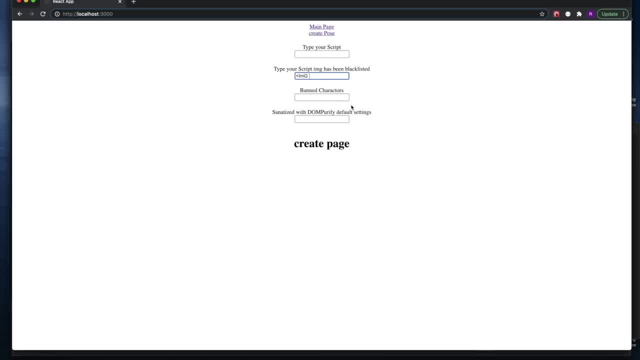 And bypass the filter, And so we could do The exact same thing That we had done before. So we'll go on error Equal Alert And then we'll just do Alert one And then we'll close it off. 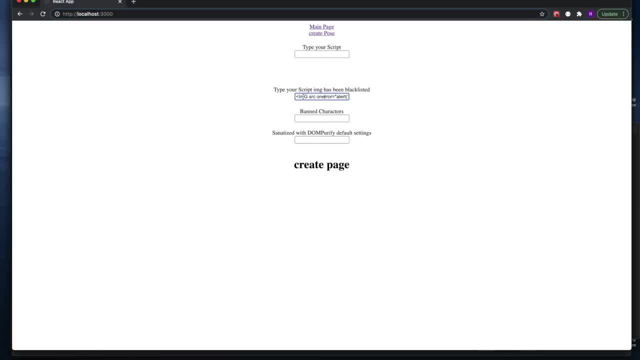 And there's the alert. So all we really had to do Was just change the image tag, Because the image had been blacklisted And we wanted to build up A different version of the image tag, And so what this looks like. 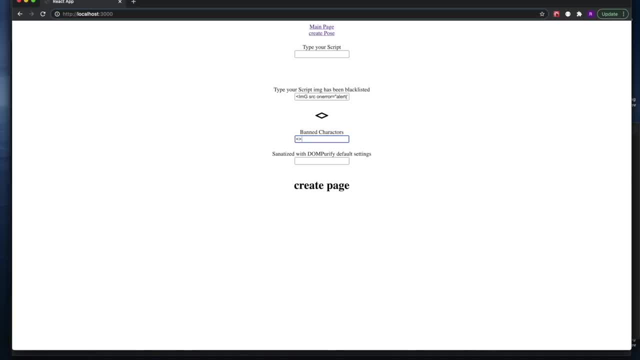 Here we have banned characters, So you can have banned Characters such as these. People will ban these characters So that you can't Inject your code into it, But we will. I will show you. So in this case, I actually banned this character. 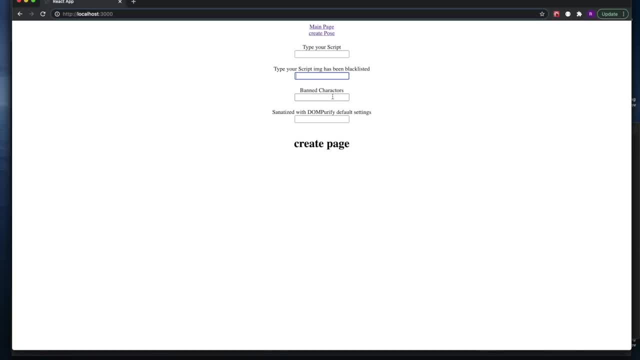 The backslash. It's not going to come in, But you can still ban this. You will find the backslash banned Because if you can't close A tag Then It's going to be really hard to pull off A cross site scripting. 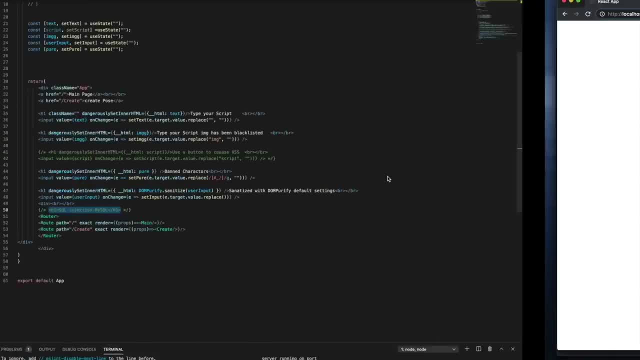 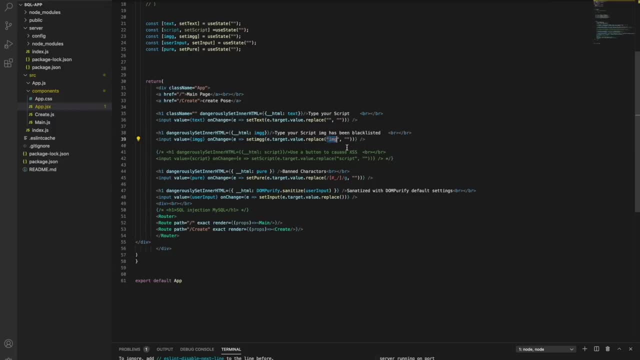 Not impossible, But you can still do it. So what this looks like Is: I am just replacing The image with an empty string, And over here We have the banned characters You can see right here. You are not allowed to use those. 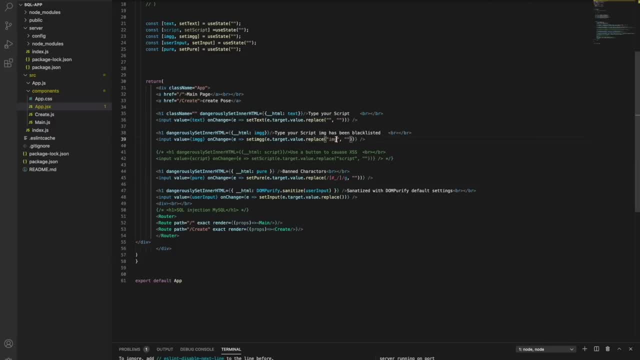 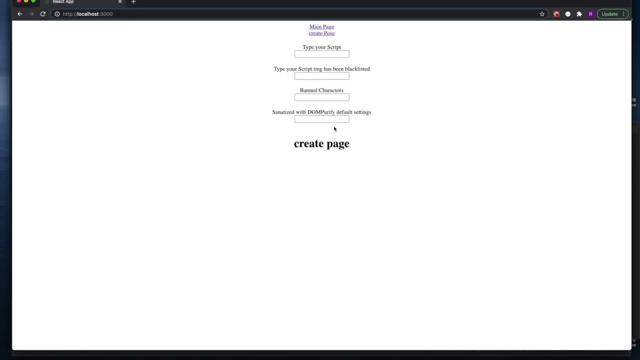 And I replace them with an empty string, And so this is what a blacklist would look like: You just have a bunch of characters listed That are blacklisted And you are not allowed to Type them in. So when you have a banned, 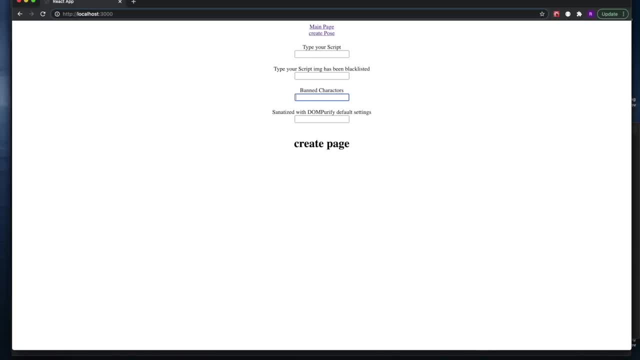 Backslash, Which you are probably Only going to see in capture the flags, Something like this. But what you can do Is you can actually Make a button tag Like this. If I can Get that right, There we go. 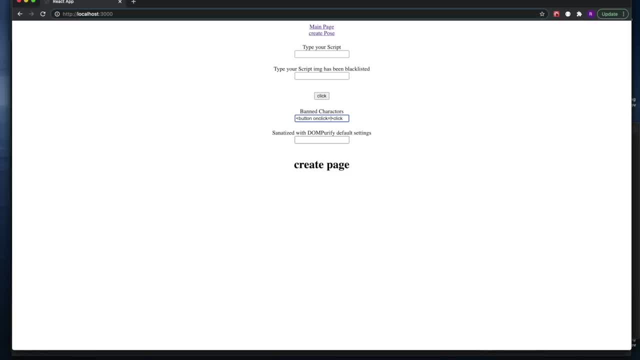 And then you can just type something in here, And then what you can do Is you can type in on click equal And then you do the same thing. You put your alert And we will put our one, And we don't have to have. 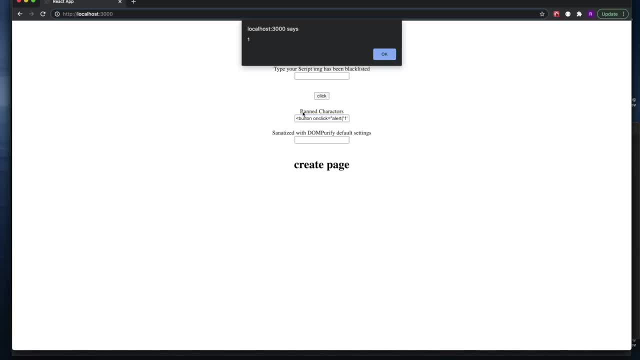 A closing tag. We don't have to close that, So we click it, And You will see this In one of our practice When we practice the cross site scriptings. So those are Just a few ways You can pull off the cross site scripting. 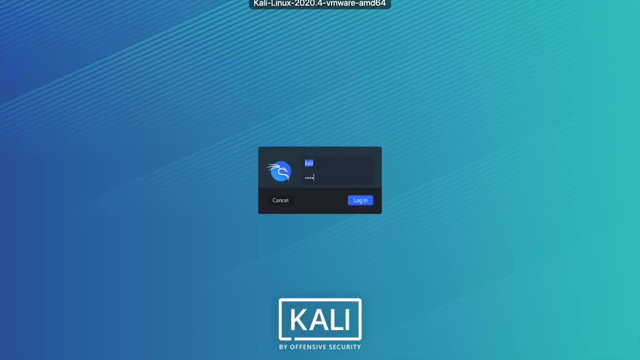 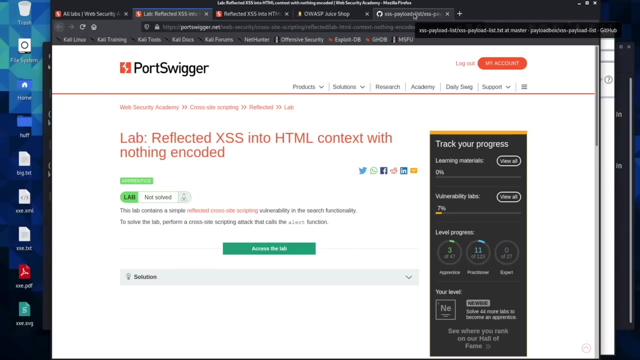 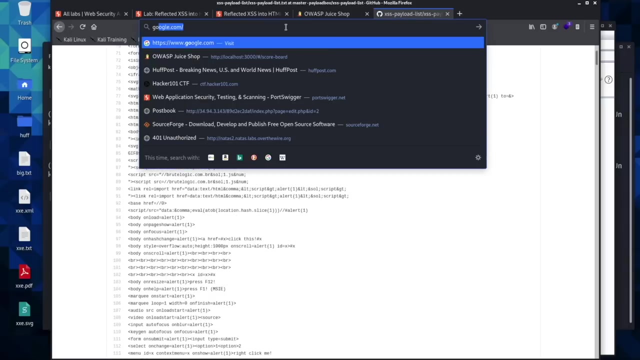 I want to show you A Page That has a ton Of cross site scripting Payloads, And here it is. You can actually just google Cross site scripting Payloads, Which we will go ahead and just do it right now. 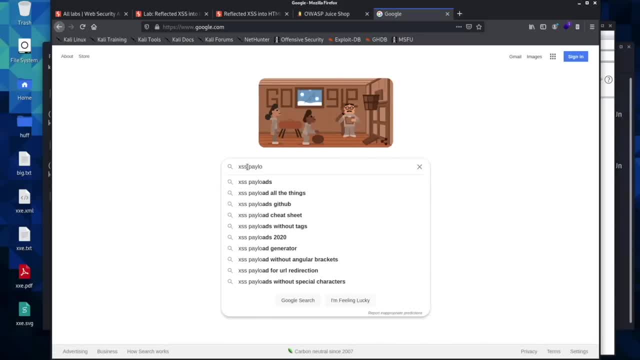 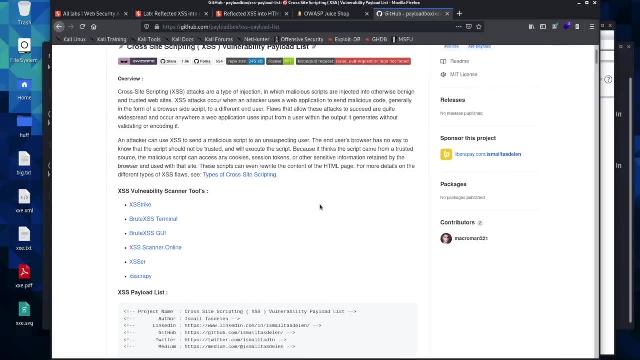 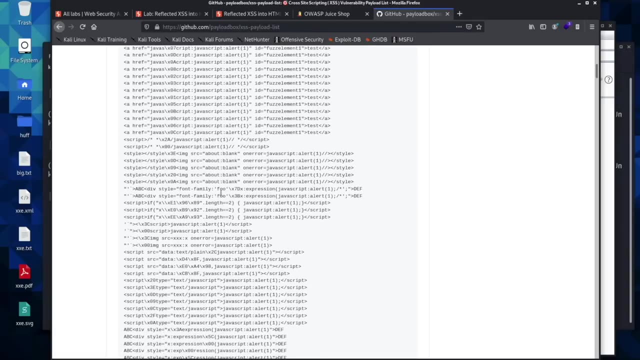 And walk you through it. We will just type in Payloads And just click the first one And here is going to be a list So you can get an idea Of how many Are out there And different ways you can do. 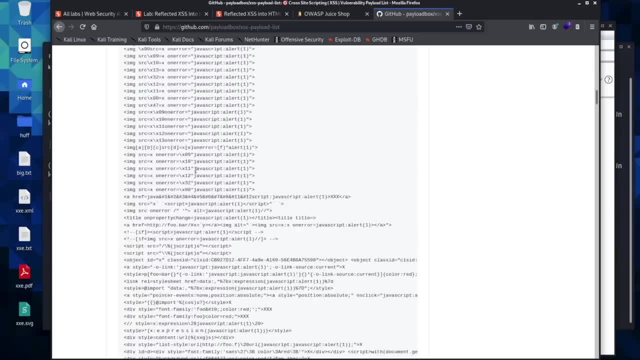 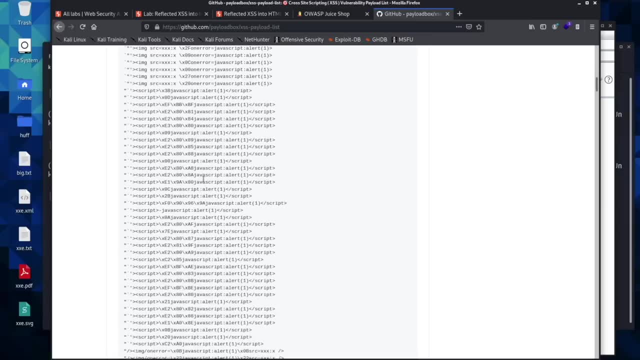 A cross site scripting, And so this is why I am telling you There is a lot of different ways to do these. You will actually see one similar to this In just a few lessons, Because you have to. We are going to have to close off a tag. 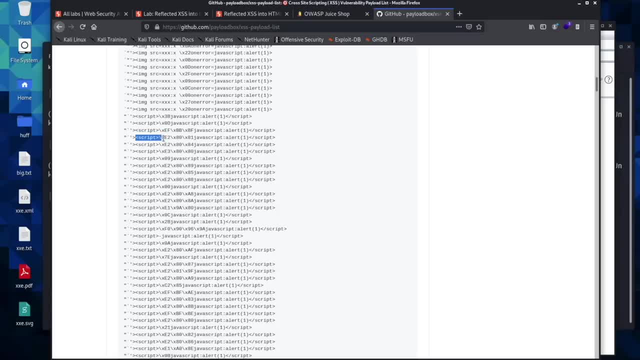 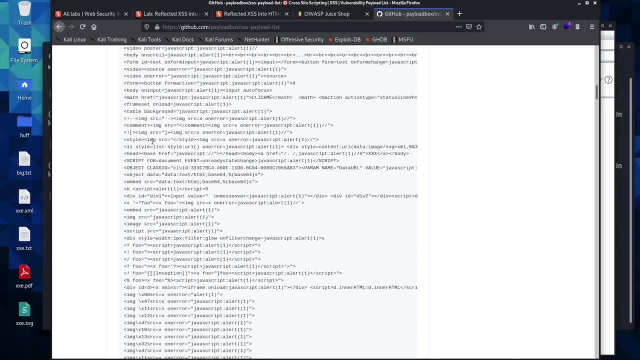 And then we are going to have a Character blocked And then we will actually be able to insert the payload. So there is a ton of different ways To pull these off. It is going to require Some knowledge of HTML and JavaScript. 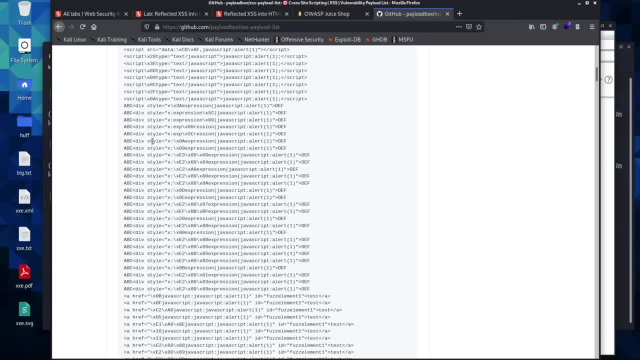 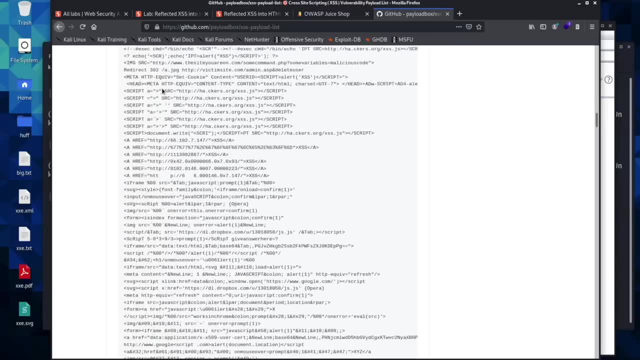 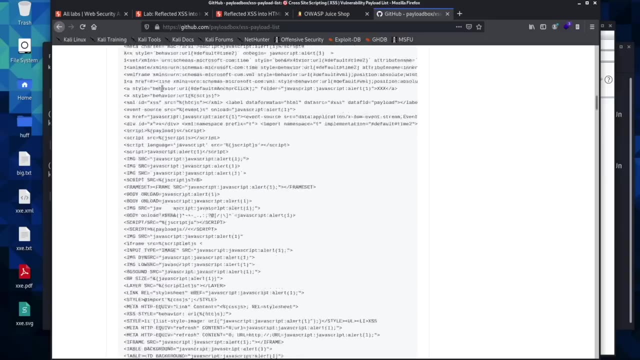 Or you can. If you are on a capture the flag, You can just go to burp intruder And it will take you to The entire list Until you are able to Receive the solved challenge. But with that, This is a basic introduction. 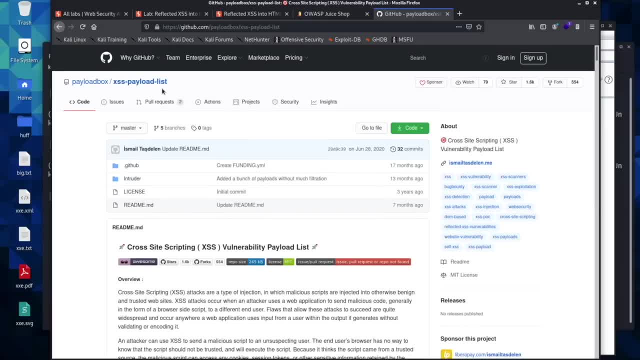 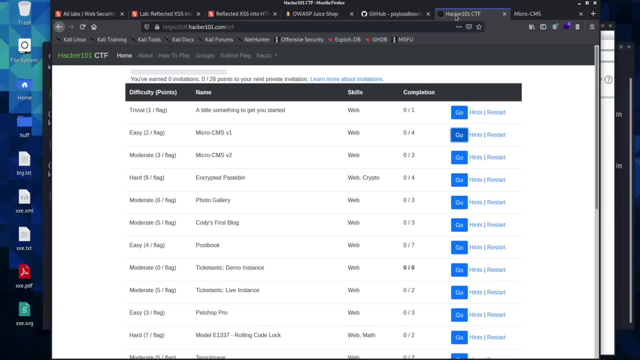 Into cross site scripting And we will get a little more hands on And I will have you guys start practicing Writing your own payloads In the coming lessons. Okay, for this challenge, I want you to come to The hacker one, Or the hacker 101.. 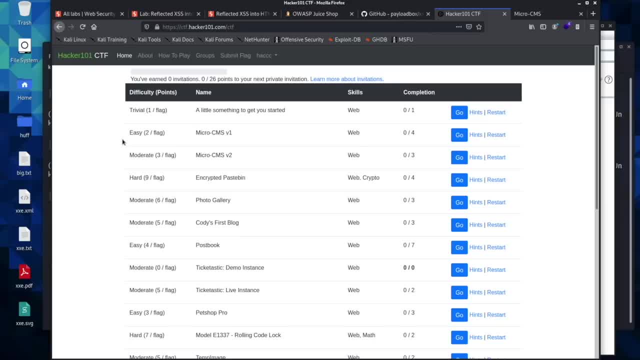 CTF. This is hacker one's practice site For us to practice what we have learned. You can come in here to the easy With two flags And click go If you would like the challenge. We have already Saw the XSS. 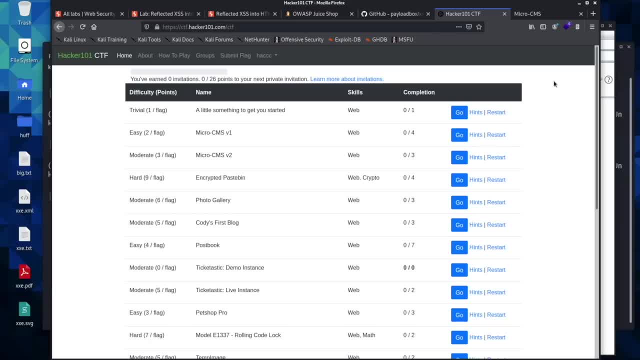 In this challenge. I showed it to you In the last lesson. So if you want to go ahead and look for it On your own, You can go ahead and do that Without the knowledge To solve this challenge all on your own. 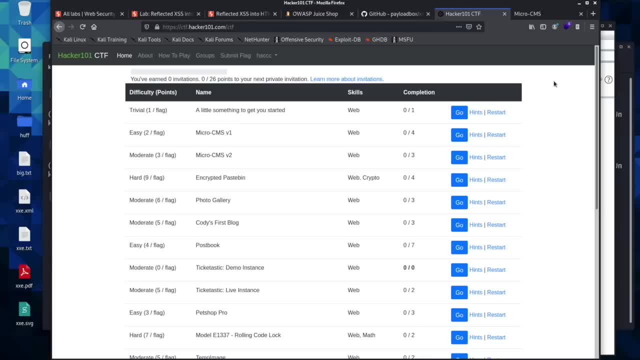 Without any help. But I will do a walk through Here in just a second. So if you would like the challenge, You can go ahead and see if you can find The cross site scripting, And you can do that now. Okay, 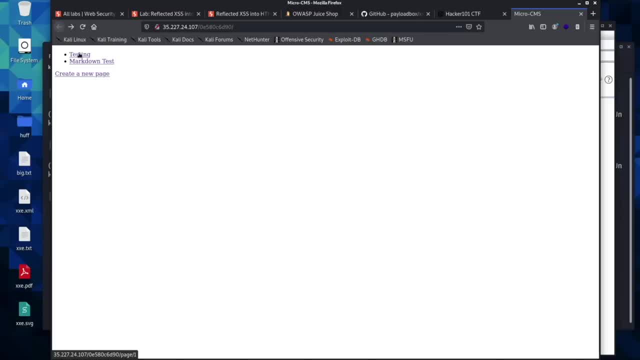 Once we are in here, You can go through, And one of the first things- If you remember from the recon lesson- Is to click through And see what you can find And what you can do. I actually just thought of another way. 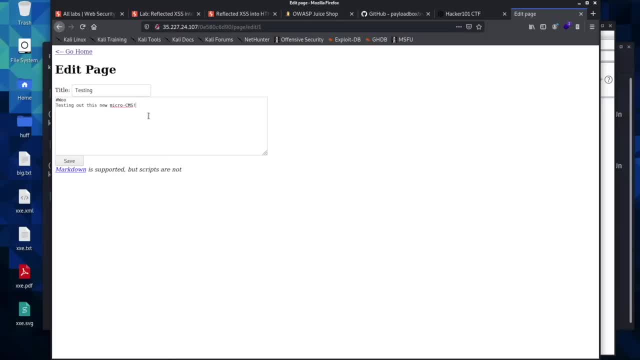 To try and solve this challenge, That I might try And see if it works, And then you can come back And you can go back to the home page. You can create a new page And you can just click through And see what you can find. 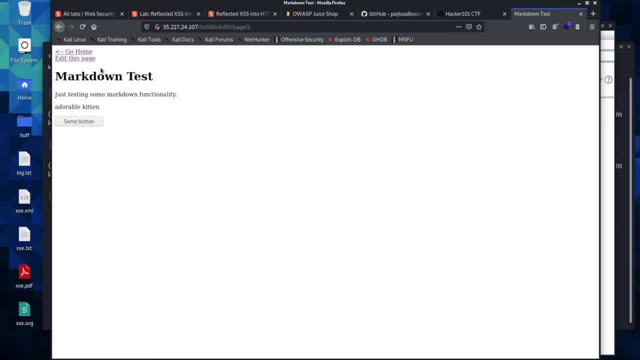 But in the mark down They actually give us a clue As to how to solve this challenge. You have this random Button here. It doesn't do anything, But if you edit this page, We have the tag For a button. 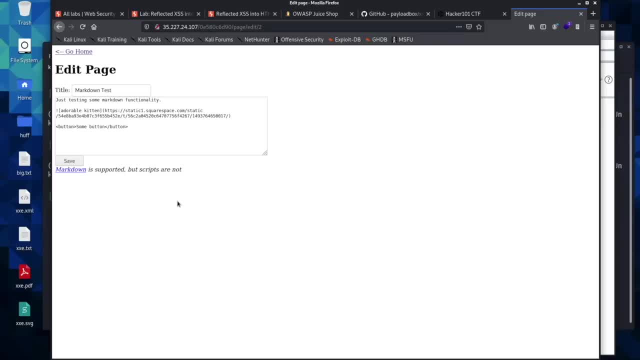 So if you were unable to find this, You can go ahead And try and solve the challenge Now, Because, if you remember, If we have a button, We can come in here And we can go on click And then we can. 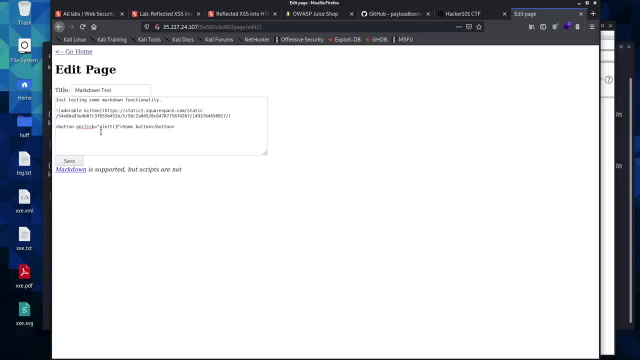 Put in Our alert And then we can Put in one And so we have our on click here And it's closed off And we should be able to save this And on our click We are given the alert I just thought of. 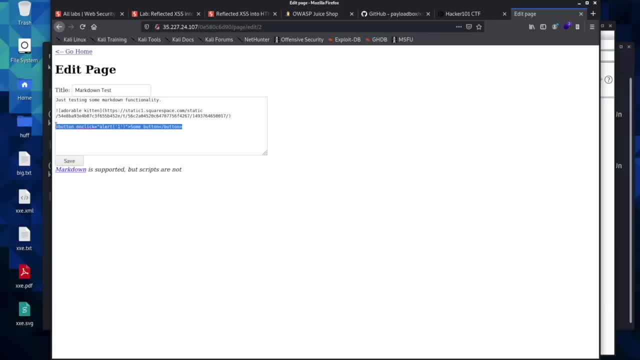 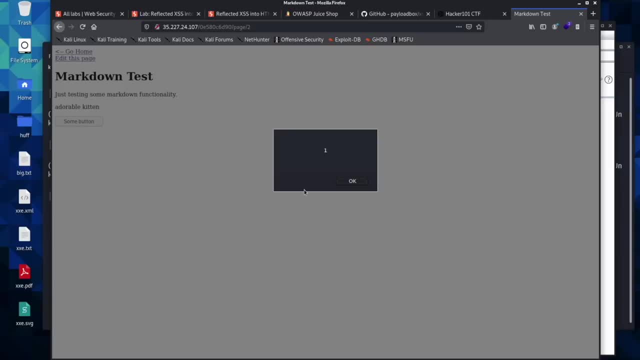 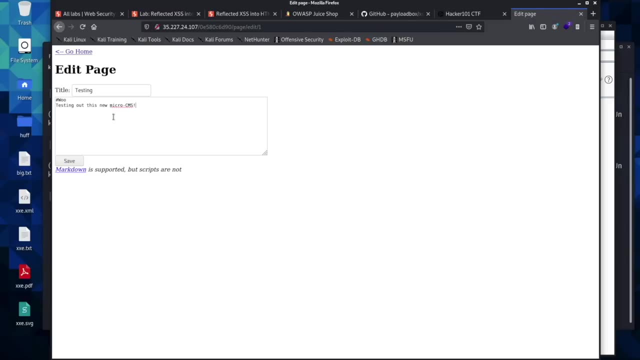 I bet we could copy this. There's another way you could have solved this If you didn't see This button here And You didn't have This clue. But you came into testing And edited And you saw this. 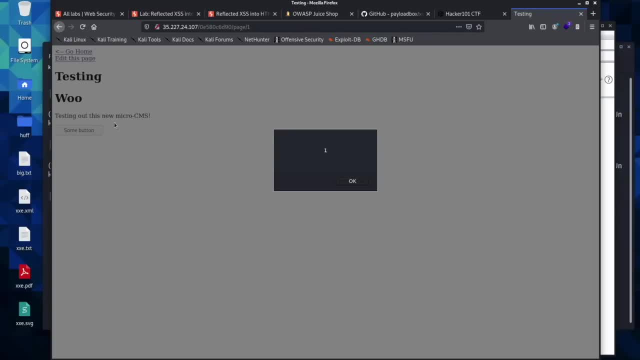 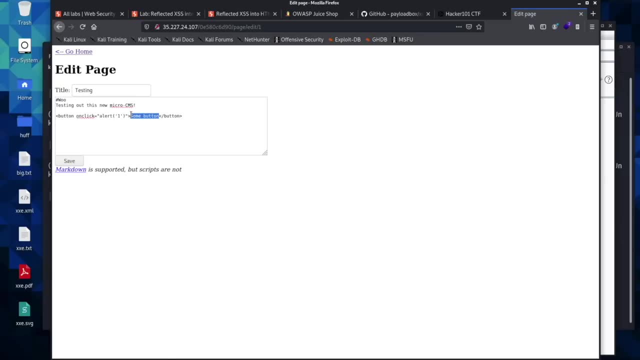 You might have thought to go ahead And just insert your own button And you could have pulled off the same thing, Just on a different page, And we'll go ahead and change this To just click, Just so you can see. it's a different button. 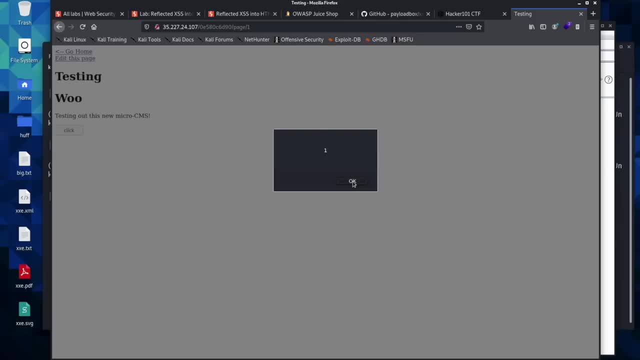 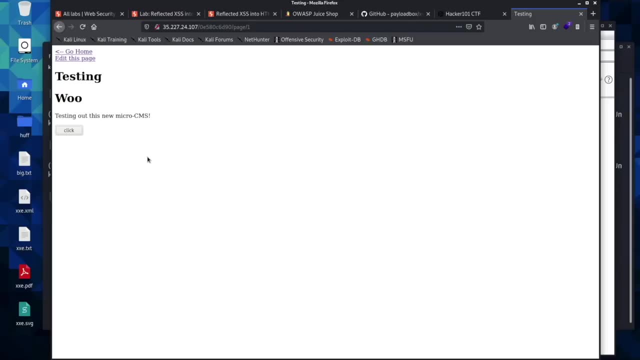 On a different page And we could have done the same thing. So that is Another way To pull this off, And we're going to see a couple of A couple of more examples. And the reason for this Is the cross site scripting. 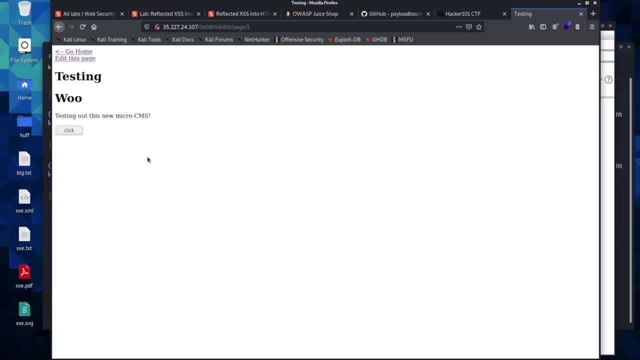 Is a rabbit hole that you can go down Indefinitely. There are thousands and thousands Of different ways To pull this off, And so I just want to show you The basic introduction into cross site scripting, Because, without knowing HTML and JavaScript, 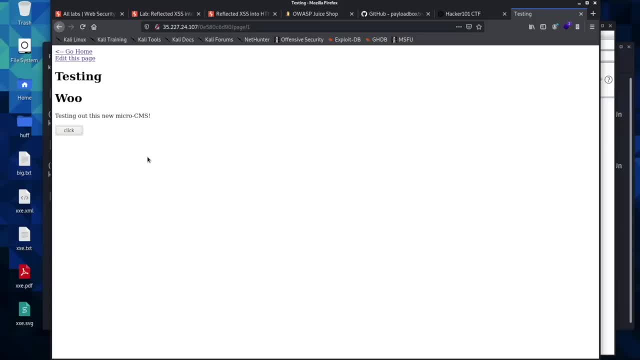 It's going to be kind of challenging To pull these off And since this is a beginner course, I'm not really expecting any Software developers to be In here wondering How to do a cross site scripting, Because if you're a developer, 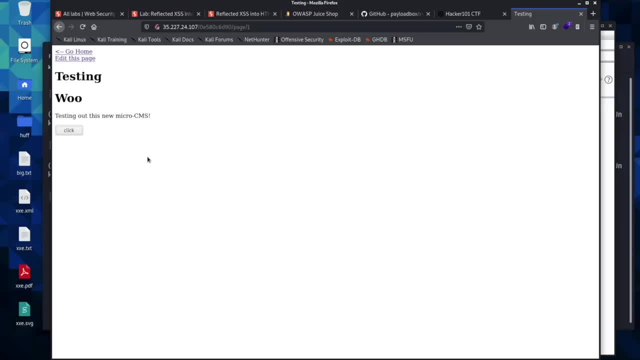 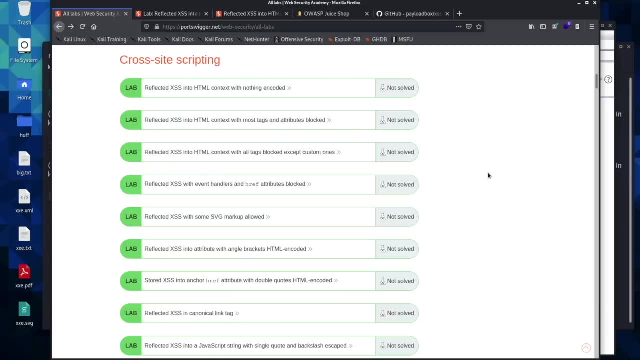 You're going to already know, Because you will have had to Write code to defend against it. Okay, we are going to Come back to Port Swigger And we're just going to do a few of these, Just so you get an idea. 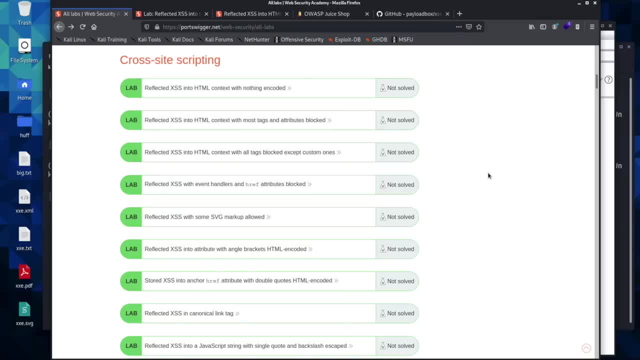 And how people can attack it, And just a little more Understanding of seeing these In context of How they relate to Pulling off these Vulnerabilities, especially To beginners, As you can just copy And paste some of these into: 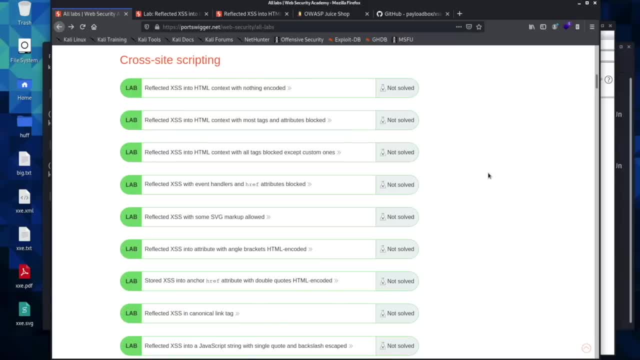 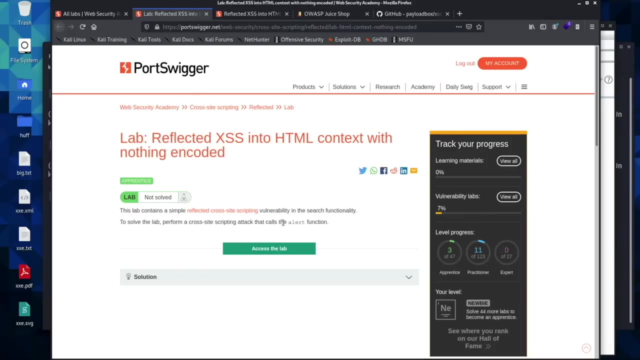 Search engines and search bars And you will See them on hacker one And the hacktivity. And just so you understand what's going on, And open up this first Lab here And we will be told What we are supposed to do. 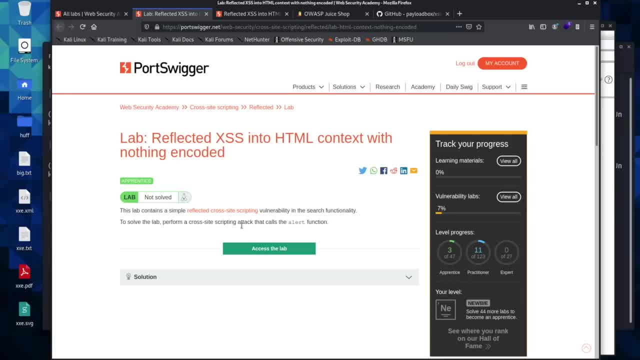 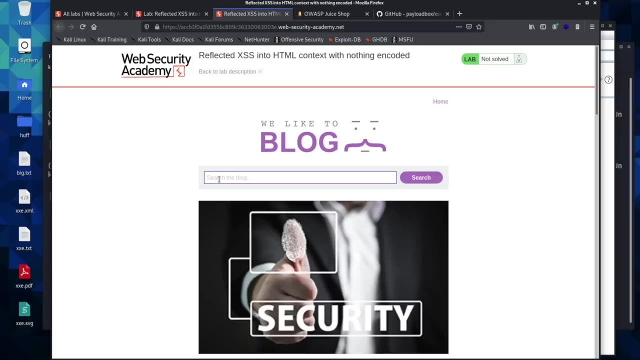 So we're supposed to call the alert Function in order to solve The lab, And this one is going to Be one of the most Basic cross site scriptings That we're going to See And one of the common ways to. 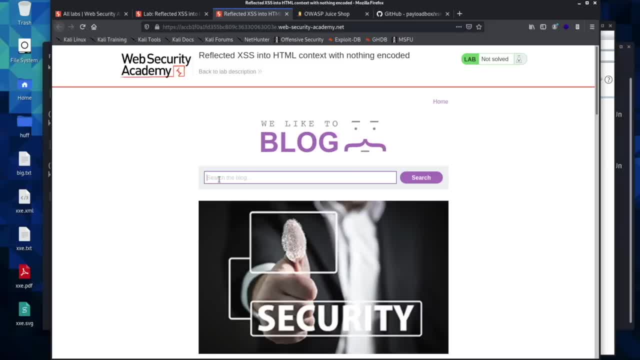 Check to see if a website Or a web application Has any Defense against cross site scripting. In a search bar like this, What you can do Is you can come in here, And this is basic javascript, So we just type in script. 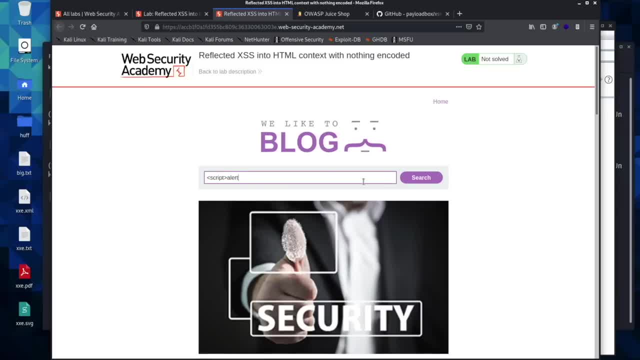 And then we Type alert One And then we close The script tag. So this is just a basic Javascript Command here, So I can type, And so if this Has no Sanitization, Then this should work. 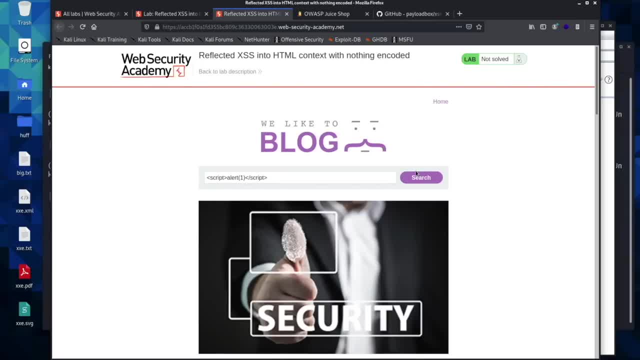 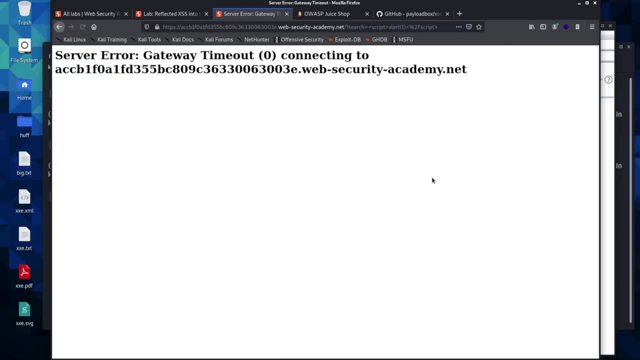 And you can try these In search bars. You can try and post This script to Any kind of social media Outlet for the web application And see if it pulls back Any cross site scripting. So we'll go ahead and search this. 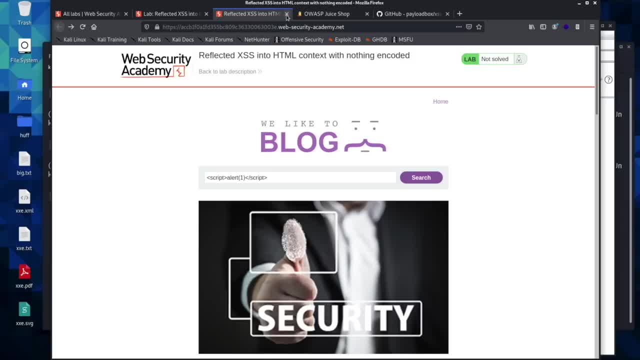 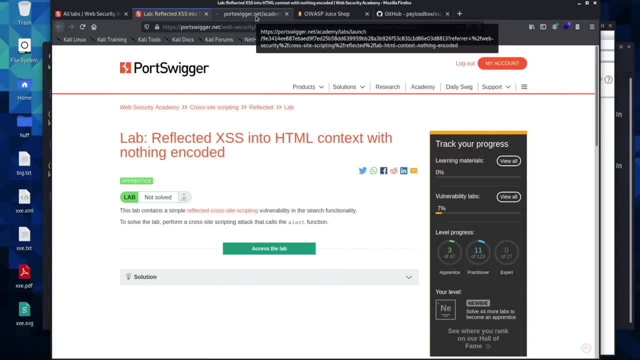 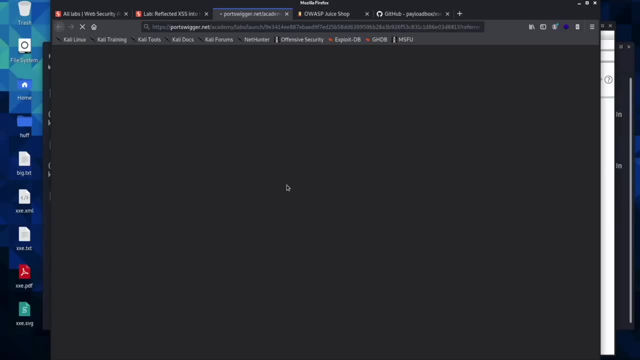 And it says we Have timed out Because I opened the Lab Before I started this video. So we'll go ahead and reopen the lab And let that load, And we'll go ahead And once this is loaded I will actually just paste. 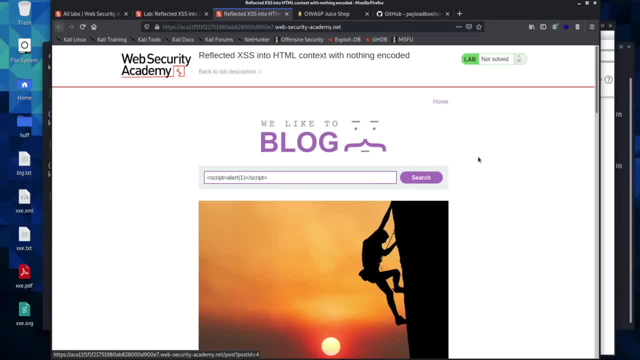 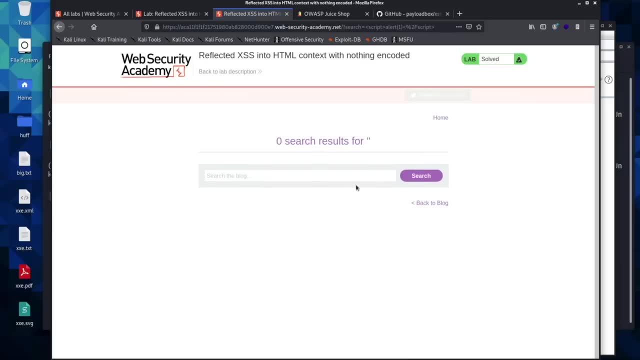 That in. Go ahead and paste that in And we'll search it And it pulls back The alert. We were able to alert one Because we have Solved this challenge. Now, in the next challenge We are going to: 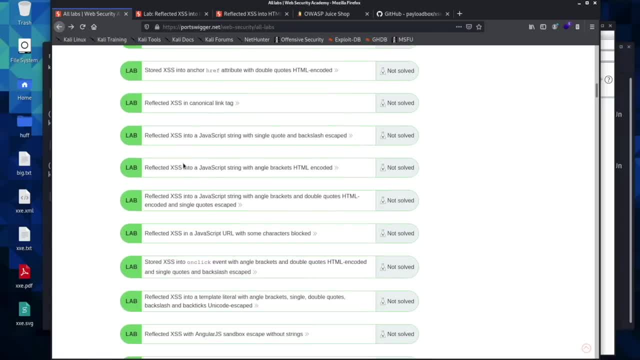 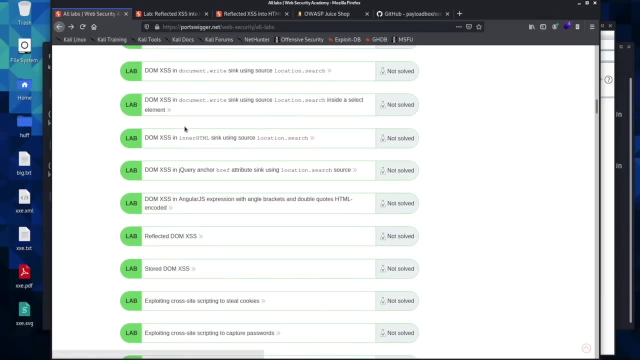 Go over The DOM Cross site scripting, Which I actually think is down here, Because this is one that we have seen With the inner HTML, This one right here. So if you would like to go ahead And open this up, 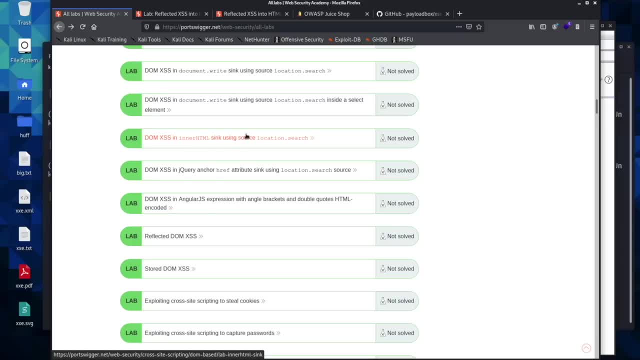 And give it a try And see if you can Look at this payload. before It's not new to you, You will have seen it. You can go ahead and try and find it on your own, Okay, so how did you Get along with that challenge? 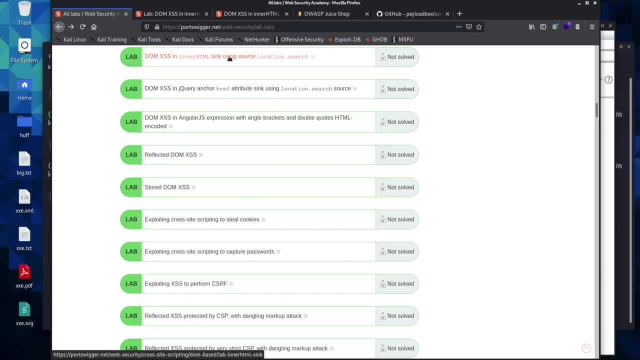 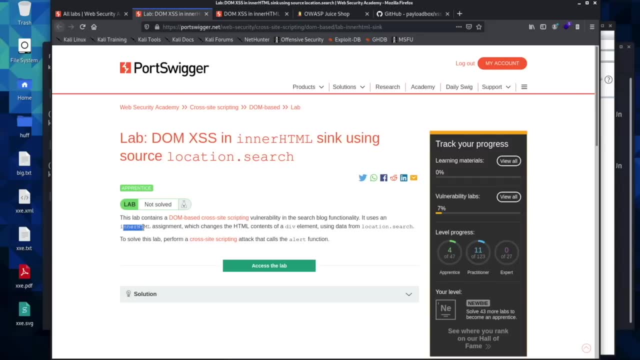 So we can actually come in here. This is the lab we are going to be working on. We can open it up And we are going to be Setting what we type in To the inner HTML, Which means what we are typing in. 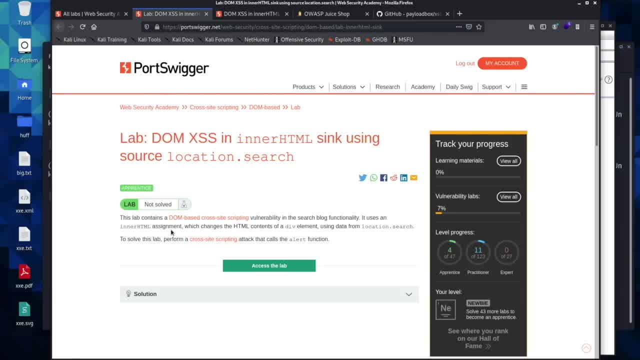 And searching for Is going to be saved on the client side, Which means it will try and render it. This is what I set up When we looked at the Very first examples On the application that I tried to Give you examples. 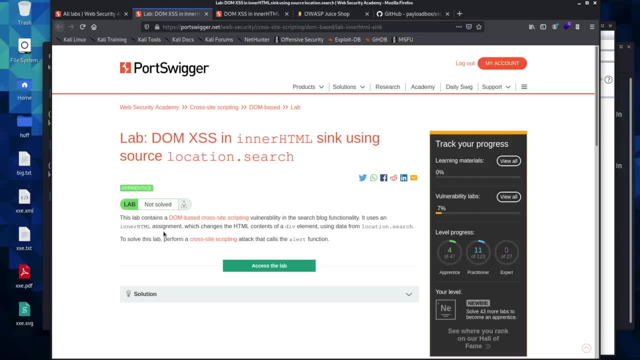 If you go back and look at it, This says dangerously set inner HTML, Which is just inner HTML With the react framework, And so this is going to be the exact same Type of vulnerability That we have already witnessed At the beginning of this section. 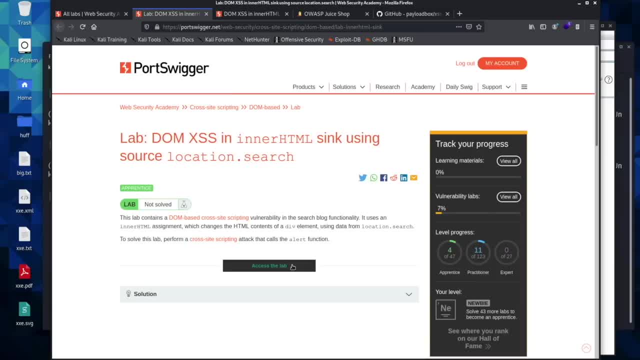 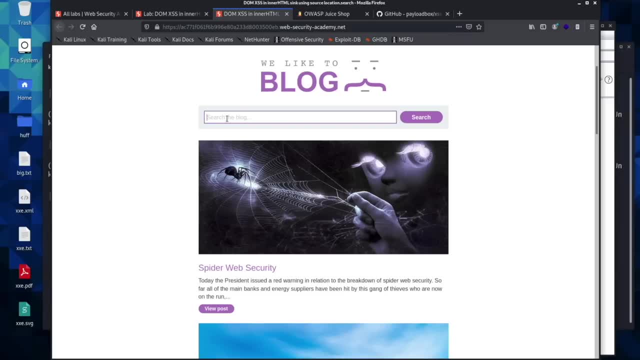 On cross site scripting, So you can go ahead and open up The lab And we will have our search bar And we are going to be doing Essentially the same thing we did In the beginning, Where what we type in Is going to be rendered on this page. 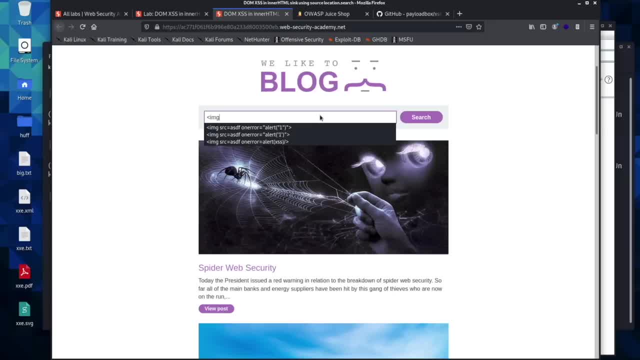 And so we can type in Our image And then we will do our source, Which is where it is going to Look for the source. You can actually type anything in here, And so it is going to look for a file Within this application. 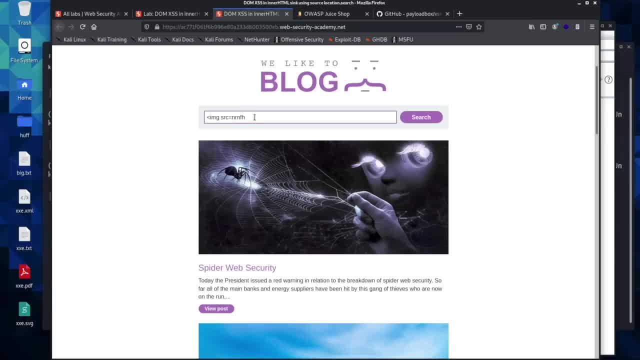 With this name And it is not going to find it, And so that is going to cause an error. And what do we want to do On error? We want to Alert, And then here You would put your Proof of concept. 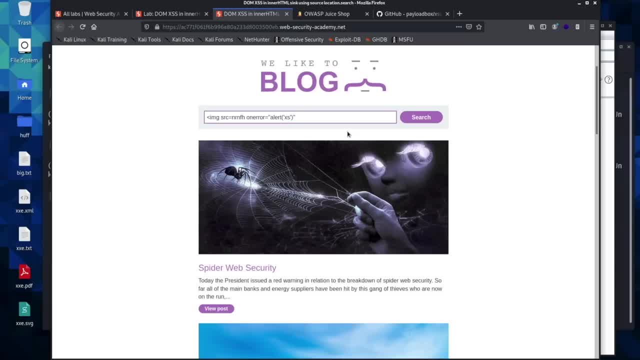 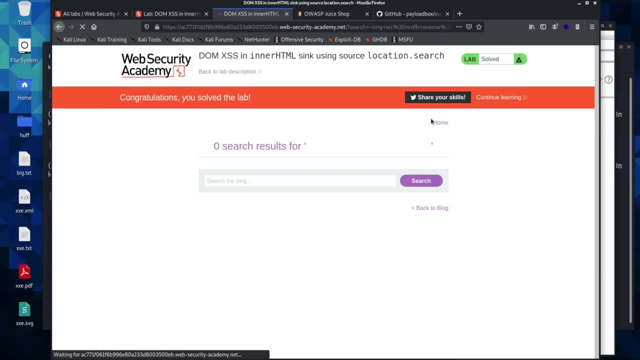 Because we just want to prove That this works And you can type in XSS Or you can type in 1.. Whatever you want, And we will go ahead And close that off, And we can search this And there is. 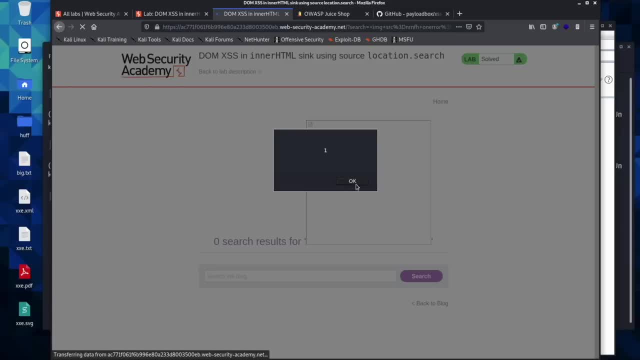 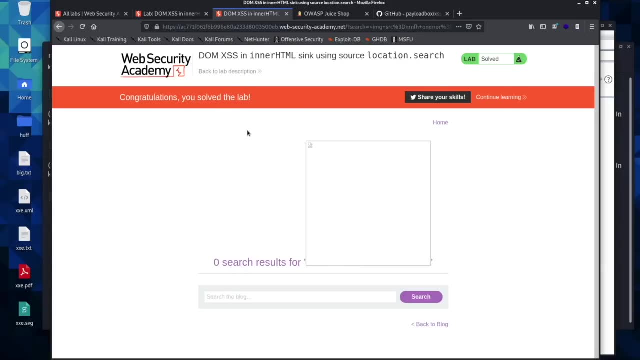 The alert For us. And so with that, That solves this lab And we are going to try one more And I am going to show you kind of. This is a little more Towards the intermediate level Of cross site scripting. 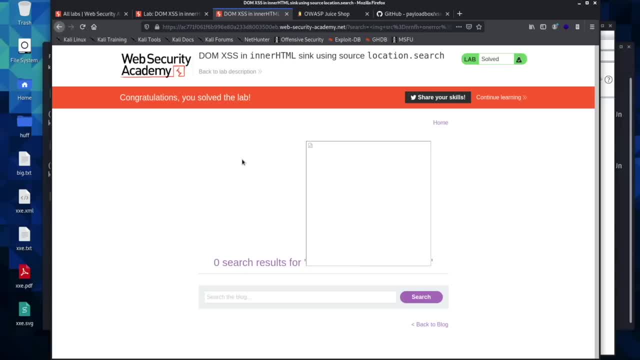 A way for you to know More about cross site scripting And if you come across it And you really think there is a cross site scripting Vulnerability in a website, Just how you can work through that And maybe do some more research. 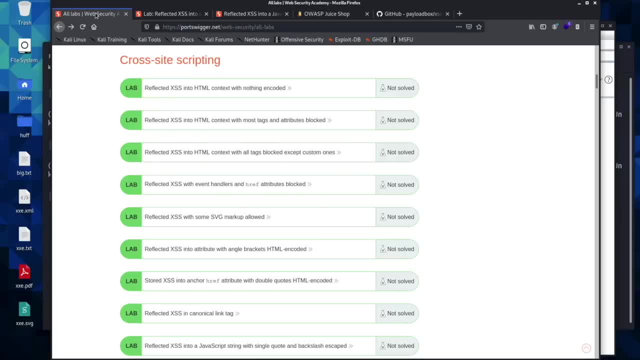 On your own To try and exploit it. Okay, this next lab Is going to be one that Is going to give an example Of what it looks like to start Looking for cross site scripting In An intermediate or advanced way. 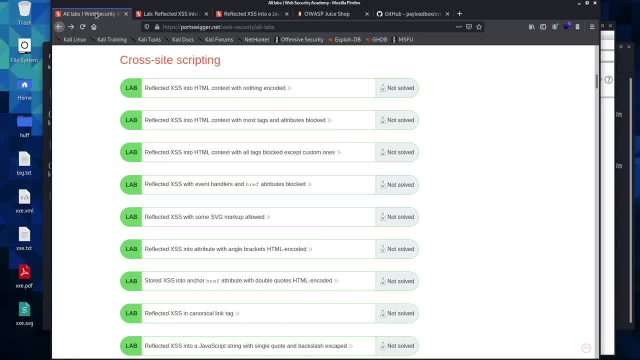 This is going to be probably The most common way That this is going to be found, Because you are going to have to inspect the element And know how to break out of The HTML or the string That you are stuck in. 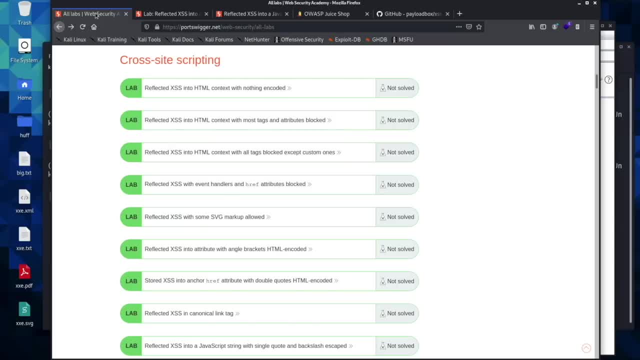 In order to pull off JavaScript And run it within the application. So we are actually going to go ahead And open up this one right here, And it will be over here. It will tell us what we need to do And we just need to. 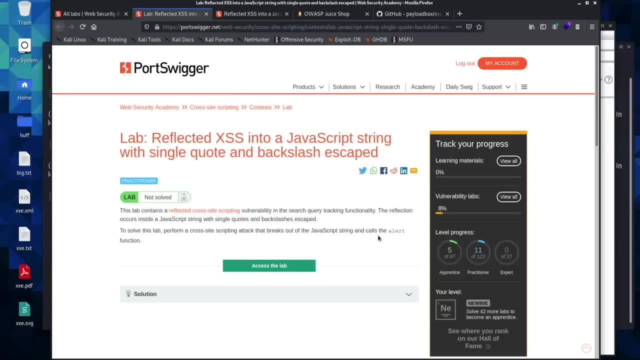 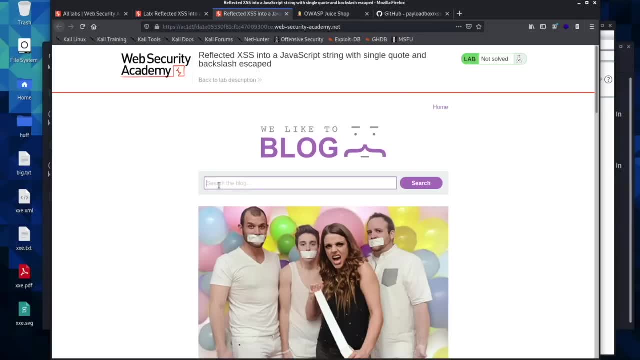 Break out of the JavaScript string And call the alert function. So I went ahead And opened this up, And the most common way to do something like this Is type in something That you can remember what you typed, Or something really easy to find. 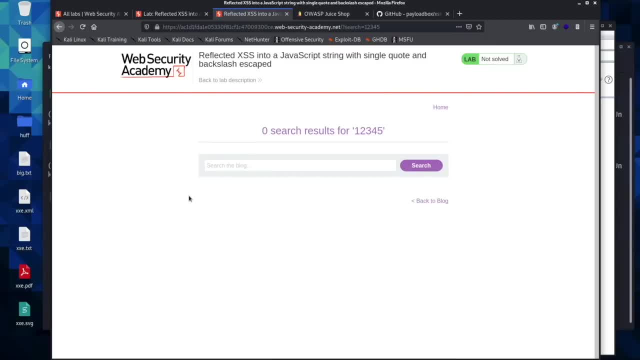 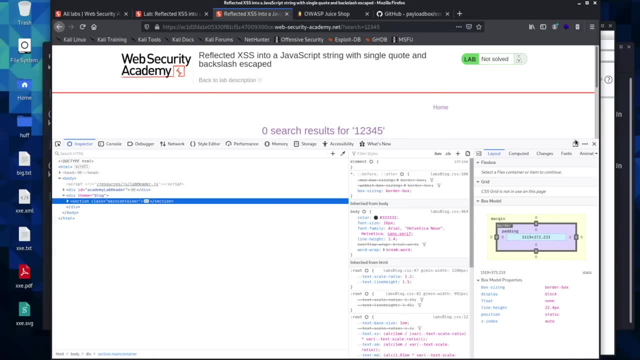 So we will type in 1234. And we will hit search And now what we will do is Inspect the element, Or you can view page source. We will actually do that And it will be a lot easier to see. 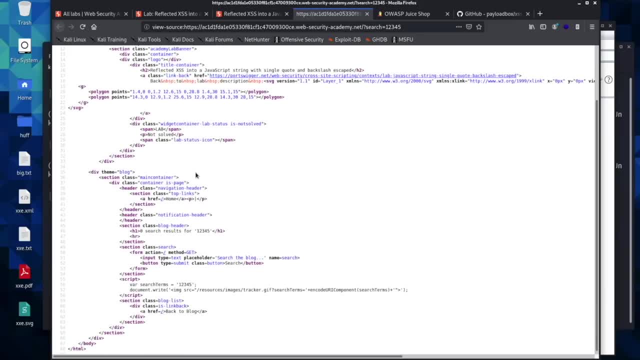 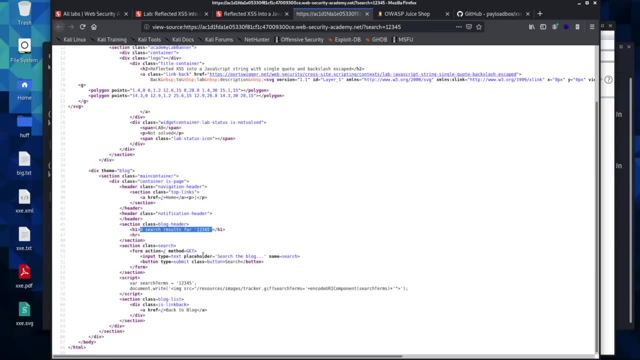 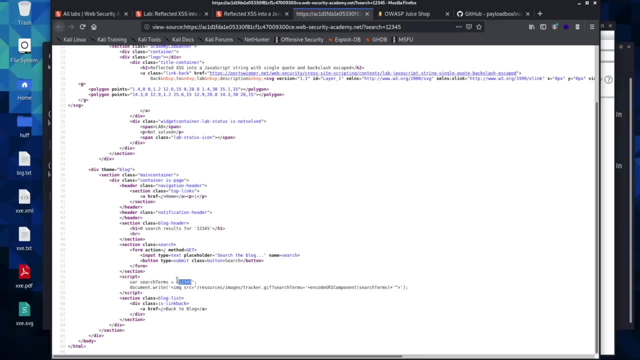 So we will view page source And then we find our 12345.. But this is not Where we are Going to be breaking out of this. See, this is a script tag, The search term. right here We searched for 12345.. 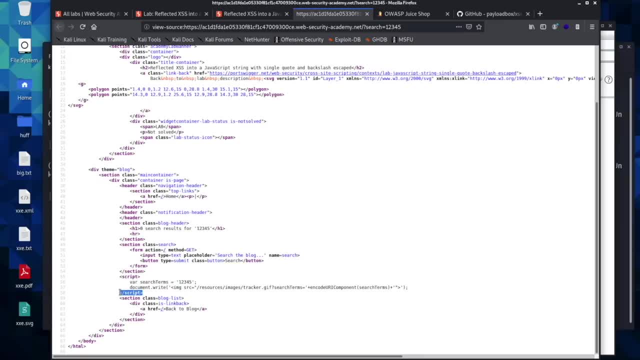 And we have The closing script tag Here. So in order to close out of this, We can actually put A script tag Up here In our search query And it will close all this off. This script tag Will match this script tag. 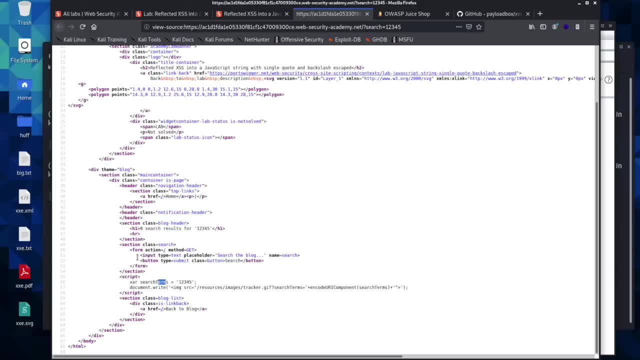 And then we should be able to open up A new script tag And it will run in the order. It will run all of this In the order that it is laid out, And then we should be able to Put in our payload. 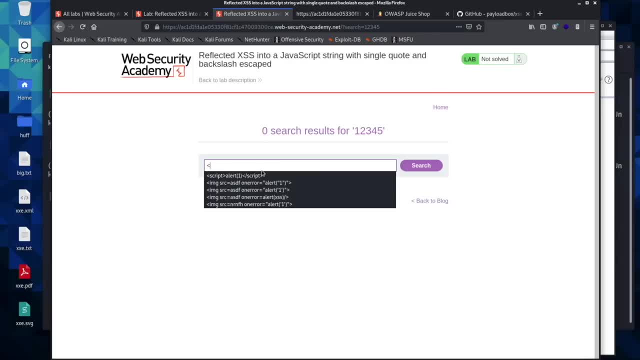 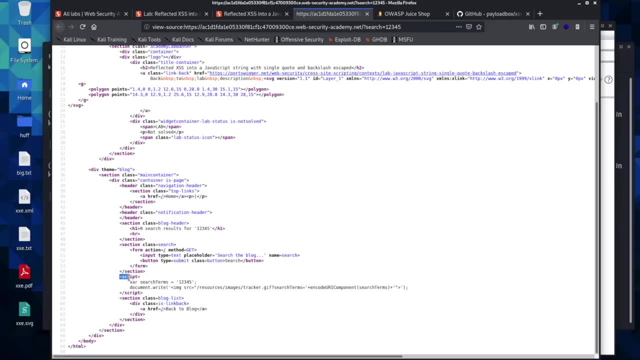 So we will come back to our lab And what we should be able to do Is close off The previous script tag, So that will close This tag And everything before it will be inside that tag, And then we should be able to. 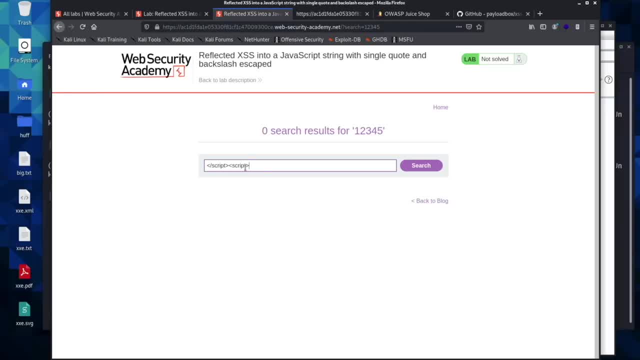 Come in here and type in Our own payload And so we will go script Alert And we will just alert one And then we can close off Our payload And Look at it and make sure it looks right And 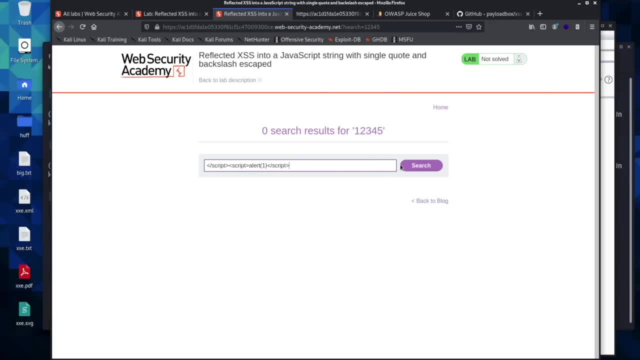 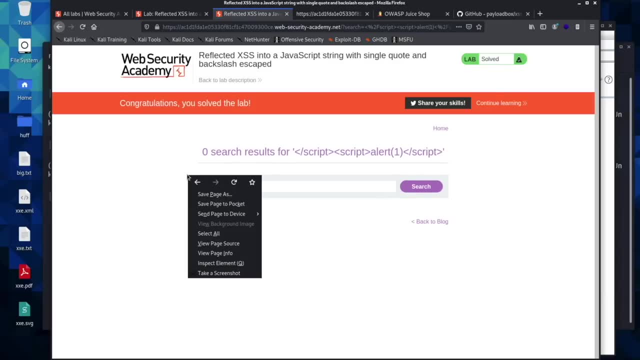 That should Work, And then we will go ahead and search it And there is The alert, which means we have solved the challenge And everything After that script tag Will get rendered on the page Because it doesn't have an opening tag. 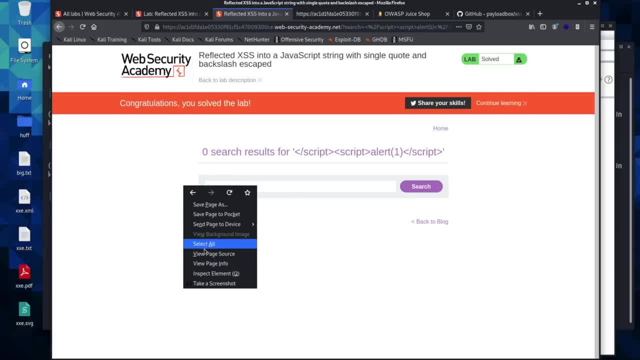 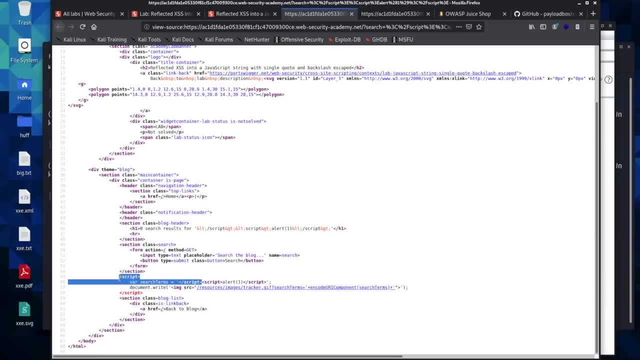 If you are wondering why this showed up, So we will go ahead and we will look at the page source And I will show you The difference. See, here is where we closed off that script tag, And then here We put in: 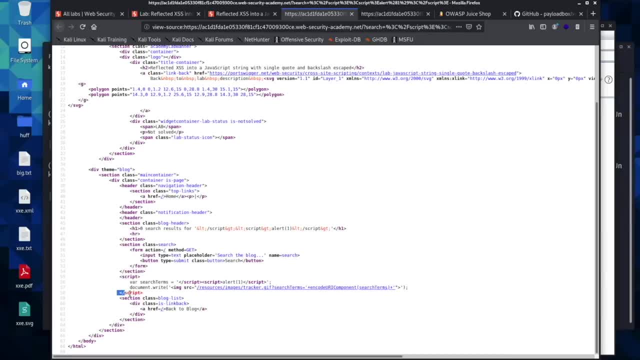 Our payload. And then, because this script doesn't have an opening tag, This Just gets rendered on the page As plain HTML. So if you are unfamiliar with programming, This probably doesn't make a whole lot of sense To you, But when it comes to cross site scripting, 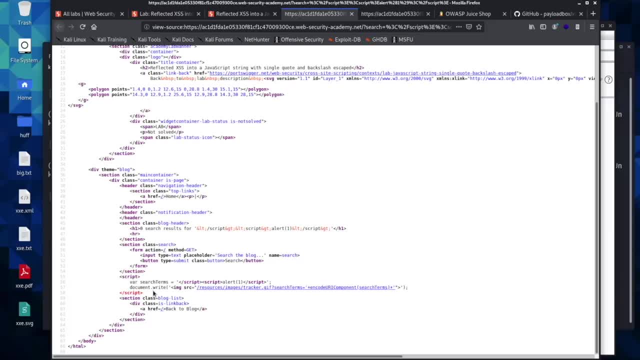 It is kind of going to be necessary To understand HTML And basic JavaScript In order to pull this off. But the reason I included This in This beginner course Is because cross site scripting Is one of the most common Vulnerabilities. 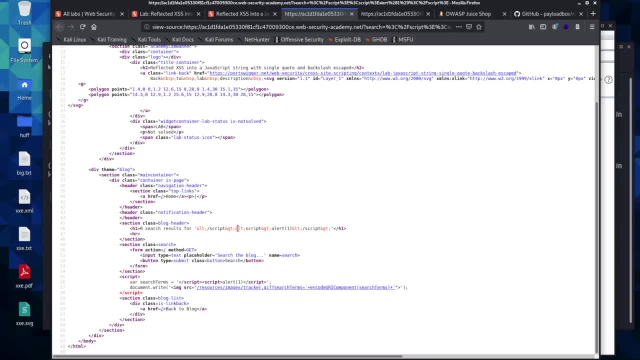 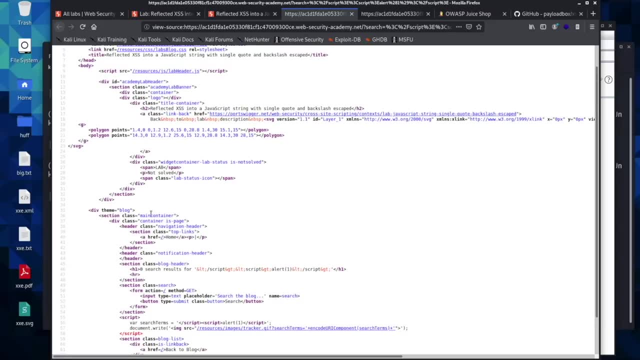 And so I wanted you to be aware of it And maybe you can practice it And see if you can get better, Or if you want to, Before you take the intermediate course, Is go learn some basic HTML, Some basic JavaScript. 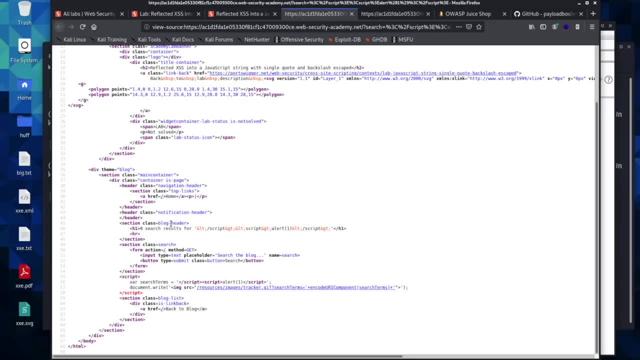 It won't take long. You can learn HTML in a week. You can learn CSS, Which is how to make a website look pretty, In a very short amount of time- A couple of days- And then you can learn basic JavaScript, Probably in another week. 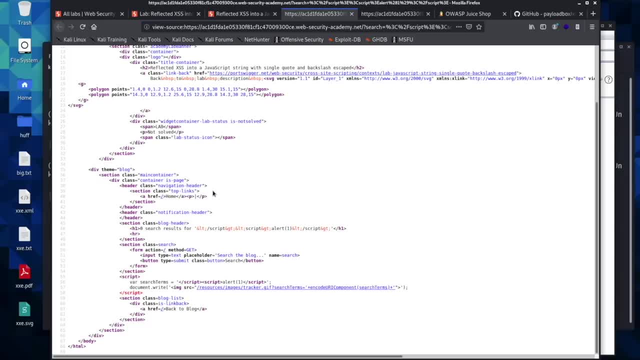 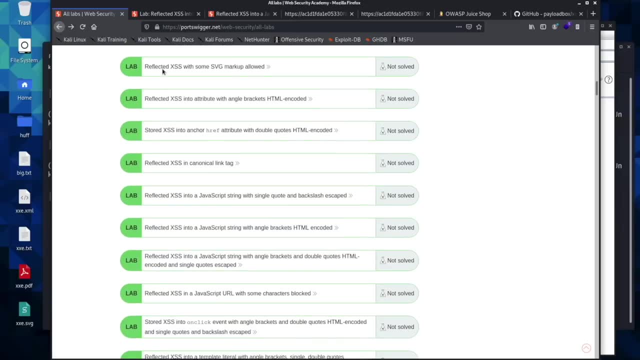 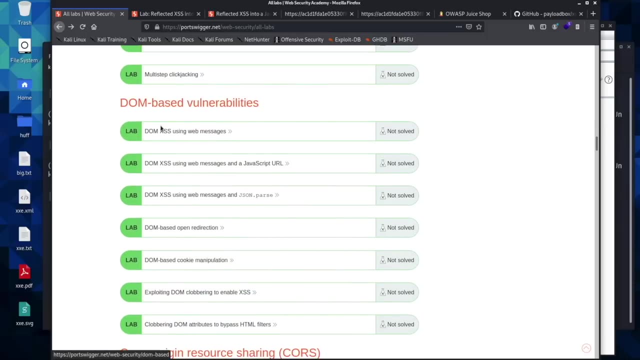 It doesn't take long, It's pretty simple to learn, And so I wanted to show you Cross site scripting. I want you to be aware of it, Because many cross site scripting labs Exist on Portswigger, And I think they actually have DOM vulnerabilities. 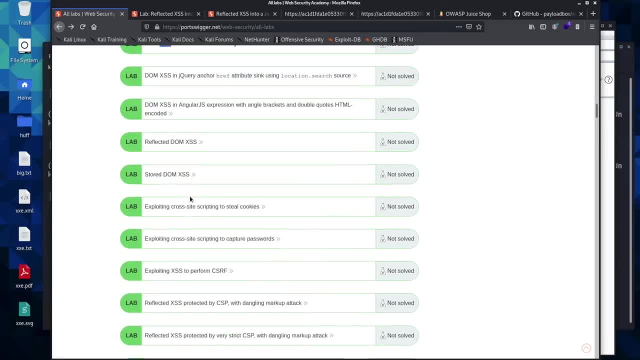 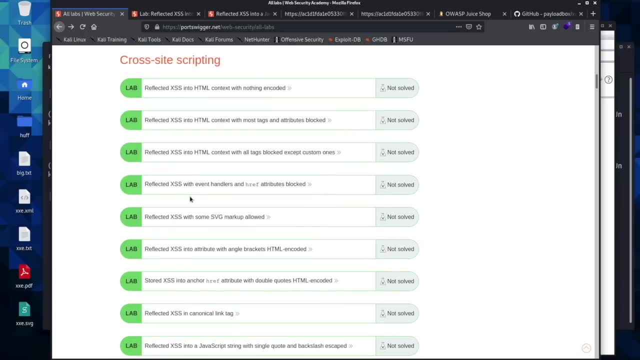 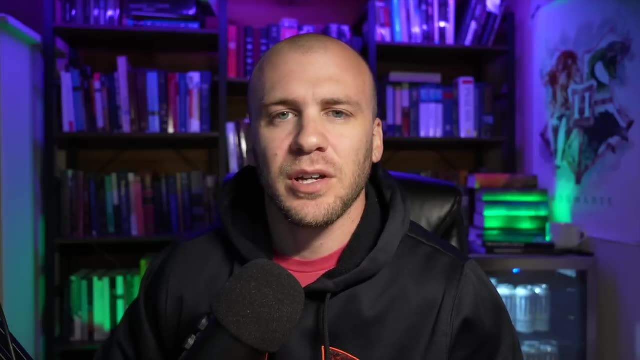 So even more cross site scripting. So there's a bunch, A bunch of cross site scripting. It's really common, But it does take some programming knowledge To solve, And so with that, I will see you in the next video. Hey, thanks for stopping by my channel. 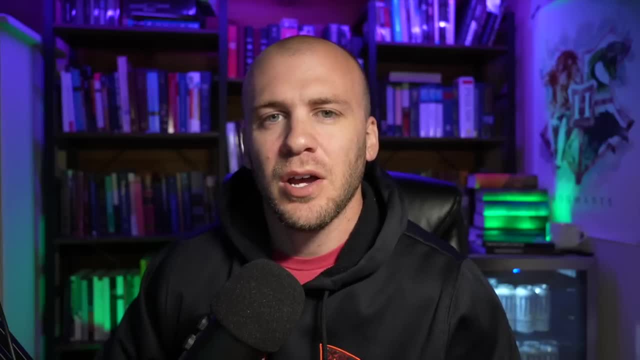 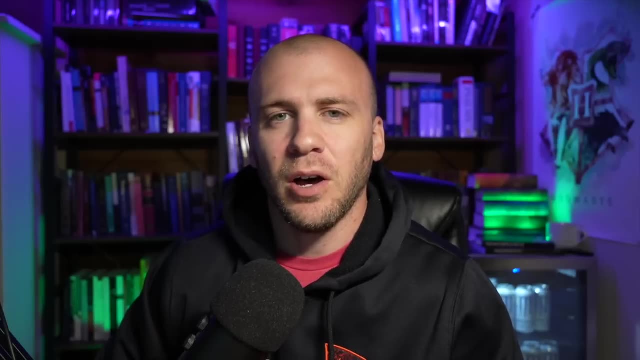 In this video we're going to cover everything I think that you need to know In the realm of HTML and JavaScript. This is just an introductory course, So if you find this video helpful, Please let me know If you'd like me to expand this course. 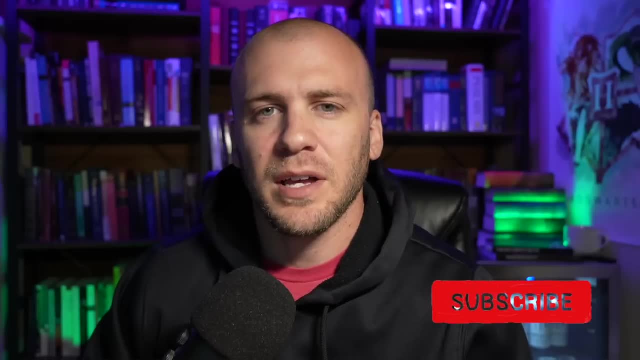 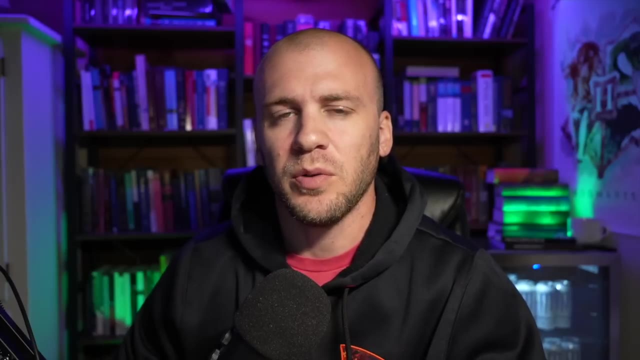 Into a full HTML and JavaScript course For the purpose of bug bounty hunting And ethical hacking. My goal for you in this course Is to come away with the ability to read HTML When you inspect the source code Or you view the page source. 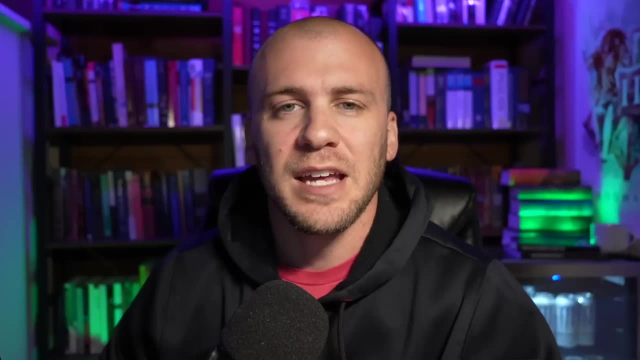 I want you to be able to understand What's going on, What are all the tags In HTML, And I want you to be able to understand How it all fits together, And so I'm going to walk you through How to actually write some HTML. 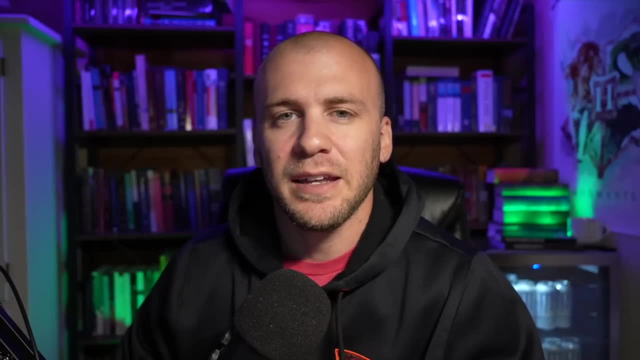 And then from there We're going to move on to view the CSS And how it organizes and beautifies the HTML, And then after that, I'm going to cover some very basic JavaScript. My goal isn't to teach you how to code in JavaScript. 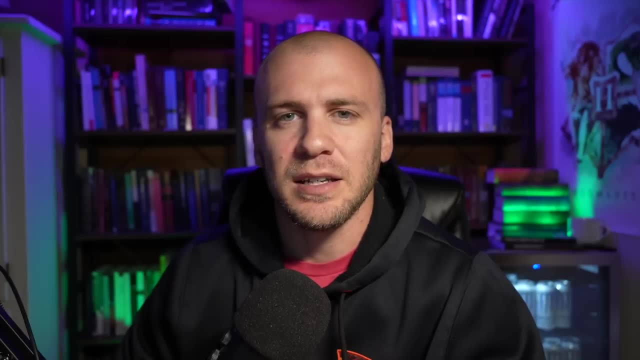 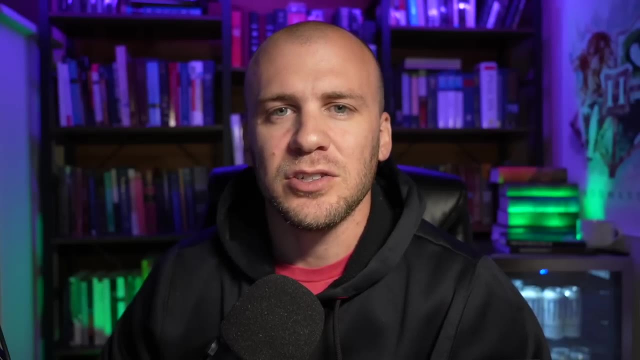 But rather just be able to understand What the JavaScript is doing When you see it. I want you to be able to recognize When you come across it. So with that, Let's go ahead and jump into it. Okay, so here we are at codepinio. 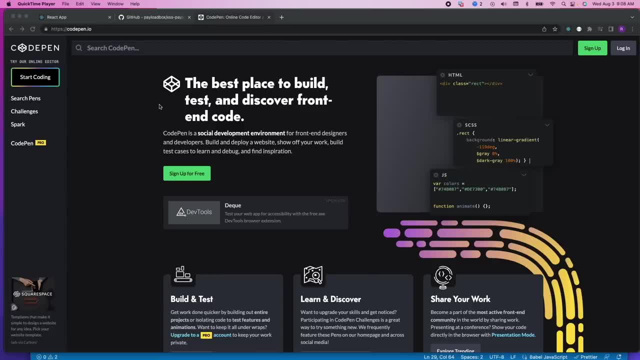 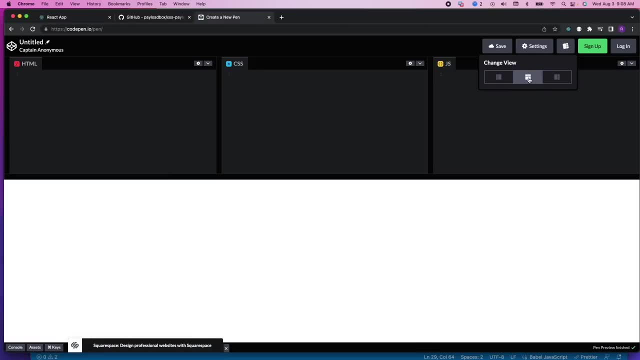 We're going to be starting out with basic HTML And how to understand it, So you can come over here And go to this web application And click start coding And it will load up for us what we need. You might have a display that looks something like this: 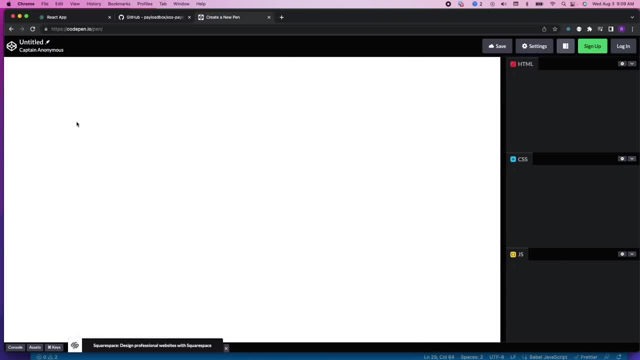 Or this. I like it all the way over here to the right, So that way, my actual website Will look similar to the way you would see it. So we can come over here And minimize this, And we can minimize this Because we're not going to be dealing with CSS or JavaScript. 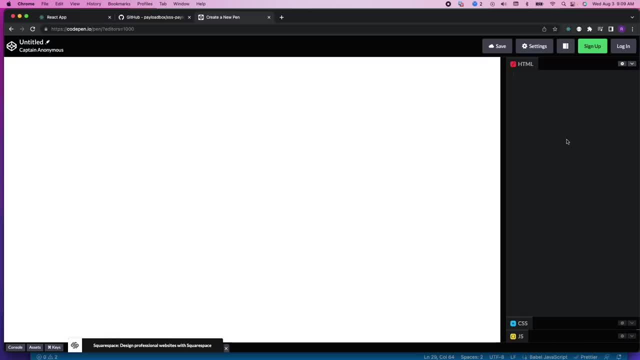 Just yet. And basic HTML and tags. I want to show how HTML tags look. So HTML: What is HTML? It is the hypertext markup language And it's the language of the internet. There's also XML, Which is another markup language. 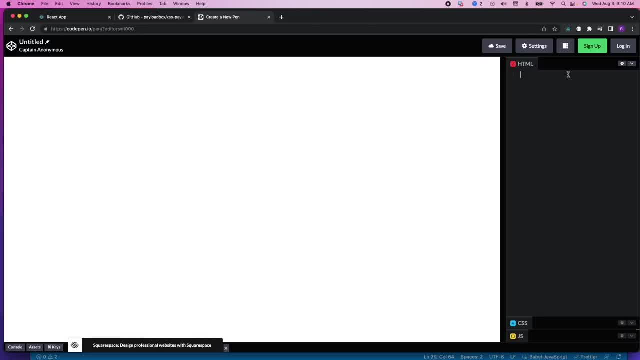 But we're not going to deal with that just yet, Because we are on HTML. You can make static websites. They won't look very nice, But you can make them. And you can do this with just HTML, And so let's just start coding along. 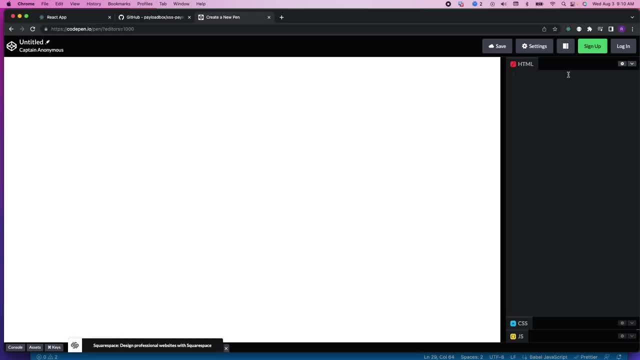 And you'll be able to understand it as we go. So let's say we're making a journal entry to a book Or we're just making a table of contents. You could start out with just a basic H1.. And then you'll make another H1.. 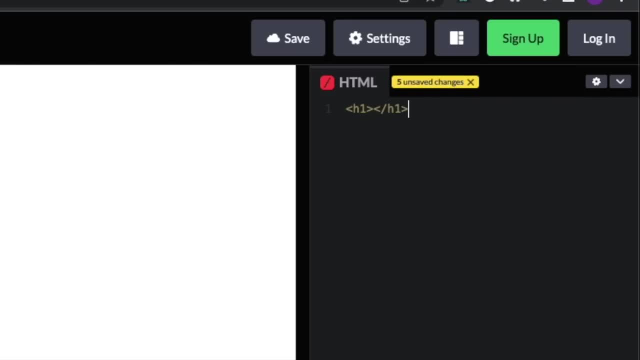 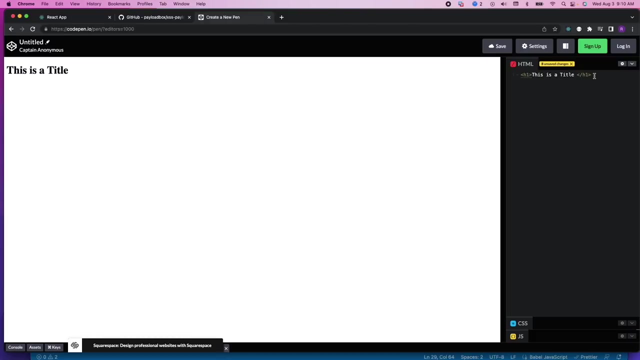 Only you're going to put a forward slash And we're going to close it out. And then in here We can say: This is a title, And then it will render for us Over here And we have this closing tag. 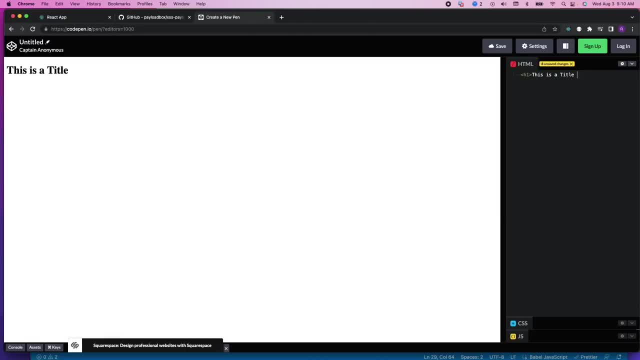 And this closing tag is actually really important Because, let's say, I had by me And as it loads this, It's going to put all of this in here And it puts it all in big font. And when we close this out, 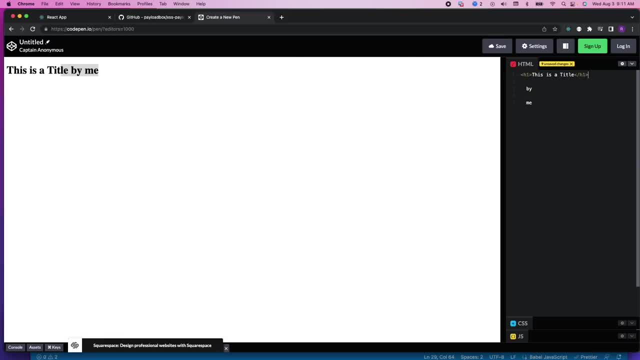 Like we already saw And the way you're supposed to do, It will load it differently. You can see the H1.. Makes the text really big And let's say we want to enclose this. Actually, We'll enclose the me down here. 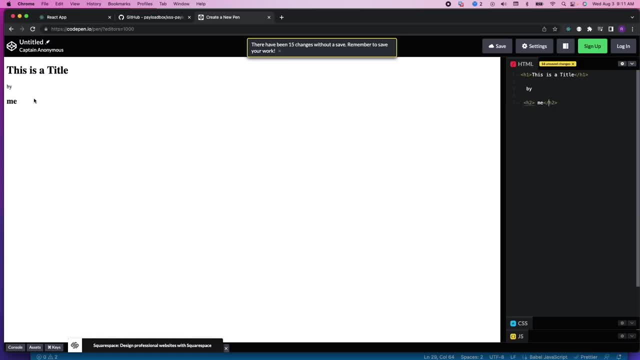 With an H2.. Just like this, And you can see this has changed Right here And you can see that it is smaller. And if we make this, Let's say we want to make this an H4.. You can see as the numbers go up. 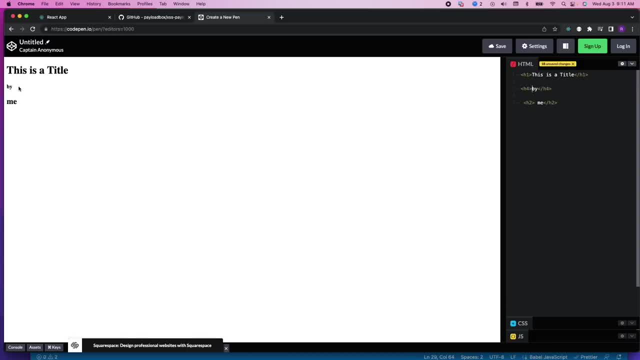 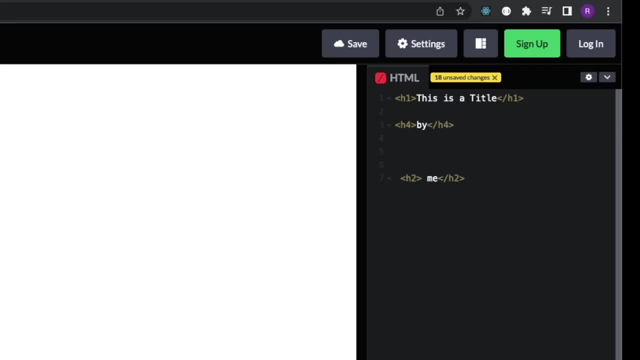 The size, The font Gets smaller, So the H1 is for the top heading And everything gets smaller. And then you also have a paragraph tag That looks like this, And in here would be what you would consider A paragraph: 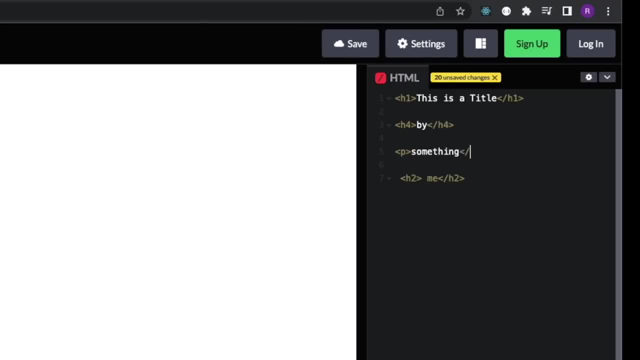 So you can just write in here something And then we can close This out Just like this And you'll be able to see that it renders just the same. And now we have this paragraph tag And paragraphs And you can format the text. 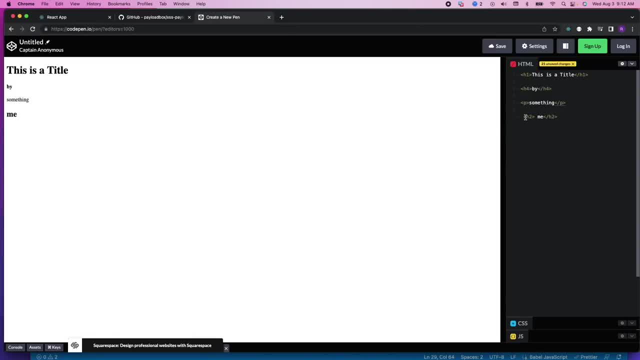 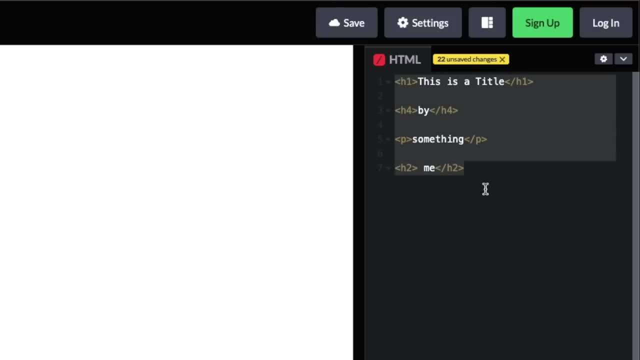 And the style with the CSS, Which we will do later, But right now I just want you to have a basic understanding Of how HTML works And get to understand And be familiar with these tags. You can actually go to a documentation website. 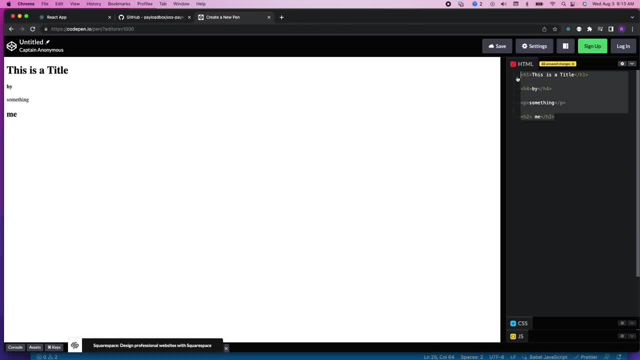 For, such as W3 schools, And so, for now, I want you to get an understanding of these tags And you can go to W3 schools And read the documentation About all the different tags, And we'll provide a few different ones. 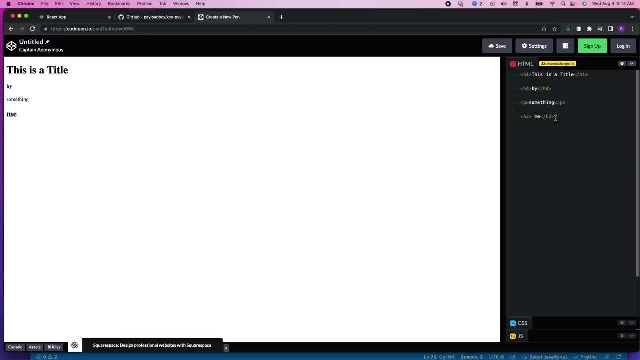 As we go along. But these tags become really important For cross site scripting And other vulnerabilities, Because we're going to have to learn how to break out of these tags In order to insert our own malicious code In the future. Okay, so, now that we are, 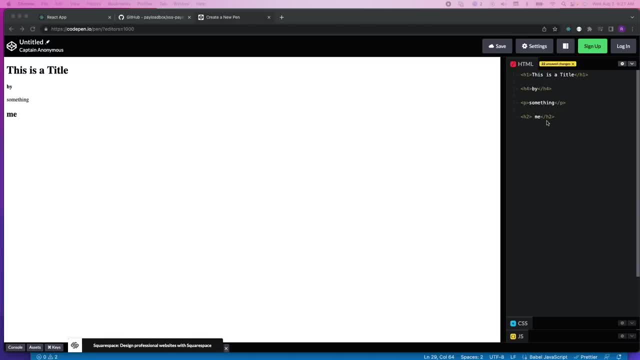 Familiar with a closing tag. There are some kinds of tags That do not require a closing tag, And these are typically tags That do not have any input. Like these, all take Some kind of text That they render on the page. 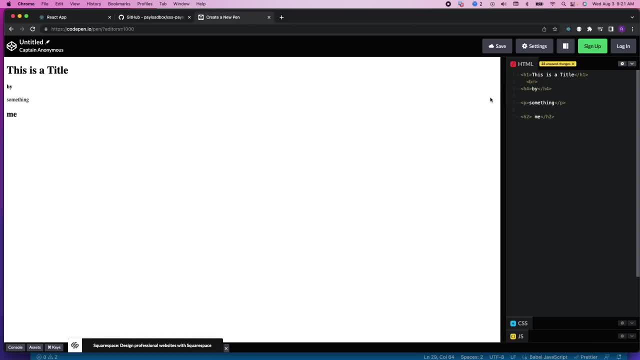 There are some tags that are self closing, Such as a break tag, And this tag does not take any text or input, And what it does is it spaces out these gaps Right here. And there is also another tag Called an HR tag. 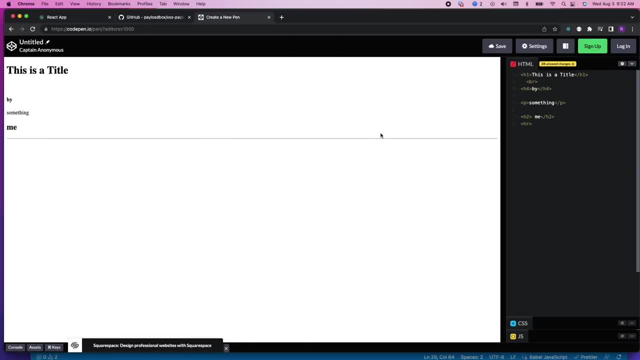 And this will place a line Underneath of the text. This is usually done in like basic Resume style HTML websites. You won't really see a whole lot of this In web applications And if you do, usually stuff like this is done. 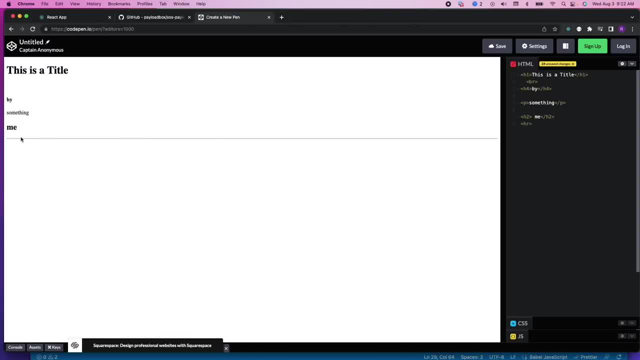 With a border inside of CSS In a div, But this is something to be aware of, That there are self closing tags Within HTML And you will probably see these. I want you to be familiar with all the different kinds Of tags you are going to be seeing. 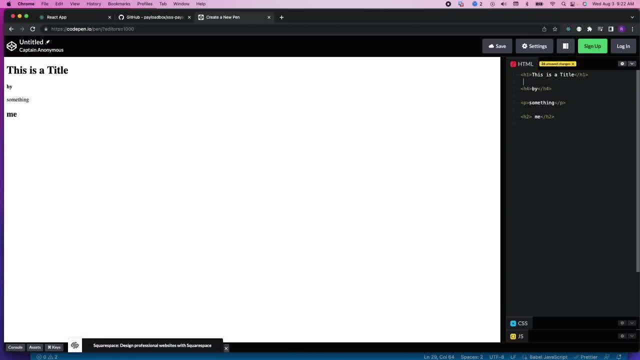 When you are looking through source code And you are looking for vulnerabilities As well as trying to figure out How to get a cross site scripting to work. And it is always helpful To be familiar with the tags, Because some tags may be black listed. 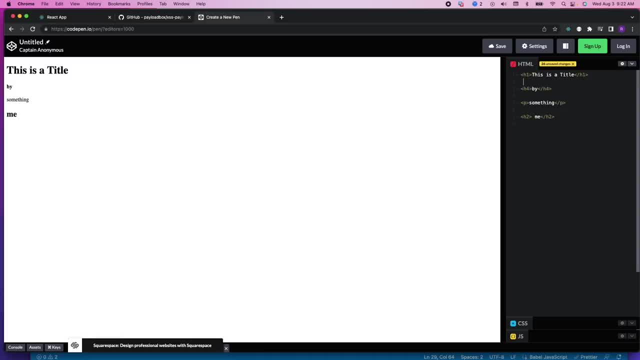 While others are not, And they can be helpful in helping you Break out of an HTML element In order to get a cross site scripting to work. And another thing To be aware of If you see something like we just saw With the HR: 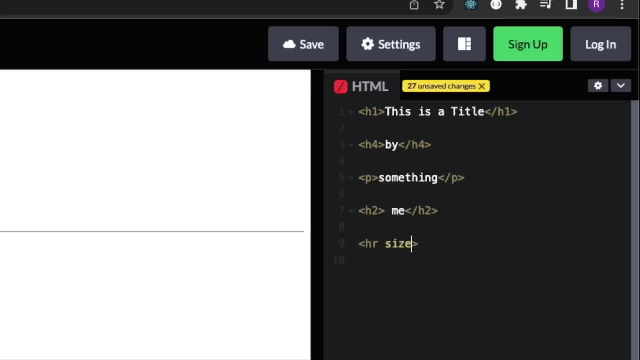 And we see this pop up on the screen And we decide We want to add a size to it And we want to make it bigger or smaller, And you can see This is running in pixels. So if we do 39, that is going to be really big. 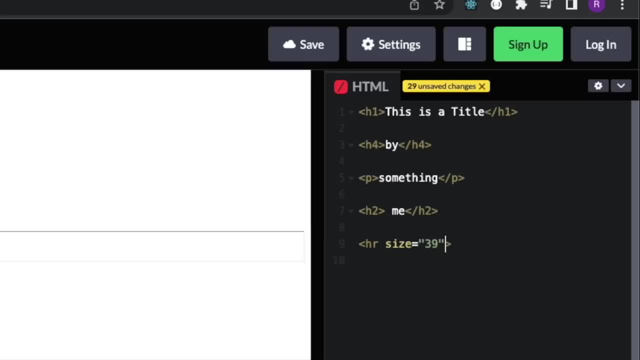 I meant to make it just 9.. You can see that our line shows up And I think you can also add a shadow, But I don't remember how to do that With an HR tag. If you ever see this And you are wondering, 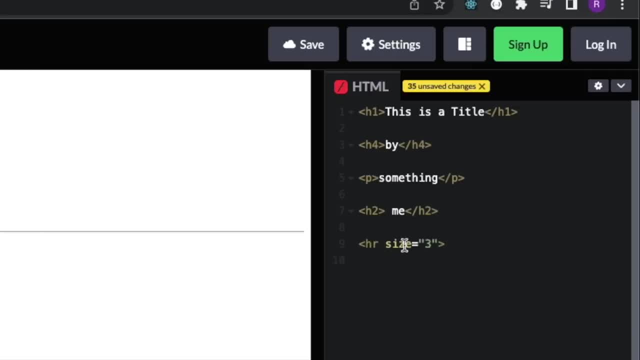 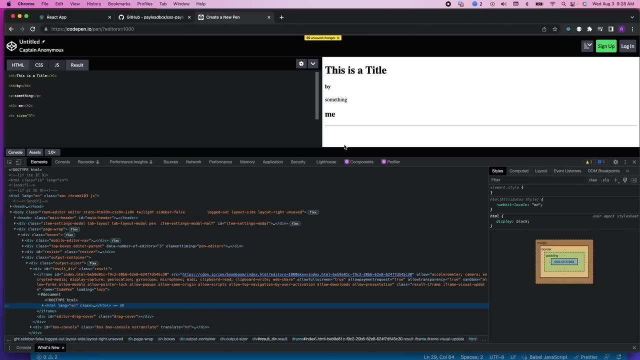 Wow, I really like how this looks. I would like to be able to make a tag That looks just like this one On a web application. You can inspect And see exactly where it is at. Let me see if I can. We will grab this. 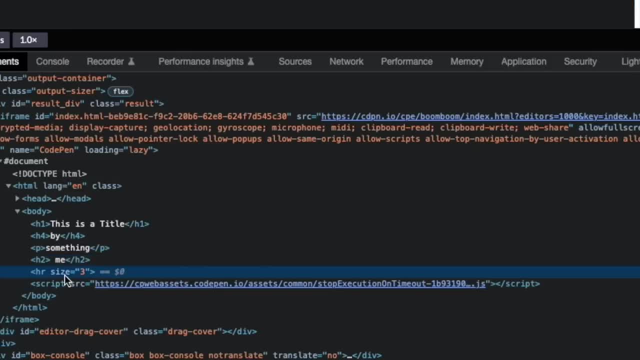 Inspect, And right here You see the HR, size 3.. And it is really important to Be familiar with inspecting specific things Because it is possible In the future that you are going to have an input field And you are able to search. 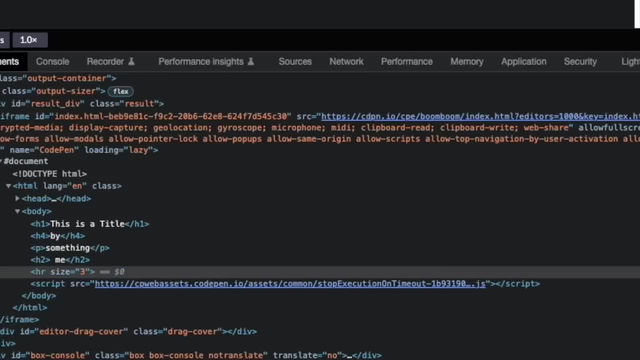 It renders within the HTML And you are going to need to be able to inspect To see where the word is Within the HTML. And that is exactly what you need to do In order to break out of it, To get your malicious code to run. 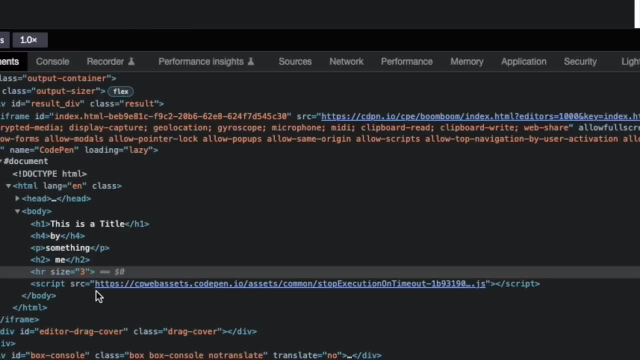 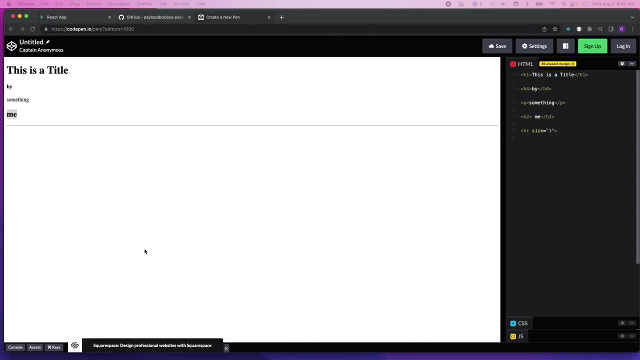 We will get more into that in the future, But for now Let's continue with HTML And what it looks like And becoming more familiar with it. We are going to move on from here And we are actually going to install a text editor. 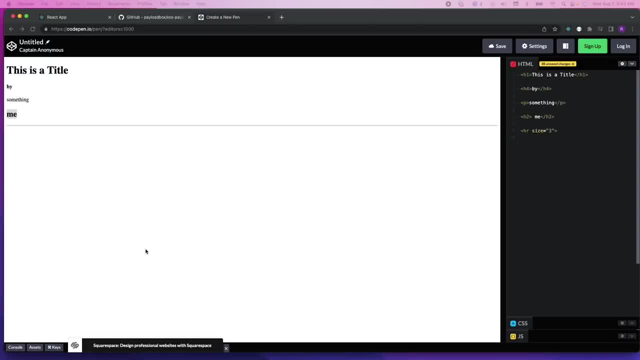 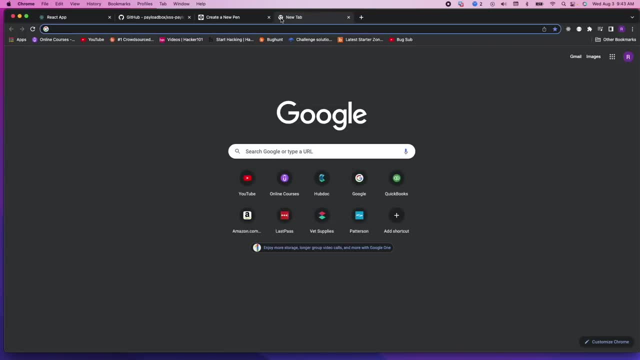 I am going to have you install Visual studio code if you are new, Or you can use whatever text editor You would like, But I am going to be using VS code, So what I am going to do Is come over here. 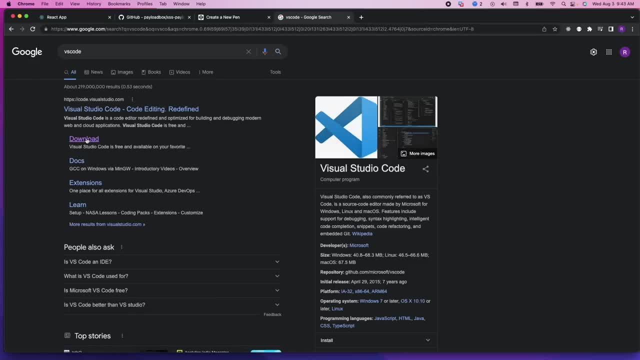 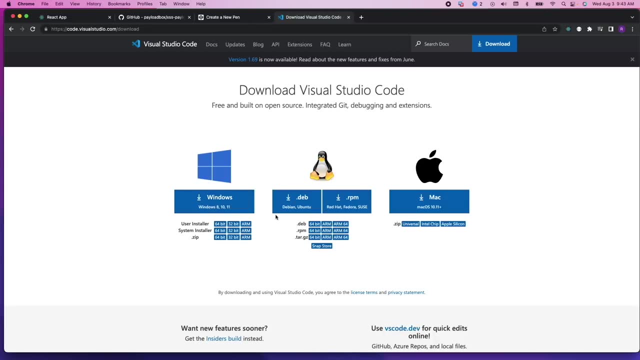 And we can just type in VS code, Just like this, And you will come to this page right here You can click download And you can download it for whatever OS system you are using, And you can go ahead and download it And then install it. 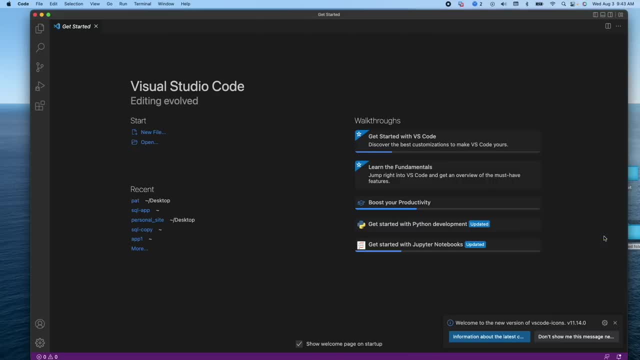 It is pretty simple to install and open up, And when you are here You will want to make a new folder, And I am just going to leave it. We can barely see my folder As test app. You can call yours whatever you would like. 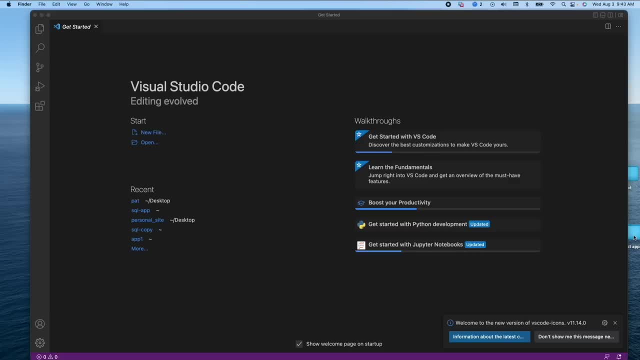 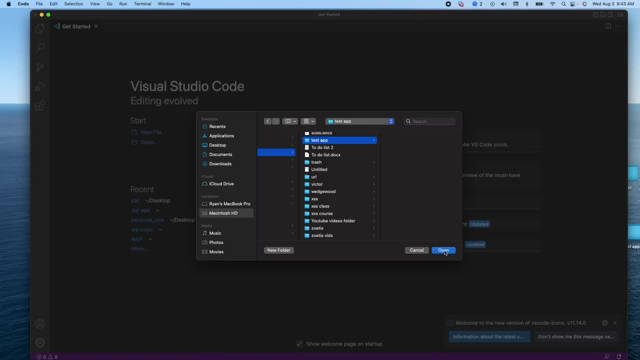 And then we are going to open it up, So we will come over here, Click open, Go to desktops And I named it test app right here And I can open this And it will open over here just like this And we can open up a new file. 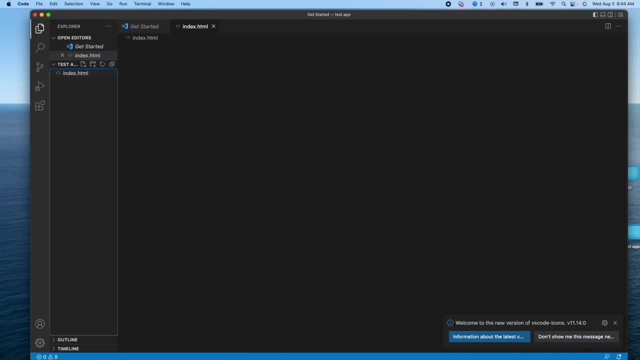 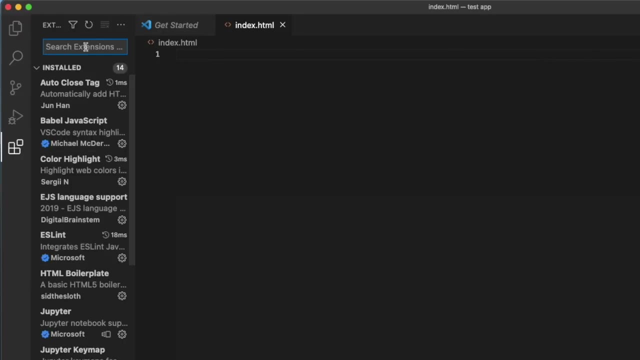 And say indexhtml, And when we hit enter It is going to open up Our indexhtml, Because we are in VS code And we want to install plugins. I am just going to have you install one plugin right now And we are going to type in boilerplate: 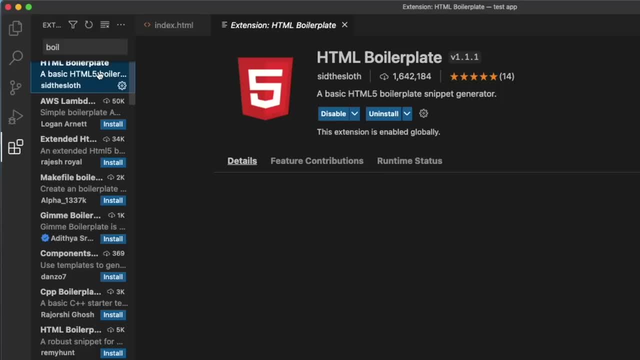 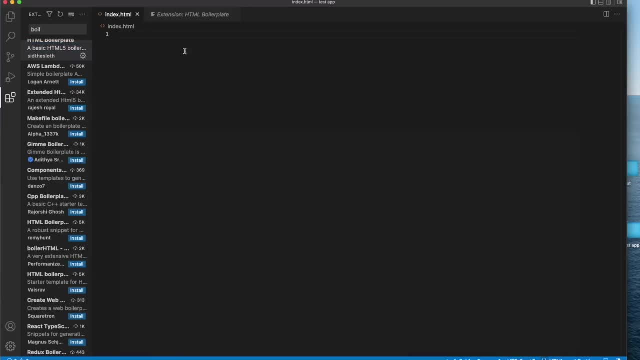 I think you can just type in boil And it goes ahead and opens this up: We want html boilerplate. And you will hit install right here I already have it installed. And then, when we come back to our indexhtml, If we just type in html, 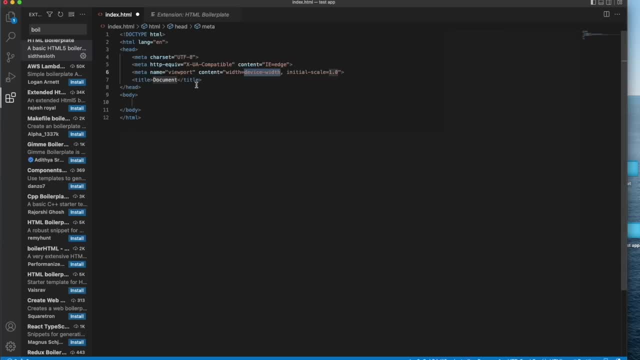 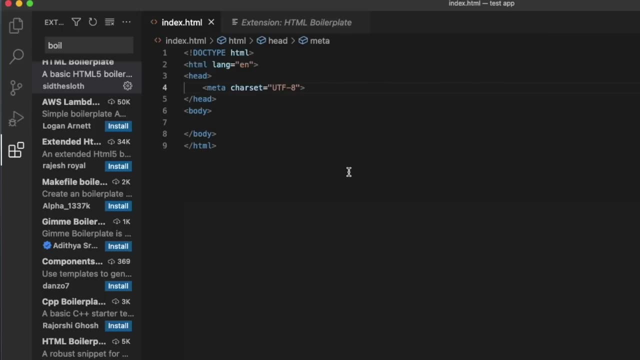 We can go down to this 5 right here And hit enter And we will be given the boilerplate And now you can delete this right here. This is how we want to keep this. Save this right here And a helpful tip. 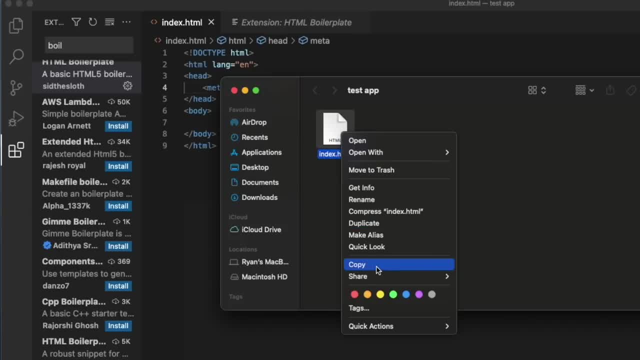 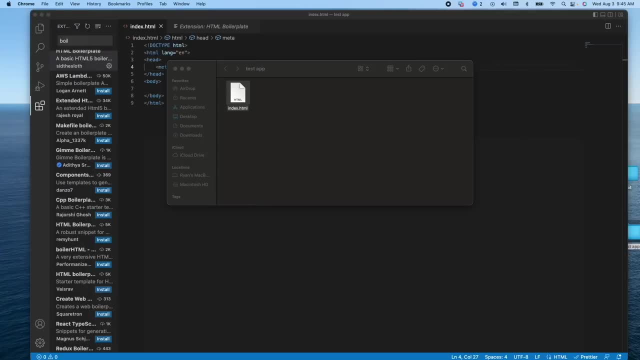 To render what we have going on in a browser. We can just right click And we can just say We want to open with Google Chrome And it will open up a page for us like this: I actually want to put this page. 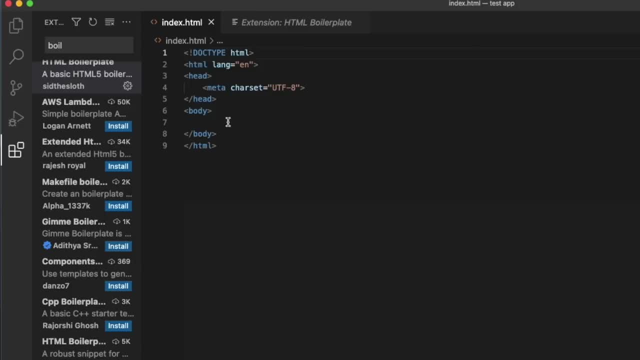 Over here, So you can see it. And if we just come over to our body right here And we just type in And let's make it in h1. And we will just say Hello world. And if we come over here, 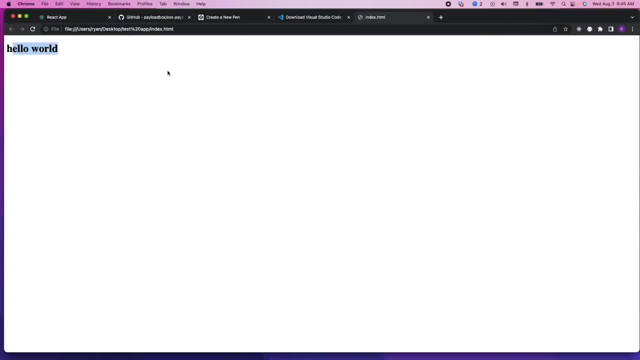 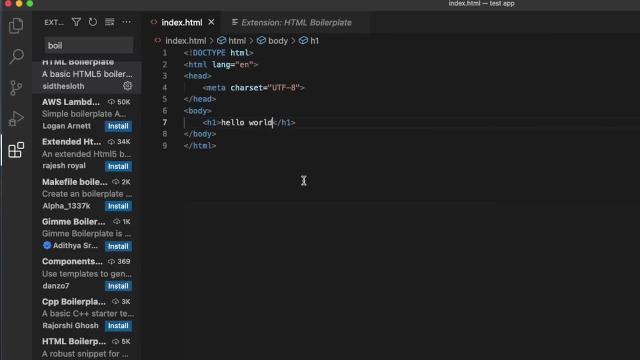 And refresh our page. It will render for us our hello world. So, now that we know everything is working, We are going to begin looking at a little more In depth advanced html That we will need to know In order to break out of our html. 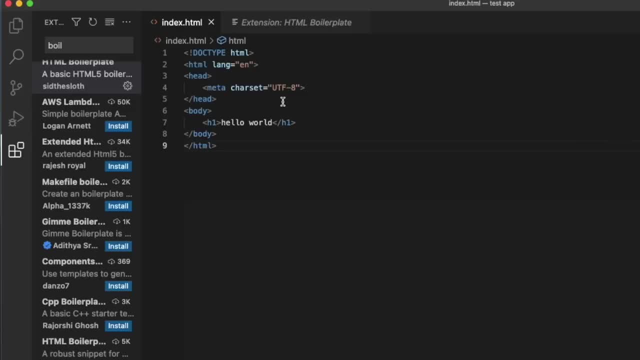 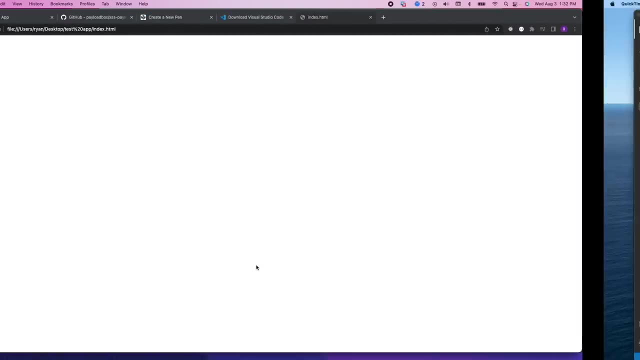 To perform cross site scripting And insert javascript. So with that, I will see you in the next video. Alright, so we have our own Little web application running over here, And now we are going to Enter a little bit in here. 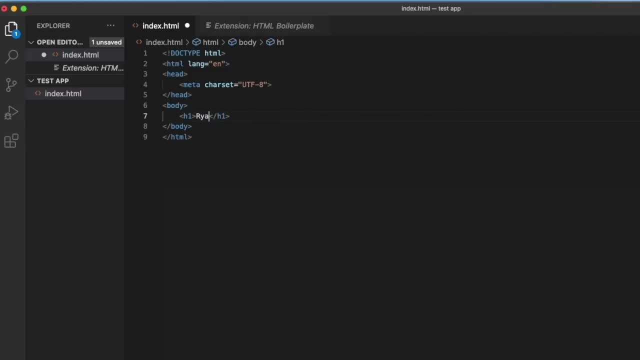 So instead of this h1. We can enter our name And we will make like an entry That we would see into Something kind of like A wikipedia page. So you have a name And then you are going to want a title. 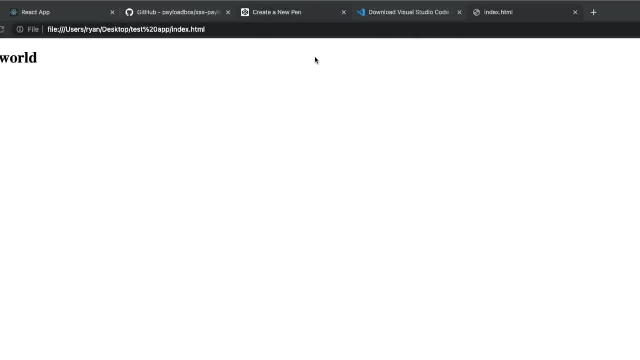 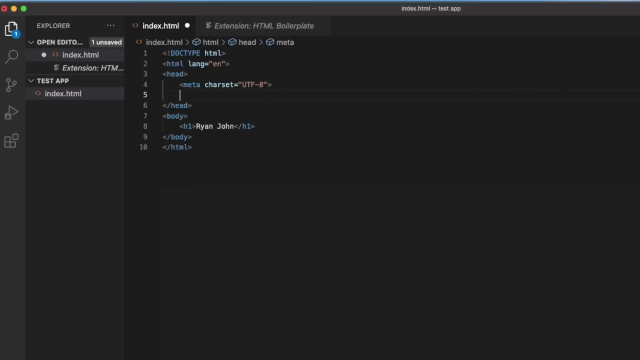 And the title is going to be: What goes on up here, Like create a plan Or a react app. We are going to go ahead and name it And this actually goes inside the head tag So we can open this up. I guess I probably shouldn't open that up. 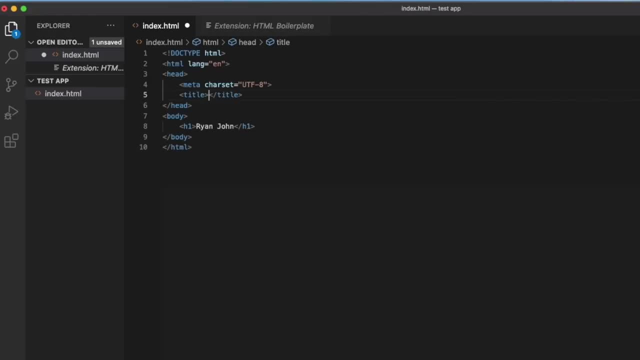 Because if I close it off, I think it will automatically close it for me And we can say: Ryan's site, And then we will save it, And then if you come over here And refresh this, It should refresh for us. 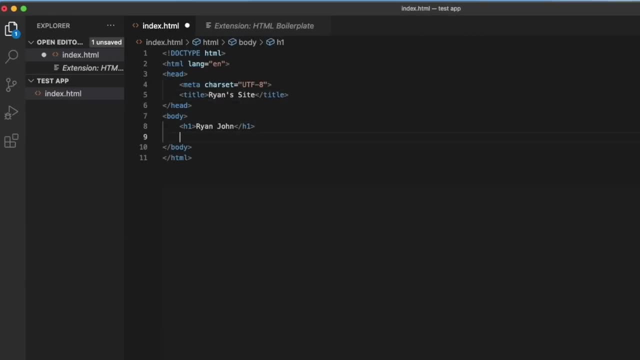 We got your site and your name And you can add in a paragraph tag So we can say: What do we want to say about ourselves? Right here inside this paragraph, We can say: I am learning to Become a Hacker. 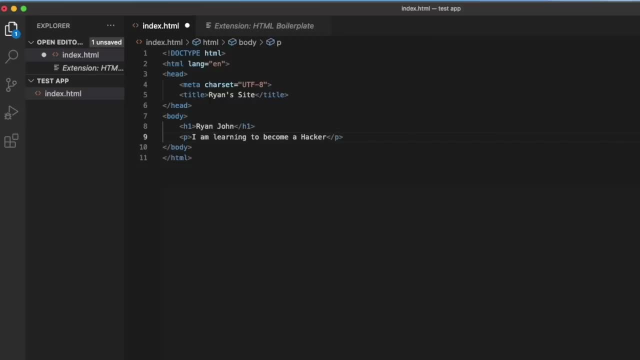 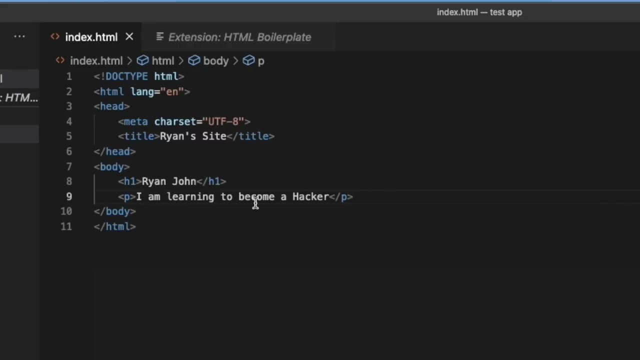 So this is true For all of us here, And maybe we want to make this Hacker right here. We want it to be italicized And bold, So we can come in here And we can say: we want all of this to be emphasized. 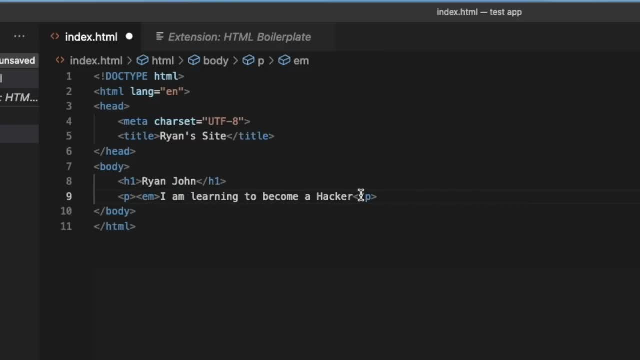 And it closed that off there for us And we will paste it over here And we will save this. So we want the word Hacker to be bold, So we can come in here And say we want this to be strong And we can move this as well. 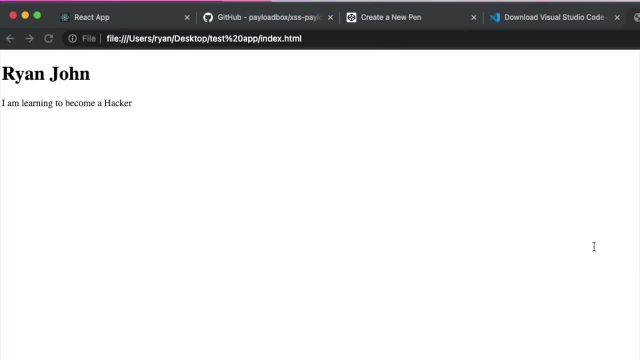 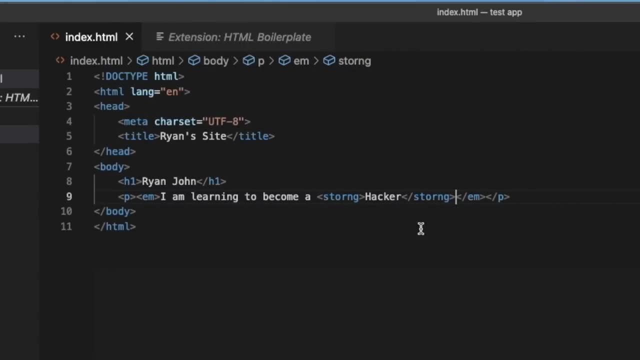 And now, If we save this And refresh our page over here, It has all become italicized. I am not sure why this didn't become Bold for me. I believe that is supposed to be bold, But that is okay if it doesn't work for us. 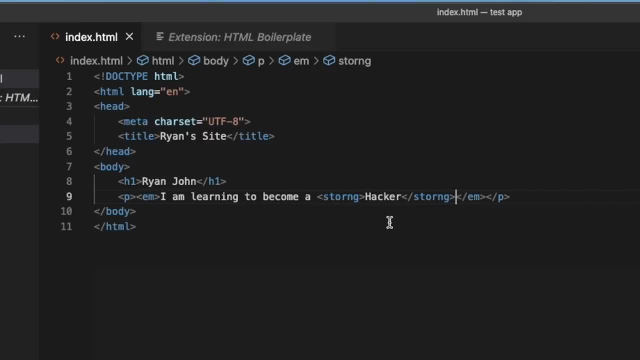 My goal right now is for you to be understanding That there are different tags And we can actually add in a break tag Like: say we want, We decide we want this word hacker right here To be on the next line We can add in a break. 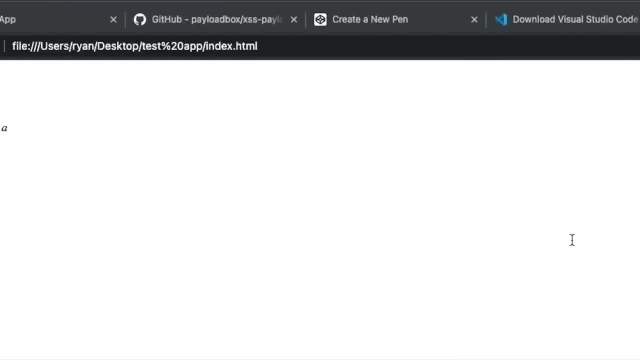 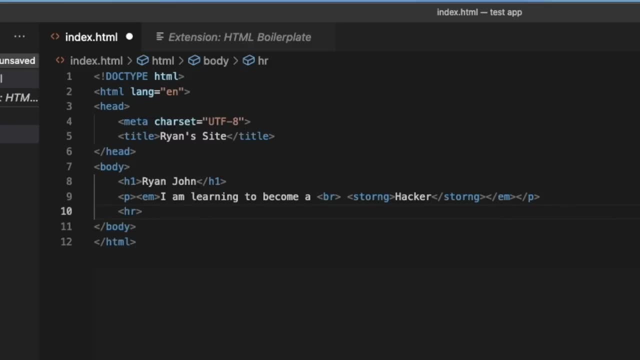 And we can refresh it. And now we have it on the next line And maybe we decide after this That we want a line Underneath everything, And so we will say: we want the HR In here for the line break. And if we refresh this, 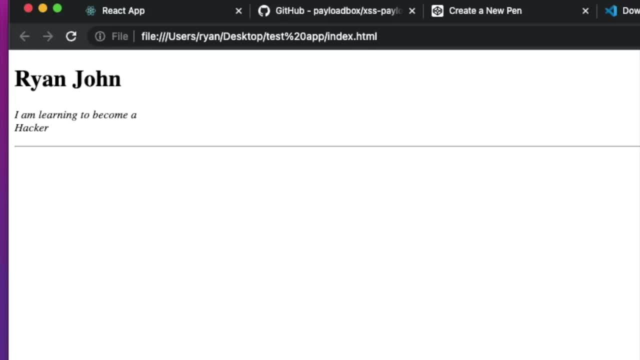 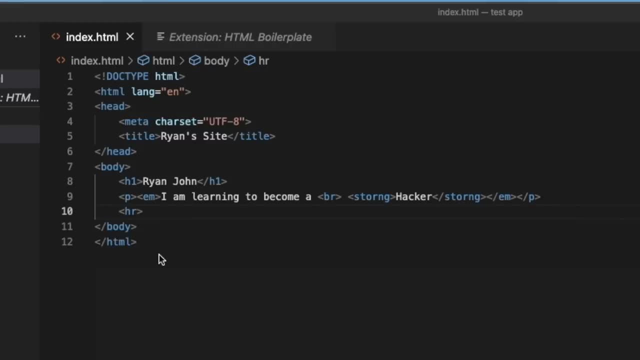 We now have our line And we are starting to get a Entry form here, Kind of like a Wikipedia page. I actually should look at a Wikipedia page So I know what they actually look like. But anyway, my goal for us Is to begin to understand these tags. 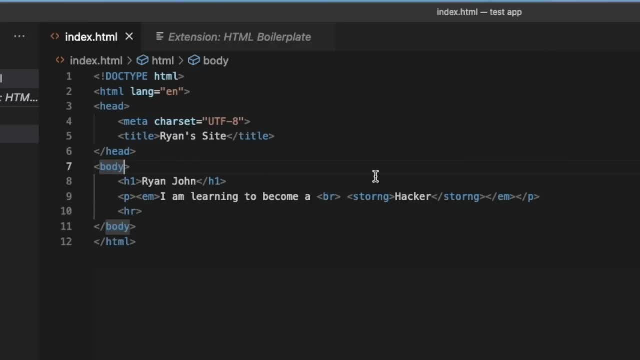 And we are going to look at a few more tags And then we are going to start looking at What goes inside these tags, Because sometimes you will be inside Of something that looks like this And you are going to have to figure out. 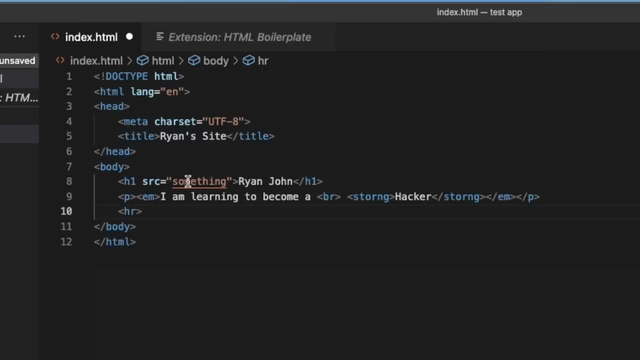 How to break out of this tag Or inside of something Within a tag, And so we are going to learn more about inputs over here In just a little bit. For now, we are going to look at a few more tags That are going to be really common. 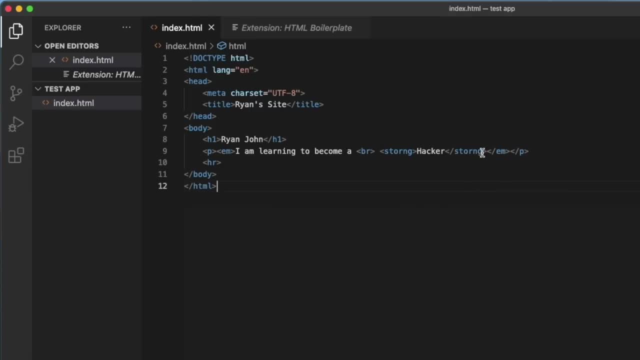 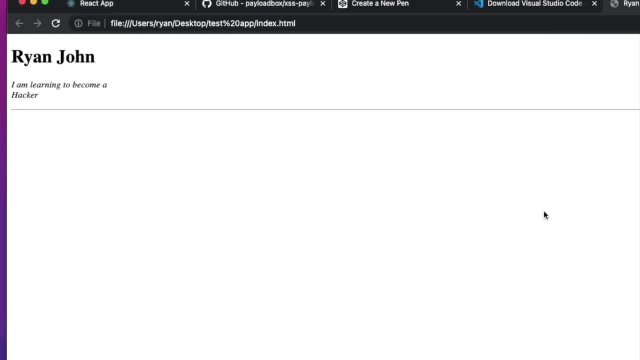 And you are going to see a lot when you look at page source. Now that I am about to close this out, I actually see that I spelled the word Strong wrong here. So if we save that and now we come over here And we refresh our page, 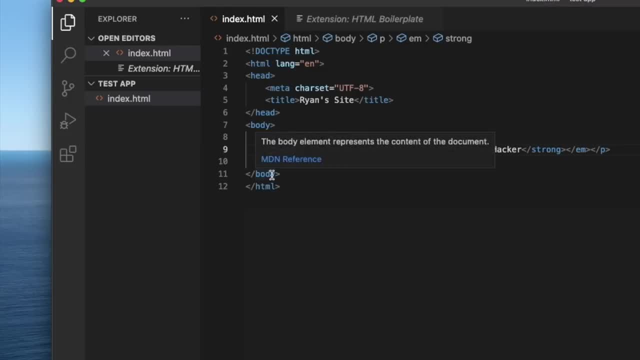 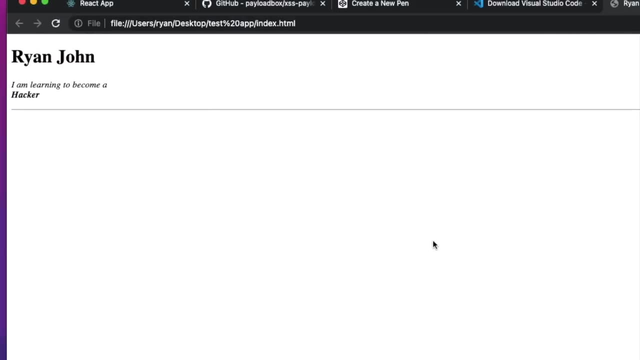 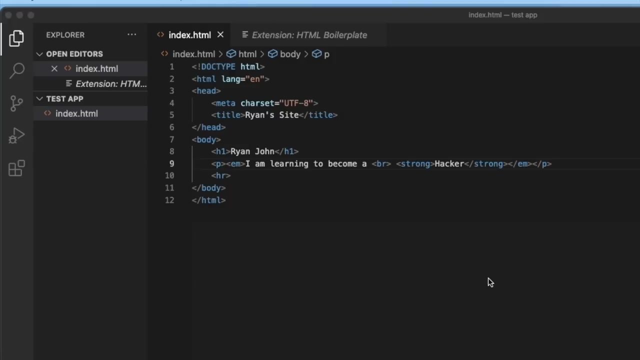 It becomes bold for us there. So inside of our HTML And our tags We need to spell things correctly, Otherwise the interpreter will not know What we are doing or how to translate it Into the webpage. Okay with that, I will see you in the next video. 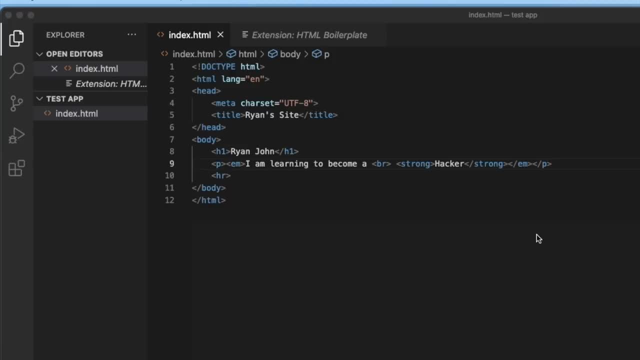 Now I want us to look at lists, And in the next video we are going to look at image tags, Which are going to be really important Because they are the main way to get an XSS to work, And so those will be coming up. 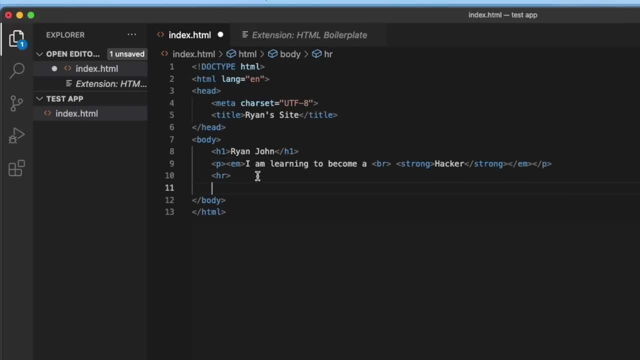 But for now we have our little web app That looks like this And underneath the HR we are going to add in a list. And the way to add in a list Can be done with a UL And you just add in an LI. 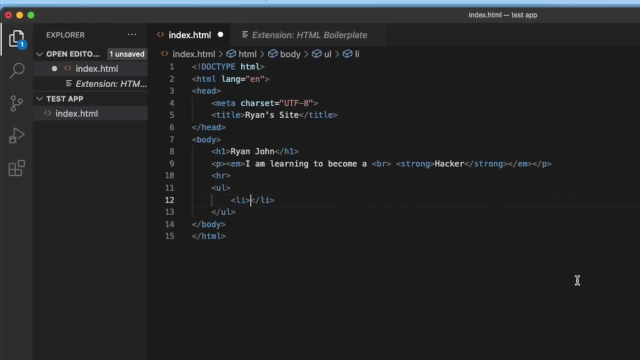 Like this: And now we are going to type into our list And we are going to go ahead and put in I have learned about tags And in our next one Dang it. In the Python text editor You can hit tab. 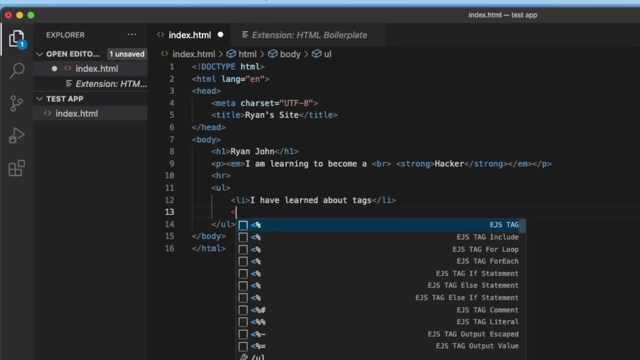 And it will go past your tag for you, And then you can go down to the next line. So we will add another list. Just like this, I have learned about Lists. And then We can say: Lastly, Next I will learn. 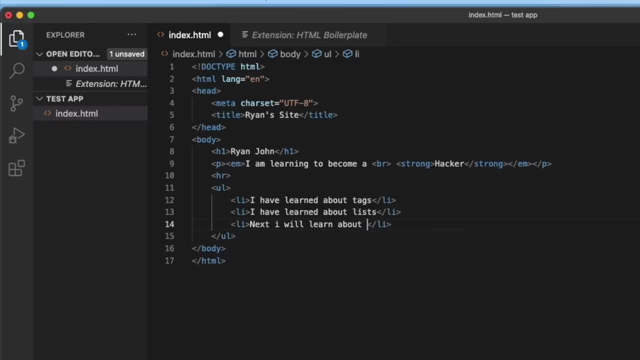 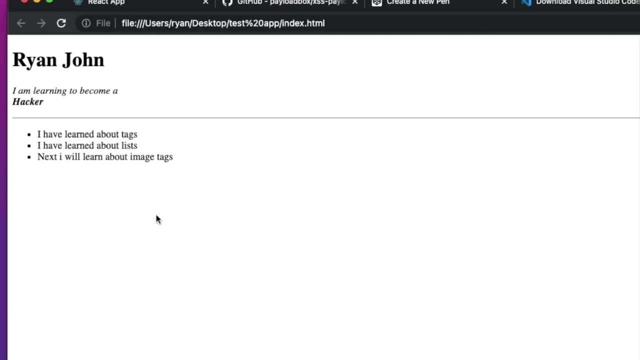 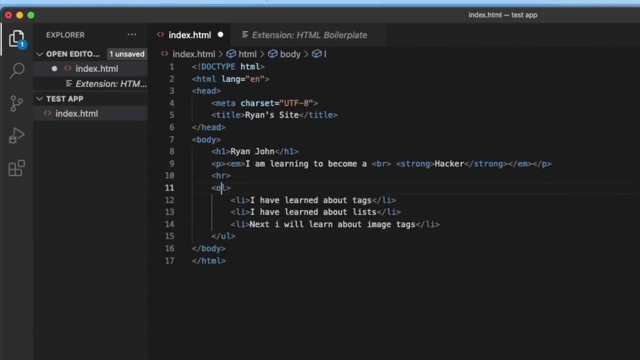 About image, About image Tags. And now, if we save this, Come over to our page and refresh it. We have these bullet points, Just like this, And if we wanted them to be numbers, You just would change this to an OL. 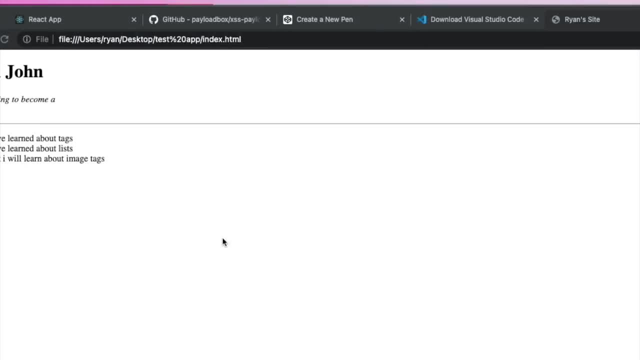 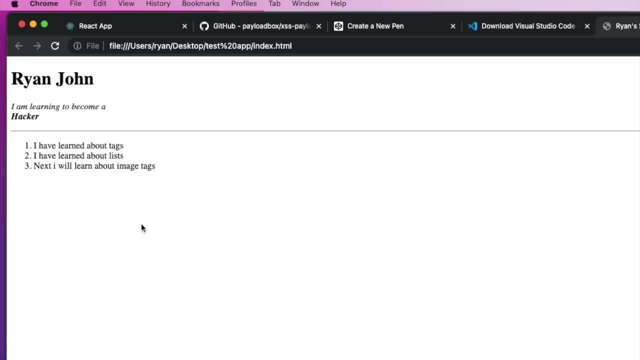 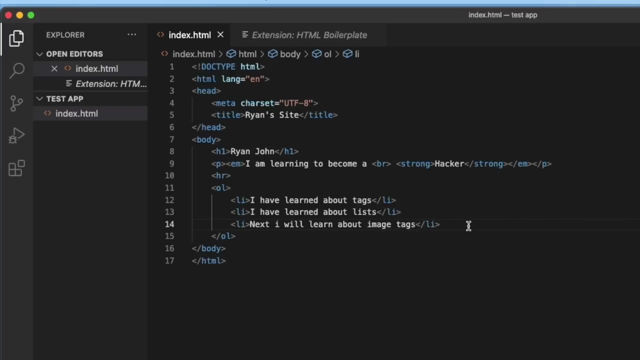 Like so And I forgot to save it And now We can refresh the page And we have one, two, three. So these are lists and tags. You will see these sometimes, You will be able to have inputs And one of the really popular places. 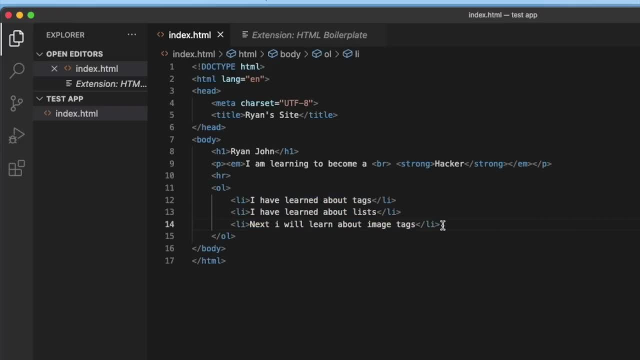 To see. something like this Is inside of some kind of task manager Or something. You will see these in live programs Or maybe in a penetration program Like a penetration test, Where you are testing some kind of application That is supposed to help you schedule. 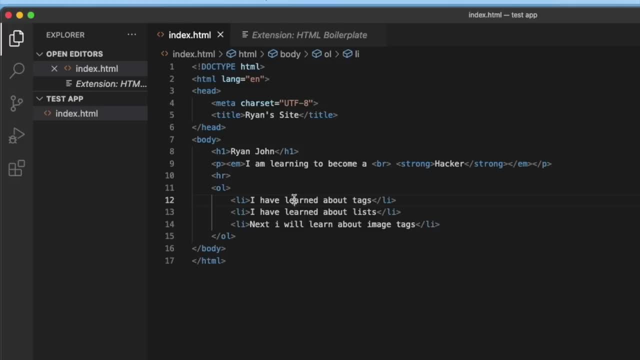 And you will be able to input lists And things like this, And maybe there will be some way for you to inject Either over here or over here. But these are the LI tags And this is the OL. So when you see these in a page source, 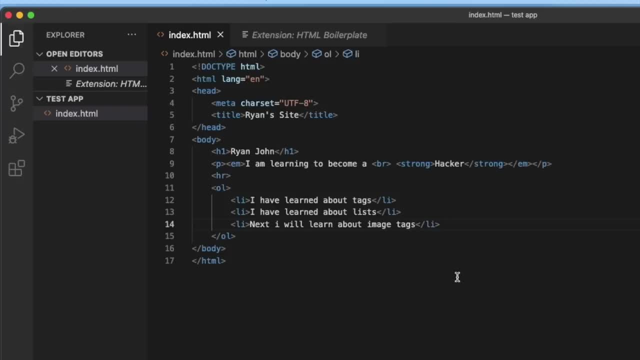 You now know what is going to be going on. Now we are going to move on to the image tag And we are going to pop our first cross site scripting. Only we are going to use an alert, Because we are not going to be injecting it into anything. 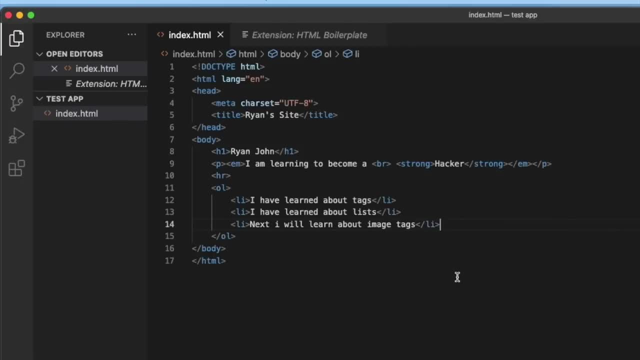 We are going to see how it works Because you are going to see these image cross site scriptings A lot in the future. They are really popular If you can get one to store For the cross site scripting to pop Every single time the page loads. 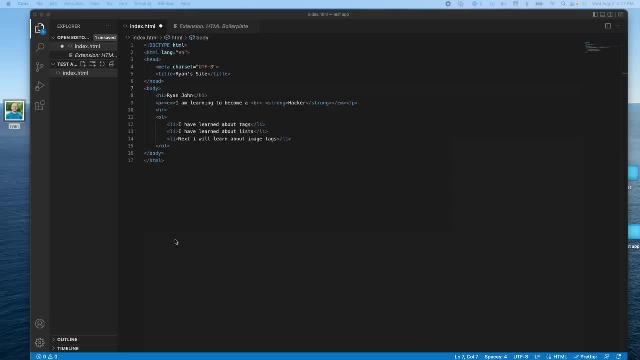 So with that we will move on In the next video. A few more things to go over and learn Before we are ready to start practicing Cross site scripting elsewhere, And the first thing we need to cover Is an image tag. The image tag is going to be one that you are going to see a lot. 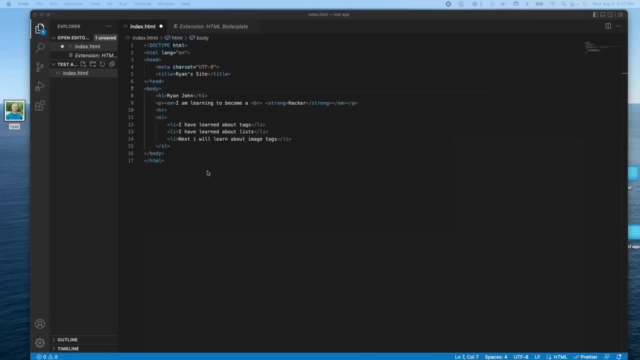 When practicing cross site scripting, Because it will automatically render on the page Whenever it is loaded, Or if there is some kind of submit button For an on error To cause an event. So with that we will just start out With a basic understanding. 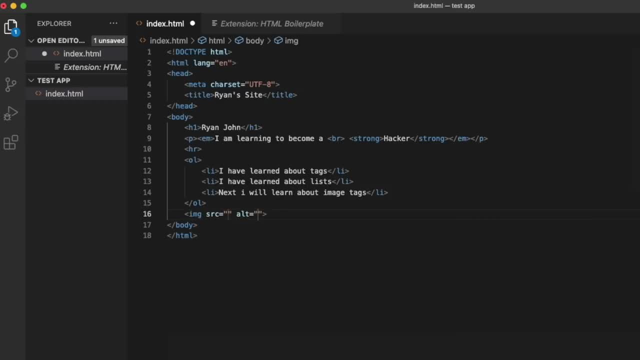 Of inserting an image. So if you just type in img, It should load for you. You have this alt, Which is what is going to load if the source doesn't work. So we can just say, Ryan, Because I am going to use my image. 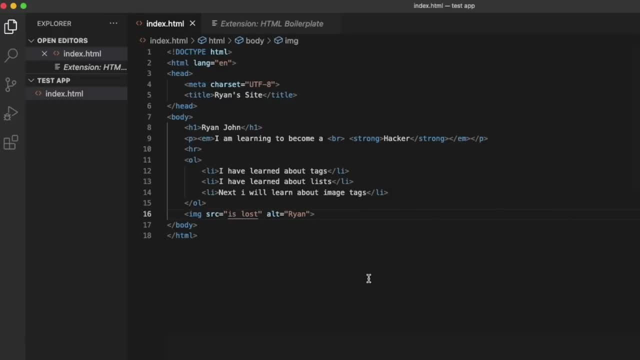 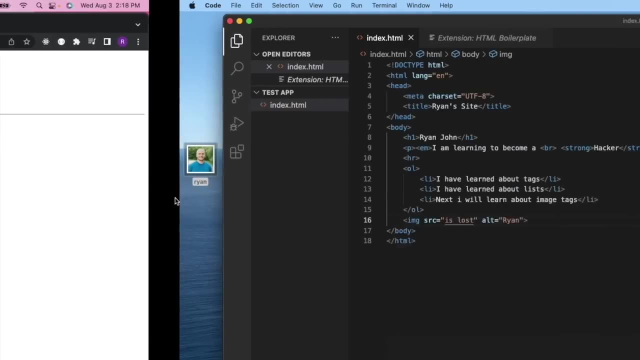 And the source is lost. So obviously there is not going to be any source. We come over here And we refresh the page. We see Ryan, And it tells us a little image is not found. But if we go out to Say Google, 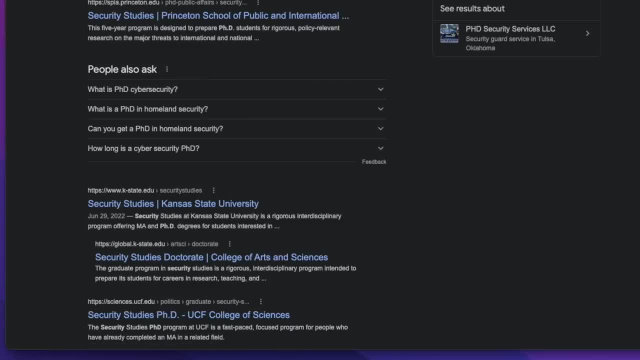 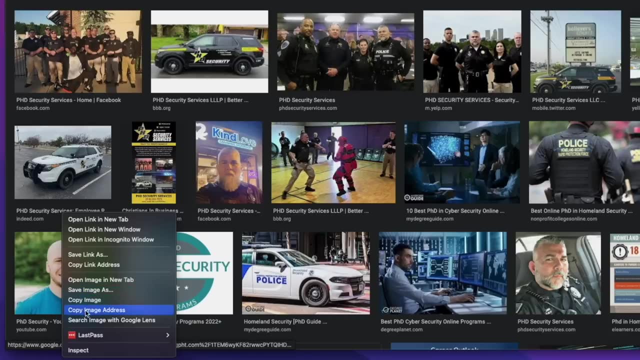 And we type in who am I, And we type in PhD security, And then we go to images. Here I am right here And we can copy the image address Right here. Make sure I am trying to read those, That is right. 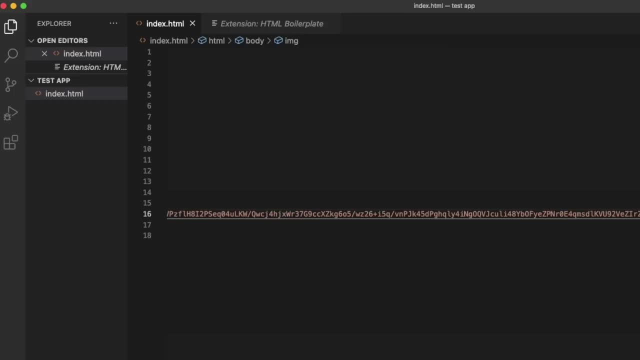 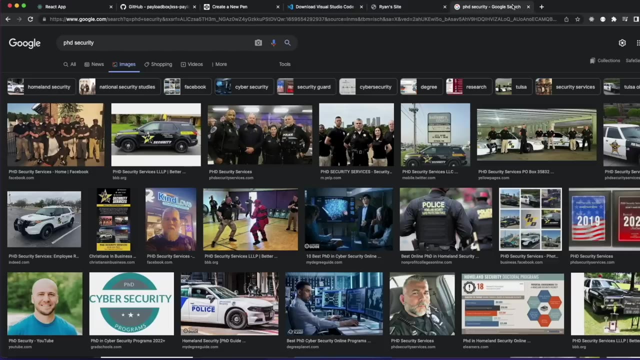 And if we paste this in here And then we save this huge link, When we refresh our page, Our little browser that we have created Right here Is going to go out to this linked address That we have right here on YouTube. 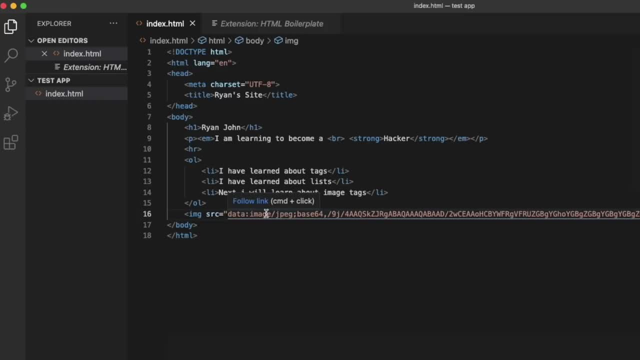 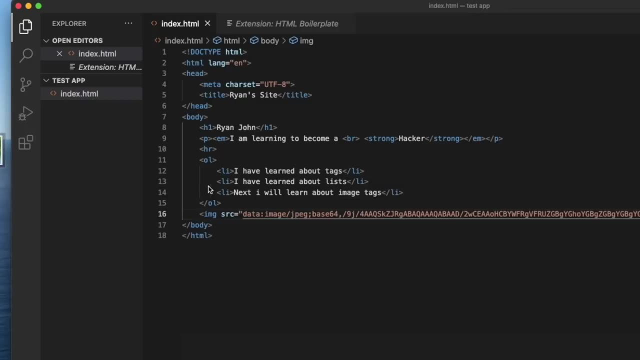 To grab my image And it is going to ping it And make sure that we have permission to load this image Right here. So if we save this and refresh, You can see my image has popped up Right there. That is where this is at. 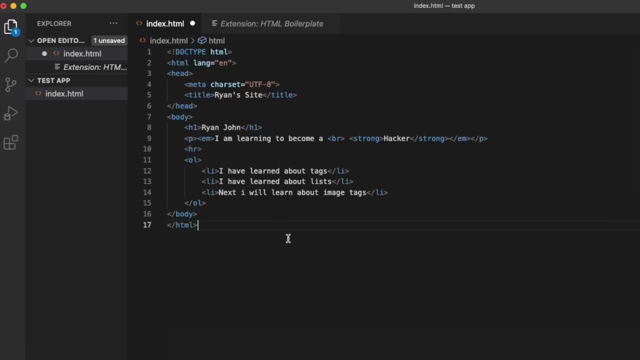 So I am going to delete this, And that is one way to grab an image, And you will probably see that in the future And you will definitely see when images are not loaded. That is usually what is happening Now. I already got the photo over here. 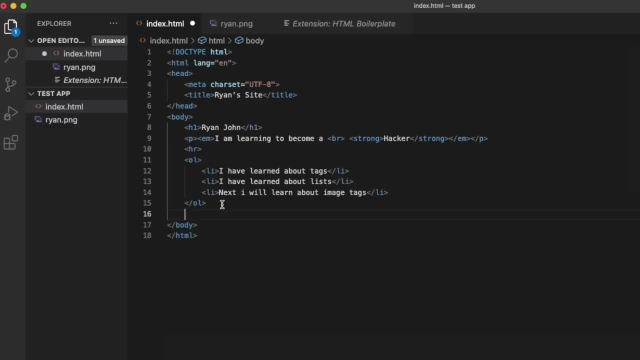 Same photo. You will see this as well. This is the most common way to load an image And it is also the most reliable way. I actually want to put it underneath my name, Because it will look better in our little wiki page right here. 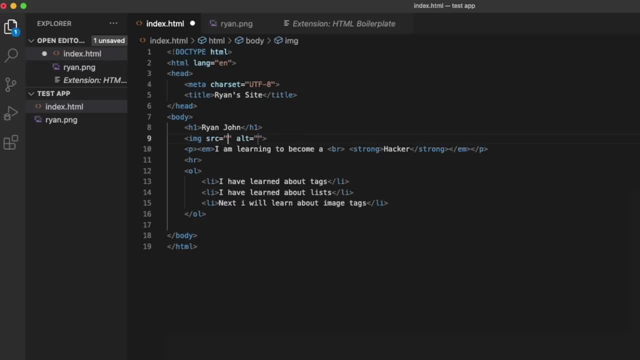 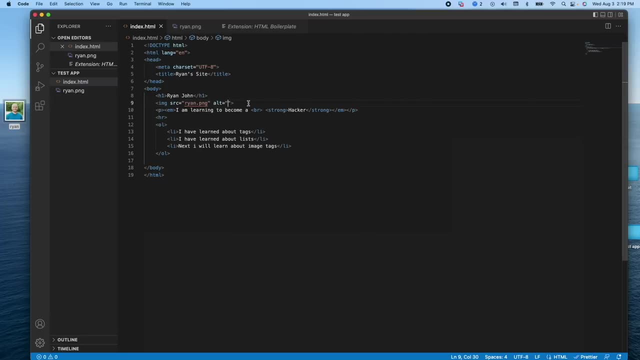 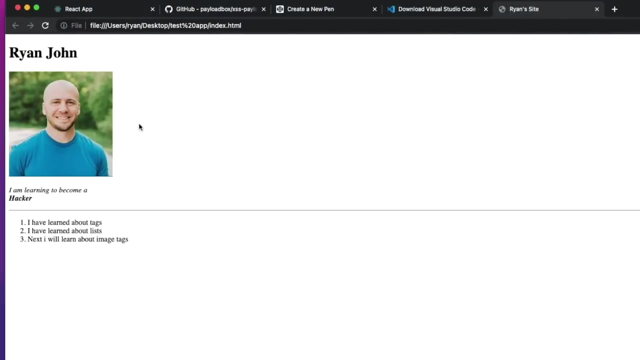 So if we do our same thing And we say image Which is just ryanpng, Because it is already loaded right here For us, And we save it, We can put in the alt, We will just say my name And we save it and we refresh it. 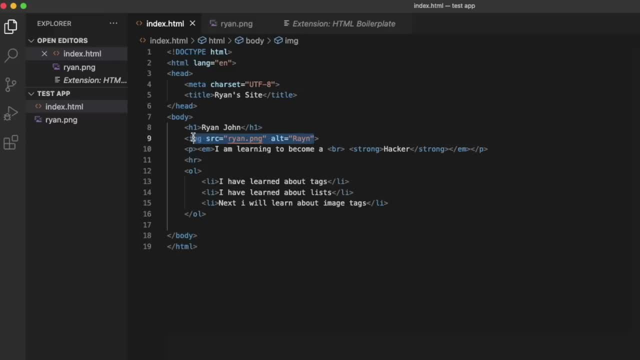 You see it moves up here And that is because it is grabbing the link right here Now. I think the most popular way to perform a cross site scripting, Especially in CTFs That don't have any kind of black listing, Is going to look just like this. 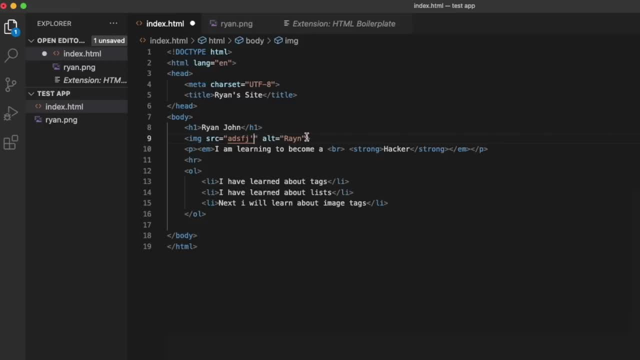 Source. You just put some mumbo jumbo in there And then an alt Doesn't really matter. What you are going to see is an on error, And then it is going to do something, And usually the do something Is going to be alert. 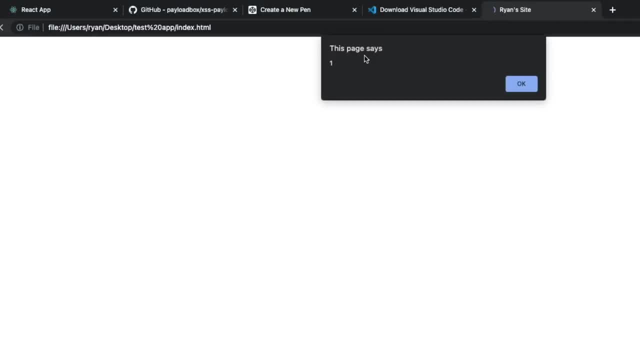 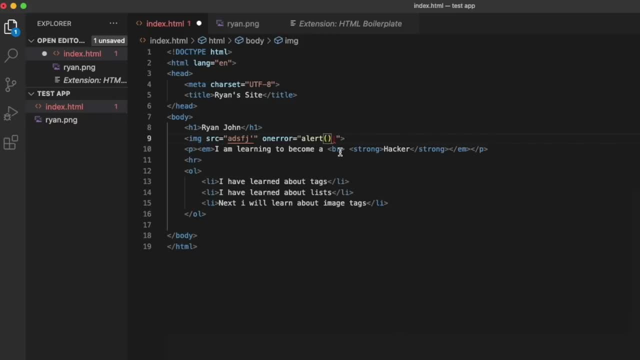 And one And then save this. Refresh our page And you see the cross site scripting pops Right there for us And you will see something like: Sometimes people will put in a one, Sometimes people will put in XSS. We got too many closing brackets. 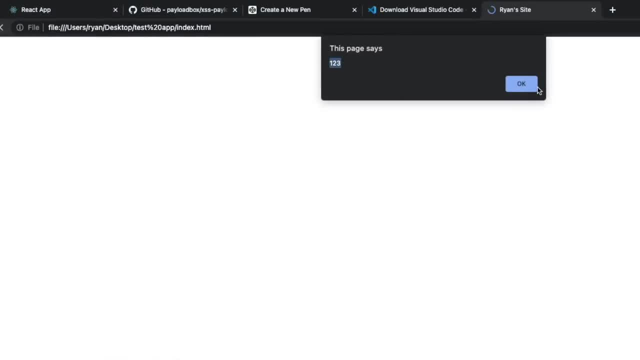 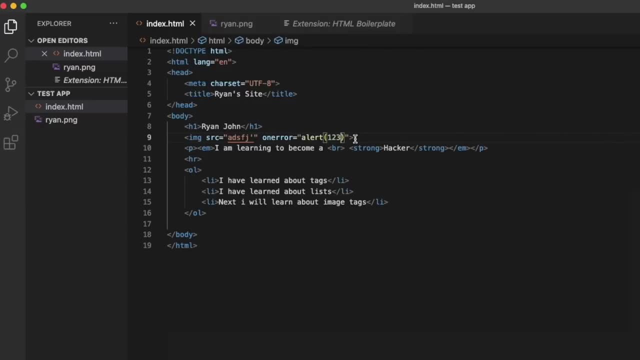 And on our page over here Refresh, we see this page says 123.. And that is going to be Probably the most common cross site scripting That you are going to see in beginner CTFs And the reason You are going to see it done like that. 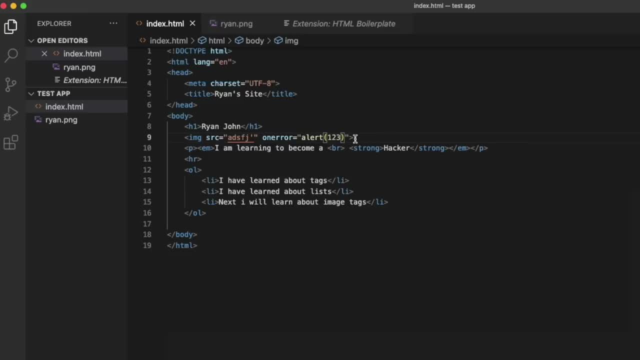 In the beginning Is because this is really easy And your input isn't being stored anywhere. We are going to get a little more complicated As we go along with the cross site scripting. This is how you are going to see images loaded in HTML. 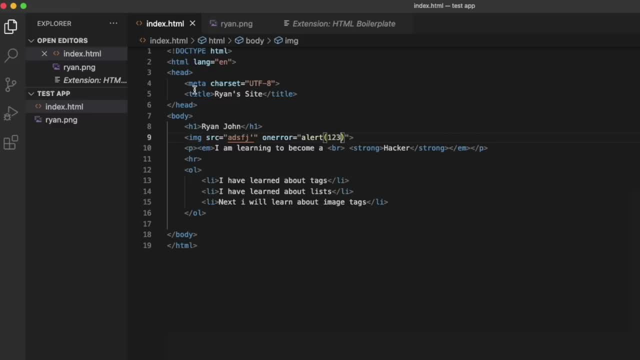 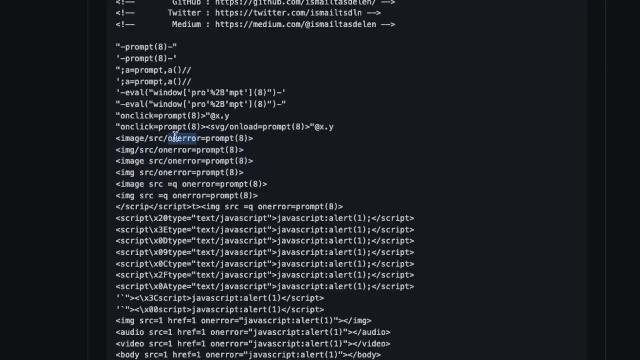 And this is how you are going to see The cross site scripting is performed. You are going to see this image payload All over the place. So if we come back to our payloads, Look, we have image, image, image, And you always see this on error. 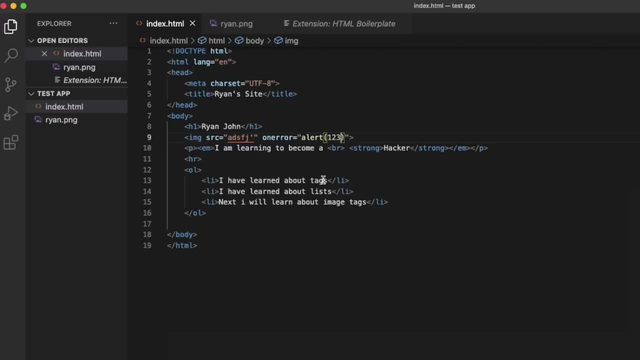 And here is an on click And you are just going to see a lot of these image tags. Here is another image tag, And so you are going to want to be familiar with Understanding the image tag And then how to perform the cross site scripting with it. 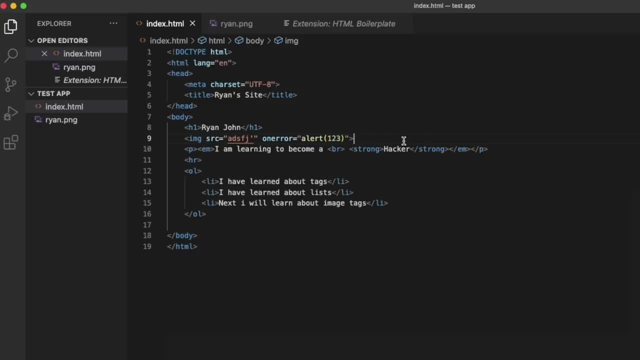 As we go along, Things are going to get more interesting And a lot more fun to try and break out of The HTML tags And bypass the bad characters. So with that We are going to look at hrefs and hyperlinks. 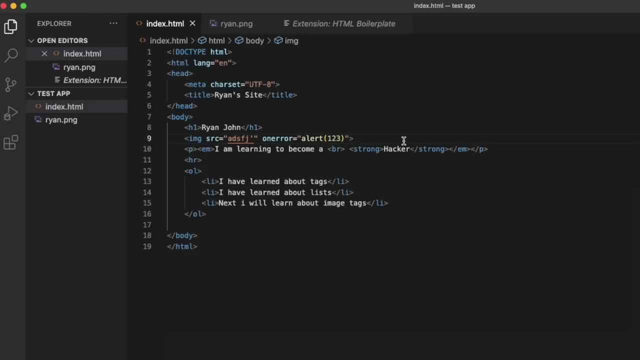 In the next section, And then we are going to start looking at Getting cross site scripting to work for us And then after that We are going to start looking at cross site scripting And breaking out of HTML tags. So with that, 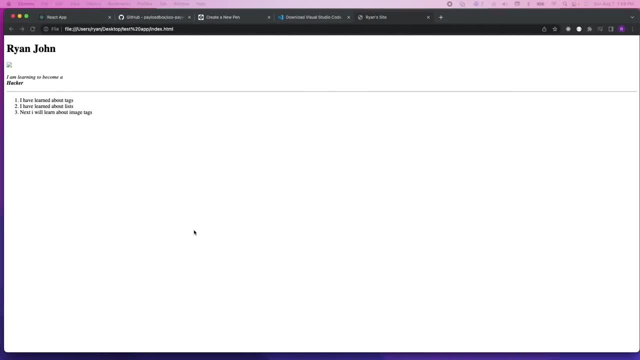 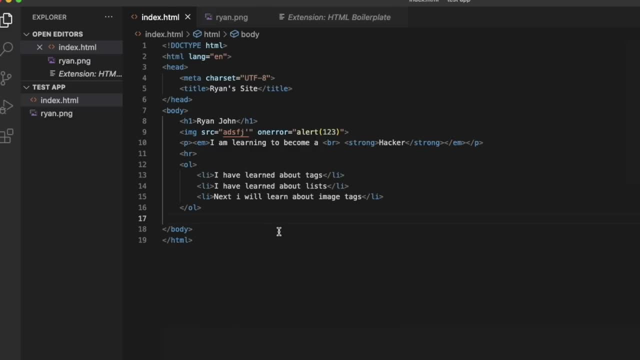 I will see you in the next video. Okay, so we are here with our code For our very simple website That we have going on right here, Cross site, with nothing really going on, And I want to move on into hrefs And we are going to build this inside of an anchor tag. 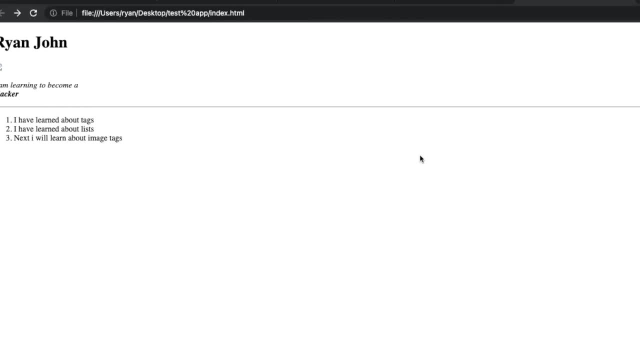 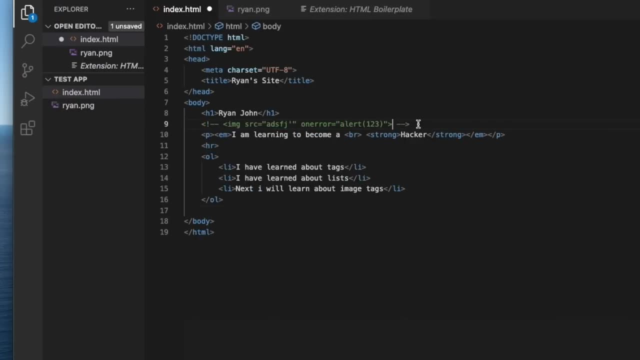 So right now, If we refresh this page right here, We are going to get our XSS, So we are going to go ahead and comment this out. I think you can just click at the end of the line. Yes, you can. You can click at the end of the line. 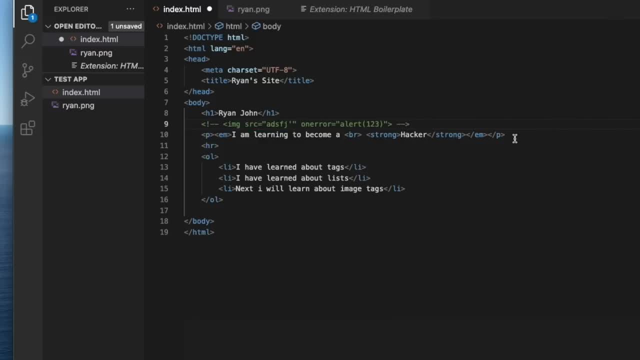 And on a Mac you hit command forward, slash Or command question mark And it comments out the line there for us And below this we are going to add in our anchor tag, Which is just going to make us have A clickable link. 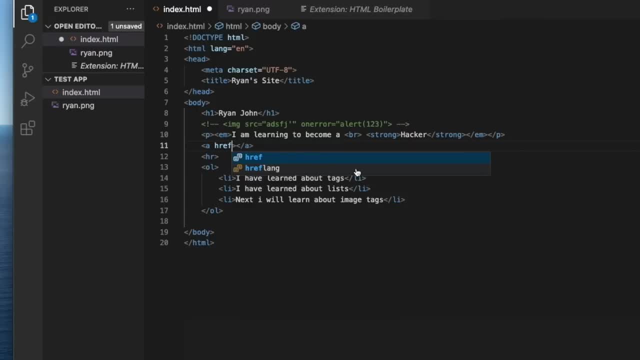 So we are going to go href, Which this is going to be the link That we are actually wanting to add to our website, And we are going to just give something very basic Like googlecom, So we can go https Forward slash. 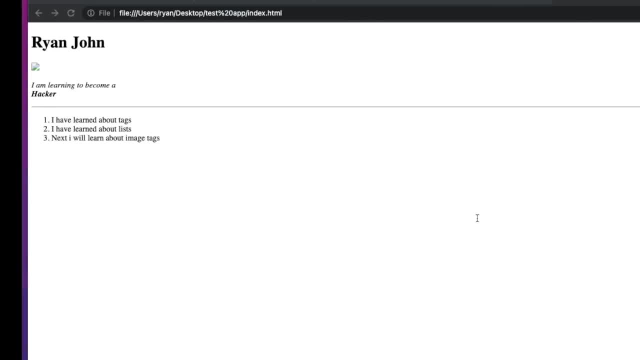 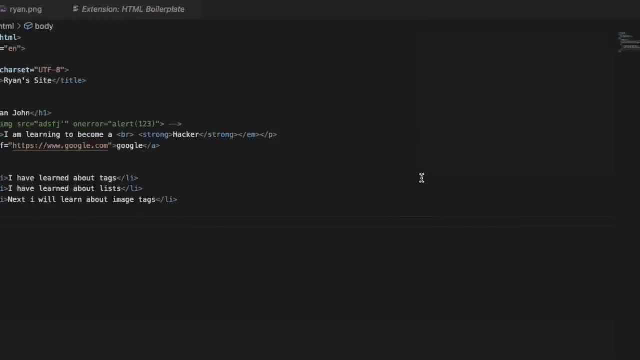 And then we go wwwgooglecom And if we save this And then we come over here and refresh, You will see our link when we add it in over here, Google. I forgot to add that text in And I forgot to save it. 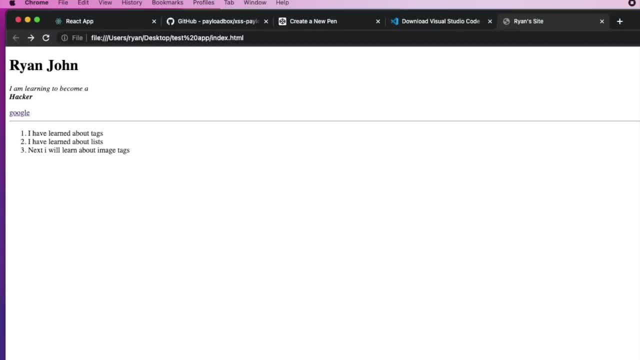 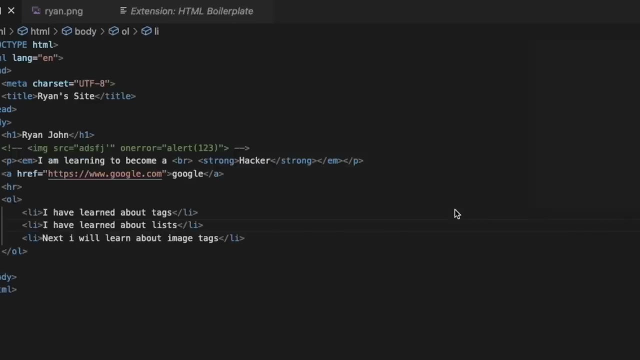 Refresh Our page And now we have this link right here And if we open link in new tab, We are taken to google. So this is really simple And you can actually. I have actually been seeing these Little anchor tags. 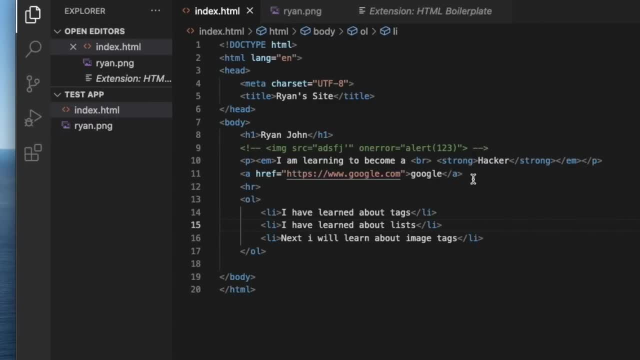 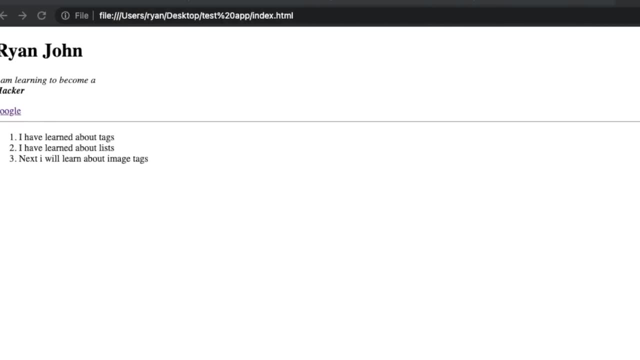 Also inside of the source right here, Become a place for cross site scripting. I am not really sure why Developers have been making it So your user input, Say there is like an input box, Or you can just come up here And you would do something like this. 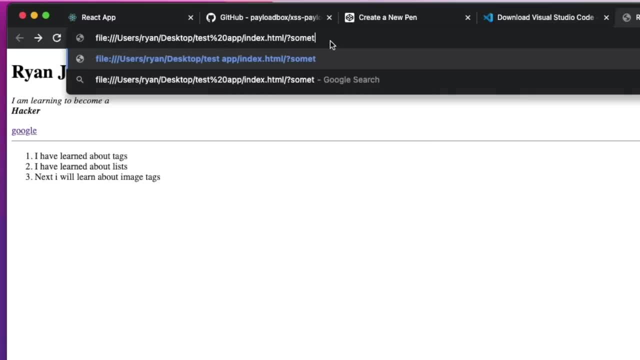 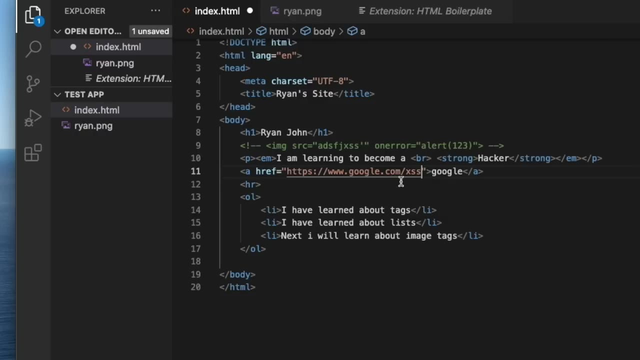 And just add in a parameter Of something Equals And then xss script Right here. I have been seeing at least twice in the last month That right there That xss would get stored either right here Or right here. 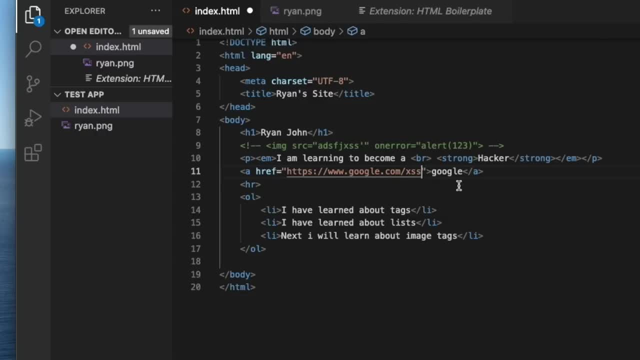 And all we have to do is break out of these little links, Or the source or the href, In order to get our cross site scripting to work. So we will just pretend for now That we build an input, Because that is going to require some javascript. 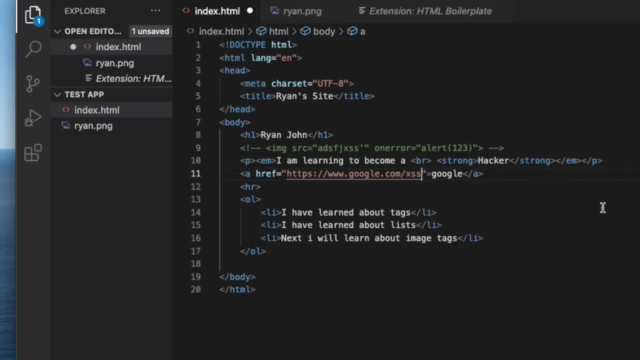 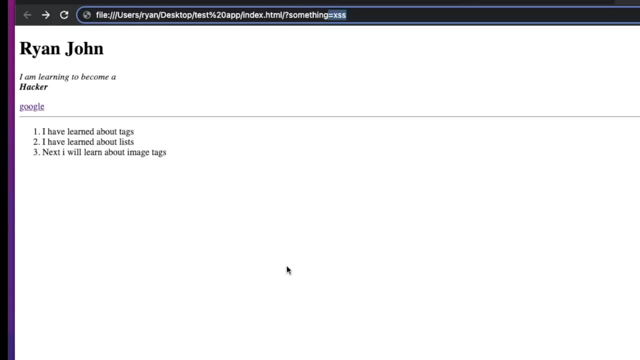 In order to get it to be saved inside of this link. But one of the things you should always do And always check for Is if you can add in a parameter right here like this: Or you are able to just insert something Into like a text field and hit search. 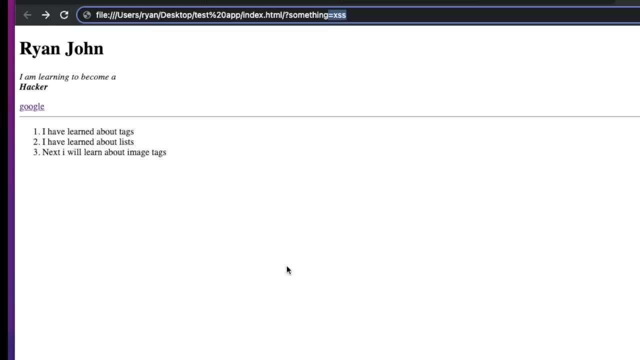 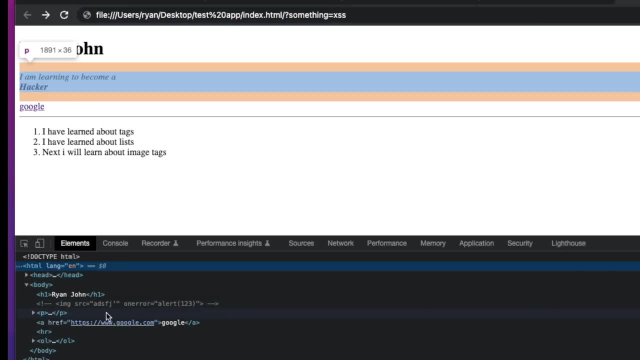 Like on a search bar On amazon or google, And then you inspect the Text like this: You should always check to see if your Information is getting stored in here, Like this cross site scripting And look for the cross site scripting. 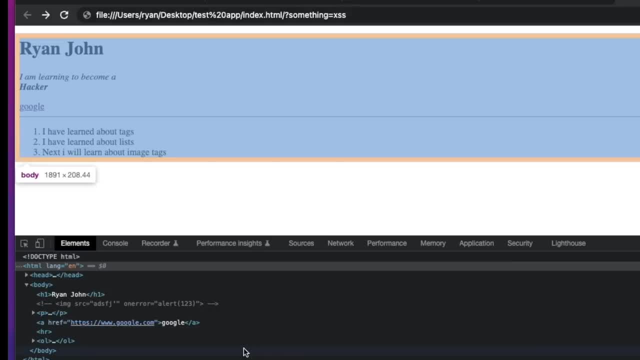 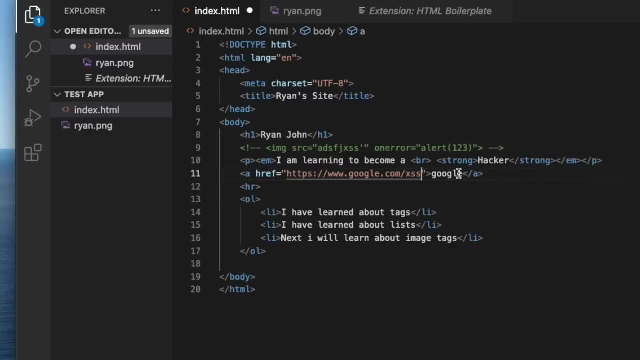 Or your keyword That you are able to Put into the input. So I want to just show you like how to break out of this For cross site scripting. Let's say we are able to add a parameter And it adds it into this googlecom. 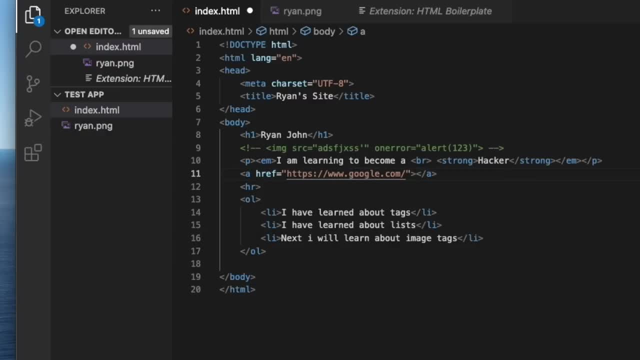 The most recent one that I saw. It was actually appending what I put in As a parameter down inside Of a page one. It was like something like this: Page one equals. And this was at the foot Of the Application. 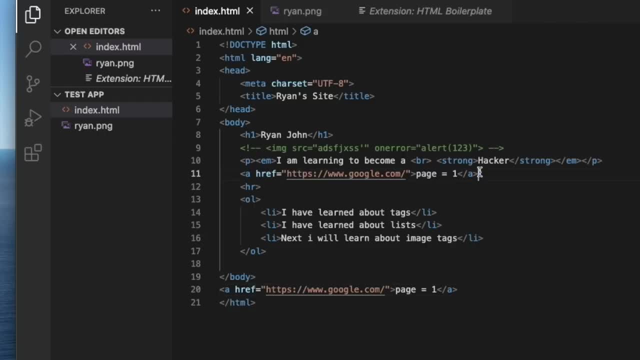 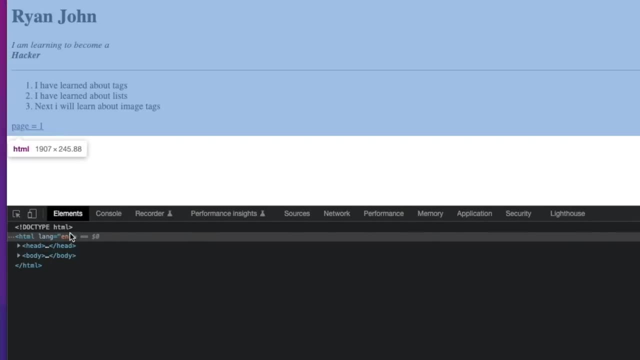 So it would have looked something like this right here, And if we save this, Comment that out And then we come back over here and we refresh this, It was down here at the bottom And it was like page one And within this page one. 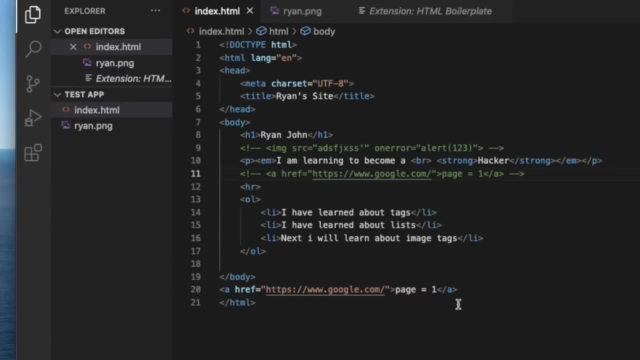 It had my little cross site scripting payload That I was adding in right here, And so we will pretend that is. what we have going on Is that we are able to add in a parameter And it is getting stored right here, So we are going to have this. 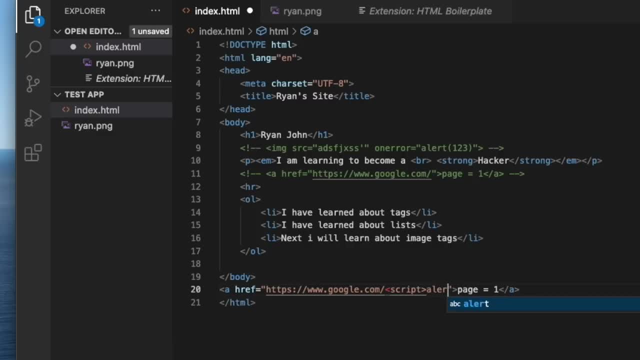 In order to get our cross site scripting to work, Because if you just come in here And type in script alert And then you close this out, Nothing is going to happen. And I will show you: We might even get an error. 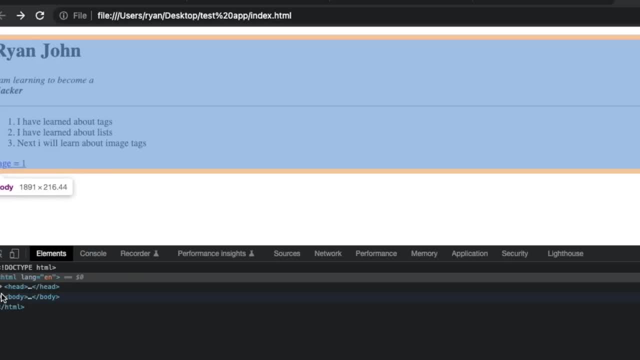 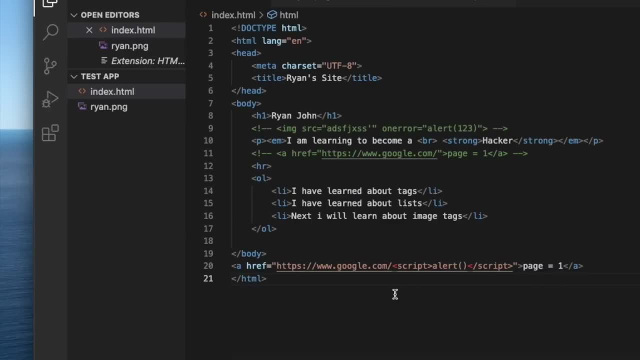 We come over here, We refresh it And nothing happens. You click on it and nothing happens. We are not able to, Because what is going on right now, And this is all going to be trial and error, And sometimes, when I come across, 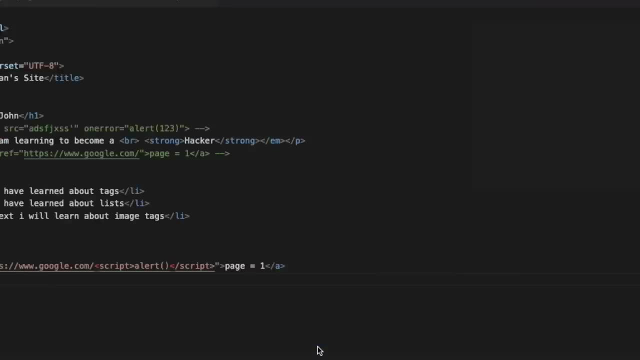 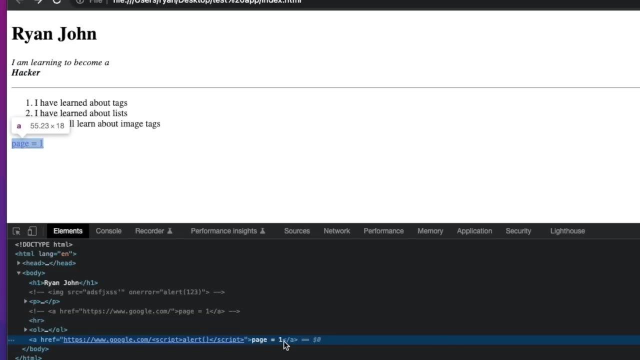 Something like this in the wild. I will just copy this And I will paste it into a text editor Just like this, Because the colors are going to change When the payload is ready to work, So you should be aware of copying this. 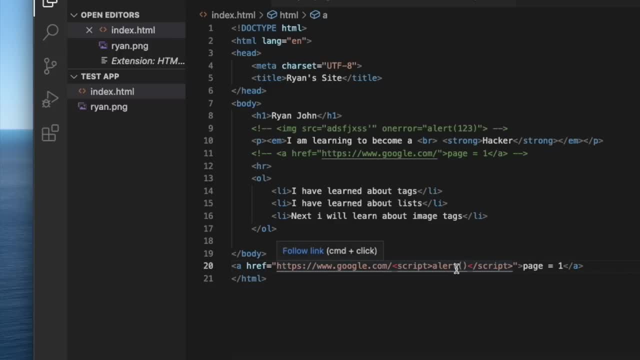 And bring it into a code sandbox Or some kind of text editor To play around with it. But I think this one is going to be pretty easy to break out of. You just add in some quotations right here In order to close this out. 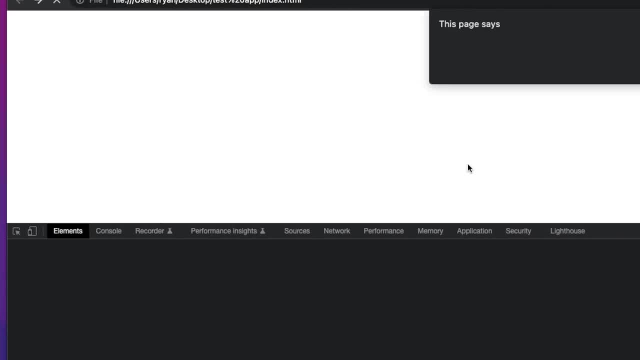 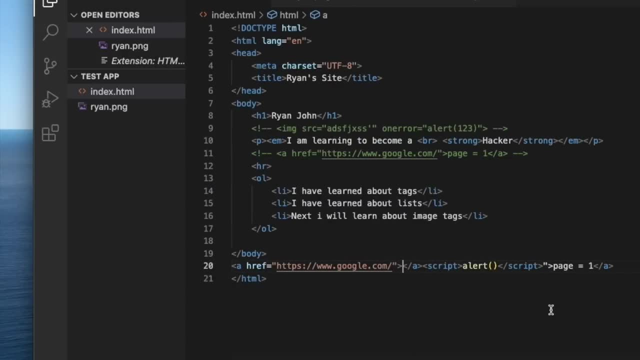 And you can see the closing tag. And now, if we save this And we come over here And we refresh the page, We get our cross-site scripting to work And they really are this easy to find in the wild, Especially if you are off the beaten path. 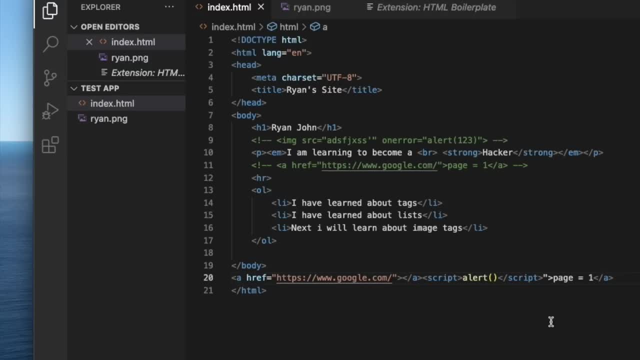 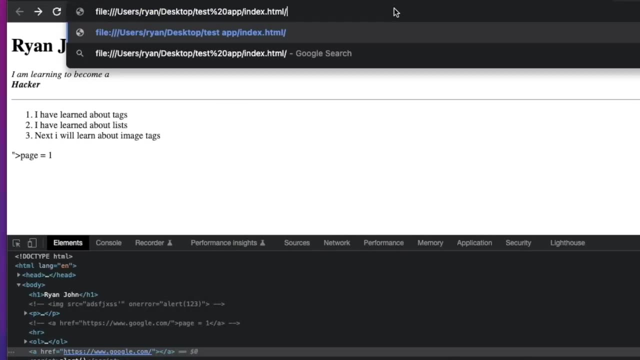 Where payloads have not been tested And people haven't been looking for cross-site scriptings like this. The one that I found really was this simple: All I had to do was come up here Into the URL And I just added in a random parameter. 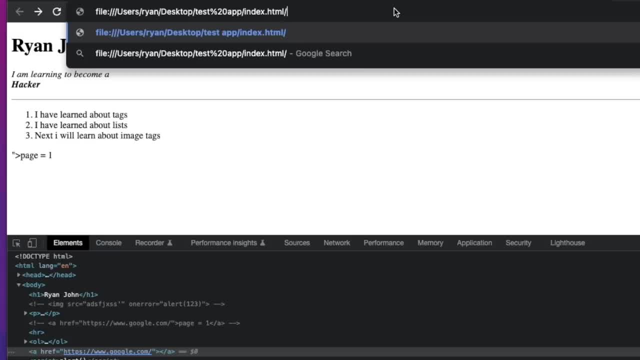 So you can just add in For this, For the sake of example, A CB Like a cache buster, Even though we are not doing web cache poisoning, And then you can just add in a parameter Of payload, And then we would say equals. 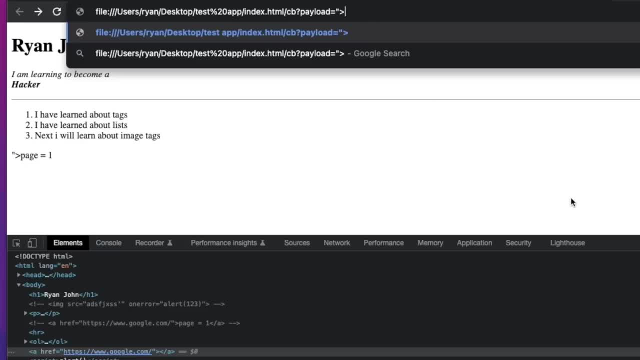 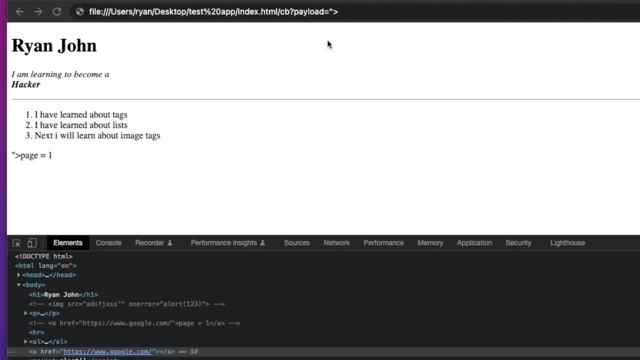 And the way you would get this to store Is you would type in our script That we put in just like this In order to close off this anchor tag, And then we just add in our payload, And so you would go like this: 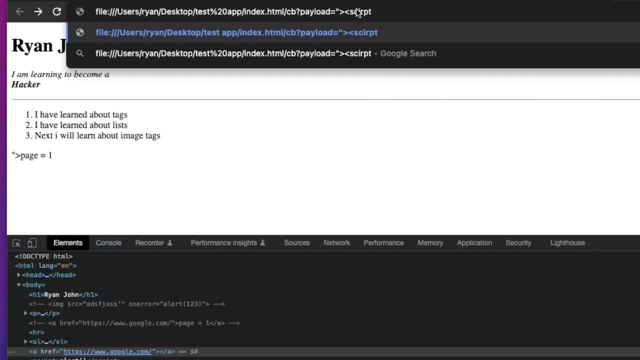 Script, Script, Spell it right, Script, And then we would have alert, And then we would close off our Payload, Just like this. And then you submit this. This is how it worked for me, And this right here was getting stored. 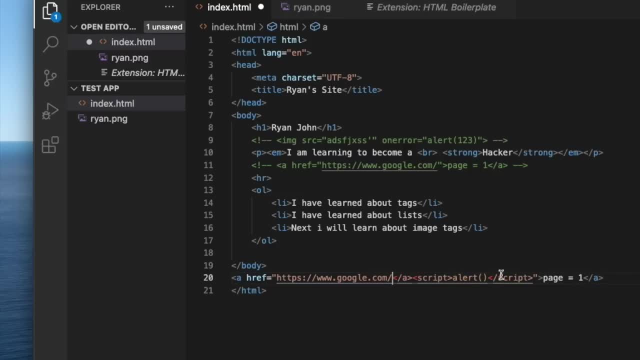 Inside of the href, Just like this. So that is one way to Pull off a cross-site scripting Inside of a Anchor tag, And sometimes you will see these Inside of something like this, Because, if you are familiar with burp, 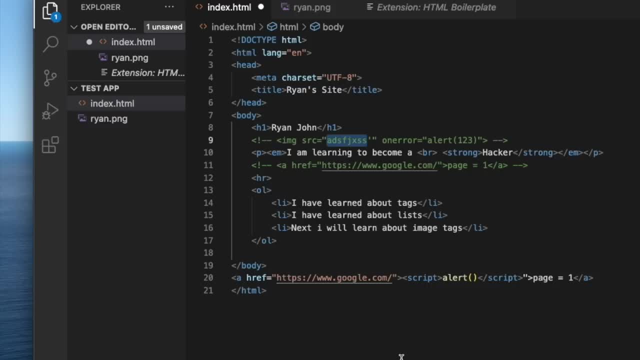 And you see the header tags And it sends a refer header Showing where you came from In order to get to the next page. It will have in the previous website That you have come from And I actually came across a website. 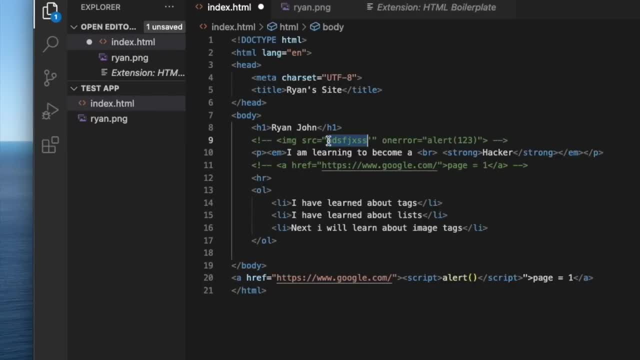 That was storing the previous url Inside the html In a hidden input field, And all I had to do was copy it And then basically do The exact same thing we were doing earlier And just add in our script, Just like this: 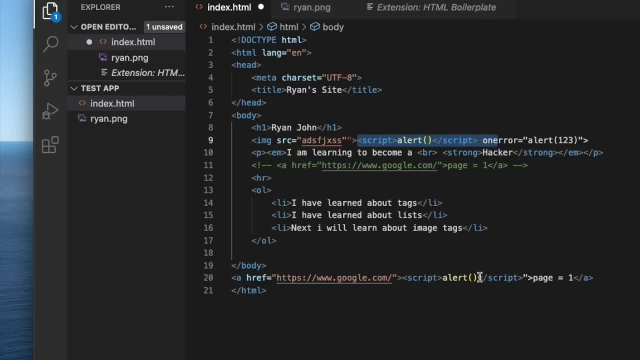 In order to get the alert to work. So you can look out for these In a lot of different places, Such as an href Or inside of a source, And just be aware that Where you put things within the input May get stored randomly within the html. 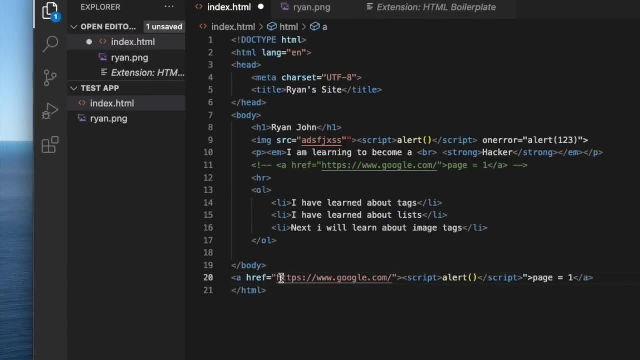 And then all you have to do Is be familiar with html, And then closing off the quotes, And then closing off the tag, And then pulling off the cross site scripting. So with that we're going to move on And look at some more html. 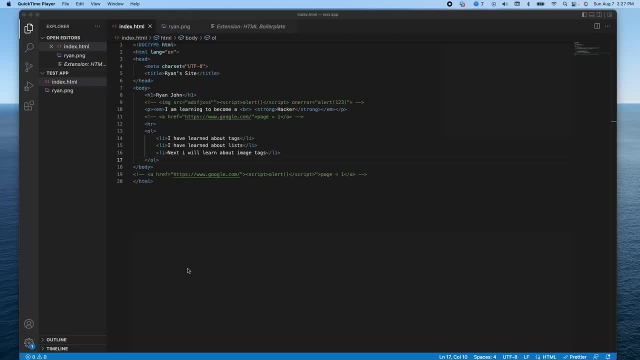 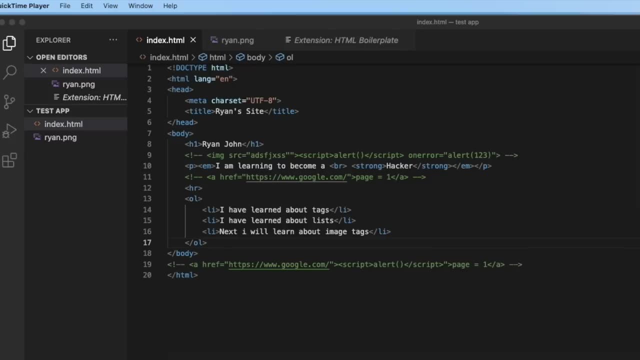 In the next video. Alright, so there's two things I really want to show you Before we move on from html And we take just a second to look at css, And then we move into javascript, And that is hidden information As well as forms. 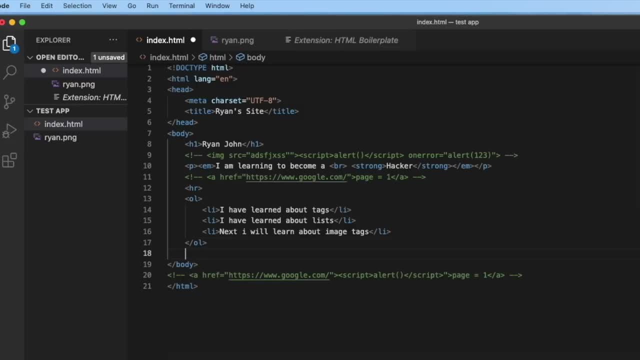 And so we'll just start out with forms. So a form is pretty much Just what it sounds like. It is one of those things That usually includes inputs and information That you're going to be taking in From the user. So usually, within a form, you'll have a class. 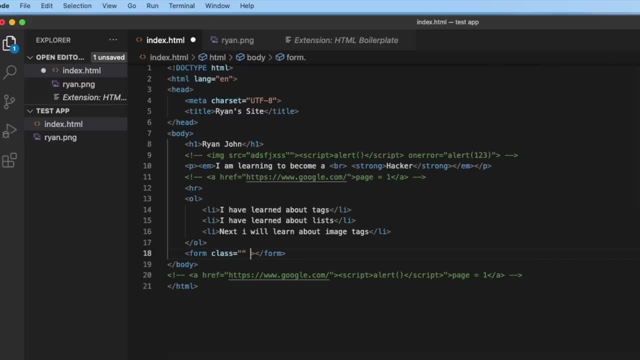 Which we're actually not going to mess with Until we get to the css. And then you'll have some kind of action, Typically, and this is going to take you somewhere, And we're not going to mess with that Really either. And then we're going to also see a method. 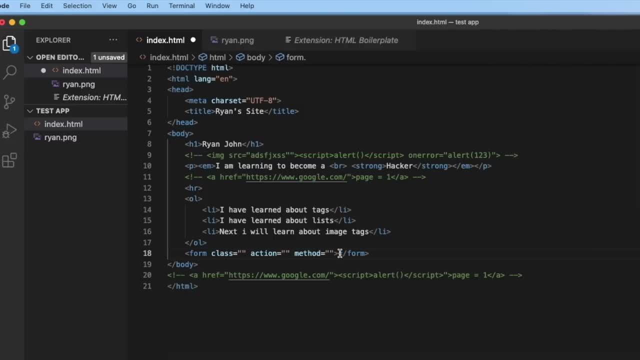 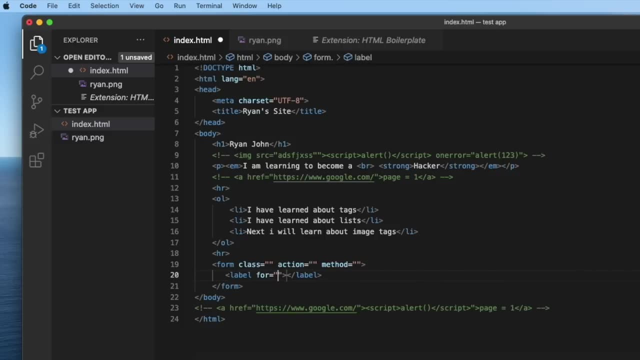 Which we're not going to mess with as well. We're going to be sending the information to the server, Okay, and now we're going to want to add in A label, Just like this, And inside of this label, We're going to delete that. 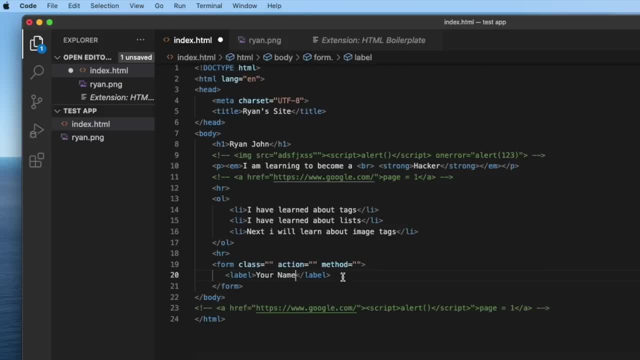 And we're just going to say your name. So we have this, your name, right here. So if we save it And we come over to our page and refresh, You will see it pop up on our page. And I added in this little hr. 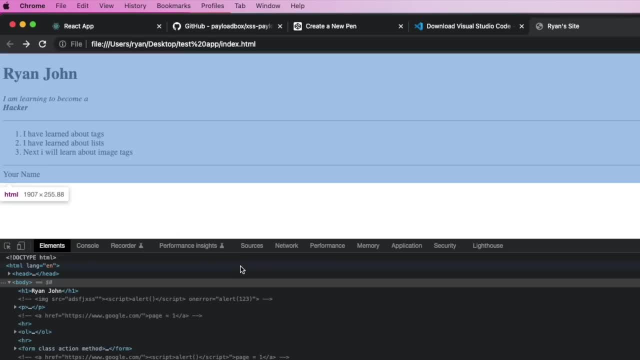 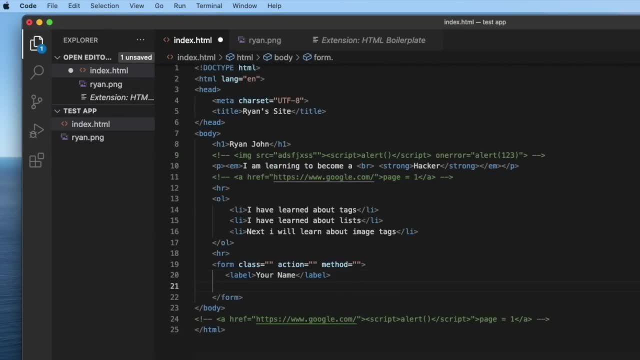 So you can see the division of the information And right here is the your name. So We have our label And now we want to take an input. So what we will do is add in an input, So we just say input, just like this. 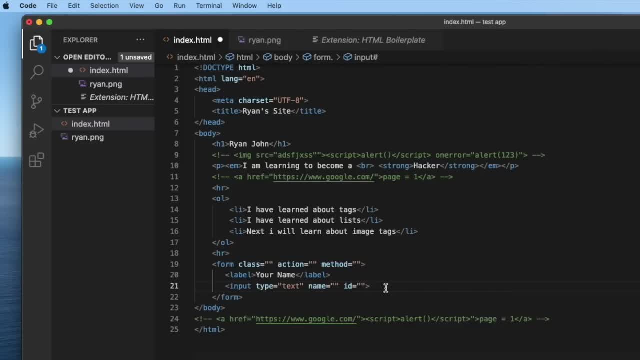 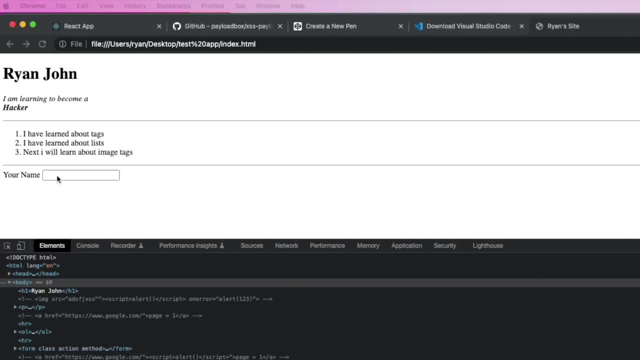 And it's going to be a type text And we're not going to mess with the id or the name At this point. And if we save this, You're going to see just a box appear over here And so it says your name. 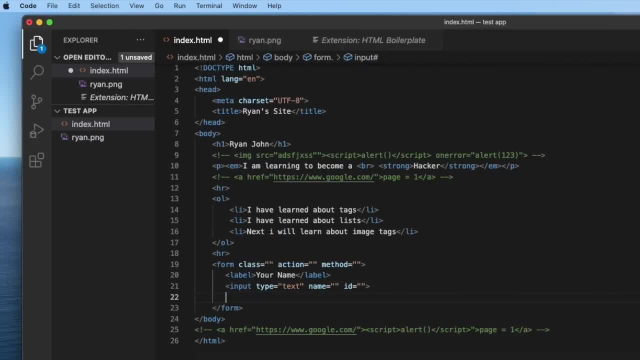 And then we have this text box. We're going to end up adding a button as well. So we will say We want a button And it's just going to say submit And our button at this point is not going to do anything. 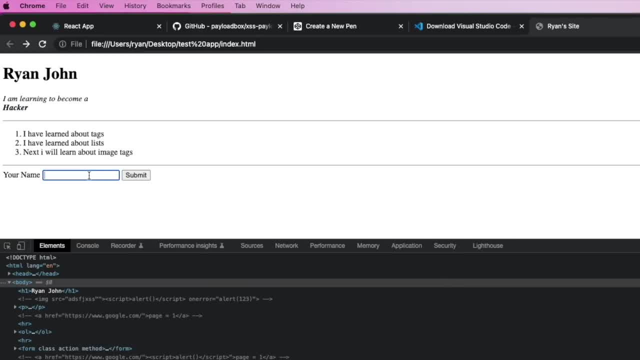 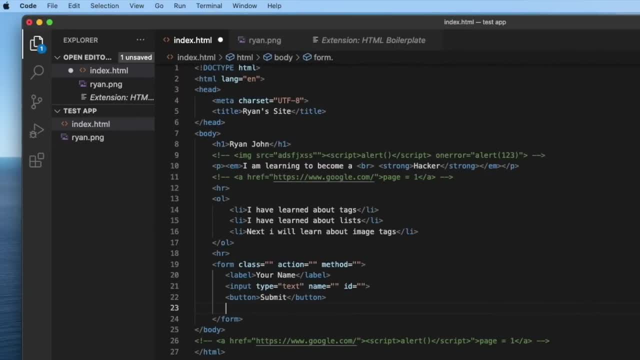 And we can save this And refresh, And now we have your name with this text box And a submit button that does nothing, And then, lastly, You're going to see within these forms Is a password, And you're going to see something like another input. 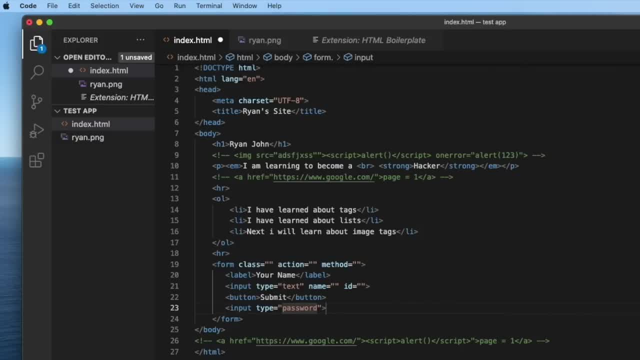 Just like this, And instead of the type text You're going to see a password. And if you save this And we come back over to our page And we look at this And we go ahead and add in a break, Because we want this on a new line. 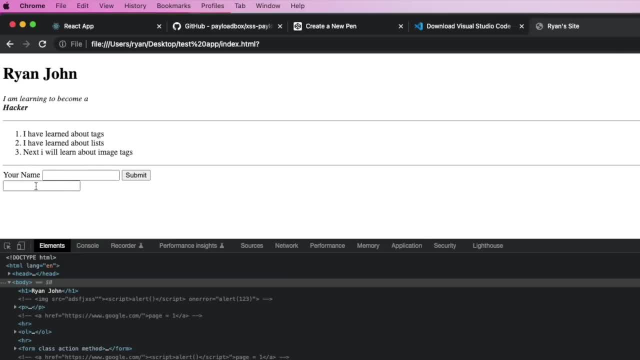 So we save this, We refresh it And that's pretty ugly And you'll see we have these little hidden dots, Just like here. This is to secure the password, And you'll see these a lot on web applications, But now they've started adding in this little eye over here. 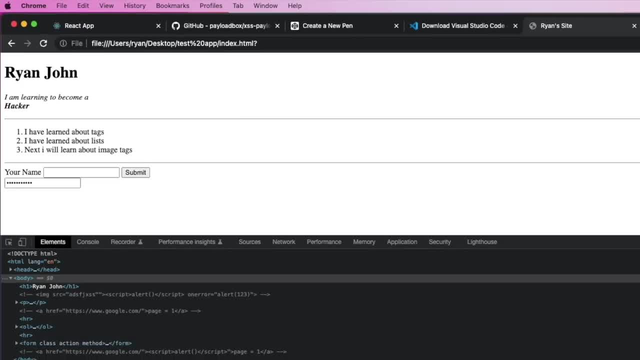 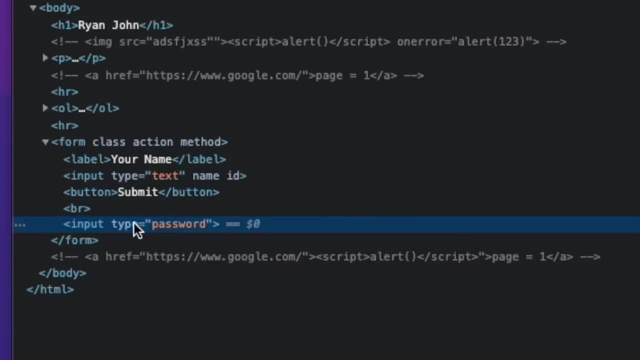 For you to be able to see what you're typing in, Because if you know any HTML and CSS at all, You know that you can just right click this And you can Inspect, And then you can come in here And just change this password to text. 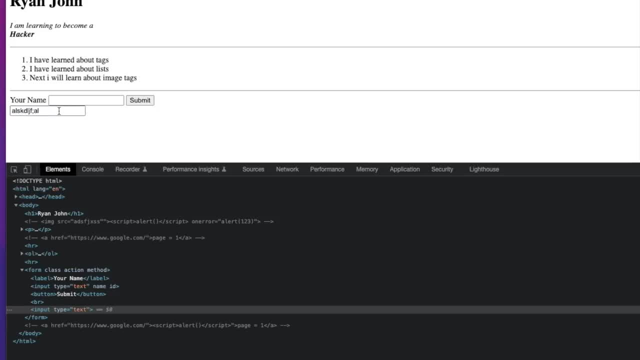 And then look at it just like this And you can see the information That is being typed in here. And this is why people, When they use public computers, Should never save their password, Because if you use a public computer And you log in, 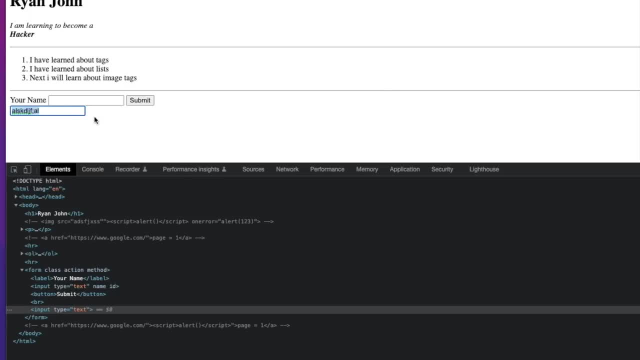 And you accidentally hit save password, Then the next user can come in here And repopulate the password And look at your email and password And have your information And then you can use public computers To enter in literally any of your data. 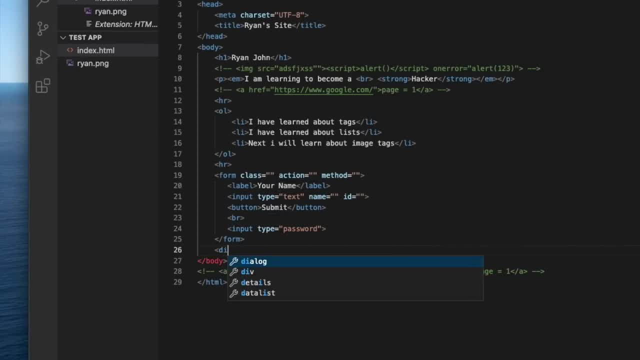 That is important to you. So there's one more thing I want to show you, And that is the hidden option, And so we're going to actually use a div here And I want to show you that you can just type in hidden right here. 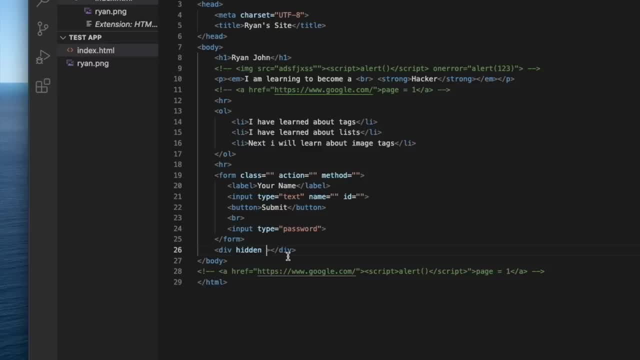 And usually this hidden will be Something other than the actual word hidden. There's other ways to hide elements within HTML, But we're going to use hidden because it's really simple, And then sometimes you'll see something like ID equals 8.. 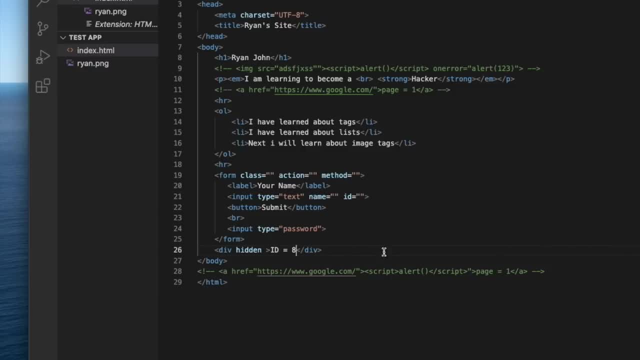 And then, if we save this, I've never actually seen this In the wild, only in CTFs. So this is not going to be something You're probably going to encounter in the wild, But you will probably see it in CTFs. 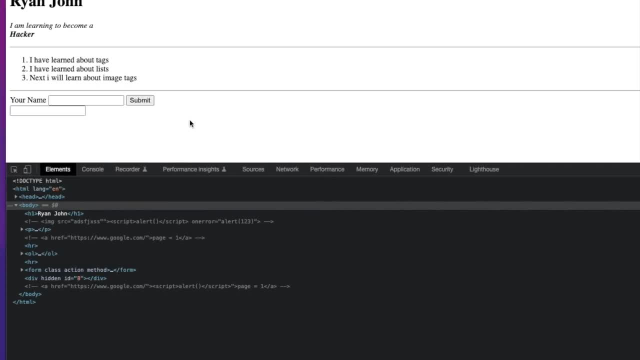 As I've seen it in several CTFs. And you come over here And you refresh this page, You can see that we have this div ID 8. And it's hidden. And we can unhide this by just deleting the word hidden. 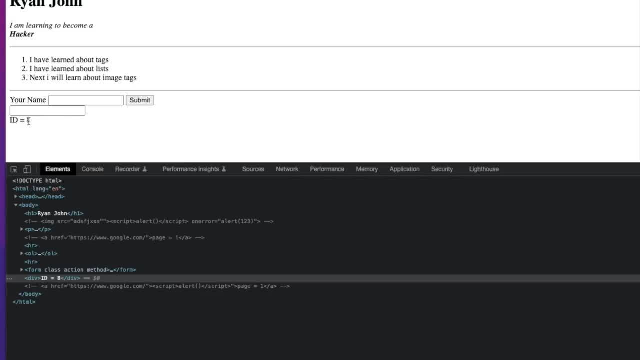 And now the ID shows up On the actual page And usually within CTFs, This ID 8 will be within a form And you would just change this 8. To something else, So you could come down here and say: 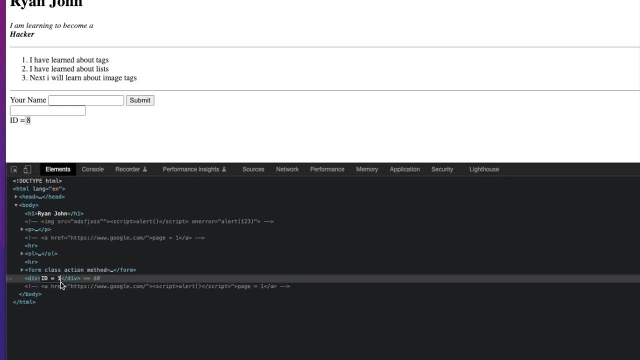 We're going to change the ID To 1.. Which would typically be an admin, And then you would hit the submit form And it would change your ID to 1.. That's usually how it will work in CTFs. I've never actually seen this in the wild. 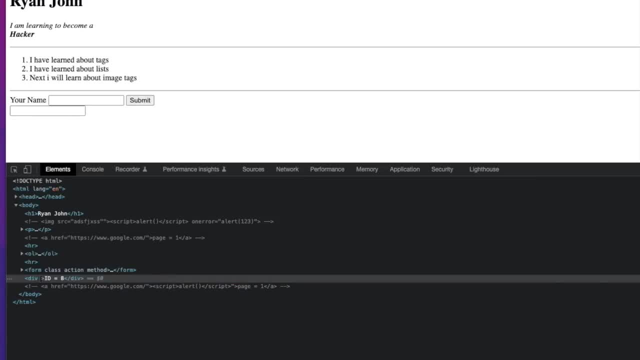 But it is something to be aware of. You can change this hidden to anything. You can just delete it And then you can change things within forms That have been hidden, Just by changing it. So that is something else to be aware of. 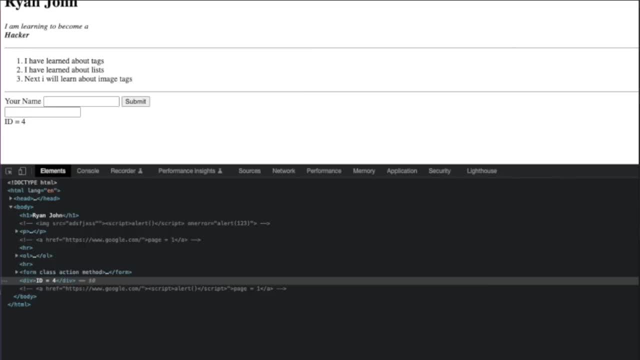 Within the world of HTML and CSS. Alright, So we have a future edit here, And I just want to say The reason that this would work in most CTFs Is because if there is no JavaScript To check the user ID input, 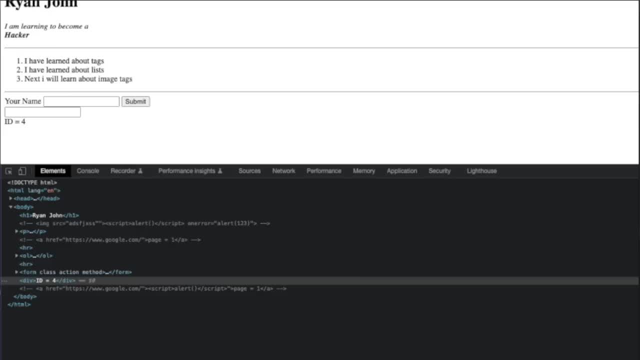 Then when you hit the submit button, It would go ahead and send it. But in most cases There's going to be JavaScript To check such functions. So a lot of times this is not going to work For sure, But for now. I have seen this in CTFs. 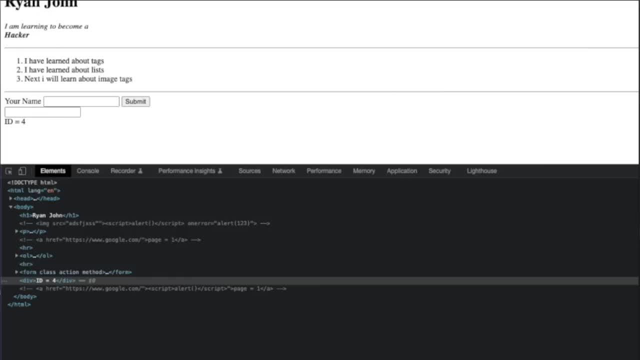 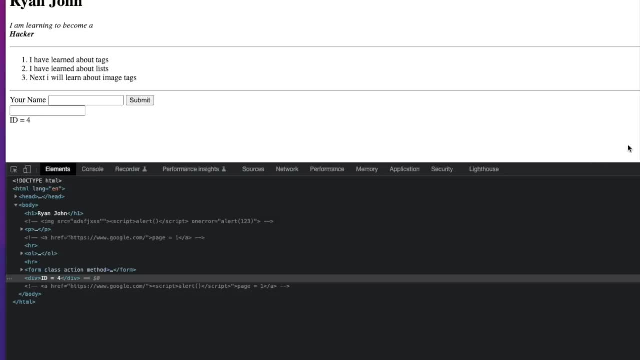 Where you can change an ID, Because there's no JavaScript checking To make sure that the user client side input Is what it is supposed to be. In the next video we're going to give Just a quick look at CSS, Because we're not trying to be web app developers. 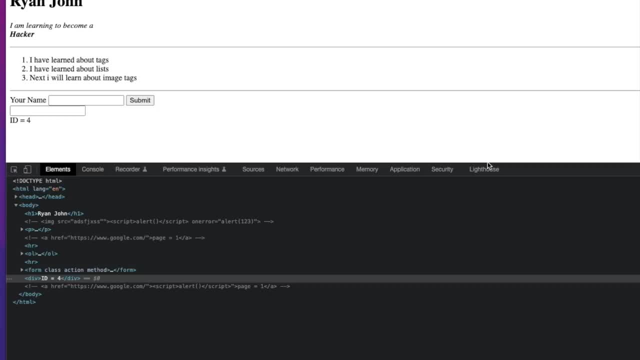 I'm not going to spend a lot of time on CSS, Just going to give you a quick overview So that you know what it is And when you see it You'll be able to recognize it And know that it really isn't anything important to you. 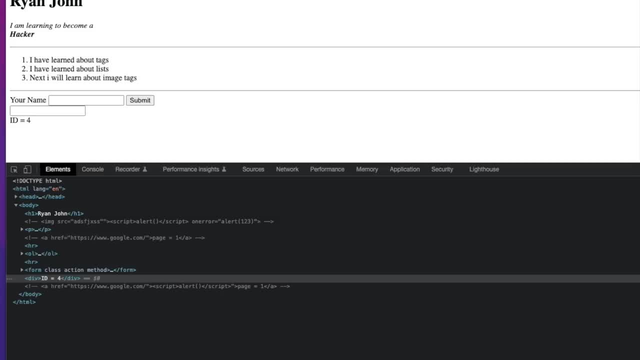 Because you are crazy good And you can pull off some kind of remote code execution Through a CSS injection, Which can happen But is really advanced. So we're going to just look at some simple Basic CSS So that you are aware of what it is. 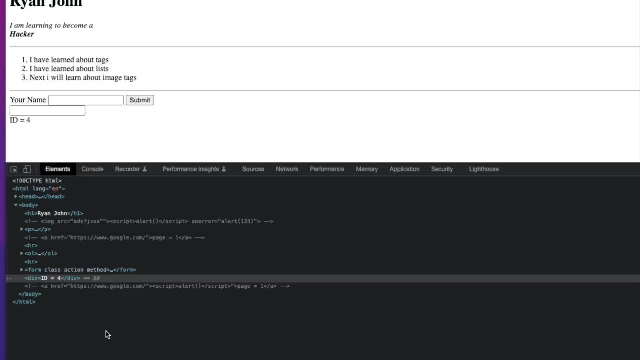 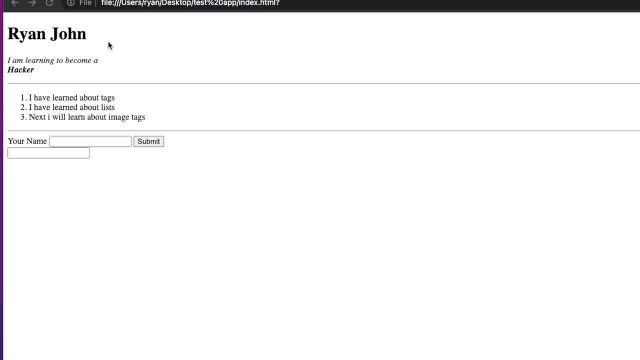 And you aren't questioning When you see it inside of some source code. I'll see you in the next video. Alright, we're going to have a look at some CSS. We're not going to spend a ton of time Working on our little website here. 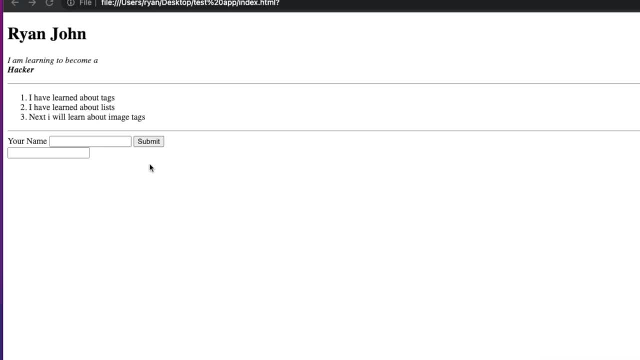 Making it look nice. I am not a designer And I don't understand web design And fashion or anything like that, Or color coordinating. So in the world of web development, This is for me The most difficult part- Is making a website look nice. 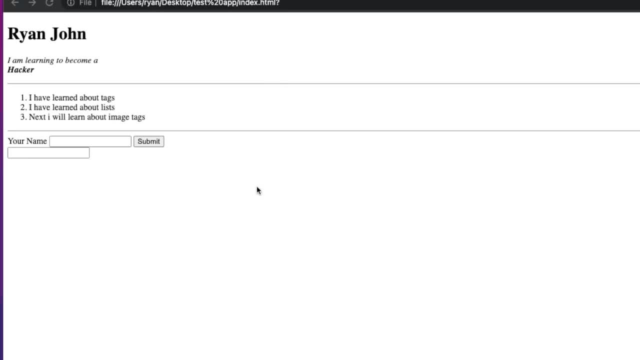 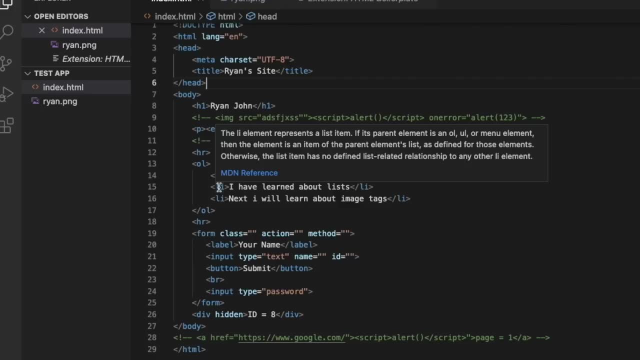 Some people are just gifted as designers, And I am not one of them, So I'm just going to show you how CSS works In two different ways. I'm going to show you internal CSS And I'm going to show you external CSS. 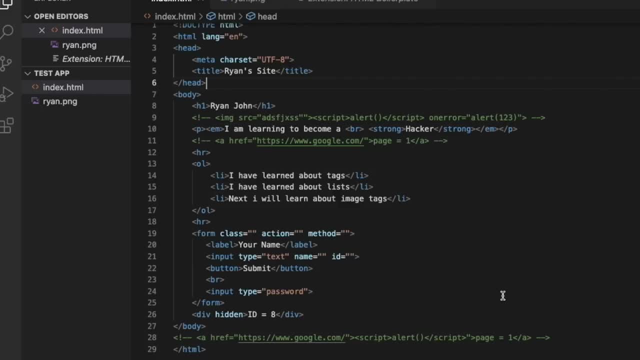 So that way, when you come across CSS And you're familiar with it, I'm not going to actually show you How to design a web app, Because that is not my area of expertise And it's not my gifting If we want to do some internal styling. 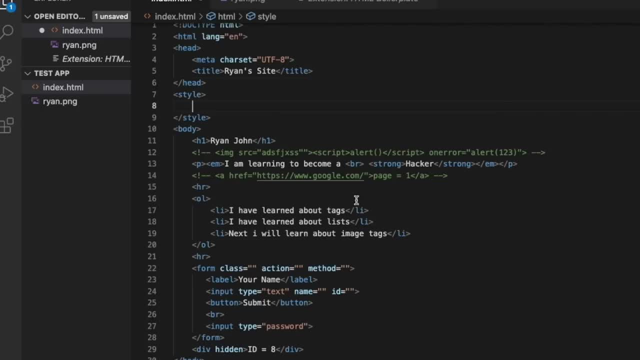 We can just come in here and type in style And we can hit enter, And then we have this H1 right here That has our name in it. So we can just very easily just type in H1. And then we open a set of curly braces. 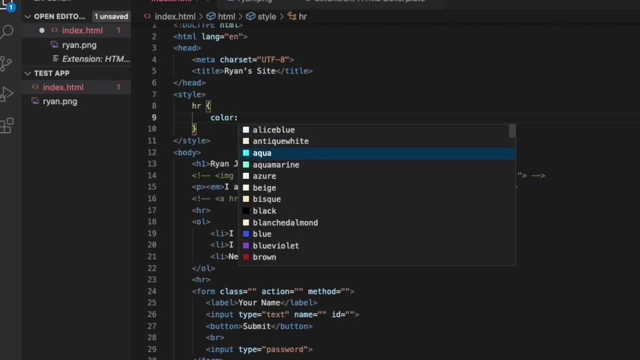 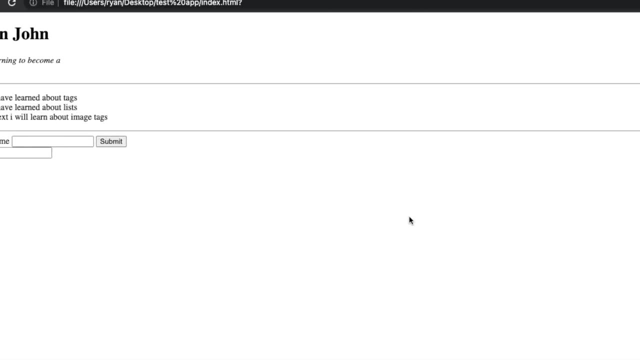 And then we can just type in color, And then we can just type in: aqua Looks like a great color. And then we close it off with our little colon there And we save it And we come over and refresh our page. 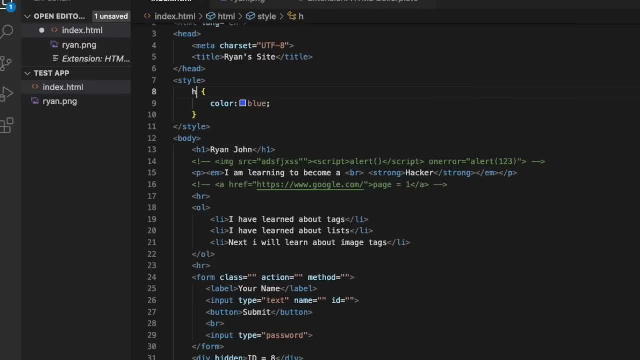 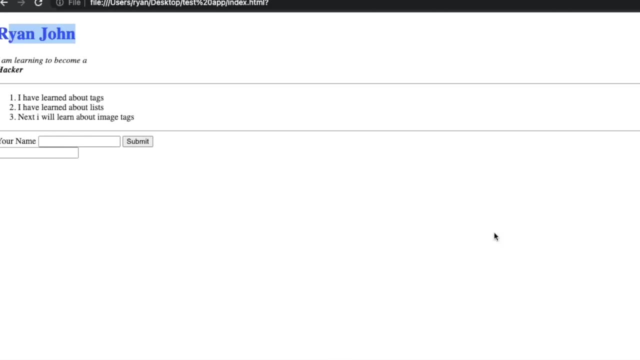 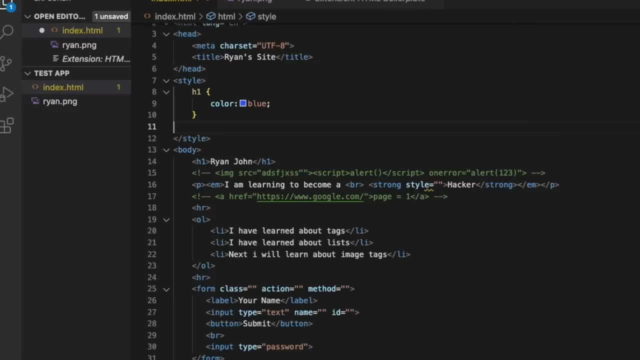 I see I didn't type in H1. Typed in HR. So we type in our H1. Save it, Refresh And our color changes to blue, And then maybe we want to change The word right here. Hacker, There's another way you can go around doing internal styling. 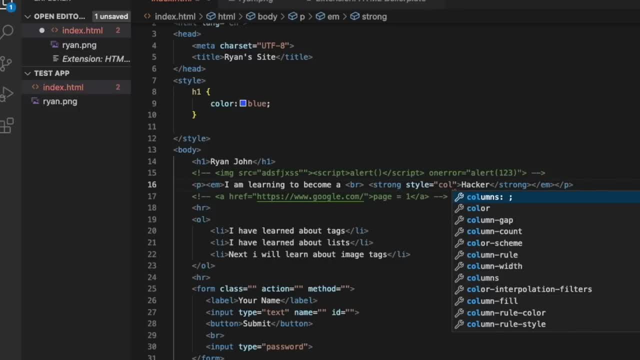 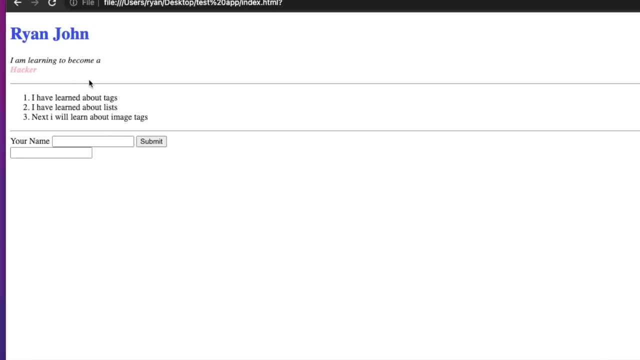 And you can just come in here and say That you want a color, And then we say We want pink, And then we can save it this way And then, if we refresh it, Our color works. So there's several different ways. you're going to see internal CSS. 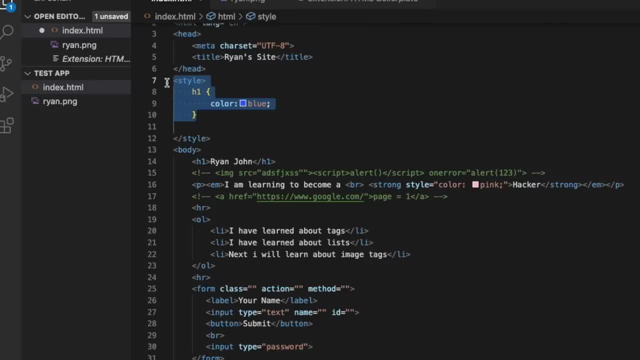 And this right here is the most common. This happens, But it doesn't happen very often. So when you're out in the wild, You will see CSS function Like this, And you can also do a lot more with this. We're not going to cover it. 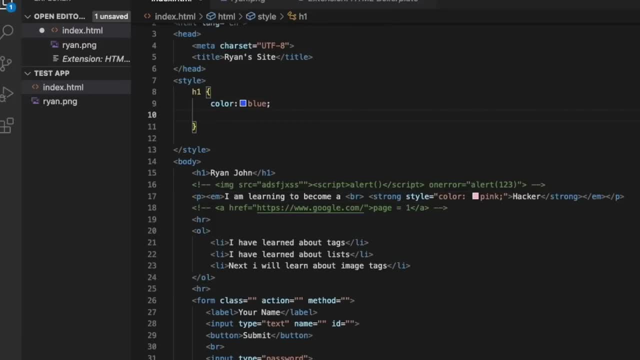 So you could come in here To this H1. And you can type in something like Padding And you can say padding left, And then we could say like 200 pixels, And then if we were to save this And come back over, 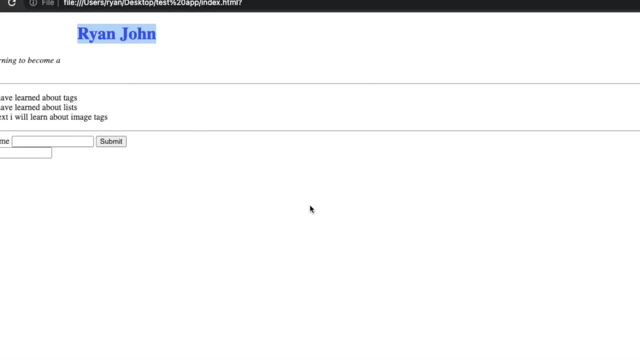 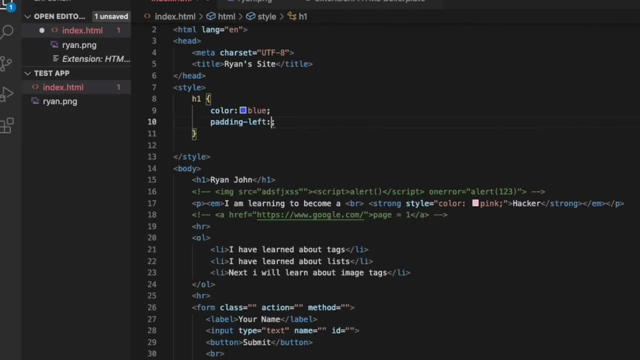 And refresh it, You'll see that the name moved. I'm not sure if there's a centered option, Let's check it out. There is not, So there's something called bootstraps. That would really help you with your styling. 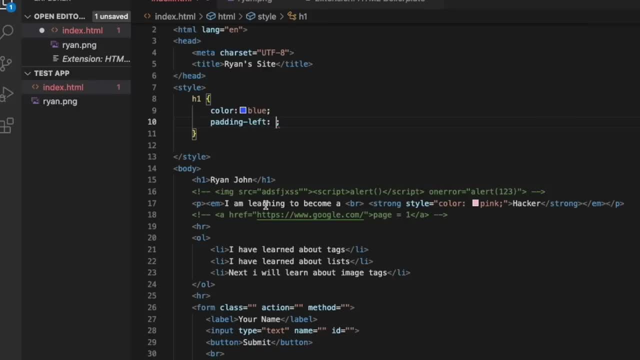 If you were trying to become An actual developer, But we're not going to spend a ton of time with that, So you can do things like the padding left. You could do a padding For the bottom If we wanted some space. 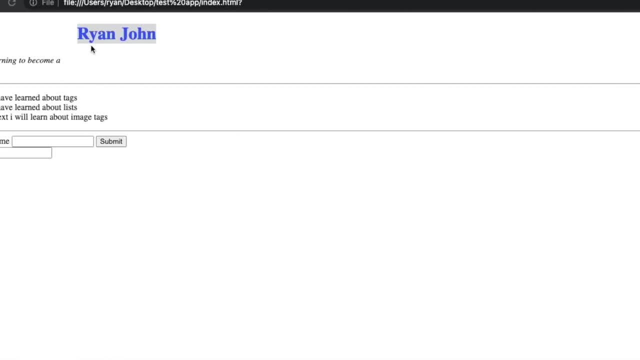 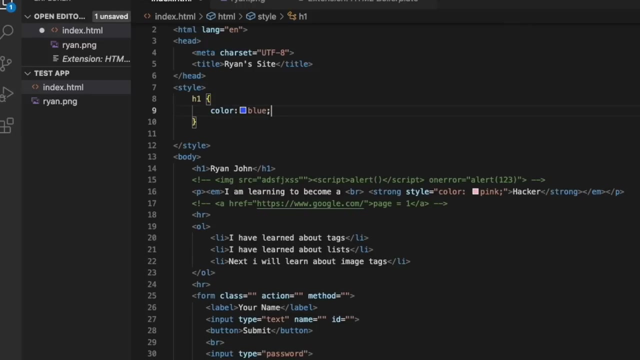 Between our Information here And you could say 100 pixels And you could save this, And if you came over here And refresh it, We'll get a padding over here. So this is a little bit of styling That you'll be familiar with. 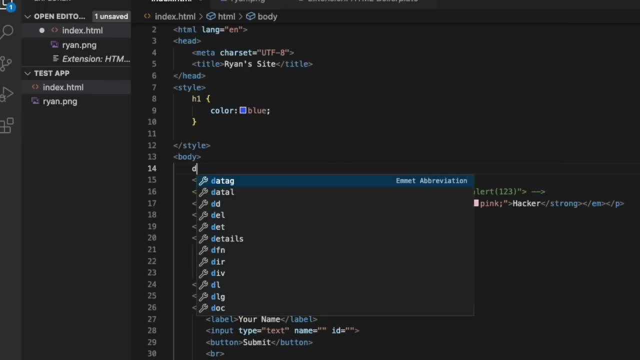 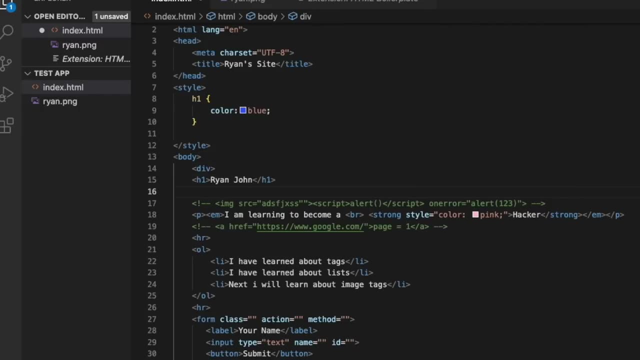 Is a lot of times things are going to be broken up into divs, So you would have something like this: Right here You would have a div And we'll just copy this And cut And we can paste that right here. 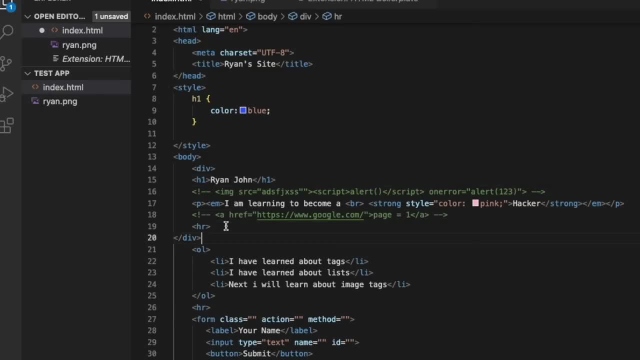 And then we'll put another one, We'll put this right here And then we'll put one down here Between our list That we have Right here And then if we were to Go to the other side of here, Like we say, this div. 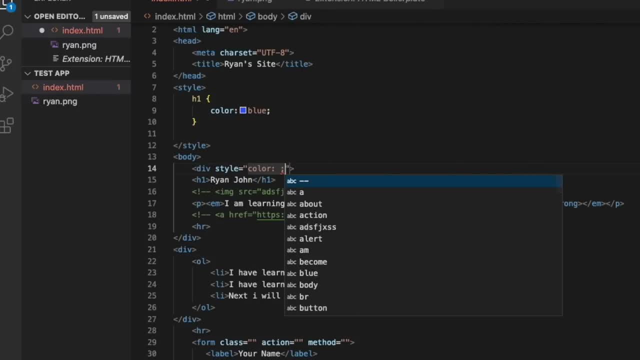 We want to style it And we say style, And then we want color, And then we're going to make this entire color Red. It's going to be very bold. And then we decided to make a different div And we wanted the entire color. 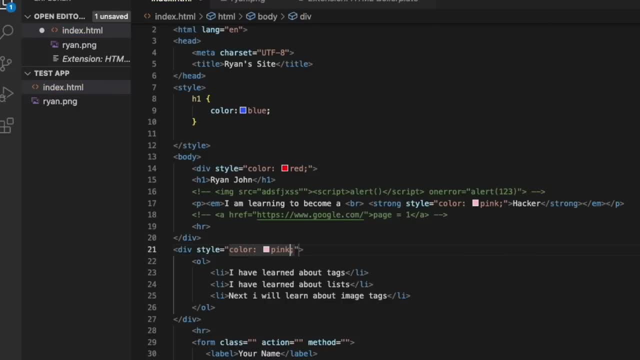 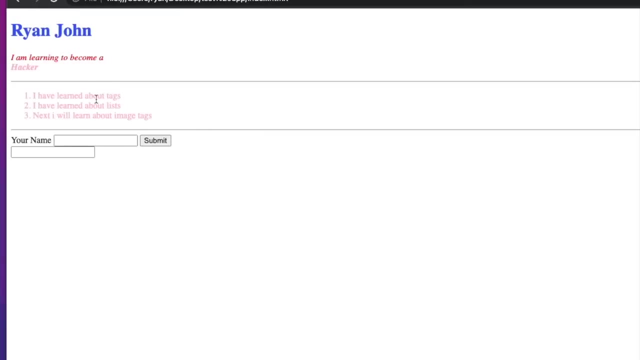 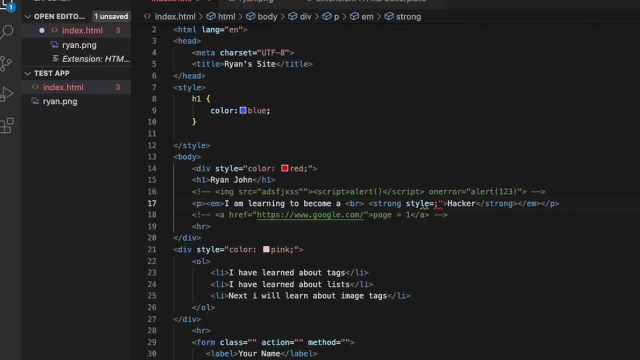 To be. Let's say, We'll make this entire color pink And we save this And we refresh our page And we can see that One of those divs Actually changes colors, Except this overwrites What was written inside the div. 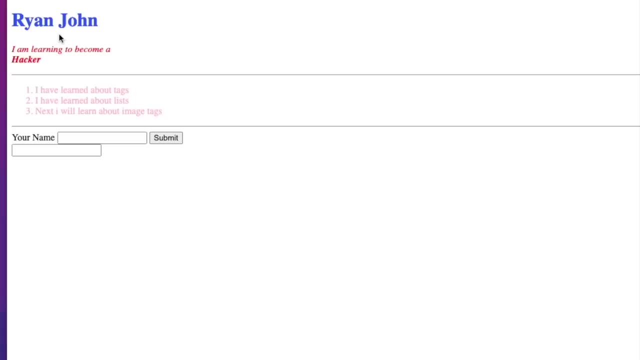 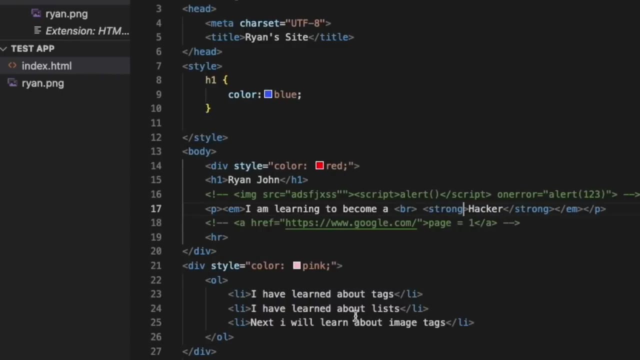 So we can actually just go ahead and close this out Right here And now. if we come back and refresh, You can see everything becomes red And pink within the specific div, And so this is an introduction To internal CSS. You can style it either up here like this: 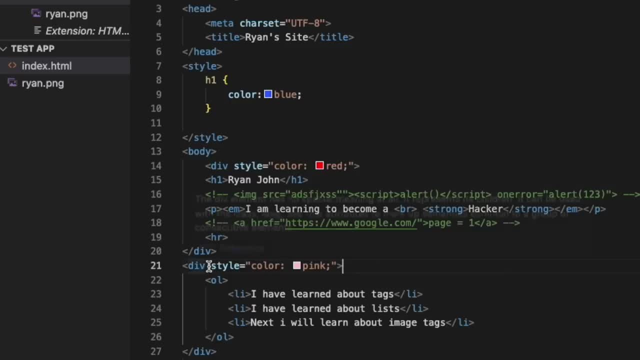 Or you can do some internal CSS And so You can be like Within HTML and CSS, You can think of everything as being inside little boxes. And there's actually a Chrome extension: It'll actually show you all of the boxes And it's called pesticide. 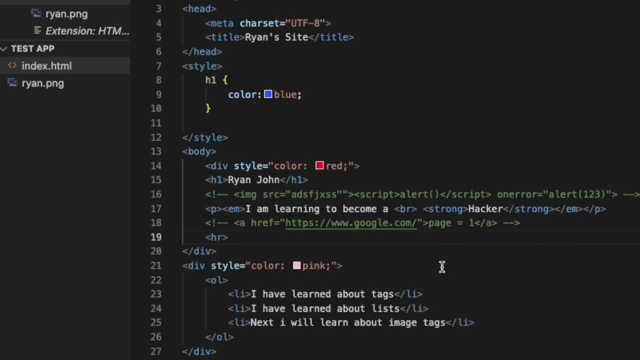 And you can install it if you want. I'm not going to show it Because the point of our course Is not to learn how to be designers. The point is for us to understand CSS Well enough To know what we're looking at. 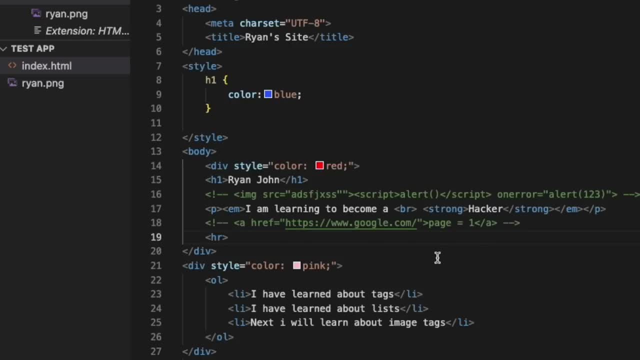 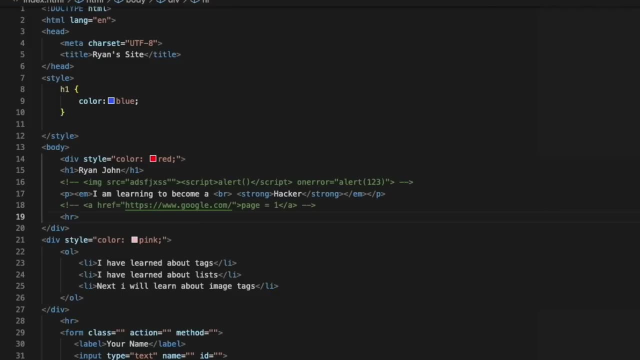 So that we can figure out how we can exploit web applications When we come across it. With that, in the next video We're going to look at external CSS. Okay, in this video We're going to look at an external style sheet. 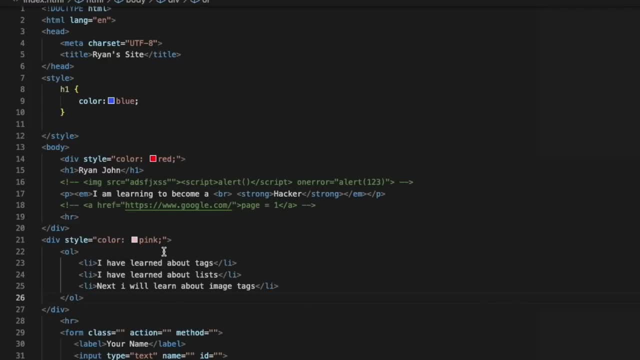 And then I'm going to show you Why this was important for you to learn. So the first thing we're going to do Is we can just go ahead And delete these inline styles That we put in right here, So that way we have our blank page. 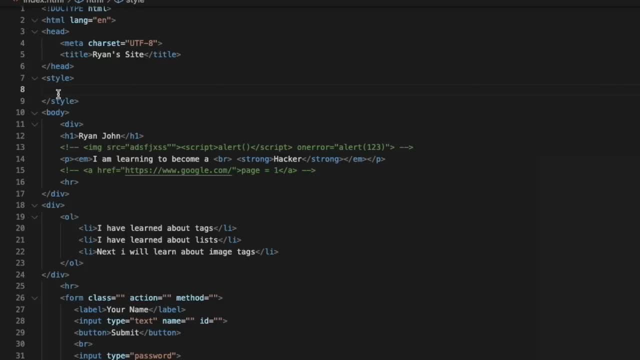 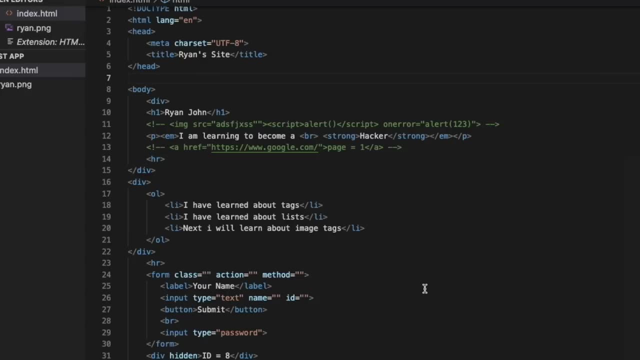 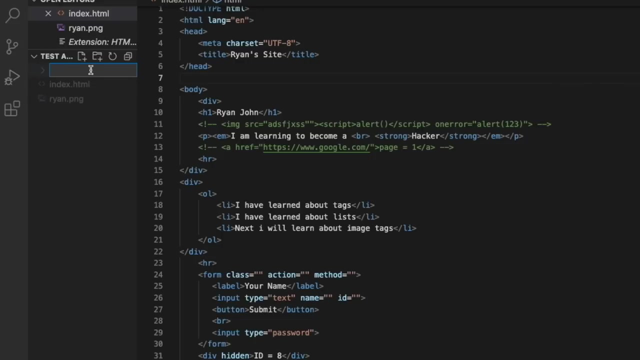 Like we did before, And we can just go ahead And delete the style altogether And then, if we save this And refresh, Everything is back to how it was before. Now what we are going to do Is come right here And we're going to add a folder. 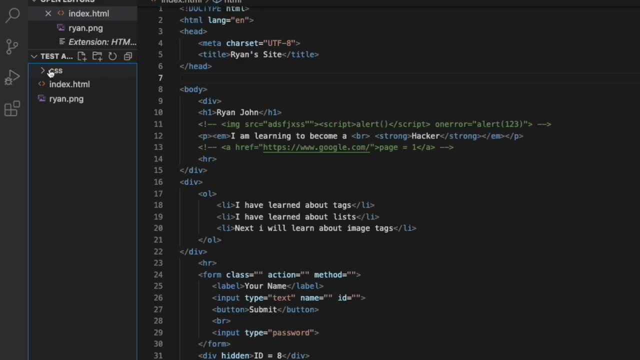 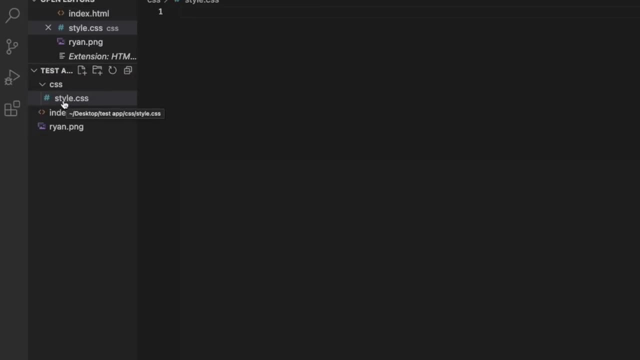 Just like this, And we're going to call it CSS. And then inside this folder We're going to add a new page And we're going to call it stylecss, And you can see our visual studio Has recognized it as a style sheet. 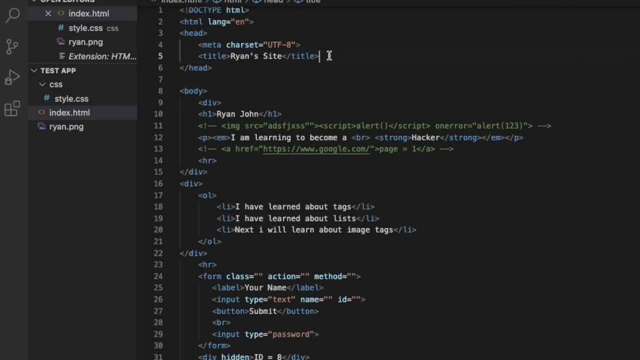 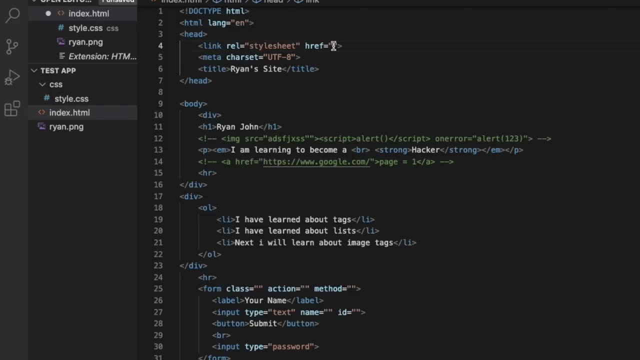 Come back to our indexhtml And inside of the Head tag up here And type in link And it tells us that it has this style sheet And we have the href2.. And we want to link our CSS style sheet just like this. 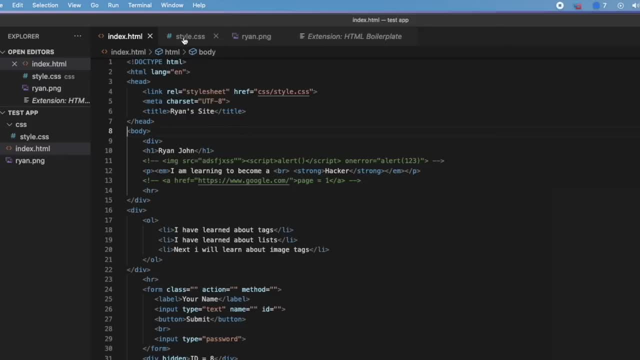 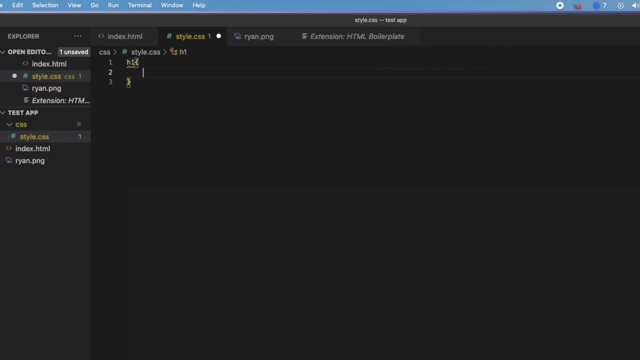 And it autosaved for us And we can now save it. And now you can come over to your style sheet And if we wanted to do like we did before, We can type in the h1. And we can type in color. 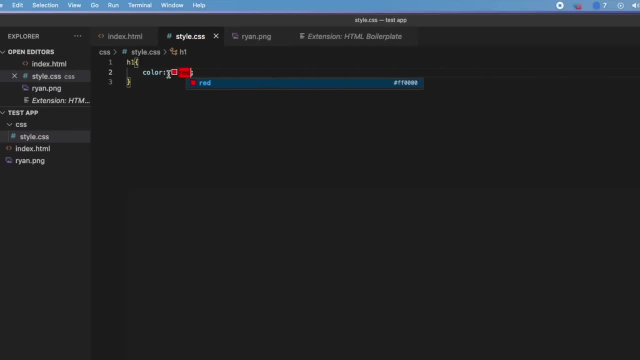 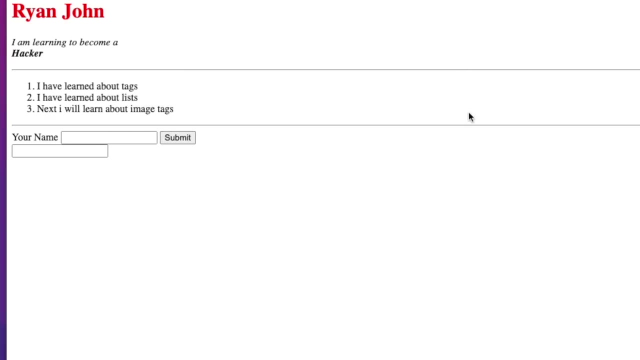 And we can say red. And if we save this And come back over to our page And refresh this, And it's now red Because that was the h1. We can do something like we did before with these divs And we can say: 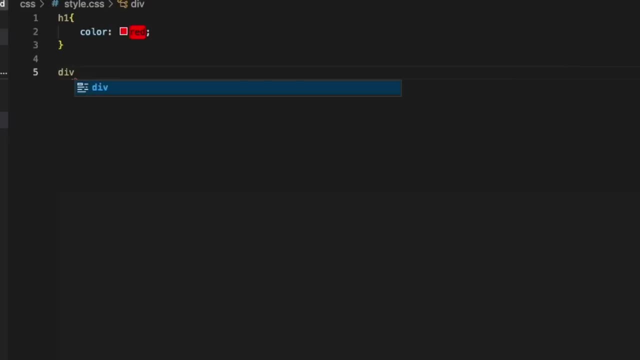 We want to give the div a color So we can say div1.. We want to have a color of blue So we can come in here. We put our period before the div And this is going to tell it that this is going to be our keyword. 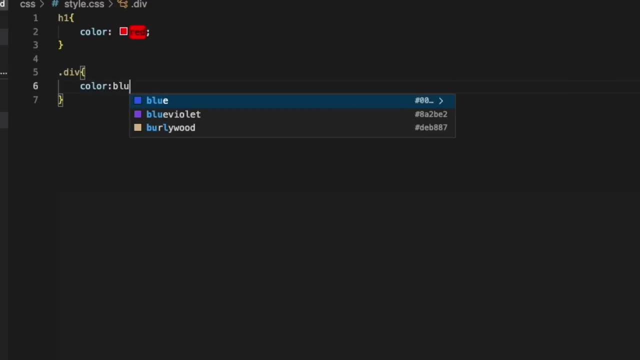 And we can say color, And we want blue, Just like this, And then we'll make a div2.. So we'll say period Div2.. I forgot this was div1.. And we can say: we want the color Of pink. 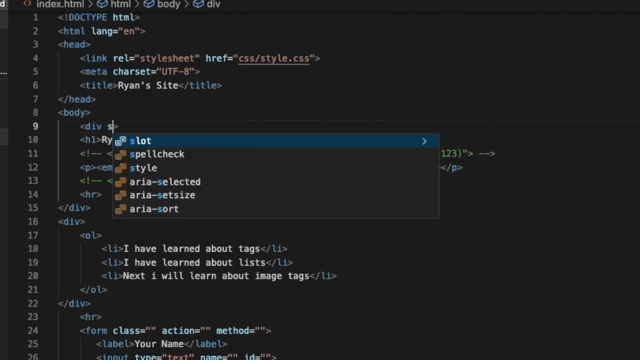 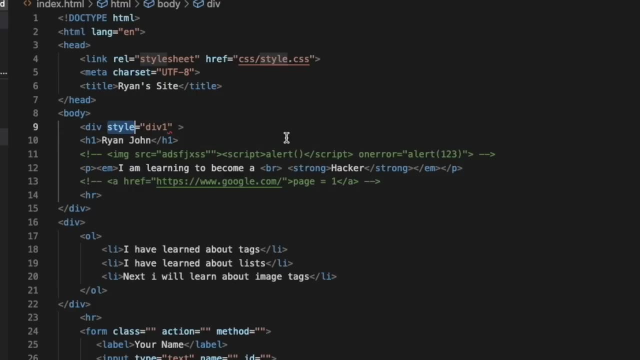 We'll go div1 right here And we can say Style: div1.. And I just realized That this is supposed to say Class Because we've given it a class name Over here, And then if we give our second div, 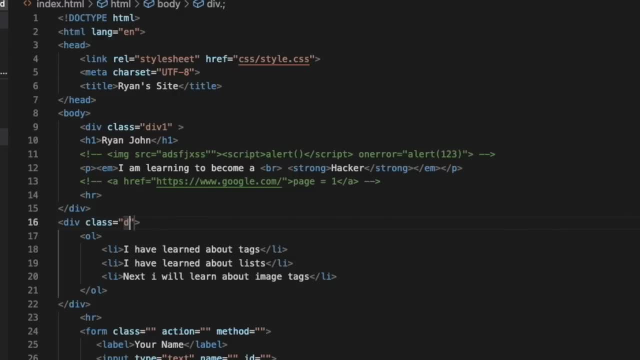 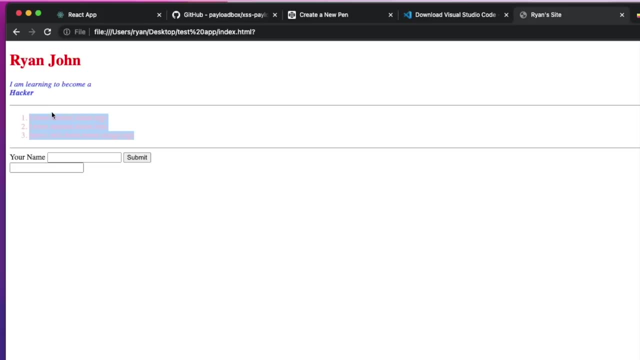 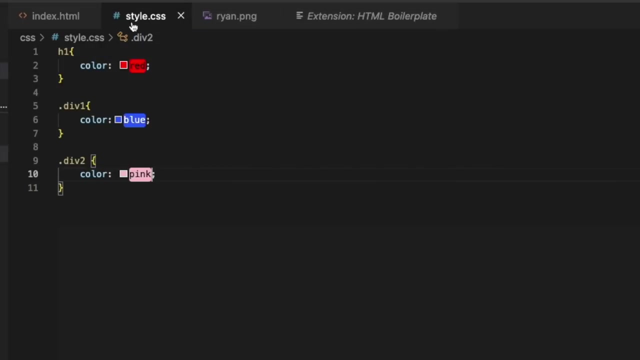 A class Of div2.. And we save this And we come over here And refresh it. We now have the colors have changed Within our div And our name color has changed. So this would be a form of External CSS. 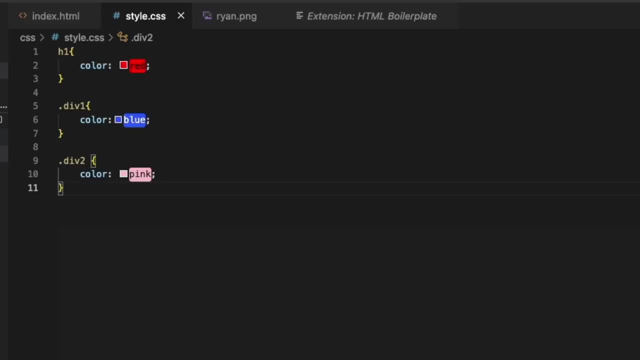 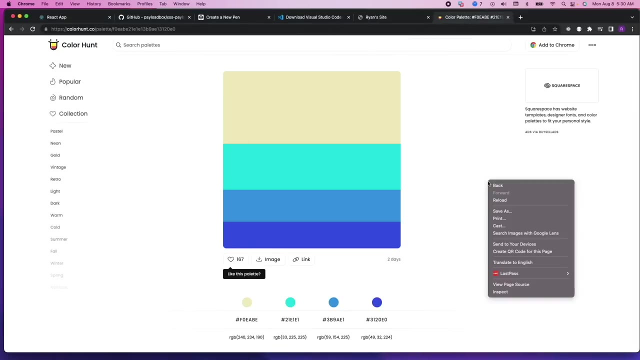 And I want to show you why it was important for you to know this. And it's important to know That this file was named CSS And then we called it stylecss. If we come back over here And we just check out this color palette, 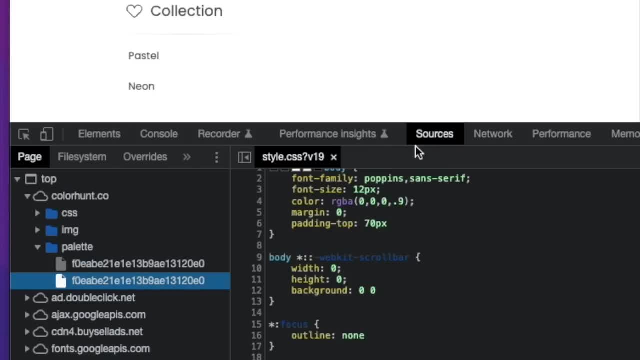 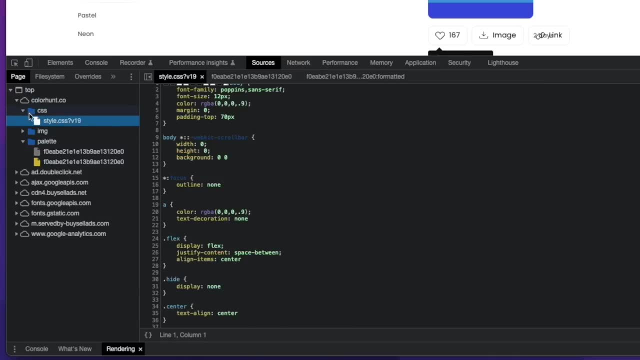 And we inspect the page And we come over here to the sources. You can actually click on this CSS right here. Yours might not be all in line like this. You can click on the CSS, Click on the style page And then click the pretty right here. 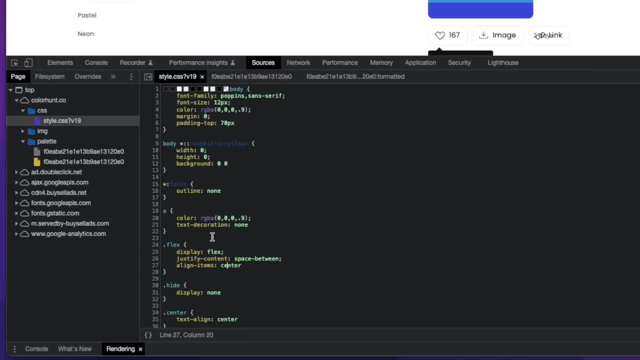 To make it look pretty And you can see, just like this, What they have done. It is organized just like ours. So this would be an anchor tag Which would be clickable, And they have red, green, blue, Not sure what the A is. 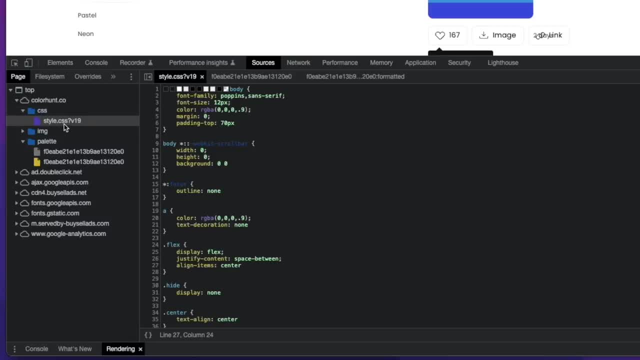 And then the style sheet is called CSS, Just like ours And stylecss, And then it is formatted exactly the same way And this would be an external style sheet. And then, if you come back to Looking at the elements, You can see the class right here. 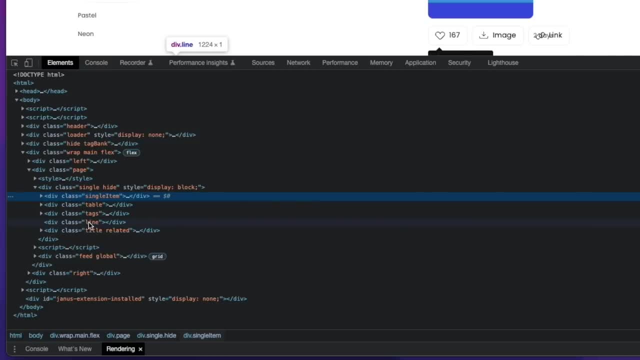 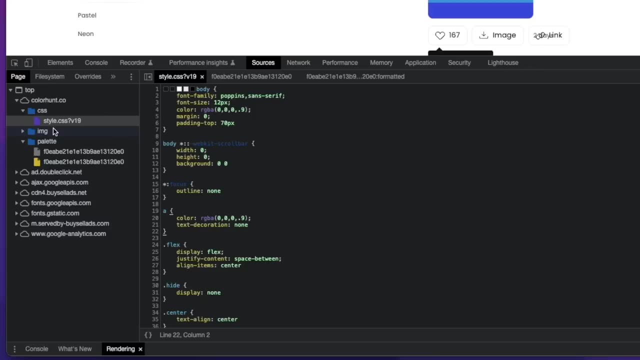 The class names for how they decided to Name their classes And organize what they look like Based on the CSS. So now, when you come in here And you inspect a page And you come across a CSS file, You will know what you are looking at. 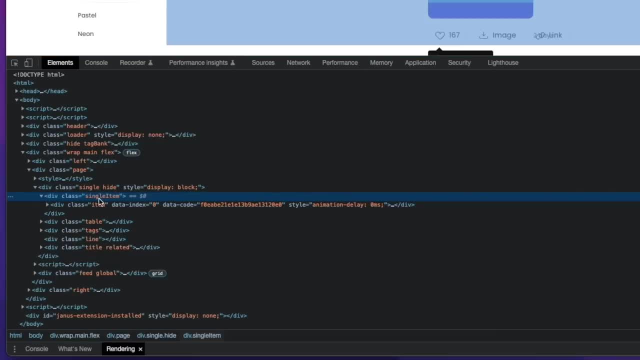 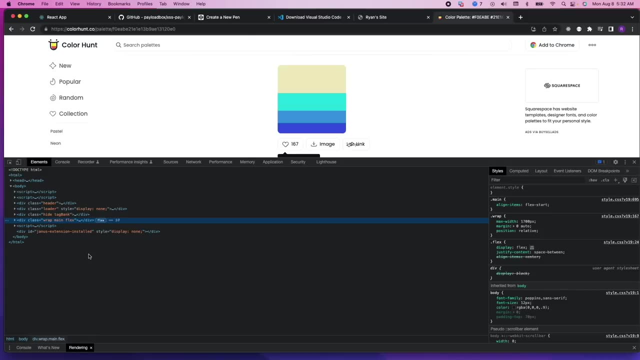 And you will also be familiar with seeing class Inside of the divs, Seeing these class names. And that is going to wrap up for us, The CSS, Internal and external. I will see you in the next video. Okay, we are going to be moving into a section. 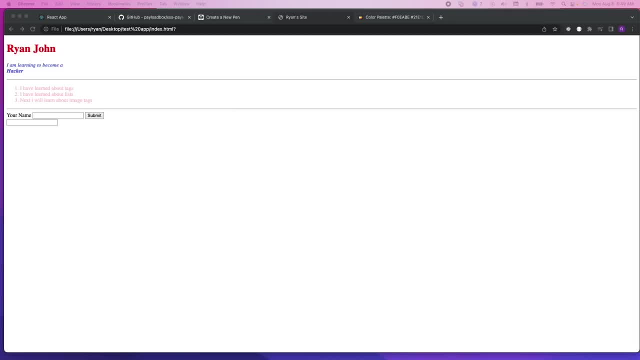 On JavaScript, And so, as we go through JavaScript, It will be helpful for you to have a great place To practice your JavaScript. And a really easy place to practice JavaScript Is within the Chrome Developer Tools, So I would suggest If you do not have Chrome installed. 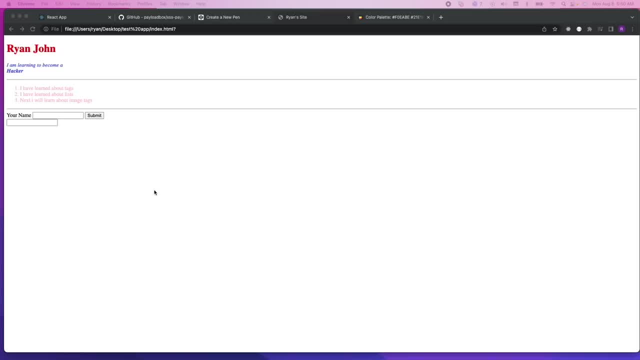 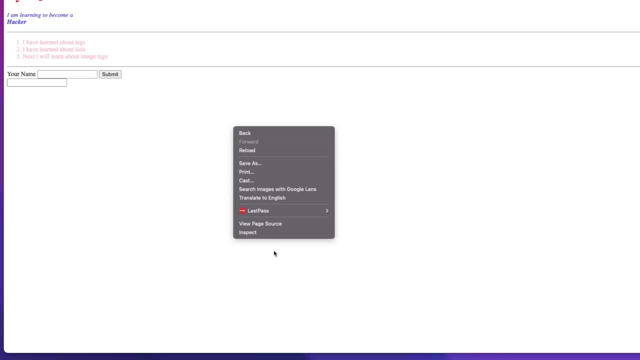 Go ahead and install Chrome, Because we are going to be using it throughout The portion of our JavaScript course, So an easy way to practice JavaScript Is: just come over to your web app That we have running within Chrome. We can go to inspect. 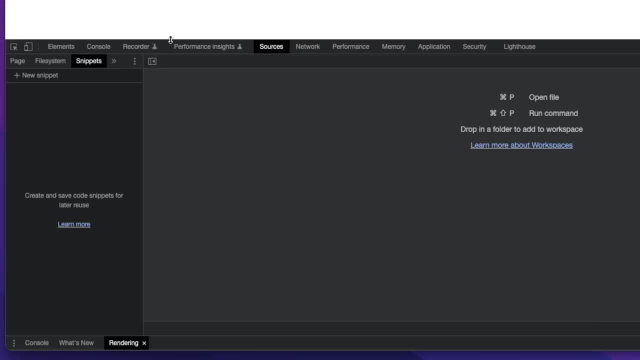 And then we will go to Sources. You are going to be on this page right here. We are going to hit these two arrows right here And we are going to say snippets, And then we will say new snippet And then we can just call this indexjs. 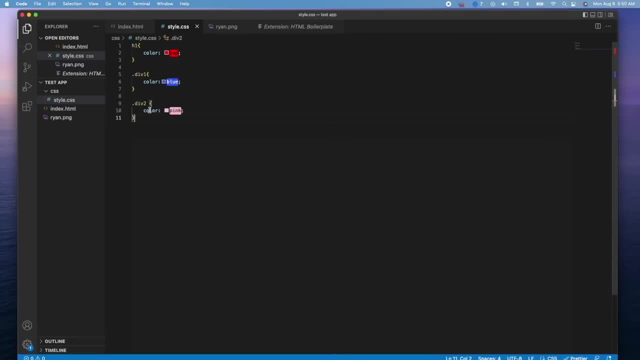 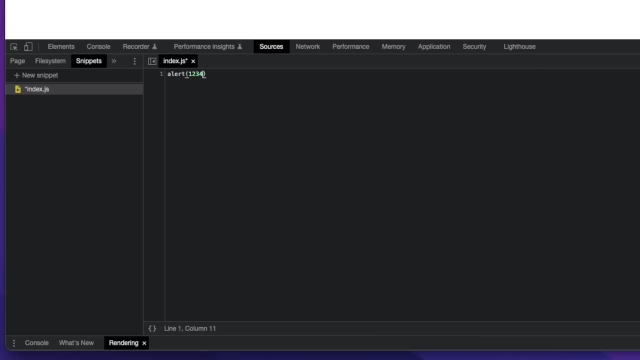 Which is the file name Within your code. You would have it named over here And then you can actually just type in Your JavaScript right over here And then, when you are done, You can run it just like this By hitting play. 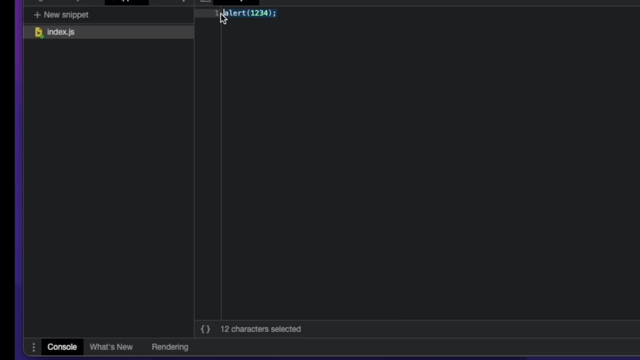 And it will hit up an alert for us And then, if we want to Do something like a Consolelog And then we want to log something, It will actually pop open For us right down here And it will tell us what we have logged. 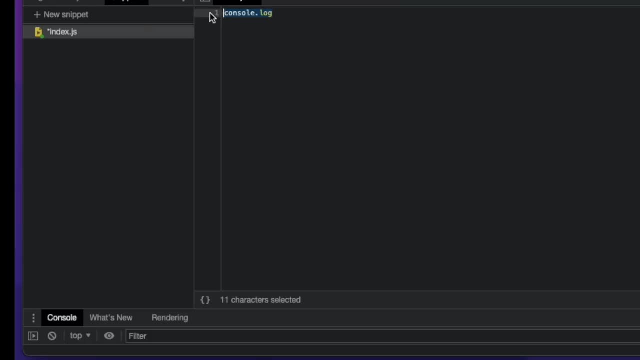 So this is going to become more Familiar with you as we are going along, But this is where we are going to be Practicing our JavaScript And if you are unfamiliar with JavaScript entirely, JavaScript is the scripting language Of the internet. 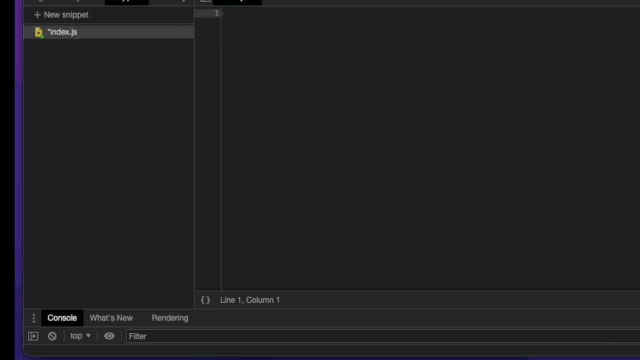 So, if you are wanting to become A web application penetration tester Or a bug bounty hunter, JavaScript is going to be something you are going to want to learn, Because it is the language of the internet. It is what gives Websites functionality. 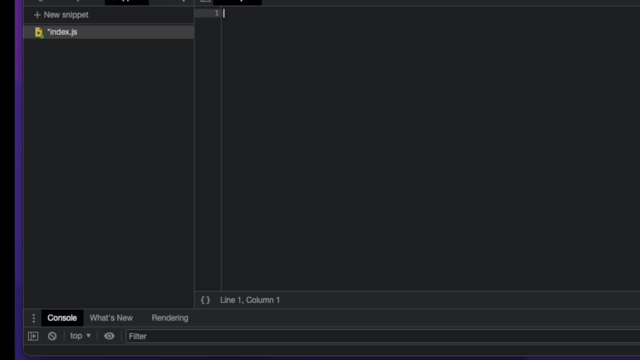 So when you go to a web application And you see things moving around And stuff happening, That is going to be thanks to JavaScript. So JavaScript is going to be very important For us to learn And we are going to spend quite a significant amount of time. 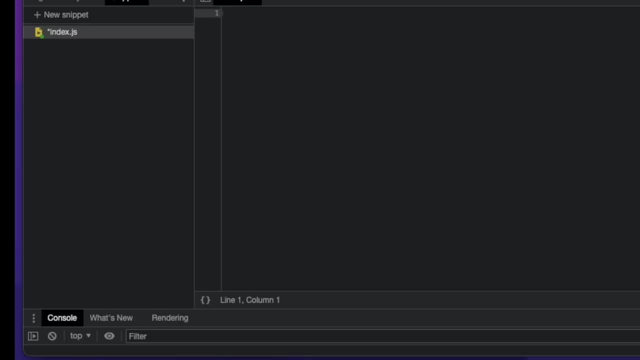 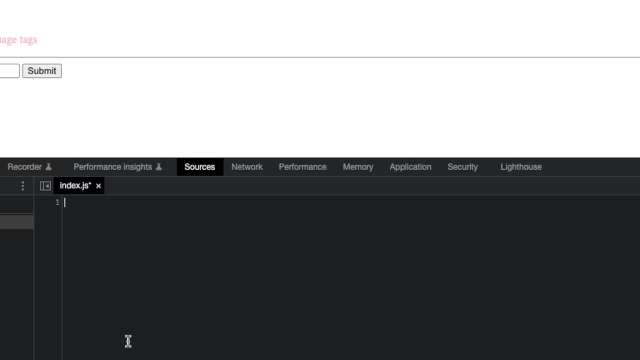 Learning this JavaScript, And so buckle up and get ready For JavaScript. One thing that is important to know About JavaScript, and really any scripting language, Is syntax. So you saw me type in alert Just like this, And then we can type in the word hello. 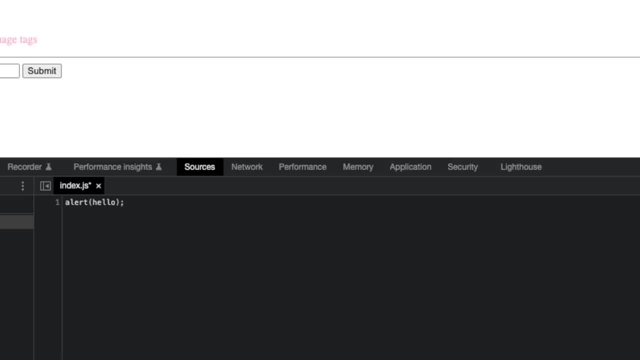 And then, if we close this off, This is not going to work for us. We are actually going to get an error, And if we open up our console, It tells us that we have an error right here. The reason is because These characters within this alert. 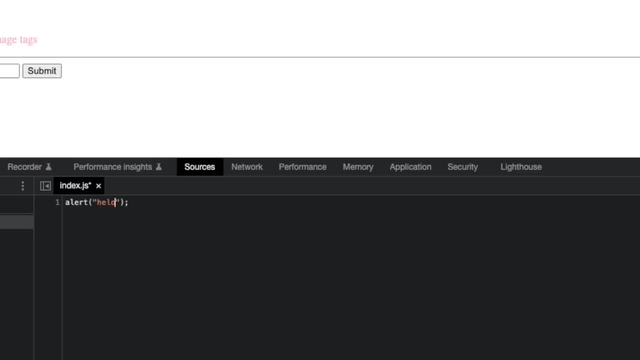 Need to be within side quotations Because this is considered a string, So JavaScript wants to interpret Whatever is inside of here Either as integers One, two, three. This will run for us And it will work Because these are integers. 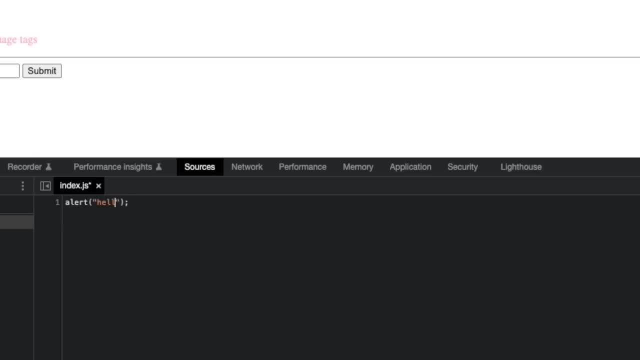 Or you are going to need to have strings inside here. So if we type in some characters, We will need them inside of a string, And now, if we run this, It will work for us. So we have this alert right here. What is this alert? 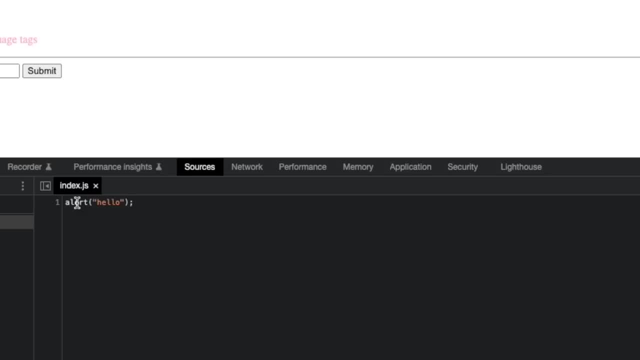 This alert is calling a function within JavaScript, And in the future we are going to make our own Custom functions, But for now all you need to know This alert is a function And it is going to pop up The string of characters that are put within here. 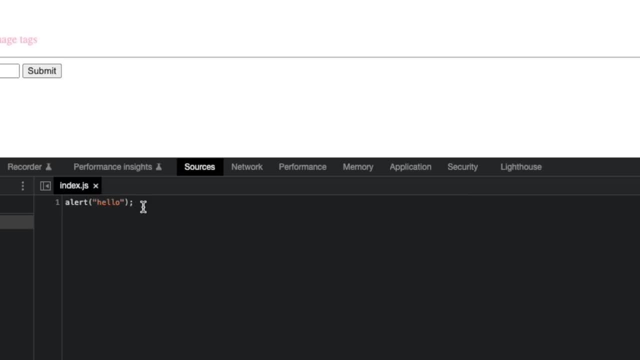 That are being passed within the function, And then I believe we need this within Chrome Developer Tools To close off our alert, And I guess we do not, But typically when you close something off, You will close it off with a semicolon. 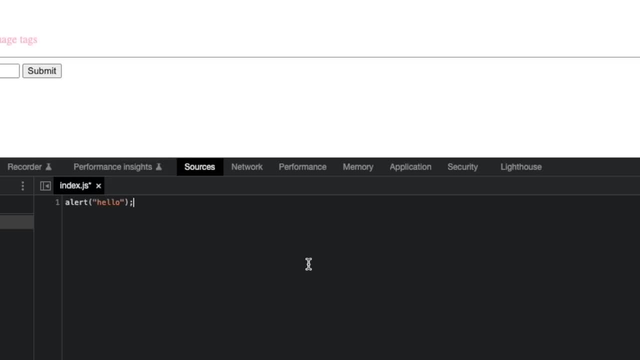 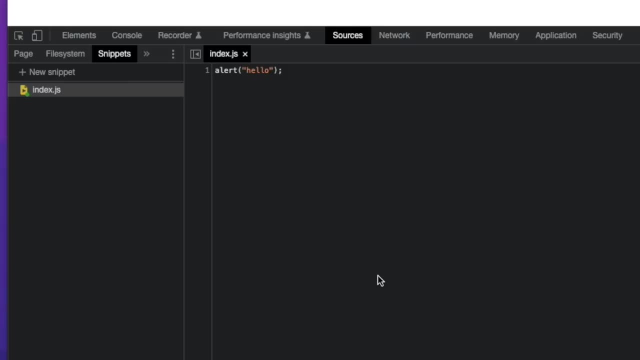 Just like this. So it is best practice to go ahead And start putting it in there now As we are practicing. See you in the next lesson. Before we make it too far into our JavaScript lesson, I think it is helpful to know. 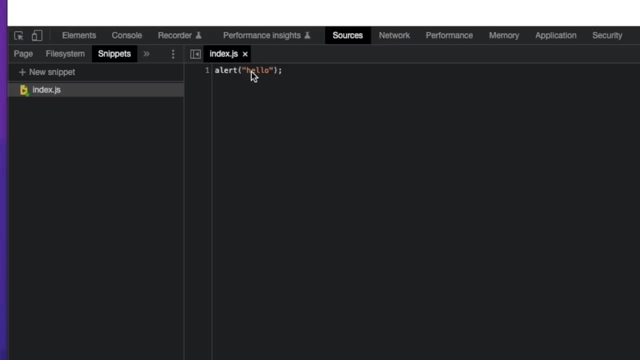 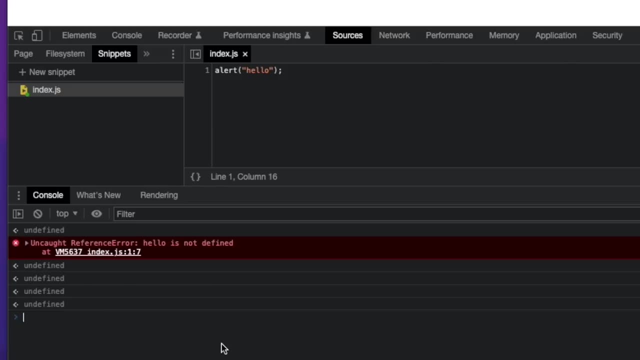 There are several different types of data types And we have already saw This one right here With a string. But if we pull open the console here, Which is really great, It is going to be a very useful tool to us As we are learning our JavaScript. 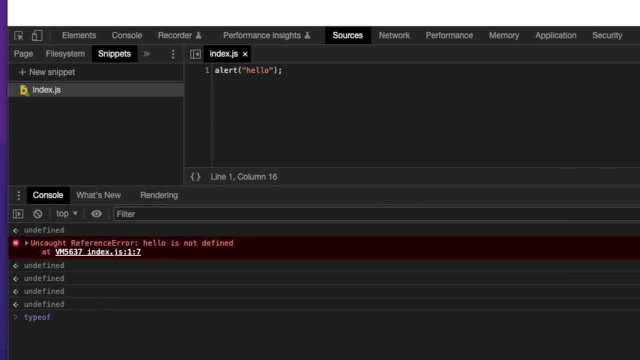 We can type in something called type of, Just like this, And then we can put whatever we want Inside of our brackets. right here We can put in one, two, three, And it tells us this is a number. And if we put in a string right here, 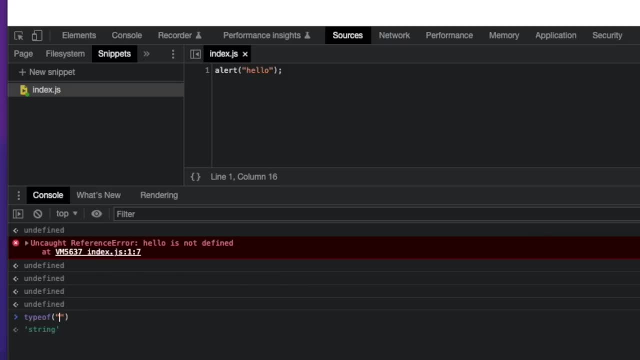 Like this: We don't even have to type anything in And it tells us this is a string. And then we also have one other type of data type That will be really helpful to us, Especially when we are running while loops. And that is true, false. 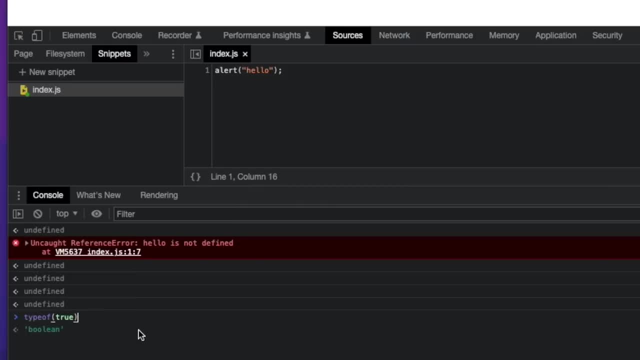 And it will tell us: this is a Boolean. So you have strings, Integers and Booleans And we are going to be using all of these As we move into our JavaScript. It will be helpful for you to remember these. You are also going to see these: 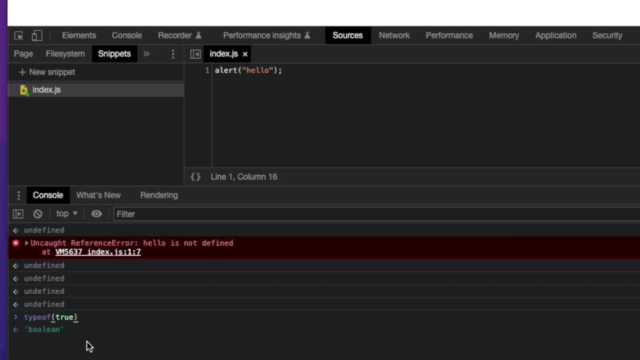 Within different exploit write ups Within the world of hacking, And so it is important to know That you have integers, strings and Booleans, Because you will come across these in the future And if you ever do any kind of programming Or you are writing up the code. 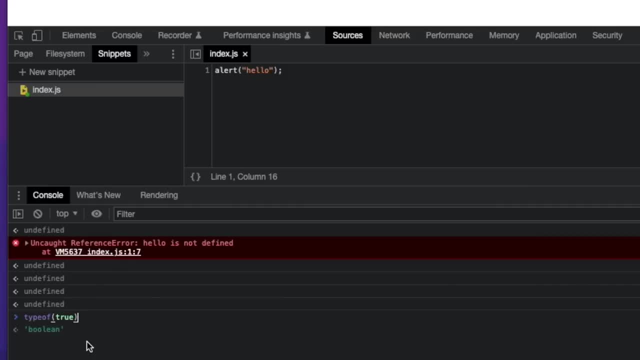 For your own exploits Or modifying exploits, You will need to know what is going on And what kind of data types you are dealing with. So with that, there is one more area of JavaScript That I want to cover, And that is any kind of code. 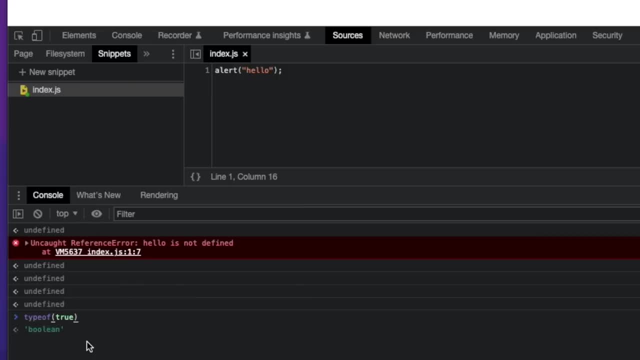 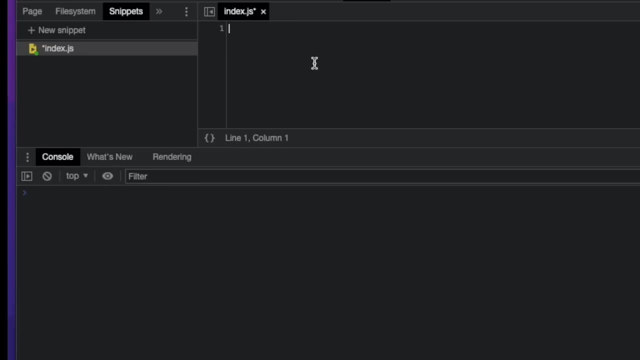 Or do any kind of exercises, And that is variables. So with that, we will check those out in the next video. Okay, so here we are With our variables, And there is a couple of different ways. I want to show you how to use variables. 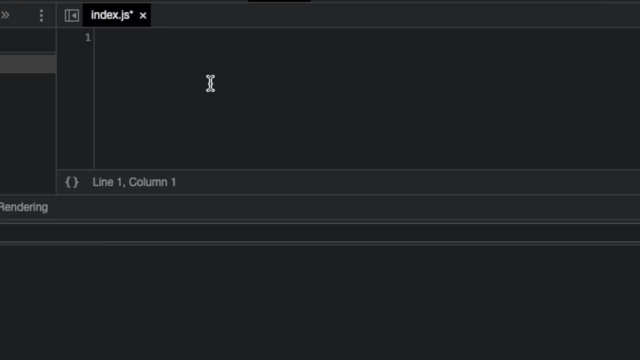 The very first thing I want to tell you about variables Is that it stores some information for you. A variable is going to store some kind of data That we can later come back and say We want this variable. What information is within it? 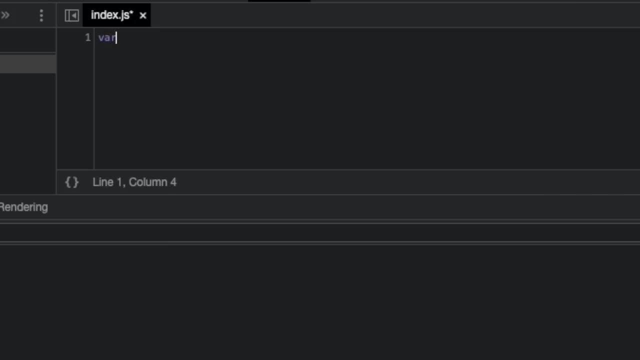 And it will tell us the information that is in it. So, for example, If I say var equals 2 plus 3. And then we have to name our variable And we will just call it num. So we have this var. 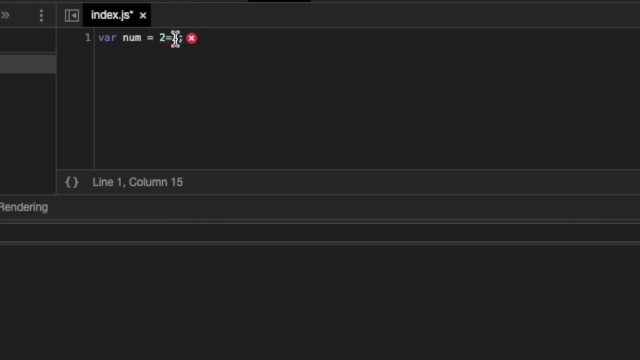 num equals 2 plus 3.. We need to close off our JavaScript here. 2 plus 3.. There we go, Get rid of that error, And if we run this, it is going to tell us That we have nothing happening. 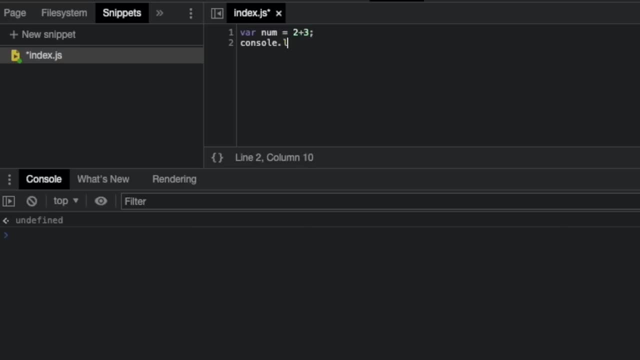 Because we need to console log this. So we go console dot log And we are going to Log the number. So this is our variable Being passed through the console log function And if we run this We get the number 5 down here. 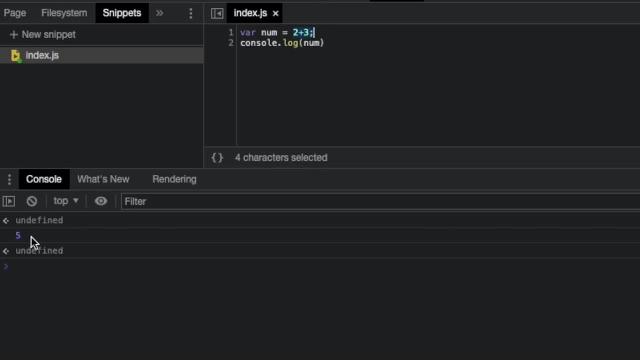 So this number contains the information 2 plus 3. Which is going to be 5.. And the console dot log just prints the variable down here for us. So we have this right here And when we run it we get our number. 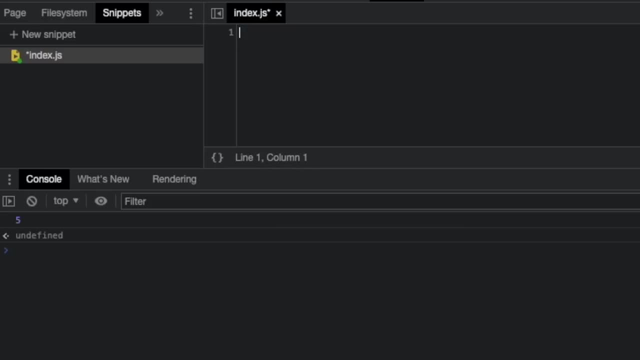 But how can we take information From the user and use it? There is a function called the prompt. If you are very familiar with cross site scripting at this point, Then you have for sure seen this in cross site scripting: Payloads prompt. 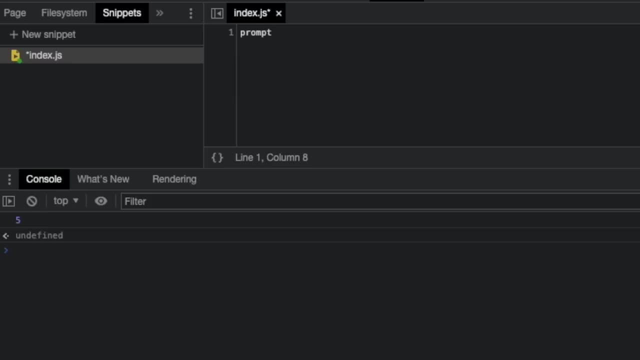 Is also another way to View a cross site scripting Instead of an alert, And so you can say prompt And then we can pass in our information here that we want, And we can say what is your name, Question mark, And we can close this off. 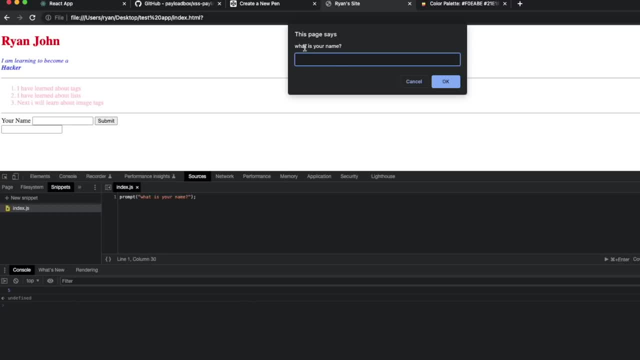 And if we run this, It should give us this little Alert here And we can say Ryan, And then it prints down here for us. But how do we get this information That we put in here? We need a variable. So, if you want, you can go ahead and pause this video. 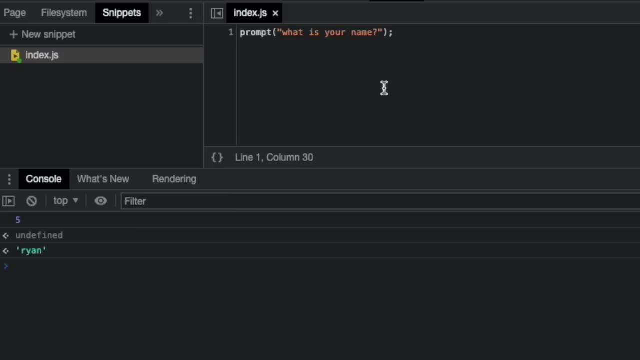 And see if you can figure out how to store this prompt In a variable called name And then get it to console log Down here What our name is Or the information that we put into the prompt, And you can go ahead and give this a try now. 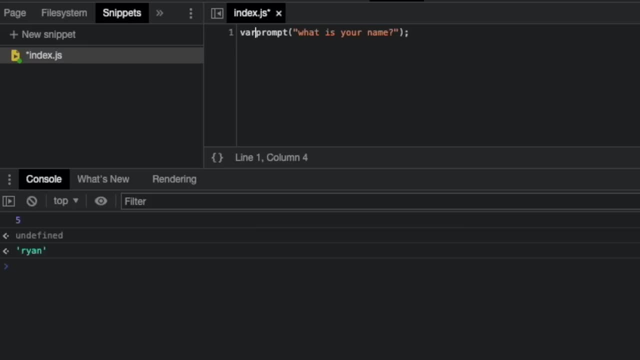 Okay, this is a pretty simple challenge. All we are going to do is change this to a var Name equals What is being put in the prompt, And then if we come down here, We can console, dot, log And then we will put up our brackets. 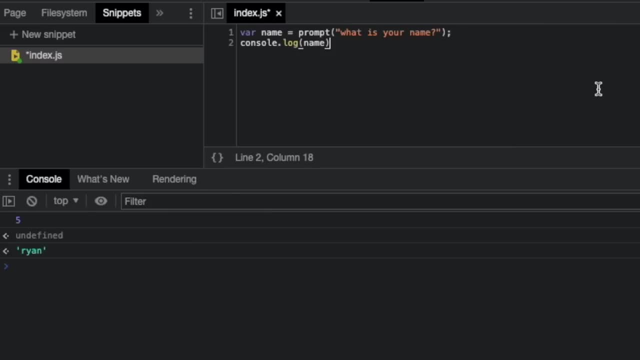 And we will say name, Just like this. And now, if we run this, We are going to get a prompt, And this time we are going to say Ryan J, Okay, and it prints out for us: Ryan J, down here for us. 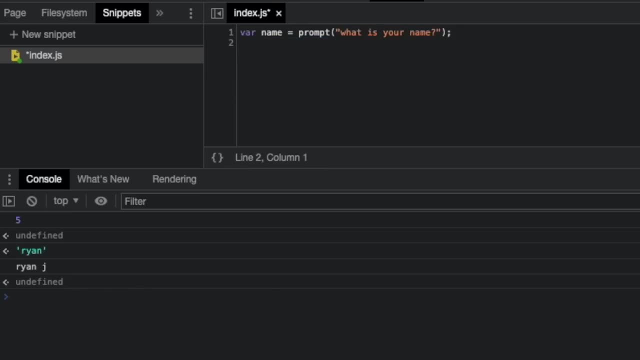 Through our console log. I am actually not entirely sure if it will print anything If we don't put the console log. It does not, But it is necessary to be here For our name to be printed, So we can try this again. 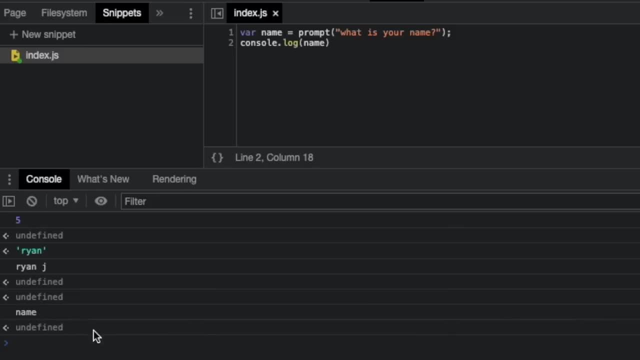 And we say name And it prints name for us. Now there is another way to go about this, Without the console log, And we could type in, like our cross site scripting That we are familiar with, And we can say hello And then we can pass in the name function. 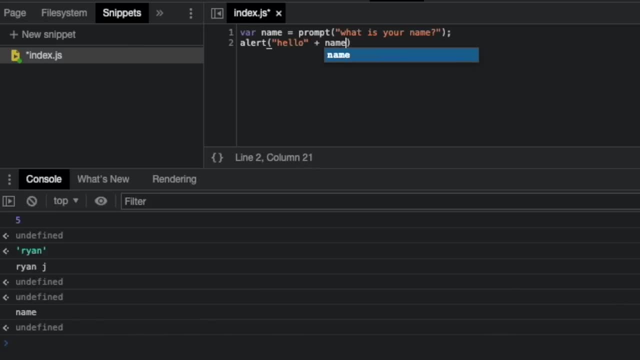 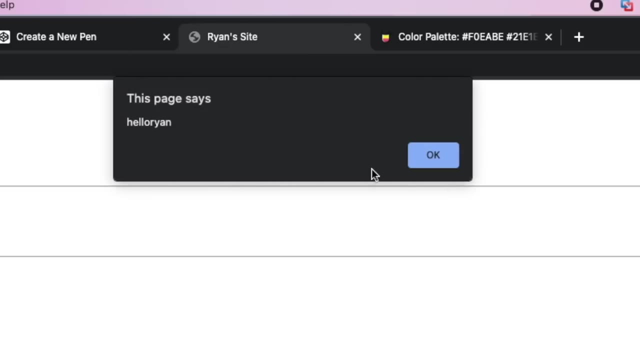 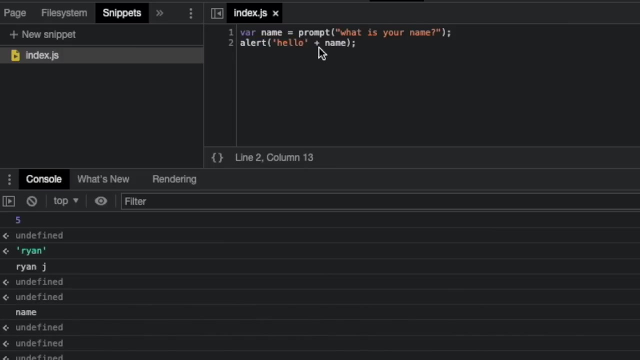 So we should be able to type in Hello plus name And if we run this And we say Ryan, We get an alert Saying hello Ryan. So this is how an alert would work With a console log. The space has to be put right here. 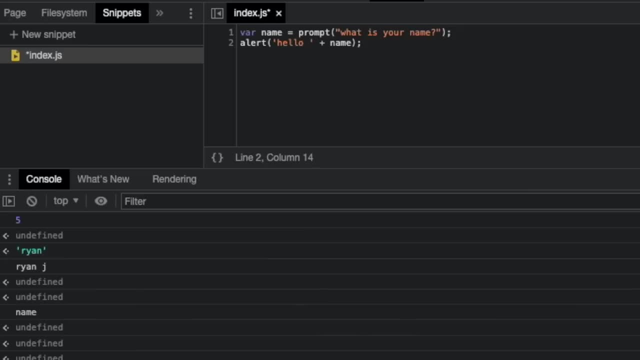 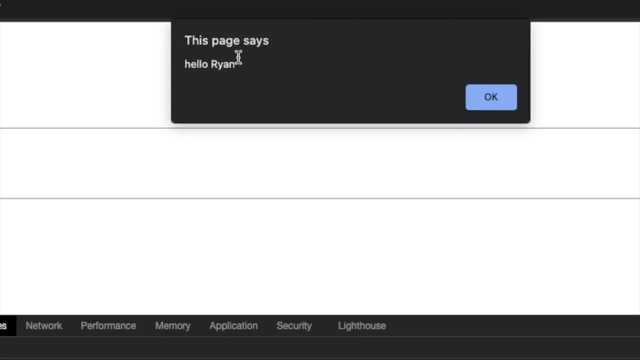 That was my problem On why I couldn't get that to space. So we just say like that, Hello space and then name, And so now it should alert: Hello Ryan, Just like that. Okay, so you just need this space in here. 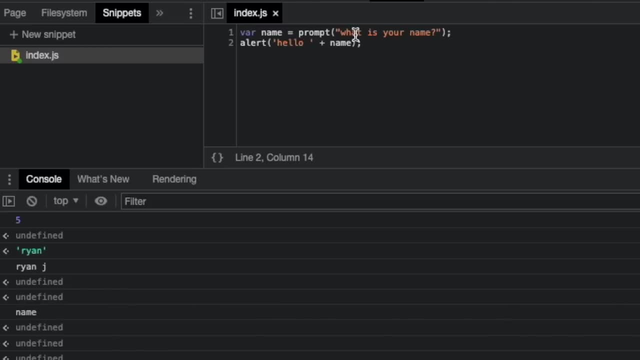 To get the space in the alert. This is a variable and a prompt, And so I want you to get used to Looking at these types of These types of variables And information. So just go ahead and play around And maybe do some simple math. 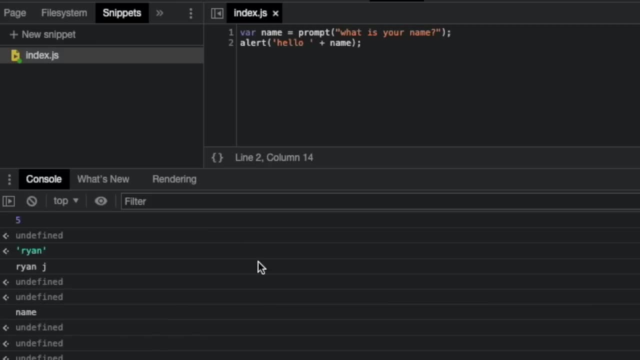 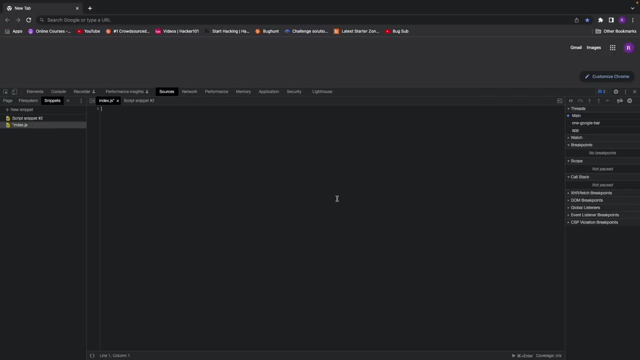 Sort in a variable, Display it in an alert. Maybe do a couple console logs Before going on to the next video. Set a way you are familiar with variables And how they work. Okay, so in this video we are going to cover the while loop. 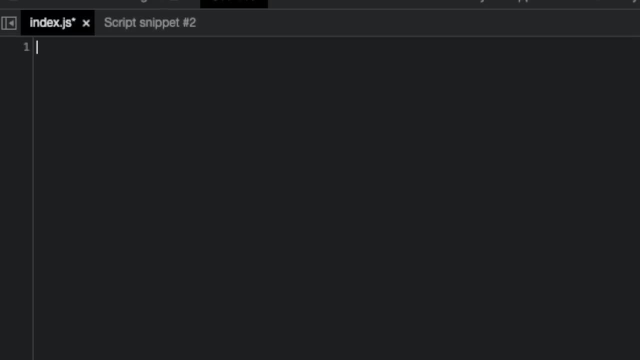 Because it is quite a bit easier to understand And we are going to just make a simple while loop And we are going to count to 100. So we can say: i equals 0. And then we will say: While i Is less than or equal to. 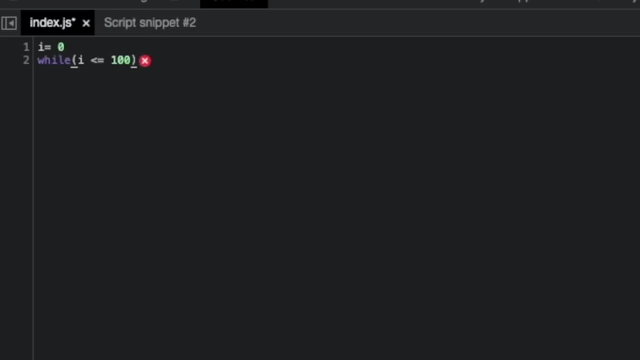 100.. We want it to do something And we want to console log i, So we will go console Log And then we will say i, So that way it prints the i for us. And the next part is very important. 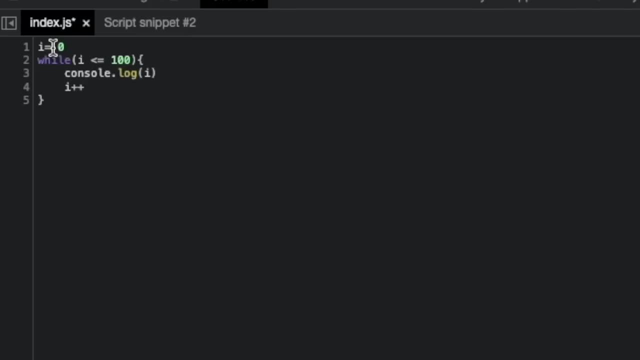 We will say i plus plus, And this will add 1 to i every time. So the first time it runs It will be 0, 1,, 2,, 3,, 4 and so on Until it reaches 100. 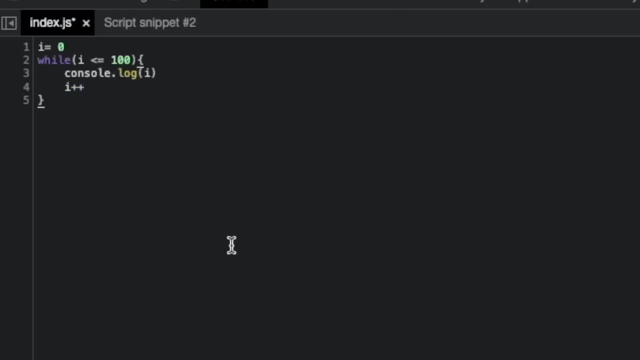 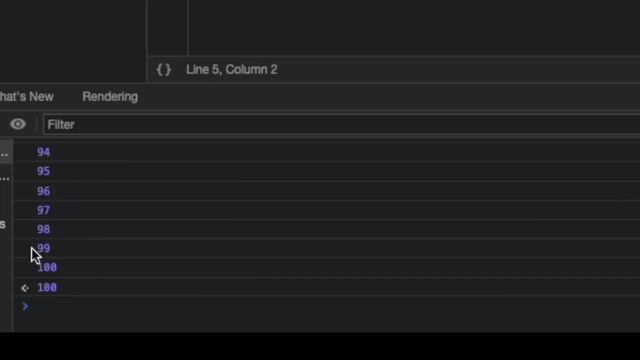 And then it will stop. If you do not have the i plus plus, You will probably freeze your computer And have to force restart. So this is very important, And so we can go ahead and run this And it prints out for us. 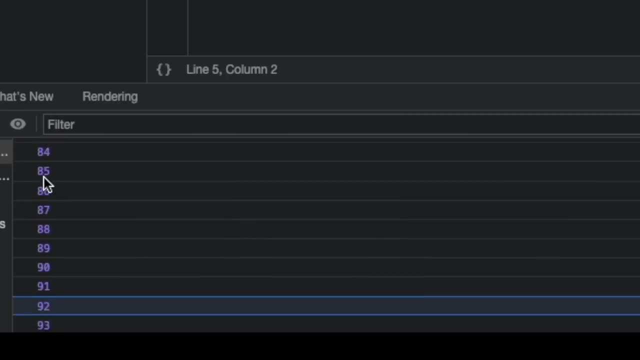 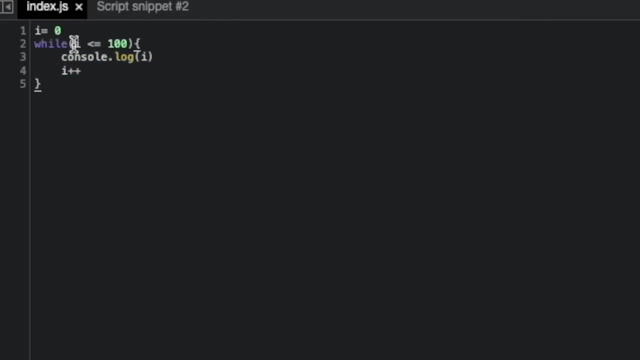 We have all of the numbers here for us, Starting with 0. It runs a function Or whatever is inside of the while loop Until it has reached The total destination, And sometimes you can Have a while loop running with Taking user input. 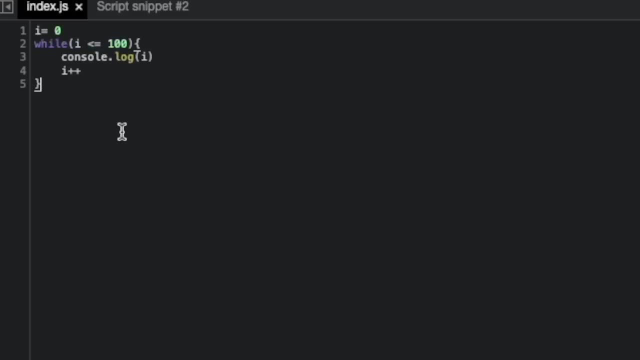 And when the user input says to quit, You can shut the while loop off. But we are not going to go into that Because i don't think it is something you need to know In order to be an ethical hacker, And with that we will move into. 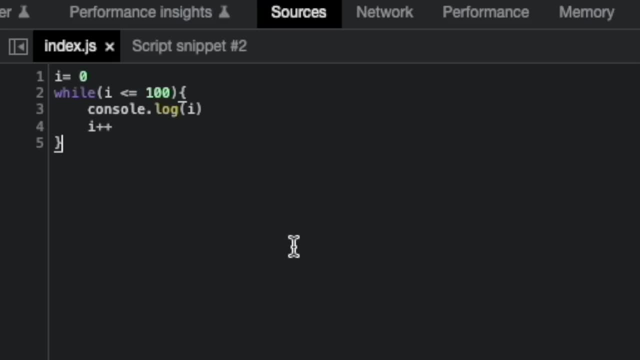 The for loop. Okay, so the for loop Is a little more daunting and scary, But it really isn't, Once you understand how for loops work. So if you are coming from another programming language, For loops are really simple, But in javascript they are a little more difficult. 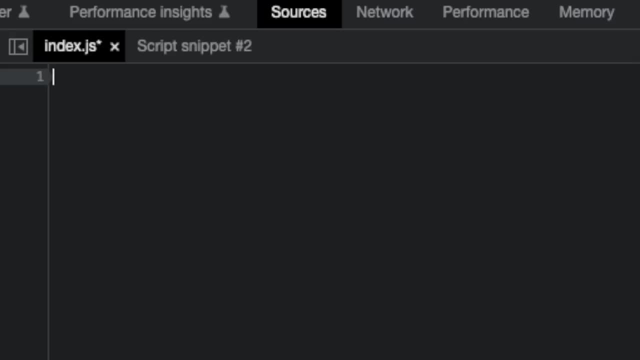 Because javascript is the language of the web. It is not made to run for loops In a simple manner like python. So if we run a for loop And we are just going to run a simple counter, Like we just saw, We can say something like for: 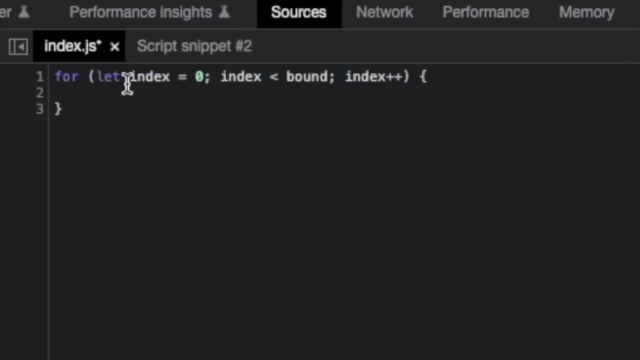 And it is going to ask us: do we want to run a for loop? And it gives us the boiler plate for A for loop. So we will just leave this index instead of i, And so we are just going to say that i equals 0.. 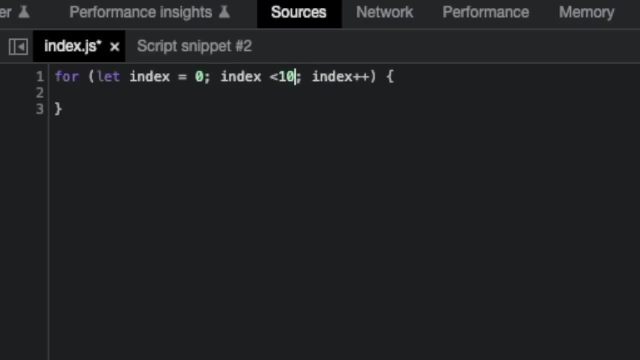 And as long as it is Less than 100.. We are going to go ahead and say i or index, in this case Plus, plus, And then we can just console log this And then we will say index, Just like this. 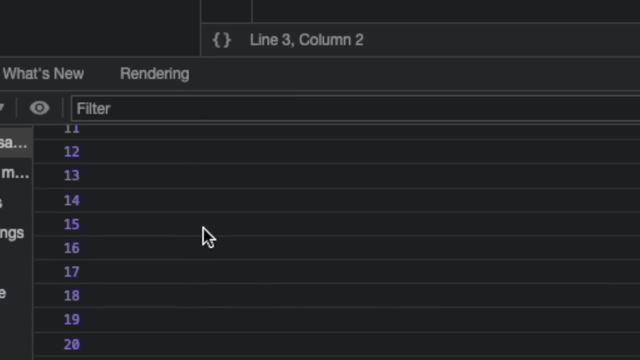 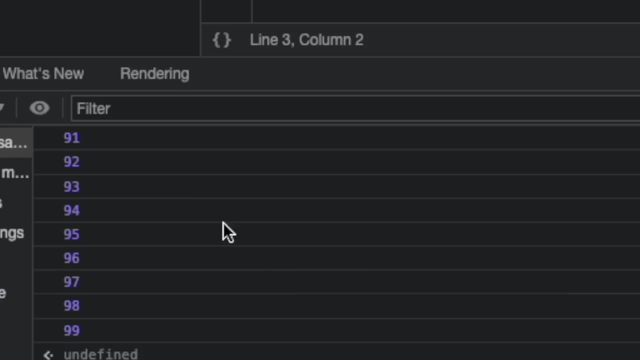 And now if we run this, We are going to get an output down here Of counting to a specific number. And just to demonstrate this with you, If I go over here in the world of programming, I almost always use for loops. I rarely use while loops. 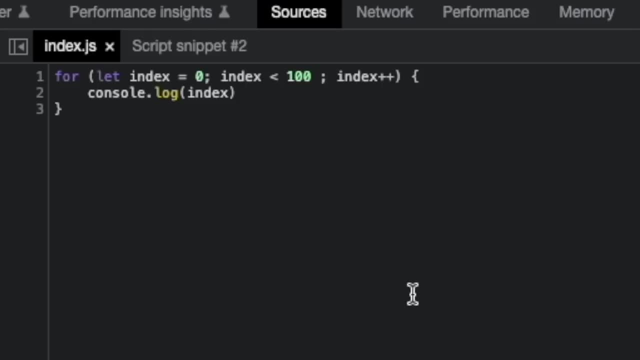 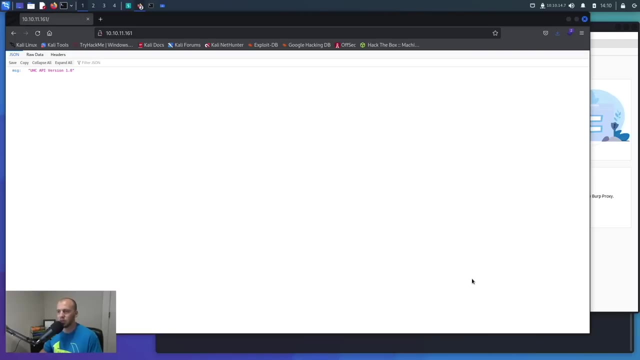 But i just wanted you to see these for loops And while loops So that you can read them When you are looking through javascript code for vulnerabilities. And, once again, I just want to show you how to enumerate API's, Because this is something that is not covered in any courses. 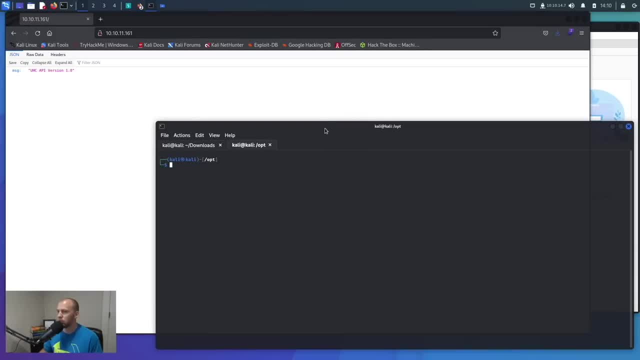 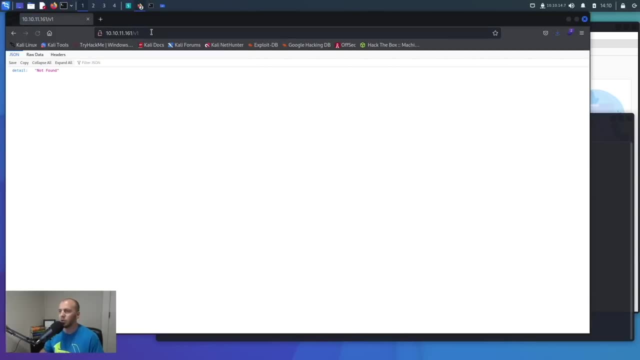 Or any certifications That i know of. So if you come into your terminal And you have an API like this, you type in like v1, or you're typing in basically anything. you're just trying to figure out. how do you get further down the line? you're looking for endpoints, the tool i like to use for api fuzzing. 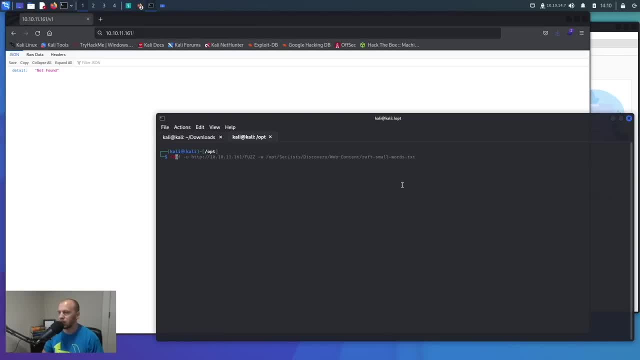 is fuff, so it looks just like this: if i can get here, buff, there we go. and i actually ran this just to make sure it was going to work before i did the video. so i like to run fuff, and then you give it the url and this is the api, and then we're going to be fuzzing for an endpoint, and then you 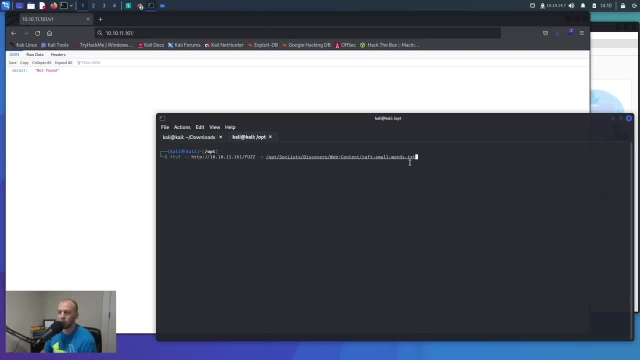 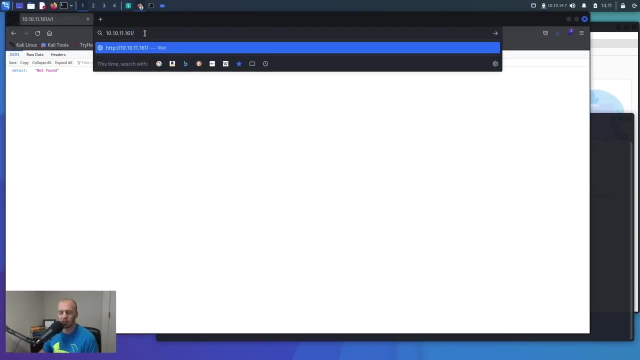 give it a word list that you want to use. go buster and derb and a lot of those- your usual fuzzing tools just don't work with api. so i like fuff, because it does work and you run this and you see it pulls down docs and api. so if you were to do this like in a live program, you'd come in here. 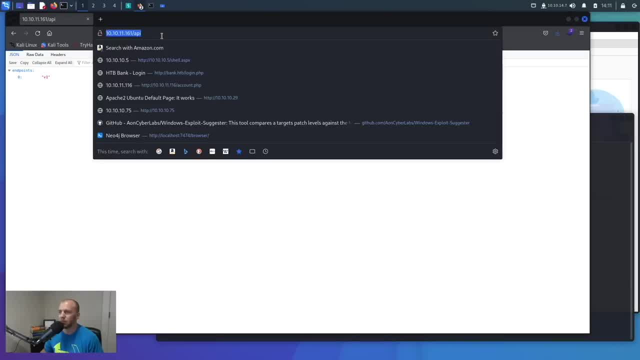 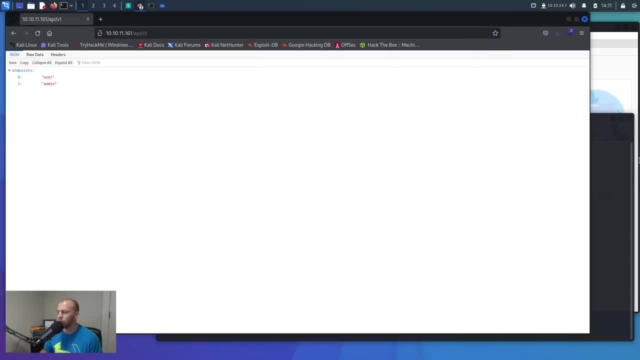 and you just type in api and then it says we have v1, so you can just type in v1 and then you'll have user and you can kind of see. if we wanted to look for more endpoints, we could just close out of this and we would just move our fuzzer over, so you would just go. 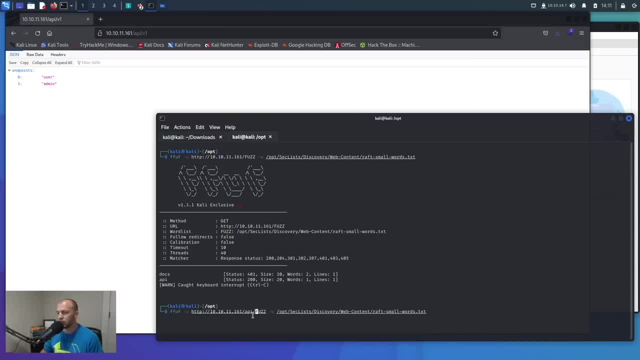 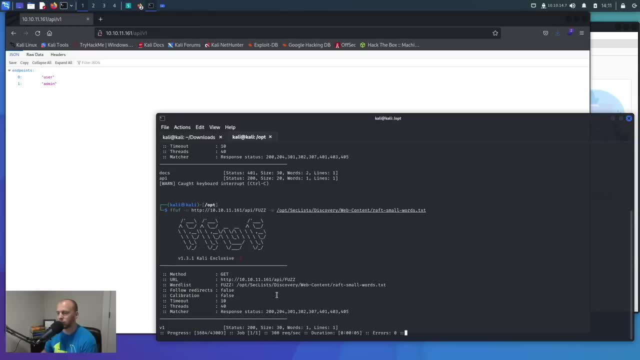 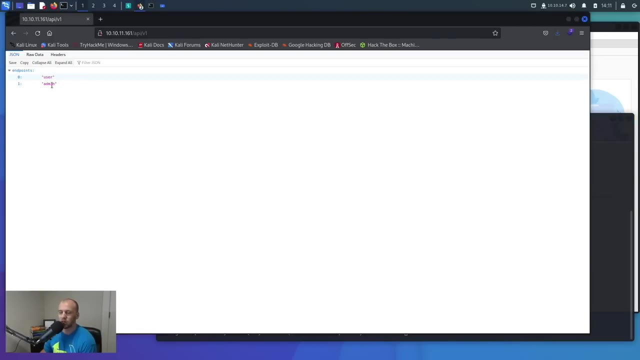 like this and then it would fuzz right here and it would look for more endpoints over on this point. so that's how this fuzzing apis work. if you're interested, you can go ahead and do the box. hack the box. it's actually really simple. you just create a username using the api. 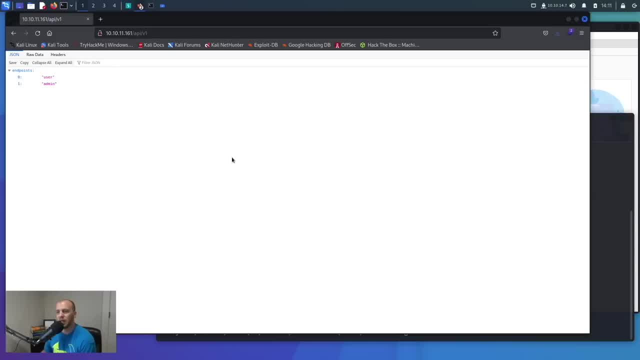 so you'll use burp. you'll just intercept the request and it'll send you back a json of what you need and then you can make, turn your request into a post request and make a username and password and login. so this is api fuzzing. you'll see these on bug bounty programs and sometimes. 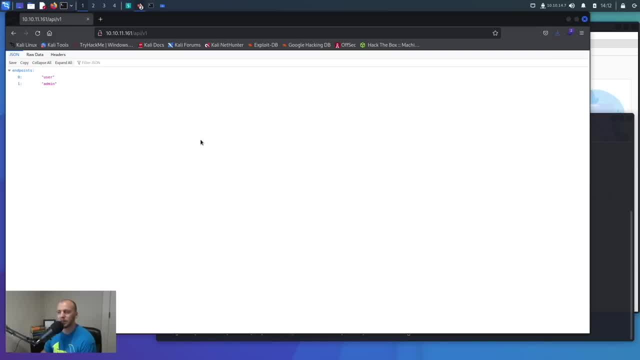 you'll come across them in hack the box machines, but this is something that's not really covered, so i wanted to make a quick video on api fuzzing and bug bounty. so sometimes you can find an api and api url like this and you can just start fuzzing away and see what information you can come back. 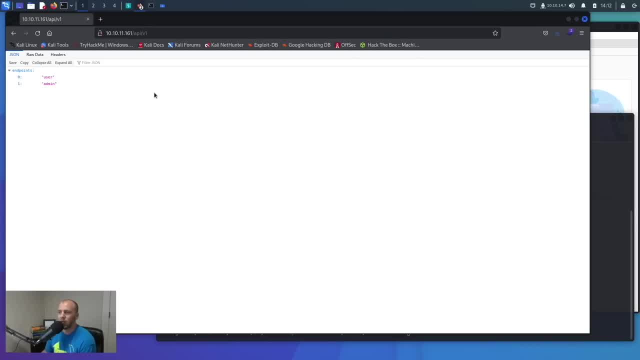 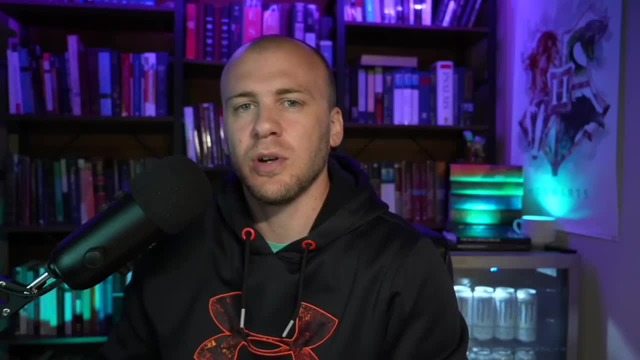 with and manipulating the request, so that is api fuzzing. we're going to cover server-side request forgery. purpose of this video is to show you what is going on inside of server-side request forgery and walk through a couple of examples so maybe you can understand what is happening. so the way 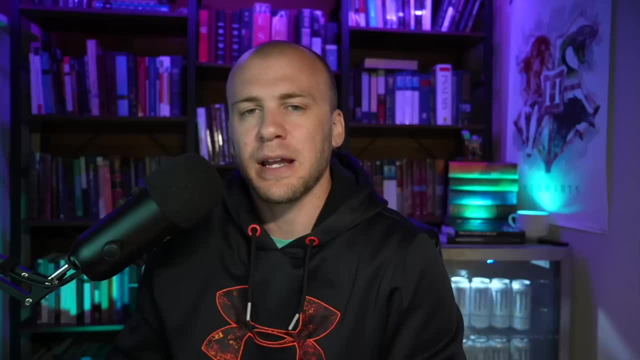 we're going to go about this is i'm going to show you a flow chart, and the flow chart might not make sense in the beginning, but i want to show it to you so that way you kind of see what is happening. and then we're going to walk through two different examples and then come back to the flow chart and 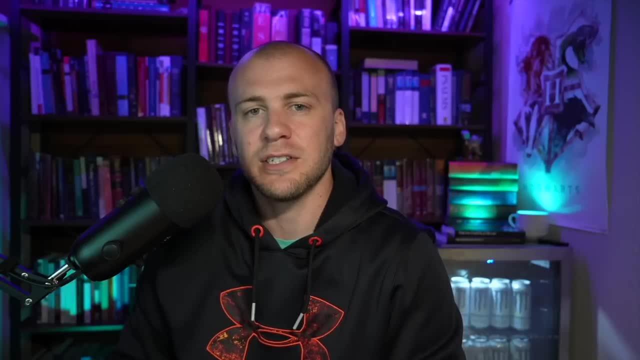 at that point, the server-side request forgery should make a lot of sense to you and you should be able to start looking for these bugs as you are browsing through programs, and you'll be able to submit a proof of concept that makes sense to the person who receives your bug report with that. 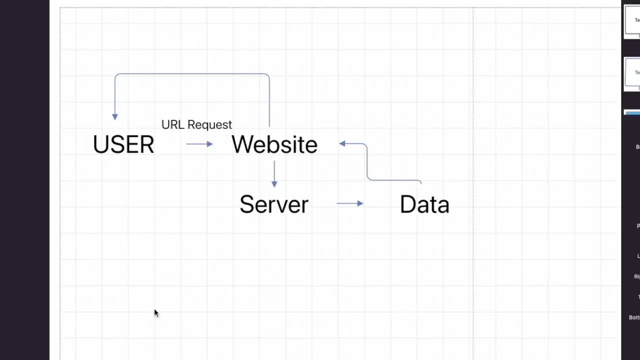 let's jump into it, or with a very simple basic flowchart. i tried to make it as simple as possible so that you guys could understand exactly what was going on inside of server-side request forgery, what's going on, and that it wouldn't be too busy with too much going on. so this would be. 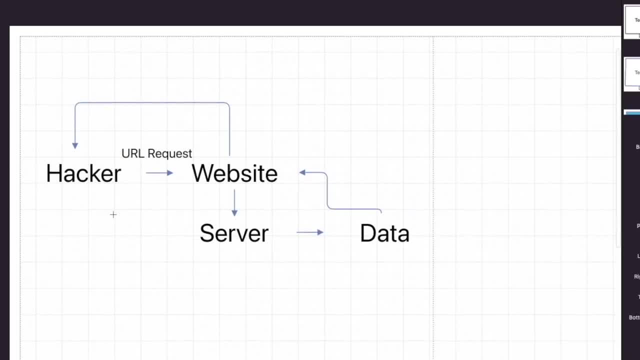 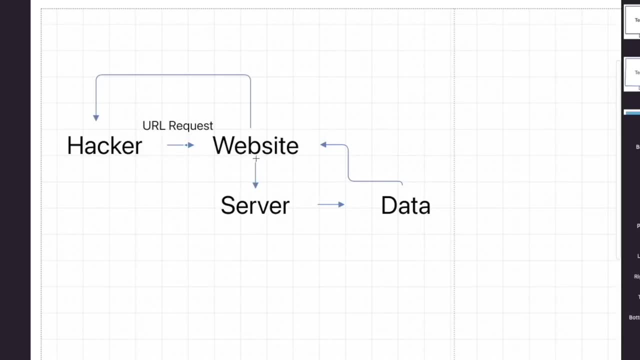 us, the user, and you can also change this to the hacker or the attacker, and so the attacker sends a url request to the website. so we're manipulating the url, and then the website makes this request that you weren't supposed to be able to make to the server, and then the server sends the data back. 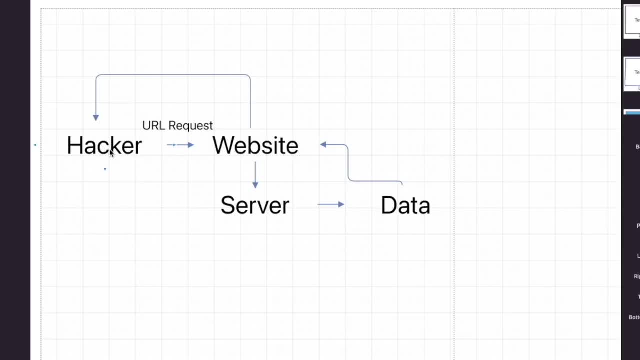 to the website and then you can view it as the attacker. so this is how the flow works. if you were a regular user, we would just have user here and you would send a request, and it's just as any request that's going to the website and the website would pull the information from the server. 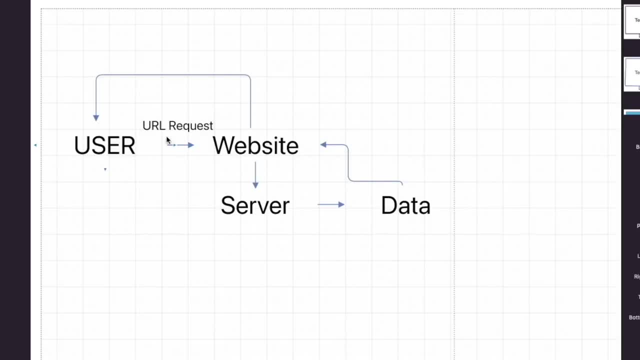 and the data would be sent back to the website and you would see the request that the website made to the server. the problem with the server-side request forgery comes in when you have the ability to manipulate this url request. so let's say it's the url wants to reach back to the home or root. 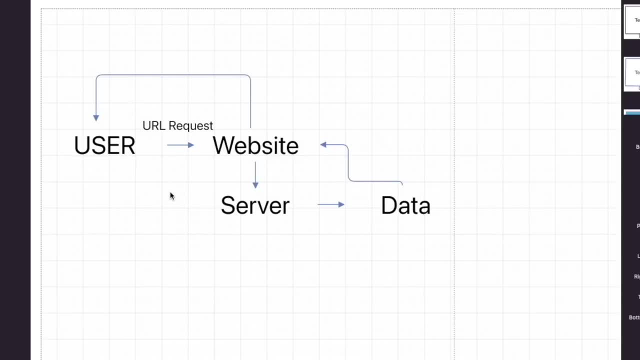 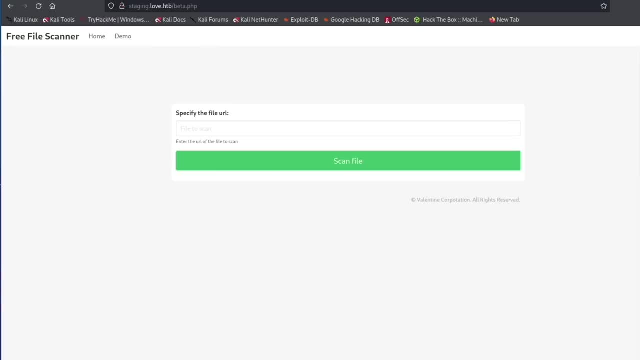 directory and you're able to file off of the server instead of the actual directory right here. so with that we're going to go ahead and move into an example. so we are going to be using this example from love on hack the box. i'm not going to walk through all of the recon and what gets you to this point, but rather just 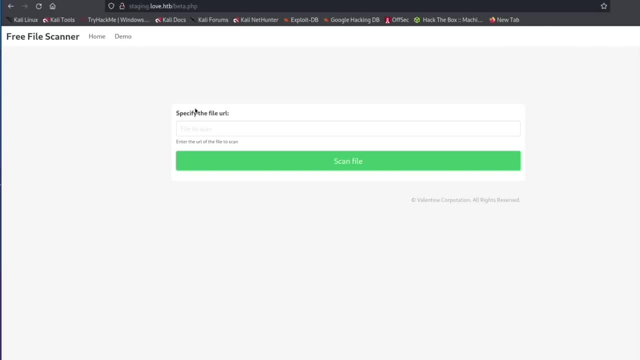 what is going on with the url. so in here we have the web application that's going to reach out to the server through this url form right here, and if you're ever doing a ctf or any kind of certification and you see something like this, this is a dead giveaway. 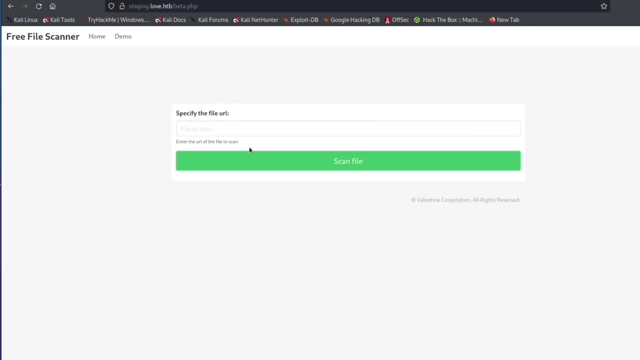 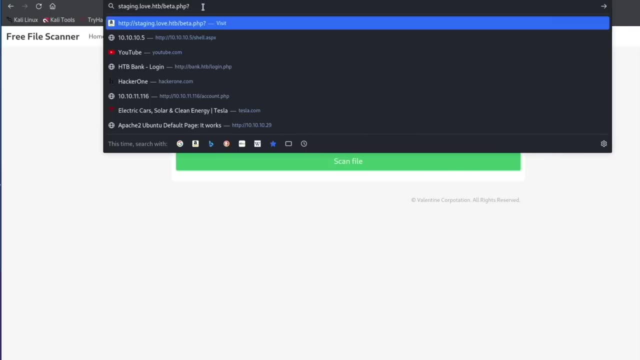 that there is a server-side request forgery anytime you see a url right here, but most of the time the url is going to look like this up here and you're going to have something like this, and then it will pass in a parameter like a url equals and then it'll have a file right. 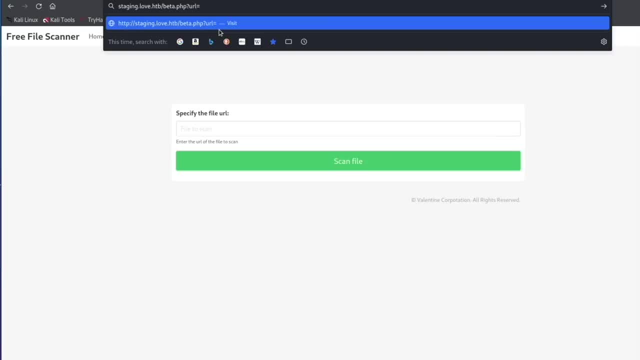 here, such as the root directory or some kind of file, so we could just put in here some file and then what you would do is you would manipulate this right here and you could pull down files a different way, but instead of having it right here in some 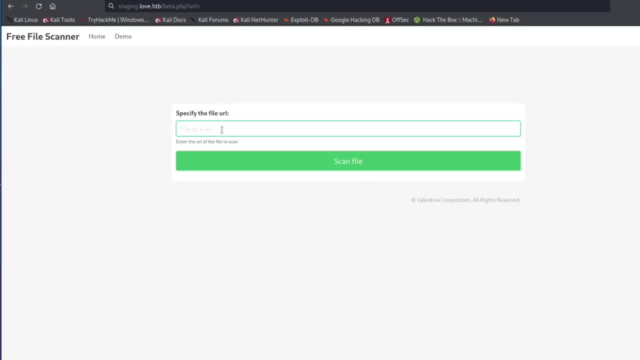 of the url. this web application has it right here and because this is an easy box on hack the box, that's probably the reason they put the url request down here in a submit format instead of being in the url, and you have to deal with it inside of burp. so this is how you're normally going. 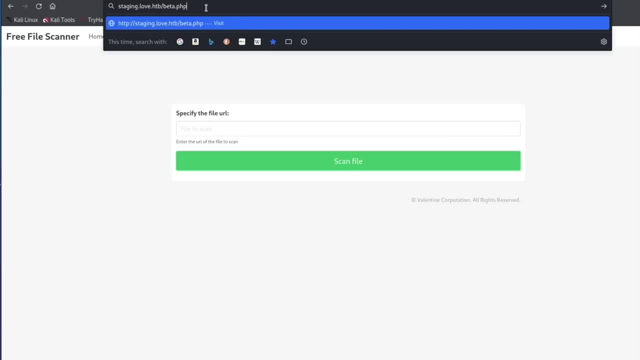 to see it. it'll be up here in the url, something like this. and in the next example we're going to see it's also not going to be up here, but it's going to submit a url request and we'll be able to see it in burp and we'll be able to manipulate it just like we would up here. only we're going to 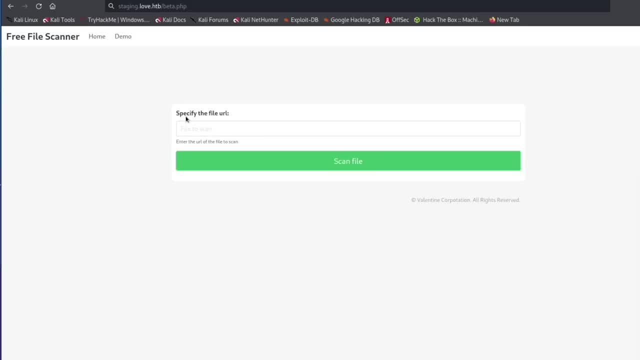 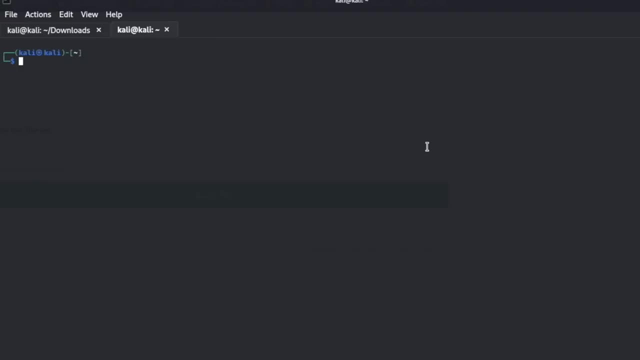 do it in burp. so inside of this file scanner right here on this, hack the box. if you ever want to test a server-side request forgery, it's pretty simple. you can just come over here to a terminal and you can set up a netcat listener on port 80. and it needs to be on port 80 because it's going. 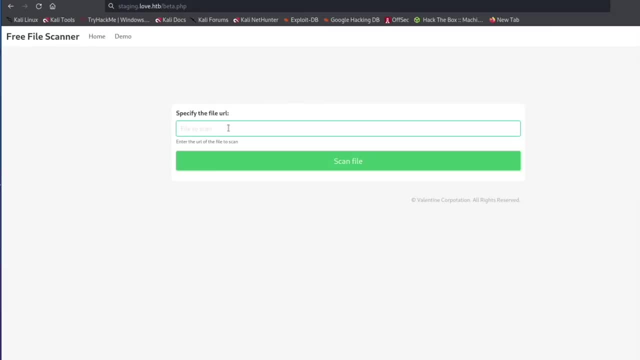 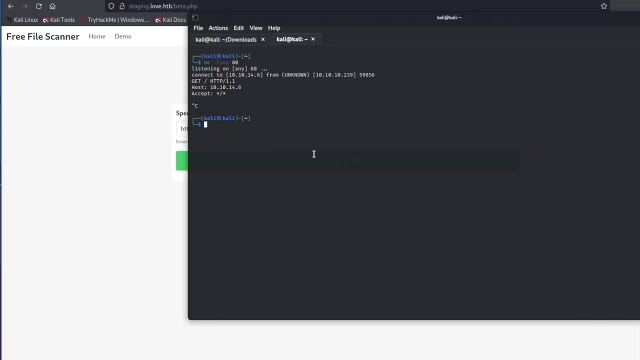 to have to go through the http protocol over here. you would just type in something like http right here. this is my vpn with hack the box, and so we can hit scan file. it's going to hang for a vpn. we can cancel it, or you can just come over here and cancel out of this. you can see that it. 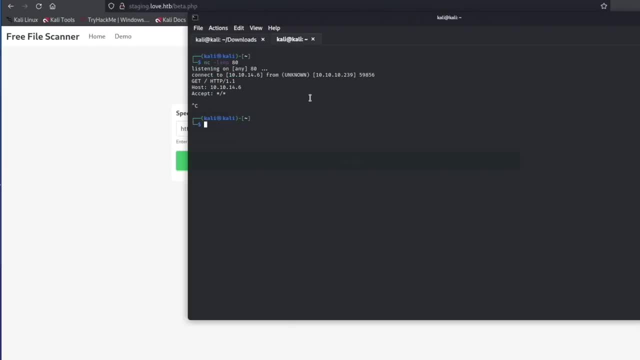 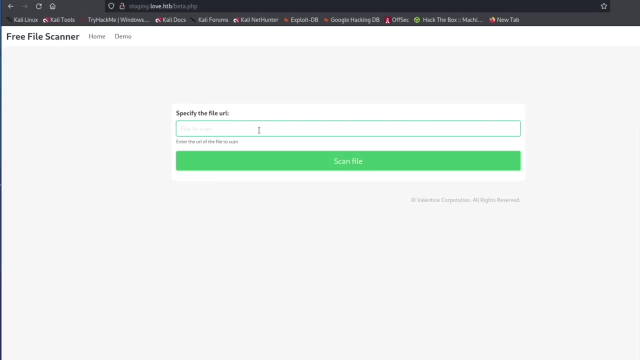 reached out to my little netcat listener here on port 80, and so we know that this is trying to grab a url, and you can check to see if it's grabbing a file from the server by typing in the actual ip address. so in this case, for this hack the box, the ip address is http slash and it's 10 10, 10. 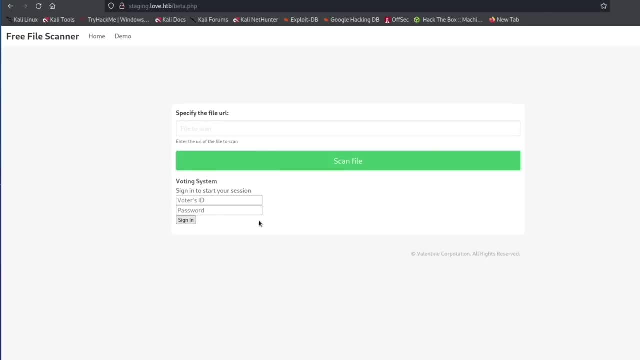 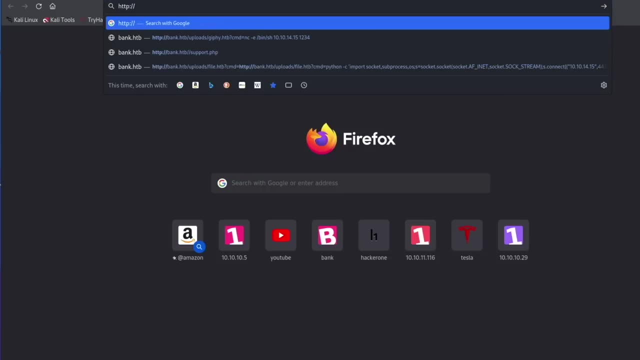 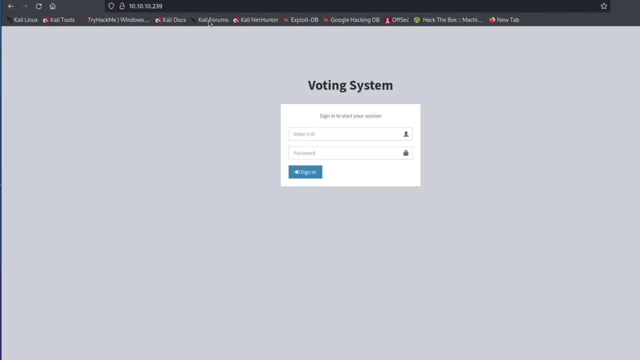 just like this, and if we scan this, it's actually going to bring back the web page right here. so if we went to this ip address right here, we said http, and then we said 10, 10, 10, 239, and then we come here, you'll see this voting system right here. this is also on this server, so i actually had to. 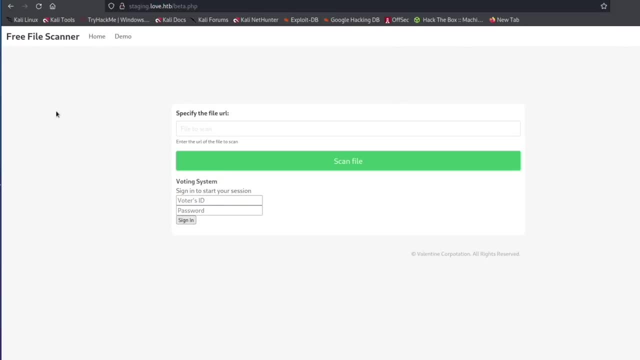 add this to the etsy host file. and if you're not familiar with that, what that is, that's okay. so, because we're able to pull down this voting system by pointing this machine to itself, we know that we are able to pull information from the server, and i want to show you why this is so bad and it's such. 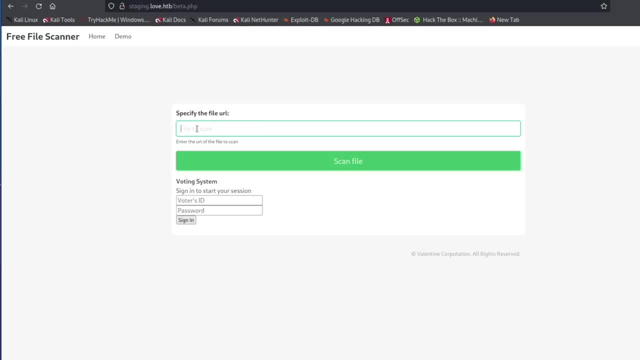 a detrimental vulnerability, because if i were to come in here and we scanned and we searched through all these files, like you would, in order to get remote code execution on this box, you can grab files off of this server and in the case of this specific box, on hack the box, you're able to. 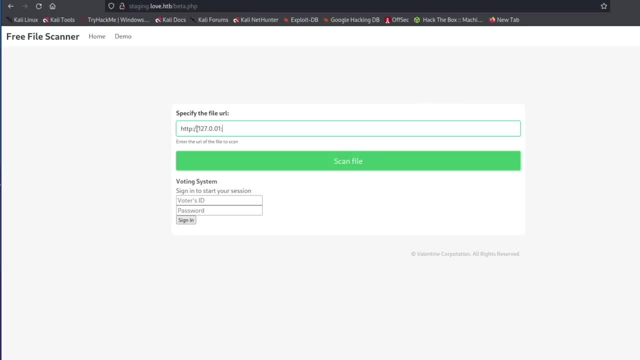 grab a password file so you would have to go through and scan the network. but just to show you we can grab. so this is the local host and it's on port 5000 and we can hit scan file. i was missing this dot here. we can hit scan file and it's going to pull this information from the server and it's. 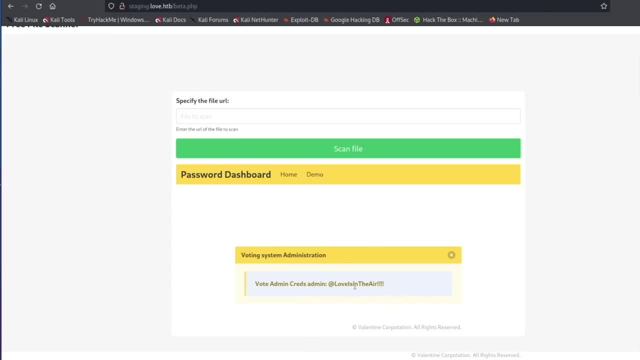 going to tell us that you have the credentials for admin right here, so this would probably be the admin, and then then you have the password right here. so this is why server-side request forgery so bad is. you can pull information that you shouldn't be able to access from the file, so 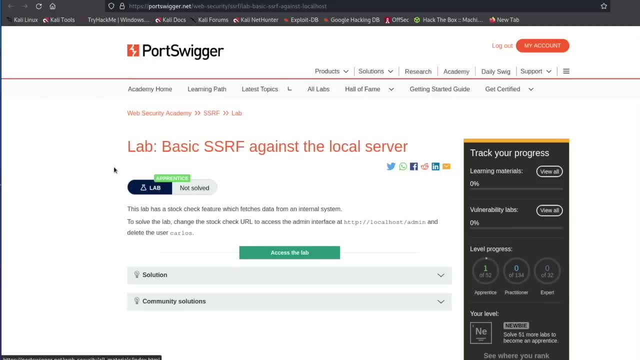 we're going to move on to port swigger right here and they have a basic ssrf against a local server. it's going to tell us to solve this lab. we're going to change the url access of the admin interface at this location and we're going to delete this user right here. so let's open up. 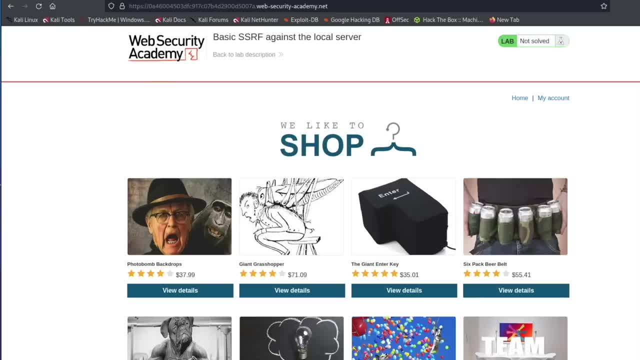 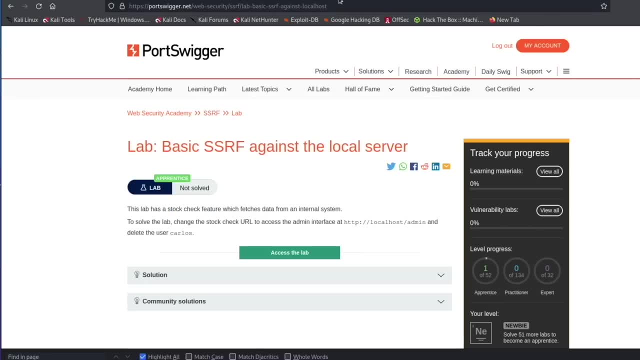 the lab and the way we're going to go about solving this is. i forgot where it told us this is located. i think it said inside of a check the stock feature. so if you come over here and we open up burp, we can turn. actually we need to be inside here. 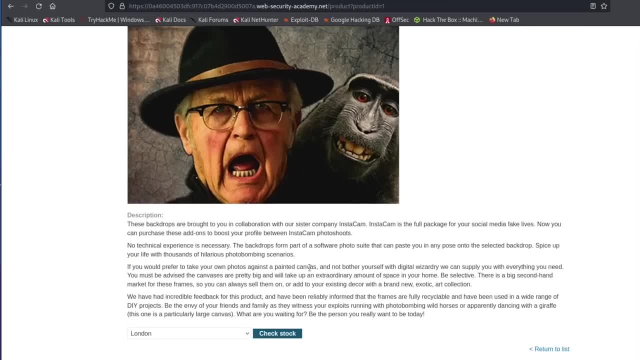 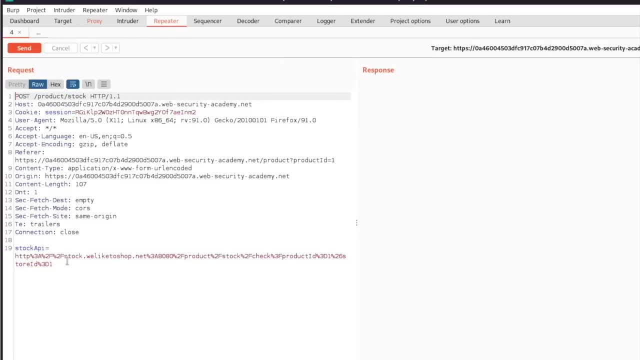 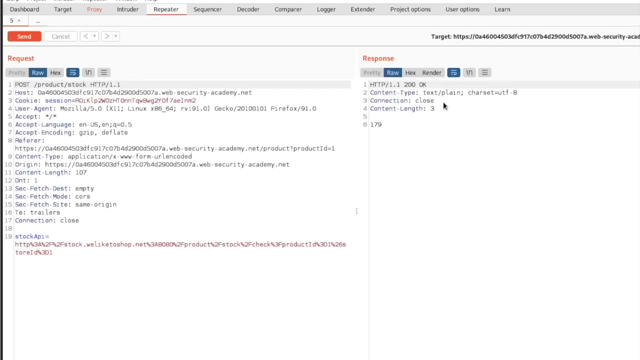 now we can turn intercept on and we can check the stock and we'll send this to repeater and then we can just turn this off. okay, before we change any of this, we're going to send this to repeater so you can see what we get back. this is the normal request. this is what we. 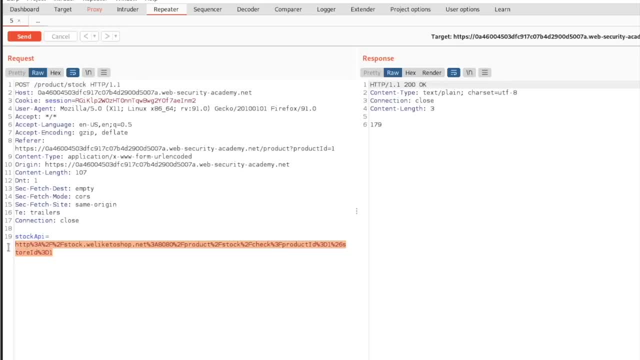 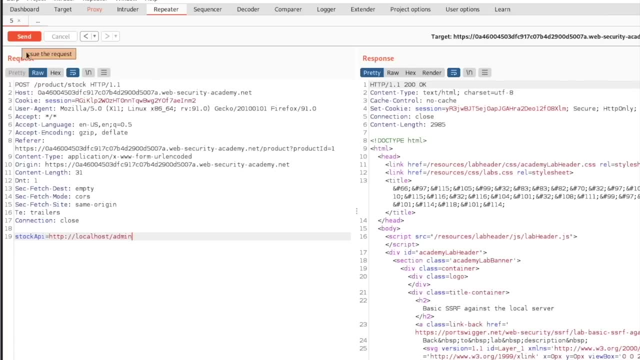 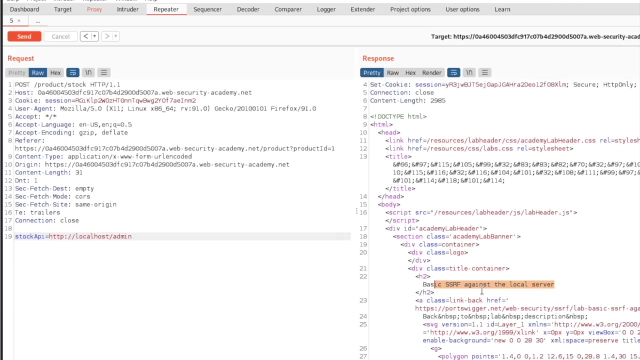 get back. we get back a response of: okay, but if we just delete this whole thing right here and we local host and then we go to the admin and we send this, we're going to get back a different page and we're actually told that we've reached the basic srs, ssrf against the local server. 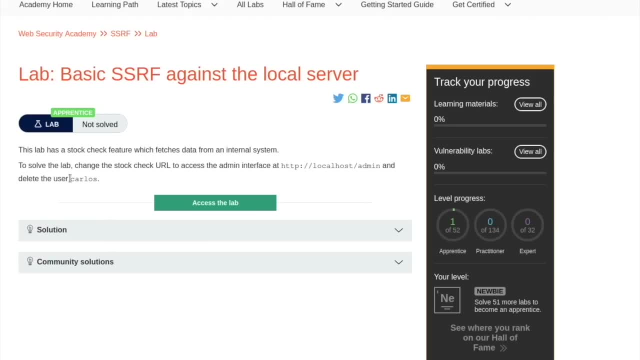 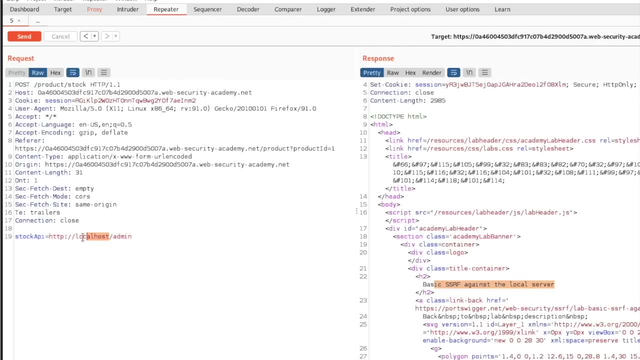 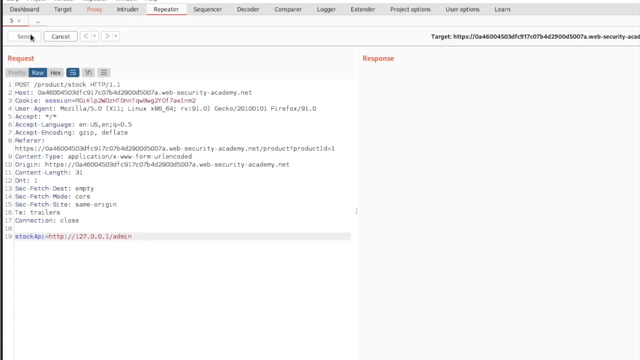 and i think we're supposed to actually delete the user carlos right here, and so the way we would go about doing this actually, before we delete him, i want to try something, just because i just showed it: we can go 127.0.0.1 and this should send us to the local host as well. 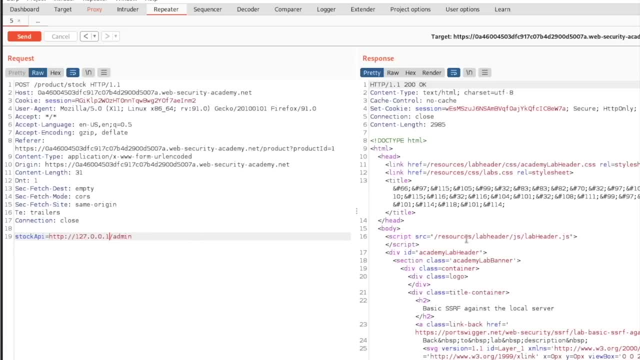 see if we get back the same thing, and we did so. this is what we would do- is you can type in local host right here, or 127.0.0.1, and then we're on the admin page. now what we need to do is delete. 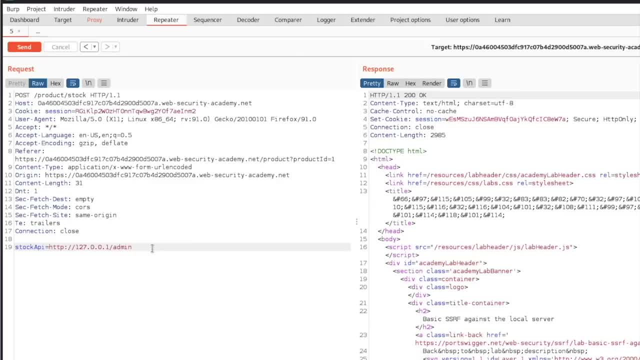 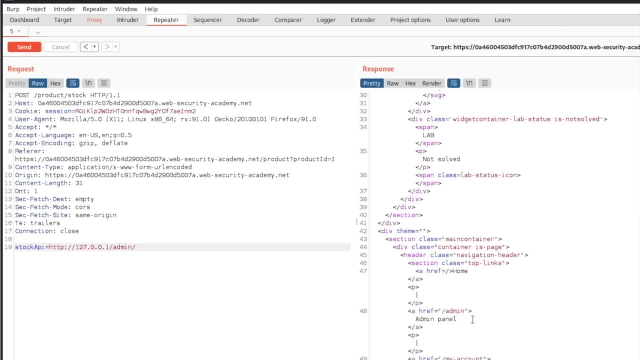 the user carlos, and i'm guessing this is supposed to be done from the admin panel. i suppose you could read through here and maybe it might tell us what we can do from the admin panel. oh, it tells us right here. it says we need to delete the user carlos. so you can actually just copy this right here. look, it says we can. 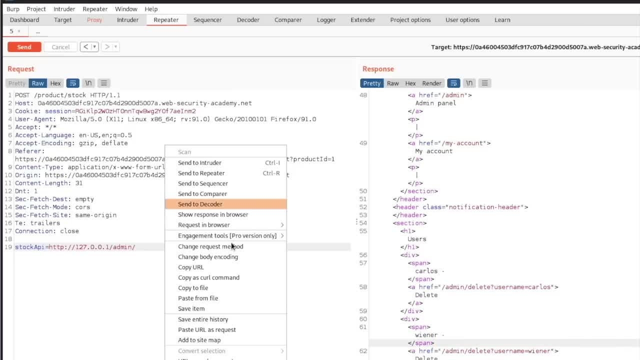 delete these users. so it actually tells us we can delete a bunch of users and we can paste this in here: um, we got too many admins going on. we can delete that all the way back now. if we hit delete, this right here should pop up to solved. so if we send this, it tells us: 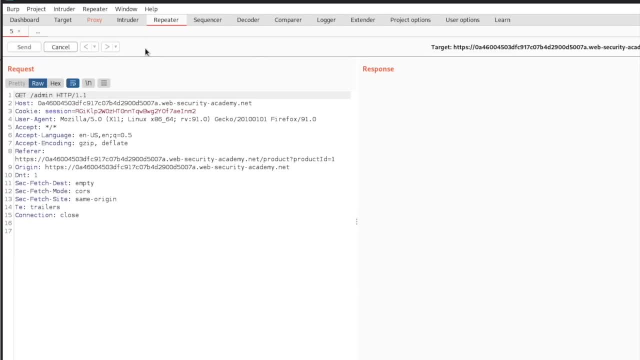 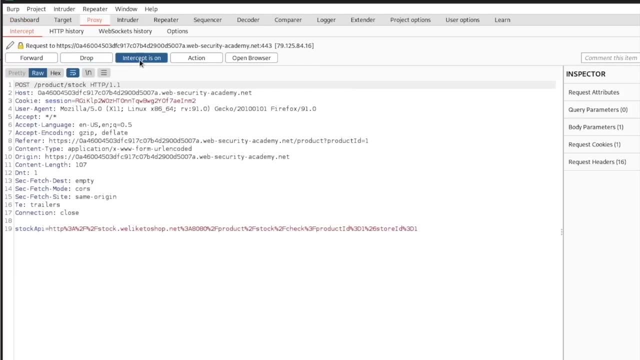 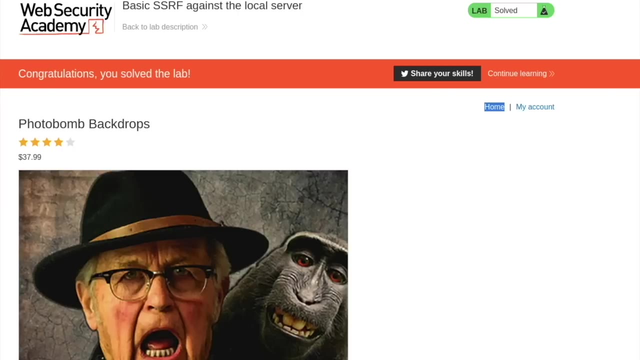 not found. i think we have to follow the redirect, turn the proxy off and it tells us that we have deleted the user carlos. so this is how a server-side request forgery works, and i want to walk you through this one more time. so i want to bring you back to 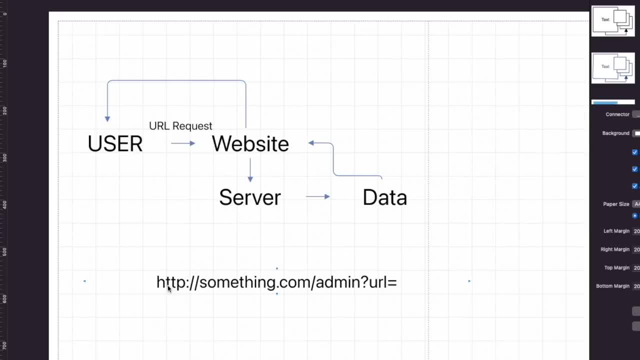 this flow chart right here and now. you understand that what we're doing. when we we are the user and we make a request through the url, through something like this, and let's say we want to get a file, you would do this right here and if you were on a linux machine. 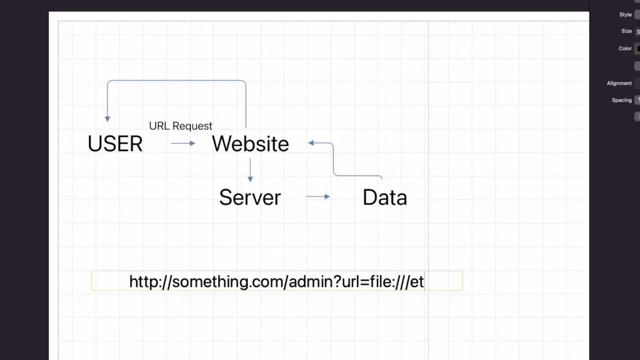 it would look something like this and you could try and pull down the etsy passwd file. actually not sure if there's supposed to be a colon there or not, so you can google and check that. i can't remember, but it would be something like this: to pull down the etsy passwd file and on windows. 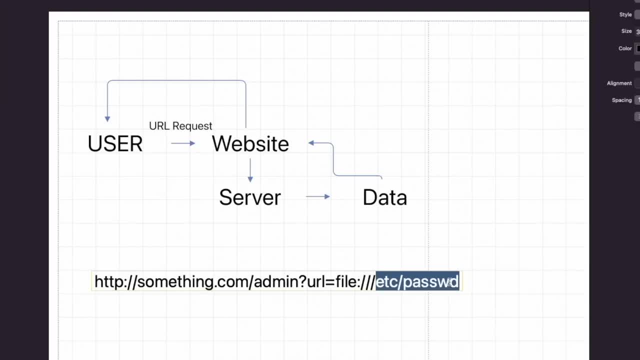 you're going to be trying to pull down some kind of windows system file that would just be on the server to see if you can get files. but you wouldn't do this necessarily in a proof of concept. what you're going to do is like i showed over here with opening up a netcat listener and then 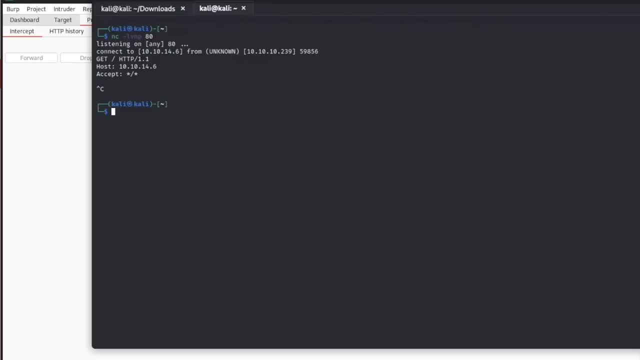 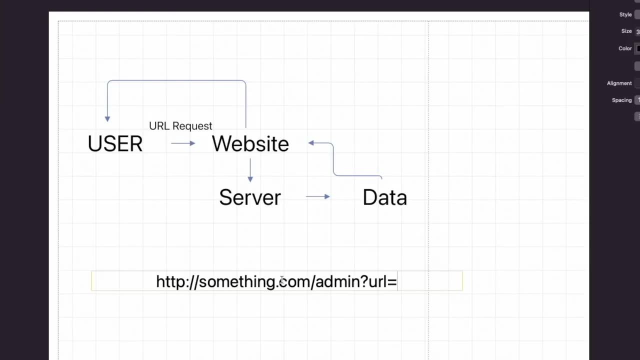 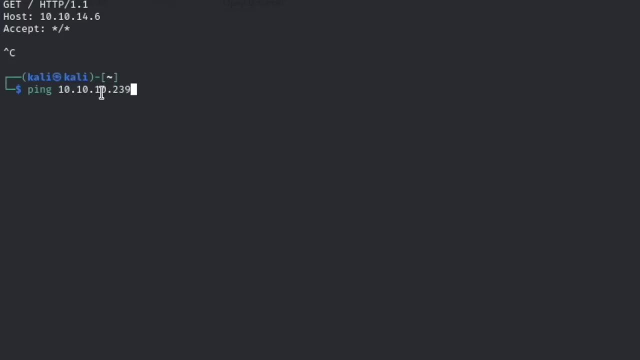 making a request to the url, which is going to be your own ip address right here, to see if you get a connection back. a quick tip to see if you're trying to figure out what the server is, if it's linux or windows and you want to know what kind of file to look for, you can actually just ping the server and see. 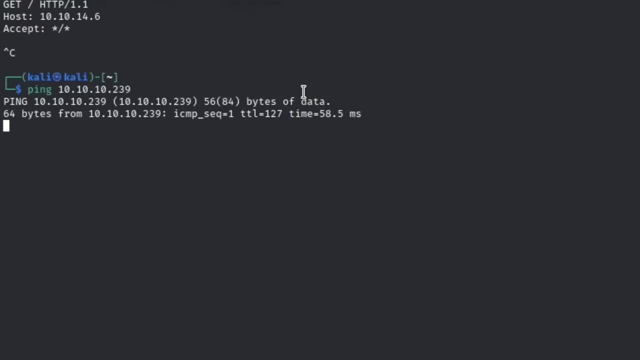 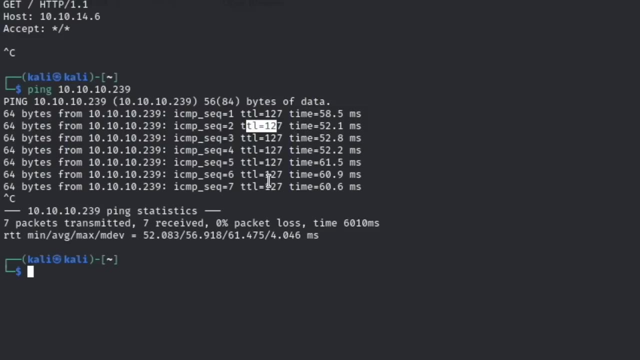 the hack. the box is a windows server and it's 239. whenever you see this ttl of a 127 or 128 or something in the 120s, it's going to be a windows server, and when you ping a linux server, it's going to be somewhere in like the 65 range, and that's one way to tell what kind of server you're going. 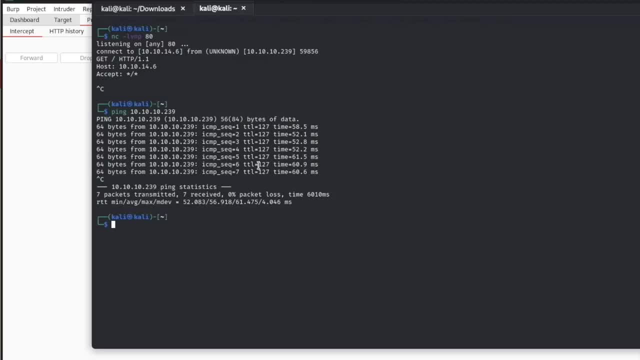 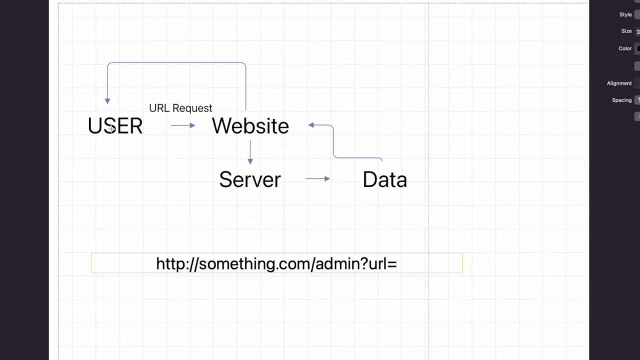 up against. you can just really simply it or you can run an in-map scan and it will tell you, but this is server-side request forgery. in a nutshell, you're going to make a, you're the user and you make a request through the url to the. 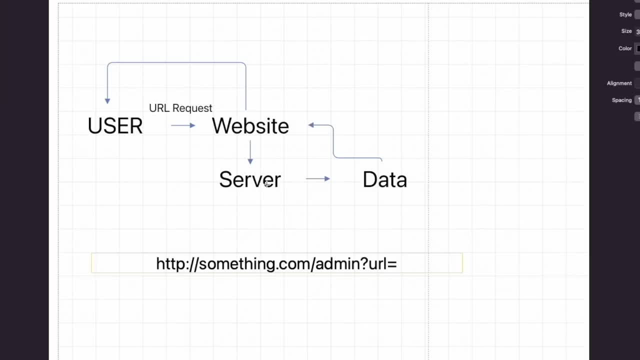 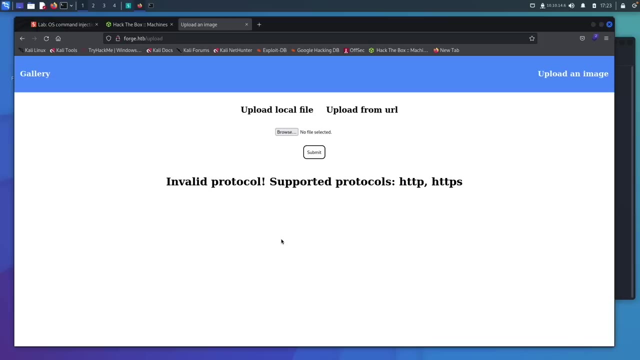 website and then the website requests the url from the server and the server sends the data back to the website and then you're able to view it as the user, and if you are able to manipulate the url request to the server, you can grab files from the server that you shouldn't be able to access. 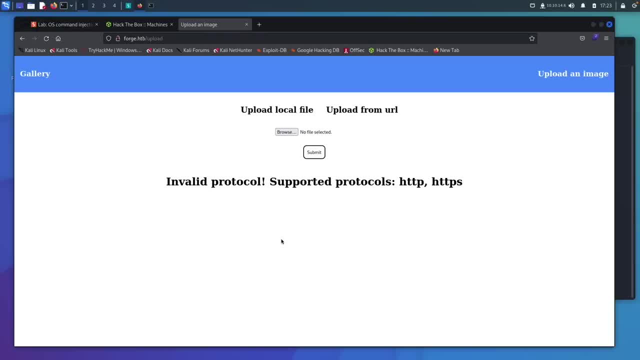 okay. so before we move on from server-side request forgery, i really wanted to show you one more thing that you might come up against in the future. so we're here on forge from, hack the box and you have this upload from url and i'm not entirely sure how it's going. 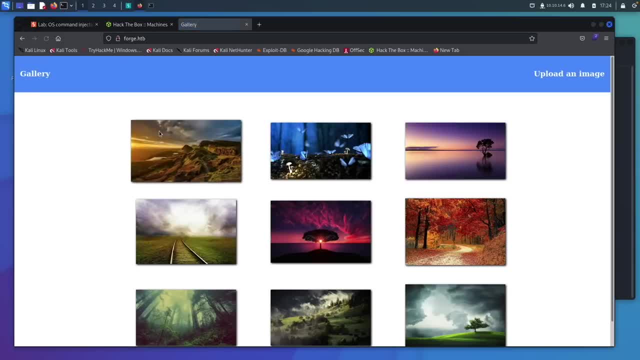 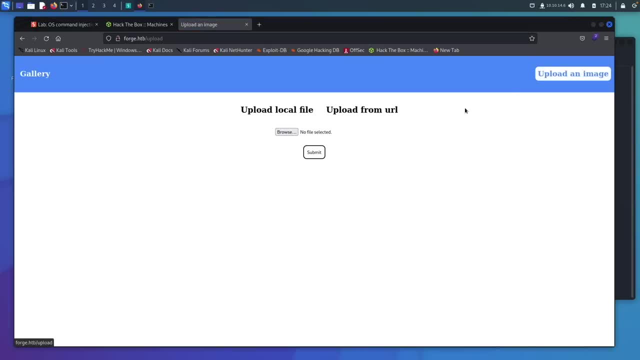 out and grabbing the url or an image from the url, because this is apparently a gallery website and you can post images to the website, so we can we have upload an image. you can upload through the browse, like like this, or you can upload from a url, so i imagine it's doing some kind of wget or something. 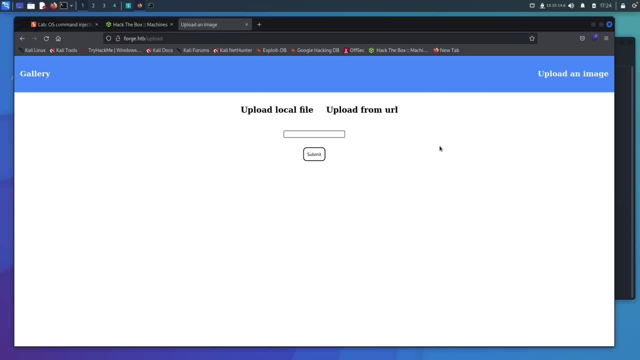 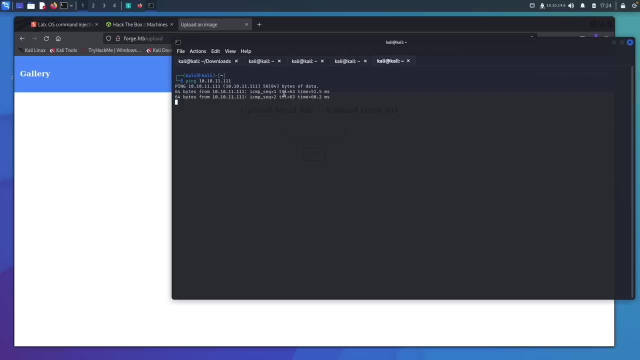 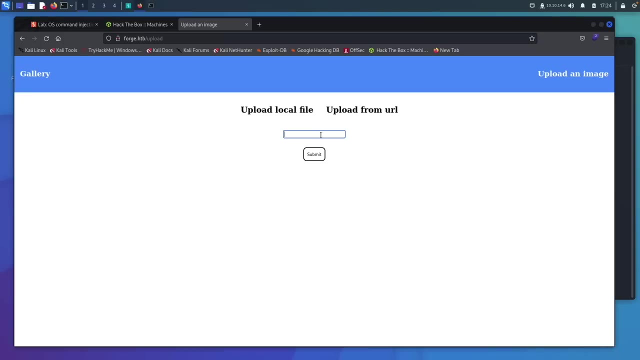 like that, and we know that we are on a linux box so you can try and do some stuff here. we'll just ping it real quick. so if we ping the ip address you can see the ttl is 63. so that tells us we are on a linux box and so if you wanted to, you could do something like a file slash- slash. 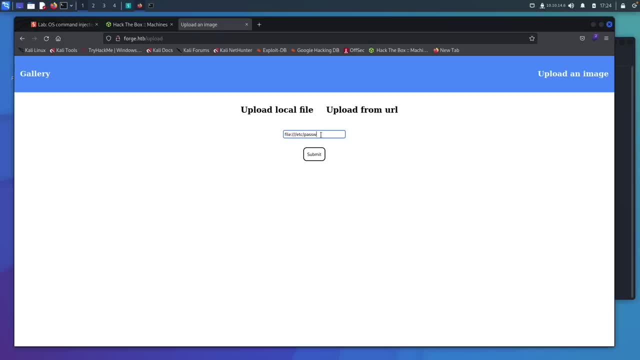 and then we would go etsy, passwd and we can try and pull this down, and it tells us that we're not allowed to do this. so we're on a linux box. we're not allowed to grab files directly from the server this way. so i'm going to put this in burp and we'll play with it in there, so we can and we. 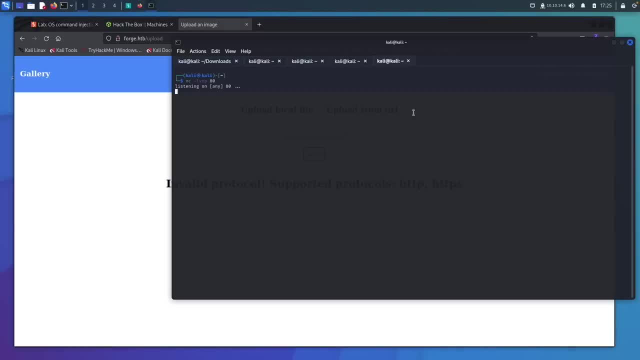 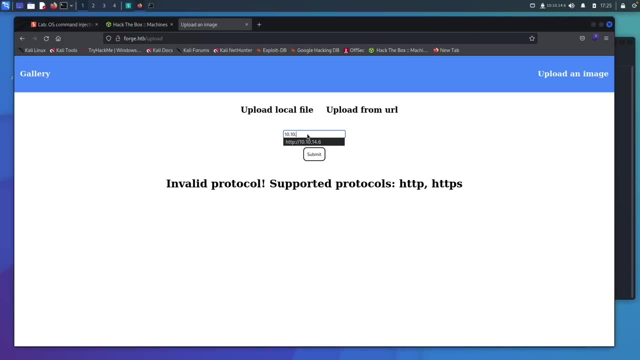 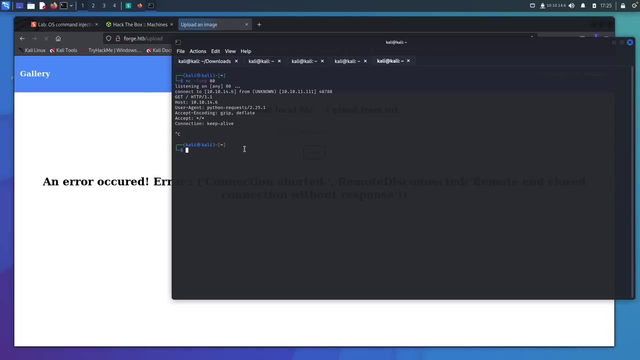 know that the url is working because if we come out here and we set out, and we set up our netcat listener, like we have been doing, and we put in our ip address, which i have up here, which is 10, 10, 14, 6, just like this, and we hit that, it's hanging and we see it reach out to our box, right. 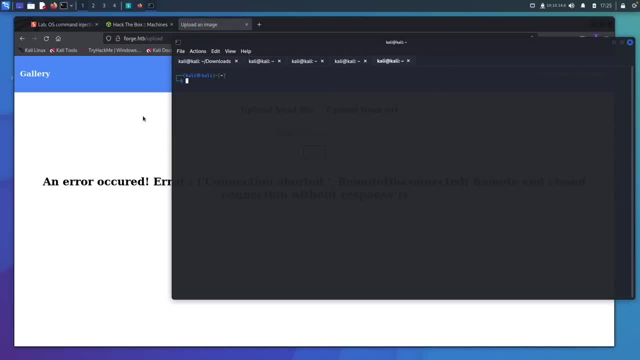 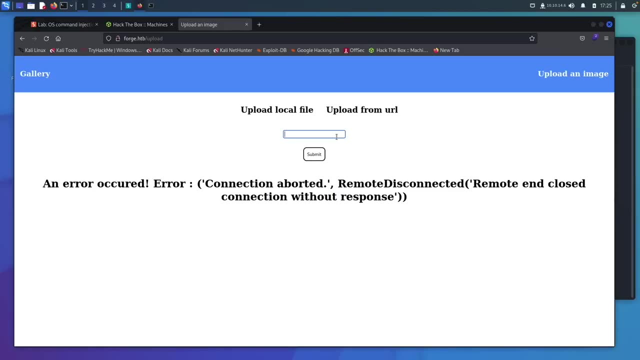 here. we can close out of that. so we know the url is working. now we just need to figure out how to get the ssrf to work so we can come back over here. we'll put this in burp and then we'll play with it. so we'll just put in some. we'll just put in our own ip address right here. we'll turn intercept on. 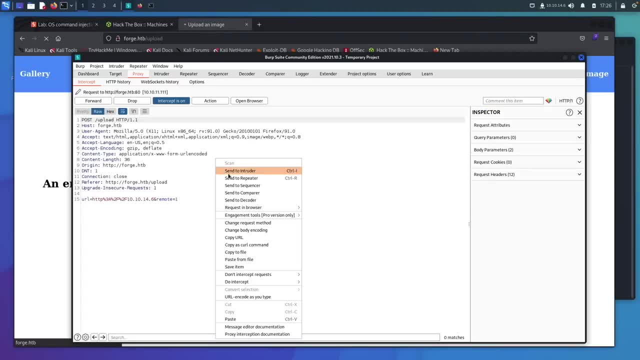 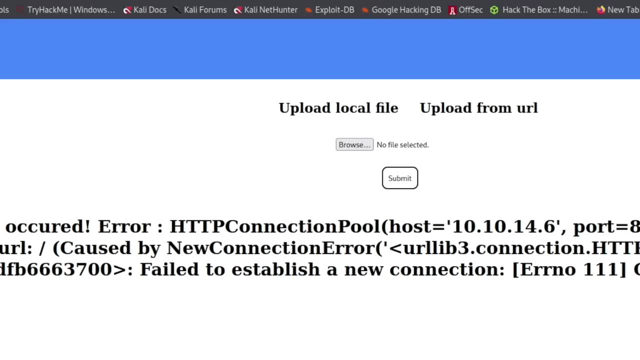 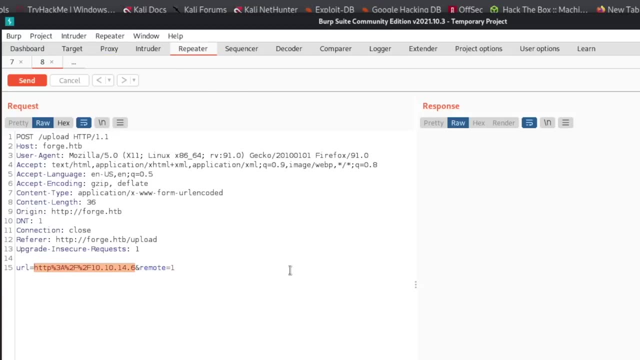 and- and we'll submit this- we can send this to repeater. we can turn that off and it's going to give an error because it's there's nothing for it to connect to, but that is okay. so over here in repeater we have this right here and, if you remember to, 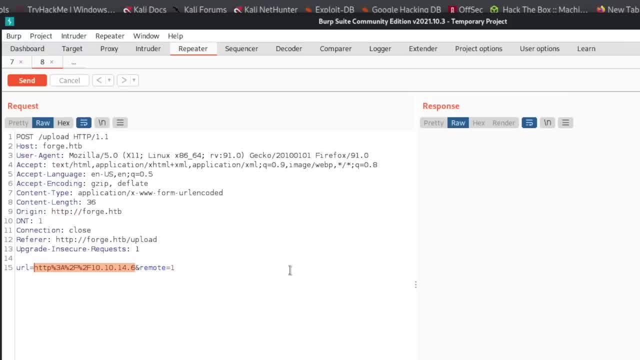 unurl encode. it is control shift u if you are on a mac, not sure what it is if you are on a windows box. so there's a couple of different ways to get this ssrf2 work and i set it up for the print default. 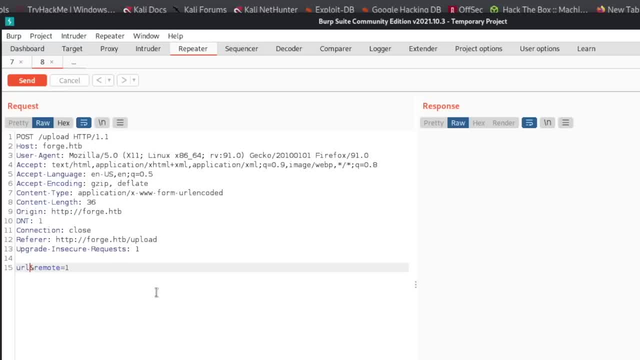 actually want to try something real quick that I have not tried on this box before. I want to see if the if we can bypass the filter by going file slash, slash, Etsy, pass, WD, and I believe this actually needs three right here to work. and so what you see we did here is we saw that it didn't work with just Etsy. 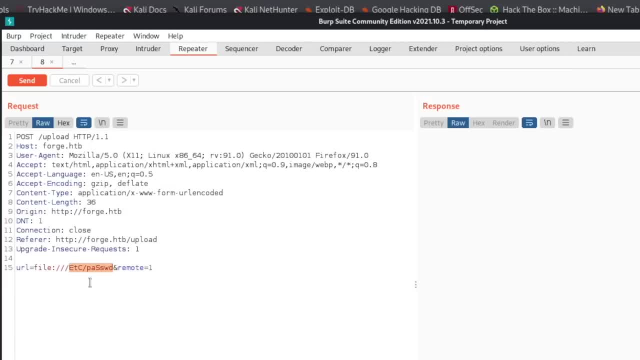 password. but it might just have a filter on the box and if we change some of the casing it may work for us and it tells us we have an invalid protocol. so it has to be an HTTP or an HTTP request, so we're not able to just pull down a file. 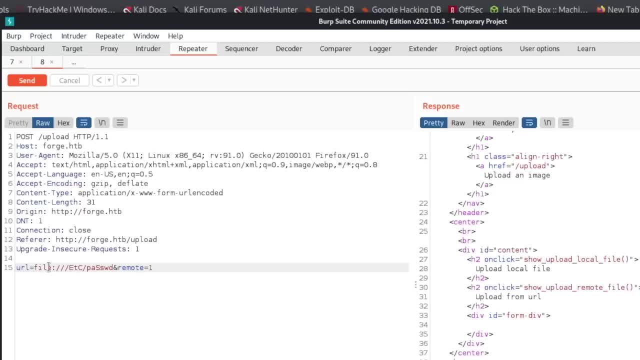 because it's requiring HTTP in order to be in the request. we're not going to try and grab the Etsy pass WD file, so what we're gonna do now is just try and make a request back to the server and get it to work. so in a bug bounty world, if you. 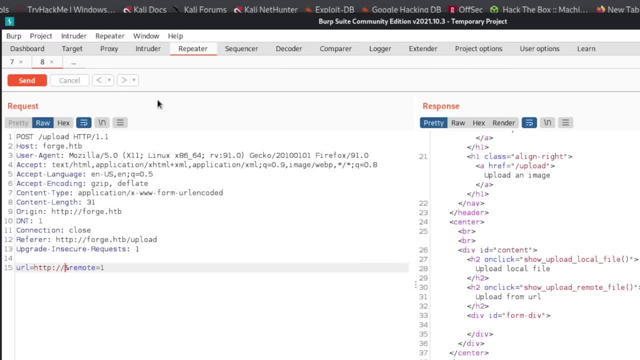 come across something like this and you're just trying to prove that you can reach back to the server with a request. what we're going to do is just try and query the server and see if we can get this to tell us something other than an invalid protocol. so if we come, 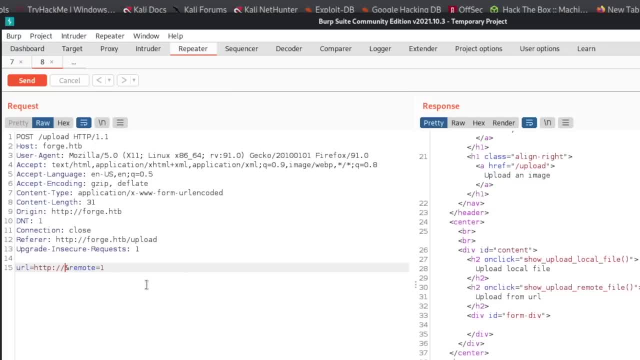 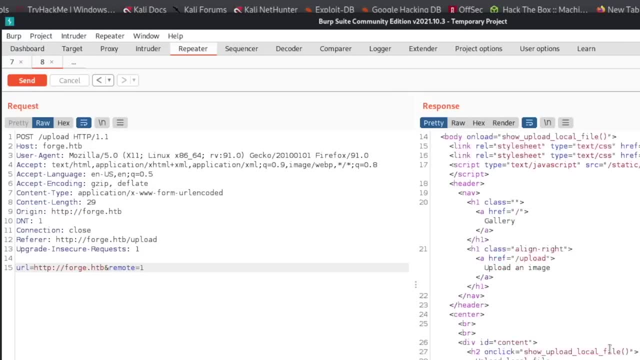 in here and we go to the actual URL which we have right here which would be forged on HTB, and we send this, we get told it is blacklisted. so you're not able to go to the actual URL right here. you can do like we tried with the file pass. with the Etsy pass WD file you can. 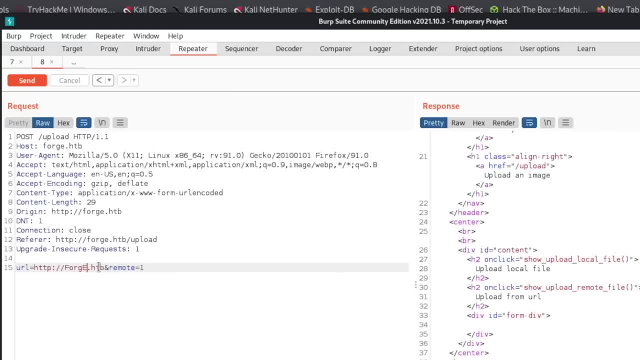 just come in here and type in forge and you can just change a few of these characters and now, if you send it, it tells us we have reached back to the server and we are not getting a blacklisted message any longer. so this is one way to try and bypass, like a blacklist or something on a server and 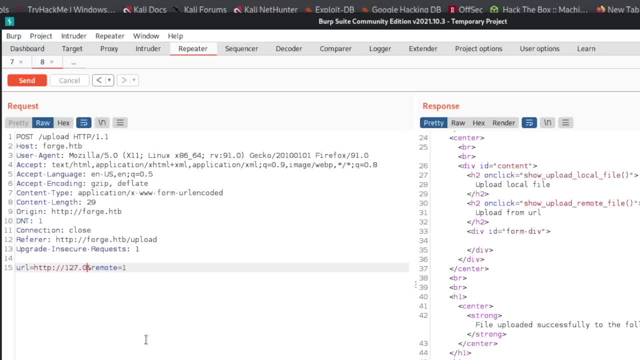 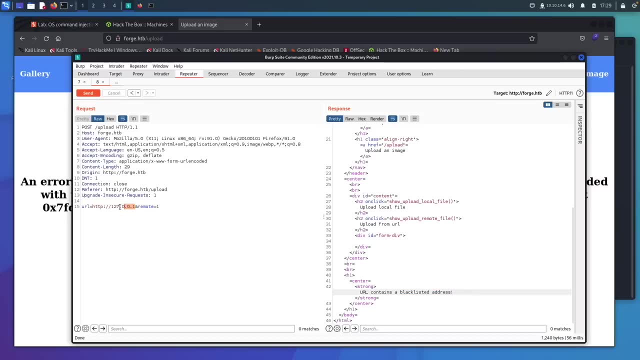 if you come in here and you do a one e seven point zero point zero point one and you send this like we were doing earlier, it is blacklisted, but the actual IP address. so if you wanted to get the IP address of this right here, it tells us that this right here is blacklisted. 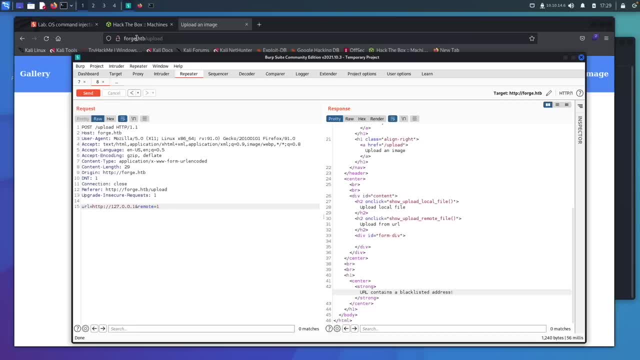 but if we actually wanted to get the IP address, let's say we're on like Yahoo or something and we want to know the actual IP address of what we have going on right here. burp will actually tell us what the IP address is really easy. you can just. 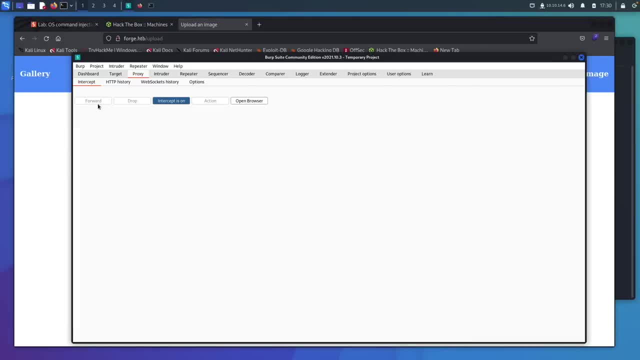 come over to your proxy and turn your proxy on and for that and we can come to our URL upload. you can just type something in here, doesn't matter what it is, submit it, and when you hit this it'll tell us like the request is being sent to forge dot htb, but the IP address is 10, 10, 11, 1, 11. 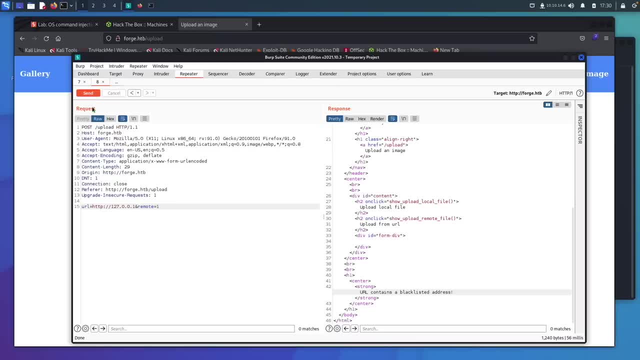 and we don't really need that request. so what you can do, since this is blacklisted and this is blacklisted, you can just try the actual IP address to the server and in this case it looks like this and you can send it and you can see that it went through. so the IP address. 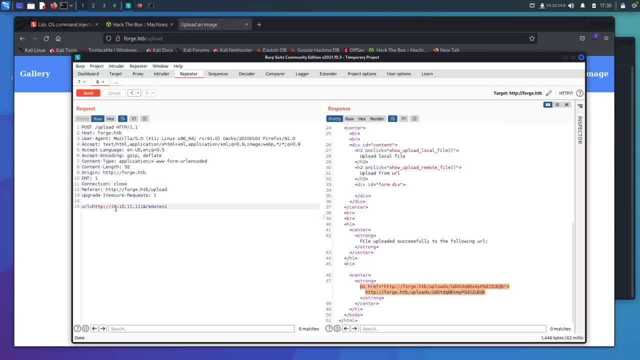 ironically, is not blacklisted. I'm not sure if hack the box meant for that to work or not, but it worked. so you can actually try several different ways to get past the blacklist within a server-side request forgery, and this is a few different ways to do that. okay, so I think we're gonna go ahead and pause. 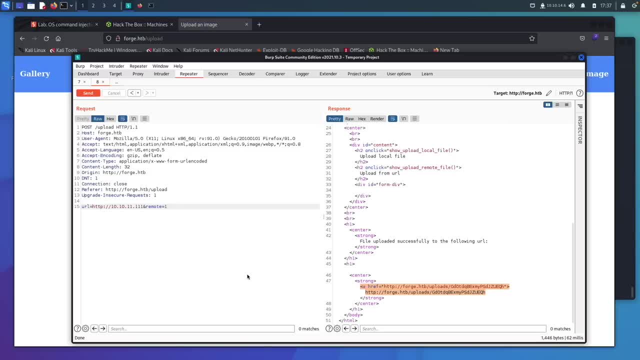 on SSRF at this point. if you have any questions on server-side request forgery and you'd like to see something in more detail, please let me know down in the comments. but in the world of bug bounty, this would be plenty to get you by. however, if you're going to be a penetration tester, you're probably going. 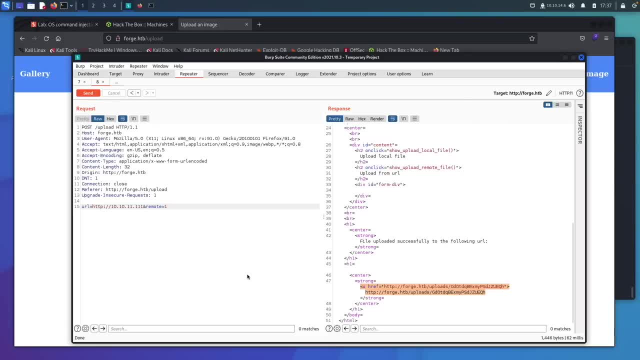 to have to dive into SSRF in a little deeper context. that way you learn how to take a server-side request forgery and turn it into remote code execution. but I think that is out of scope of this video, so we're going to go ahead and pause this. 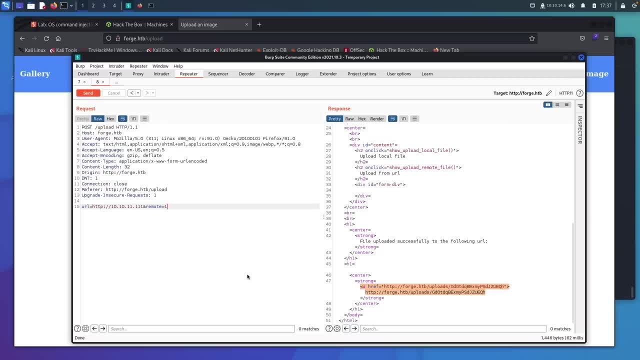 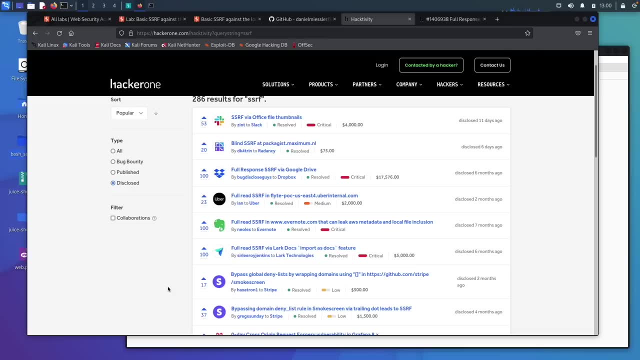 here, and if you would like to see more server-side request forgery in the future and turn this into remote code execution, please let me know and I'll get to that all right before we close out this section here on the server-side request forgery. I 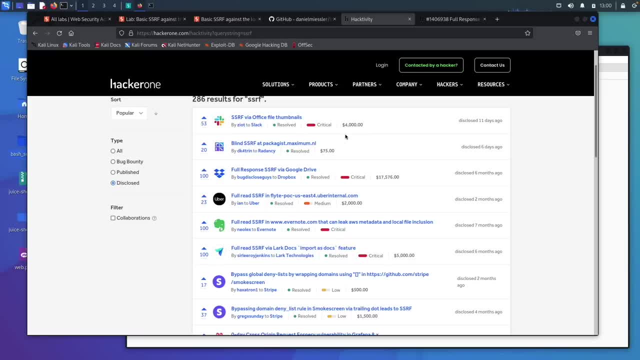 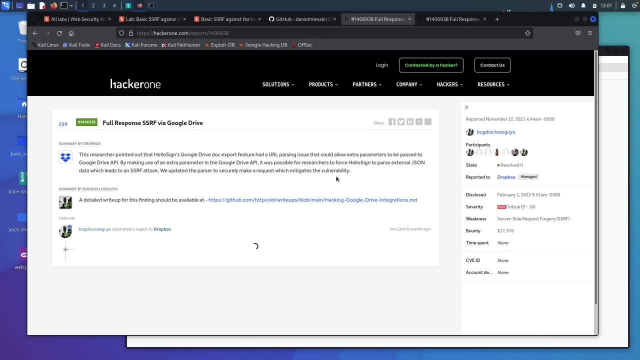 thought I would pull up the activity and I was reading through some of these recently and you can just see- look at how high the impact is for server-side request forgery- and I was reading through how some of these were done and this one right here was really cool and I thought 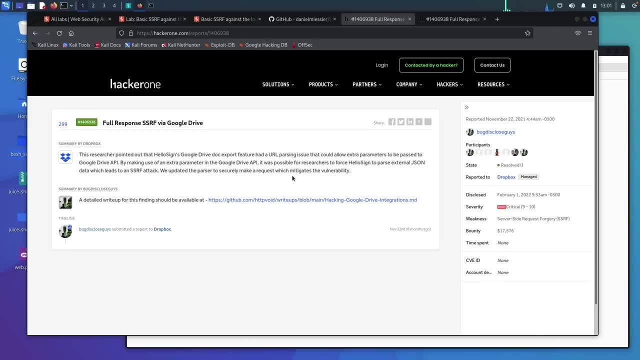 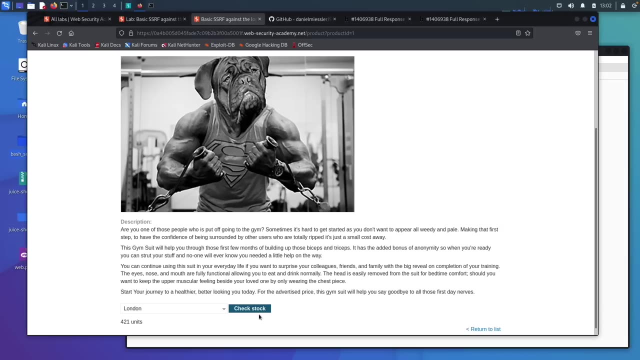 I would show you how this actually works, and I and so I went and read through this and I actually did learn a little bit about the exploit and it was pretty cool. and I came back to the port swigger Labs and was playing around and I found out something I did not know before. so if you come in here, where 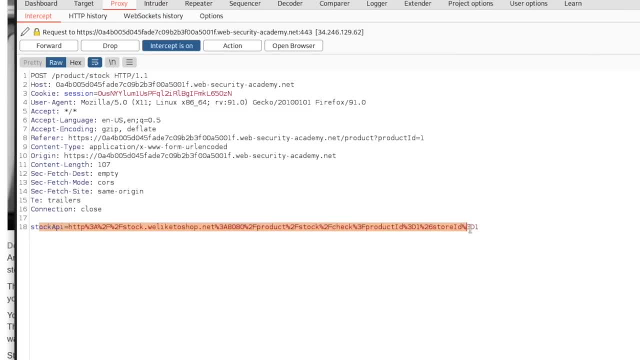 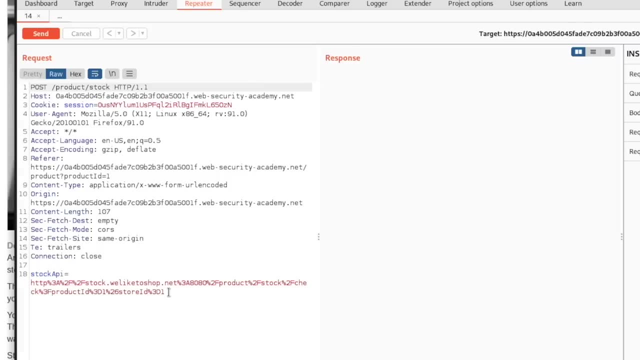 this server-side request forgery is, and you remember it's right here inside this stock API. we can send this over to repeater and if we do, the unurl encoded, we have this right here and we can see what's being sent. but we'll go ahead and 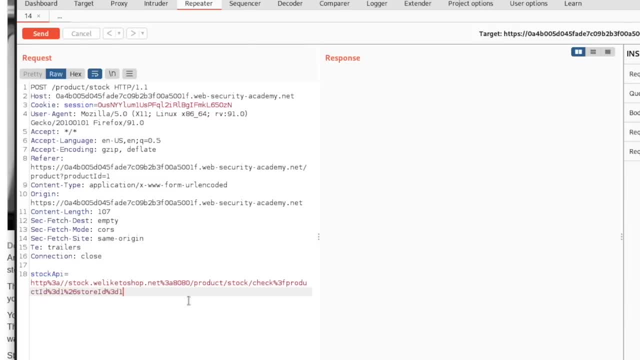 put that back. but what you can do- that I didn't realize we were able to do- is you can just add in another parameter. if we were like breaking this right here and it wasn't working, we can just come, come in here, put the and sign and type in: stock API equals, and then we could just do the. 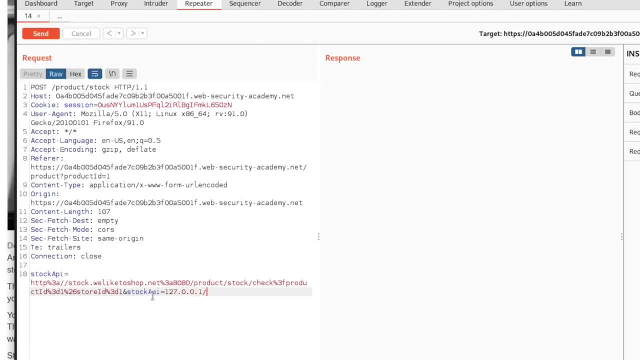 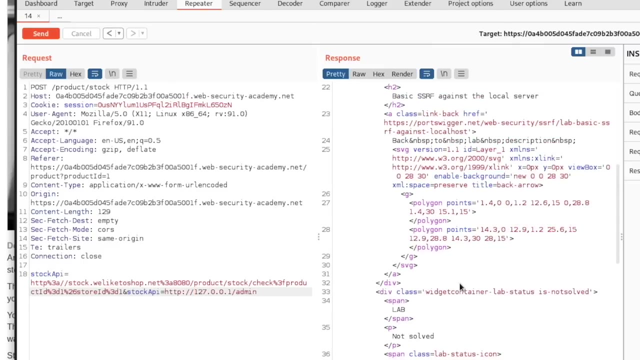 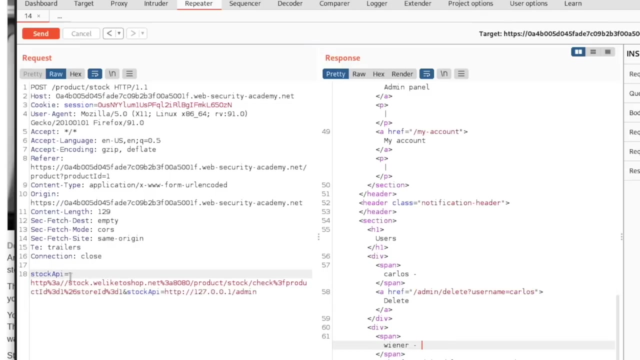 local host and then we can go slash admin, because we're supposed to pull down the slash admin panel and we can send that and we need HTTP slash slash and it works for us and it pulls down the information we needed in order to delete the user Carlos. so I didn't know beforehand that we can just add in. 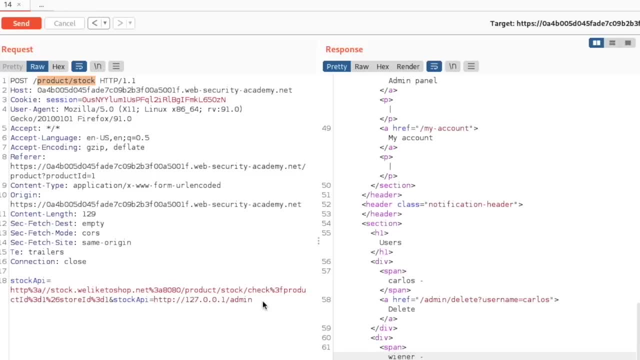 new parameters right here, and so I thought this was something that was really cool: that you can add in extra parameters in here, uh, in addition to the one that's already there, so you don't actually have to delete this first one, you can just pull down a, pull down a second one and then also reading through the 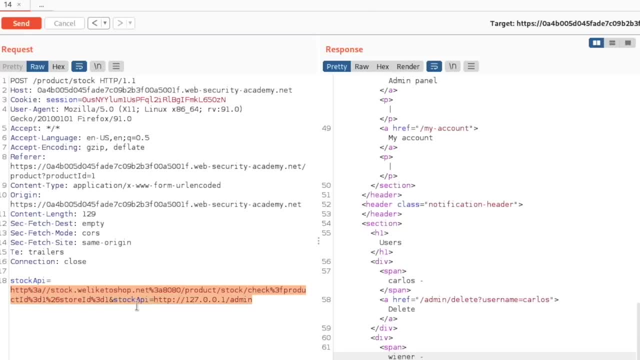 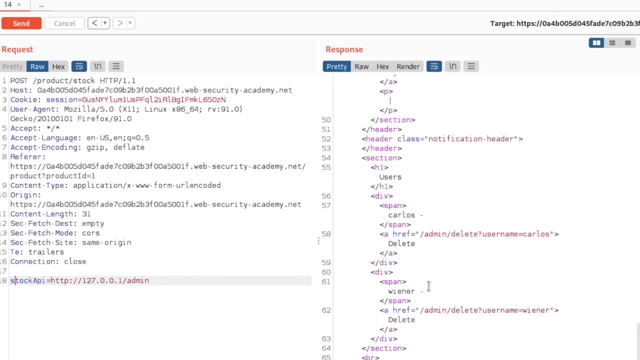 activity I noticed. I think what we'll do is just delete this first one so that way it looks nicer, so you can see it, and so we'll send this and we don't get quite as big of a page back when you're doing something like searching for an ssrf. 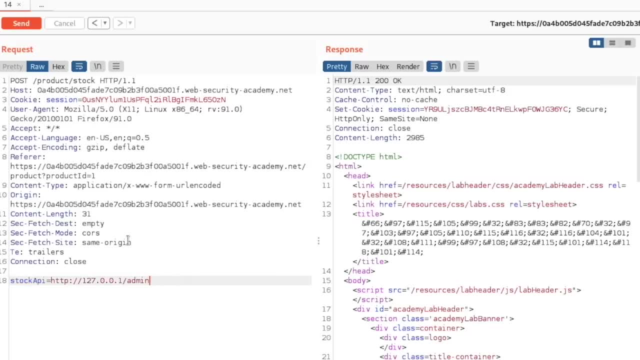 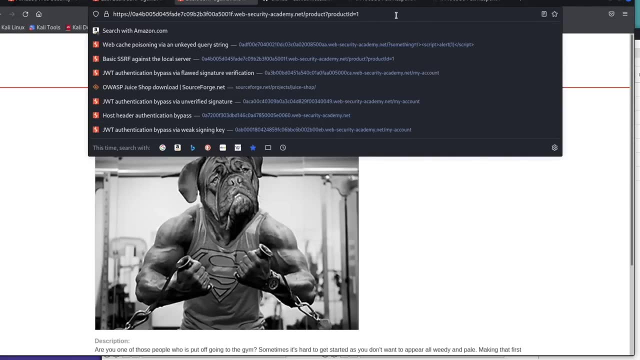 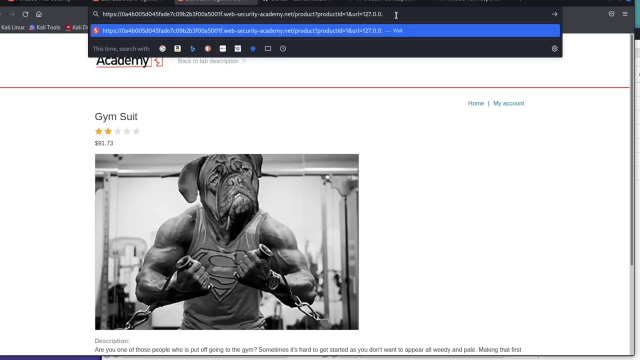 list. a few of the activities were: they had hit a line like this, that's accepting in a parameter, or even up here in the URL, and what they just started doing was they would say: and URL equals, and then they had put in 127.1 and then, and then you could just leave it like that, and they were sending this. 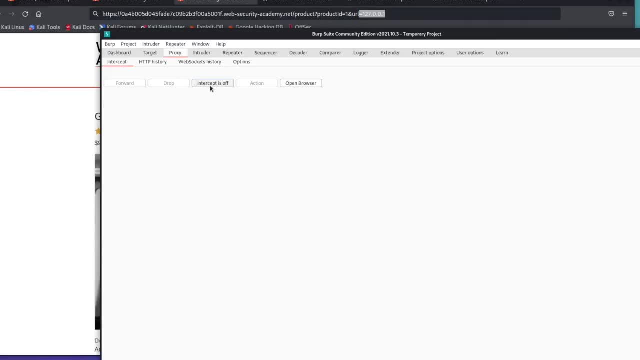 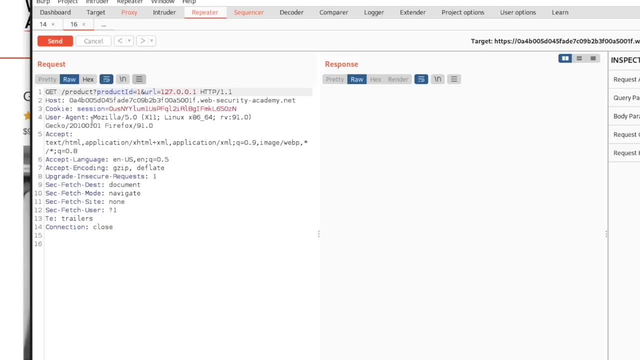 and it would be easier to test for this if you had it in repeater, so we can grab this, send it to repeater, not sequencer. send this over, turn that off and then, if you send this, you'll see it doesn't actually pull anything back for us, and you can search for the word delete over here. 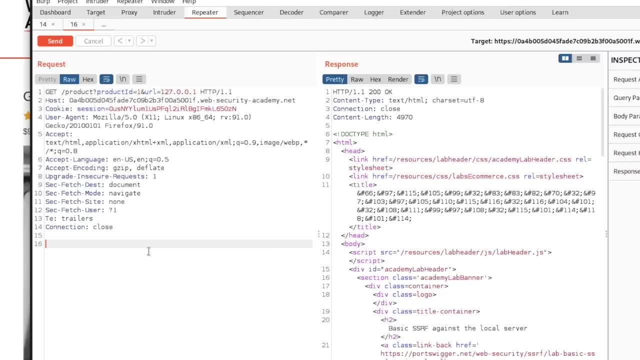 as if we're going to delete the user and there is nothing. but you could church, you can. but you can try this URL. you can try urls and send that to see if this is a parameter that will actually reach out to the server. usually it's going to be saved as a urls or a URL something like this, and this is: 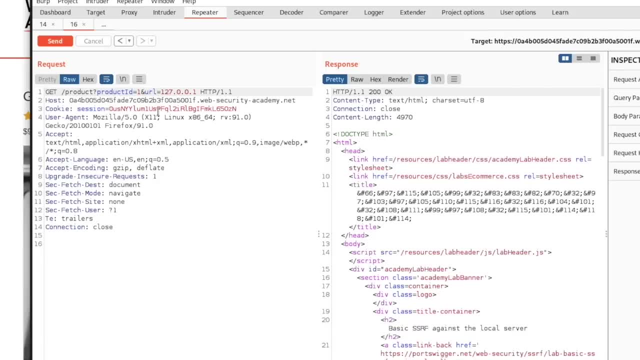 not vulnerable. this actual lab is not vulnerable with the URL parameter because the URL parameter is not the one that's making the request out to the server. but you could very easily change this with a change. request must change the request method and then delete this and just add in the. 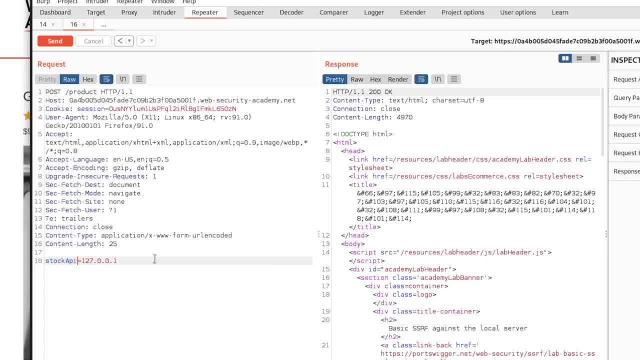 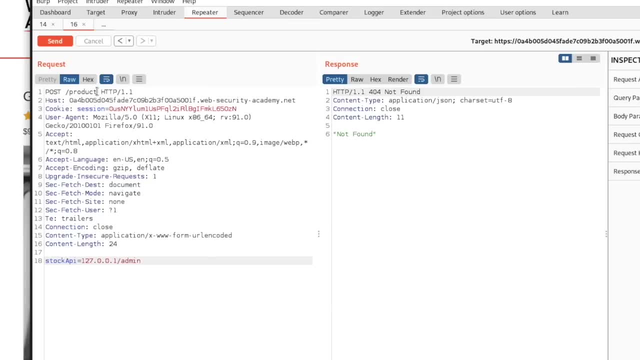 stock a api, just like this, and this should work. i think we have to make it so. it says it needs to go to the admin panel- uh, it needed this up here, products, and then in the stock directory and then- and i forgot- http, slash, slash. so basically, this is just remaking this request over here, but this should. 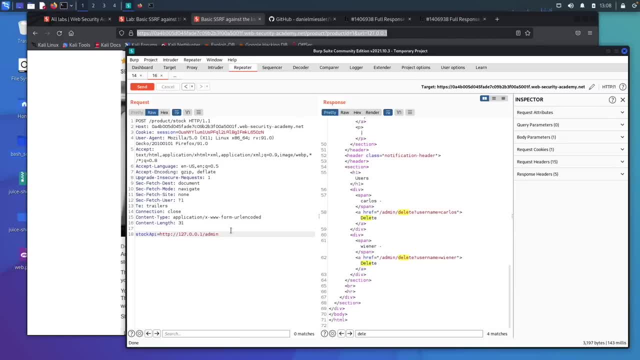 work now and it does. so you can play around with these when you're in a live program and see if you can find a parameter that actually does hit the url. so if you come over here and you open up this and you're reading through it, what's really interesting inside of this guy's? 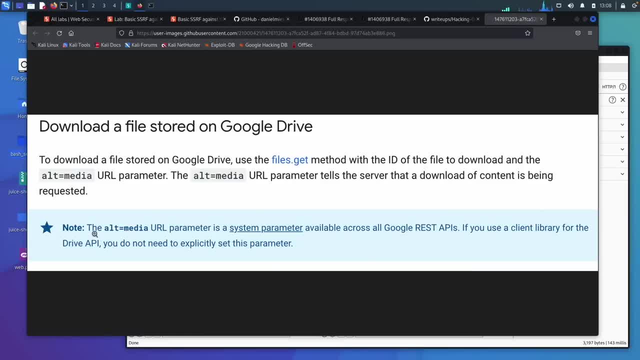 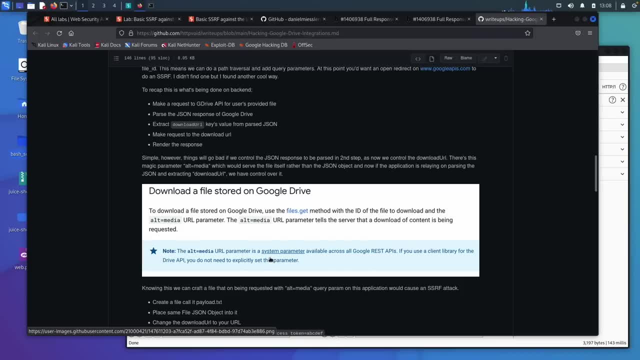 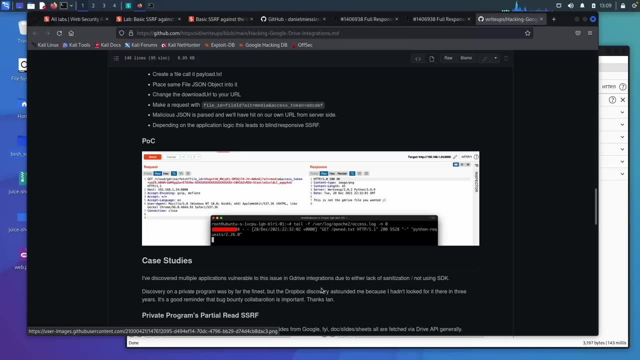 explanation is there was actually a notification that says this right here is reaching out to the url parameter, which just pretty much tells you that it's going to be vulnerable to a server-side forgery, and when he tested it right here, it works. now this guy had to do a little more to it and i 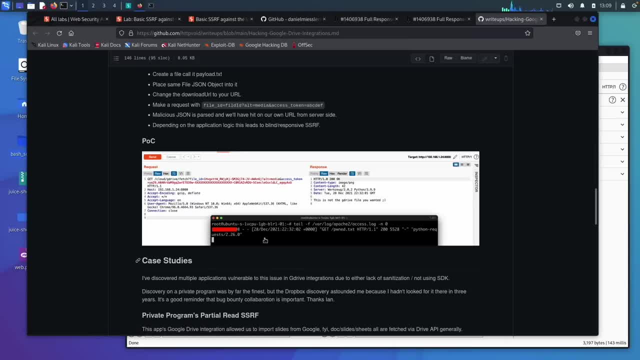 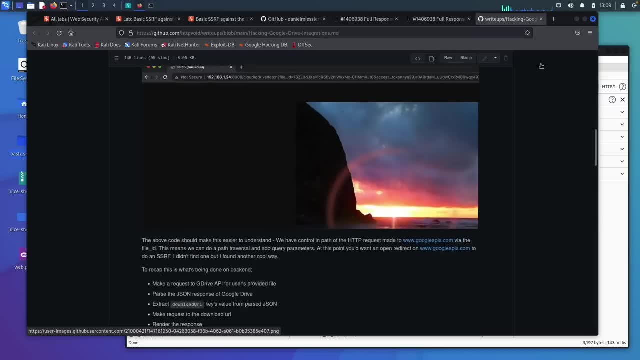 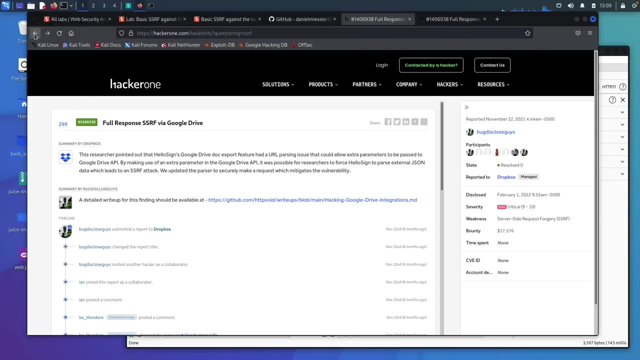 don't want to read all this to you, so you can come out here and read it, but he had to do a little bit more in order to get this to work- through a token, i believe it was, but it was a pretty cool server side request forgery and you can come over to the activity now that you understand how server side. 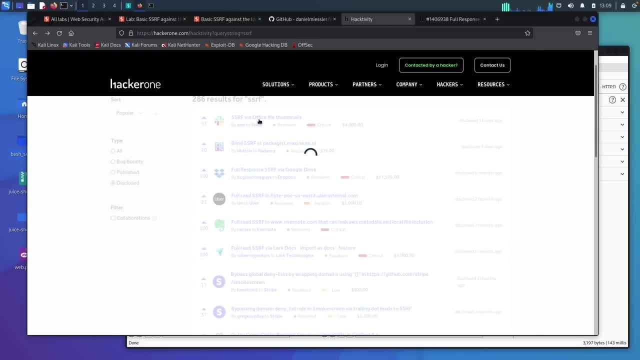 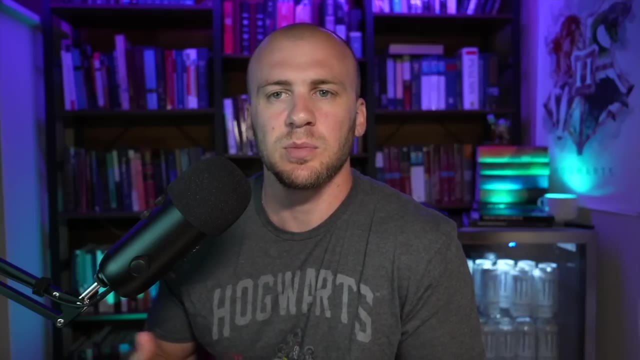 request forgery works and you can read through some of these and see if you can learn additional ways to pull off server-side request forgery. so with that, i'll see you in the next vulnerability. all right, welcome to the section on a command injection. this is probably going to be one of the most severe. 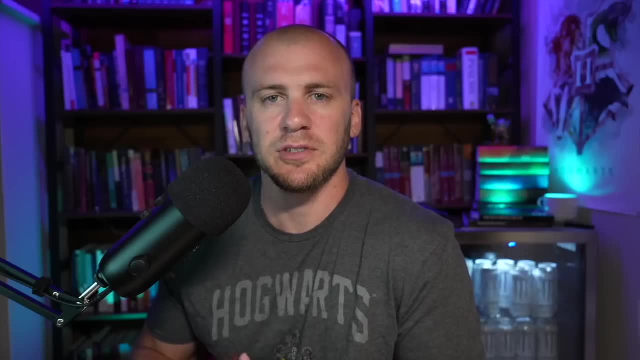 vulnerabilities that you will ever come across. this vulnerability gives you the opportunity to execute commands on the server and get information back, and possibly even get a shell on the server. so this is one of the most severe vulnerabilities that you will probably come across, because you can just compromise the server and all of the information on it and if 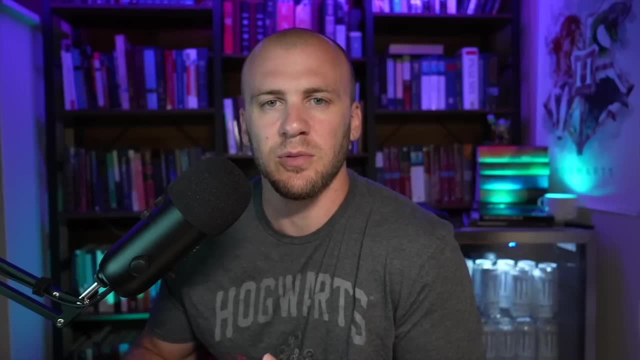 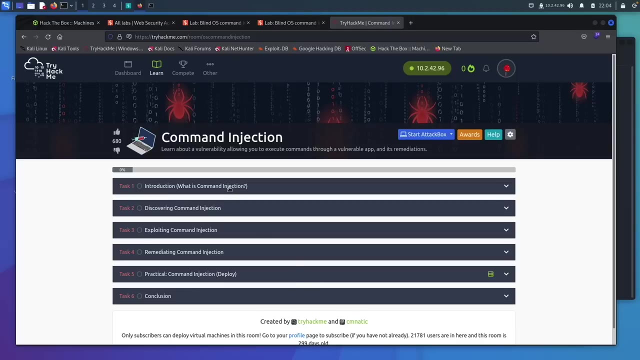 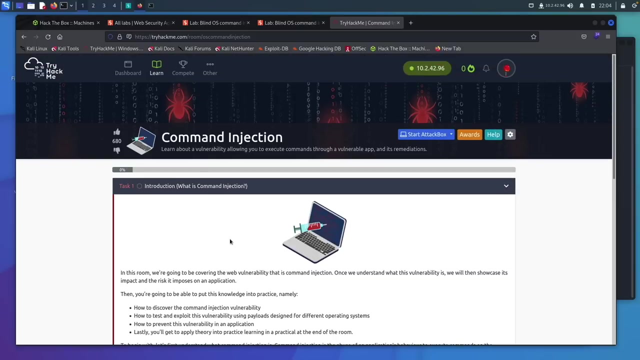 you're in a penetration test, then you can try and move around within the network. so let's go ahead and dive into command injection. okay, we are going to be talking a little bit about command injection, and there's not really a whole lot of places to practice command injection that i know of. really, 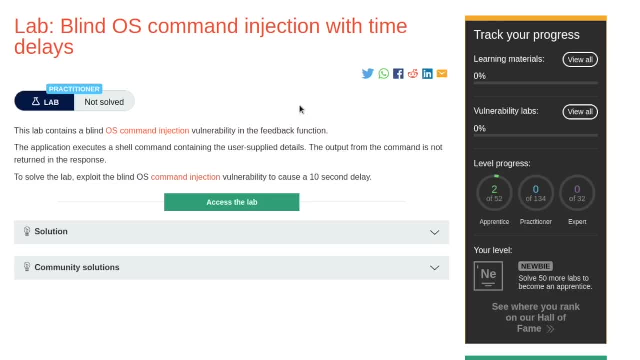 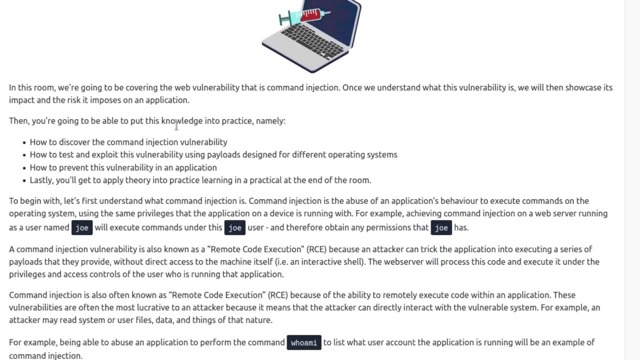 it's just try hack me and then port swigger- which we'll come to here in a little bit in practice on. so with command injection what we are able to do is put commands into the server and then it tell us back. it'll give us the information back for whatever we sent the command in for. so if we send, 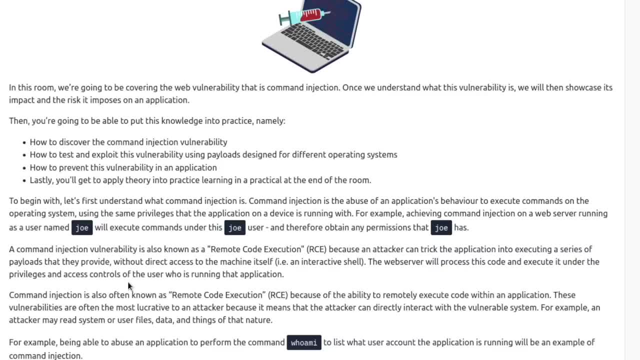 a who am i command. it will tell us who we're running as on the server, and so it says here a command. injection vulnerability is also known as remote code execution, because an attacker can trick the application into executing a series of payloads- payloads that they provide without direct. 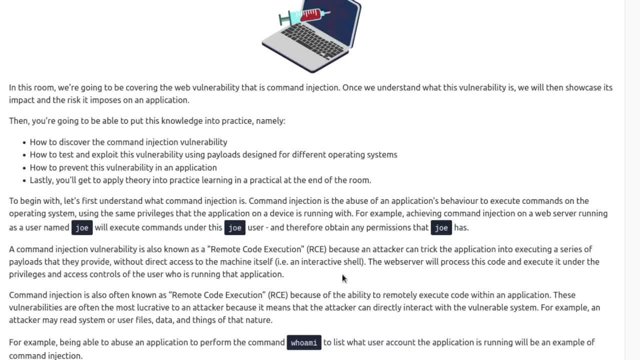 access to the machine and the server. so that's what we're going to be talking about in this video. so let's go ahead and go ahead and show you what we're going to be doing here. so i'm going to go ahead and show you what we're going to be doing here and i'm going to go ahead and launch this. 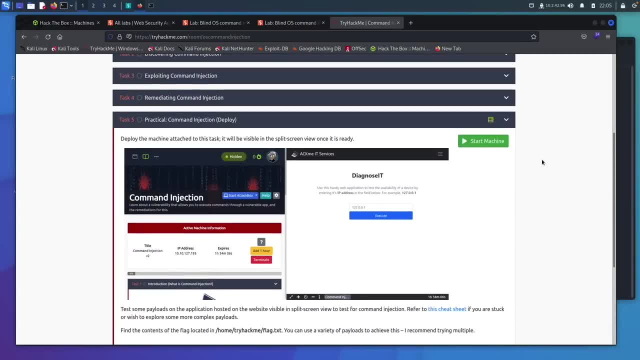 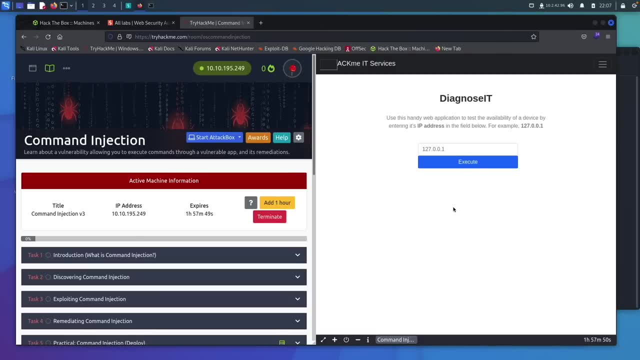 command and i'm going to go ahead and launch this machine. so this might sound a little confusing, but it's going to make a lot of sense here in just a second, and so their example here is the who am i command and i'm going to go ahead and launch this box and then, once it is loaded, i will bring you. 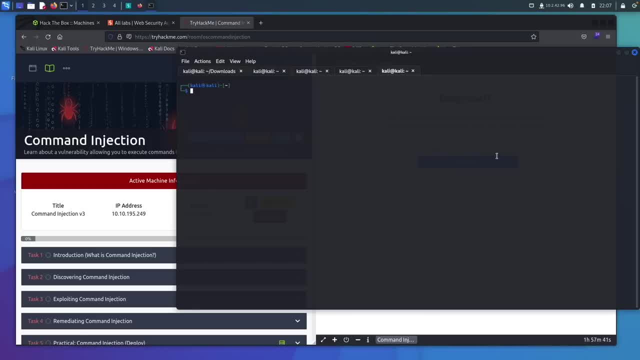 back. okay, so this is now loaded up and ready for us to practice some command injection. but before we do i want to show you kind of what is happening if we come over to a terminal here and the first make sure we know what kind of commands to send through to the server. But really you could just 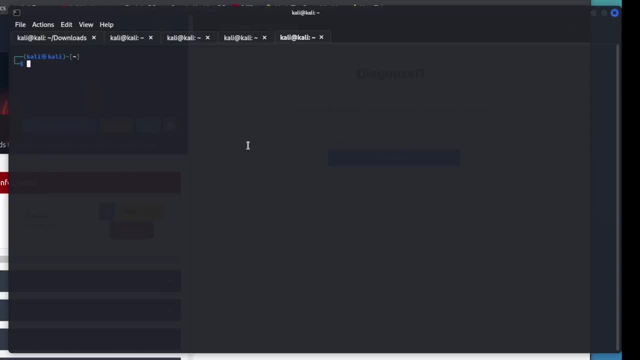 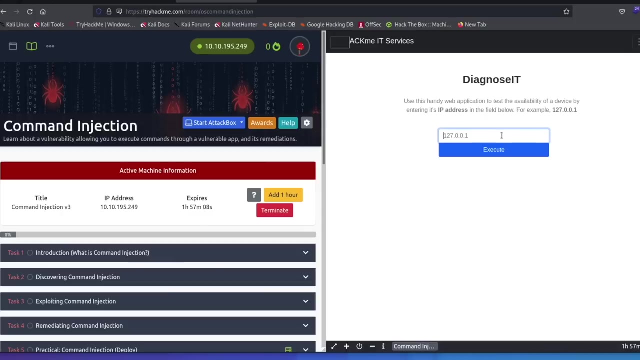 put in an I. who am I? and you could probably figure it out by that. But we can also type in ping and then the IP address that we just copied, And then you can hit enter And we see that the TTL is 61. So we know that this is going to be a Linux server that we are up against. So now it. 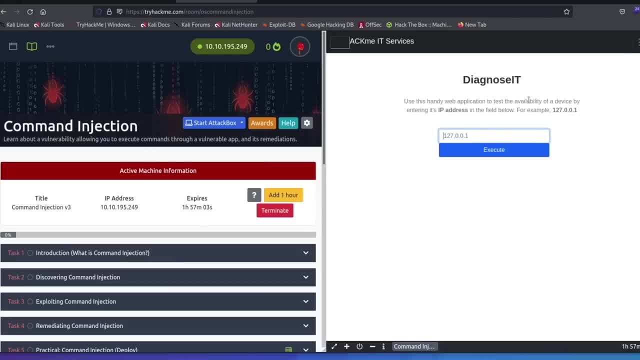 tells us to use this handy web application to test the availability of a device by entering its IP address, And it's just going to go out and reach to an IP address. So a way to test this is to see. if we wanted to check our device, we could come over here and set this up And my IP address. 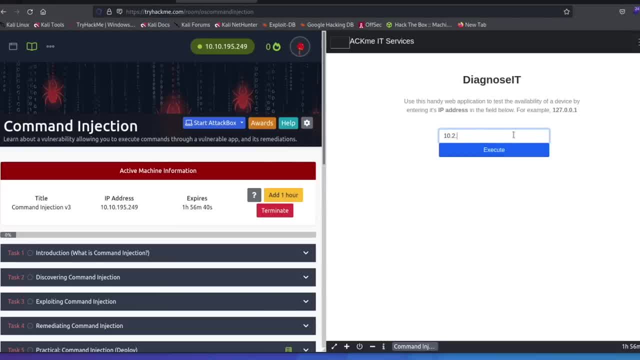 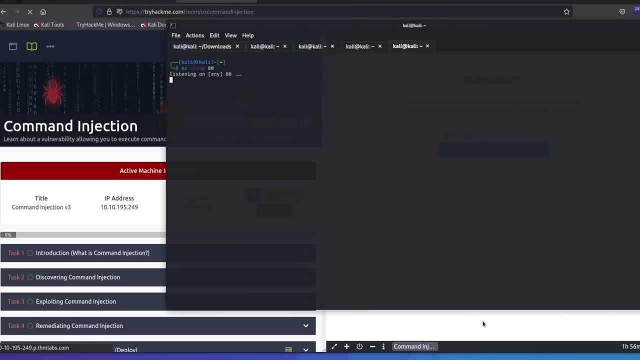 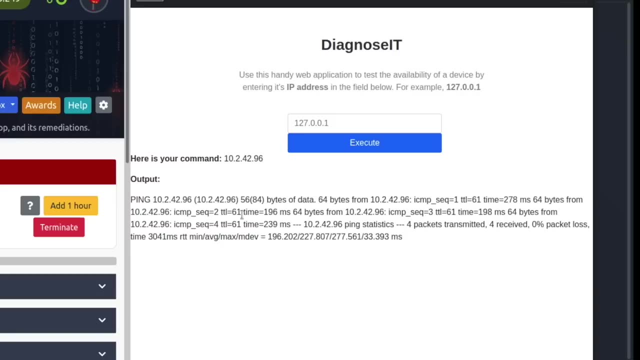 is up here, So we could say 10 to 4296 and execute and see if we can get it to reach out. And it sent a ping out to our box and it did not connect, But it pinged our box. So this is just. 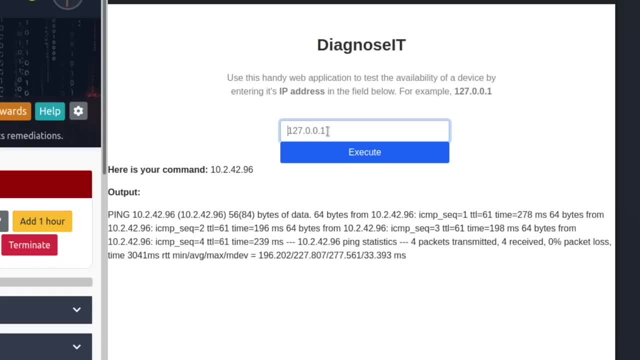 sending a ping, It's not actually trying to connect. So what we can do with this now is you can just type in 127.0.1 and you can execute it And it's going to tell us it's going to give us back another. 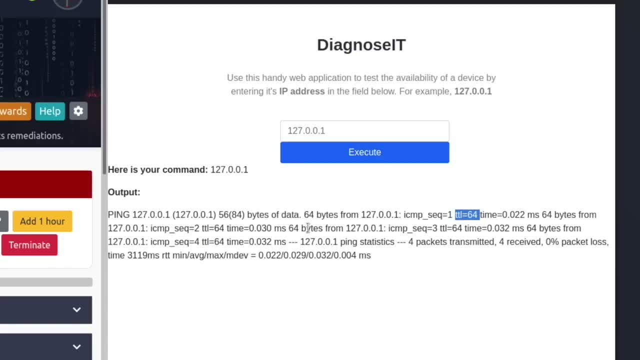 ping of the box, And I guess I didn't need to ping it because it tells us right here it's going to be a Linux box. So some of the things we can do. I actually played around with this. That's why you can see these in here. 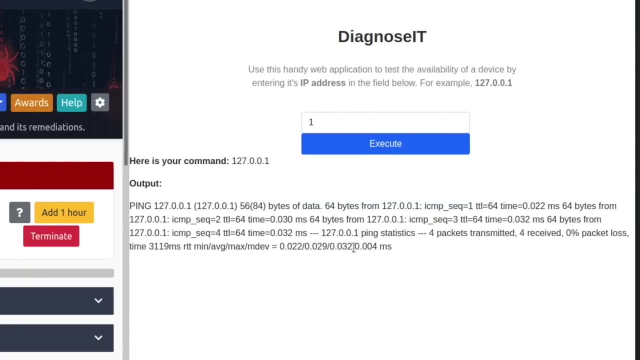 So you can see all the different commands that it actually let me send. So I wasn't just sitting here testing everything for the first time. So here's a couple of the command injections that you're going to need to know. If you come in here and we type in 127.0.1,, you can do an and sign. 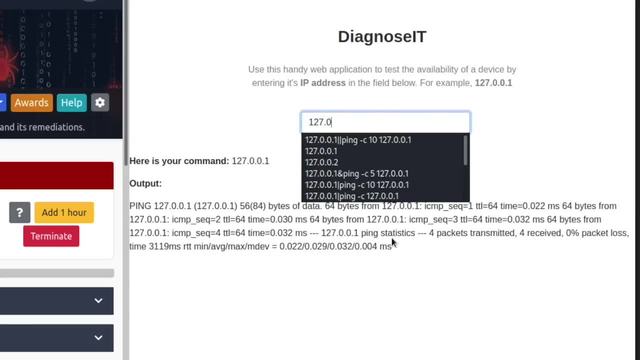 like this: 0.0.0.1.. We can put in an and sign, just like this, And then we can do a who am I? And it will send a ping, And then you can see that it actually sent a ping, And so I'm going to. 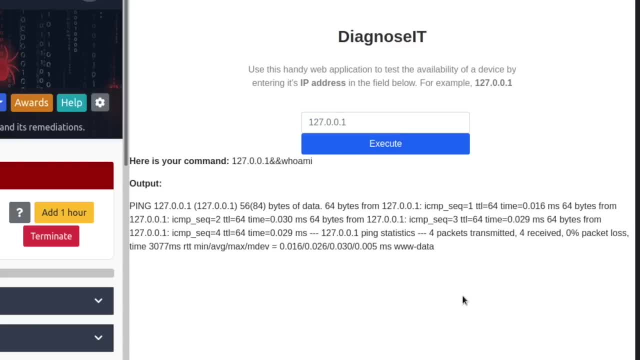 I'm going to type in 127.0.1 and then we can do a who am I, And then we can do a who am I, And then we can it'll execute and you can see that it says we are WW data, but we still get. 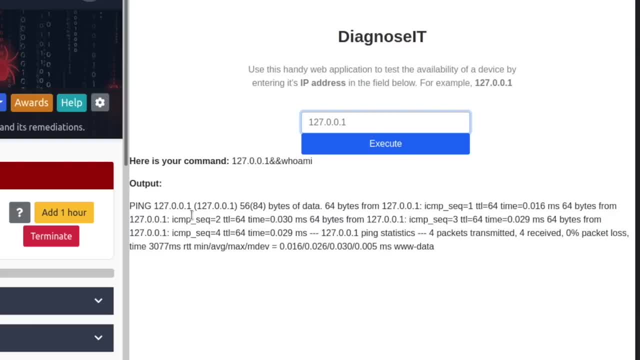 this ping right here, and it is possible in the coming lessons that we're gonna. we just don't want to see all this ping right here, so what you can actually do is just put in a bunch of mumbo-jumbo and then you can use a double pipe and 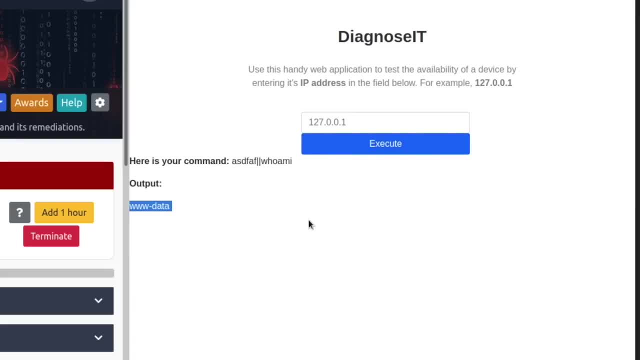 do the hue who and then do the Who Am I and it skips the ping and we get the WW data. but if we run this command right here and we don't double pipe it, you only do one pipe. oh, it still works. okay, I was gonna say that it doesn't work. but 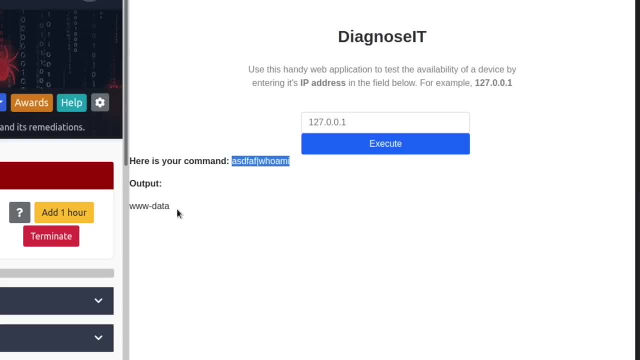 it worked for us. so we still get the W, the WWW data. so sometimes it won't work with one pipe and you'll want to send through two pipes and then sometimes you'll also have to have like a pipe afterwards and run it, and that time it 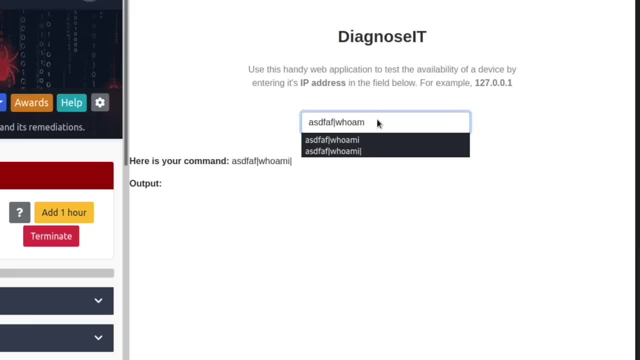 doesn't work for us, so you will, in the wild, just have to play around with this. so we get the Who Am I and it tells us where WWW data and you can type in ID and see how work we're sending commands through. so if we come back over here and 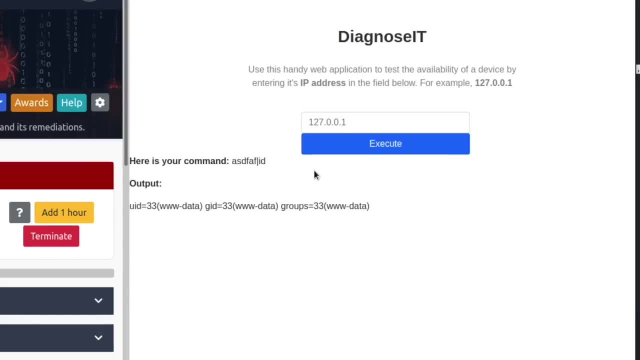 I type in ID. you can see we get this back. so we're actually communicating with the server, and this would be a very, very bad thing in the real world. so there's one more thing I wanted to show you, and that is this ping right here: if 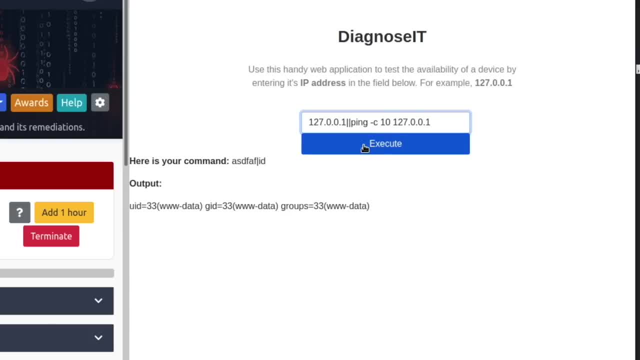 you were doing this in your classroom. you might want to make sure that you a blind command injection and you weren't, and you wanted to know if you could reach the server but you weren't getting any information back. you could run the regular whatever's up here. sometimes it's. 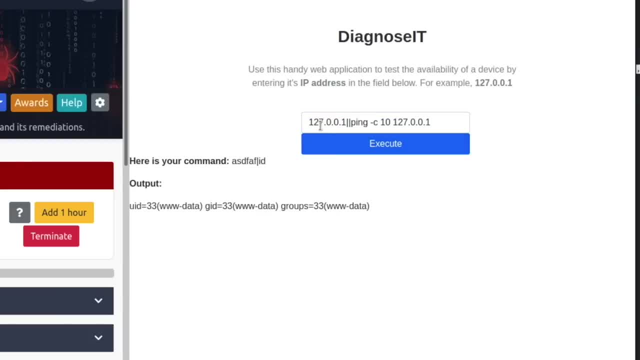 not, it's not going to be something like this. you're not going to be pinging a server, it'll usually be a parameter with an equal sign, and then you put a command in over here. but you can ping in the dash c with the 10 is going to tell it to delay 10 seconds, so we'll actually put in five. 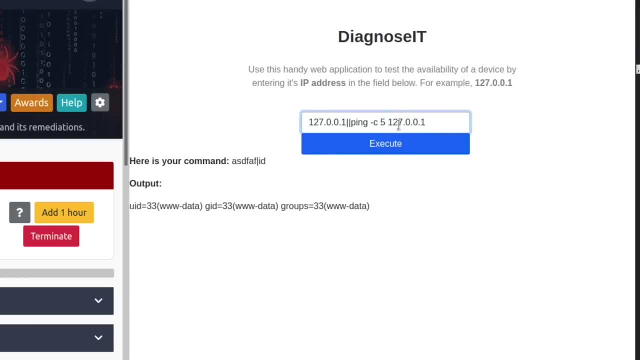 seconds so we don't have to wait quite so long and it's going to ping itself. so if you watch down here, we have the seconds and we'll hit it when it hits 10 seconds and wait for it and see if it comes back in five seconds. if so, then that works and it did so. we pinged it and that's how. 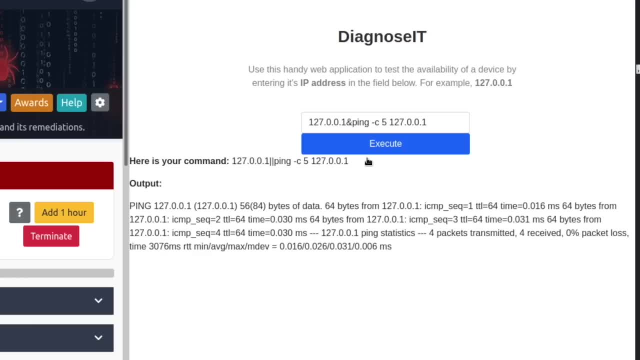 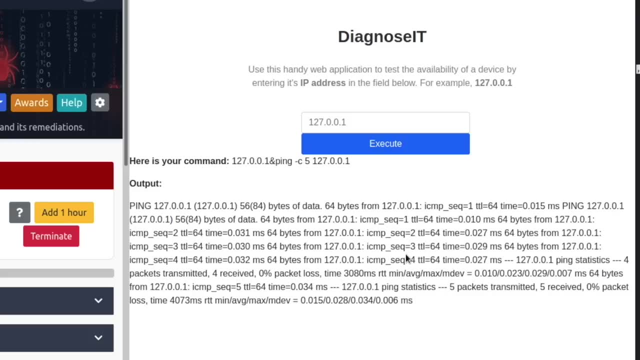 you do a time delay, which we're going to see in just a little bit. you can also run these with this and sign right here. there will be times that you'll need to try this, and you can. actually, if you're getting stuck on command injection, what you can do is go. 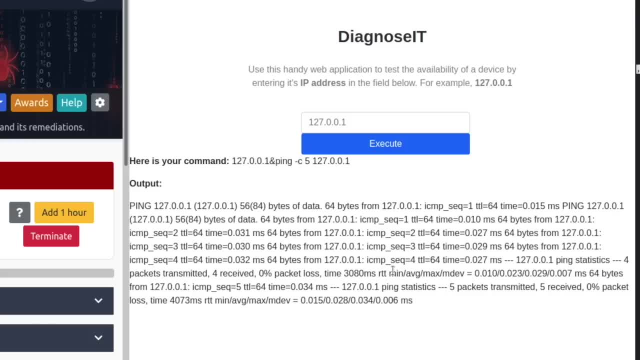 out to google and just type in command injection bypass and just look for different windows command injection bypass. maybe you'll have to do some url encoding or something of that nature and you can just bypass whatever filters they have. so you can also do with this. you can do two. 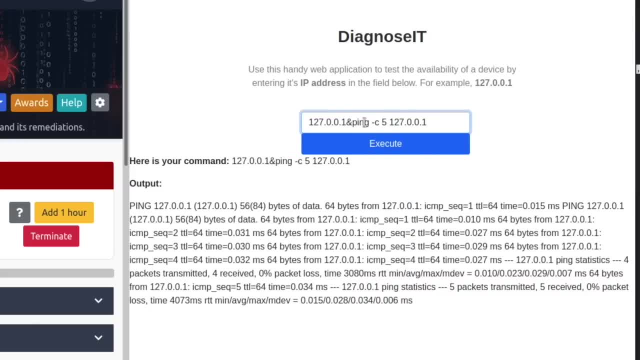 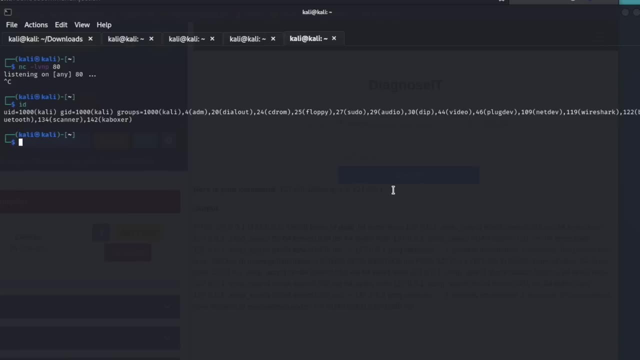 two and signs just like this, and it should still work for us and we'll send that over and see if it takes five seconds and it comes back. and then i want to try one more thing. i actually have not tried this yet, but because this didn't reach back on our netcat, i want to. 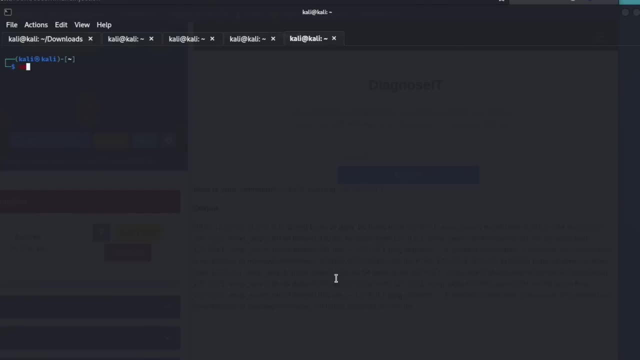 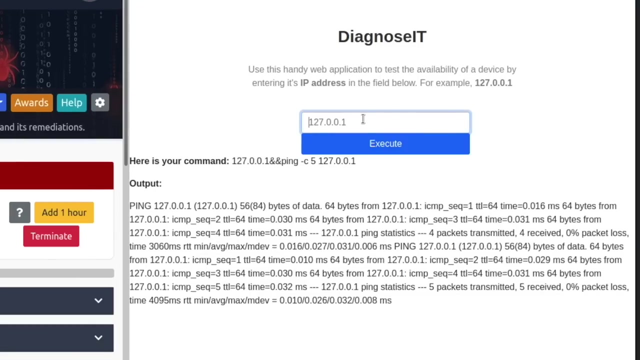 try this again. we'll set up a netcat listener and we're going to set it up on port 4000 and see if we can actually get this to connect back to us. so if we do this right here, we can do our pipe. we'll actually do a double pipe and then hopefully we have netcat available. 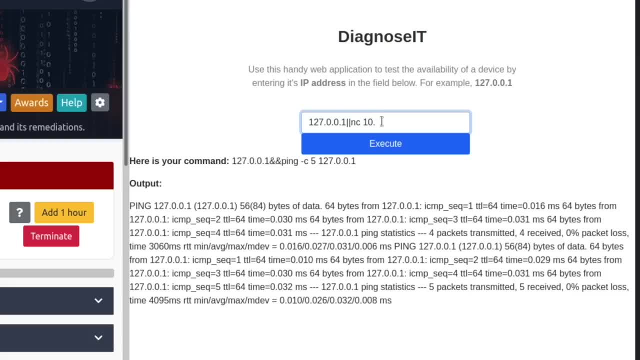 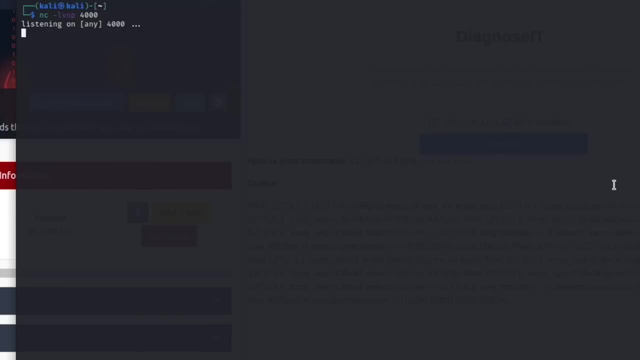 and we can type in our ip address for it to connect back to. so 10, 2, 42, 96 and then dash e and then we'll go ben bash, and then we can execute this and see if it reaches back. it doesn't look like it's going to because i did not type in the port. 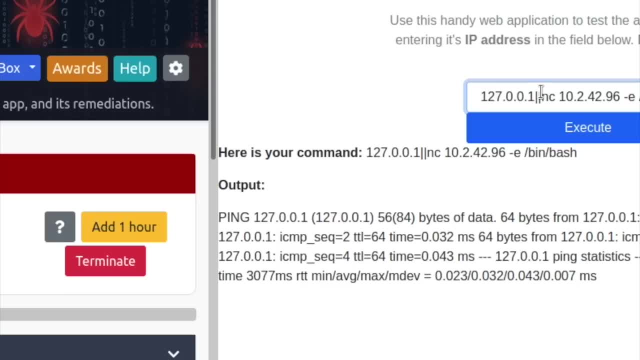 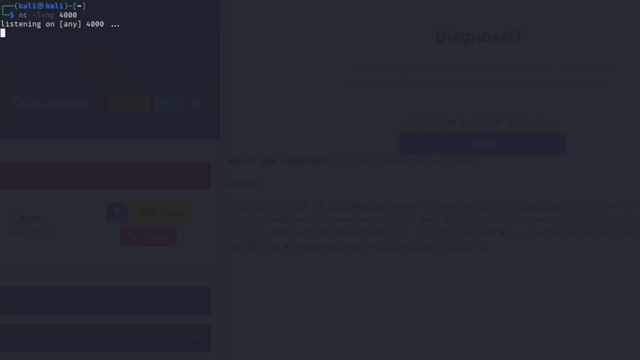 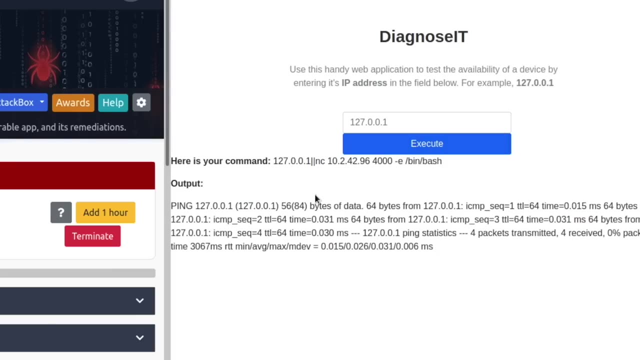 so we'll highlight this. we need to put a port in here, and i think i did 4000 execute. it was port 4000 and it did not reach out. so maybe this doesn't work. we'll try one more time and then we'll move on. and i want to show you one other thing you can try. 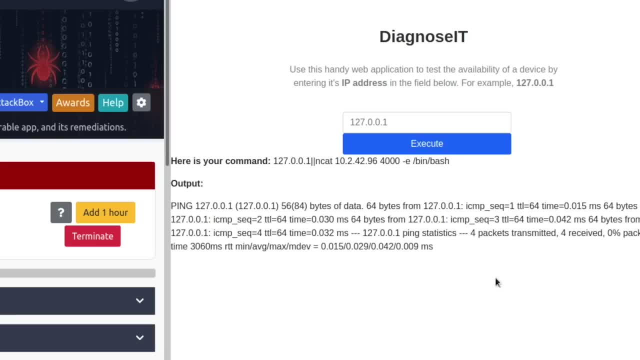 with this. so netcat doesn't work, didn't reach out to us. so one thing you can also do in this command injection, like if you were going to capture the flag, one thing i would do is i would come in here and i would type which python and see if we could get a python: reverse shell. 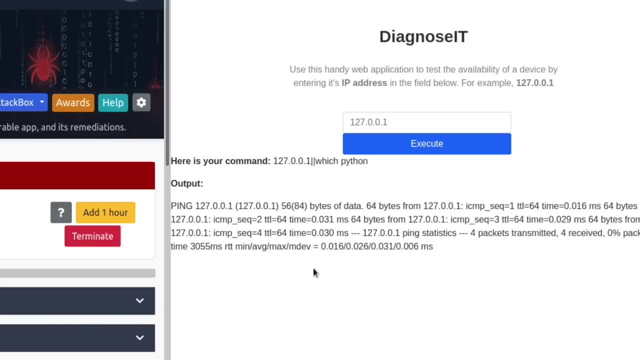 and we can close out of that and let's do something like this so we can get just what we want back here. let's do a command injection and i'm guessing we just, oh, we have python3 so we could try to get, and we don't have any output. let's see. 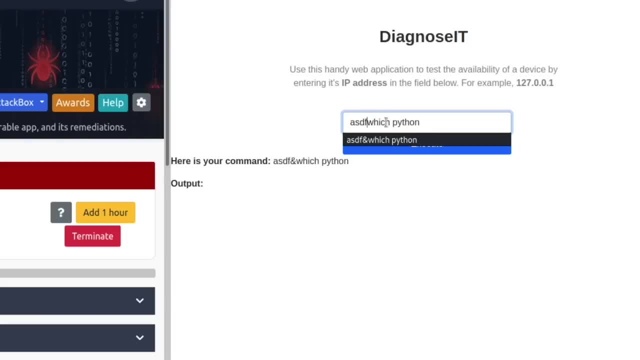 so this, this box might not let us get a reverse shell on it. so i guess we're not gonna be able to figure out what kind of python's on here, but this would be command injection in a nutshell, and i'm guessing we just- oh, we have python3. 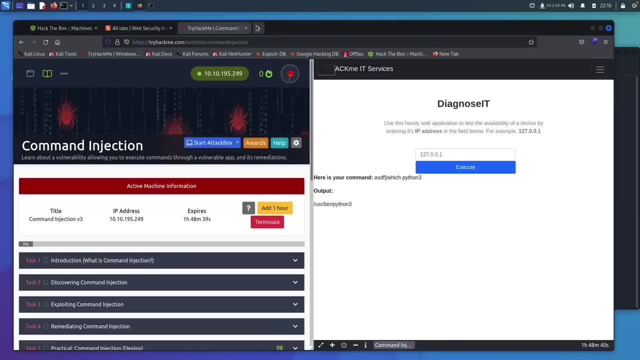 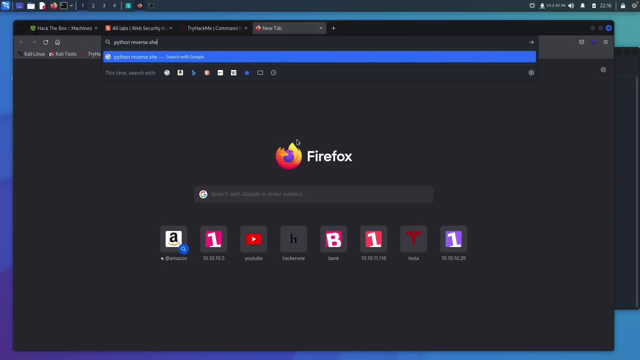 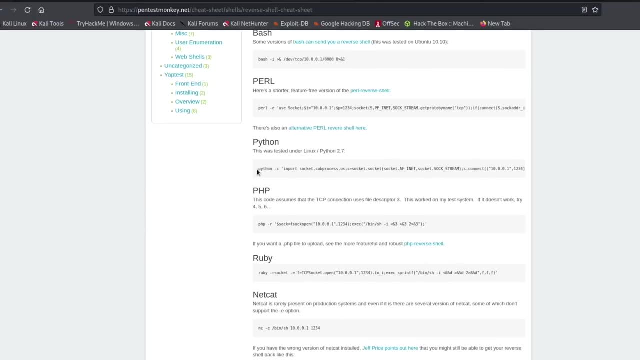 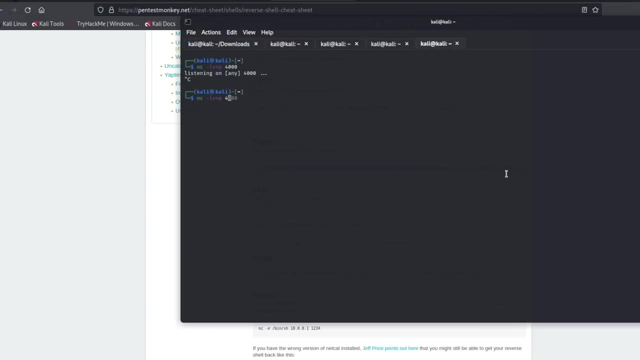 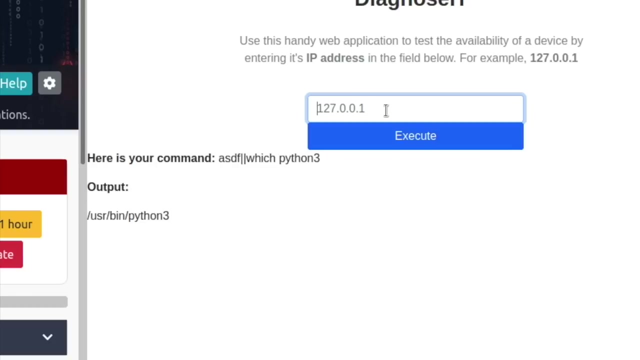 so we could try to get reverse shell with Python. so you could come to Google and we would type in Python reverse shell. we can try a pen test monkey and we could try this right here so we can set up our netcat. listener will go poor, for, for, for and we. 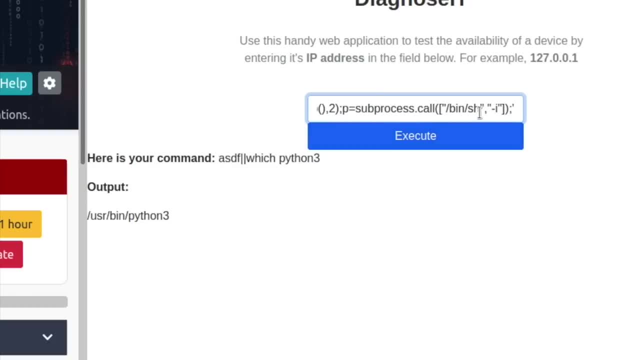 can type something in here: we got been, I want been bash. we have over here, and it's possible that this won't work either, and I would suggest typing something out like this in a text editor: save some time. point 96 and make sure this is: we need Python 3. 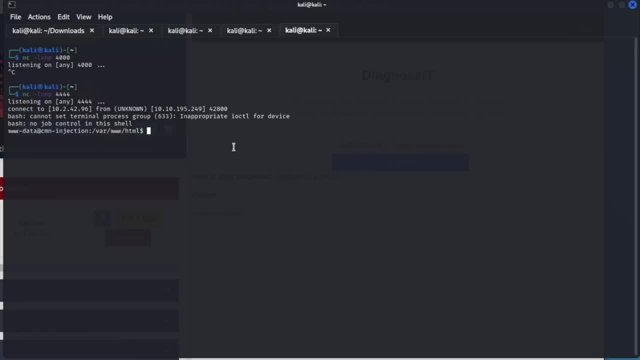 execute and we get a shell back over here. so now, if we say Who am I, we are on the box and if we type in ID, it'll tell us who we are. so you can get a reverse shell this way rather than just be sitting over here with command injection. 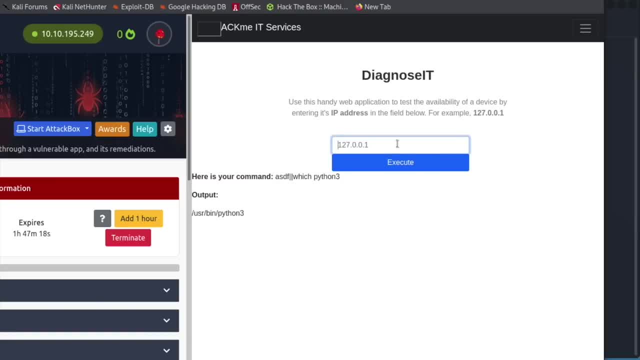 and sorry, I kind of fumbled around there. I actually didn't try that before. we did this little video here. so this is a command injection in a nutshell. this is a great place to practice. if you have a subscription to try hack me, this is a really good place to come over here and practice your command injection. but if 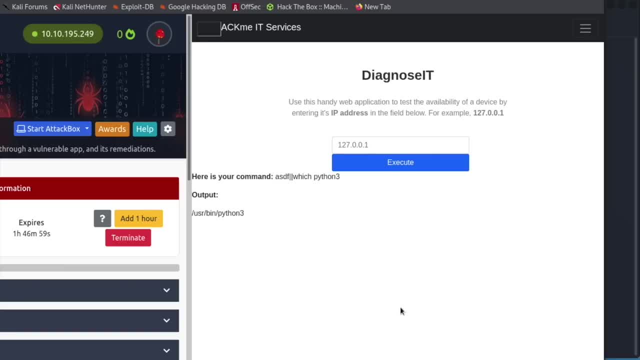 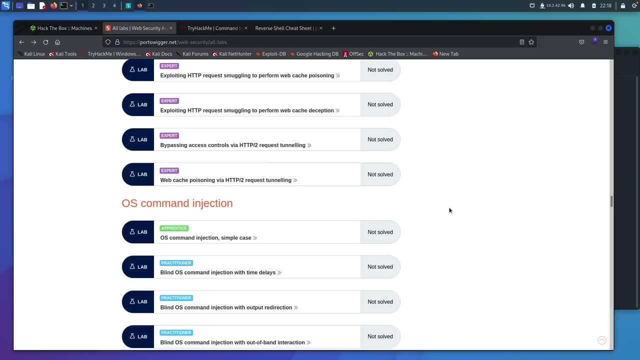 you don't? there is also a free way to practice command injection, and we're going to practice it here in just a second on a port swigger. so let's go ahead and I'm going to get things set up and we will start command injection over here in port swigger, if you would like to go ahead and open up port swigger and get this. 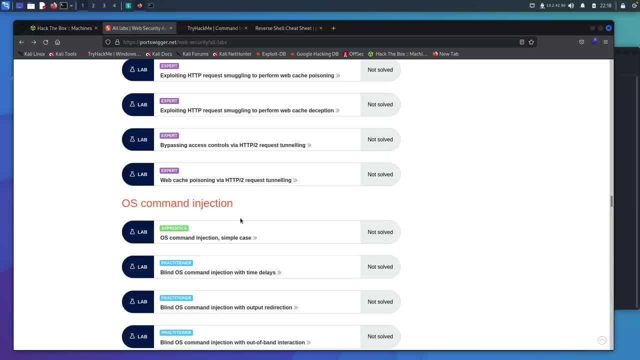 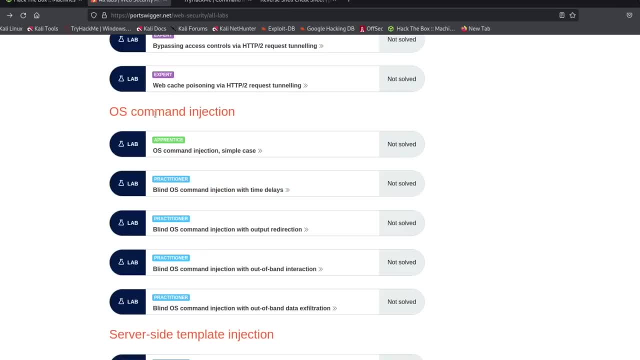 setup so you can follow along or try them on your own. then you can do that, okay. so here we are at port swigger and we are on the os command injection. we're going to do these first three right here, because they're pretty easy and i believe you had to have burp pro for this, and so we're not going. 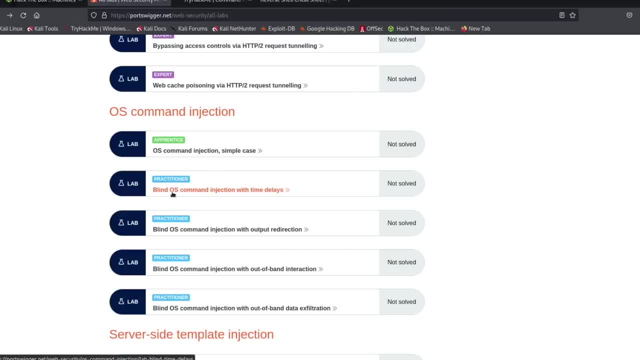 to do these ones down here, but the first three of these are actually pretty easy and you should be able to, i think, solve them. i think you probably could solve all three on your own, but for sure you should be able to solve these first two. so we'll go ahead and open this up. 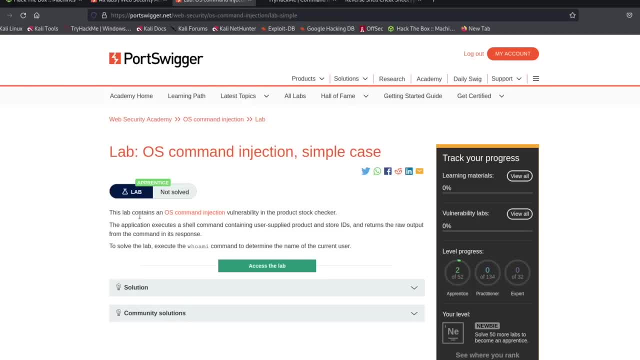 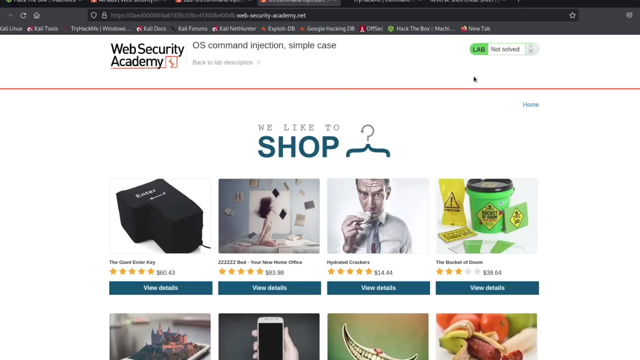 and it tells us this lab contains an os command injection vulnerability in the product id checker. the application executes the shell containing the user supplied product store id. so we've seen stuff like this in the past. so we'll access this lab and it tells us we are not solved because we haven't done anything. so when we have finished this, this should say: 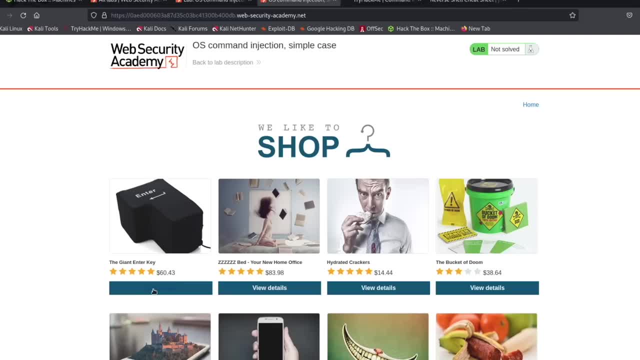 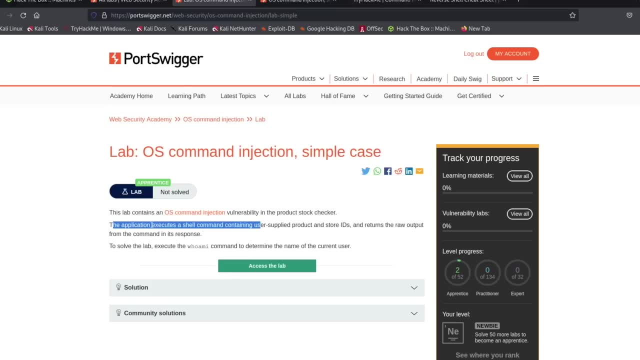 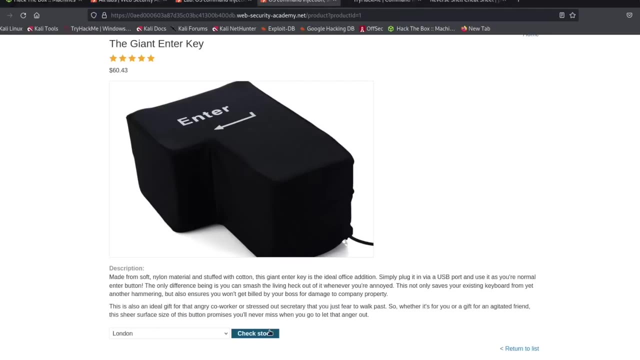 solved up here so we can see what burp is doing. it's doing nothing, it's not hooked up. so down here in the check stock, like we've been doing, and following the instructions right here in the product stock checker, we can forward that we're going to check stock forward and right here is. 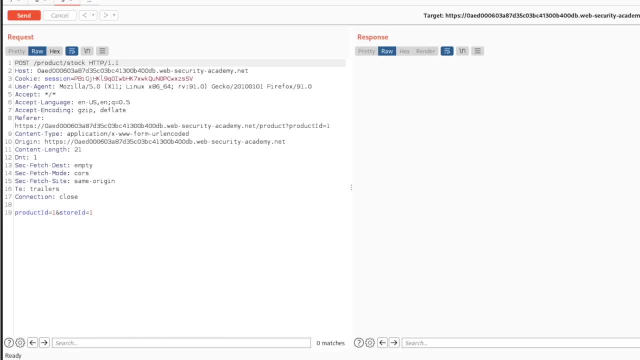 what we need. send that to repeater, we can turn that off and now we have the product id and the store id and this is going to be where the command injection is at. so if you would like to try and solve this command injection by yourself, i would go ahead and give you this challenge. we have found the location and i think you can figure. 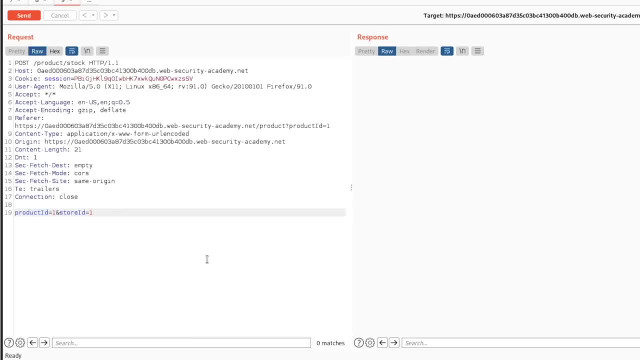 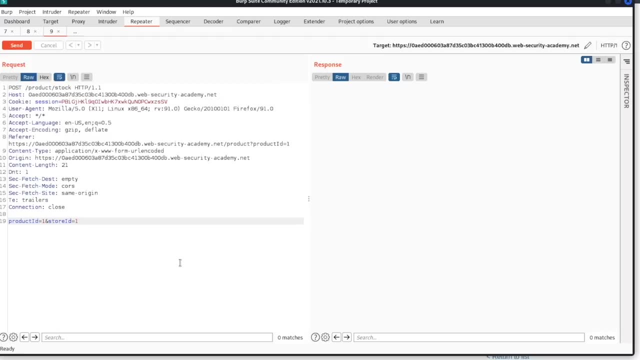 it out. it's right here. you should try and see if you can figure out some of the command injection commands that you just saw previously and give it a shot. but if not, here we go. so we have this product id right here of one, and what we were doing in some of the last ones was we 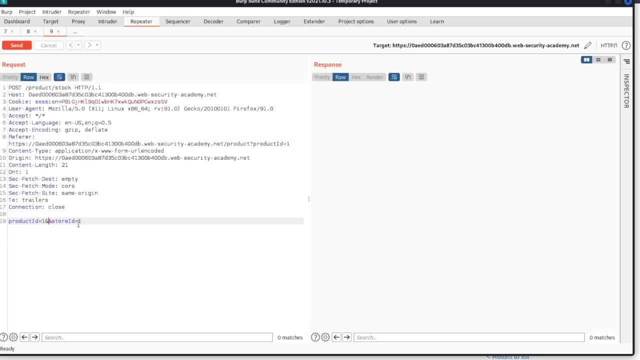 were able to put this and sign in here, but because of the location of the command injection in this post request, we're not going to be able to use those. we will have to use a pipe, and so you can type in a pipe right here and do something like a who am i, and we can send this and see what happens. 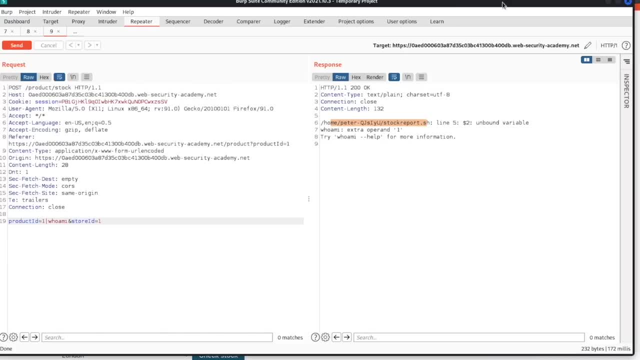 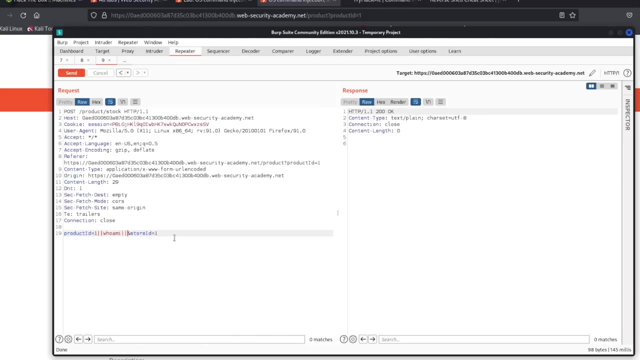 and it tells us who we are. so that's probably right there, so we're going to go ahead and do that. solved this for us, and it did. but while we're here, let's play around with this. let's see what happens if we do two pipes and we send this. it does nothing. what happens if we do two pipes at? 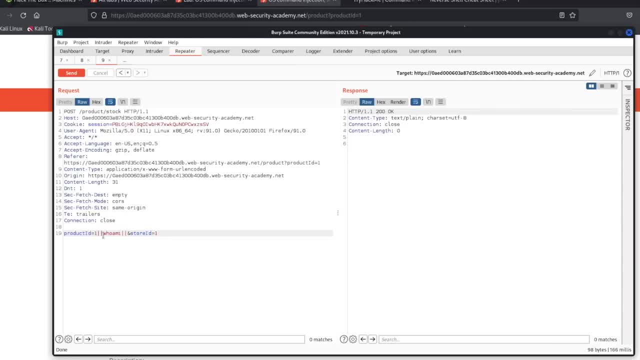 the end and send it. nothing comes back. what happens if we just do one and one- and this is just something that i would encourage you to do, as you find across? you come across things like this, so we actually have it come back with a pipe at the end, in the beginning. what happens if we change? 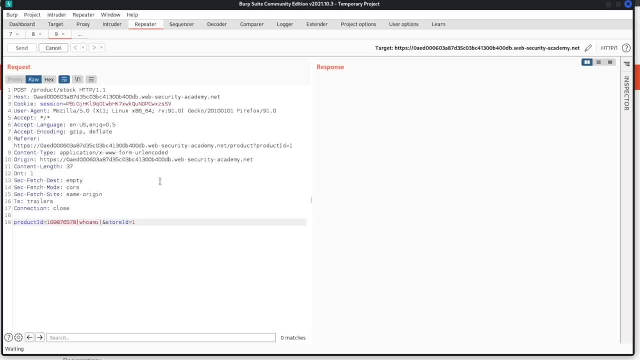 this to very clearly: a product id we don't have and it still works. what happens if the product id is wrong and we have two pipes and we send it nothing? now what about this store id right here? what if we try two pipes and we go, who am i? 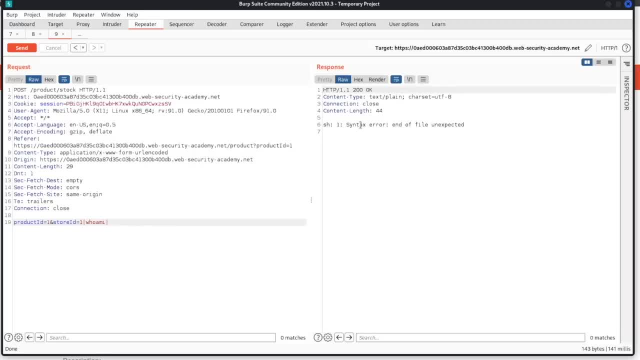 it gives us a syntax error. what about two pipes? and we send it? it gives us the same thing. we can come over here and maybe we can say an id. it tells us who we are, and so you can really just play around with this and see what happens. what if we put a crazy id number in here? it still works, and then you can. 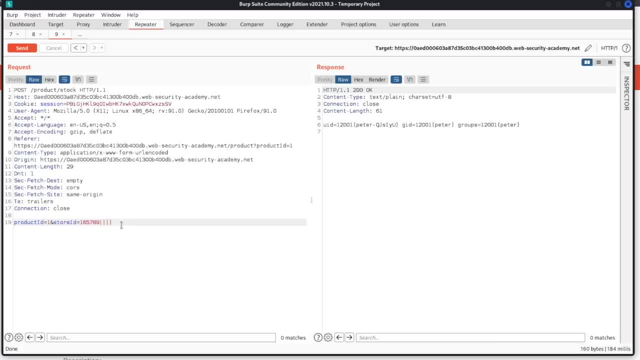 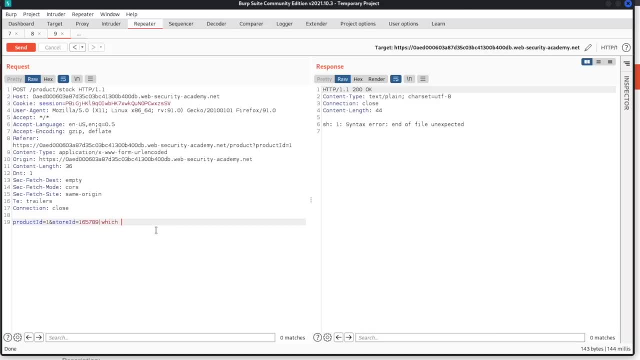 just mess around with this and see what works and what doesn't. if we check it, who am i? syntax error. we could go which python, like we did before, and this is black because it needs to be url encoded, which is a plus sign, and we don't get. 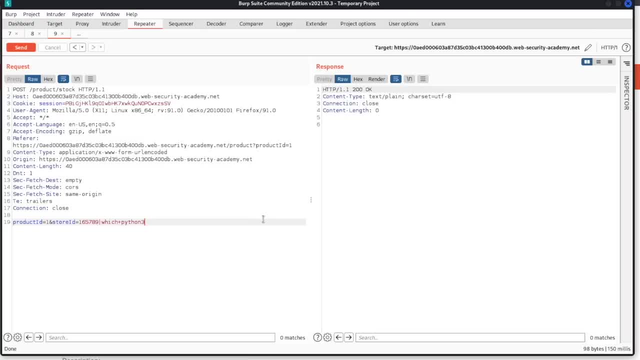 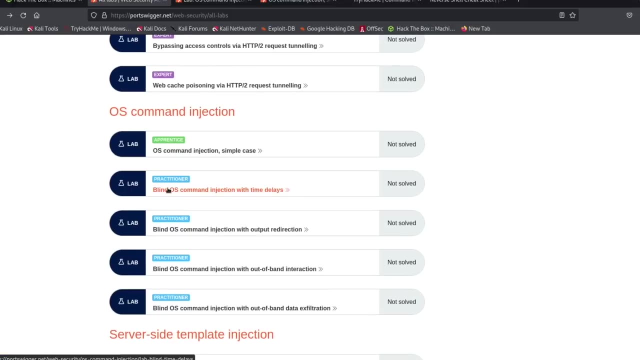 anything back, and i don't think that you're able to get remote code execution on this. so here we go. this would be your command injection right here. we're going to try and do another one on this lab right here. so if you would like to go ahead and open this up and read the instructions, then i. 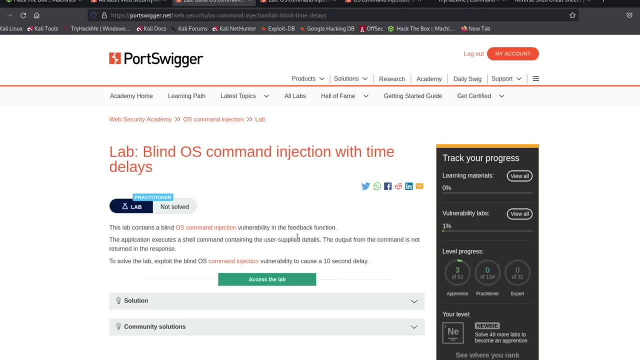 would say: go ahead and see if you can figure this out. i'm not going to read it just yet. i want you to go ahead and read this and try and figure it out on your own, and if you get stuck then we'll go over it, okay? so this says the lab contains a blind os injection. so if you're familiar with the 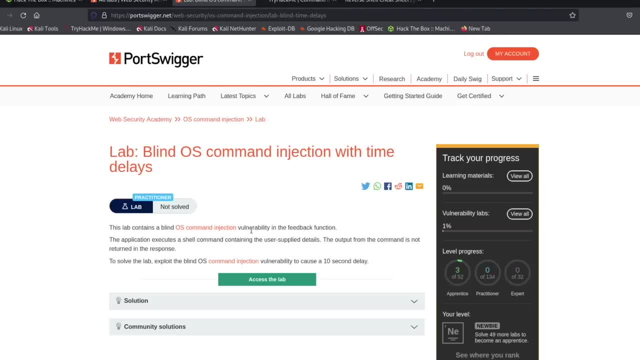 bug bounty- for beginners, of course, that i already have out- then we know that a blind injection means we're going to have to do some kind of time delay and it's not going to tell us what's in the response. so we have a 10 second delay in order to solve this challenge and it 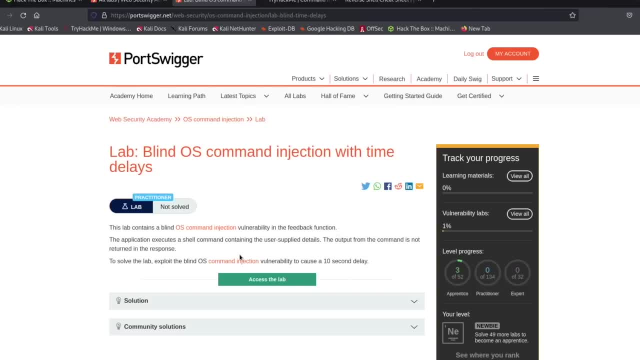 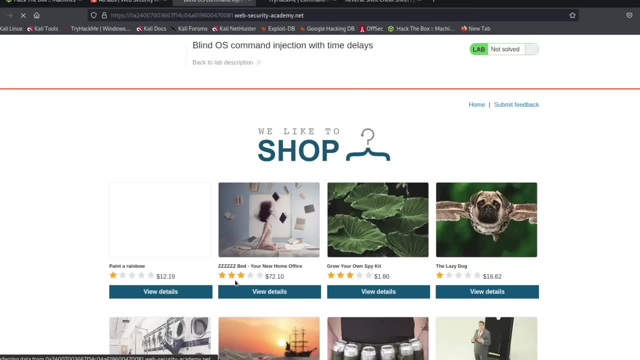 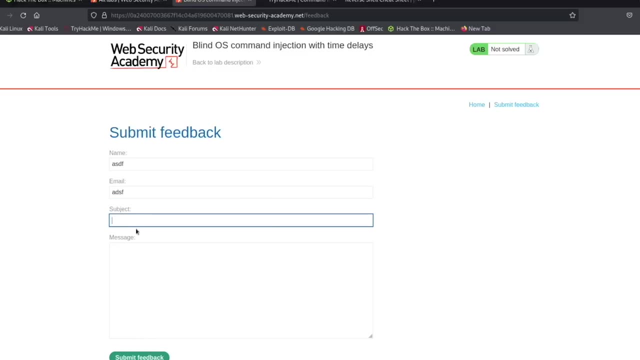 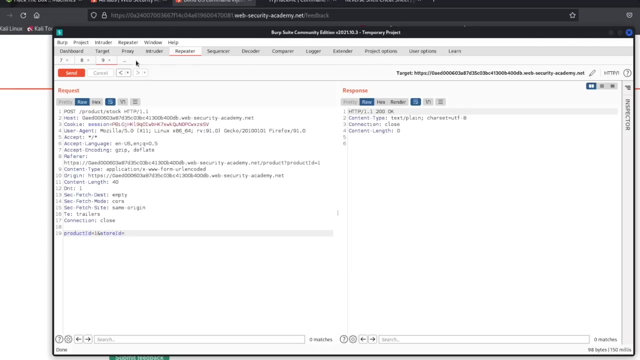 tells us that the vulnerability is in the feedback function. so with this you can go ahead and open up the lab and we have this, submit feedback right here and we can just type in a bunch of gibberish and i think this is going to ask for some kind of ending for an email account and we can come back. 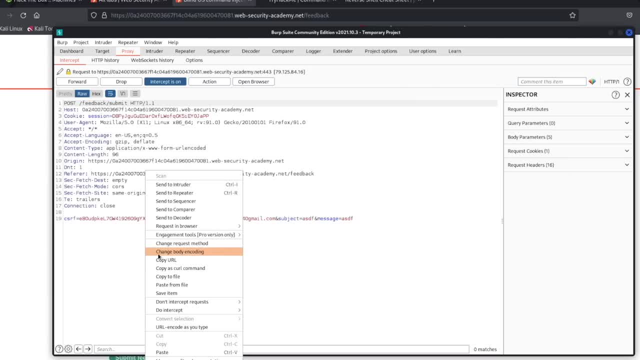 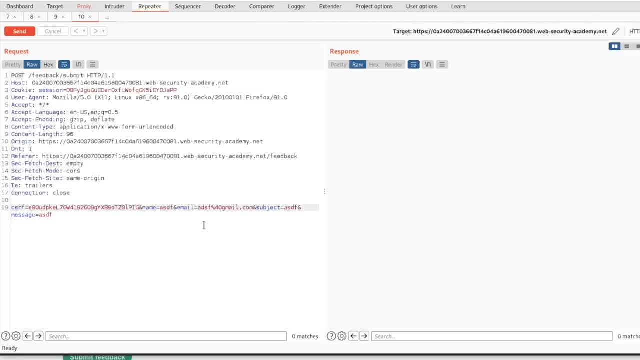 and intercept this, send it. we'll send this to repeater and it is possible that this took you much, much longer to figure out because we have a bunch of different parameters in here that we are testing against. so we have the name right here, so in a time delay we 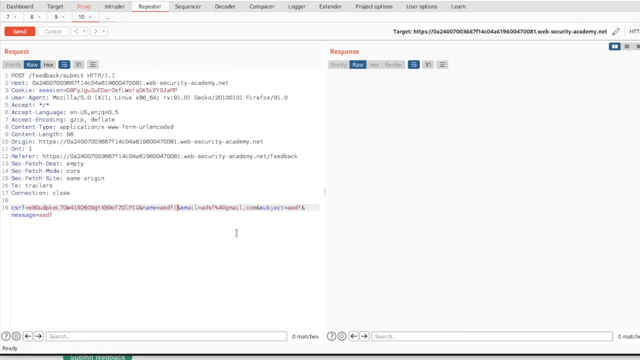 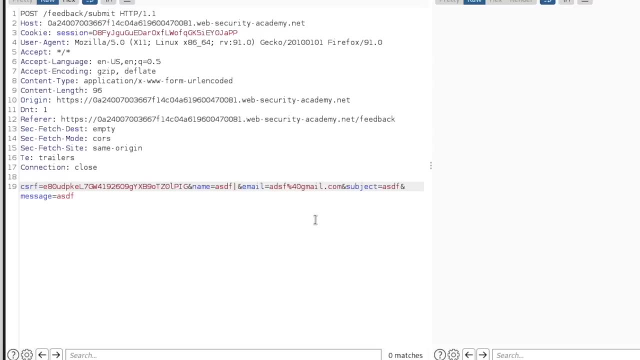 saw this in the try hack me example that i i showed you. you're going to try and do a ping against the server itself and wait for the time delay. so what we would do in a time delay- command injection or a blind command injection with a time delay- you will type in ping and then we have. 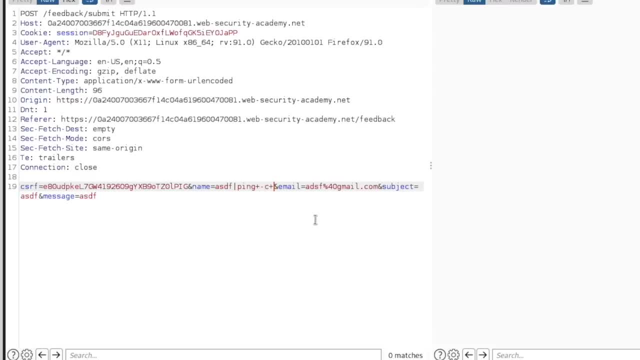 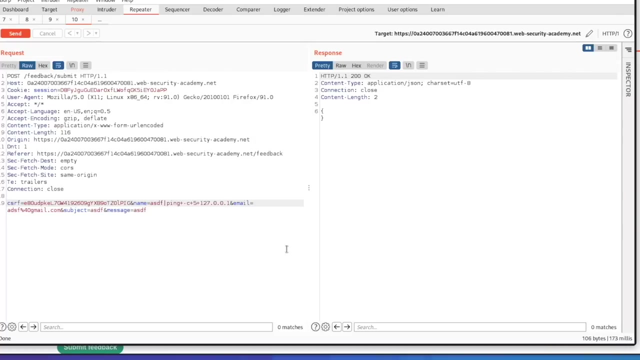 to url, encode it and it will look just like we did previously. i'm going to do five seconds to start out, so we don't have to wait: 27.0.0.1, and then, if we send this, we'll see right here. this should be like four or five thousand. 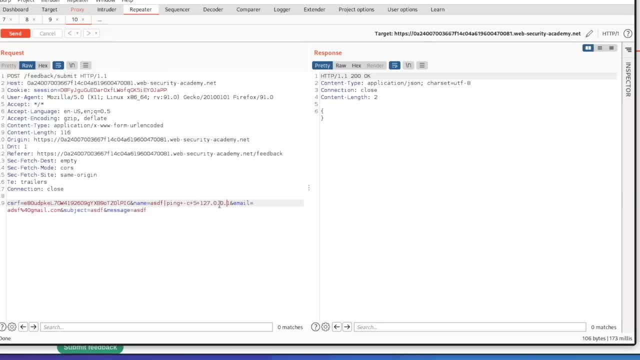 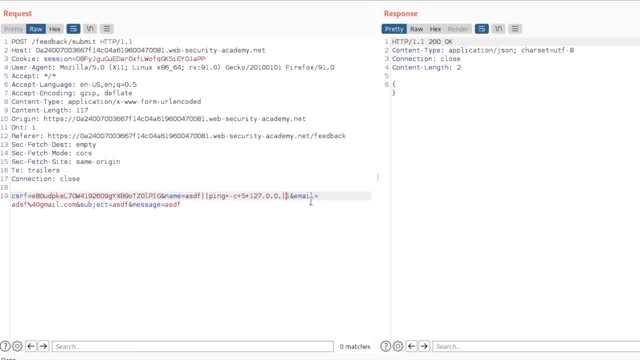 when it actually works. so we can try a pipe at the beginning, pipe at the end, we can try another pipe, and i see that i made a mistake. i didn't have the one in there, so we'll try this again and say go, still not long enough. 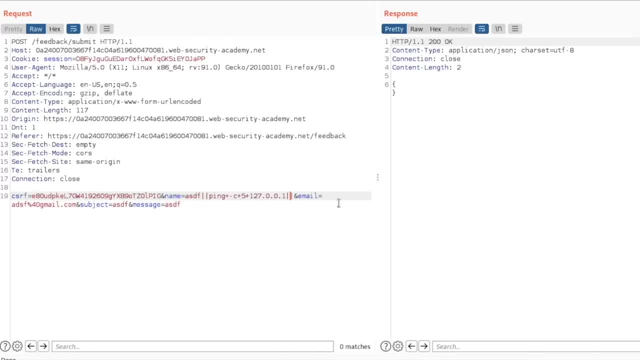 we can add in another one and see if this works, and it doesn't seem like this is going to be our spot, otherwise one of these would work. we can't use the and sign in there, so we'll just move on to the next one. we'll say: pipe ping, and i have this. 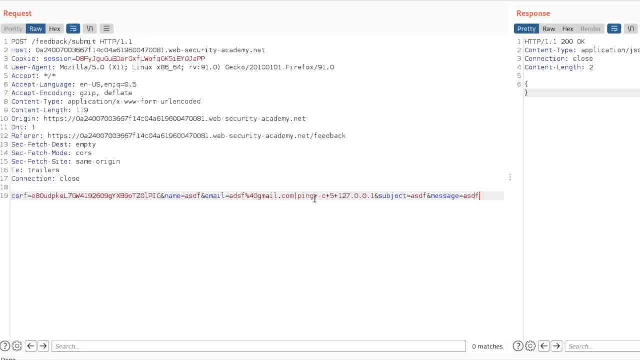 i fast forwarded typing this in so you don't have to watch it again. so we got our pipe and our ping command. we can send this. we'll turn this proxy off and we can see that it's working. and we can see that it's flashing. we can see that the time did not work, so we can throw a pipe on the end. 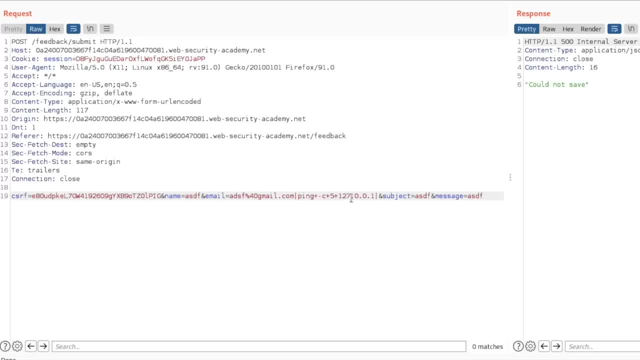 send it not long enough. let's try two pipes and we can send it, and our time is much longer and we can see that it was almost five seconds. so now to solve this, i believe we can type in a 10 right here and send it, and this should. 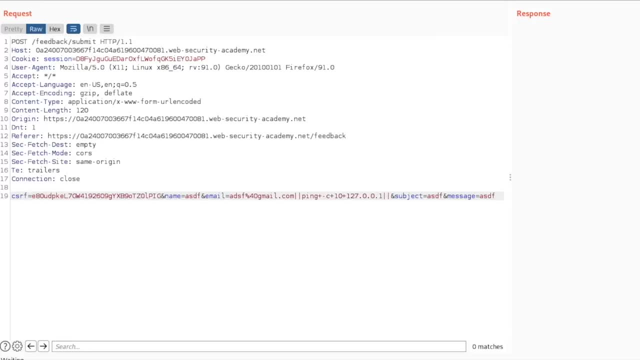 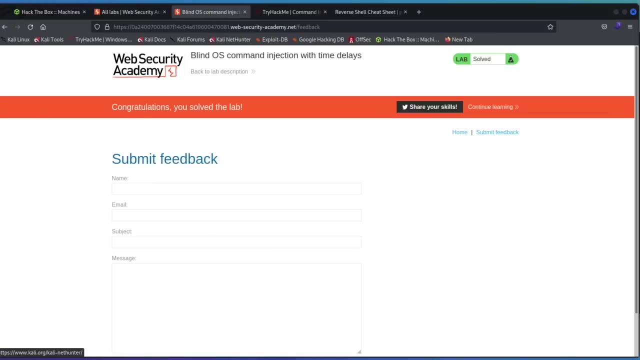 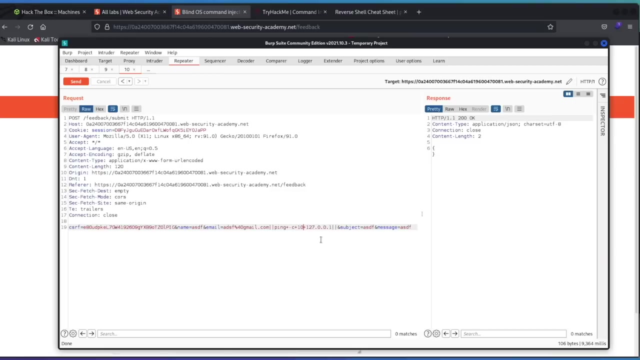 give us the solve, because the five seconds was pretty close so it's not solved. and it just came back and it tells us that it has solved. so this is a timed command injection or a blind command injection. this is how you test it: with a ping against the server itself and give it. 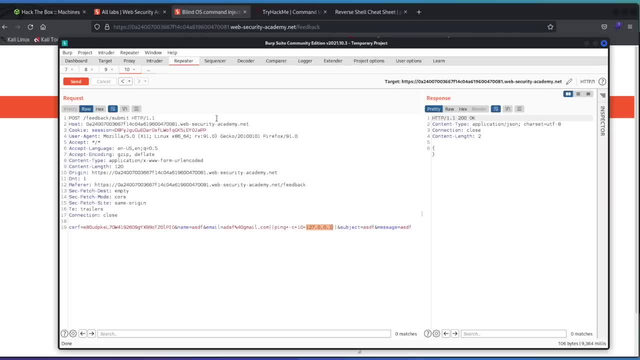 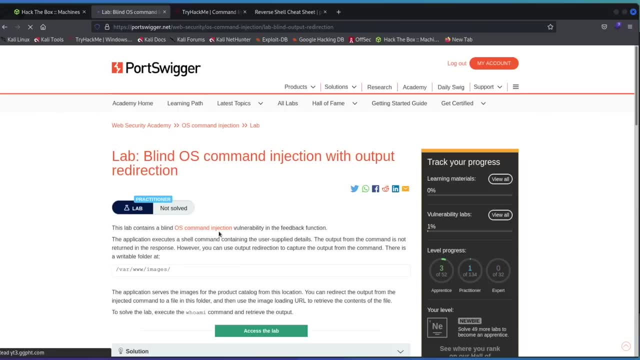 a time delay. so with that we're going to move into the last one of our command injection labs. this one is going to be a lot harder. i think you can figure it out if you've done the my bug bounty course and you've also gone through my free ethical hacking course, because the ethical 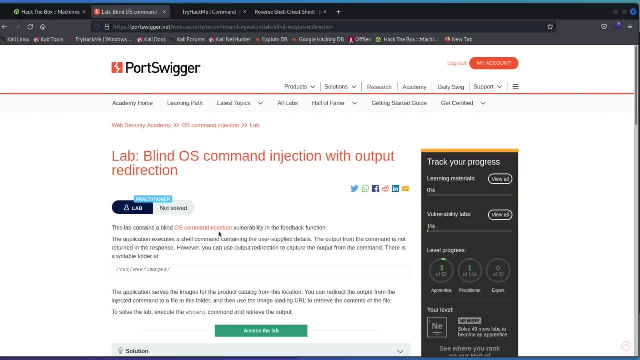 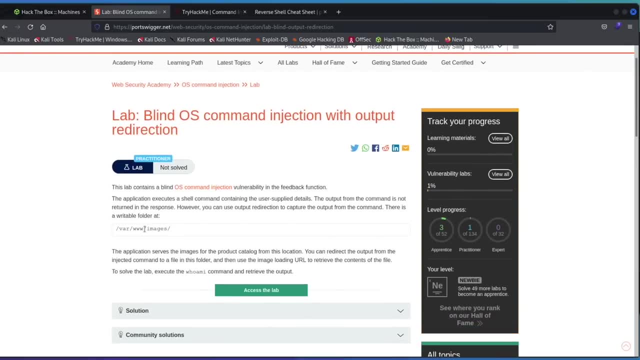 hacking course is going to cover things that are kind of like this when you get into the actual penetration testing portion of that course. so if you've gone through both of those, i think you can solve this. if not- and you're pretty new, you're probably going to struggle with this one. but 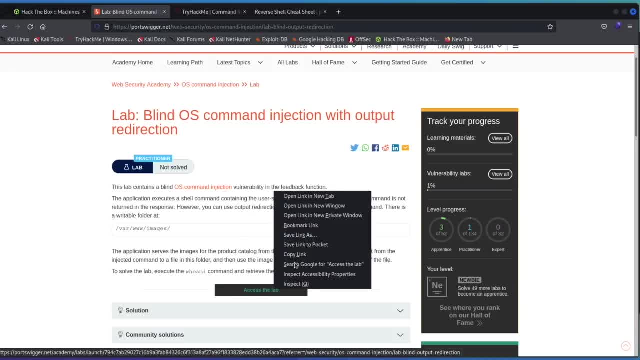 we'll go ahead and solve it anyway. so we'll open up the lab in the new window and then we'll read what it says. so it has a vulnerability that is blind. in the feedback function, just like we had before, the output is not returned in the response, like before. 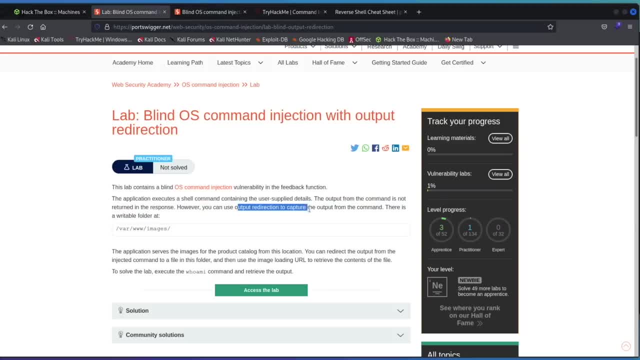 however, you can use the output redirect to capture the output from the command and it says that we have a writable folder, and then it tells us to solve the lab, we need to execute a who am i command and retrieve the output. so what we're going to end up having to do is send a who am i command? 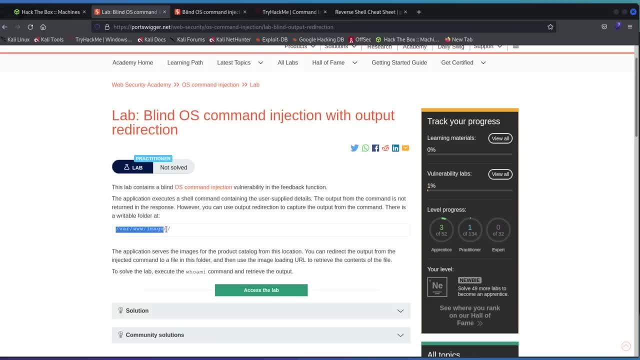 to the server and then we're going to have to save it in a file inside of this images directory, so it's going to be var dub, dub, dub images and then the file with an output. so if you went through the ethical hacking course, i think you can solve this. if not, we'll go ahead and solve it together now. 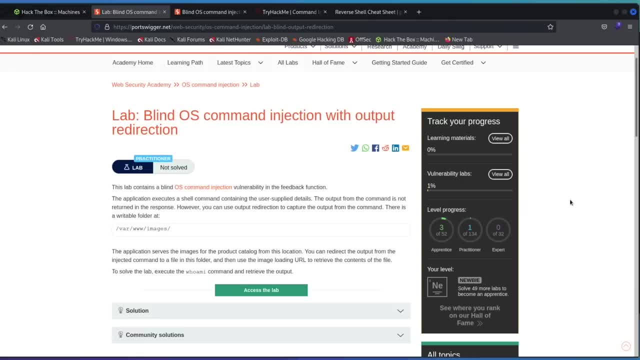 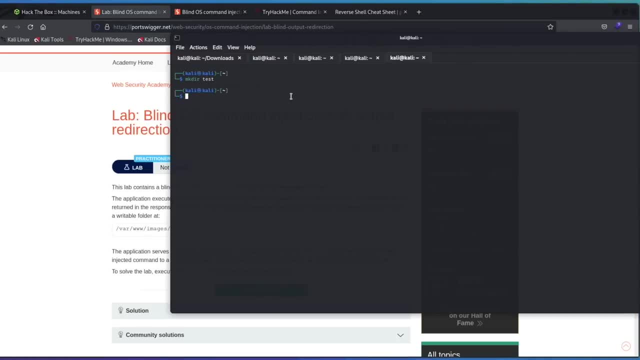 so i just had an idea. if you want to try this on your own, um, i can actually show you over here. we can make a directory and we'll call it test, we'll cd into test, cd to test, and then what we can do is if i type in: 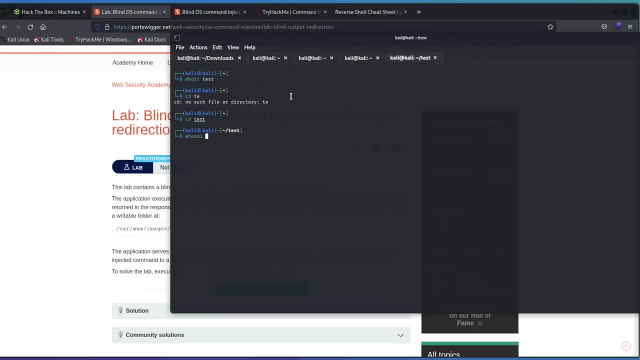 who am i command? who am i? i can send this command and i can put it in a file dot txt. and now, if i hit enter and then we cat will ls- you can see this files here and i cat out file dot txt. it tells us that we. 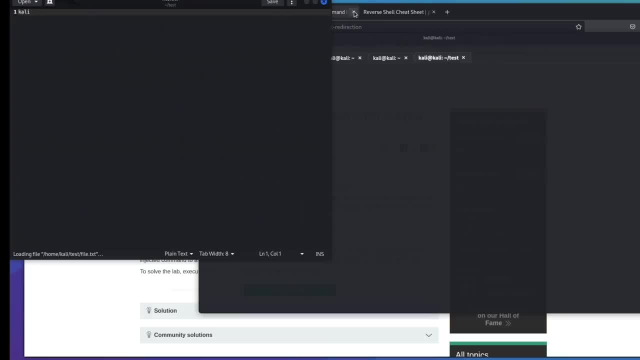 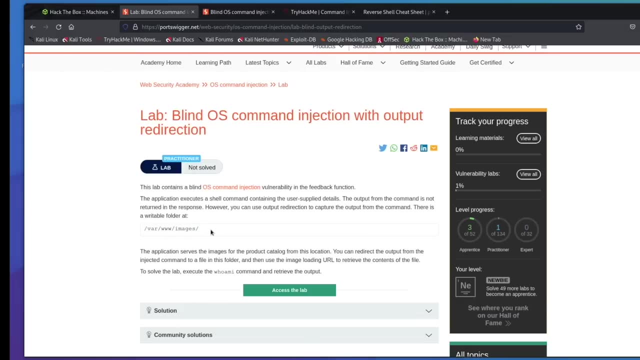 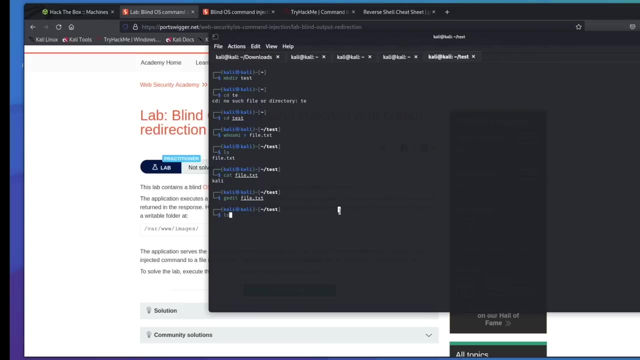 are cali or if i g at g edit this file, it'll save the response in there. so we're basically going to be doing this right here, inside of this directory, right here. so what we're going to do is give a command to this file and we're going to say: who am i like, like we did up here. only it's going to be 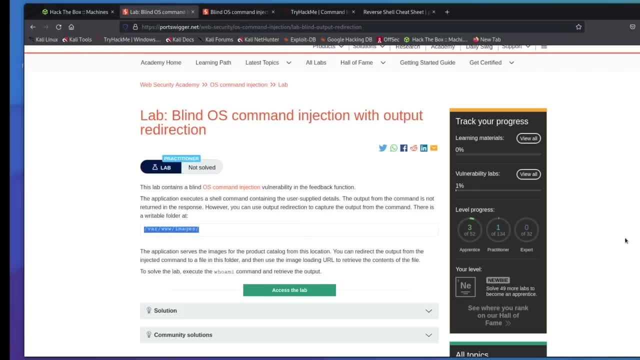 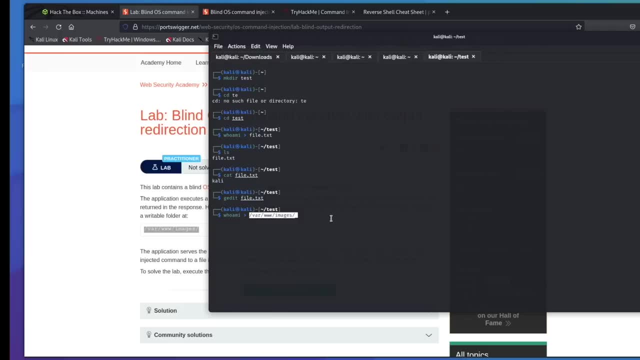 in this right here, and so your command is going to look like this, and if it has to be url encoded, you'll need plus signs right here. um, if not, you can just you might be able just to delete this and do it with no space, and then you're going to need to try and retrieve the file with the. 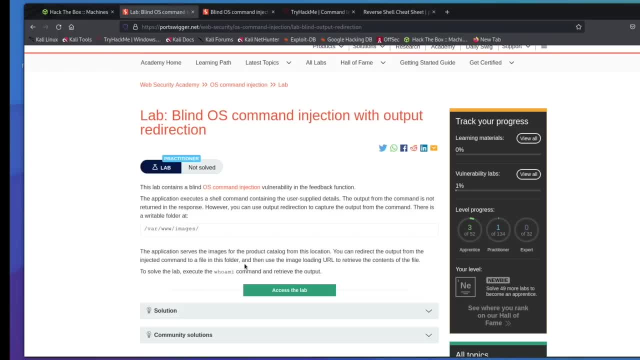 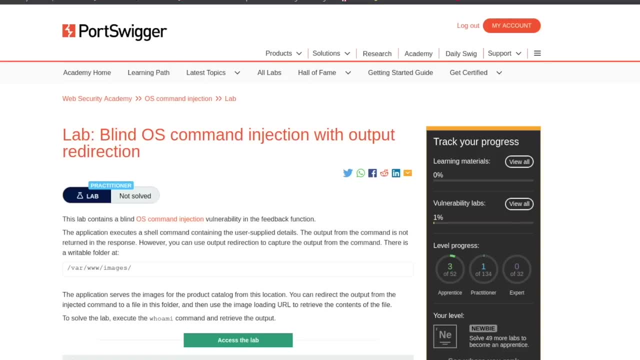 command injection, and i want to see if you can figure this out, so i'm going to go ahead and do it. so go ahead and give it a try, now that i have given you a hint with this clue right here. okay, so let's go ahead and solve this challenge. it said it was in the feedback, so we'll come back to. 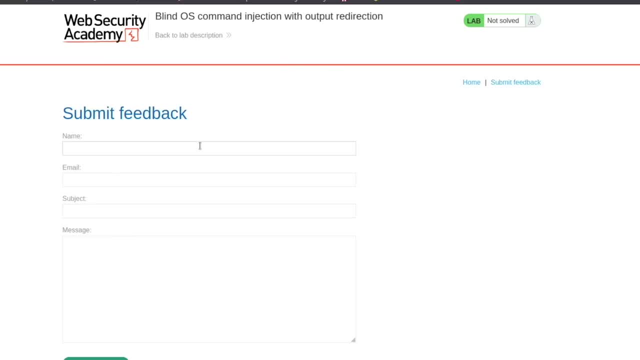 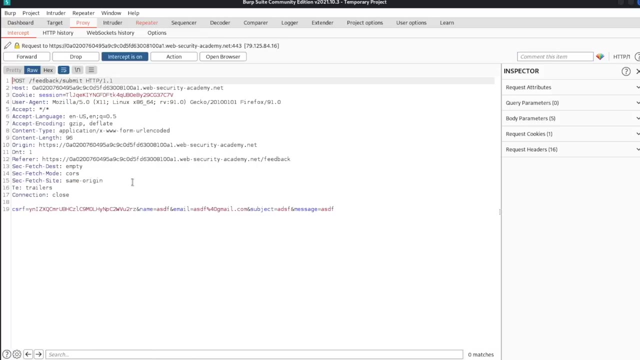 the proxy we can come to submit feedback. we'll do the same thing we did before and just type in some mumbo jumbo at gmailcom and turn our proxy on, submit feedback, send this to repeater, turn the pro, turn the proxy off, and so here we are, at this same page we were at. i'm. 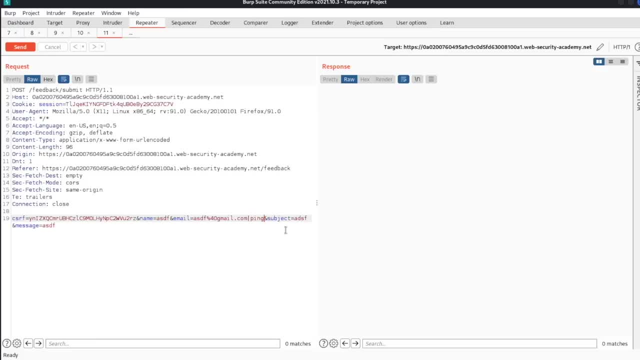 actually going to make sure that this is in the exact same. the command injection is in the exact same place, so we don't spend a bunch of time trying to send this somewhere that it's not so, we'll go ping. so i wrote the ping command out so you didn't have to watch it. i sent it and we'll. 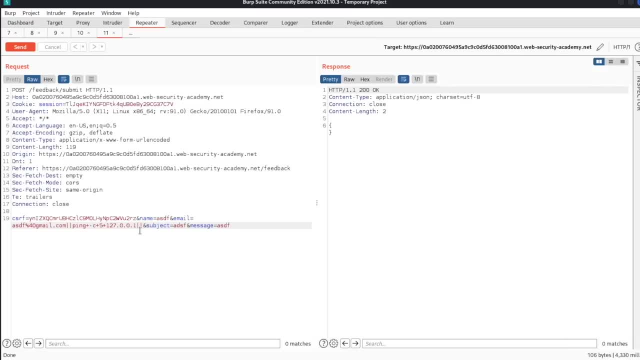 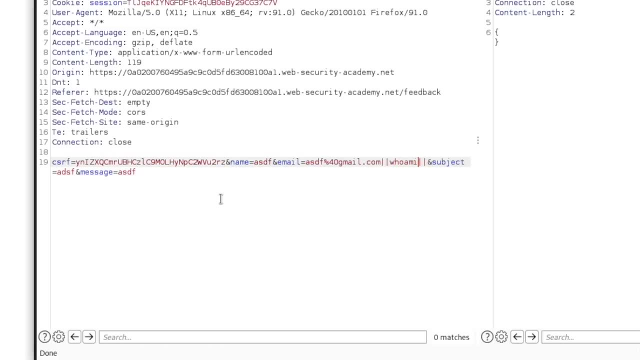 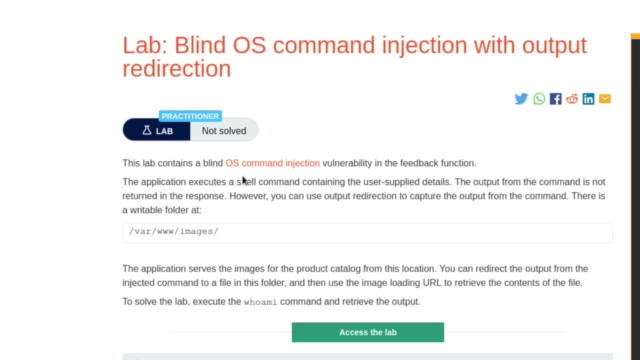 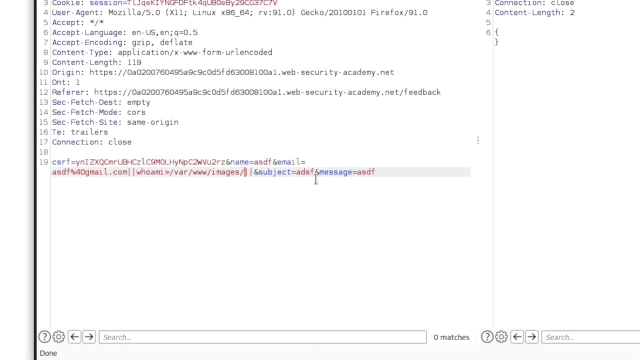 see it was a five second delay. so the command is the command. injection is in the same place. so we should be able to come in here and say who am i, and then we'll give our caret, and then we'll give it the location that we were supposed to give it, right here. paste that in. 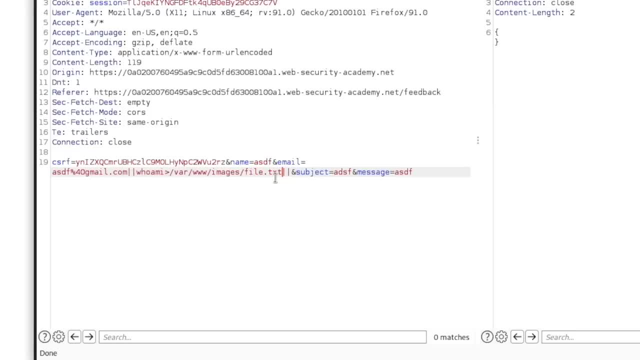 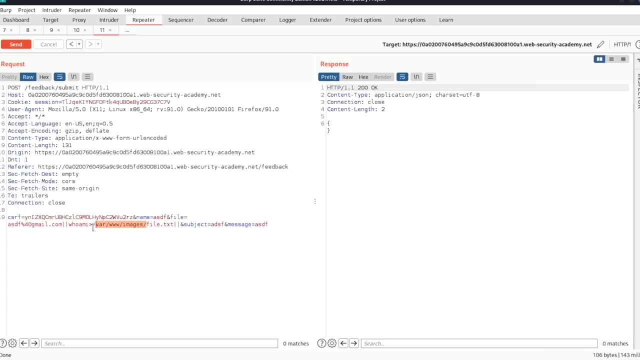 and then we'll say file dot txt, and send this and hope that it worked. and now i think the way to check this is going to be: we'll need- i think it'll be- file, and then we'll want to read this file dot txt, so we'll send this. okay, since this right here, 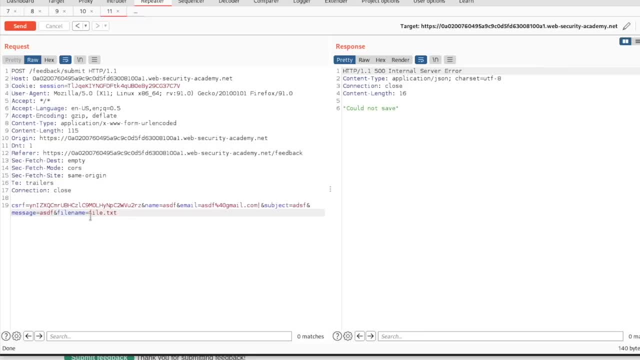 isn't working, we're going to just go ahead and assume this is not going to be in the right place. so what we can do with this right here is: we know we had to send it into the var www, and i think it was images, and then it was our outputtxt, which is where we, and then it was our filetxt. 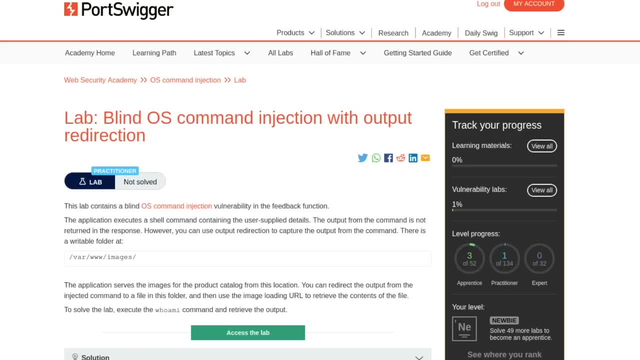 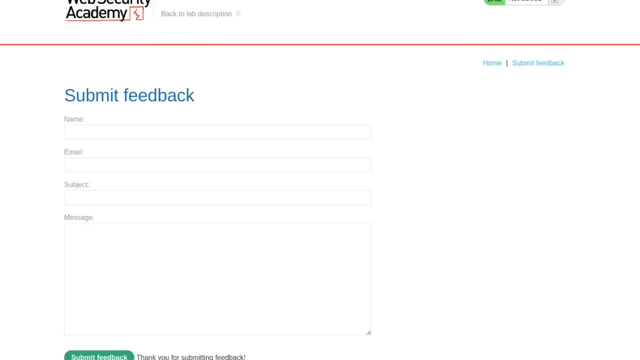 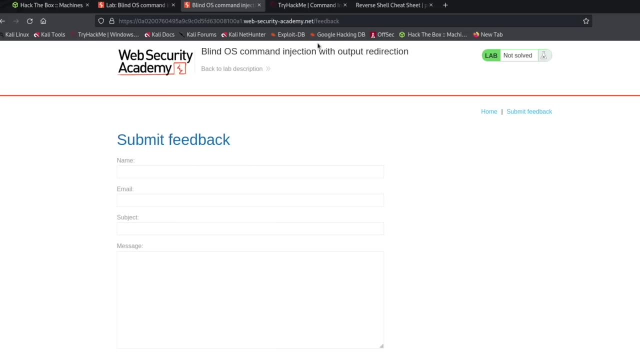 which is where we put our command. who am i right? that's what it says we do. yes, it's in the images. so what we're going to probably have to do at this point is find the images, because we're not able to pull anything from here. so what we'll do is go to the home page and see if we can pull. 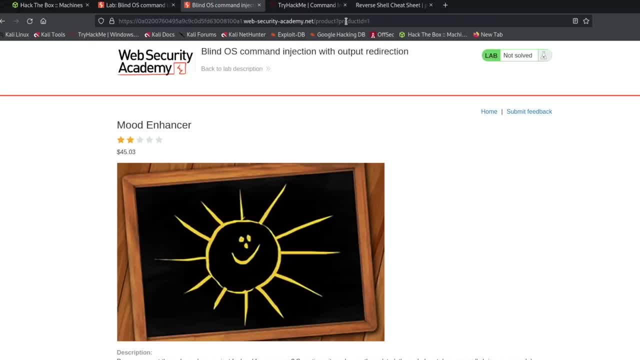 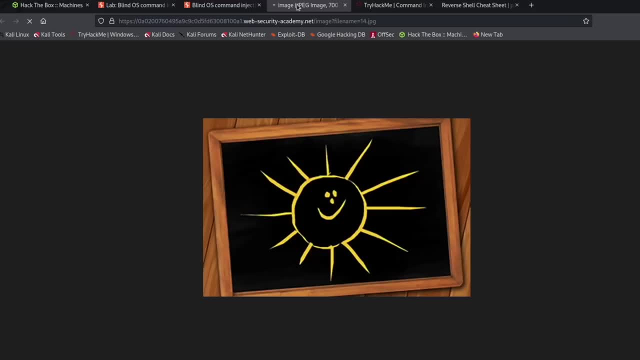 an image somewhere around here. see, we have the products, we have the product ID, we have the image. okay, so we right click the image and hit open image in new tab and we have the image and now we have a file name. I bet we can do this without burp and then, if we can't, we'll open it up and burp. so 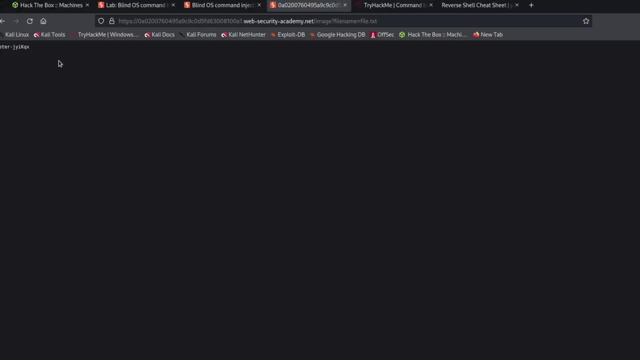 we'll type in filetxt, which is where we put the file, and it tells us who we are as the user. so that's one way to solve this challenge. it was a lot more- this one was a lot more difficult- of a command injection. in the real world. you wouldn't do anything like this the only time you're going. 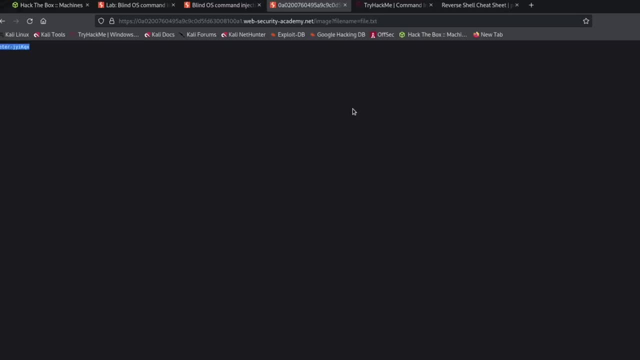 to do something like this isn't a CTF. or if you were on a live pen test in the real world in a bug bounty, what you would do is probably just send a ping with a time delay and submit that and you would stop right there. but because this is a CTF, it wanted us to grab. 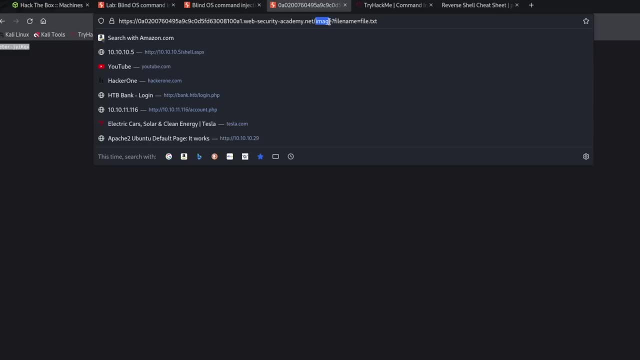 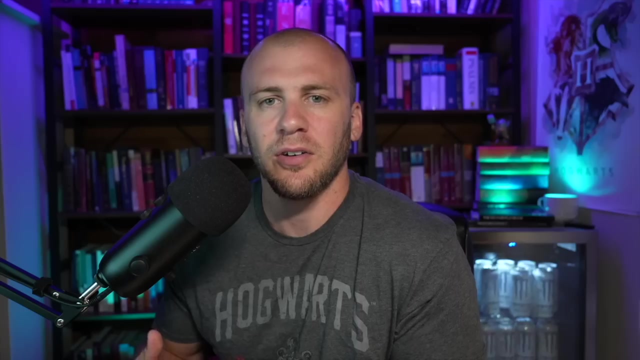 this user right here, and this is where we did it. we saved it in images and we needed the file name and the filetxt. so that is the last of the command injection that we're going to be covering and we'll move on to the next vulnerability. all right, in this portion of the course we're going. 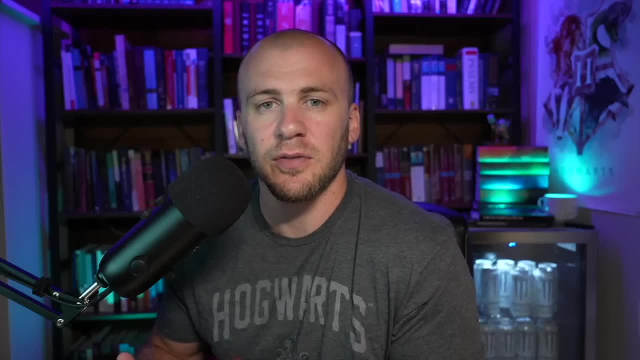 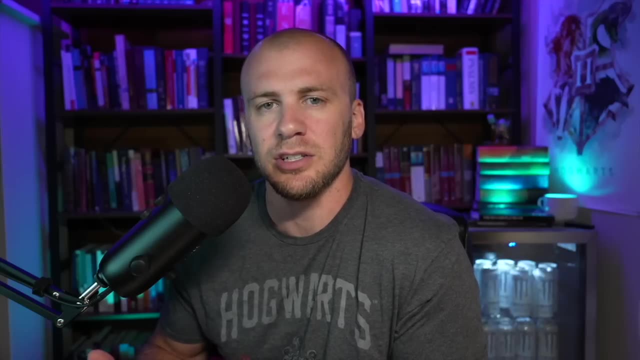 to be covering file upload. this can be a severe vulnerability, especially if the file is placed somewhere that you can execute what you have uploaded and get back a shell on the server. so file upload is one that you're going to see. a lot in CTFs they do. 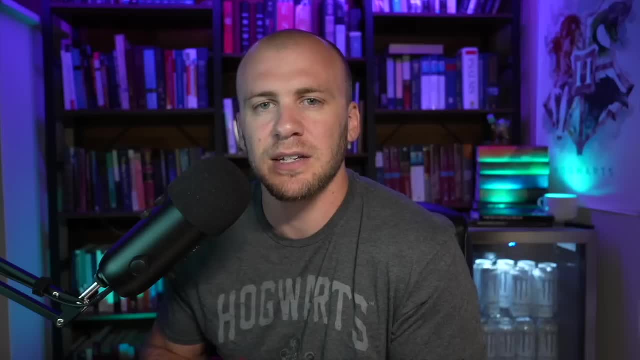 happen in bug bounty programs. you can go and read on the activity about some file uploads. but in the world of bug bounty hunting most of the time they're probably not going to lead back to a shell. but in the world of penetration testing and CTFs or if you're going for any kind of 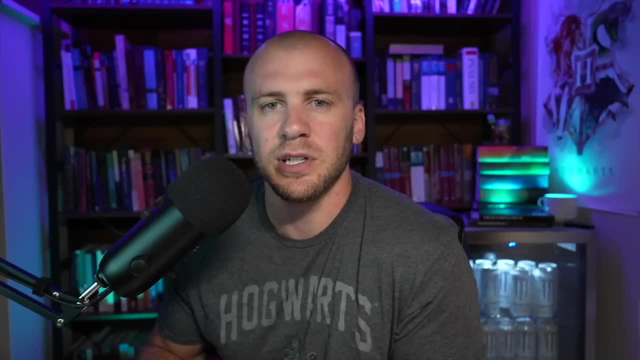 creation to become a penetration tester, then file uploads are always a good place to look and make sure, when you're uploading a file, to see if you can bypass any of the filters that may be keeping you from uploading a specific file with a payload inside of it. so with that, let's go ahead and jump. 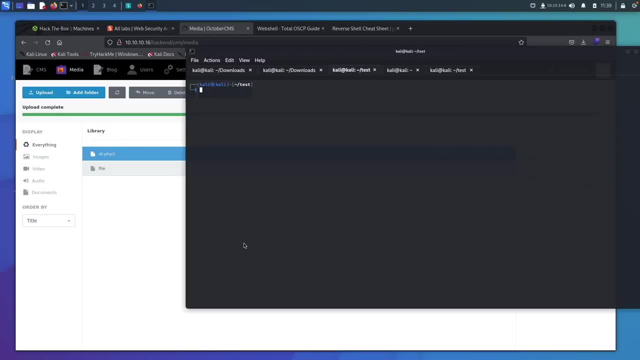 into it to the file upload. so we're going to be going through a few hack the box file uploads. and the reason we're going to be doing hack the box is there really is no great place to practice file. the box really has the best systems to practice file upload. if you have a hack the box, subscription. 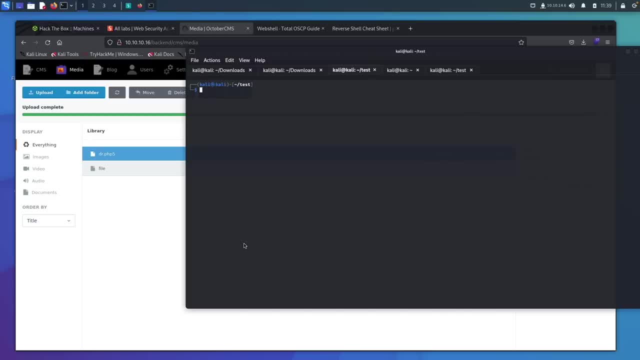 then you can open these up, you can play around with them yourself and actually test these out, if not, in the world of bug bounty. if you go to the activity, you can read about file uploads happening all over the place. so file uploads do happen. we're going to start really basic and then we're going 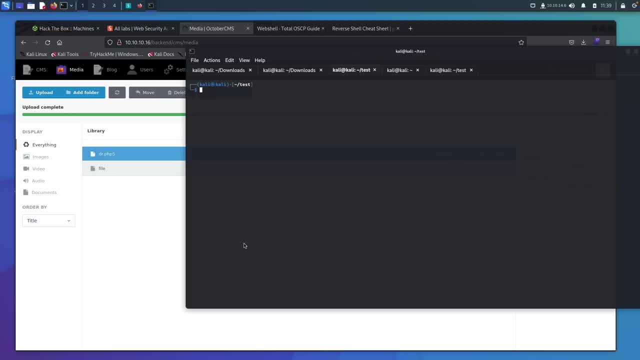 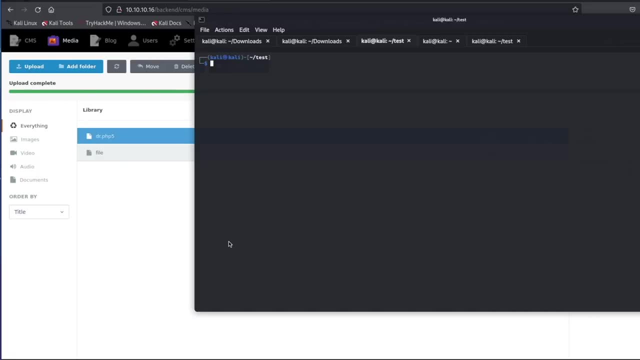 to have to go through bypassing different filters within the file upload, so this one is really one. the box is called October with hack. the box and its IP address is right here, and I'm not going to show you how I got to this spot because really we're just. we just want to see the file upload in. 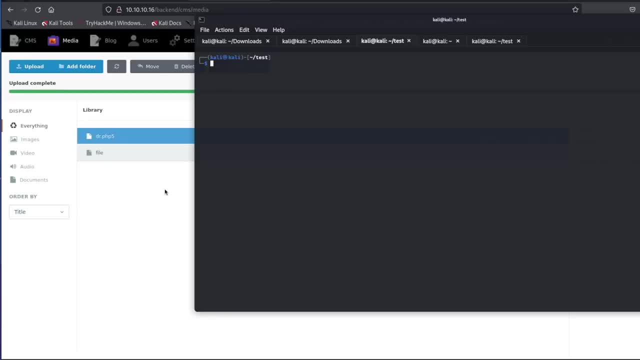 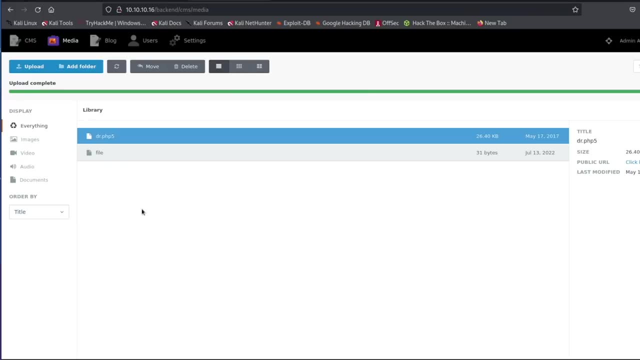 action and what happens and why. this would be a really huge vulnerability in the penetration testing world. so the first thing we're going to do is we can click this file upload, and I tested it. you can upload a file right here, and so what we're going to do is we can just click. 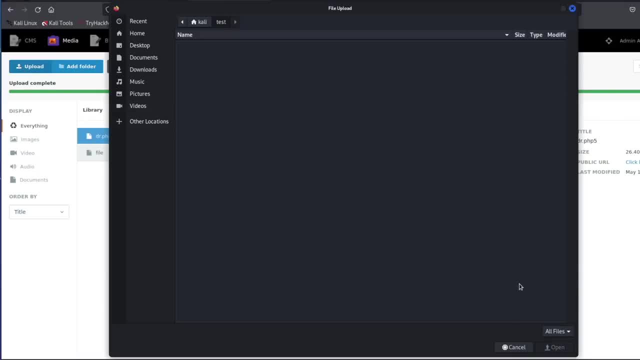 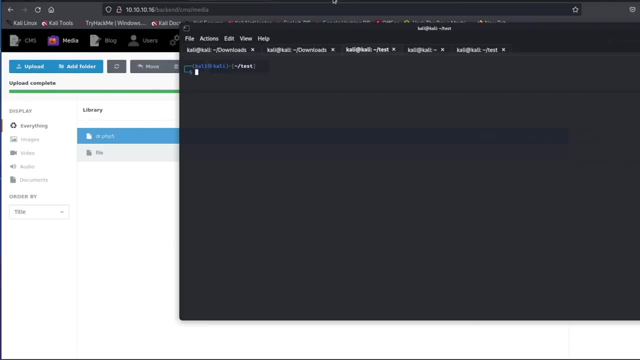 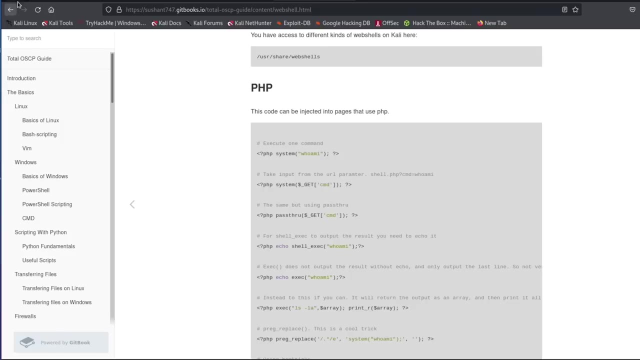 the file upload button, and I'm going to show you two different ways to go about uploading files and testing this out. so the first is with a web shell, and what we can do is we can come over here, like we did before, and what we can do is we can go to Google and just look for web shells and I 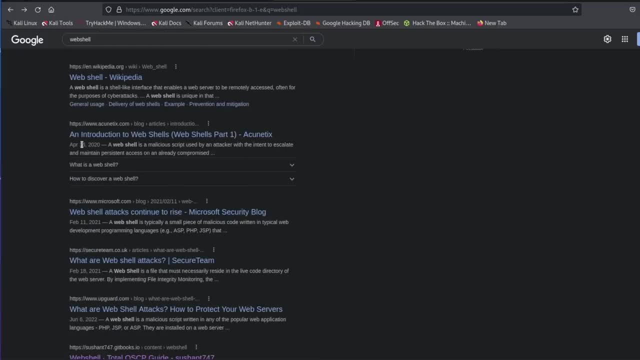 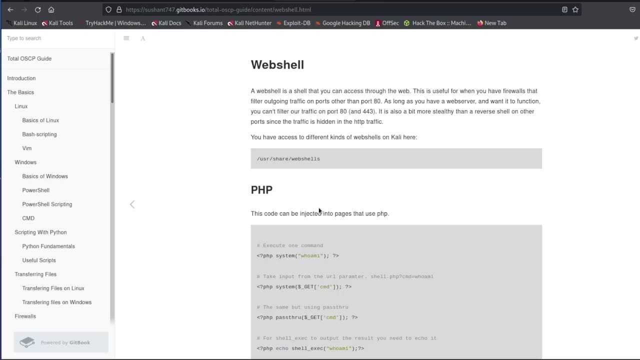 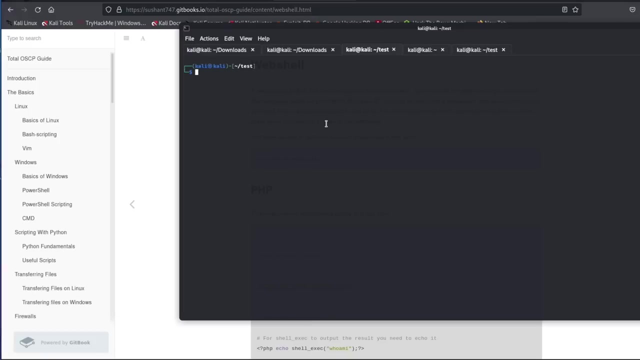 can just show you right here. I just typed in a web shell and I scrolled down until I came to the shoe shant 747. clicked on it and we're brought to some PHP web shells. this one right here is one of my favorites. it's the one I use the most and we can just say that. 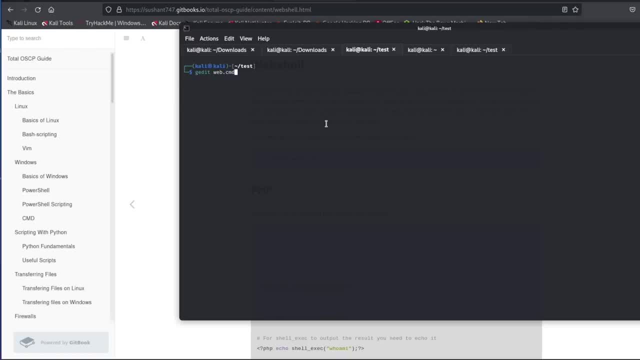 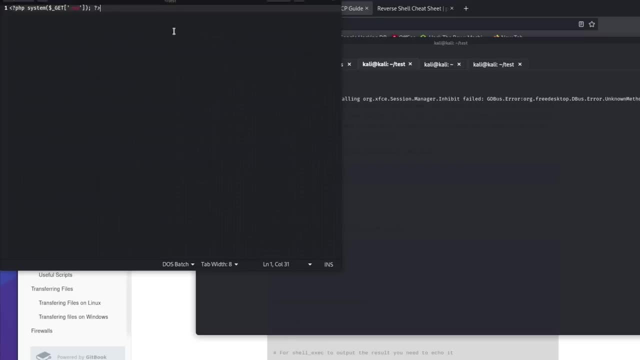 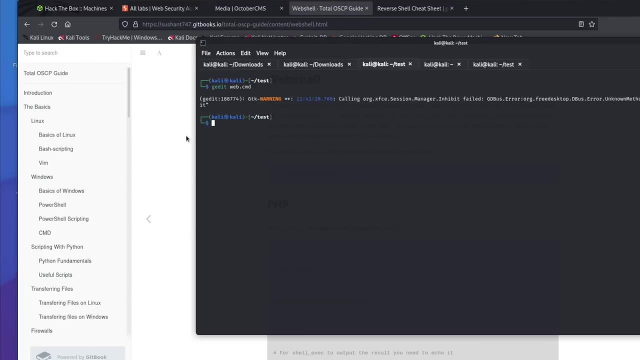 we want to create a g-edit and we'll call it webcmd, and sometimes you might have to name this like PHP, if that's what this server is running in order to get a web shell to run. but we're going to run with cmd and we'll test this out. we may have to change that to PHP. I'm not really sure, and so 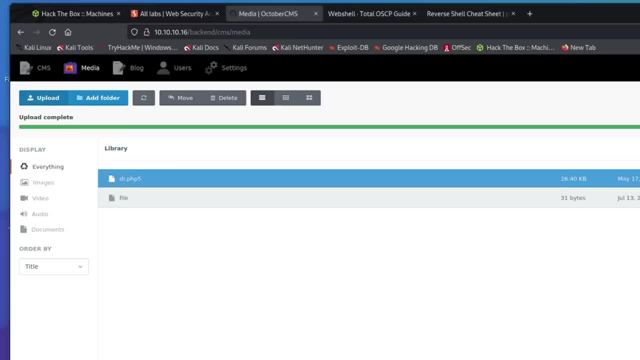 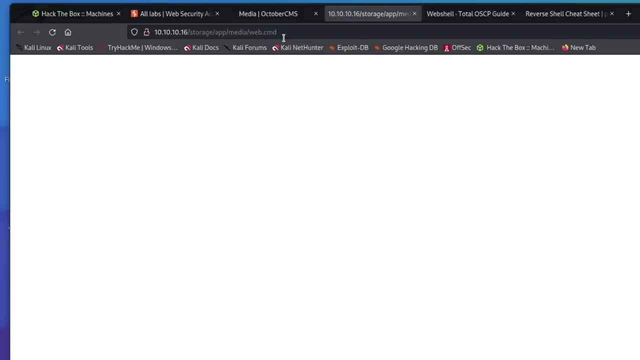 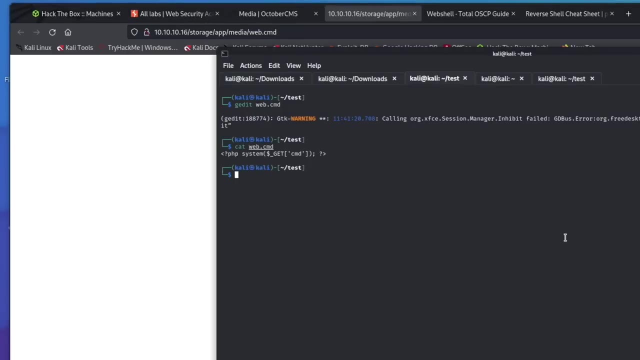 we can come back over here, we can upload our web shell just like this, and if we go to the URL, this is a good sign that it didn't give us an error. now we had to pass in a parameter. because we have this right here, it's going to call our. 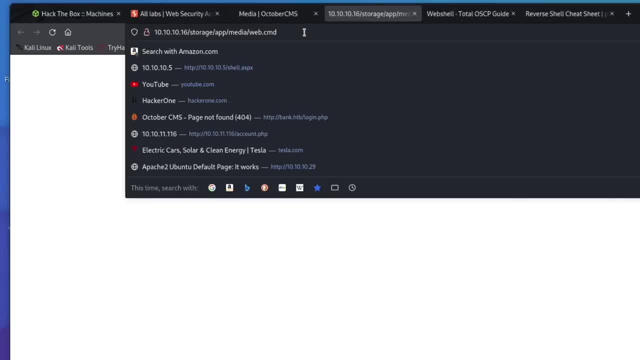 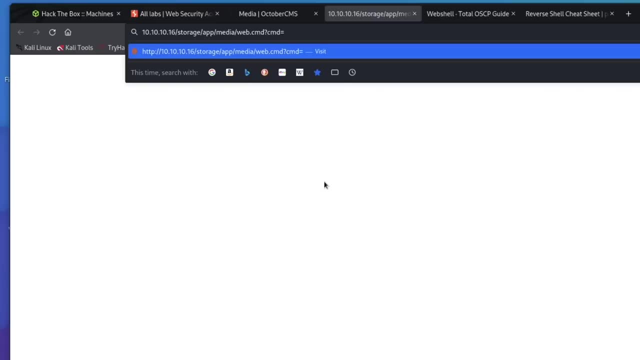 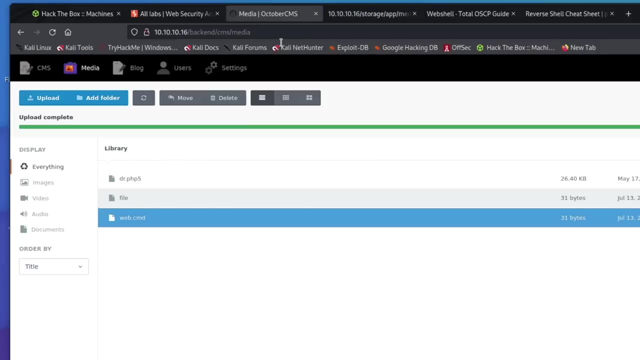 web shell when we pass in the parameter cmd, so we can come over here, go question mark. cmd equals and now we should be able to type in a command here and if our web shell works, we will receive an output on the page so we can type in who am I and run it. and this doesn't seem to work, so we 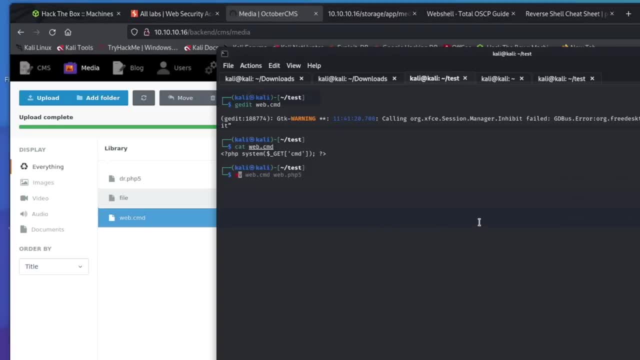 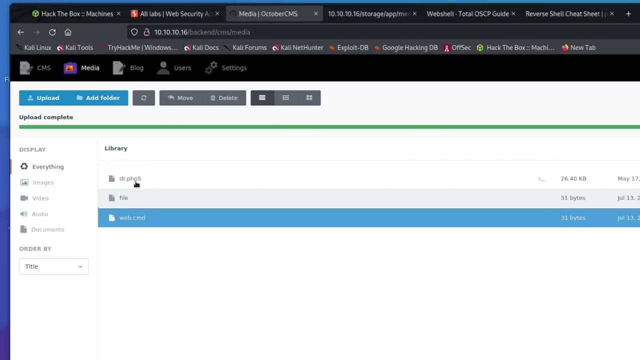 will rename this, we'll just go move. so we will type in our web shell and we will just move it from web cmd to web php5. and the reason I went with php5 is because right here I should have solved this the first time. it says php5, so we can save this and now we can upload. 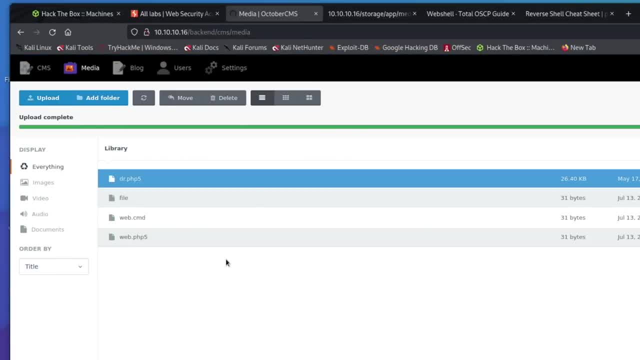 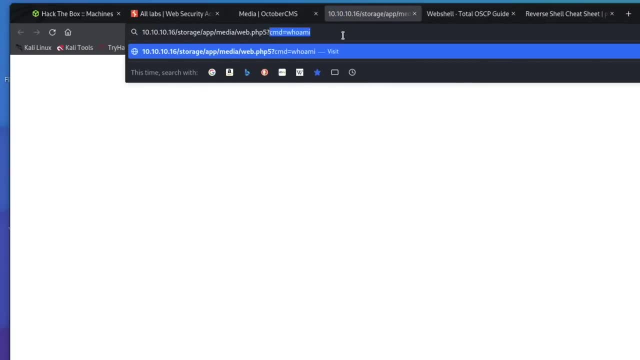 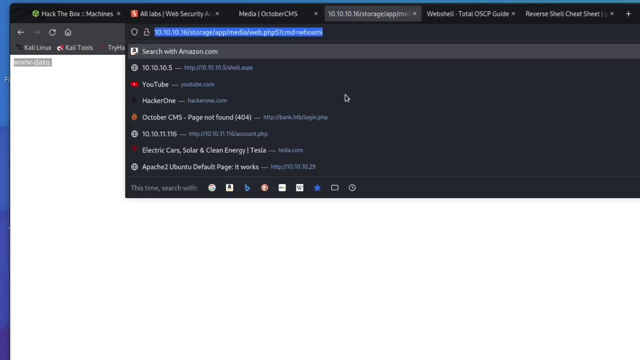 it and we'll re-upload our web shell just like this, and now we can click on it. click here: move that out of the way and we can put our parameter in here. so we want a cmd- who am I? and now it tells us we are WW data and you can use this right here to try and get a reverse shell back over here. but 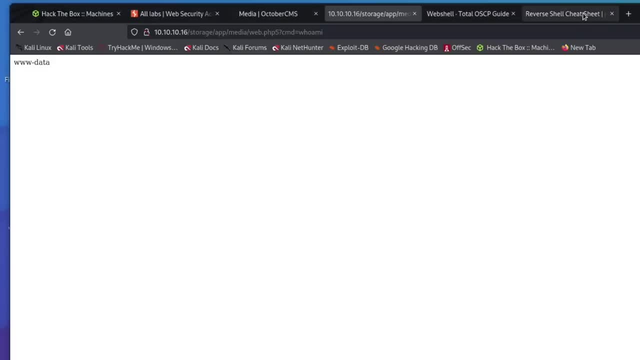 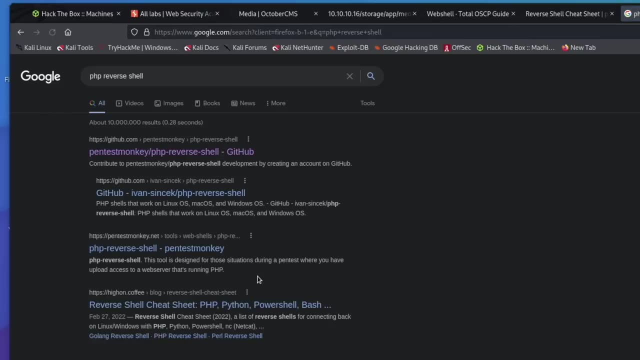 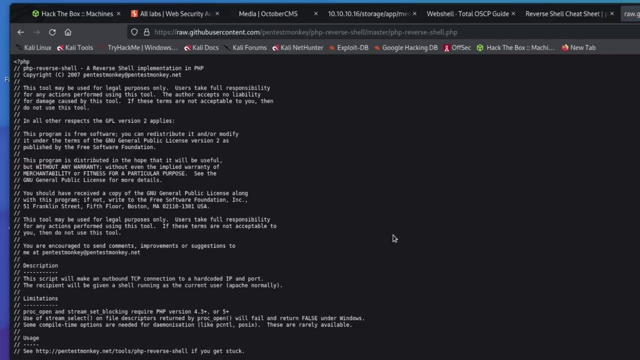 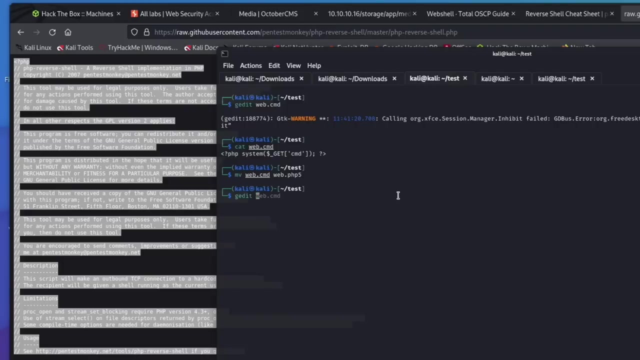 I think what we will do is: we will just use the pen test monkey, PHP, reverse cell. so we'll just say reverse shell and it should be the first one, and so what you can do is go to raw cmd a, cmd c. we will come over here and we will just say g, edit, and then we'll call it shellphp5. we can paste this: 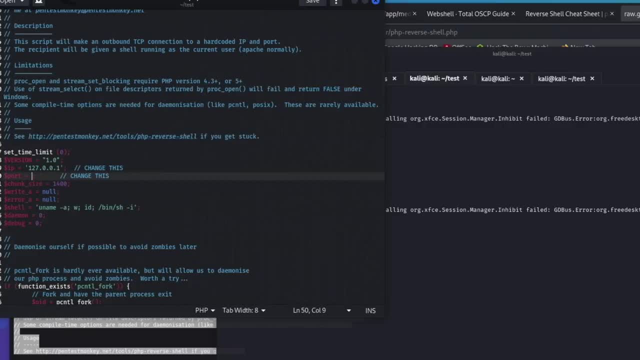 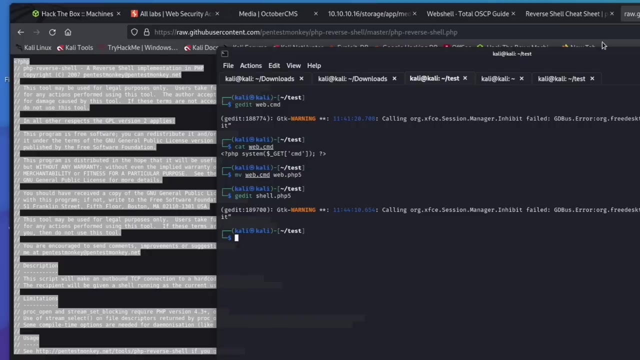 in and then we'll need to change our port, because we're listening on port 444 and over here we are listening on 10. my IP address is 10 10, 14.6. we can save this. come back over here. we could probably close that. 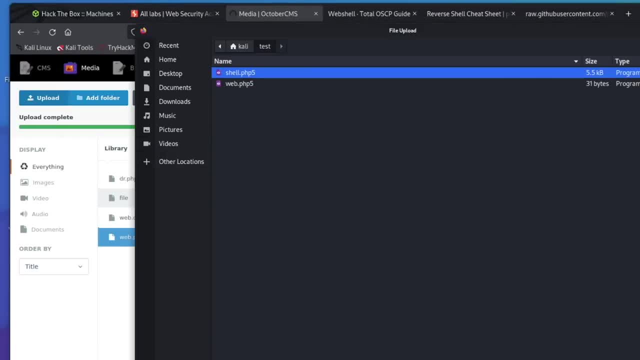 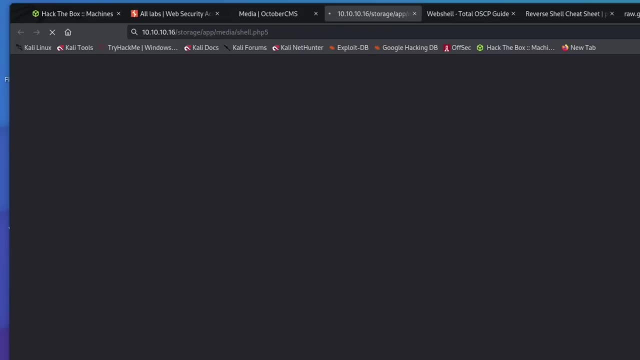 out. we'll upload this file. we want our shell open and then we click this right here. it hangs, which means we probably have got our call back over here and we now have a shell in our box. so I want to explain what is happening. now that you've seen this. 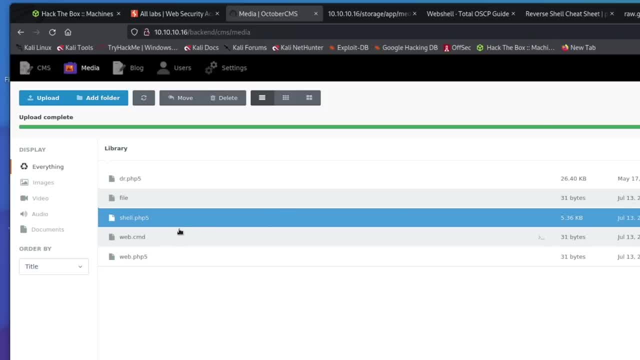 the way a file upload works. if you upload a file, you have to make sure that you know where the actual file is being stored, because when we upload our malicious code, if you can't execute it on the server, it does you no good. so let's say you can upload some kind of shell like this web shell: 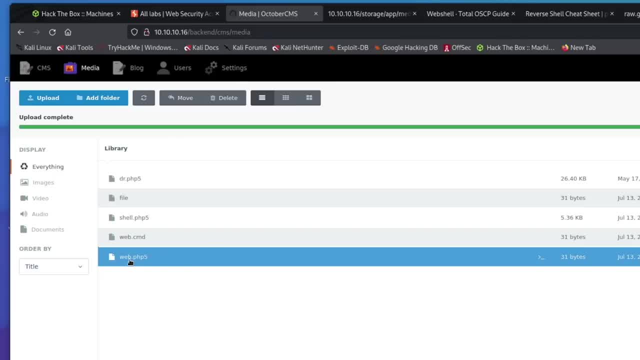 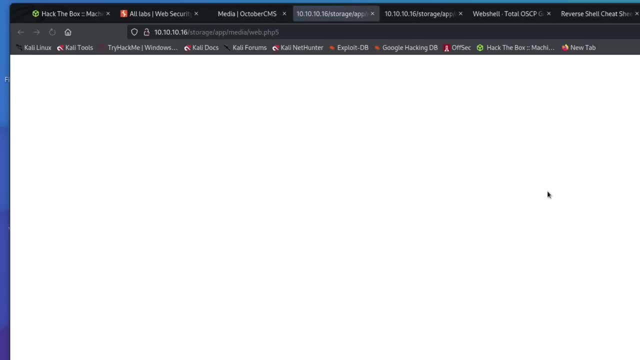 ventilation on the server of this web shell to execute it. it does you no good, so you have to be able to locate it, and for us, this is a really, really simple file upload. you just click here and it takes you to the location right here, of where our file is that we uploaded. 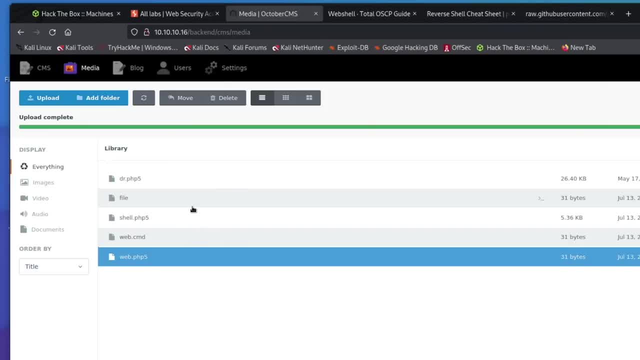 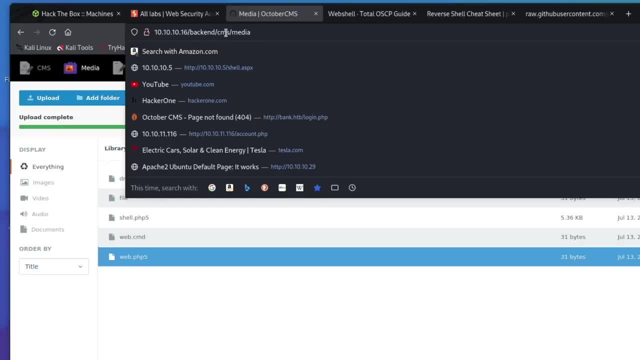 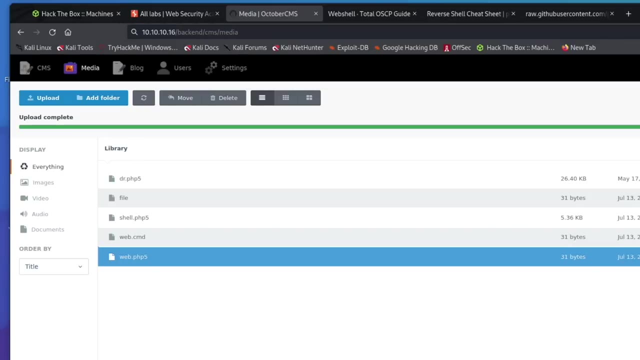 so these- this is a really simple file upload and we have this right here- tells us it's running PHP. sometimes it'll just say, like we'll have a, a back end. it'll say something like backendphp like this, like backendphp like this, and then you'll know it's running phd. or if it's windows, you may try. 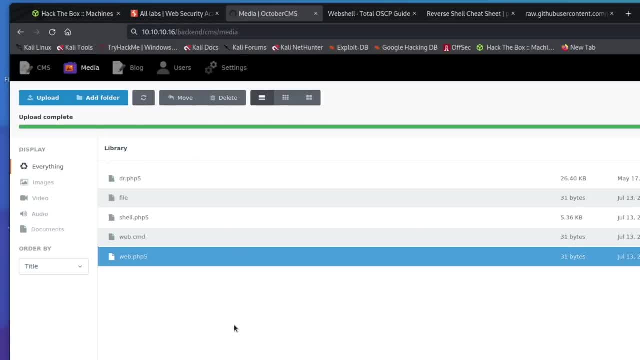 aspx or asp, and so you're just going to have to get familiar with the systems you're going up against and what you see on the particular on the server that you're attacking. but this is a really basic introduction into a file upload. we're going to do a couple more that are going to be a little. 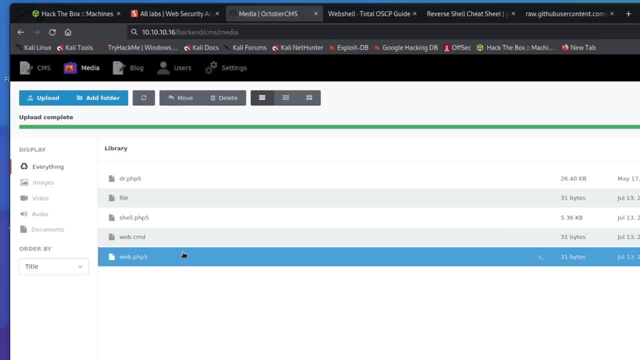 more challenging, which is also going to be a lot more realistic in the real world. the chances you just come across something that just says file upload in a bug bounty is almost zero. maybe on a penetration test it might happen, but in the world of bug bounty probably not going to happen. 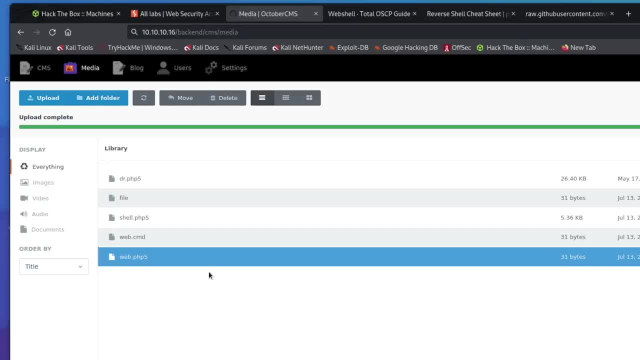 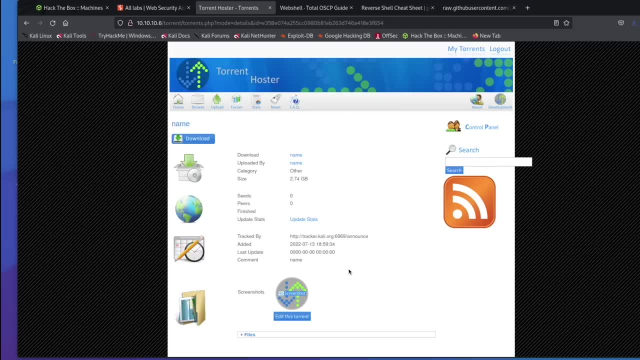 you're going to have to bypass some sort of filters and we're going to do some pretty simple filter bypassing in the next file upload. all right, we are here on the box- popcorn, same thing. i'm not going to show you how to get here because we're just covering file upload and 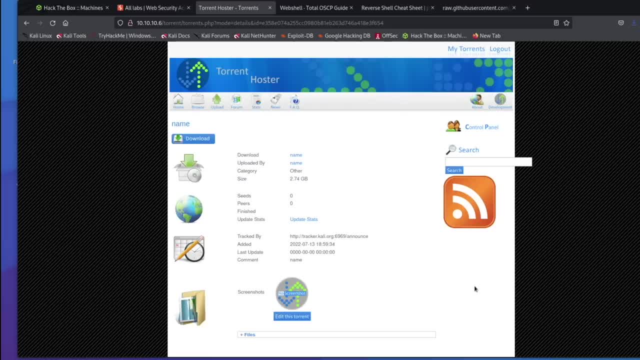 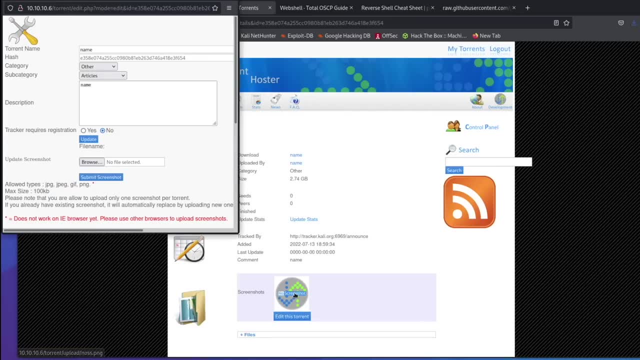 in this one we're going to talk a little more about bypassing different filters. so if we come in here, we have this edit right here and it tells us we can update the screenshot, which is going to be this image right here, and it tells us it allows a jpeg or a png. and i've never tried jpeg, so we 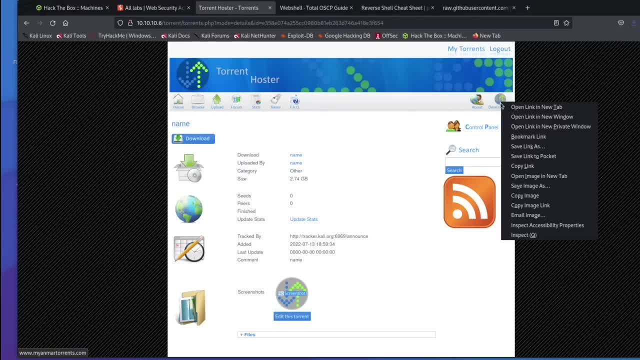 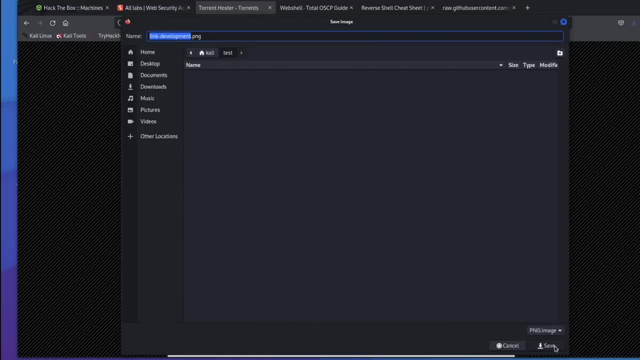 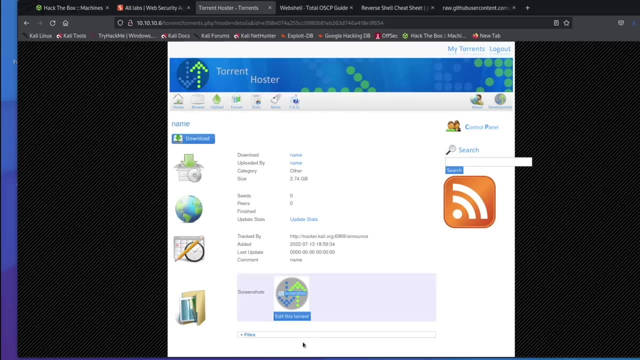 might try that just on the fly and see what happens. but we can save this right here. we can save image as: and we're in our test file right here or test directory, so we'll save that and if we come over here to update the screen, the screenshot we will need to browse. click on our. 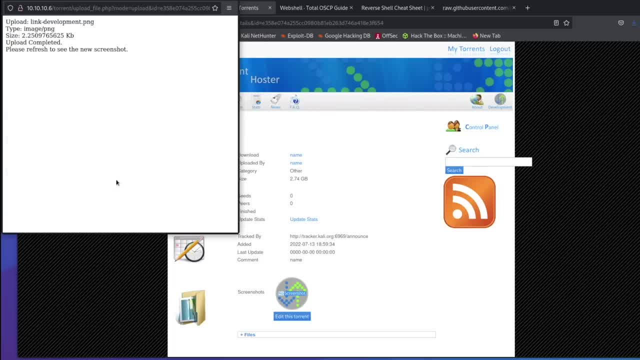 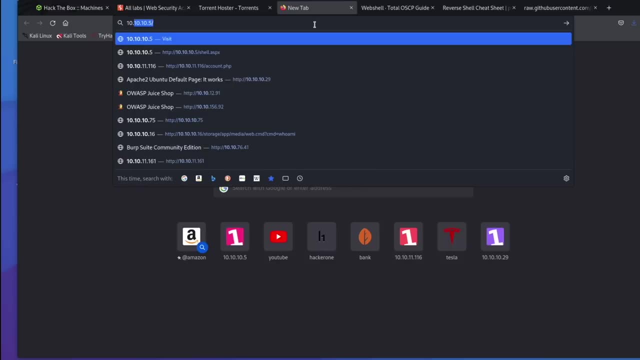 little png right here, update it and submit and it tells us that it worked. the type was a png and now we should be able to come over to the upload page and we're going to go to our png and we're going to type in 10, 10, 10, 6 and we'll go. 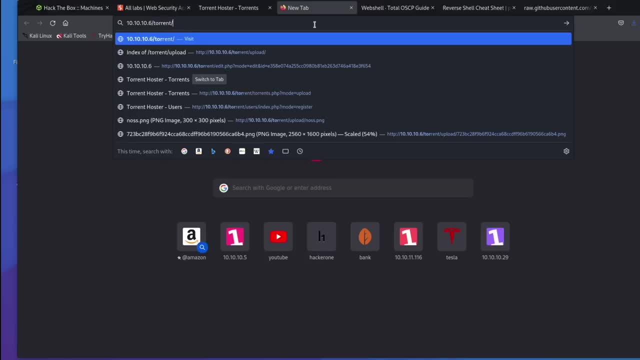 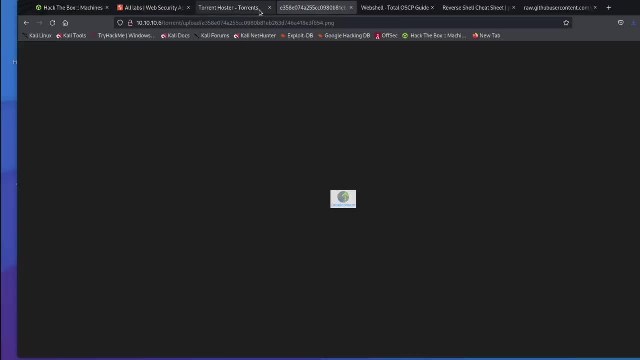 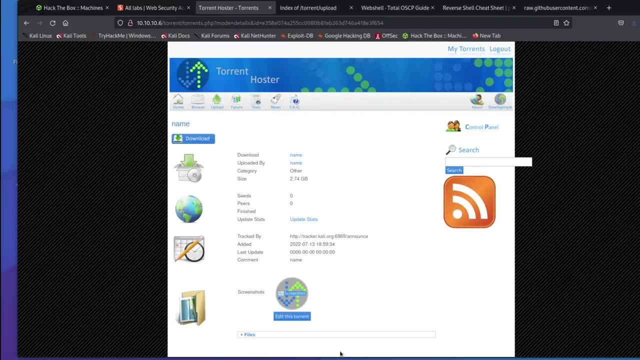 slash torrent, and then we want the upload, just like this, and it tells us: here is the image that we just uploaded. so that works. so what we will want to do now is see if we can upload some kind of shell. so we'll just use one of our php shells that we already have and we're going to go to the. 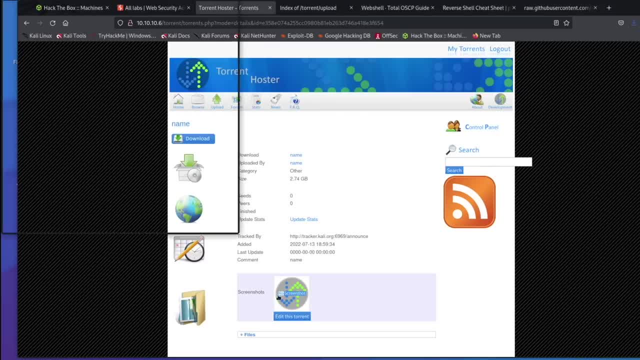 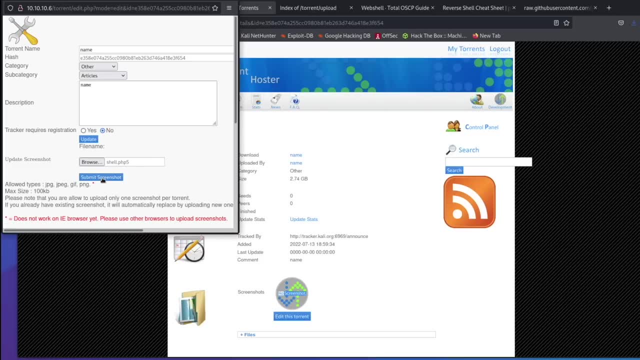 png and we're going to type in 10 10- 6 and we're going to type in 10 10- 6 and we're going to type in 10 10- 6 and we'll browse and we can just try this shellphp5 and if we open this and we submit it, 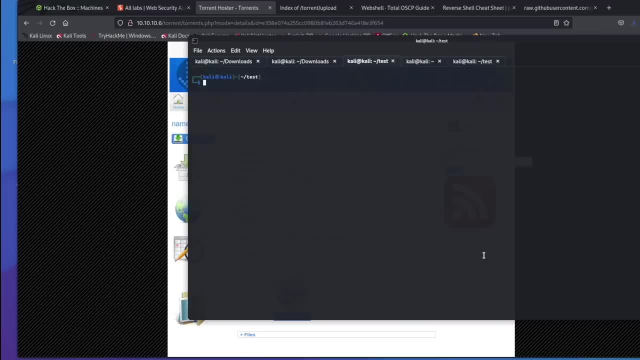 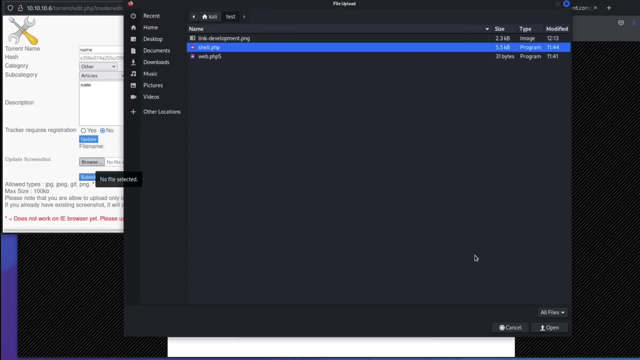 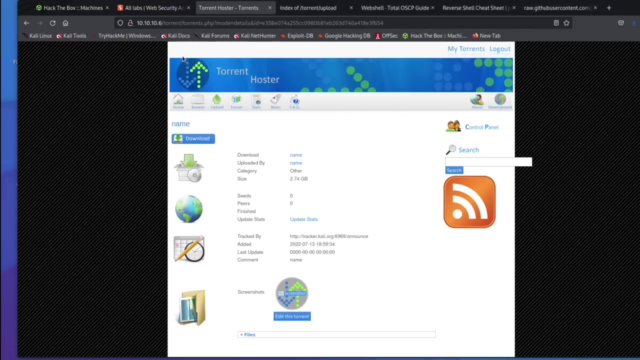 it tells us we have an invalid file, let's come over here and we will move our shellphp5 and we'll just call it shellphp, and we can try this and it says invalid file. now what we can try and do is intercept the request and see what the 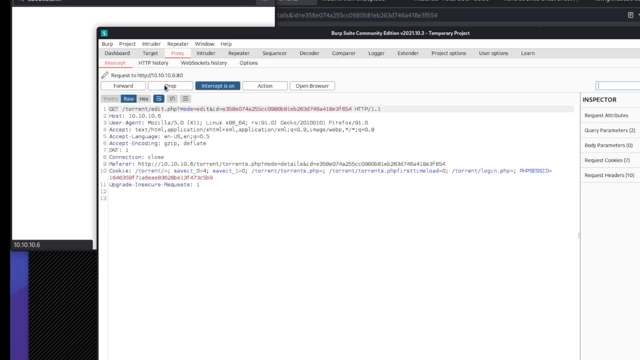 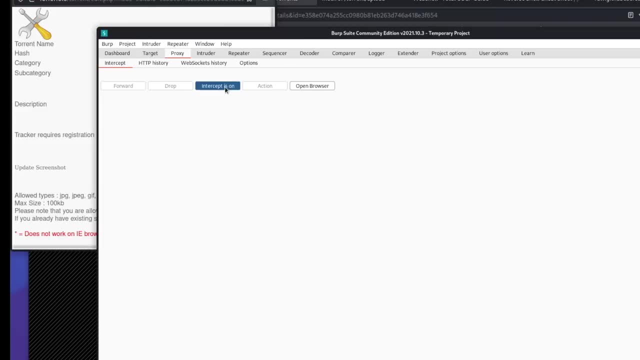 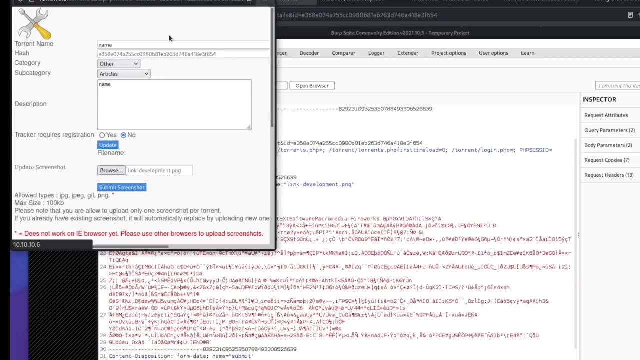 difference is between these. so if we come to update this and we want to update this image again and we upload it, and now we turn our intercept on and we submit this, we can look at the difference and we'll send this to repeater just to save it, and we know that this is going to. 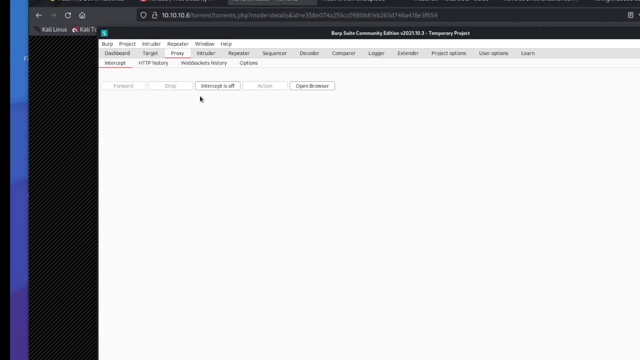 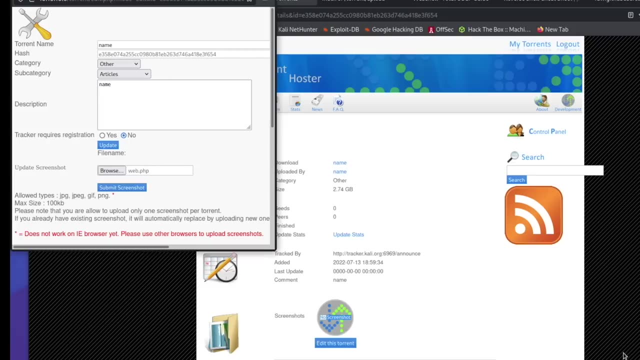 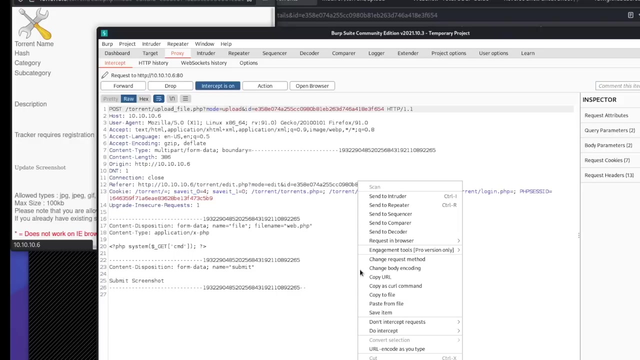 go through tells us that it worked. now we'll come back and upload our php shell and see what the difference is so we can come over. we'll try our web shell this time and turn on our interceptor send it. we'll send that to repeater and we can turn this off now and we can come over to repeater. 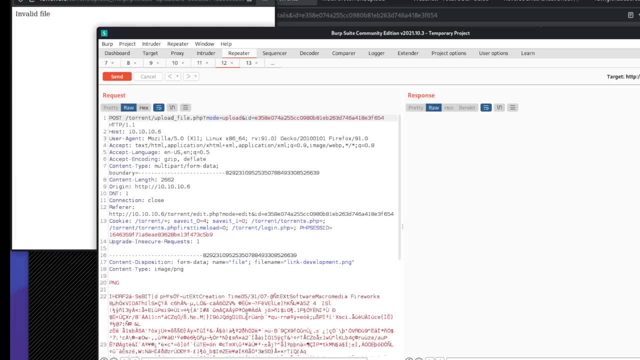 and look at these and see what the difference is. so when you come over here and you look at this, right here is what we're looking at. so we have a content type of image, png, and we can come over here and look at this and see what the difference is. so when you come, 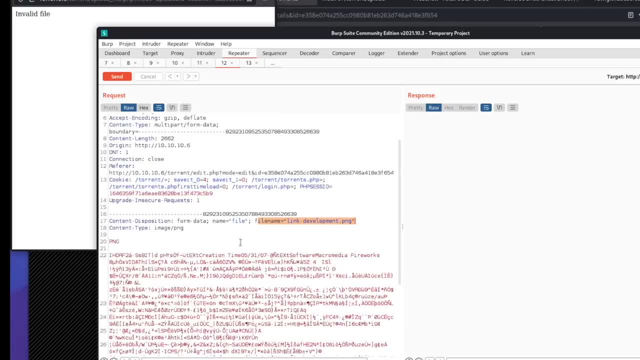 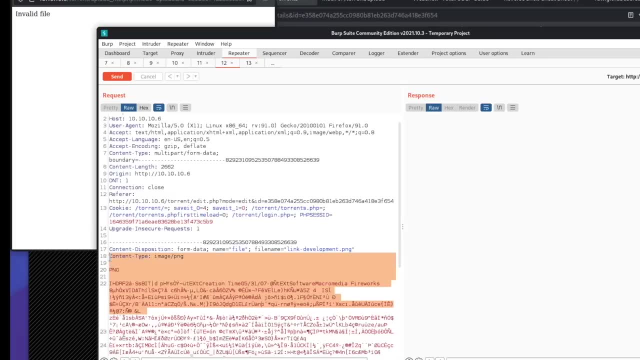 over here and we have our content, type of image: png, the file name, which was the link that we downloaded, and then it tells us it's a png file and we have all this mumbo jumbo right here, and so what we can do is just copy some of this, and we can copy, and now we can come over here. 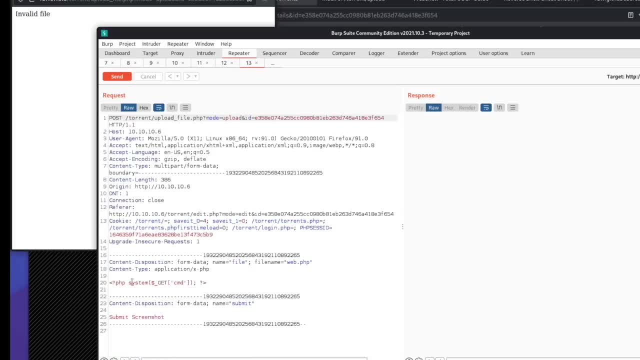 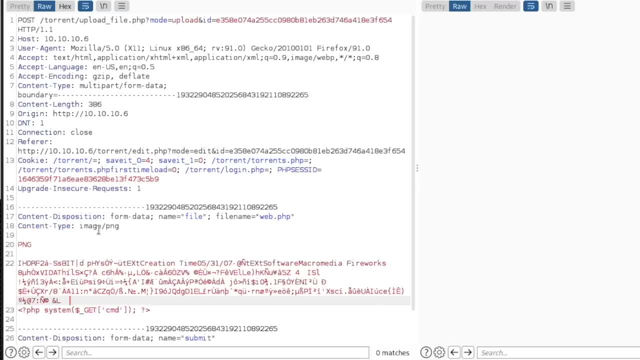 and we have a file type, of webphp, and then we have our little web shell that we used before and we could just paste this in up above, and so our content type has now come over here and we can changed, and we have these bytes to try and confuse it, and then we have this: 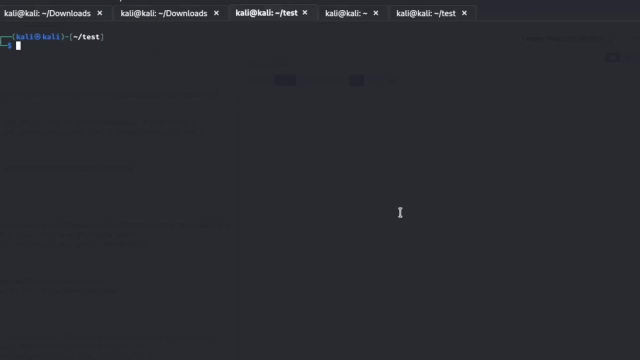 image. or we have our web shell right here, so I want to show you a little bit of how a server would read this file type. if we come in here and we just say G at it and we want to make a file dot, we'll make a file dot gif, and we'll see. 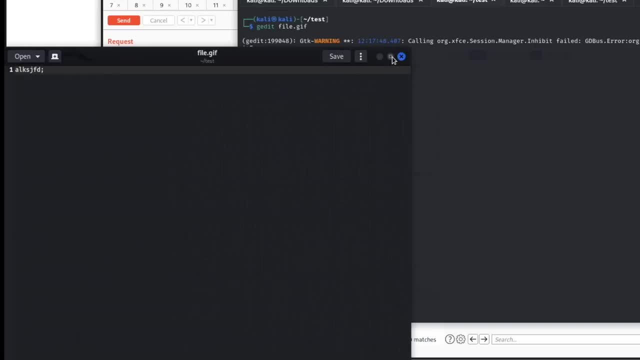 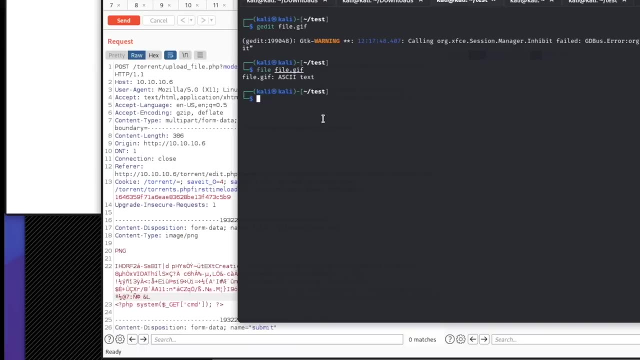 what happens and we'll just put in some letters and we save this, we close it and we go file and then we say file dot gif, it tells us that it is actually text. so if we then come into our file dot gif, there are something. there is something. 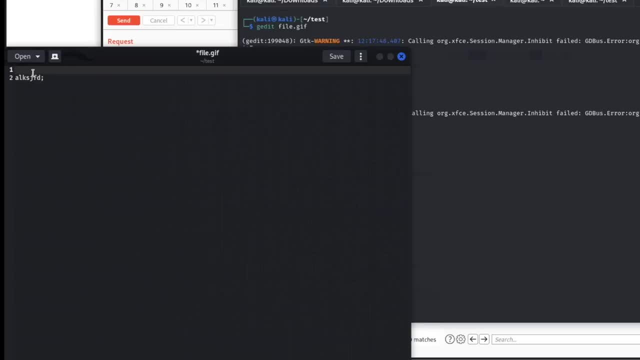 called magic bytes that we can add in here to try and trick it. the way a gif starts is with a gif eight, nine or eight, seven a and if we save something like this and run file on it now it tells us we have a gif and image type and the 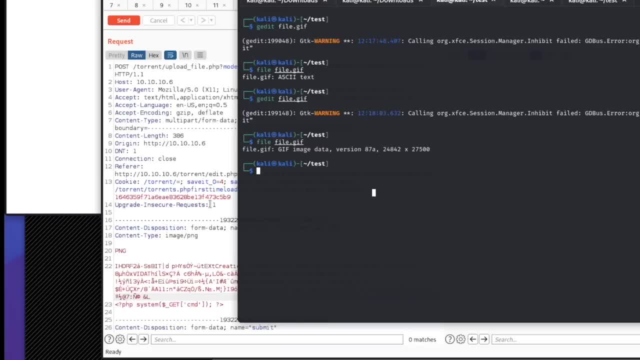 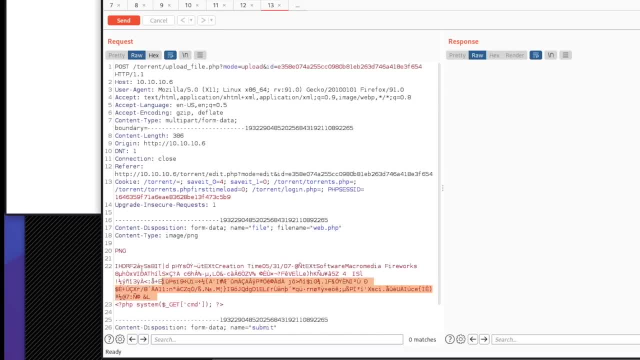 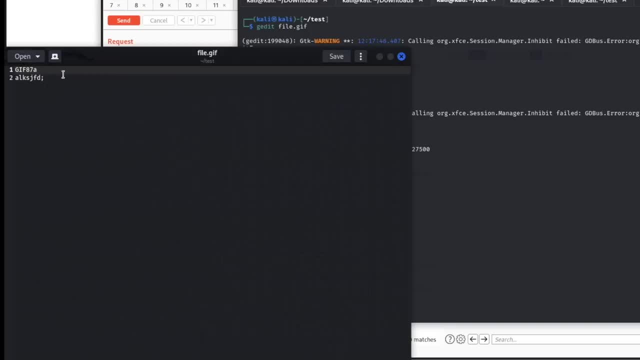 just has text in it, and so when we copy all this right here with the PNG, basically what we're trying to do is trick it by putting something in like this: gif eight, seven a, so that way when it reads it, it will read it as a PNG and 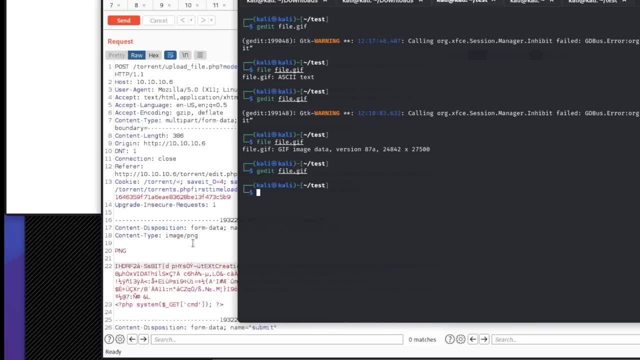 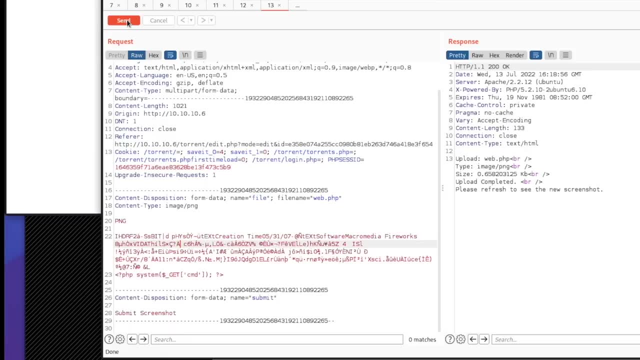 we'll actually try this gif because I've never actually tried it on this box so I don't know if it will work or not, and we'll just try the file upload on the fly. so if we send this over, it tells us that it looks like it uploaded, so we can. 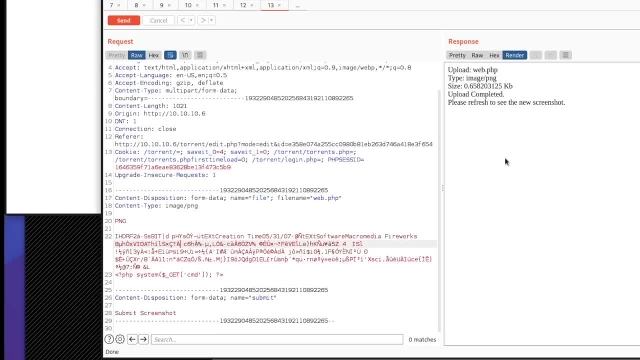 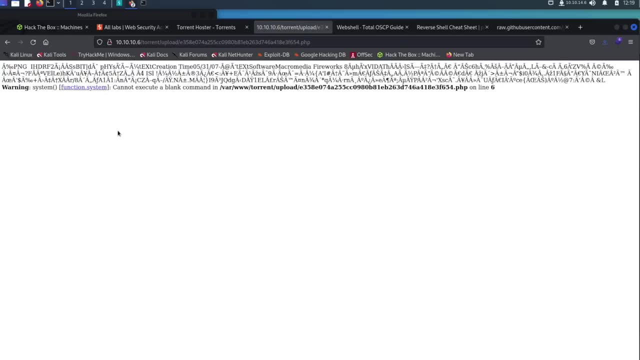 see what it looks like it did upload, so I'm kind of surprised that worked. we'll go check it out. so if we come over to our uploads, we refresh the page and we open this up. it looks like it worked. we should be able to pass in our parameter. 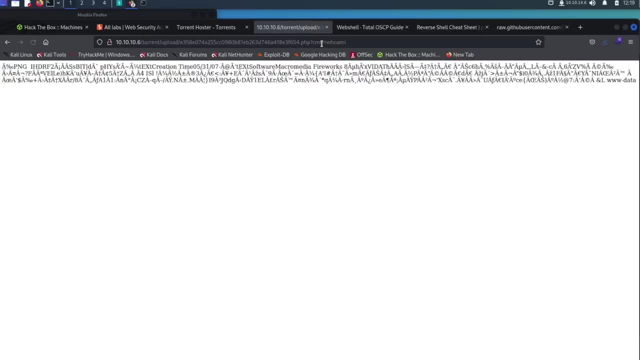 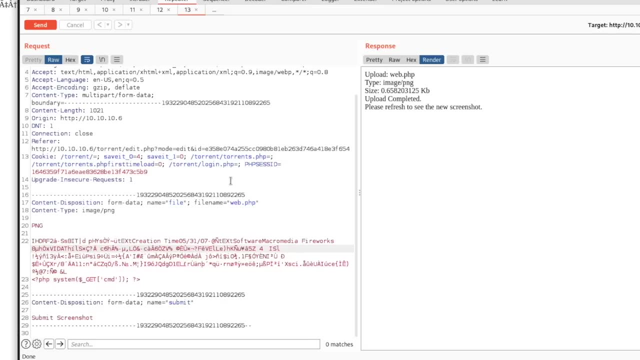 of cmd equals and we can say Who am I and it tells us right here www data. so that actually worked. I was expecting it to not work and sometimes when you hit a file like this and it does not work, it might for just a dot png inside the file dot and then the dot php. and if you just go out to google and 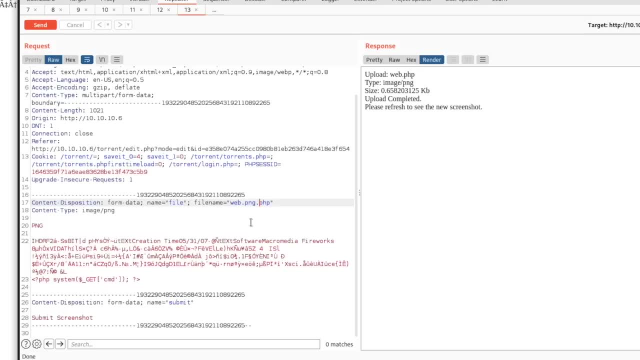 you read about different ways to bypass filters for for file upload, you're going to have a lot of information, and that's really what i would recommend you to do. this is just the tip of the iceberg on how file upload works, so i'm just showing you some basic, some basic ways to bypass. 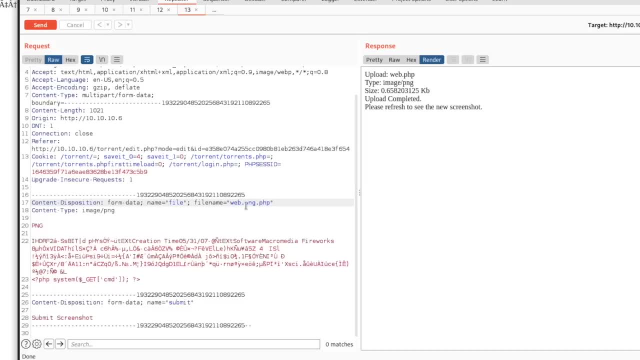 it. but i would also recommend going out to google and reading about how to bypass a png file upload filter or a jpeg and see all the different ways you can bypass and bypass this. so if we come in here and we send this and it renders, it tells us, this worked as well, so we can actually go back. 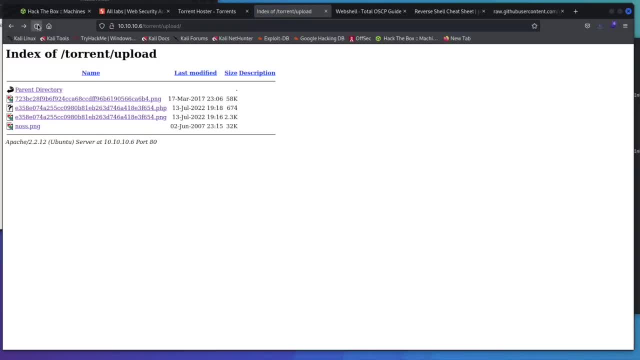 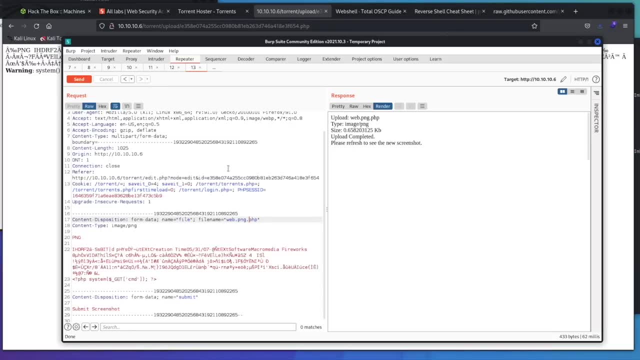 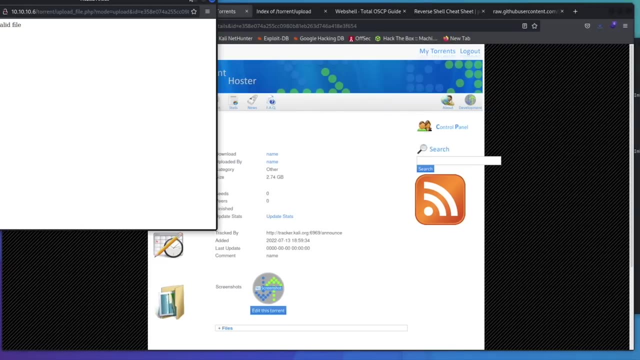 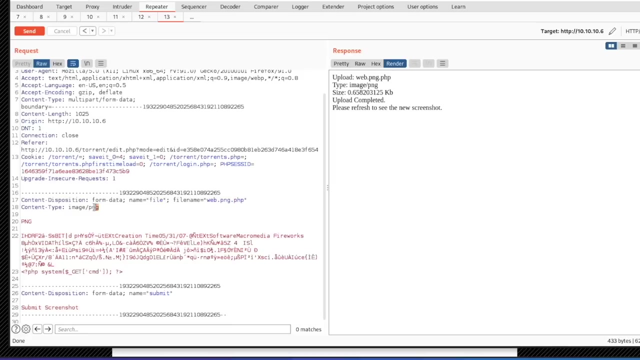 and if we refresh this right here and it tells us that this worked. so there's one other thing: let's play around with the jpeg. so if we come in here and we close out of this, let's actually just play with it in repeater and see what happens. so if we say it's an image and we say actually let's try the gif, because we 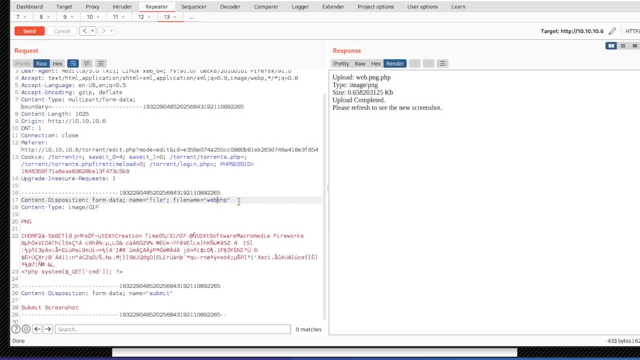 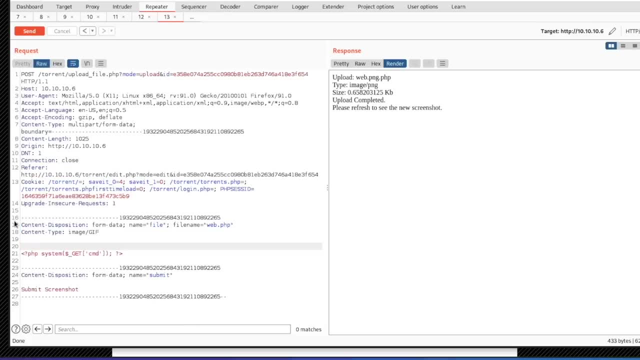 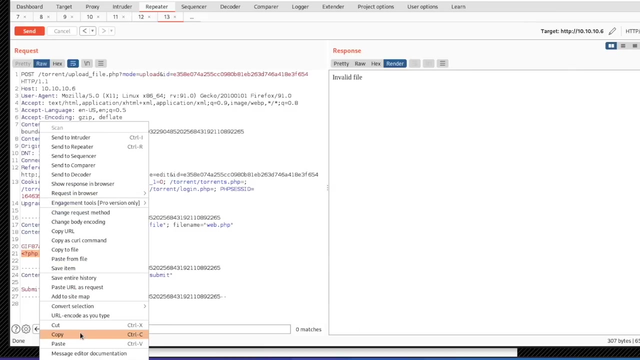 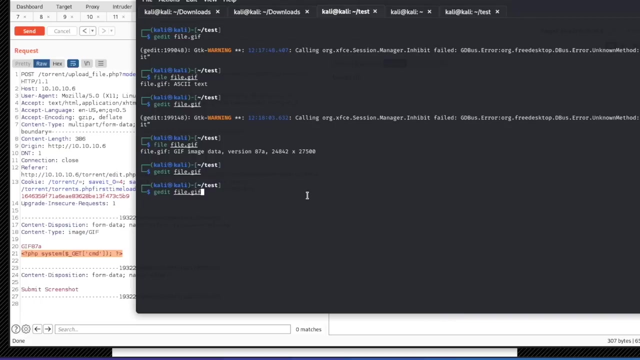 already have that set up and we just leave this like this and we delete all this and we just type in the 87a with the gif at the front. let's see if this works. it says invalid file. so let's take our php shell, we'll copy this and let's see if we can just say: let's g edit this file and we'll call it file php. 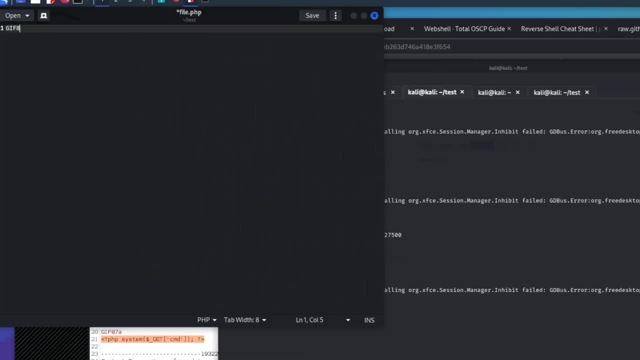 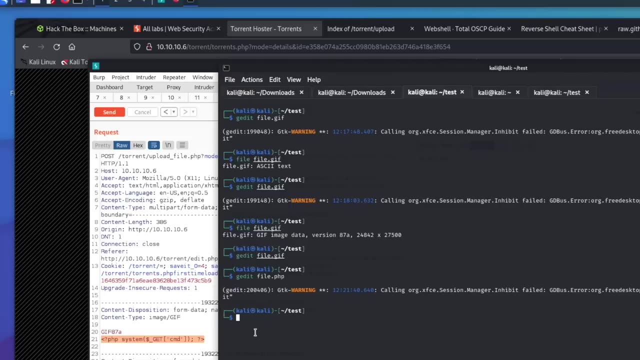 and we'll add in the gif 87a and then we'll put our php in here and we'll save this, and then we're also going to need our gif file, so we have that in there too. so that way we can make sure that our content type right here is right. so we'll go to a proxy, so that way it is. 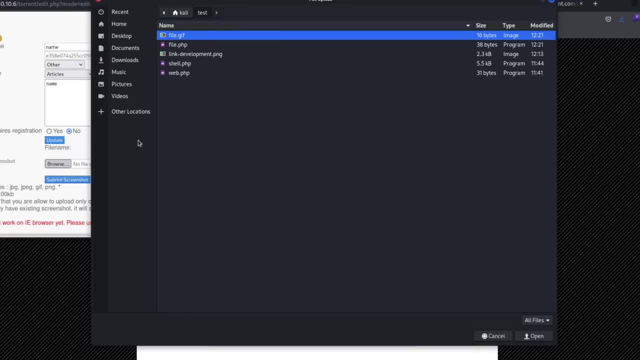 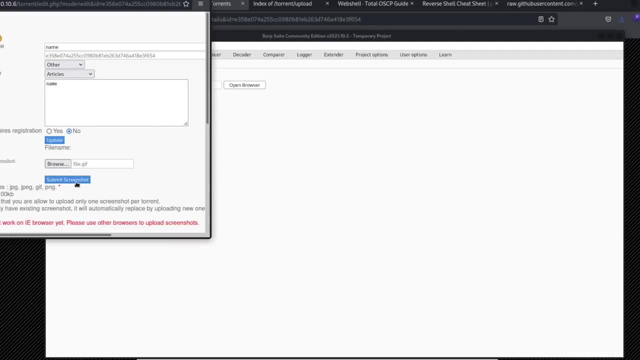 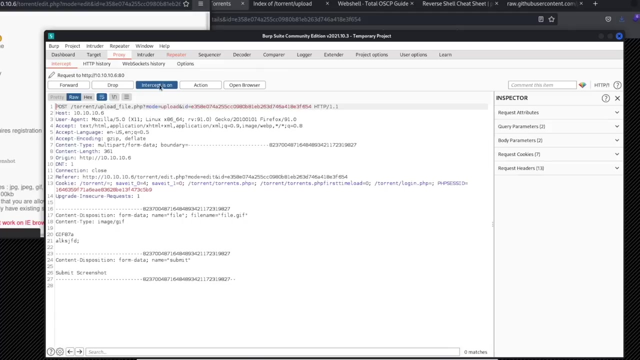 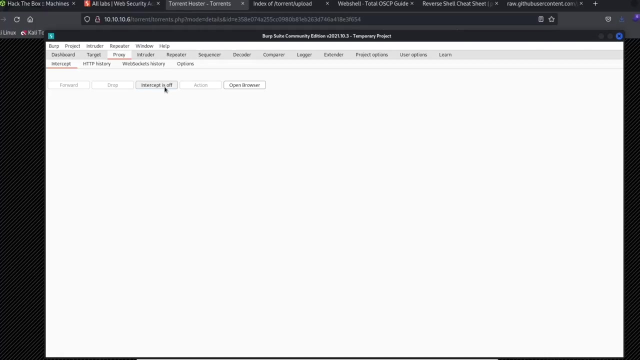 ready, we can try this. upload browse. let's upload the file with the gif open. make sure that we catch this, send it to repeater. it looks like that is how it goes. i actually want to use the gif file to turn this off. it says that it worked okay, so it does accept the gif as well. now let's upload our. 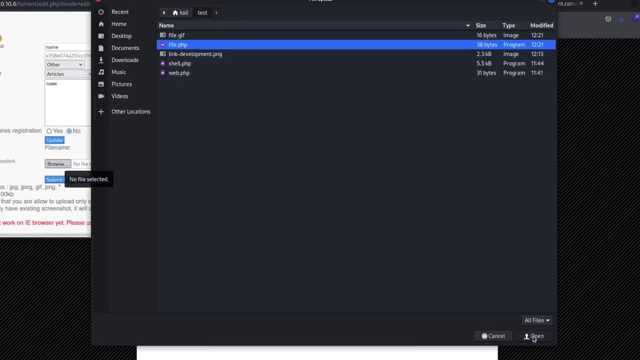 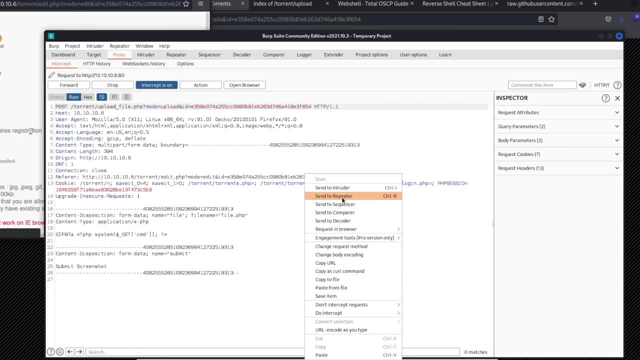 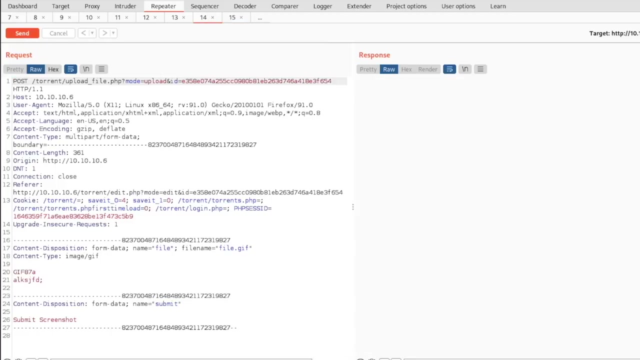 reverse shell that we saved in filephp and we'll send this on over to repeater see how we have this. application type is different so we can turn this off and see if we can get this to work as well. so we'll send this and it says invalid file. and when we send this it says that it worked. 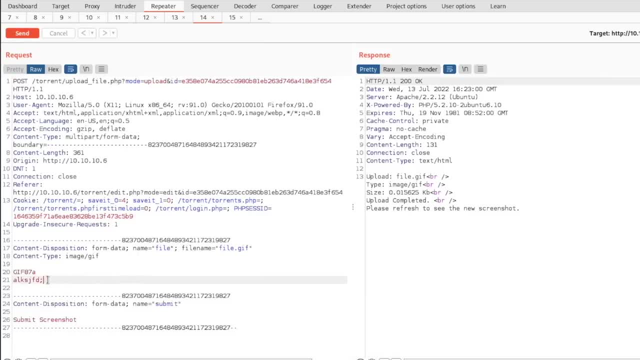 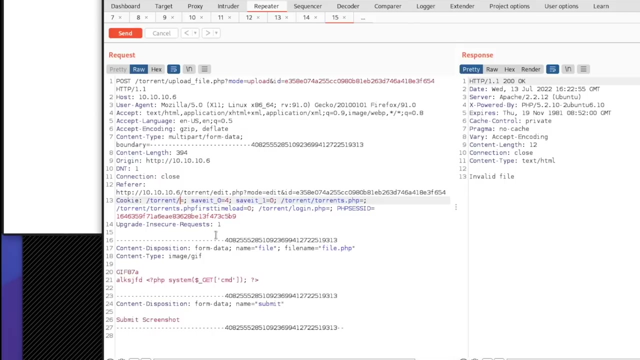 so what we can try and do is just grab this, like we did before. we'll copy it and paste this in. should be able to delete this. does that actually have a semicolon in it? it does, so should work like that. if we send it, it says that it worked, so let's go see if we can. 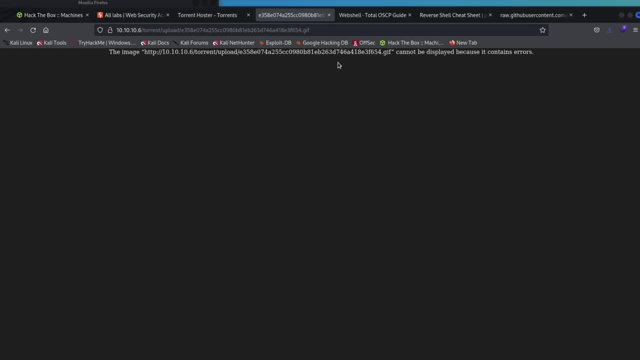 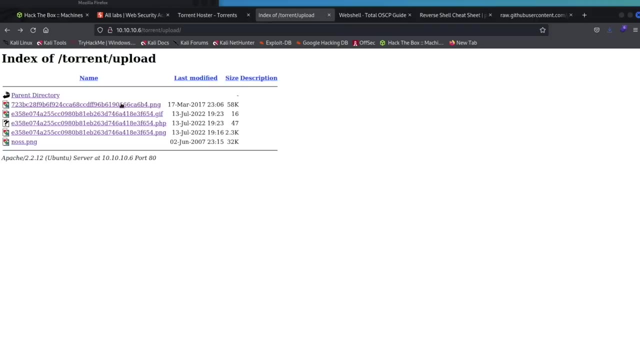 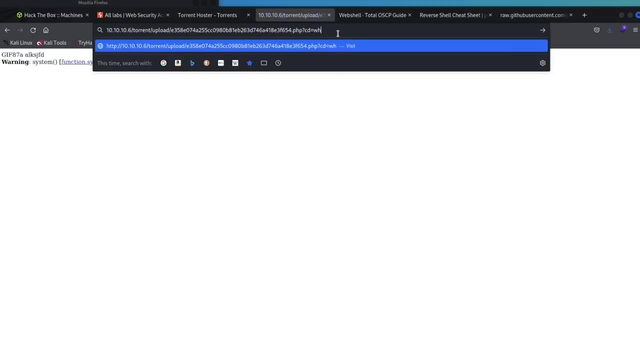 find that here's the gif. it says it didn't work. that's not surprising, because it's not actually an image. we need our other php shell. here's our gif with our php in it, so let's try and pass in the same parameter equals who am i, and if we send this, it tells us this gif works. 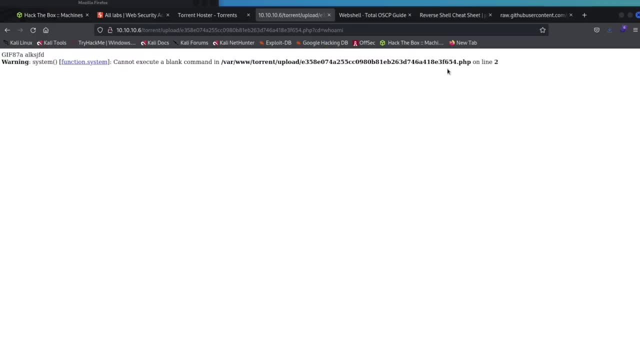 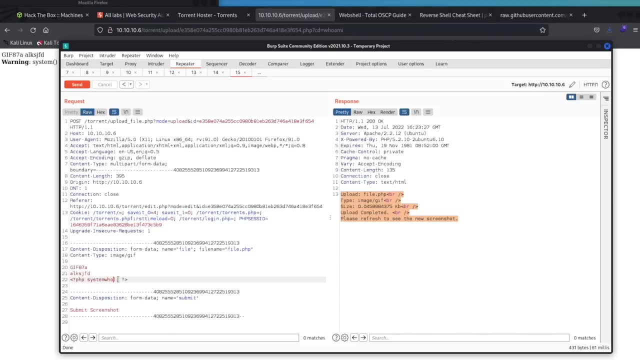 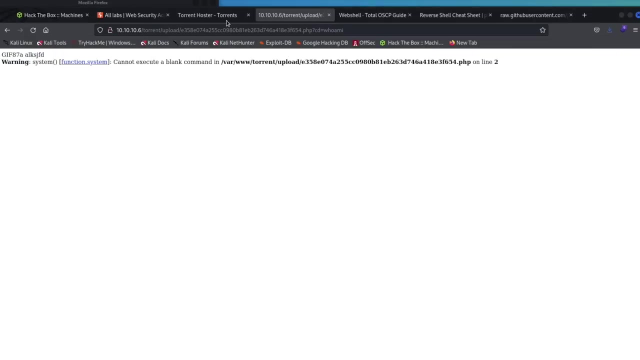 and it cannot execute the command within the file. let's try and just delete this and see if we can get a who am i? this way, we'll send that. come back back. refresh. check out this php and it tells us where ww data. so it does. let us inject a command. 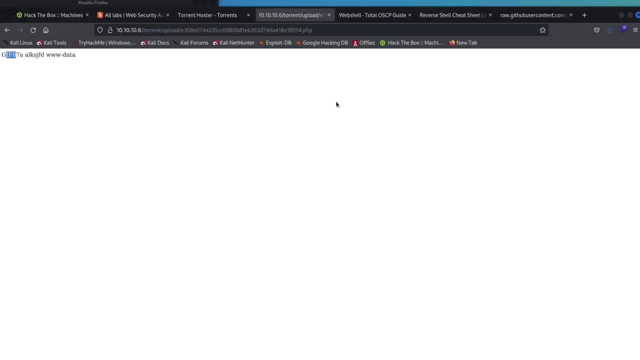 with a gif, but for some reason i wasn't able to get the web shell to work. but there's another way to go about this. so this would be a really roundabout way to do this. you could come in and we could try and upload like a python shell in here, or, because we know we have php we could put. 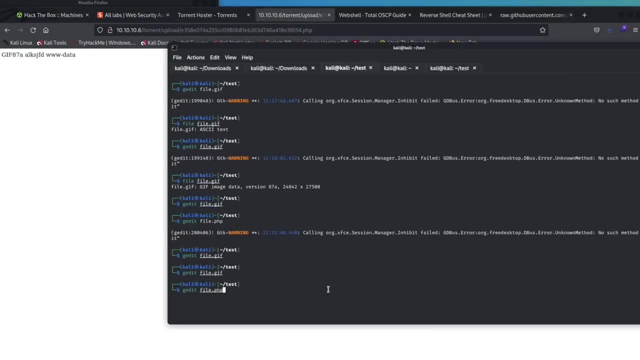 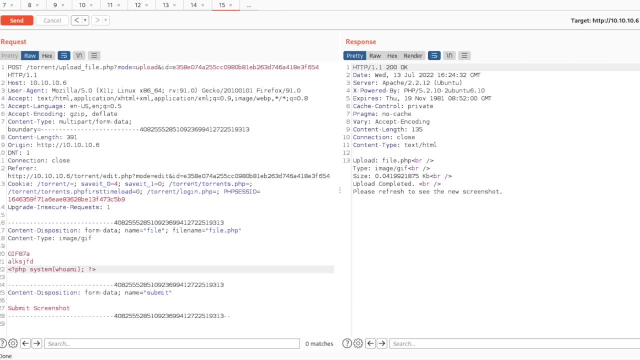 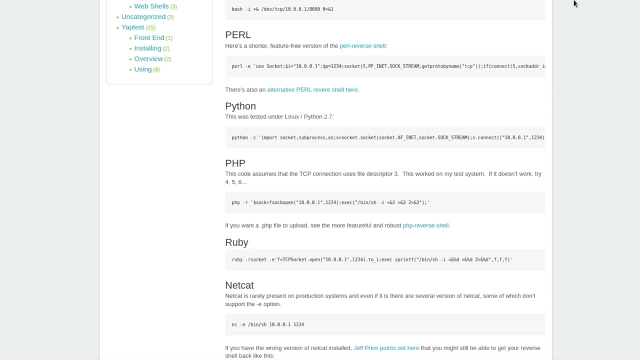 inside of here, here and sort of we could put inside of our command right here, instead of doing a system. who am i? we could come to this web shell and we could execute a php reverse shell like this, but you saw us use this recently. let's just try and upload this php shell and see if we can get. 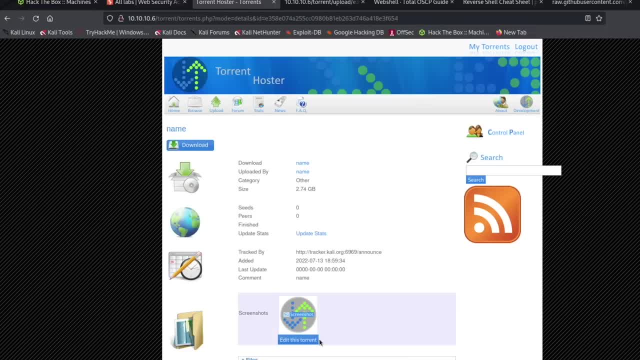 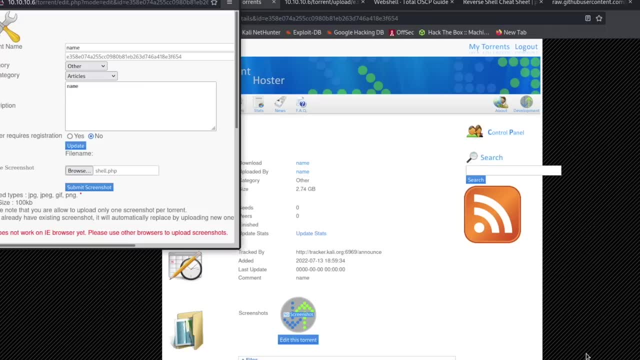 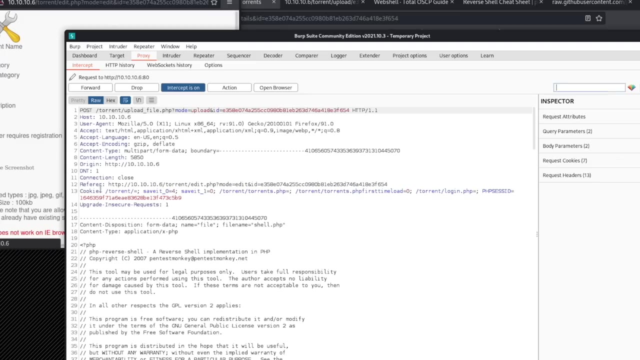 this to execute a reverse shell for us. so we'll come back over here. we can edit this again. we'll put in our php reverse shell we can open. we'll need to catch this inside repeater, turn our interceptor on, submit and send over to repeater. we can turn this off. come to repeater, tells us. 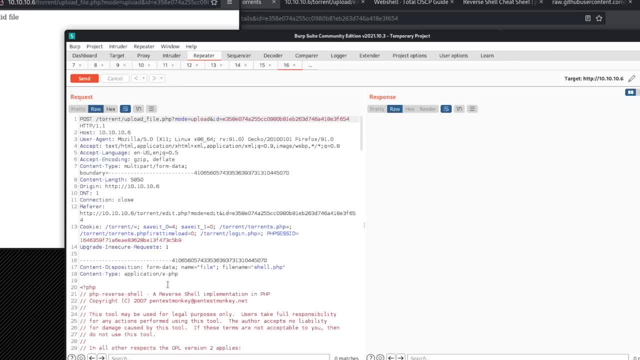 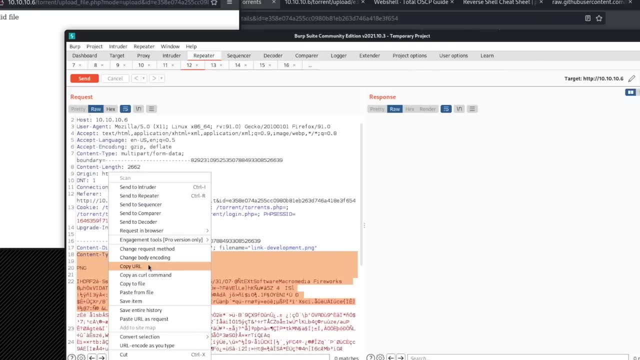 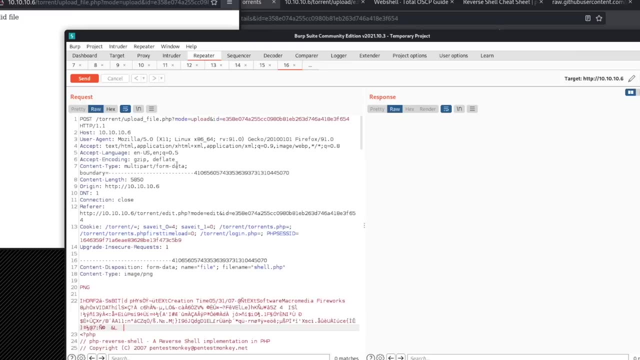 we have an invalid file, which we expect. we have the shell dot PHP and we'll just use the one with the PNG because we know that it's going to work for us. so we can come over here and we can just highlight this paste in the PNG. now, if we send this, it tells us that this worked. we can set up a netcat. 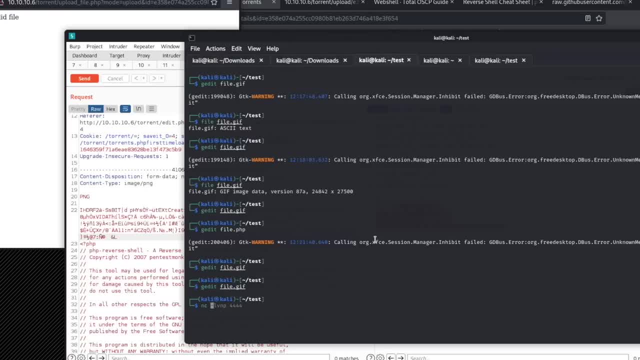 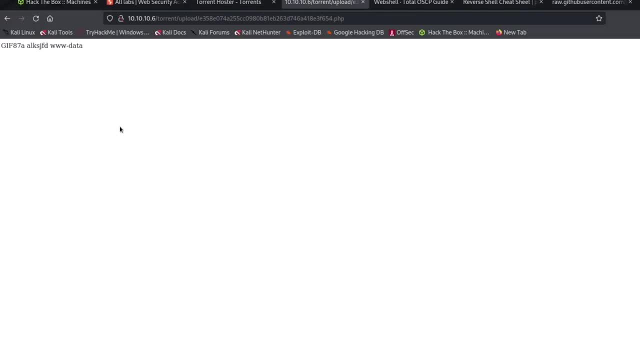 listener over here, netcat, and I think we originally made that on port four, four, four, four, and now that's listening. so now when we open up that file, it should execute on the server and it will give us a shell back. we can see our PHP file. we can see the size has changed, so we open. 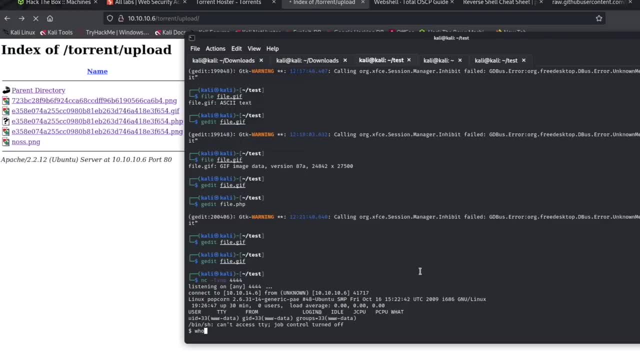 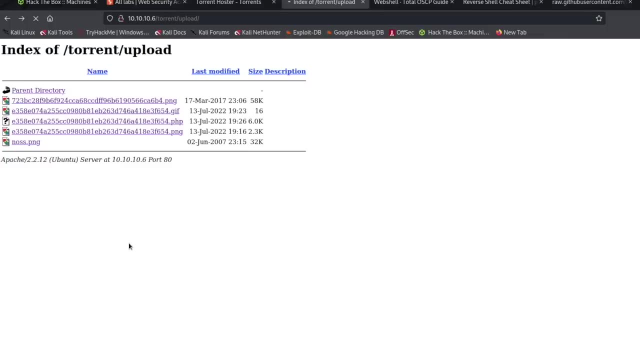 this up and it's hanging and we have a shell returned back to us and it's going to tell us: I am wwdata, so that is file upload. so there's a bunch of different ways you can play with this. if you have hackabox, I would recommend coming into popcorn because you have a lot of different ways. 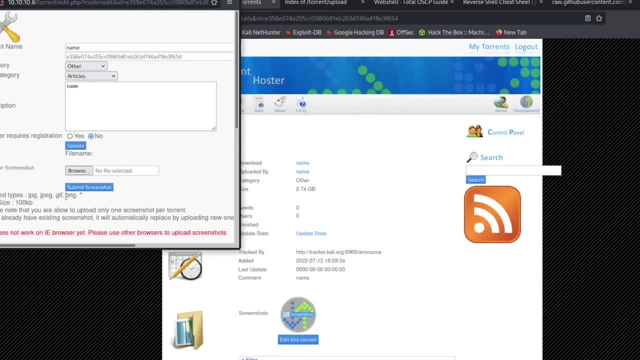 to play with this. you have the jpg, then the gif, the PNG, and so you can just come in here and play around with these and see all the different ways that you can their sweet and you will have a pop corn program working on Linux. בvoll啊, this is the encoder. it's going to give you all the sorts that I will lay jpg, then the GIF, its DD g, and so you can just come in here and play around with these大概 بل notchutterr. 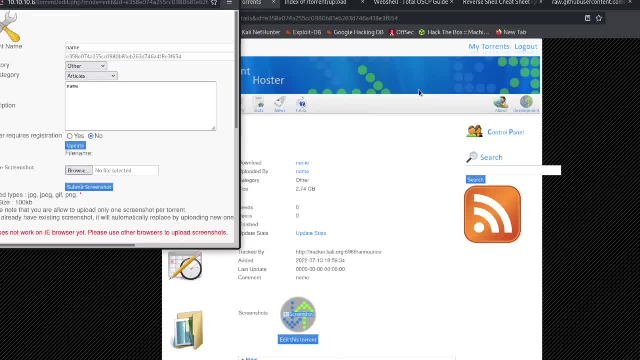 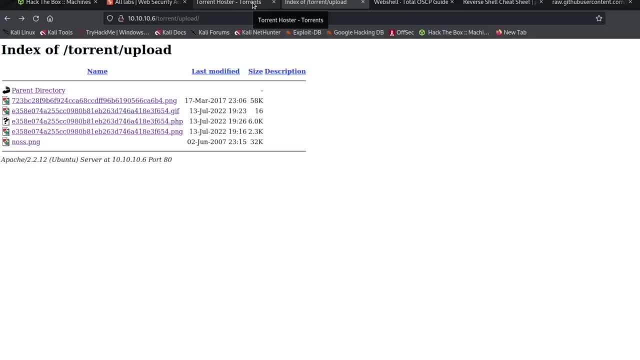 the different ways you can get a reverse shell from a file upload and i would recommend- because we were not able to get the gif web shell to work- you could play around with that and see if you could get a web shell rather than just executing commands one at a time, and then maybe see if you. 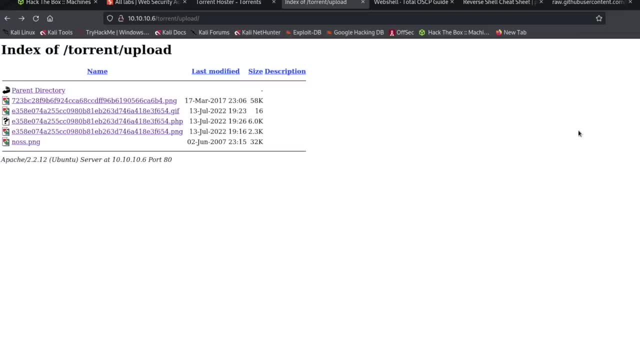 can get a reverse shell from the web shell, because there will be times that you have to do that inside of ctfs. but in the world of bug bounty you really wouldn't be trying to get a reverse shell. you could just simply do a web shell into who am i for a proof of concept? and file uploads are: 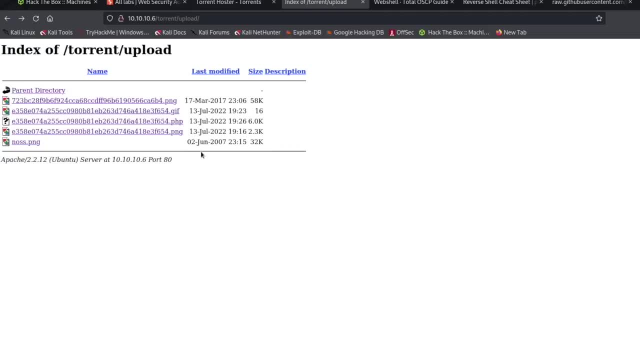 something you're going to see, so you can read about those and hack the box. and i would definitely recommend going out to google and continuing your research on file uploads. but, like i said, there's really not a lot of places to practice file upload and it's because if there's a file upload, that is. 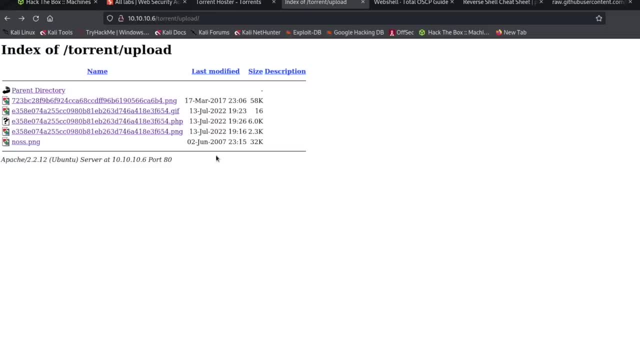 going to be vulnerable. on a server you can get remote code execution and, for this reason, hack the bot. is a very common problem with web shell and ctfs. but if you're using a web shell, you can get a reverse shell from a web shell and ctfs. but if you're using a reverse shell from a bug bounty. 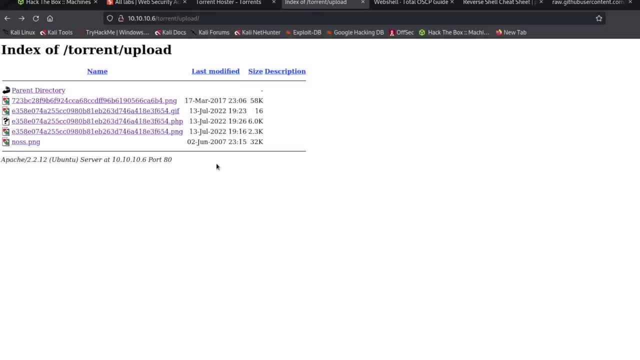 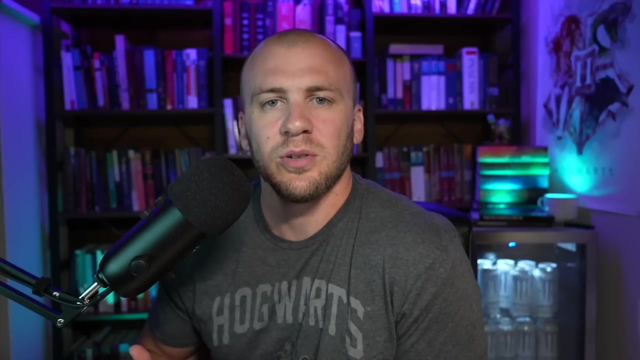 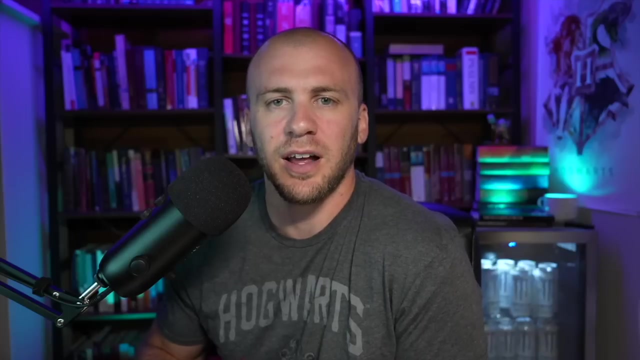 and you're using a bot didtc, you're going to get a pro peak interview. that because it's just a one-stop shop, if you can get that. because if you're using a web shell and and RFI portion of this course, The LFI is going to be one that is more common than the RFI and 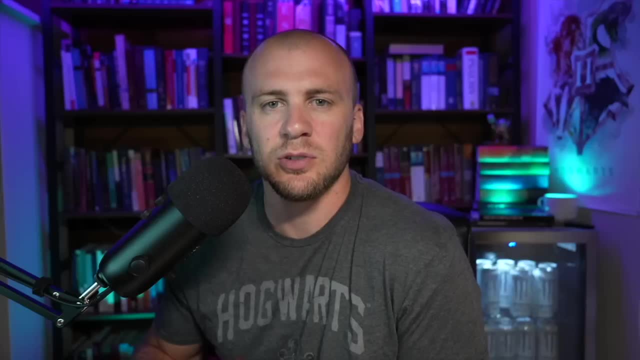 the LFI is going to give us the opportunity or the ability to read local files on the server, which could lead to a compromise of sensitive information or data that we're not supposed to be able to access and files on the server that we should not be able to access. The RFI is going to. 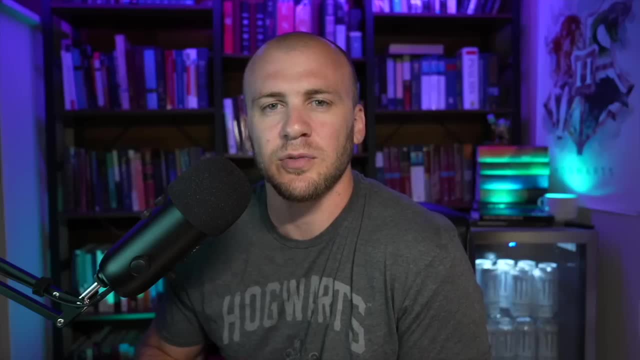 give us the ability to host up our own files and then have the server reach out to our server that we make on our Kali machine and then execute that file and will lead to remote code execution on the server. So we're going to jump into the LFI and the RFI. now Let's get started. Welcome to the LFI. 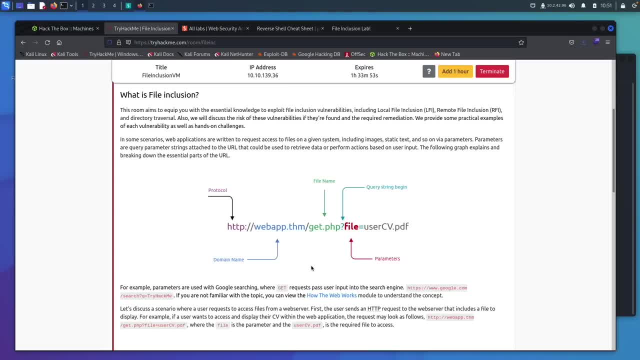 RFI. so the local file inclusion or the remote file inclusion portion of this course, We're going to be using TriHackMe for our example, and TriHackMe is just too good to pass up when it comes to practicing LFI and RFI. 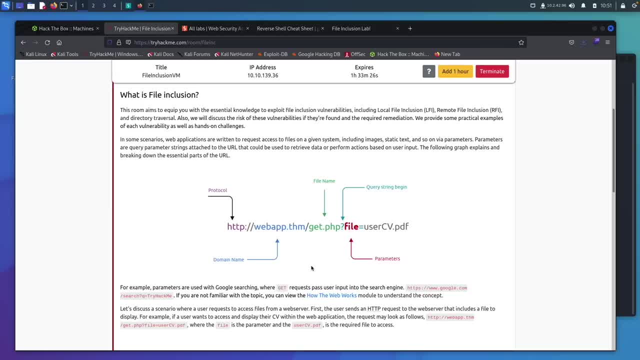 If you can afford a TriHackMe membership, then it is worth it just to come in here and practice your LFI and RFI along with other things. and when it comes to Hack the Box, Hack the Box- doesn't have any really good place to practice an RFI, so sadly, you're not if you have only a Hack the Box. 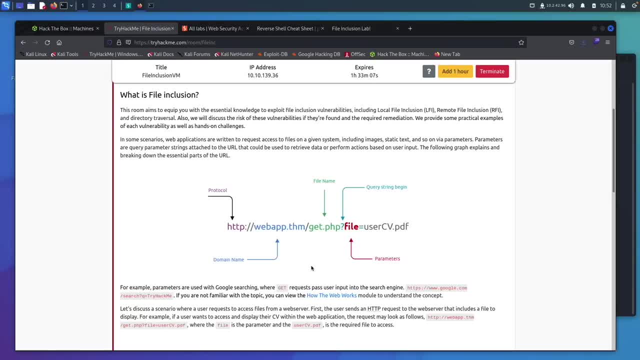 membership, you're not going to be able to practice this. So what we have going on right here, this is really great explanation. I'm really happy with how they have this all structured. So you have your basic web application right here, You have the HTTP, the URL, and then you have a getphp and 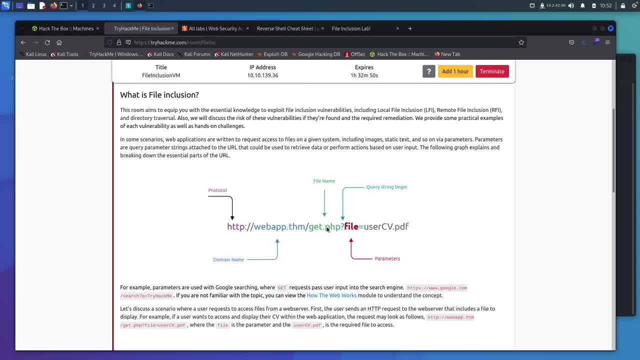 this PHP right here is going to be a giveaway of the way we're going to go about trying to pull this file down. So oftentimes you're not going to see a php, but sometimes you will, and when you see a php and then a file equals just like this, you can think you can try for an LFI. 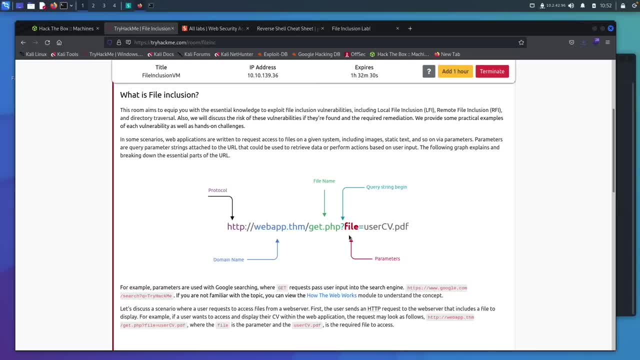 and we've already talked about directory traversal and typically if something is vulnerable to a directory traversal, you are going to be able to pull down files as well. and once you have LFI- which is pretty bad- if you can turn that into remote file inclusion, then you have 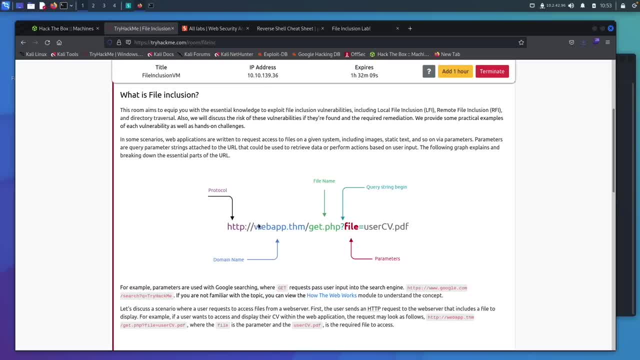 got something really, really big going on for you. So we have this URL that's going to make a get request to the server for a specific file and it's going to equal the file that you click on, and I'm going to show this to you and I think it will make a lot more sense. I've already opened up the lab. 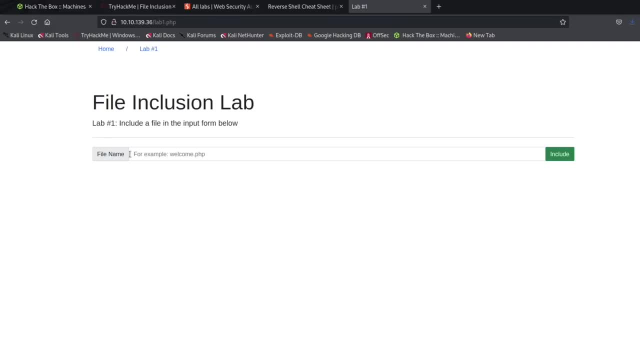 here, When we click on lab one, it tells us it's got this lab1.php and you can come in here and you can just type something in. So if we just type in anything, because we don't really want to look for a file just yet, Actually, I'll just show you this way. So if we come in here and we type in, 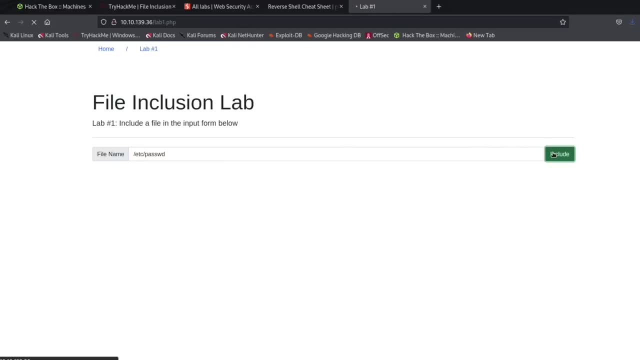 etsy passwd and we say: include it pulls it down for us. but this is not, this is not going to happen, Not real world. So what will happen is something like this: you'll come to a page it'll have like this request: right here you're searching for something and say it's a search bar and we just 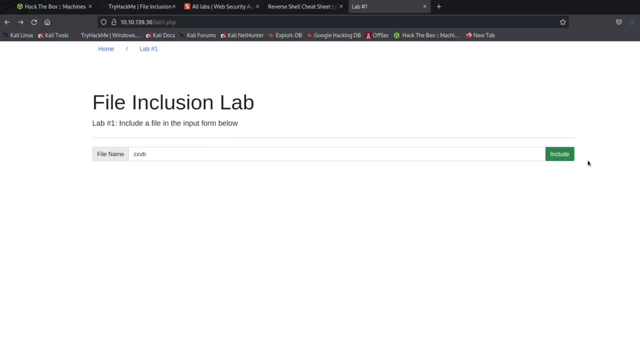 type something in and we intercept this in our proxy and we hit include. we'll send this to our repeater. we can turn this off. and now what happens is it tells us we'll just pretend all this isn't here because this is not going to happen in the real world, but this will happen right here. this. 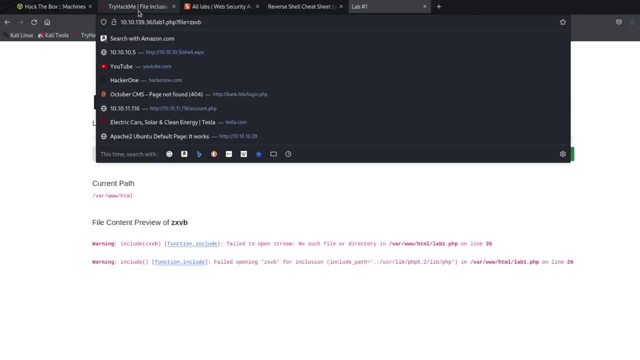 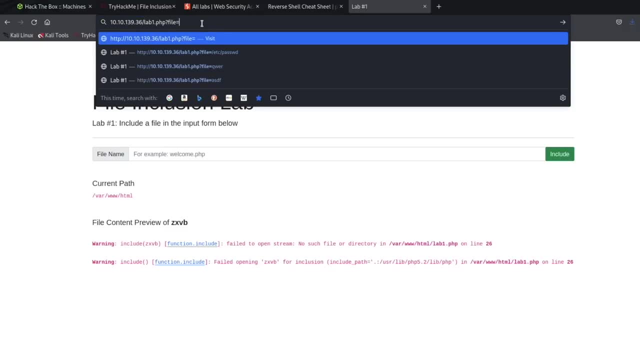 file equals and then what we typed in Looks like what we had going on over here and this really does happen and up here we can change this and we can now put in this etsy passwd and it will pull it down like this and a lot of times you'll. 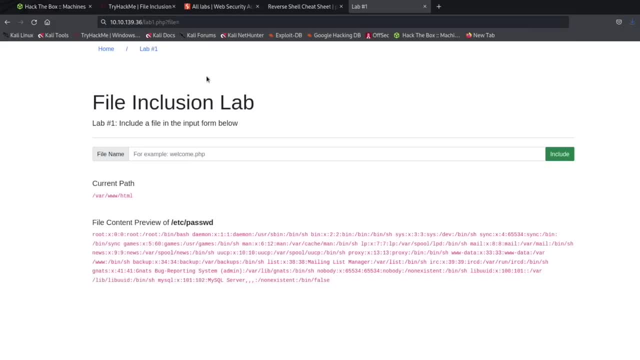 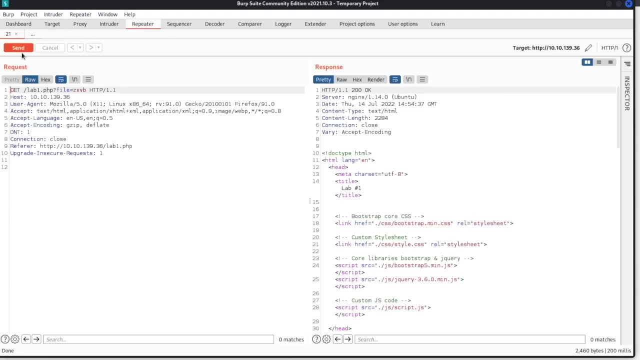 have this file equals up here and you can play around with it. but rather than using the URL I would rather use burp, So we can come over here and we can say send, and I like that. it tells us we have this nginx server right here and I'm sure if we ran like an nmap scan it would tell. 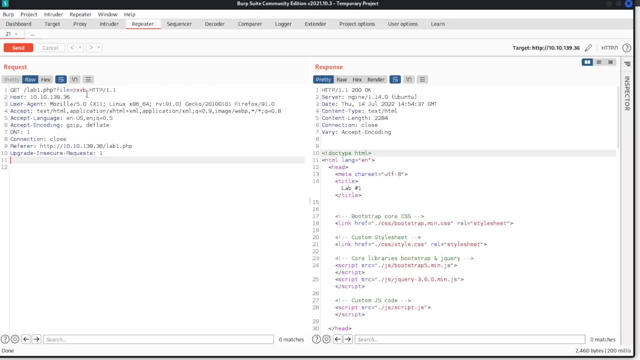 us what we're up against completely. but we're not going to do that. we'll do that in just a minute with an LFI on a hack the box system and we will test it there. but we have this file equals and then we have right here where we can ask whatever file. we can ask for whatever file we want, so right. 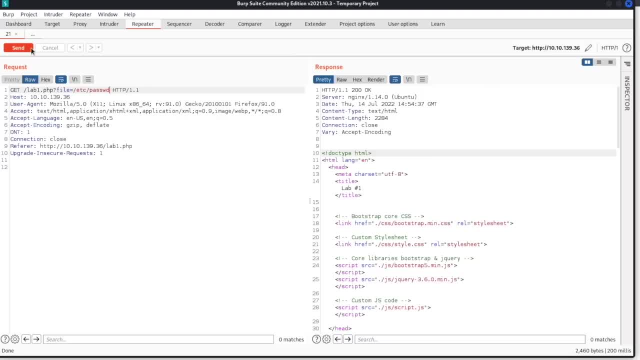 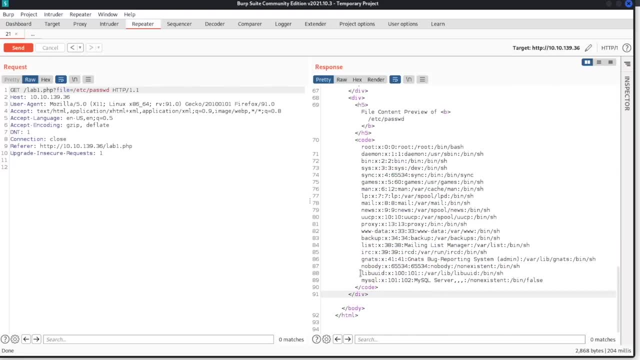 here we can put in our etsy passwd and we can send this and on the page it tells us we have users bash. that's going to tell us people who have actual users on this box. there's actually quite a few of them- or a bin sh, not a bin bash. we have root has a bin bash. so when you pull this down, 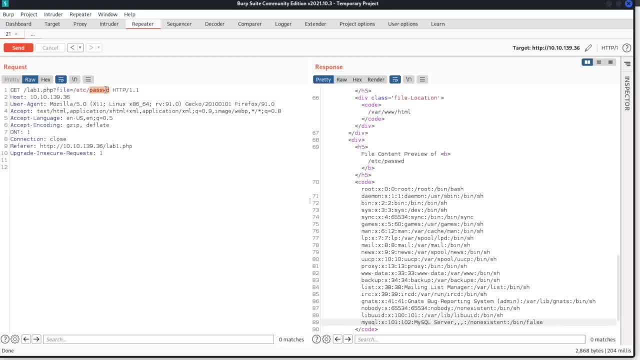 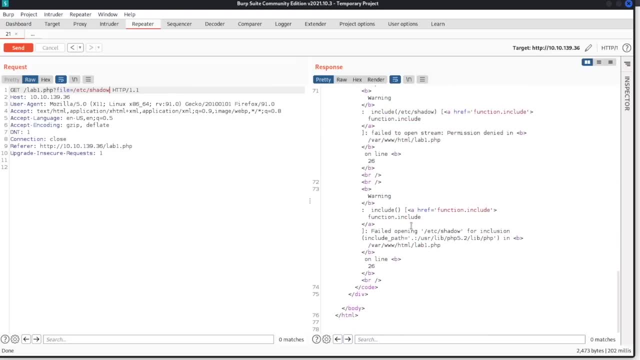 you can look for users. and it's even worse if you can access the etsy shadow file, because then we can actually pull down password hashes, and we don't have the ability to do that. so this would be a file inclusion and you can pull down all kinds of files. 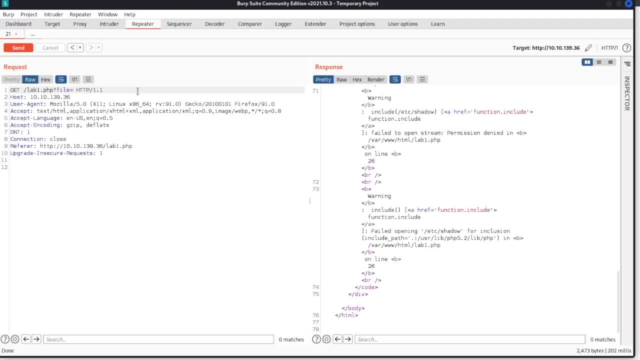 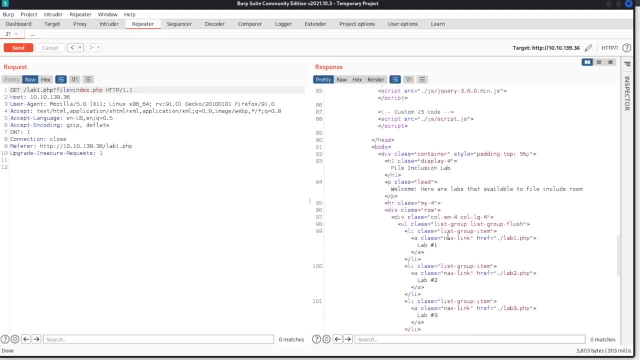 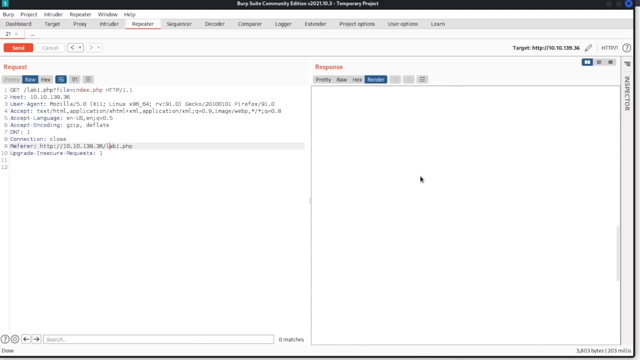 from the server so you can actually pull down. let's say, we wanted to look at the indexphp. you can send this and it'll pull down. I can't tell if that worked or not, because there's just a bunch of html. let's render it, maybe we can see it. yeah, so it just pulled down the home page, like right here. 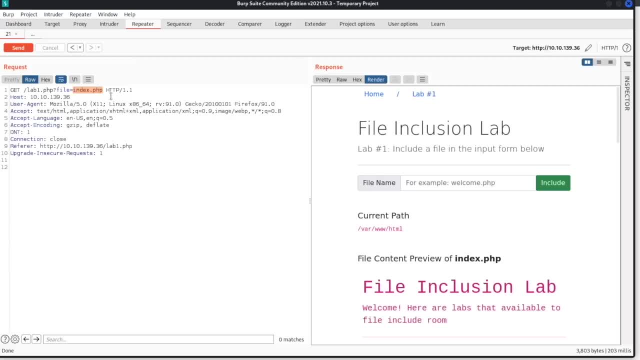 so you can look at different pages in here. so let's say you were able to director, you were to do some kind of fuzzing on this page and you were looking for different directories and you had a directory that you weren't allowed to look at like a hidden directory in here. you could probably include this. 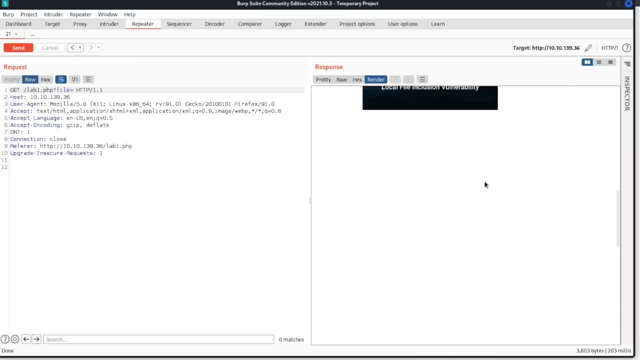 in the file and it will pull down that hidden page below right here, and because we're able to do this local file inclusion. when you have local file inclusion, it's a great vulnerability to find. it's one that it's a pretty severe vulnerability. but if you can turn this into a remote file, 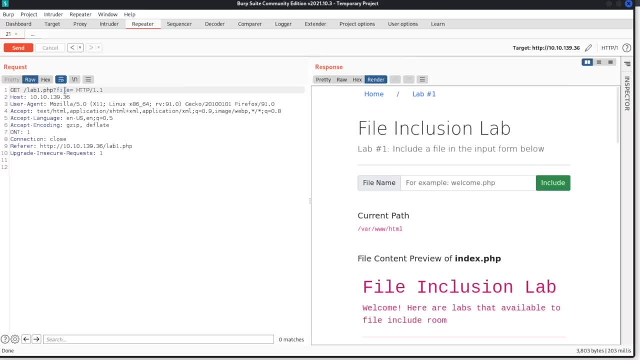 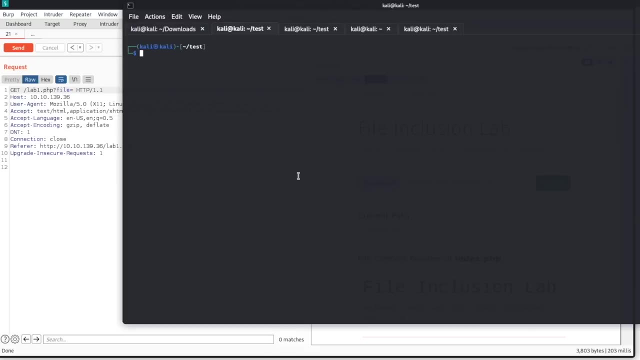 inclusion, then it becomes something more. so right now we have what's called local file inclusion. we're able to get local files that are hosted on the Target server, but if you're able to have remote file inclusion, that means we can include files from our box over here. so if you look at what we have in 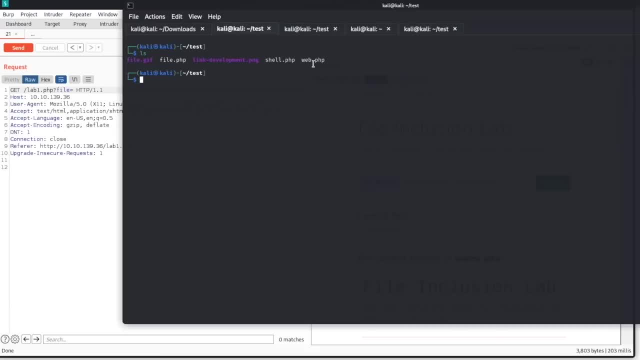 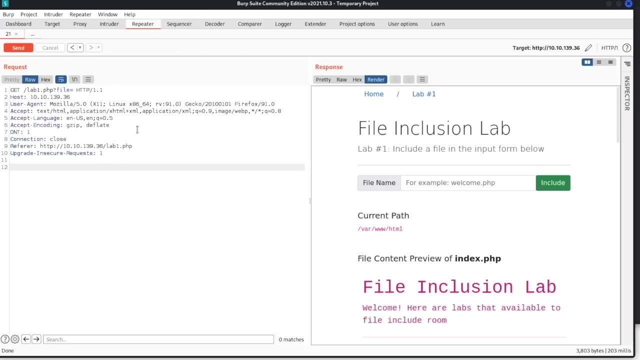 this file. we have a shellphp right here and a web shell over here. if I have remote file inclusion, I can. I can have this get request. reach out to my server over here that I can host up, and I can host up this file right here and it will go get. 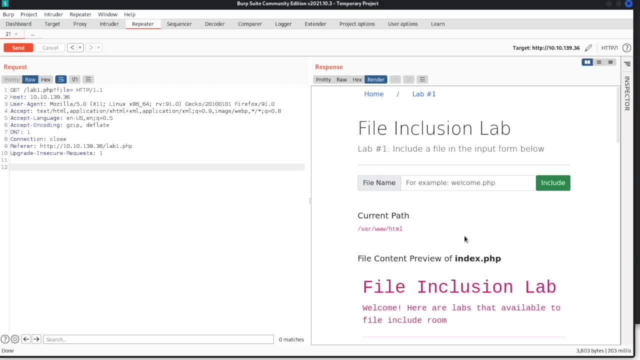 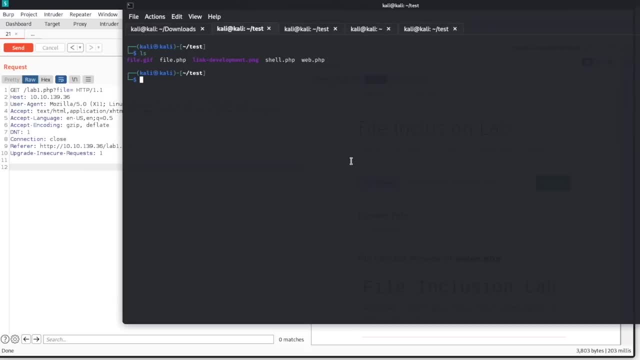 that file and then execute it, and then I can have remote code execution on this server and I will own this Network. so what? this looks like an easy way to test for this, like if you were to do this in a bug bounty program and you were just looking for a proof of concept. you would just type in: 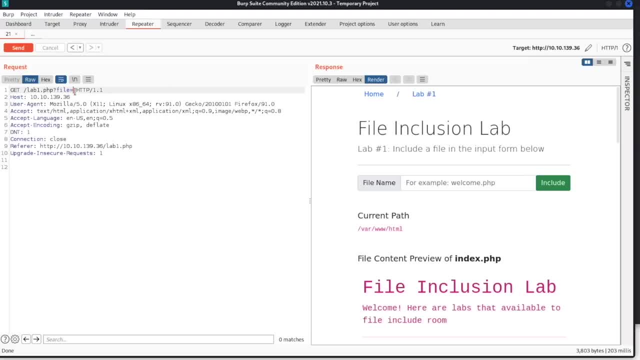 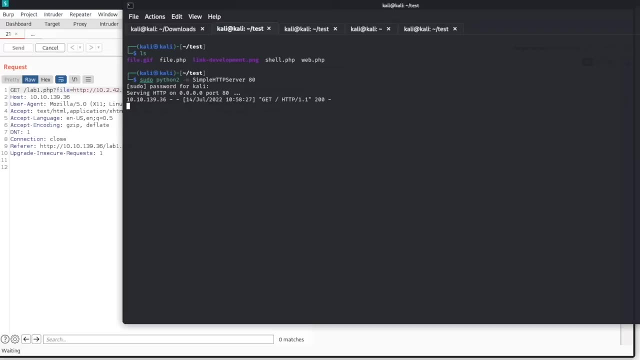 pseudo python 2 with a simple server and then we would just put in our IP address and see if it got to us. so we can go HTTP 10 to 42, 96 and we can send this and see if we get a hit over here and 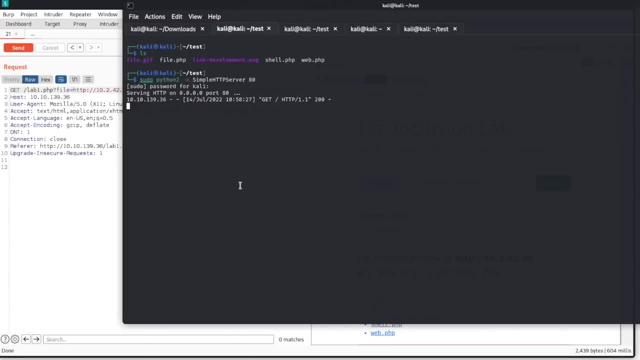 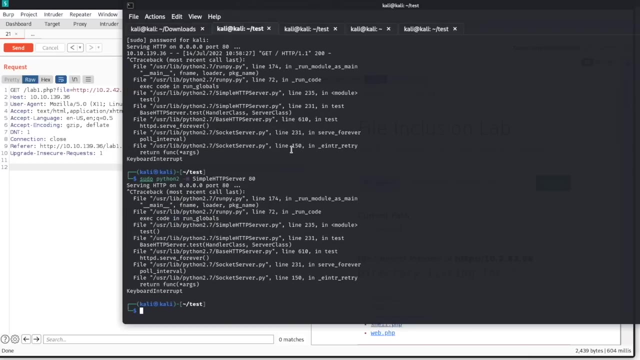 we do so. this is so. this means we can actually get remote code execution on this server. so what we can do now is close out of this. we'll re-host up those files and I've already edited, and I've already edited the shellphp, so you wouldn't have to watch me change the IP address. 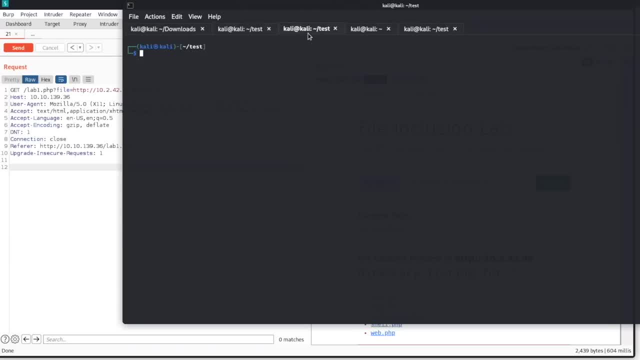 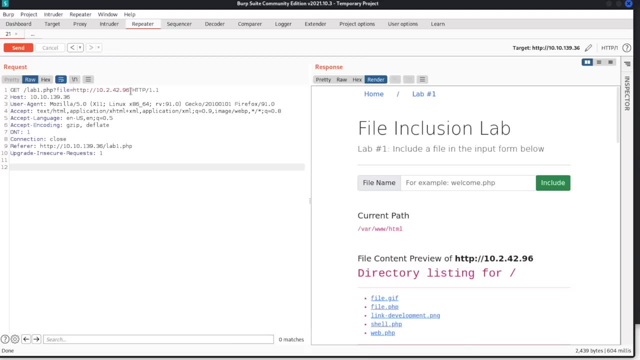 right here. so it's all set up and ready so we can host this back up. we can come over here and say netcat, port 444, and if we send this right here, we want it to grab shellphp. and now if we send this, it's going to hang right here because we have a shell and we could say who am I? and it now tells: 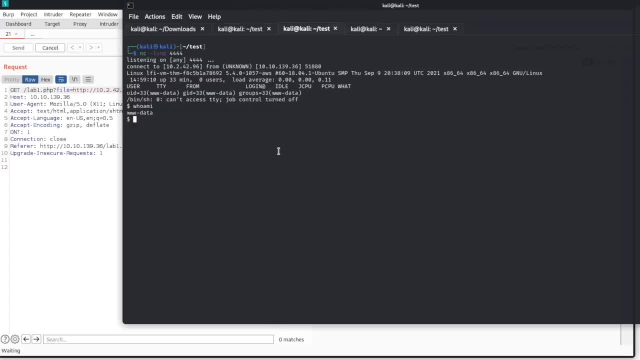 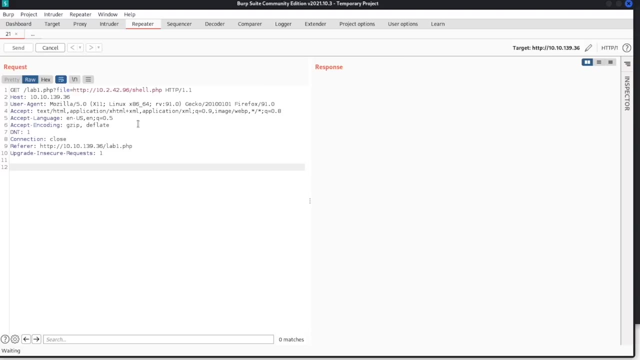 us our www data. so we now have code execution on this server and this would be pretty much as bad as it gets. now I want to show you a little more local file inclusion and how to read pages when they don't render over here when we ask for a specific file and we want to see what's happening. 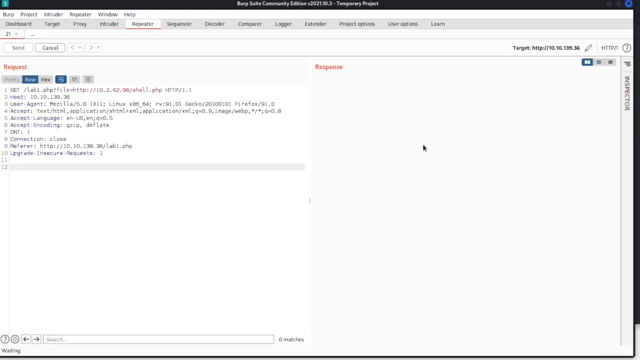 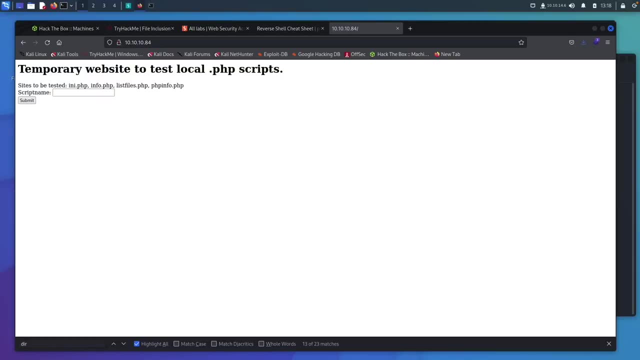 and I'm going to switch over to hack the box for this. all right, I have loaded up the box poison here for us and if you have a hack the box subscription, it would definitely be worth your time to open this up and play around with it so you can see if you're able to find any of these. 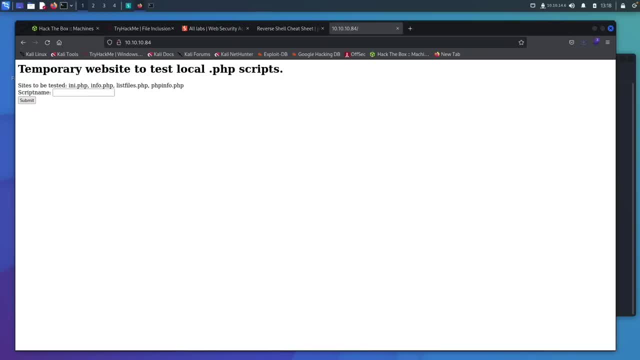 LFI files on your own. so we're going to go ahead and just play around with this for a little bit and I want to show you some of the things you can do with lfis. that can really save you a lot of time and, if you're doing CTFs, help you find files that are that you shouldn't be able to access. so 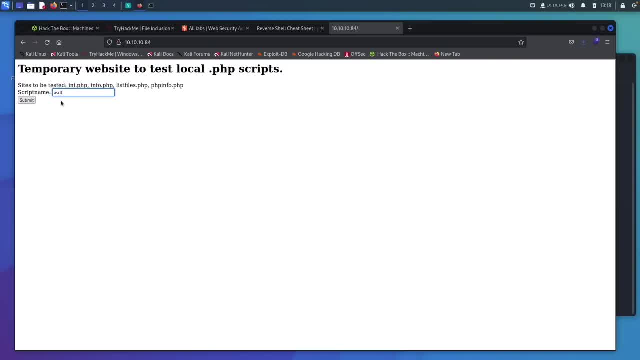 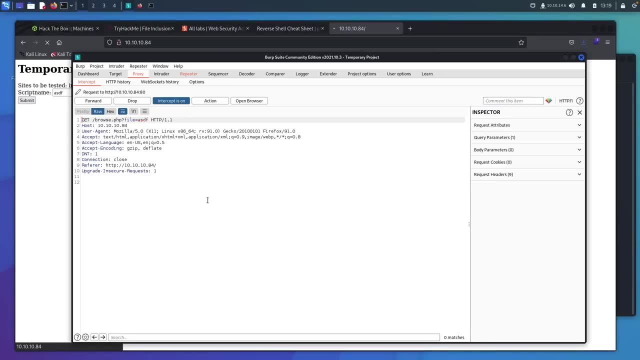 we're going to do the same thing we did before: we'll just put in some characters in here and we're going to catch this over in our repeater, so we'll hit submit, we'll send this over to repeater and then we can turn this our interceptor. 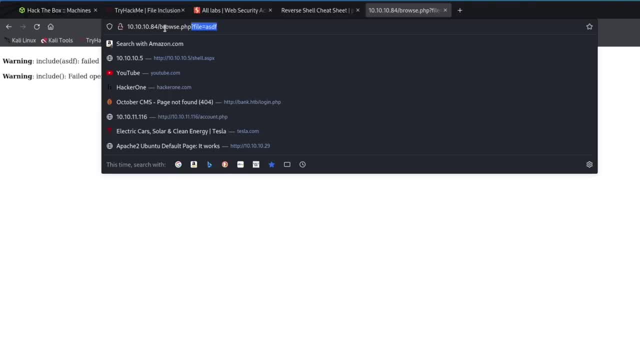 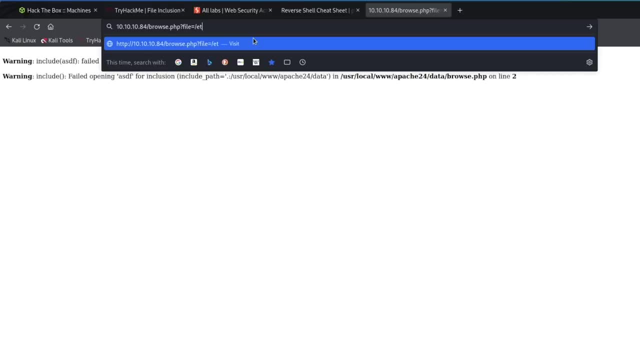 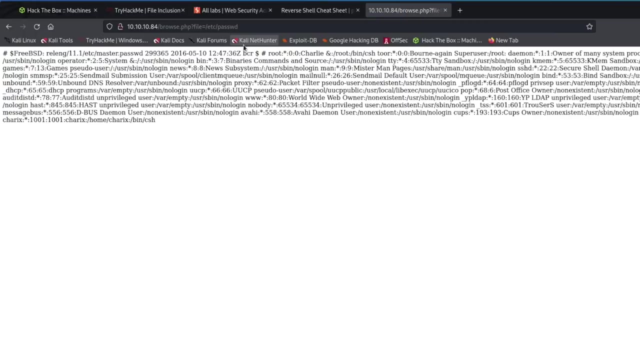 off, and now you can see. before we didn't have this file right here with the browsephp and then the file and then our request, so you can, like I showed earlier, try and get files right here like this, which is fine, but I like to use repeater, just because it goes a lot faster. so we're going to go ahead and use. 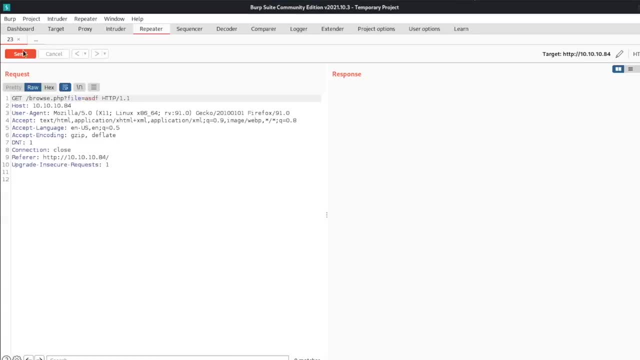 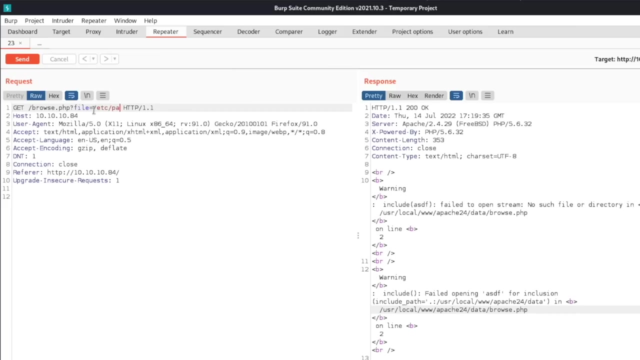 repeater. so we'll hop over here and if we send this, we get this simple message over here saying that it failed to find this through the inclusion and it tells us the path we're using right here. so what we can do at this point is we can try and type in etsy pass WD and if we send this, we can. 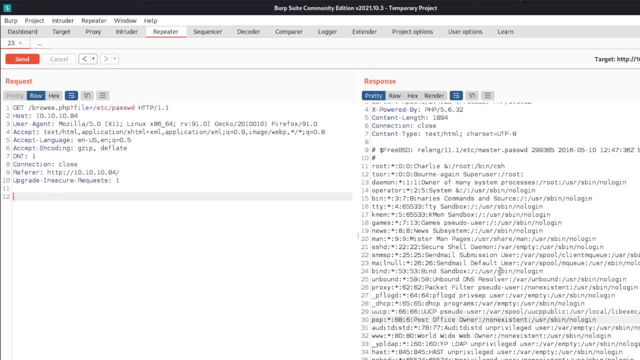 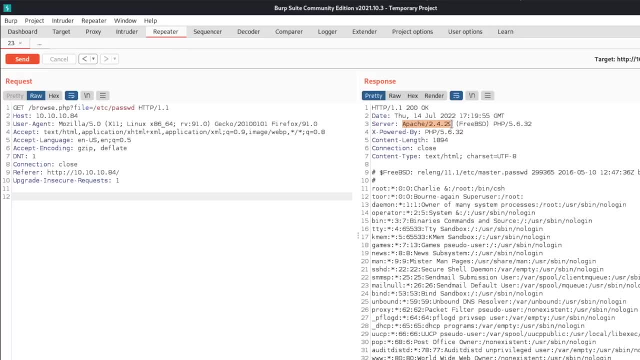 see we have the etsy pass WD file right here and something to always look through is these: the server version you can highlight. you highlight this, copy it, go to Google, see if there's any vulnerabilities and check that type of stuff out, especially when you're hunting for bug bounties, as 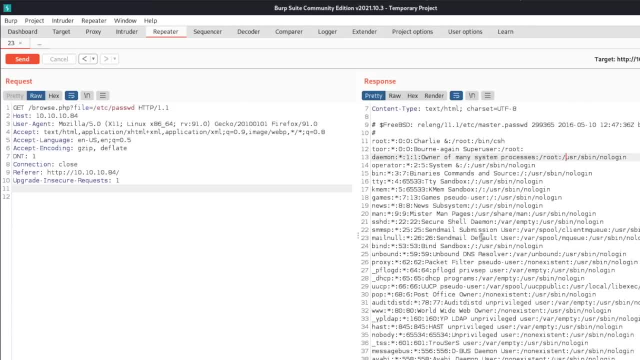 well as penetration tests. it's always worth looking at and then we can see the users on here is going to be this one right here, and then we have root. right here is a user. the rest of these don't look like they have the ability to log in. now on to looking for. 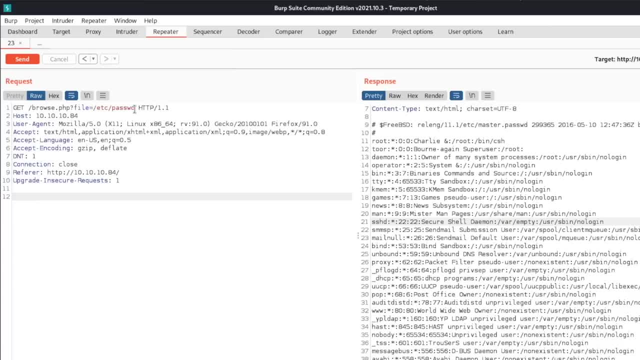 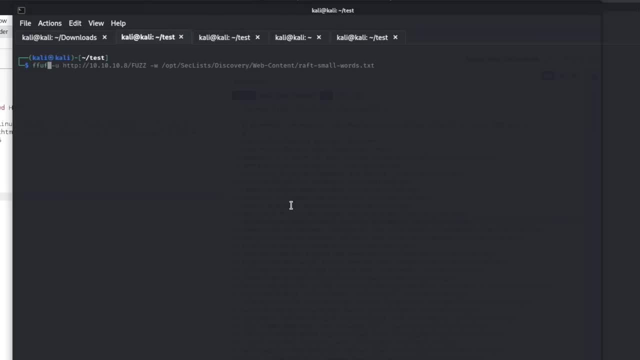 more files. there's a really simple way to go through the files really quickly and I've used the tool fuff a lot with a lot on my channel. so we're going to go ahead and we're going to use fuff and I'm just going to leave this in here and delete this a little bit at a time. actually, we'll. 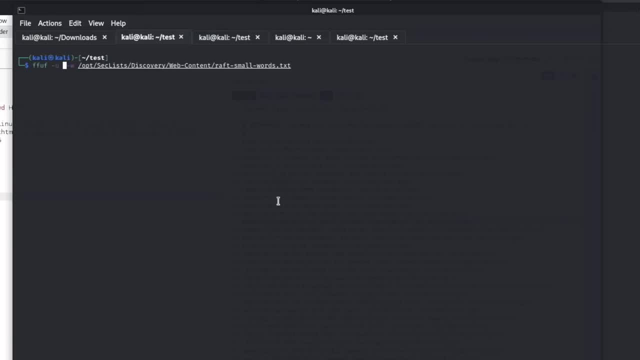 just delete this whole thing. so we can delete this, what we'll need to do is highlight this and copy it, paste it into fuff and then, right here, we're going to want to fuzz, but to make sure we make it all the way back to the root, I'm going to just put some of these dot dot slashes in here. 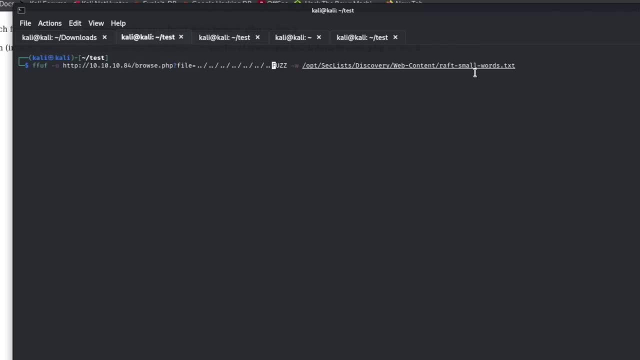 so that we can make sure we go all the way back to the root. and then we're going to fuzz- and we don't want to fuzz this with the web content. what we want to look for is the LFI content, so we can come back over here and I think we just type in web. nope, we don't want web shells, we want. 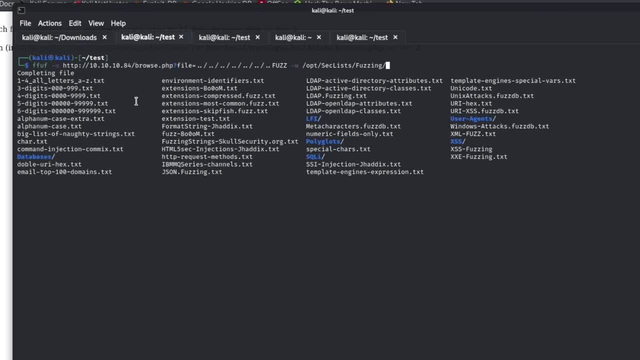 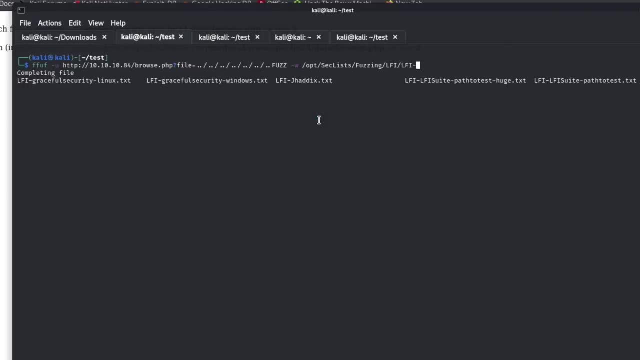 fuzzing right here, so we can type in fuzzing. and then we want LFI, which is right here. so we're going to go into that directory and see what's in here and we'll use this one, because we're up against a Linux box. we can just type in Linux. that did not work for me. we'll type in like that. 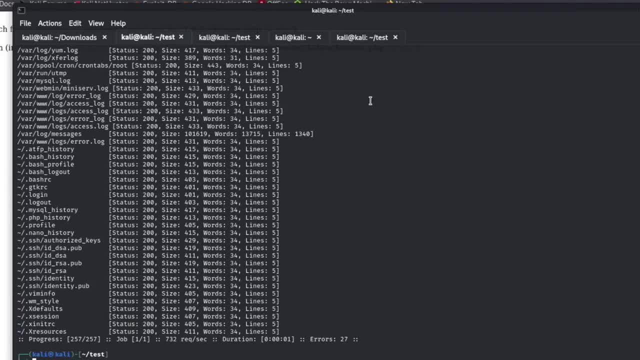 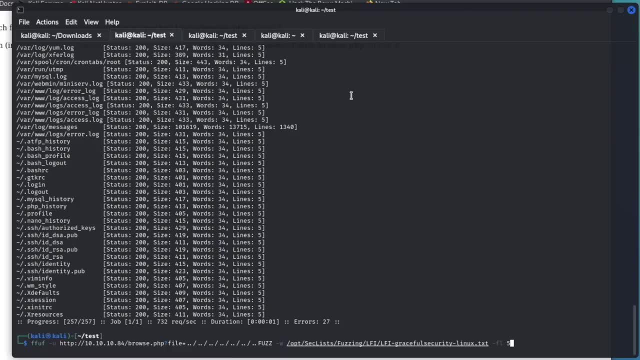 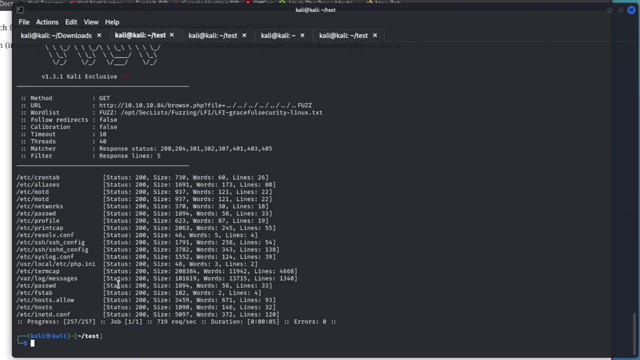 if we run this, it should work for us, and it does. but we don't want all of that output, so we're going to filter by lines and we're going to say: if it has five lines, don't include it, and it's going to give us all the files that we're able to look at. now. if I was actually doing a CTF, I would look. 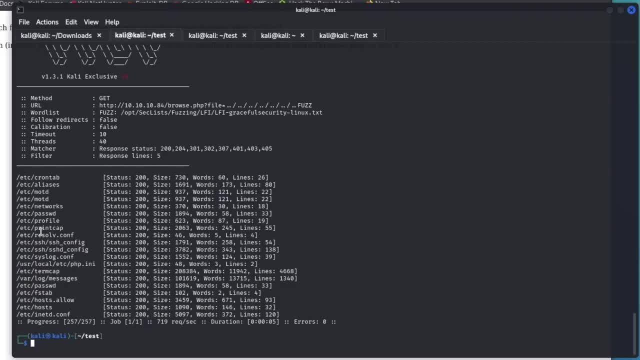 through every single one of these to see what we can find. now. obviously we tried the etsy pass WD, but you can come through and check out all of the files and see if there's anything helpful for you to try and get remote code execution on the box. and because we don't have an RFI, which I have not actually tried, so we'll go ahead and try. 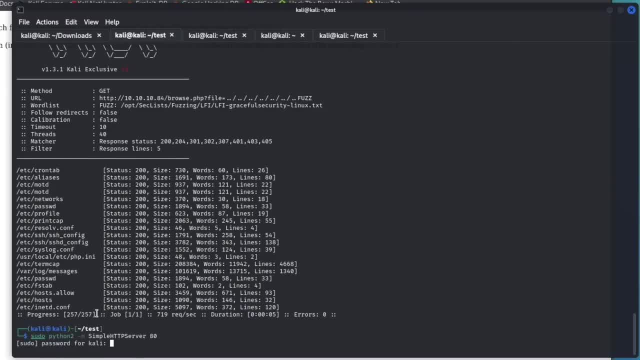 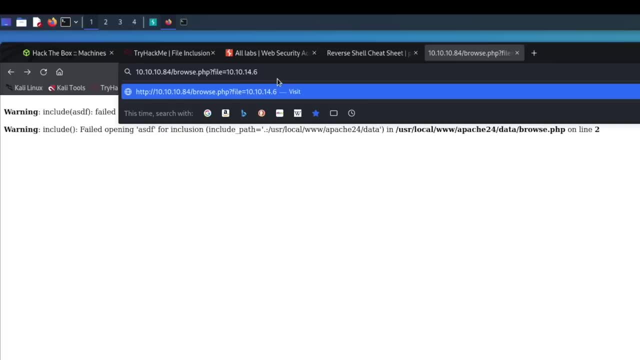 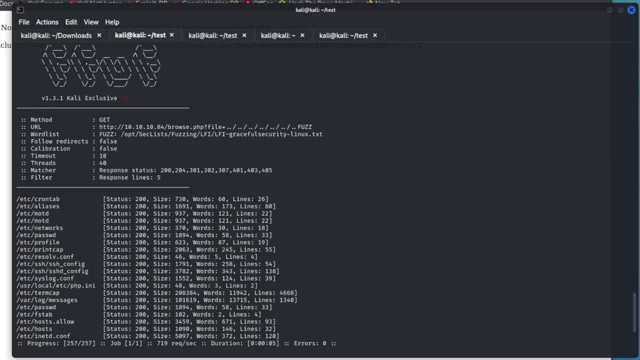 it and make sure that this does not work and we can put my IP address in here which is 10, 10, 14, 6, and it doesn't hang no RFI, so we aren't able to include any of our own files to get a shell back. 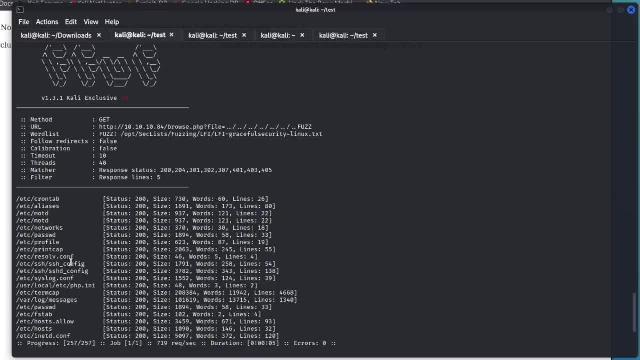 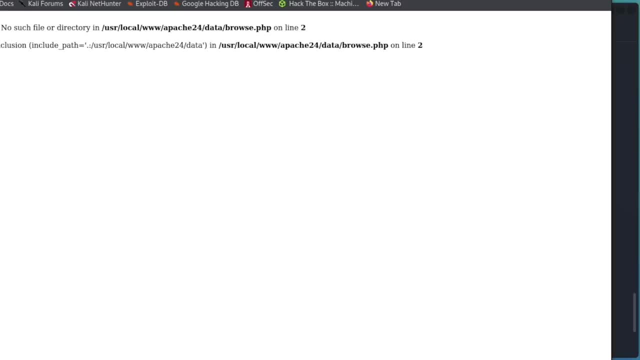 that way. but you could look through all of these and see if maybe you can find some credentials or something or maybe be able to SSH into the box. but this is a quick, easy way to fuzz when you have an LFI and in a real bug bounty situation. you wouldn't want to actually enumerate any of this. you would 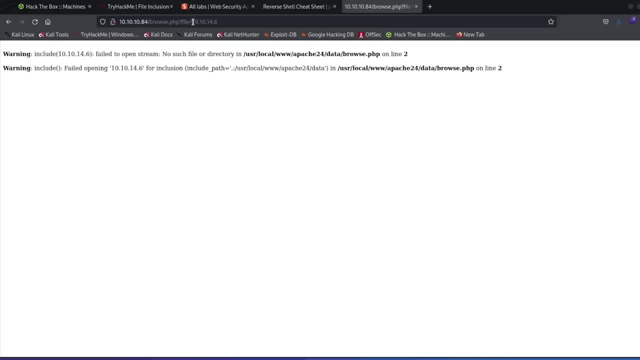 only do something like that on a CTF. you would really just test for an LFI, like I've already shown you, and make sure that it is there, and then you would submit a report. or if you were testing it right here and set up a simple server and see if you can reach out to yourself for an RFI and 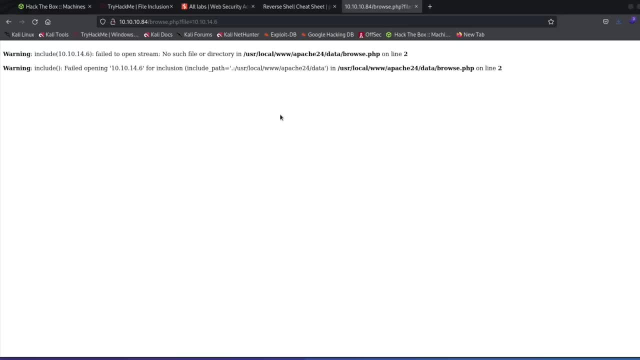 that is the remote file inclusion and the local file inclusion. you can go ahead and play with these. if you have a try hack me and a hack the box subscription and get used to seeing these, you're going to see them a lot inside of CTFs, especially LFIs. RFIs are a lot more rare, but 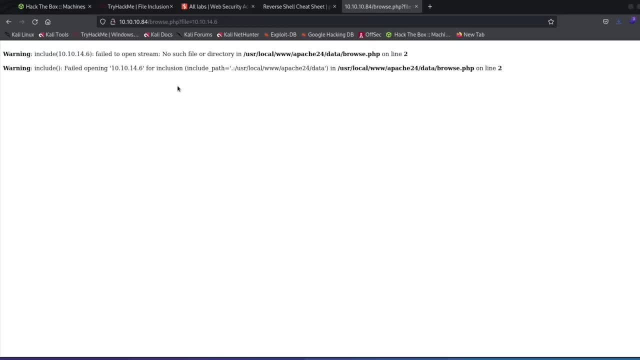 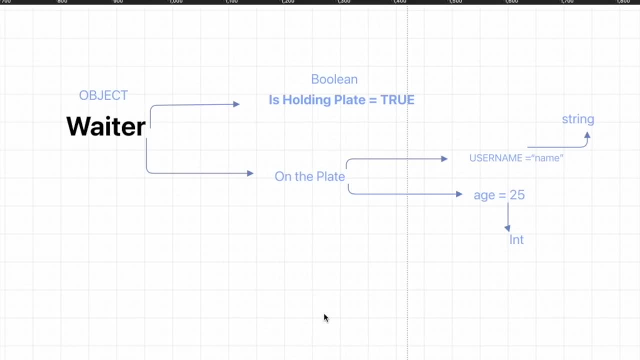 they do happen. so with that we will move on to the next vulnerability. all right, we are going to be going over some insecure deserialization and I decided to make a little flowchart here so that you could kind of see what is going to be happening. and this is for PHP, but the concept is: 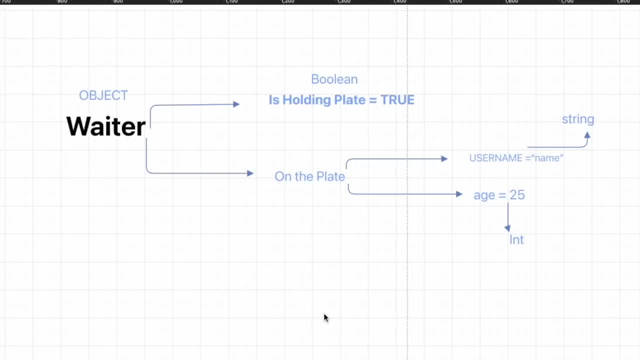 going to be the same for Python and JavaScript as well, but the examples we're going to be dealing with is PHP, so I decided just to show you PHP. it'll make it a lot easier for you. as we continue going, we're going to have just a few places to practice. this is something that there is not. 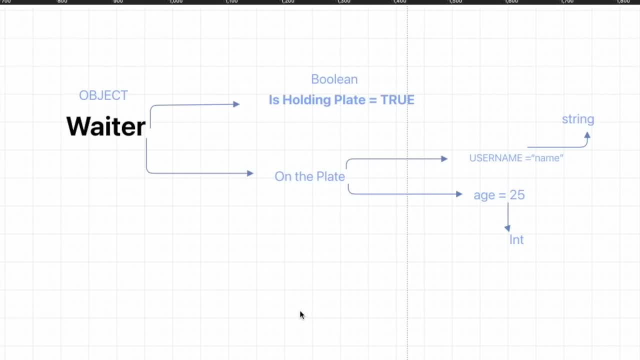 actually a lot of. so I'm going to go ahead and show you some of the things that we're going to do. a lot of places to practice, so I wanted to show you here and then I think I'm going to show you an example, and then you should be able to solve a few challenges on your own, and if not, we will. 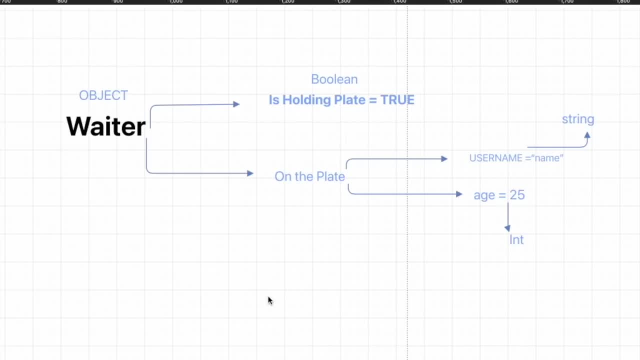 walk through them together and I think you'll get the hang of this pretty quick. it's not super difficult, but it is something that a lot of people are afraid of, but nonetheless, let's jump into it. so we have what's going to be the waiter and he is the object. this would be like if you have. 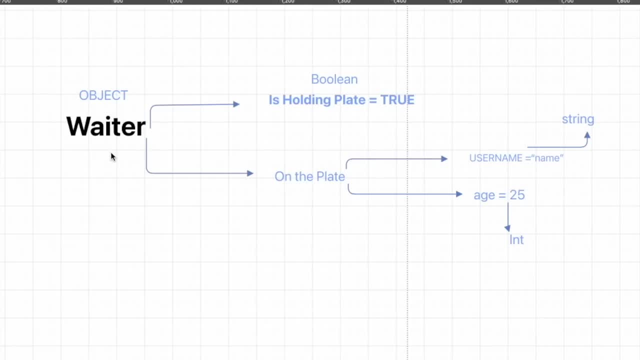 a inside of programming there's something called object oriented programming, and I don't want to get too much into it, but just know that like, this is the object, and the object can contain different things with inside of it. so you have the waiter and he carries a plate, and so with the waiter, the 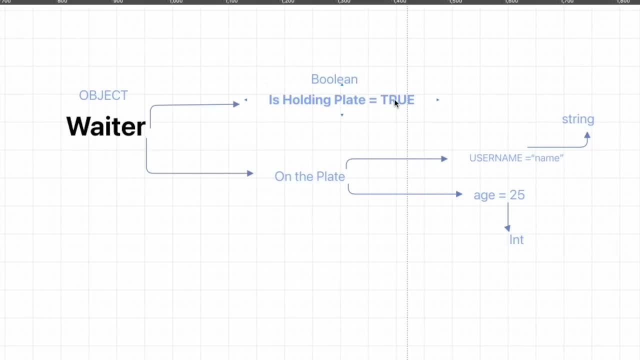 question would be: does the waiter have a plate? and it's true or false? this would be a Boolean and within PHP it's represented as just a B and then it'll say B equals, and it'll be one or a zero, so that'll be either true or false. so does the waiter have? 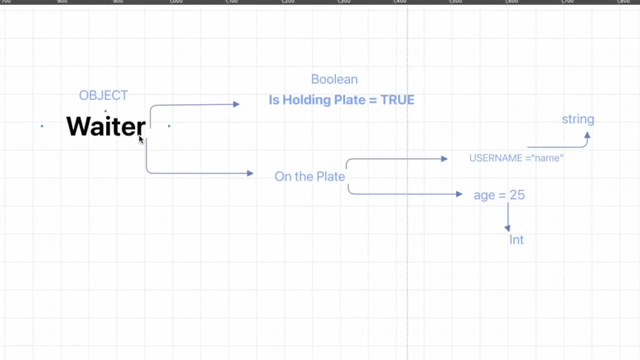 a plate and it would say true. and so in this case it would say: waiter, have a plate, B equals one. and so you'd say, here the waiter has a plate. and then, if he has the plate, we come down here and it says, like, what is on the plate? well, on the plate there may be a username and the username. 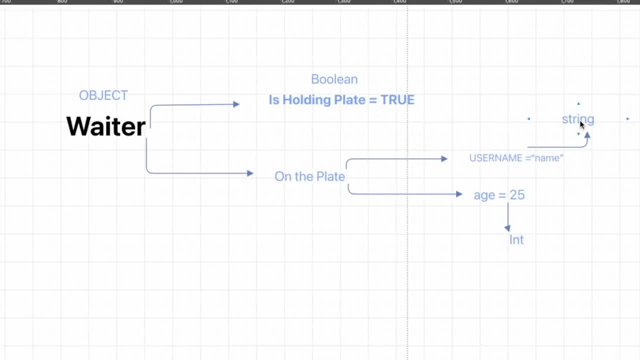 when you see these quotation marks like this is stored as a string and so the username has a string and so Within a object you would see something like S username and then it would have the name, And the S is going to stand for the string. 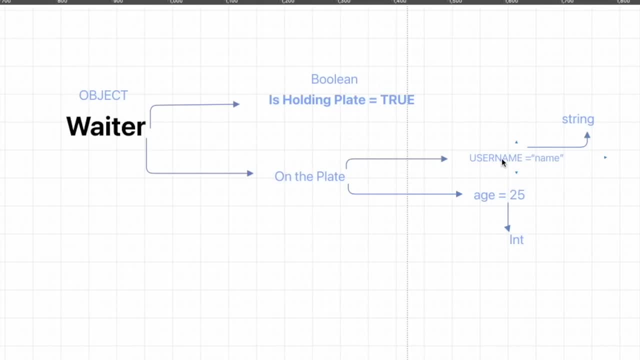 And then you will have, like, maybe the person that is being and maybe the object is going to contain an age, And so on the plate, there's going to be more data and it is going to be an age, and it's going to be 25.. 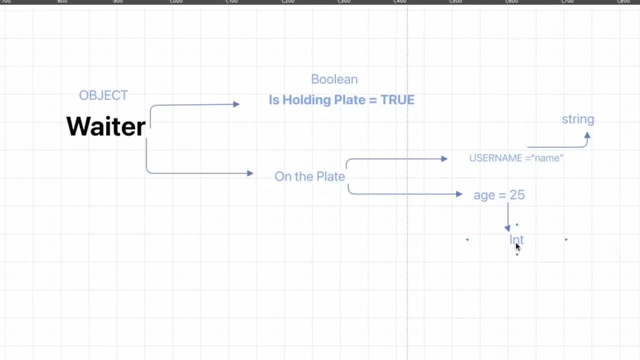 And it is an integer because it's a number, And so this would be represented as an I, So it would be like I age equals 25.. And it sounds confusing, but we're going to see what this looks like here in just a minute. 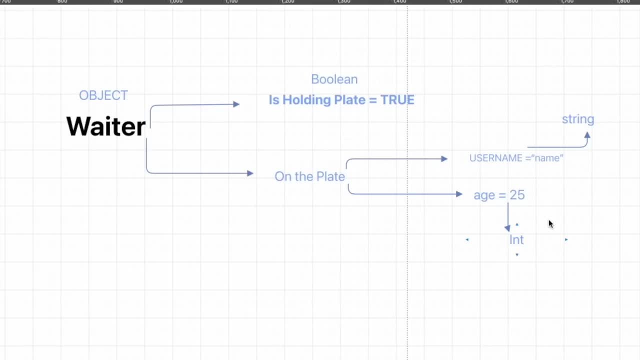 And it will all make sense, And I'll come back to this and show it to you once we get a look at once we look at the full picture of what this looks like inside of a cookie. So let's take just a step forward, just a little tiny step forward, and look at how you're going to go about exploiting this. 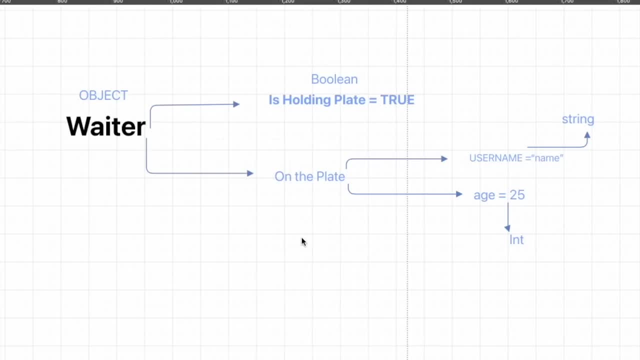 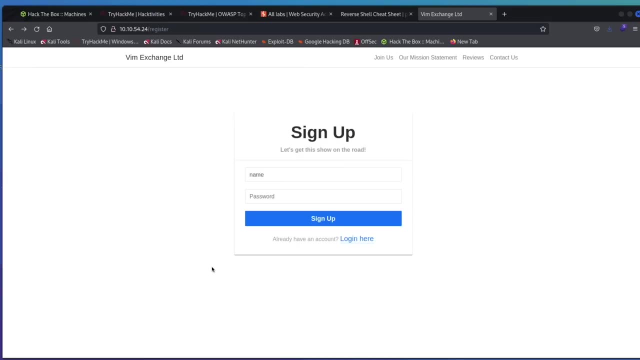 And then we'll go ahead and exploit some of these insecure deserialized objects. All right, So I have. So I have opened up a try hack me box here And sadly it's not a real great example for an insecure deserialization vulnerability, because I already created a username with the name name. 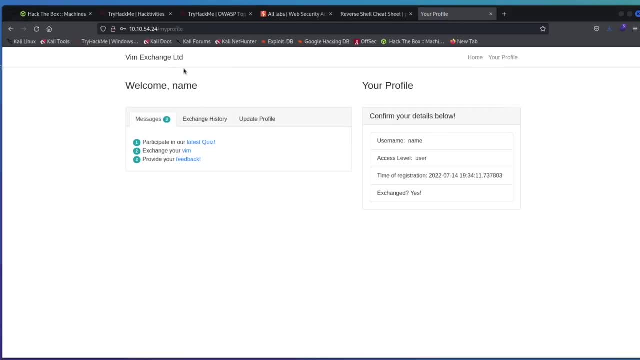 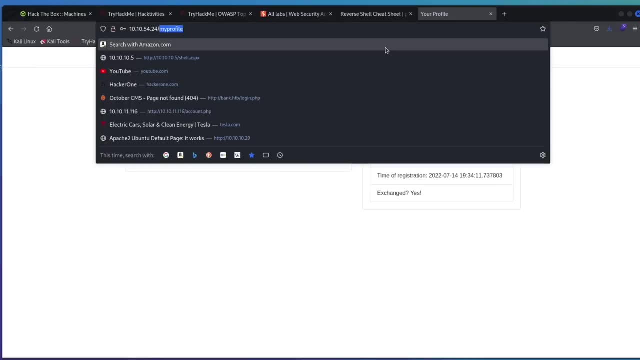 My password is name And if we log in it brings us to this page. But in the real world, if you came to something like this and you just fuzzed this with a fuzzer- something like fluff or go buster or derp- and you would find this directory called admin and bam, you're here. 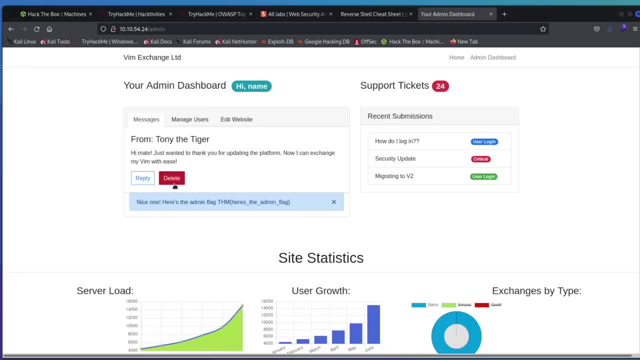 And you're in the administrator dashboard, which is kind of a bummer because you're just automatically in here and it tells you like here's the flag and you've made it inside of the dashboard And so what we can do from in here. I want to test this in here and then we'll go back to our user profile and we can just inspect this like we normally would. 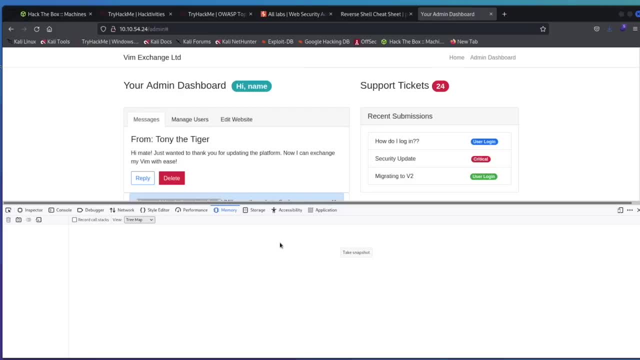 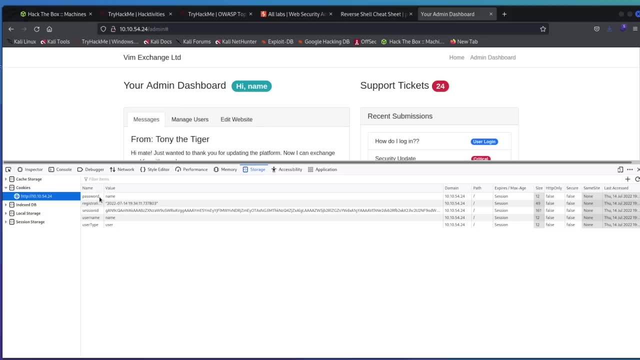 We'll come over to the memory, which is where the cookie is going to be stored. We'll come over to the storage- Sorry, not the memory- Where the cookie is going to be storage- and it's going to say: we have a password, our session, our session ID and our username and our user type. 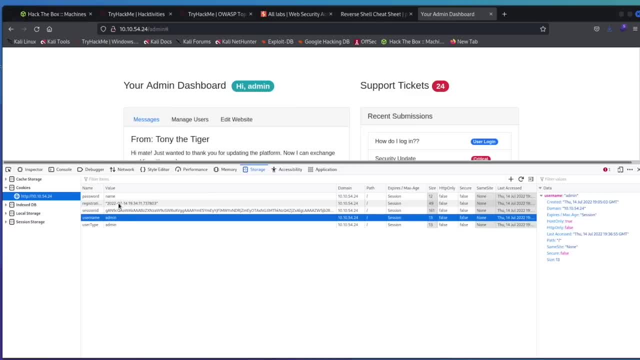 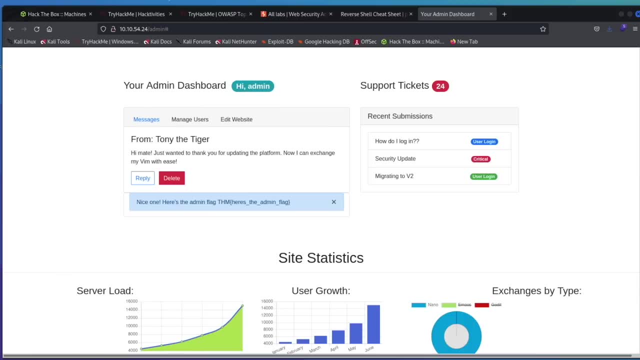 And in changing these cookies right here, you can manipulate the user type and the username. Now inside of burp. this also wouldn't be in plain text like it is right here. But if we intercept this and we refresh this and we say forward, we'll come and we, we have our interceptor on and we'll come. 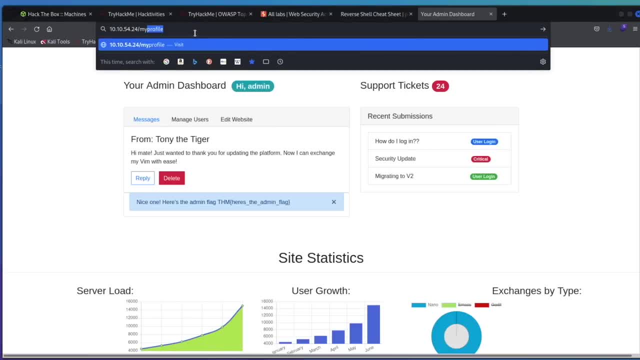 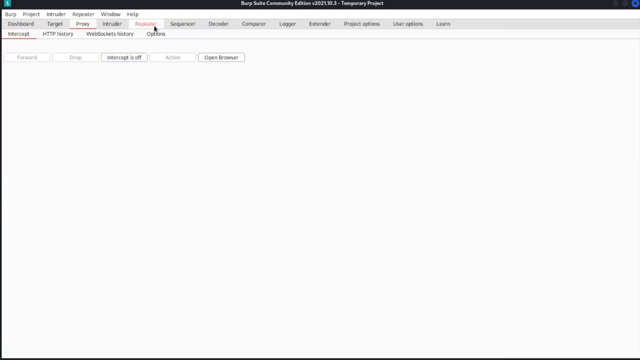 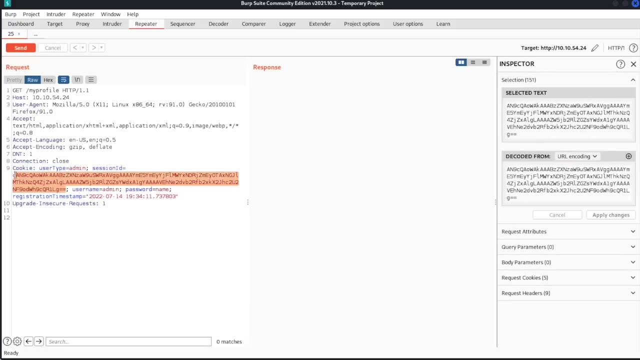 To the my profile page again and we forward this to right here and we send this to repeater. you can get a look at this. Like here's a username, admin password right here. like this is what we changed and we have this base 64 cookie right here. 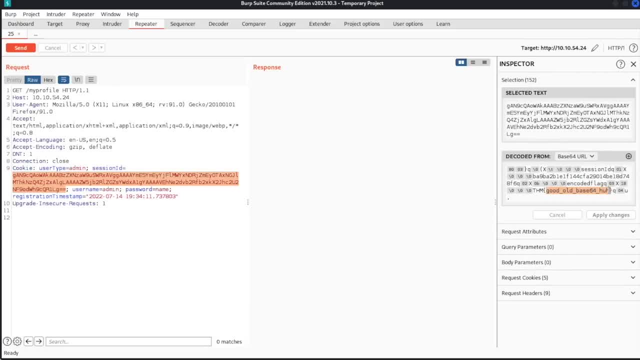 Let's see if we can decode it. Um, we get, we can get some of it, but what you would do with this is usually not going to be in plain text. It would be base 64. And you would have to decode it, and then you can change these things right here. 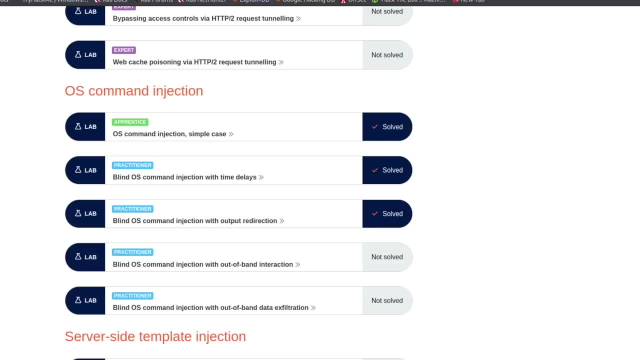 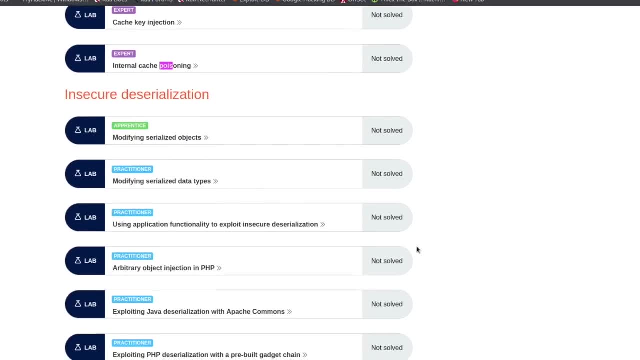 So with that, I want to send you over to a port swigger and we're going to go to the insecure deserialization right here And we're going to walk through some of these and you're going to get the hang of them pretty quick. 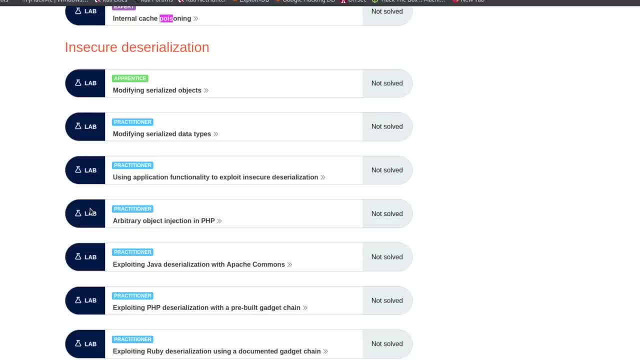 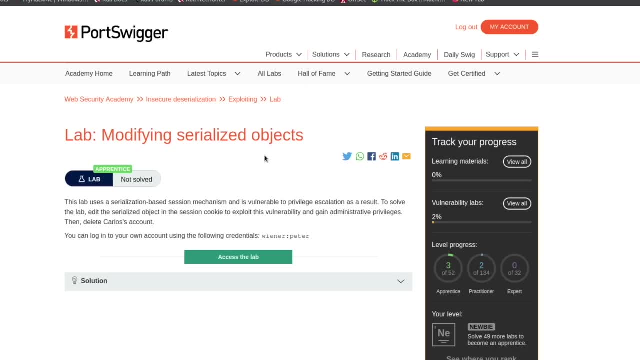 They're not as challenging as you might think. So we're going to do this first one right here And, if you want, you can go ahead and give it a try And see if you can figure out how to pull this off. But I want to walk through this one right here and then we're going to go back to the flow chart, because I think it's going to make a lot more sense once we do. 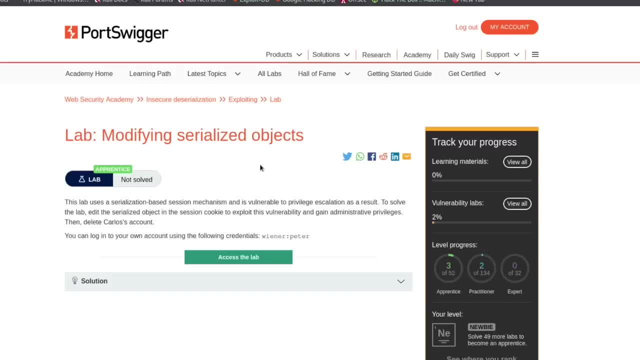 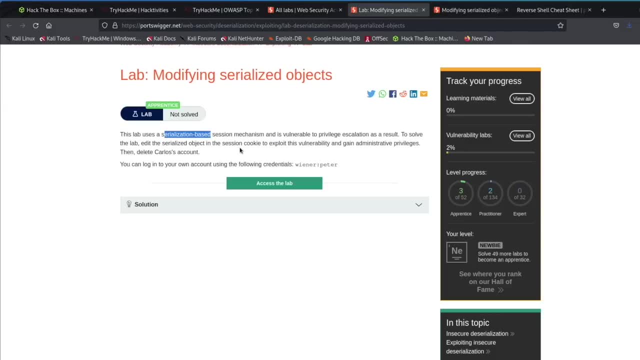 So you can go ahead and give this a try If you would like, loaded up here and the instructions tell us that we need to use a serialized based session mechanism and vulnerability and we're going to try and exploit it. And it says: here's our credentials to log in and we need to delete. 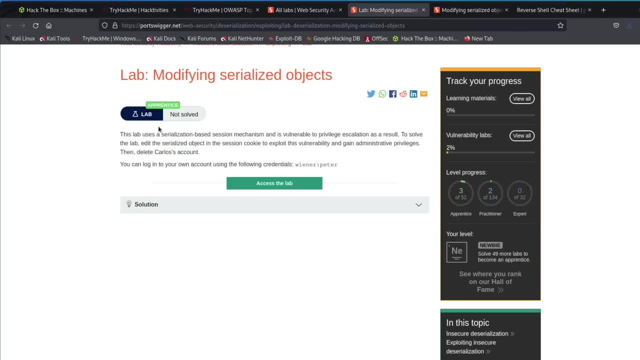 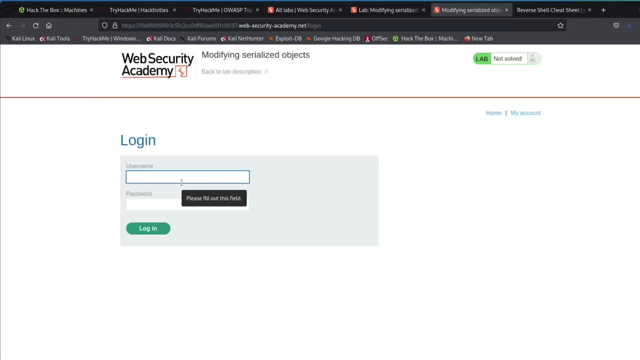 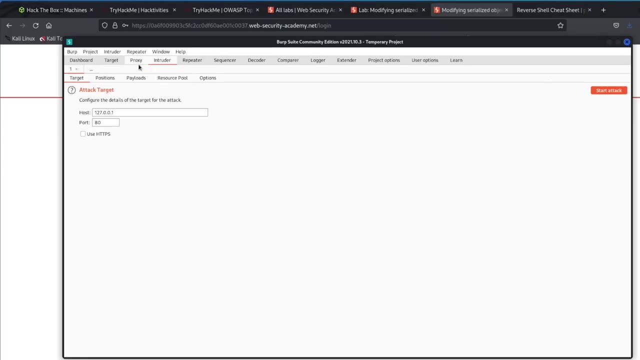 Carlos's account in order to solve this challenge. So what we'll do is we can just come over here and we'll need to make an account, and I'm going to call my account name and my password name. I'm going to intercept this just in case we end up needing it. 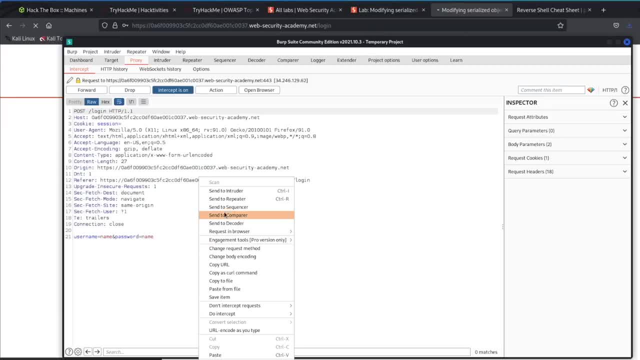 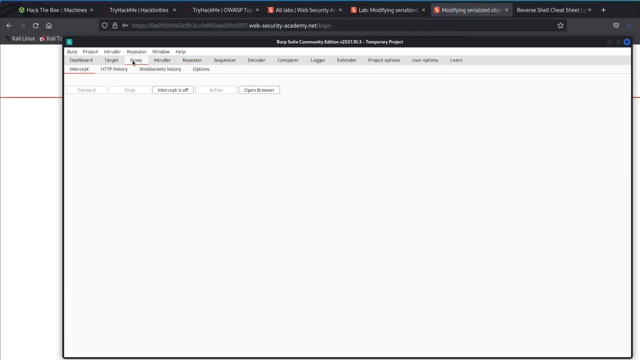 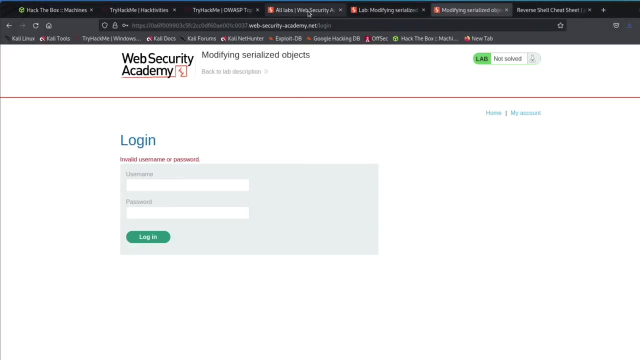 So intercept this, we'll send it. I'm going to send this to repeater. I don't believe we're going to need it though, So we'll leave that there. Come back over to our proxy. Oh, we have. we need to log in with the username that it gave us. 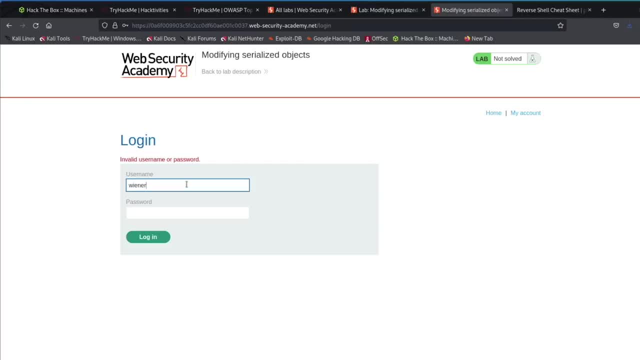 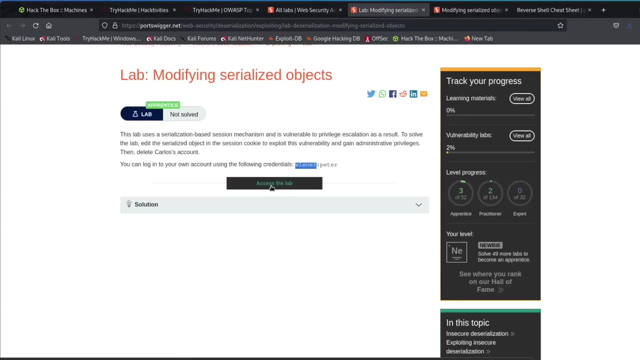 So we have right here our username and Peter, So we'll log in with this. and then it tells us we need to go to the to the admin panel. We need to use the session cookie to get, Go to the administrator panel or privileges, and delete Carlos. 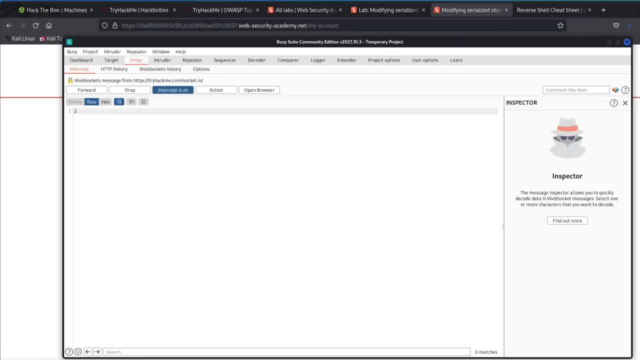 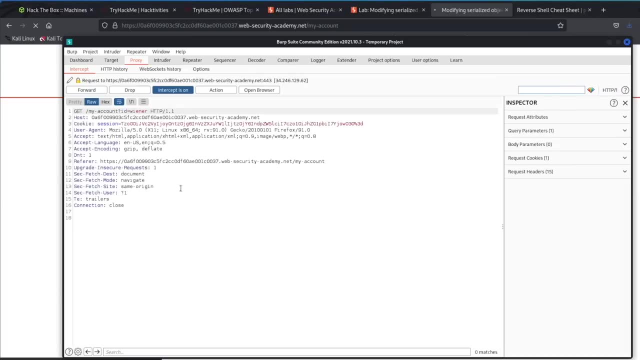 Okay, So what we can do here at this point is: you're going to come to this on my account, but we're going to need to intercept the request. It will look like this: You can send this to repeater: forward forward. 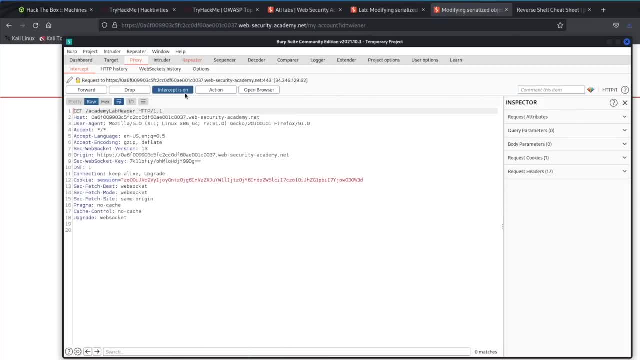 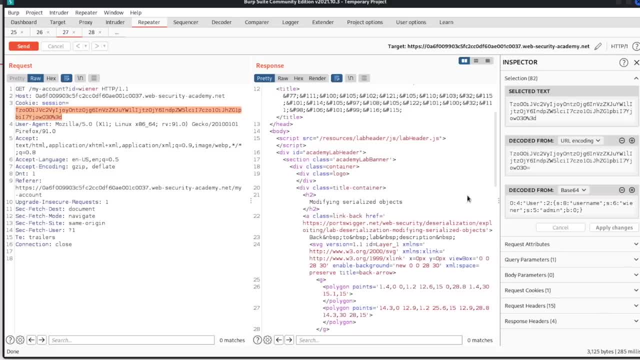 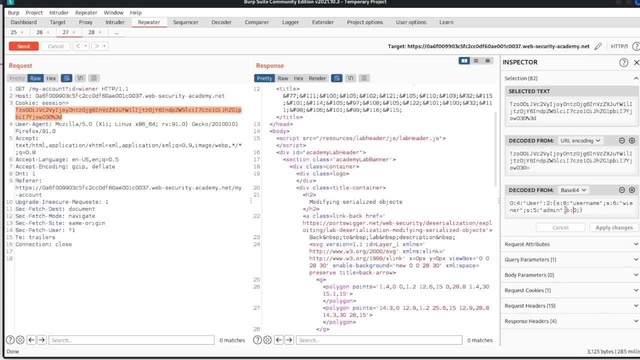 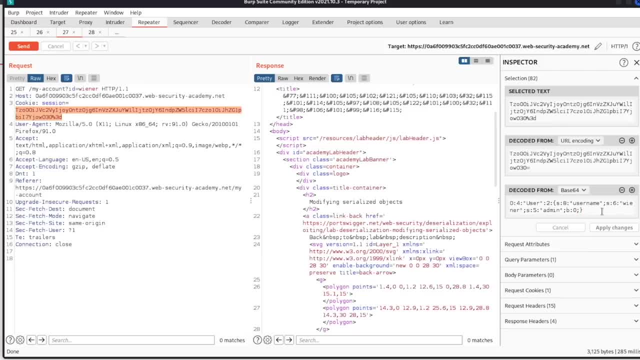 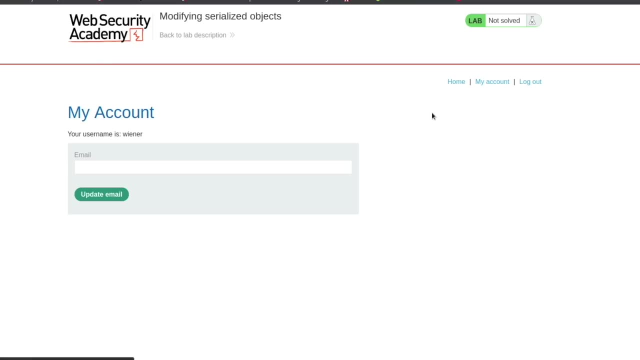 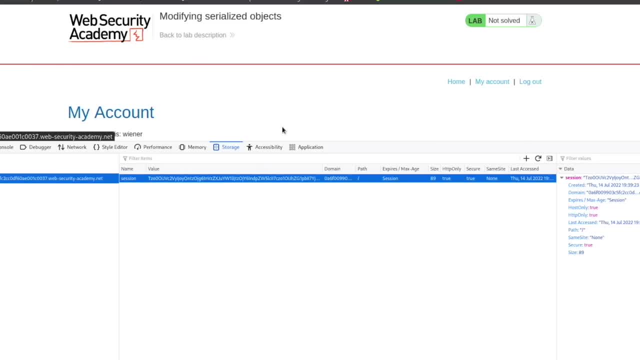 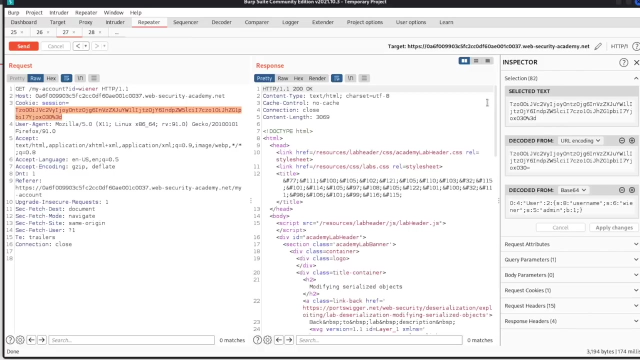 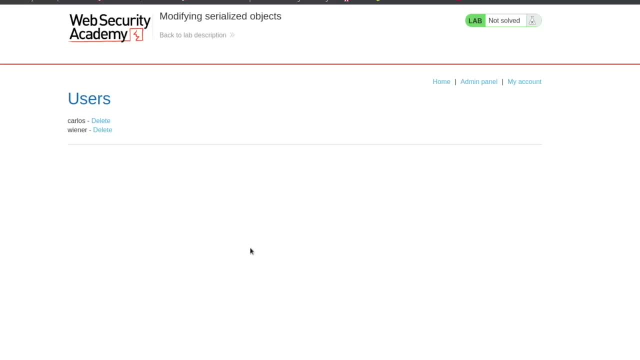 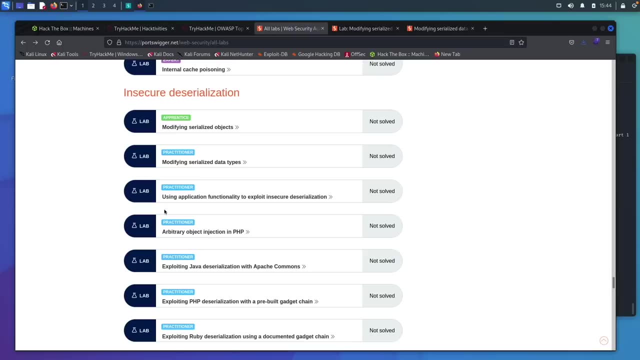 Okay, Okay, Okay, Okay, Okay, Okay, Okay, and hop over there and check that one out. All right, so we're going to go ahead and do this second one right here, and what you will need to do is- I just opened it up in a new tab and I also 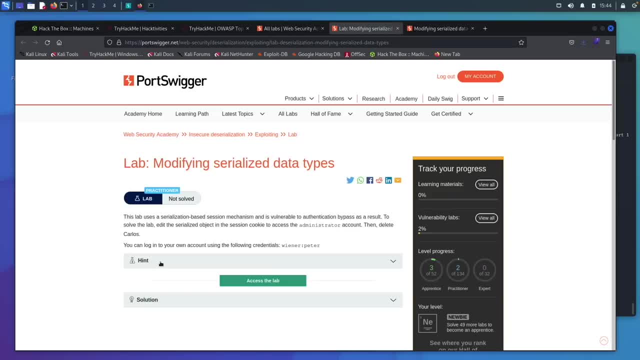 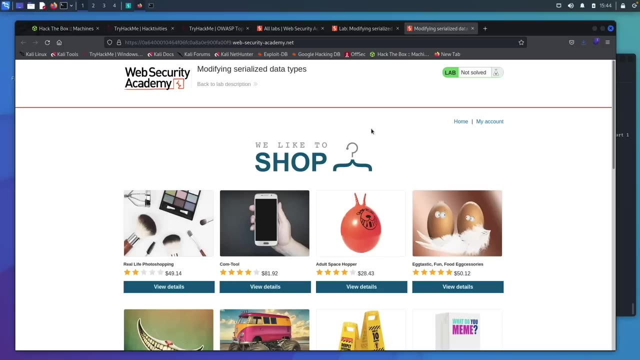 opened up the labs. that way we don't have to wait for that to load. So we'll read the instructions and it tells us we're going to need to gain access to the administrator account and delete Carlos once again, and we have the same username and password. so if we come over here, we're going to 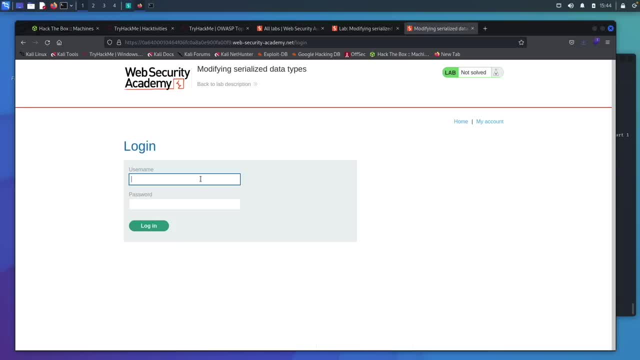 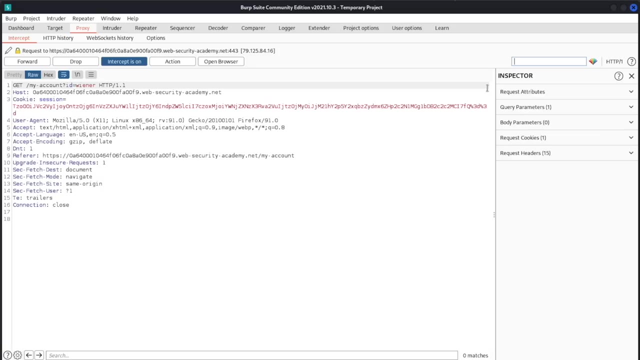 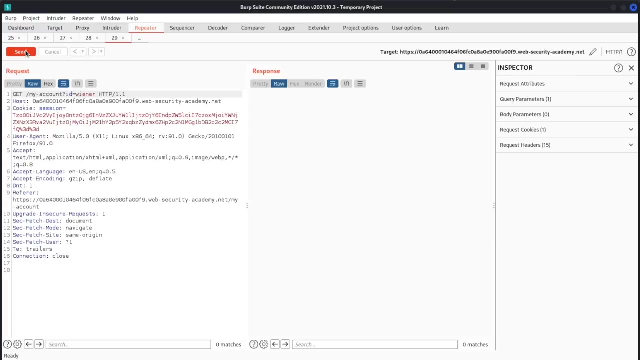 do the same thing we did before and we will log in just like before, and now that this is logged us in, we'll come to our proxy. we're going to intercept the request. check out the my account page. send the to repeater. come over here, send it, see what happens. we get a 200, okay, and now we're going. 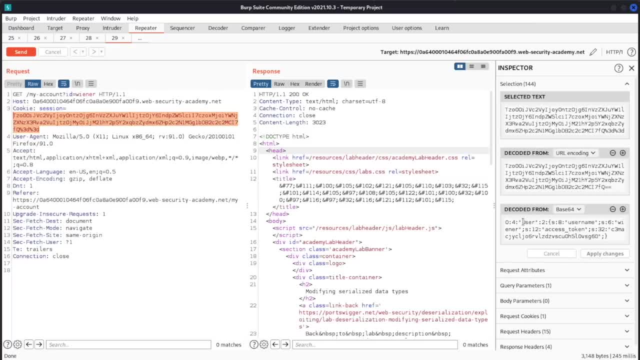 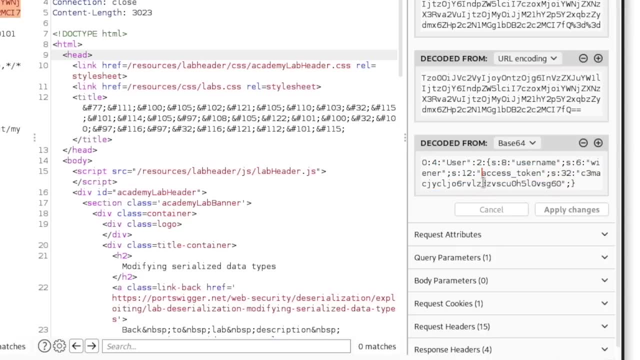 to mess with this cookie once again, and you can see there's. it looks like there is a lot more going on in here than last time, but you can break it down just like before. we have our object and then we have a string with our username right here. we have the username and then it. 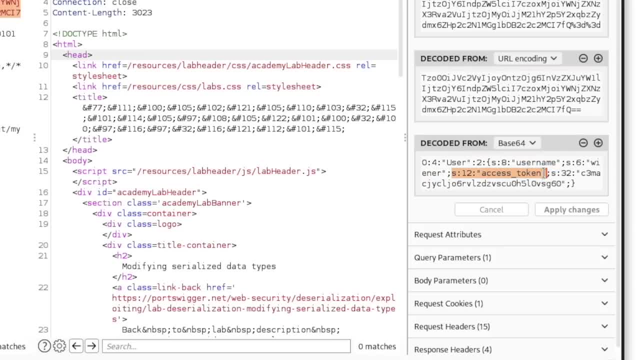 tells us we have this string right here with our access token in it, and then we have this going on right here. so what we would need to do with this at this point is this access token is obviously going to be bad for us because it is going to be telling us what we can. 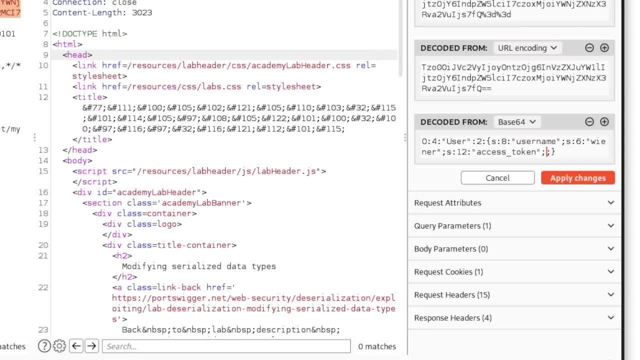 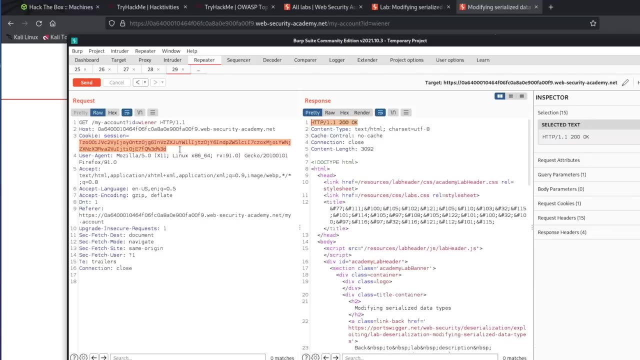 access what we can't access. so if we just delete that and then we just put in here the b1 to make this true, we can apply the changes. we can actually send this to make sure we don't get an error and it says 200 okay, which means this token should work for us right here, and so we can. 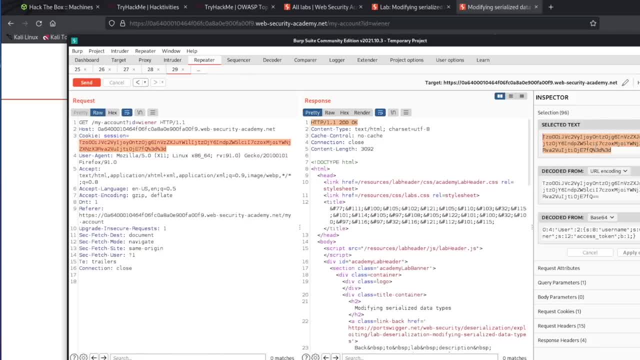 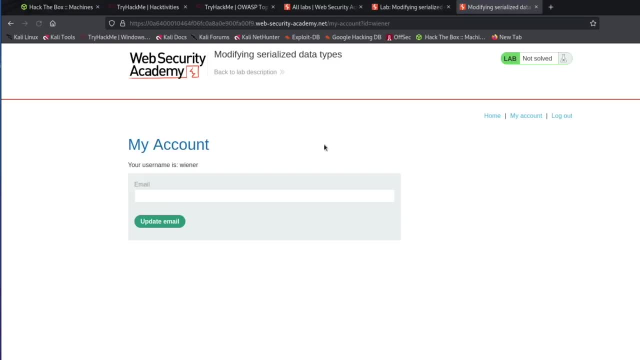 i'm going to copy it out of the box just to make sure i don't get anything wrong. and now what we'll need to do is come back to our page. if we refresh this, nothing happens. even though we sent it from burp, we'll have to inspect and check out the cookie over here. 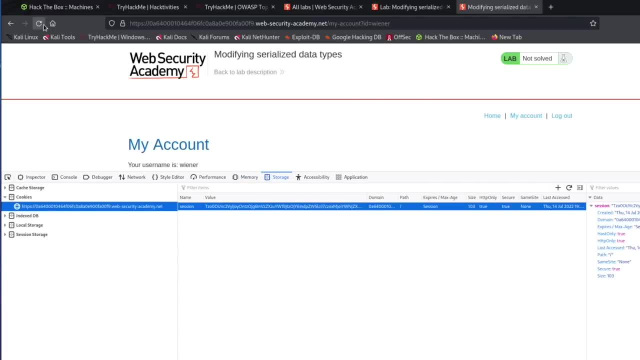 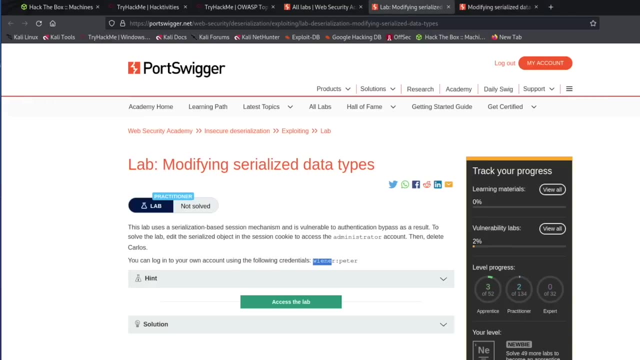 change our cookie and then refresh the page and we have the admin panel. so this looks really easy. but this one actually took me, like i would say, almost 15 minutes to 50 minutes to get figure out what exactly was going on inside of repeater. I am not a super great, I'm not real. 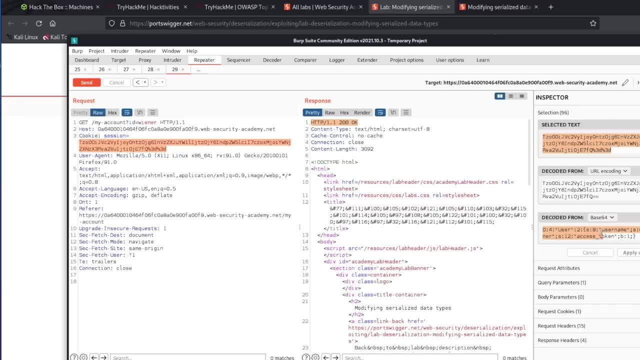 great with PHP, And so when I was trying to figure this out, I finally got this to go. I accidentally left this in a string the first time, which is something you may have done, And if you try and leave this inside of a string, it is going to give you this error over and over and over again. 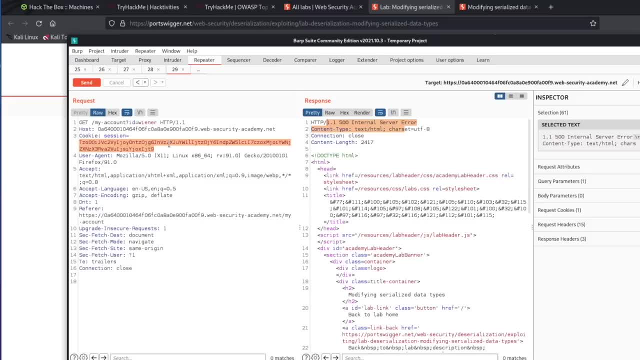 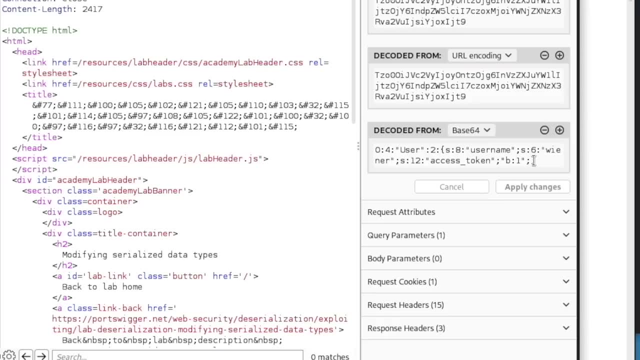 And that's one mistake that I made over and over as I was messing with this. And then the other mistake I made was I was able, I deleted this and apply changes, And if you send it you'll get the same error, And I forgot to delete this. So this is really finicky. 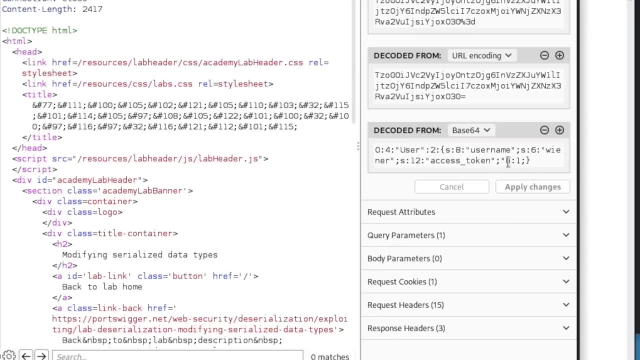 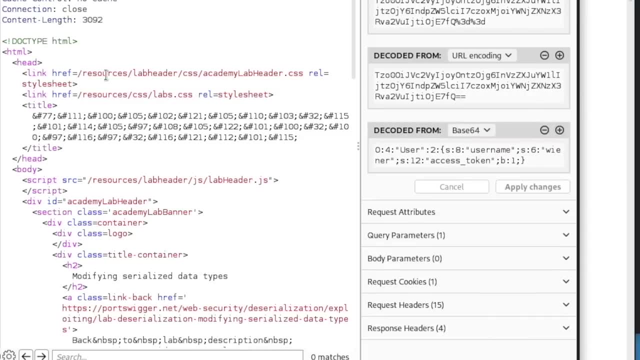 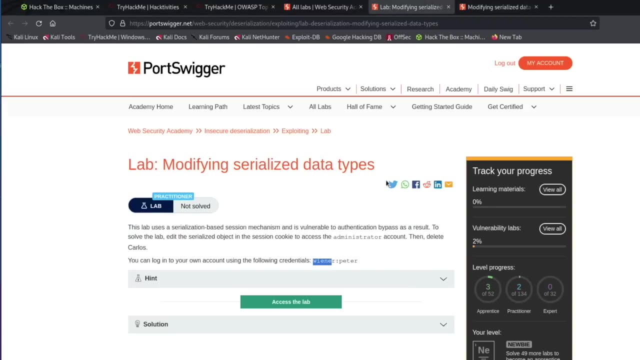 And in the real world you're going to have to do pretty much what I did and just keep testing this over and over and over until you get a 200. And then you'll know that something has worked And one of the other things that I didn't understand and I don't understand still. So if 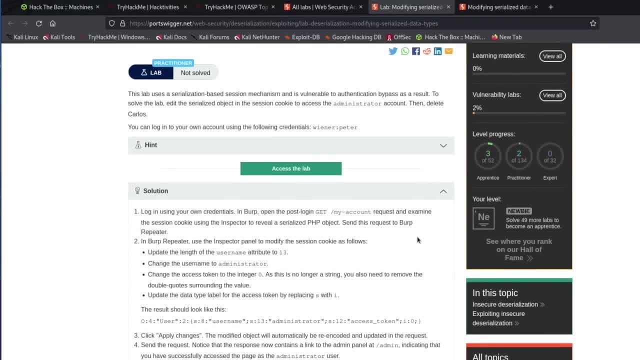 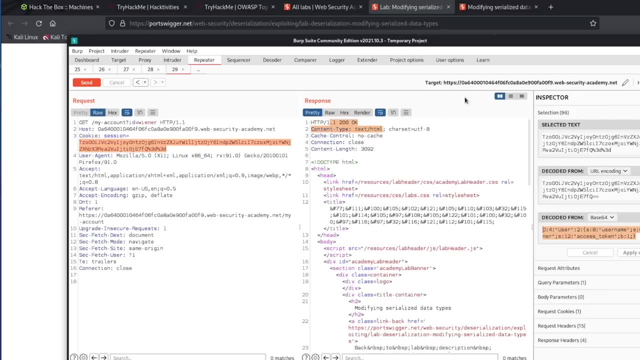 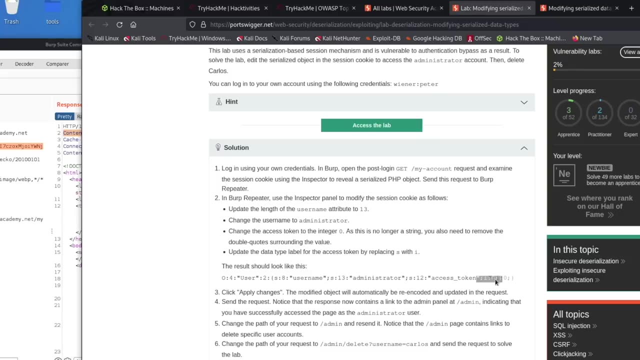 you know PHP, you might understand this better than I do. I have no idea why this says we have an integer of zero in order to get this exploit to work. This is not how I solved it And I honestly don't have any idea why this access token is an I with a zero, but it does work And the way. 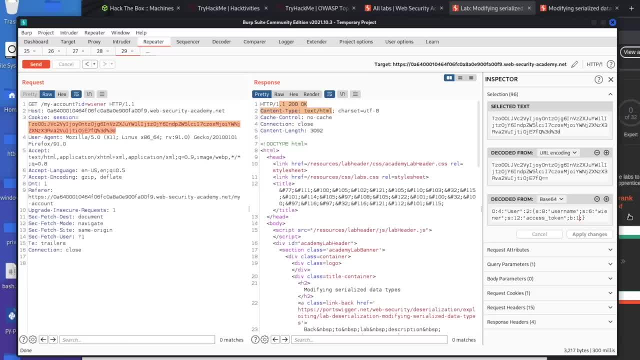 I solved it. I don't have any idea why this access token is an I with a zero, but it does work And the way I did it ended up working. So if you come over here and you change this to a zero with the boolean, 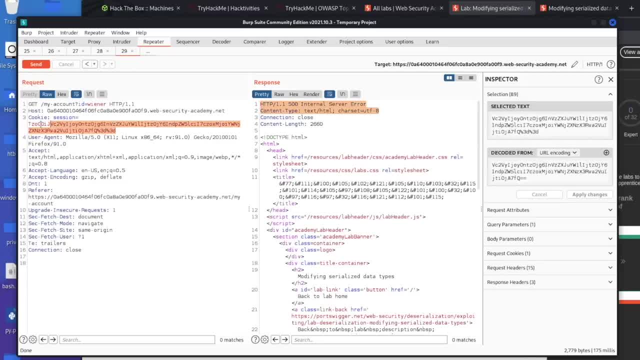 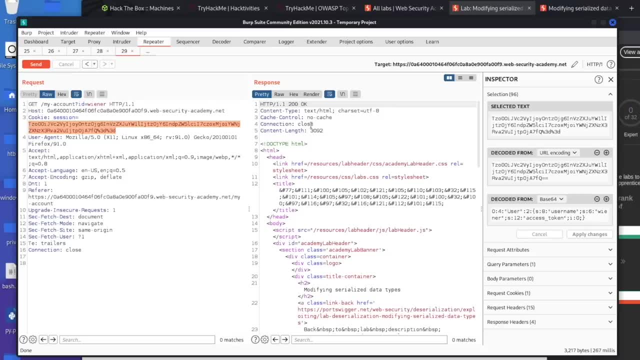 you are going to get this error And then, if you come in here and you solve it the way the solution says, with the integer of zero, apply the changes you can send it. it works this way as well, And this cookie works. But just being honest, I don't know why this works. My version makes sense to me. 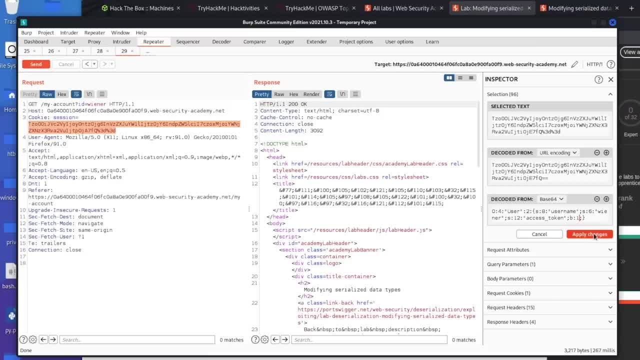 because I have the access token and I'm just going to send it. So I'm going to go ahead and I'm going to say that it's true that I have access to wherever I want to go and I send it and it works. So if you know why this works with an integer, you can feel free to leave a comment. 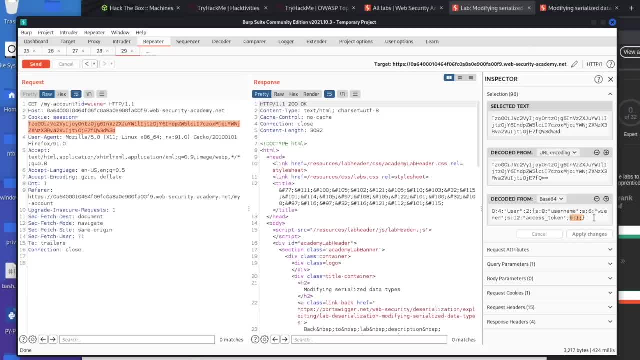 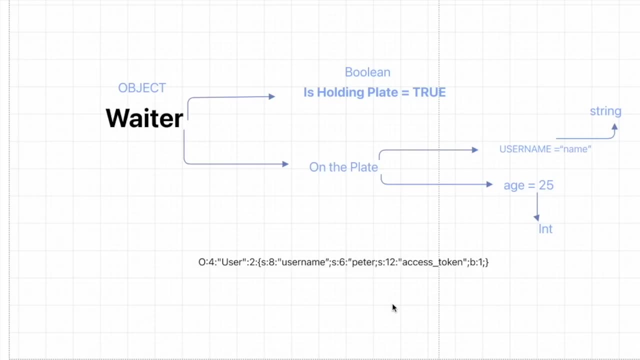 down below Because I'm really interested. I don't actually know. I actually Googled to try and figure out why this works with an integer And I couldn't find anything. So with that we will move into the next vulnerability and keep going. Okay, so now that we have looked at the 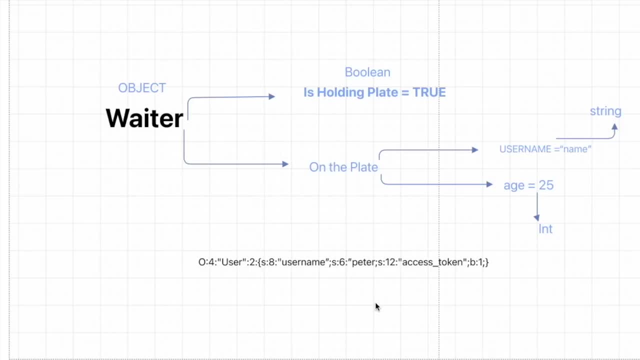 insecure deserialization examples. we're going to come back to the flowchart. So now, if you remember the object right here, so we have our object, which is the waiter, and it is carrying the plate, And on the plate we have a username, which is Peter, and we have the access token. 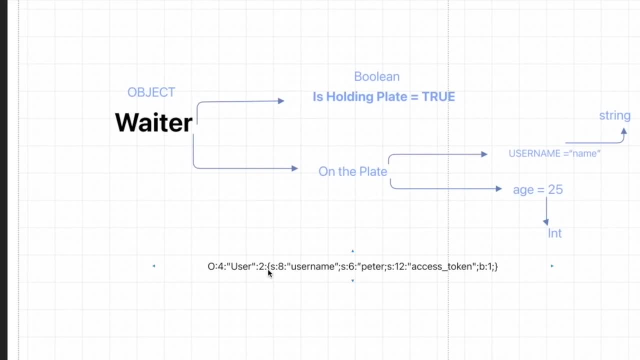 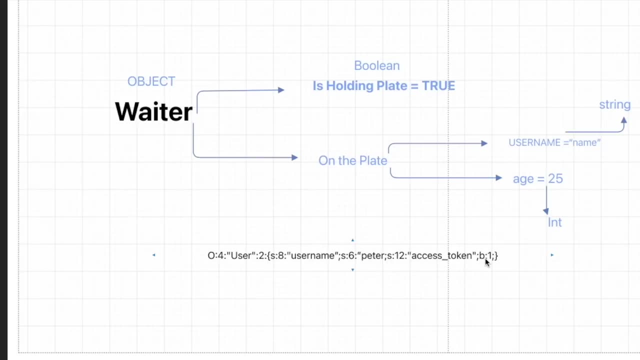 right here, And so we have a object, we have a string and another string right here And it says that this is also carrying a string, And then we have our Boolean, which is going to be true, which allows us to log in as the administrator. So now, when you see something like this, 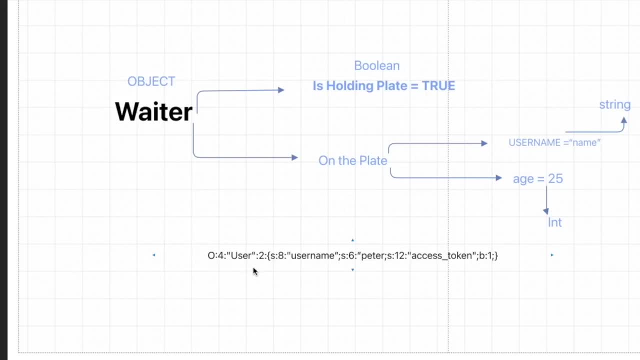 you should be able to understand what's going on at least, without it being really, really complicated. So here's the flowchart Once again. this is how the insecure deserialization works. I hope, going from the beginning of this flowchart to now, it all makes. 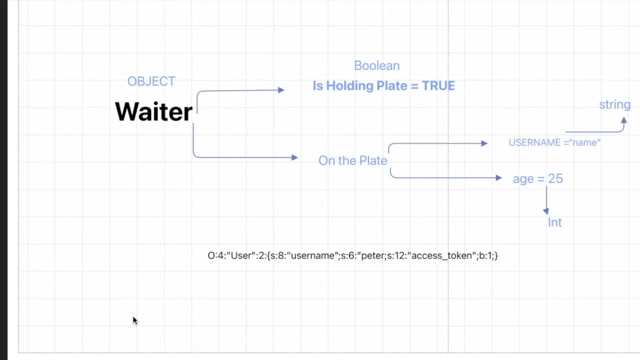 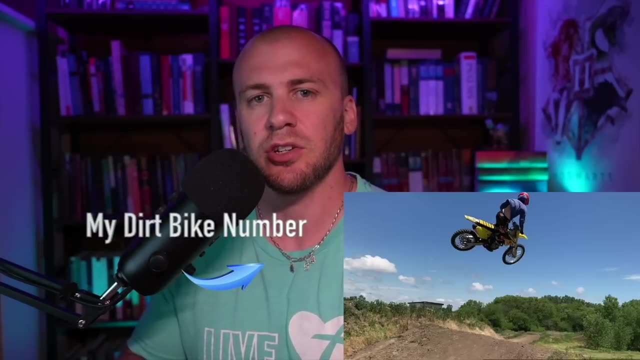 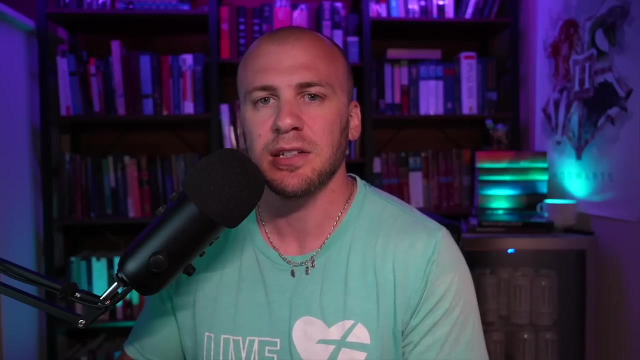 sense and you can understand what is going on. I'll see you in the next vulnerability. Okay, so as we move into this next section, we're going to be dealing with cookies and auth tokens, So I decided to go ahead and do the first half of the box, Luke on, hack the box. it's going to be. 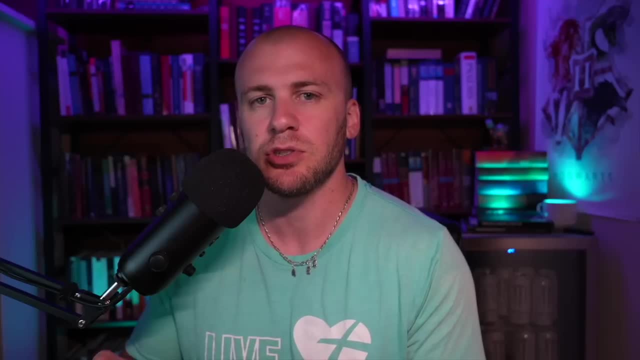 dealing with a JSON web token, And I decided to show you this because I wanted you to see walking through the process of finding a token and changing it and just how to understand what is going on. And then, after we look at this box, I'm going to set you loose on two labs. 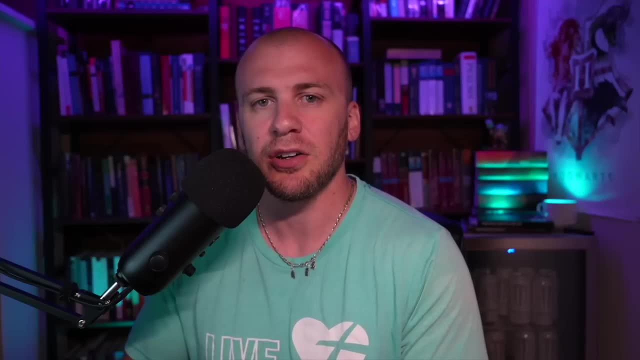 and you'll be able to practice manipulating these tokens on your own, And then we'll do walkthroughs with those as well. I thought it'd actually be helpful to go through the first half of the box, Luke, so that you could see a little bit of the enumeration, And I've had a few people. 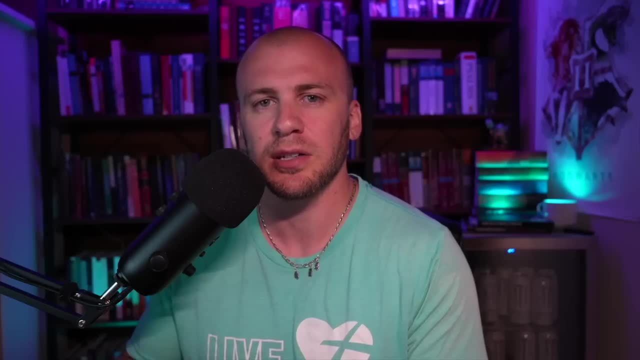 asking to do more with APIs And this box I'm going to be doing a little bit of a walkthrough of, So I'm going to go ahead and show you how to do it. So in this first half of the box, we'll 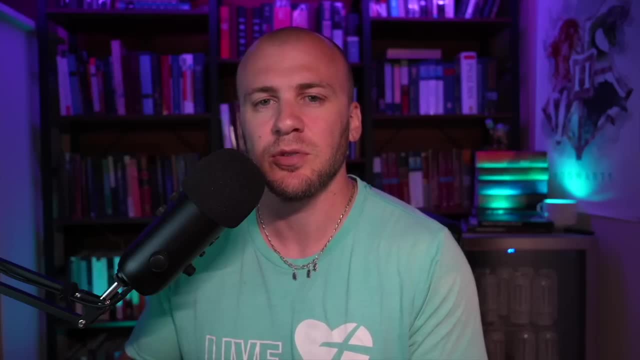 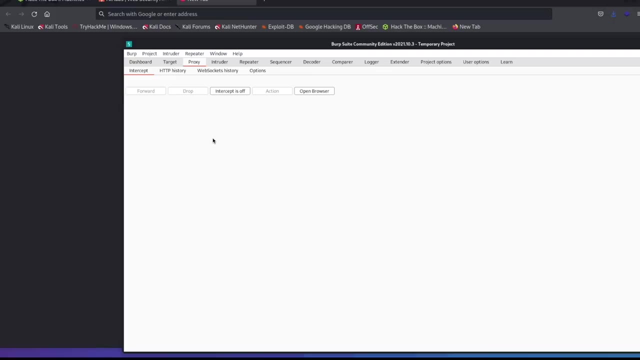 actually show you how you can communicate with an API. I'm going to show you with the actual command line, as well as enumerating an API with burp as well, And so we'll go ahead and jump into this. All right, I have already set up the box and I have it running, So we should be able to ping the. 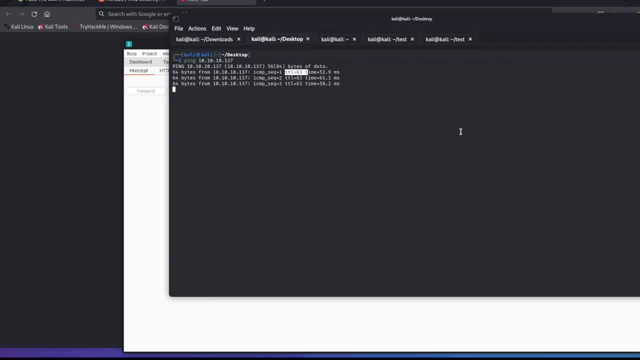 IP address is 137.. And we can see it's a Linux box right here And it is all up and running. and it is is all up and running and it is ready for some enumeration. we can run an in-map scan like this, and so we can go ahead and run this in-map scan and we can see port 80 comes back really quick. so 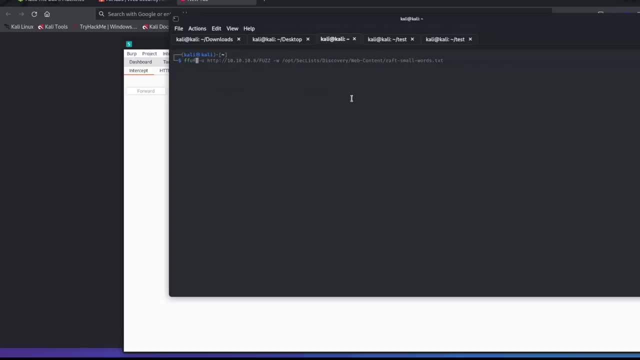 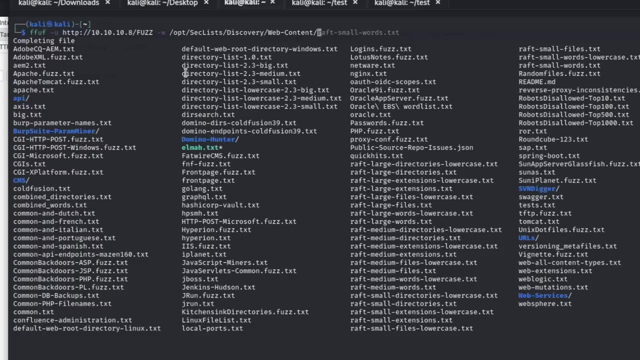 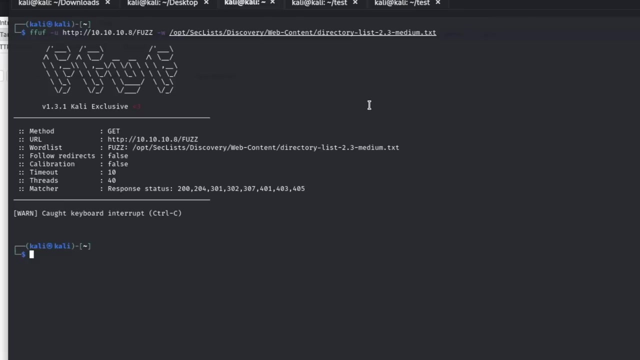 we can run a go buster or we can try and use fuf on this box and we will use a directory list. i imagine a small one would be just fine, but we'll use the medium one just to make sure we're able to find everything that we need. and i forgot to change the ip address here, so we'll fuzz this. 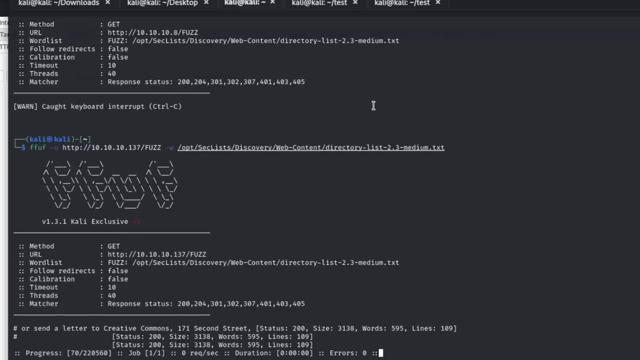 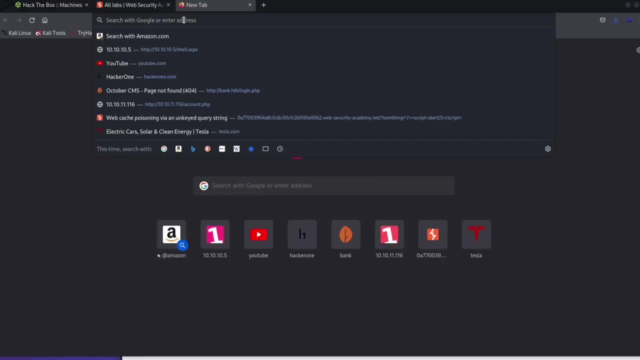 while our in-map scan runs. so we got 137 and we'll go ahead and send this on our way. we can actually come out to the ip address by typing in 10, 10, 10, 137, since we know port 80 is open. we can actually come out to the ip address by typing in 10, 10, 10, 137, since we know port 80 is. 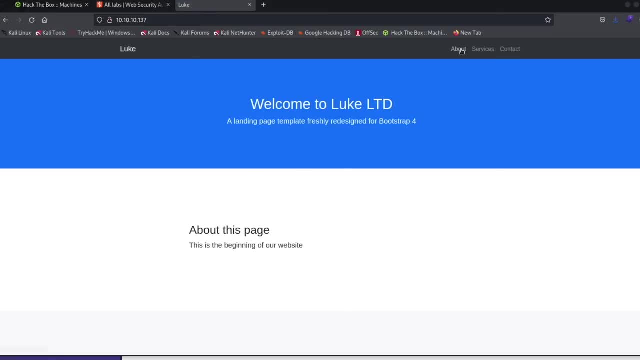 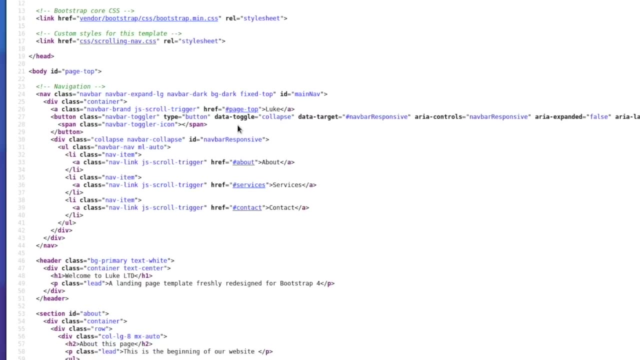 open and we are brought to a web page like this. we can click around, see what's going on. you guys know I like to view the page source. I like to look at a lot of the hrefs and see what's in here. I wonder if it has a login in here. nope, 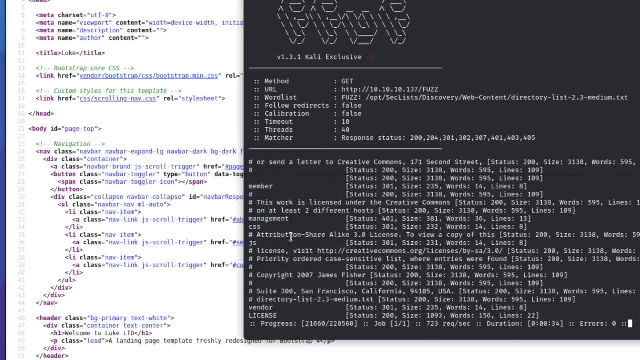 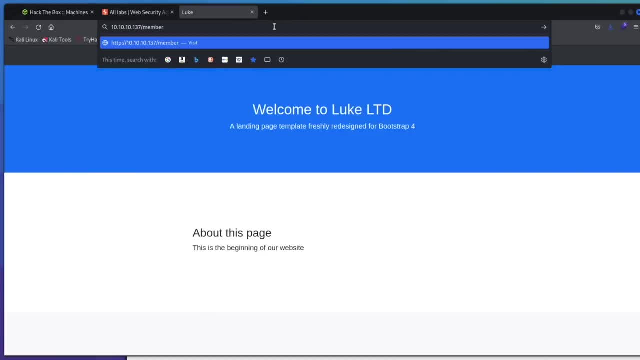 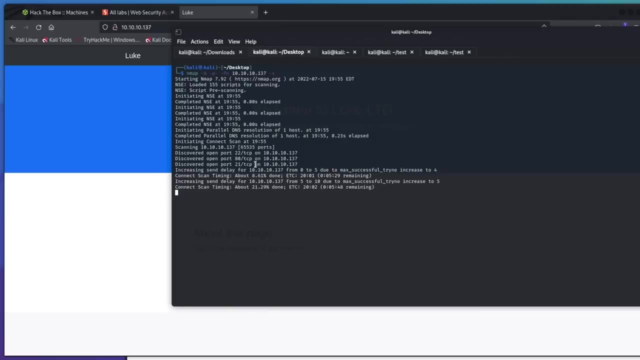 and we can come back and see if buff has found anything. we got member which was a redirect. we can check that out, see where it redirects to and it doesn't tell us anything and we can check. our in map scan is still going. we have port 21 if 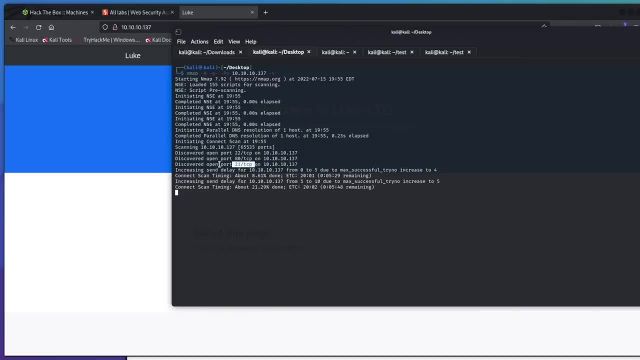 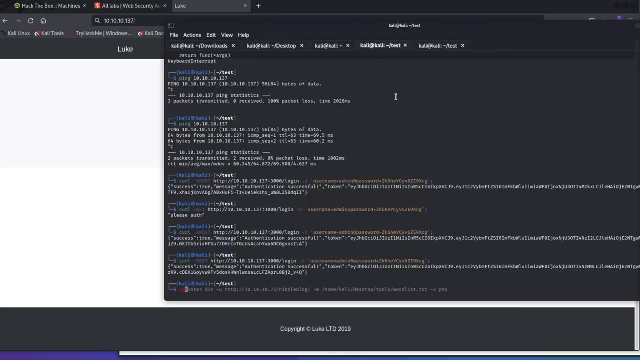 this was a penetration testing course. I would go out and check port 21 and FTP, but because it is not, I'm gonna let these scans run and I'll bring you back once they have finished, and it seemed to be taking longer than I anticipated. so what we're gonna do is we're gonna check out a go Buster, because I like to use go. 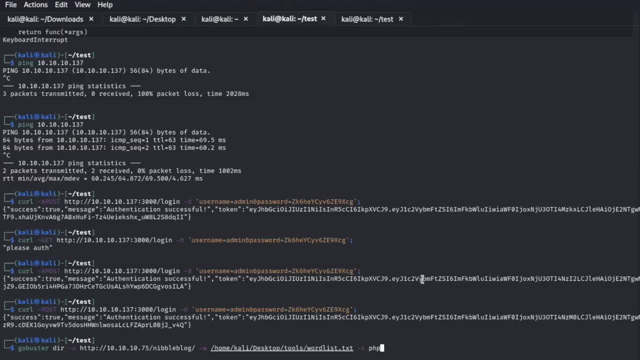 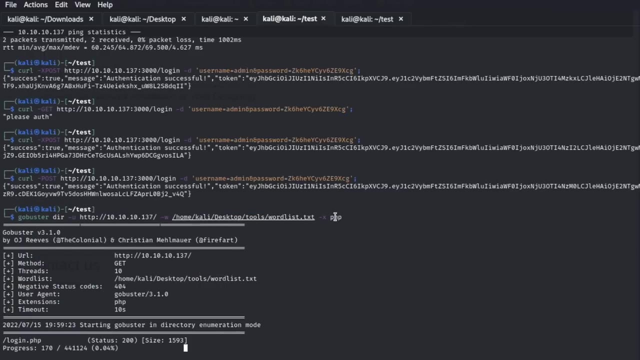 Buster for when I need to run an extension such as PHP, and fluff does not allow me to do this, so what we're going to do is come back over here and we're gonna run our go Buster with, as well as fluff with the extension PHP, because this isn't this. 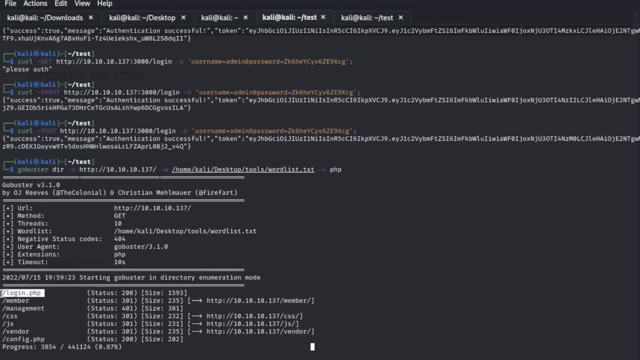 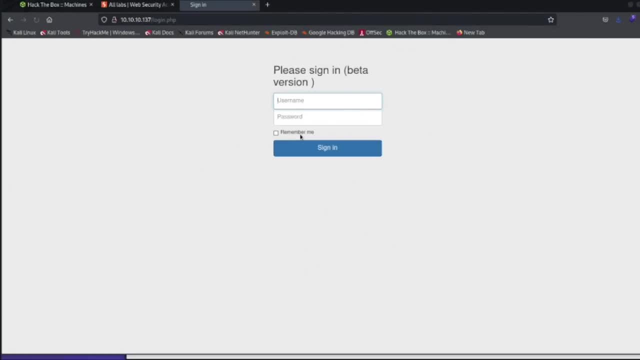 wasn't working for us and we have a bunch of stuff coming back so we can check out the login page. this usually is not gonna work in a bug bounty program, but you can type in something like admin and it doesn't work, and so you can try default credentials and see if it works. 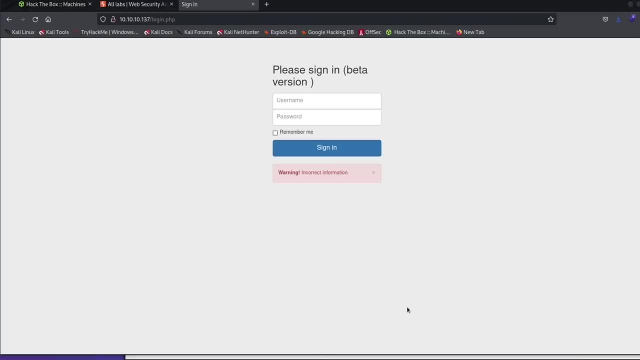 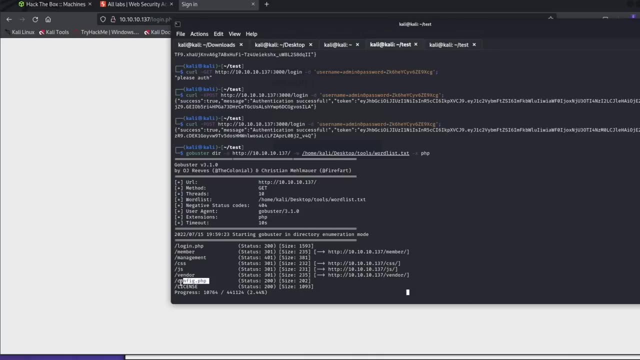 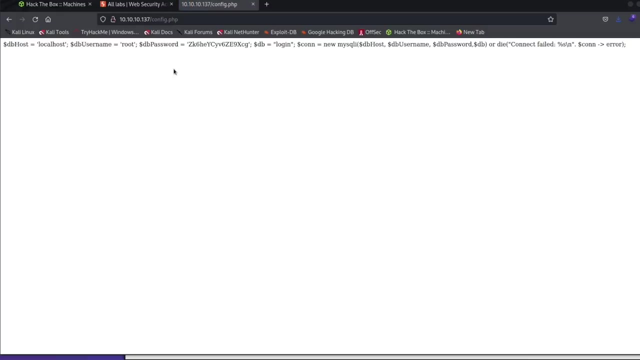 usually there will be like a made by down here, but there doesn't seem to be, so we can't check for any default credentials on this page. we have a config PHP, which is always a good thing to look at, especially when you have code execution on a box, because it will pull down often the username to the database. 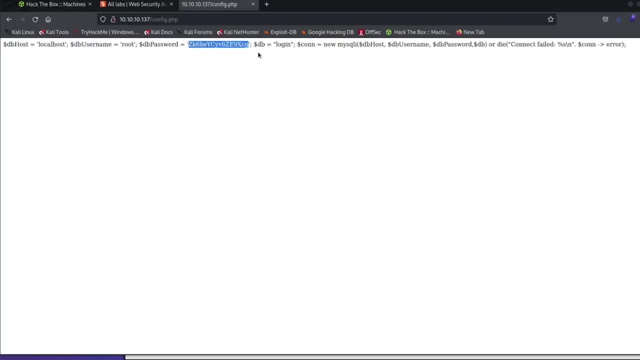 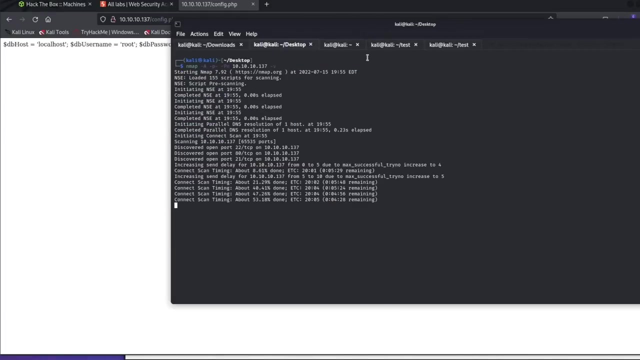 which is root, and we have a password as well, and one thing you should know by now, especially if you're in an intermediate course, is that people reuse their passwords. so we can copy this password and we'll check our in map scan and it has not told us, but it will tell us when it is done that there 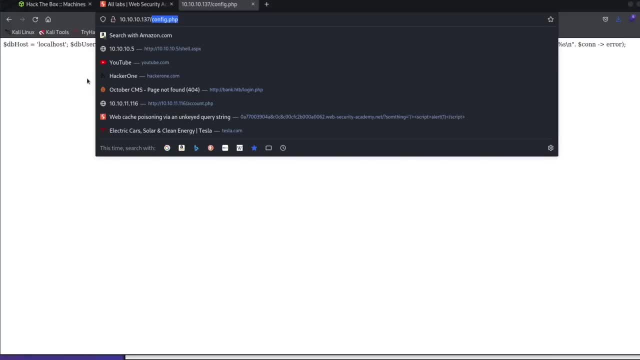 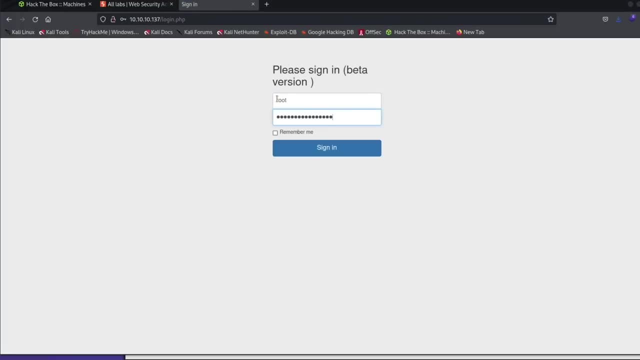 is a port 3000. but before that you could come back to this login page right here and try and login with root and that password we just copied to see if it would work. and it doesn't, you can and we could try admin with that password to see if it works and it doesn't. 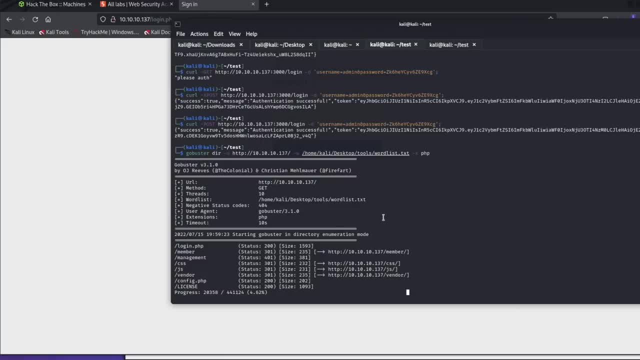 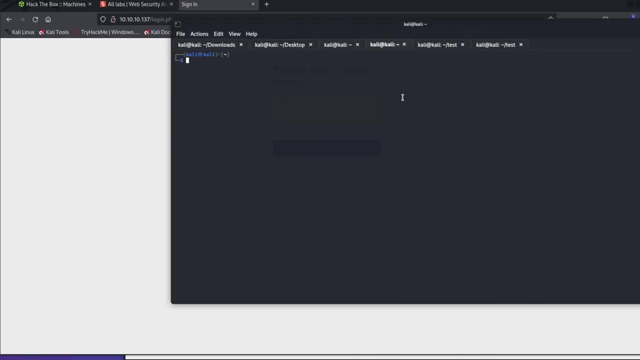 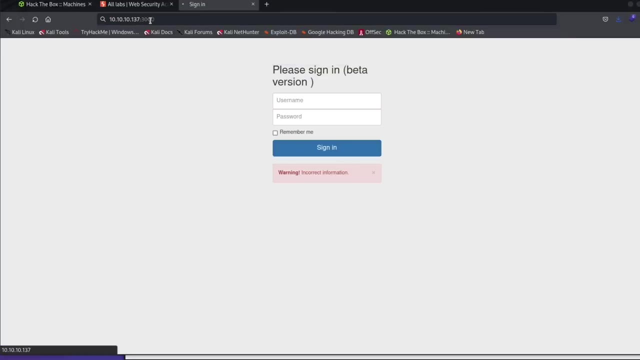 you can also try administrator or other things like that, but we're going to go ahead and open a new tab and at this point we are going, and before we mess with this new tab, let's go and check port 3000 and we find that this has a, that we are getting back jason and this. 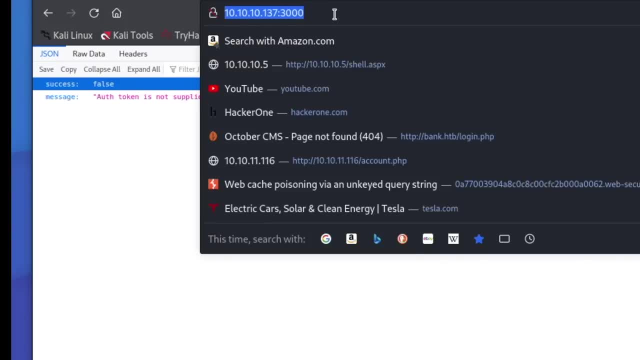 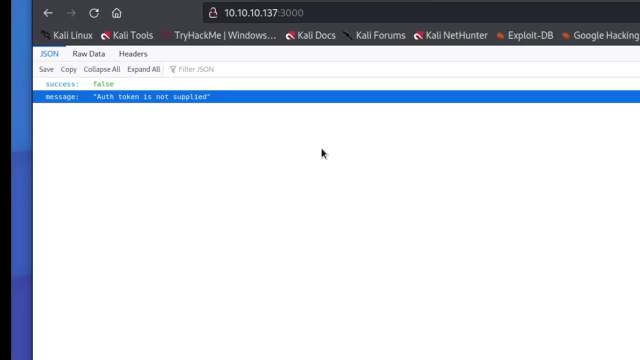 is an API, so we are going to see what we can figure out. it says an auth token is not supplied and we can curl this and see what happens and see if we can log in, because that is how we're gonna have this auth token so we can come over here. 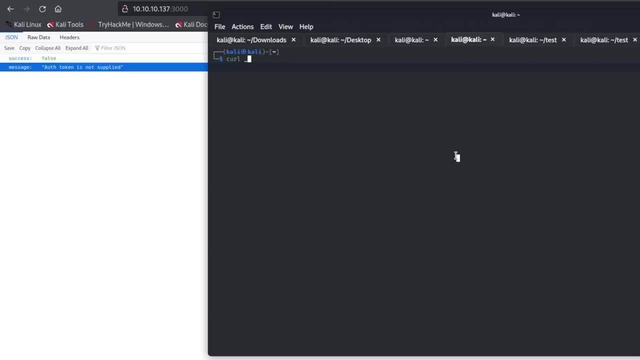 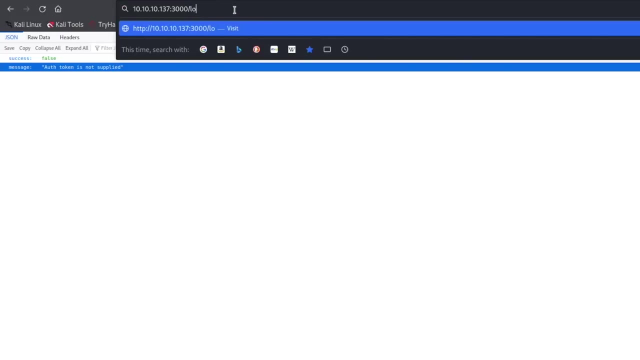 and type in curl and we're going to use a post and then we will go HTTP and the IP address 10, 10, 10, 1, 37, and we're on port 3000 and we want to log in and I can show you this right here: if we go slash login and the way you would find, 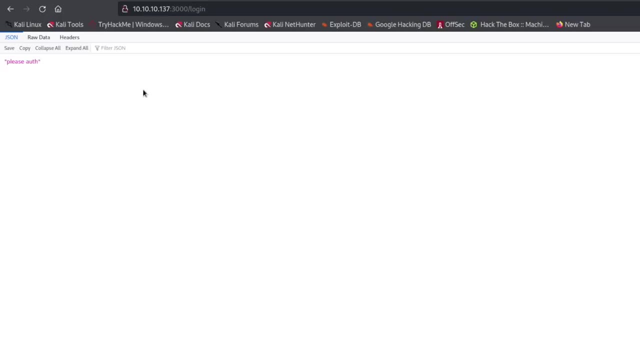 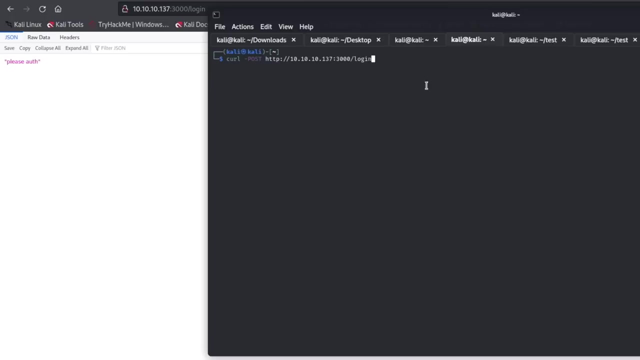 this login page is by fuzzing the API which I showed in the beginner bug bounty course. so we know that we need to authenticate because that's what it tells us and we need this login page right here and we need to pass in some parameters, which is going to be our username. so we'll go username and we 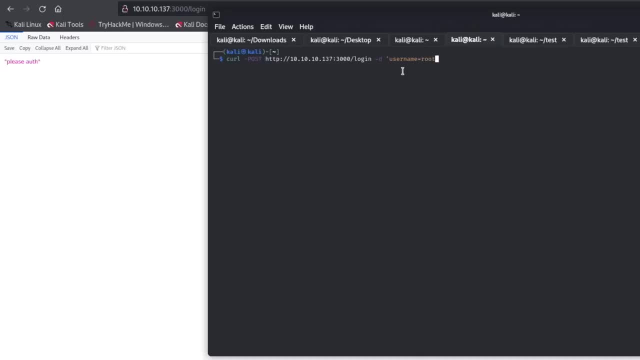 were told the username route. we can try this, because that's what we saw on the configPHP and we'll need a password as well, and we can try the password that we found, and then we can close all this off and send it, and it tells us: 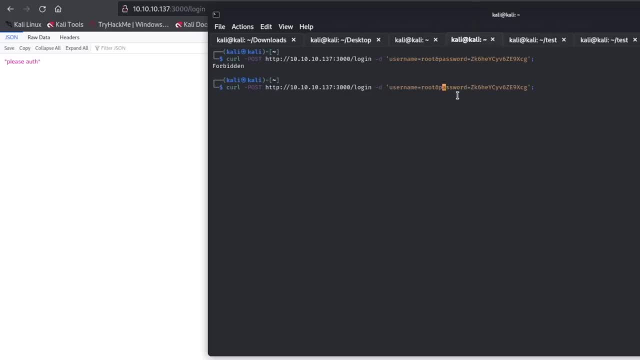 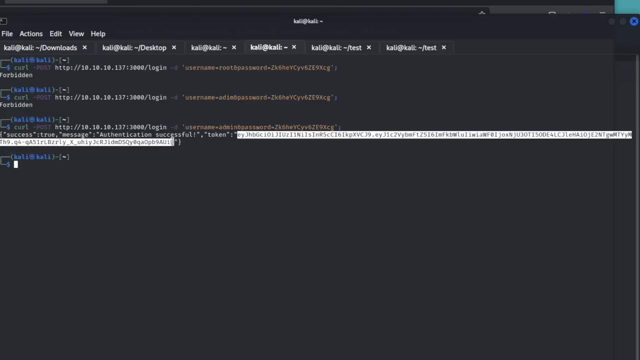 forbidden. it does not work. we're not able to curl it, so you could come over here and try admin, like we tried before, and I spelled admin wrong, and we get a token in return, which is what we needed. so now what I would do is come back here. 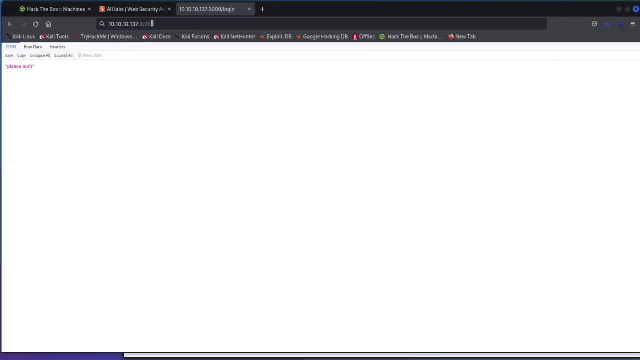 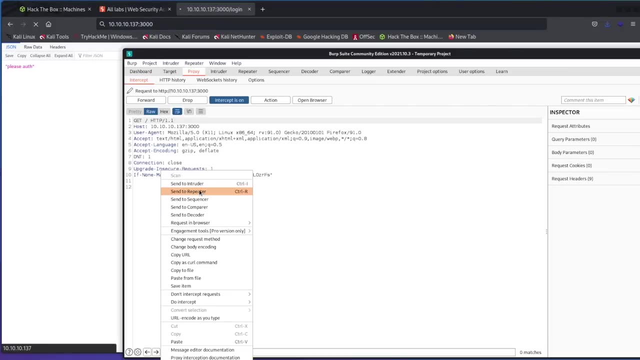 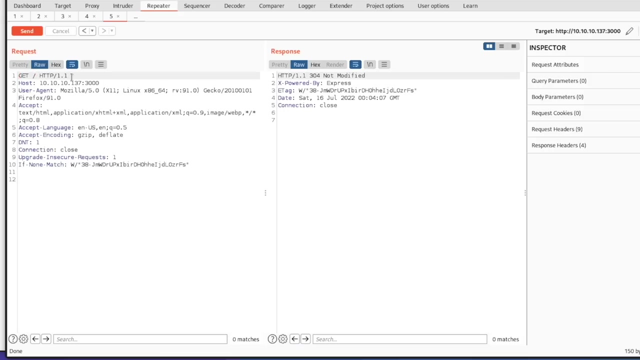 like this: we're gonna go to burp and we're gonna intercept this request. we'll send this to repeater and we can let that go. if we send this, it tells us let's try login and send this ok, and we get an ok back and it tells us we need. 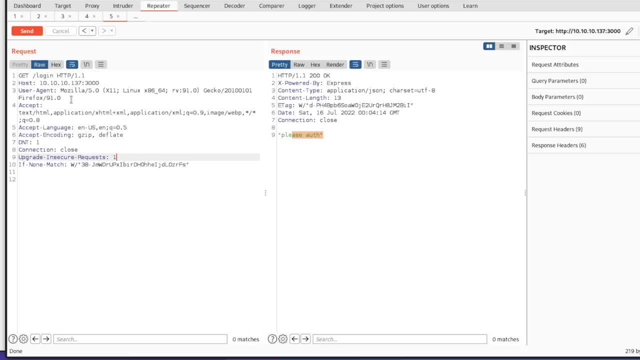 to authenticate. now what we need to do is create a token, and so we'll need an authorization token so we can go authorization, and then we could go back and we could go to one of the options here. if I click, we'll use a bearer and then we're going to paste in our token right here and you can, nice, and 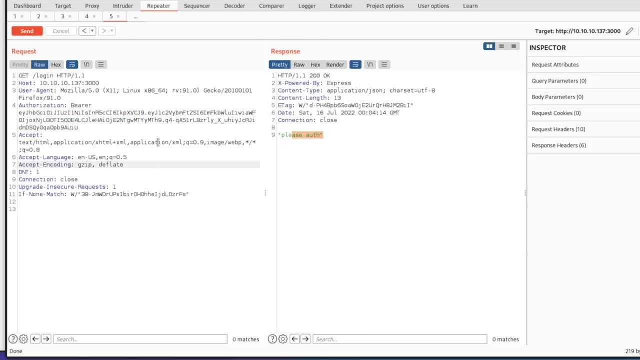 easily highlight to see what's going on here. So, because this is a JSON token, we have this right here and this is going to decode this for us over here in our inspector and if yours is closed, you can open it up and we can see that this is just telling it. it's a token, looks like it's SHA-256. 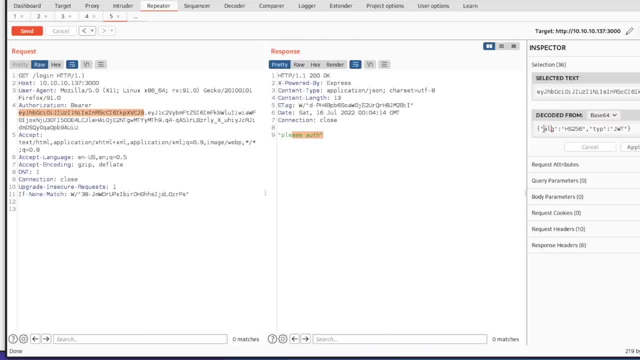 and this is the algorithm for it, so you'll see this again later. and so this is about the token, and then this second part is going to hold the information inside the token. We have the username admin. I think this is when it was created. I think this is the time that it would expire. 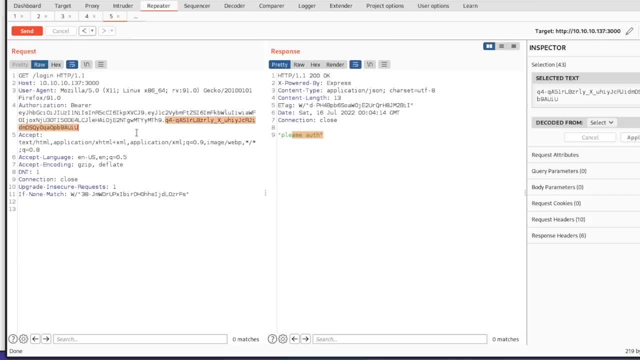 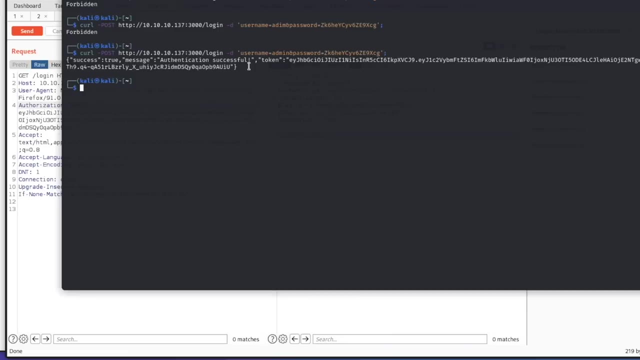 and this right here would be the signing token, would be the signing key, And now we should be able to manipulate this. we'll send it and it says we need to authenticate. so what we can do is come back to our terminal and it says we have this token right here on. 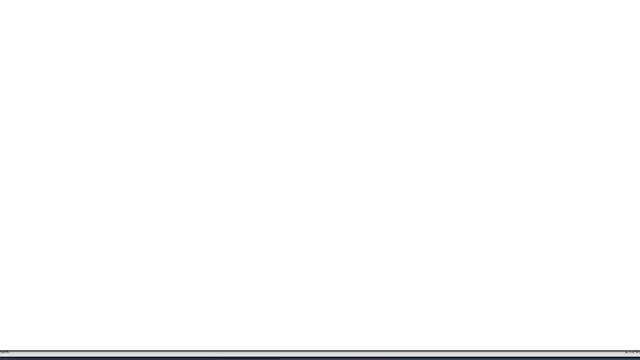 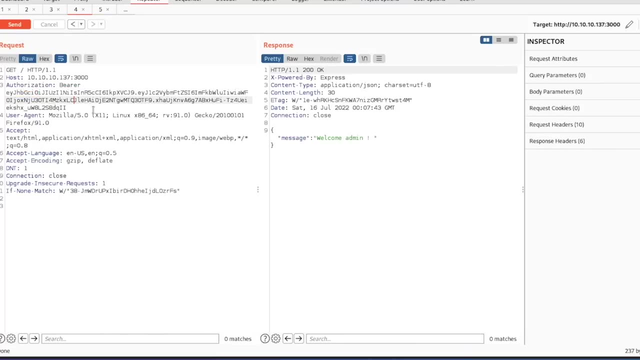 the login page. so go back to burp. we have the login, we have the bearer and I had to mess with my authorization here to get this to go through. we now have our JSON key right here and we're going to go ahead and paste this in our inspector and we're going to 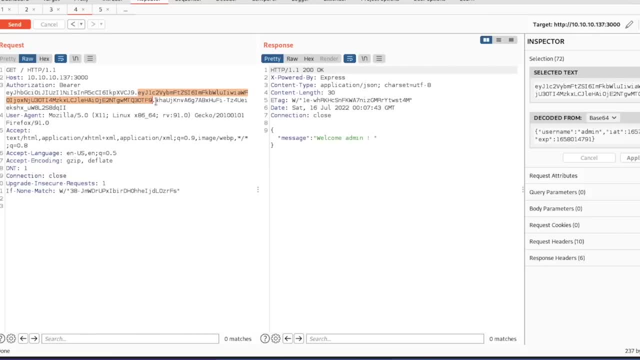 go ahead and paste this in our inspector, and we're going to go ahead and paste this in our inspector here with our username and our shared key right here. so now that we have this, we should be able to, now that we have this, we should be able to start enumerating the endpoints of the API and 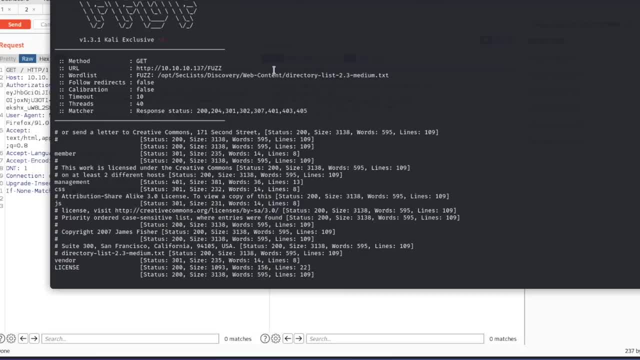 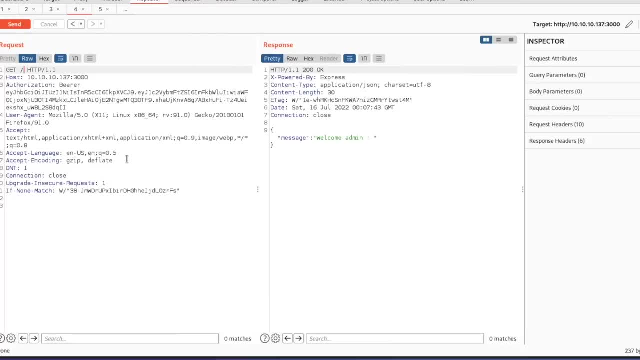 we can check out and if you remember, over here, where did we run that? over here we have all these different things and, as we enumerate these endpoints, one of the first places we should check is the endpoint something like users and we can send this and it says: we get the users back on the box. 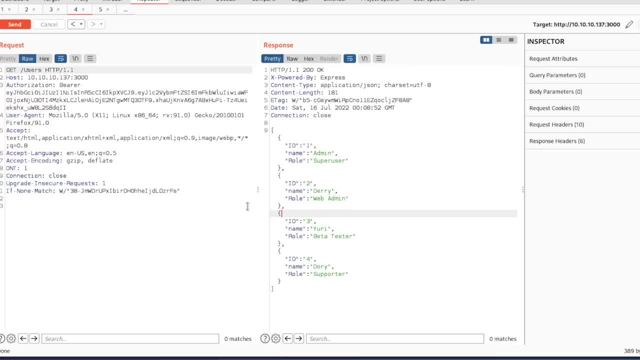 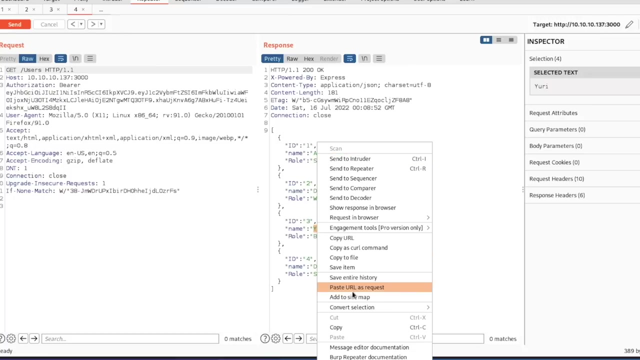 and because we have this right here and because we now have control over what is going on, we can go users and then we could try and see if maybe there is an endpoint with this person. so we can copy this, paste it in, send it and we now have a password for this user and we can also go back and maybe see if this person has a password. we can copy it. 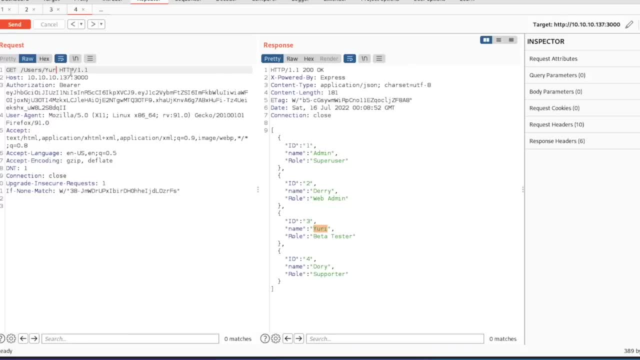 guess we don't really need to copy it. I could just type it out and send it, and we have their password as well, and with these usernames you could go out and try and log in to the actual web page and see if you can figure out what the 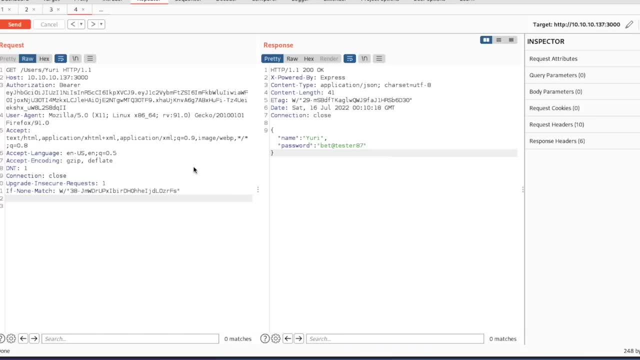 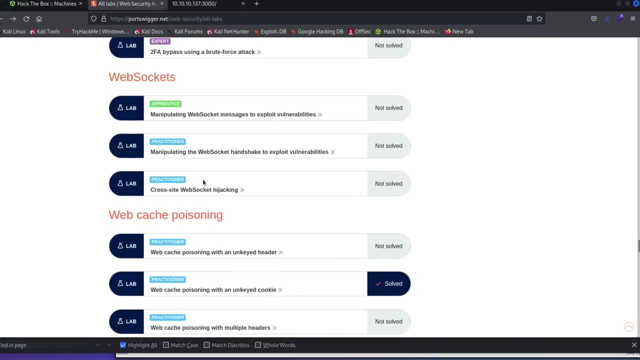 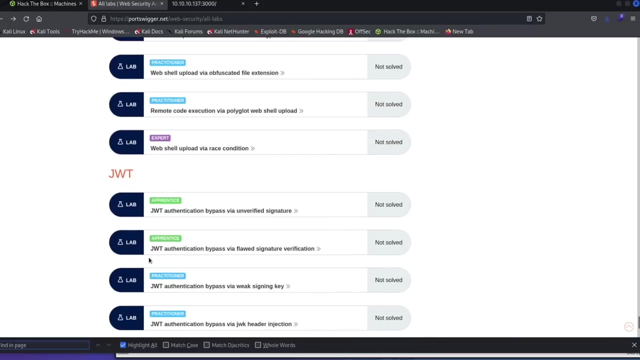 here to get remote code execution, but this is the direction of the box now. we're not actually trying to get remote code execution. what I wanted to show you was these off tokens and what you can do with them. so now we're going to come over here to our port swigger application here, where we have the free labs to practice, and we're going to go all the way to the bottom, because that's where these are located, and I think with what I just showed you, you should be able to solve this. 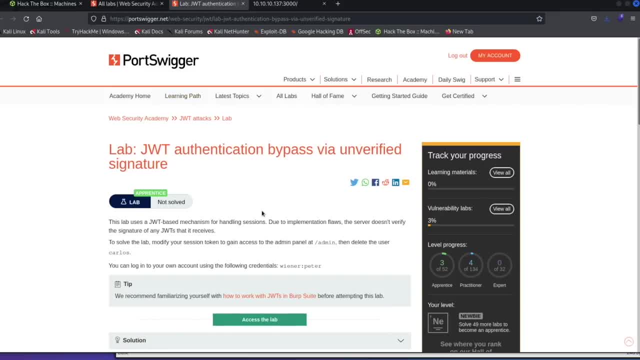 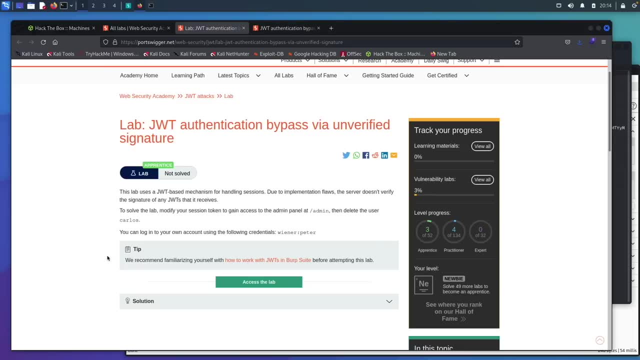 first lab, all on your own. so if you'd like to go and give this a try, then you can do that, and if not, we'll go ahead and walk through it. all right, so let's go ahead and read what we are supposed to do. it tells us: this lab is a json web token based mechanism for handling sessions due to. 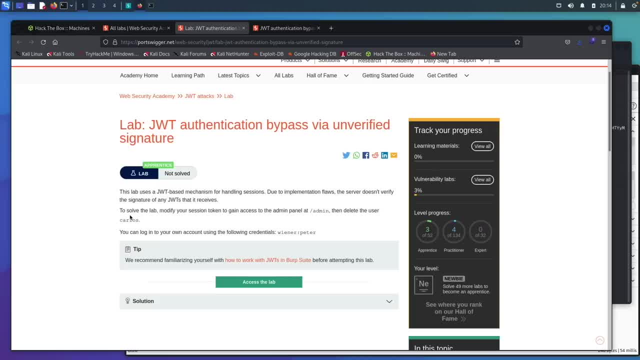 implementation flaws. the server doesn't verify the signature of any of the tokens that it receives. to solve the problem, we need to gain access to the admin panel located right here, then delete the user carlos. so i've gone ahead and clicked access the lab. we can come open this up. we are. 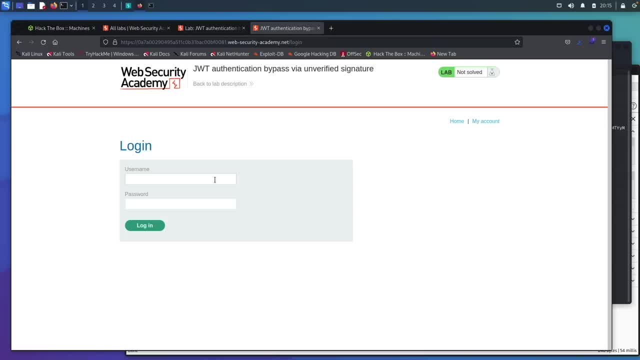 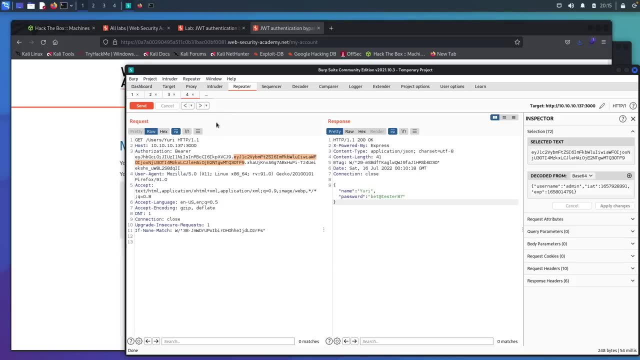 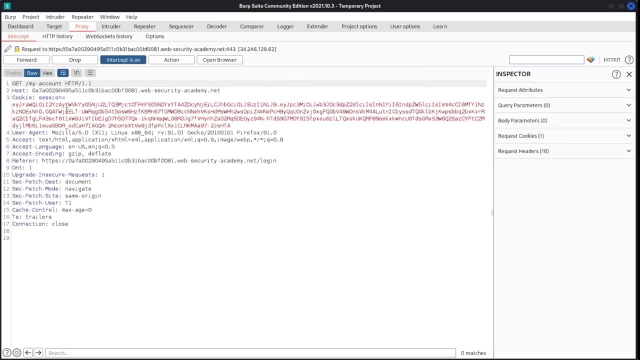 told we have the good old same username that we have been using and we can log in. we'll log in just like normal. we can come over to burp and we will grab the proxy and we can refresh this page and we see our cookie session right here. we'll send this over to. 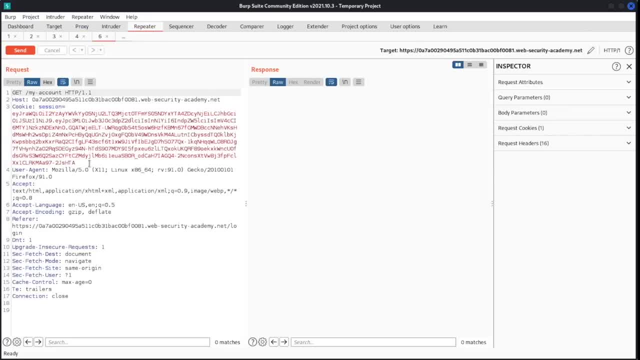 repeater, we can turn that off. and now we can look at this token. right here we have this. right here we have the decoded portion of the cookie, and then we can check this out and it tells us, right here: it was issued by a port- swigger- and we are signed in as this user. 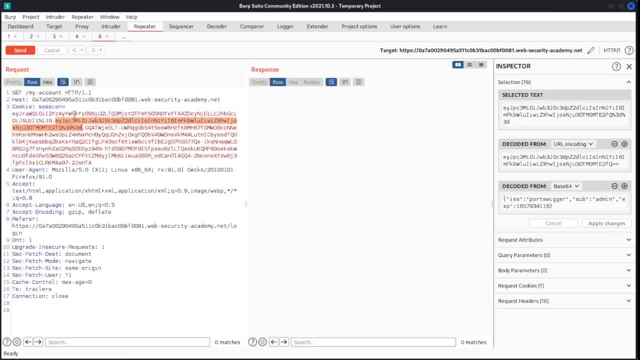 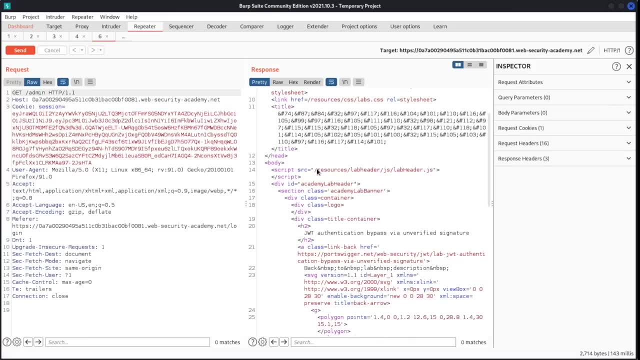 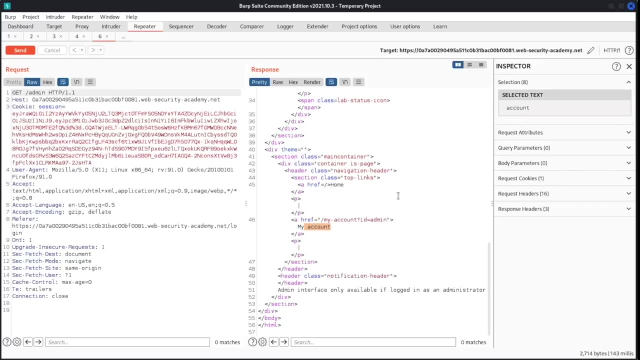 so we'll change this to admin. we can apply changes. and now let's check out the see if we can go to the admin panel and it says let's see my account. so it looks like we are able to go to the my account admin. so actually, let's copy. 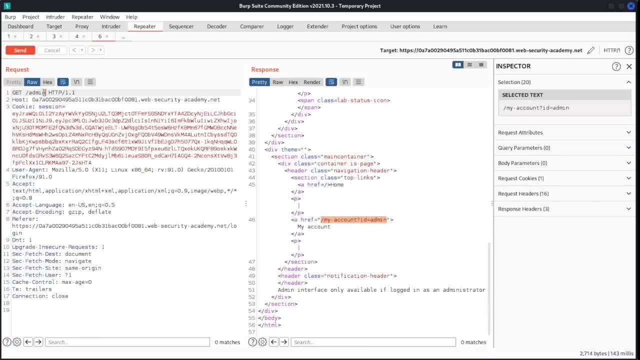 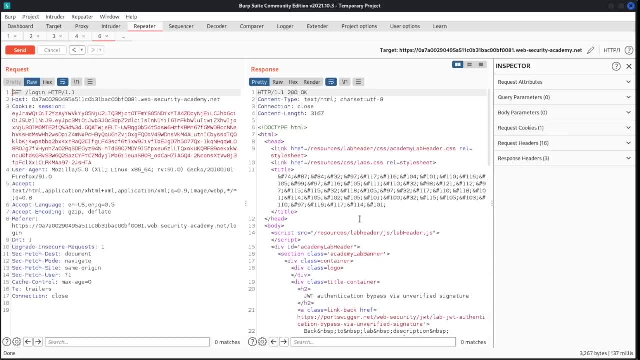 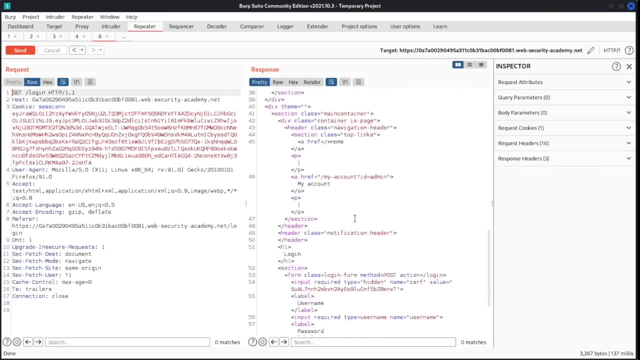 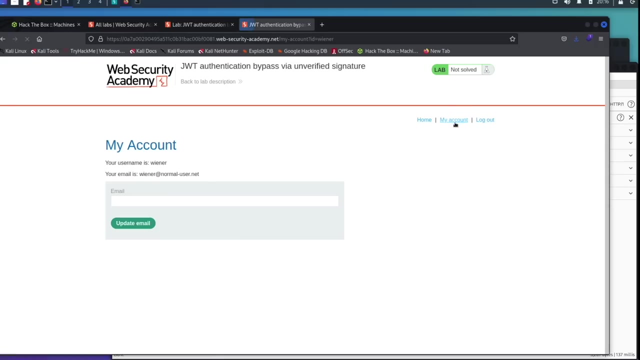 this: paste it in right here. delete that. send it. not found. follow the redirect. where does it send us to? it tells us we need to log in. so that did not work. let's try it again. let's go. my account tells us we are still logged in, so let's grab. 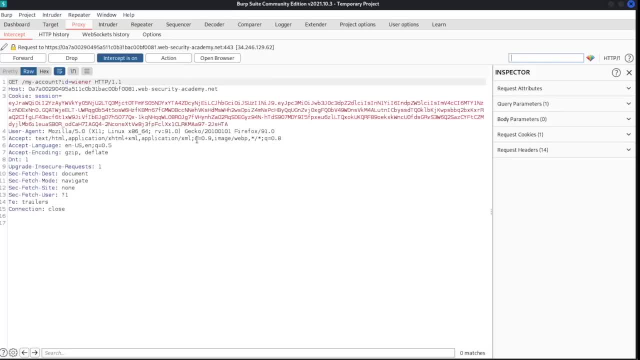 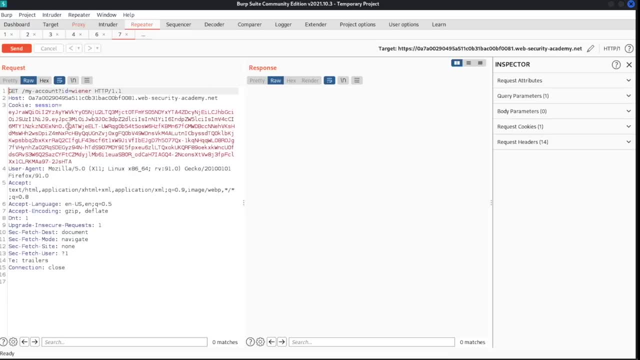 this again right here. we're told that we need to go to the slash admin in the instructions, so we'll come back to this see what we can do with this token we needed- was it admin or maybe it was administrator? like this, we can go to the administrator, sign is and sign it. we'll try and sign in as the. 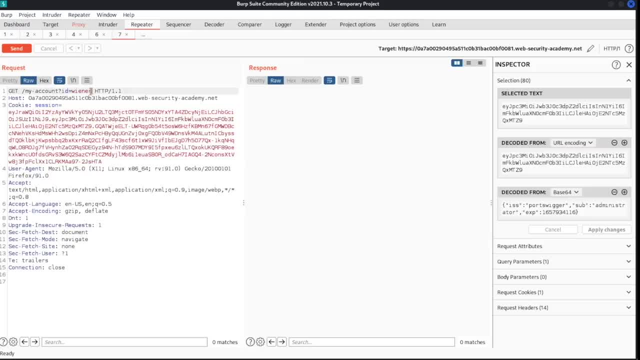 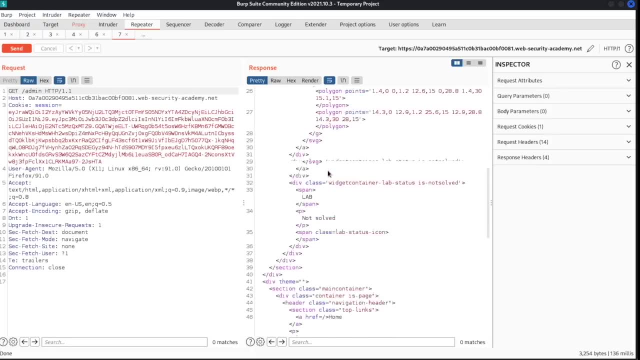 administrator apply changes. we can go to the administrator sign in. we'll try and sign in as the administrator apply changes. and now we need to go to the admin directory and this already looks different. we have the users right here, so if we wanted to delete the user, we could just copy this right here. 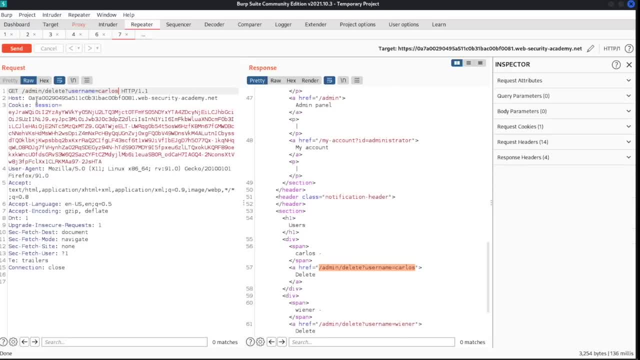 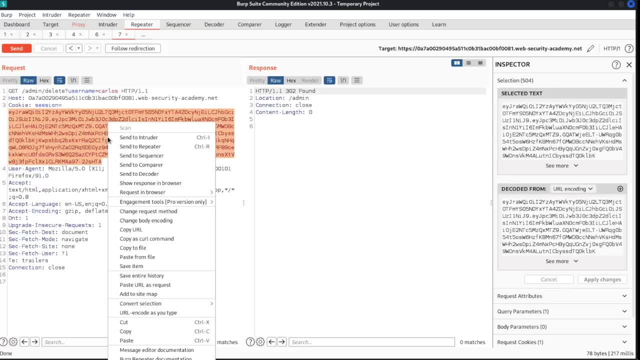 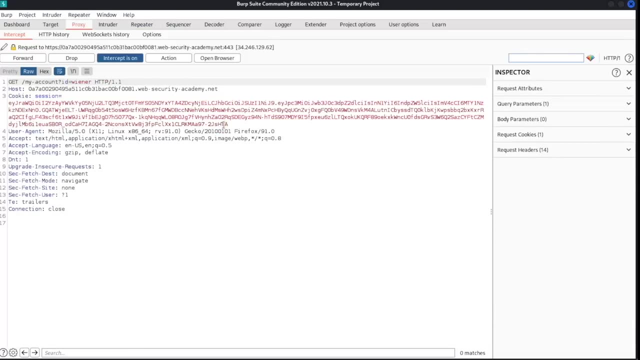 and i think it should delete him. so if we send this, that does not work. so what we'll do is we'll just grab this entire token right here and we will copy it, come over here and we'll just put it in place of that one forward. 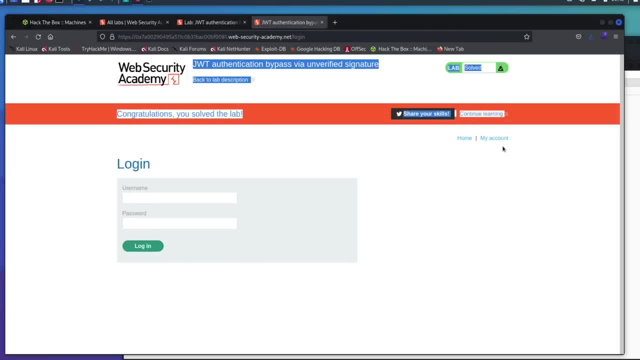 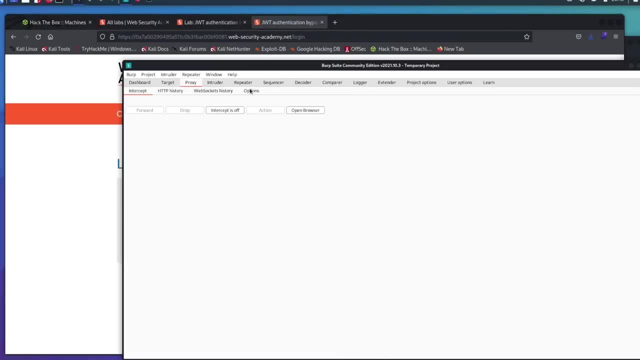 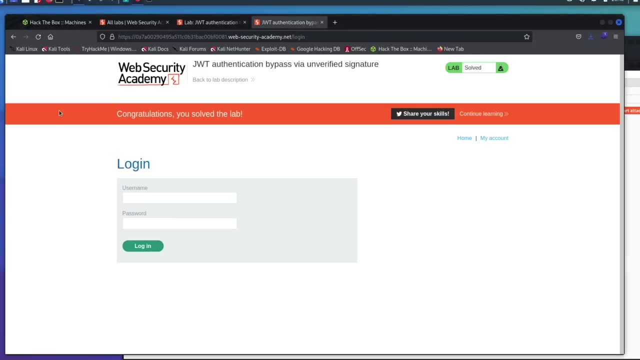 turn the interceptor off, it tells us that we have solved the lab, i guess because we have the interceptor on. when we sent the request right here to delete carlos, it didn't refresh this the page because the interceptor was on, so it went ahead and deleted the user for us. so that is one. 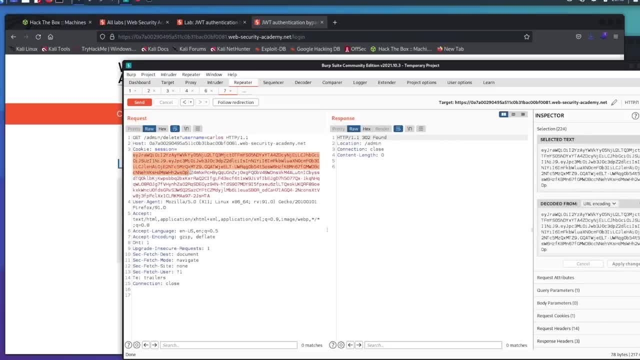 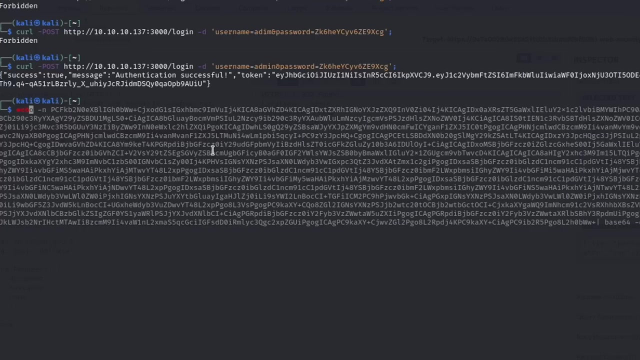 way to use these tokens and they might be a little bit difficult in the beginning. but i really love this interceptor over here that just decodes stuff for you. otherwise you can try and decode this stuff by copying it like this and you can come over to your terminal and you can go echo dash in. 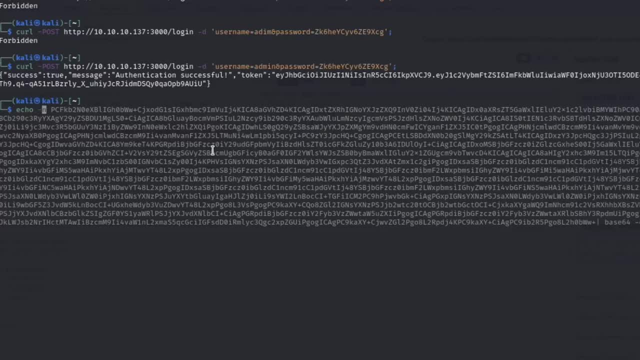 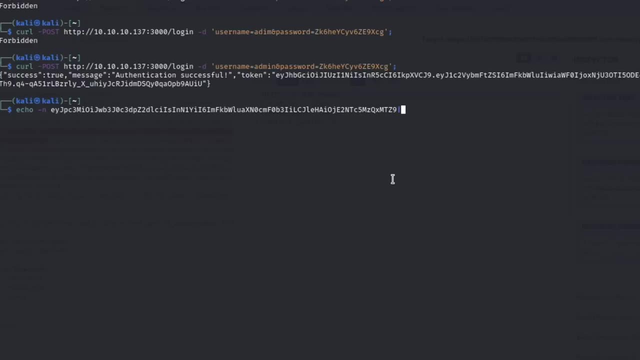 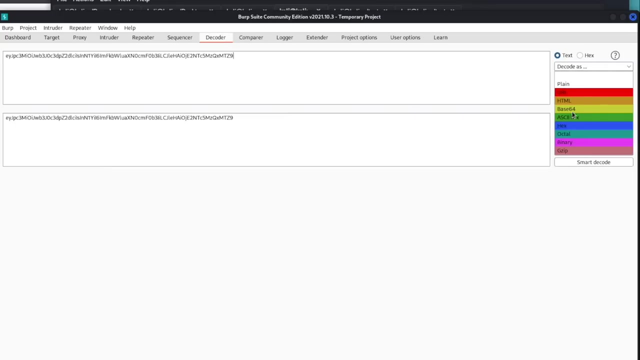 just like this, and then you would just paste in the token that you wanted to decode pipe. and then we go: base 64, dash d, and that will you decode it for us. you could also just come over to the decoder, paste that in and decode as base 64. 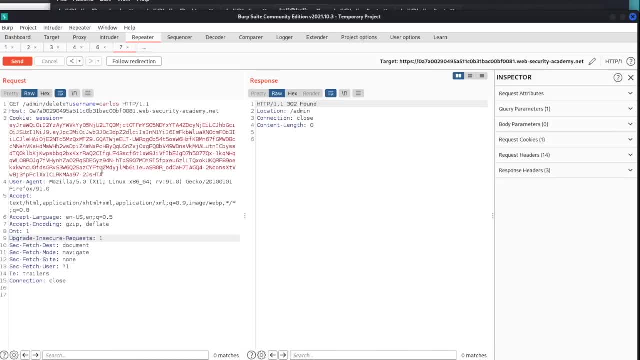 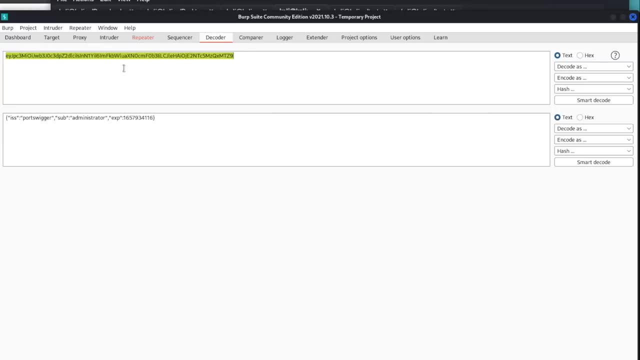 and it'll tell you over here as well. so those are different ways to look at these cookies. i'm actually curious. now this leaves it all as a jumbled mess, but i am curious. if the decoder can figure this out- and i accidentally copied it, we'll recopy this. 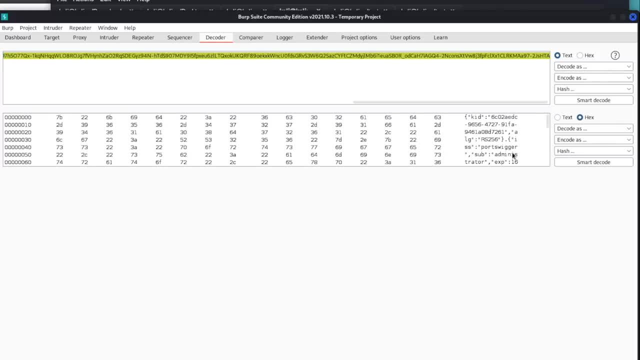 and this over here, and it does. it does get some of it right here. if you didn't know that it was separated by the periods, you could have brought it over here to the decoder and you could figure out what's going on. it's not really that easy to read, but you can see that we got the administrator right here. and we were issued by port swigger. so i mean you could have figured it out, but that is thealy a check out here and we just left this alone. i just cigarette control its own jscom code. it's a really easy. fix us something like auto sp. mejor json grammar bits. we are not going to need another. 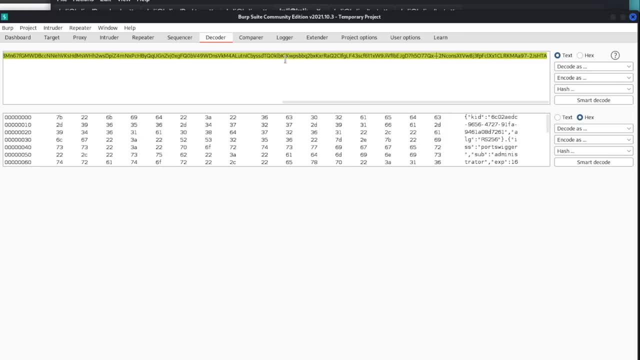 profiling function, bull grip as well, but you can get some really great tips. we came across where you just gotta- so, basically, with all these things- and some of those things get super fast as ghosts will- is this challenge. There is another one right here that we are going to walk through, so if you 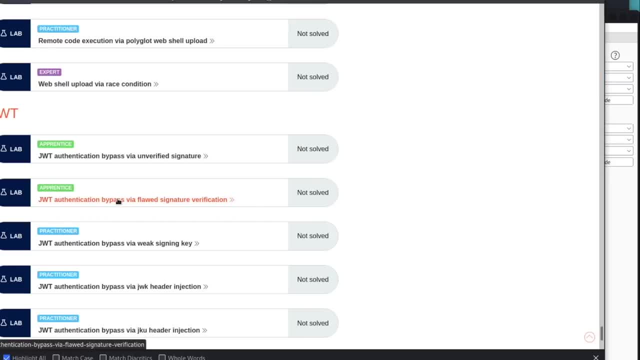 would like to open this one up. there is a little more to it. I'm not sure you'll be able to figure this one out completely on your own, but you can go ahead and play around with it and see if you can figure it out and we'll go ahead and I'll open it up and then we will solve it. I have opened up. 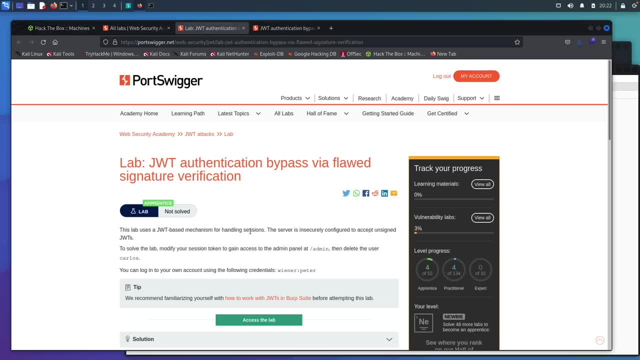 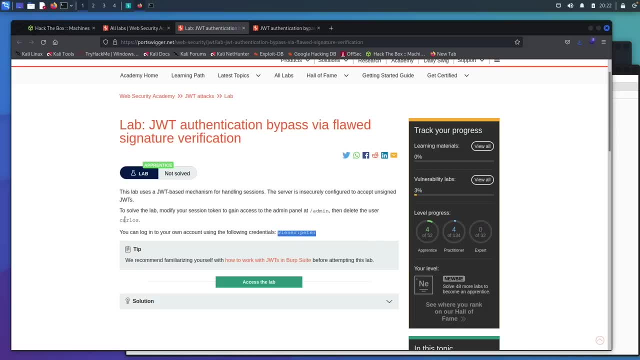 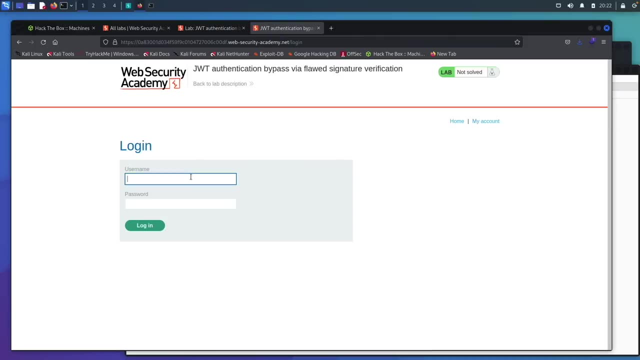 the lab right here and we are brought to this page. The instructions are pretty much the exact same. We need to make it to this panel, We log in as this person and we delete this user. So we can come over here, go to my account. We'll get logged in and then we'll intercept the request. Log in. 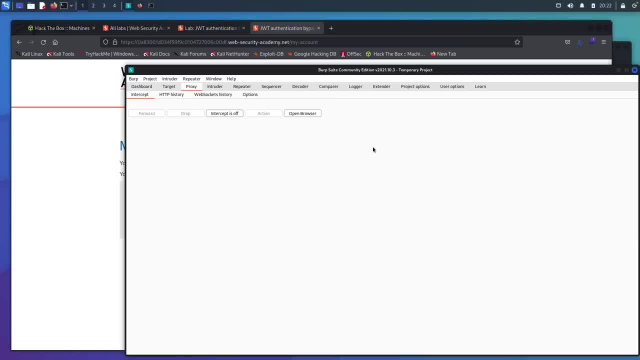 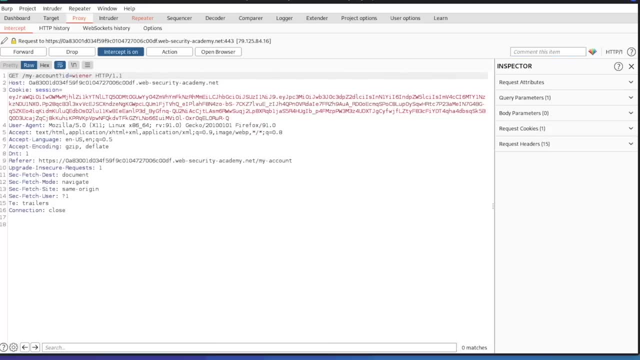 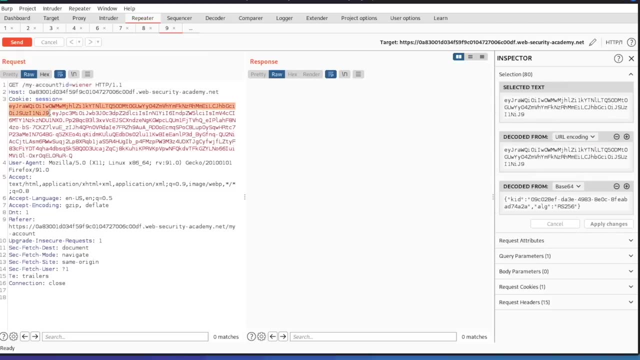 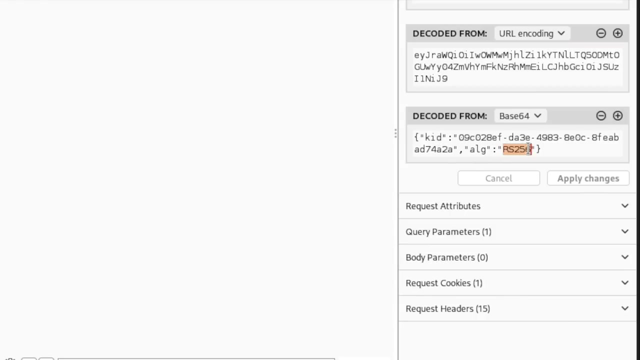 Don't save. It says we are logged in, so we'll go ahead and intercept the request, Send to repeater. We can shut that off, Come over to repeater and we can do the exact same thing we had just done before. and we're told right here that it's using SHA-256 as the encryption, which I'm guessing is. 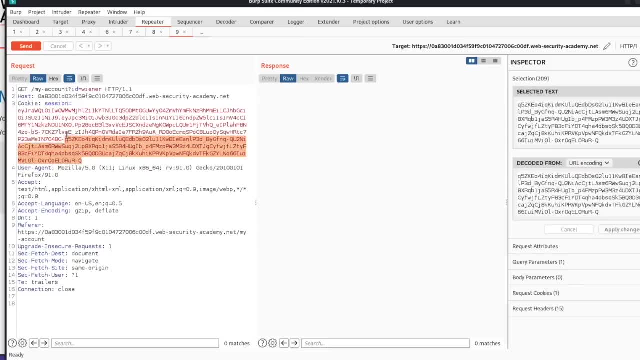 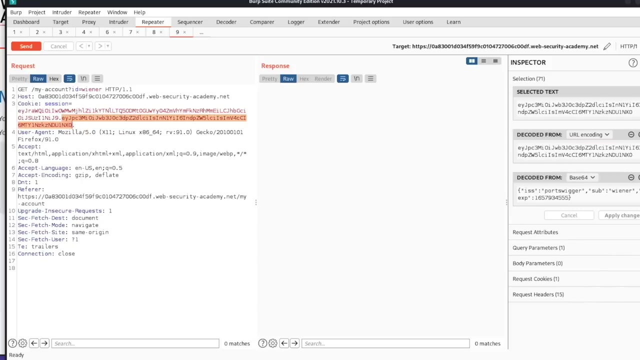 going to be for our session key right here, And so what we can do is come back up here and we can change this To none, And then we can delete our session key, Highlight this And we are supposed to be the administrator this time. We're supposed to be administrator. Learned last time that it is not the 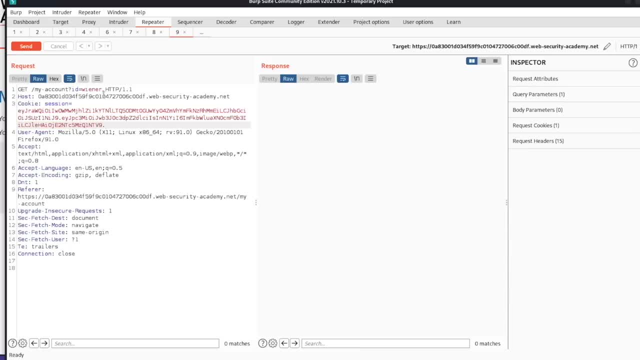 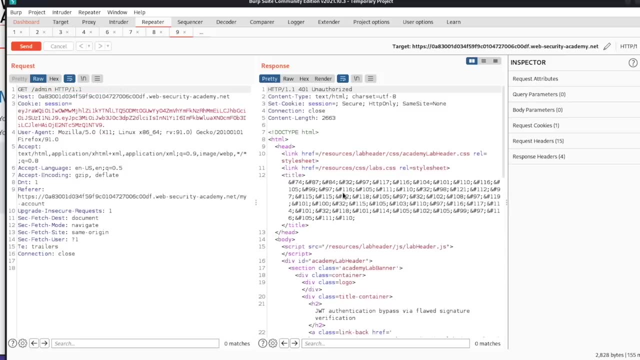 admin, We can apply the changes And we'll come back over here and see if we can go admin And we can send this. It says we are unauthorized. Let's try and look at this again. I did not apply the changes right here, So we can say none Apply. Send this And we. 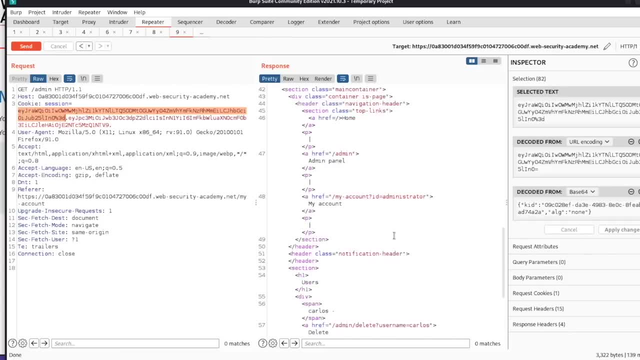 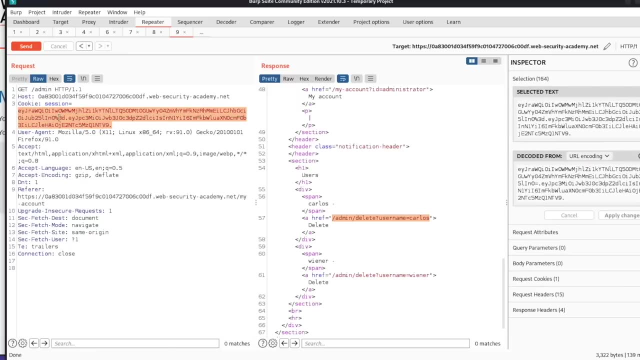 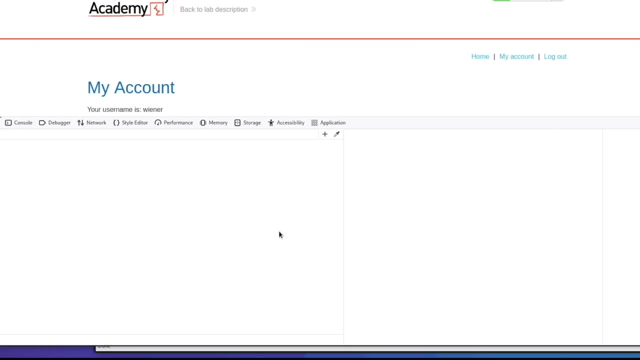 have made it And from here we know what we need to do with highlighting this and going over here and trying to delete it. But I want to try this a little different this time. So I want to copy this token and I want to put it in directly myself. 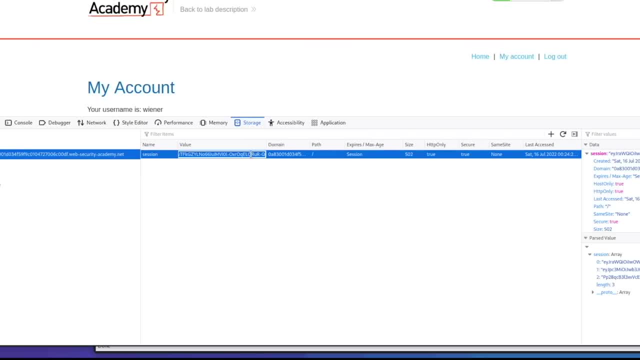 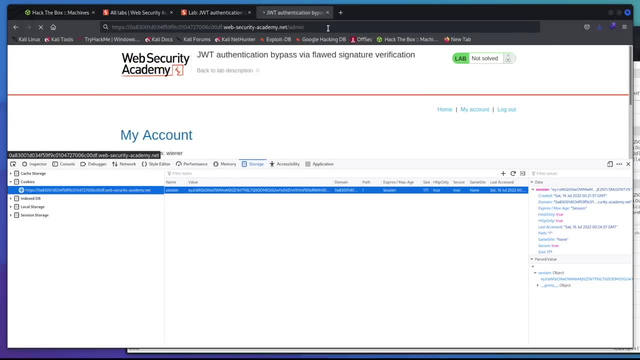 and see if I can make it over this direction, Make it over this way. I think it should work. Try this a little different. And it works. So we can come over here and delete the user This way And you can put the session token in right here. So these are a few different ways. 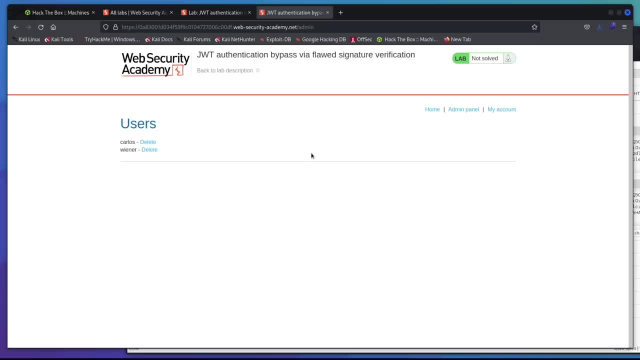 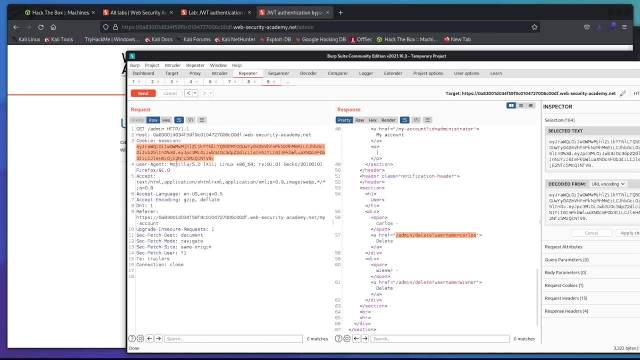 you can bypass authentication through tokens and session cookies. You will just have to play around with these as you find them on live programs. They're not always going to be really straightforward, So what you could do is look for what uses a period as a separation inside of a cookie, or 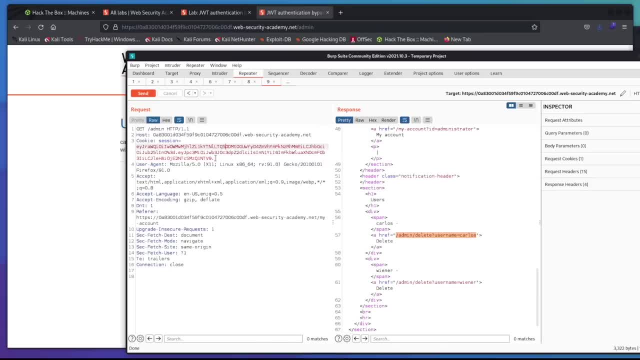 inside of a session token, And these are things you're just going to get used to over time: seeing and not understanding what it is and then looking it up. this is also one reason it would be great for you to read the web hackers handbook and other web application penetration testing. 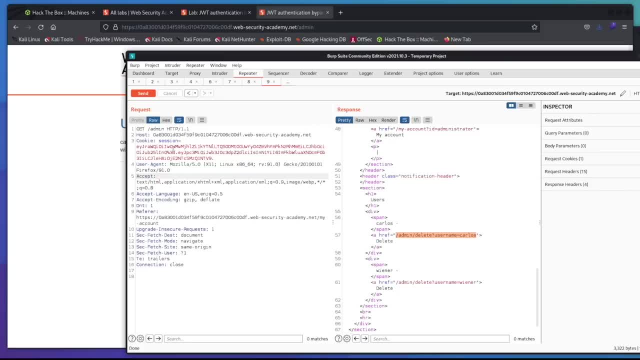 books or even the activity, because you're going to see things like this and you'll be like: what is this period, what is going on right here? and as you read, you will learn how to recognize these different things. it's okay if you didn't recognize them this time. i bet you will recognize it. the 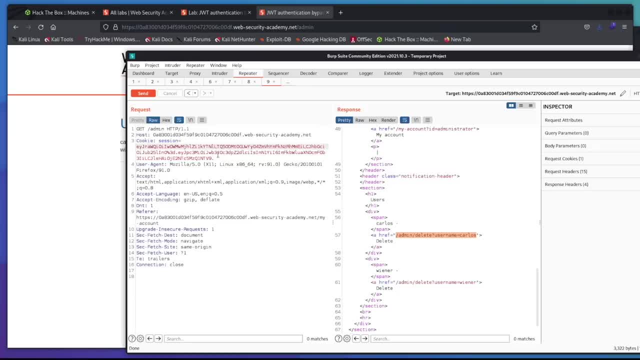 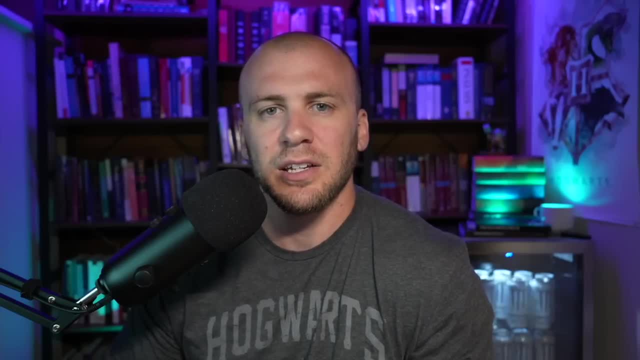 next time you come across it. so with that, we will continue on. okay, i decided to include this little section right here on attacking wordpress websites because, to my surprise, the more i am in the web application testing world, i am surprised at how many people use wordpress, and even if they, 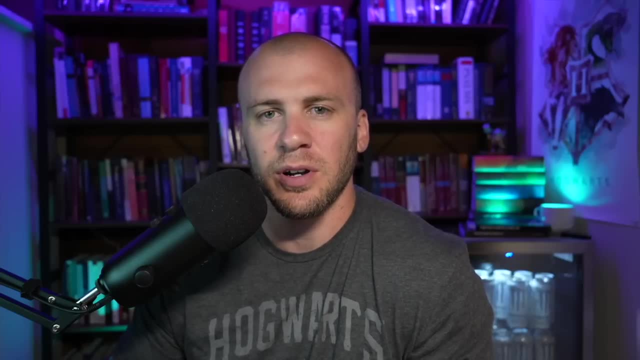 don't use it on their main site. there will be subdomains, or sometimes they'll have other domains or subdomains that are also in scope- that will have wordpress especially, especially if you're using it on your main site and you're using it on your main site. 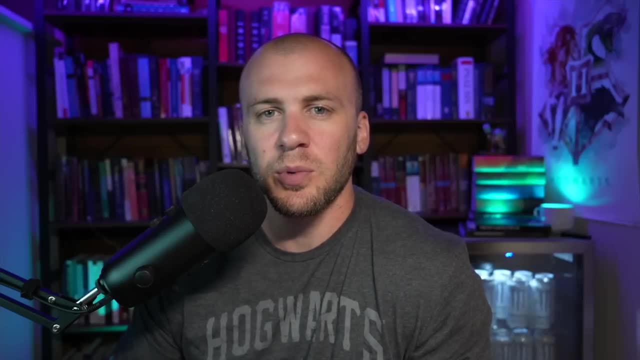 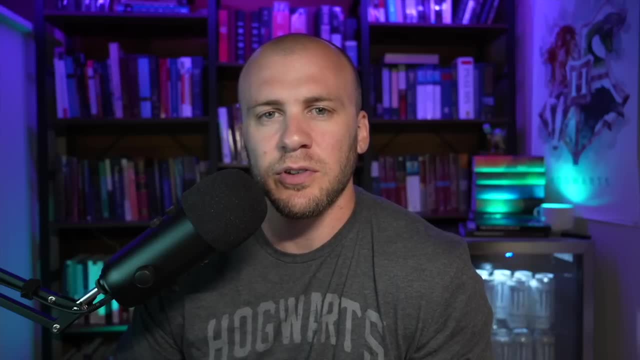 of and know how to enumerate and attack it, and so we're going to do a few hack the box wordpress walkthroughs now, just until we get remote code execution or find vulnerable files. so the way you can see how you should attack wordpress and wordpress is becoming more common, so i decided to 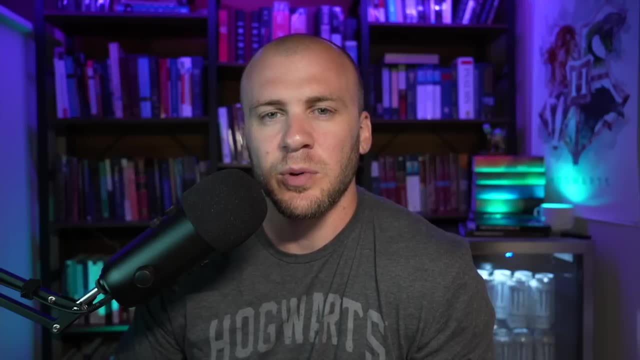 include this in here, because i don't think a lot of people in the bug brownie world attack wordpress the way a penetration tester would. so we're going to look at these for a penetration tester perspective and how you would go about attacking them, but also along the way you. 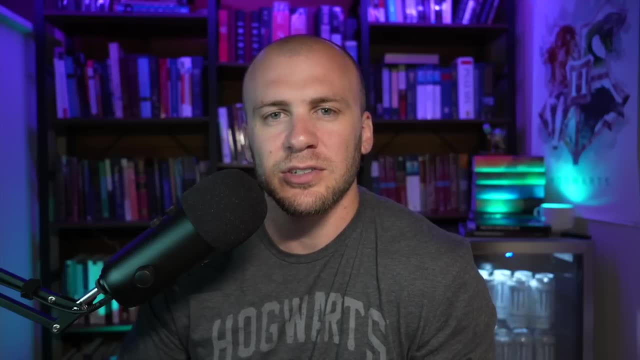 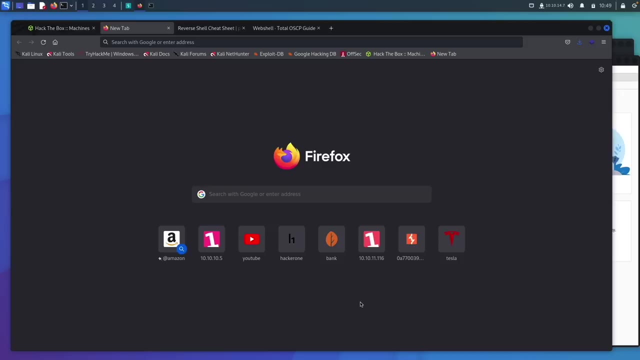 can look for bugs as you enumerate wordpress sites, so let's go ahead and jump into this. all right, i have a spun up the box, tenet, for us to walk through. we're going to be doing two different boxes that have to do with wordpress, and i think this is something that you should really know well. 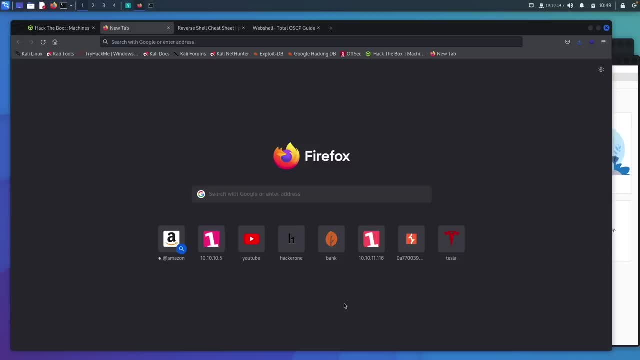 because you're going to see these definitely in ctfs as well as in bug bounty programs. a lot of bug bounty programs are going to be in ctfs as well as in bug bounty programs. a lot of bug bounty programs, you'll notice, actually will put the blog or some kind of forum sites in the not eligible category. 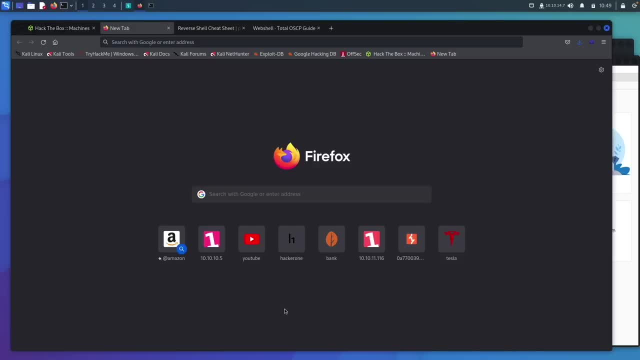 or out of scope, which really is a mistake, because a lot of wordpress sites actually do have vulnerabilities in them and you're going to see them a lot in ctfs and we're going to cover a couple of those now. so i have already opened up, i have already started the server, so we are going to 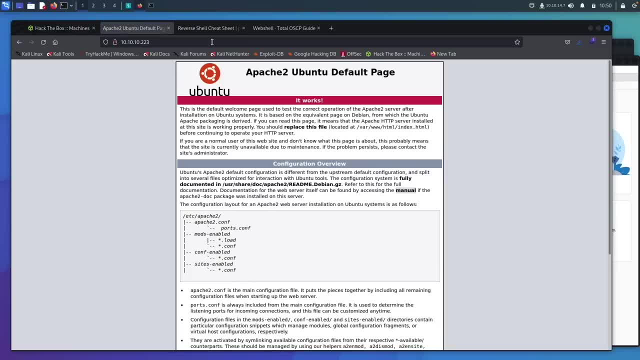 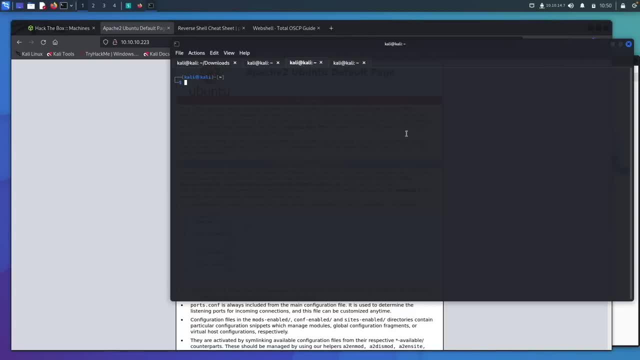 be at ip 10, 10, 10, 10, 2, 2, 3, and then we can come here and we're brought to the default page and one of the things we should always do is try and run fuff or go buster. i'm. 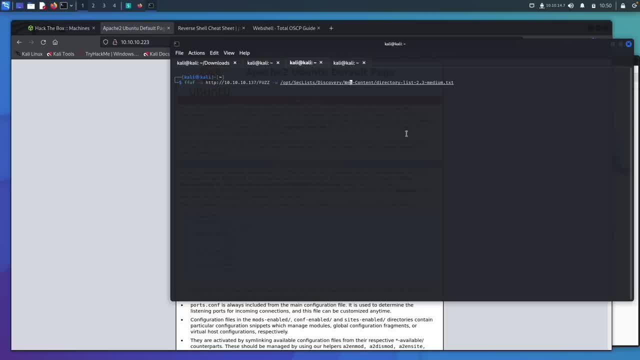 going to use fuff, because it is already set up here for me, so we'll just change this to actually, because this is going to be a wordpress site. we're going to run go buster because we will want to have this extension for the php right here so we can come back here. 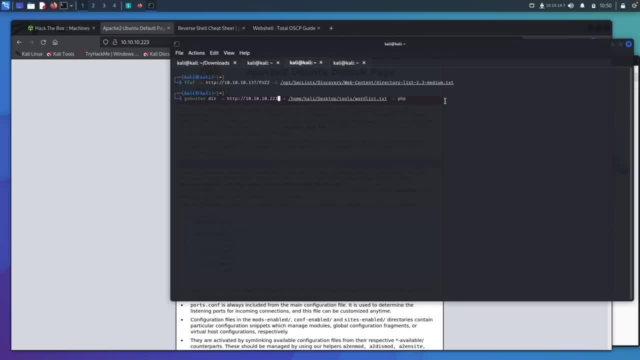 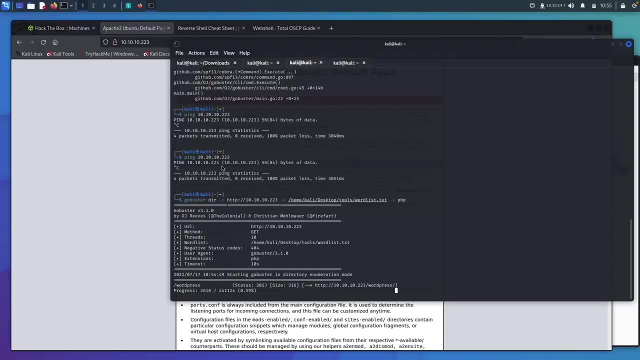 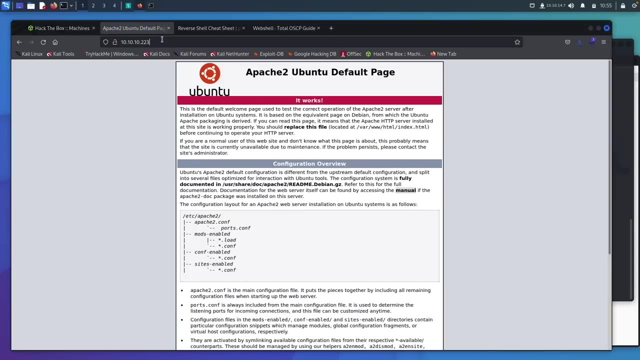 set this up: two, two, three and let that run all right. so i got go buster working. it turns out that it wasn't working because i had been disconnected from the box. but now it is up and going and we see that there is a slash wordpress so we can come up here, type in slash. 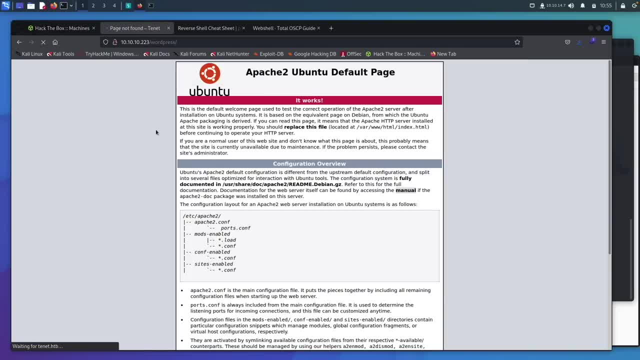 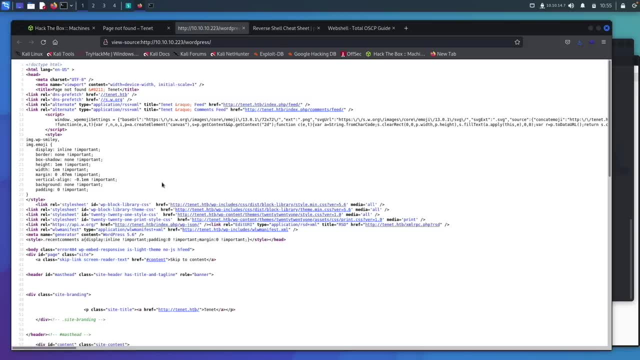 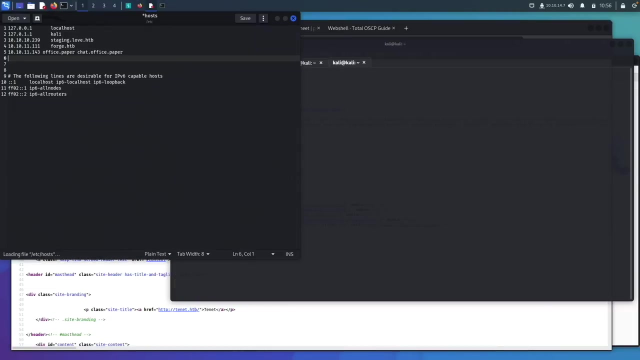 wordpress and see what we come across. we come to this page right here, we can view page source, see what is in here and there is an href to this tenanthtb. and if you're familiar with hack the box and then you know that you frequently have to add things to your etsy host file and the 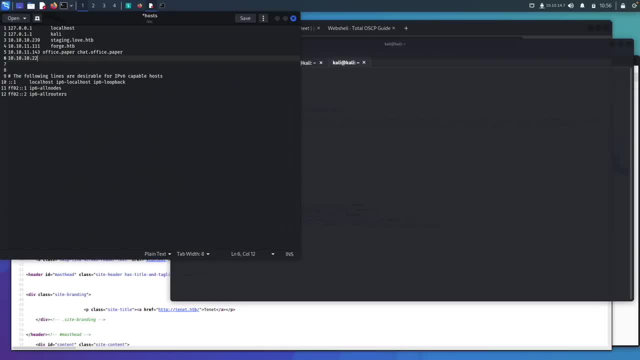 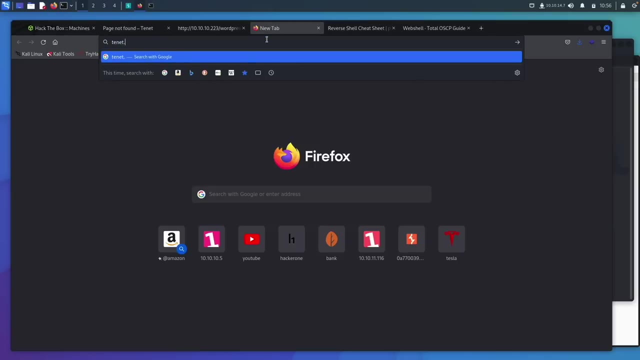 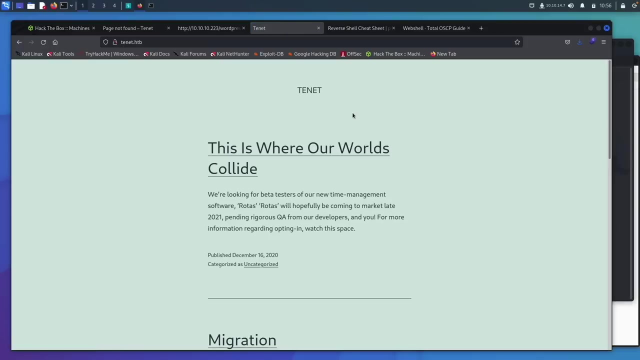 ip address is 10, 10, 10, 2, 2, 3 and it is tenanthtb. now we should be able to save this and browse out to this page. so, tenanthtb, i want to go here and it loads this page for us now, one of the first things you're going to do anytime you 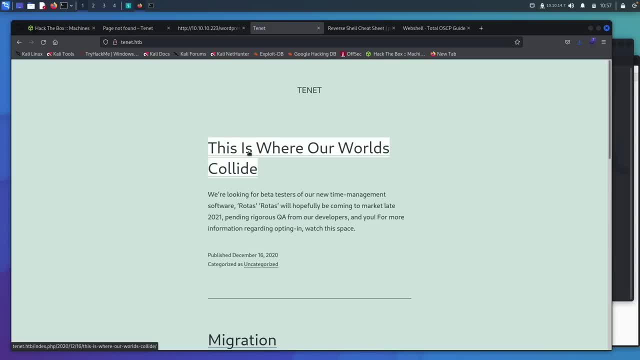 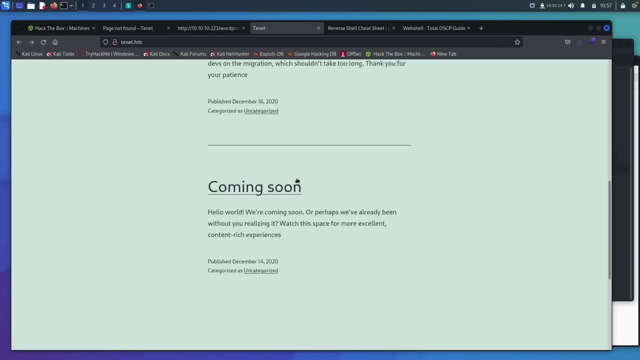 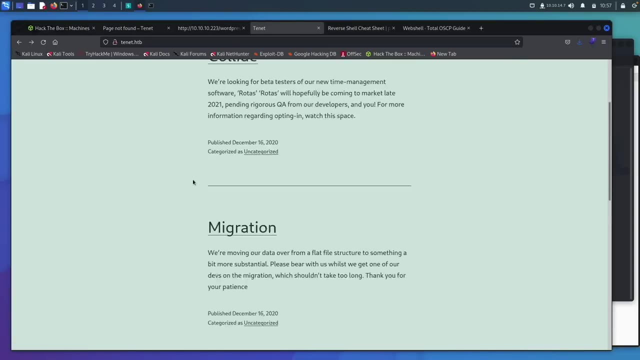 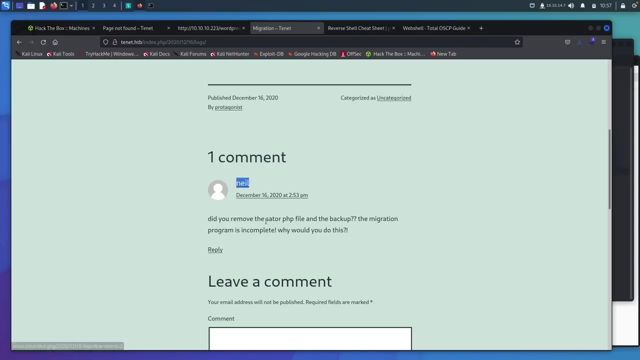 come to a wordpress page or a blog page in general is: just look at these posts here and you can see you have protagonist as an author, which could possibly be a user. we can look at this- one same user, same author. and we can look here- same author. there is a comment by neil. you could put this in: 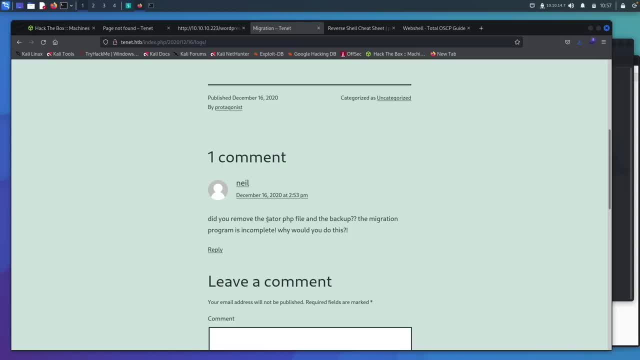 your back pocket as a potential user. and then it says: did you remove satyr php file from the backup? i'm not really sure why somebody would have write this right here rather than let the person know elsewhere, but you could try and come in here and type in the. 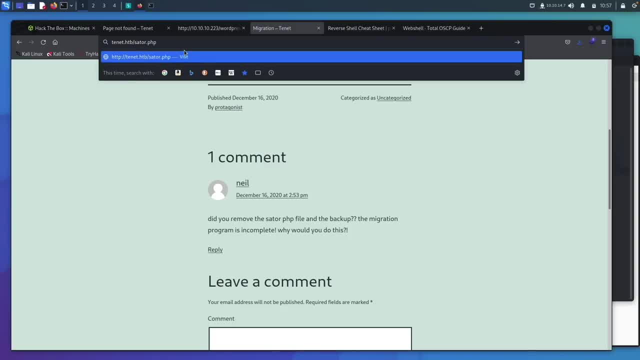 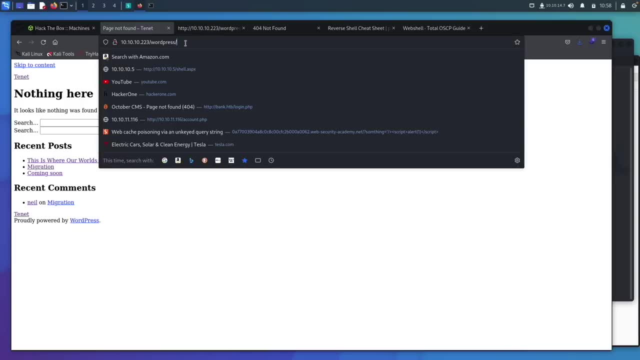 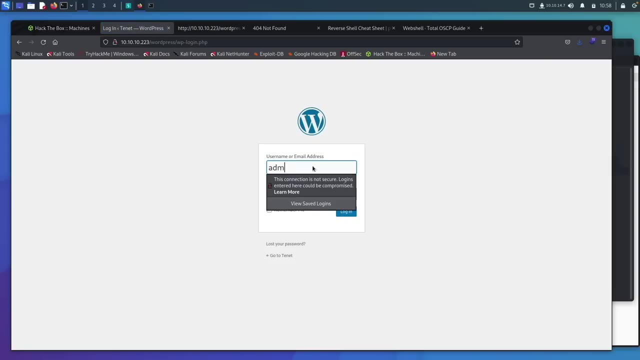 satyr dot PHP and see if anything is there. it doesn't look like it, but you could come over to where we know we have this WordPress and we could say: WP dash login dot PHP, my, and you could try and log in with admin admin or admin administrator. 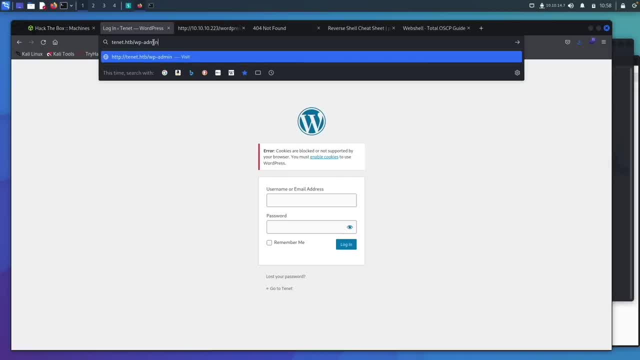 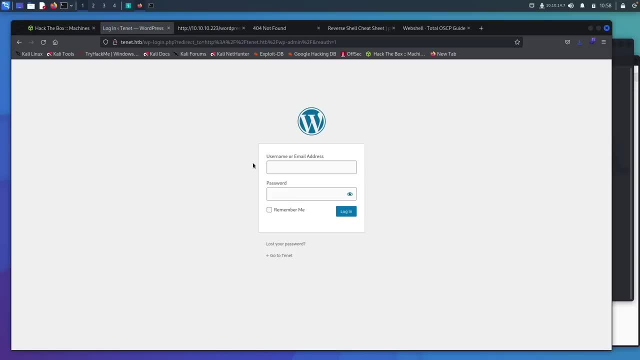 I think you actually can come over here and do an admin dot PHP. nope, let's see if it's just slash admin and there is this login page. it tells us it just redirected us here to the login page, so not able to do anything with this, and 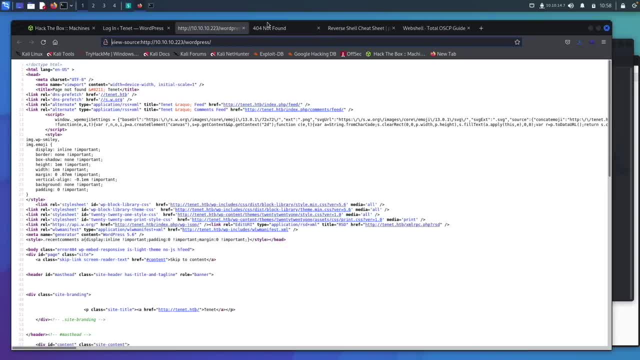 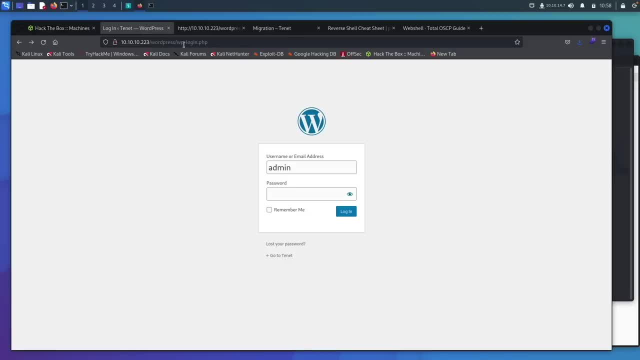 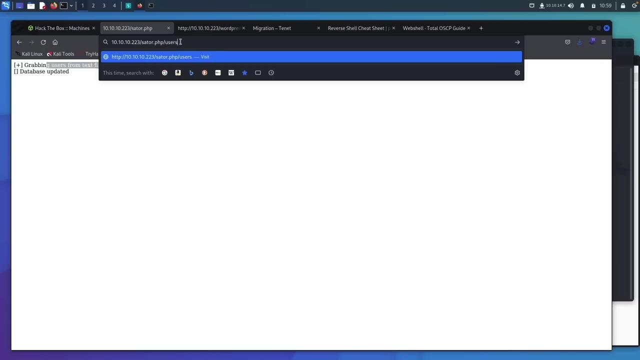 we'll just come back to that main page. we can come back over here to this. there was no SATA dot PHP, but we could try it over here and we can run it and it tells us that it's grabbing users from a text file, which would be interesting. I wonder if you can go: users dot txt, nothing and you. 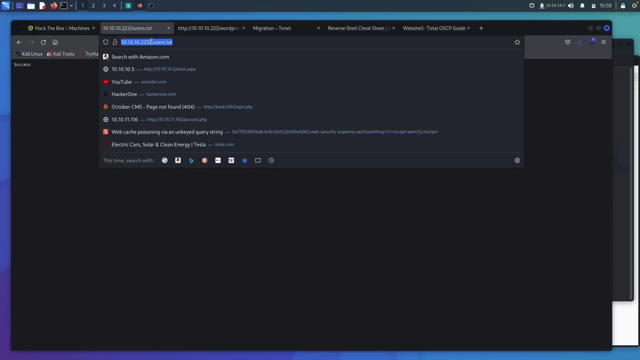 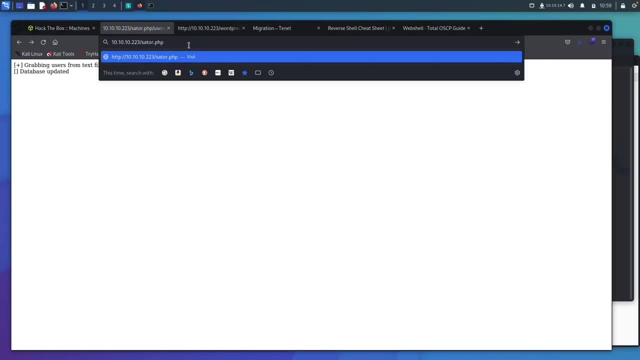 go back and it just tells us success. we're not able to actually grab any of those users. so he said it was from a backup file and often when you see a backup file it's going to be a dot back and it works for us so we can save that. 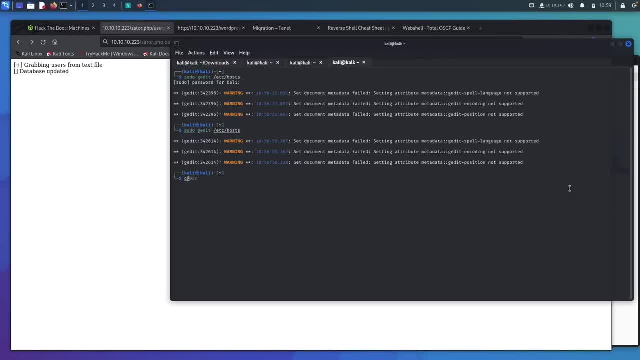 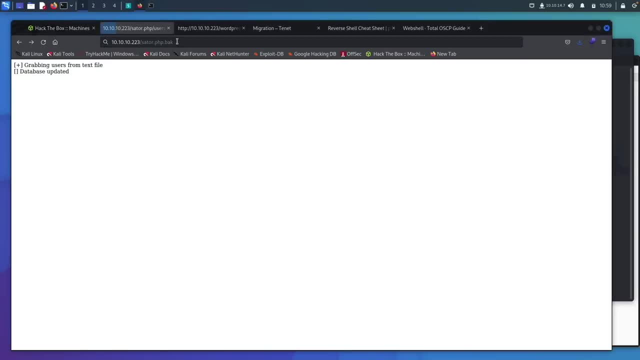 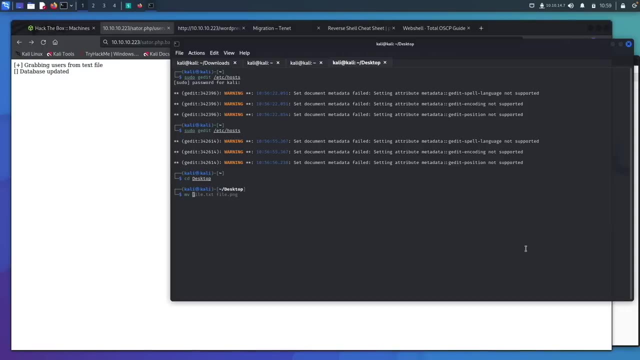 to our downloads and we can and we can save that to our downloads and we can save that to our downloads and we can cd to desktop. we can move- I'm not sure what that save does- saved as SATA dot back. so we come over here, move, and then we'll go and we'll move this to. 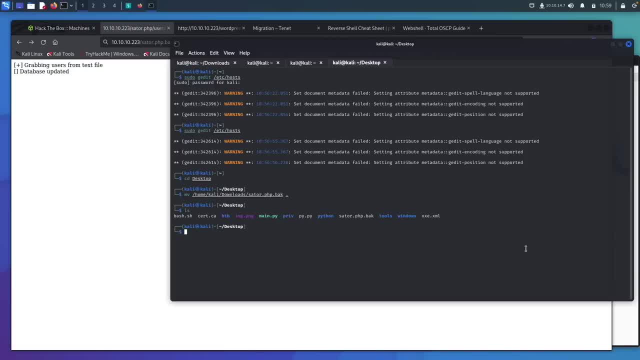 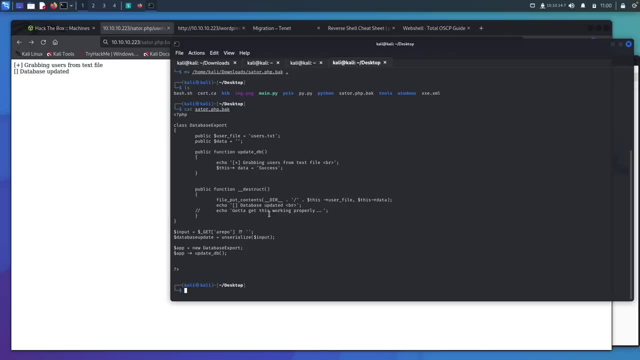 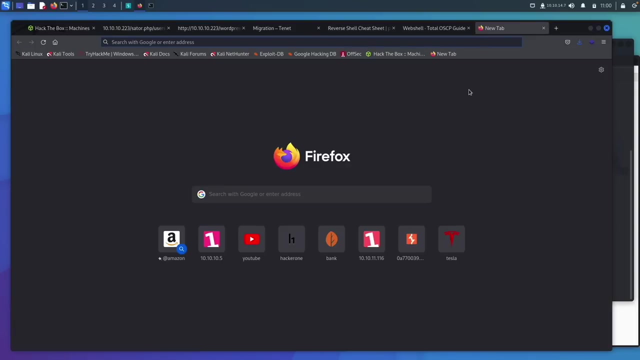 the current working directory, which is going to be our desktop. now, if we LS, we have it right here. we can cat that file out and look to see what's going on now. when I Saw this, I had to go straight out to Google and look up Serialization for PHP, because I am not really familiar with it. And when you come out to Google and you just look up, 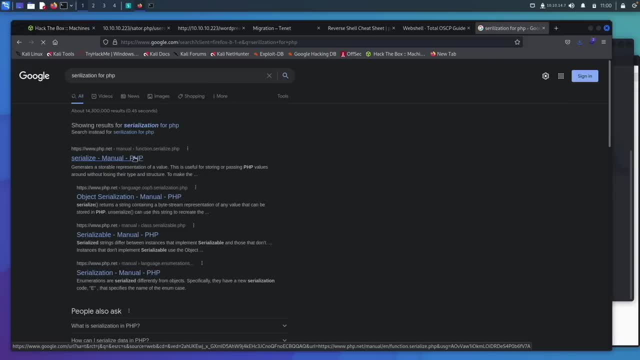 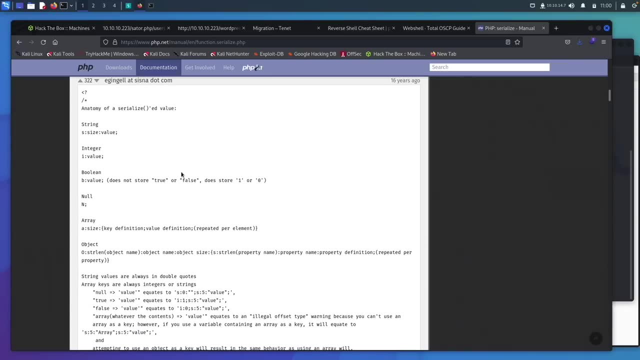 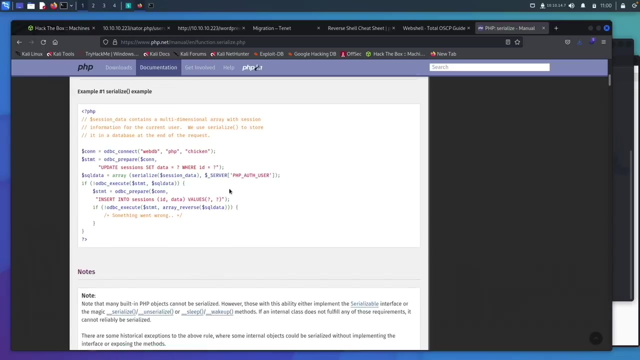 Serialization for PHP. and then you can just click this top one and when you look through here, It looks really similar to what we just saw. and then it actually walks us through how this works. so when I saw this I was like okay, this must be what is happening and you're gonna have a. 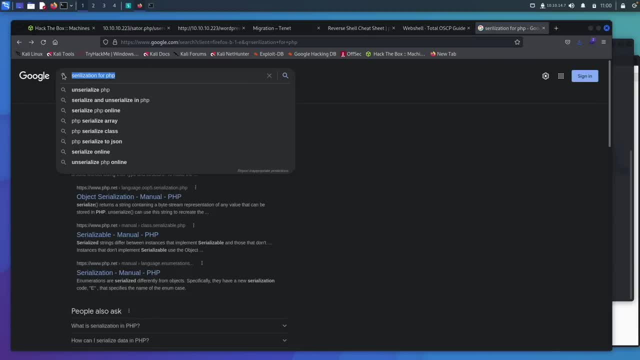 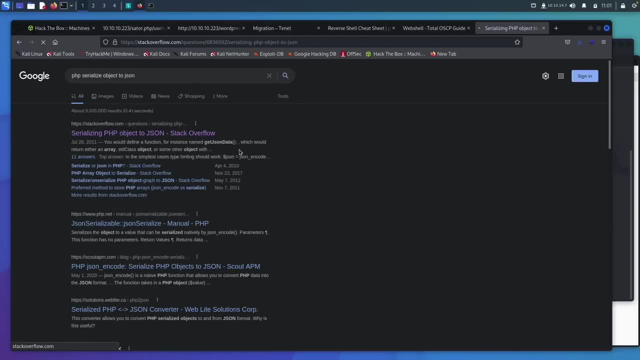 Serialized object, and so you might even be able to go and type in Object like this and let's see what happens if we get it into a JSON. This is a stack overflow and you can just look through here. This is what I did to figure this out. 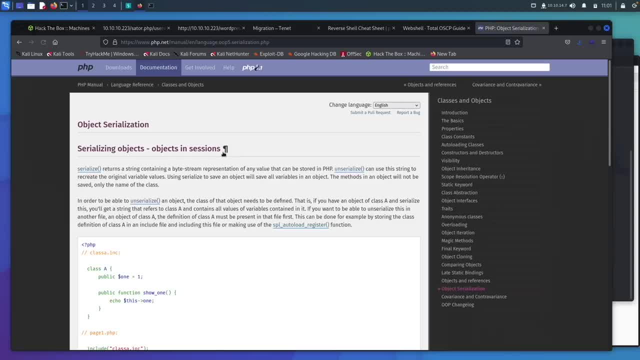 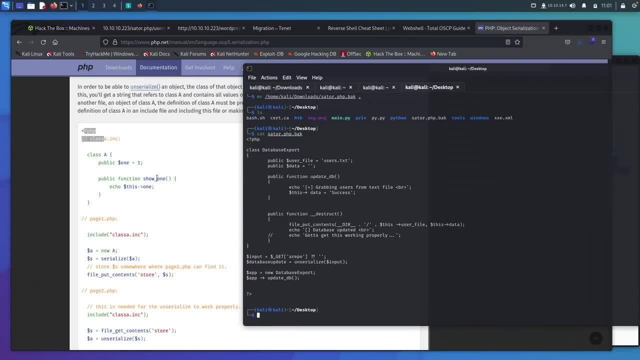 remembering that you're gonna have to use your Google skills, and this looks even more like what we just saw right here. So we know we're gonna have to do something along these lines and we have it Getting a repo, and then it has this unserialized input being called. 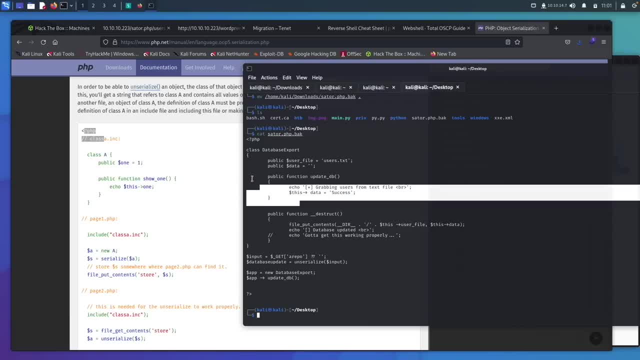 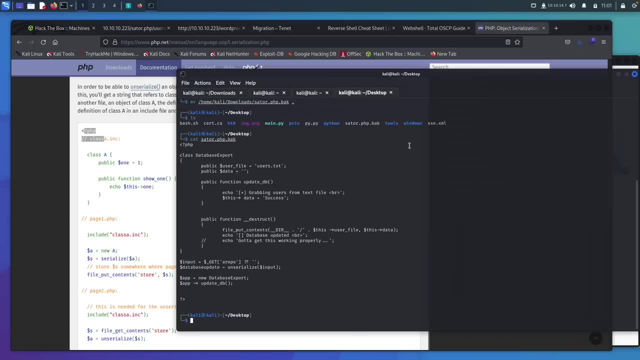 So what we can do is just grab This right here and we can make our own serialized object. so We'll do this here, We'll CD into the desktop and we'll get it and we'll call it minephp, and Now we will change this to fit our needs. 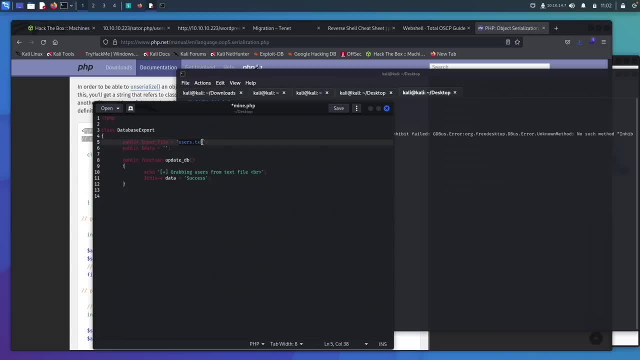 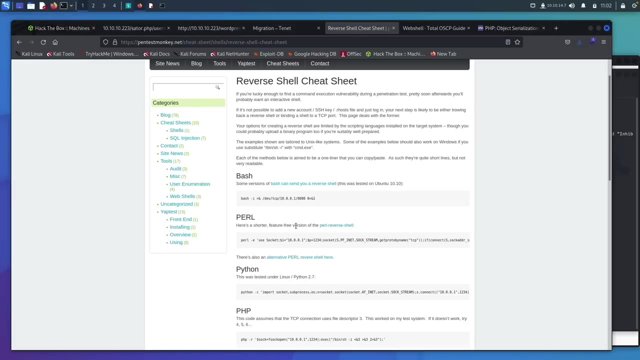 So instead of going user text will go Pwnphp. We can leave this, because this is where that's this is going to be our object, and then, inside the data, we can put in our little Reverse shell that we have seen earlier. So we'll grab a PHP now, we'll do a web shell first and then we'll do a reverse shell to make sure that it works. 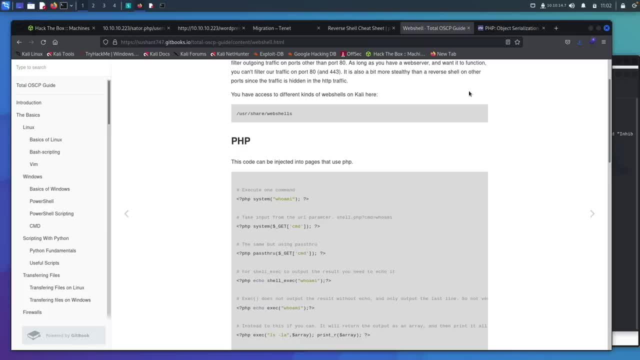 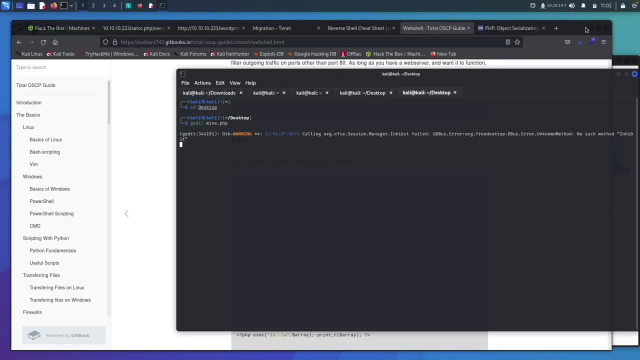 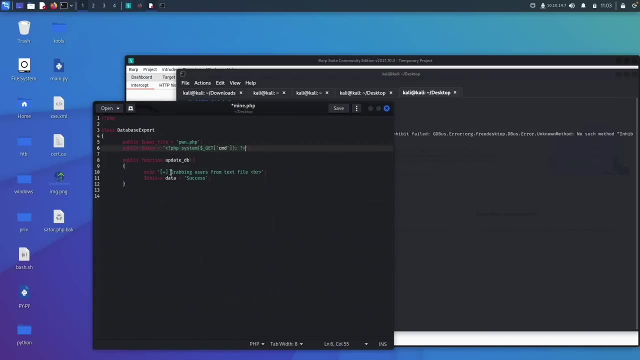 For remote code execution. We can just grab this same one We've been using throughout this course. Where did my Text file go? Right here and we can just paste this in and now, instead of We can, now we can delete this, delete this extra line here and up here we're going to say mine. 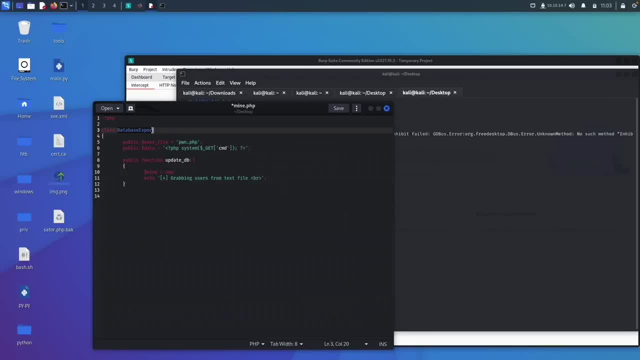 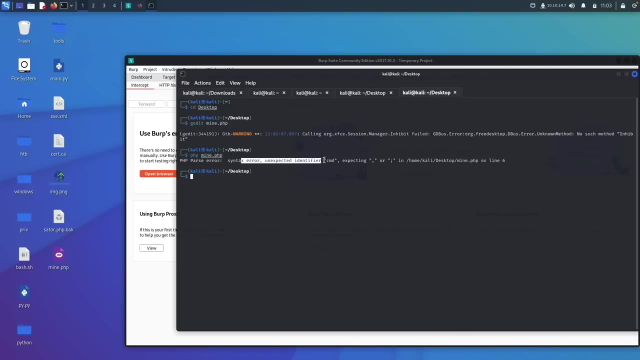 equals new, and then I'll just copy this so I don't have any typo and This looks like it should work. Let's try it real quick So we can just say PHP, Minephp, and it tells us we have a syntax error at the CMD. 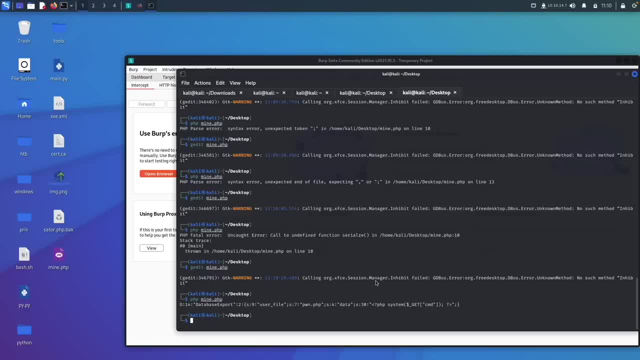 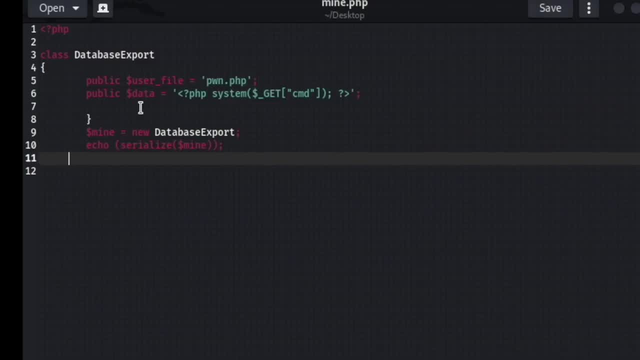 So we'll come back inside here, okay, And thanks to the magic of video editing and much debugging here, I Finally got this to work. I had in here- I had left in here- the public function to update the database and I had spelled Serialized wrong, which took a little while for me to figure out what was wrong. 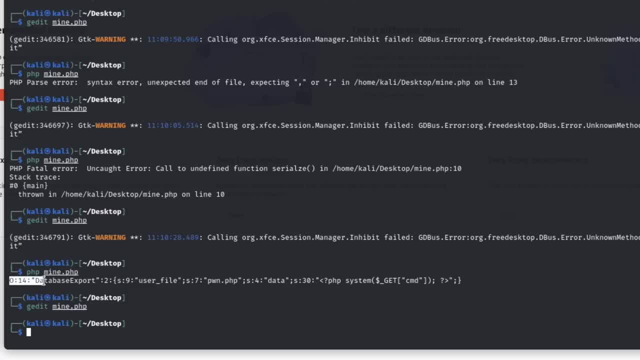 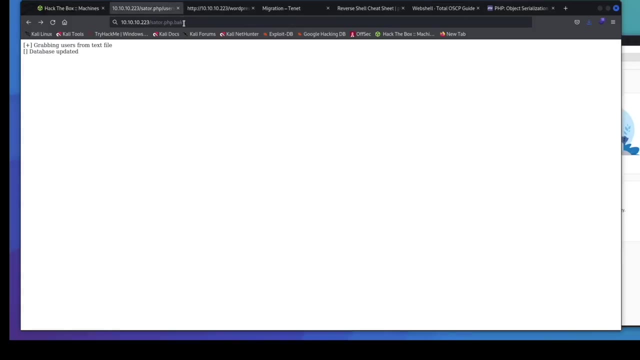 But now we get this output and this looks really familiar with what we have just went through with our JWT tokens. So now, if we now if we copy this string right here and we come back to our page, we should be able to enter it in right here and 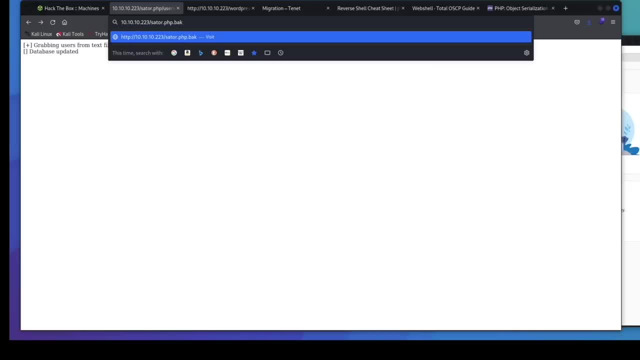 Pull down a web shell. so, if you remember from This, right here We have this a repo being called. so we can come over here and we can add this in by deleting the back, add in a parameter and we can say: a repo equals and then paste in the. 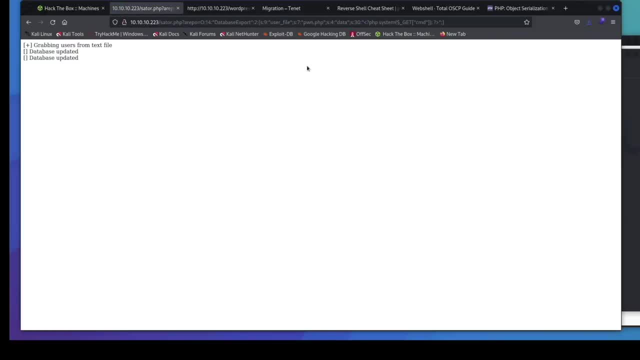 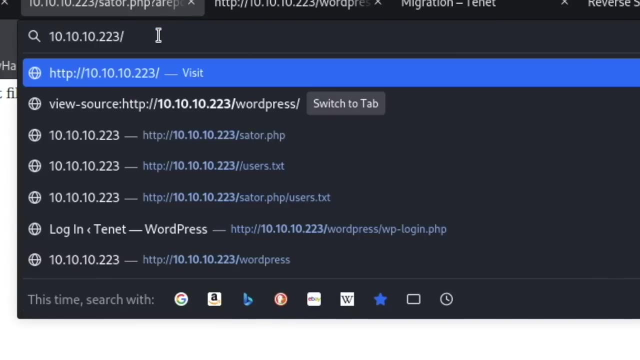 Serialized object that we just made. it tells us that it has added it, and now we should be able to come to our CMD and See if we have code execution on the box. so let's give this a try. Delete all of that and say: what did we name? I think we named it. 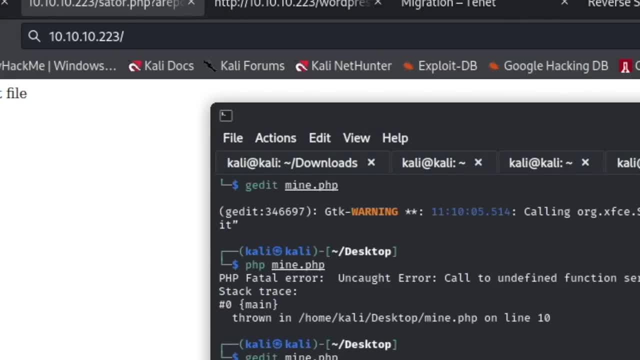 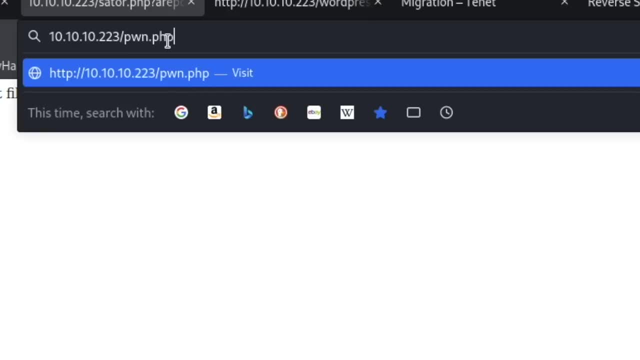 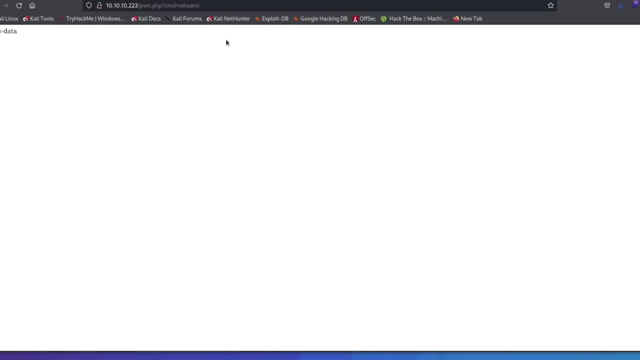 minephp, So we named it pwnphp. so we can come up here and we can say pwnphp. CMD equals who am I, and it tells us we are WW data. so now we should be able to get a reverse shell on this so we can come back to our reverse shell cheat sheet. 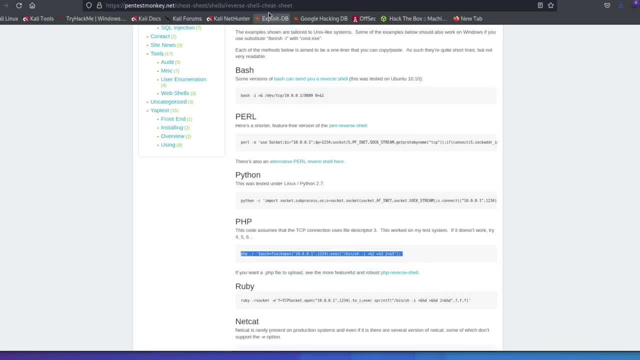 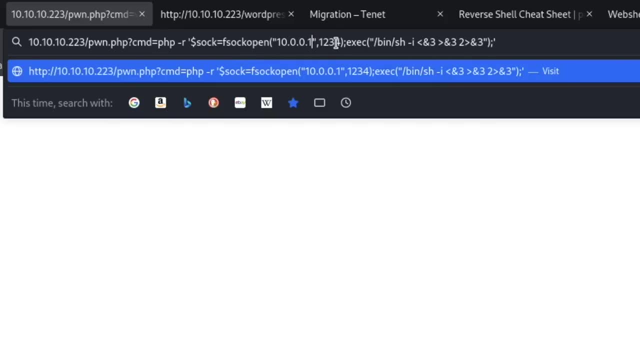 Since we know this is running PHP, We can try this with PHP. We can paste this in: my IP address is 10, 10, 14, 7 and we'll go on port 4, 4, 4, 4 and we'll go bin bash and. 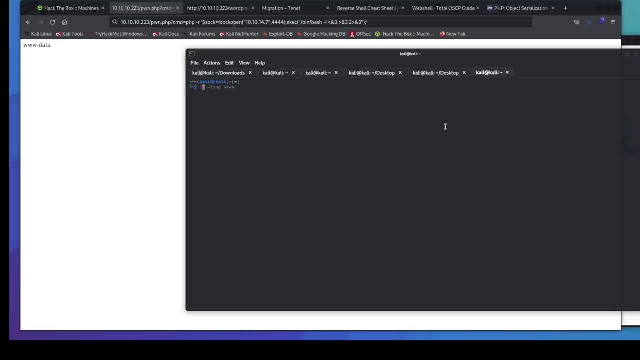 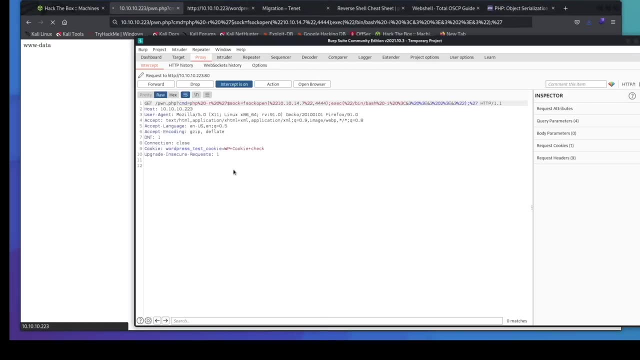 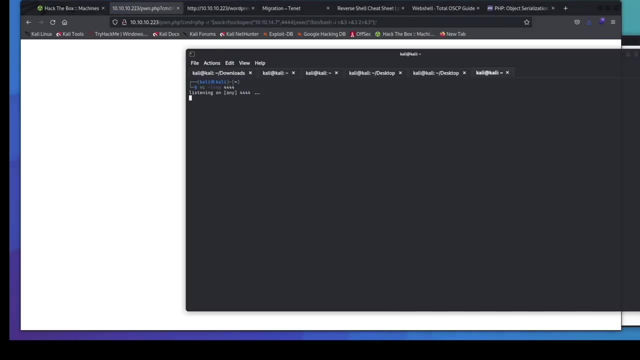 We can set up a Netcat listener Just like this, and we're also going to grab this in burp. just in case it doesn't work, We'll send to repeat repeater. we can turn that off and it doesn't work, so we can come back to burp here and if we send it, 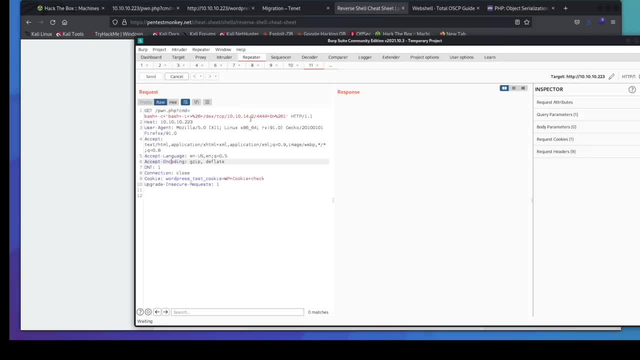 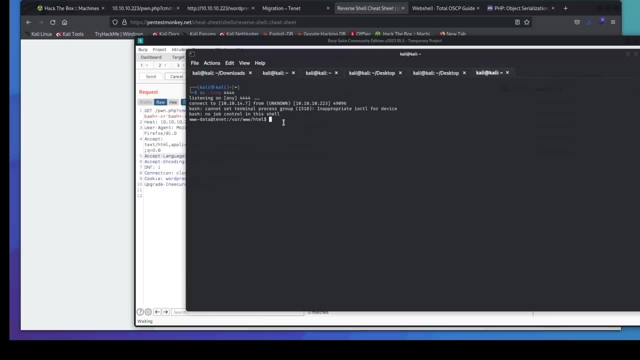 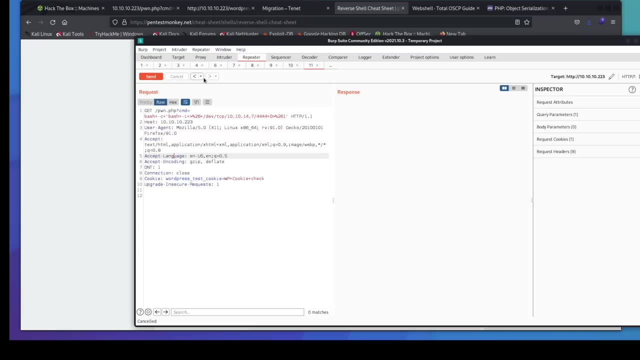 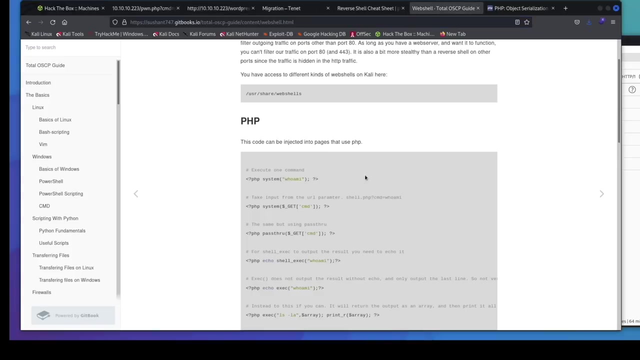 tells us that it went through really quickly and it turns out that i am dash seven and we send it and we get a call back. so i had my ip address wrong that entire time that i was trying to get that to work. so now i actually want to go back and try my php shell and see if that works. 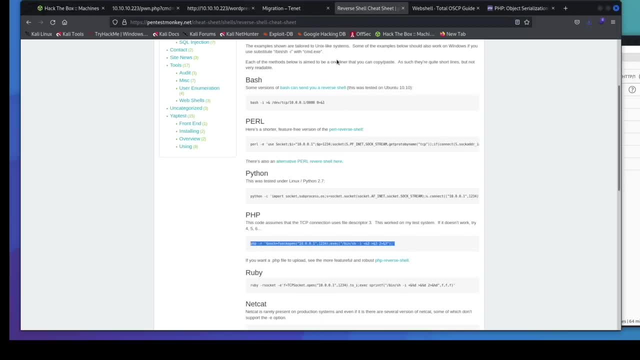 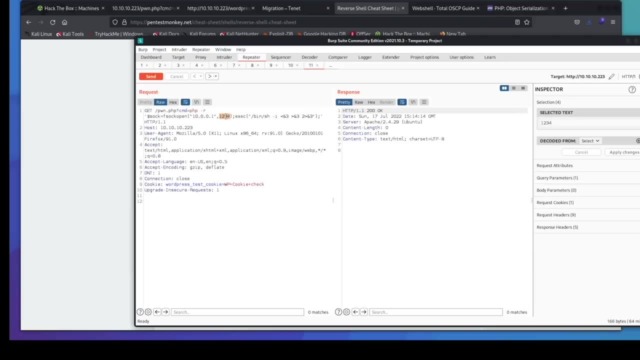 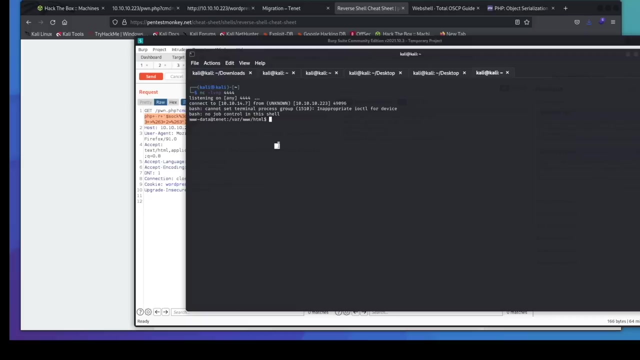 where is my php? come back over here, paste that in one. two, three, four. this is a seven 14, 10 here. this is my php one. so i'm going to go ahead and just Cornetto shelf and grab all of this url encoded. kill this shell. try a new one. send. 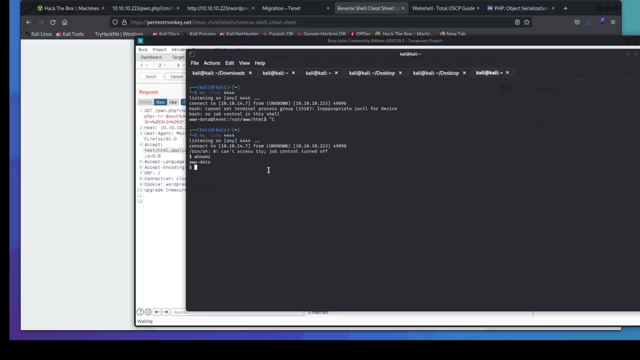 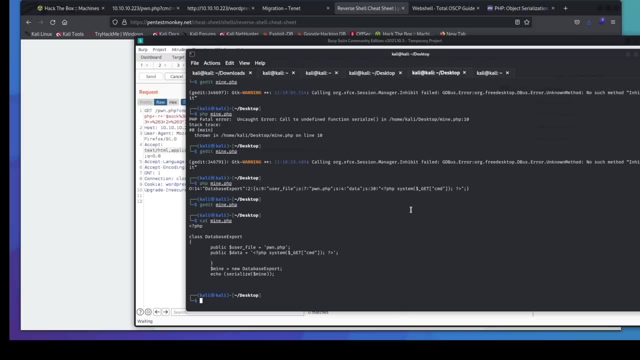 and the php one works also. so that was a bit of a work around, but i think it'll be helpful for you to see one more wordpress box, just to see that the enumeration process for wordpress is in php. so i wanted to show you this one because it just came off of what we saw with a serialized 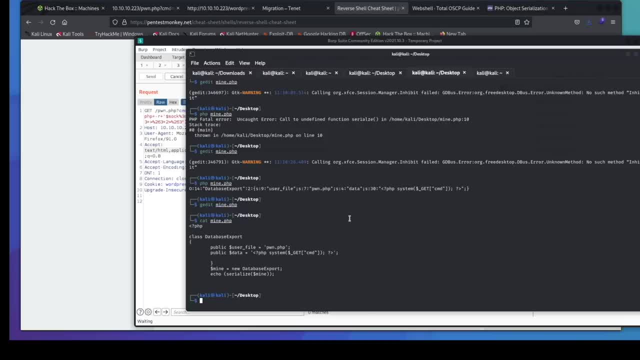 object like this and i thought it would be helpful for you to see a little bit of code outside of. i thought it would be helpful to see how it would work with wordpress, with php and with that we will go ahead and attack another wordpress box. okay, so i've gone ahead and ran an in-map scan and 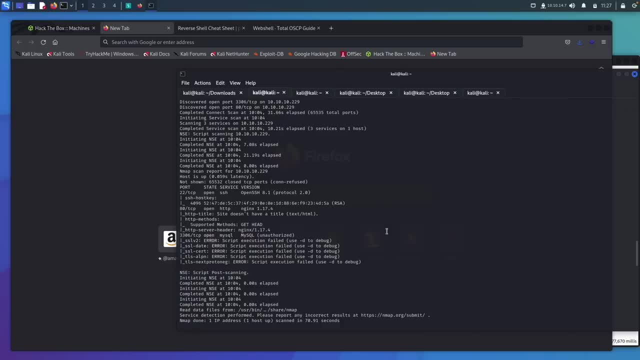 remember, if you run an in-map scan, to do so just on the common ports or the most common ports, because your target, if you're doing a bug bounty hunt, you don't really want to just be banging on their door looking for a bunch of open ports. but if you're doing a penetration test or some kind, 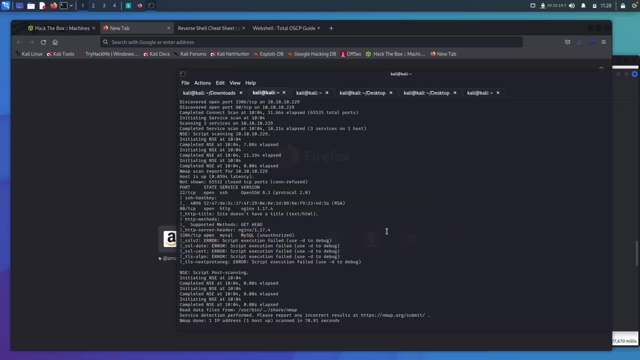 of ctf, then you can scan all ports. i've scanned all ports here, but just remember, if you're bug bounty hunting to only scan the common ports and if you are scanning quite a few ports, maybe slow down the in-map scan. with that said, you can run an in-map scan to do so just on the common ports or the most common ports, because 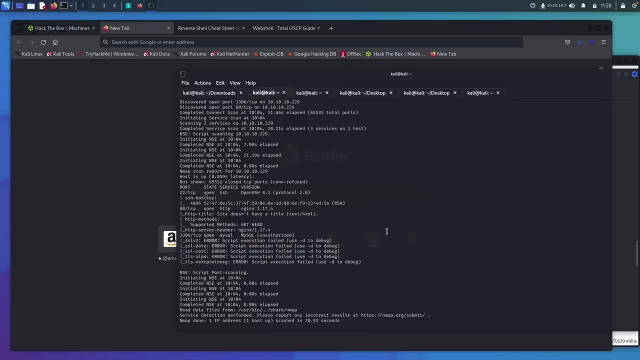 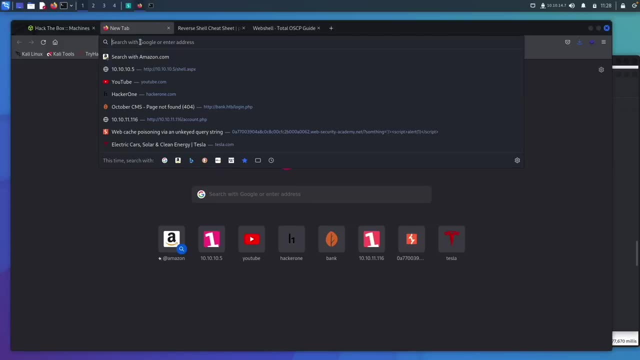 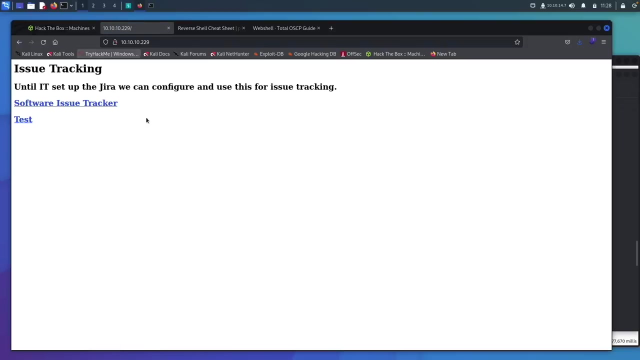 we have three ports open: port 22, which is ssh, port 80, http, and then we have my sql running on 3306. so the first thing to do is just come out to the http server and see what is here, and it tells us that we have. it says there's an issue tracking. until it's set up, we can. 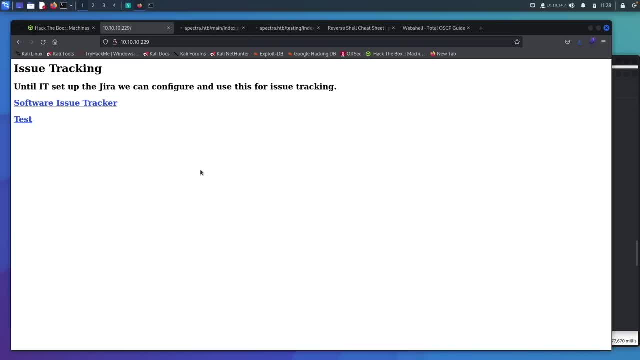 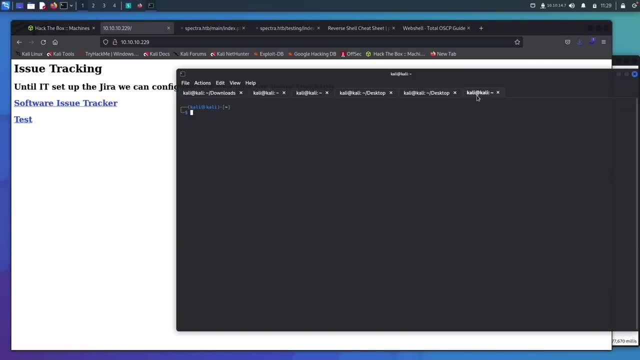 check out these links right here and see if they take us anywhere. and it tells us right here it's taking us to spectrahtb. so we probably need to add this to our host file so we can sudo g edit, sudo g edit our etsy host and now that that's added we can try and come back here and see if. 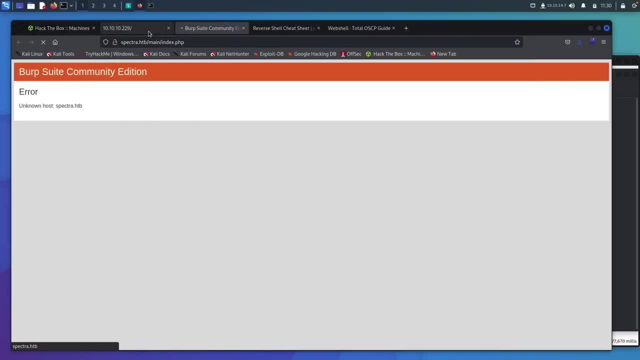 this will load for us and go and see if we get anything different this time, and it looks like it's working. i must have spelled it wrong, so it tells us there's an error establishing a connection, a database connection. so that doesn't work. did we test this one? and we get a wordpress site right here, and this is a basic. 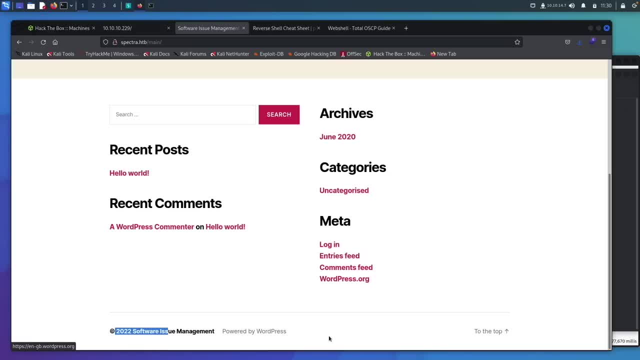 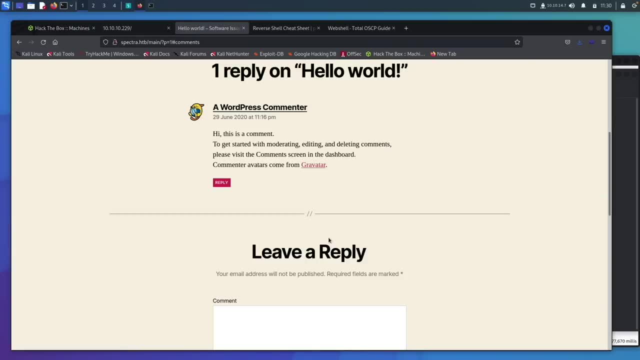 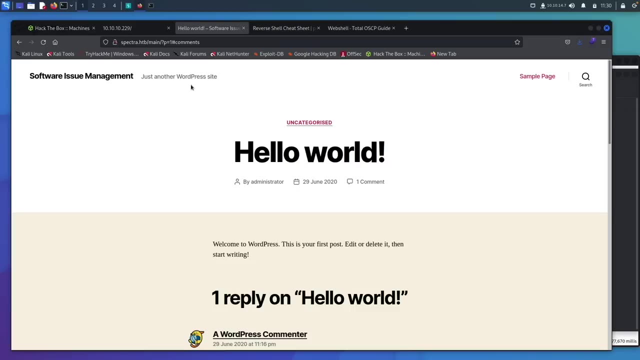 wordpress site. we are told that it is up to date. it's powered by wordpress and one of the things to look at is there is a user which would be administrator. see who commented and we don't have anything. it just says a wordpress commentator. so there's probably not another user there we have. 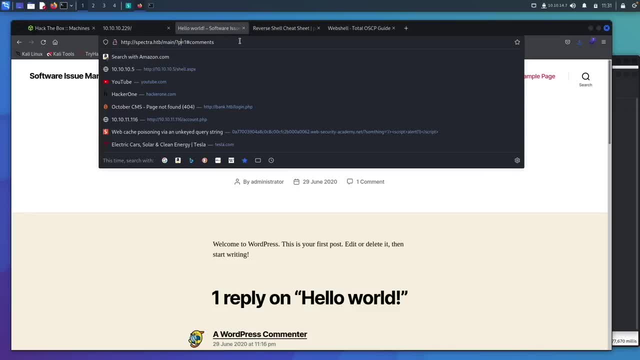 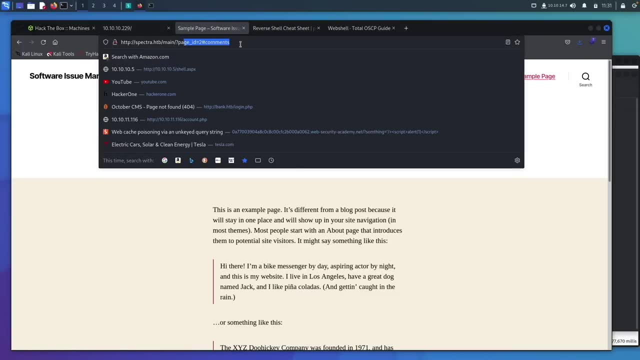 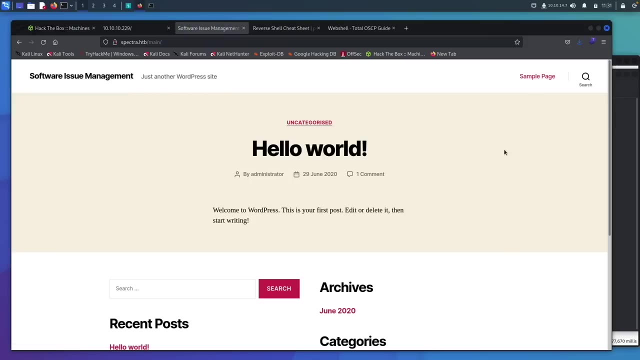 this right here: this p1- uh, it looks like that could potentially be different users, so you could come up here and just try and enumerate this. it'd be easier to send this over to burp and try and do this now. it says we have page ids. we can look for different pages, but i'm not going to run down this road just yet. 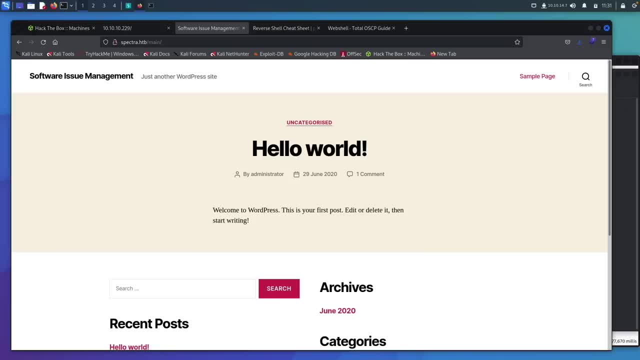 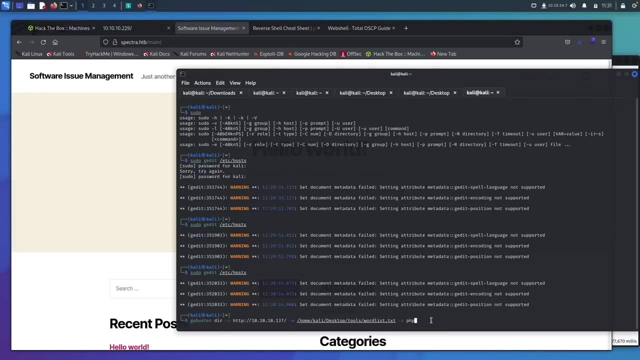 while we're on a wordpress page, one of the best things to do really on any kind of page is to fuzz it. so we will do two different types of fuzzing. we will fuzz with the extension php because we are on a wordpress page, so we can come back over here and it is 229. 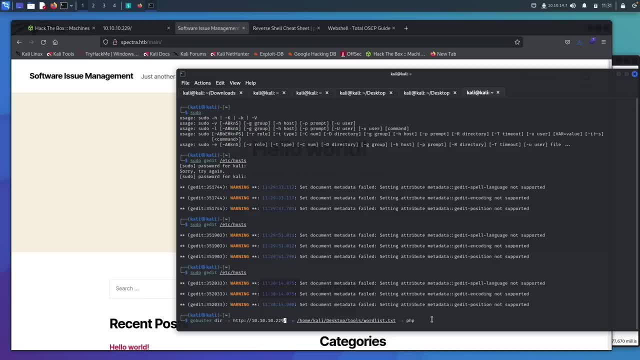 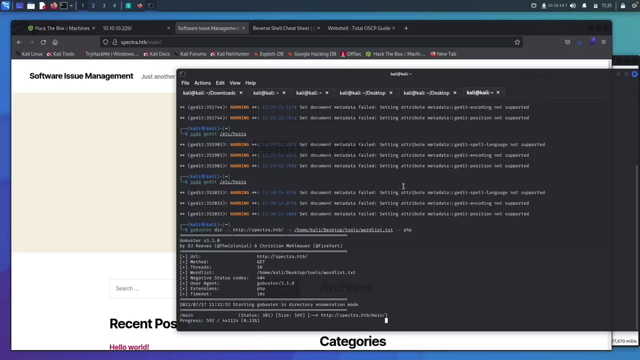 and we can run this. actually i'm not sure that will work because we are on a virtual host. we'll go sp e, spectra dot, htb and see if that fuzzes and it says that that's working. so we have this main and then also i want to run fuf and see if we can. 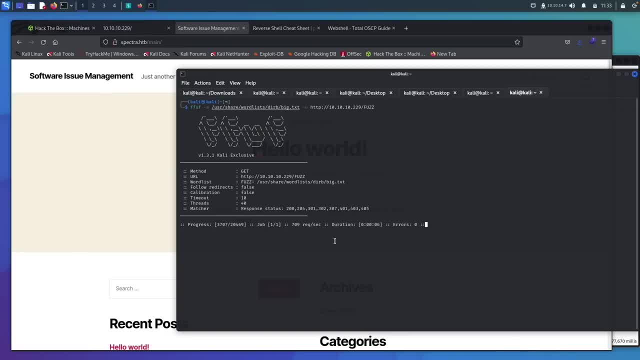 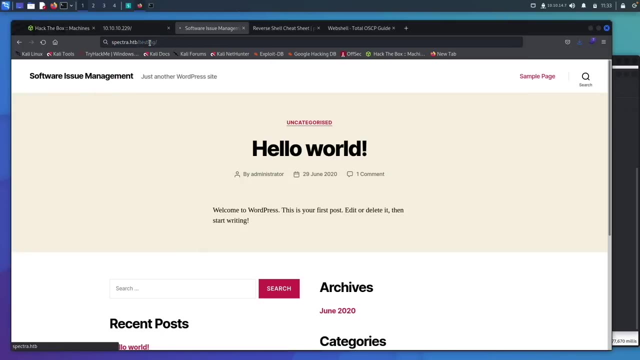 run anything else on this server. we actually want to run this on spectra dot htb and we've pulled down main and testing so we can come over here and we can just type in testing and we are brought to a bunch of files. we've already been to indexphp, one of the things you 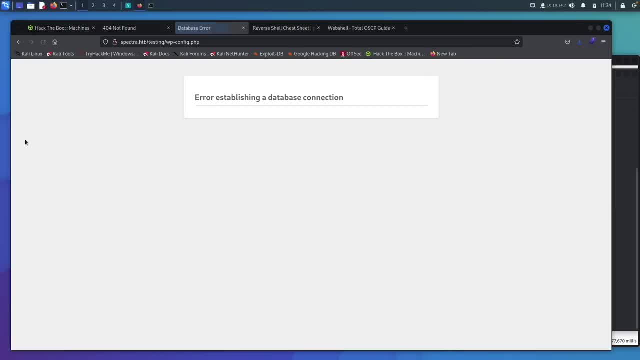 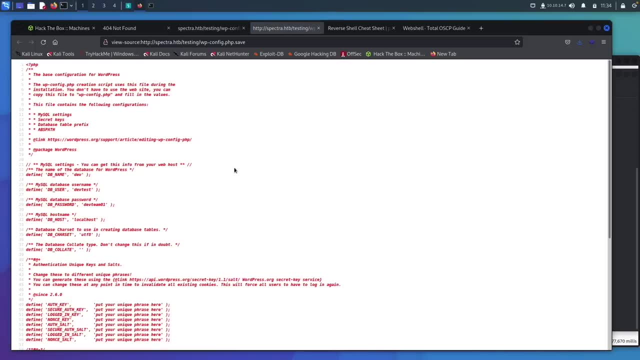 should always check for when you come to a page like this. when you see these config files, config- very yummy place to search for vulnerabilities, we can use page source. we know that when we see a blank page that there might be some hidden files. and over here we see we have a database user and 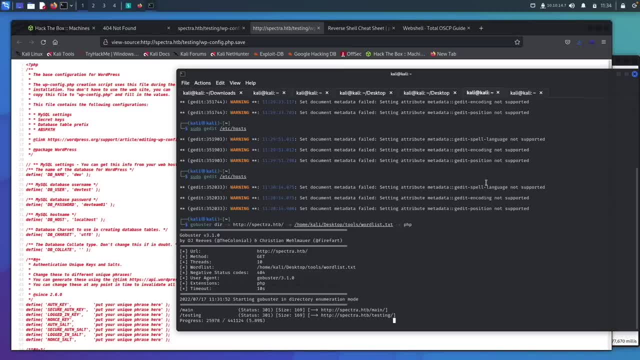 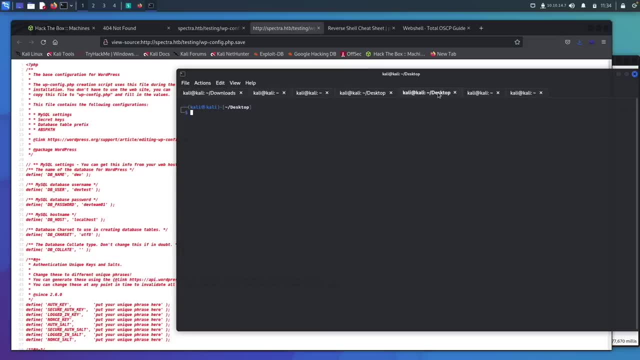 we have the database username. now we saw that on this in-map scan the mysql was open and you could try to log into mysql and the way we would go about this is typing in my sql and we'll put in the host: 10, 10, 10, 2, 2, 9, and then the username was right here: dev test. so we would go dev test. 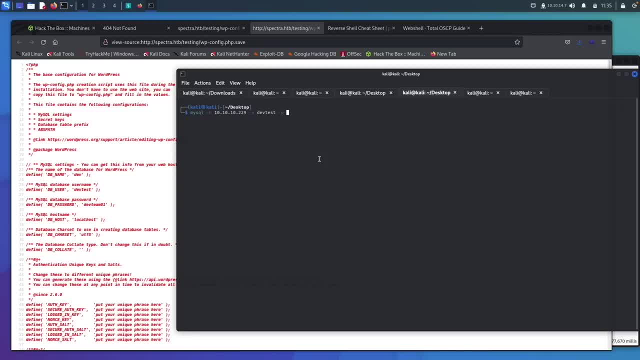 and then we could for our password and then see what happens. like this: we can copy paste and see if it will let us log in and it tells us we're not allowed to log in and it looks like it's because of our ip address here is not allowed to log in, which is fine. you probably have to be. 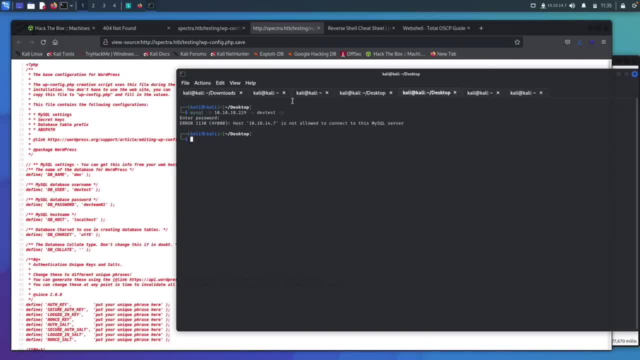 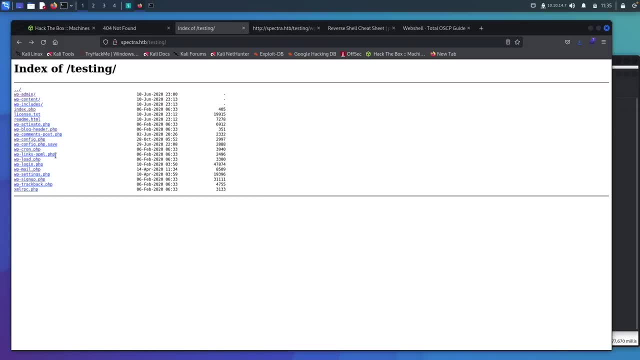 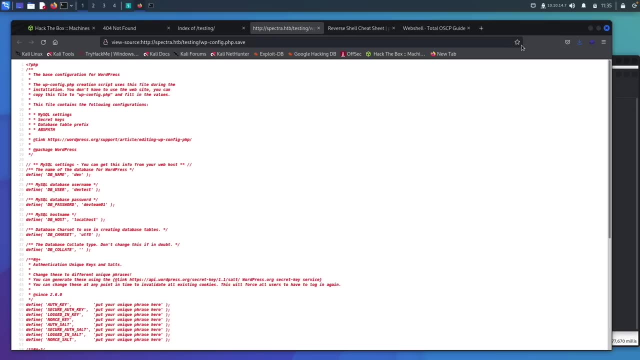 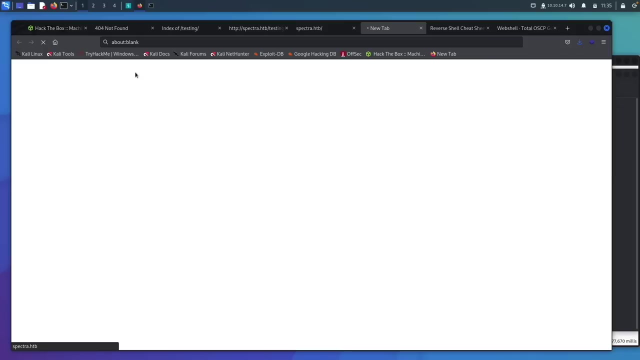 running on the local machine to log in. so what we can do is we can actually come back to this page right here and we see that your, the admin, is allowed to log in. so we have a wp admin, so we can open a new file type in spectrahtp. come back over. 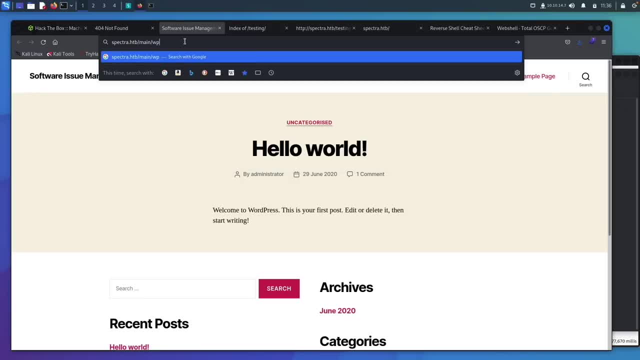 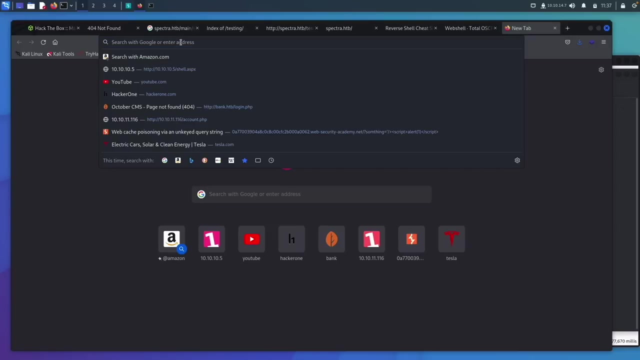 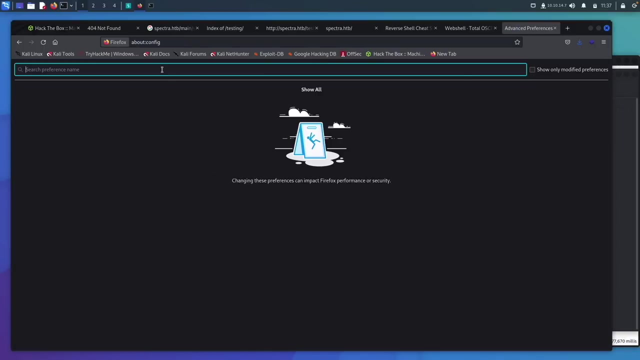 here we can try and log in with the wordpress dash admin and that keeps sending me to, and every time we type in this wp slash admin, it keeps sending us to google. so we're going to turn this off. we're going to come over here and say about config, accept the risk and we're going to go. 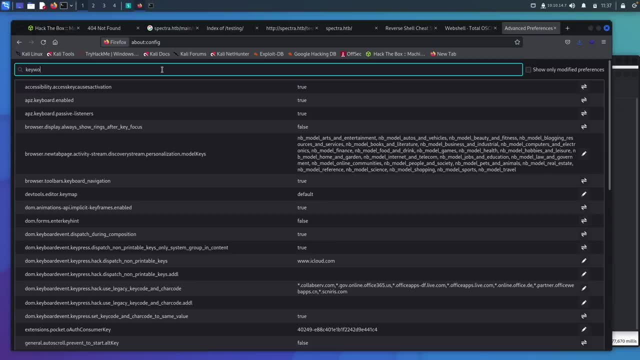 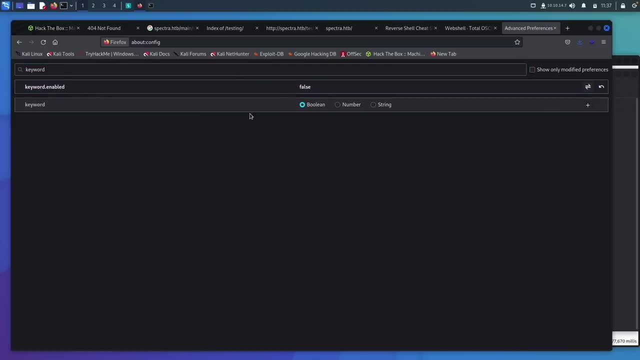 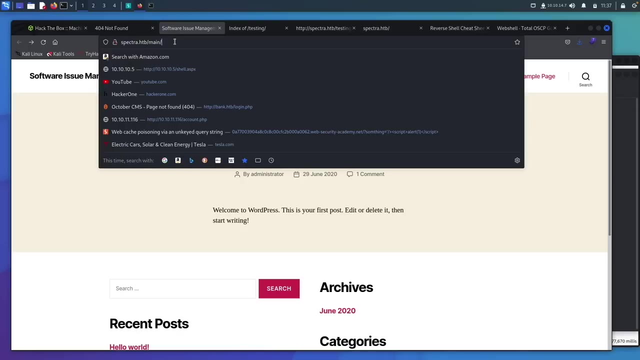 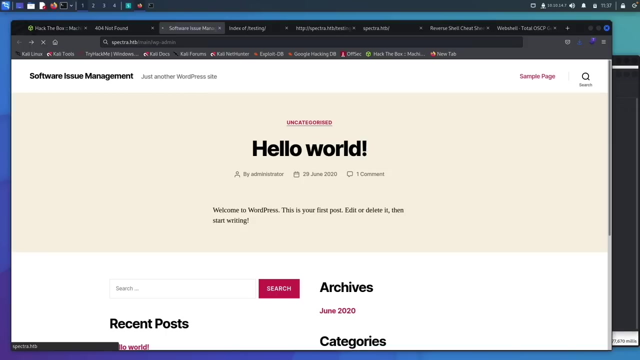 a keyword and we're going to set this to false. now. that should be saved and close out of it. now, if we come back and we type this in, it should stay on track: wp admin and it loads for us now, if you remember, we saw- i think it was- administrator. 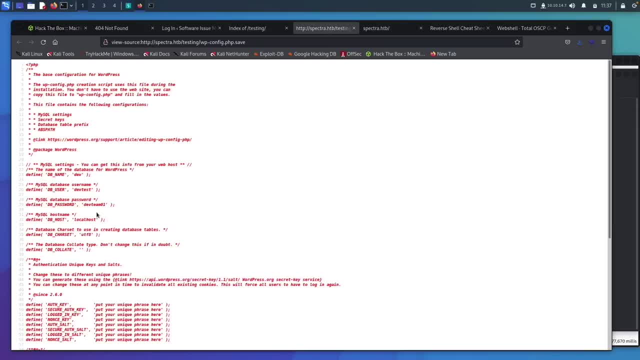 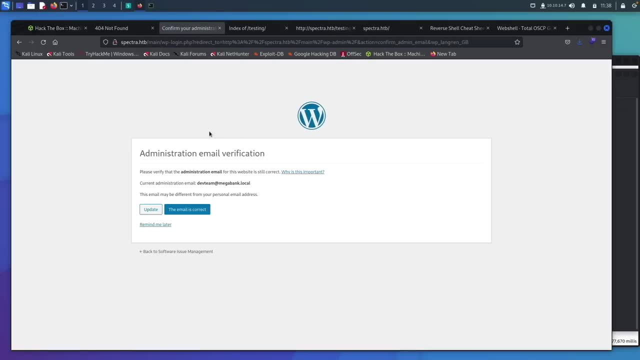 like this, and then we can grab this password and see if maybe this person is reusing a password, the website if different, but har chloro, the native people or something like that. so again we can use flash data itself. we can see here. we do access that itbr, you can do. 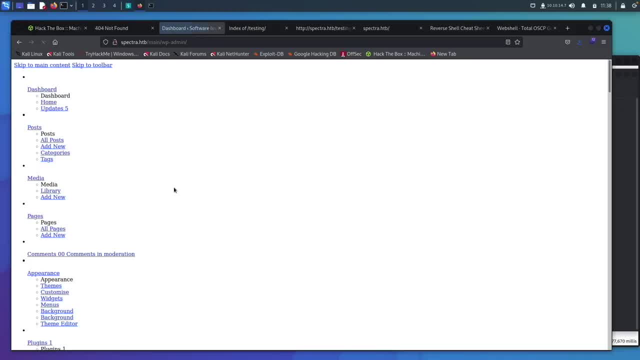 things in plain text so it doesn't load very pretty. we're just going to go ahead and nothing else that weologists have to do here. since we've extended them to emptiness, we'll just mount this here and we'll just massage 엄청. 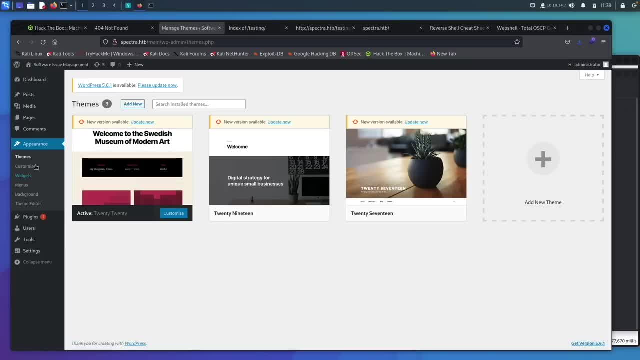 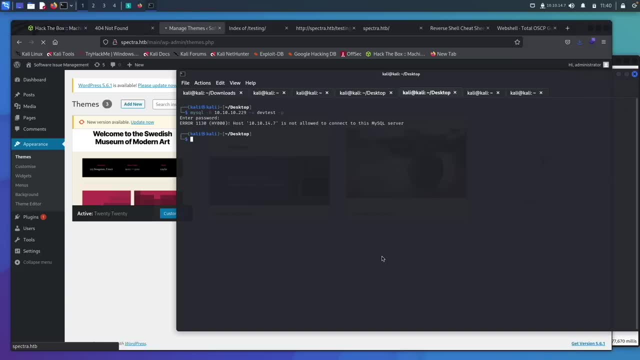 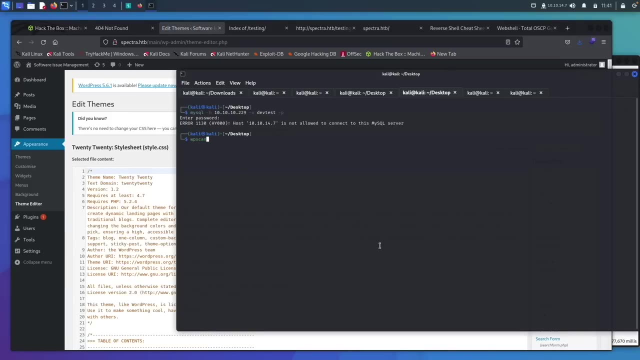 to load for us and it loads for us and now we can come to. while that loads, there is one thing that you should always look to run on wordpress sites- what on wordpress sites? and that is a wp scan. so we can go wp scan and then we would run dash, dash url and then on this box we would run. 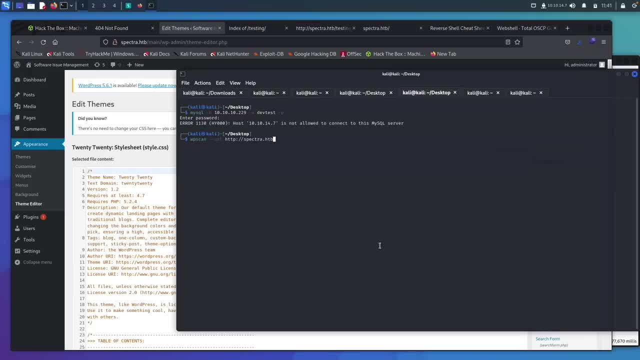 on the box name and the page was main. so this is going to look for the plugins, because sometimes there are vulnerable plugins on these wordpress boxes, especially if they don't update them. so it would look like this aggressive dash enumerate and then we want all plugins. so 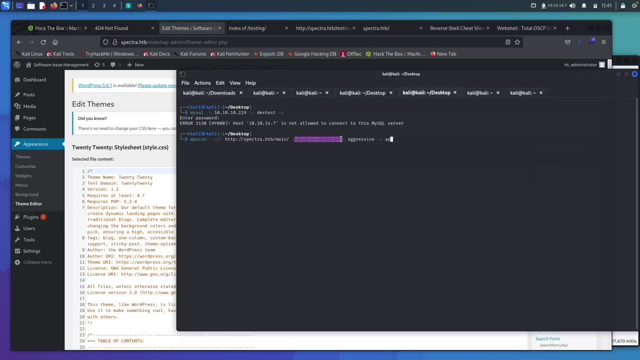 if we were to run this, it would look like this, and the reason you would need to run this plugins detection aggressive is because we want it to enumerate all the plugins, not just the ones that it finds in the source code. So if you're ever up against WordPress box, especially in a CTF- 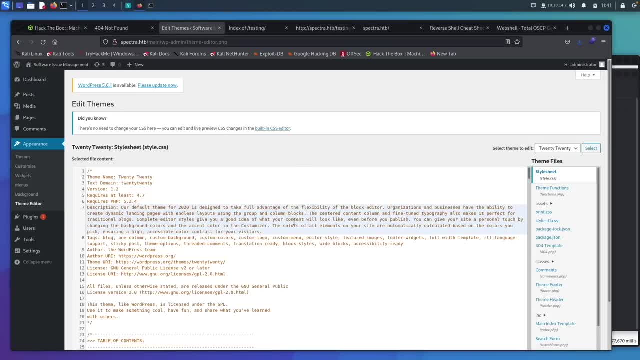 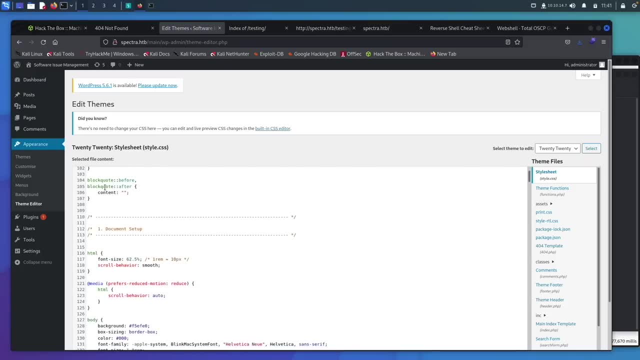 this is something you would want to run. But now that this has loaded, we can come over to our themes and look inside of the PHP code, right here inside the 404 templatephp, and we can actually add in a reverse shell right here. 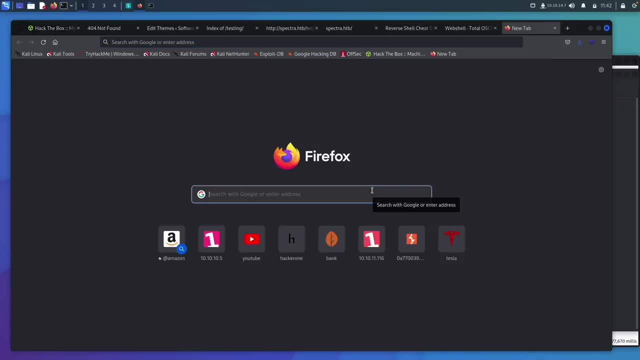 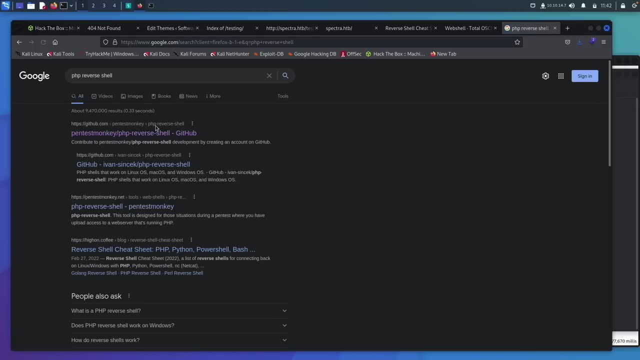 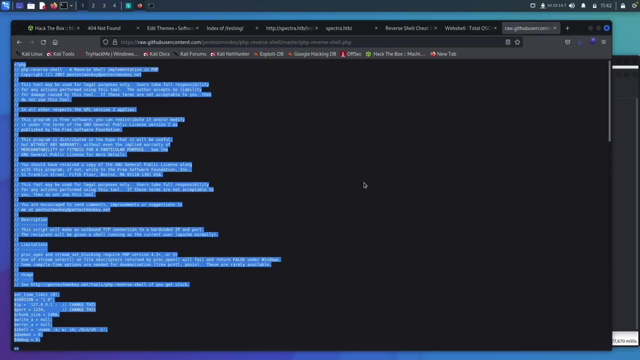 So we've seen this earlier in the course. We can go PHP reverse shell and then we can find Pentest Monkey and just grab this entire shell and we can just edit the IP address and the port number. So we'll go to the reverse shell. go raw: command A, command C. 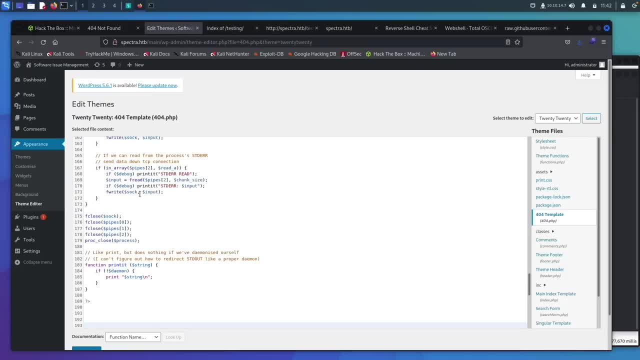 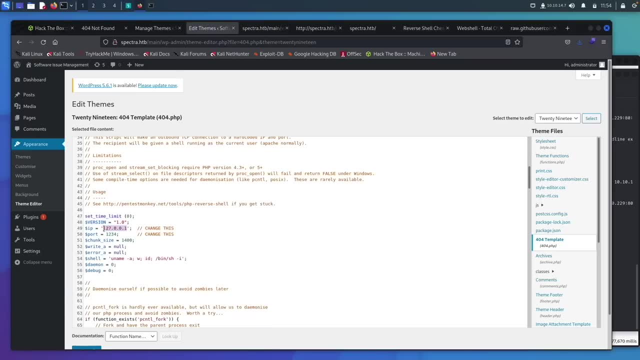 come back to this spot where we were. We can just paste all of that in: Come back, Come back, Come all the way up to the top. Change our IP address to 10.10.14.7, and we'll listen on port 4444. 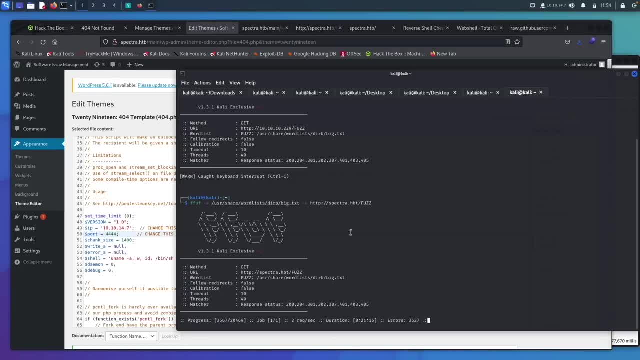 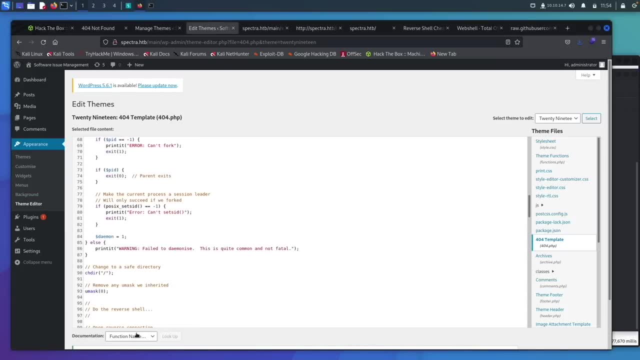 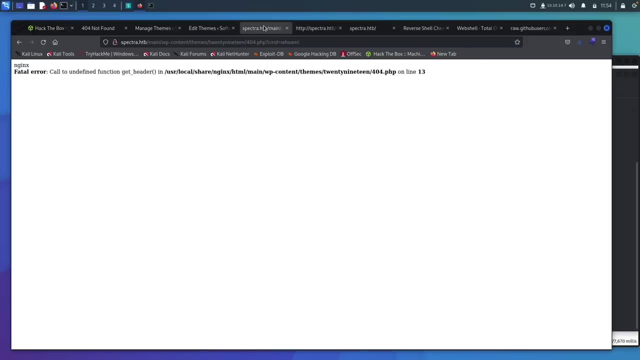 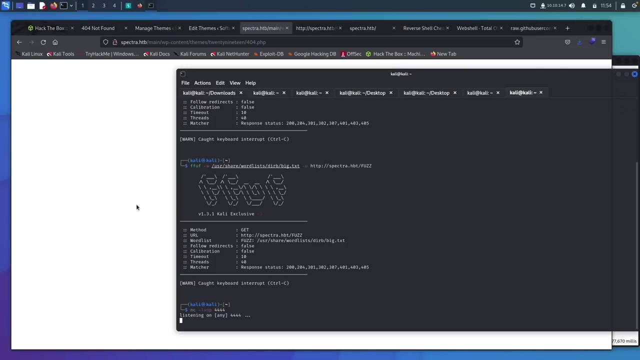 We can update this. Make sure we have – see if we can start up a Netcat listener Listening and it tells us this right here updated successfully So we can come back to whatever page. that was This one right here. Now, if we delete this and we just run this, it should execute that code for us that we just saved. 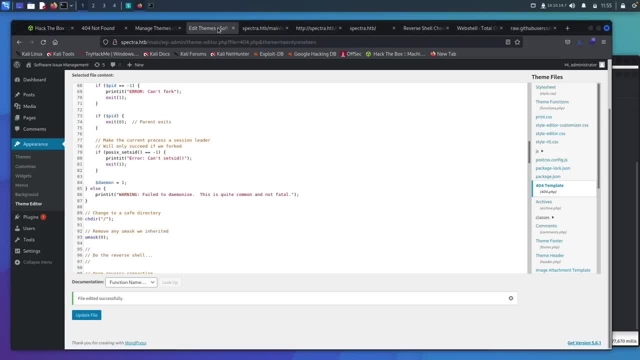 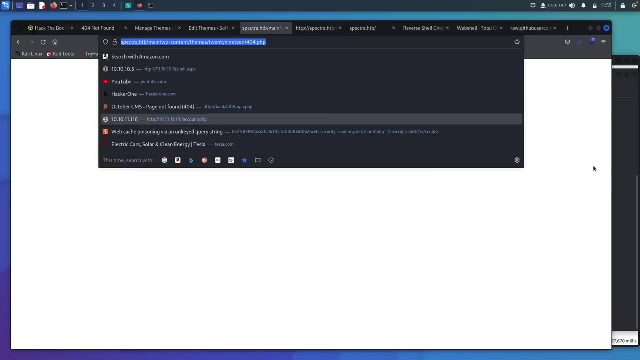 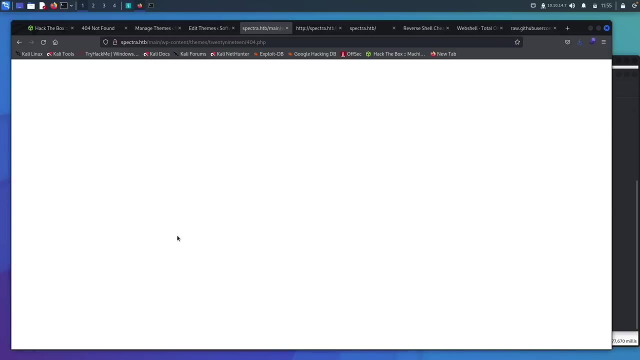 It says that it has updated successfully. Make sure we have the port and IP number right. It is, It is, And we got the reverse shell back Over here. So who am I? And we are finally on this box. Sorry for a bit of the workaround, but this is just really the life of doing any kind of hacking. 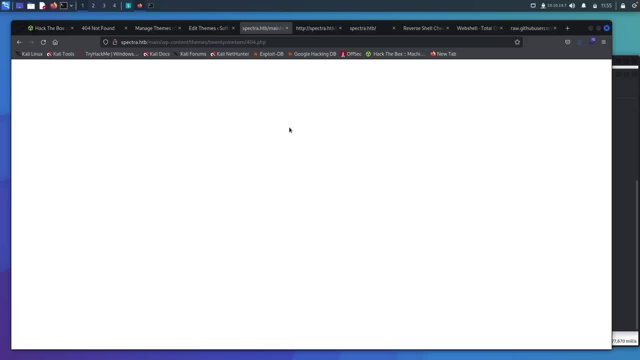 It is going to be a lot of trial and error and fixing mistakes. So this is WordPress. So these were a couple of WordPress boxes. You're going to see WordPress in the future. especially in the world of bug bounty hunting, WordPress is really popular. 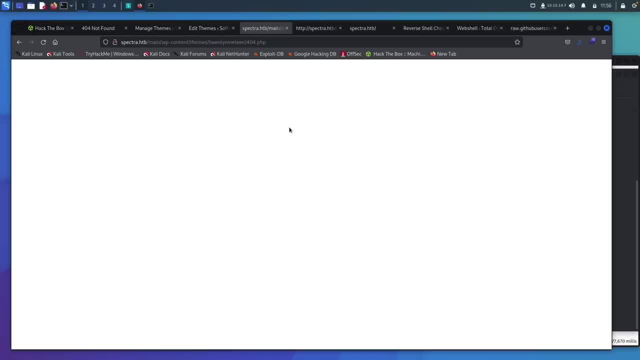 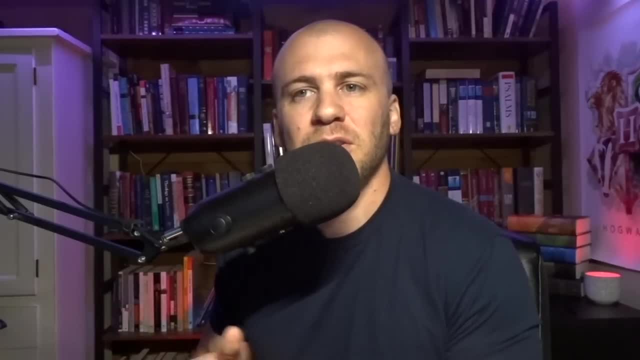 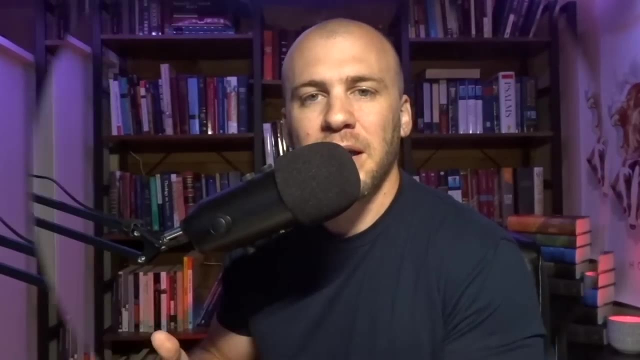 And this is just a few different ways to go about Hacking WordPress sites. So with that, we will continue on. Comes next is usually the question of what kind of programming Do I need to know? So in this video, what we're going to cover is the Python that I think you need to know as you're entering into cybersecurity. 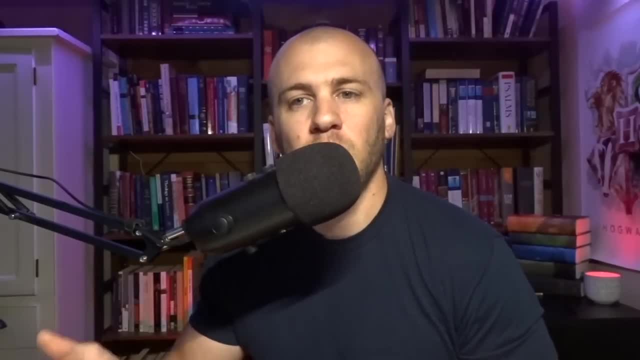 This is an introductory course into Python for the purpose of cybersecurity. I have tried to keep it as streamline as possible to keep you away from having to watch a six hour course course on Python for cybersecurity that is just full of stuff that I think you're not really. 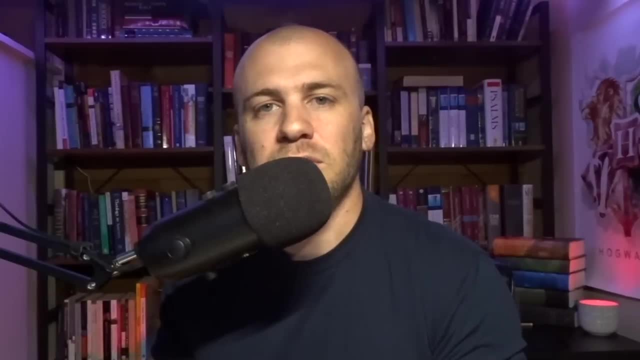 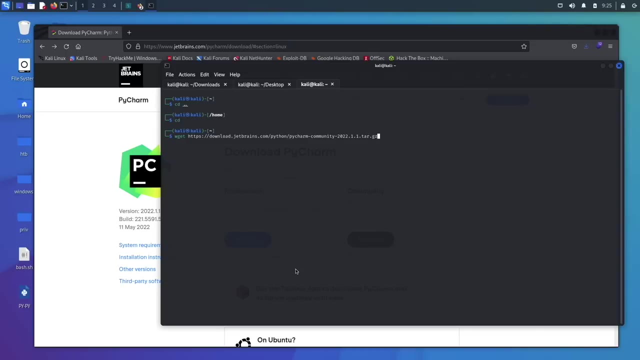 going to need in the future. So this is a beginner course And if you have any questions, as you're going through it, please leave some questions down in the comments. I decided to go ahead and show you guys how to install PyCharm on your Linux VM. If you have a Mac or Windows, it's. 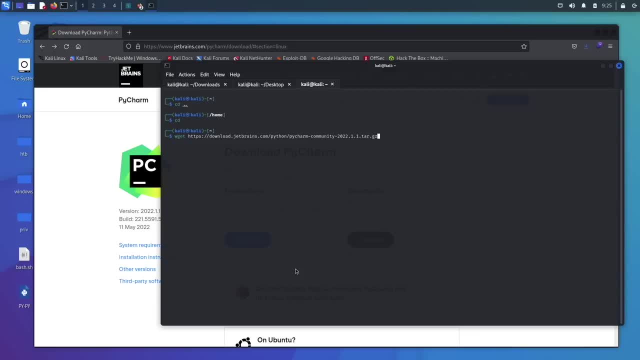 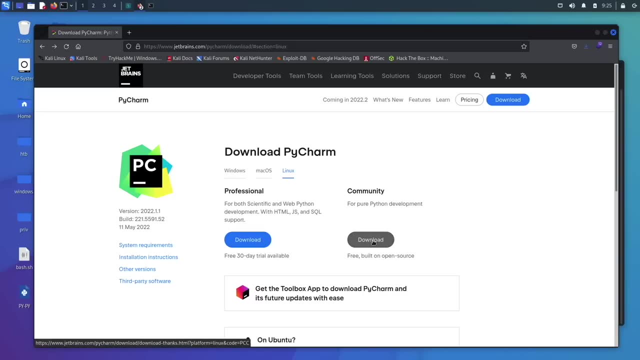 really straightforward. You just go to the JetBrains, you download PyCharm. I'll have this link in the description and you'll click Windows, Mac or Linux And then you'll just hit download and it will automatically start to download, unless you're on Linux. So I have had to do this for 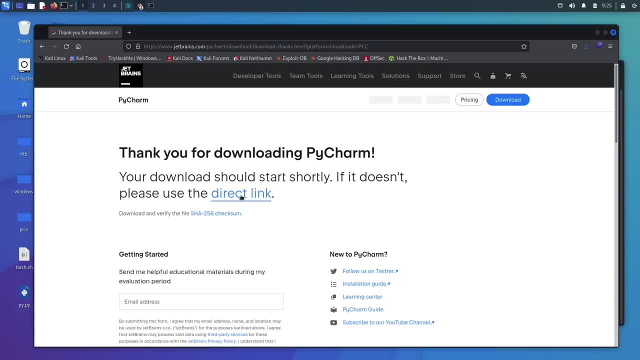 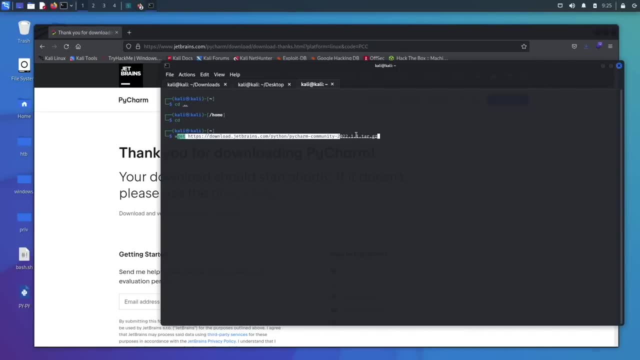 several virtual machines that I've had, It won't download, And so what you have to do is right click the direct link and you'll copy link. Then you will go to your terminal and you'll run a wget wherever you want this file to be saved. So if you want its own PyCharm folder, put it in its 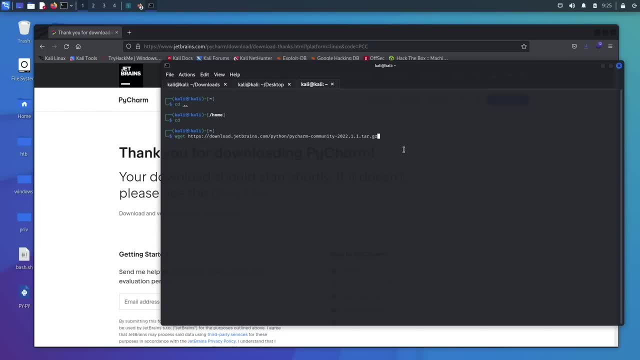 own PyCharm folder For me. it is in my downloads and you can save it wherever you want. You'll hit enter- This might take a little bit, depending on your speed, that you your internet speed- And then you're going to unzip it wherever you downloaded it with this command right here, And then it will unzip a bunch. 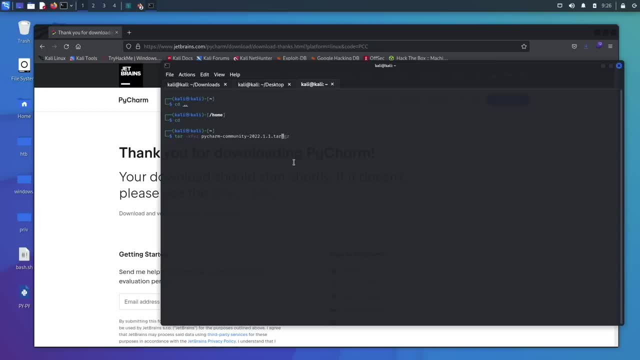 of files will come out and then you will be able to CD into the folder. So for me I will CD into my downloads, because that's where it is, And then I'll go into PyCharm And then I'll LS inside here and I'll go into my bin, And then this is the executable I want to. 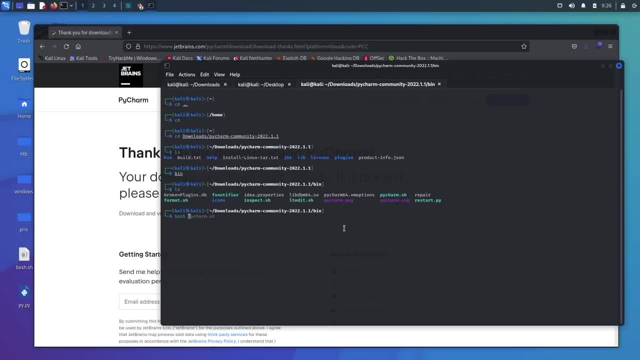 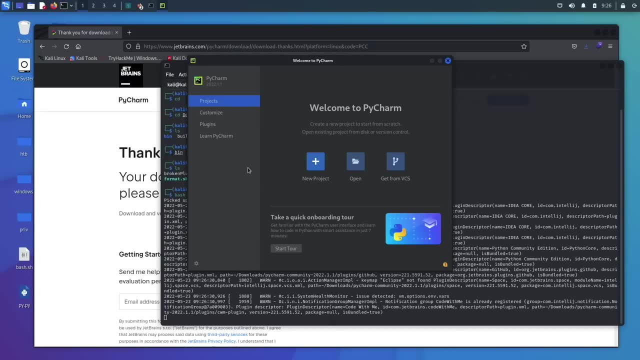 launch in order to launch PyCharm. So I will type in bash and then I will type in PyCharmsh and it will automatically launch PyCharm for me. So this is how you get PyCharm on Linux, If you are wanting. 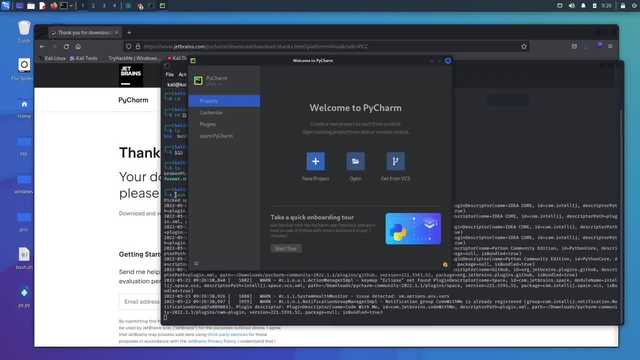 it on your Linux. I usually write everything on my Mac And then, if I need to run the code over on Linux, I will pull it over To my Linux machine and run it over here. So with that we will get started in the next section. 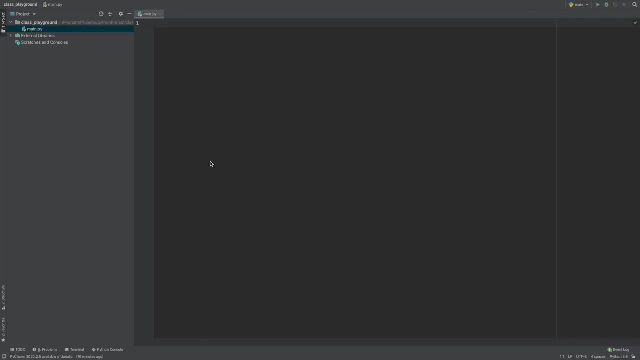 All right, we are ready to start our Python course, So we're going to start out very simply with a string. A string is a sentence that is a data type, So we're going to have several different data types coming up, but a string looks very simple. It is what I think of as a sentence in. 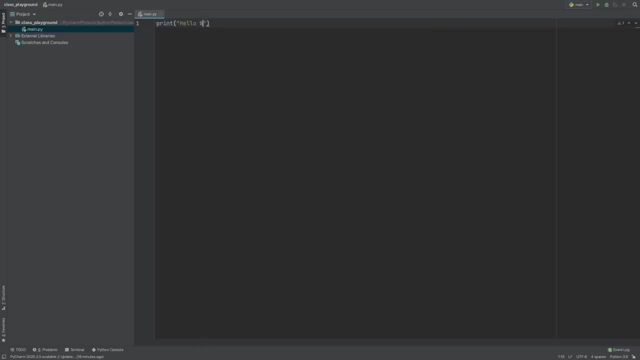 English. So you just have hello world. A string is always going to be stored inside of quotations, So if we were to print this, it would print right here: Hello world for us. And if we change it, it's going to change along with us. So this is really simply. this is a string and we can store. 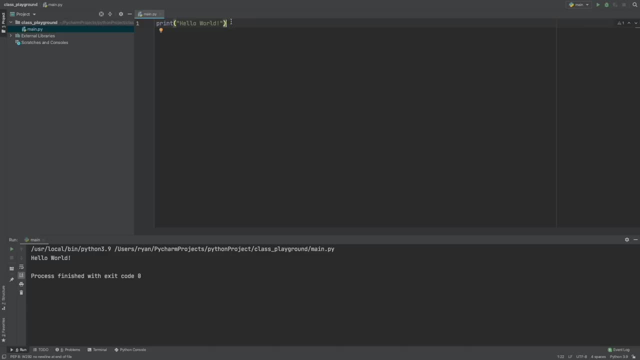 strings inside variables, which is going to be coming up in the next section. But first, before we go on, you will see sometimes that you need a string on a new line, especially if you're going to export something into a CSV file you're going to want. 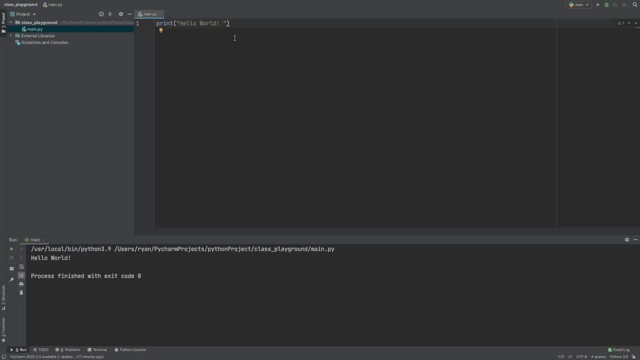 things on new lines And at the end of your string you can type something like this and then say hello world number two. And then we can print this and we have hello world and hello world number two. And if I wanted to get rid of that space, I would do it this way. So we have hello world and hello. 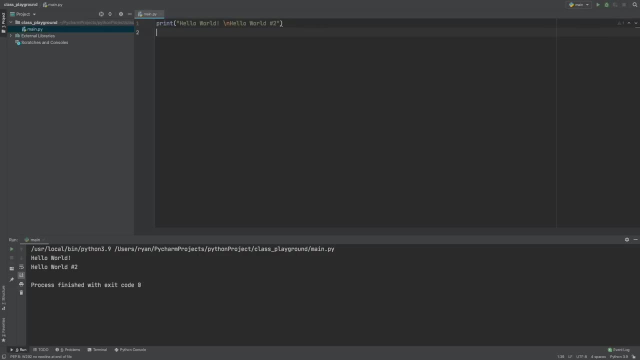 world number two. Another way to go about printing this would be like this: So print, print, and then we put our quotations and we say hello, And then we can add this like this: Hello world, Just like that. And now, if we were to print it, we have hello world, Hello world number two. And 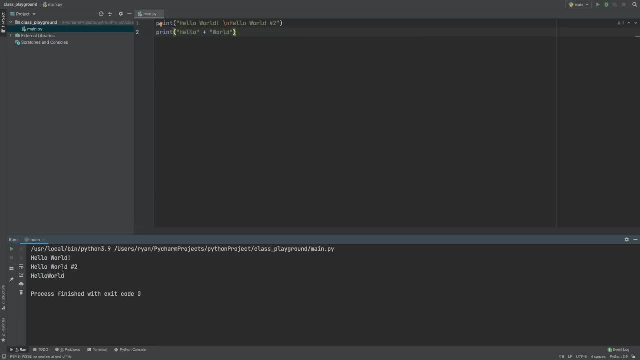 then, hello world, You see how there's no space right here. This is something that I run into regularly, and I just had happened the other day. There's two different ways you can put a space right here, And I'm going to show you the easiest way. first is just to add a space right there. 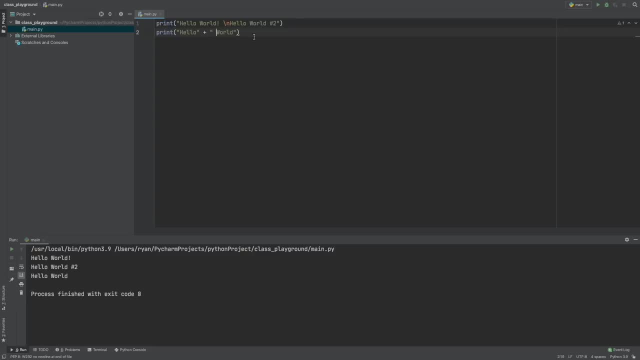 rerun it And now you have a space. But I think it's helpful to know more than one way to do this So you can add another quotation and a space in there and add another plus sign. so you can run it this way and you still have that space. 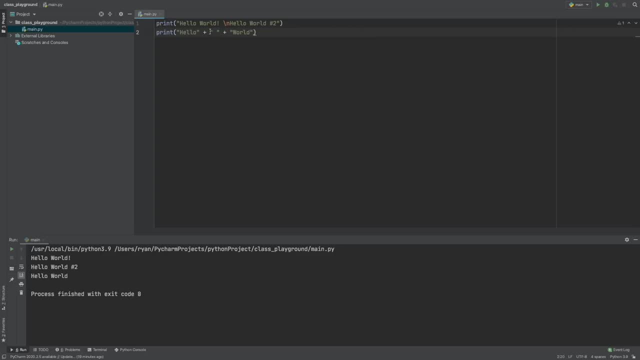 and it's really important to know this right here, because sometimes you'll be running a for loop and everything is just smashed together and you want a space in there and you can add spaces simply just by doing this. so what I'm showing you right now you may be thinking this is not ever going to be. 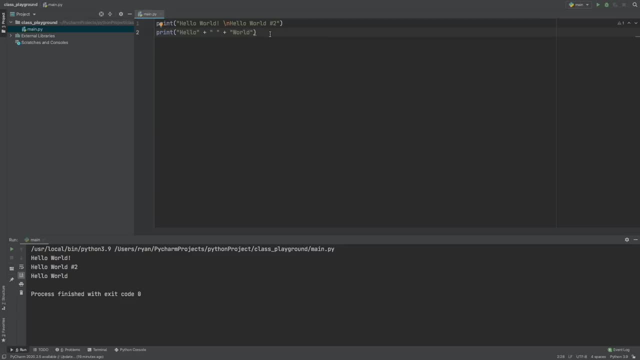 helpful and I wouldn't be showing it to you if this wasn't helpful, and it's something you're going to run into in the future. so this is a very streamlined course and I'm showing you just what you need to know in the world of cyber security. now we're going to be covering something called 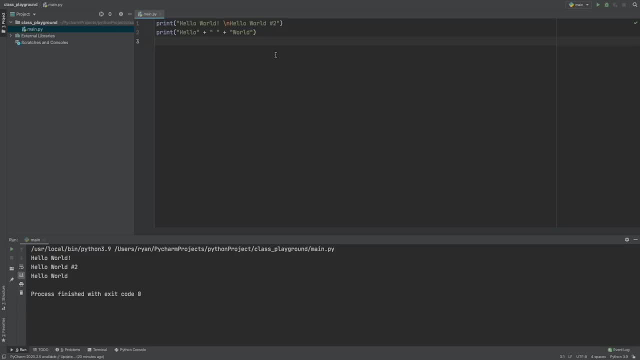 a variable, and a variable holds the place of some kind of data that we're going to want to use later. so we'll go ahead and comment this out, and on a mac it is command and then question mark, and so we'll comment that out. so now, if we run our program, there's no output and we're going to look. 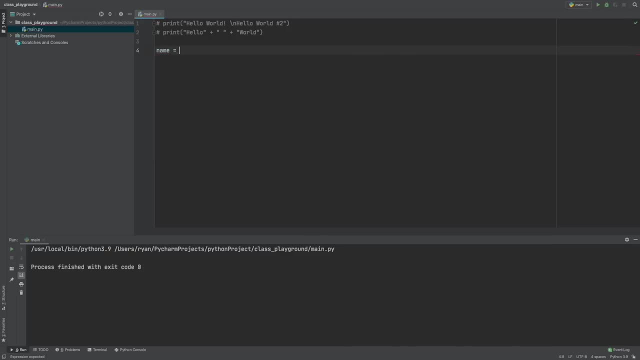 at a variable. so a variable can be something like this name and then the name Jim. this name is going to hold whatever is right here. so this is our variable which is going to represent the name Jim. so if we come down here and we print and then we type in name and then we run this, it's going to 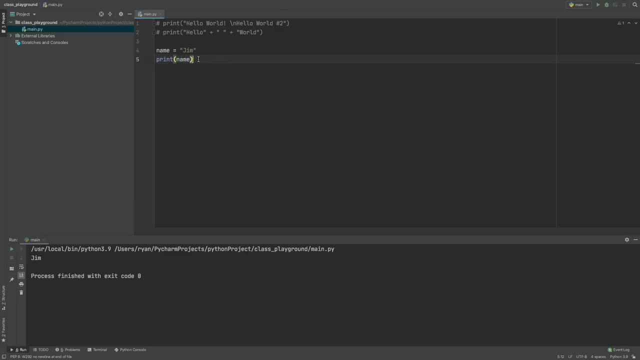 print what is stored inside of the program and then we're going to print what is stored inside this variable. when we look at variables, one of the things you're going to want to be able to do- especially in the world of cybersecurity, if you ever want to write your own tool- is you're going. 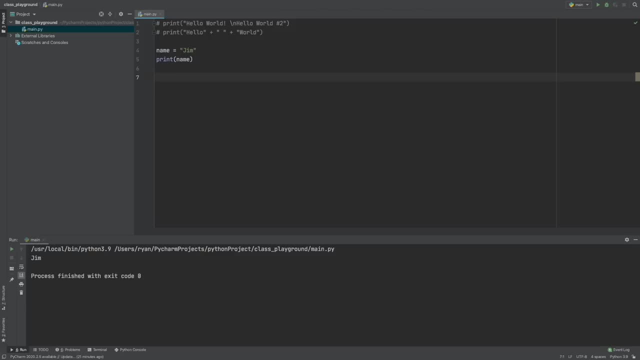 to be saving variables, only they're going to be input variables. so if we were to go like this and we say name equals input, and then we type what is your name, and then we'll want to space right here and then we'll print name. so we're going to print the variable, whatever the user inputs here. so now, 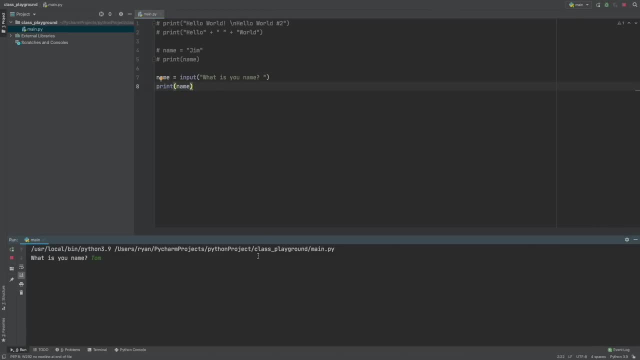 we can say what is your name and we can say Tom, and when we hit enter, it prints Tom. and there's something else that's really cool that I use all the time. it's called an F string and what you do is you add an F at the beginning of your string, but you can print. 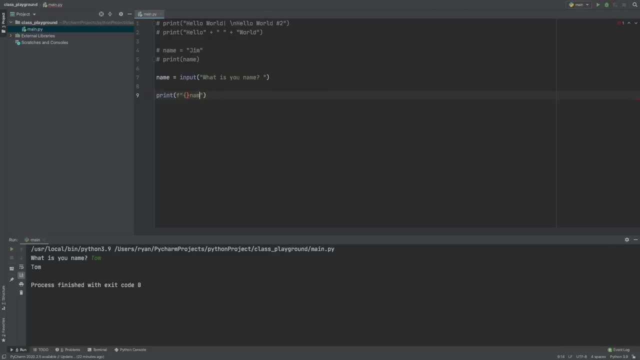 variables inside your string. so we'll go ahead and put name inside here and so we can say hello, and then the name. so we'll say: run this, what is your name, Tim, and it puts out: hello, Tim. so this is an F string. this is something you're going to want to know. this is something I use. 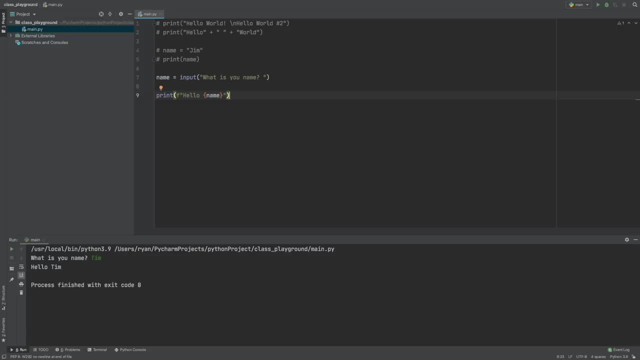 all the time and in the next coming up videos we're going to look at data types and how we can pull information out of a specific string, and this comes becomes really useful whenever you run a script on a victim machine or on your target machine or your target server. you'll you. 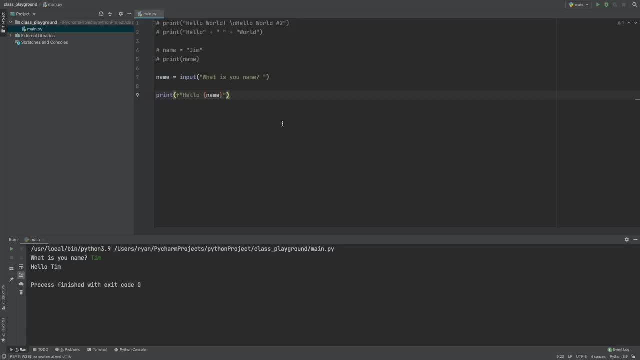 may get a lot of output that you don't really need, and this is a good way to start extracting data, so we'll start that here in just a moment. okay, it is time to draw out some information from our string, so what we can do here is we can save a variable and we'll call this variable name and. 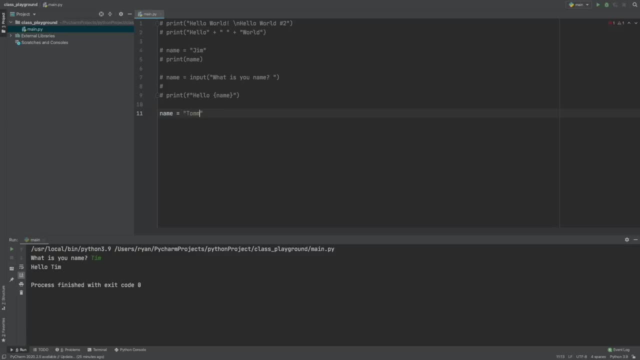 we can put inside of our name Tommy. so we have Tommy here and let's say we want to grab just this M right here. what we can do with this is we can say print, we want to print our name, and then we can go to the square brackets just like this, and when you're running python, it always starts. 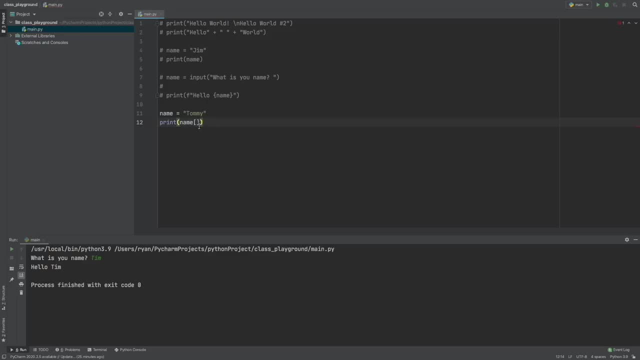 at zero. so it goes zero one, two, and so that first M is going to be two, just like this. and so if we run this, it's going to print that M for us and just to show you, if we want to print the T, we would enter a zero here, and this is one of the most basic ways to draw out information, and it's 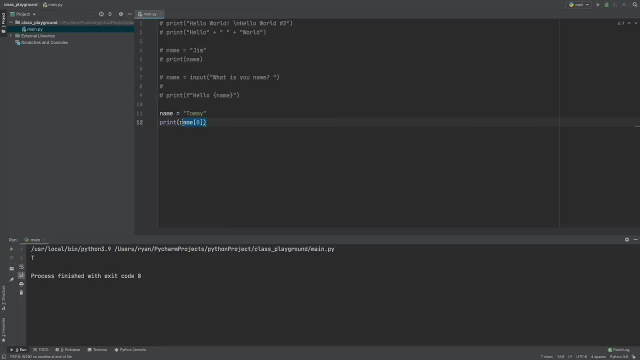 going to get a lot more complex as we go, but this is what the square brackets do. when you see them and when we start to the lists and arrays, these square brackets become a really useful tool to remember. so, as we continue to go through this, I want to pause right here and I want you to go ahead and play around in your own. 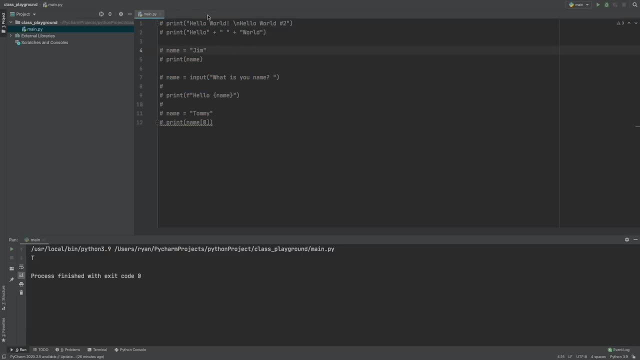 text editor and print some, make some print statements, make them on new lines, add in some spaces, make some inputs and actually practice gathering information and maybe have two or three inputs and have it print things back and forth and you have a little conversation with your text editor. so I want to go ahead and give you this challenge for you to go. 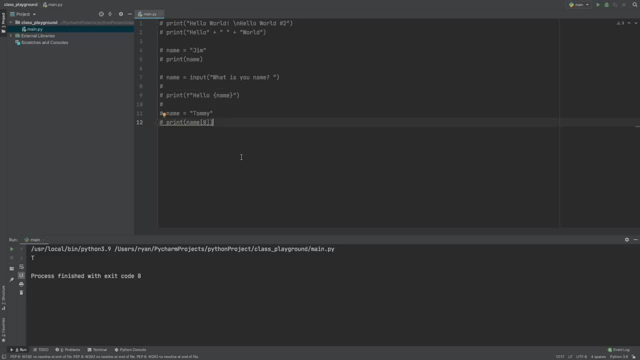 ahead and play around with the things you've learned so far and try and really ingrain this information into your mind. these are the foundations of python programming and you need to know and understand how they work. you're going to notice is you can name variables whatever. 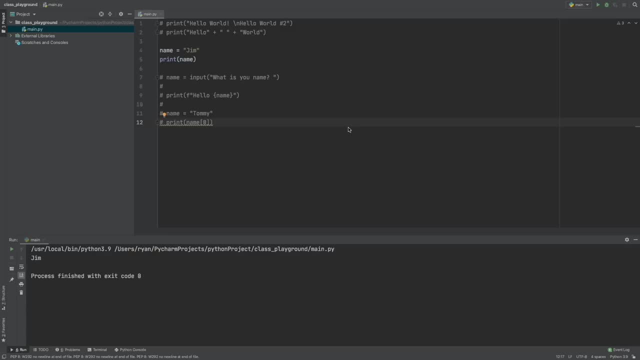 you want, and I name my variables really poorly, mostly because the programs I write I write for myself and I am not working with a team of developers. but maybe you will someday and when you name your variables you can name them whatever you want and you'll want to make. 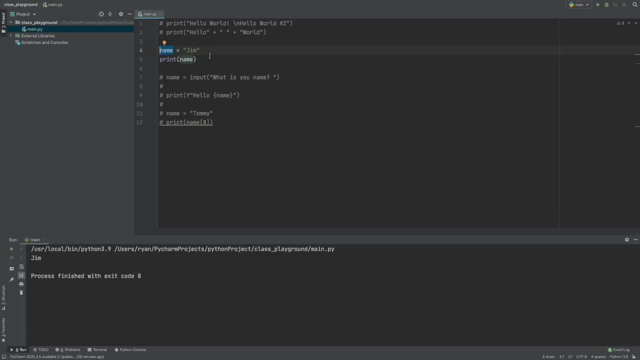 them names so other people can understand what is going on. so if you look at some of the code I've written in past videos, I do this right here. I name everything like this and it is not really the best way to go about naming these, so I'll name one guy, one and I'll go. 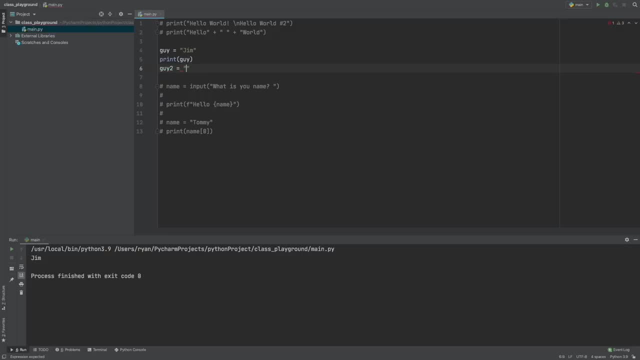 to guy two and he'll equal Bob, and then I'll come down here and I'll print guy two and then I run this and then I have Tim and Bob. you can, you can name variables whatever you want. literally, you can go whatever I want and you can make this a variable, and then you can come down. 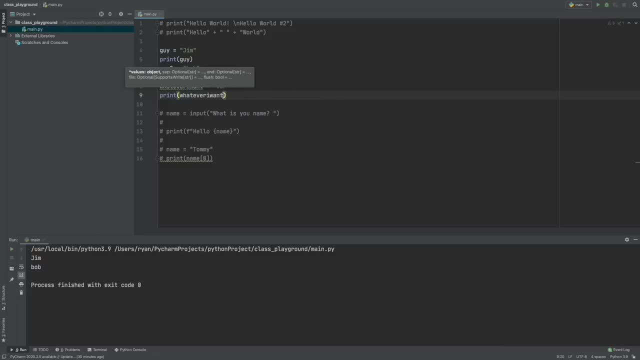 here and you can print whatever you want right there and you can name variables whatever you want. so I would recommend getting in a good habit of making your variables something that you can recognize. and it's a very bad habit that I have because I make my variables so that people cannot read what I have done. 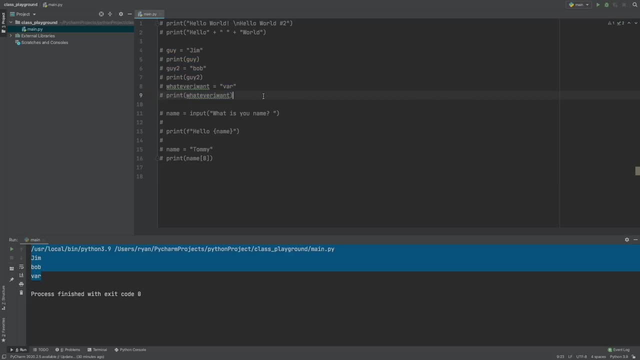 so this is something I'm trying to get better at- but I probably won't, because this is a bad habit that has formed over many years. but I want you to have a good habit of naming your variables, something that you can understand and other people's can understand, so, as you go through, 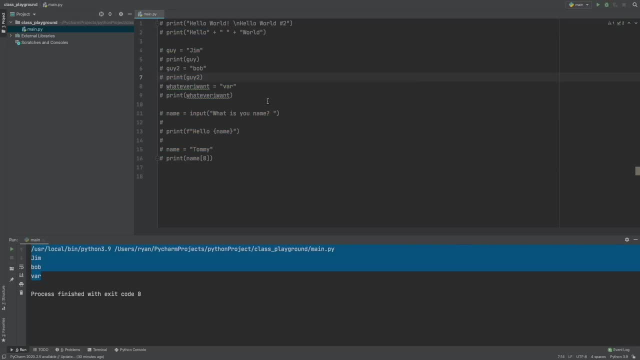 and work through your challenge. try to name your variables different, things that you will be able to understand in six months after you have written a program and you need to go back and edit it. okay, I have created this a little challenge here for you. if you want, you can go ahead and pause the. 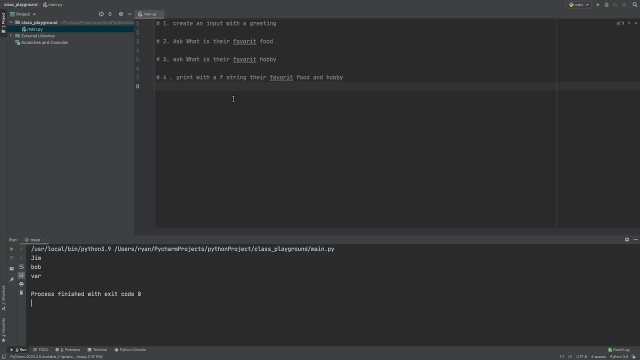 video and open up your text editor and see if you can create this little program right here. so we want to one. create an input with a greeting. so just say hello, what is your favorite food. let them put it in. and then take another input and say what is your favorite hobby and store. 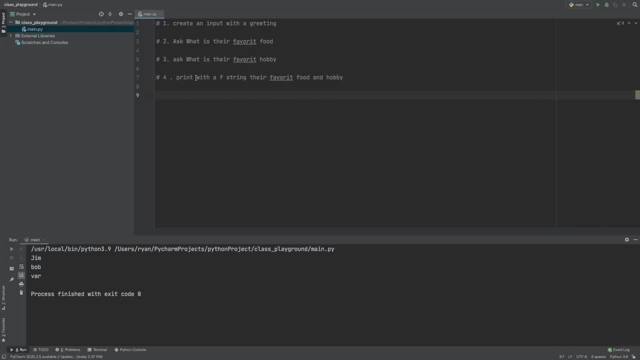 that also in a variable, and then we're going to print with an f-string their favorite food and their hobby. so if you want to give this a go, you can go ahead and give it a try. if not, we will start it now. so we're going to start out with: create an input with a greeting. 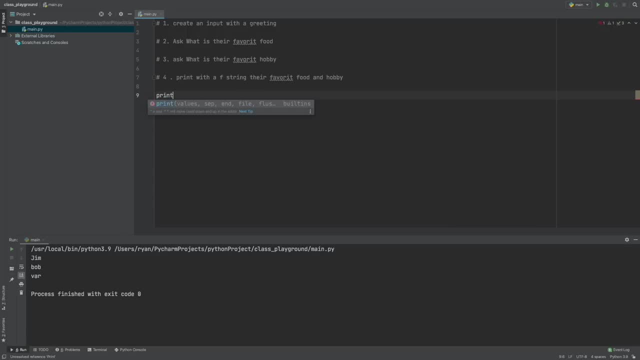 so we'll just say print hello and then we're going to take an input. but we got to save it as a variable. so we'll save this as food and it's going to equal and input and in we're inside the input, we're going to have the question: what is your favorite food? question mark space. I see that. 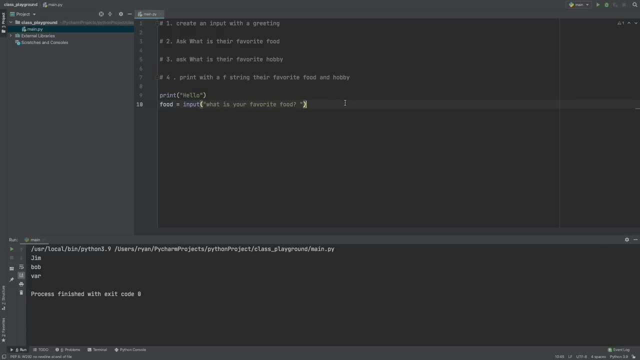 we have a typo here, all three, and then that's going to be saved as their food. then we're going to say input and this is going to be: we'll just save this as hobby. and we're going to take an input and we're going to say: what is your favorite hobby, question mark space. and then we're going to print with an f-string: 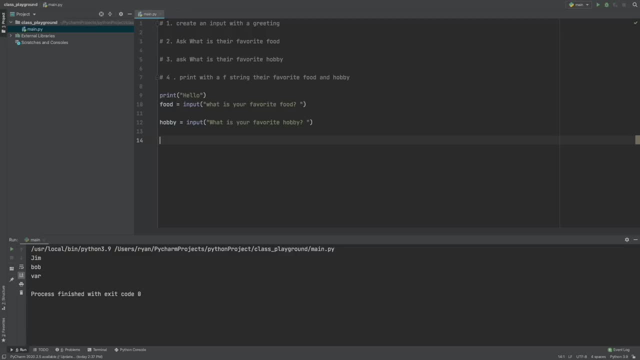 all of this together and we'll say: print your favorite food is. and then, if you remember, we need our f-string here and we should grab our curly braces and say: food and your favorite hobby is curly braces hobby. now, when we're done this, if we did everything right, it should print for us this final statement after: 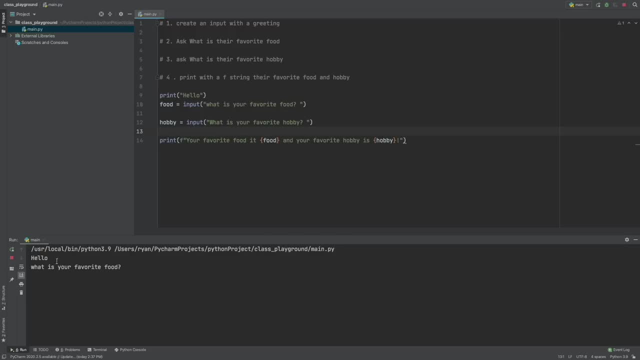 we give these inputs. so we say run and it says hello, what is your favorite food? and we'll just say chips. what is your favorite hobby- running? and it says your favorite food is chips and your favorite hobby is running. so this is a simple input form and it's going to print out with our 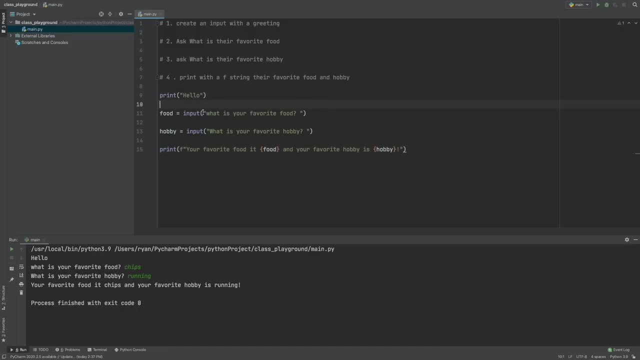 variables we have stored. and this is a good practice because when you write a program for a tool, maybe that you develop in the future, you are going to want to know how to do inputs, so that way you can take the input, save it in a variable and then later do something with it. so later on in the course I'm 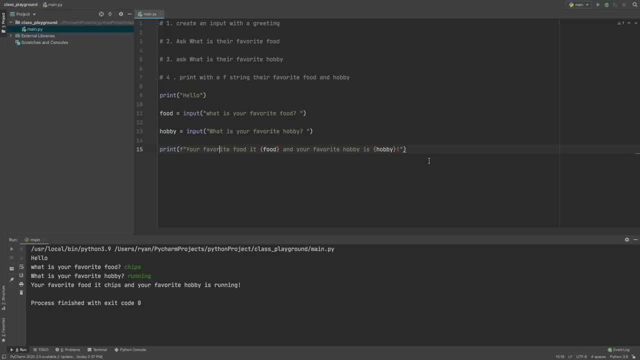 going to give you a practical example of taking input and then running it in a program. that is really helpful and I will cover that when we are ready for it. all right, so we have covered the string. so far, this integer is a whole number. so if we say int, we have a number of seven floats. we're not really going to use these a whole lot. 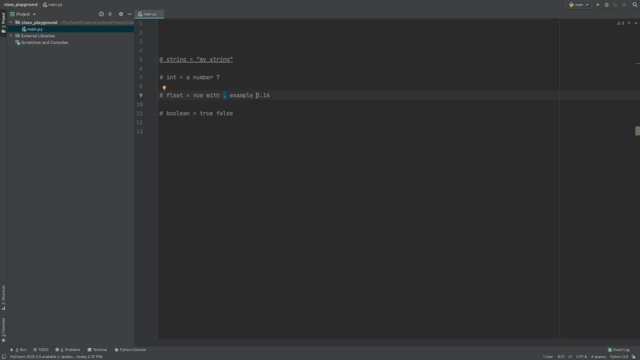 in the world of cyber security they have a point within the number, so 3.14 would be an example of a float. to date, I cannot remember a single time I have used a float in cyber security. usually that's more towards data science or something of that nature. 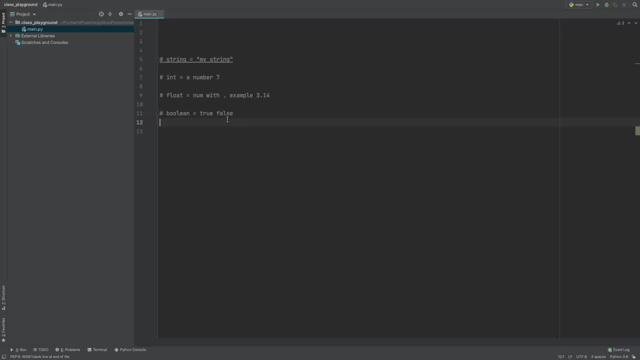 boolean is true- false. you will want to remember boolean. we'll cover these a bit in the future. when we do our while loops we'll be using the true- false. so these are some of the different data types and just to get an idea of what these look like. if we save a variable and we make it a float and we say: 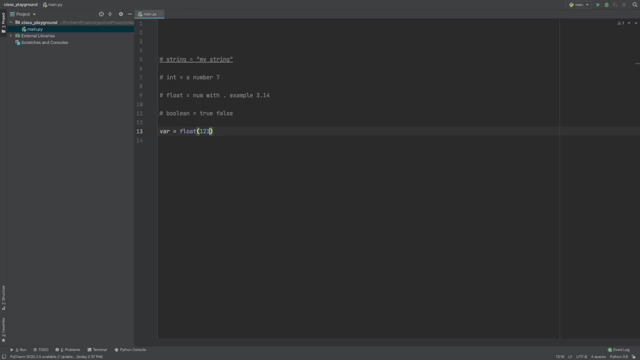 like one, two, three, and then we print this. it will tell us what we have, so we can come down here and say print and then we can put type and then we can put in our variable and when we run this it will tell us that we have a float and if we put in an integer, it will tell us that we have an integer. 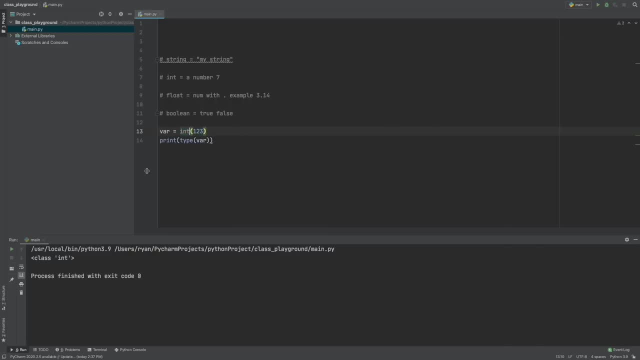 and then so on and so forth. we can do this with an, and then we can also do this with a string, and we can hit, run and it tells us we have a string. sometimes we will do something like this, and then we have this saved as a string here, and then, when we go to add this to something else, we 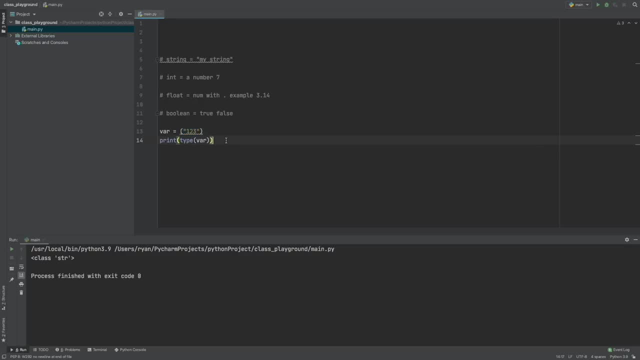 can get an error and it's because we have a string and we'll be trying to add together a string and a integer and it won't work. so we'll go variable two equals three and then when we say variable three equals variable one plus variable two, 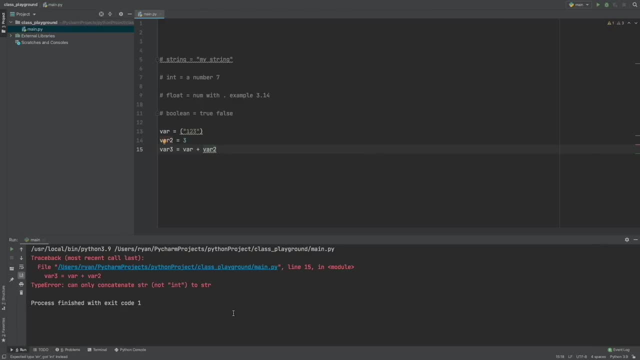 we're going to get an error and it's going to tell us that you can, you can't add these together. so this is one version of how these matter. another version of this is: let's say we want to print and we say we have an integer right here and we want to add it to a string, and we can go like this and: 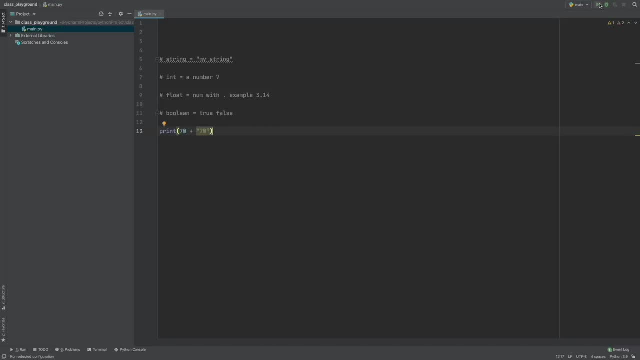 we say 70. what do you think is going to happen? it tells us we can't add these together. but if we take this and we turn this into an integer, what will happen now? now it works. so this is the difference. so this is an integer, this is a string, unless we declare it to be an integer and you can do the. 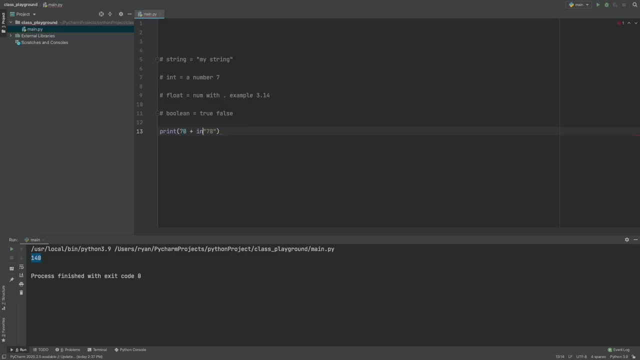 same thing with floats, so I'm not going to cover those. and then what happens if we do this here? what do you think the output will be? and the answer is 70- 70.. so this is the difference between integers and strings and how they work with numbers and data. so if we wanted to, we can. 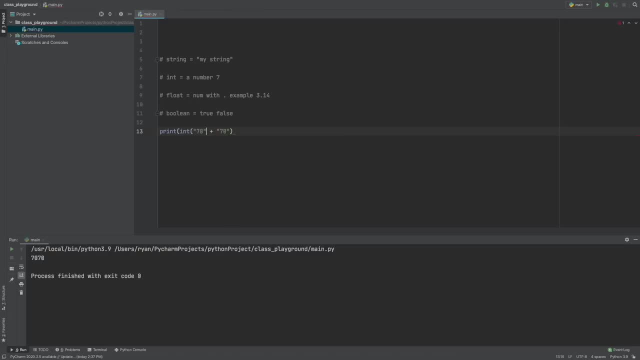 turn both of these into integers. and this is the last example. I promise I don't want to bore you with adding these together and then we say enter and we're back to 140.. so this is a little bit of strings, integers and booleans, and we'll kind of skip floats because I 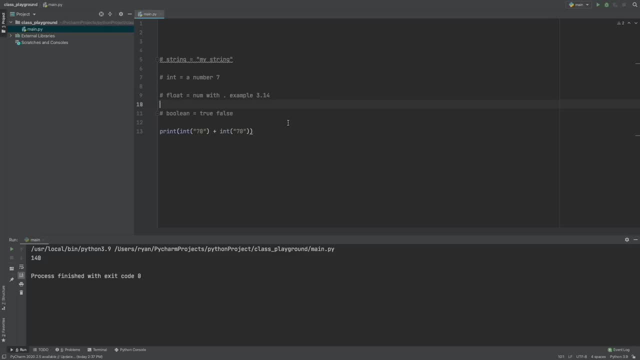 don't think we'll really need them, but it's worth mentioning. so you know they're here and with that we will continue on with our next challenge. okay, so we have these numbers here: number one, two, three, four, five, saved as num one, and then num two, and then num three. what? 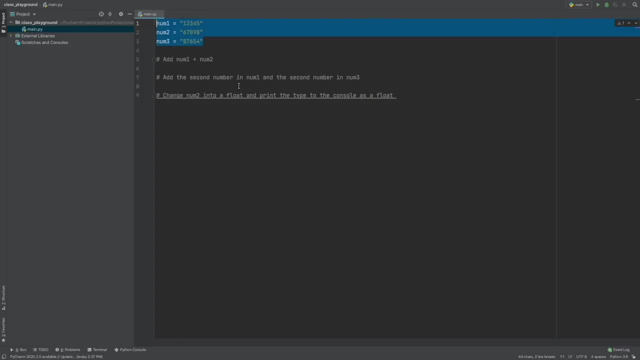 I want you to do is to write this to your console or write this to your text editor, and then I want you to add this variable plus this variable and see what the output is. and then I want you to take the second number in num one, so it would be this two right here, and I want you to 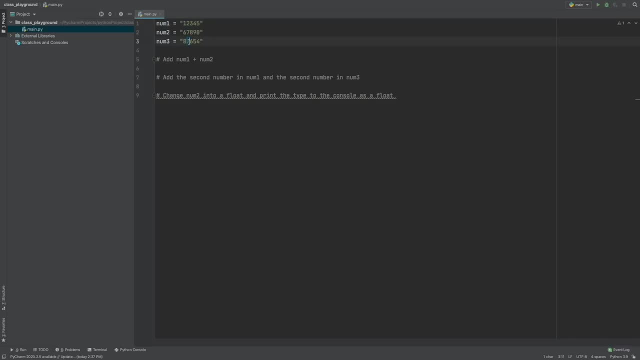 add it to the second number in num three, which is this seven, so your output should be nine. I want to see if you can figure that out. and then the third challenge is to take num two and change it. change num two into a float and print the type to the console, so that way the 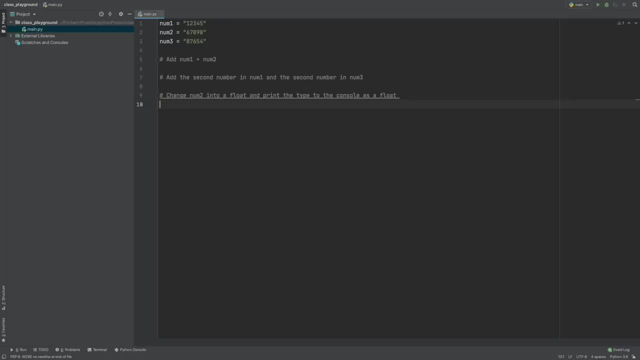 console tells us that it is a float. so if you'd like to go ahead and pause and give this a try, you can do that now, or we will go ahead and tackle this right now together. so what we are going to do just first is we're just going to print and we're going to say: we're going to turn this into an 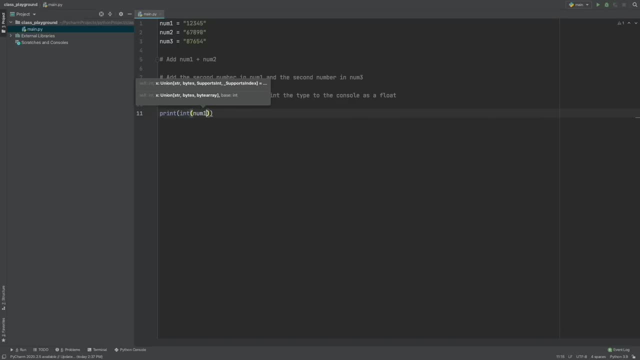 integer and we're going to go and write in num one and then we'll add this as an integer and then we will say num two and this needs to be closed off, or we are. we will get an error and this should print it for us. so it tells us: here is the total. 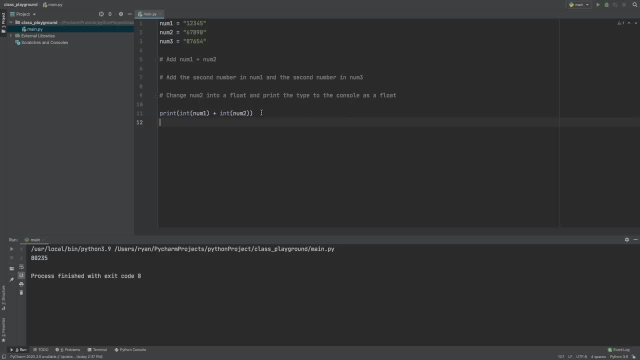 if we add those together, and then the second challenge is to add the second number. so we'll just take this just a heads up. copy and paste and programming is always a bad idea, because if I have a bug here, I just now copied and pasted it and I have two of them. but 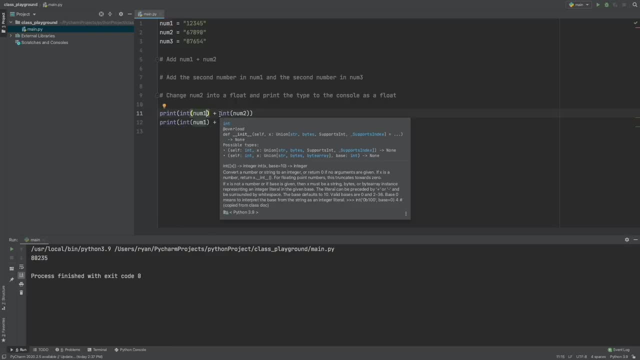 what we're going to do is we're going to take this and we're going to put in our square brackets and, if you remember, it says zero one. so we're going to say one, and then we're going to say one- I guess I didn't really need this- and then we'll print this and our output is nine. so now we've grabbed. 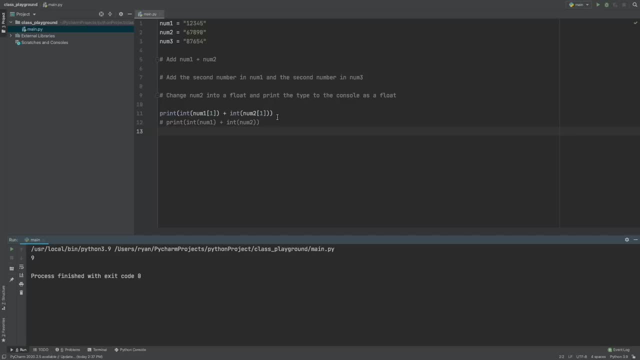 the second numbers. and then our third challenge is to change number two into a float so that it prints float. so what we want to do here is to say print. and then we're going to tell it: we want a type and we want to print out the type of num2 and 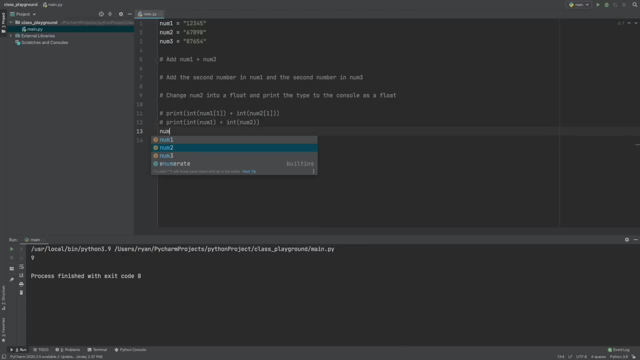 then, above that, we're going to just type in num2. you can do this two different ways. I'm going to do it this way: I'm going to say num2 equals num2 and we'll just go like this and we'll type float and we'll close this off. and now, if we print, 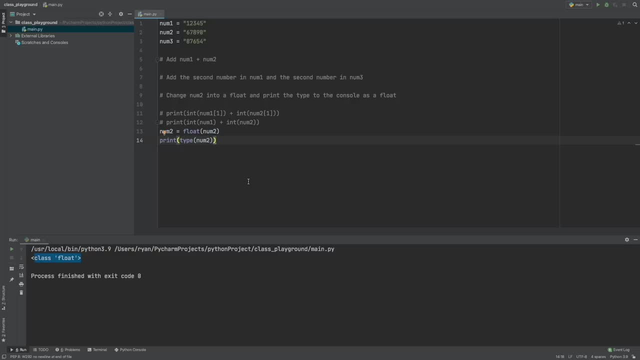 this. it tells us it is a float and we will continue on with our python course in the next section. okay, we are going to do a walkthrough of if, elif and else statements. so this is the instructions for the little program I'm going to write, but when I finish this, 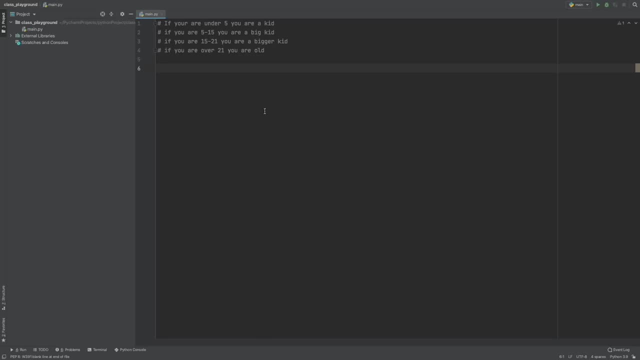 program. I'm going to give you a challenge to do something similar on your own, so I'm only going to give one example. you're and you're going to need to pay attention and maybe watch this, walk through twice and then go on and try the challenge. so the first thing we're going to do is, if you are under 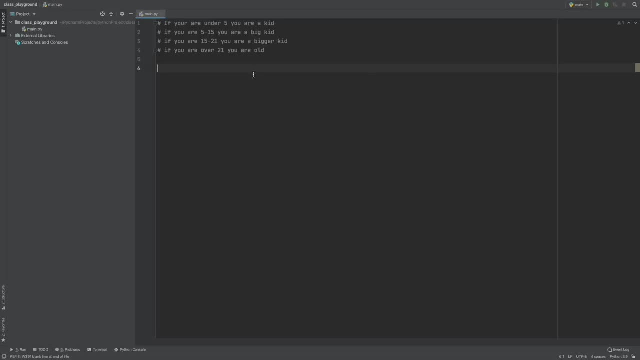 five, you are a kid. so our if statement is going to first need an input from the user that is going to tell us what is their age. so we'll just say we have a variable and we want it to be an integer and integer and we want an input and we're going to ask them what is. 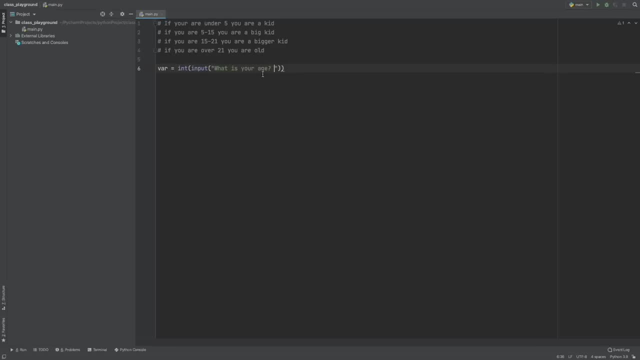 your age question mark space. and we have to have that space, otherwise it's really ugly in the terminal. and then we're going to start our if statement. so we're going to say if a you, this person's, their input, which is their variable, is less than the age of five, 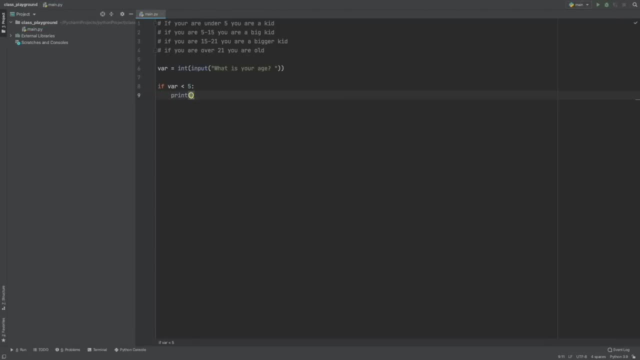 then we want it to print that they are a kid. so we'll print: you are a kid. now, one thing we want to do is if they hit the age of five, we'll need an equal sign here. otherwise I'll just show you if we say we'll need an else statement so this doesn't air out. actually we'll. 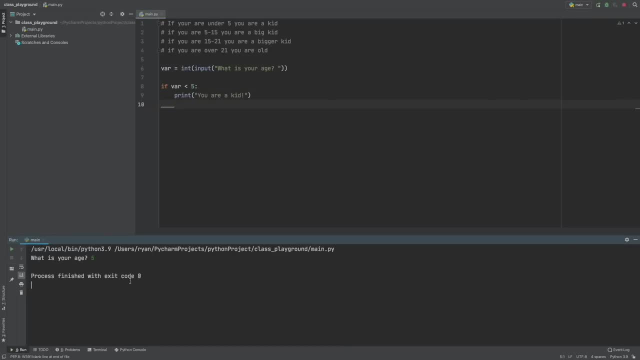 just let it air out. we'll say what is your age and they say five, and we hit no output because they this doesn't include five, remembering that the computer starts at zero and then it's going to stop at four. so if we want to include five in as yours a kid, we'll need that. 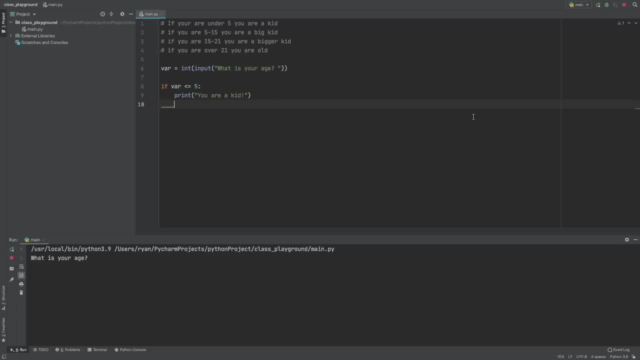 the variable is less than or equal to a five. now, if we put the five in here, it will print for us. you are a kid. so what we we need to do next is we're going to type in l if, because we're going to make an LF statement and we're going to say: 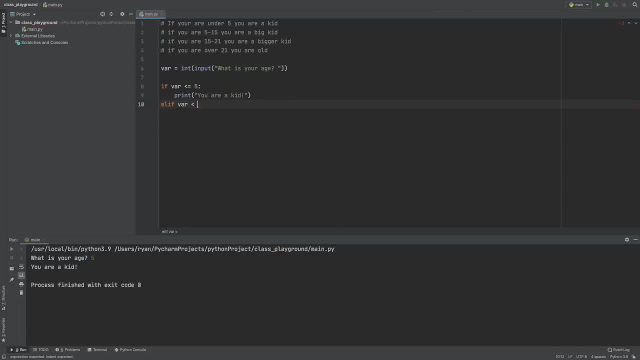 the variable is less than 15.. And the reason we don't have to worry about anything under five is because it will catch this if statement and then this whole program we write after this will stop and the computer will actually skip it. So we don't need to worry about adding anything else in here. 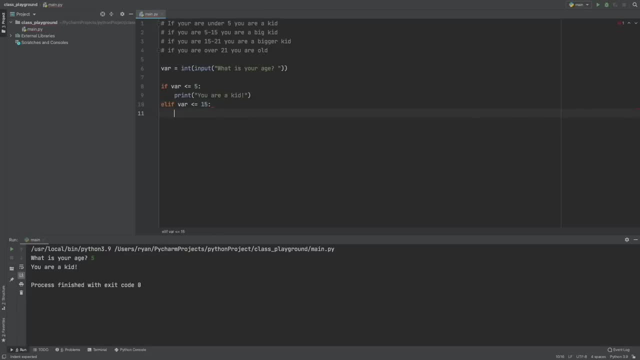 And we can say: actually, if you are less than or equal to 15, then we are going to print: you are a big kid. And then, for the final elif, we will say the variable and we will say if it is greater than or equal to 21,. 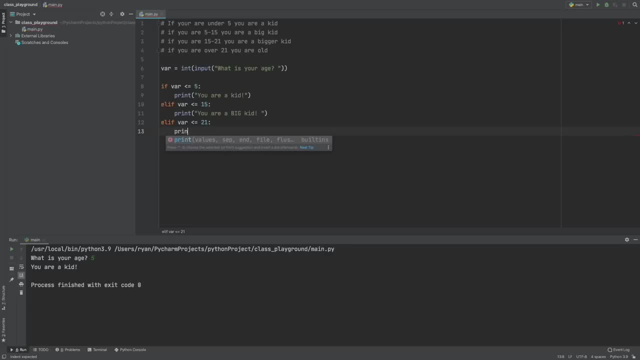 and that's ugly. and we will say print. and we're going to print. you are a big kid, Bigger kid, And now we're going to put in an else statement And in our else statement we're going to print anything. 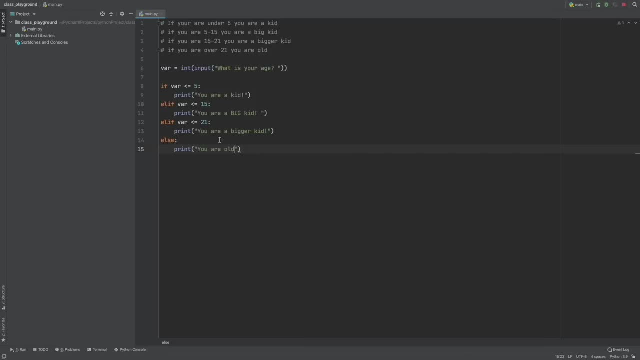 that's over 21.. We're just going to print: you are old. So now, if we run this and we rerun the program, we run it and we say how old are you, And we say three, we get your kid. 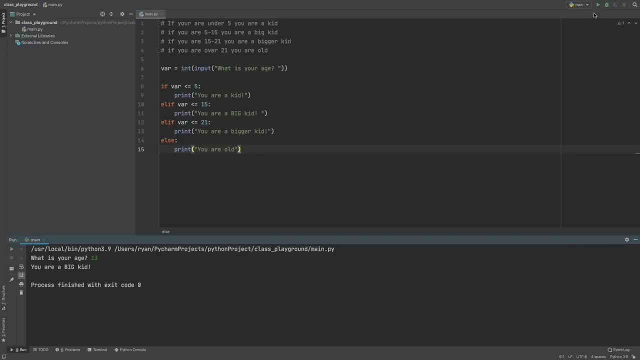 If we say 13,, we get your big kid. If we say 18, we see you're a baby- Bigger kid. And if we say you are 44, we get you are old Now, because we're going to be using this as a tool. 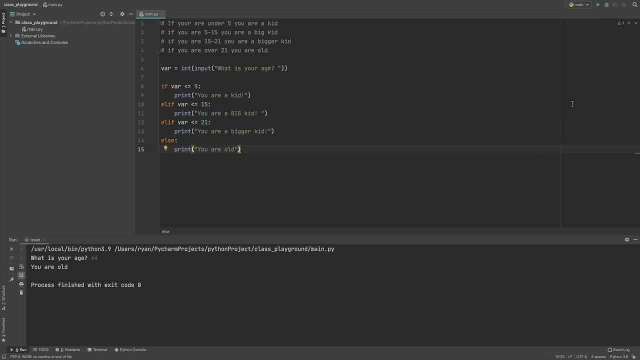 for us to be able to write tools and modify tools. I'm not going to cover this because I think that it's not really necessary for cybersecurity, But if somebody were to run this and they put in the letter A, it's going to crash our program. 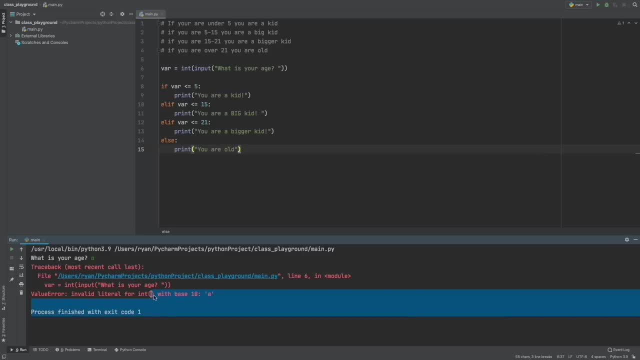 because the letter A is not a number, It's not an integer. So what we'd have to do is we would have to make this so that, if they put this in and it was an A, it would print, enter a number and then rerun. 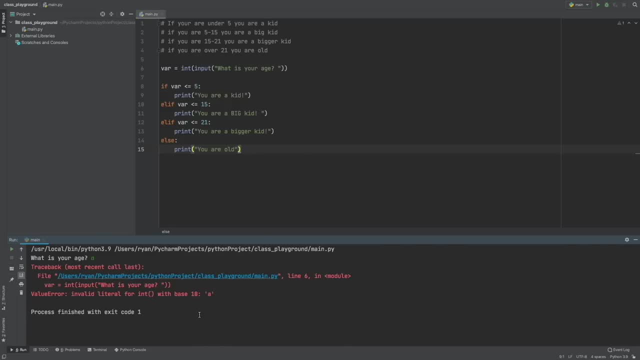 But we're not going to do that because it's not really necessary for cybersecurity. It's just something to be aware about. Now what's coming up is your challenge. Let me delete all this and I will write up your challenge for you in the next section. 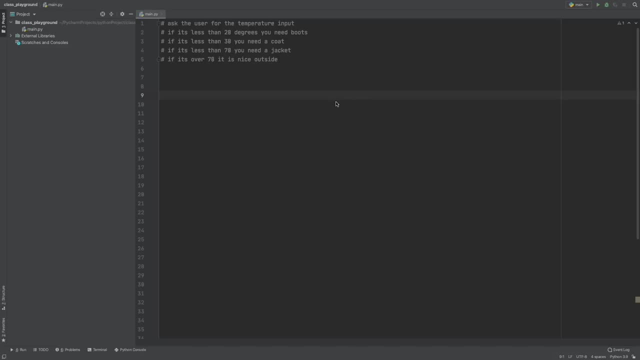 Your challenge here. The challenge here is to take the temperature from the user and then tell them: if it is less than 20 degrees you need boots- And this is from the US, So I'm running in Fahrenheit, not Celsius, And if it's less than 30, you will need a coat. 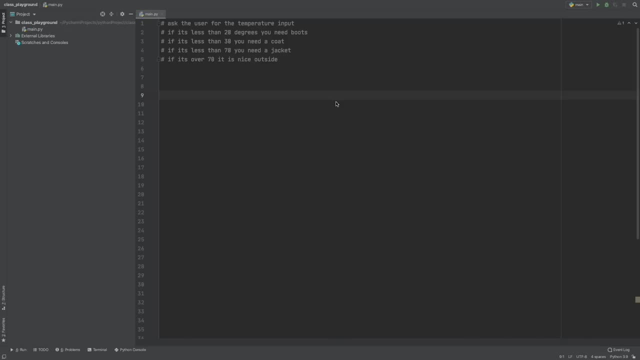 If it's less than 70, you will need a jacket. If it's over 70, it is nice outside. So take this input or take this information and make a program with your user. It's if, elif and else statements. 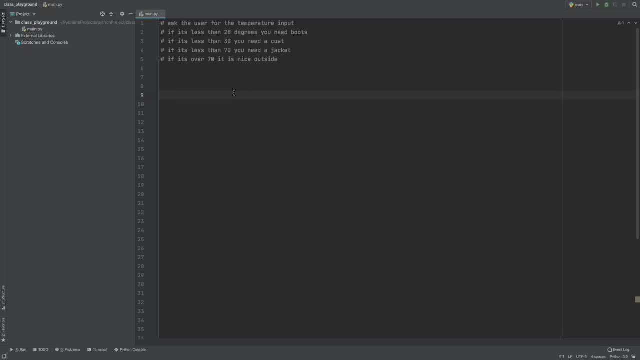 Okay. So here is how I would go about doing this. I would take an input and it will say what is the temp outside, And this will need to be an integer because we're going to be comparing this as a. So we'll say: if var is less than 20, then we're going to print. you need boots. 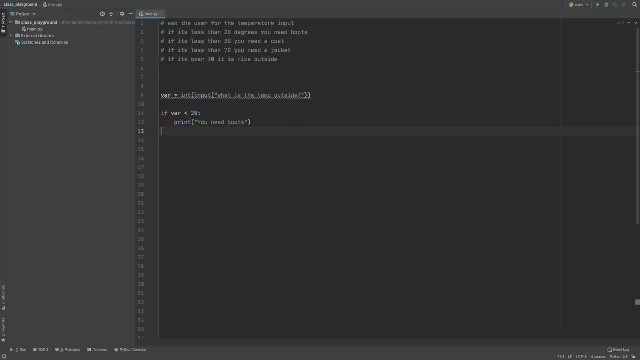 And we'll say: elif var is less than 30. Print, you need a coat. And then we're going to use one more elif here. Elif var is less than 70. Print, you need a coat. 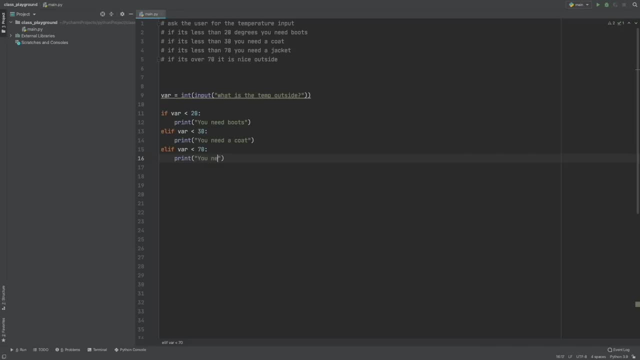 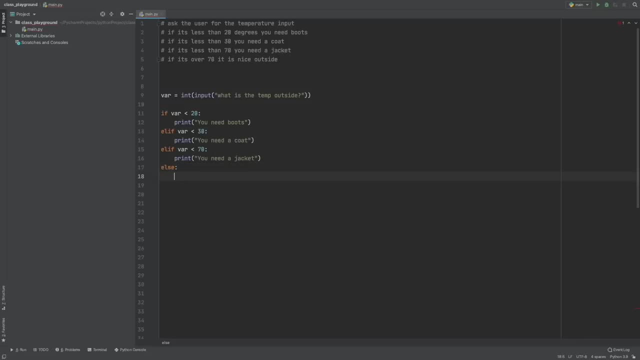 else statement. So everything that's above 70 will automatically print. It is nice outside. So when we run this, if we put 12, we need boots, If it's 22, we need a coat And if it is 65, we need a jacket. 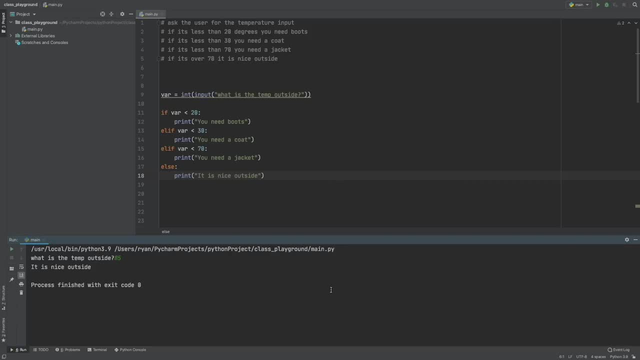 And if it's 85, in my opinion it's perfect outside. So this is the if and the elif and the else statements We're going to be moving into for loops and later we're going to look at nested if statements And they'll look something like this: 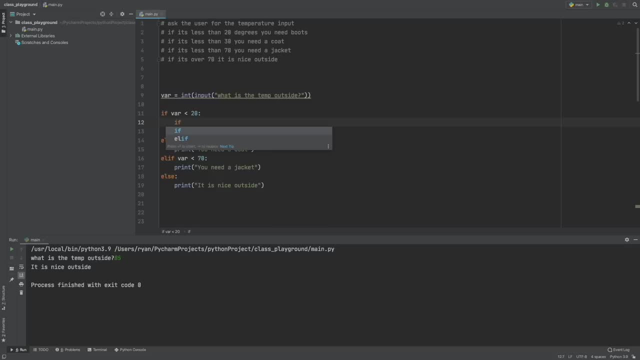 If it's less than 20, and then we can say: if it is, if var is less than, we'll say it's actually it's greater than 25, then we can print: you need boots. And then we'll print something like gloves. 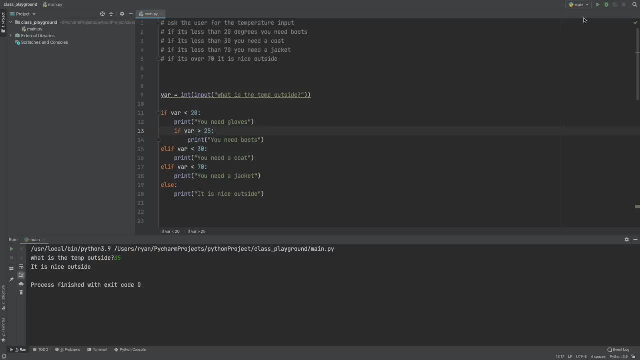 So nested if statements look something like this: And you can have nested if statements, just so you're aware of it. So if we say it's 26,, it will, Oh, because we're hitting this one, We'll hit, We'll say this is 15.. 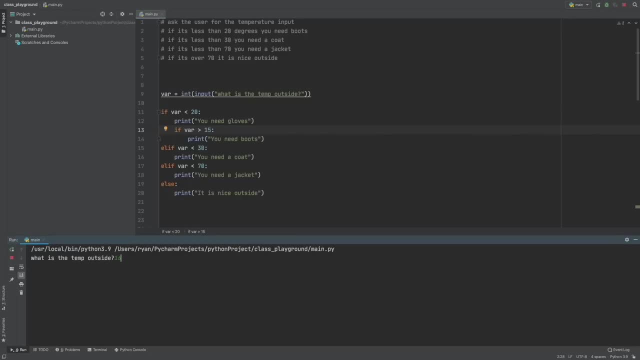 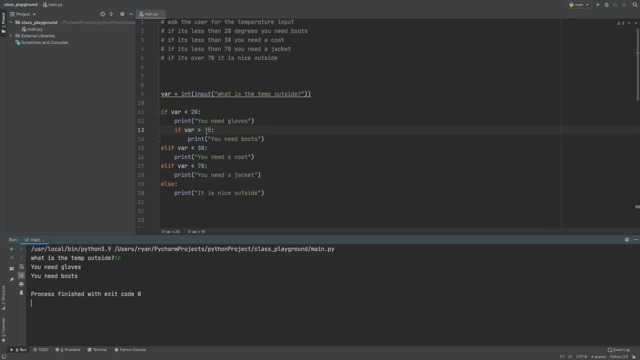 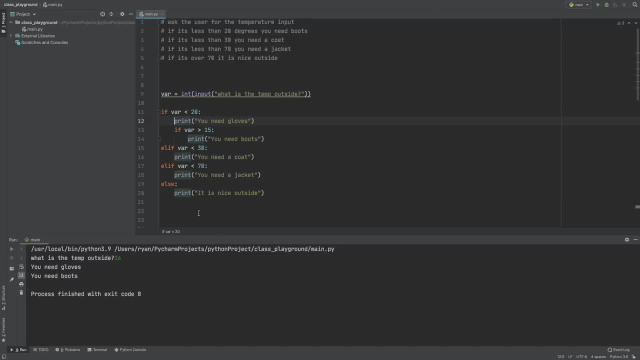 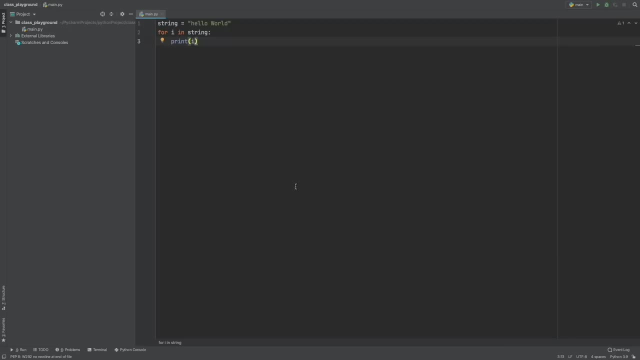 So it's nice to know that you can run nested if statements. But for now we're going to move on to our for loops. Before we get into for loops too far, I want to show you why for loops are important And I also want to show you why lists are important, which we're going to be going over. 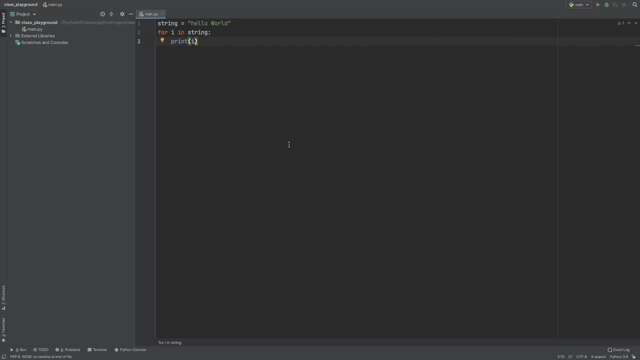 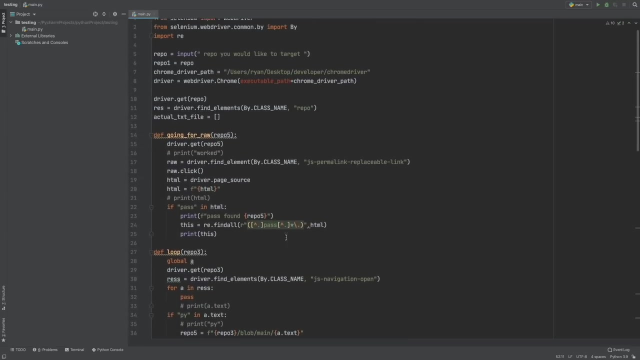 here In just a minute after we get the basic understanding of a for loop. So this is a program. I've shown it before. It don't worry about what it looks like. It looks kind of complicated, but it's really not. 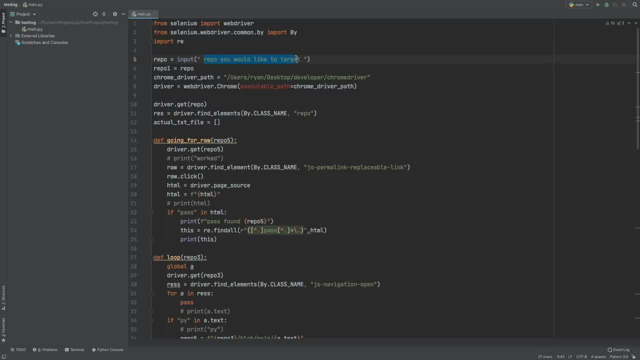 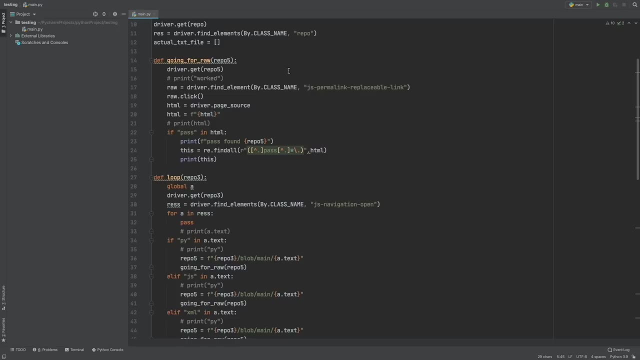 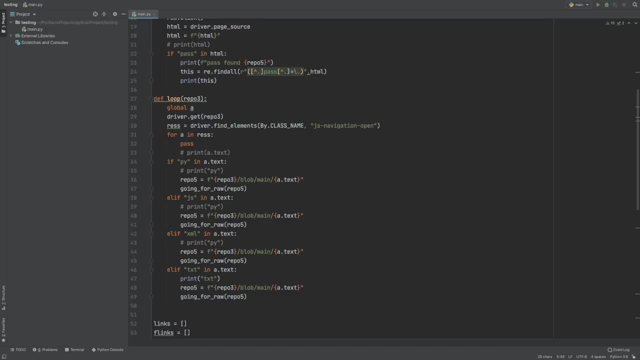 What happens is you put in a repo that you would like to target on GitHub to go and search for all of the usernames, passwords and files that just shouldn't be made to the public. So in this case it's looking for pass for passwords on GitHub. 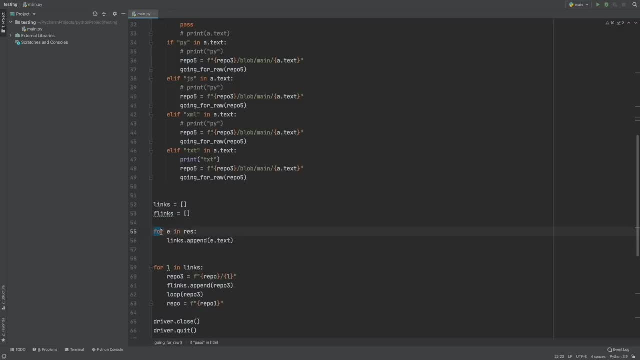 But what we have done here is a for loop. So this for loop: right here we have an empty list, which we're going to cover in a second, and it goes out to GitHub right here and it will go through all these links, everything. 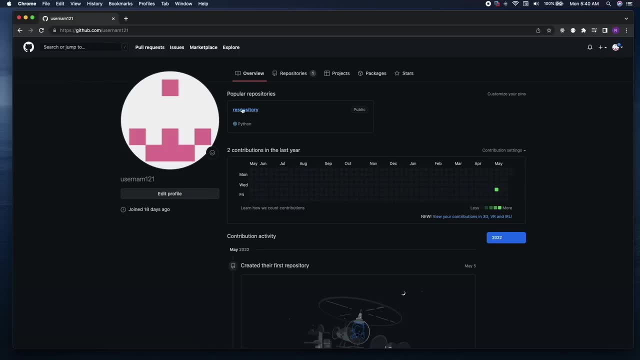 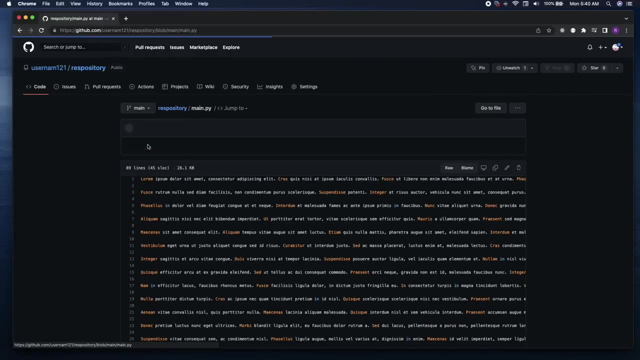 you can click on and it's going to narrow it all the way down to the repositories and it will click this link And then it will click to, It'll click the file and then it will click the raw, then it copies this entire thing. 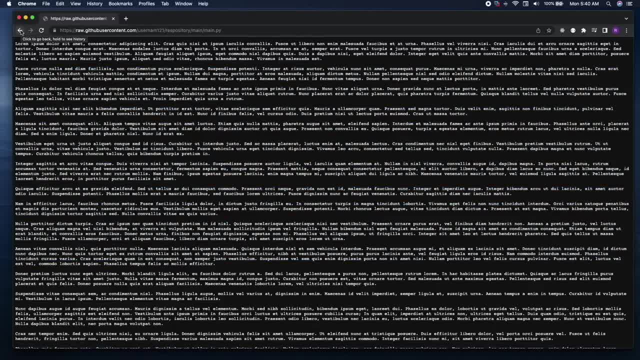 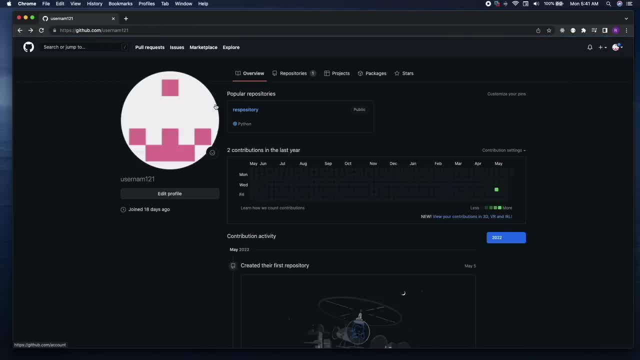 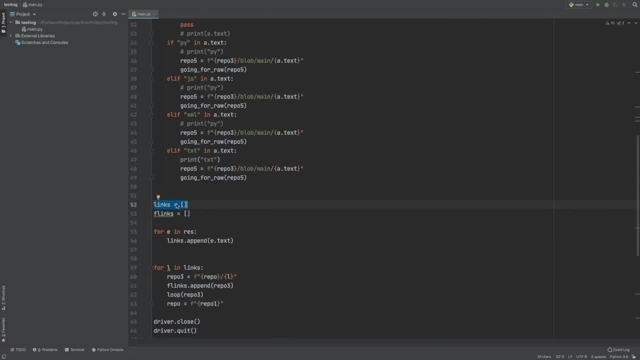 and it puts it into a text, It puts it into a CSV file and then checks for the word password. So that's the program itself. But what's important to remember is what happens is it goes out and it pulls all the links and puts them in a list. 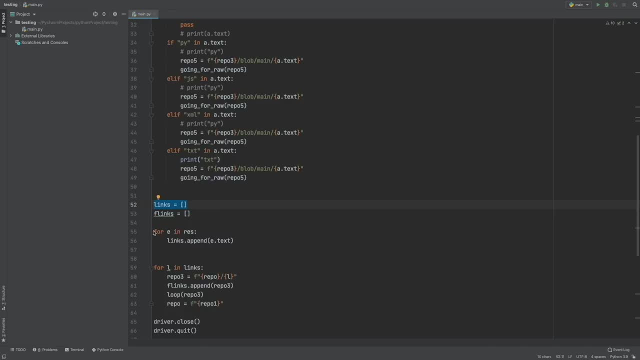 Then it goes through this for loop and it puts: takes all of these And it says, for every one of these items that is inside of the links, which is actually this variable that I have up top, it's going to do something. So for loops are very important. 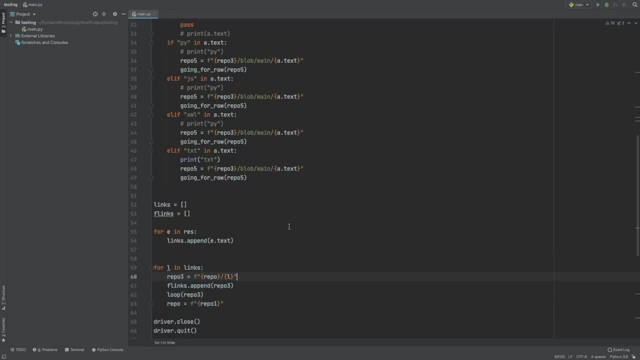 You can see I have another one right here. So for loops, we are going to need them, lists, You are going to need them as well, And I just wanted to show you this because sometimes what happens is you'll be going through trying to learn something. 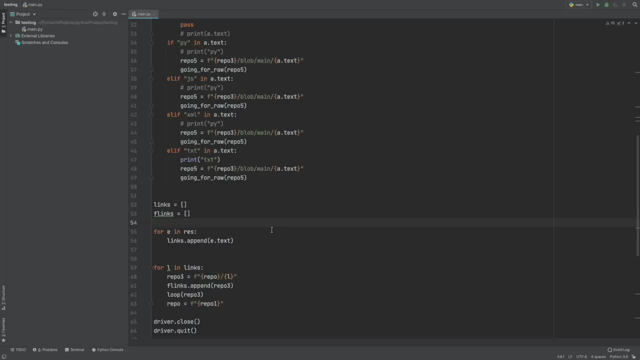 And I'm showing you. Okay, You're in elementary and you are like: why? why do I need to know a program that tells me to put on a jacket? This is all building up to something that is going to be able to help you build tools. 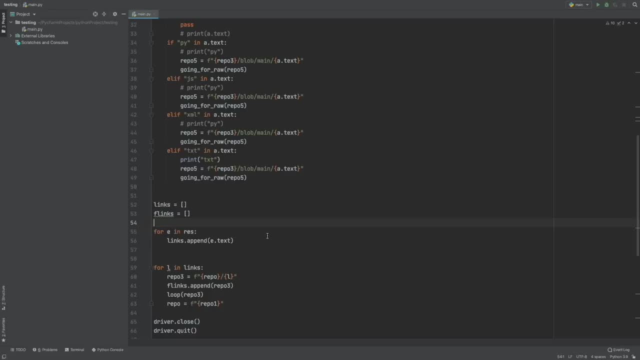 And, more specifically, if you're new, just be able to read through exploits and be able to edit them, because you're going to need to know how to read Python and edit exploits as you grow in the world of cybersecurity. Okay, So here is a very basic for loop and I'm going to show you it in a string, because 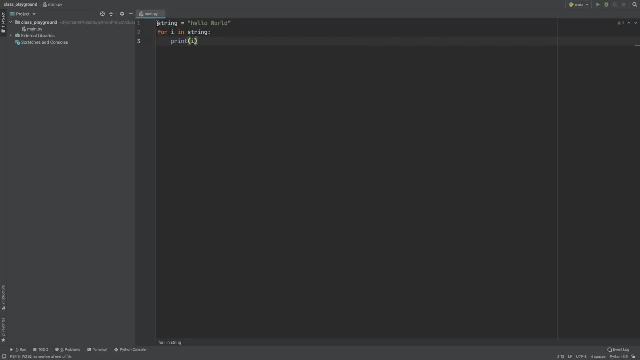 we've already covered strings and what this all this does is we have our variable string right here that is holding hello world, And so the way the for loop works is it says for I in string. So this I right here is going to be another variable that holds one letter each time, the. 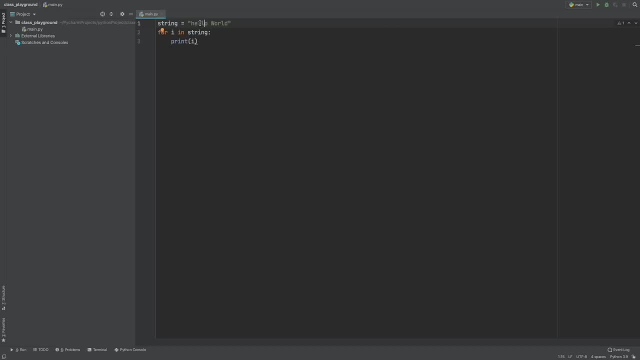 for loop. So this I is going to represent one letter and in a list it's going to represent each item in the list. So this will run. I'm going to run it so you can see what this looks like. The way it runs is it goes for I in string. 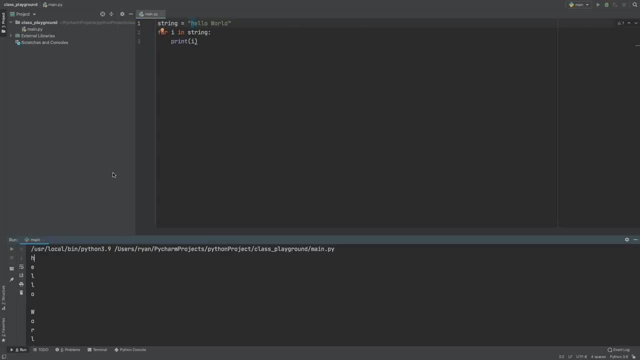 So it's going to grab the first letter, which is going to be the H, and then it prints it. but the for loop is not over, So it runs the loop again and it'll grab the E and it'll print just the E on a new line. 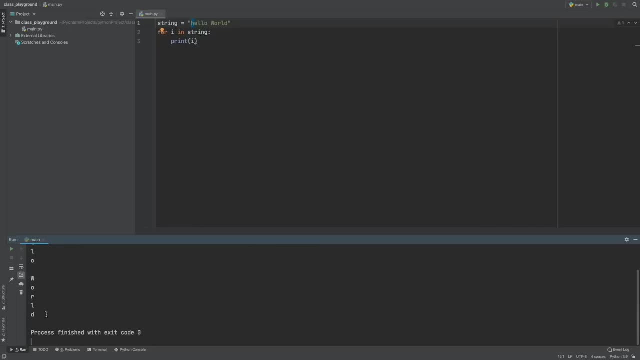 And then it goes through. It runs every single time until it is out of things to run, and then it closes the loop. So this is how for loops work. I'd like for you to go ahead and write out your own for loop and maybe put something. 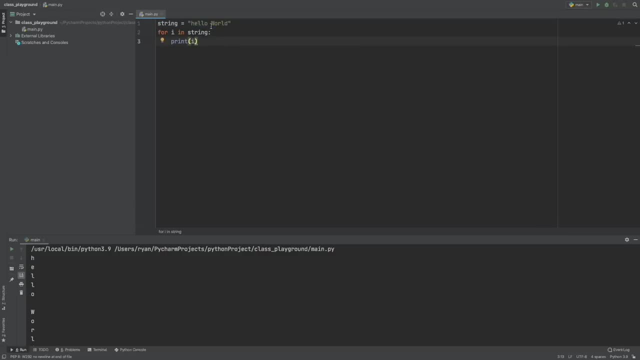 different in here and try to get an understanding of how it works. And if we wanted this to print all of this together, you would have to store this into a new variable and then print it outside the for loop down here like this, And this is where we would print our new variable. 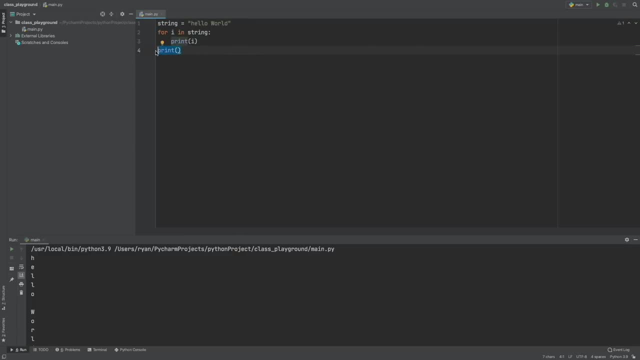 And we're going to cover this in lists, because this is something that you will need to do in the future. So go ahead, play around with the for loop, write one, get an understanding of how it works. If this doesn't make sense, rewatch it and hopefully it makes sense. 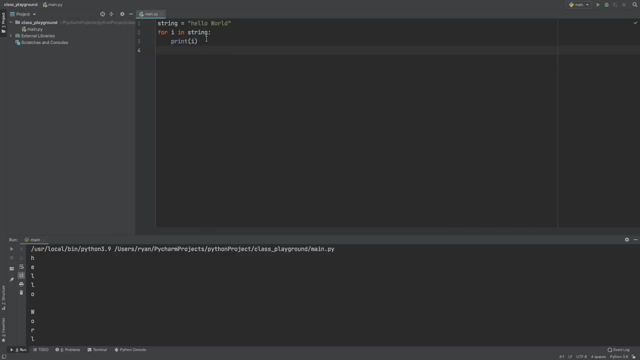 I know, after teaching for loops to several different students, that for loop sometimes can be hard to understand, but they are really useful and something you need to learn. So we're going to be covering lists in the next section. We're going to be looking at lists and a list is something that is going to be useful because 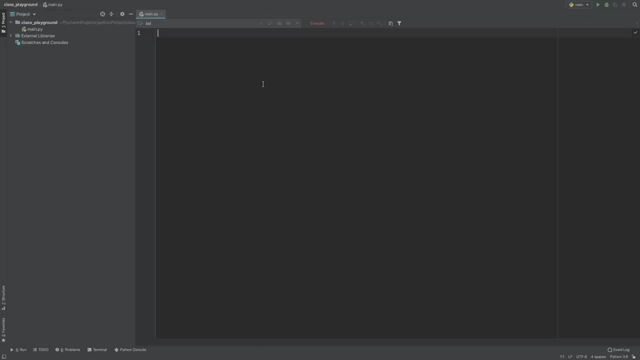 we're going to be appending to lists all the time within our for loops, So a list can look like this: My list equals square bracket and lists always go inside of square brackets and we can say item one and then comma, item Okay, Two and then we can do an item three. 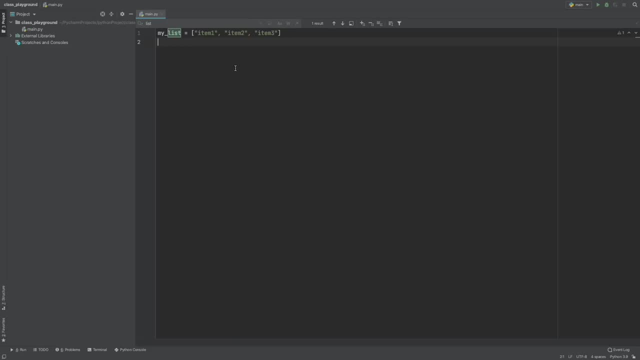 So we have our list here and if we want to run a for loop through this list, we will say for i in my list, print i, And now if we run this, It will run Item one, item two, item three. So this is a list. 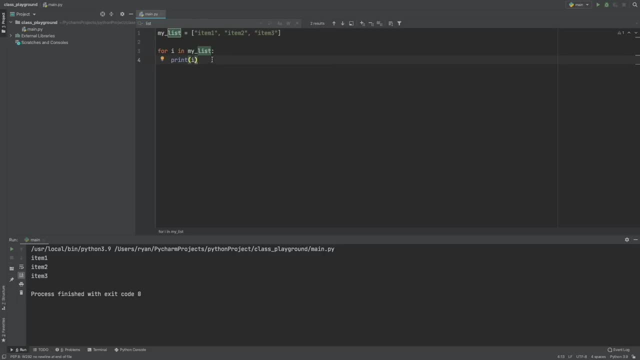 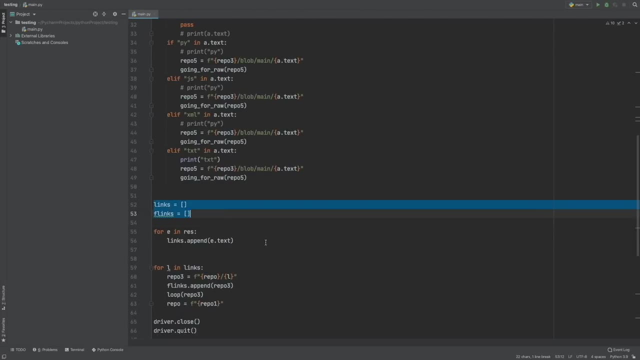 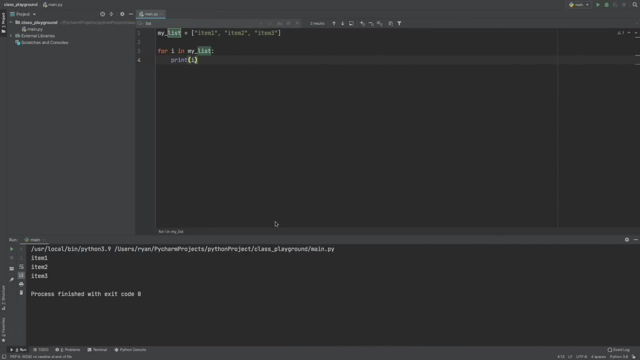 We will be using these in the coming lessons and they will be helpful for you in the future. As you've seen in this program, I have two lists right here and they are used regularly to append to, So lists is something you will need to know. 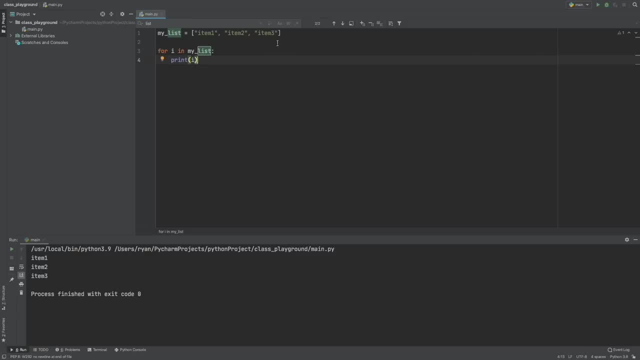 So go ahead, make your own list and see if you can loop through your list And maybe try and just print something like this later: Just print the item two, So you'll have item one, two, three, and then print number two and see if you can remember. 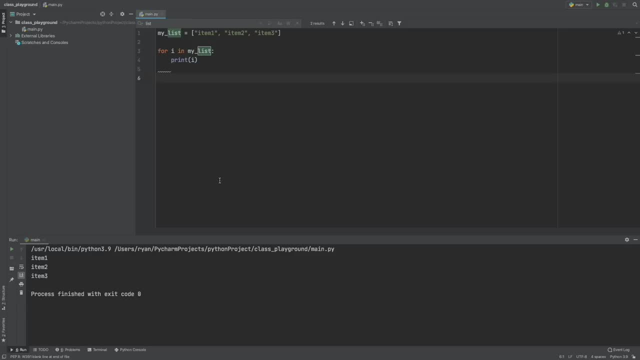 how to do that, If you have forgotten. it would look something like: this print and then we can say my list, and then we can put this in square brackets and we'd say zero one, and then we have a one, and now we could print this. 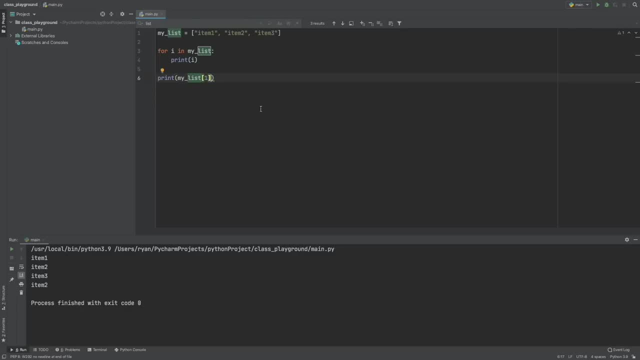 And we have one, two, three, two. So that is going to be it for the list. We're going to move on and we're going to start using lists in a more comprehensive manner, So we're going to try a while loop now. 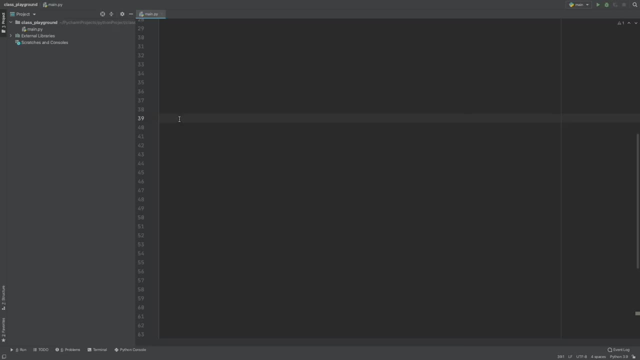 And the way we're going to do a while loop is by using a Boolean. I like to set a variable and then set it to true, And then, at the end of the while loop, I will set it to false. So the way this works is make a variable. 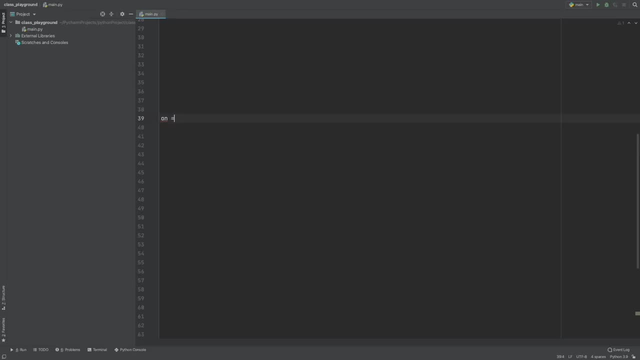 And we'll just say variable. actually, we'll name it on- That's a good way to name the variable- and we'll say on equals, true. And then we'll say while on, and we'll make a variable and we'll just call it variable. 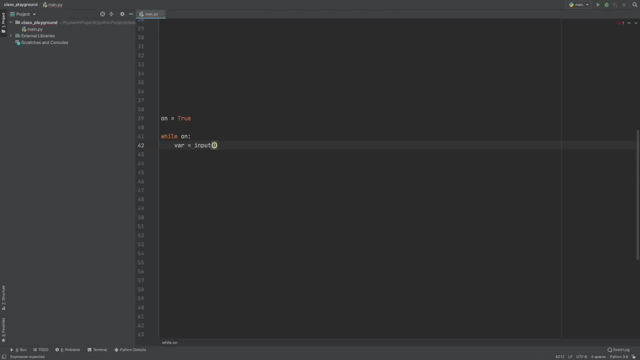 because I don't know what to name it- And we will take an input and we will say: continue running while loop. And then we will put a Y or a no. So would you like the while loop to continue, yes or no? And then we can say that we can go do something like this: 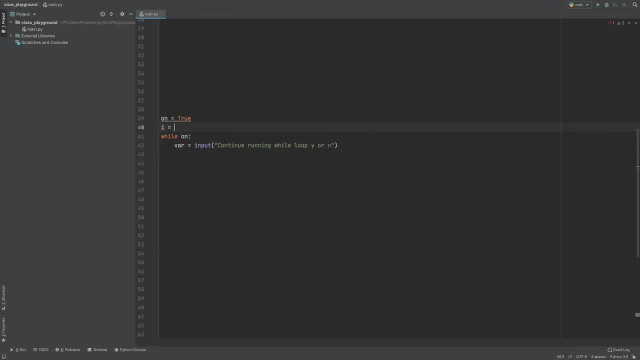 And then we can set a variable up here and say: I equals zero, just so you can see how many times this is running. And then we'll say I plus equals Y- Okay, I equals one, And then this should just continue to run. 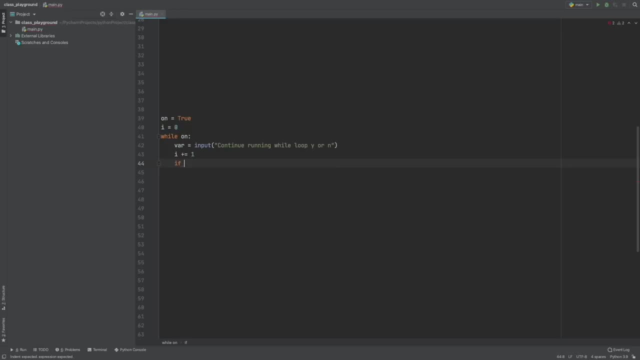 And then we'll put an if statement. Say, if the variable equals equals in, then we'll say that on equals false, And this will kill our for loop. So now, if we run this, it will say: Would you continue running the while loop? 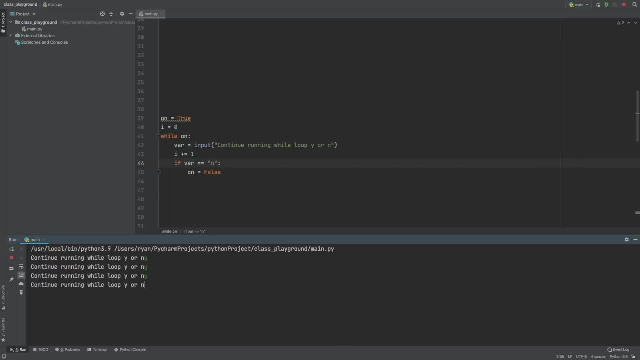 And we will say yes, yes, yes. And then, when we say no, it'll kill the while loop. I forgot to print. I forgot to print our I so that we could see this. So now we can say: would you like to continue? 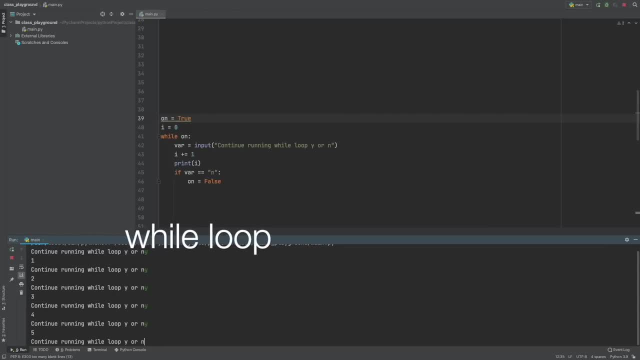 Yes, yes, And you can see our variable. Every time The for loop runs, our I gets added to one. So our for loop has run. Now it says seven times, eight times, nine, 10.. And then, when we're done, we can say no and we can end it. 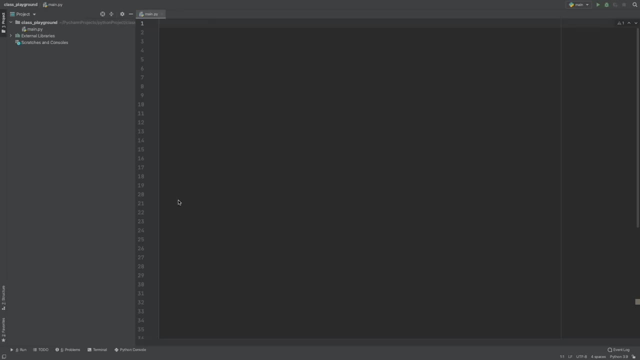 We are going to be starting functions And, just to be clear, I have not pre-written any of the code we're about to go over or mostly anything we've gone through in this course. That's why you've seen me make mistakes, And so, as we start functions, I'm going to try and make this. 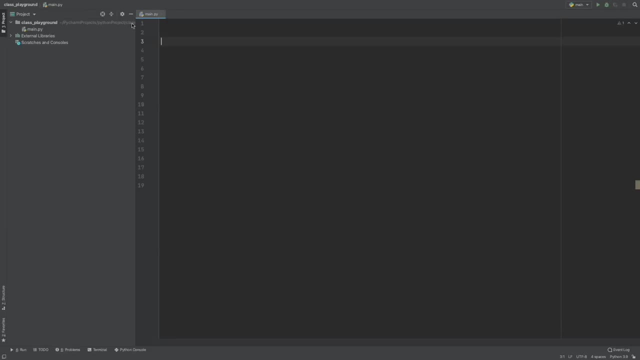 A little more realistic for us so that when we are thinking through functions and writing code in the realm of cyber, in the realm of cybersecurity, you can start to get an idea of how this can be used. So we're going to start with functions, and a function just calls something very specific. 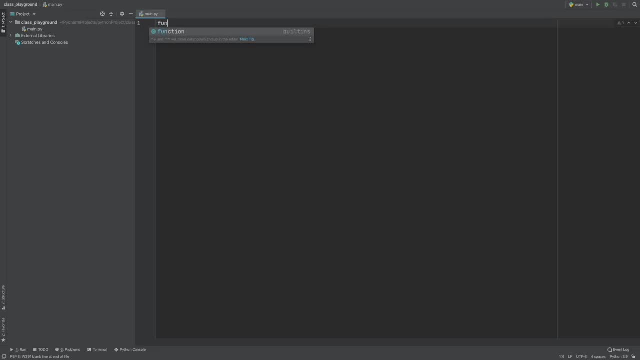 that we want to happen. So we can just say we'll call it my function, Okay, Okay. And then the way your function is going to start is with a def- my function. And then we close it off like this: And then down here, we want our function to do something very specific. 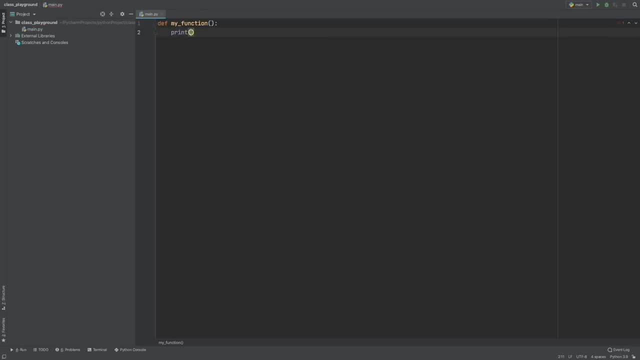 So we can say print and then we can say it worked And the way a function gets called is usually somewhere further down inside the code. Something happens And it triggers this function back up above it. Okay, So if we run this, it's going to print it for it to actually do something. 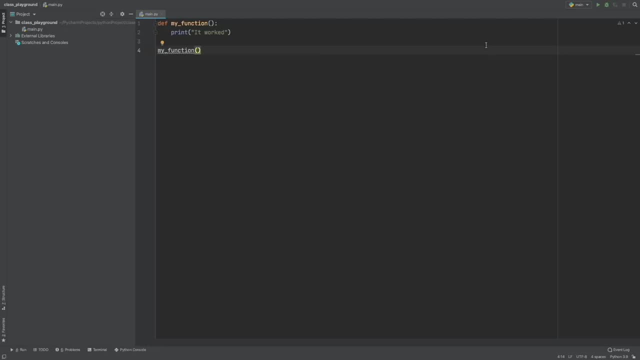 So what would happen in order to call this is, we would just say, my function. Now, when we run this, when the computer reaches this right here, this closing bracket right here, I usually like to think of this as the call sign for the function. 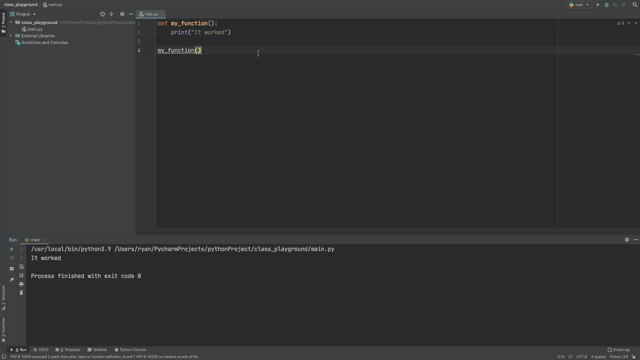 So if we run this, it's going to print it worked, And this will become more clear as we write more of these. but this is the basic concept of functions, And one thing we can do with functions is we can pass through. 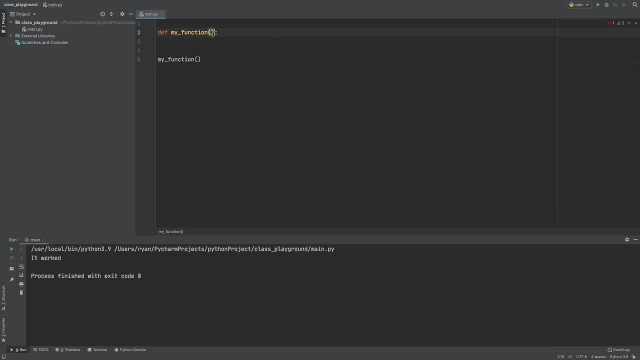 Okay. So we can say something along the lines of I, and then we can say I or we'll make it a different variable. We'll say: variable equals I plus three, And then we can say print. and then we can say we want to print our variable. 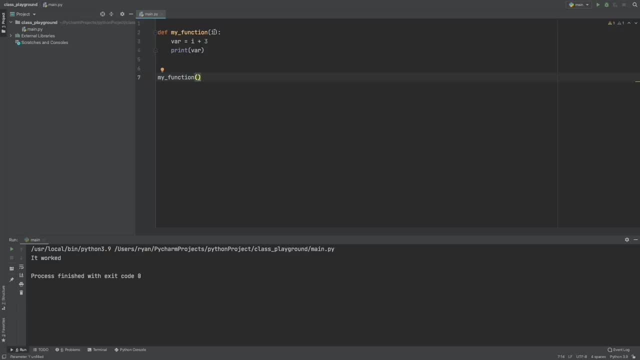 And so in our function we can pass information through like this. So when we say my function, We can now say input and then we can say what would you like to add? And because this is a string, we're going to need to make this into an integer. 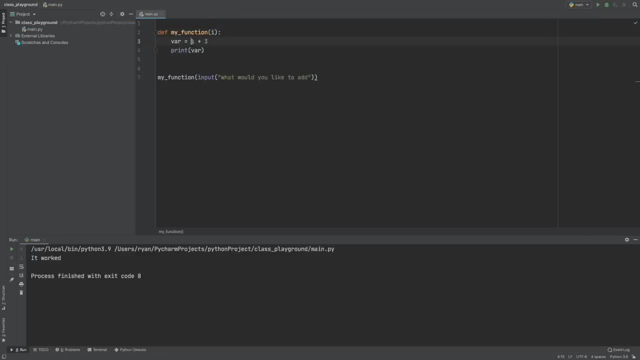 I guess we can go and make it an integer right here and we can say int, and then we can close this off. Now, when we run this, it's going to ask us what would we like to add, And we can say three, enter, and it'll say three plus three equals six. 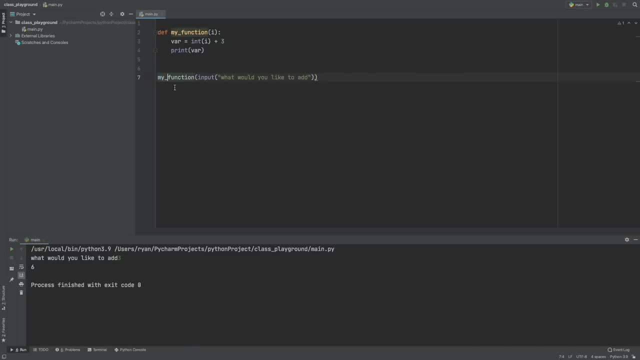 So this is a very basic function. So we take some kind of input right here. This is where we call our function. So now this function is being triggered, but we want to pass something into our function, some kind of variable or some kind of information that we've grabbed somewhere else. 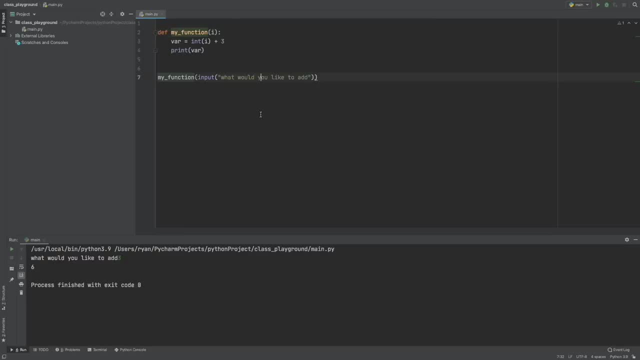 And what happens is it can now use this inside the function. This you may be thinking like: in what case would I possibly ever need to use this? And so I'm going to just show you my GitHub dumpster diving tool, once again that I've 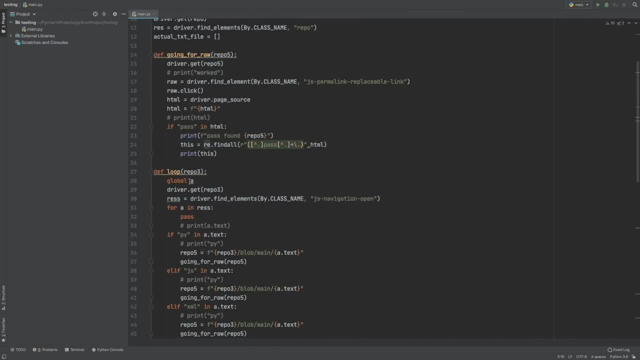 used. I've used it multiple times on this channel, This right here where it's grabbed a repo. I call this function and it's going to loop through to see every single file inside of the repo. Is it a Python file? Is it a JavaScript file? 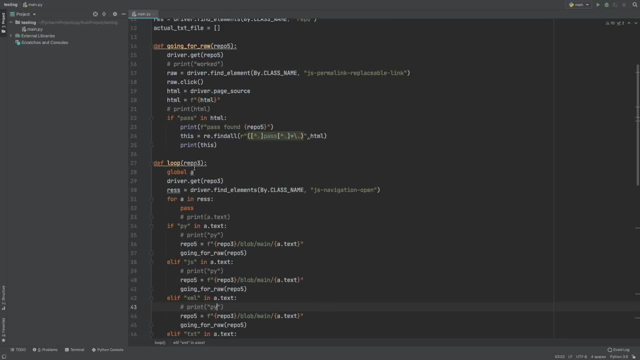 Is it an XML file, And what happens is, when I pass this repo through, it now is able to use this variable that has come from somewhere else inside this function, And then I do the same thing up here. I pass through a variable inside of a function. 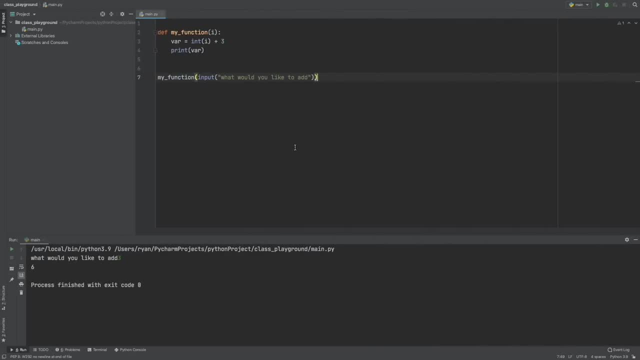 So this is really important to know and you will use it And we're going to go ahead and give another example And actually, before we give another example, I want you to try and write your own function and see if you can get it to take an input. 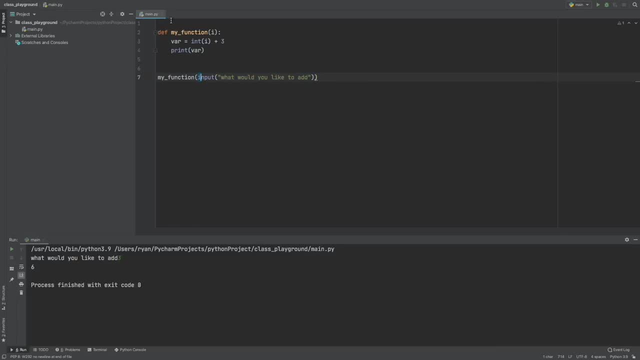 So let's take the input and make it the first letter of your name. So I'll write out the instructions. You want the Okay. Okay, We'll say first letter of your name and you want to take this as an input. 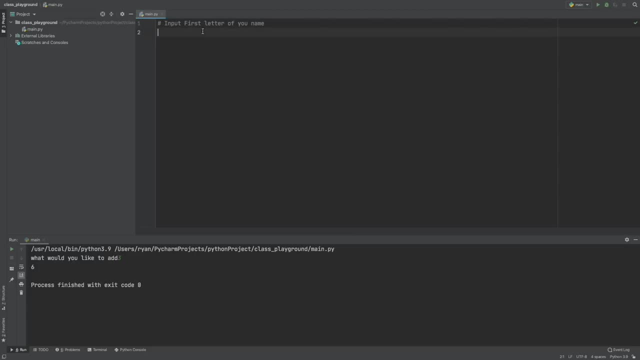 So we'll say input, and then you want to call a function that adds your first letter to the rest of your name. So here's your instructions. You're going to make a function And then it's going to take a variable and that variable is going to be the first letter. 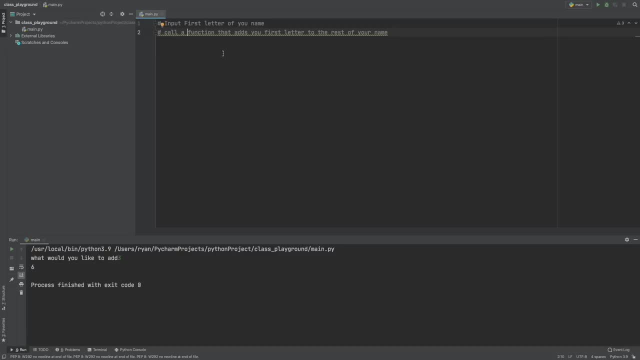 of your name And then you're going to add that to the rest of your name. So I hope this makes sense And I'll go ahead and walk you through what this would look like. So we'll go def my function and then we're going to call this function. 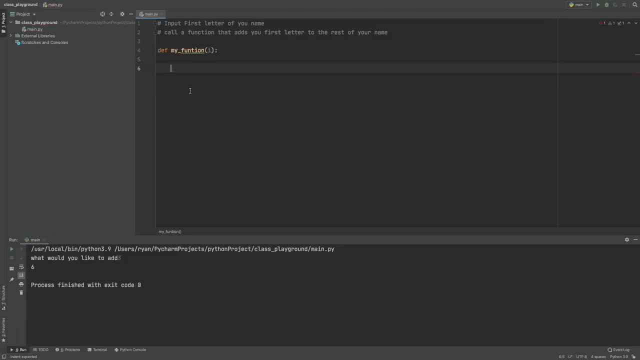 We're going to pass through. Let's use I as our variable, So that stops giving us Okay. Whenever this is giving us an error and I can't stand looking at it, I type in pass and that will not give us the error. 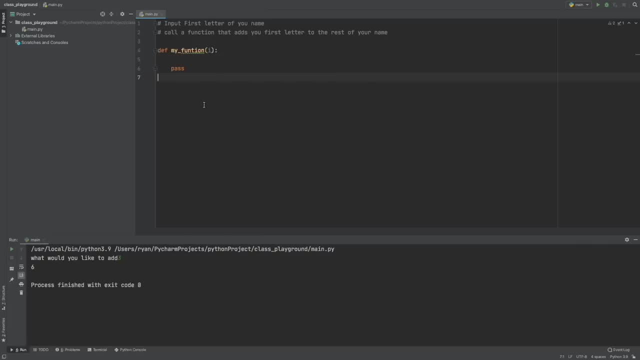 And we'll come back and delete that in a second And we're going to call my function and we're going to take another input and we're going to say what is the first letter of your name? Now we can delete this and we're going to come back up here and we're going to use 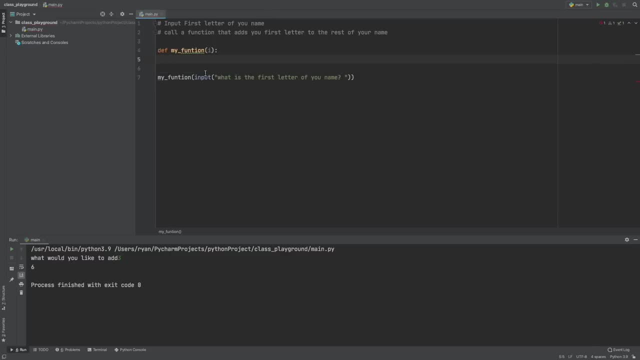 this. We're going to say that my function and we're going to take this input and it's going to be a pass through as I, And so down here we're just going to say my first name is Ryan. So we will say: I we'll call it the variable equals I plus, and then we can put the rest. 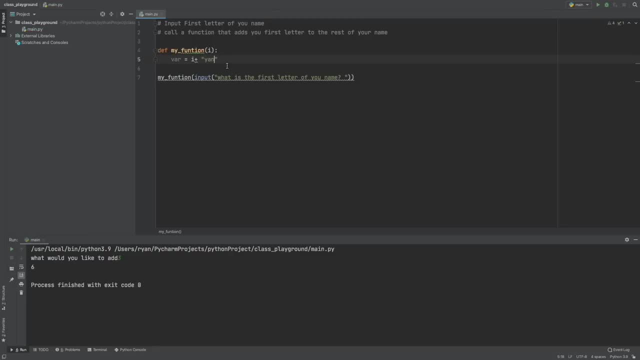 of this inside of a string and we can say something like this And then we can print: Okay, Let's print our variable. So when we run this, if I put an R in here, it'll print out my name. So I hope you're able to figure this out. 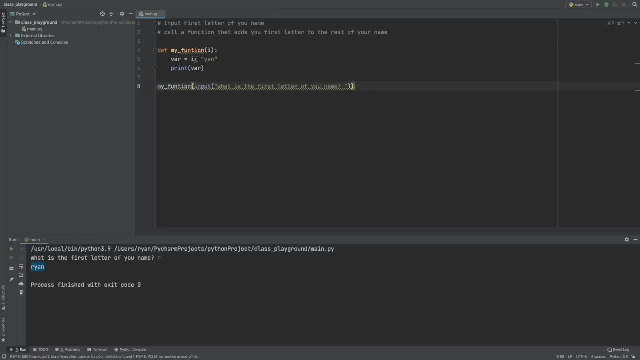 Maybe try to come up with another way to write a function and practice writing functions and see if you can get the hang of it. And in the next section we're going to go over something that will show you how this can be really helpful in building your own tool. 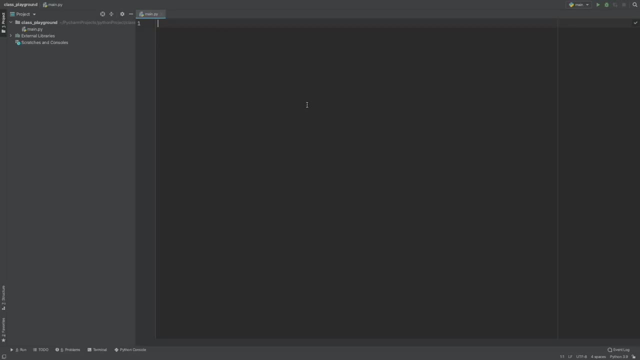 Okay, I hope you have played around. We've played around with functions and you are now ready to try and become a little more advanced and we're going to try and gear it towards cybersecurity now And I hope you're familiar with maybe the in-map scan and some other tools. 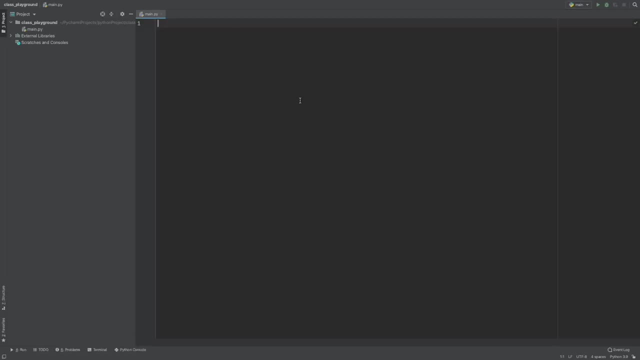 So we'll just use an in-map scan right now And we'll just say, like we're going to call a function and we'll call it in map And this is going to take a variable and we'll actually call it the IP because we're going. 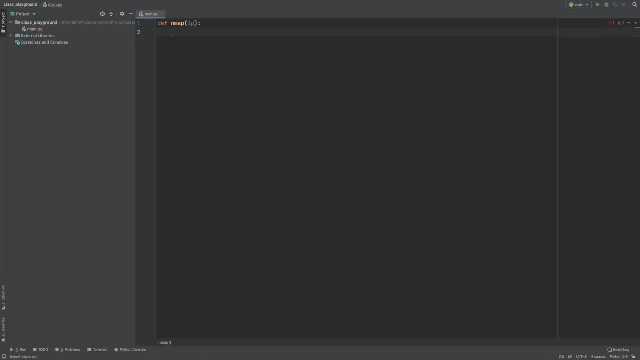 to take an IP address, And the way I like to run my in-map scans is with the. they'll look something like this in map dash, a like this, And then we're going to pass in the IP address and then I like it to be verbose. 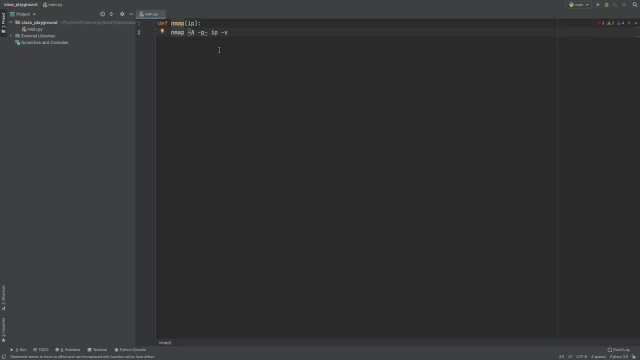 Now, in order to get this to run, we would have to import a module called OS, but we're not ready for that, So this is just to show you how the functions will work, And so I will wrap this entire thing inside of curly braces. 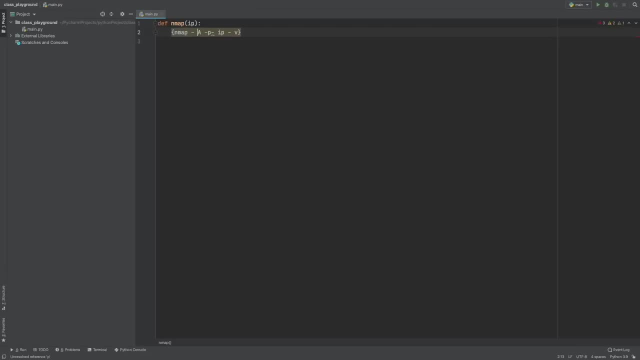 I got dashes in here that shouldn't be there. I don't know why I did that. And then we'll wrap this inside curly braces. This is not supposed to be inside curly braces. That is supposed to be inside of quotes. and we'll make this an F string and we'll say: 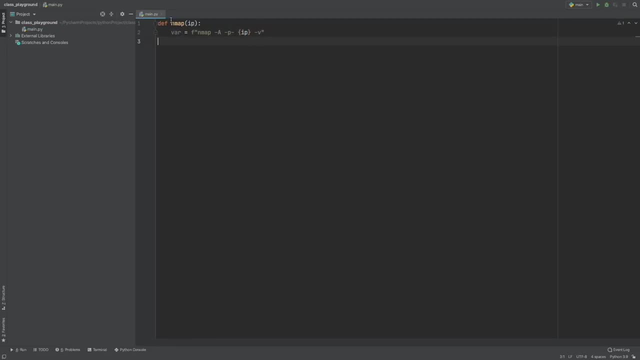 okay, this is our variable equals. instead, this would be an OS command If we were actually going to run this in our Linux machine or windows, whatever you choose to use as your hacking VM. And now what we do is we'd come down here and we would say, um, something like in map: 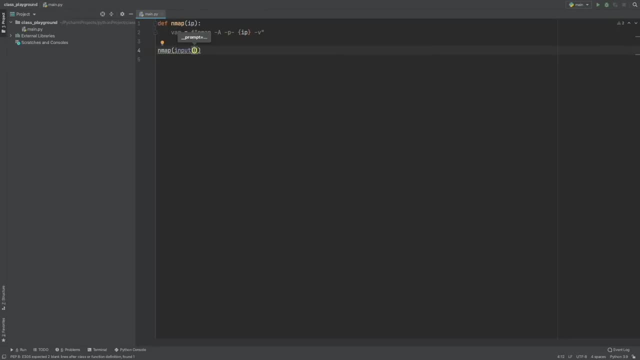 to call our function And then we're going to take an input and we're going to say: what IP would you like to scan? And then right here You're going to print running in map: scan against. and then we will put in the IP address. 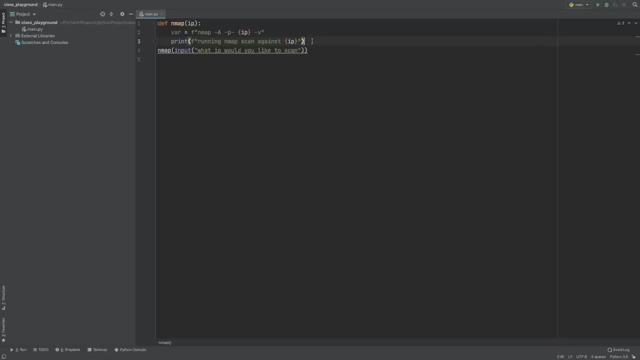 and this will need to be an F string. So the way this, or sorry, that will not be the IP, that will be against the variable. So it will tell us that it is running the in map scan right here. Okay, So when we run this we can say: what's w? who would we like to scan against? 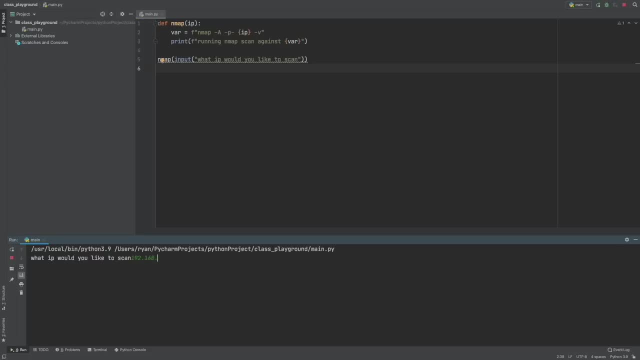 And we'd say 1, 9, 2.1, 6, 8, point something, point something else. Then we run this, it'll print running in map scan against and then it gives us the output right here. So this would be a way that if you were trying to write your own tool to automate your recon. 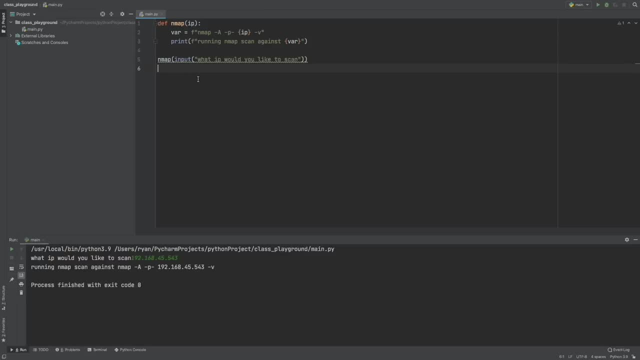 this would be one of those ways. you would use a function in order to automate your, your recon, And there's a lot more you can do with this IP address and you could pass it into multiple different tools, And then you have written your own tool. 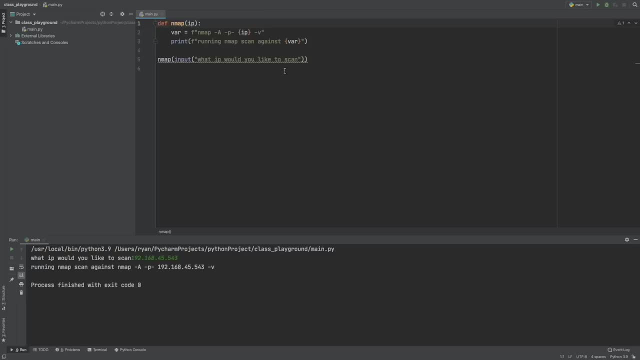 So this is how we can use functions in cybersecurity that are really helpful for us, And whenever you're going for a certification, it'll be really helpful for you to be able to read through functions and maybe modify them, especially in exploits, because vulnerabilities and exploits change over time. 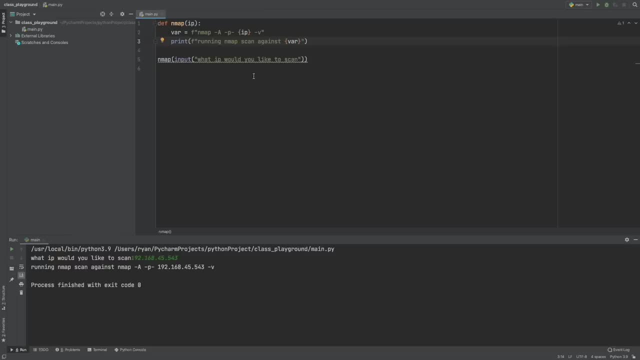 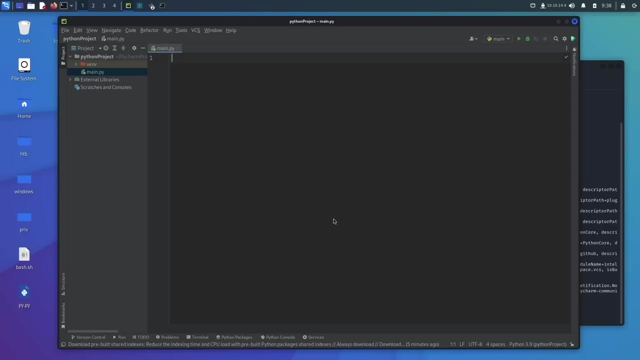 And you will need to be able to Change and modify different X different exploits that you come across on a Google in order to gain access to a machine. before we end this course, I want to give you a little bit of an introduction into making your own tools. 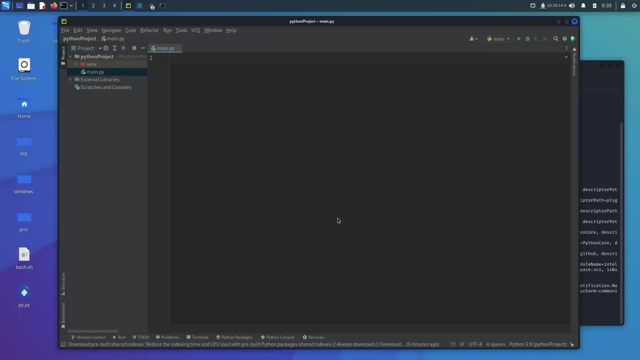 And then I want to challenge you to add to this recon tool that I'm about to show you and you can start to build your own tool for Recon And You, If you remember the Python code that we've gone over so far in this course. 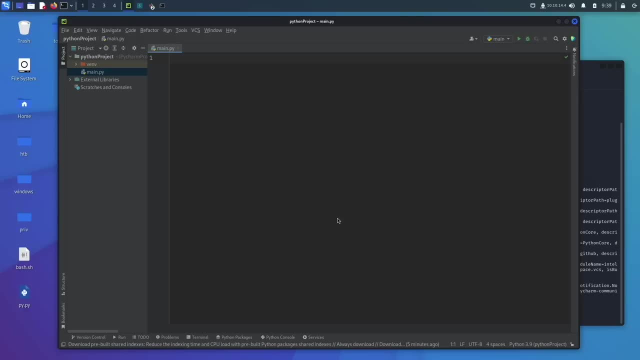 So I've gone ahead and connected it to hack the box and launched the box develop, And so I want to just show you what OS system does. So we'll import OS system. You've seen this before and this is just our operating system. 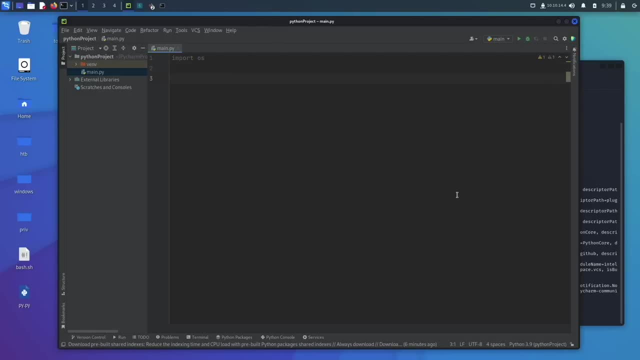 It just means we're going to be able to tell our Linux machine to carry out commands the exact same way you would inside of a terminal. So we're going to make a function, Okay, And we're going to call it recon, And we're going to pass through an IP address. 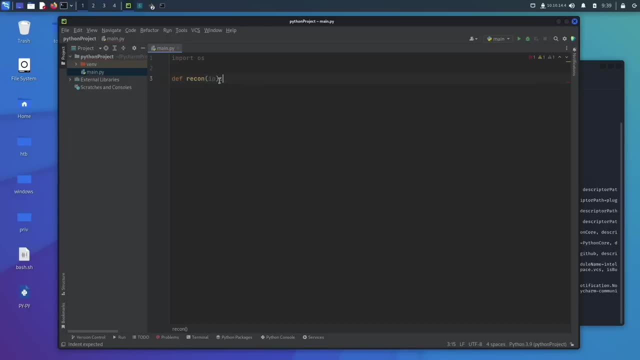 Really, if you remember, this is just a variable that we're going to be passing through into the function, And then we're going to call our function down here and we'll just call it recon, And then we're going to ask for an input and then we're going to say what IP would. 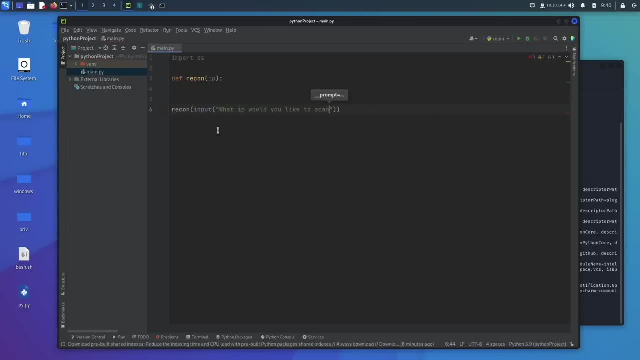 you like, And then we're going to say what IP would you like to scan, And then we'll put a question mark and a space there, so that way it's not all smashed together. And now inside of here, what we can do to make this program run, our recon and automate. 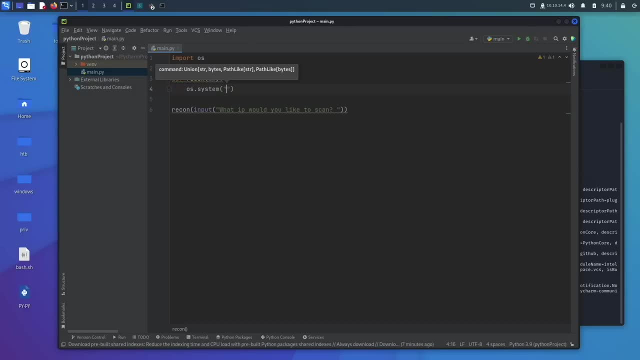 it for us is we can type OS system and then we can put in here. we're going to make this an F string what we want to do. So we're going to run an in-map scan and we're going to run it on all port, or we're going 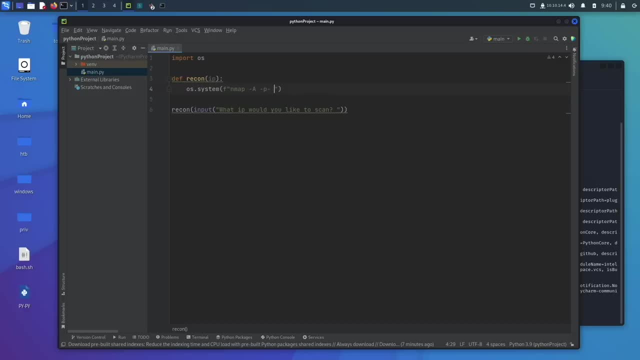 to want all outputs, We're going to run it on all ports. Okay, So just in case it is blocking the ping, we'll put the P and you don't have to put this in here, It's optional. And then we are going to put in the IP address that we run through. 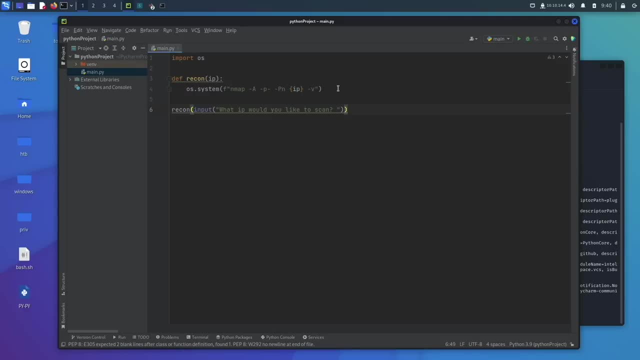 And I really like to run everything as verbose. So this: when we run this, you'll be able to see. it'll say what IP would you like to scan And I'll put in the IP address and it will now start the scan for us. 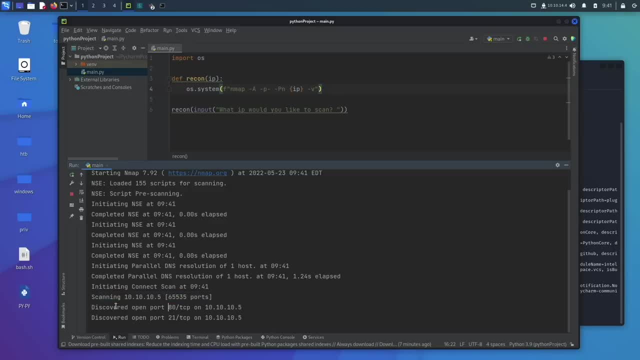 So this is the same thing we would see inside the terminal. We're going to see port 80.. Port 21 is open And at the end of the scan it will tell us everything that has happened on this scan. Now you can add to this. we'll stop this. 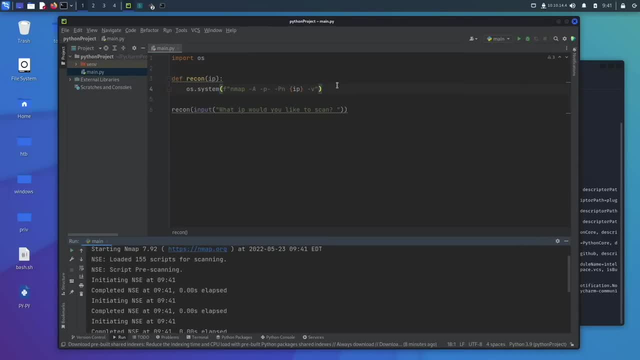 You can add to this same scan. when it gets done running the in-map scan, you can come down here and maybe you want to look for different directories, And so you could go ossystem and we're going to make an F string, Okay. 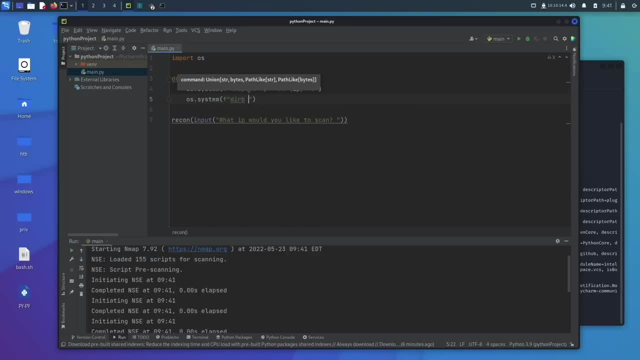 And we can add in: maybe we want it to run derb and we want it to run on the same IP address that we've already passed in, And it will now launch this right here as soon as it gets done with in-map. 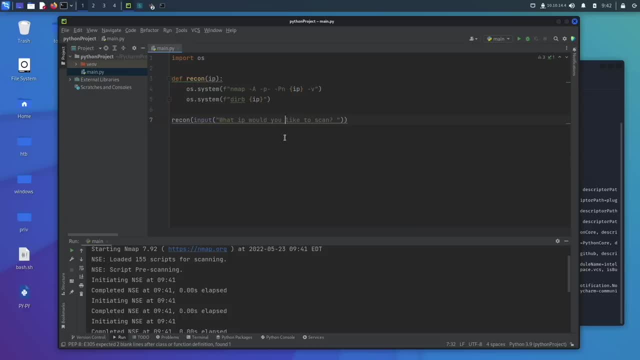 And the cool thing about this is if you have your own recon tool set up, you can go ahead and run the program, send over the IP address and then you can leave and it will automatically run your recon, Or maybe while your recon tool is running. 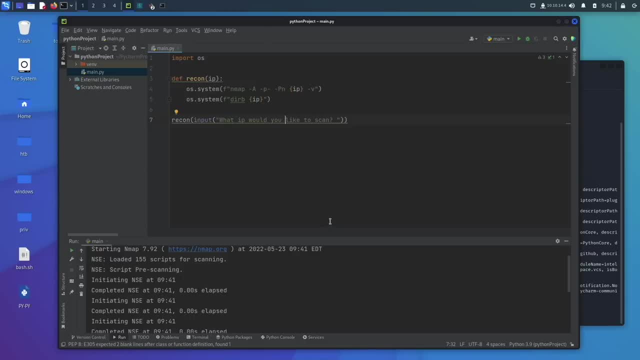 Okay, You can do other more manual enumeration. Maybe it has port 80 open and you see that real quick with the in-map scan And you want to start looking at what's on port 80 and it will run your in-map scan. 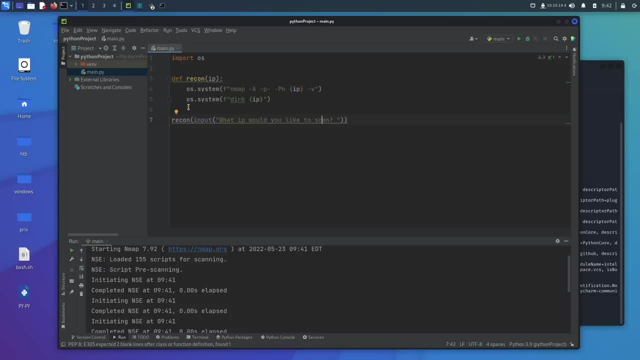 It will run your derbuster for you, And maybe you want to run W fuzz or maybe you want to run a sub lister. I want you to go ahead and start off with what I have given you right here, And you can add to this tool with the information that you have learned. 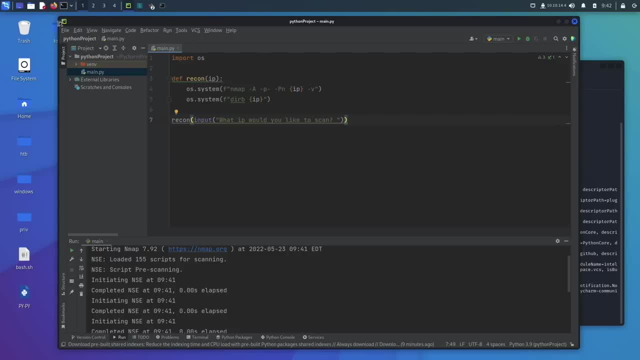 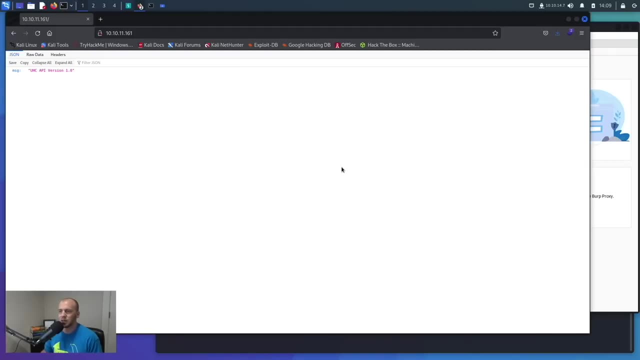 That you have learned so far. Okay, so in this video we're going to be covering enumerating APIs, or backend APIs, And I see this in bug bounty programs sometimes, and I'm sure you guys have come across a page that looks exactly like this. 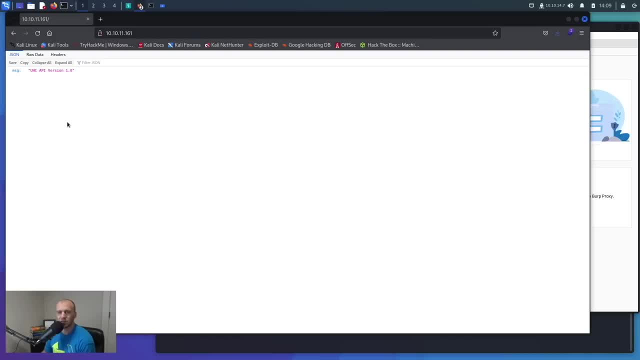 You come in, you go to the URL and you get some JSON in return. And I actually was looking through a bug bounty program just a few days ago and I actually saw it said backend And I was like what, What, What? 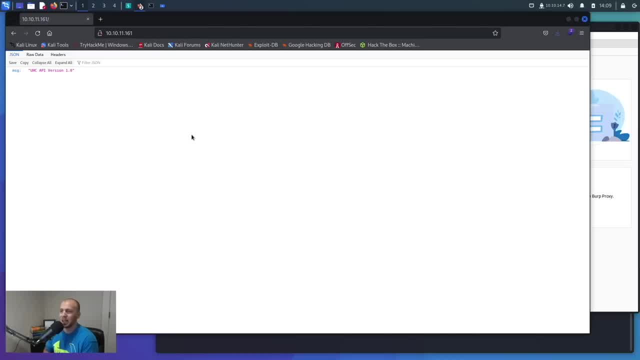 And then API dot, the program, dot, com, And so if you're new and you're not really sure how to enumerate APIs, then this video is going to be for you. We're going to keep it really short and specific, So the way you can go out and do this yourself. 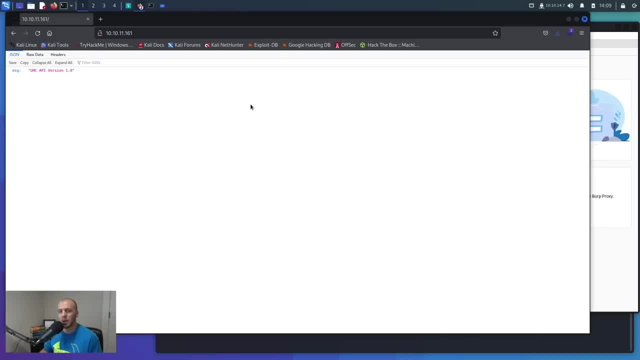 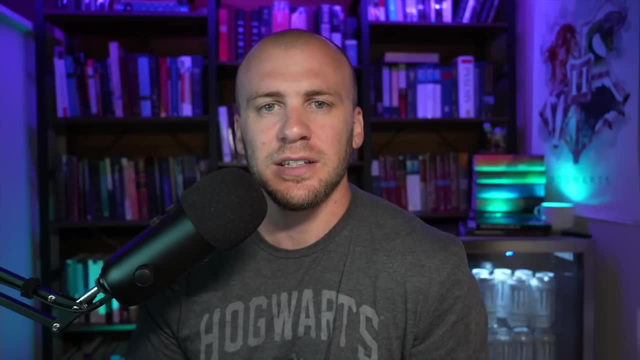 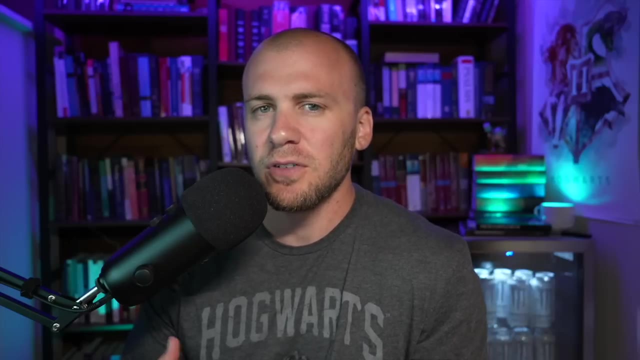 We're going to be looking at the box backend on hack the box, but we're not actually going to walk through the box, All right, So I have decided to include this little section here on making a GitHub recon tool tool in Python for you, because I figured, if you have went through my first bug bounty course, I 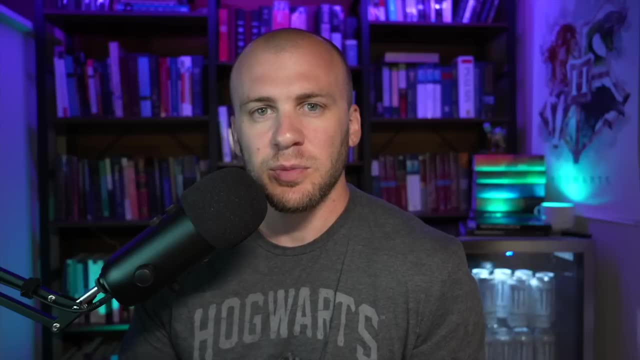 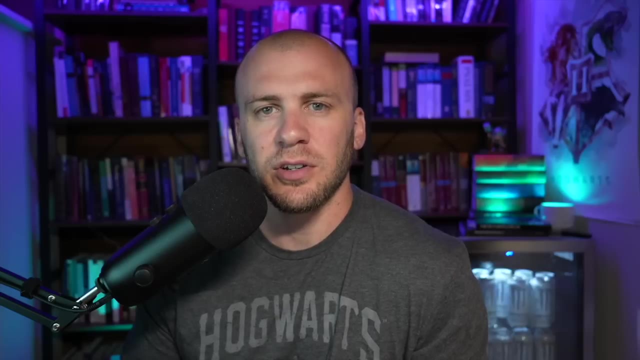 had this section on the understanding the basics of Python, and as you become a more well-rounded bug bounty hunter or penetration tester, your programming skills are going to improve as well. so I decided this tool was easy to make. it includes a lot of really easy concepts within Python. 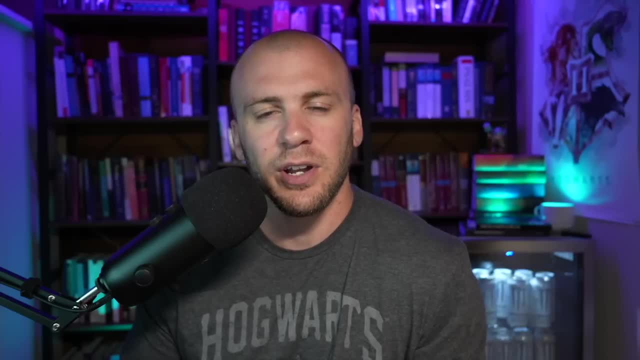 but it is actually a lot of code. I guess if you are a beginner, if you're going to continue down the road of penetration, testing or bug bounty hunting, you're going to want to develop your own tools and have a better understanding of Python, and I figured this was a really great tool. 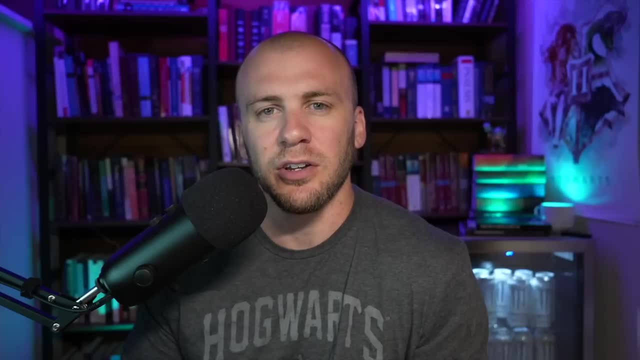 to give you an idea of things you can actually build that are useful. and even with this tool, you can add on to it and make it your own and give it new functionality. so I've decided to include this in here because it will help you and save you time in the future if you decide to. 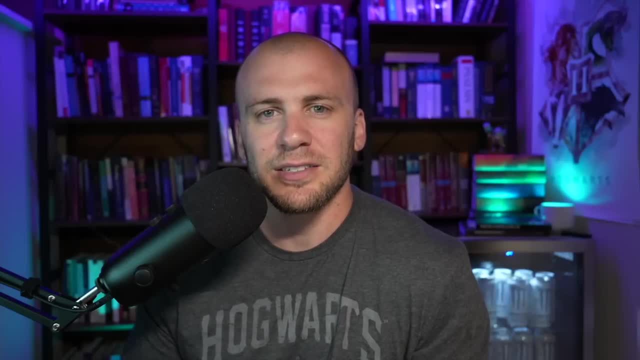 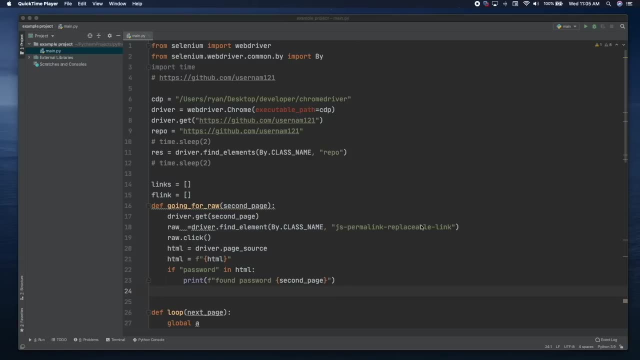 continue bug bounty hunting. so enjoy this tool and use it well. Okay, So the setup for Selenium is going to take a little while, and I don't want you just to close out and think this is too hard. I want to show you how cool this tool really is. so if you follow along, 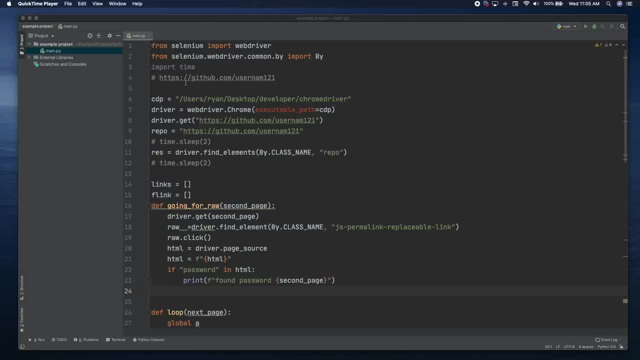 with this video. in the end you're going to have a program and you're going to understand all of this code and then you're going to have a program that goes out to GitHub for you and goes through the repos, opens all the pages, goes through all the links and pulls out if there's any passwords or 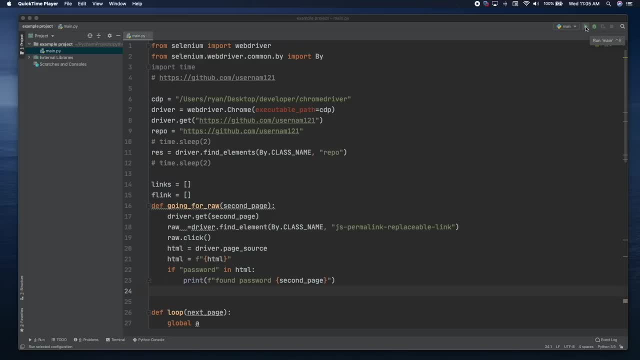 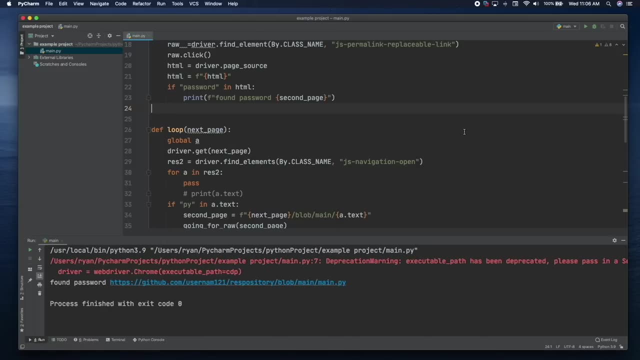 not stored in the code on the GitHub page, and so it will look like this when you run it. And it automatically went through all of those links on GitHub. it pulled down this page right here. it says a password was found at this link and so if we click on this link it'll take us to this page. 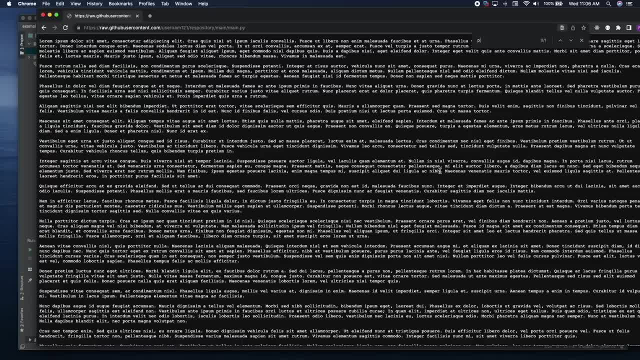 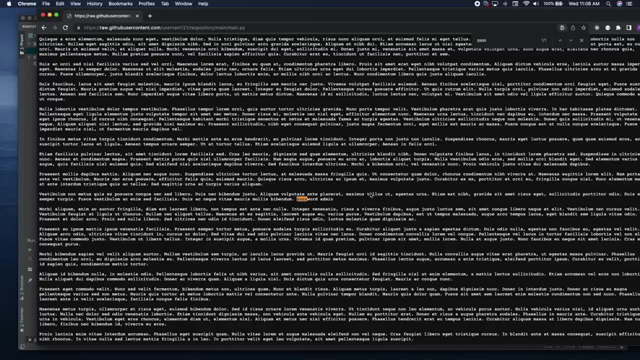 right here and we can look at this, and we can go to the raw and we can type in password and right here it tells us it has found a password and the password is admin and it found this on this GitHub page. So that is where we're going. 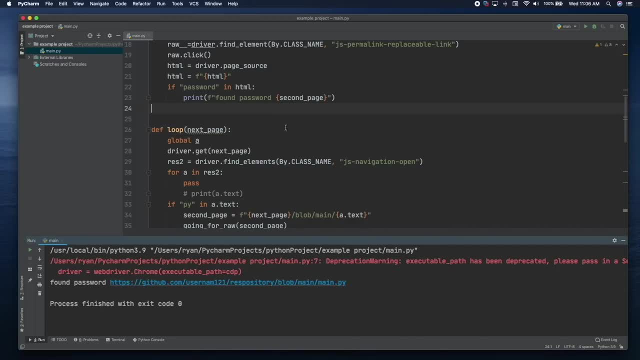 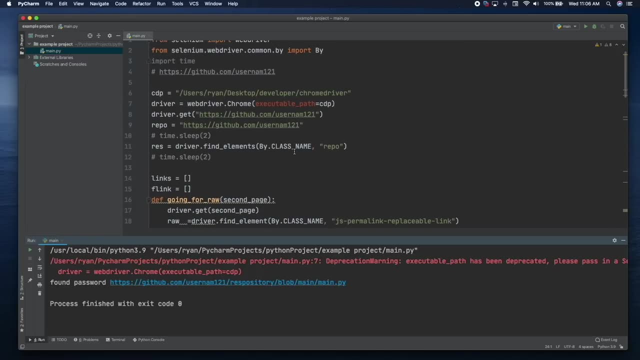 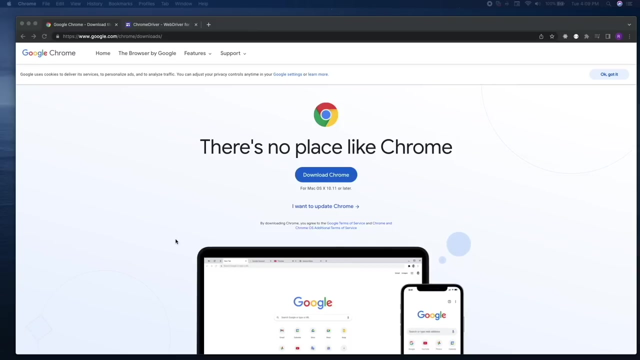 And if this tool looks like something you would like to add into your bug bounty or a penetration testing arsenal, then you can stick around and go through and make this tool with me. We start with our program and using Selenium. there's a few things that you have to do and I'm 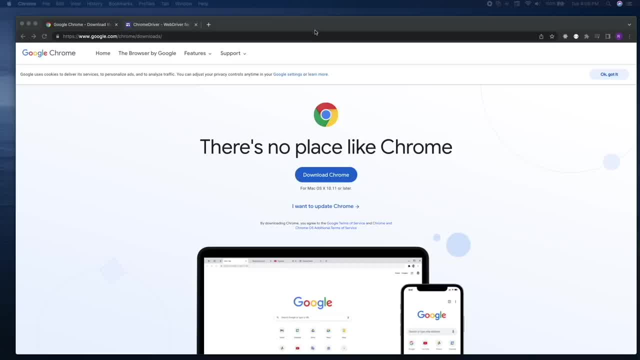 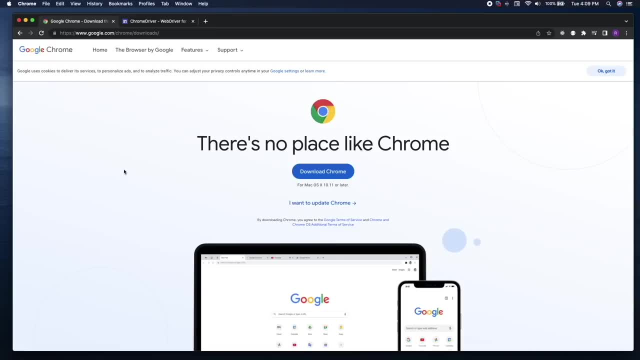 going to walk you through installing this both on Mac and Windows. You will need your PyCharm editor that we used in the first Python for ethical hackers, and now you are going To need Google Chrome installed, and so I'll have this link down in the description if you don't have. 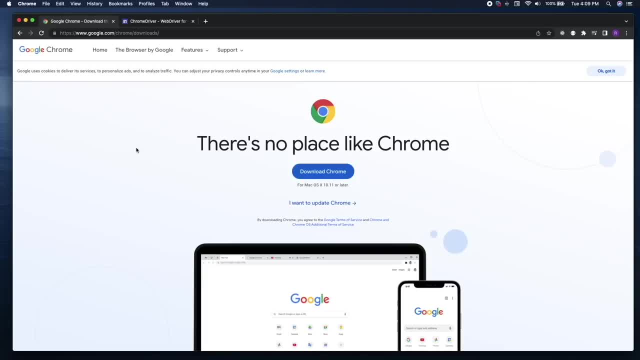 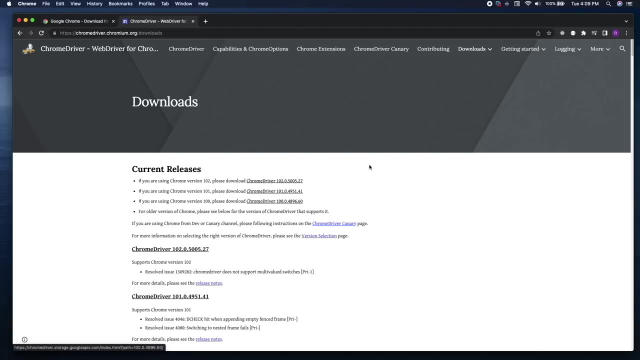 Google Chrome. it is best if you use it. you can also do it with Firefox, but it's really easy if you just download Google Chrome and follow along with me, and we're going to also need to install the Chrome Web driver. So what you will need to do is download the version of the Chrome driver that matches your Google. 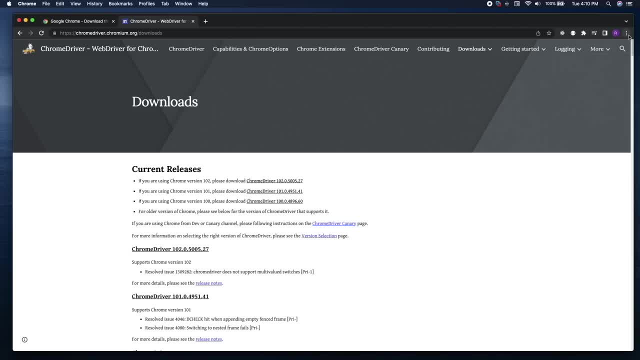 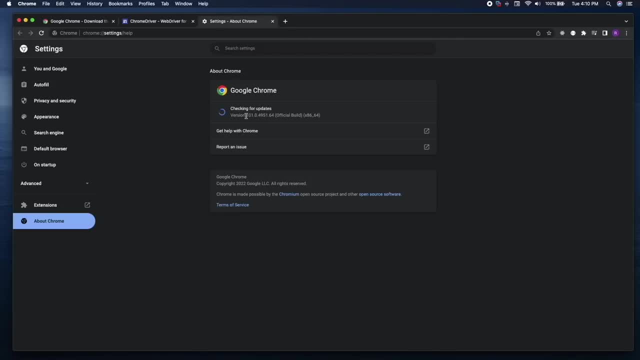 Chrome installation in order to find out what version of Chrome you are running. You will Come up here, click the three dots, you will go down to help and you'll click about Google Chrome. and then I am running this version right here in order for me to update my Google Chrome if it doesn't match any of these over. 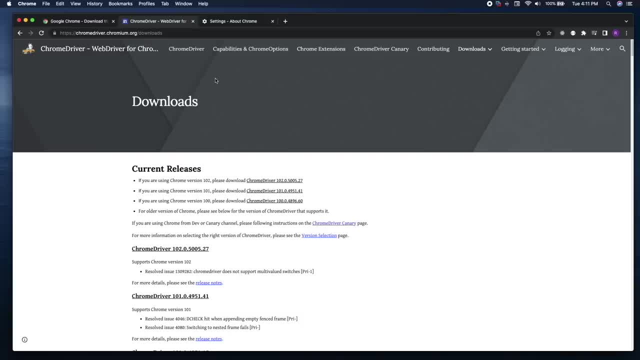 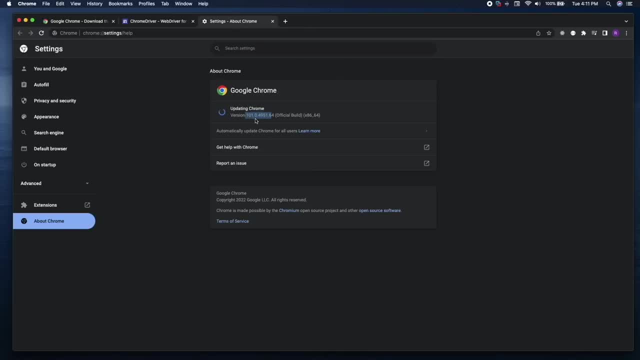 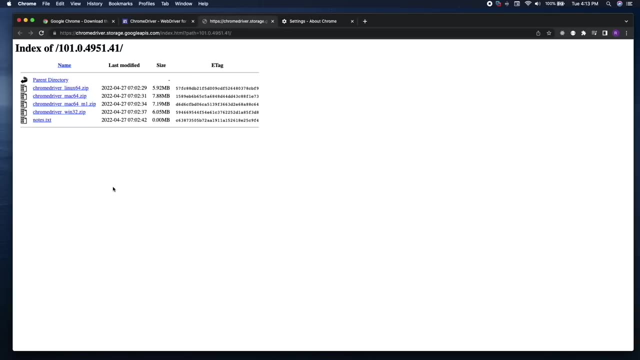 here, then I would just have to close out of Chrome completely. you just go and close the app and it will automatically update. and I am running this version right here: 1 0, 1.0. and I would come back over here and I would say 1 0, 1.0, for me it would be this one. I would click this and then it will bring you to this page. looks. 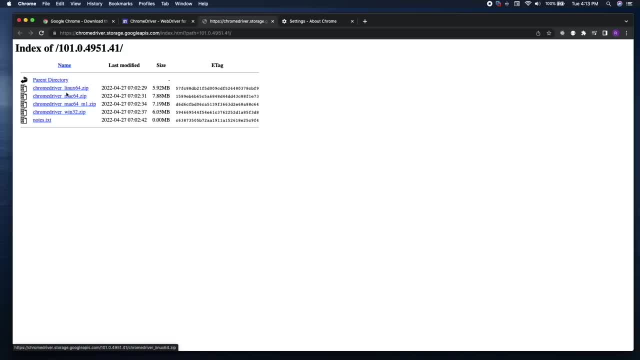 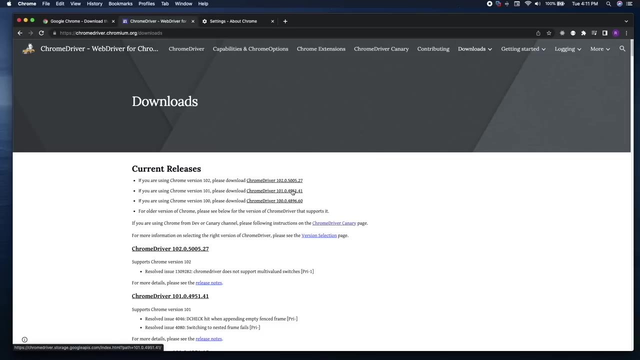 exactly like this and it will tell you what version of software you're running and you will click that version. so if you're running Windows as you're operating software, you click Windows, Mac, Mac or Linux for Mac. I use this one right here- and when you install it, remember where you put it, because we are going to need to know the. 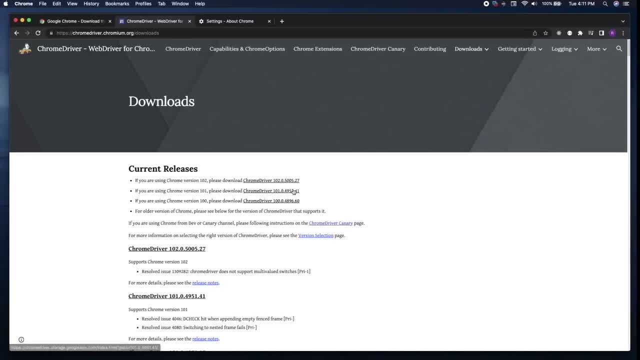 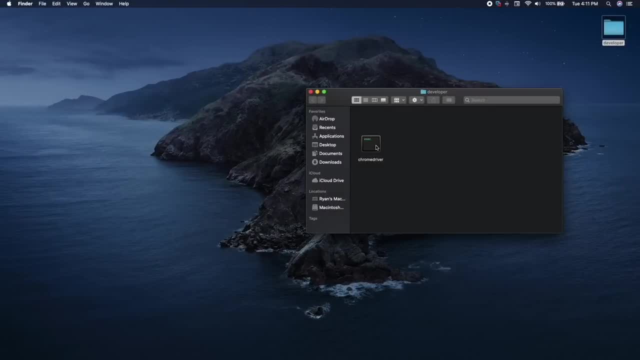 complete file path in order to reach the Chrome driver. I have mine stored right here in a folder on my desktops. So if I, if I open this up, I have my chrome and driver right here and I will need to know where this is. we will need to know the entire path and you can do. 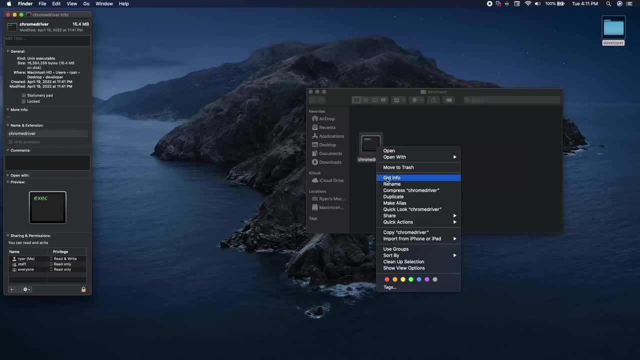 this. you can see the full path by clicking, right clicking and going to get info, and then it will tell us where the full path is, right here, that other swear. and then we say Mac user Ryan desktop, the folder is developer. and then we hit the chrome driver so you will. 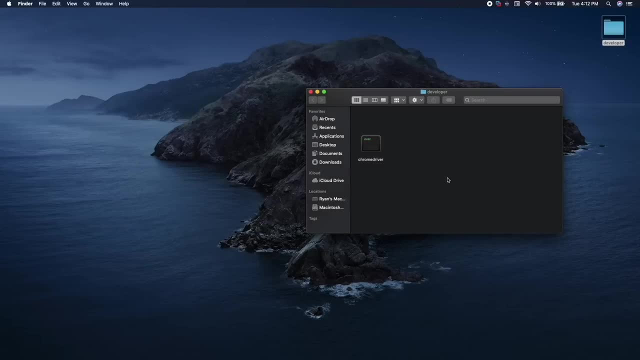 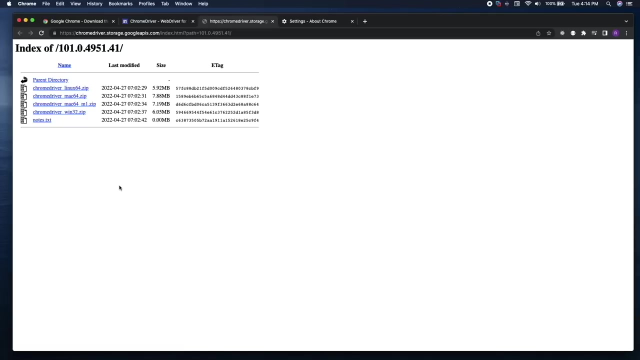 need to go ahead and install Google Chrome and then install the Chrome driver, and we will continue walking through how to finish setting up Selenium. when you have finished doing that, After you have downloaded the zip, go ahead and unzip it and it will automatically unzip into your downloads. and 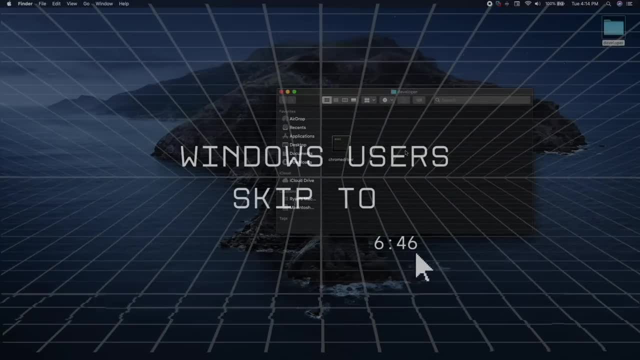 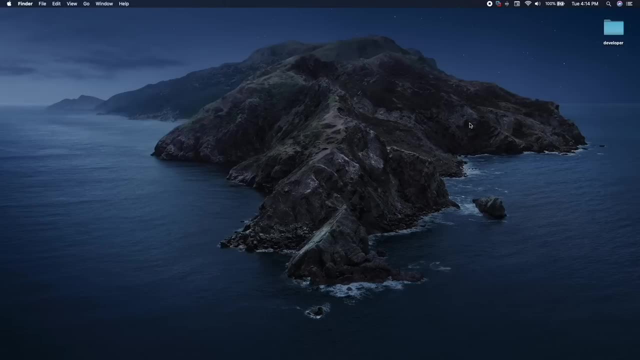 then you can drag it into a different folder, like I have. I've just made one called developer, and you can go ahead and drag yours out of your downloads or you can leave it in your downloads, if you choose. The only reason I move it out of my downloads is because sometimes I go and delete. 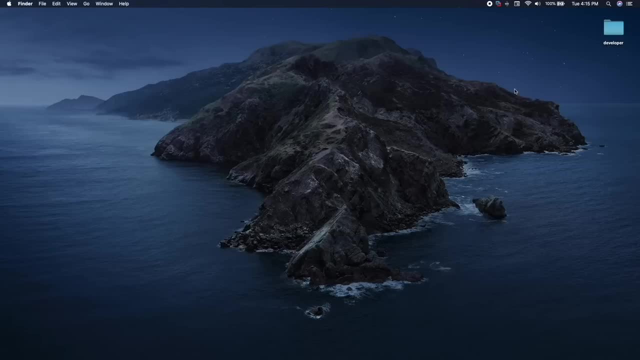 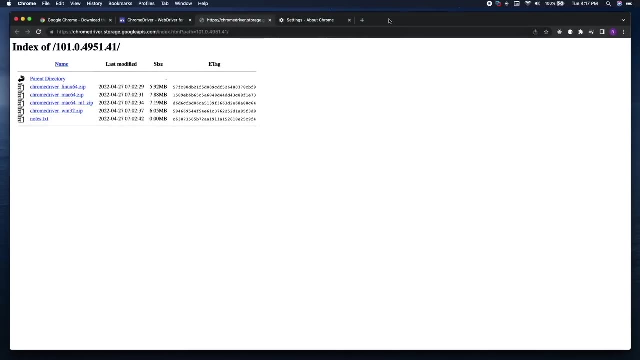 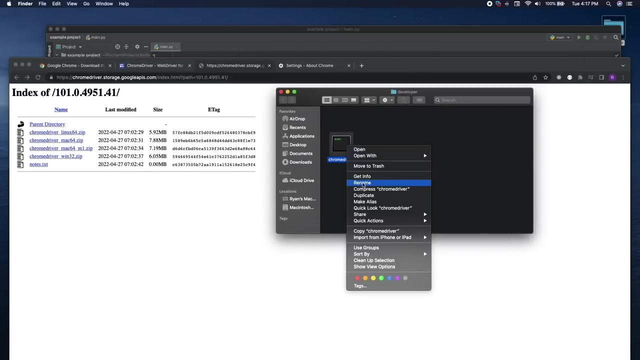 everything out of my downloads folder and I don't want to delete this if I am using it For the Mac users. after you've downloaded this and you have moved it into your location where you would like to keep it for me, I'm going to just go like this: I will open back up this folder. I'm going to show. 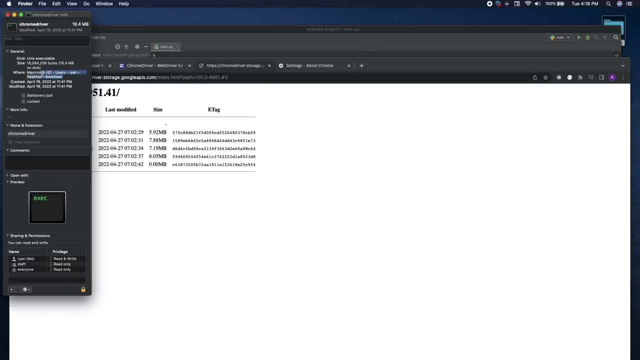 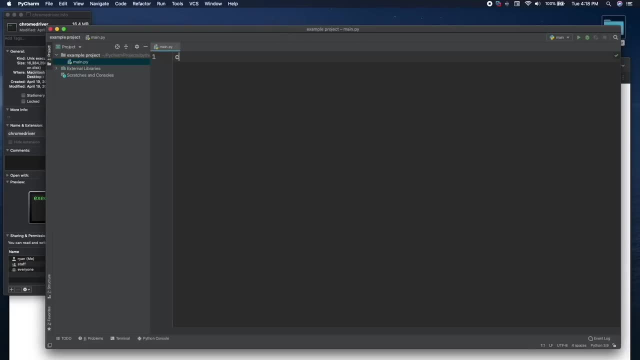 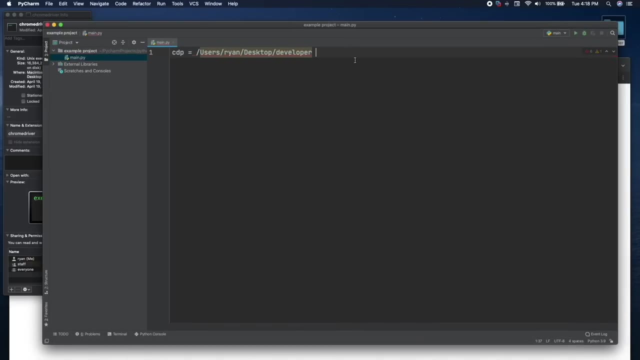 you what we did earlier: Just go to get info. You can now copy this as your full path And then we can say: our Chrome drivers will go CDP for our path. and then you can paste it in here just like this: And I believe we need our to go slash Chrome driver, So we'll go slash Chrome. 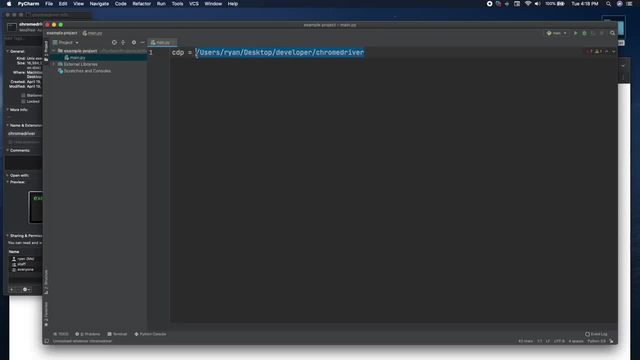 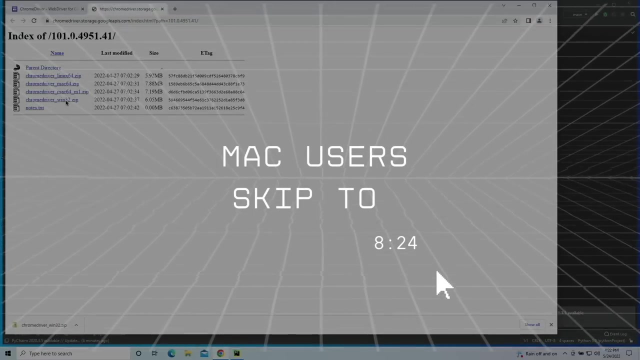 driver, and this entire thing will need to be inside quotations. Now I'm going to cover the installation of Selenium for Windows users. Okay, for our Windows users. what we're going to do now is click Chrome driver Win32 and it will download. We will open up where this is. It's going to say: 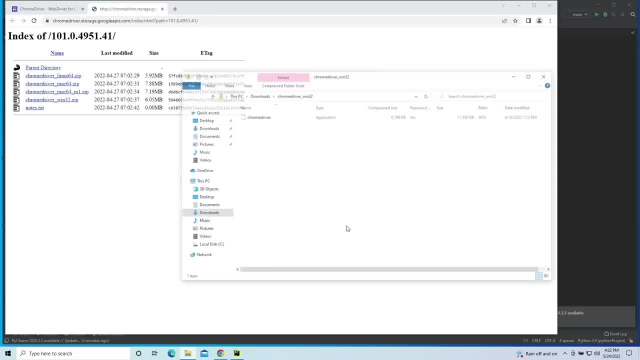 we want to. how do you want to open this file? We'll just say we'll just go ahead and open it. It says we now have this Chrome driver and it tells us that this is an application. If you don't have any place in particular you want to store it, go ahead and put it in your C drive. But 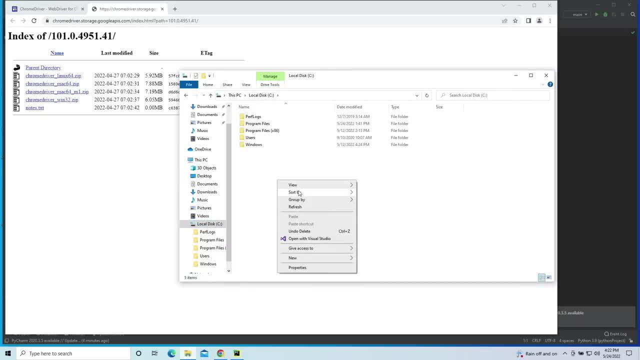 before we do that, we'll just open this up, We will make a new folder and do the same thing we did on the Mac and we will say developer and we'll just leave this here and we can go back to our downloads, where we grabbed this folder and we extracted our Chrome driver and we're going to put 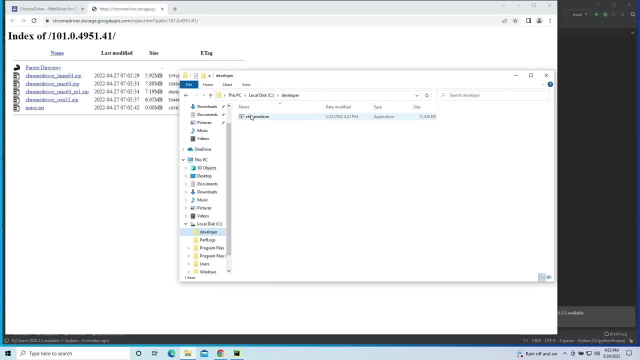 this into the developer. Now, the reason I had you do that is because when you look at the location of where this is stored, it is really simple to get to. It tells us that it is in C slash developer. We can copy this. We will. 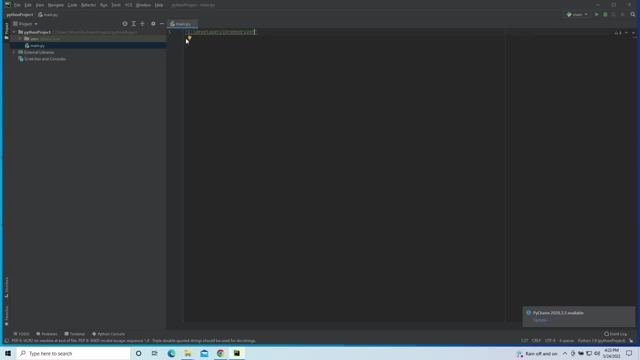 put it inside of a string and then we will put slash, and now we will do the same thing we did on the Mac and we will say the Chrome driver path, and now we have that stored as a variable. Sorry to my Windows friends, I forgot to mention that when you run this Chrome driver, you will need 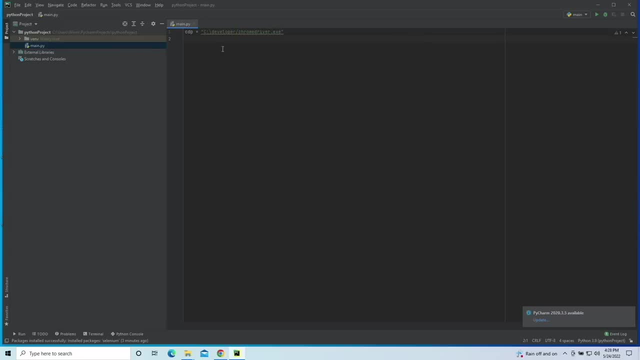 to have the executable to run, and pretty much everything from this point on is going to be the same, as I run it on my Mac. If you have any problems, please let me know in the comments and I will try to help you out. Okay, we are ready to install Selenium. So the way we're going to do, 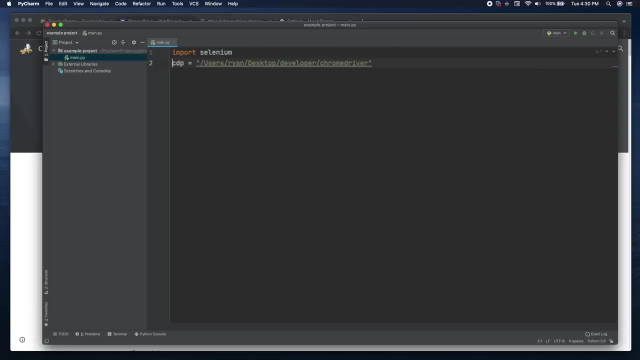 this is: we're going to import Selenium, just like this, And, because I have done it before and I have already installed it on my Mac, this is here and ready for me. But what you may need to do is it wiggly line and it'll pop up a window like this and you're going to click install or import. I. 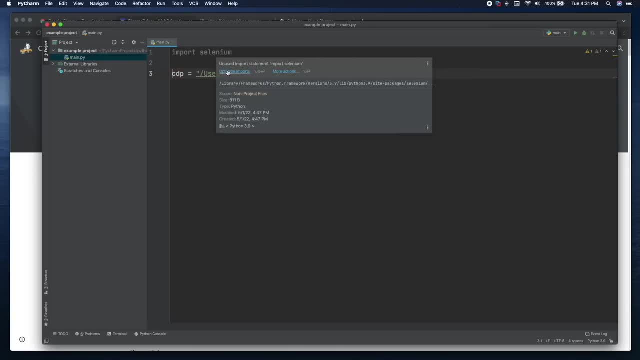 can't remember which it is, but I think it's install and you'll click install and it will take just a second to go ahead and install that, and then what you're going to want to do is type in from selenium, and then we're going to import the web driver Now that you have installed selenium. 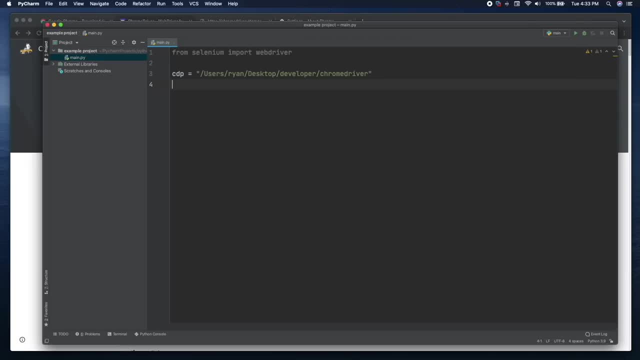 and typed in from selenium import web driver. we're going to initialize our web driver and we're going to type in: driver equals web driver dot chrome, because that's the browser we're using. There are other browsers, if you've chosen to go that path, and now we're going to type in our executable. 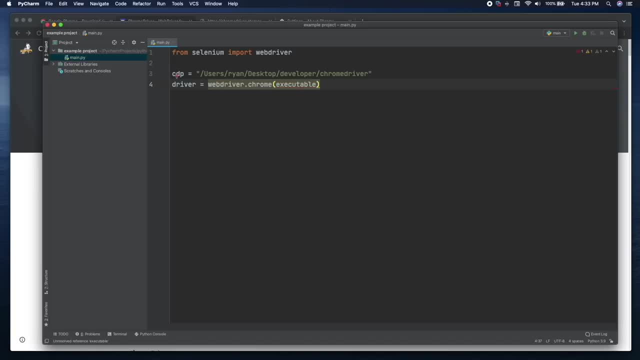 path and the reason this is yellow is because this has to be capitalized like this and we're going to type in executable path, which I believe is actually deprecated, and I have not gone back and read the documentation For the new way to run this without the executable path, but we're going to type in cdp, it's just going. 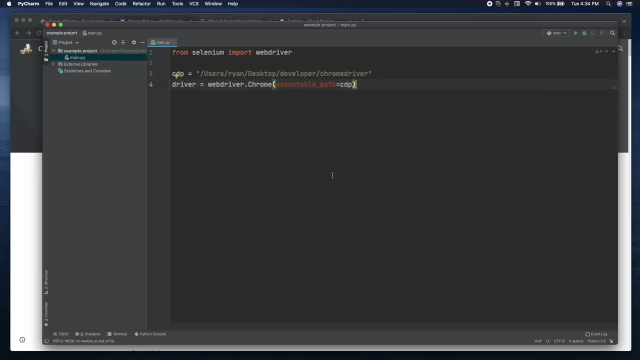 to give us a error when we run this or it's just going to give us a warning saying that this is this version is deprecated for running the window, the web driver. but that's okay, we will get our program to run without it. It just means that they are not updating the executable path like this. 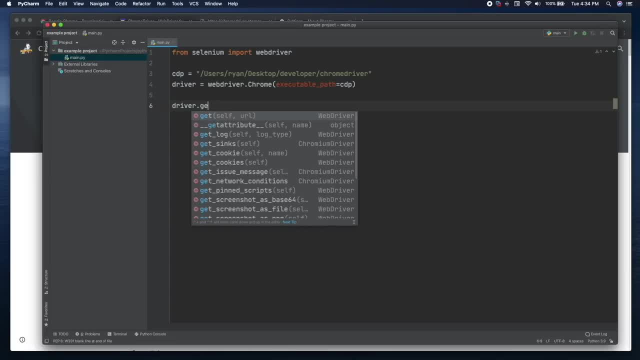 anymore. and now what we're going to do is type in driver dot get and then we're going to type in something like www dot google dot com and then, once this is done, we're going to want our driver to close the window. so you can type in driver dot close. but I don't like to use. 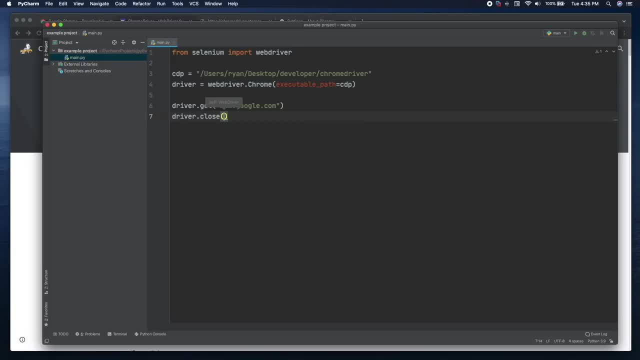 driver dot close personally, because it just closes the window, but we will be still running the chrome down here in our browser. I want it to quit. I want it to close that window all the way out, to save on my memory space on my mac type driver dot quit just like this. and if you run this like i will and you were on a windows, 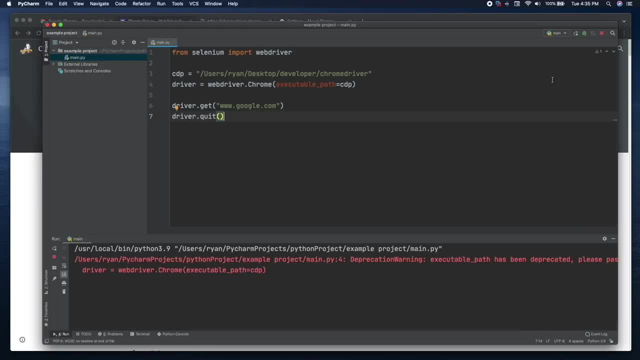 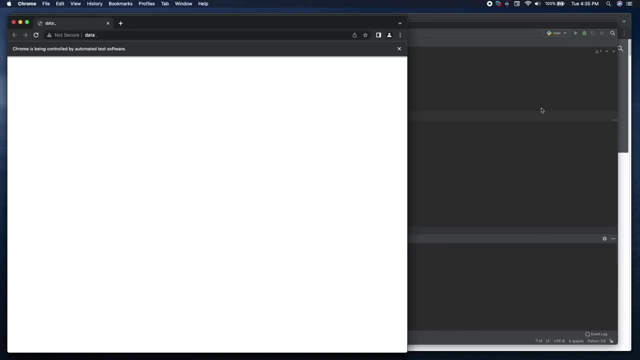 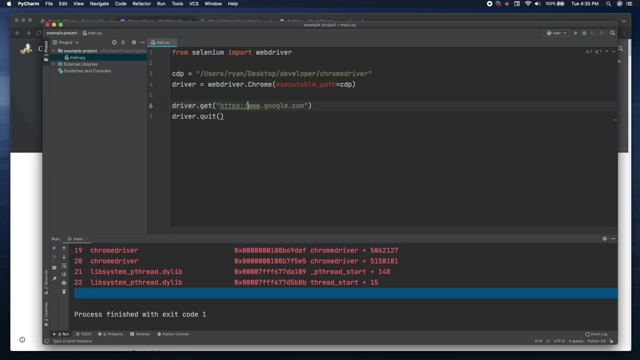 it's automatically going to run for us. it should open without any warnings and give us googlecom, and then it will close this page for us. all right? the reason this is giving this this airs because we need to type in https, slash, slash, googlecom. now, when we run this, it should open up google for. 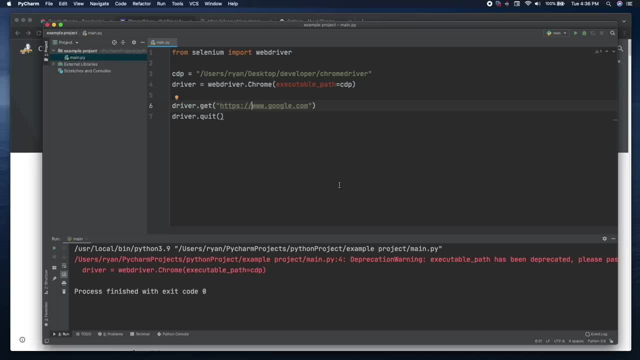 us and close the file. so that is how we run it. but if you're on a mac, if you're on windows, that worked for you and you didn't get any problems. if you're on a mac- and this is the first time you've ever ran selenium- you're going to get a little error that pops up with a window and it's going. 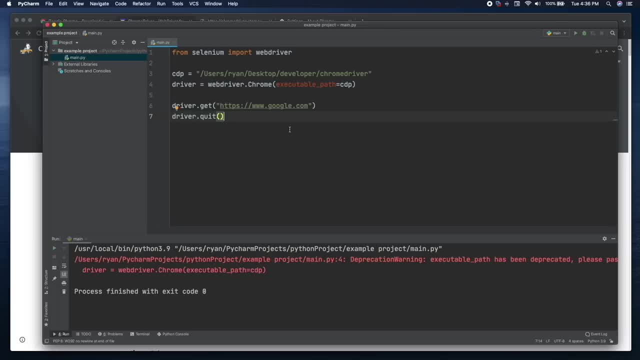 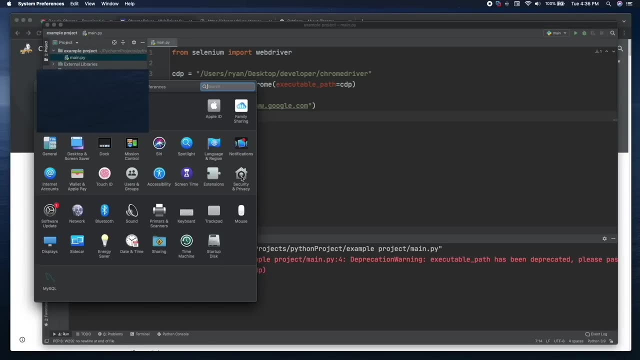 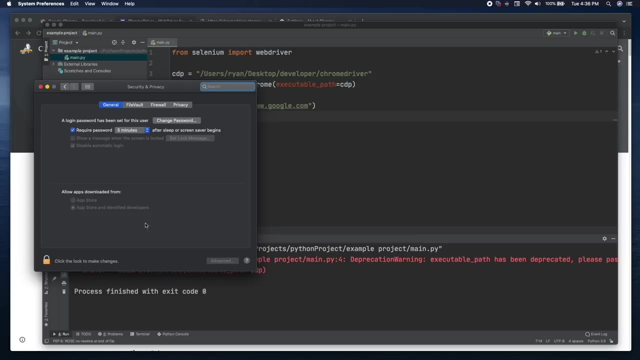 to say move to trash or cancel or close. you're going to click cancel or close, out of your two options. you're going to come up here. you're going to go system preferences. you're going to go security and privacy, and right here it will say that you tried to run a chrome extension and it was blocked. you will click allow. if you're not. 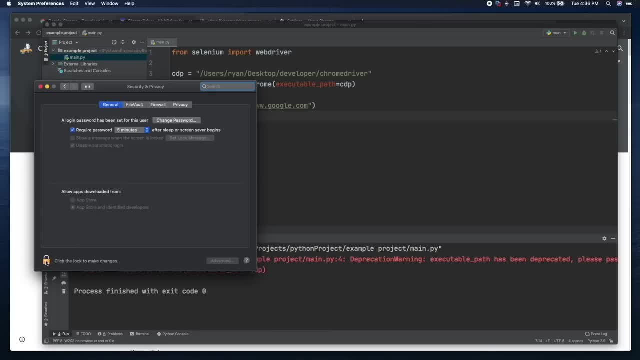 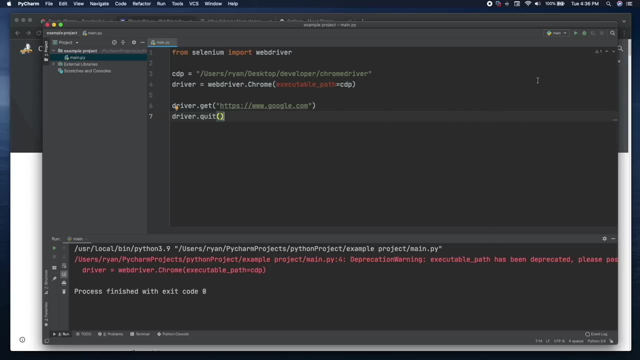 allowed to click allow. you can unlock it by clicking this and typing in your password to unlock your mac and then click allow and then you can relock it. then when you close out of this and you rerun it, it will give you the option to open anyway and you'll have a new pop-up and you will 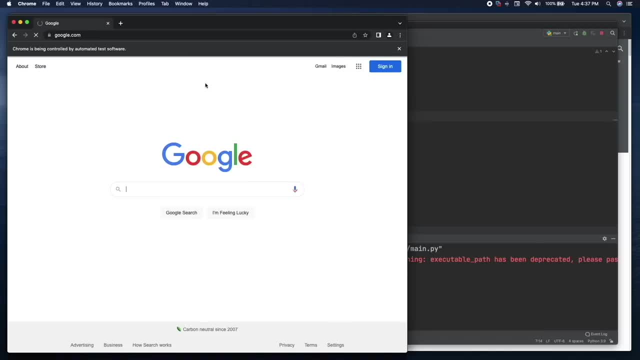 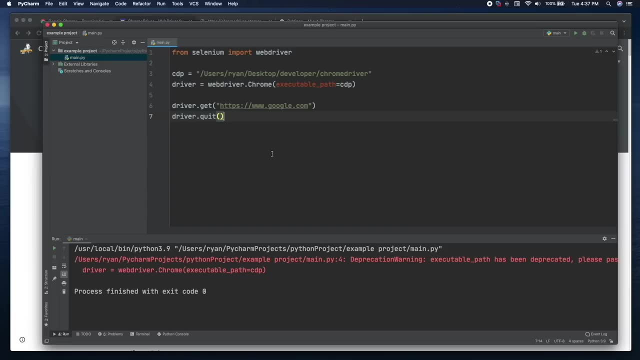 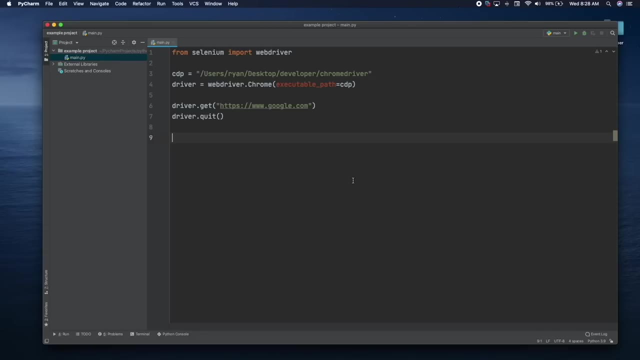 just click open and it will begin running and working for you, just like this on windowscom, your mac. now it is time to begin some of our web scraping. okay, so we are at our screen and it looks like this. i've decided to go ahead and show you how to get rid of this deprecating warning. so when? 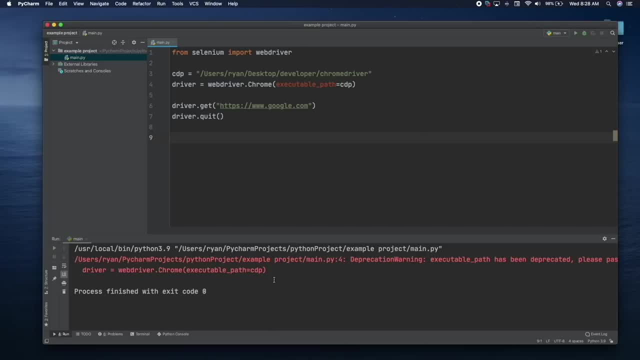 we run our program and it runs this right here, telling us that the executable path has been deprecated. just in case they stop using this in the future, i want to go ahead and show you the way to get rid of this. i'm going to use running the executable. 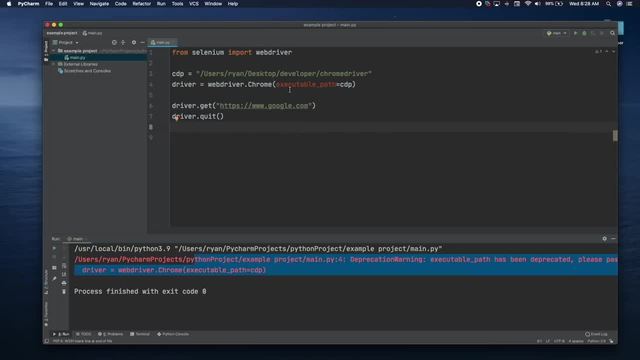 path because i believe that it is faster. and i might be wrong, and that's okay, and you can run selenium however you choose. you can run it the deprecated way or the current version- i think they're version four if you choose- but we'll have to import a few more services from selenium. so 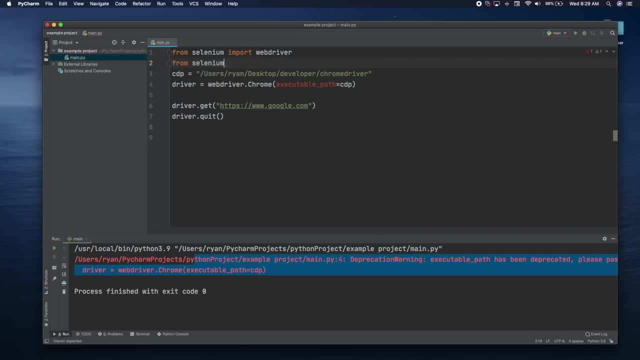 we'll go from seleniumwebdriverchromeservice import and then we're going to import the import service and then we're going to need to import the chrome driver manager. so we're going to go webdrivermanagerchrome and we're going to import chrome drive manager, just like this now. 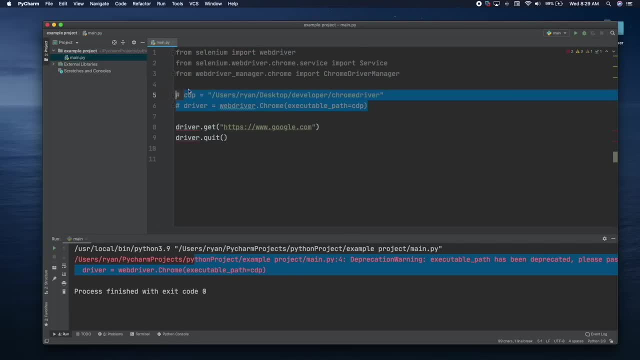 i'm going to comment this out because i'm going to use it as we go through, but you can delete this if you want to use the non, the non-deprecated version, and i think you're still going to get these red inputs down here or these red warnings that's going to tell you like it's installing the. 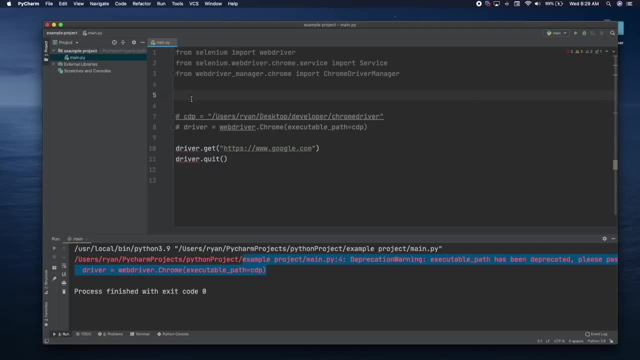 new version of the system. so we're going to go ahead and import this, and then we're going to go ahead and import the newest version of the web driver every single time you run it, but that's okay. and we're going to type in s equals. and then we're going to type in our service. 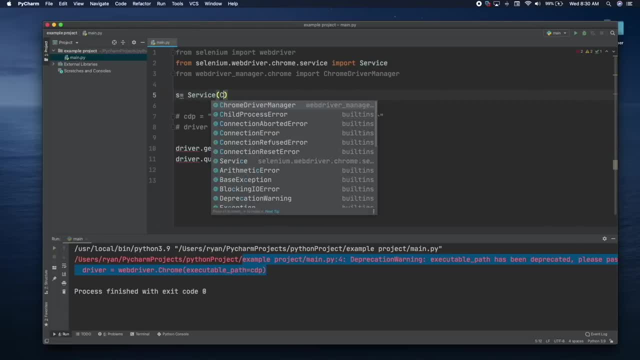 and then we're going to run our chrome driver manager and we're going to call this, and then we will call the install function. and the reason we're going to do this is because every time you run this service, it is going to check to see what version of the system you're running. 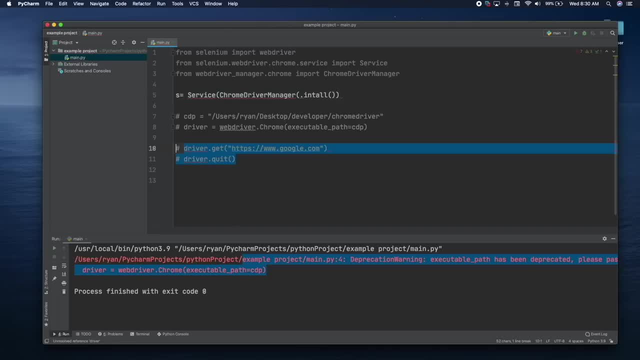 of chrome you are running, so we'll just comment this out. so we're not getting this warning and this dot needs to go. i did this wrong. we'll go like this. all right, it is not wanting to work for me, so we'll close it off manually and then we're going to hit dot install. right here we're. 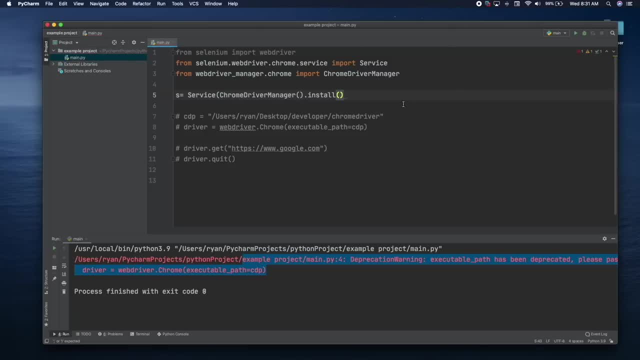 going to call this method, and then we have to close off this whole line here and now. we're going to turn this over to our driver and it's going to equal the webdriverchrome. and then we're going to use the service and it's going to equal s. just like this. now, if we uncomment our driver down here, 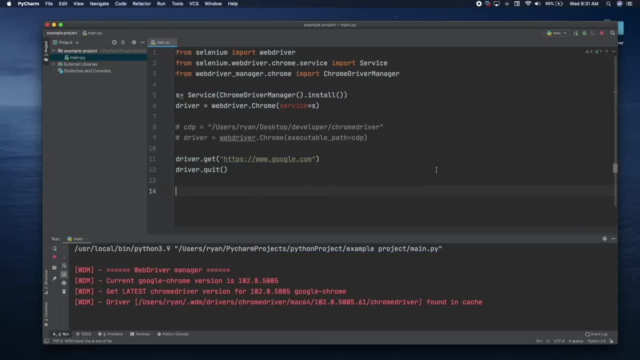 we'll have no errors and when we run this, it will now work for us and it's going to tell us we are using this is the version of google chrome that we're using. if you remember, we checked our version earlier and then we installed the chrome driver and it tells us we have the chrome driver that. 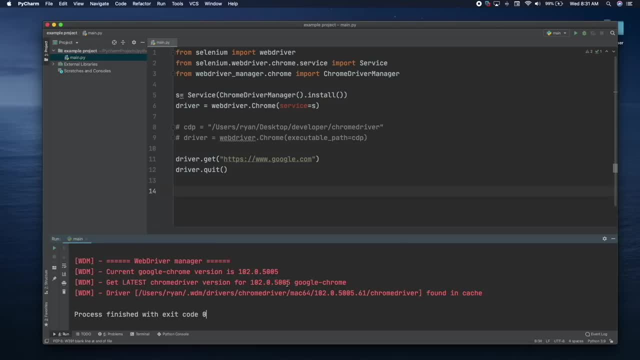 matches our version and it is found in cache, so it now works. this is the non-deprecated way to run this tool. i decided to go ahead and show this to you, like i said, just in case the way right here, the deprecated version to get to the chrome driver, is no longer supported in the future. all right, i. 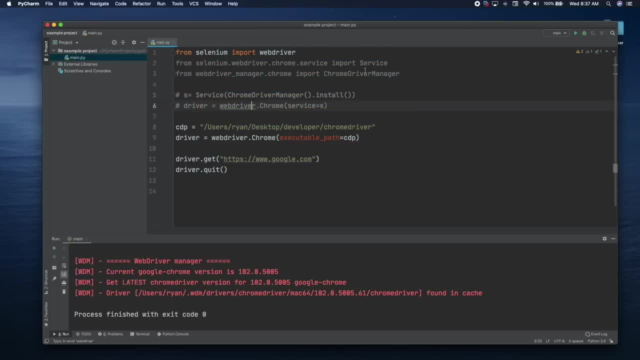 have gone ahead and commented out this code and i'm going to use the chrome driver that is on my computer, that we already installed. there's one more thing we're going to need to import in order to not get any deprecation errors, and that is the buy we're going to import by. 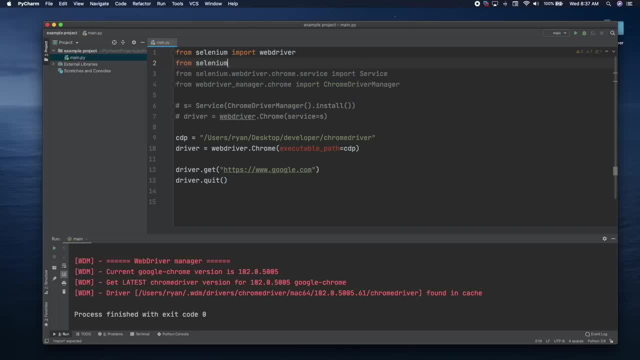 so we're going to type in from selenium dot webdriver, dot chrome or- sorry, not chrome- dot common and then we're going to use buy and then we're going to import and then buy, like this, if i can get back there like this, and this is another update with: 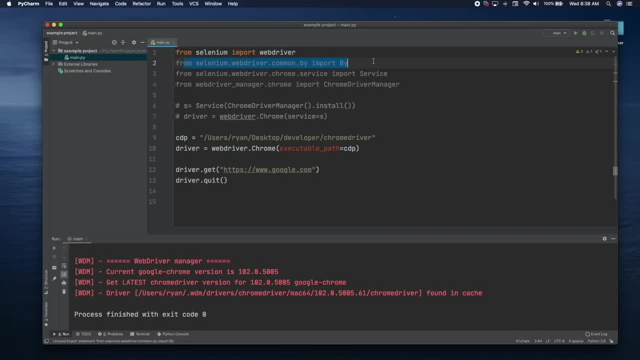 selenium the way i originally learned selenium. we didn't have to use this, but they have updated it again, so we will need to use this by module here. so what we're going to do is open up amazon. i'm going to show you how this scrapes. if you've ever wondered why you have to answer questions to make, 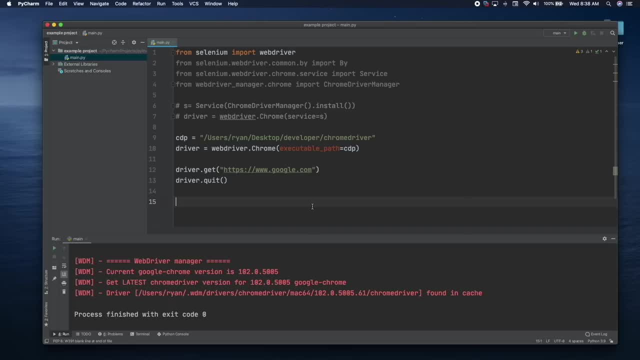 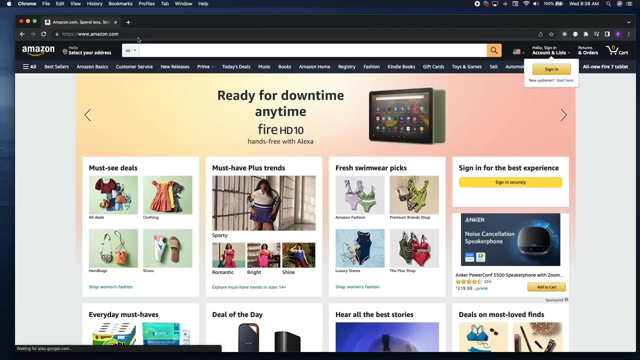 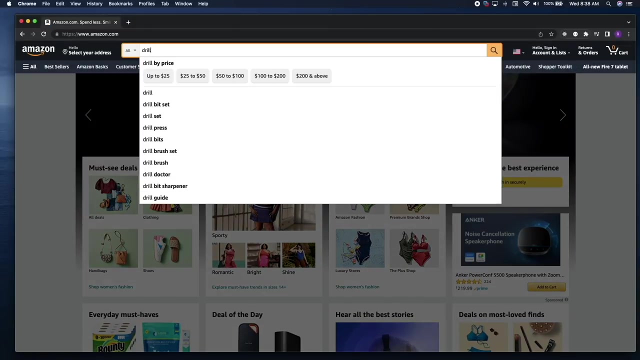 sure you're not a robot. you're going to find out in this course. so if we come over to a web browser and we type in amazon and we go to amazon and let's say we want to buy a new drill bit, so we just say we want a drill set, okay, we're getting a drill set, not a drill bit, and we click on this. 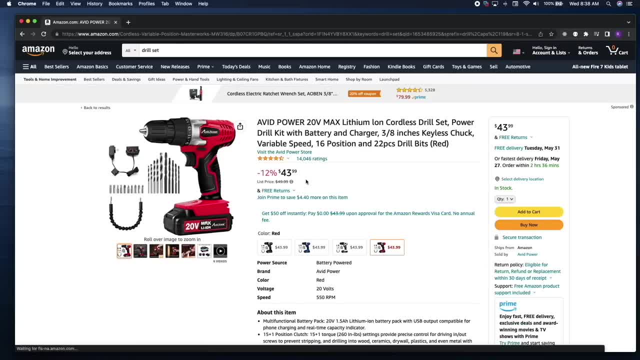 drill and we really want this drill, but we don't want to pay forty three dollars for it. we want to it. we want to pay $38 for it. We can actually set up our web driver to go out and check this price for us. So what we would do is we would inspect this and we can look for the class. 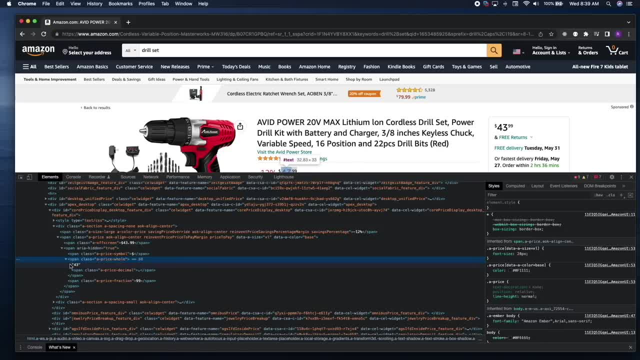 right here And it's going to tell us that it's a 43. So you could set this up, Let's say, instead of 43.99, we don't really care about the 99 cents and we just want it to be less than 38.. 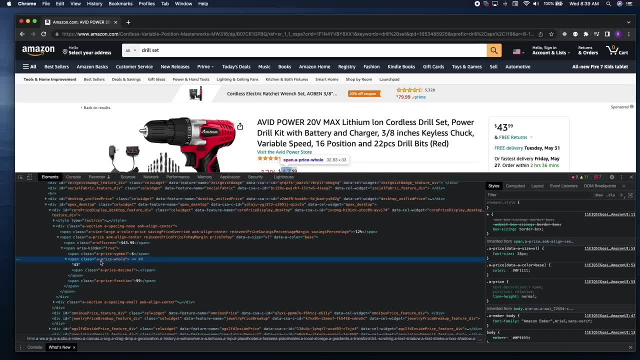 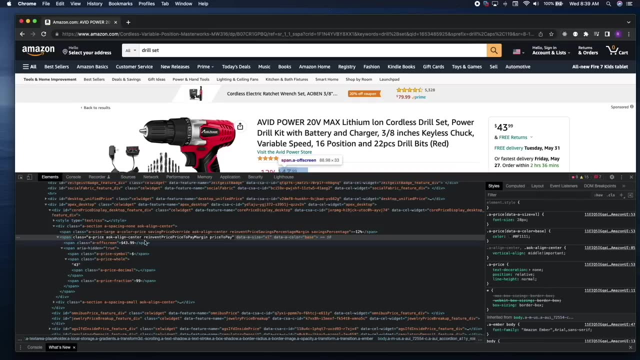 So 37.99 would work. We could use this span, but for the sake of getting the 99 involved, we will use this one right here for our project. So we'll go ahead: click on this and we're going to use this class right here And we're going to grab a class out of these. 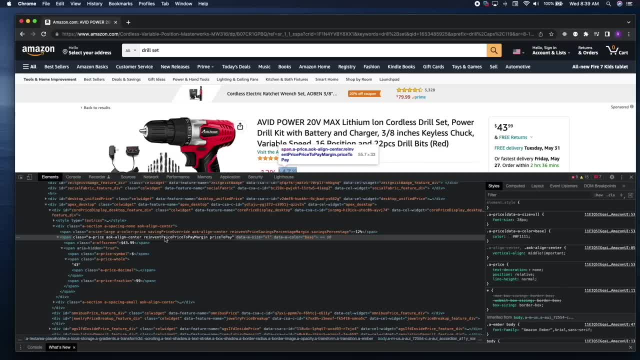 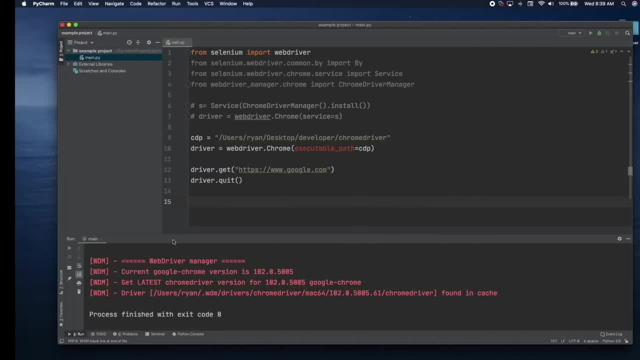 right here And we want to grab one that looks really unique, that isn't going to be used anywhere else. This class looks really unique to me, So I'm going to go ahead and copy this and then we'll come back to it. And we're going to go ahead and copy this and then we'll come back to it. 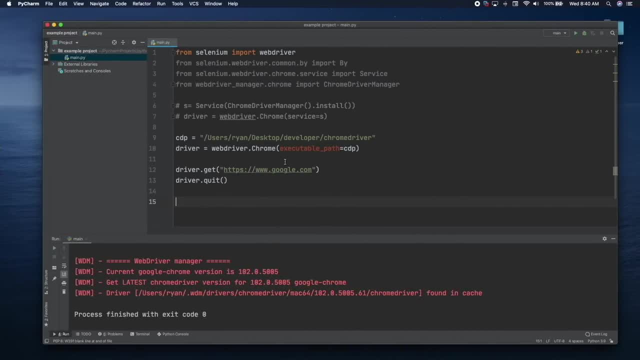 And we'll come back over to our Chrome driver And underneath of our googlecom we're going to type in price equals and then we want the driver to scan through all of this source, right here the HTML, And we're going to tell it we want to find an element and we want an. 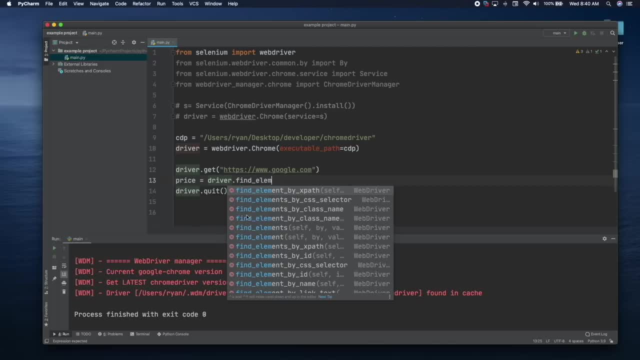 element by a class name. So we want to make sure we don't have elements by class name. We want a single element by the class name. Later we're going to use the one with the S, and this is the deprecated version I forgot. This is the version that I learned when I was using this. What we do. 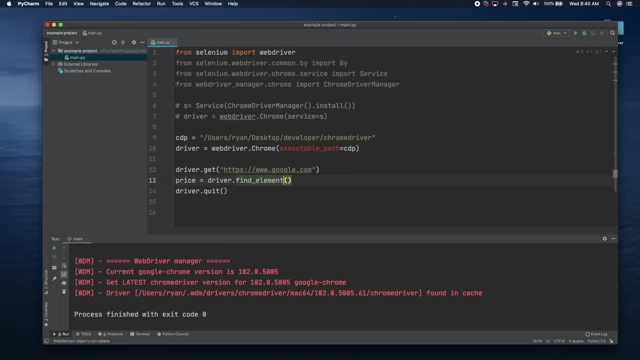 here now is we delete all of that. and we delete that. and we come in here and we say by dot class name, And and we come in here and we're going to put that class name that we just copied, just like this. The next thing we need to do is update this HTTPS right here, And it. 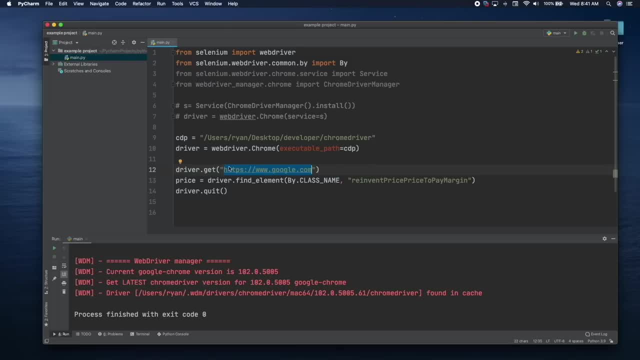 needs to be this URL right here, so that away our chrome driver opens up the right URL, scans through all the HTML, it's going to look for the class name that possesses this, and then we want it to print the price like this. So we'll say print And then we want to print the price. so if we were to go back and kind of: 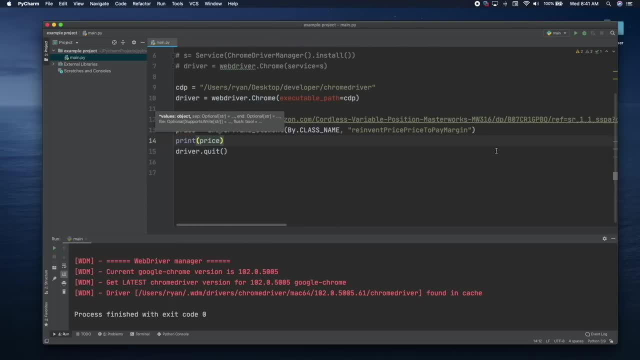 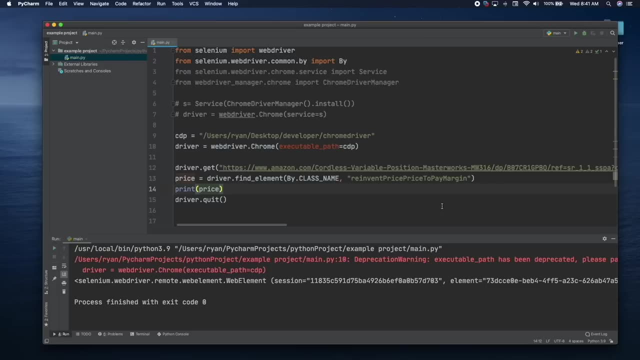 Then we want to print the price. So we'll say print and then we want to print the price. So if we wanted to have the price at 430 rubles? So if we run this how it is right now, I'll show you what our output is. 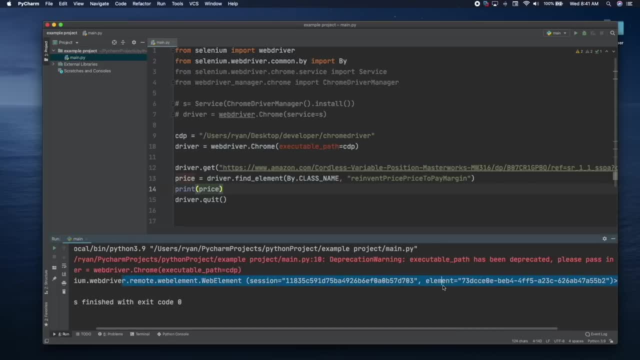 It gives us this as our output, and this is not helpful. So what we need to do in order to grab the plain text is type in text. So now, if we run it, it's going to print out for us our 43.99, and I'll show you what would. 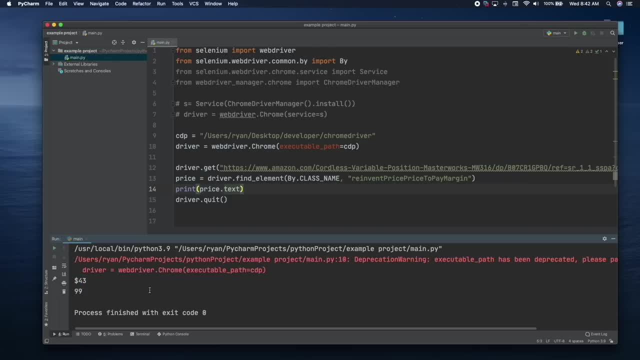 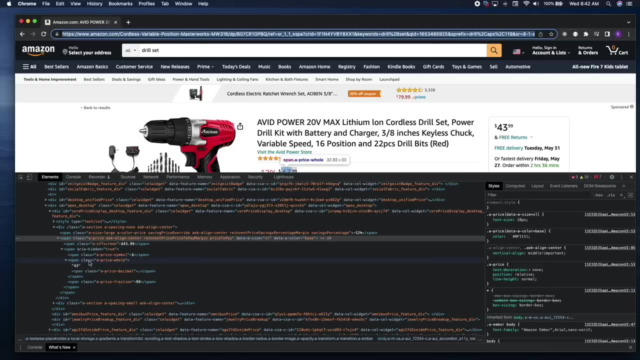 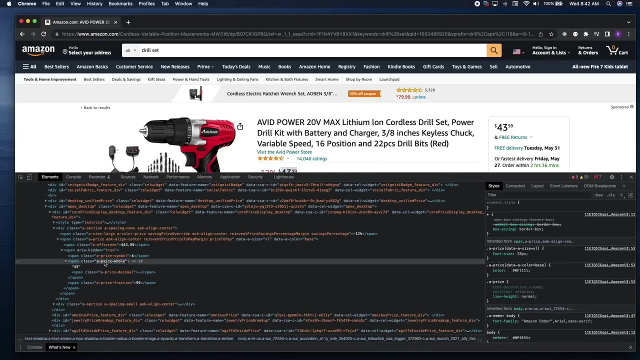 be useful. if we're really going to turn this into a web scraper for us, It really would be useful to get rid of this 99 and just use this right here So you can see why it's printing the way it is. This span 43.99 and it's given it to us on different lines. 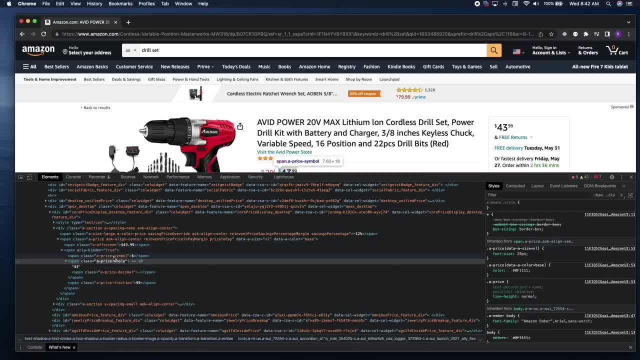 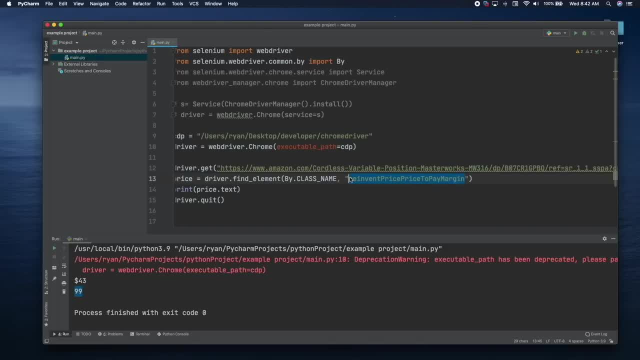 So we should be able to copy. let's try this class right here. And this really is when you're making these going to be a lot of trial and error, as you're going to see in a little bit, when we make our new dumpster diving ethical hacking tool. 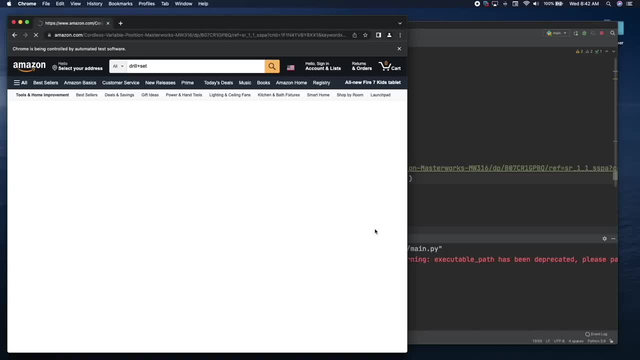 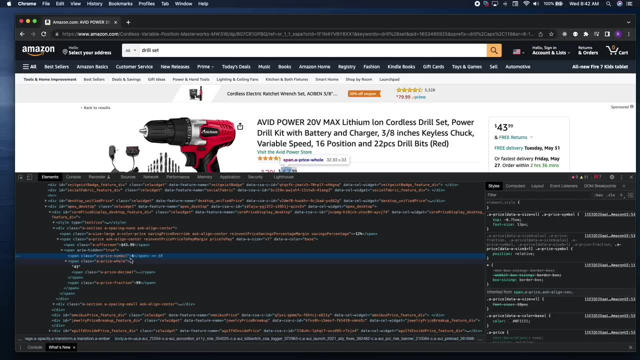 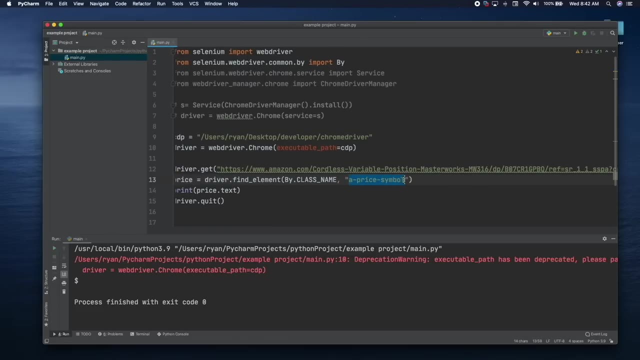 and we try to automate some of our recon where it's going to be a lot of trial and error. So we'll let this run and we get the dollar sign. That is not what we want, So we'll try. Let's try this one and we will paste this in here and now we can run it and see what. 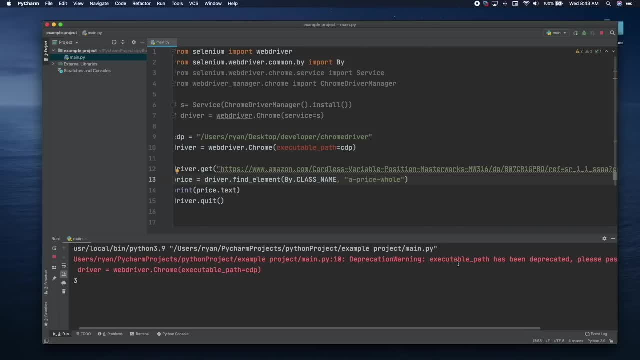 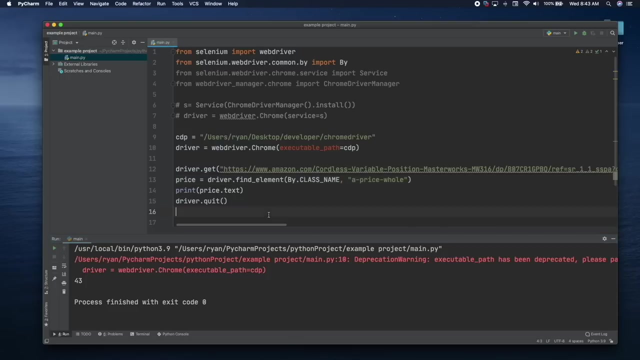 comes back and we grab just the 43.. So now, if we wanted this to run, say, every 20 minutes, to see if Amazon has updated their price and brought it down below $38,, we're going to put all of this inside of a function. 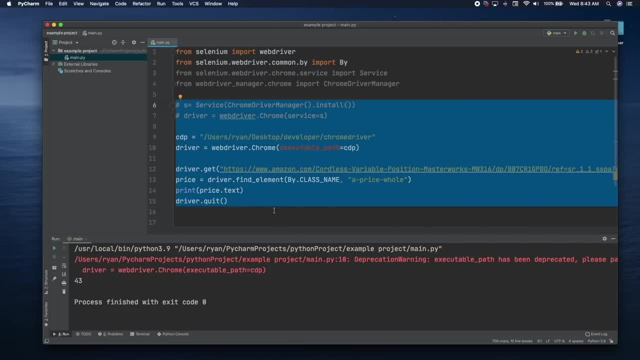 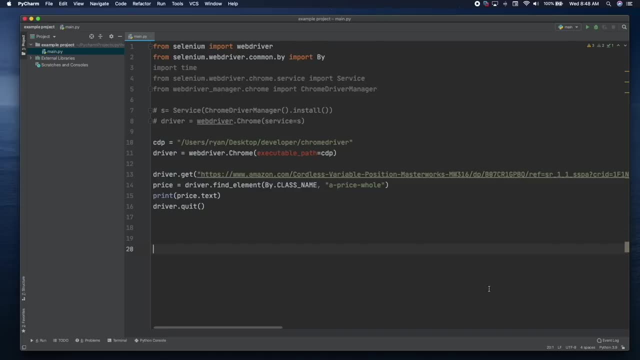 that is going to get called every 20 minutes and we're going to have to import a new module for this, and we're going to do that in the next section. All right, Now that we have our web scraper working, let's say we want it to go out and check the. 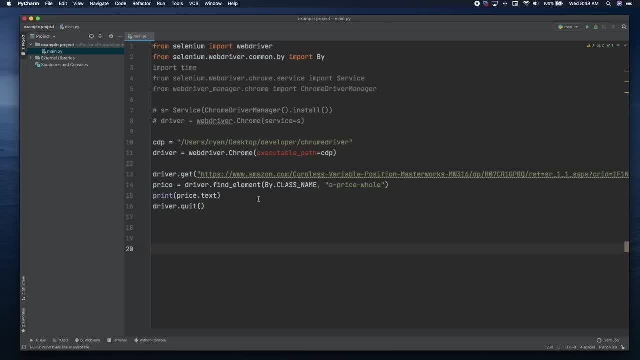 price every five minutes or 30 minutes or whatever we want it to be, And then let us print it into the console. What we would do in this case is put this into a while loop, And so what we can do Is take this and we can say while on, and then we want the on to be true all the time. 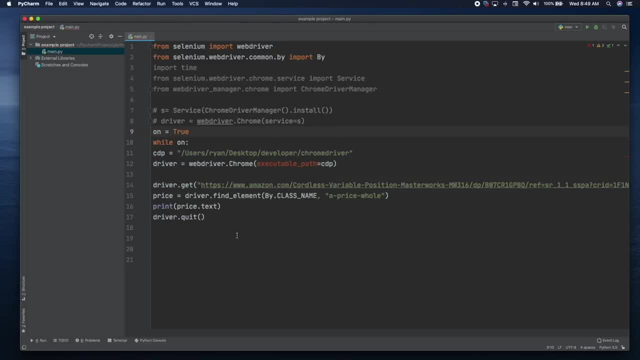 So we'll say, on equals, true, And this should be familiar to you if you have gone through the first part of our Python for hackers- And then we're going to need this inside of a function that gets called every four seconds or 30 minutes. 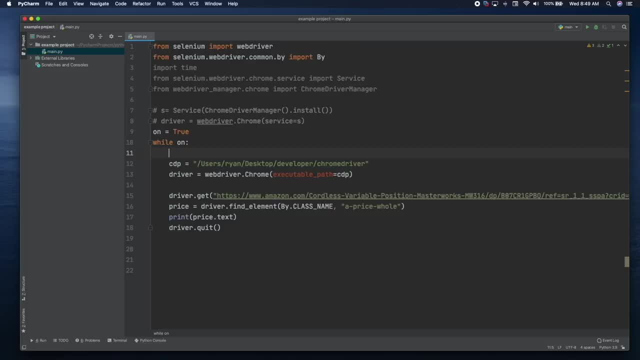 And we'll need this inside of a function that gets called Every so many minutes. In our case, I'm going to set it to only five seconds, so that way we don't have to wait very long. but in a real case scenario, you would make this run maybe once a day or every. 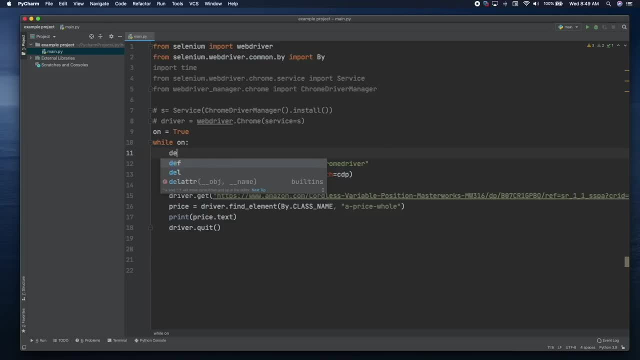 couple of hours to check the price. But for now we're going to make a function and we're going to call it five. We'll call it five seconds, We'll call our function and then we will need all of this to be inside of our function. 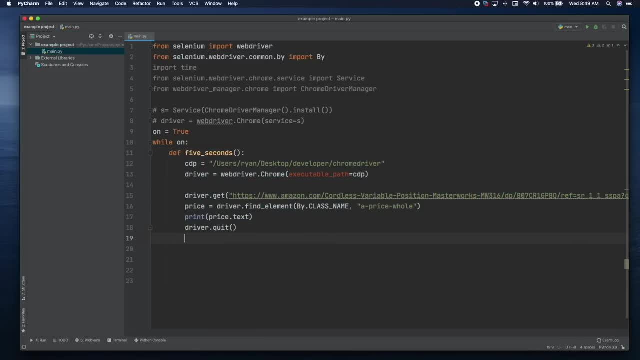 Okay, And now we need to call the function like this and we will say five seconds, And then we are going to take this and we need this to sleep. So we'll say timesleep and you will need to import time up here, if you have not already. 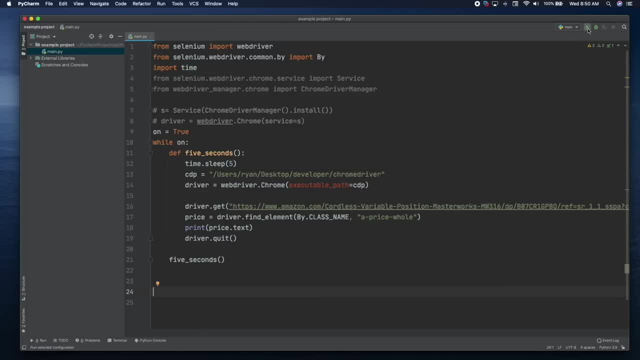 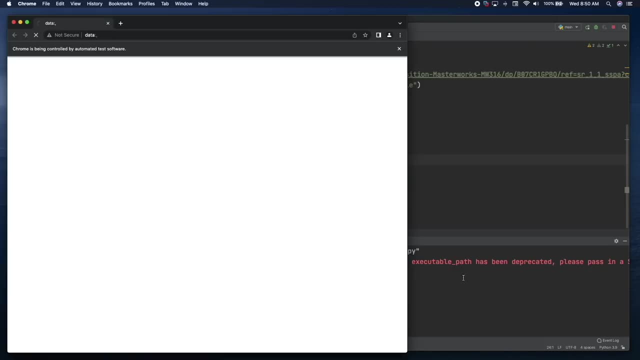 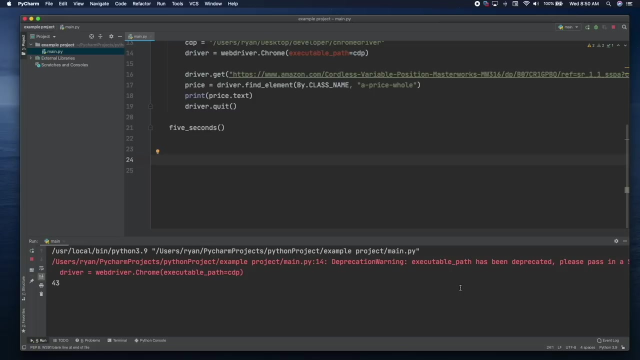 And we're going to say: sleep for five seconds. Now, when we run this, it's going to take five seconds. It's going to launch our driver, Go out, Check the price and print it down here in our console for us And then, once it gets done doing that, it's going to wait five more seconds. 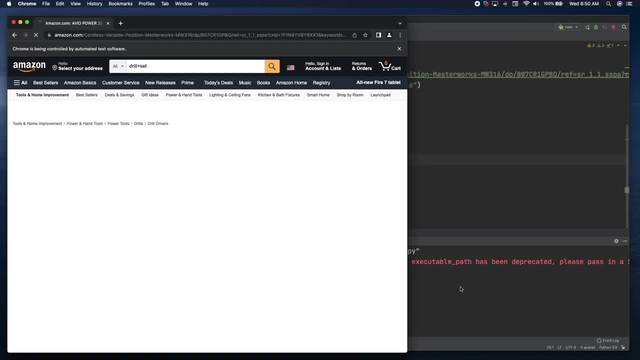 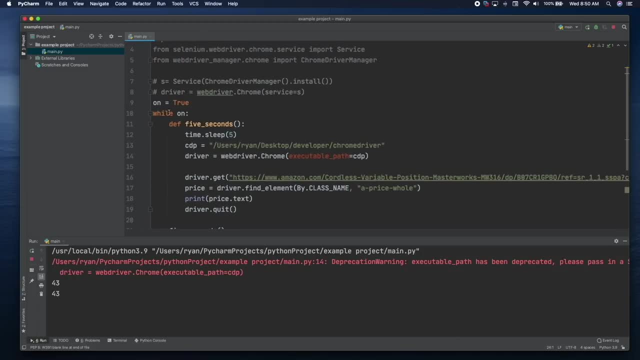 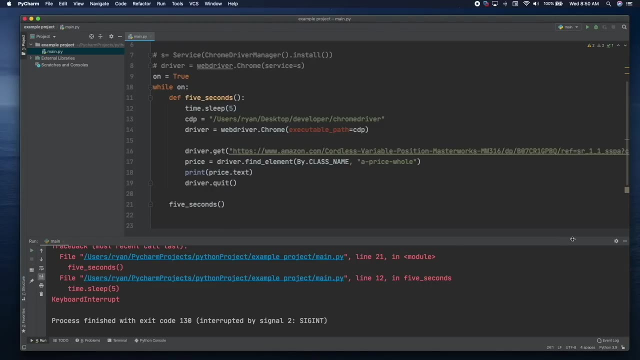 And then it is going to launch the browser again and check the price for us, And it will do this for all eternity, because we are inside what's called an infinite loop. There's no way for this loop to end, And so it's just going to keep on going and printing for us the price until we stop the. 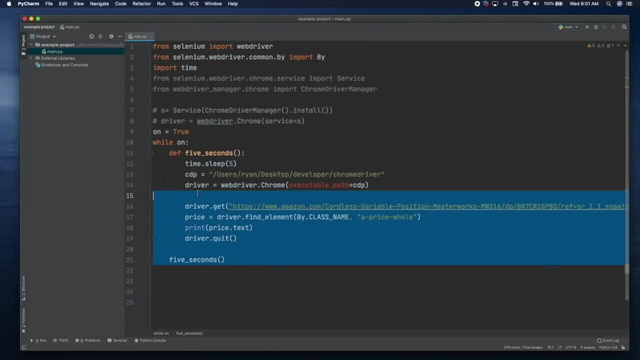 program. So this isn't really helpful for us in the world of hacking, So we're going to stop here. I just want you to get this concept down of using Selenium setting up functions using a while loop. If we were to use this completely for our daily use, we would have to make an if statement. 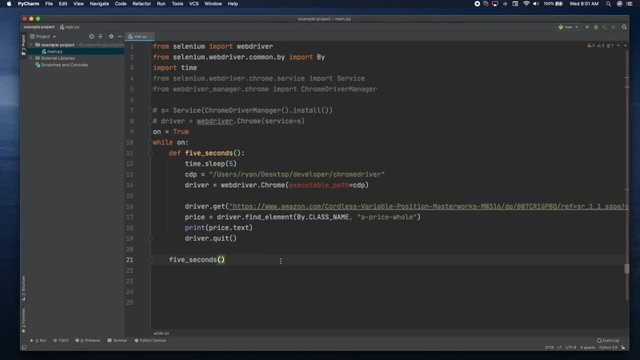 and say: if the price is equal to or less than $38,, then have it. We would import another module and we would have it send us an email or a text message saying the price is ready for us to go. So we're going to stop here and buy it, but we're not going to finish this out, because 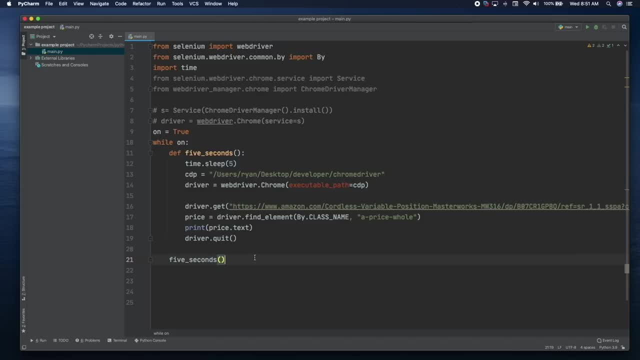 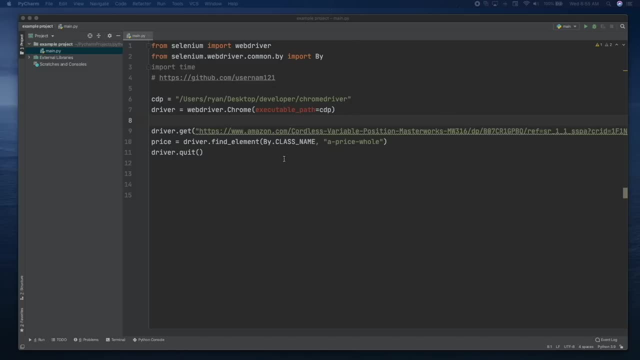 it's not really going to be helpful for us in the world of hacking, So we'll move on to building our actual tool for hacking. I have cleaned out my text editor here just to get it down to the bare bones of what we are going to need as we build this tool. 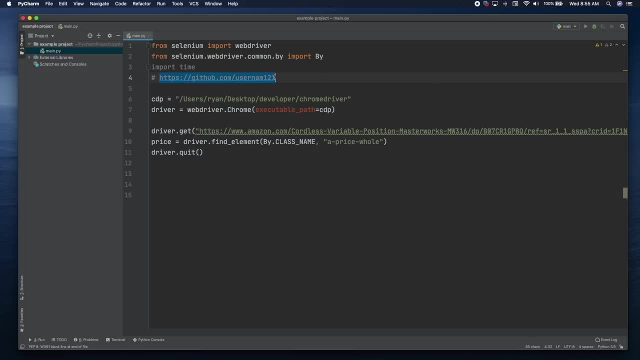 I have put this right here. This is the GitHub repo that we're going to be going through and dumpster diving for Now. this should work for any GitHub page if we program this right. but I made this GitHub page just for us to test. 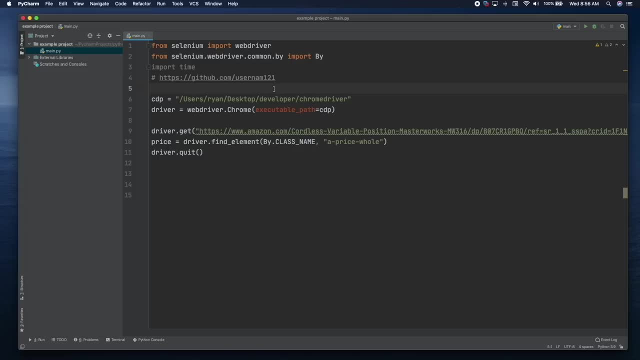 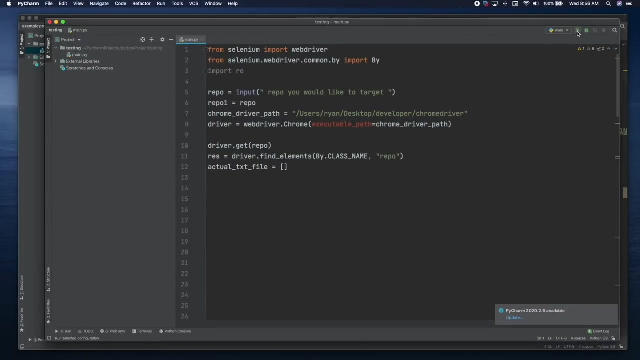 against to make sure our tool is running. I didn't want to spam an actual GitHub account that is in use, So this is just a GitHub account that I made for the purpose of showing you how to build this tool. So what we're going to make in the end is a tool that, when we run it, it runs what target? 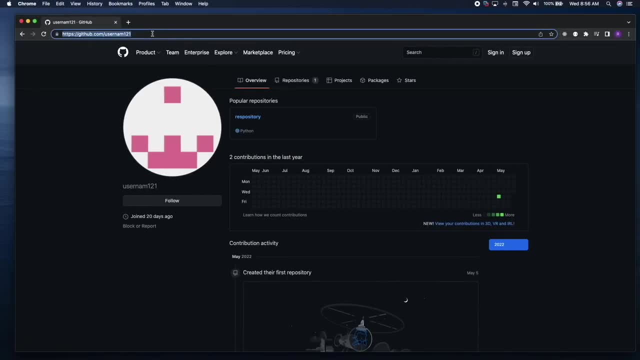 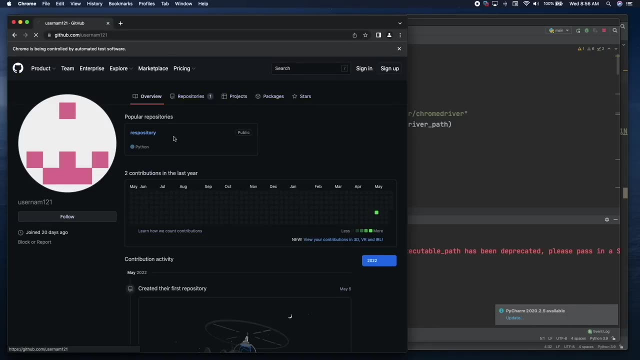 would you like to run against? And so We're going to copy the URL of the GitHub page that we want to scan And when we run it, it's going to go out to GitHub. It's going to click on the repo. 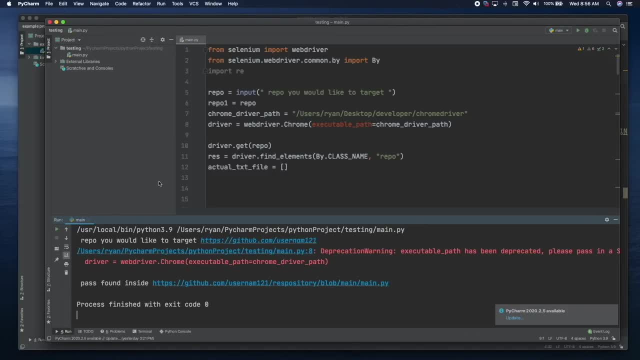 It's going to click on the pay, on the code, It's going to go to the role, and then it is going to tell us a password was found inside this page, And so what you could do is just copy this or click on it, and it will take you to this. 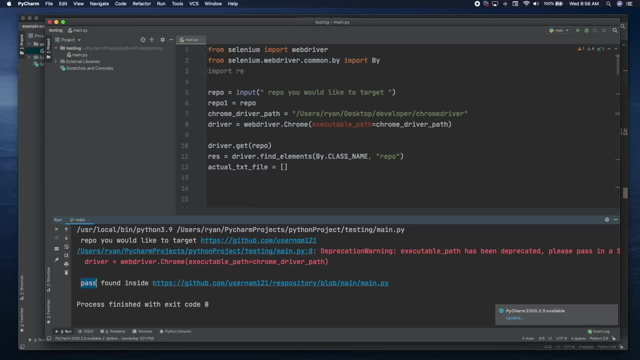 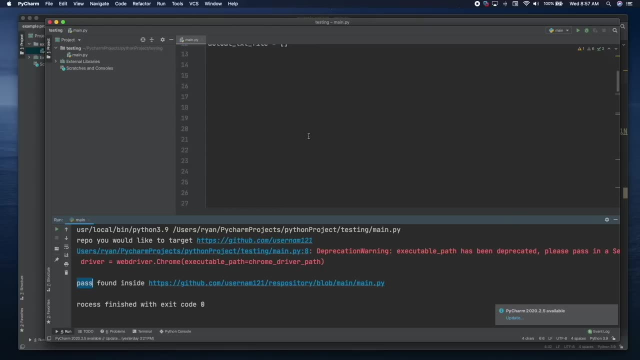 GitHub page and you can search for where this password was used. So we're going to make a very basic program Just like this one, And I hit a lot of the code. It's down there. I didn't want you to get a head start. 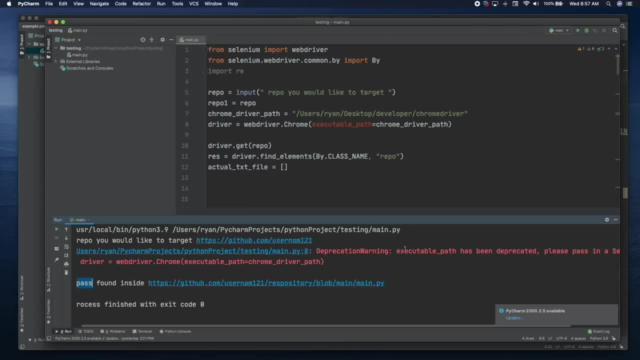 So, as we make this tool, when we're done, it's going to be very basic, but I would challenge you to make it your own and add to it different files that you want it to search for, different keywords, Make it print the entire line where the passwords found. 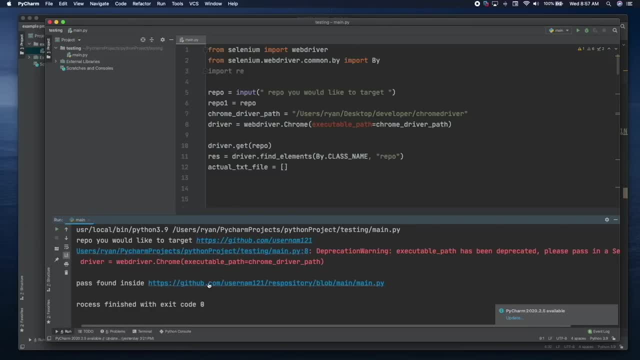 So you don't actually have to go out to this page and check it. These are things that I've done with my tool that I've made just like this. Okay, So I'm going to show you guys how to get started making this tool and then add onto it and 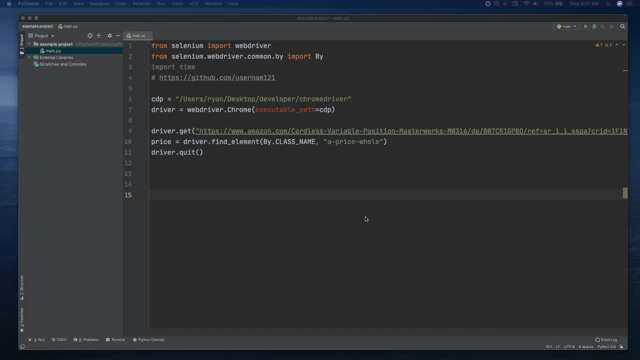 make it your own. Okay, As we go through building this tool, there are a few things we're going to do at the beginning that I'm going to tell you to change at the end to make the entire tool work well for you. So what we're going to do at the beginning is we're just going to get rid of this, right. 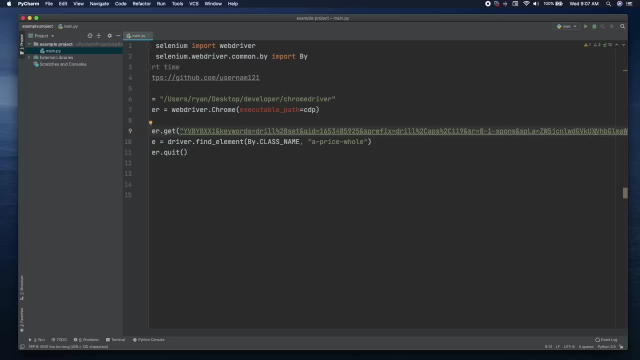 here because we want to put in our repo that we're going to be scanning against, And I'll leave that GitHub repo up unless it ends up getting taken down by GitHub, because it is getting scraped over and over and over by people from all over. 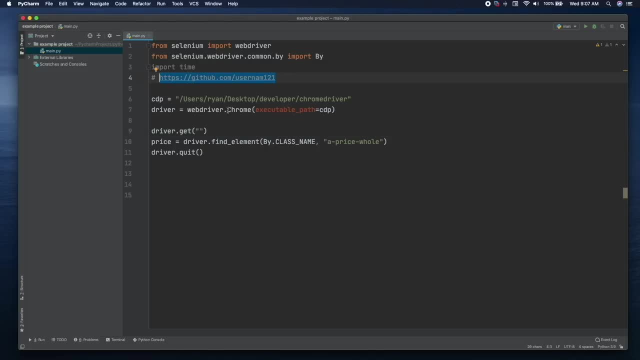 But until then I'm going to just leave this GitHub page up for you guys. So we'll just put that inside of our GitHub page and now we can comment this out, and it should open up that page for us and then quit. And it did. 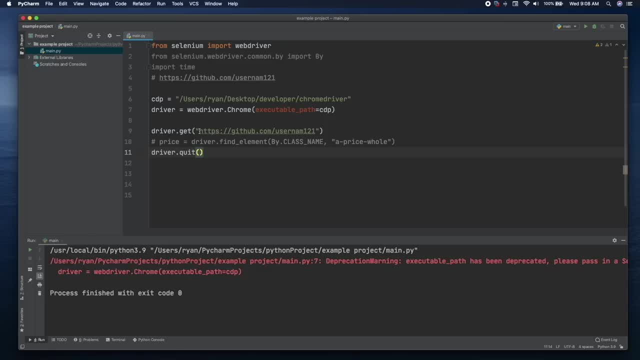 So there it ran, And what we're going to do in the end is we will change This and we will make this an input, but we're going to cover that at the end when we get to that section, Now that we have it, so it'll open up this page for us. 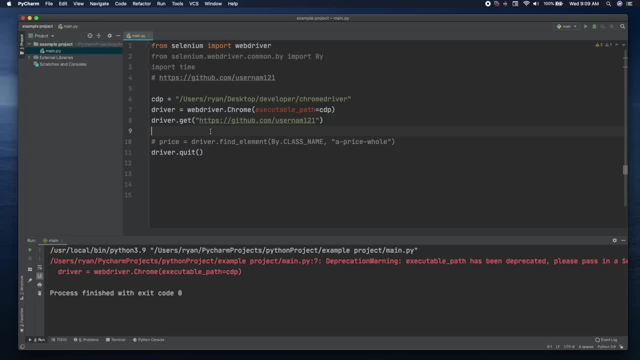 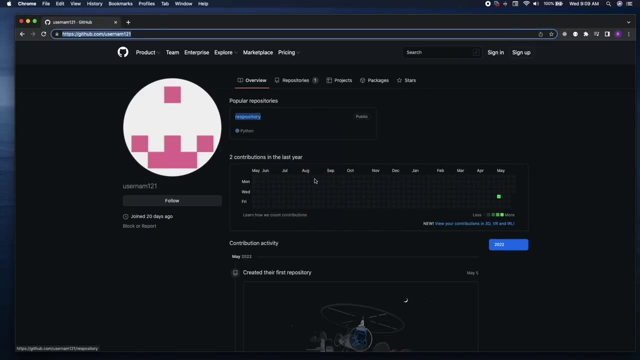 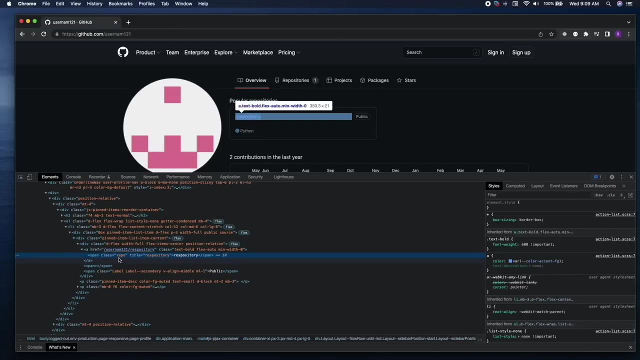 We want it to grab something for us by an element, And because usually there's a bunch of repositories in here, we're going to just use the repositories instead of getting the element by, let's say, the class name. get at the element. 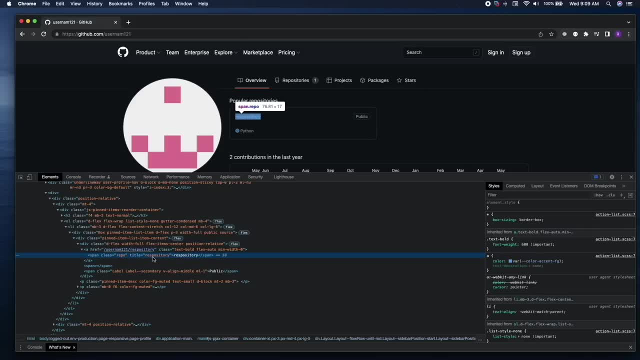 We're going to make it get elements by classmate, By class name, And I'll show you what I mean in just a second. So we'll go in here and we will say: we need this class titled repo, Okay, And this is what these will be titled, as for us. 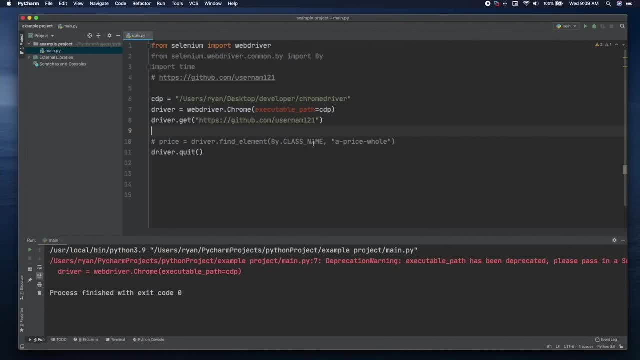 And we have this anchor tag right here. So what we're going to do is we'll do the same thing we did in the last one. We're going to say that the repository- and we'll name this as we'll call this- our res for resources. 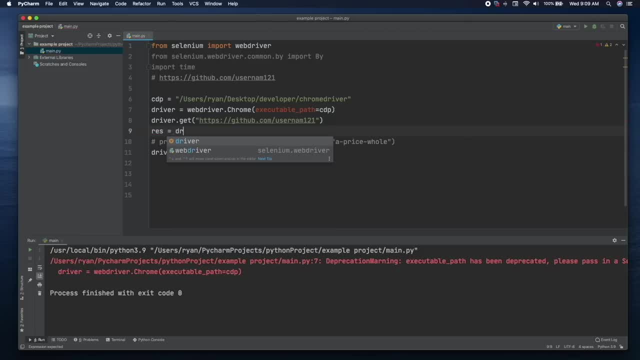 And we're going to turn it into a repository, We're going to give it a variable and it's going to get for us all the repos by the class name. So we'll say driver, dot, find element, And then we want this to be an S. and the reason we want this to be an S is because we want 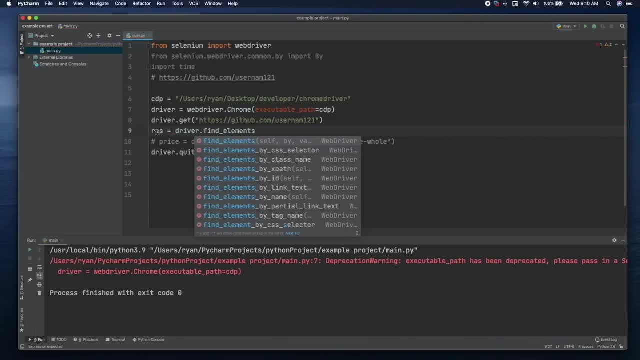 to find all the elements and we're going to store them inside this variable. Now, for this cause, there is only one right here, but this should work with many repos If you scan a GitHub page with many elements. So we're going to go ahead and we're going to go ahead and we're going to go with the class name of repo. 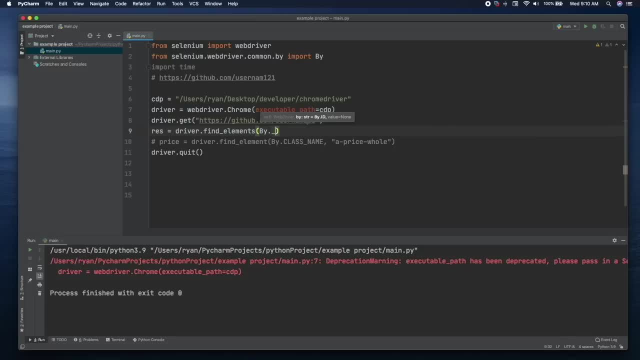 So we'll go, we'll continue and type in by dot class name. We don't want a class, We want the class like this class name and the class name is repo, just like this. Now, if we run this, it will go and it will click this page and then it will close. 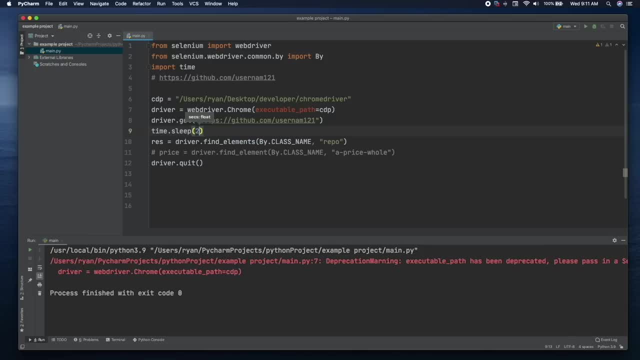 So what I want to do is I'm going to add in timesleep And we'll make this two seconds. We can see what's happening, and then we'll make another timesleep right here so that you can see that it clicks onto the next page. 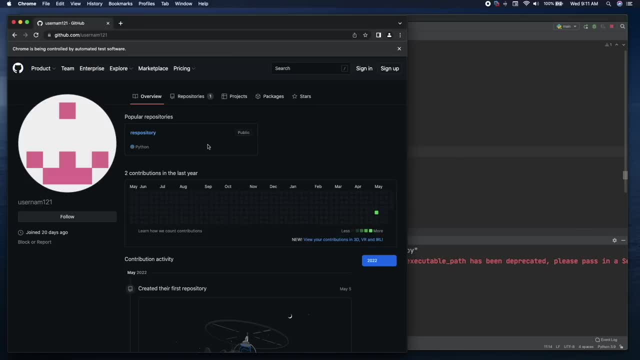 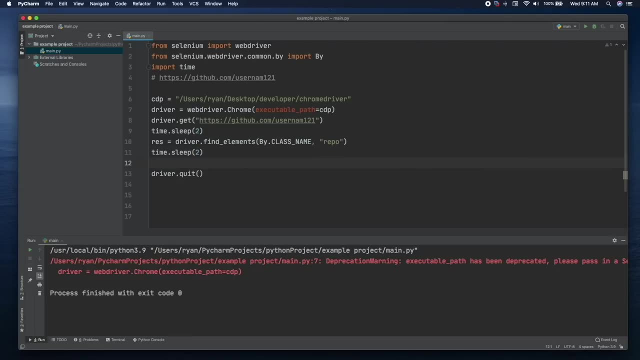 So we'll run this. It's going to open, wait two seconds, and then it's going to open this repository right here and close. So now what we are. so now what we need to do is make a for loop so that way we can print. 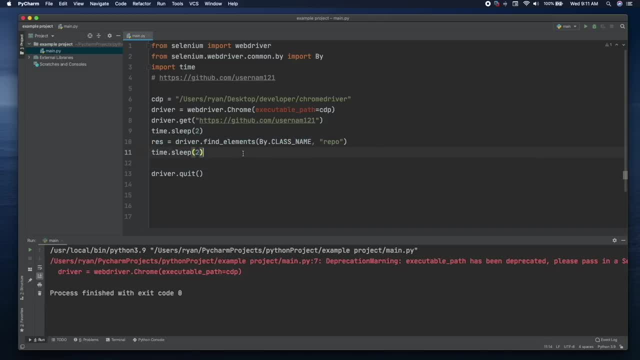 the repos that are on this page, And in this case there's only going to be one, but we're going to go ahead and make this for loop. So we're going to say, for I, in all these listed resources we want to print, and we 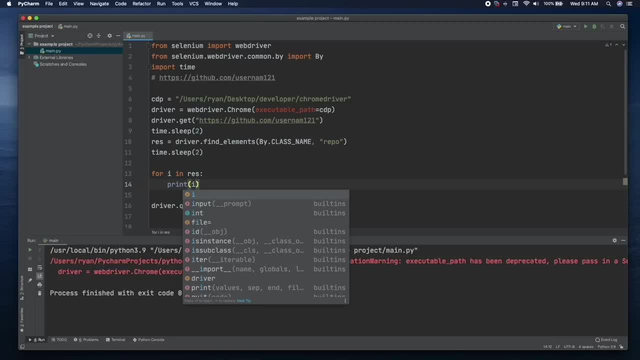 want to print I, And what we would do here is we'd say: print I dot text because we want to see it in the text format, and then it will quit for us- I should have gotten rid of the sleep- for us. Uh, I see I spelled that wrong and that's okay. 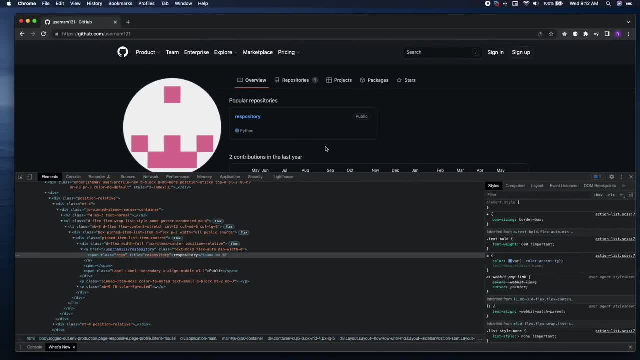 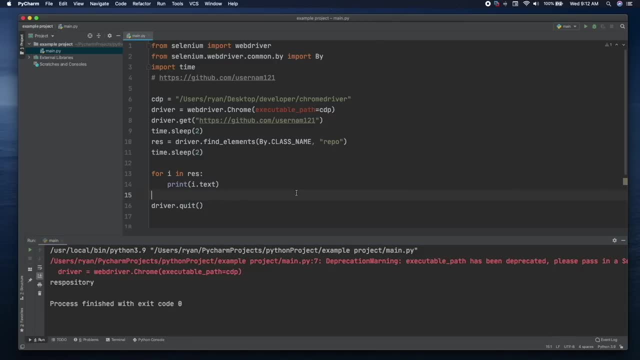 I made that repository late at night and it's all right that it isn't quite right. It's still a repository and we can still scan against it. So it prints for us this repository right here. So now that we know, we can loop through all of the resources that have the element class. 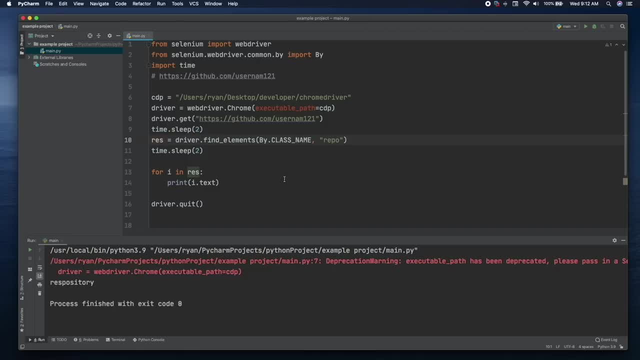 name repo. we need to figure out how can we click on those, And there is a click function that we're going to use Later, but right now I want us to go through and see how we can do this a different way. It's going to be a little more complicated, but it's always best to know there are multiple. 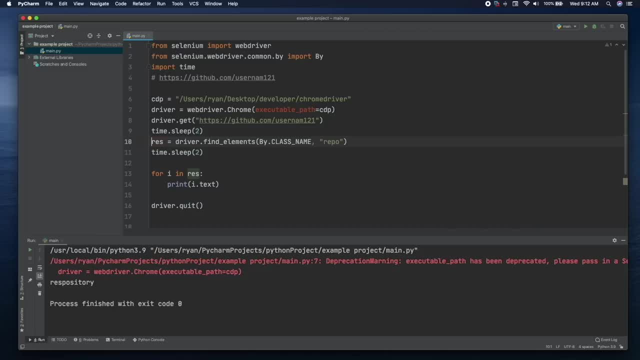 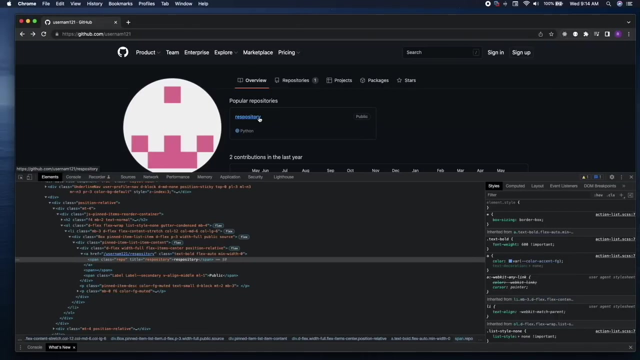 ways to do something, especially in the world of coding and in the world of hacking. All right, because we're not going to use the click function. we need to see what happens when we click on this link right here Now. this is something in cybersecurity that you're going to need to always do when you're 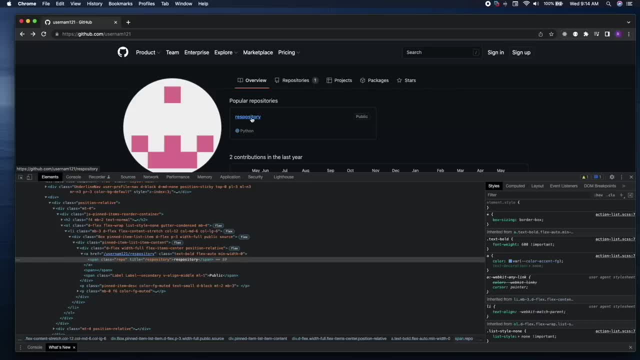 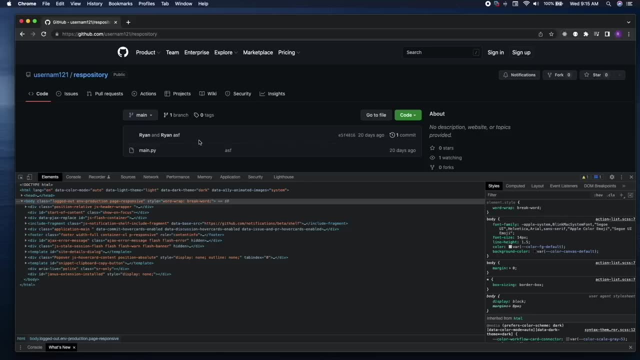 testing a page. not that we're testing GitHub, But when you test a page, it's always good practice to click and see what happens, how to use the page to see what's going on, And what we're going to do is check out this URL. 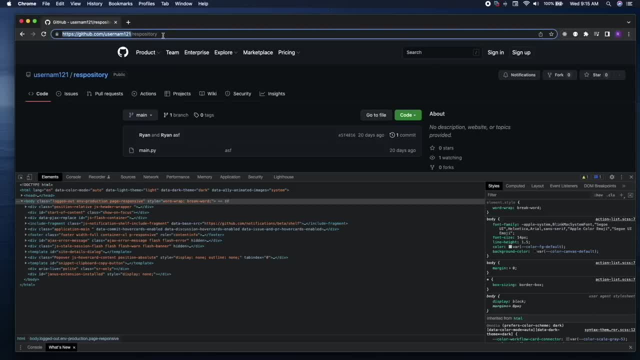 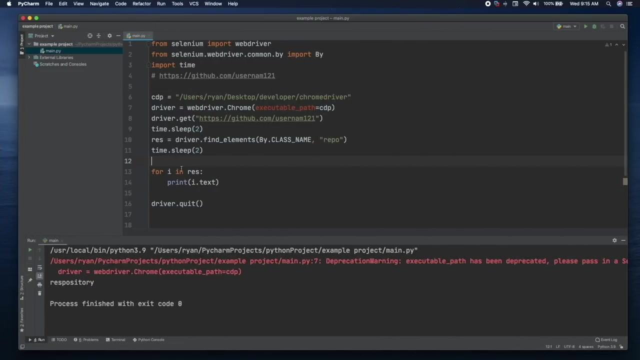 So this is the URL that we start out with And since, since it just changes the repo name as into the new directory, what we're going to need to do is take this directory and put it into a new link and get our web driver to open this up. 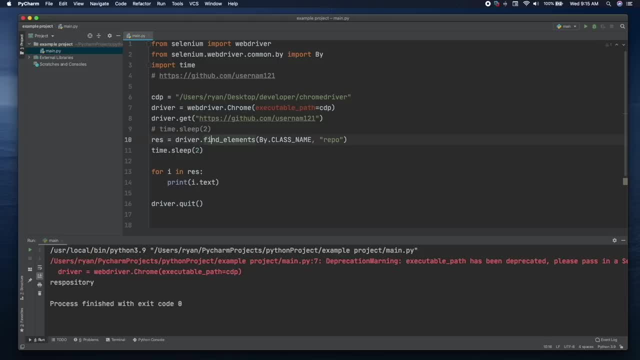 Since we know we can run this- And I'll go ahead and comment out these times, sleep, because we don't need those no more. Since we know we can run this and we can get it to scrape all of the repositories and then print them down here. 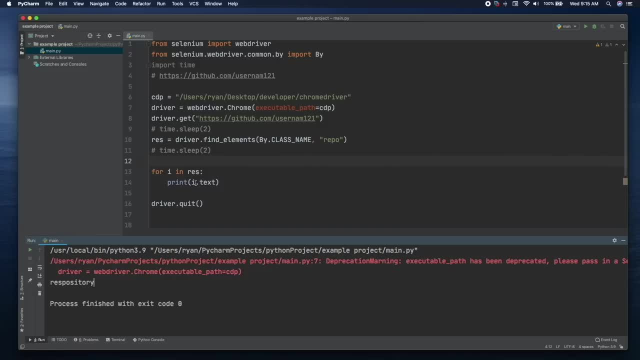 Now we can just save these into a list and then we can loop through that list and get it to append that to our URL. This is a little more complicated than the click function, but it's helpful because we will need so that a way we can get it to open every single repository that we go through. 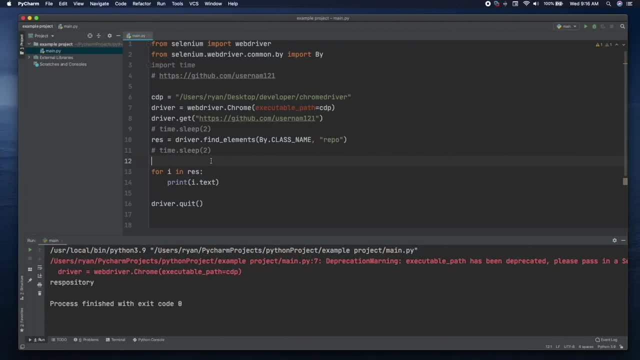 in the future, When we go through a page, It has a lot of repositories on it. So what we will end up doing is making a list, which you've seen in the past, And, if you want, you can pause the video and see if you can figure out how to make a list. 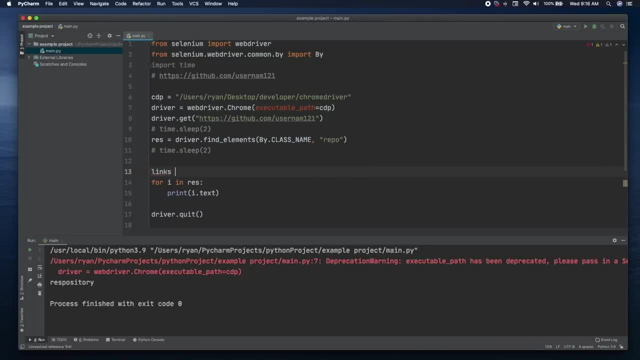 on your own, if you remember. And so I'm just going to name our list as links and we're going to make it empty. And what we are going to do now is we're going to take this and we're going to say linksappend. 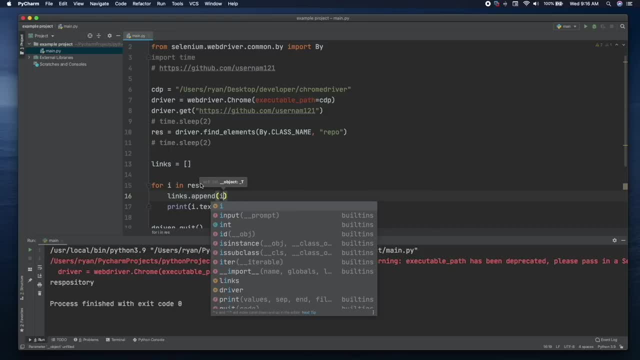 which I don't think you've seen before- And we want to append I. So now We take this And we move it over and we print: We need to append I dot texts. that way we get it right I dot text. 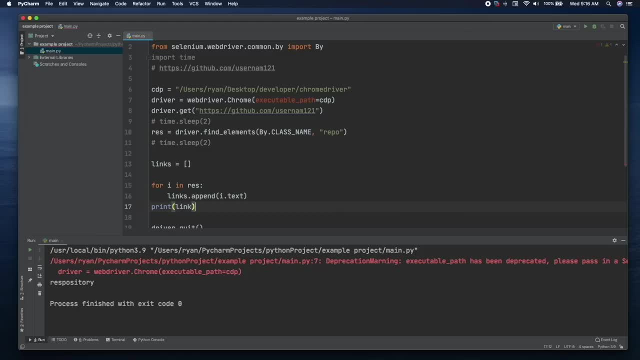 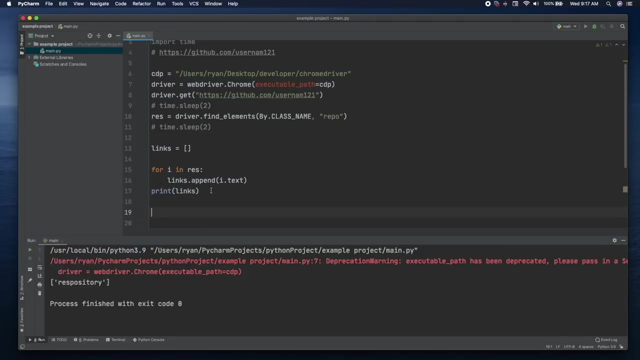 And now we print the links right here. We should get the repository to print from our list. So we'll run this and give it a test And it says we have repository and we have the brackets and it is inside the list. So what we will do now that we have this list is we're going to make another for loop. 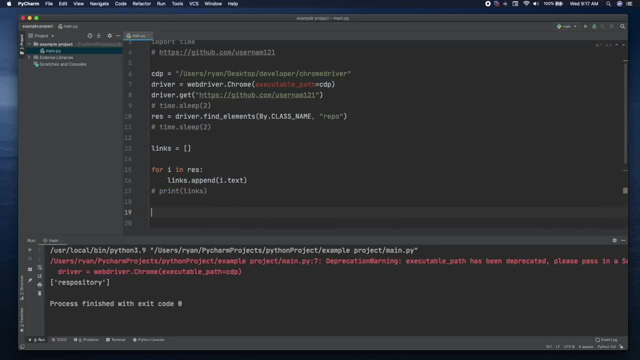 and we can comment this out because we don't need that to print every time, And in this for loop we're going to name it for L for the links inside the links list. We're going to make a new, we're going to make a new variable and we're going to call: 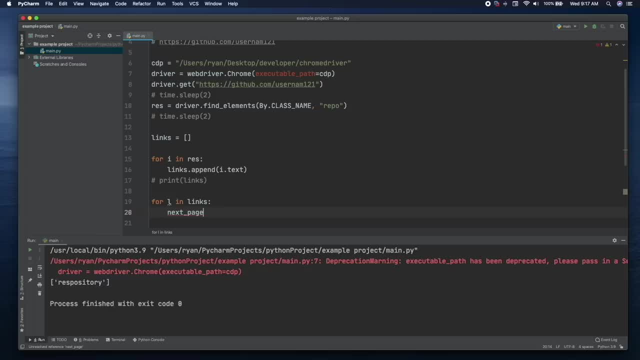 it. next page, And this is when I tell you my variable naming Naming becomes very poor because I'm not very creative And we're going to make this an F string and we're going to call the repo, And, if you remember, and we're going to call the repo, but we need to first name it something. 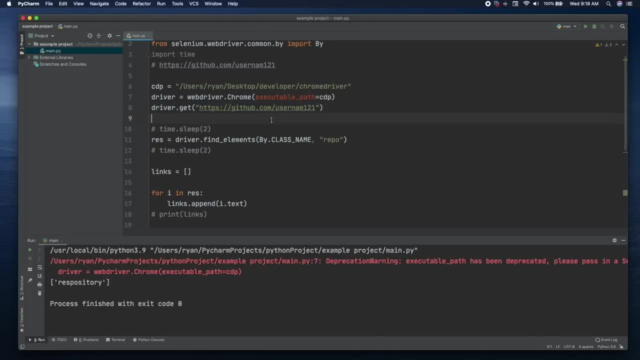 So we need this URL to be assigned to a variable, And so we'll just call this our repo And at the end we're going to change this, because this is going to be an input and we're going to make this a string, just like this. 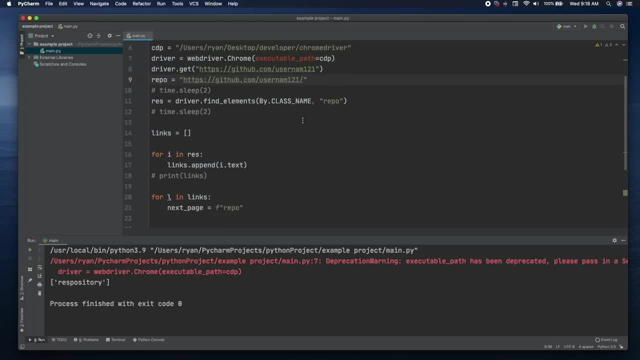 And now we have this repo right here and we'll add a slash- By the way, we don't have to later, Actually, we'll delete the slash and we'll add it down here in our string. Give us some practice with that. So we're going to take this repo and, because it's a variable, it needs to be an F string. 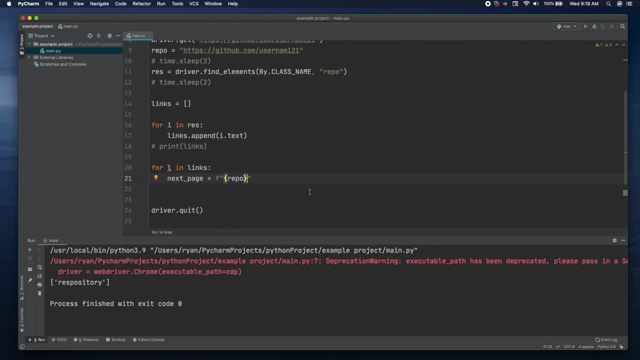 with these curly braces and we're going to add in our slash And then we will add in another variable which is going to be our L. So what would happen if we had a bunch of repos? This is going to go through all of the links which we saved right here as our resources. 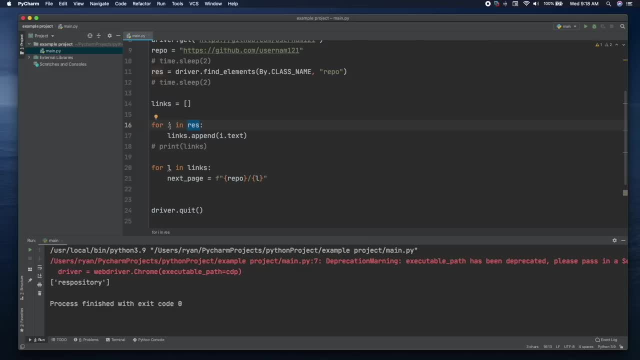 It's going to get all the links. This for loop is going to run through all these links and it's going to put them into our list that we have called links And, if you remember, this is where our repositories will be saved. Now we need to loop through there. 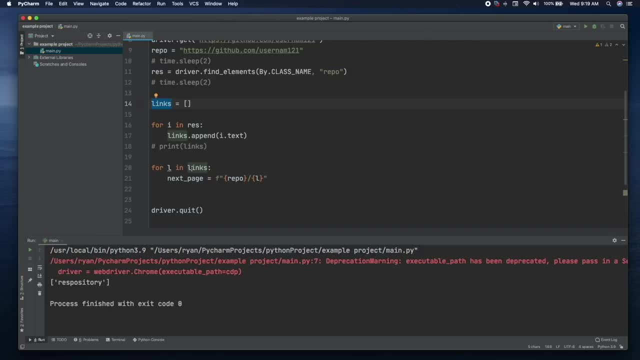 And in this for loop it's going to loop through our links and it's going to give us a new URL. So what this URL will look like after it runs through this second for loop is it will look like this And it will come out with our repository. 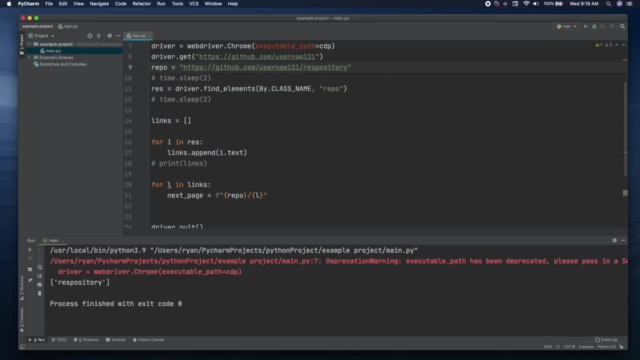 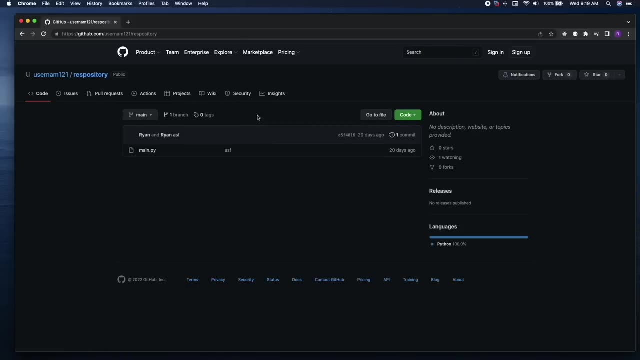 That I spelled wrong And it's going to open up this page and it will go and click this link for us. So this is the repo we want to attack. It will click this and it will bring us to this page. So let's try. go ahead and try this. 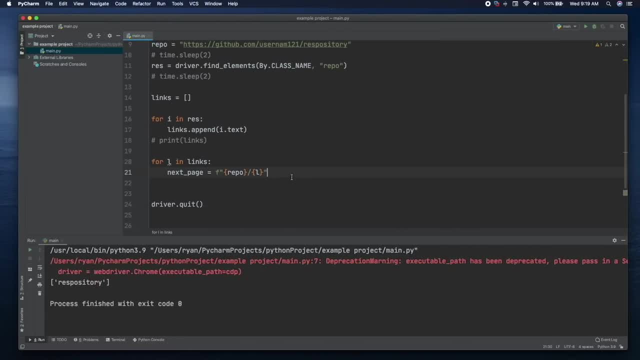 We're going to run this with a sleep command when we are ready. So what we need to do at this point is store our next page in a new link And we'll just call this our final link. So we'll just call it F link and we will save this into a list. 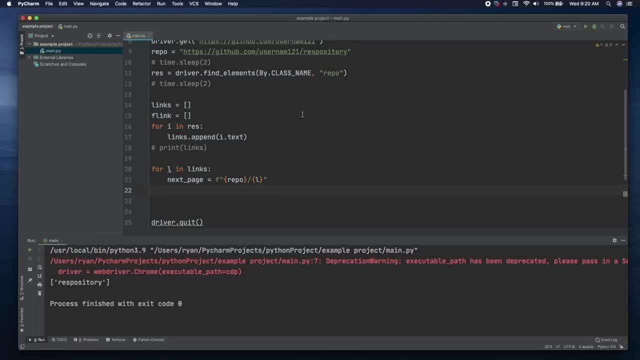 And then we're going to append our new URL, Remembering what this one right here is going to look like, because it's going and looping through a second time of this links and it's making our new URL that we want to test, which is going to be this one right here. 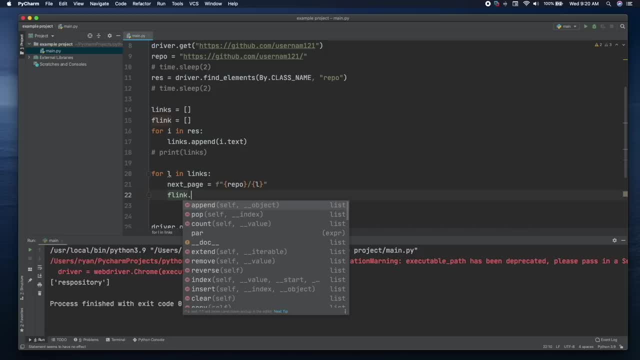 And we will tell this to append. So we're going to do F link dot append And we want to append the. So we're going to do F link dot append And we want to append the Next page And we're going to want it to append to the next page right here. 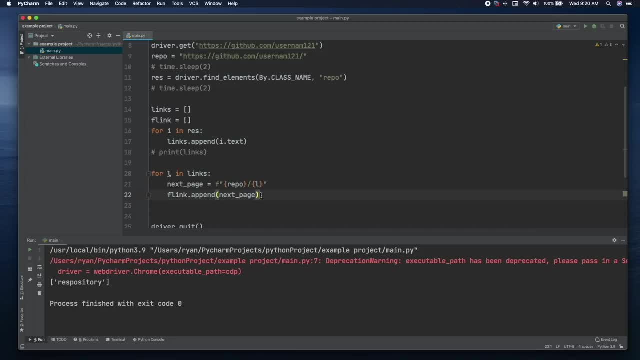 So, as we have this next page, it's if we print this it's going. I'll show you what it looks like. So if we print this, we can say print, and then we're going to print the F link and we'll. 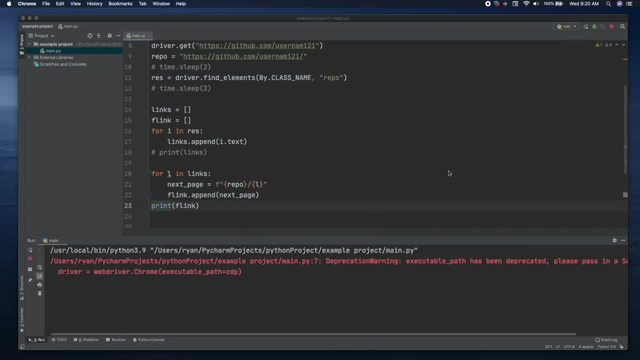 just go ahead and pull this back here and we will run this and it'll show us what our new URL looks like. I accidentally left this slash. That's okay. The browser would have just deleted this second time, That slash. So now, if we run it again, it's going to spit out for us this new link. 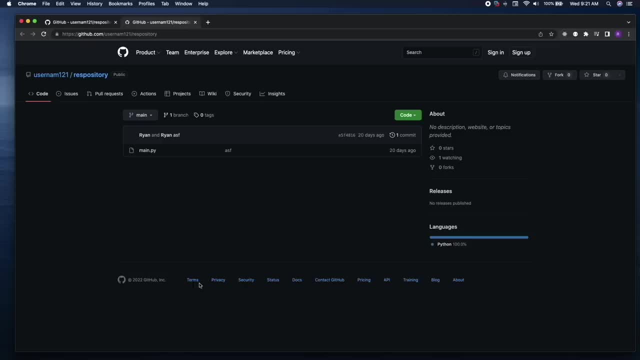 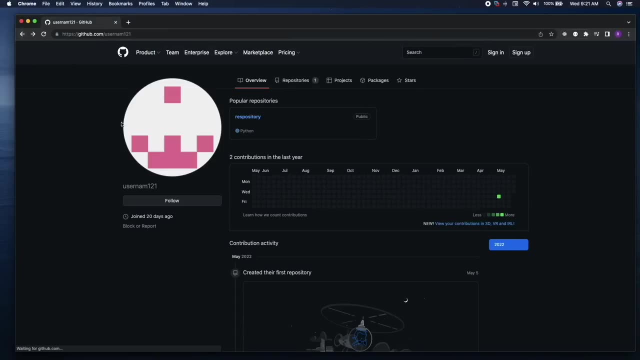 And if you copy this link or just click on it, it will take you. we'll just click on it, It'll take you to this page, And so that is how far we have gotten So now we have moved with Selenium from this page to the next page and where we're headed. 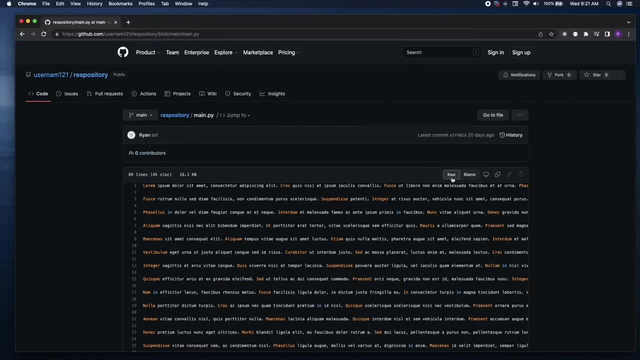 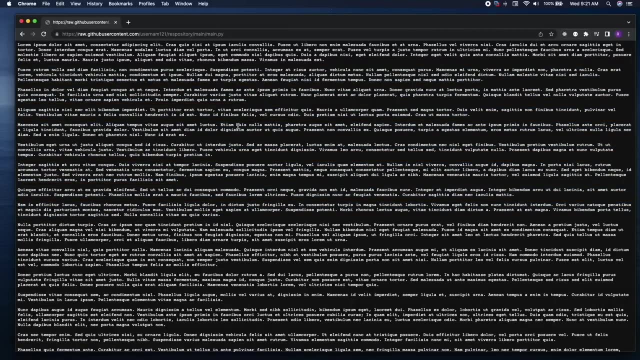 is inside this mainpy, And then we're going to go into the raw, And then we want to know if in any of this there is a password or some kind of key Word. And so I'll just show you if we type in command: fine. 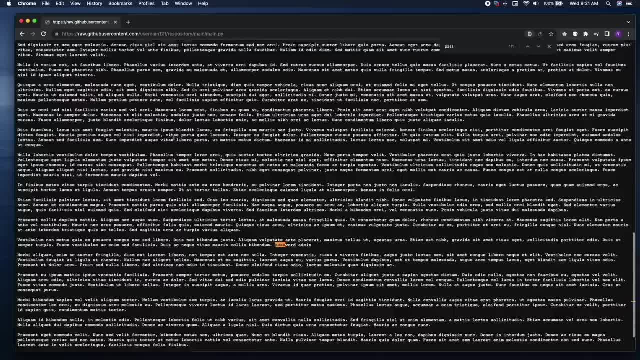 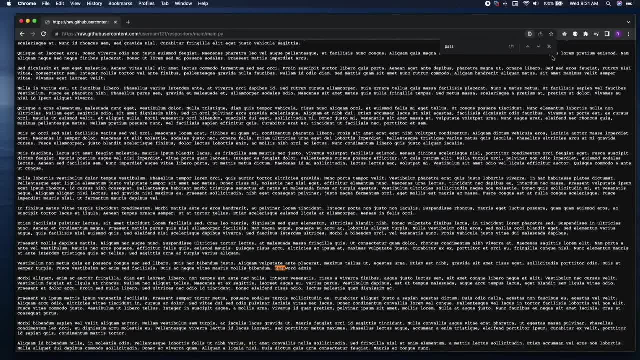 And we type in pass, we'll see this password admin. We're going to make our program go through all of these words and all of these lines inside this text and pull down the password for us. So that's where we're headed, But right now we've got a few pages more. 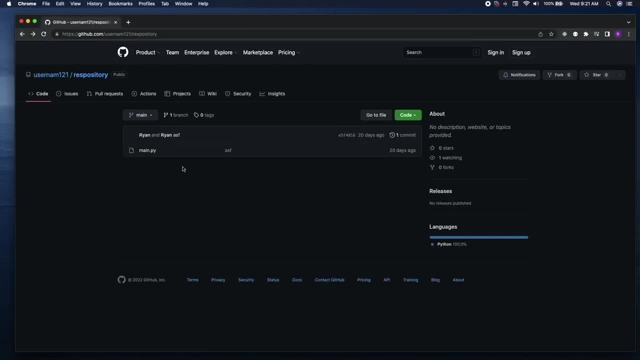 We need to move. We are right now on this landing page right here, So we'll make, we'll try and figure out how to make it open this page and then go into the raw and then search for the password. Okay, So we'll keep going in the next section. 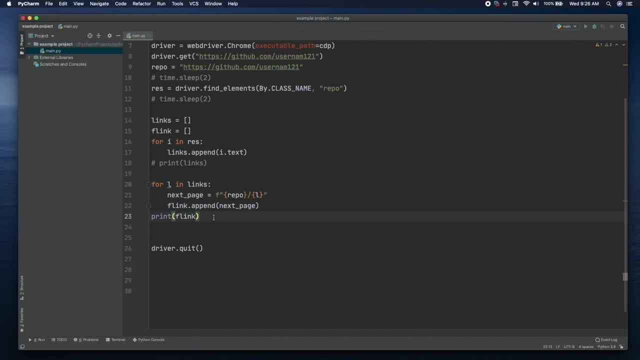 Okay, It is time to call our first function. So we can go ahead and comment out this print statement right here and we can call our first function. and we're going to call it above our for loops because we need our function to be called above where the function needs to be located, above where we call the function. 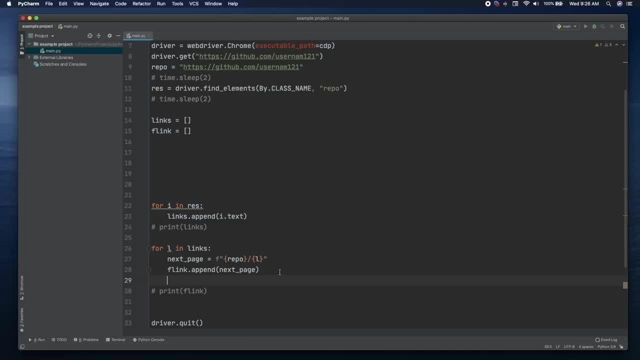 So we will call this function, We'll just call it a loop, because we're going to loop through all the links. So we will call it like this: We'll say loop and then we're going to pass in the next page, because that's what we want. 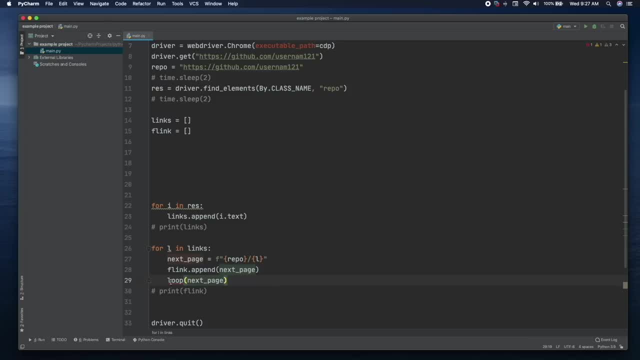 to go searching through in this function. So this is red because we haven't declared our function and we'll declare it up above and we will say def and we'll call it our loop And then we're going to pass in a function. We'll actually just call it our next page. 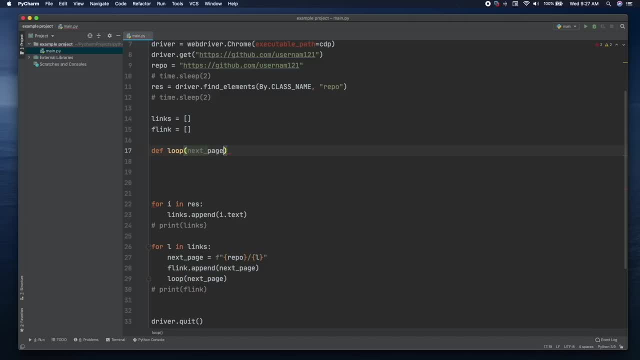 So that way we understand what's happening next page And we have to add in our two dots there And now. what do we want to do now that we can get to the next page? Now, there's a couple of things we need to do. 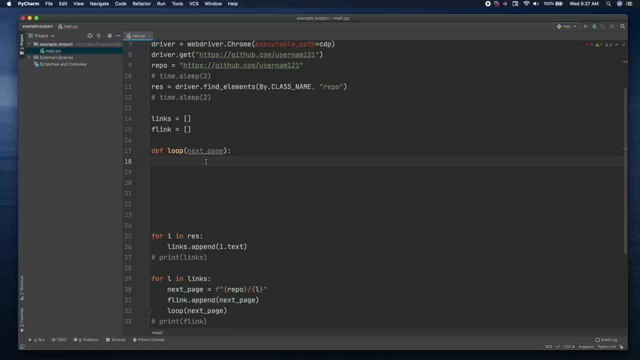 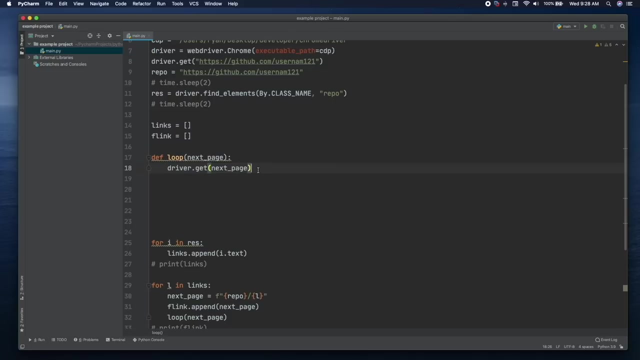 The first thing is we need to open that new page. So we're going to type in driver dot get and then we want it to open that next page. So let's see what happens. We can come right here- We'll just not run the time function and have it sleep and see what happens. 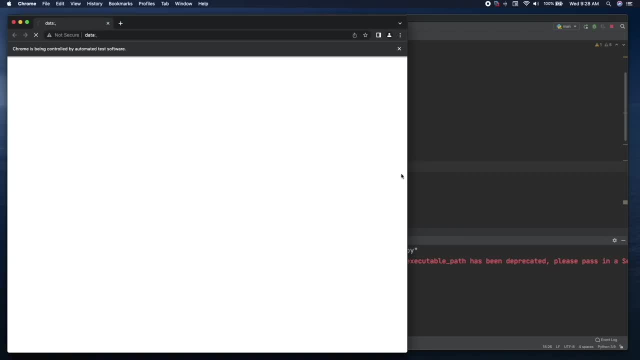 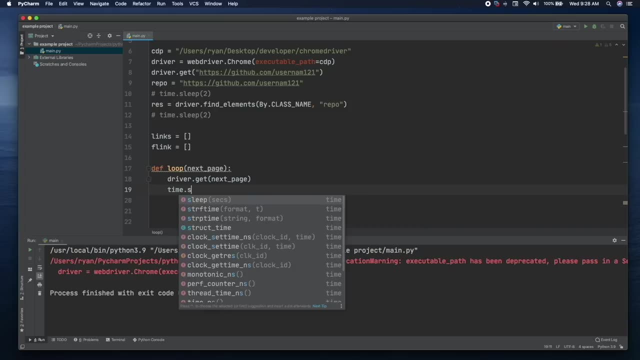 So we'll run this and see if it opens the page And we can see: Or it goes too quick, It went too quick, So we'll stop right here and we'll say time, dot, sleep. and we'll sleep for two seconds so that way we can see if it actually opened the next page. and it opens the next page and 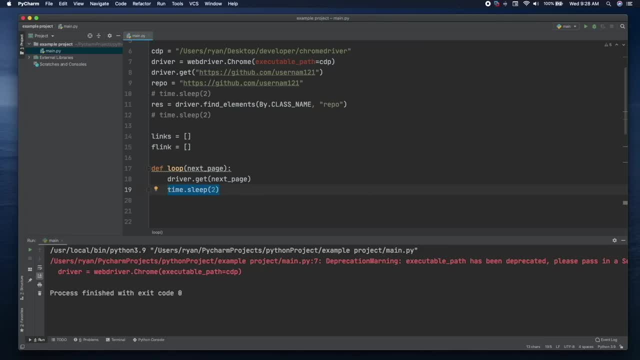 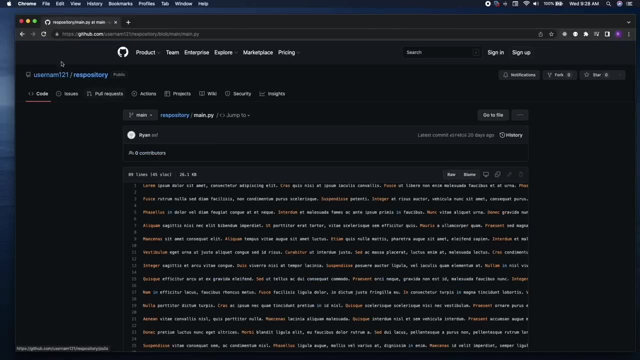 then it quits. So now that we know we're able to get to the next page, we need to be able to open this file right here and get to this raw button. So in order to do that, what I think would be best is to inspect this link. 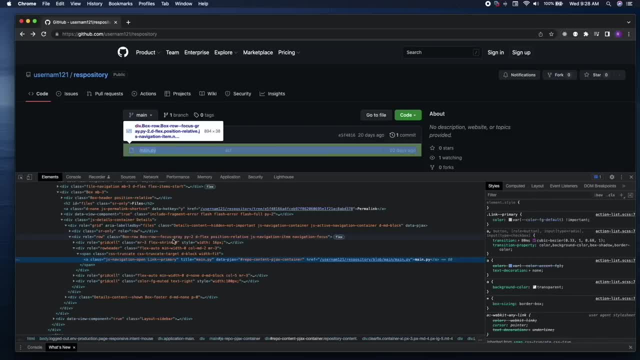 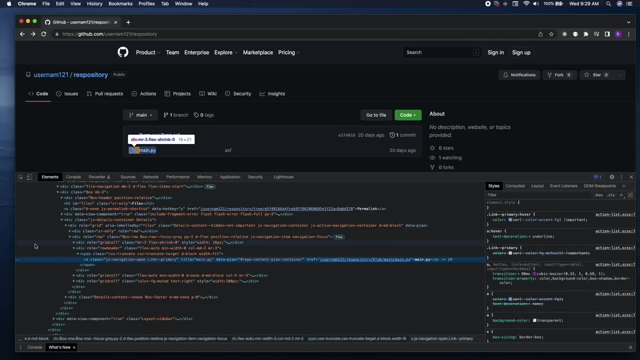 And see if we can find what these links. we'll see what specific class these links all have in common, so that way we can run Selenium to pull all the links. that would hold every single file within this repository. So we can inspect this and it will tell us: this is the line. 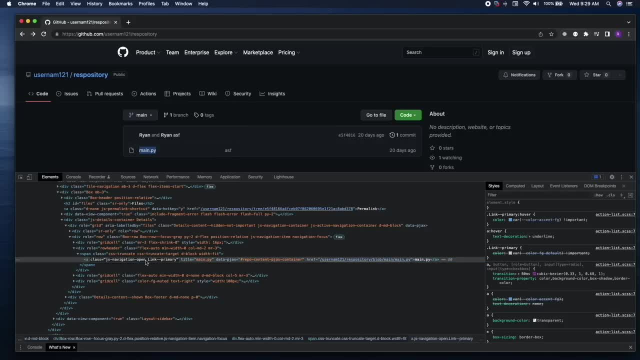 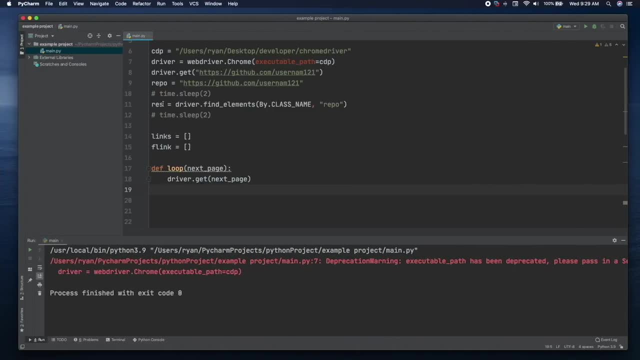 And so we'll just go ahead and click this first class and see if it works. So we'll just copy this. And now we'll need a new resource, So we'll call this. we'll just call it resource two, because I'm terrible at naming variables. 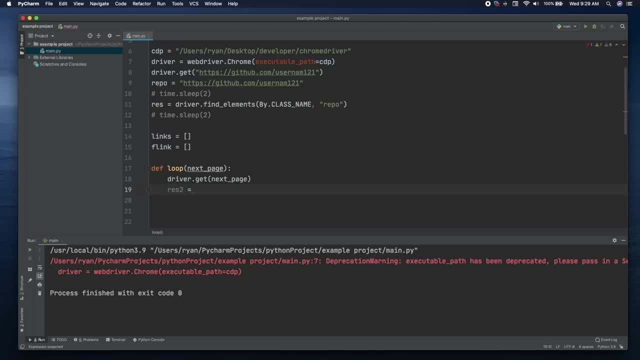 And if I had more time to think about it I would probably come up with something better. But you can name it whatever makes sense to you. So if I made this tool and somebody else just saw it online, they wouldn't be able to understand. 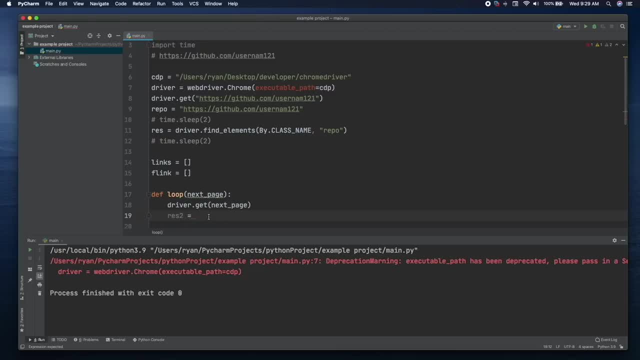 what's going on? because I suck at naming variables, But you can name your variables better than me, And so we're going to. I'm going to let you name your own variables, but I'm going to name mine resources, And I'm going to name it resource. two, because I suck at naming variables. 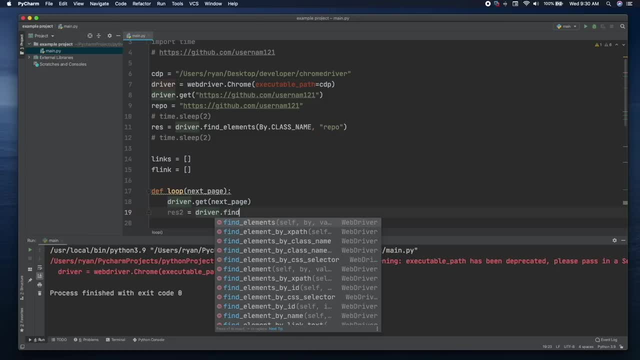 So we're going to go driver dot and we're going to do a find elements just like this one, And then we're going to say by class name- this should be getting familiar to you by now- And then the class name is the one we just copied. 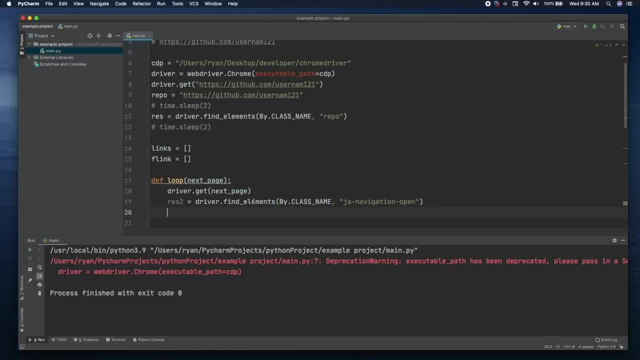 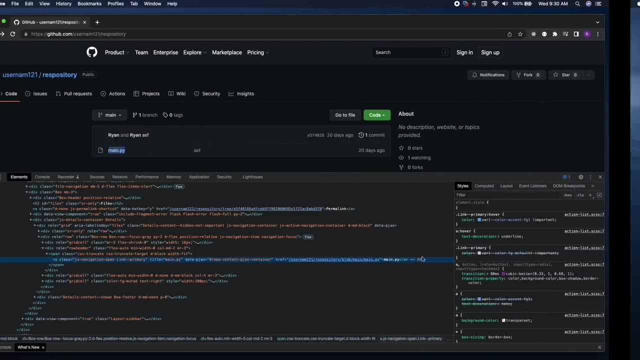 If this works, it should be able to print for us. that it should be able to print for us this class right here. We'll see we can actually get it to print mainpy. So what we'll do is we'll print And then we're going to copy this. 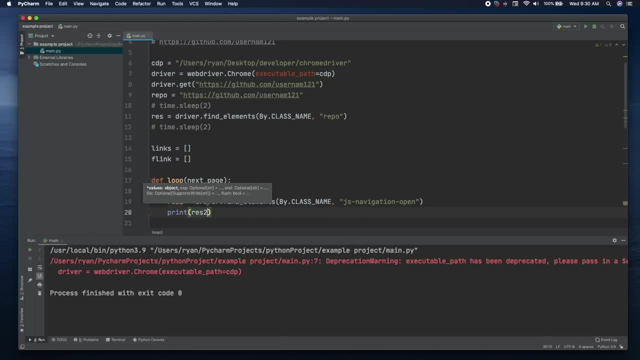 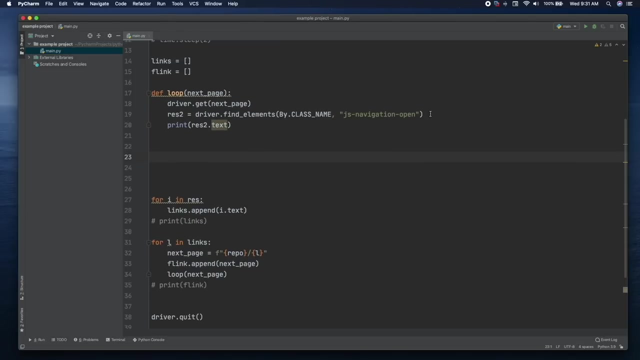 And then we'll print the resource two dot text. Okay, Apparently we don't need dot text, We'll just print resource two and see what happens. And that has run. and it does need resource two dot text And the reason that this is not working is because we need it to loop through this links. 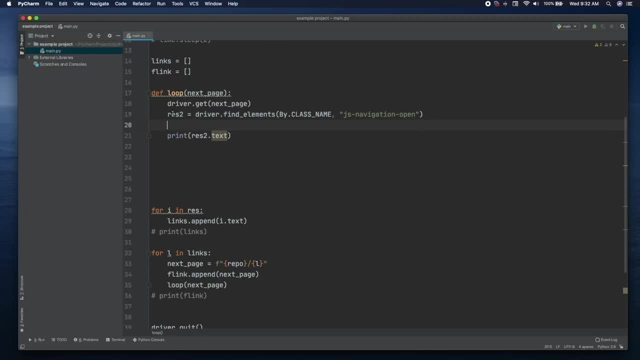 this resource that could be holding multiple This variable. It's holding multiple links within it. So, like we did down here, we will need to go for and we can call this I if we want, but I'm going to change it. 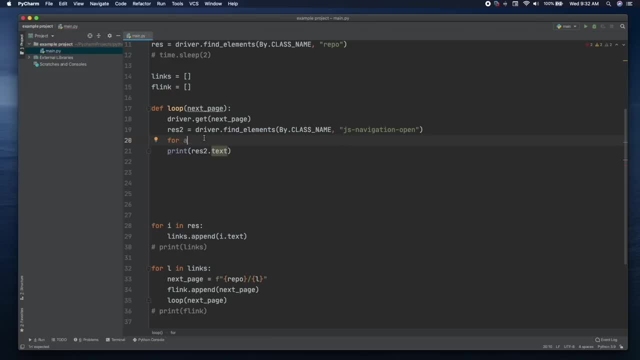 So, the way you don't get confused by all these different variables in our for loops, we'll call it for a in resource two And then we're going to print resource two dot text. We're going to and we're going to print, instead of resource two dot text we're going to print. 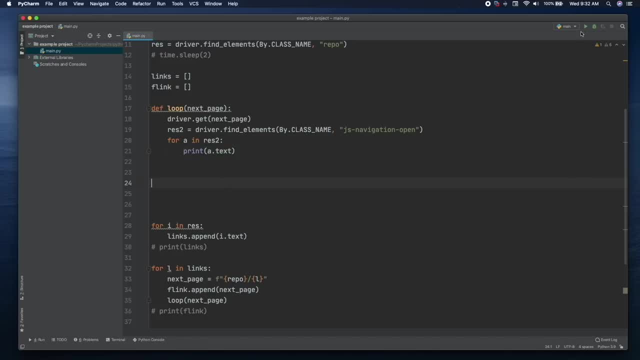 a dot text, So that a way we can make sure it is printing for us the mainpy, So that a way we can tell it to click on mainpy, So we can. and now what we're going to do is we're going to do a comparison inside of. 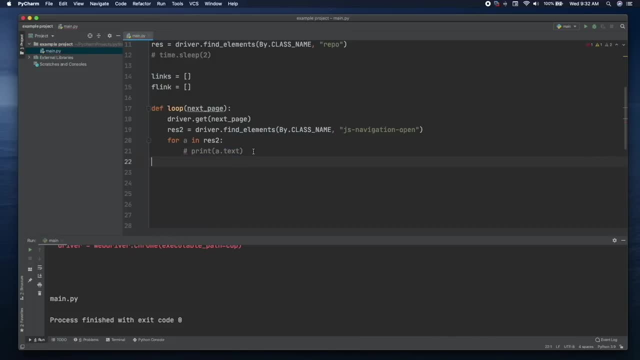 an if statement. we're going to comment this out And instead of getting this little error right here, we're going to type in pass So that a way it will ignore the air for us, And we're going to say: if the letters together is pi, are in a dot text. 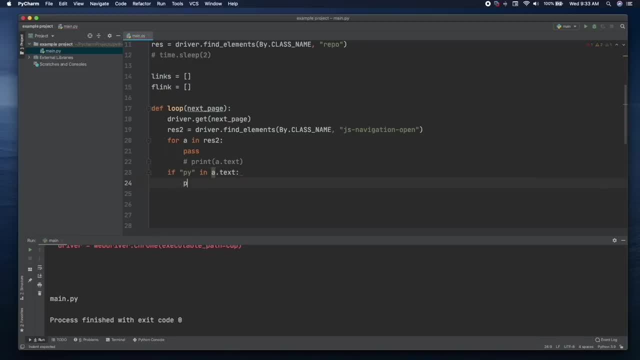 Okay, Then we want to do something. We're going to say: print It worked. pi is in the text. So now, if we run this right here- Oh, I see an error- We're going to get a problem. It says it worked right here. but the reason this rate we get this right here is it says 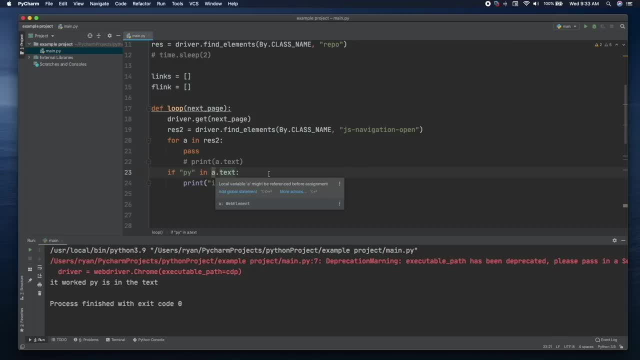 this is a local variable inside of this segment, So this is really not good practice. If you were working for a company as a programmer, you wouldn't do this, But we're not looking to work in a company as programmers. We're looking to use programming for hacking. 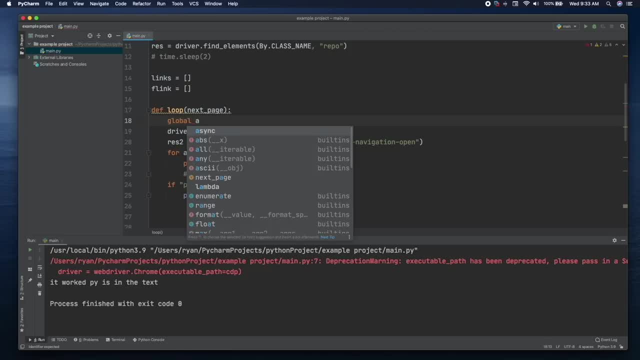 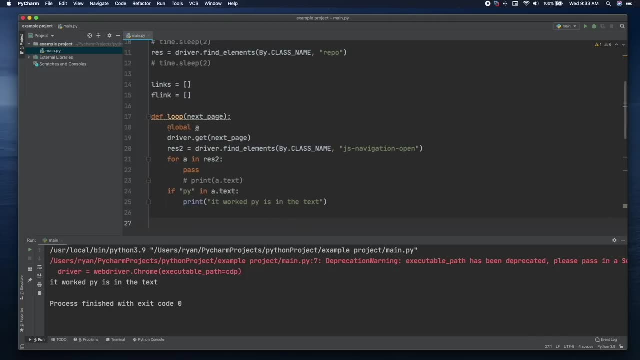 And so what we're going to do is we're going to make this a global variable. We're going to say a is now a global variable and can be accessed anywhere, And it gets rid of this for us, The reason you wouldn't want to make this global. 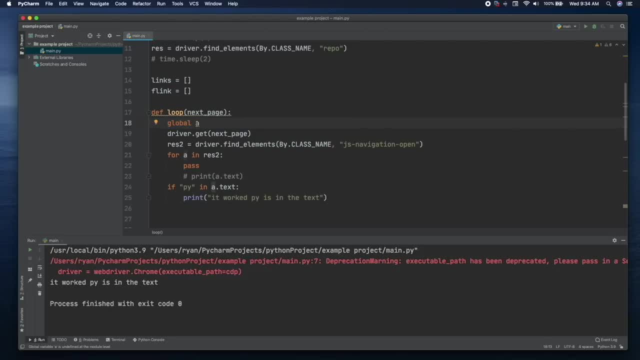 Let's say we made this this for loop with the eye and we said it's a global. Now this I variable everywhere we used. it is going to be everywhere in our code. Okay, We're going to use the variable a anywhere else outside of this, because we have made 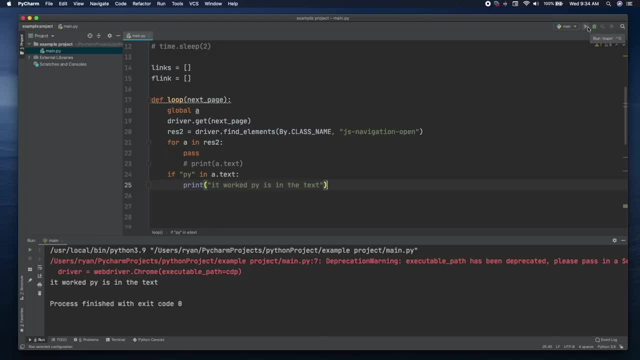 it a global variable And that is really not good programming practice. but for the sake of our tool it doesn't really matter, So we're going to use it. We'll run this and it should work for us. And it says it worked. 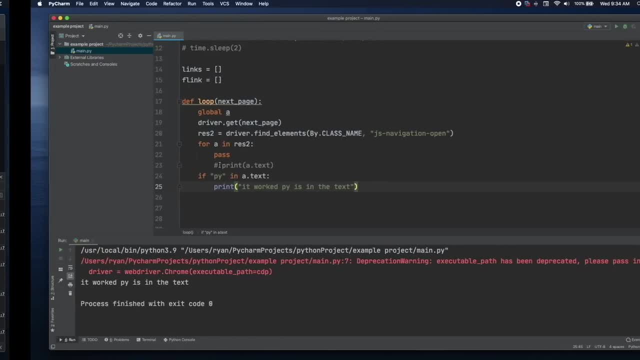 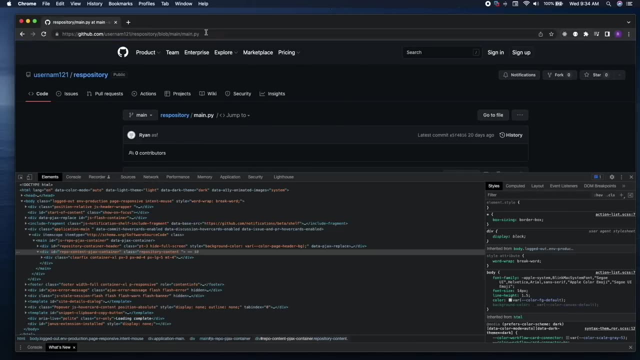 Pi is in the text. What we'll do is we can do the same thing we did before and we can click on this main dot PI and look at our URL so that the way we know how to structure it. And then, after this time, I promise 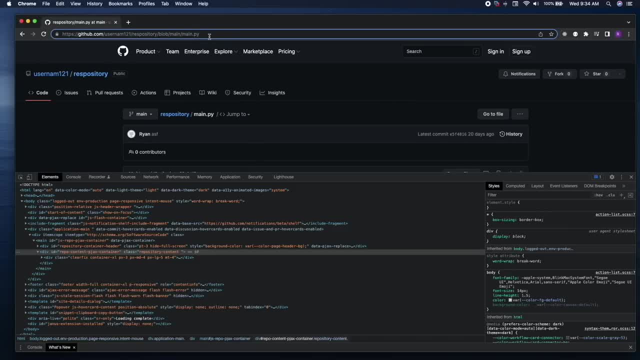 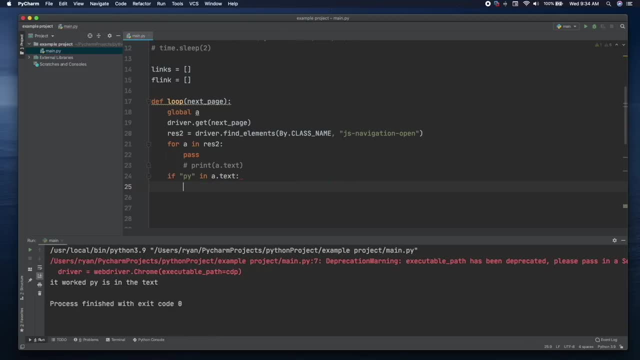 We'll use the click function or the click method actually, And it'll make it much easier for us. So the way we would go about this- we'll delete This- is going to be similar. If you want, you can try and do something like this and get the next page based off. 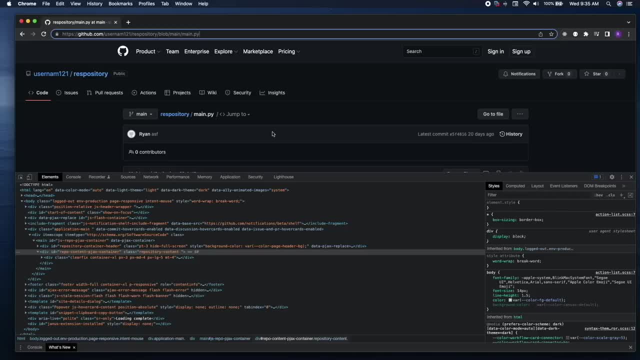 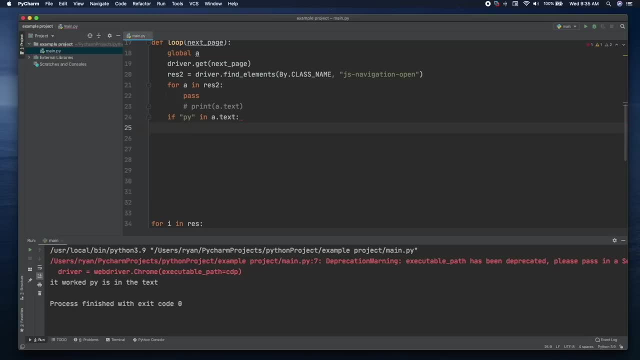 of this URL that we see right here. So if you want to take this challenge, you can go ahead and do this now And for everyone else. I'll walk you through it Now. We'll call this. Uh, we'll just call it. 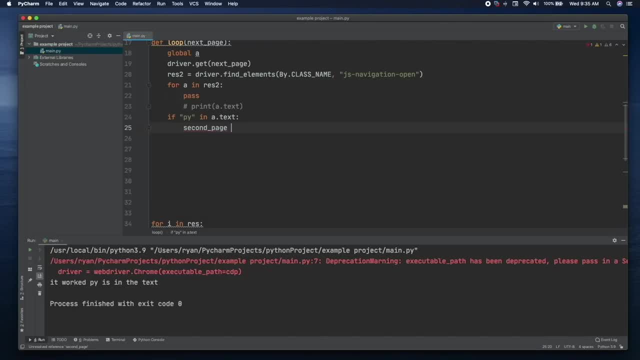 The second page, because I'm so good at naming variables, And then we're going to make this an F string, just like we did down here, And we're going to add all this together to get the that new URL. So we're going to go ahead and we're going to say: repo. 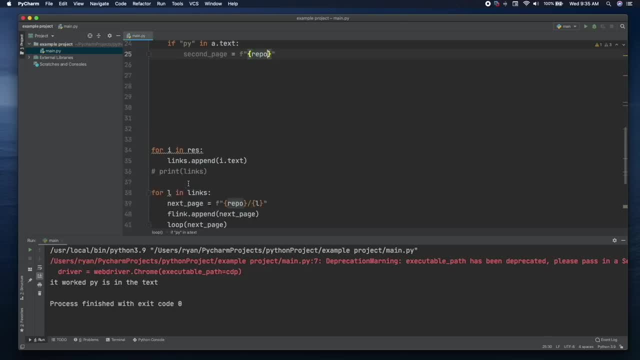 And let's see what did we name this one down here? We named it. We'll just call it repo, because we have the repo up here. We'll just copy this. Actually, we'll just leave it. So we'll just use the repo how it is. 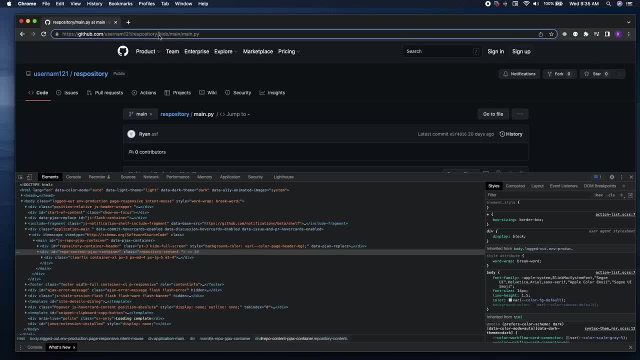 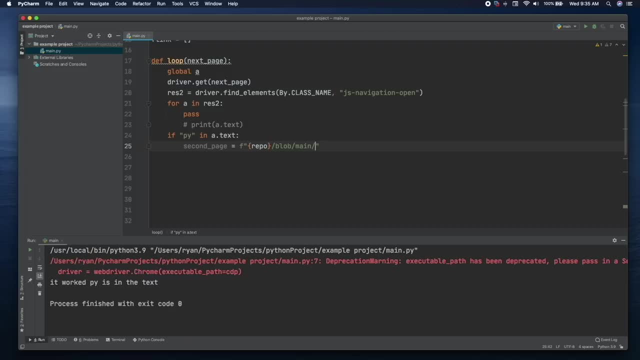 Okay, So we'll just add in this right here and we can copy that and paste it in, And then we'll add our slash for the new page that we're going to want to go to And we'll add this variable in right here, a dot text. 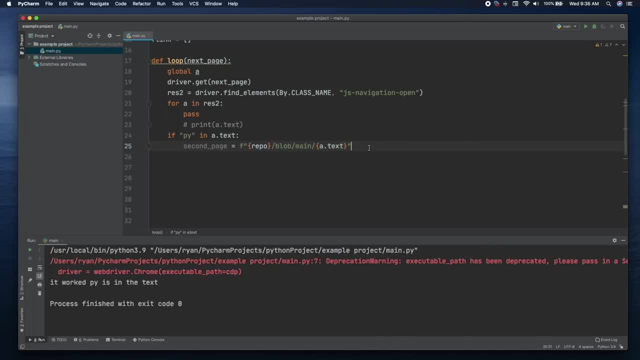 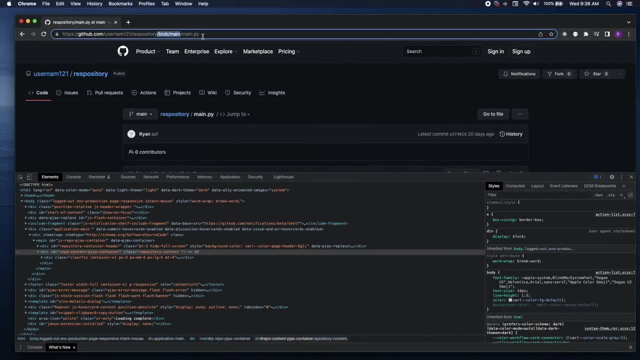 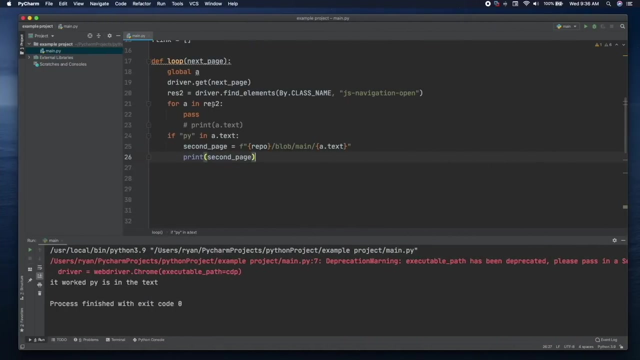 So we'll say a dot text And now if we print second page, we should get a URL printed that looks exactly like this. And the reason we did it this way is because we're going to be looping through in this for loop all of the links, and we need these links right here. 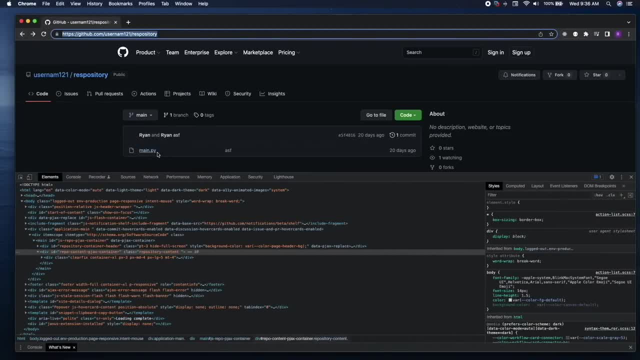 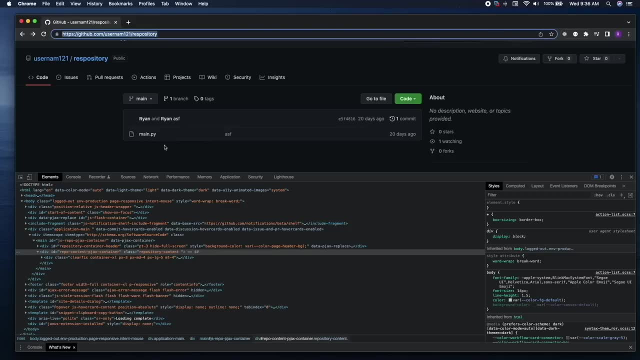 So if there was, let's say, we had a mainpy and then we had a CSS, a maincss, and then we had a indexjs and then we had indexhtml or we had filephp And there was a whole bunch of files inside this program. 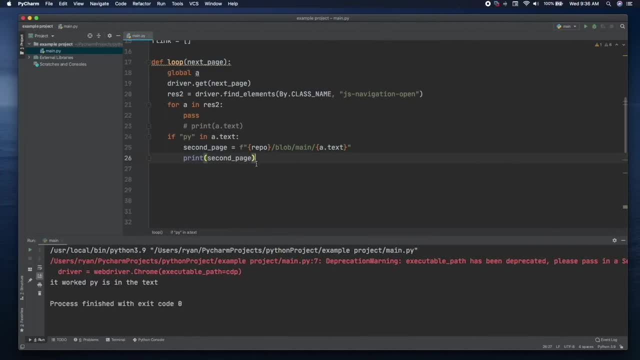 We would want to loop through all of these files for us. So what we're going to do is set it up this way so you can add to it. So, as an example, it'd be like if js was in a dot txt, then it would do the js instead. 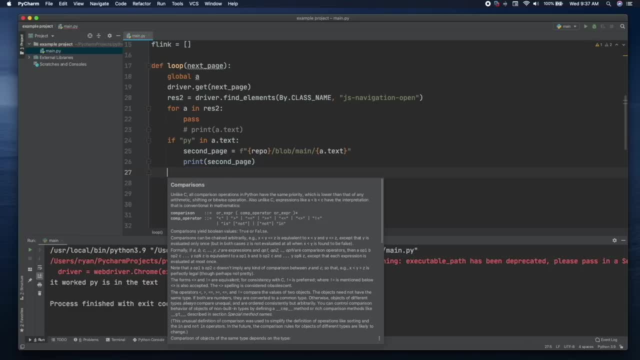 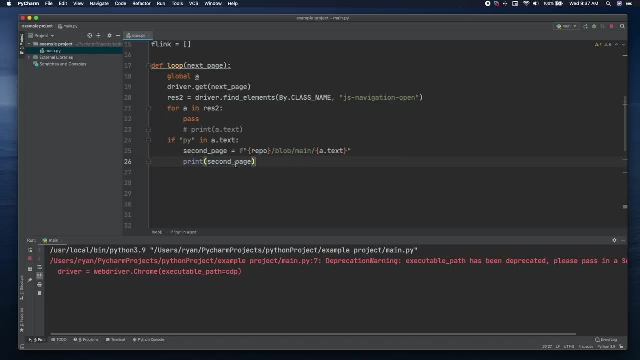 of pi for us. So that's actually a challenge for you. I'll show you how to add those on, and then I'll let you complete the tool as you see fit. So what we're going to do for now is we're just going to print this second page, and it's 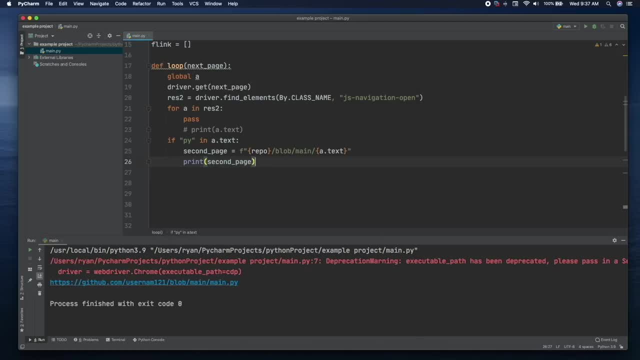 going to open it and it's going to tell us right here: Okay, We're going to add in a timesleep so that way you can see that it has worked. So it did print for us right here, Okay. So I just noticed, if you click this page, it takes us to a page not found. 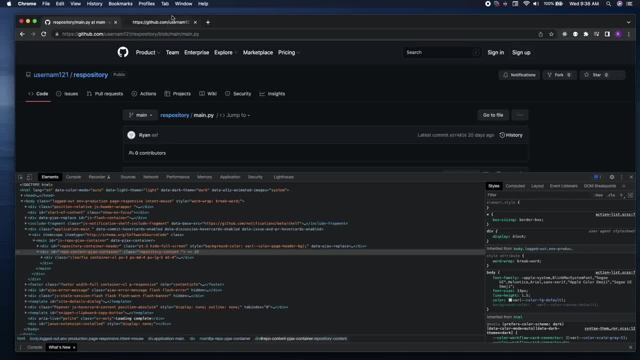 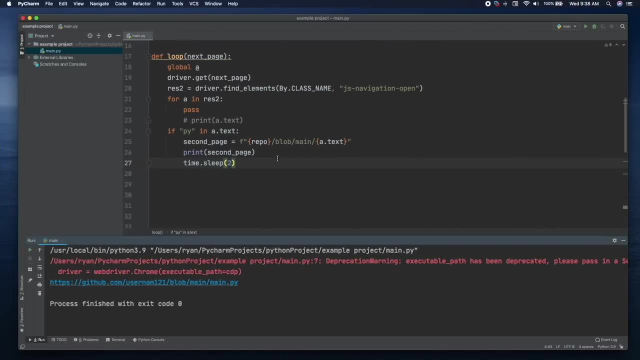 And when you compare the two URLs, we're missing this repository right here. So what we will need to do is add in an extra repository and let's actually see if we can just grab this next page right here. So we're looping through what would be considered the next page. 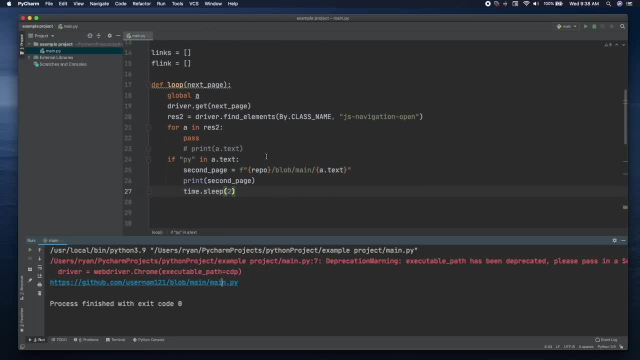 Where's our links at: Okay, So we'll see if we can loop through the next page right here. So we'll add in instead of repo. we need it to have that repository on it So we can say next page which is getting passed through our function. 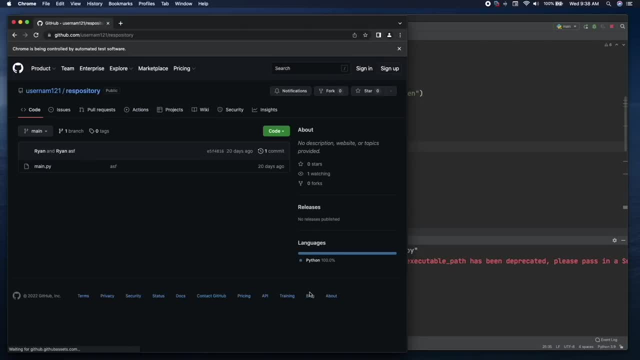 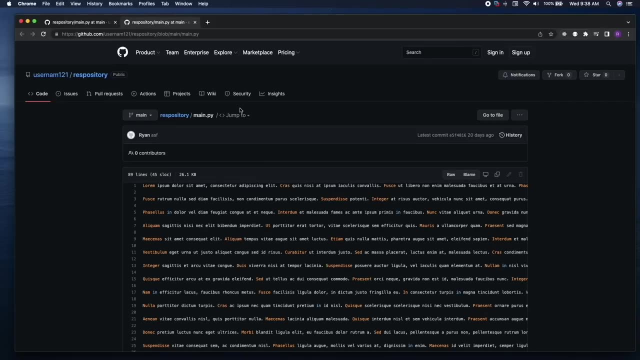 And now let's print it and see if this works for us. It's paused and we have the repository And if we click on it it brings us to the next page that we want. Okay, And if we were going to add on to this program, let's say, like I was showing you, if there's 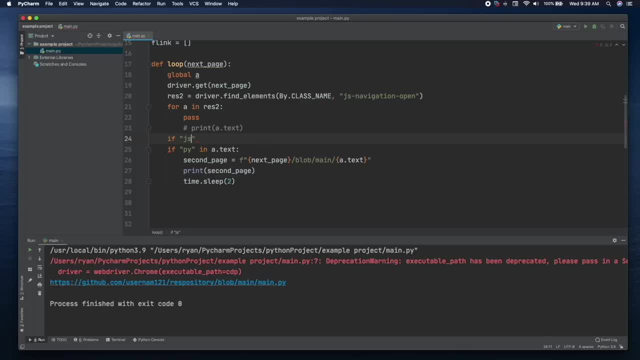 a JS inside the file. So like, if this is a JavaScript file instead of Python, or maybe we want to check for JavaScript and Python and maybe later we want to add PHP, we can do that, And so we can say atext and then we can say, right here, we need to close this off. 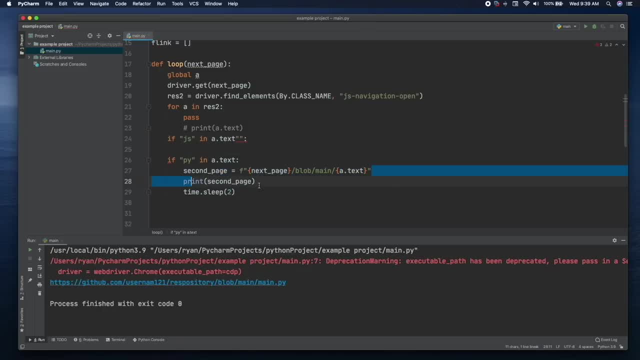 And then we could say this exact same thing, And then we would print whatever it is that we want to test for. So we would say: we're going to go to a new page If a JavaScript is found, then we're going to do this. 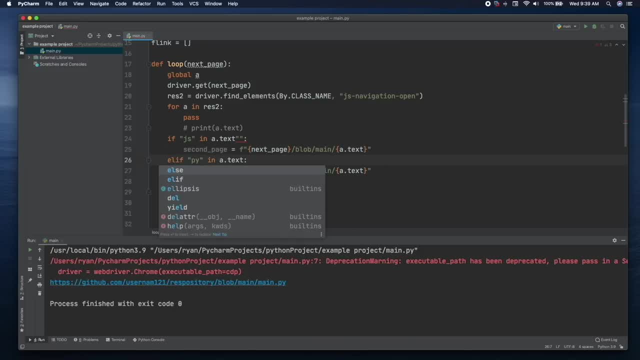 And then we can turn. we would turn this into an LF and it would say: okay, there's no JavaScript file. So, because there's no JavaScript file, we're going to check for a Python file, And so we'll go ahead and run this, make sure we have no errors, and it's going to pass this. 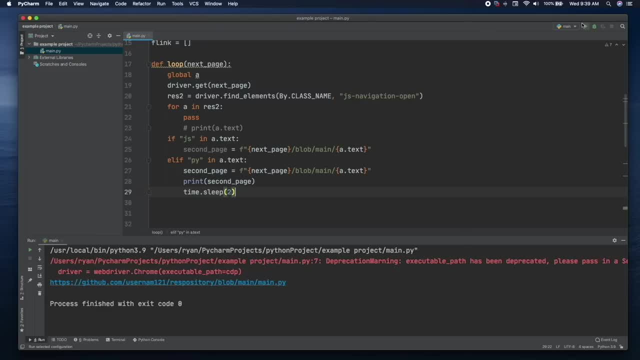 JavaScript file And it's going to go straight into the Python file for us. So we run this and it passes this right here and then it closes and it pulls down the mainpy. So what you would do if you wanted to make this a comprehensive tool, you would say: 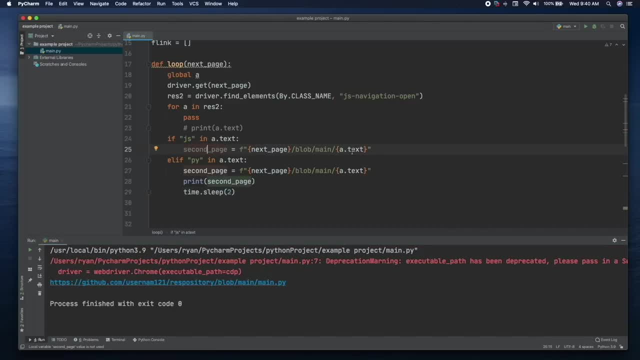 if there's PHP, if there's JavaScript, if there's a JSON and any other kind of file that you might want to check for sensitive data. but because the repo we're working with to build this tool doesn't have any of that, I'm going to just leave it with Python. 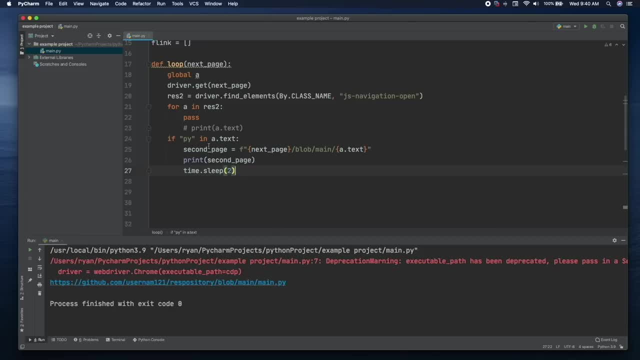 And I'm going to challenge you to make the if statements and the LF statements and the else statements all on your own, And maybe you can go look at repos and see what you want the program to open up to look for passwords. Now that we know that works, we're going to comment out this sleep function because we 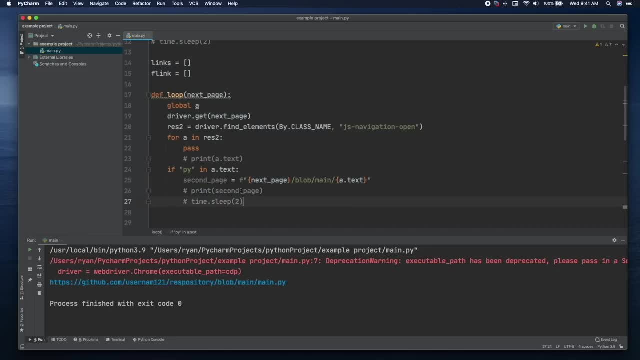 don't need it. We also don't need it to print the second page. What we're going to do now is we're going to call a second function inside of this function. So it's kind of getting like a the movie inception. 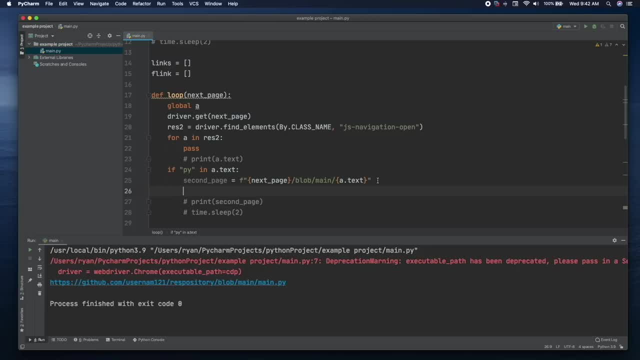 We have a function that we're calling inside of another function, but we're going to do this one in a much easier method, So we're going to go ahead and we're going to call this. one Function is going to be called going for raw, and I'll show you why I'm naming it that: going. 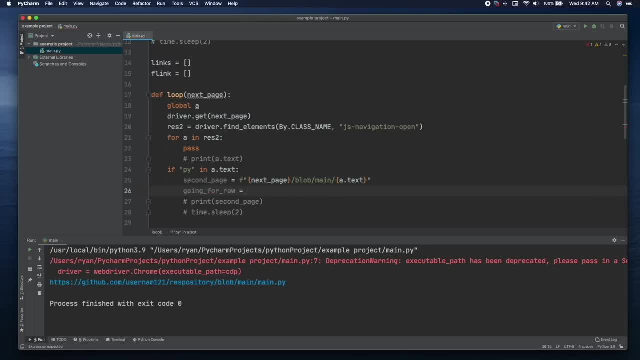 for raw. This is going to be the best variable name I have ever come up with. And then we're going to pass in the second page and then we'll make the function appear and we'll call it deaf, And we're going to call it going for raw. 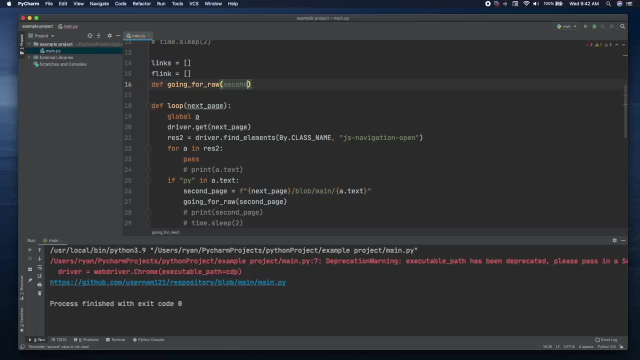 We'll call the function We're going to pass in second Page. This is actually going to be the third page. We might actually change this inside here, this parameter, in just a second. So what we are going to be doing is going for the raw. 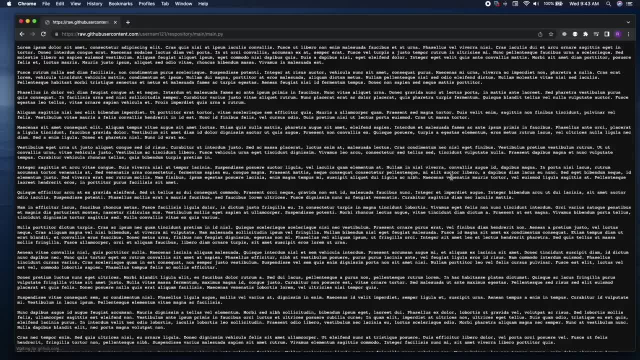 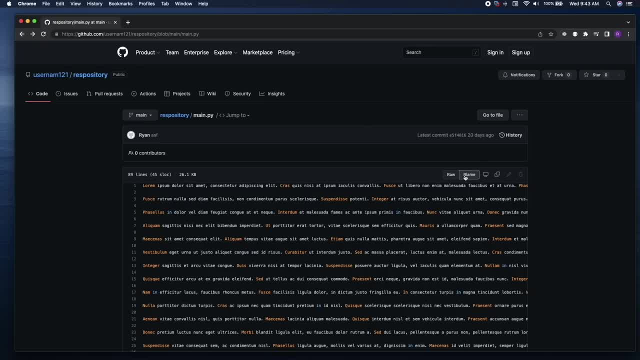 So, now that we are able to get to this page, we want to click this button so that we can get to this page. So, in order to click this button- it is going to be so much easier than what we've been doing, as we've been editing this right here, the URL, and adding to it. 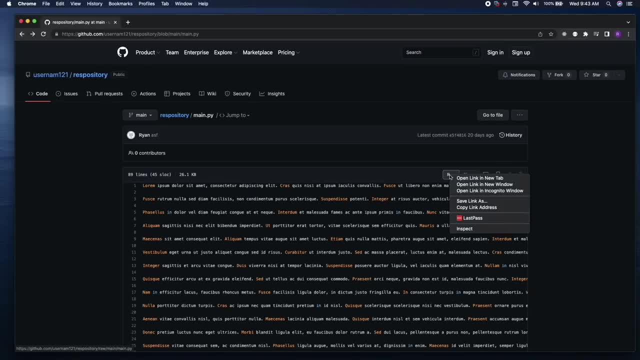 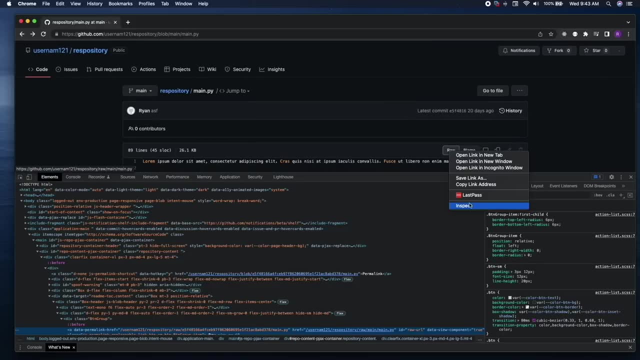 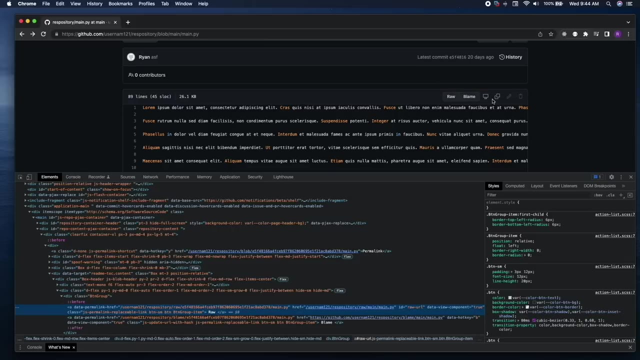 What we're going to do is just click the button So we can inspect this right here and see where is it will inspect, see if it can pull it up for me. Okay, Now that we have inspected it and you can see when we hover over this, right here we. 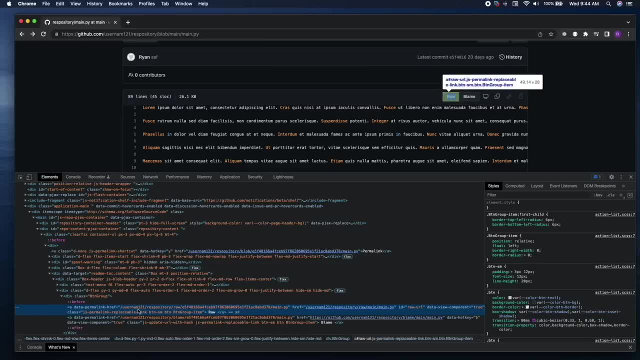 can see this raw button. So now what we need to do is the same thing we've been doing, and we need to find a class and see if we can find a class that is used only with that button and get it to open up this raw. 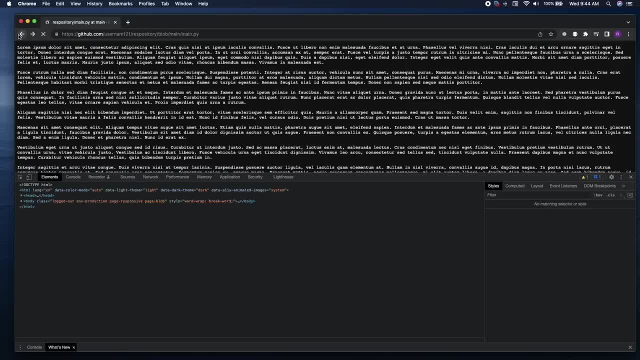 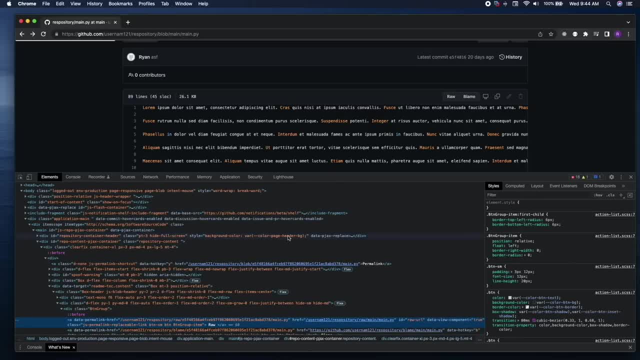 So that way we land on this page right here. We're just going to copy that class name that I just showed you right here and see if that can open up this tab for us. So now, under this function, what we're going to do is we're just going to say we're going. 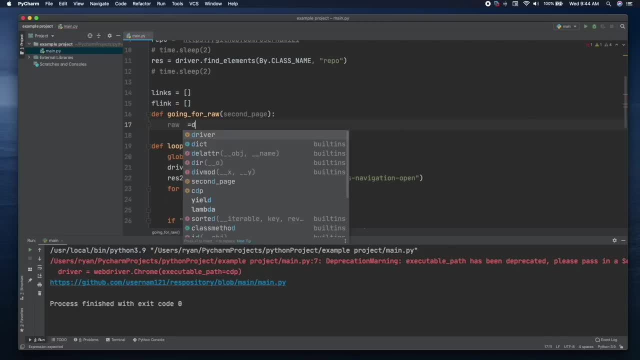 to type in raw equals and then we're going to say driver dot find elements. Actually, this time, instead of elements plural, we're going to do just one element and we're going to say by Class name, just like we have been. 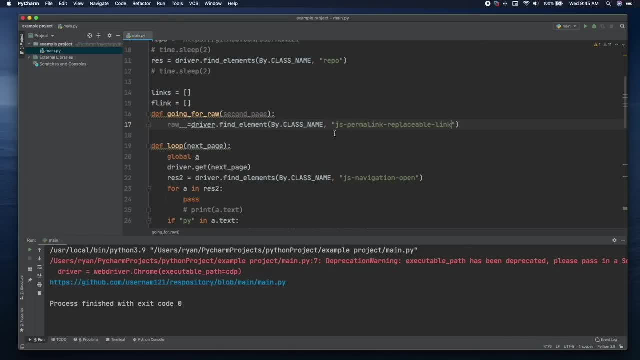 And then we will type in, we'll paste in our link right here. And now what we're going to do is something really simple. We're just going to say raw, dot, click, and it's going to click that button for us. And then what we'll do is we'll come over here. 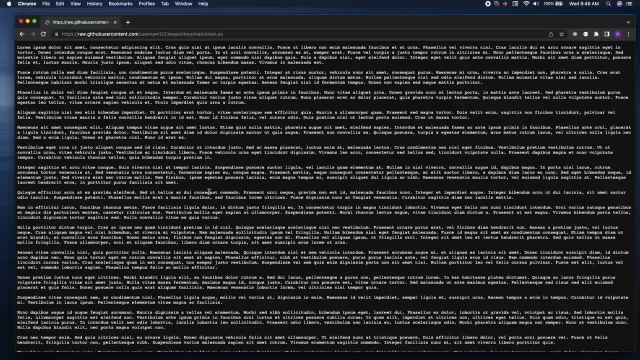 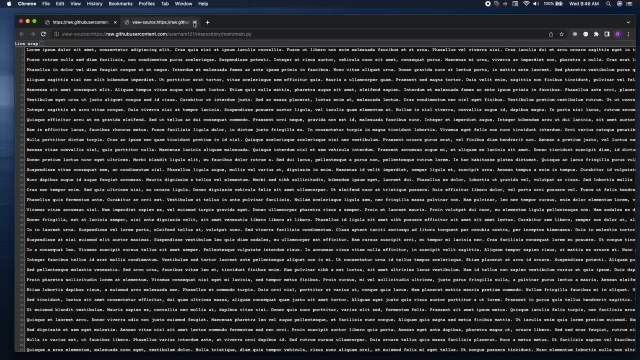 We'll click this. Okay, Now that we're able to get to this page, we're going to tell it that we want the page source. We're going to want it to right click and say view page source, And then we're going to 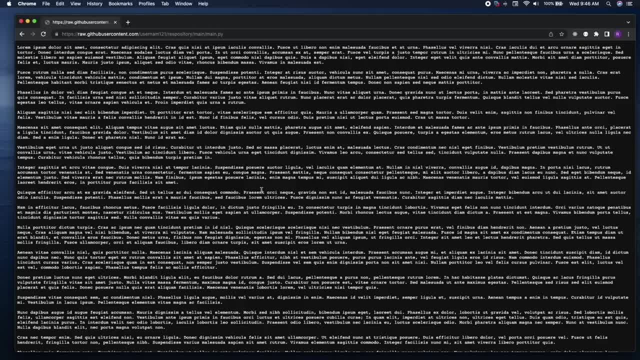 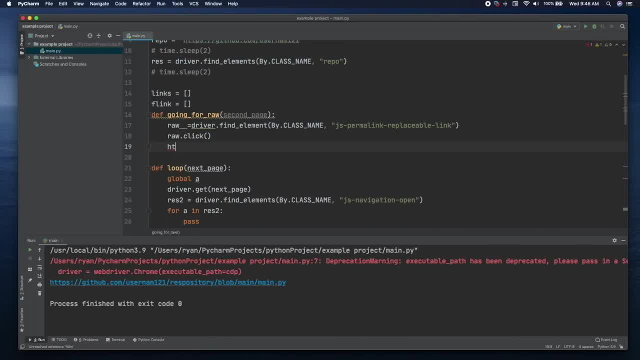 Grab all of this inside of an F string and then see if we can find a password in it, And what that's going to look like is something like this: We want the HTML, HTML, and we're going to say driver dot page- source that away. 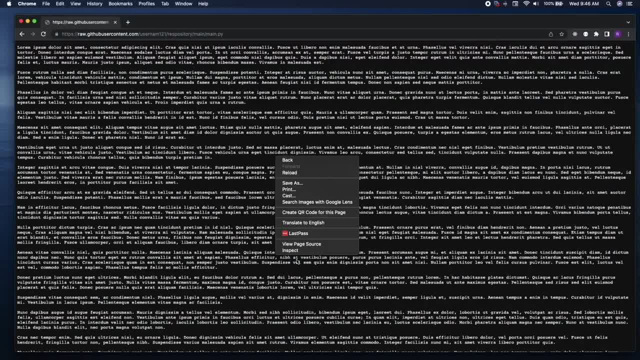 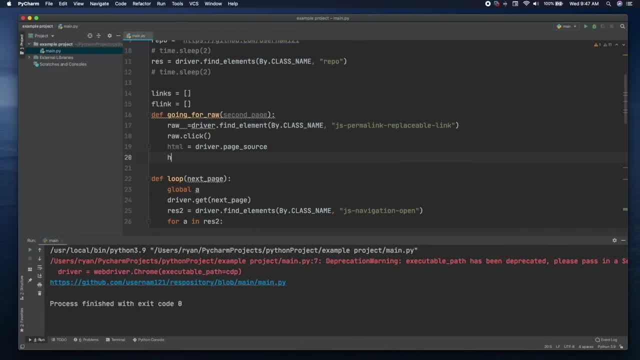 It grabs the page source for us, Like we I just showed you as the same as right clicking it and view page source. We want it to grab that. And then we're going to put this into an F string and we're just going to change the. 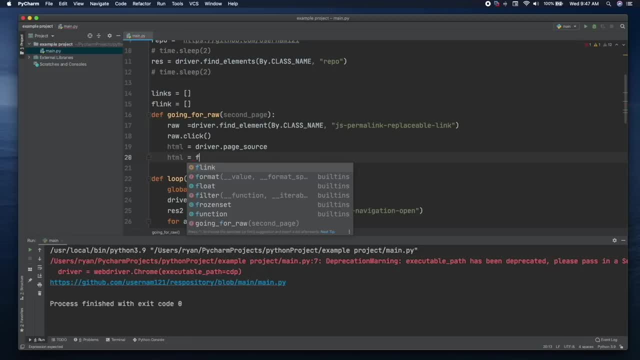 HTML. It's going to be a variable and we'll say: HTML is going to be equal to this HTML inside of an F string, because we want it to be converted into a string. So we'll say HTML. So now we have this in a string and just to check it, we can say: and just to check this: 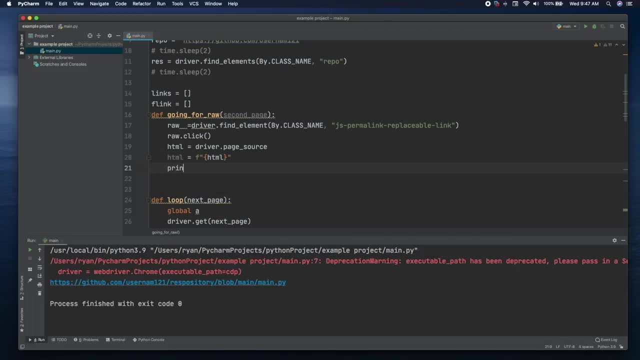 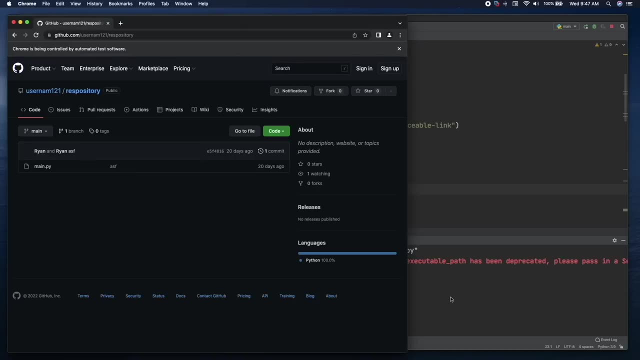 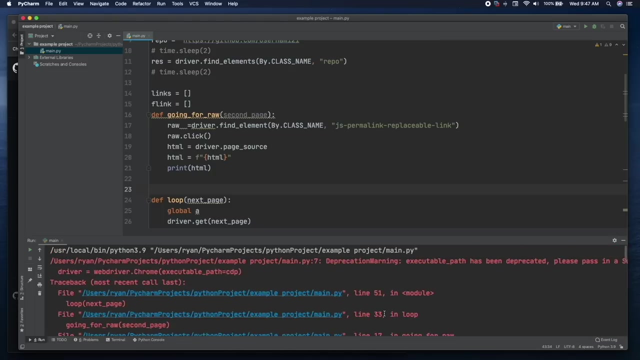 we can say print And then we want to print HTML And now when we run this it's going to print All of that page source for us into our console And we want to make sure that it is in a string that I we have an error. 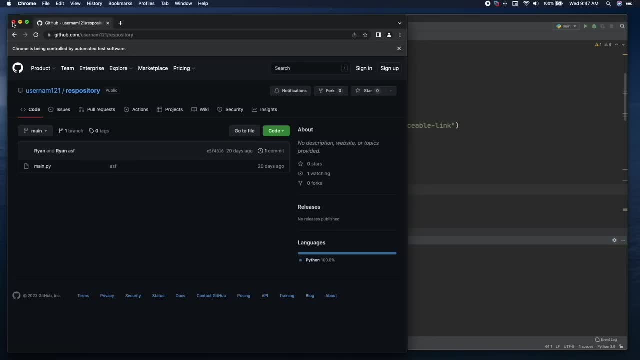 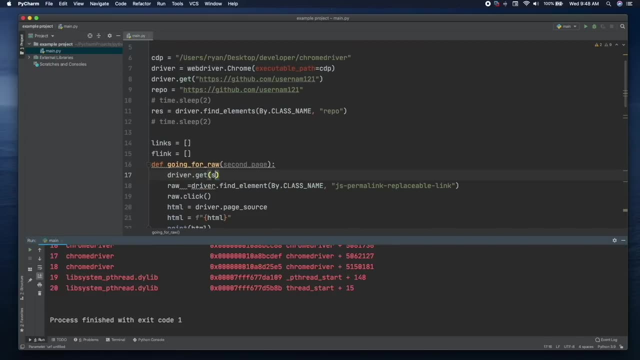 Let's see if we, let's see if we can find the error here. We need to use driver dot get and then we need to get the second page right here. So now, if we run this, it should work. And it clicked the button. 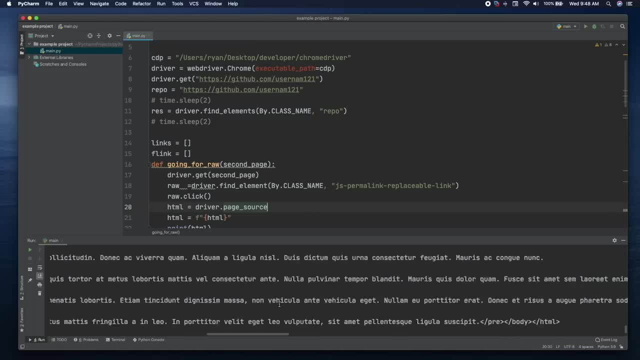 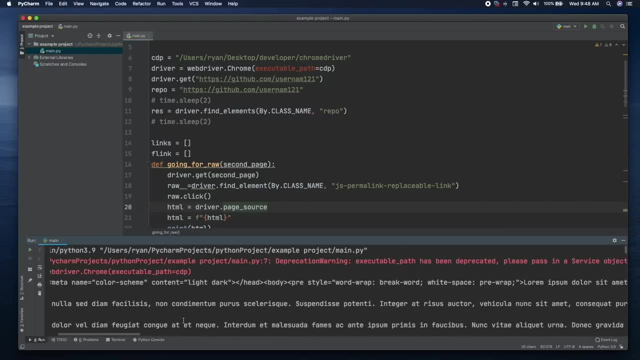 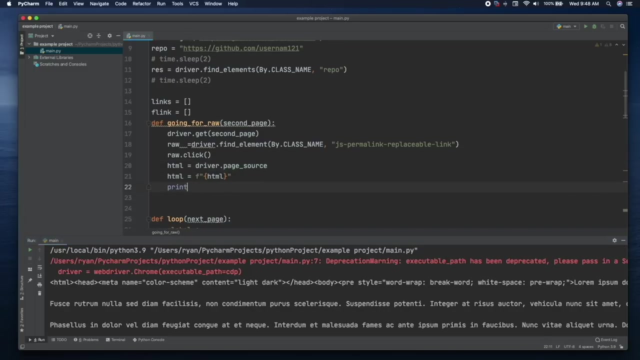 And it printed all of this for us And let's see if it printed. here We have the tags for us And now that we have this printed and it's printed inside of the HTML, So we know we grabbed the entire page. We can close out of this. 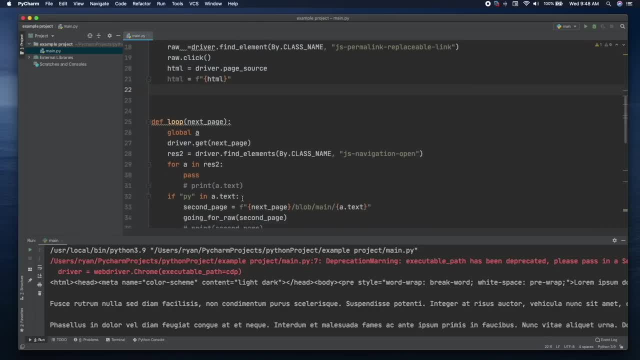 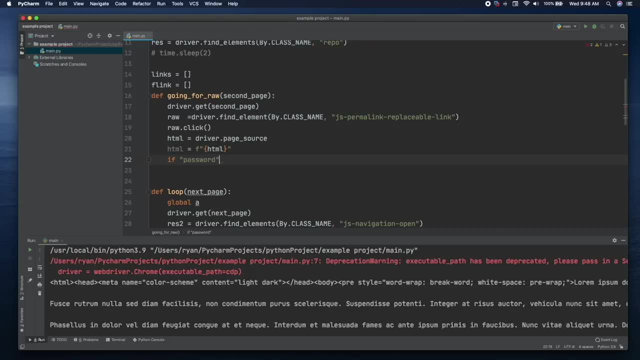 We don't need this print statement. What we're going to do now is really similar to what we did down here. We're going to say: if the password is in HTML, Yeah, Yeah, If the password is in HTML, We want it to rent. found a password. 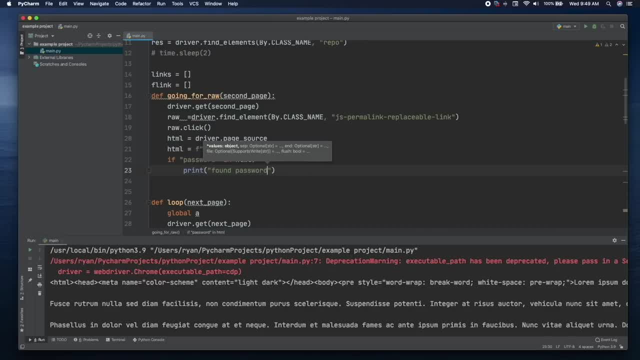 And so we'll say print found password. and now we can run this and if it finds the word password inside of the HTML, it's going to print found password. And if we wanted to, we can turn this into an F string and it we can get it to print. 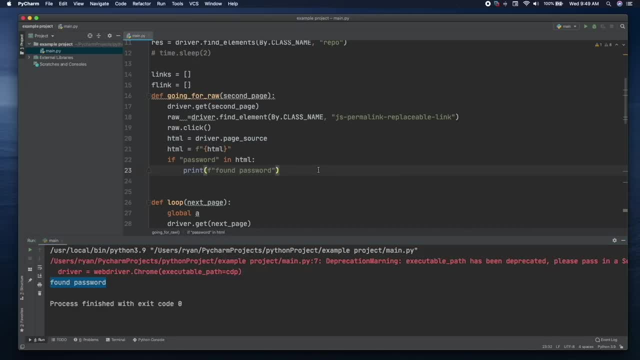 for us the actual URL where the password was found. And we can say something like this: we'll make this an f string and say: we want to print second page. so it'll say: found the password and it'll print the page for us and we could click on this second page and go. 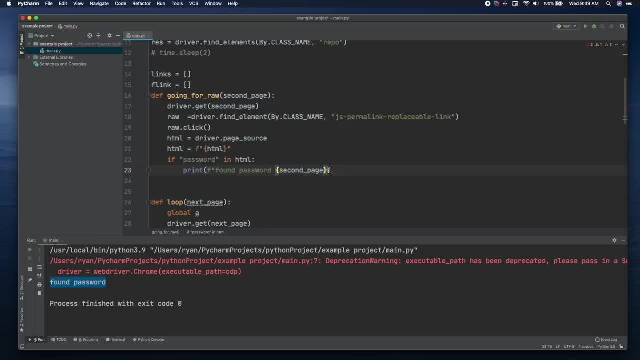 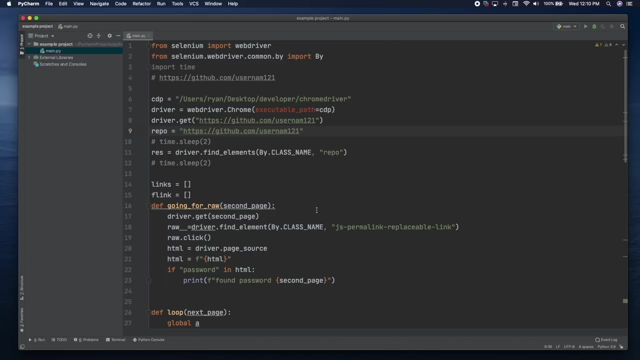 to it. we're getting this error here because we need to put this inside of our string. so if we print this now, it'll tell us it found the password and it'll give us the page to go to, right here to check and see what is the context of this password. now to finish off our tool. so that way, 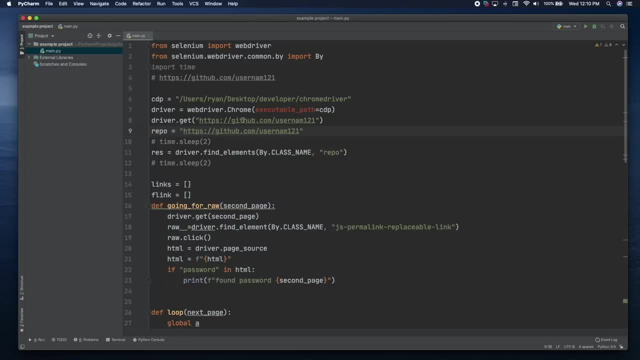 we can scrape any page on github that we want, remembering that we have to get to the page like this: we can go ahead and copy this and we're going to make an input and we're going to name our input: scrape, scrape, just like this, and we will say equals, and we're going to make this an input. 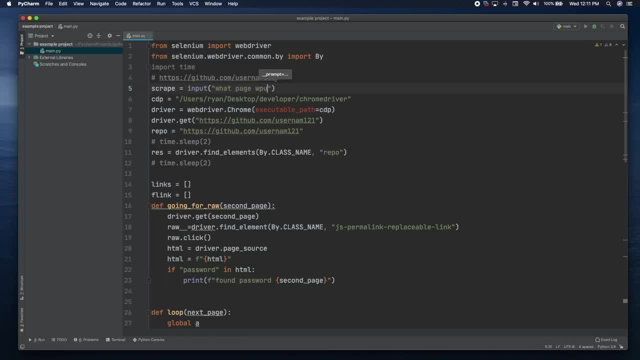 and we're going to say: what page would would you like to scrape? just like this question mark space. and now this scrape we're going to pass into our driver dot. get right here, so we will to pass in scrape. we're going to make this an f string and we'll say scrape. and then we'll. 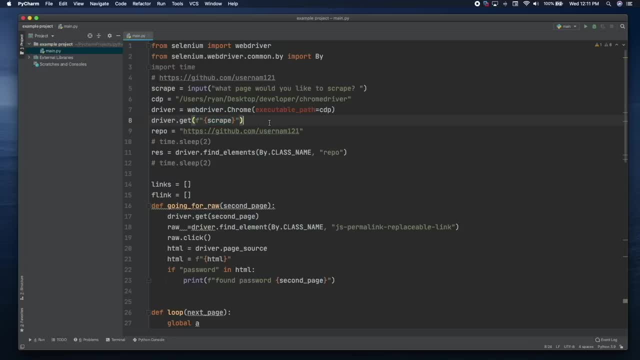 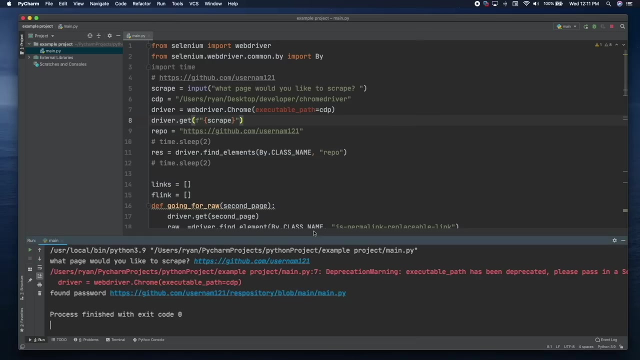 highlight it and put it inside curly braces, and now, when we run this, it should ask us for an input- what page would you like to scrape? and then we put in our page making sure we remember the https, and now, when we run this, it should run the page for us and now you can run it against. 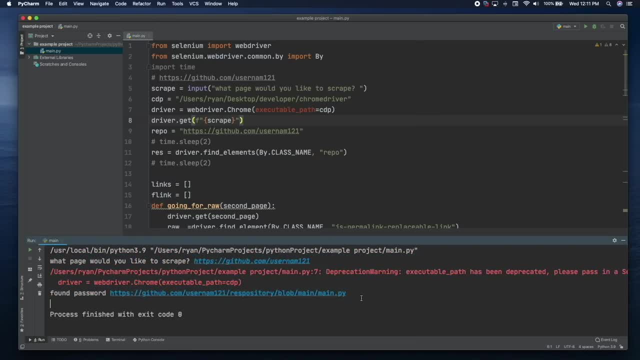 other repos and it is a complete tool for you. if you have any suggestions on a tool that you think we should build next, that shouldn't be too difficult for us, as we are just learning python. please let me know down in the comments, and if you have made it this far in the video, please. 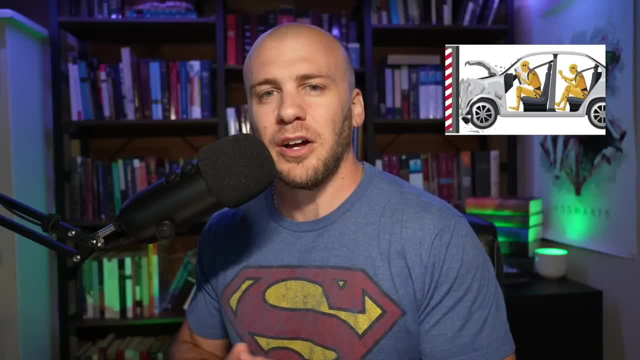 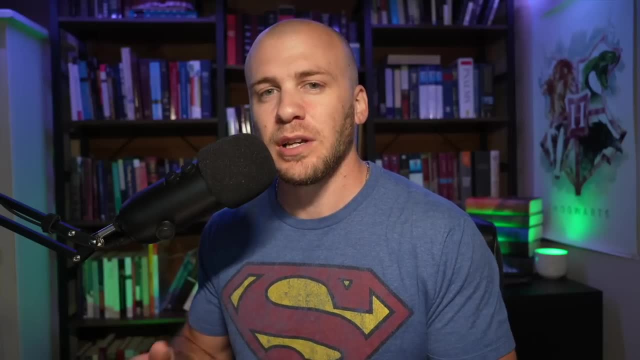 like and subscribe to our channel and we'll see you in the next video. welcome to my crash course on bash. this is not a complete course. i am currently working on a complete course in bash for hackers that is going to be really comprehensive and more focused on if 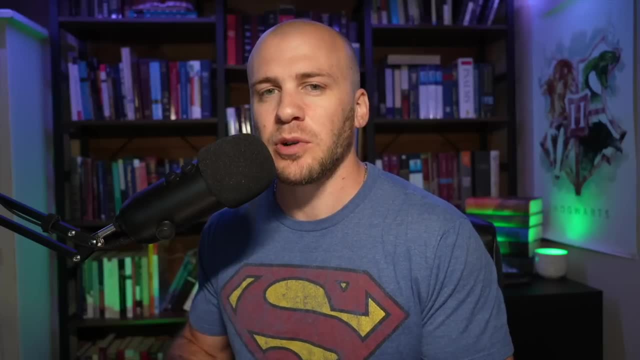 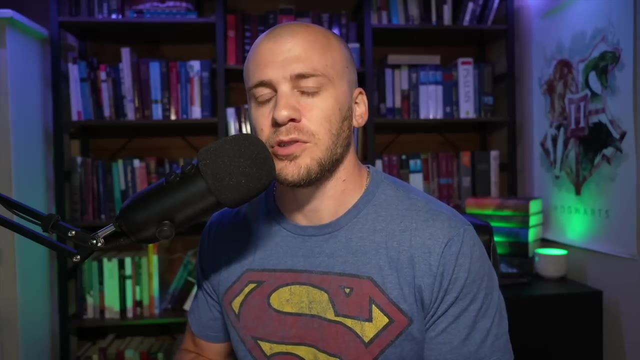 you want to learn how to become a bash programmer or how bash programming works, if you were to work in a company and you needed to know the bash language. this course is specifically for those who want to be able to modify exploits and be able to be an effective penetration tester or 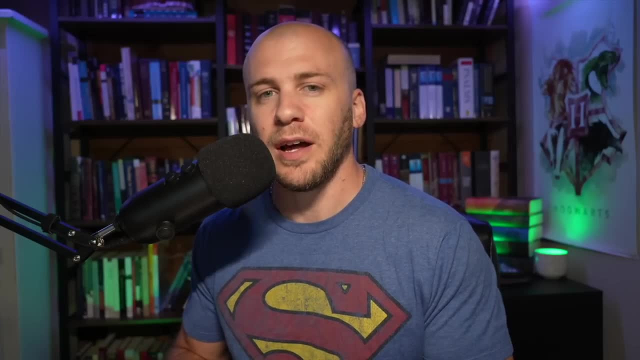 ethical hacker and know the bash language and how to become a bash programmer. and how to become a bash programmer and know the bash language and how to become a bash programmer and know the bash language well enough that you can modify exploits and maybe even write some of your own scripts so that you 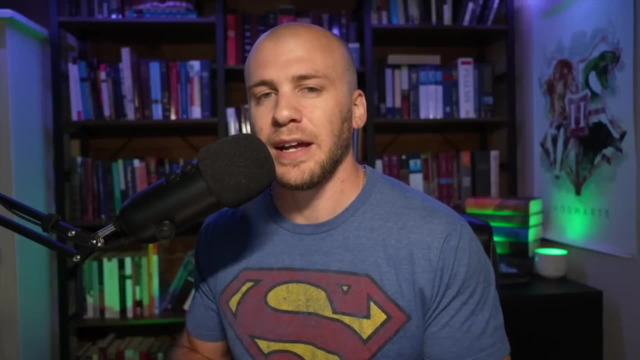 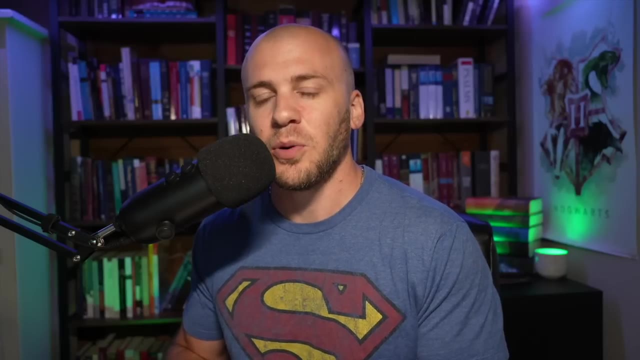 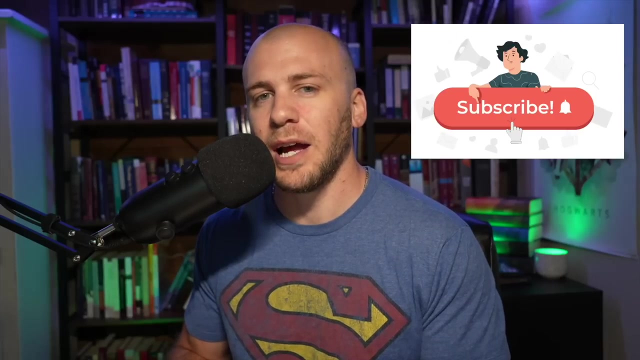 can accomplish all your purposes in the bash world. i know that is hard to believe you can do in the short span of 45 minutes, but that is the goal of this course. so if you are interested in the more advanced course, it is coming and you are welcome to subscribe and wait for that course. 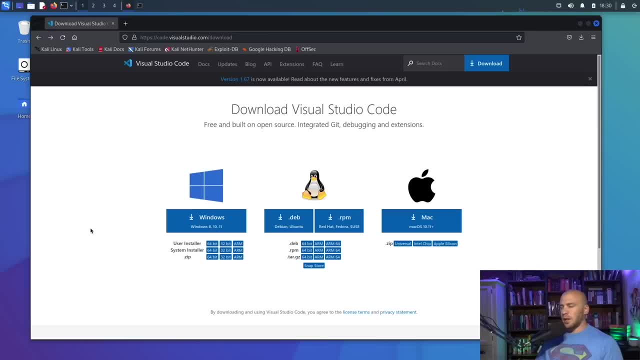 to come out, but in the meantime, enjoy this one. all right, welcome to our bash scripting course. we're going to start off with the download of visual studio code. a lot of people like to just write bash scripts inside nano or gedit or vim, but i don't think that's very useful. 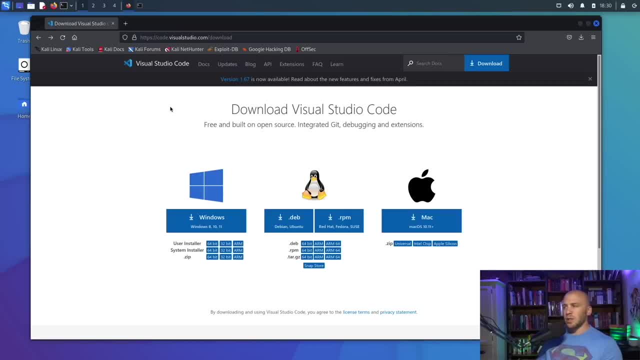 for you as a beginner, because we're going to use a few plugins that we can install on visual studio code. so you can go right here to the link right here which is in the description, and you can click this download right here and you can click it and then you can click download if it. 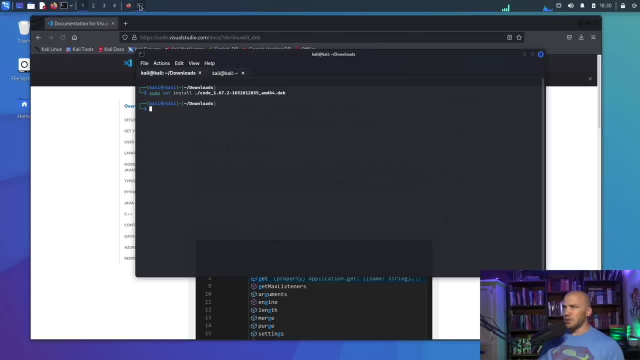 doesn't go, then you will save and say, okay, i have already installed it, so i'm not going to download it again. it will look like this when it's downloaded into your downloads: okay, and then the command that you will need to insert into your terminal is this one right here, so you will be in. 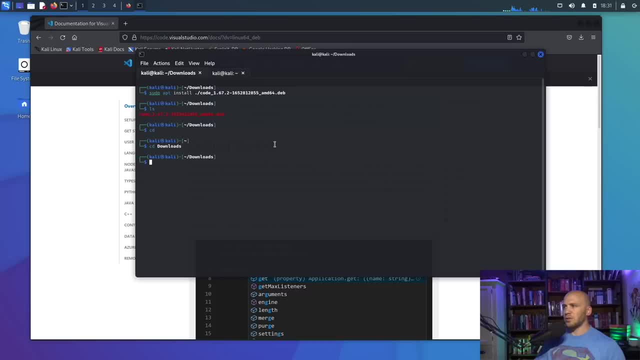 your home directory so you will cd over to your downloads, you will ls and you will see this right here. you will type this into your terminal right here and then hit enter and it will install. this might take up to about 30 seconds, but i have already. 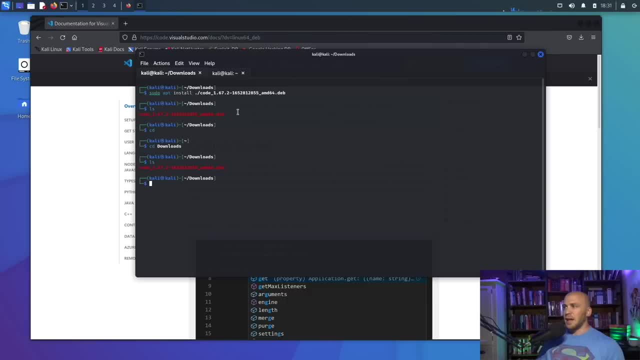 installed it, so i'm not going to run this right here again. and just for reference, if this is not the exact same file that you have, you can just type in sudo, apt install, and then you can type in dots- your dot slash- and then just start to type in code like this and then hit tab and it will. 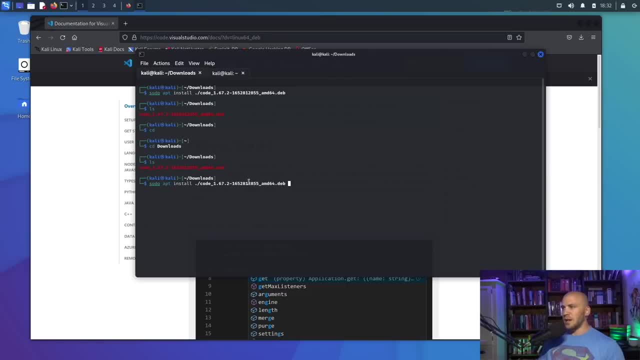 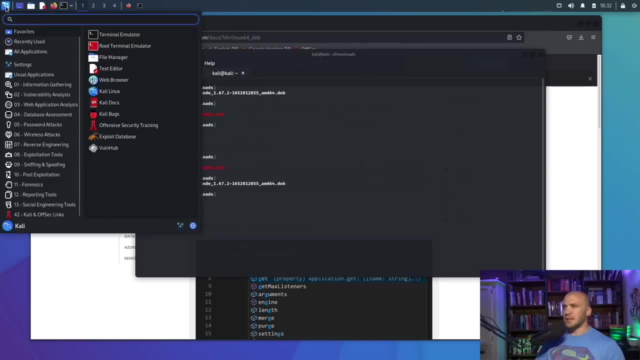 auto complete that for you, so you don't have to go through and do that again, and then you can type in all of these numbers in. so once that is done installing, you can come over to your the drop down and type in visual studio code and it will be right here and you will launch this and 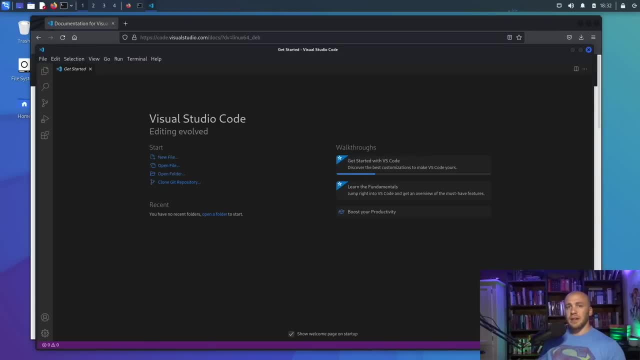 this is where we're going to be writing our code. now. some of the plugins we're going to be installing is shellcode, and you can come over to your little bar right here and you will click this one right here and you're going to search and we are going to search for shell check, just like this, and install this top one You can click. 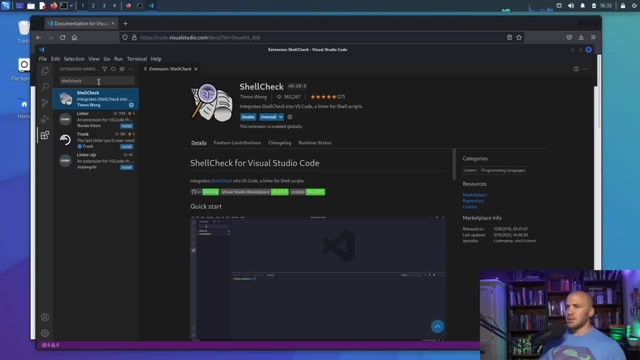 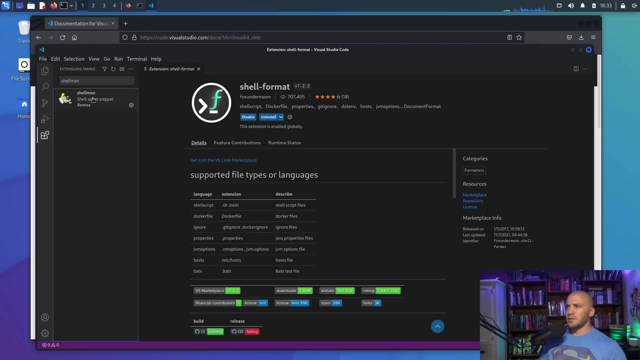 it. I already have it installed. You'll be able to click install, just like this right here. Then we're going to use shell dash format, just like this. It'll look like this and you will click install. Then we're going to want shell man, and it is right here, and you will install, and then we 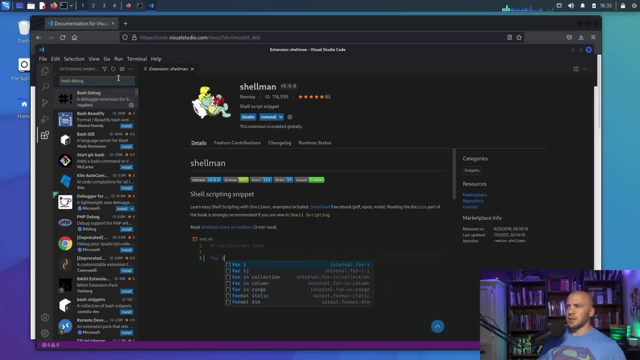 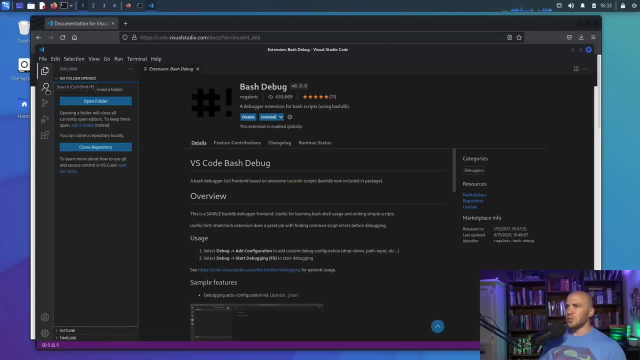 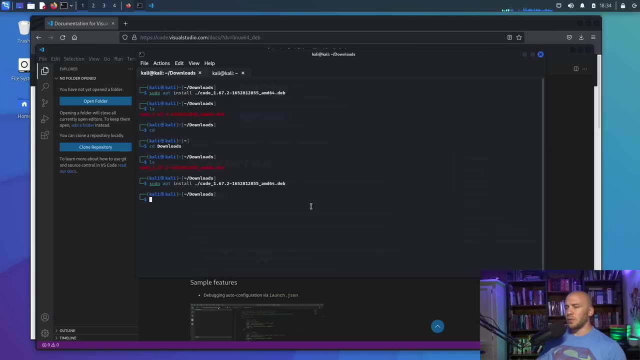 want bash debug, just like this. You can click on that and click install, and now our text editor is up and going and it is ready for us to open up a file and get started. So now what we're going to do is make a folder on our desktop. We can come back to our terminal and type in cd- cd- desktop. 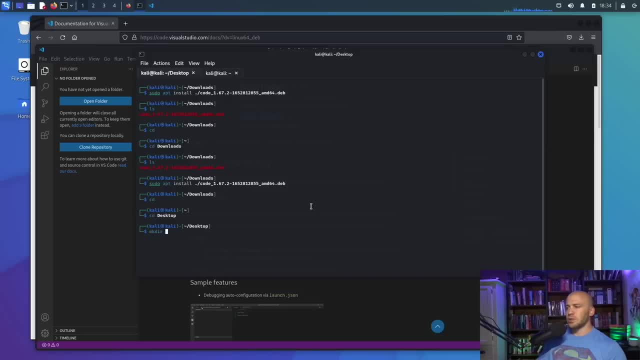 and now we can make a directory and we'll just call this bash and then actually we're going to name that something else. So we'll move bash and we'll call it bash scripts, and if we ls, we have bash scripts right here and we can cd into bash scripts and then we can touch and we'll call this file dot sh and we're going. 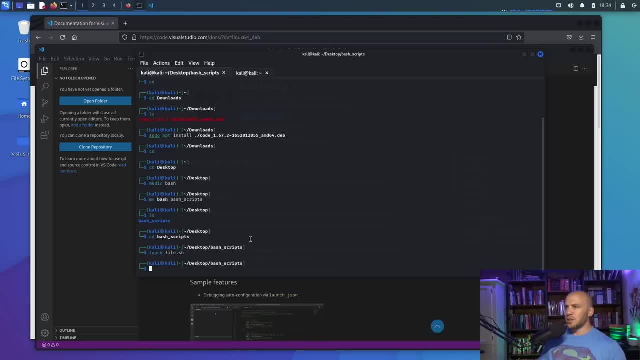 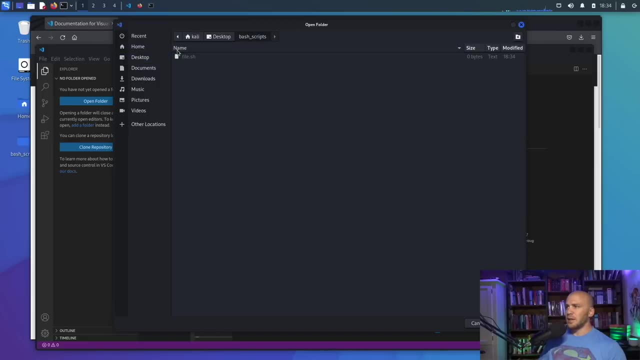 to name a bunch of different files as we go through and write programs. This is just to get us started. so now we'll open our folder. We'll go to desktops, We'll go to our desktop bash scripts and then we'll open up. We'll want to open up the whole folder. We're going to go to our desktop and then we'll. 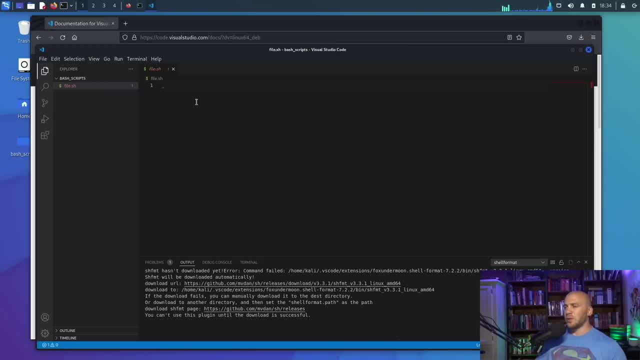 go to our folder and it will have our bash file in here. Now, in order to get this started, we'll just type in bash and hit enter, and it's going to give us our shebang up here, without going into too much detail here, What we're going to do instead of running the default that our plugin uses for us. 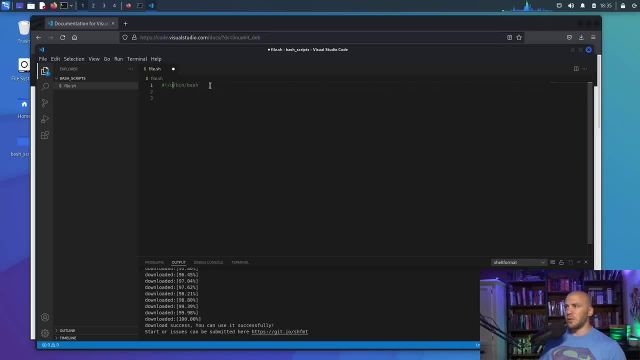 is: we're just going to run a bin bash and you're going to see this a lot and I don't want to confuse you with a bunch of environmental variables. So we're just going to run bin bash and if you want to, you can go read about why we would run bin bash instead of. 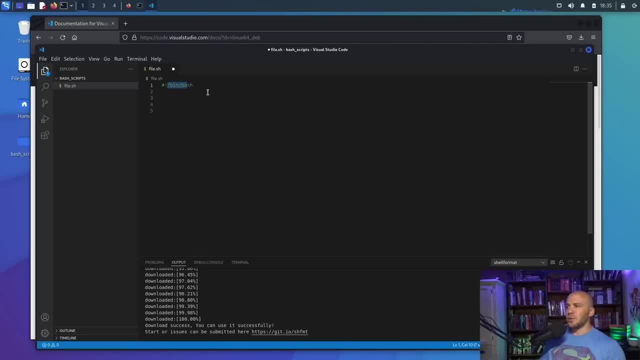 user bin nv, bash. and so this is how we're going to run this. and then, just to make sure everything is working, we can type in echo and then say hello world, and then we'll hit command save, and after we type in hello world, we'll come down to our terminal and this should be in our bash. 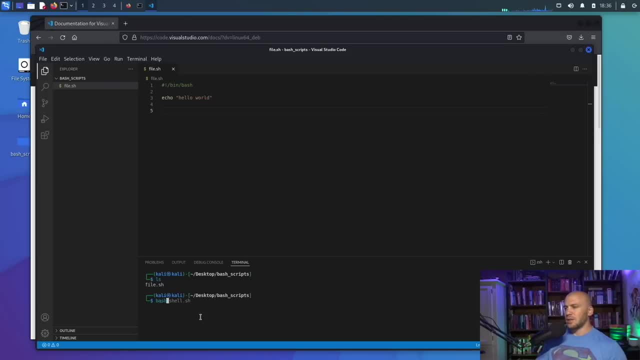 scripts. You can ls and it'll tell us we have our file right here. You can type in bash filesh and it prints hello world for us. so we know everything is working. We're going to go ahead and type in bash filesh and we'll see that it's up and going and ready All right, now that we know we have 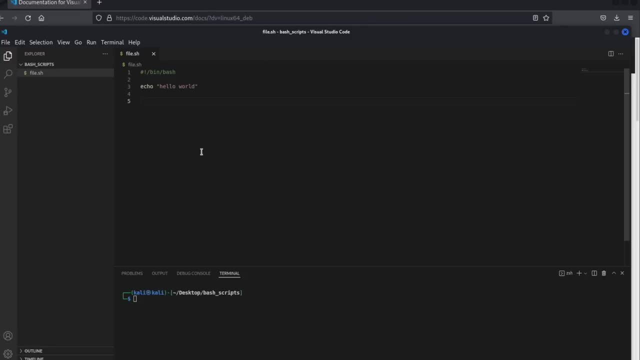 everything working. let's go ahead and cover a few things that we have typed in here. So when we see this right here, this is the hash and the exclamation point, which can also be considered as a hash and a bang- which is where the shebang comes from and this tells the Linux machine when 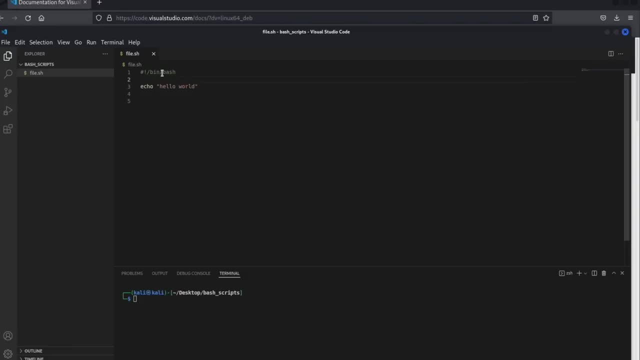 it runs this file, it's going to be running it as a bash command. So that's why, when we come in here and we type in bash and then we run this bash with this file, it's going to execute everything after this as a bash. And so then we have this echo which, if you're familiar with Python, it looks: 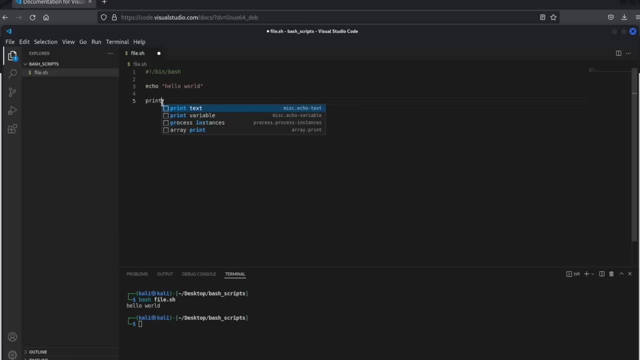 like we would run a print statement like this and then we would put our text in here and then we would say hello world. So the echo is the same as the print in Python, And so when we run this, that's why we have this hello world printed out. 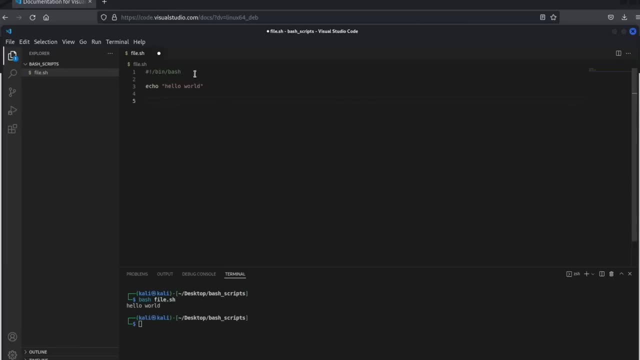 At the bottom. Now there's a couple of the things I want to cover just to help you as you go along and you make notes. Sometimes we'll write scripts and you might not remember. OK, what is the echo command? You can make what's called a comment on a Mac. You can press control and then the. 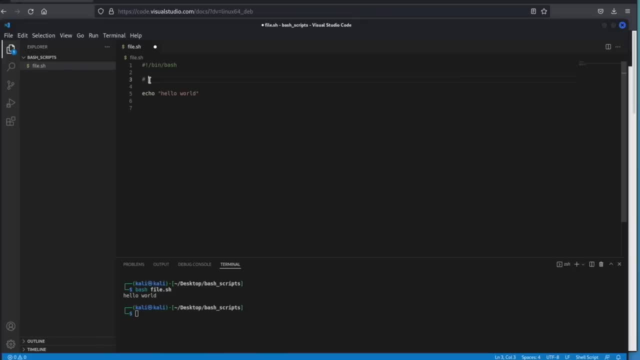 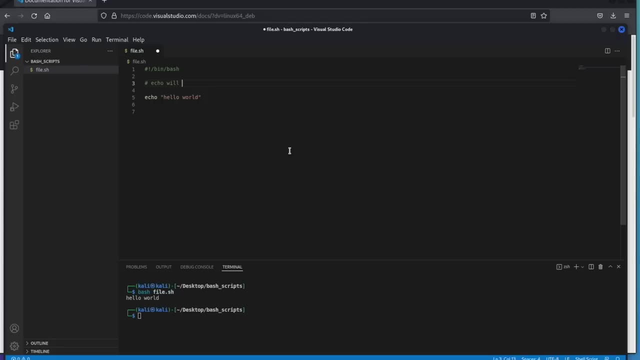 question mark or the slash, and then you can type anything in here And this is commented out so it won't show up in the file. So we can say echo will print the text. And then when we come down here and we save it and now if we run it it'll say hello world. And this does not get. 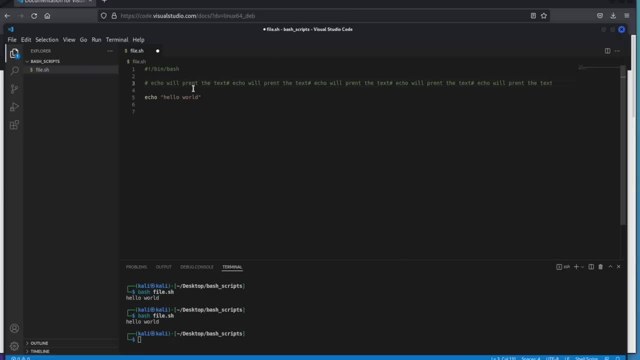 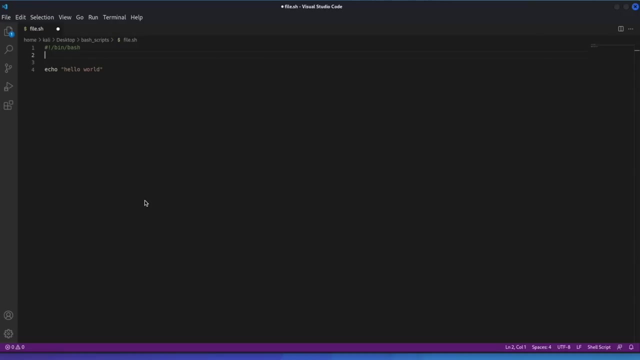 printed. no matter how many of these we have in here or on however many lines, it won't. It will not make a difference. So when we run this, this is all commented out. So now that we have a basic understanding of what's on the screen, we're going to move on. The first place to start is with variables. variables store data and it. 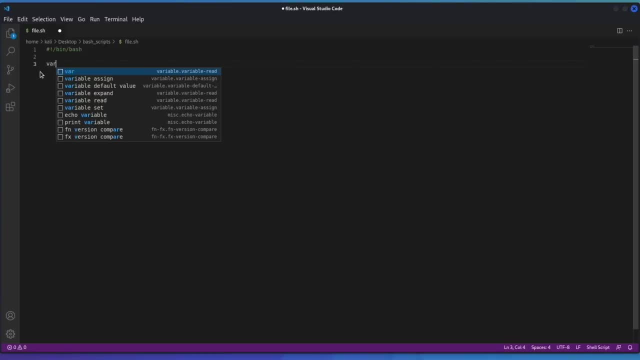 can look like this. So we're going to name it just VAR, because it is simple for us to understand that it is a variable, and then they will go inside of quotations because it's going to represent a string and you can put your name in there. So if I put in Ryan, you can think of the variable as holding my name Ryan. So if I decided to echo. 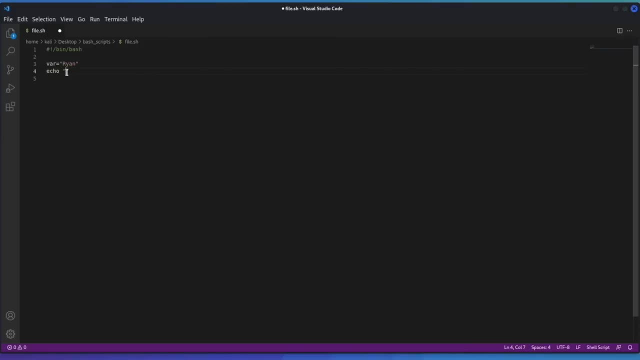 and I wanted to not echo an array, and I wanted to echo out the variable. we put the dollar sign, just like this, and then we type in VAR. And if I wanted to say hello, like this, and then VAR, and I need a new terminal which is right here, and we can come down here and we can just say bash, file, dot, sh, and it says: 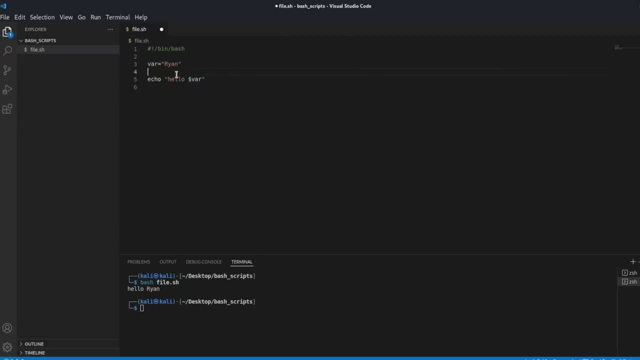 hello Ryan. So this seems really simple, but you will need to grab variables. They are super important and we will be using them all the time in the program. So right now, as you look at this, you think this seems very silly. Why wouldn't I just go like this? That seems like awful. 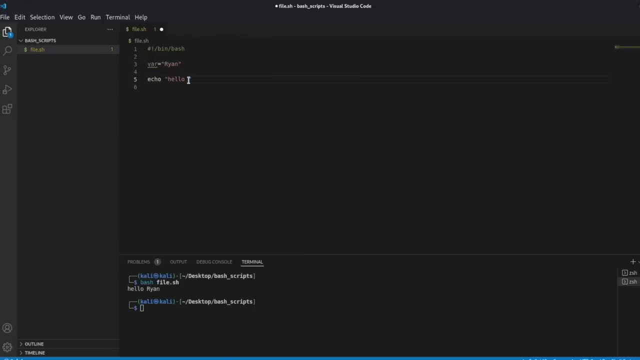 A lot of work. Why wouldn't I just type in, Ryan? And the reason for that is because you may need to take input At some point later on. we will do this, But for now we're just gonna type in here. We could just put in an IP address so we could. 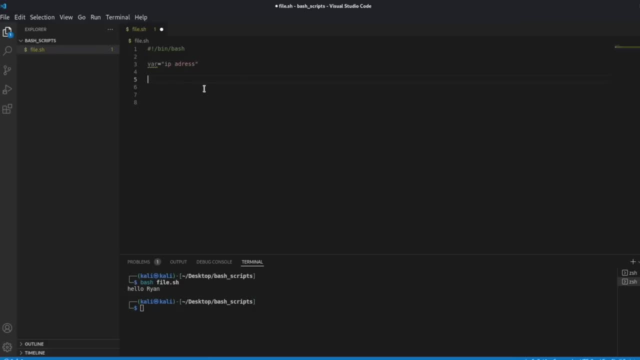 Say IP address Right here. I'm not going to put a real IP address in there Just for the sake of humor. I think so of this video and down here you can type in in map and then you can say dash, a dash, p, dash, and. 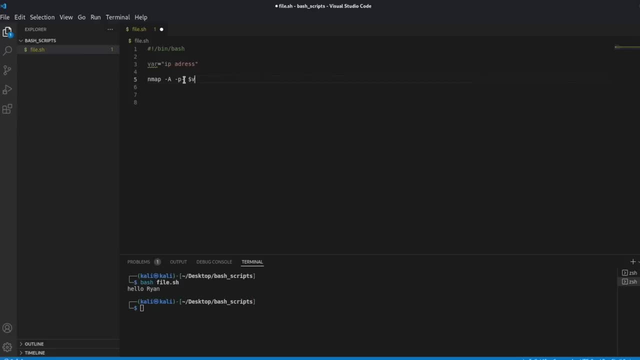 then now, where we would normally put the ip address, you can just type var, and then we'd put a dash v for for verbose, and now, if we save this and run it, we would get the variable would be the ip address. so if we had an ip address in here of 10, 10, 10, 10 and we ran this right, here it's going. 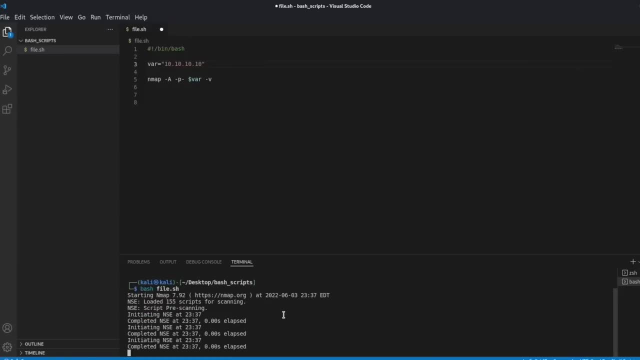 to start scanning this for us and you can see that scan started. so variables are really important because later we could make a complete recon tool. we could ask the user when they run the file what ip address would you like to scan, and we would put in this and then our variable, whatever the 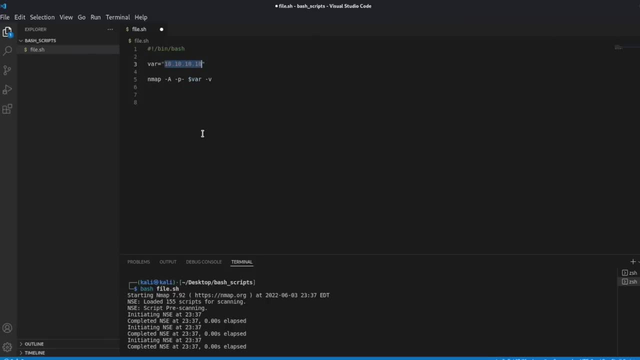 user puts in would be stored and our in map would run. so that's an example of how we would use a variable in the world of hacking. you will see this all the time in exploits. when you grab them off of exploit dp, they'll ask for inputs which will be stored in variables. 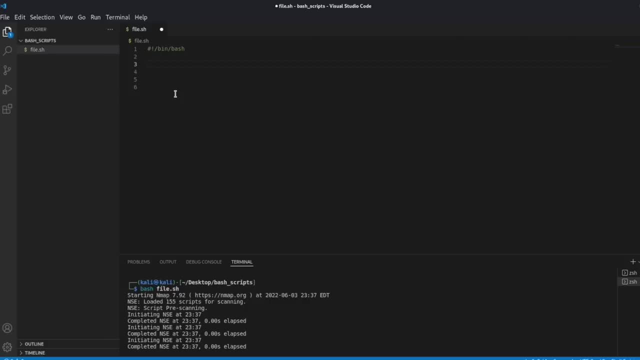 and maybe in the future you will need to modify them. so that is a variable, a very simple version of a variable. okay, so one of the reasons i struggle with bash so much is because the way they name their functions. for example, in python, if we made a name and let's say we had an input and 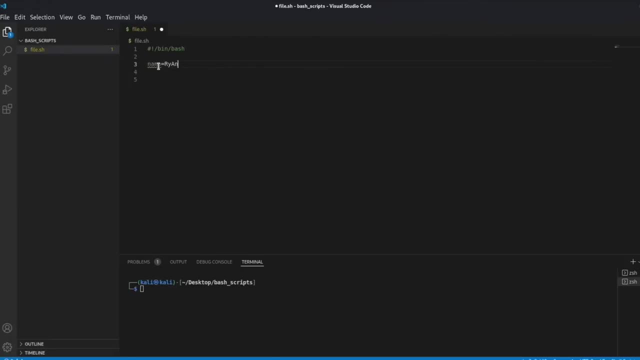 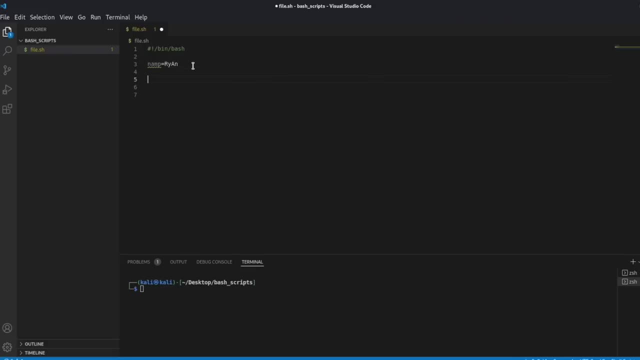 of our function, call or dot lower. but in bash we do it a little different. i notice this is supposed to say name. if we echo this and we say echo dollar, sign parentheses and we say name, and then we don't forget to save it and we run this, we get my name out. 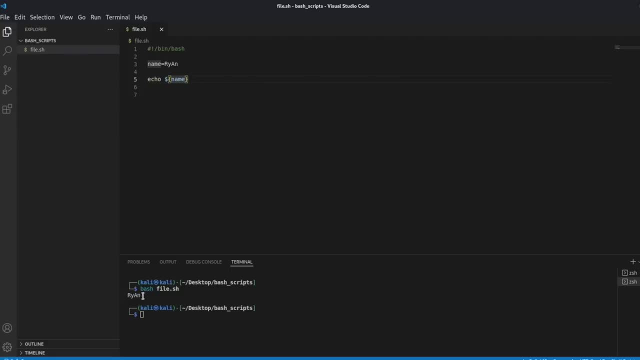 output here. but if we wanted to get just the first little letter capitalized, we would put in a carrot and then we had to save it. and now when we run it- my bad, we need a double carrot. i forgot to save it. now when we run it, we get all caps just like this. and then, if we wanted all lowercase, 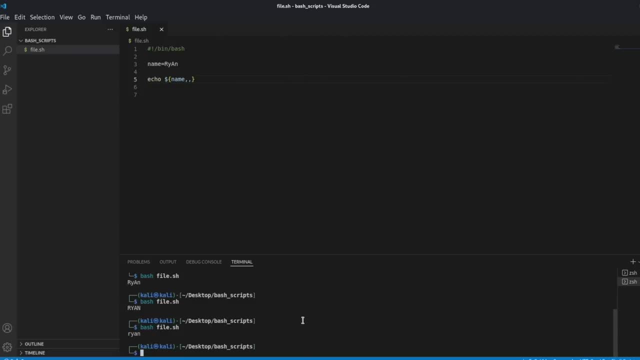 we just put in two pure two commas and we can save it and run it, and now we get all lower. so in the world of bash, when you need to do something, if we don't cover it in this class, you may have to google just to see exactly how to run this. but this is really helpful because a lot of bash. 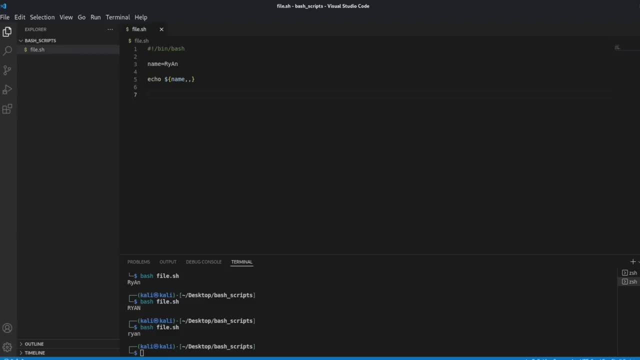 commands and a lot of bash scripting is going to require all lowercase or all uppercase. so, for example, a lot of times when you run against an active directory name, let's say you have the active directory name- a lot of times they will be in all caps and you can use. 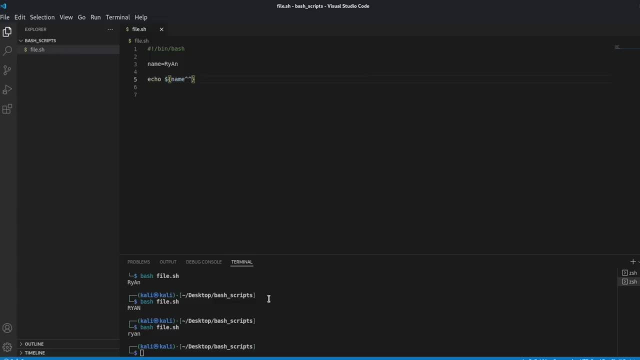 the double up carrot, just like this, if you're running a script against it and you don't want to type it, and you get all caps. so that's an example of when you would want to use something like this in the world of hacking, and there's a couple other things that might be useful for you. 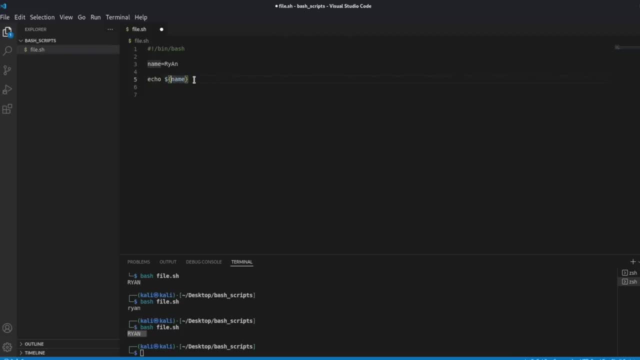 that you can do. if we wanted to, we could come in here and we can put in the an exclamation or sorry, we can. if you wanted to come in here and put in a hashtag, we can save this and run it and we get the length of the output and with this word count we can. 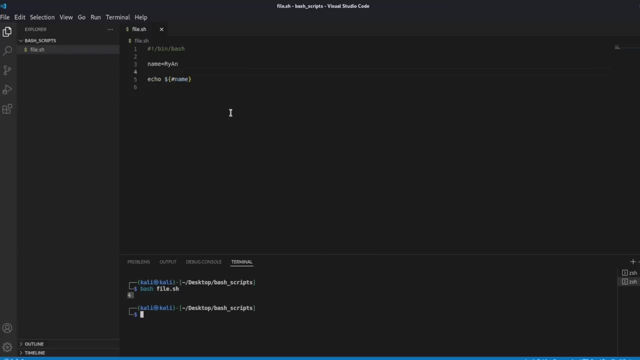 use this later. let's say, if we have a list and we want to know how many items are in a list, we can use something like this to check what is going on within the inside. and lastly, there is something we're going to need to know in order to grab numbers- or, in our case, we may want to grab. 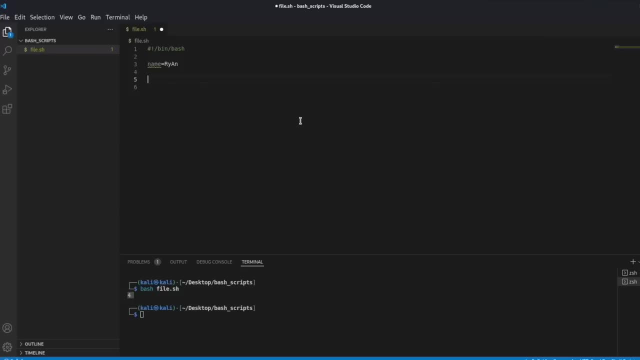 something out of a, out of a string, and we want, like every third word is help, would be beneficial to us to grab if we have something instead of name, let's give this as num equals one, two. actually, we'll start at zero because bash, all programming languages start at zero. 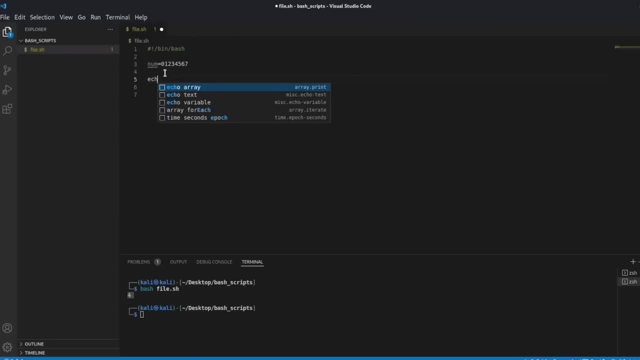 when they start counting. so if we come down here and we echo, we say dollar, sign our parentheses and then we say num, we should get our number, our string of numbers, put out down here. but if we wanted to grab numbers out of here, we would do something like this. it will be. 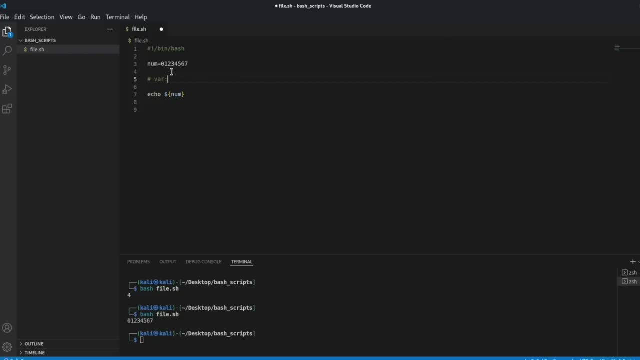 the variable right here. so we'll have the var, the variable, and then the offset, meaning what, how many over would we like to start? and then we have the length, meaning at what number would we like to stop. so in here we can say colon, and if we wanted to grab numbers one and two, you would say zero, one, two. so a lot of times. 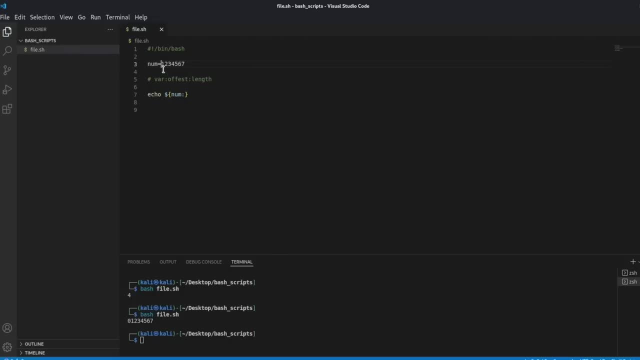 you won't start at zero. so, for example, we would say: zero one, two. so if we wanted to grab the two and the three, we would say something like this: zero one and then two, and then if we save this and we run our file, we get number two and three. but for the sake of this not being super confusing, 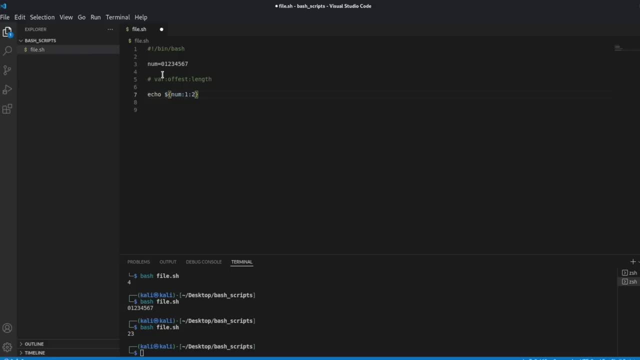 we'll start with zero, one, two, three. but what you just have to remember, but you just have to remember, in the world of programming, computers start at zero and this is our number one. so one, two, three, just like this. or in this case it'd be zero, one, two, three. and if we got rid of this, 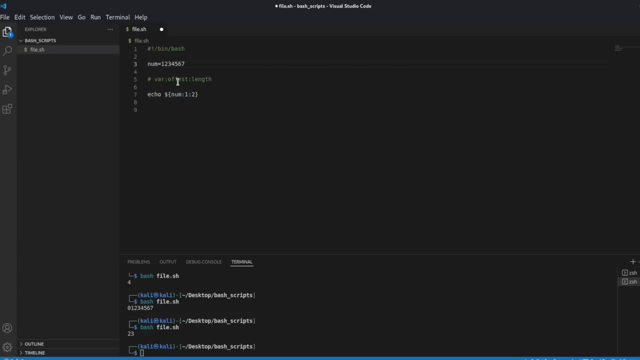 we would have to say zero, one, two, three and so on. so i hope that makes sense and you are able to grab numbers out of this string and maybe you can go ahead and try and practice with grabbing numbers. you can also do something like this. you have to have a. 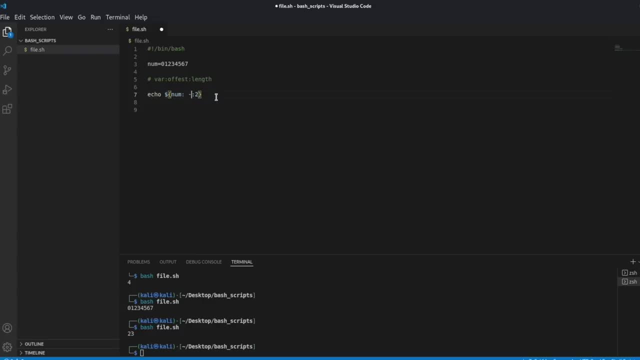 space in order to run a negative offset. but let's say we wanted to go backward four and then we want to grab the next two afterward. we can save this and you can run something similar to this and you get a totally separate set of separate numbers, and i do use this every now and then. 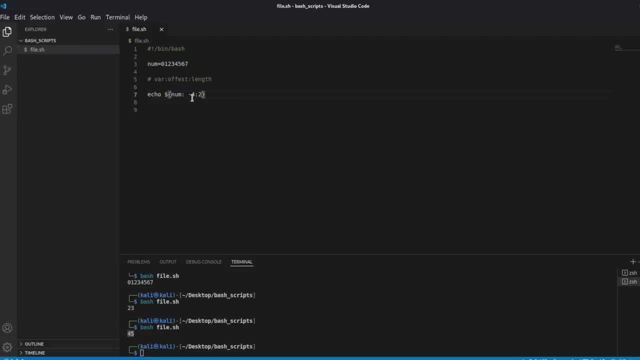 it's not super common and you might see it in the future, so it is something worth noting and keeping it in your back pocket. okay, i want to show you that we can save commands inside of variables and then we're able to run them inside of our scripts. this will be helpful in the future. 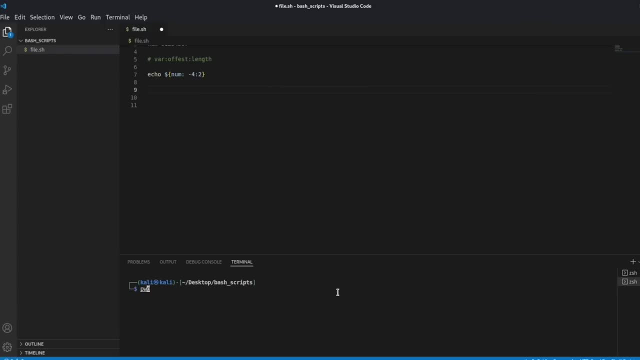 so you're probably familiar if we come down to our terminal and we type in pwd of seeing our present working directory. but we can save commands inside of scripts and then use them. so for example, we can say directory equals. actually we can say current, say curders for our current directory equals, and then we say dollar sign and then we put 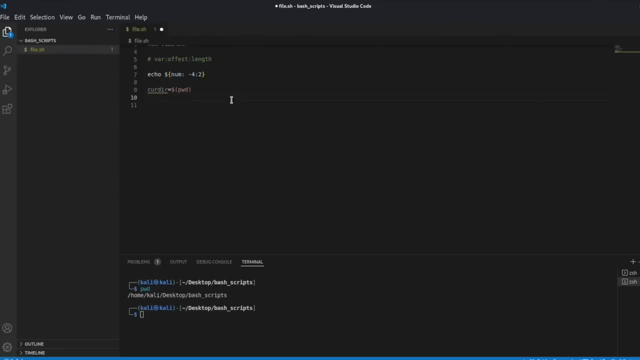 our parentheses and we say a pwd. now, if we come down here and we echo a variable and we say current directory, just like this, and we save this out, and then we run our script, we get our present working directory down here. so another example of this is if we say time. 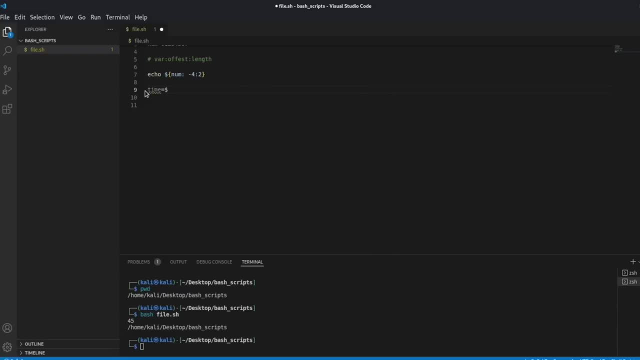 and we said equals and then we put in date. inside of here we could say echo and then we want to echo a variable, but before that we could say the current time is and this is going to give us our time and date. if we save this and we now run our script, it tells us that we messed this up because we didn't write. 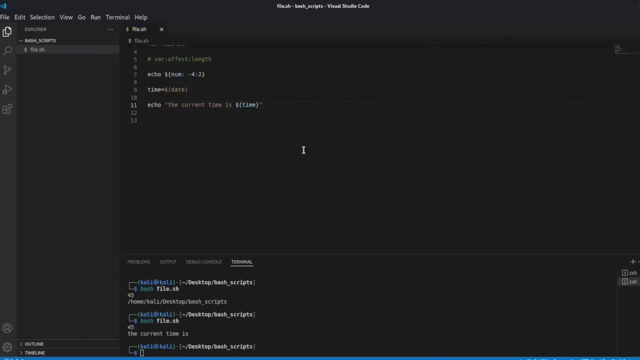 in the time rate here and we save that. now we run it, it tells us the current time is saturday, june 4th at this time. so that's how we can save commands inside of variables, and this is going to be helpful in the future whenever we have to write specific scripts and use them with commands that are. 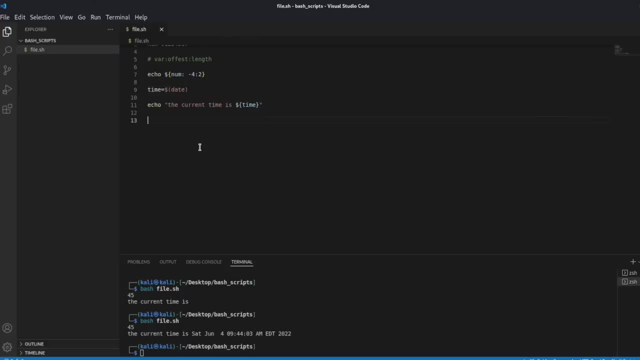 already within our linux machine. so from here we're going to move more into working with numbers, and the numbers will matter when dealing with things like ip addresses, or sometimes you may want to print a word list that you want to use, as with a fuzzer that has numbers on the end of it. 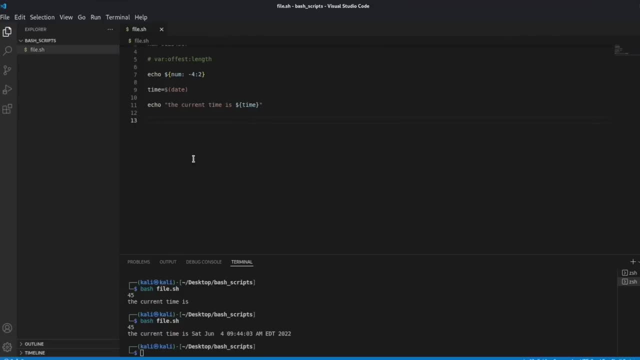 and we're going to be covering this in the coming up section. okay, we're going to be covering some numbers and adding them together and using a sequence of numbers in order to grab a range of ip addresses or possibly even make a password list with numbers. but with bash this is a little different than other programming languages. 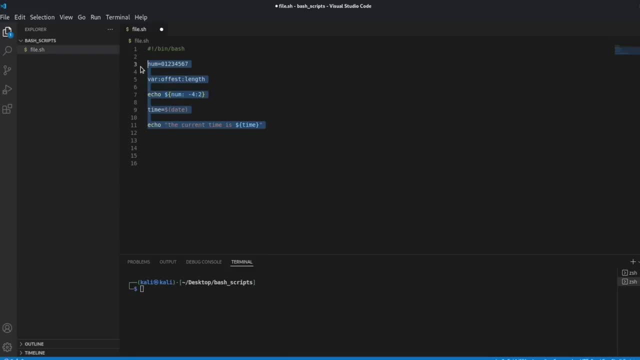 so you can either take this whole block right here that we've already written and comment it out, or you can just delete it like i'm going to. if you want to, you can save it and keep it as notes for later. so within bash, if we say something like other programming languages, x equals. 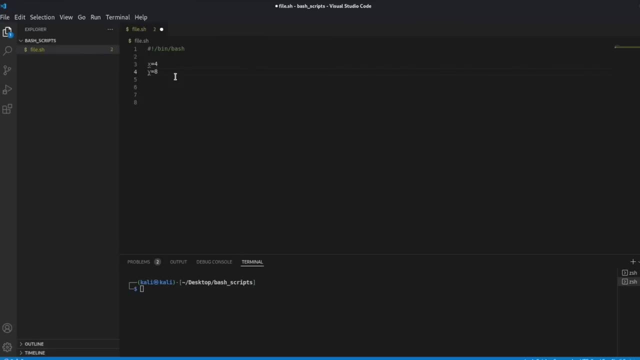 four, and then we say y equals eight, and then we echo: and the thing about bash: when we want to add these together, it's going to require a little different syntax than you might think. so we use dollar sign, then we have double quotes and then we would say dollar sign x plus dollar sign y. and now, if we save this and we run it, 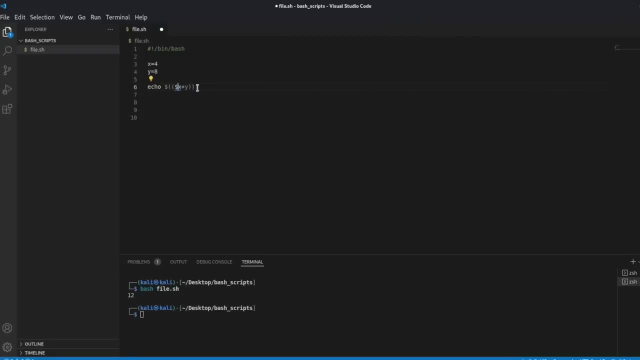 we get 12 down here and i believe within bash you don't even actually have to have the dollar sign. so we'll give this a try right here and it still gives us 12 and this works with. also, we have minus and you can run divide and other commands like this. so if we run division, 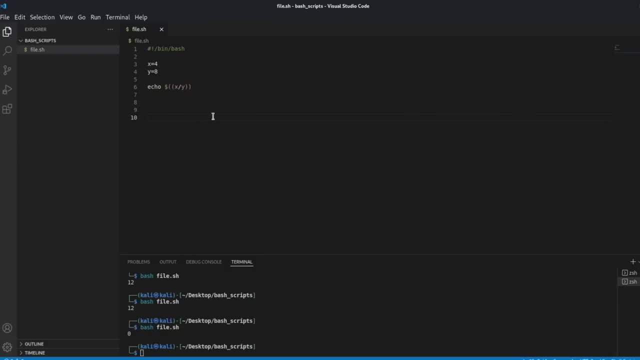 we have zero, which is right, because eight doesn't go into four and bash won't give us any decimals and it won't give us any negative numbers, which is really interesting. so if we say y minus x and we save this, we now get four. if you want to run something such as a calculator within. 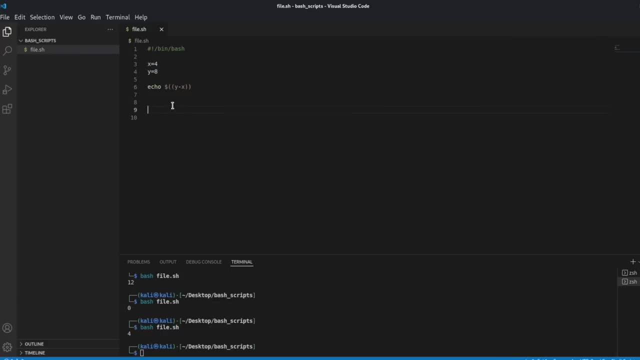 bash you have to use bc, but i'm not going to cover that for the sake of this course. i would rather tell you: just use a calculator, because it's going to be a lot easier than using the command line to run some kind of math. so this is how we would use variables and numbers within bash, but when it 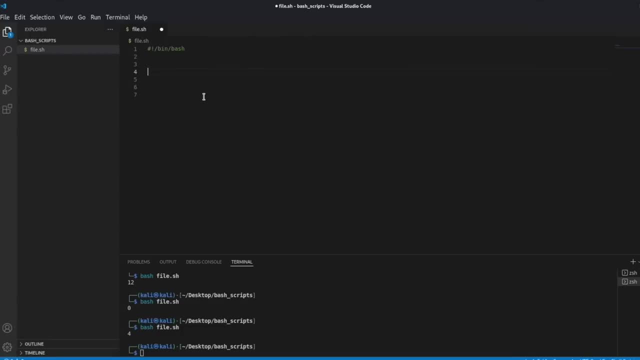 becomes useful for us is when we want to create a list of, say, numbers. so if we say echo month, and then we put curly braces and then we say 1.12, when we run this command it should print month one, month two, month three, and so we'll save it and i'll show you what this looks like. so we have. 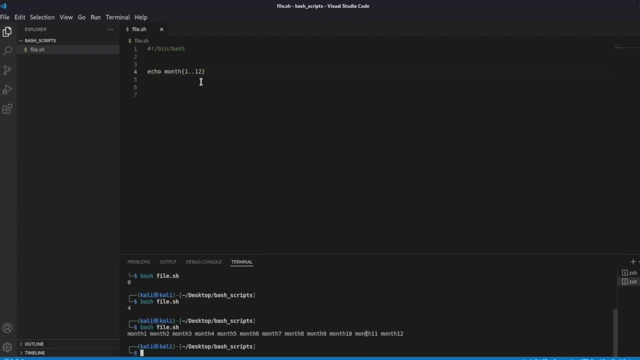 the output like this, and this may seem like it's not very useful in the world of hacking. let's say, we have an ip address and we want to create a list to scan against in the future, and maybe we're creating some kind of tool that is going to take an input of an ip and the range. 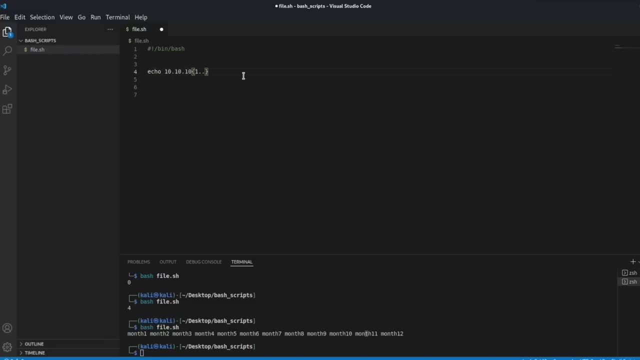 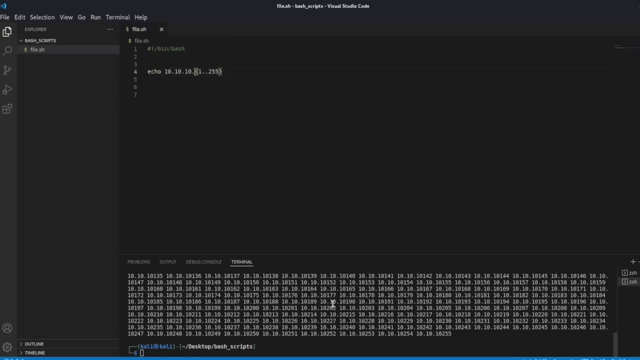 we could say we have a subnet of a 124, so we'd say 1, 255 through one, one through 255. then we save this and then we run it. we now have all of these ip addresses. i forgot to put a point right here. save it and we'll try this again. and now we have all of these ip addresses and we have this list. 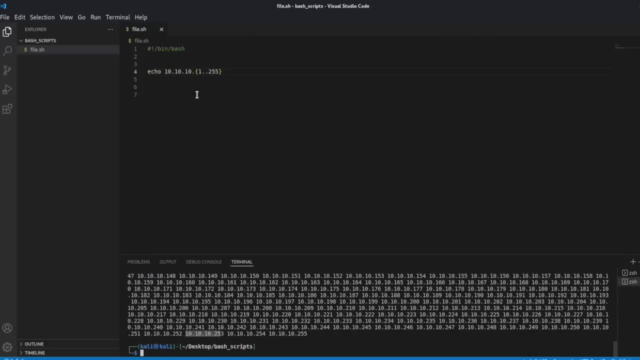 that has a complete range of ip addresses for our range. so this is a helpful way to know that we can append numbers to something preceding it. so this will be helpful in the future. i don't use it a whole lot, but it is helpful to know that it is available for us if we ever run into any kind of 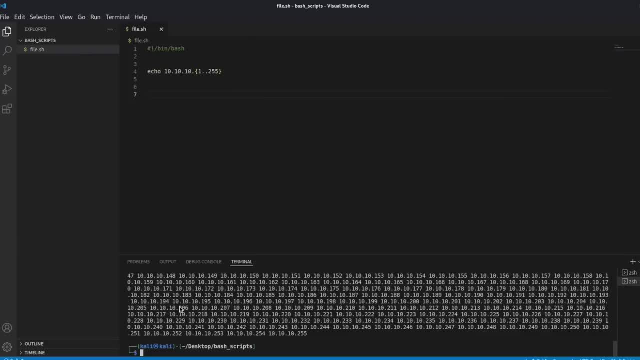 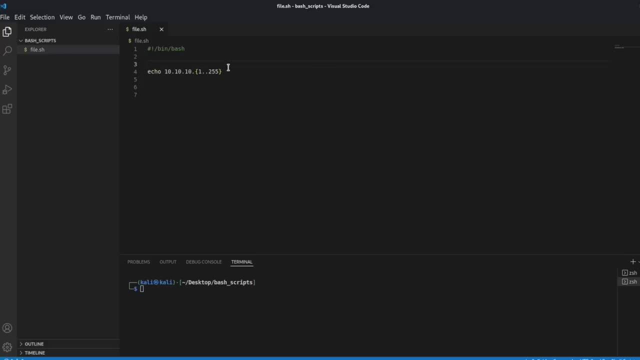 problem. okay, i want to cover something called specialization and i'm going to talk about that- parameters, because it is something you're going to run into in the world of cyber security. so we'll clear this and we can comment this out, and the reason you're going to run into this is when 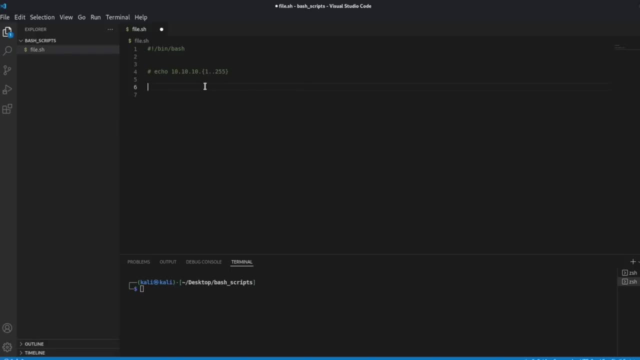 you run something, a tool or some kind of exploit that requires input from the user, say us whenever we want to run this. it'll ask for a ip address that we want to attack and a port to connect back on. you may see it say that you didn't enter everything required. 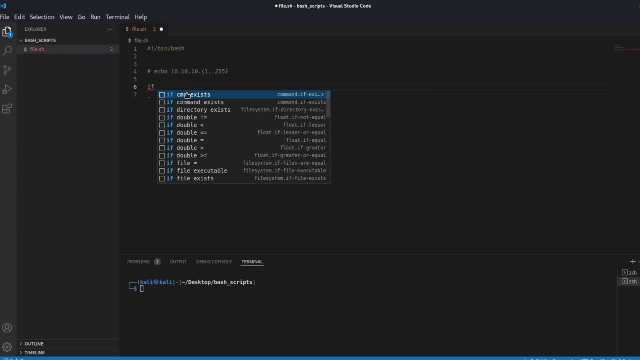 and an example of this is if we say if and then we go square bracket, square bracket, and then this right here is a special parameter. so this is going to tell us that we need, right here, two inputs from the user when they run the file. so we have this if and. 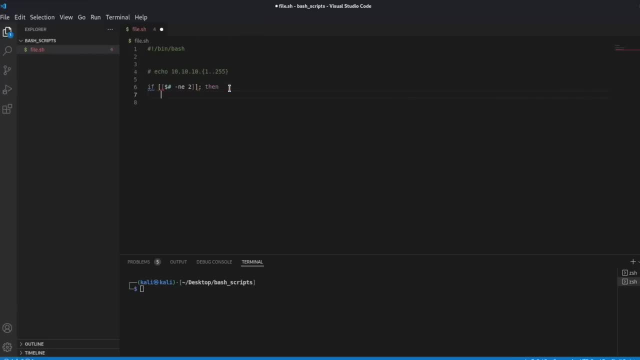 then it's going to be a then, and then this will be tabbed over and we'll: echo: need more parameters. and it'll tell us: echo: usage requires usage needs too, and then we can give it an exit of one which means we have an error, and then in then. 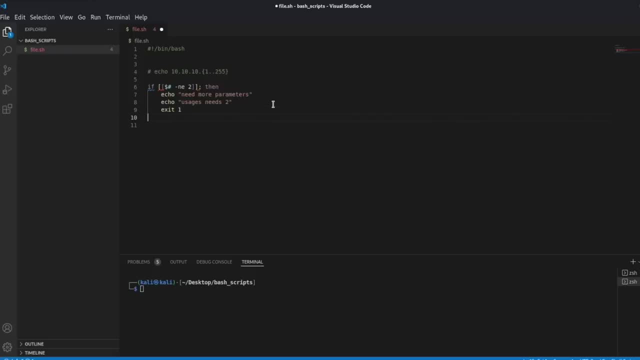 for bash instead of an if else or an if or an elif. like Python, it uses a in fi and we can run it like this, so we should be able to now save this. okay, we should now be able to save this after putting in those spaces, and it should run for us. so if we run this, it'll. 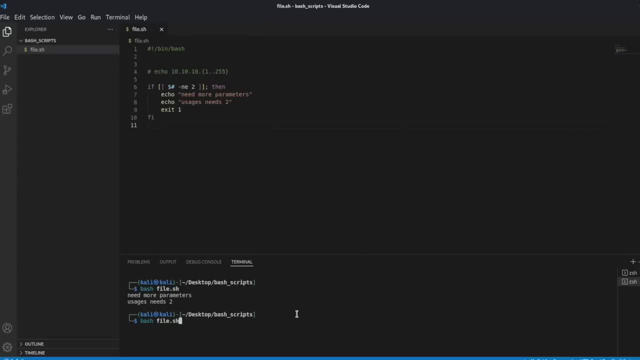 tell us, you need more parameters. but if we run it and we say: um, let's just use one space two, these are going to be two inputs from us and we run it, it doesn't give us any issues. in fact, we could do a, we could have a print. uh, script worked, but in this case we'll just leave it so that way. 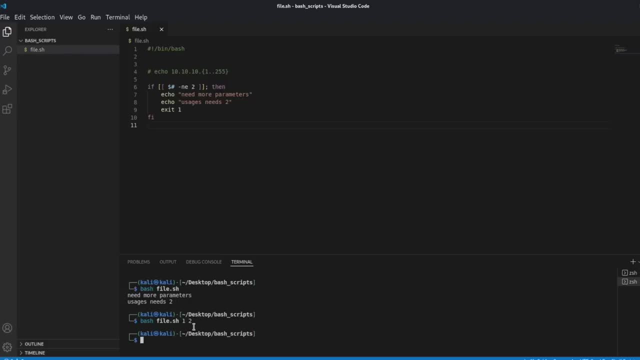 you can see, we didn't get any exit code. it needs two inputs from the user in order to execute, so with that, this looks really, really scary. but really, what i wanted you to see was: this is the special parameter that tells the file that we need, the. the bash will tell us that we need. 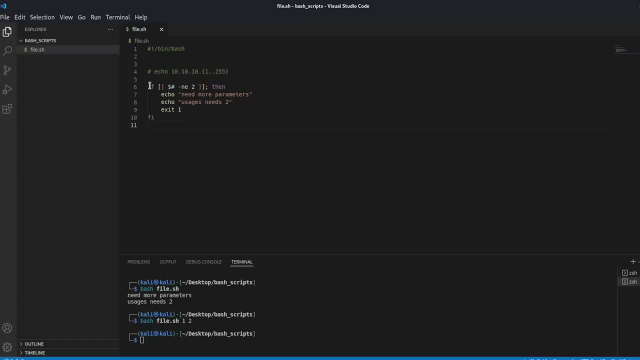 two inputs from the user in order to make this script actually run. so these are special parameters and they are going to be one of those things that, if you want to memorize them, i would suggest- which i rarely ever suggest, things like this is flashcards and memorize, usually when 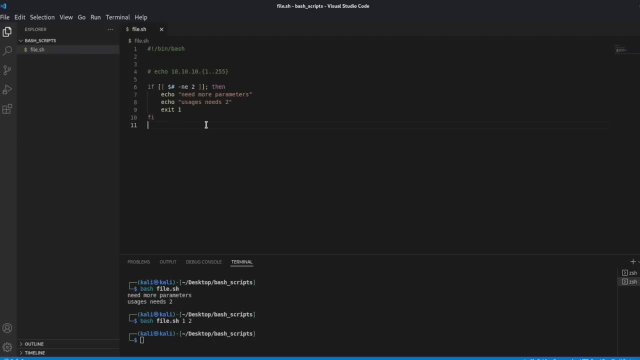 you're in the world of programming as well as cyber security. you would just say: i know there's a way to use a dollar sign in order to get two inputs from a user, and i just need to know it, and later, when i run into this, i can just come back and google how to do this and read how to. 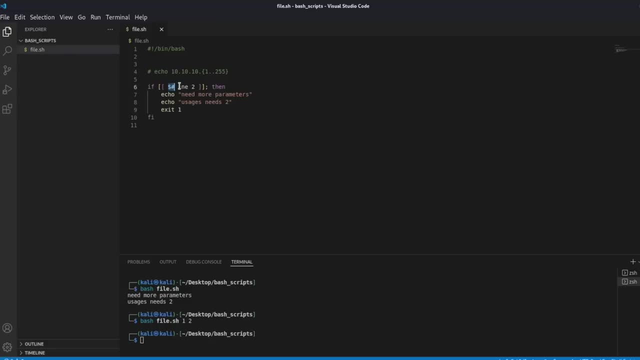 do it. it saves you a lot of time and it's really easy to do so. so if you want to do that, you can just come back to the browser and go to the browser and click on your computer and just go to the browser and just run anything that we can do. it's really easy and it saves a lot of. 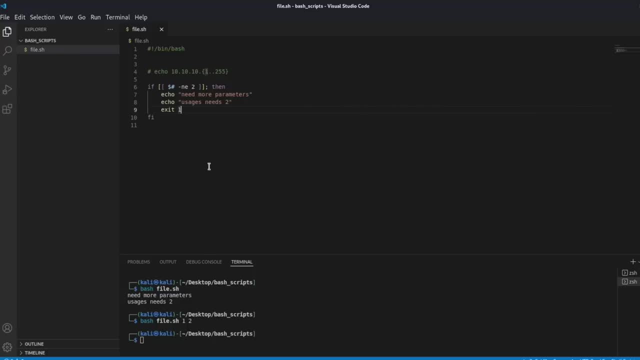 headache and a lot of time memorizing, because you're probably not going to use this very often- you're, and we'll forget it, but it's. it's important to know that this exists because maybe in the future you will run into an exploit that has something like this, but the exploit is old and 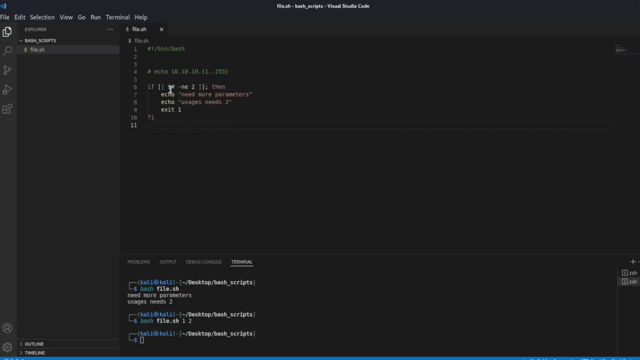 maybe it has been deprecated within the version that we're running our exploit against and we need to get rid of one of the parameters. you now know that you can come in and say, instead of two, it has been deprecated and it no longer needs four inputs, It only needs three. You can come. 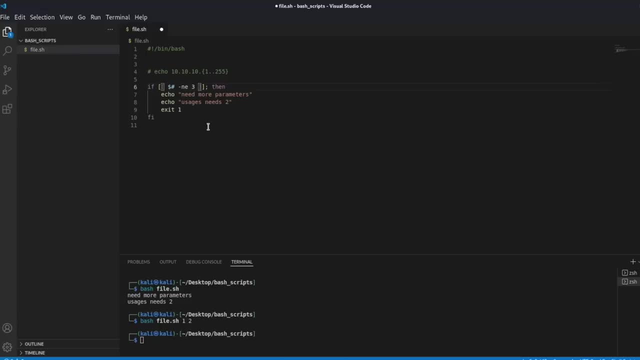 back and just put in three, and now you can run the exploit as you need. So this is the reason I would suggest trying to remember that this dollar sign hash has this specific special parameter function, because it is something you may run into in the future and need to know how. 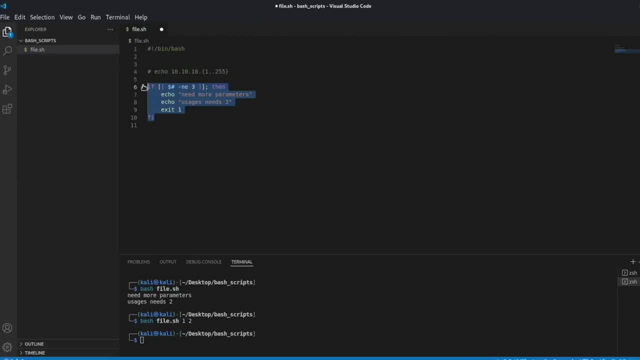 to modify. We're going to ignore the if statement for now and we're going to look at a different way to take input from the user, and that is with the read command. So you can just say something like this: read. and then we can say: maybe we want an IP address and we want a port number. We'll just 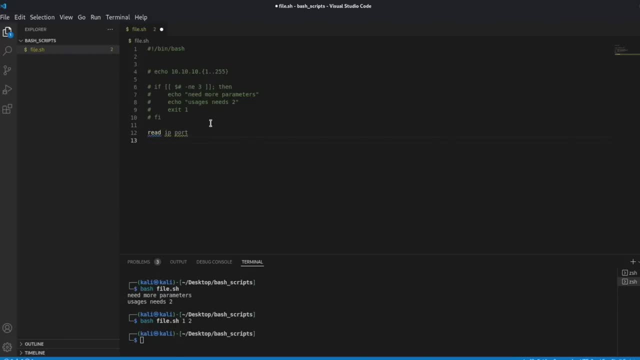 leave it at that for now, So we can go enter and then we could say something like echo, It is going to be with a variable, The variable is IP. Then we can come back here to the front say something like the IP. 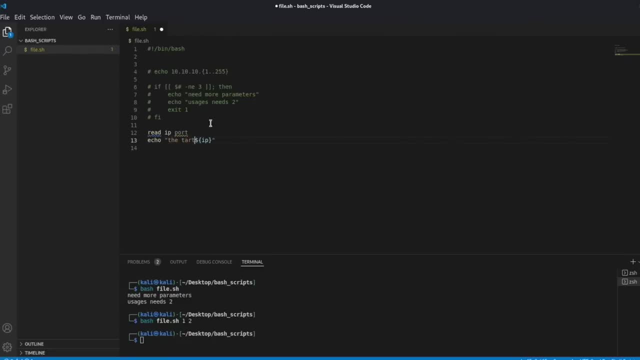 We'll say that the target target IP is, and then we'll have that IP and then we'll say echo with another. that was with the text. That's okay, We can just add our variable in later. We can say the connection port is, and then we'll go. dollar sign: curly braces. I accidentally did two curly. 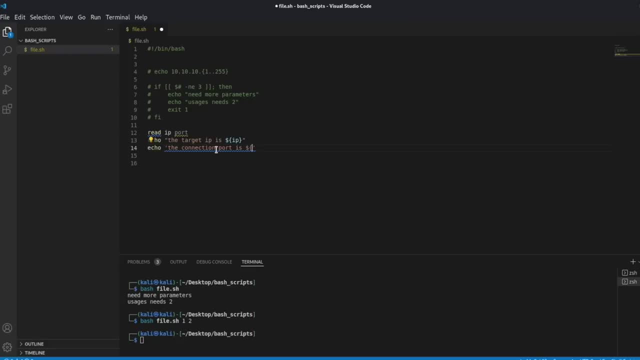 braces, We will say the port And then close off our curly brace there. Now, one thing that you're going to notice is why is our variable not lit up? And the reason is because single quotes get rid of every special character inside of a string, and double quotes will leave all variables alone. So that is something to note. 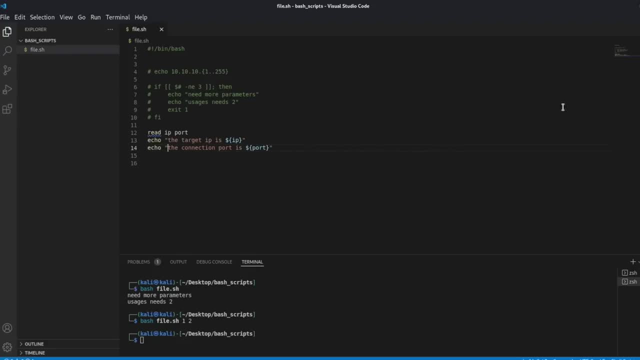 for the future. So now, if we save this and we come down here and run our file, it's going to leave a prompt and we could say the IP address is 10, 10, 10, 10.. And then the space puts us on to the second variable and we'd connect back on port. 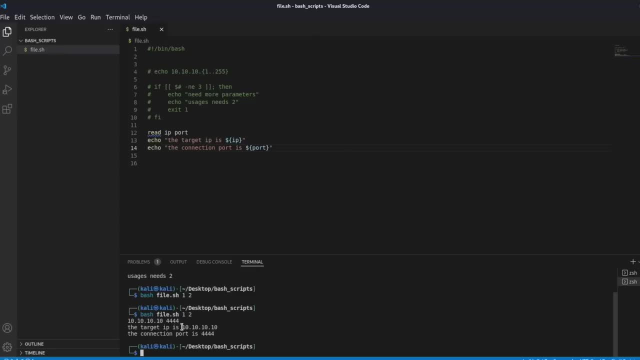 444.. And then we hit enter and it tells us the target IP is this and then the connection port is this. Now, there is a better way to do this, And what we could do is something like this: We'll delete the port. 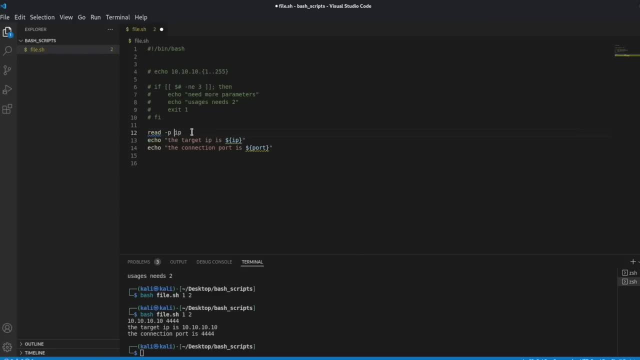 And we can put a dash P and this is going to give a prompt To the user and Will say: input the target IP colon space. We'll add space in here and now. we could say re- louise, and then we can do the same thing and say input. 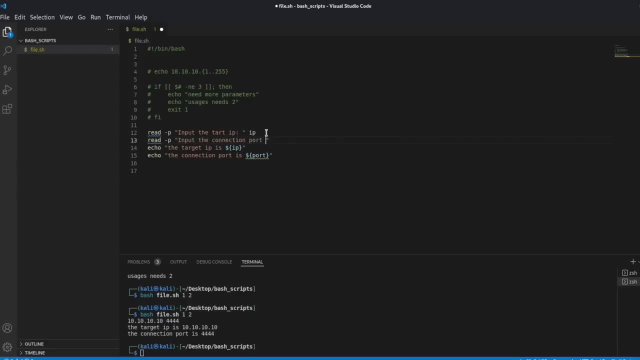 The Connection port Colon Space and then we can come in here and put in port. Now, if we save this and we run it again, we have a prompt down here and then we hit enter and then it asks us for a connection port and we put in our connection. 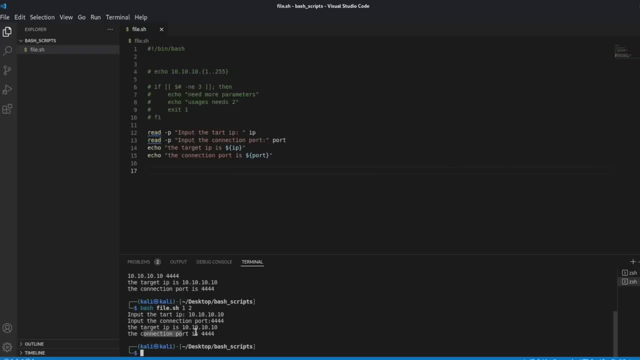 port and then it prints out for us the target IP port or the target IP and the target port. So this is how you take input. I like this a lot better because it is user friendly and it's really simple for us to read what is going on and this way we cannot skip, say, an input, and if we put in an empty. 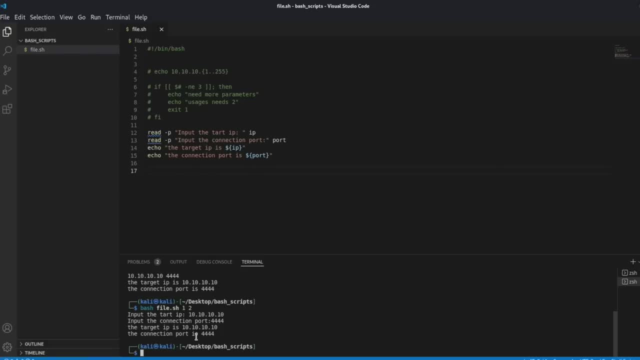 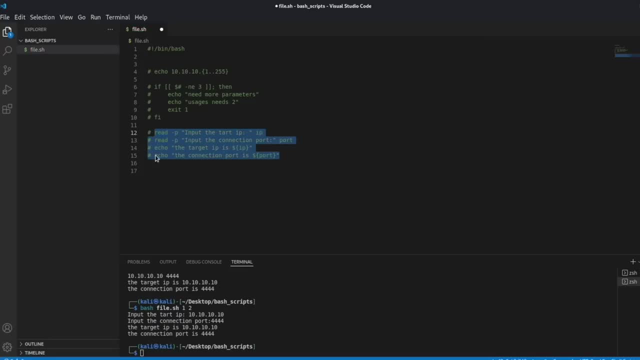 statements and this code right here. I hit the wrong button. We'll comment out this code right here and we will see things like this: You'll see a dash eq, which is going to be an equal to, or maybe we will see something like a dash ne, which is not equal to. You can see something. 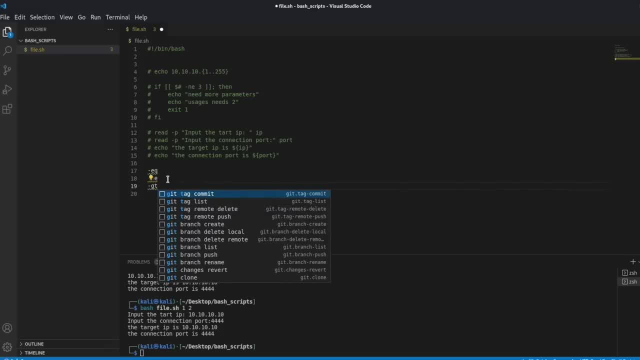 like a dash gt, which is going to be a greater than. I'm going to go ahead and comment this out, so it stops suggesting things. So we'll see a dash eq, a dash ne, the dash gt which is greater than, and then a dash lt, which is 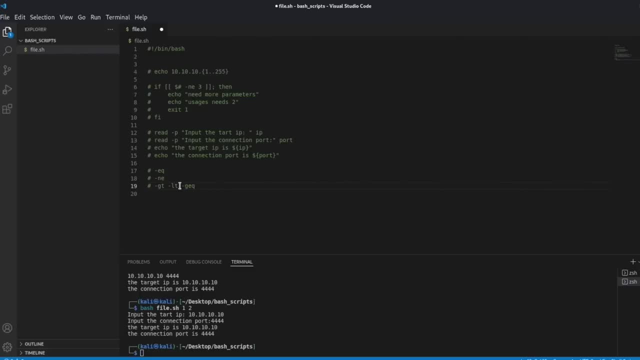 less than, or a dash geq which is greater than or equal to, which is the one we probably will be using the most, and then a dash leq, which is less than or equal to. These will be really helpful when running our for loops, and so it is helpful to know. So let's give a look at these in action. 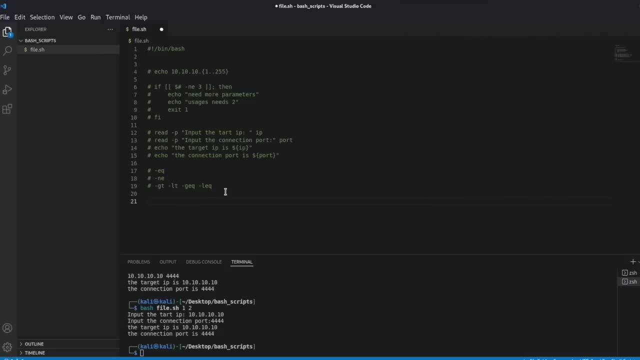 So the way we would write this is, if we wanted to give a statement, we'd put our brackets, and there has to be a space in between the bracket and the first number. So we would say: if 2- and then we'd say dash eq is equal to 2, then we're going to have it do something and we would tell it to echo. 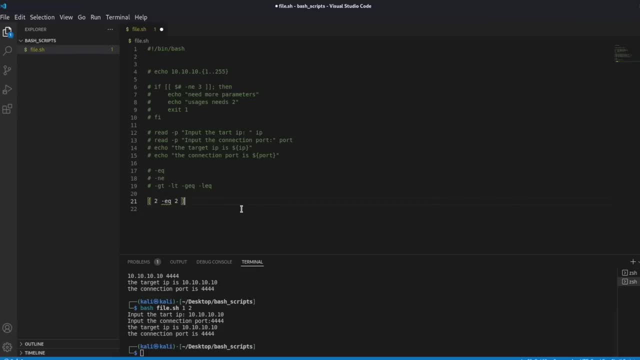 that the statement is true. And the way we would do this is by adding the colon and then say echo and then dollar sign And then question mark. and the reason we're using the dollar sign, question mark is because it's going to return a boolean. So a boolean is something that is going to be true or false, So it's going. 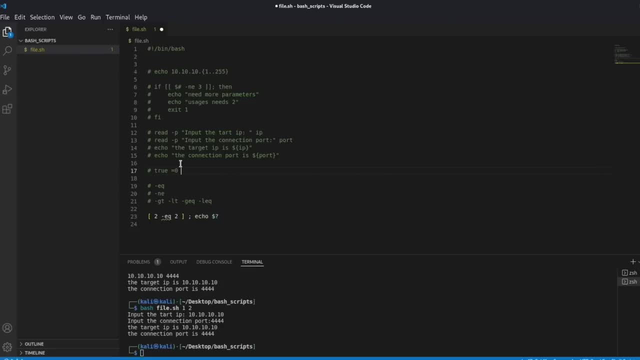 to return a true which is going to be equal to zero, And if you're from another programming language then you will know this is not normal for most other programming languages. but bash true is zero and false is going to be equal to one, So this is going to return a boolean. 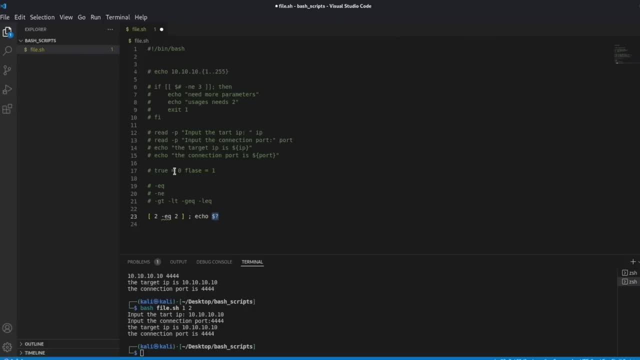 This is going to return true or false in the form of a one or a zero. So when we run this, we'll save it. and now, when we run this, we should return back a true statement. Two is equal to two, but if we change this to three and we save it and we run it, we get a false. This is not true, So this equals. 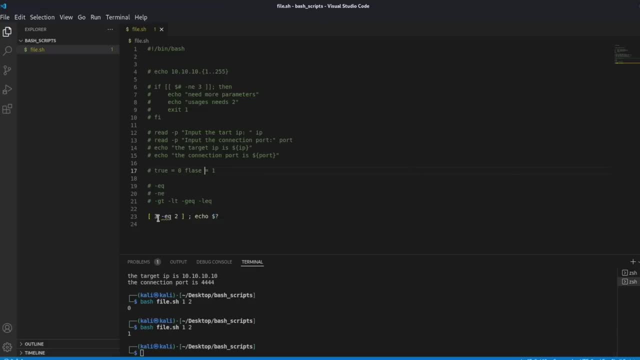 right here- only works with integers, which is which is numbers. It is really important To remember that it only works with numbers. So we can do something like this and we can say: not equal to So is three not equal to two. Delete this and it returns true. We have this true given to us. 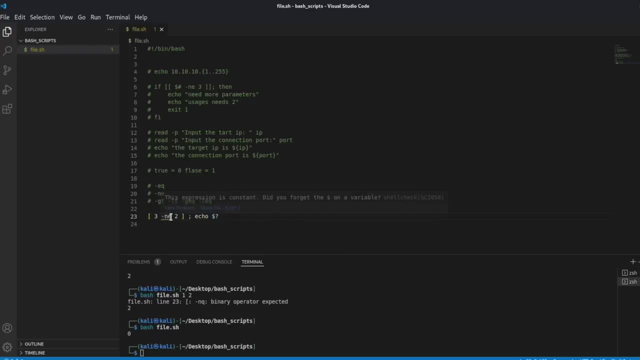 right here. When we run something like is three greater than two and we'll save this, we can run it and we get a true than two and we will get a false. This is really helpful when we run our for loops in the future. 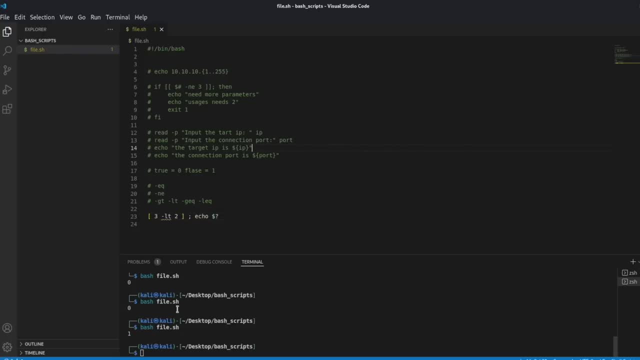 You're going to, you will run into this, You're going to see it and it's something to be aware of. OK, We can also look at conditional operations for strings. An example of this would be: will- uncomment. this would be something like this. So we'll use an equals and we'll say the word word. 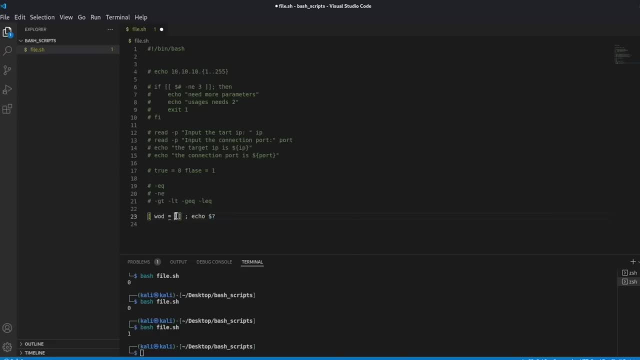 word is equal to word And now if we save it and we run this, we get it is false, because I spelled it wrong: Save and we run it and we get a true. So this, this equals, is used for strings And if we want to, 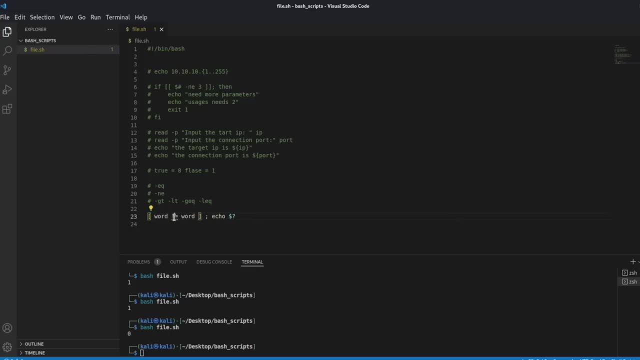 say a not equals, you put a bang in front of it or an exclamation point And then if we save and run this, we will get a false because it says they're not equal, But they really are equal. So if we take off at the end of this word, save it and we run, they are not equal is. 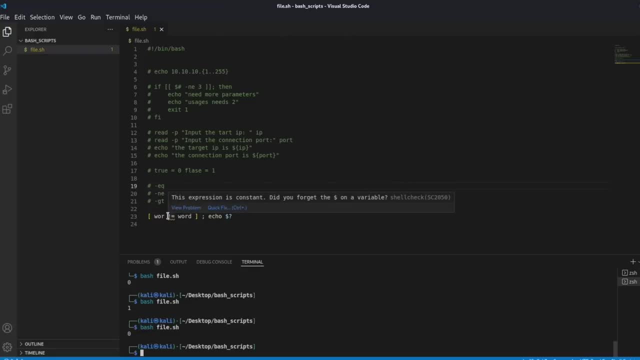 true. So this is helpful, especially if you're running a script, that you are looking for a specific keyword within a text that has been fed in through an input. you can check to see if they are equal and then have it do something afterward. So now we're going to move on into if statements and we're going to see how this plays. 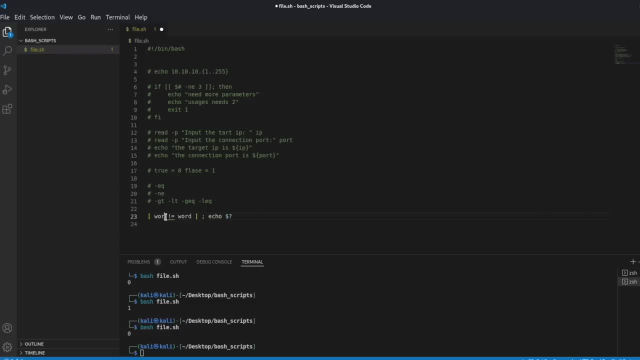 into writing our if statements Statement off of what we already have here. We'll just make this a word and we'll make this equal to and then the way if statements work is: you start an if statement with if and you can also use and else. But when you're done with the if, 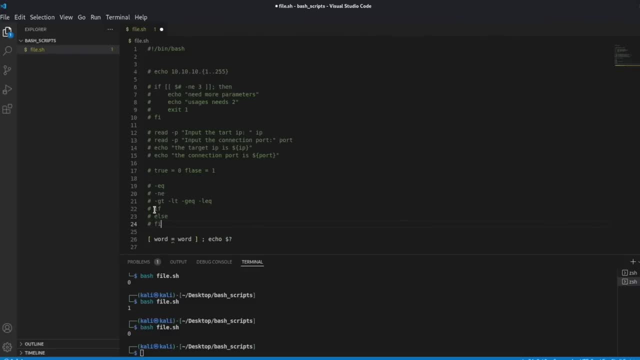 statement you write in fee, just like this. So we can do: if this is true, then do this portion of code. else, if it's not true, Do this portion of code And then when the script hits fee, it will exit. So if we come in here and we just say if word equals word, we're going to tell it, then we want it to do. 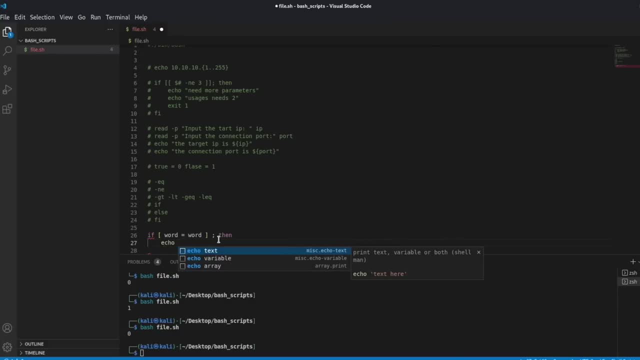 something. so we can come down here and say: echo, and we're going to use echo a text and we'll tell it to echo words match. and then we can come down here and tell it else. we can do an else and we can tell it to echo a text. 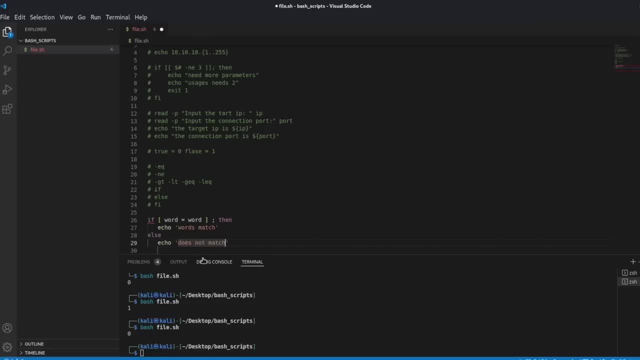 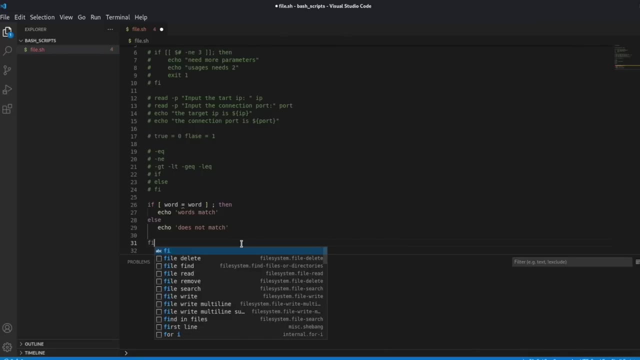 And we'll tell it does not match. just like this: I accidentally clicked the debug, but we're not going to mess with that right now And then we're going to close this off. Now, if we save this, come back to our terminal and we run the file, it tells us the words: 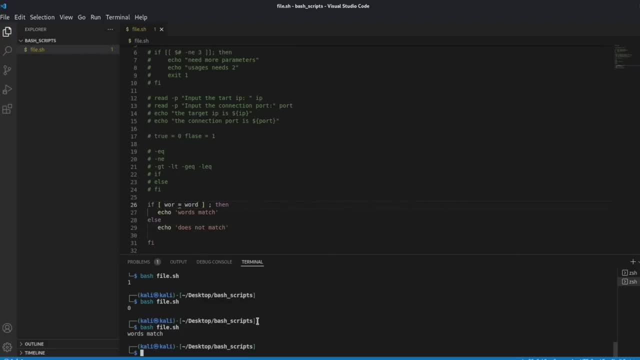 match. If we get rid of our D again and we save and we run this, it says they do not match. So this is how you can use a comparison with an if, Then we can do the same thing here. We're going to go back to our terminal and we're going to say, echo a text and we're going to tell it does not match. 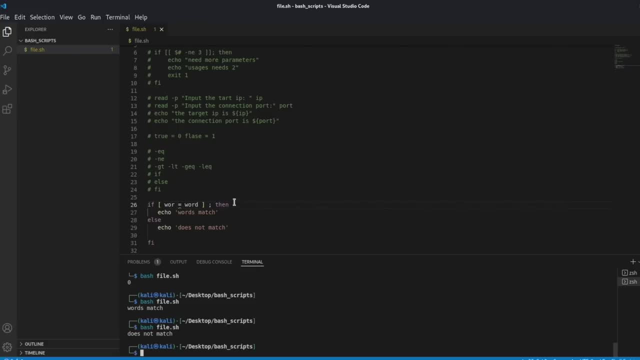 Then else fee statement. So if it is this, then we want it to do a specific function and if not, then we can have it do something else. This is a very basic if statement. So I would challenge you to change this if statement and see if you can do and if the number two is equal to the number two. 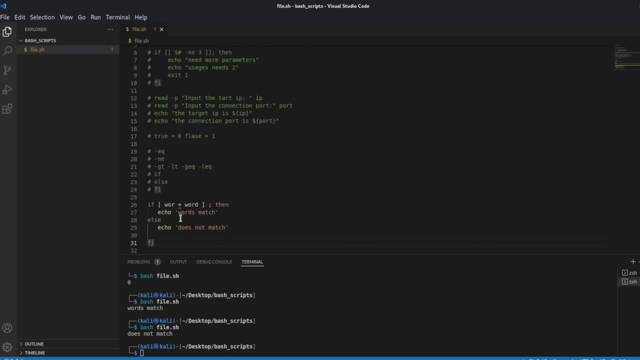 then you want it to echo the numbers match, else they do not match. and then do the same thing with a not equals and just work your way through these and see if you can play around with the if statement and really grasp these concepts and make them your own. 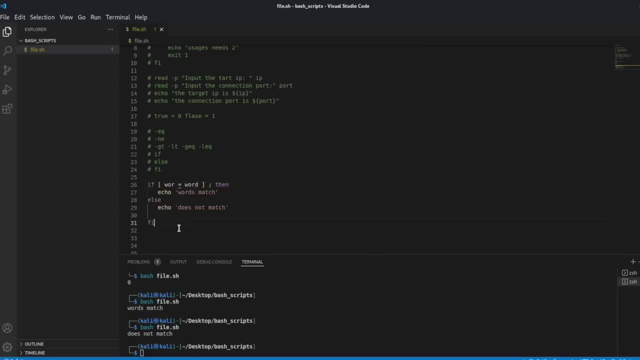 We're going to be moving on to while loops and we're going to cover these really quickly because we won't use these a whole lot. But an example of when a while loop is used is in a buffer overflow. When we want to crash a program, we're going to send it so many bytes until it crashes. 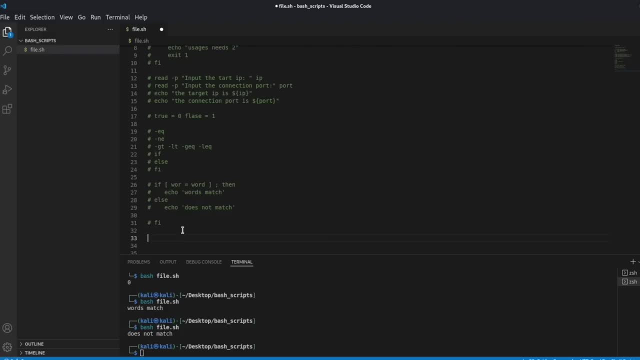 And so the example is: we're just going to say, while this is running, we're going to send bytes to the server until it overflows. So while loops are used, But I use them very infrequently. I don't use them often. I know there are other programmers out there who love while loops and use them all the time. 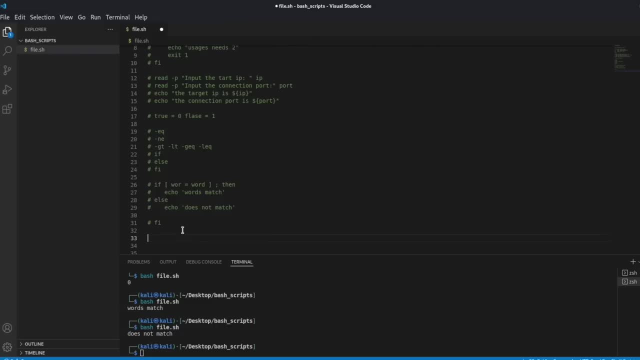 I would much rather use a for loop. So for that purpose, we're going to cover while loops really quickly. So while we're in our file here, we're going to write a while loop and we're going to use a really common while loop that is used pretty much in teaching: while loops. 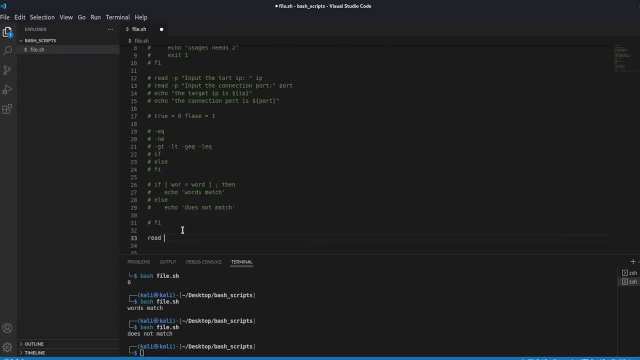 no matter what the programming language is. So if we take an input from the user like this and we say enter a number, and then we do our colon space, and then we're going to assign it a variable of num, just like this, And then we say, while the condition which is going to be the num is, we'll say less than 10, we want to do something. 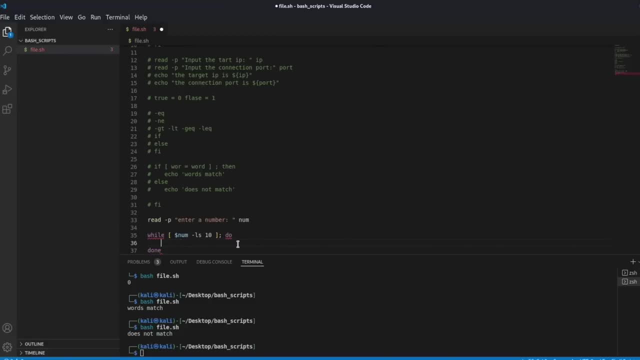 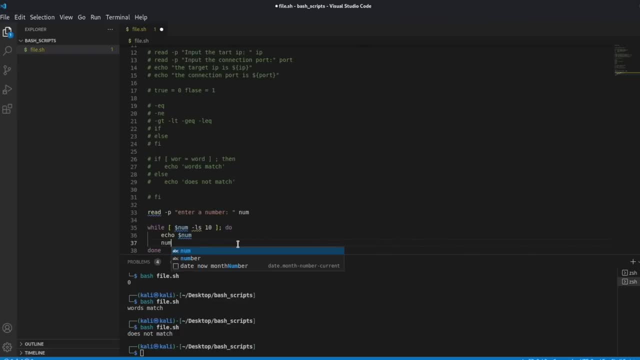 And then down here we need to make sure that our number continues to go up. So we'll say: num equals dollar sign, and down here we will need two sets of parentheses and we will say dollar sign num plus one And the reason we're adding in this plus here. 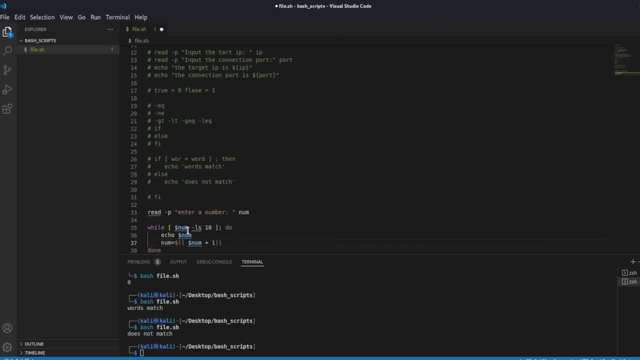 is, each time the while loop runs, we're going to add one to the number, and so the first time the loop runs, let's say we enter the number zero, it will run through the while loop and then, when it hits this line of code, it'll be zero plus one. the second time it runs through this loop of code, it'll. 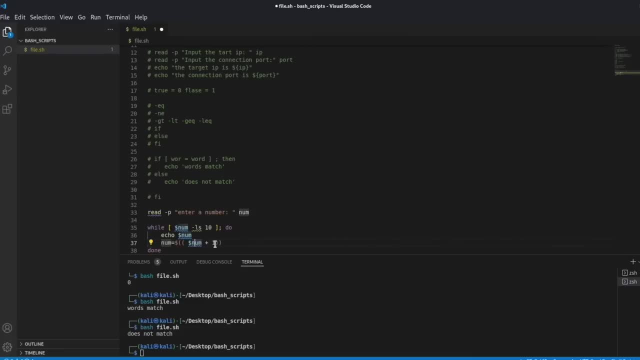 be one plus one, which is two, and then two plus one is three. every time it runs it's changing this variable, so what we are going to do is save this and run it. we'll run it a couple of different times so you can see how this works. so let's say we enter zero as our number- i have an ls here- and 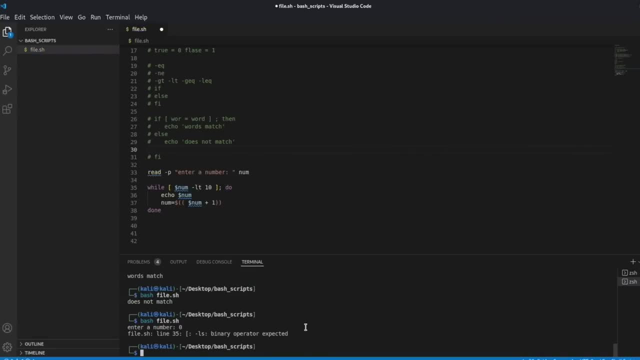 that is not. it is a less than which is an lt. so we'll save this. run it and our number is zero and it shows us it runs one, two, three, four, five, six, all the way down. and remember that it starts here at one, two, three, and here we go, so it runs for us from zero all the way to ten. now, if we run it, 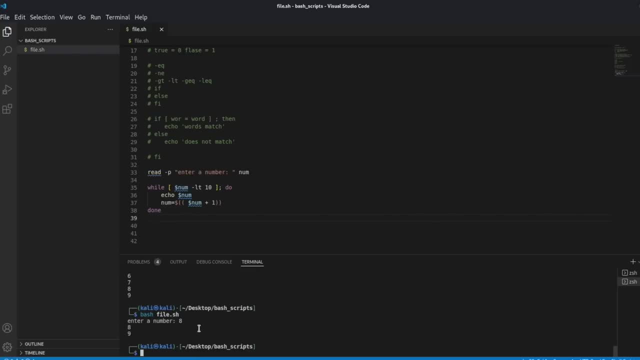 again. and let's say we put in the number eight, it only runs twice, because nine when it hits ten, when the number equals ten, it is no longer less than ten. so now that we see how the while loop runs, we can also do something like this if we enter in a number that is already greater than. 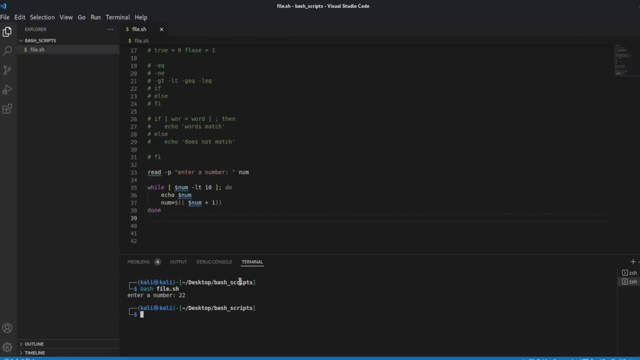 the number ten, it will just exit the code because it is no longer a less than so. this is an example of how a while loop runs over and over and over until the statement up here is no longer true. now i would challenge you to use this with a greater than, and maybe change this to a minus and see if you can. 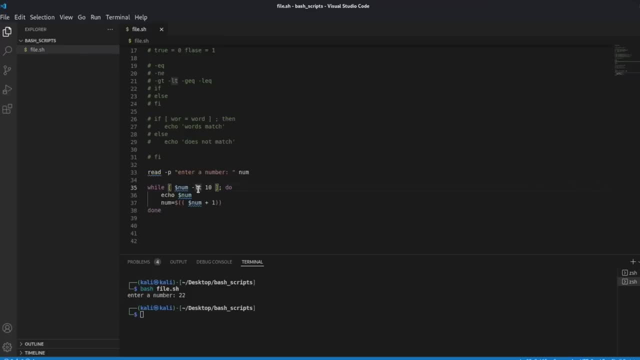 use an input of a number and say that you need this to be as long as the number is greater than ten. you want it to do this, and then you're going to minus one, and so you can kind of play around with the while loop and get an understanding of how this works. so let's go ahead and run this. 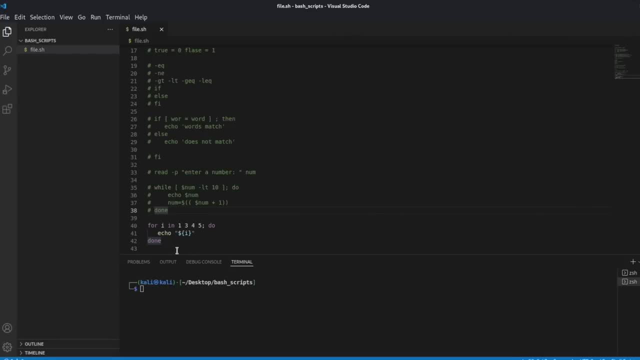 example of how it works. all right, i have typed out a for loop here for us and this is a very basic for loop. so we have this for loop here in four. we have this. four is how we're going to start it- i, which is going to be the variable which iterates through the list that we give it. so we're saying: 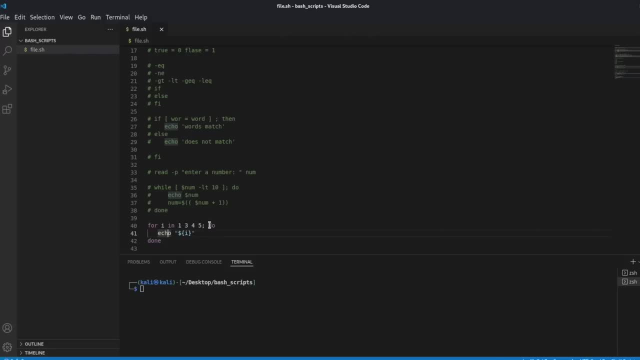 for i in this list of numbers. we want it to do something and we want it to echo out the variable i every time this loop runs. so the first time the loop runs, i will equal one. the second time it runs, we'll put a two in here. the i will equal two. the third time it runs, it's gonna equal three. 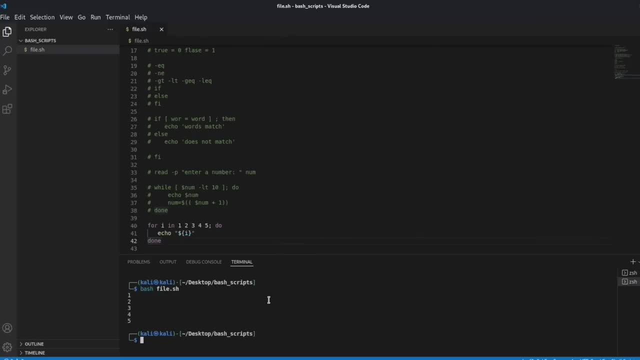 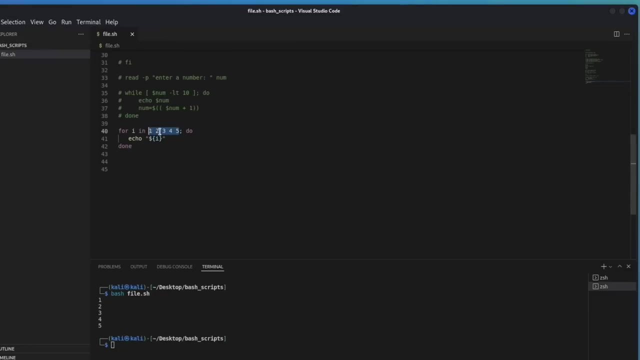 and so on. so if we save this and we run this file, you can see i echoes out one, two, three, four, five and so on. so every time we use something like this, and so this is the for loop, and you can play around with the for loop in a lot of different ways and even use these to loop through lists or 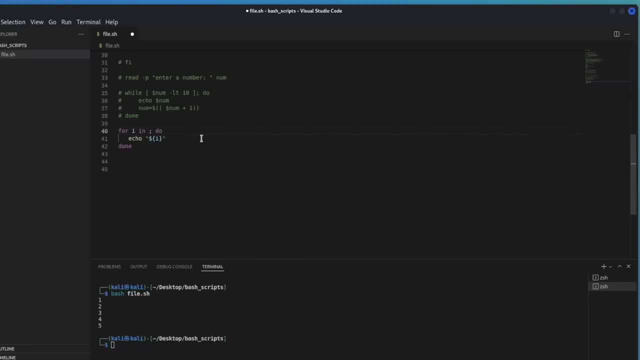 arrays in order to get it to print, and we want to have this jump around, so we're going to type in this. but the point of this course is not for us to learn how to program with for loops, but rather understand them and know how to edit them as we go through our cyber security journey, remembering 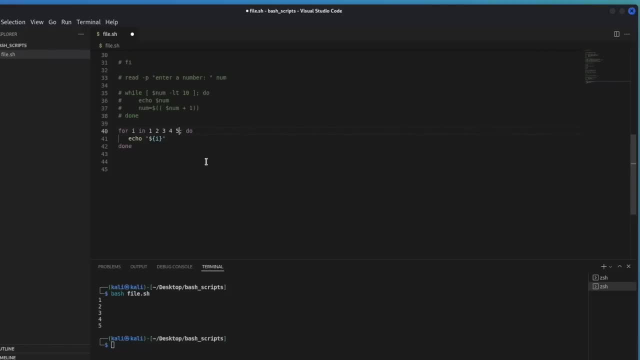 that the point of us being able to understand bash is not to be bash programmers, but in order for us to know how to manipulate bash scripts that are already written, as well as bash exploits. so when you see a for loop like this, you now know how you can edit it and change it and, if you need to, you. 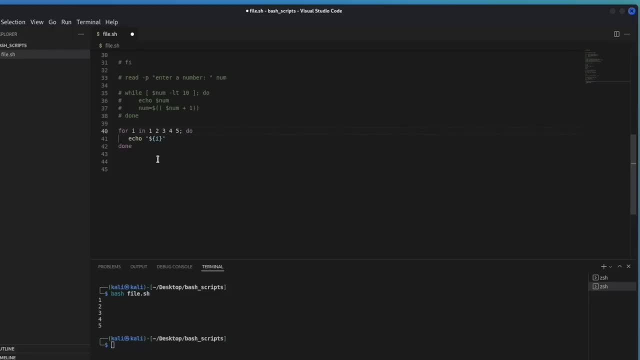 can write simple bash for script for loops and loop through different arrays and lists.